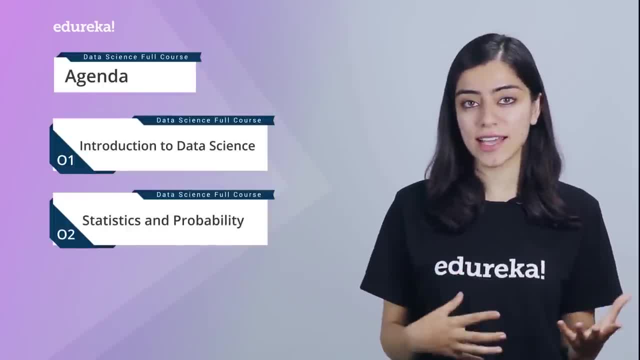 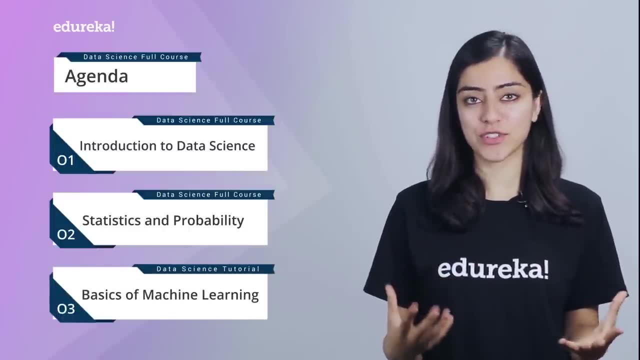 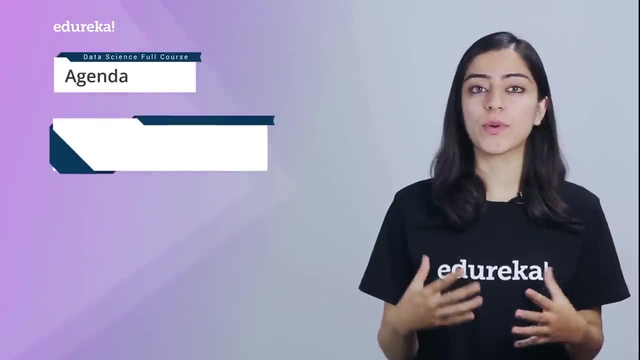 where you'll understand the statistics and the math behind data science and machine learning algorithms. The next module is the basics of machine learning, where we'll understand what exactly machine learning is, the different types of machine learning, the different machine learning algorithms and so on. The next module is the supervised learning algorithms module. 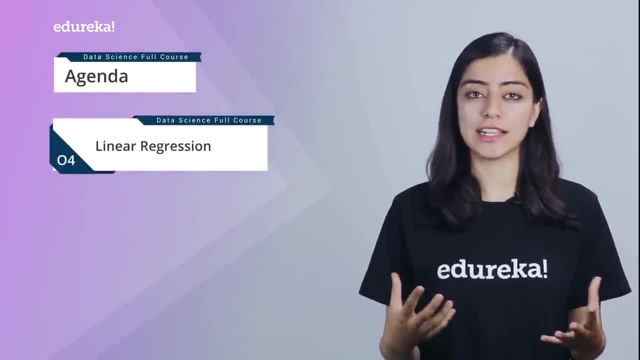 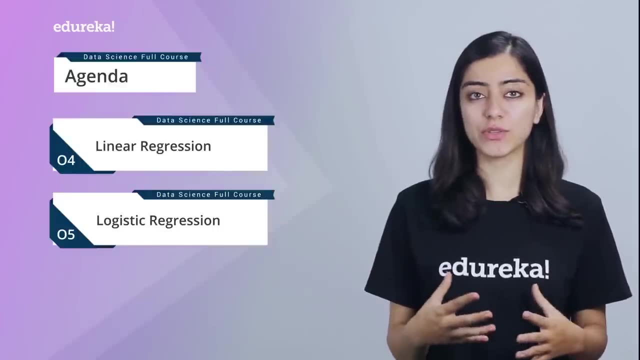 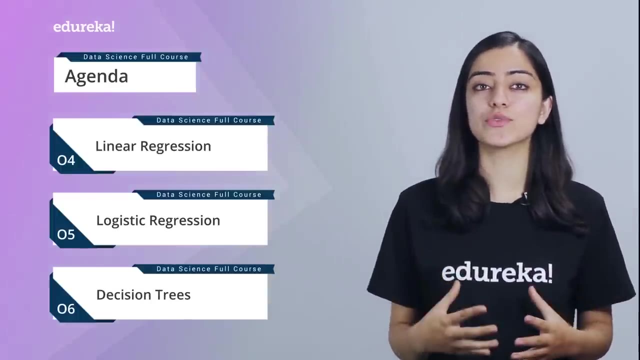 where we'll start by understanding the most basic algorithm, which is linear regression. The next module is the logistic regression module, where we'll see how logistic regression can be used to solve classification problems. After this, we'll discuss about decision trees and we'll see how decision trees can be used to solve complex data-driven problems. The 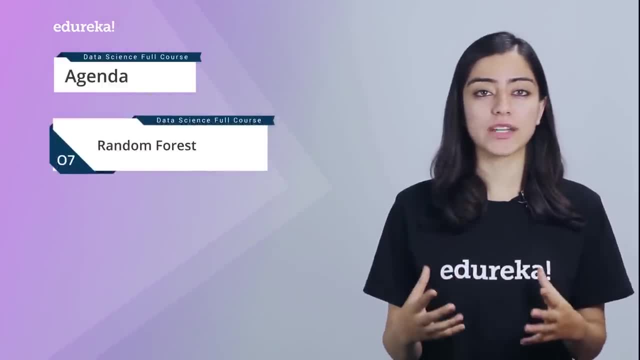 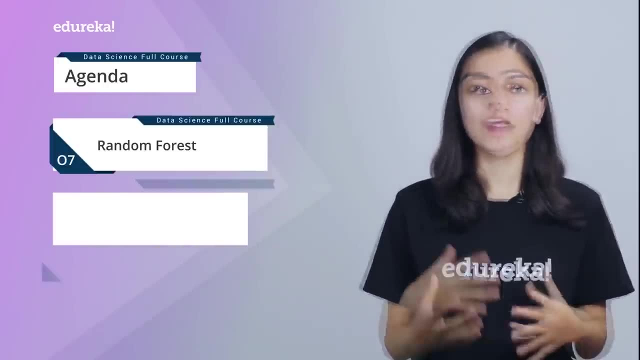 next module is random forest. Here we'll understand how random forest can be used to solve classification problems and regression problems with the help of use case equations and deep learning. The next module is linear regression. In this module we'll start by cases and examples. 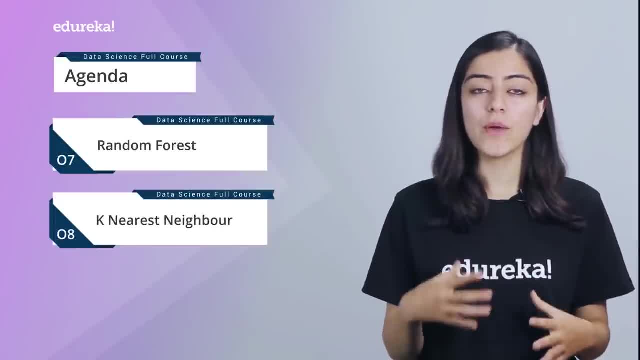 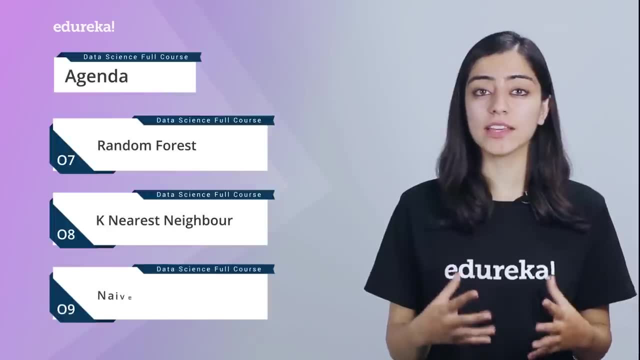 The next module we will be discussing is the k-nearest neighbor module, where we will understand how KNN can be used to solve complex classification problems. Followed by this, we will look at the naive bias module, which is one of the most important algorithms in the Gmail spam detection. 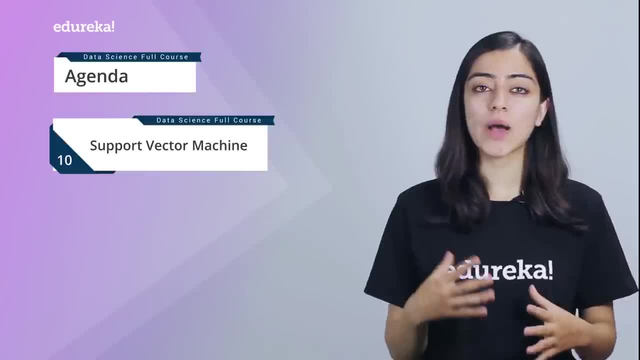 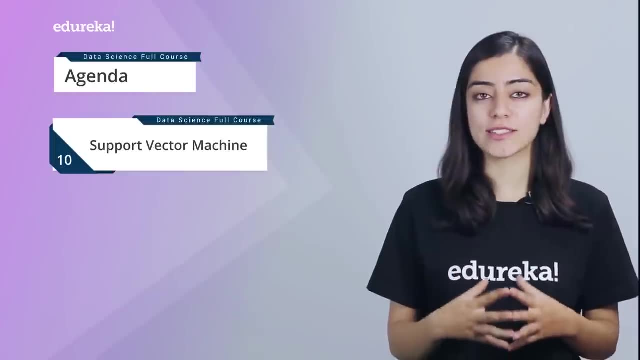 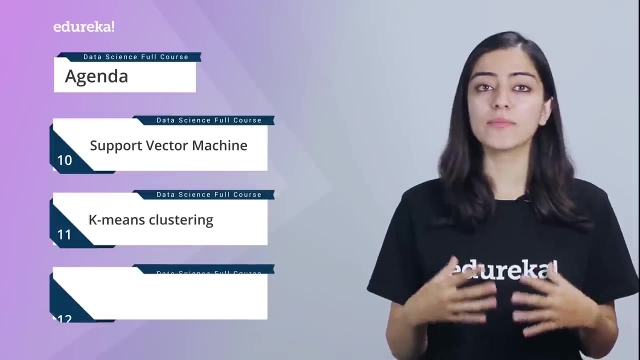 The next algorithm is support vector machines, where we will understand how SVMs can be used to draw a hyperplane between different classes of data. Finally, we will move on to the unsupervised learning module, where we will understand how key means can be used for clustering and how you can perform market basket analysis by 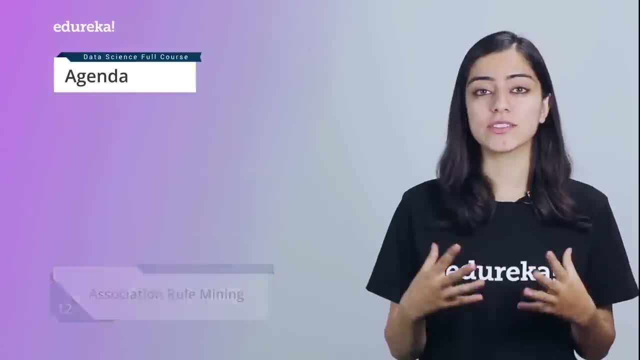 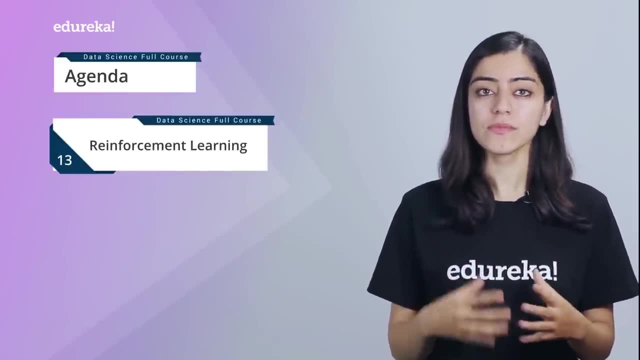 using association rule mining. The next module is reinforcement learning, where we will understand the different concepts of reinforcement learning, along with a couple of demonstrations. Followed by this, we will look at the deep learning module, where we will understand what exactly deep learning is. what are neural networks, the different types of neural networks. 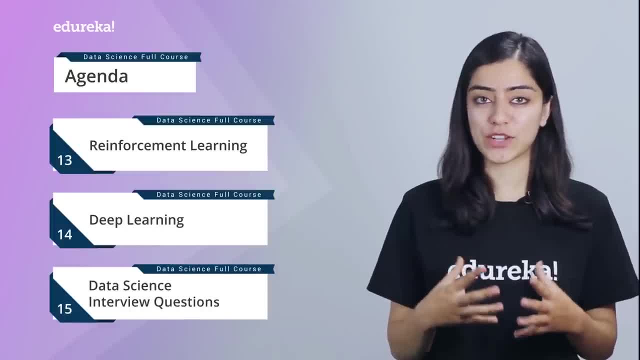 and so on. The last module is the deep learning module, where we will understand the different types of neural networks, and so on. The last module is the data science interview questions module, where we will understand the important concepts of data science, along with a few tips in order to ace the interview. 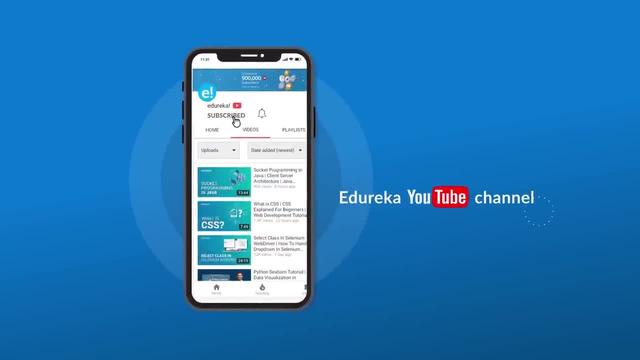 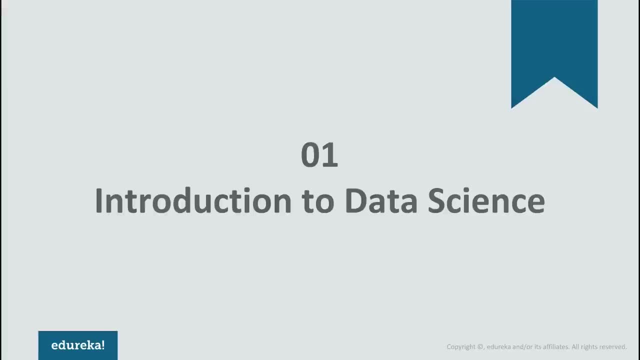 Before we get started, make sure you subscribe to Edureka YouTube channel in order to stay updated about the most trending technologies. Data science is one of the most in demand technologies right now. This is probably because we are generating data at an unstoppable pace and, obviously, 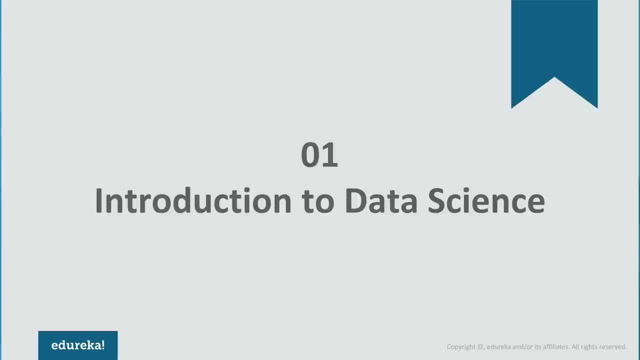 this is a very complex process and makes sense out of this much data. This is exactly where data science comes in. In today's session, we will be talking about data science in depth, So let's move ahead and take a look at today's agenda. 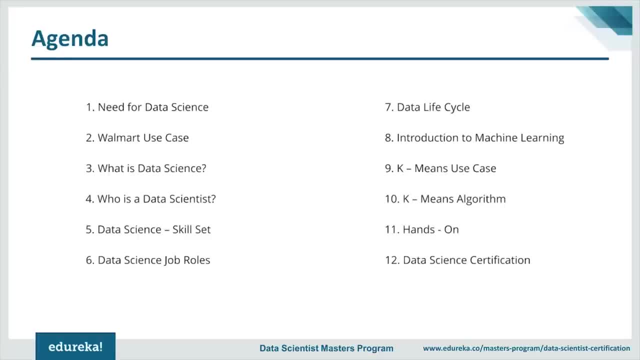 We are going to begin with discussing the various sources of data and how the evolution of technology and introduction of IoT and social media have led to the need of data science. Next, we will discuss how Walmart is using insightful patterns from their database to increase the potential of their business. 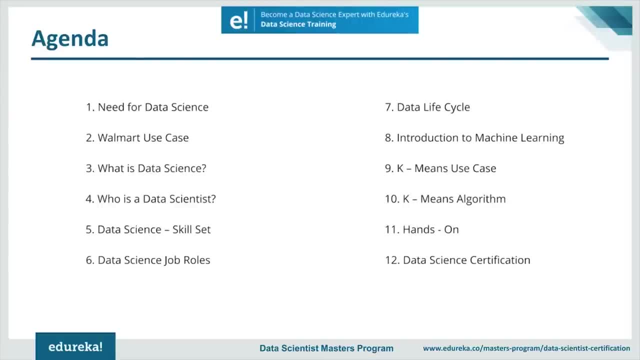 After that, we will see what exactly data science is. Then we will move on and discuss who a data scientist is, where we will also discuss the various skill sets needed to become a data scientist. Next, we will move on to see the various data science job roles, such as data analyst, data. 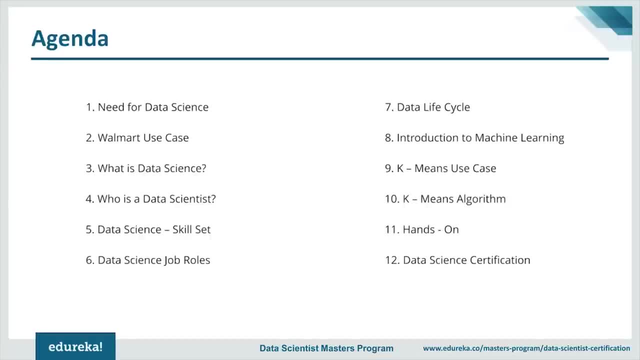 architect, data engineer and so on. After this, we will cover the data life cycle, where we will discuss how data is extracted, processed and finally used as a solution. Once we are done with that, we will cover the basics of machine learning, where we will see. 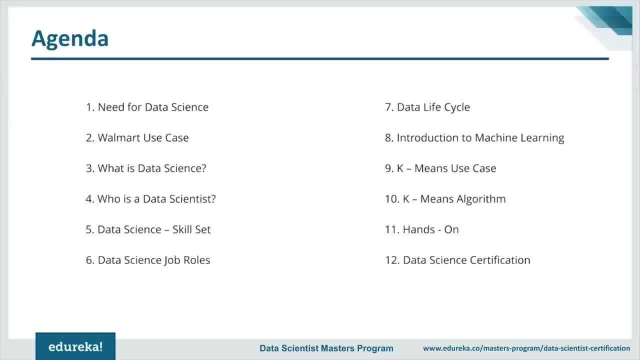 what exactly machine learning is and the different types of machine learning. Next, we will move on to the k-means algorithm and we will discuss a use case of the k-means clustering, After which we will discuss the various steps involved in the k-means algorithm. 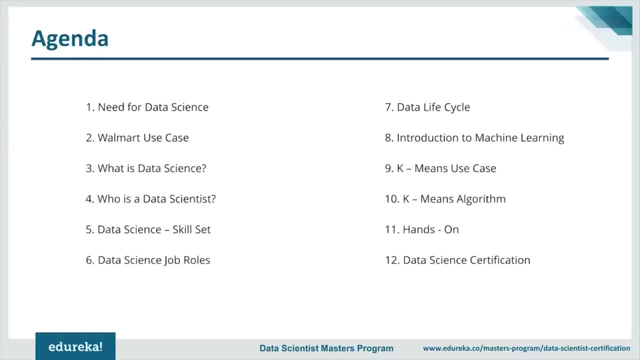 And then we will finally move on to the hands on part, where we will use the k-means algorithm to cluster movies based on their popularity on social media platforms like Facebook. At the end of today's session, we will also discuss about what a data science certification. 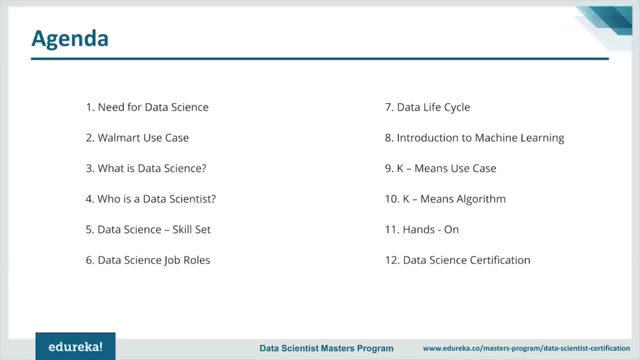 is and why you should take it up. So, guys, there is a lot to cover in today's session. let's jump into the first topic. So, guys, there is a lot to cover in today's session. let's jump into the first topic. 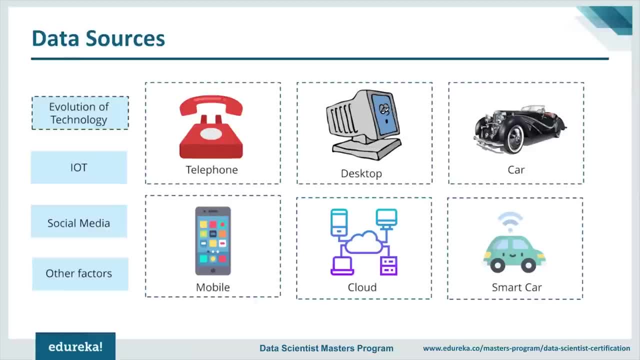 Do you guys remember the times when we had telephones and we had to go to PCO booths in order to make a phone call? Now, those times were very simple because we didn't generate a lot of data, We didn't even store the contacts in our phones or our telephones. 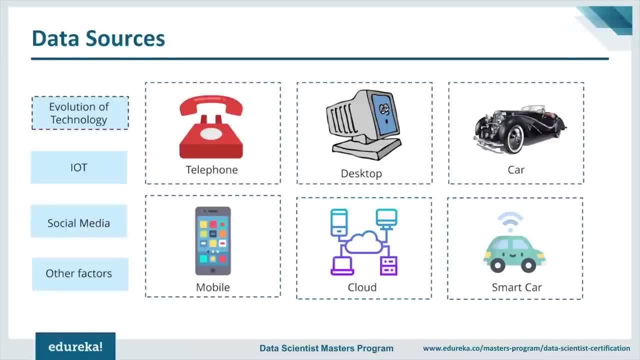 We used to memorize phone numbers back then or we used to have a diary of all our contacts, But these days we have smartphones which store a lot of data. So there is everything about us in our mobile phones. We have images, we have contacts, we have various apps, we have games- everything is. 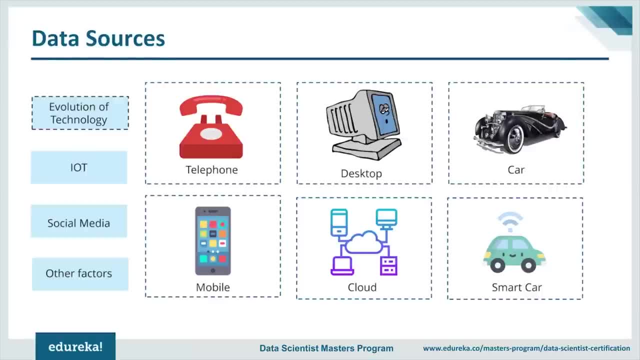 stored in our mobile phones these days, Similarly the PCs that we use. in the earlier times it used to process very little data. There was not a lot of data processing needed because technology wasn't evolved that much. So, if you guys remember, we used floppy disks back then and floppy disks was used to store. 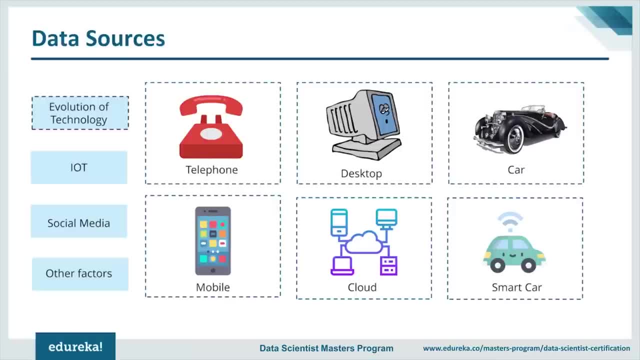 small amounts of data, But later on, hard disks were created and those used to store GBs of data. But now, if you look around, there's data everywhere around us. We have data stored in the cloud. we have data in each and every appliance at our houses. 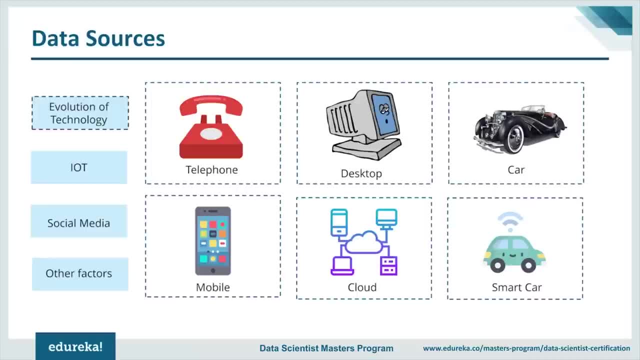 Similarly, We have smart cars. these days, they're connected to the internet, they're connected to our mobile phones, and this also generates a lot of data. What we don't realize is that evolution of technology has generated a lot of data. Alright now. initially, there was very little data, and most of it was even structured. 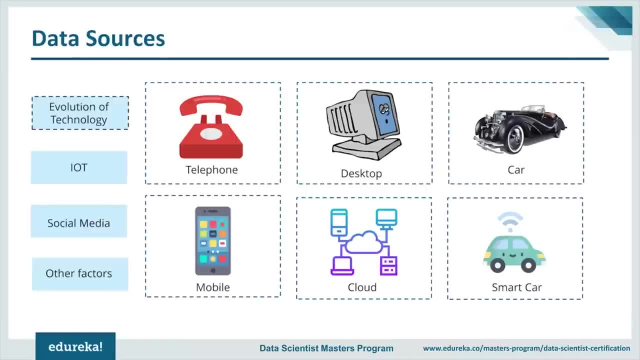 Only a small part of the data was unstructured or semi-structured and in those days you could use simple BI tools in order to process all of this data and make sense out of it. But now we have way too much data and in order to process this much data, we need more complex. 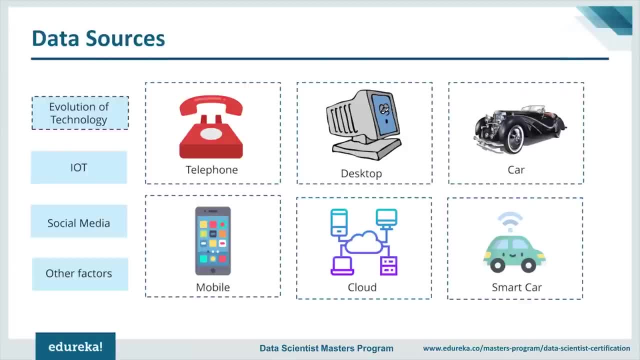 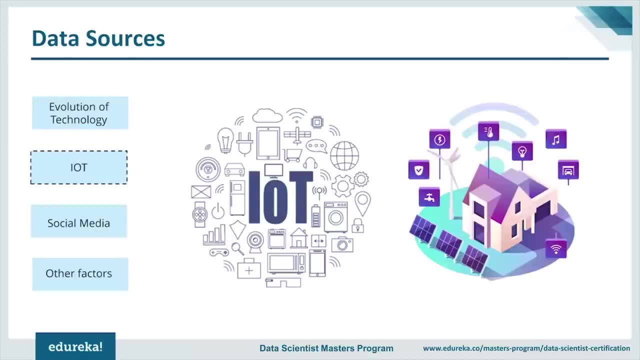 algorithms. We need a better process. Alright, and this is where data science comes in. Now, guys, I'm not going to get into the depth of data science yet. I'm sure all of you have heard of IOT or Internet of Things. 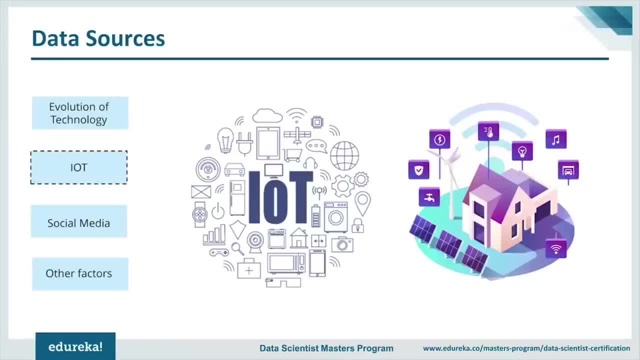 Now, did you guys know that we produce 2.5 quintillion bytes of data each day, and this is only accelerating with the growth of IOT? Now, IOT, or Internet of Things, is just a fancy term that we use for network of tools or devices. 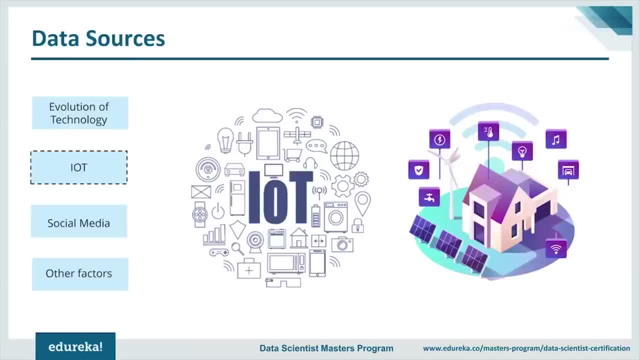 that communicate and transfer data through the internet. So various devices are connected to each other through the internet And they communicate with each other. right Now, the communication happens by exchange of data or by generation of data. Now these devices include the vehicles we drive. 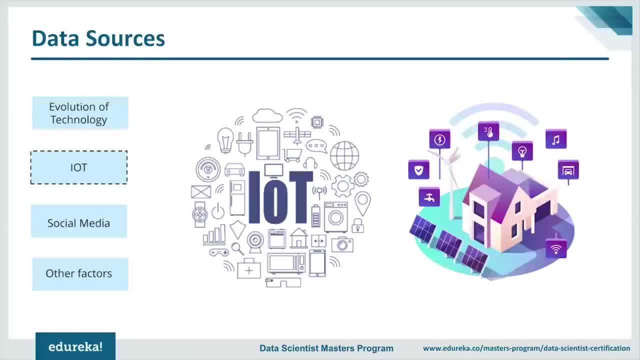 They include our TVs, our coffee machines, refrigerators, washing machines and almost everything else that we use in a daily basis. Now these interconnected devices produce an unimaginable amount of data, Guys. IOT data is measured in zettabytes, and one zettabyte is equal to trillion gigabytes. 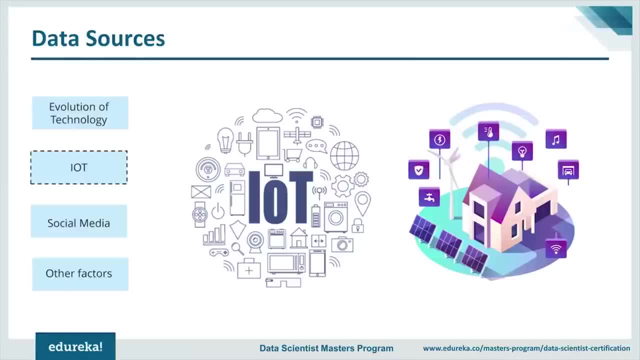 So So, according to a recent survey by Cisco, it's estimated that by the end of 2019, which is almost here- the IOT will generate more than 500 zettabytes of data per year, And this number will only increase through time. 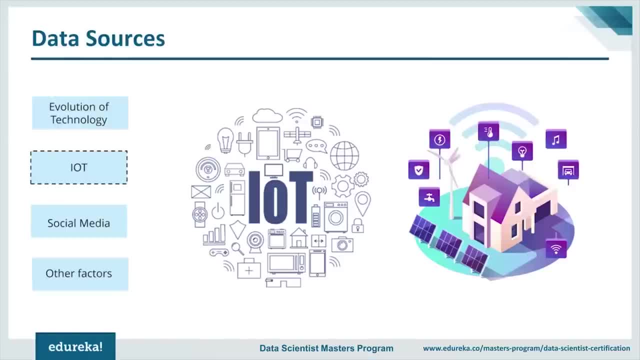 It's hard to imagine data in that much volume. Imagine processing, analyzing and managing this much of data. It's only going to cause us a migraine. So, guys, having to deal with this much data is not something that traditional BI tools can do. 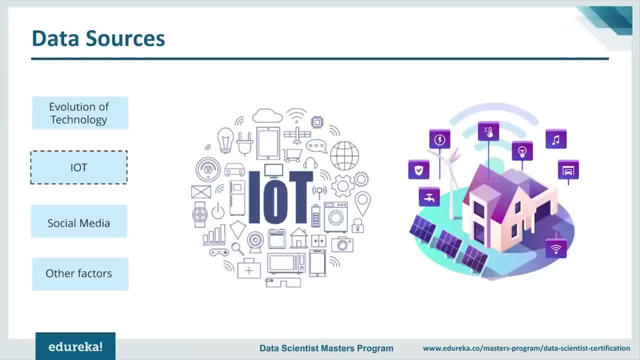 Okay, It's not something that traditional data processing methods. That's exactly why we need data science. It's our only hope right now. Now, let's not get into the details yet. Moving on, Let's see how social media is adding on to the generation of data. 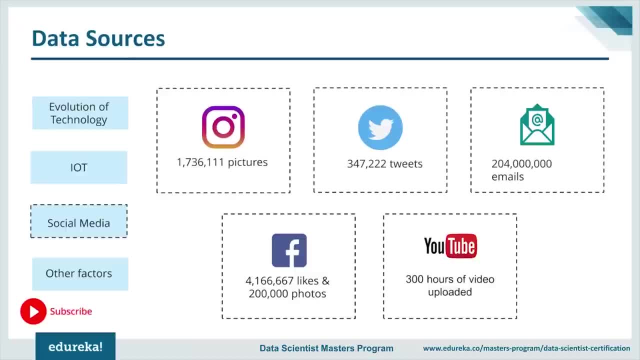 Now, the fact that we are all in love with social media. it's actually generating a lot of data for us. Okay, It's certainly one of the fuels for data creation. Now, all these numbers that you see on the screen are generated every minute of the day. 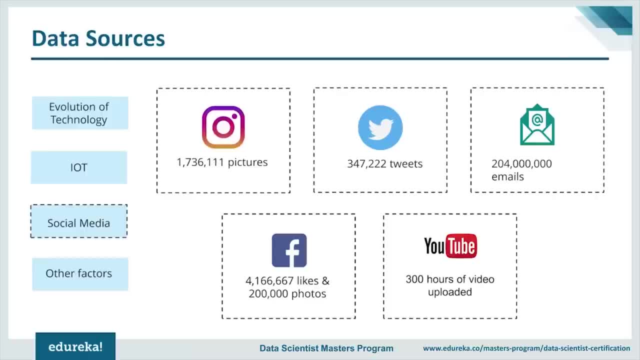 Okay, And this number is just going to increase. So for Instagram, it says that Approximately 1.7 million pictures are uploaded in a minute, And similarly on Twitter, approximately 348,000 tweets are published every minute of the day. 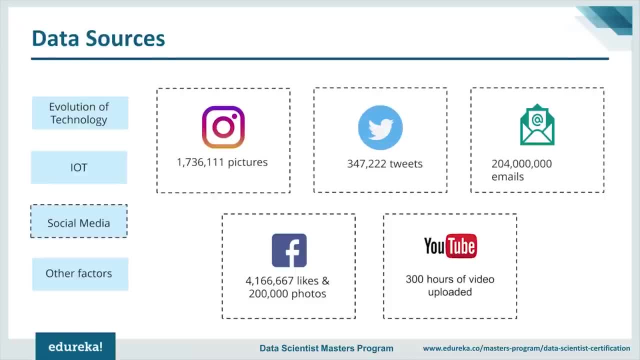 So, guys, imagine in one hour how much that would be, And then imagine in 24 hours. So, guys, this is the amount of data that is generated through social media. It's unimaginable Imagine processing this much data, analyzing it and then trying to figure out, you know. 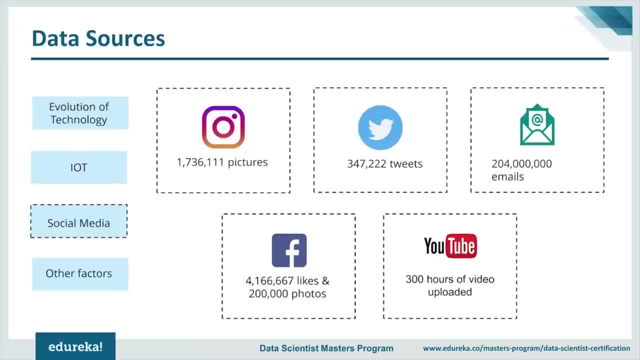 the important insights from this much data. analyzing this much data is going to cause a lot of problems. It's going to be very hard with traditional tools or traditional methods. That's why data science was introduced. Data science is a simple process that will just extract the useful information from data. 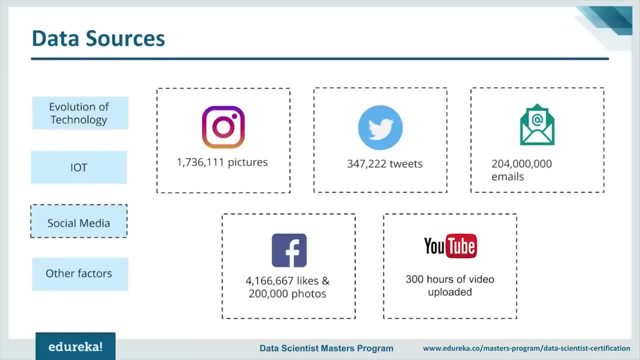 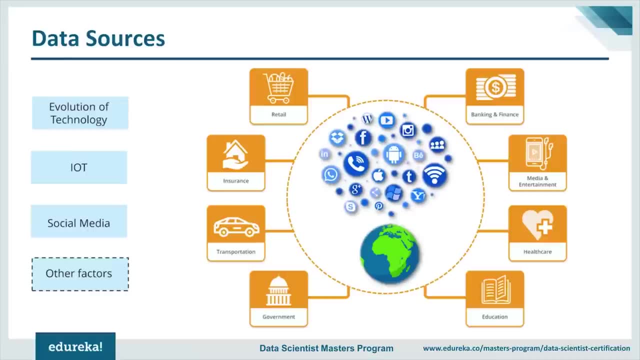 All right, It's just going to process and analyze the entire data, and then it's just going to extract what is needed. Now, guys, apart from social media and IOT, there are other factors as well, which contribute to data generation. 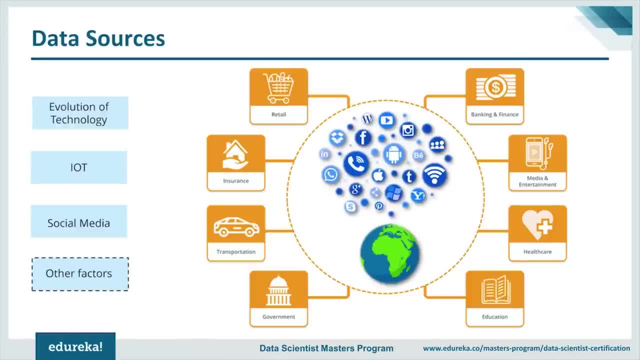 These days, all our transactions are done online, right? We pay bills online, We shop online, We even buy homes online. these days, You can even sell your pets on OLX these days. Not only that, when we stream music and we watch videos on YouTube, all of this is generating. 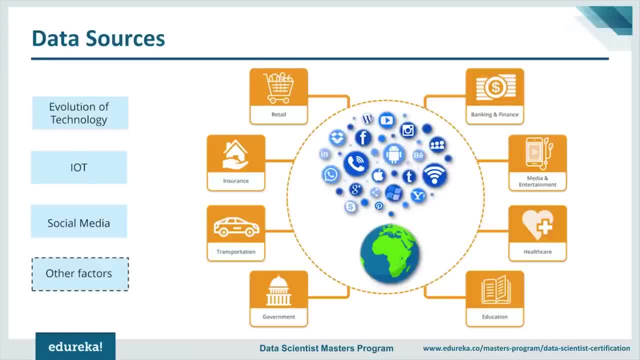 a lot of data. Not to forget, we've also brought healthcare into the internet world. Now there are various watches like BitFit, which basically tracks our heart rate, and it generates data about our health conditions. Education is also an online thing right now. 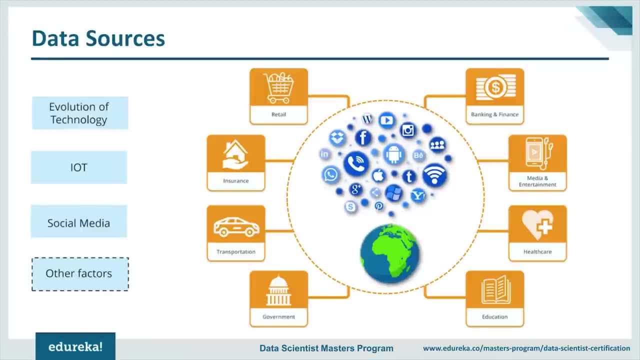 That's exactly what you are doing right now. So with the emergence of the internet, we now perform all our transactions online. We have a lot of data. We can use it to manage all our activities online. Obviously, this is helping us, but we are unaware of how much data we are generating. 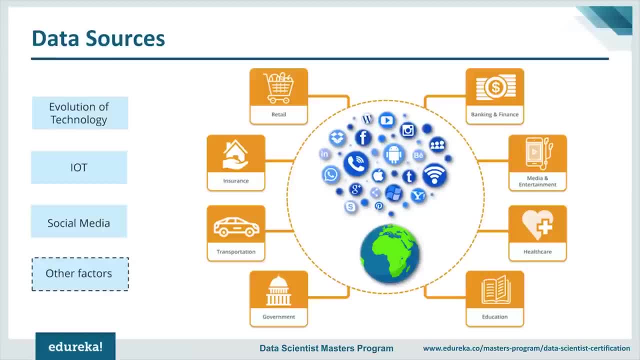 What can be done with all of this data, and what if we could use the data that we generated to our benefit? Well, that's exactly what data science does. Data science is all about extracting the useful insights from data and using it to grow your 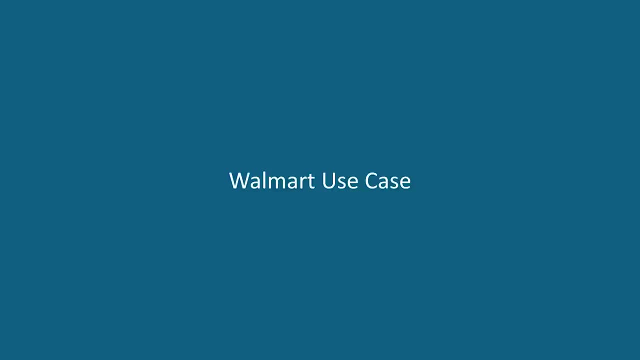 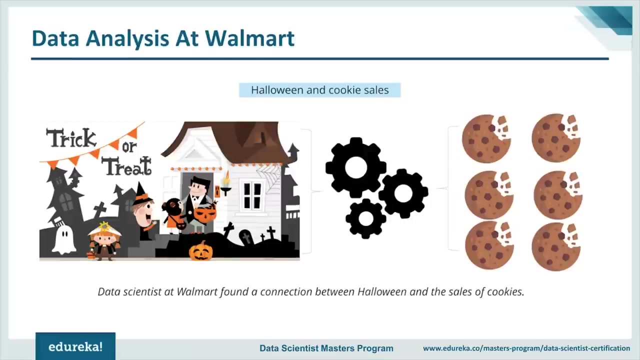 business. Now, before we get into the details of data science, let's see how Walmart uses data science to grow their business. So, guys, Walmart is a big device. It's a huge company, the world's biggest retailer, with over 20,000 stores in just 28 countries. okay, 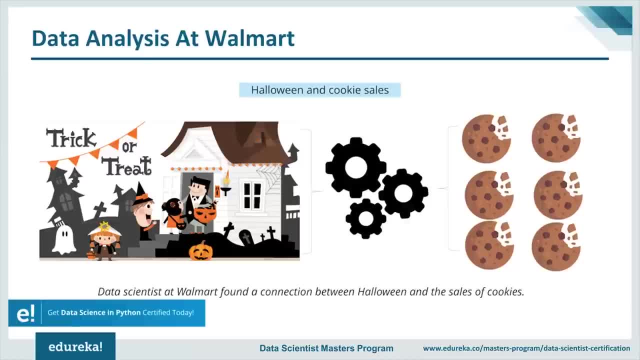 now. it's currently building the world's biggest private cloud, which will be able to process 2.5 petabytes of data every hour. now the reason behind Walmart success is how they use a customer data to get useful insights about customers shopping patterns. now the data analyst and the data scientist at Walmart. they 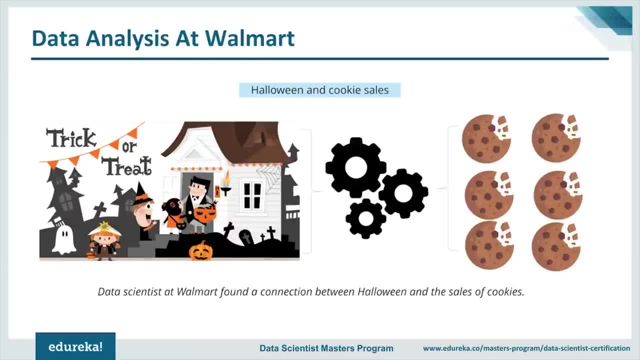 know every detail about their customers. they know that if a customer buys pop tarts, they might also buy cookies. how do they know all of this like? how do they generate information like this? now, they use the data that they get from their customers and they analyze it to see what a particular customer is looking. 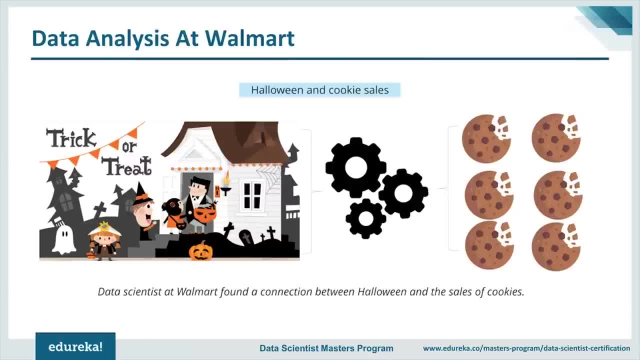 for now, let's look at a few cases where Walmart actually analyzed the data and they figured out the customer needs. so let's consider the Halloween and the cookie sales example now, during Halloween, sales analyst at Walmart took a look at the data, okay, and he found out that a specific cookie was 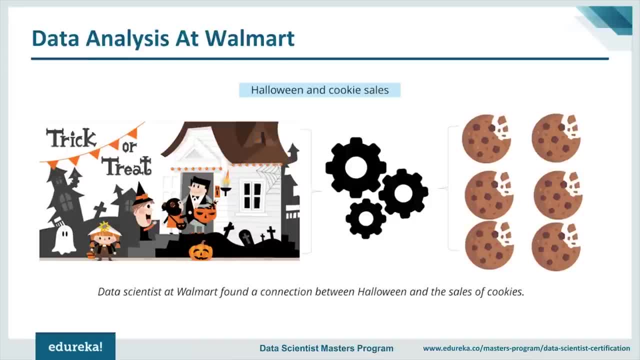 popular across all Walmart stores, so every Walmart store was selling these cookies very well, but he found out that there were two stores which were not selling them at all. okay, so the situation was immediately investigated and it was found that there was a simple stocking oversight. okay, because of which 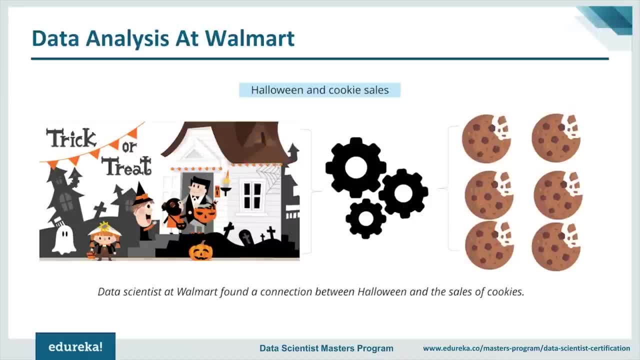 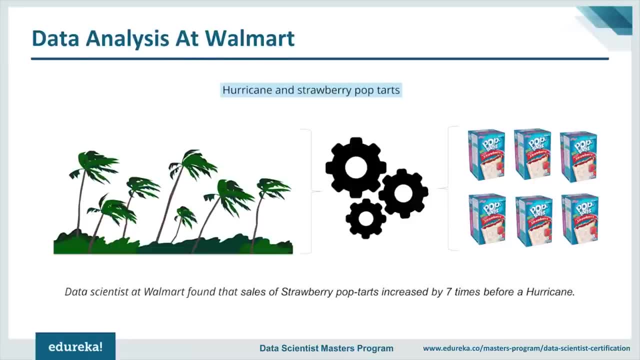 the cookies were not put on the shelves for sale. so, because this issue was immediately identified, they prevented any further loss of sales. now, another such example is that, through association rule mining, Walmart found out that strawberry pop-tart sales increased by seven times before a hurricane. so a data analyst at Walmart identified the association between. 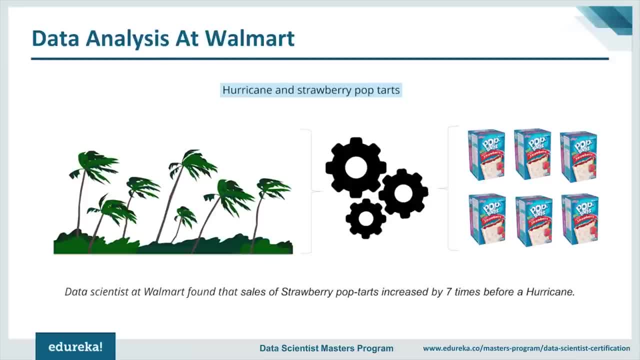 hurricane and strawberry pop-tarts through data mining. now, guys don't ask me the relationship between pop-tarts and hurricane, but for some reason, whenever there was a hurricane approaching, people really wanted to eat strawberry pop-tart. so what Walmart did was they placed all the strawberry pop. 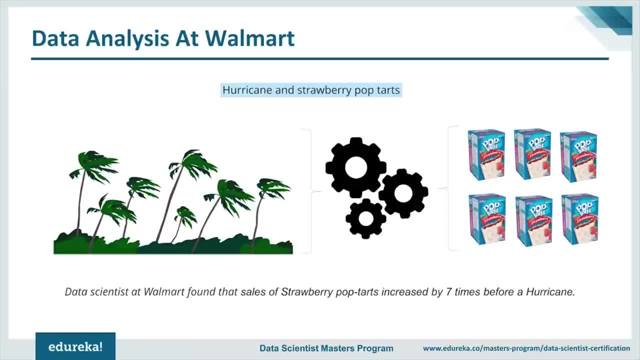 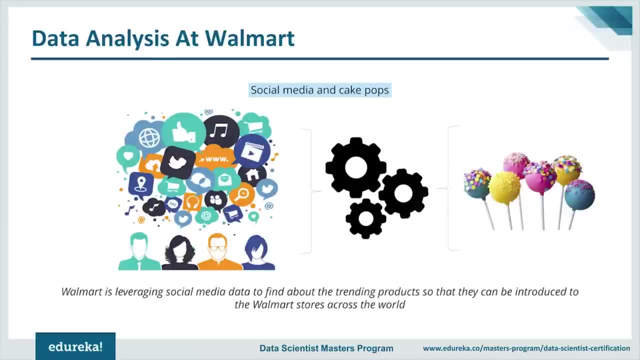 tarts as a check out before a hurricane muddakur. so this way, they increased sales of their pop-tarts. now, guys, this is an actual thing, I'm not making it up, you can look it up on the internet. not only that, Walmart is analyzing the data generated by social 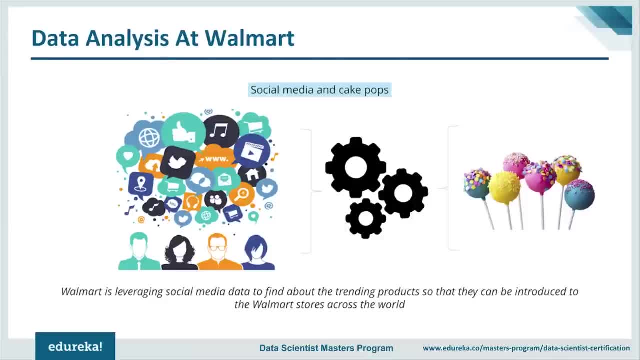 media to find out all the trending product. so through social media, you can find out the likes and dislikes of a person, right? so what Walmart did is- they're quite smart- they use the data generated by social media to find out what products are trending or what products are liked by customers. okay, so 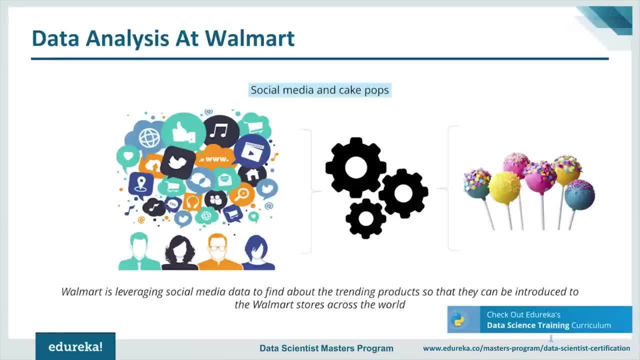 An example of this is Walmart analyzed social media data to find out that Facebook users were crazy about cakepops. Okay, so Walmart immediately took a decision and they introduced cakepops into the Walmart stores. So, guys, the only reason Walmart is so successful is because the huge 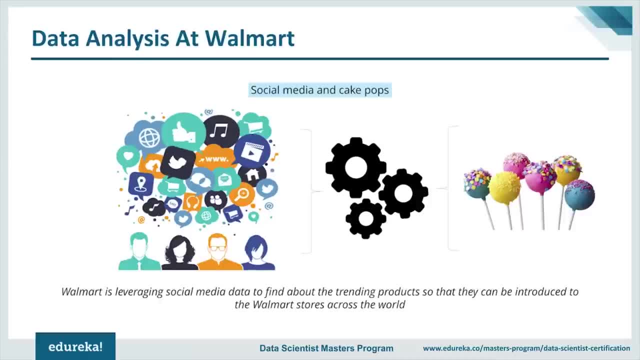 amount of data that they get. they don't see it as a burden. Instead, they process this data, analyze it and then they try to draw useful insights from it. Okay, so they invest a lot of money, a lot of effort and a lot of time in data analysis. Okay, they spend a lot of time. 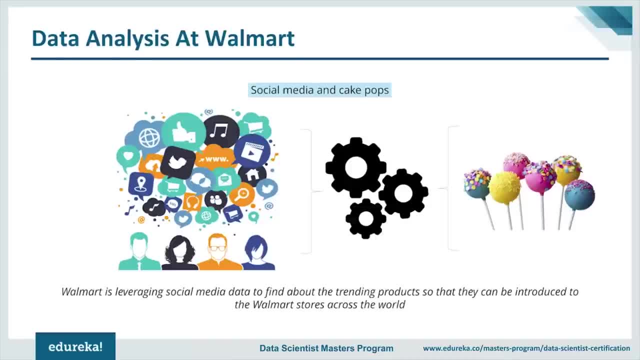 analyzing data in order to find any hidden patterns. So as soon as they find out hidden pattern or association between any two products, they start giving out offers or they start giving discounts or something along that line. So basically, Walmart uses data in a very effective. 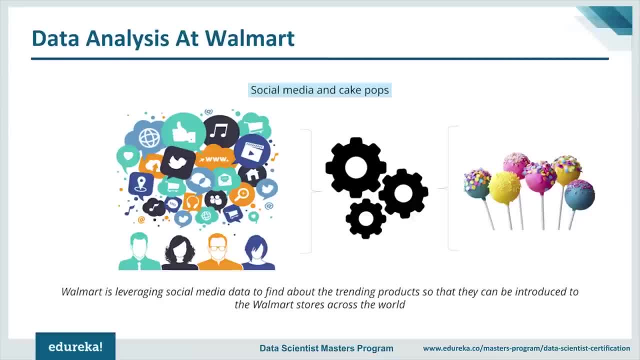 manner. They analyze it very well, they process the data very well and they find out the useful insights that they need in order to get more customers or in order to improve their business. So, guys, this was all about how Walmart uses data science. Now let's move ahead and look at 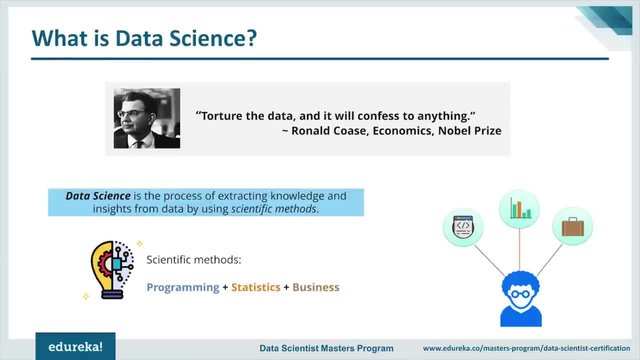 what is data science? Now, guys, data science is all about uncovering findings from data. It's all about surfacing the hidden insights that can help companies to make smart business decisions. So all these hidden insights, or these hidden patterns, can be used to make better decisions in a business. 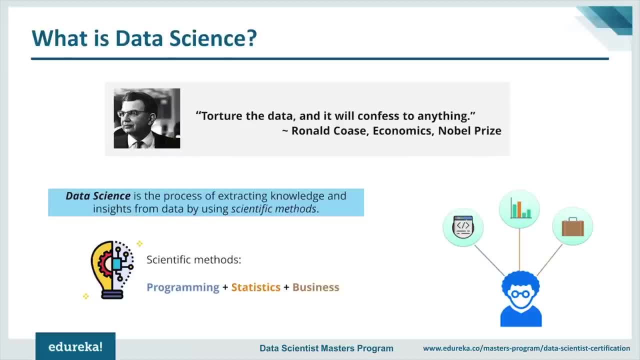 Now, an example of this is also Netflix. So Netflix basically analyzes the movie viewing patterns of users to understand what drives user interest and to see what users want to watch, And then, once they find out, they give people what they want. So, guys, actually data has a lot of power. You. 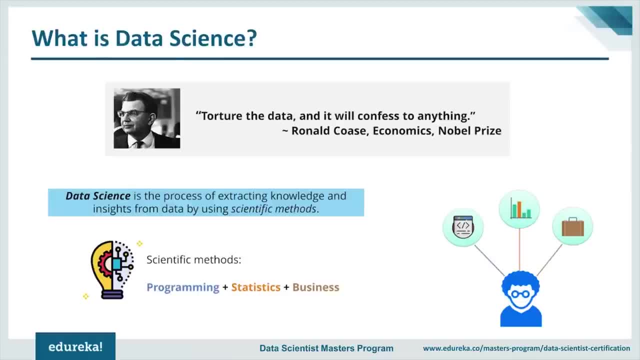 should just know how to process this data and how to extract the useful information from data. Okay, that's what data science is all about. So, guys, a big question over here is: how do data scientists get useful insights from data? So it all starts with data exploration. Whenever a data 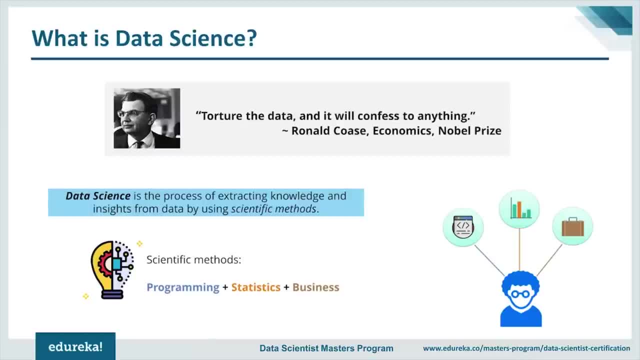 scientist comes across any challenging question or any sort of challenging situation, they become detectives. So they investigate leads and they try to understand the different patterns or the different characteristics of the data. Okay, they try to get all the information that they can from the data. 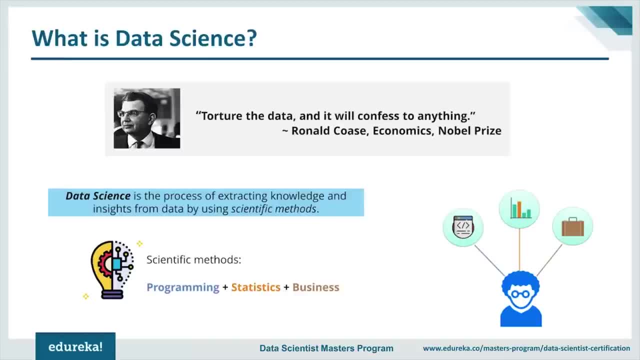 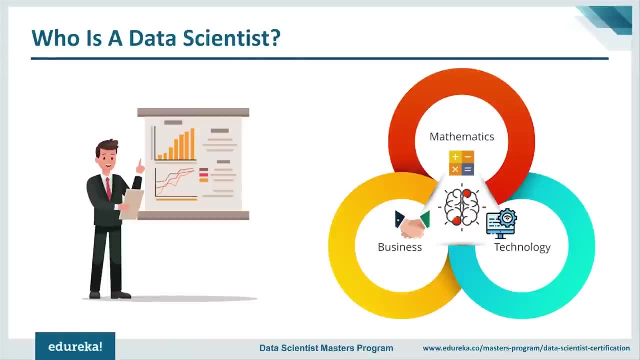 And then they use it for the betterment of the organization or the business. Now let's look at who is a data scientist. So, guys, a data scientist has to be able to view data through a contratrative lens. So, guys, knowing math is. 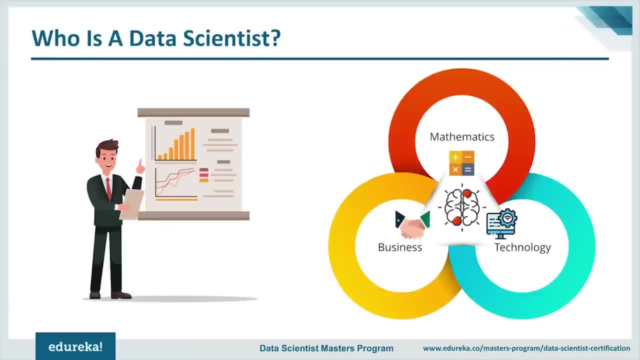 one of the very important skills of a data scientist. Okay, so mathematics is important because, in order to find a solution, you're going to build a lot of predictive models, And these predictive models are going to be based on hard math, So you have to be able to understand. 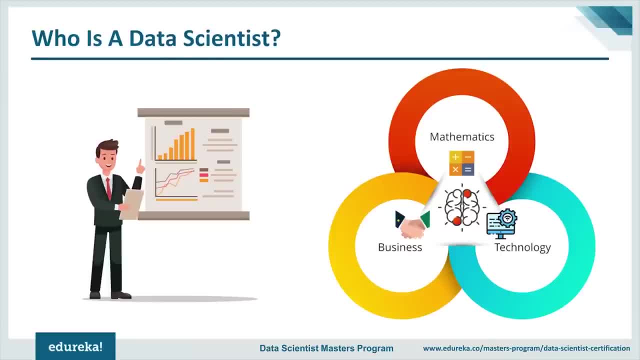 all the underlying mechanics of these models, Most of the predictive models, most of the algorithms require mathematics. Now there's a major misconception that data science is all about statistics. Now, I'm not saying that statistics isn't important, It is very important. 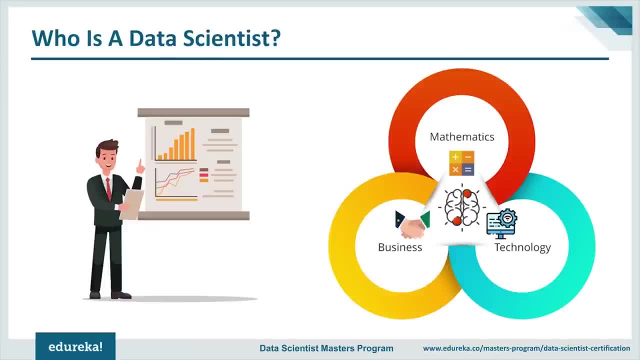 but it's not the only type of math that is utilized in data science. There are actually many machine learning algorithms which are based on linear algebra. So, guys, overall you need to have a good understanding of math And, apart from that, data scientists utilize technology. 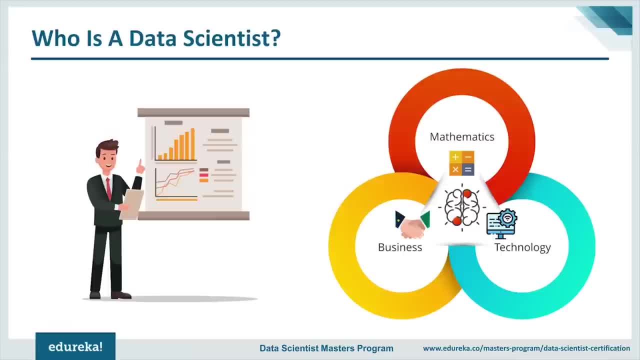 So data scientists have to be really good with technology. Okay, so their main work is: they utilize all the technology so that they can analyze these enormous data sets and work with complex algorithms. So all of this requires tools which are much more sophisticated than Excel. 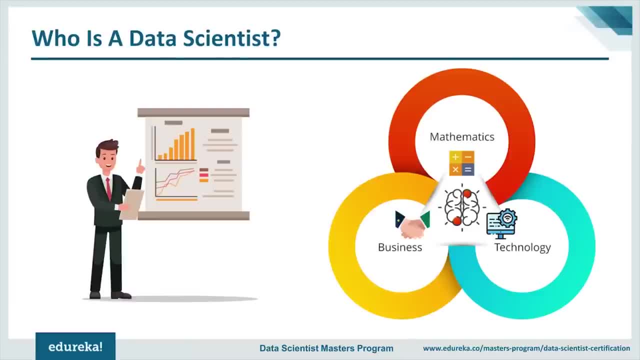 So, guys, data scientists need to be very efficient with coding languages, And few of the core languages associated with data science include SQL, Python, R and SAS. It is also important for a data scientist to be a tactical business consultant. So, guys, business problems can be only solved. 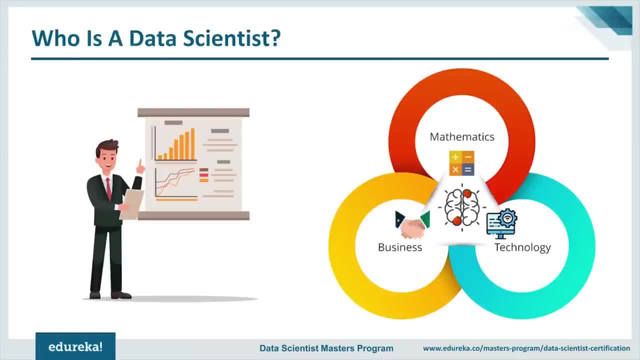 by data scientists. Since data scientists work so closely with data, they know everything about the business. If you have a business and you give the entire data set of your business to a data scientist, he'll know each and every aspect of your business. 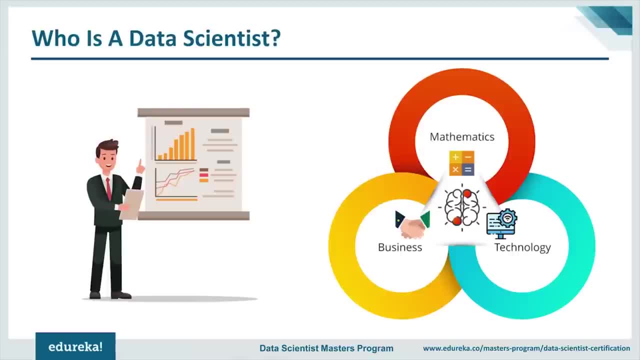 Okay, that's how data scientists work. They get the entire data set, they study the data set, they analyze it and then they see where things are going wrong or what needs to be done more or what needs to be excluded. So, guys, having this business acumen, 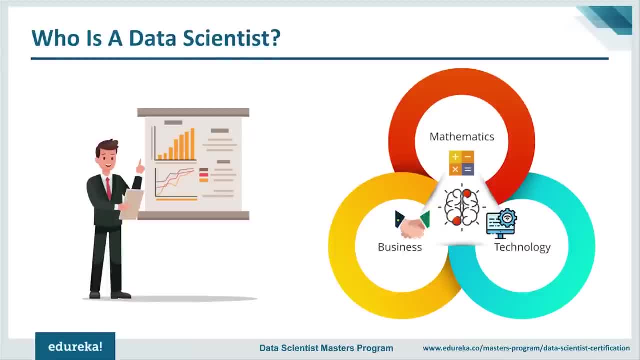 is just as important as having skills in algorithms or being good with math and technology. So, guys, business is also as important as these other fields. Now you know who a data scientist is. let's look at the skill sets that a data scientist needs. 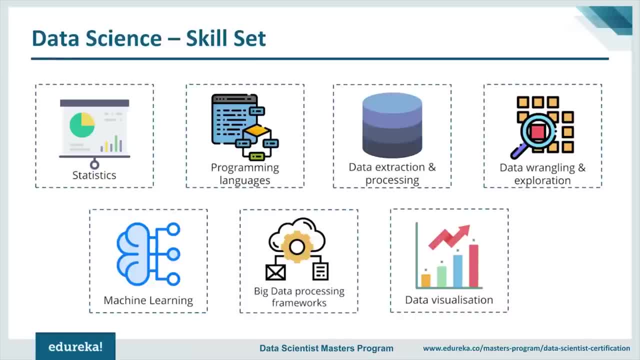 Okay, it always starts with statistics. Statistics will give you the numbers from the data, So a good understanding of statistics is very important. for becoming a data scientist, You have to be familiar with statistical tests, distributions, maximum likelihood, estimators and all of that. 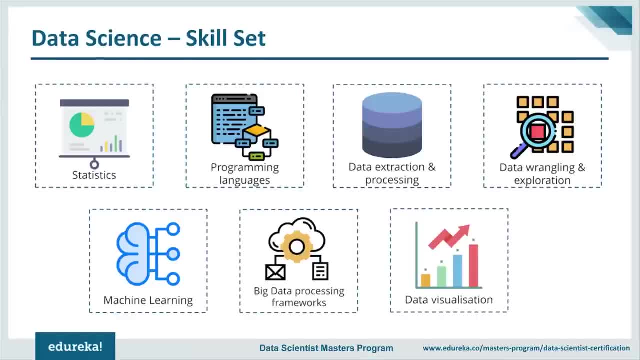 Apart from that, you should also have a good understanding of probability theory and descriptive statistics. These steps will help you make better business decisions. So, no matter what type of company or role you're interviewing for, you're going to be expected to know how to use the tools of the trade. 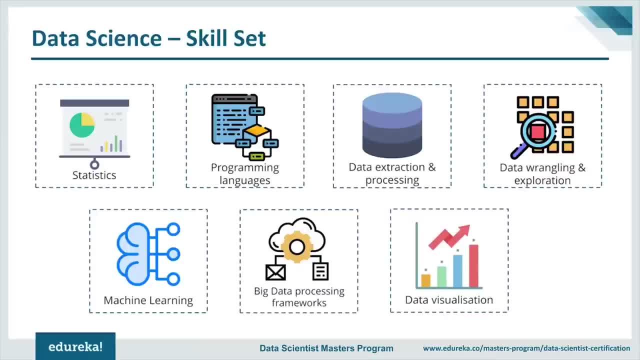 Okay, this means that you have to know a statistical programming language like R or Python, And also you'll need to know a database querying language like SQL. Now, the main reason why people prefer R and Python is because of the number of packages that these languages have. 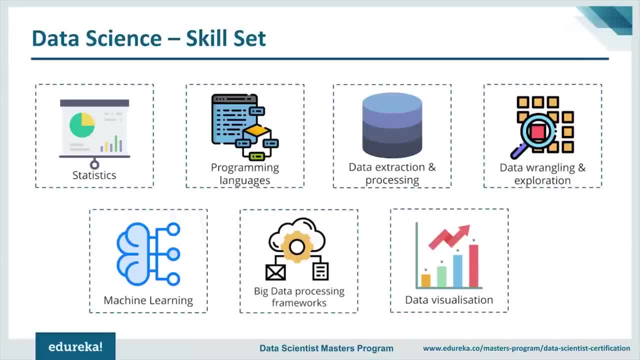 And these predefined packages have most of the algorithms in them, So you don't have to actually sit down and code the algorithms. Instead, you can just load one of these packages from their libraries and run it. So programming languages is a must. At the minimum, you should know R or Python. 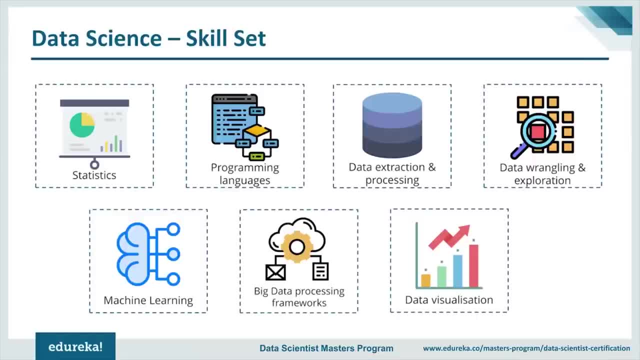 and a database querying language. Now let's move on to data extraction and processing. So guys suppose that you have multiple data sources, like MySQL database, Mongo database. Okay, so what you have to do is you have to extract from such sources. 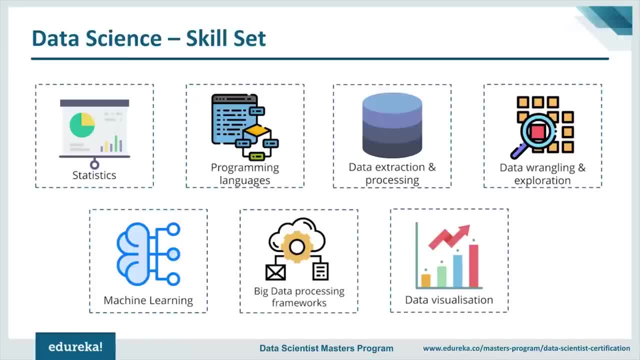 And then, in order to analyze and query this database, you have to store it in a proper format or a proper structure. Okay, finally, then you can load the data in the data warehouse and you can analyze the data over here. Okay, so this entire process. 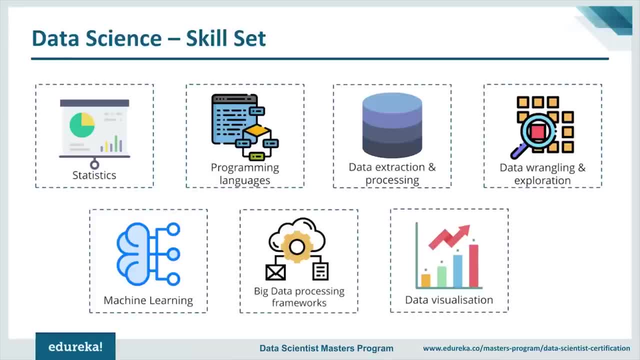 is called extraction and processing. So, guys, extraction and processing is all about getting data from these different data sources and then putting it in a format so that you can analyze it Now. next is data wrangling and exploration. Now, guys, data wrangling is one of the most difficult tasks. 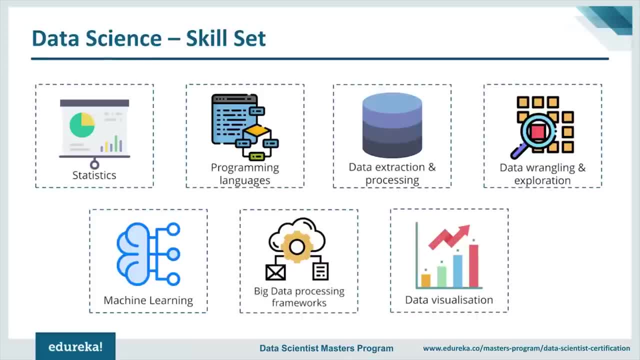 in data science, This is the most time consuming task, because data wrangling is all about cleaning the data. There are a lot of instances where the data sets have missing values, or they have null values, or they have inconsistent formats or inconsistent values. Now you need to understand what to do with such values. 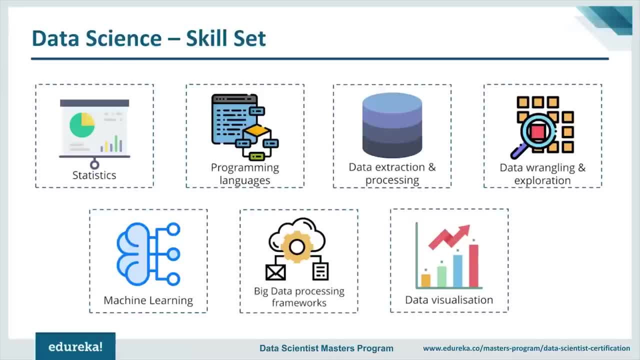 This is where data wrangling, or data cleaning, comes into the picture. Then, after you're done with that, you are going to analyze the data. So, guys, after data wrangling and cleaning is done, you're going to start exploring. This is where you try to make sense out of the data. 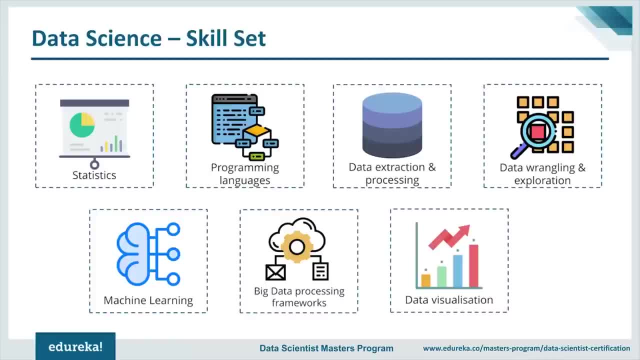 Okay, so you can do this by looking at the different patterns in the data, the different trends, outliers and various unexpected results, and all of that. Next we have machine learning. So, guys, if you're a large company with huge amounts of data, 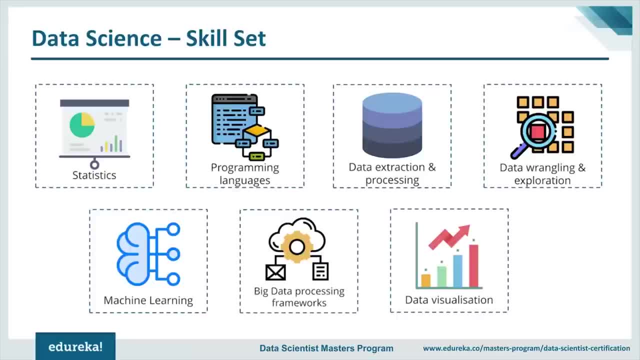 or if you're working at a company where the product is data driven, like if you're working in Netflix or Google Maps, then you have to be familiar with machine learning methods. All right, you cannot process large amount of data with traditional methods. 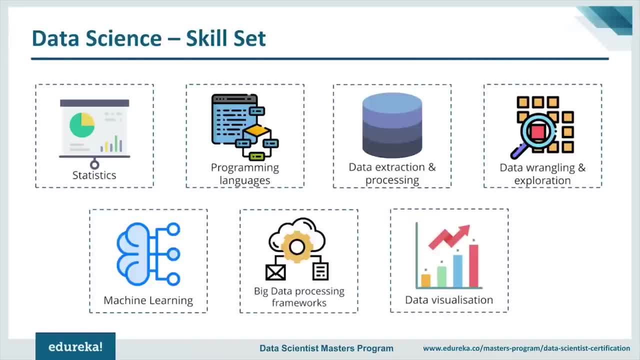 So that's why you need machine learning algorithms. So there are a few algorithms like KNN or K-Nearest Neighbor, There's Random Forest, there's K-Means Algorithm, there's Support Vector Machines, All of these algorithms. you have to be aware of all of these algorithms. 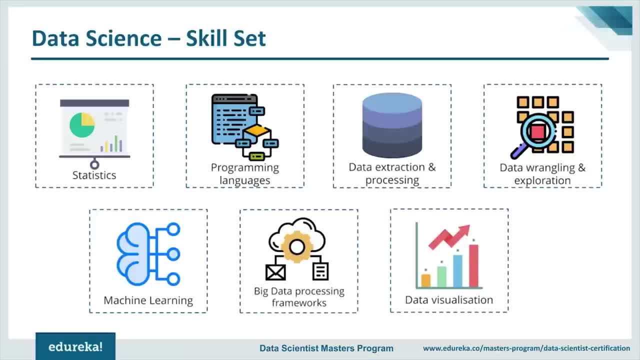 And let me tell you that most of these algorithms can be implemented using R or Python libraries. Okay, you need to have an understanding of machine learning if you have large amount of data in front of you, which is going to be the case for most of the people right now. 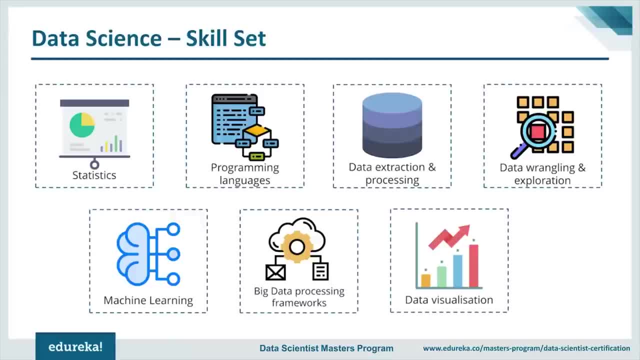 Because data is being generated at an unstoppable pace. Earlier in the session we discussed how much of data is generated. So, for now, knowing machine learning algorithms and machine learning concepts is a very required skill if you want to become a data scientist. So if you're sitting for an interview as a data scientist, 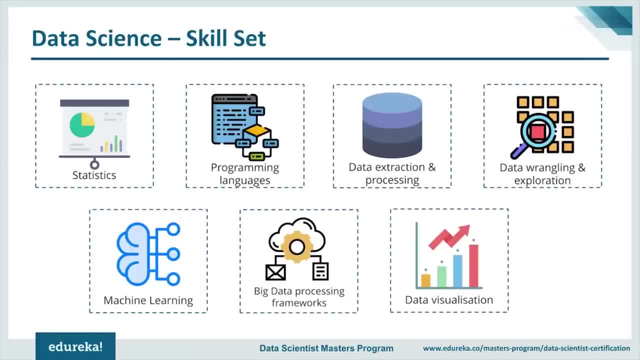 you will be asked machine learning algorithms. you will be asked how good you are with these algorithms and how well you can implement them. Next, we have big data processing frameworks. So, guys, we know that we've been generating a lot of data, and most of this data can be structured. 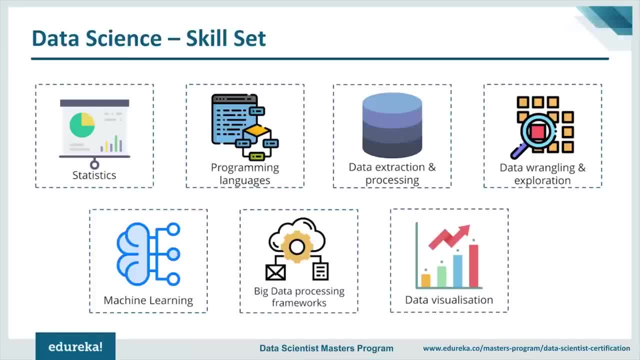 or unstructured as well. So on such data, you cannot use traditional data processing system. So that's why you need to know frameworks like Hadoop and Spark. Okay, these frameworks can be used to handle big data. Lastly, we have data visualization. 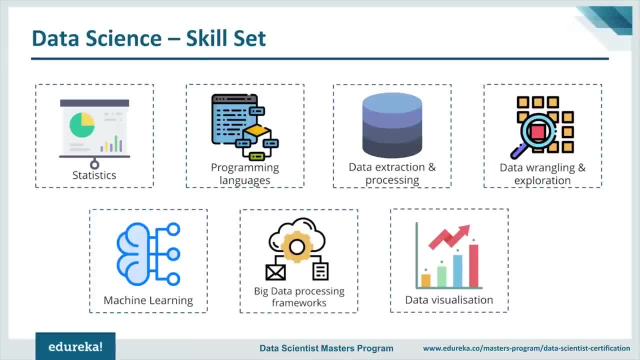 So, guys, data visualization is one of the most important part of data analysis. It is always very important to present the data in an understandable and visually appealing format. Data visualization is one of the skills that data scientists have to master. Okay, if you want to communicate the data? 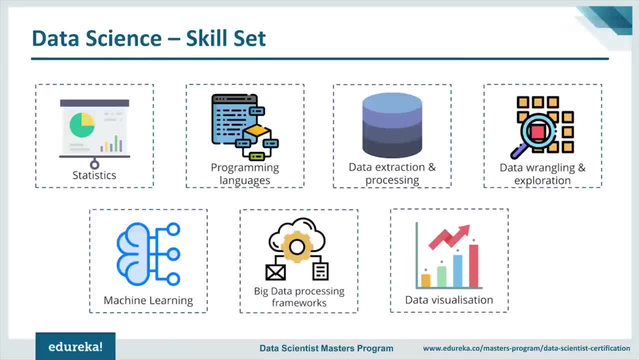 with the end users in a better way, then data visualization is a must. So there's a lot of tools which can be used for data visualization. Tools like Tableau and Power BI are few of the most popular visualization tools. So with this we sum up the entire skill set. 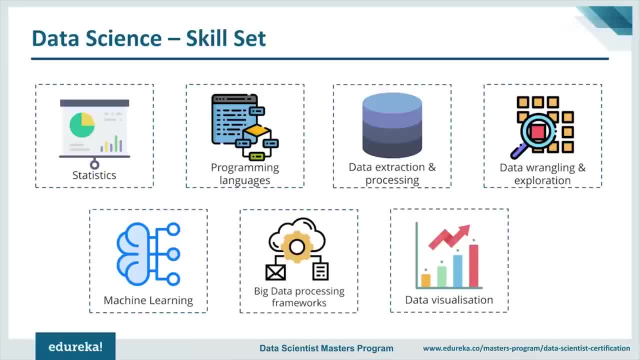 that is needed to become a data scientist. Apart from this, you should also have data-driven problem-solving approach. You should also have data-driven problem-solving approach. You should also be very creative with data. So now that we know the skills that are needed, 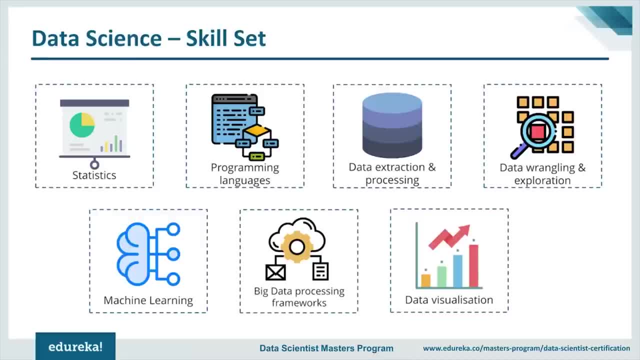 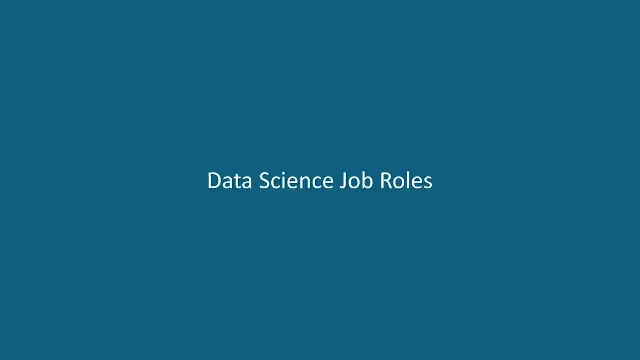 to become a data scientist. let's look at the different job roles, Since data science is a very vast field. there are many job roles under data science, So let's take a look at each role. Let's start off with a data scientist. 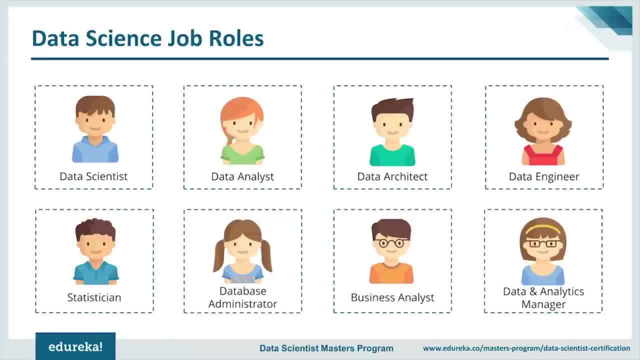 So, guys, data scientists have to understand the challenges of a business and they have to offer the best solution using data analysis and data processing. So, for instance, if they are expected to perform predictive analysis, they should also be able to identify trends and patterns. 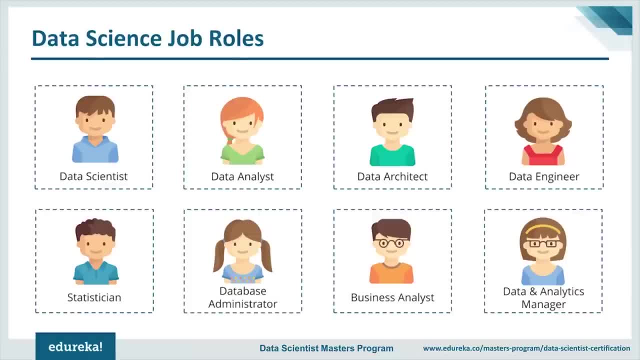 that can help the companies in making better decisions. To become a data scientist, you have to be an expert in R, MATLAB, SQL, Python and other complementary technologies. It can also help if you have a higher degree in mathematics or computer engineering. 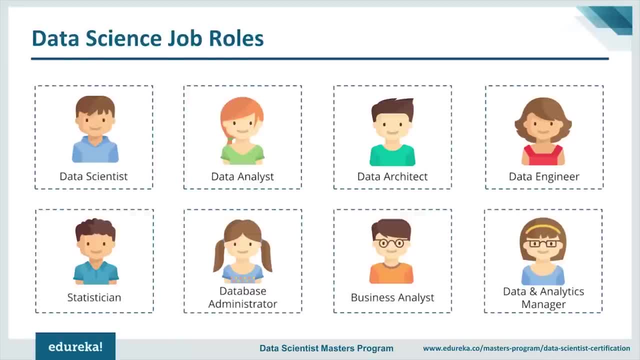 Next we have data analysts, So a data analyst is responsible for a variety of tasks, including visualization, processing of massive amount of data and munging. They can also perform queries on databases, so they should be aware of the different querying languages. 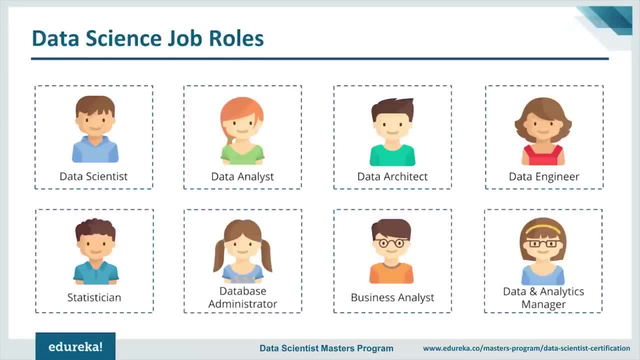 And guys, one of the most important skills of a data analyst is optimization. This is because they have to create and modify algorithms that can be used to pull information from some of the biggest databases without corrupting the data. So to become a data analyst? 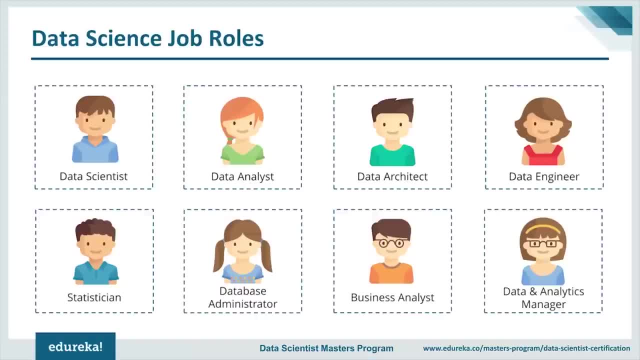 you must know technologies such as SQL, R, SAS and Python, So certification in any of these technologies can boost your job application. You should also have a good problem-solving quality. Next, we have a data architect. So a data architect creates the blueprints. 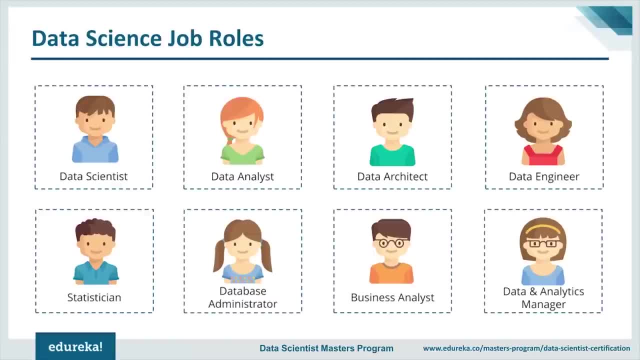 for a data management so that the databases can be easily integrated, centralized and protected with the best security measures. They also ensure that the data engineers have the best tools and systems to work with. So to become a data architect, you have to have expertise in data warehousing. 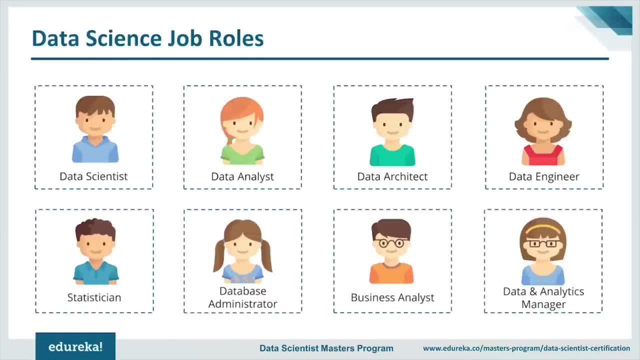 data modeling, extraction, transformation and loan. Okay, So that's the first in Hive Pig and Spark. Now, apart from this, there are data engineers. So, guys, the main responsibility of a data engineer is to build and test scalable big data ecosystems. 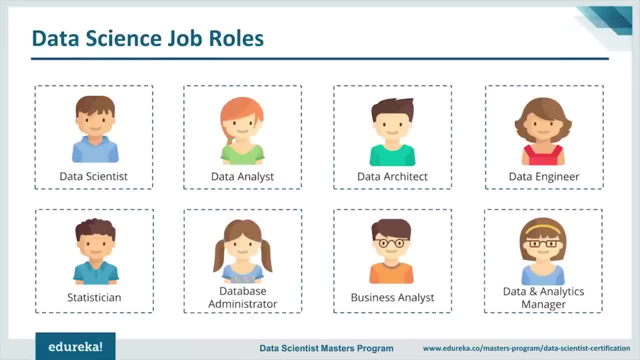 Okay. They are also needed to update the existing systems with newer or upgraded versions, and they are also responsible for improving the efficiency of a database. Now, if you're interested in a career as a data engineer, then technologies that require hands-on experience. 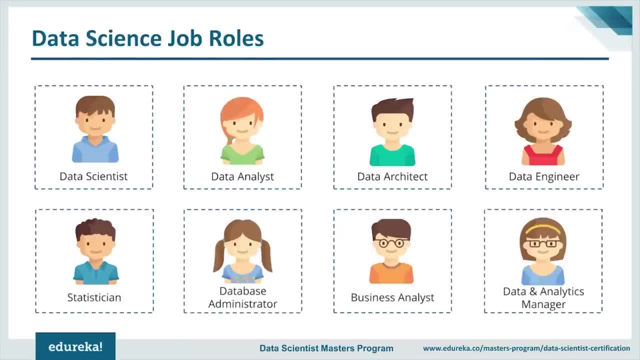 include Hive, NoSQL, R, Ruby and Python, Java, C++ and MATLAB. It would also help if you can work with popular data APIs and ETL tools. Next, we have a statistician, So, as the name suggests, you have to have a sound understanding. 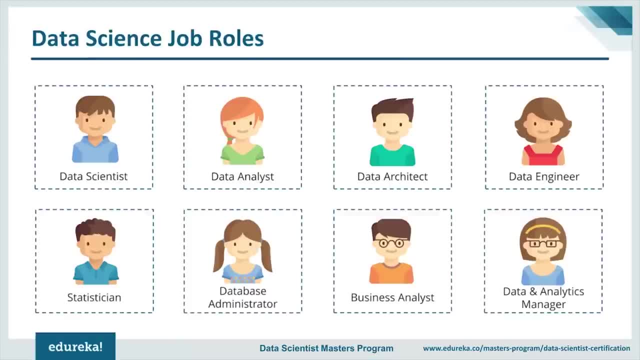 of statistical theories and data organization. Not only do they extract and offer valuable insights, they also create new methodologies for engineers to apply. Now, if you want to become a statistician, then you have to have a passion for logic. They are also a good variety of database systems, such as SQL, data mining and so on. 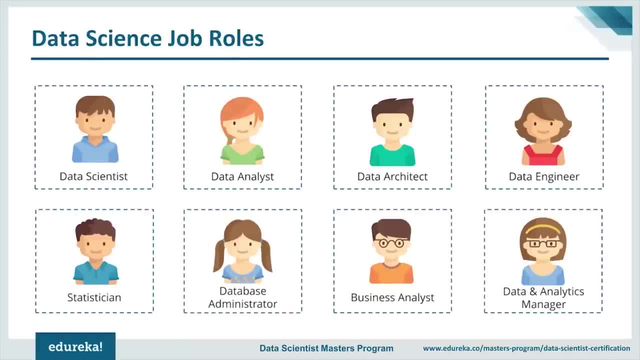 They are also a good variety of database systems such as SQL data mining and so on. They are also a good variety of database systems such as SQL data mining and so on. By that I mean you should be good with math. 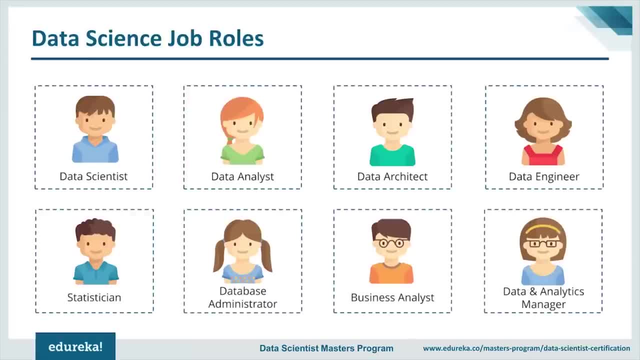 And you should also have a good knowledge about the various database systems, such as SQL, And also the various machine learning concepts and algorithms, is a must. Next we have the database administrator. So, guys, the job profile of a database administrator is pretty much self-explanatory. 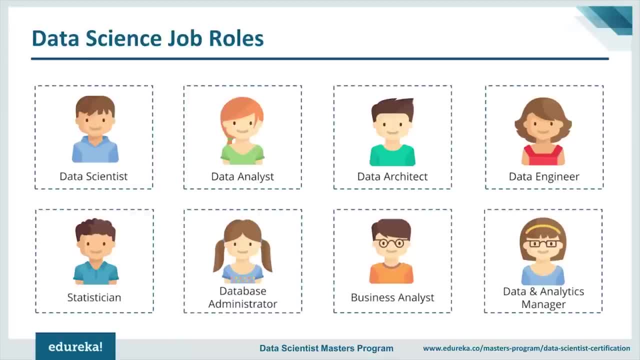 They are basically responsible for the proper functioning of all the databases And they are also responsible for granting permission and revoking its services services to the employees of the company. They also have to take care of the database backups and recoveries. So some of the skills that are needed to become a database administrator include: 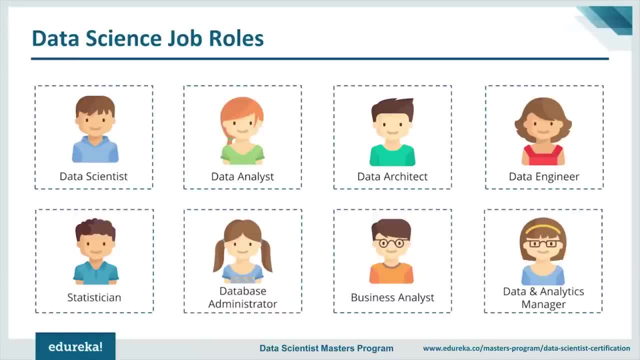 database backup and recovery, data security, data modeling and design. Next, we have the business analyst. Now the role of a business analyst is a little bit different from all of the other data science jobs. Now, don't get me wrong. they have a very good understanding of the data-oriented 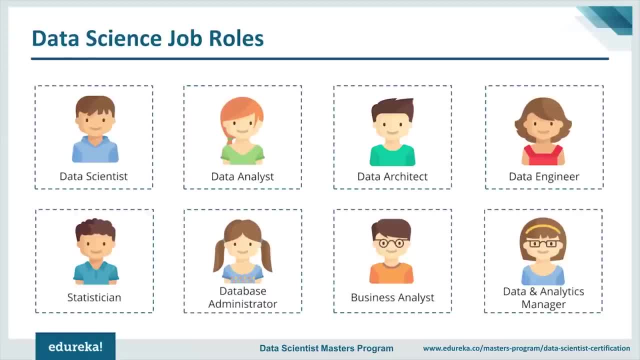 technologies. They know how to handle a lot of data and process it, but they are also very focused on how this data can be linked to actionable business insights. So they mainly focus on business growth. Okay now, a business analyst acts like a link between the data engineers and the 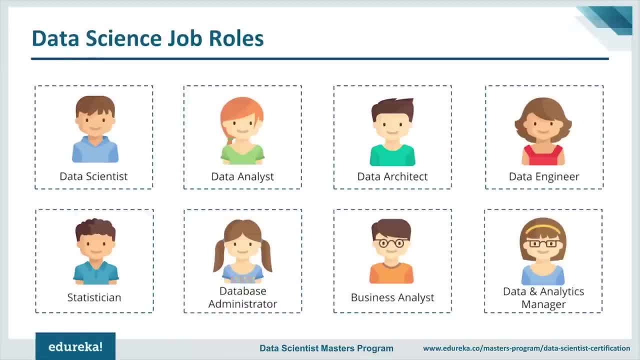 management executives. So, in order to become a business analyst, you have to have an understanding of business finances, business intelligence and also IT technologies like data modeling, data visualization tools and etc. At last, we have the business analyst. So the business analyst. 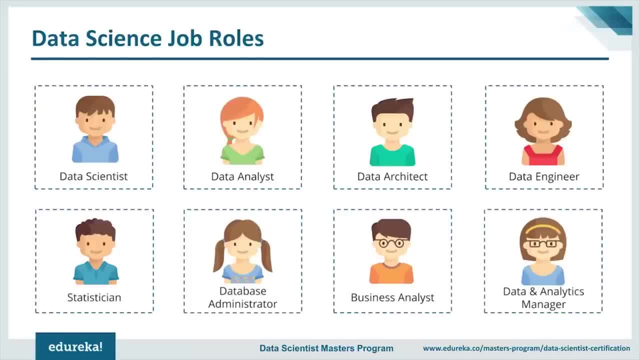 has a data and analytics manager. A data and analytics manager is responsible for the data science operations. Now, the main responsibility of a data and analytics manager is to oversee the data science operation. Okay, he's responsible for assigning the duties to the team. according, 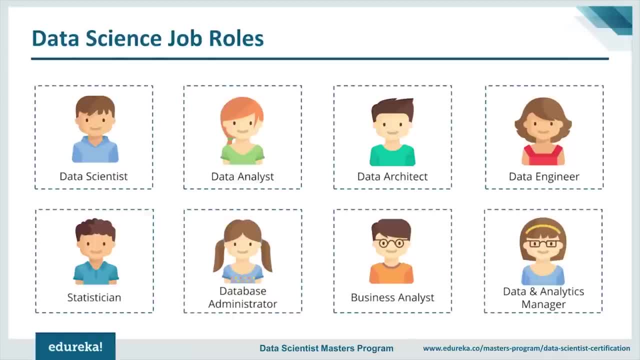 to their skills and expertise. Now their strengths should include technologies like SAS, R, SQL and, of course, they should have good management skills. Apart from that, they must have excellent social skills, leadership qualities and a good management skills. 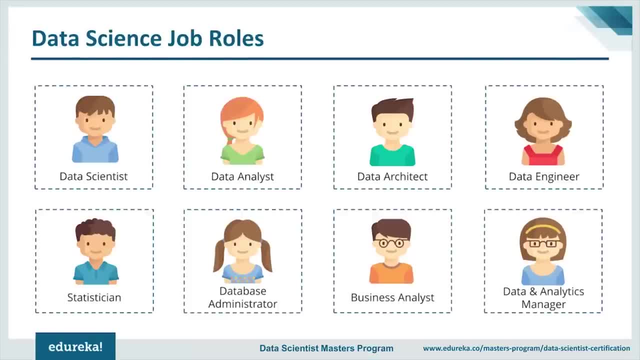 And an out of the box thinking attitude And, like I said earlier, you need to have a good understanding of technologies like Python, SAS, R, Java and etc. So, guys, these were the different job roles in data science. I hope you all found this informative. Now let's move ahead and look. 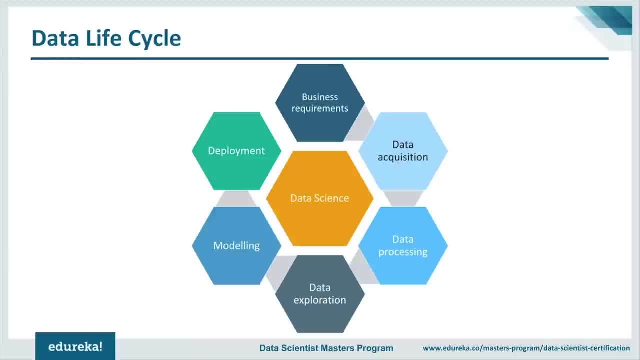 at the data lifecycle. So guys are basically six steps in the data lifecycle. It starts with a business requirement And next is the data acquisition. After that you'll process the data, which is called data processing. Then there is data exploration, which is called data. 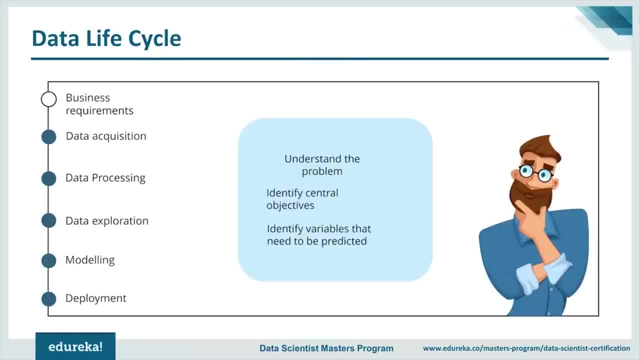 integration, modeling and, finally, deployment. So, guys, before you even start on a data science project, it is important that you understand the problem you're trying to solve. So, in this stage, you're just going to focus on identifying the central objectives of the project And you'll 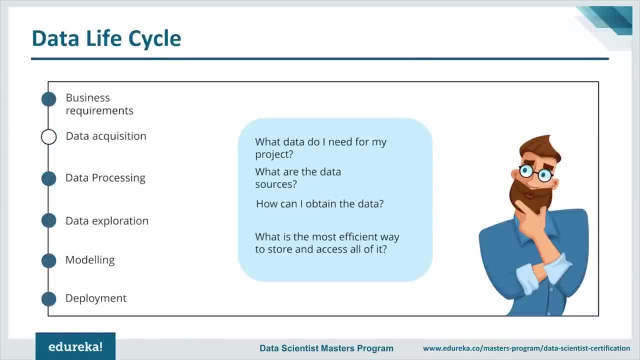 do this by identifying the variables that need to be predicted. Next up, we have data acquisition. Okay, so now that you have your objectives defined, it's time for you to start gathering the data. So data mining is the process of gathering your data from different 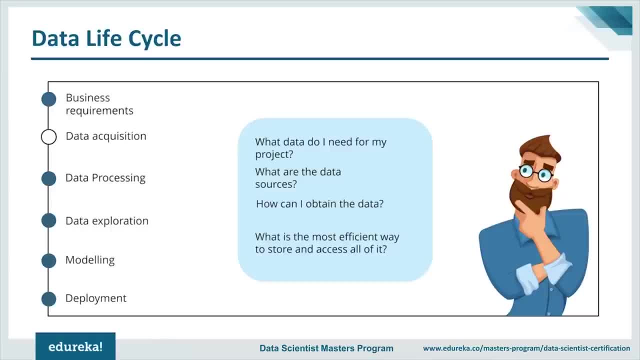 sources. At this stage, some of the questions you can ask yourself is: what data do I need for my project, Where does it live, How can I obtain it And what is the most efficient way to store and access all of it? Next up, there is data processing. Now usually all the data that you 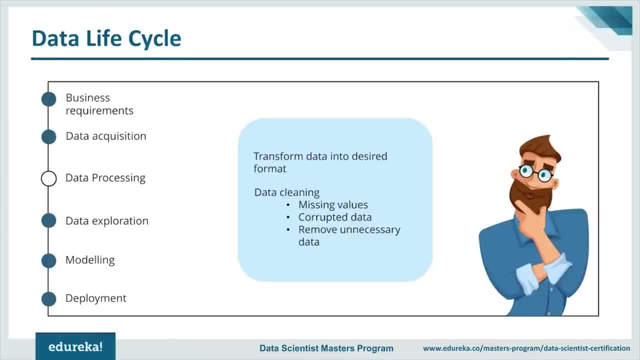 collected is a huge mess. Okay, it's not formatted, it's not structured, it's not cleaned. So if you find any data set that is cleaned and it's packaged well for you, then you've actually won, because finding the right data takes a lot of time and it takes a lot of effort, And one of the major 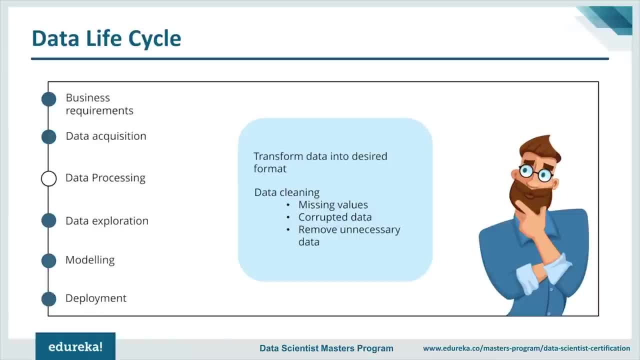 time consuming tasks in the data science process is data cleaning. Okay, this requires a lot of time. it requires a lot of effort because you have to go through the entire data set to find out any missing values or if there are any inconsistent values or corrupted data, And you also find the 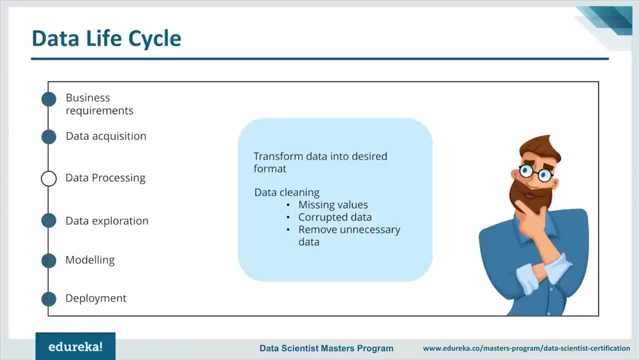 unnecessary data over here and you remove that data. So this was all about data processing. Next we have data exploration. So now that you have a sparkling clean set of data, you are finally ready to get started with your analysis. Okay, the data exploration stage is basically the brainstorming of data analysis. 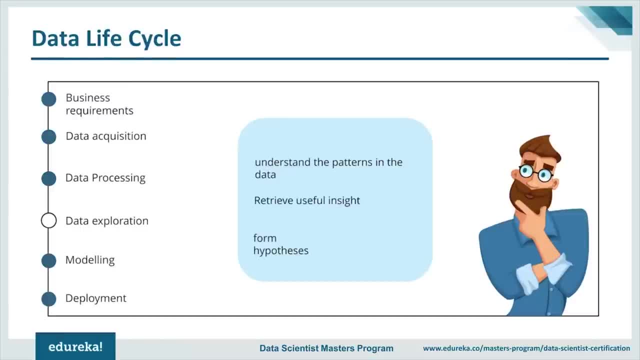 So, in order to understand the patterns in your data, you can use histogram. you can just pull up a random subset of data and plot a histogram. you can even create interactive visualizations. This is the point where you dive deep into the data and you try to explore the different models that can be applied to your data. Next up, we have 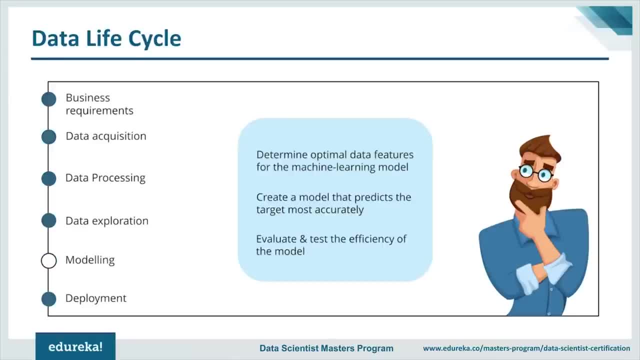 modeling. So, after processing the data, what you're going to do is you're going to carry out model training. Okay now, model training is basically about finding the model that answers the questions more accurately. So the process of model training involves a lot of steps. So, firstly, you start by 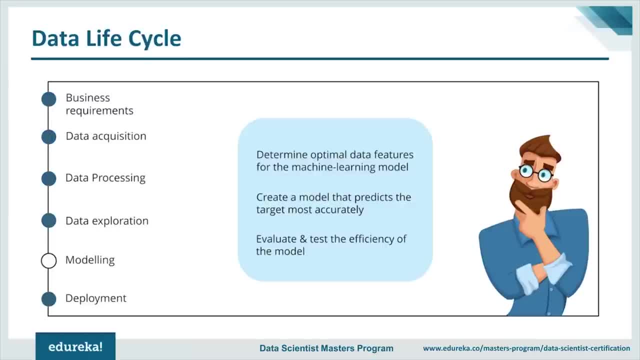 splitting the input data into the training data set and the testing data set. Okay, you're going to take the entire data set and you're going to separate it into two parts: One is the training and one is the testing data. After that, you'll build a model by using the training data set And 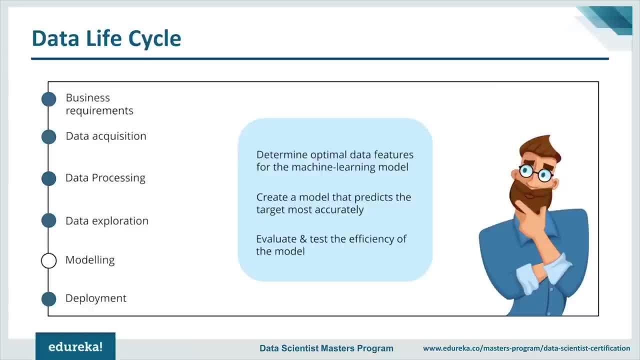 once you're done with that, you'll evaluate the training and the test data set. Now, to evaluate the training and testing data set, you'll be using a series of machine learning algorithms. After that, you'll find out the model which is the most suitable for your business requirement. 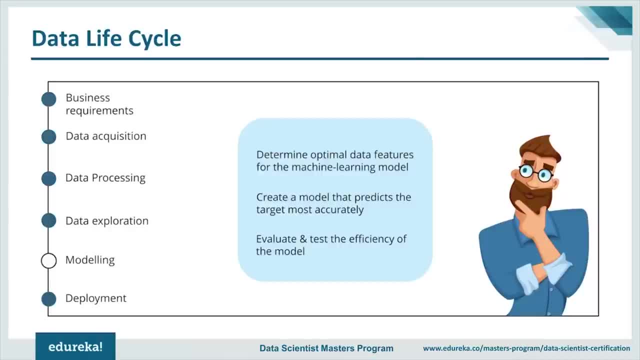 So this was mainly data modeling. Okay, this is where you build a model out of your training data set And then you evaluate this model by using the testing data set. Next we have deployment. So, guys, the goal of this stage is to deploy the model into a production, or maybe a production. 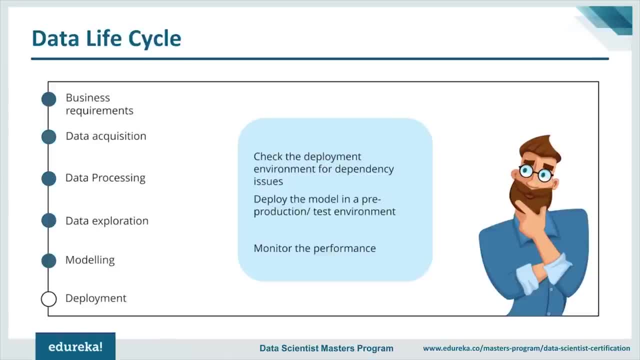 like environment. So this is basically done for final user acceptance, And the users have to validate the performance of the models, And if there are any issues with the model or any issues with the algorithm, then they have to be fixed in this stage. So, guys, with this we come to the end. 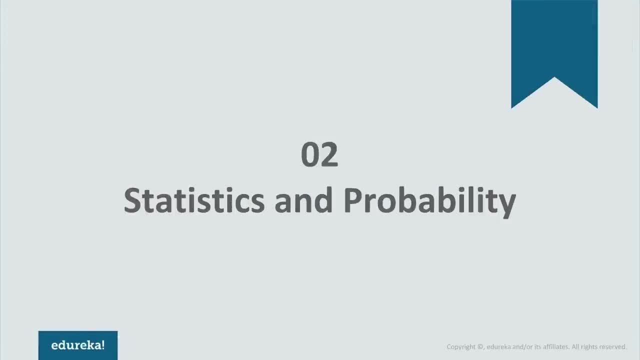 of the data lifecycle. I hope this was clear. Statistics and probability are essential because these disciples form the basic foundation of all machine learning applications, Algorithms, deep learning, artificial intelligence and data science. In fact, mathematics and probability is behind everything around us, From shapes, patterns and colors. 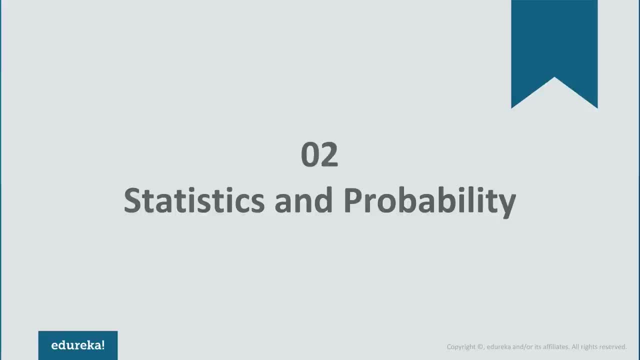 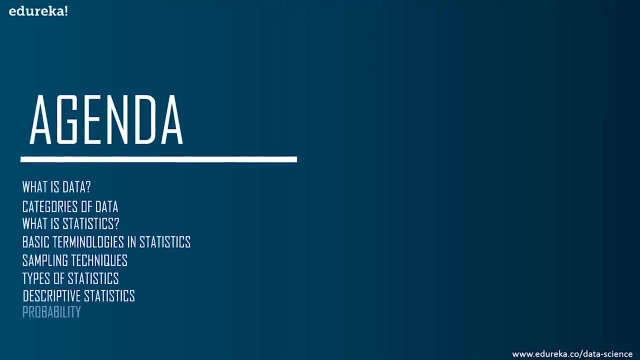 to the count of petals in a flower. mathematics is embedded in each and every aspect of our lives. With this in mind, I welcome you all to today's session, So I'm going to go ahead and discuss the agenda for today with you all. We're going to begin the session by understanding what is data. 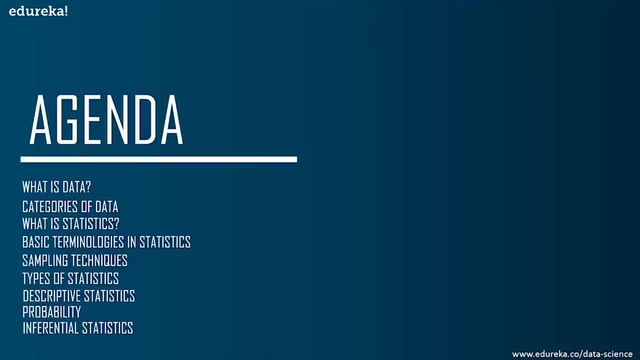 After that we'll move on and look at the different categories of data, like quantitative and qualitative data. Then we'll discuss what exactly statistics is, the basic terminologies in statistics and a couple of sampling techniques. Once we're done with that, we'll discuss the 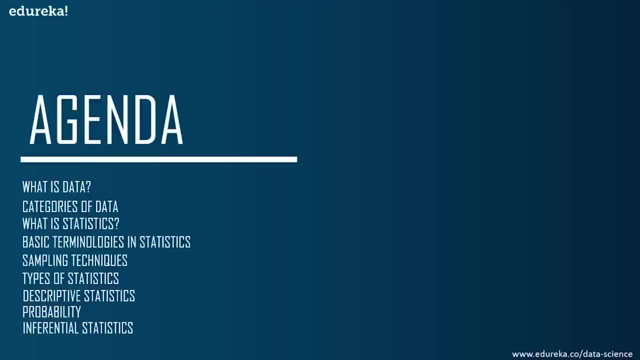 different types of statistics, which involve descriptive and inferential statistics. Then in the next session we'll mainly be focusing on descriptive statistics. Here we'll understand the different measures of center, measures of spread, informative data and, most importantly, data science. So let's get started. 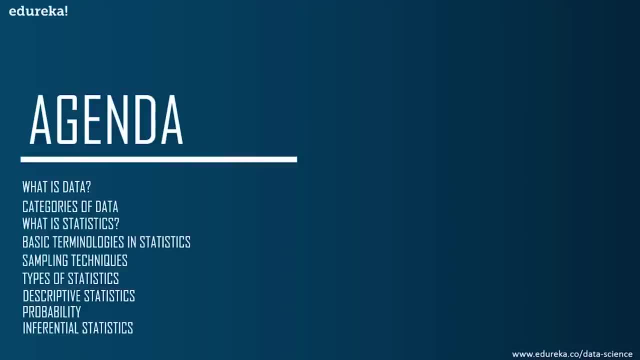 gain and entropy. We'll also understand all of these measures with the help of a use case and finally, we'll discuss what exactly a confusion matrix is. Once we've covered the entire descriptive statistics module, we'll discuss the probability module. Here we'll understand what exactly probability is. the 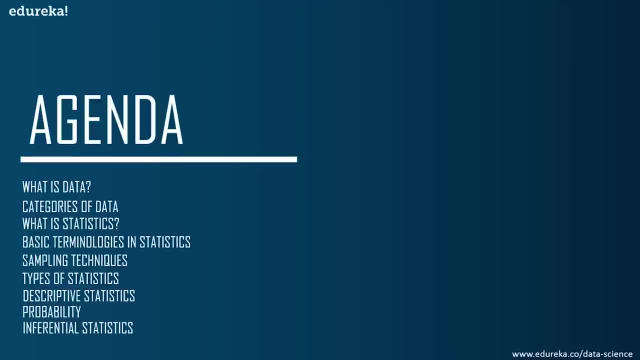 different terminologies in probability. We'll also study the different probability distributions. Then we'll discuss the types of probability, which include marginal probability, joint and conditional probability. Then we'll move on and discuss a use case wherein we'll see examples that show us how the 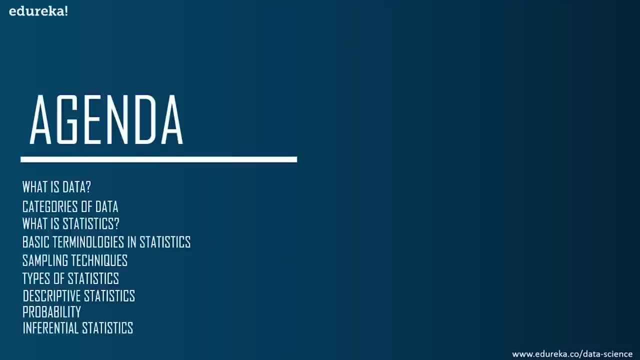 different types of probability work And to better understand Bayes theorem, we'll look at a small example. Also, I forgot to mention that at the end of the descriptive statistics module we'll be running a small demo in the R language. So for those of you who don't know much about R, I'll be explaining every line in. 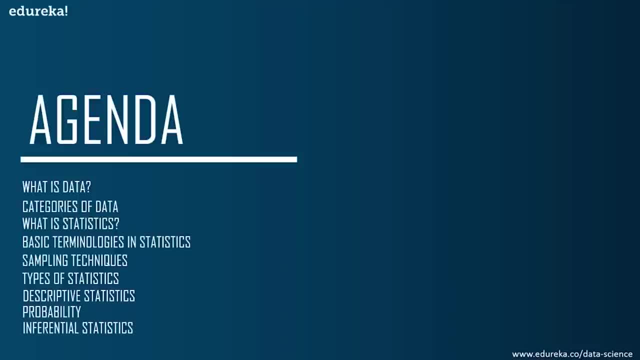 depth. But if you want to have a more in-depth understanding about R, I'll leave a couple of blogs and a couple of videos in the description box. Y'all can definitely check out that content. Now, after we've completed the probability module, we'll discuss the inferential statistics module. We'll start this. 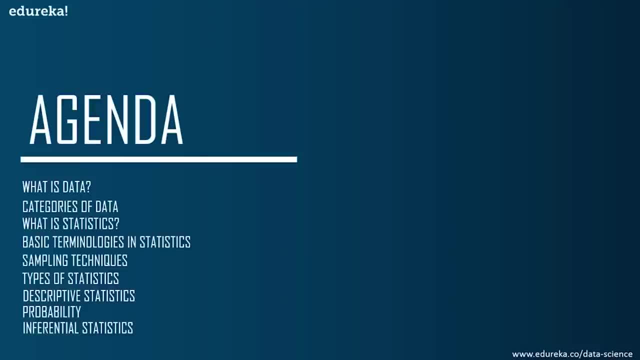 module by understanding what is point estimation. We'll discuss what is confidence interval and how you can estimate the confidence interval. We'll also discuss margin of error and we'll understand all of these concepts by looking at a small use case. We'll finally end the inferential. 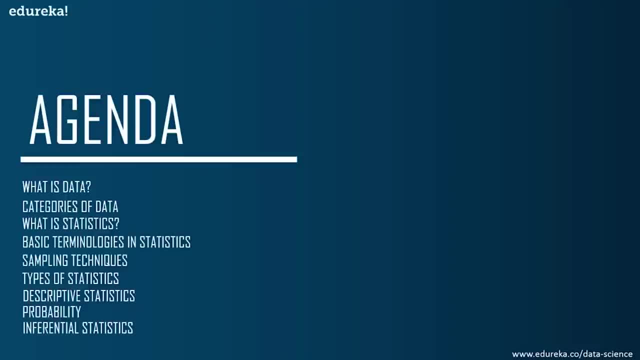 statistic module by looking at what hypothesis testing is. Hypothesis testing is a very important part of inferential statistics, So we'll end the session by looking at a use case that discusses how hypothesis testing works And, to sum everything up, we'll look at a demo that explains how inferential statistics 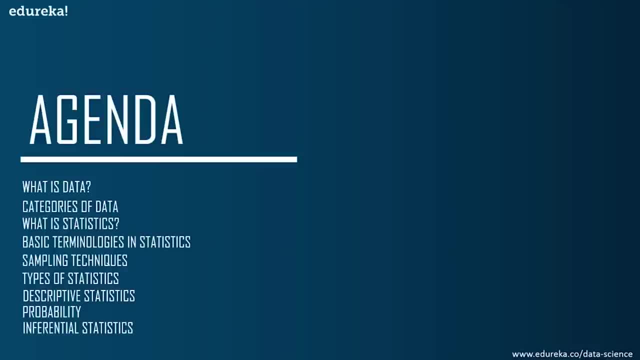 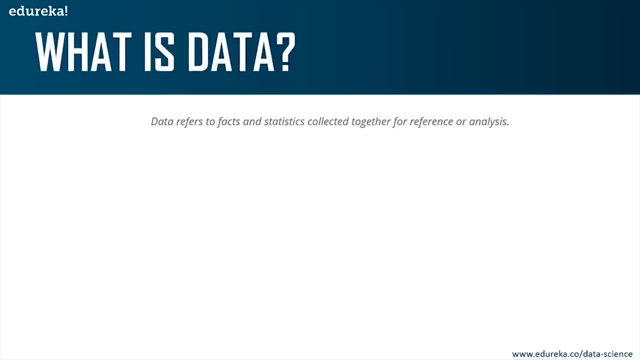 works Alright. so, guys, there's a lot to cover today, So let's move ahead and take a look at our first topic, Which is: what is data? Now, this is a quite simple question. If I ask any of you what is data, you'll see that it's a set of numbers or some sort of documents. 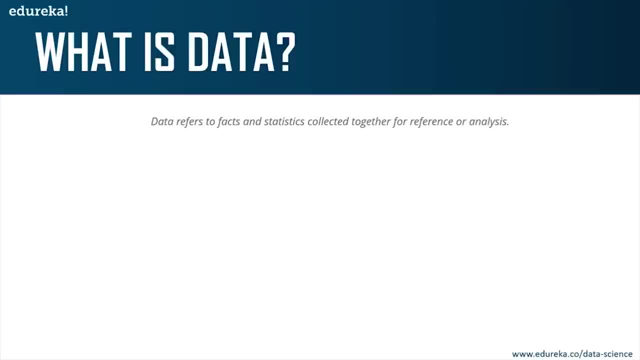 that I've stored in my computer. Now, data is actually everything. Alright, look around you. There is data everywhere. Each click on your phone generates more data than you know Now. this generated data provides insights for analysis and helps us make better business decisions. This is why data is so important. 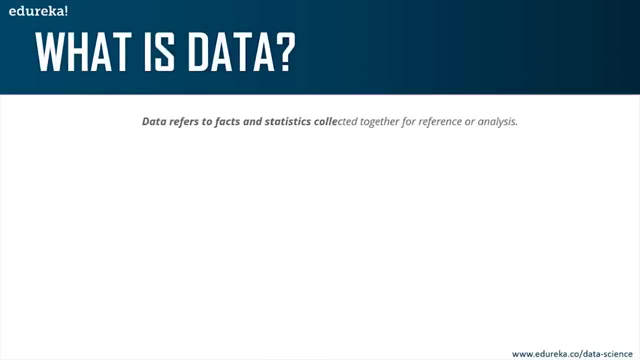 To give you a formal definition: data refers to facts and statistics collected together for reference or analysis. Alright, this is the definition of data in terms of statistics and probability. So, as we know, data can be collected, it can be measured and analyzed. it can be. 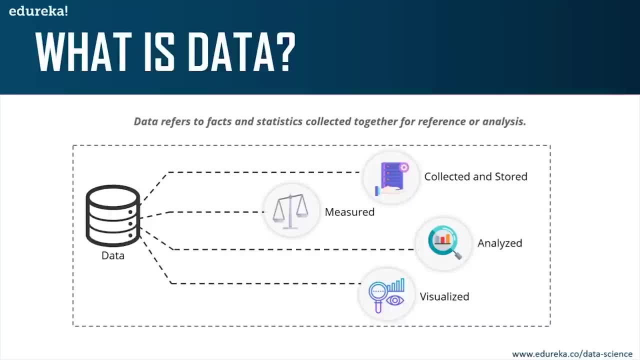 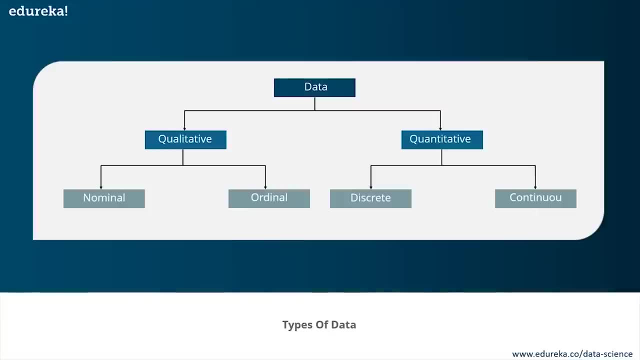 visualized by using statistical models and graphs. Now data is divided into two major subcategories. Alright, so first we have qualitative data and quantitative data. these are the two different types of data. under qualitative data, we have nominal and ordinal data, and under quantitative data we have 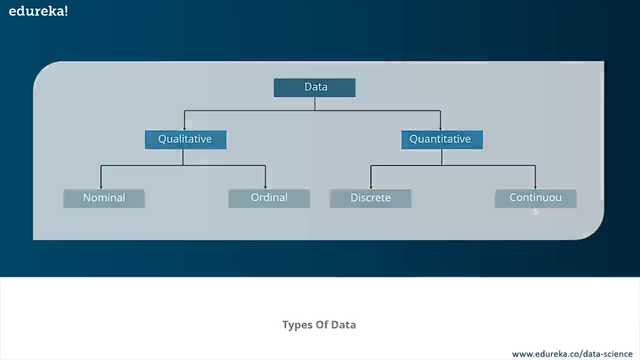 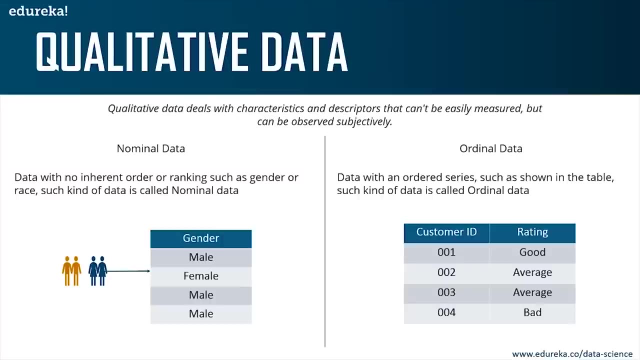 discrete and continuous data. now let's focus on qualitative data. now. this type of data deals with characteristics and descriptors that can't be easily measured, but can be observed subjectively. now qualitative data is further divided into nominal and ordinal data, so nominal data is any sort of data. 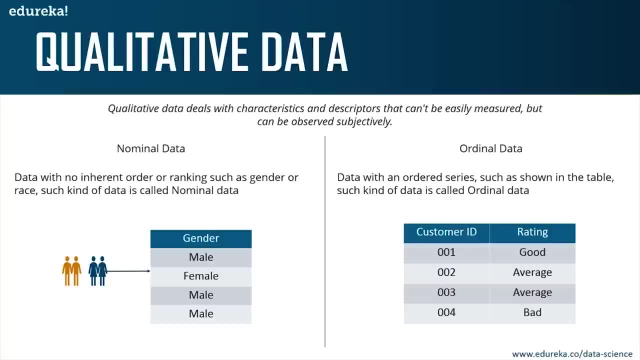 that doesn't have any order or ranking. okay, an example of nominal data is gender. now, there is no ranking in gender. there's only male, female or other right. there is no one, two, three, four or any sort of ordering in gender. race is another example of nominal data. now, ordinal data is basically an ordered 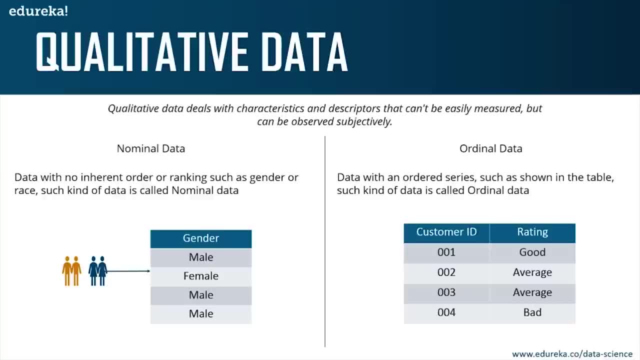 series of information. okay, let's say that you went to a restaurant. okay, your information is stored in the form of customer ID, alright, so basically, you are represented with a customer ID. now you would have rated their service as either good or average. alright, that's how an ordinal data is, and similarly, they'll have a record of. 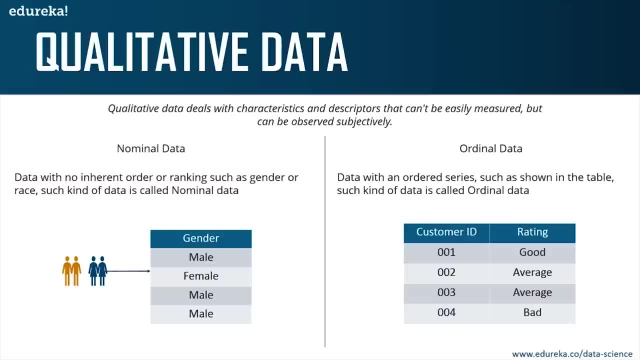 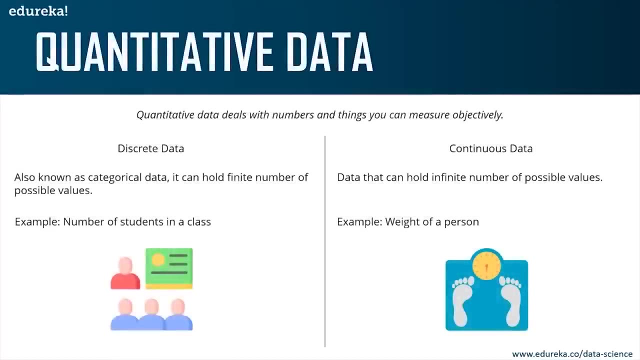 other customers who visit the restaurant, along with their ratings. alright, so any data which has some sort of sequence or some sort of order to it is known as ordinal data. alright, so, guys, this is pretty simple to understand. now let's move on and look at quantitative data. so quantitative data basically deals with: 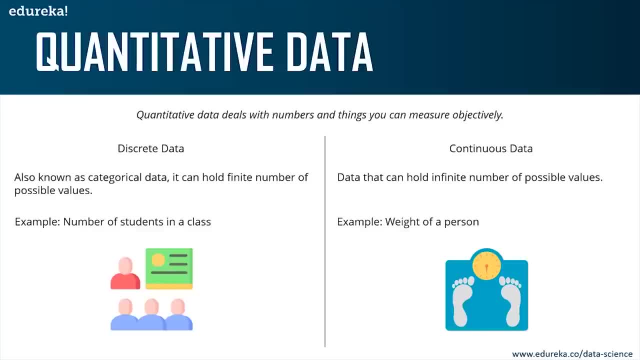 numbers and things. okay, you can understand that by the word quantitative itself. quantitative is basically quantity, right? so it deals with numbers, it deals with anything that you can measure objectively. alright, so there are two types of quantitative data, that is, discrete and continuous data. now, discrete data is also known as categorical data, and it can hold a 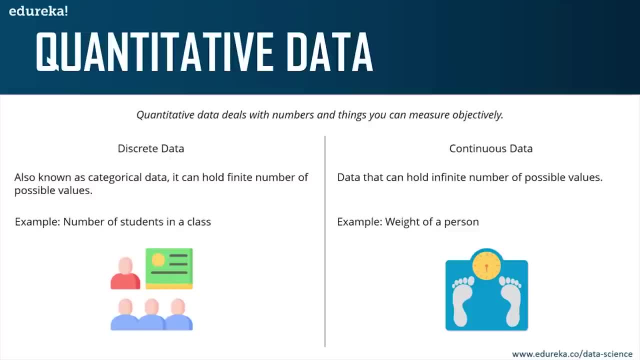 finite number of possible values. now, the number of students in a class is a finite number. all right, you can't have infinite number of students in a class. let's say in your fifth grade there were hundred students in your class. alright, there weren't infinite number, but there was a definite finite number of students. 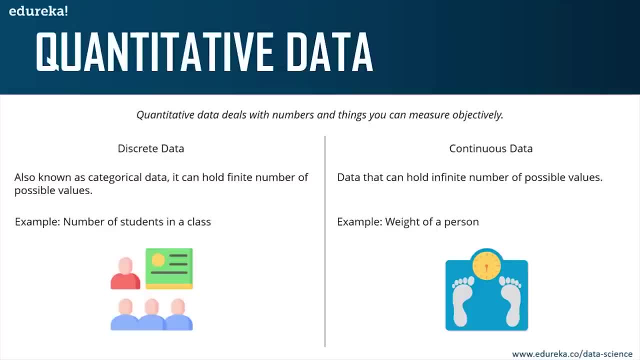 in your class. okay, that's discrete data. next, we have continuous data. now. this type of data can hold infinite number of possible values, okay. so when you say weight of a person is an example of continuous data, what I mean to say is: my weight can be 50 kgs, or it can be 50.1 kgs, or it can be. 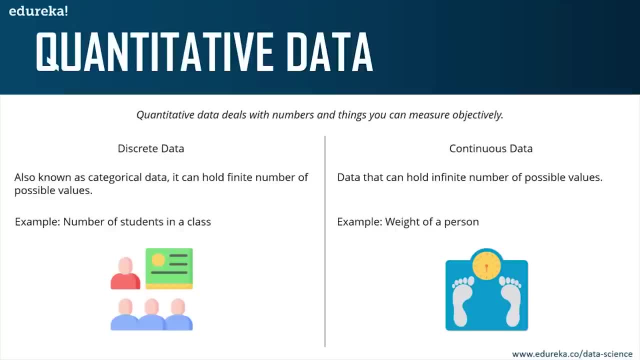 50.001 kgs or 50.0001 or 50.023 and so on, right, there are infinite number of possible values, right? so this is what I mean by continuous data. all right, this is the difference between continuous data and continuous data, and. 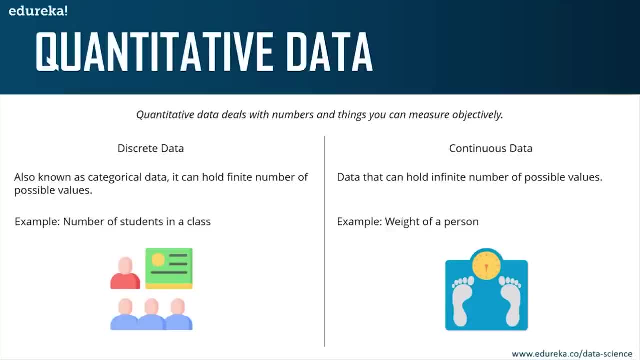 between discrete and continuous data, and also I'd like to mention a few other things over here. now, there are a couple of types of variables as well. alright, we have a discrete variable and we have a continuous variable. discrete variable is also known as a categorical variable. alright, it can hold values of different. 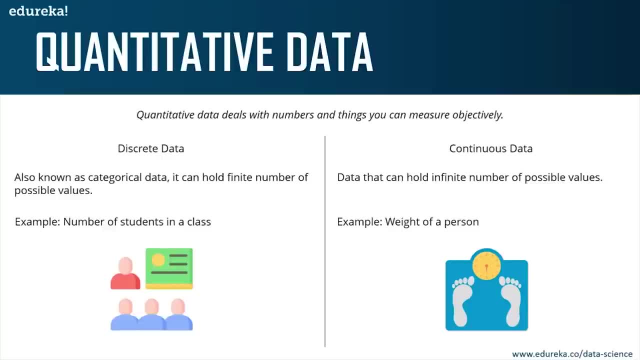 categories. let's say that you have a variable called message and there are two types of values that this variable can hold. let's say that your message can either be a spam message or a non spam message. okay, that's when you call a variable as discrete or categorical variable, all. 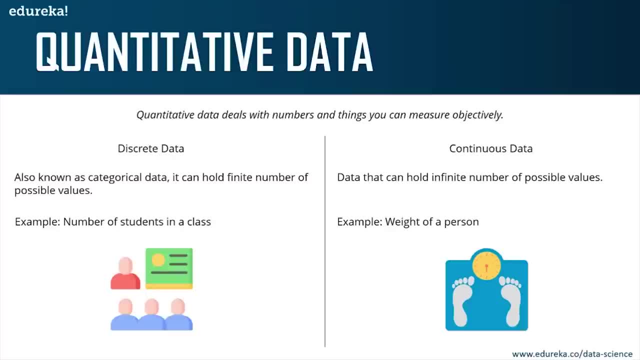 right, because it can hold values that represent different categories of data. now, continuous variables are basically variables that can store infinite number of values. so the weight of a person can be denoted as a continuous variable. all right, let's say there is a variable called weight and it can store infinite. 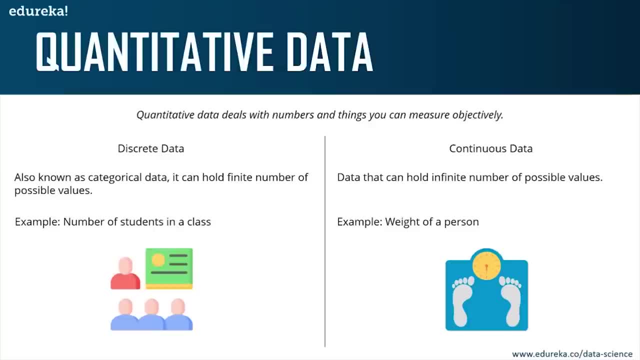 number of possible values. that's why we'll call it a continuous variable. so, guys, basically, variable is anything that can store a value, right? so if you associate any sort of data with a variable, then it will become either discrete variable or continuous variable. that is also dependent and independent. 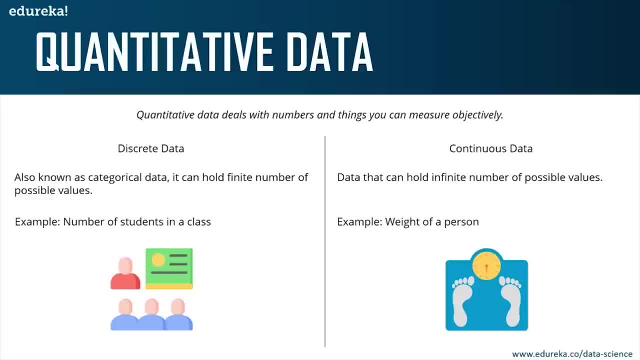 type of variables. now we won't discuss all of that in depth, because that's pretty understandable. I'm sure all of you know what is independent variable and dependent variable. right, dependent variable is any variable whose value is dependent on any other independent variable. so, guys, that much knowledge I. 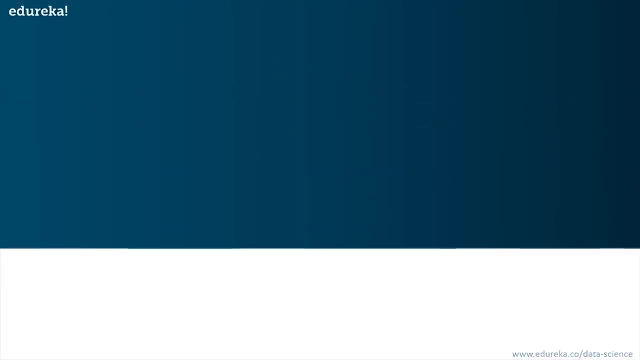 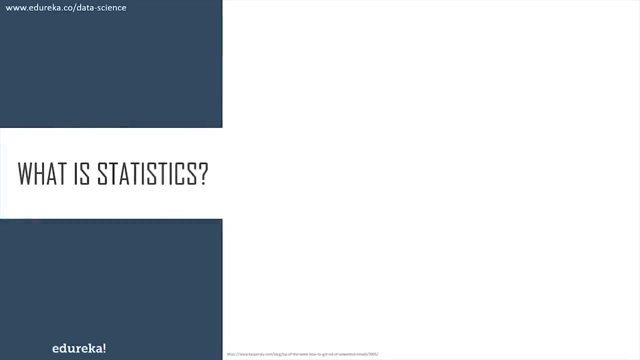 expect all of you to have all right. so now let's move on and look at our next topic, which is: what is statistics? now coming to the formal definition of statistics: statistics is an area of applied mathematics which is concerned with data collection, analysis, interpretation and presentation. now 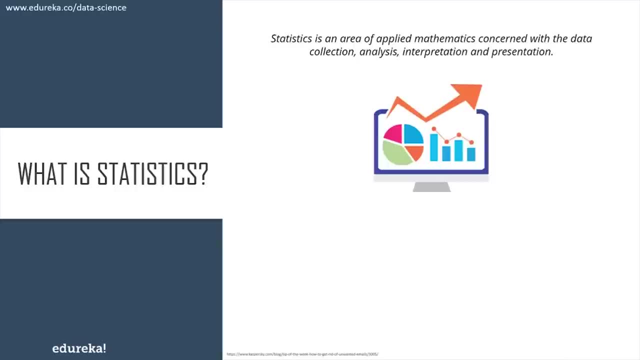 usually when I speak about statistics, people think statistics is all about a, about analysis. but statistics has other parts to it. it has data collection is also a part of statistics. data interpretation, presentation, visualization- all of this comes into statistics. all right, you're going to use statistical methods to visualize data, to collect data, to interpret data, all right. so the 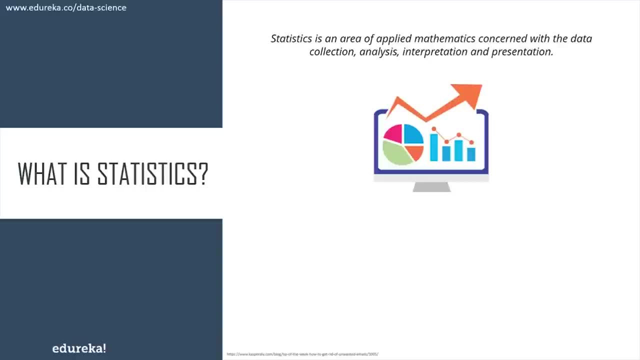 area of mathematics deals with understanding how data can be used to solve complex problems. okay, now I'll give you a couple of examples that can be solved by using statistics. okay, let's say that your company has created a new drug that make your cancer. how would you conduct a test to confirm the drugs? 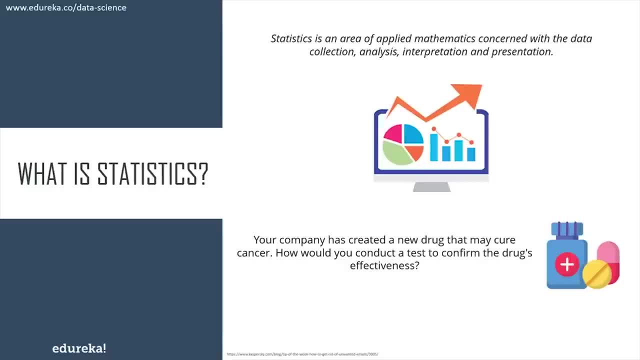 effectiveness. now, even though this sounds like a biology problem, this can be solved with statistics. all right, you will have to create a test which can confirm the effectiveness of the drug. all right, this is a common problem that can be solved using statistics. let me give you another example. you and a 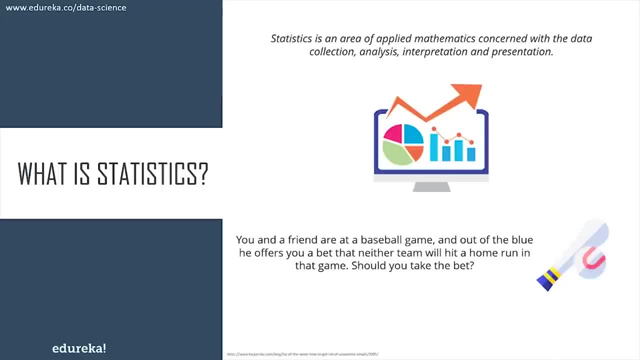 friend are at a baseball game and, out of the blue, he offers you a bet that neither team will hit a home run in that game. should you take the bet? all right. here you just discuss the probability of whether you'll win or lose. all right, this is another problem. 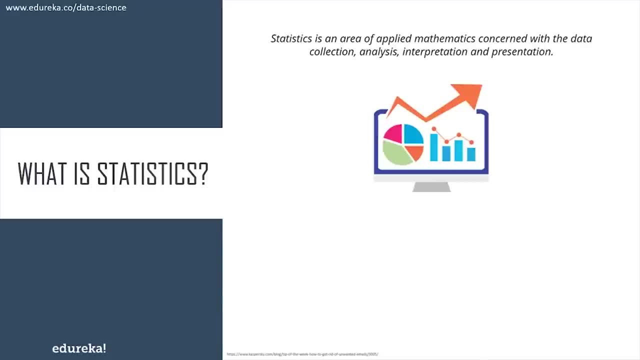 that comes under statistics. let's look at another example. the latest sales data has just come in and your boss wants you to prepare a report for management on places where the company could improve its business. what should you look for and what should you not look for? now, this problem involves a lot of data analysis. you'll have to look at the 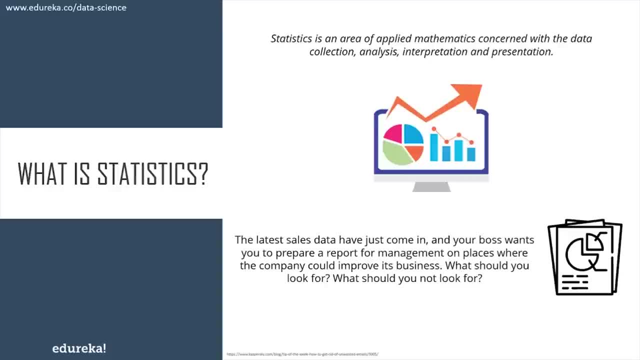 different variables that are causing your business to go down, or that you have to look at a few variables that are increasing the performance of your models and thus growing your business. all right, so this involves a lot of data analysis, and the basic idea behind data analysis is to use statistical 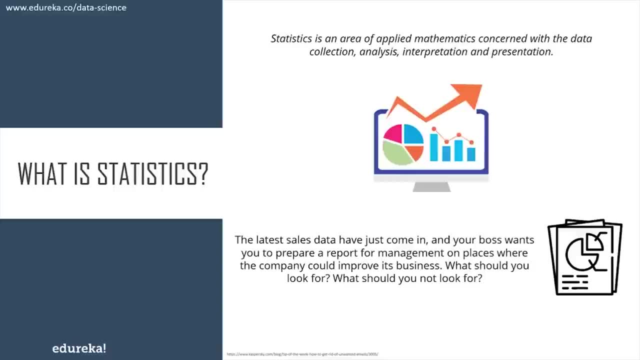 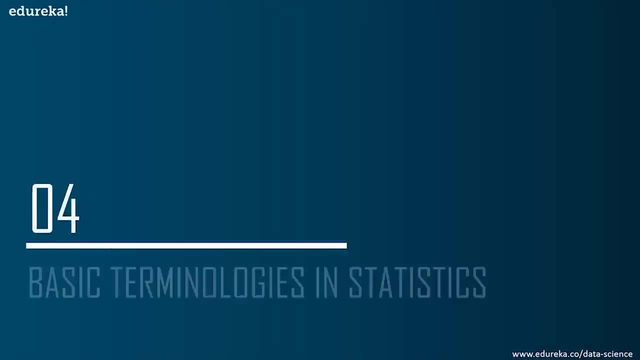 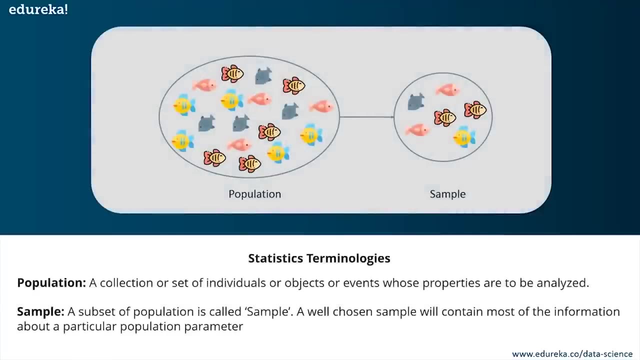 techniques in order to figure out the relationship between different variables or different components in your business. okay, let's move on and look at our next topic, which is basic terminologies in statistics. now, before you dive deep into statistics, it is important that you understand basic terminologies used in statistics, the two most important. 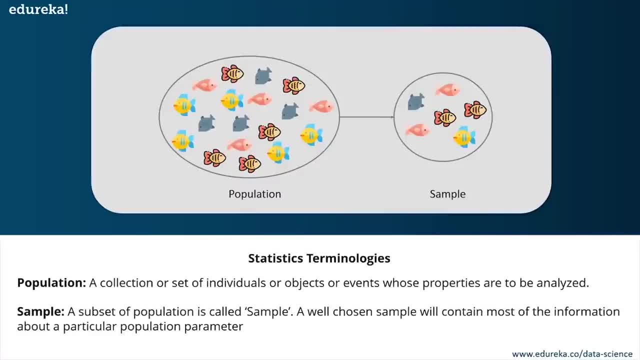 terminologies in statistics are population and sample. so throughout the statistics course, or throughout any problem that you're trying to solve with statistics, you will come across these two words, which is population and sample. now, population is a collection or a set of individuals or objects or events. 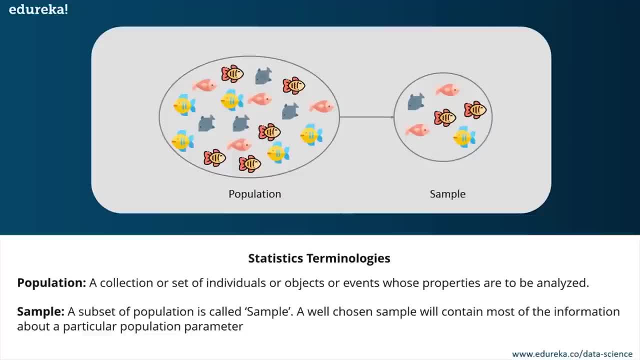 whose properties are to be analyzed. okay, so basically, you can refer to population as a subject that you're trying to analyze now. a sample is just like the word suggests: it's a subset of the population. so you have to make sure that you choose the sample in such a way that it represents the entire population all. 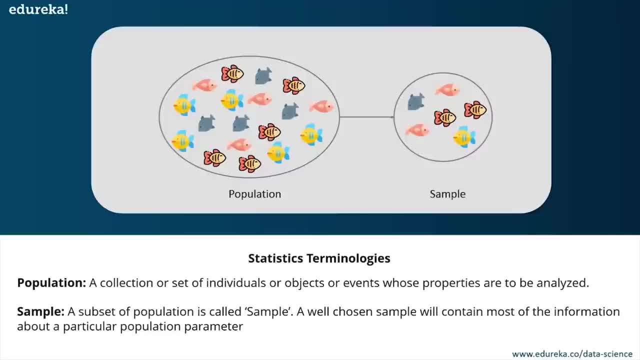 right. it shouldn't focus at one part of the population. instead, it should represent the entire population. that's how your sample should be chosen. so a well-chosen sample will contain most of the information about a particular population parameter. now you must be wondering: how can one choose a? 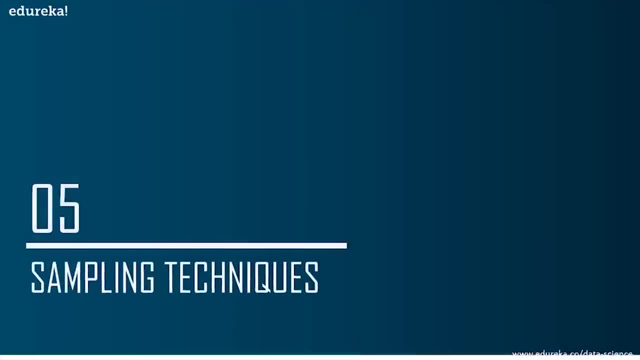 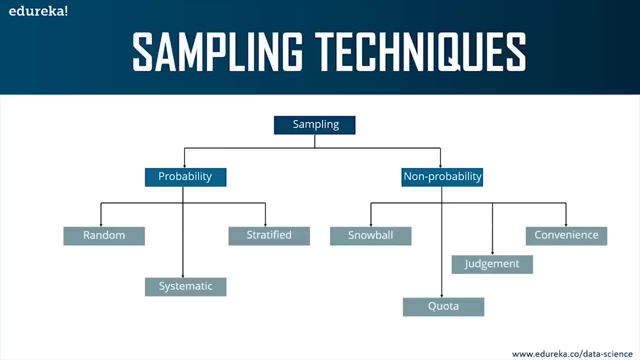 sample that best represents the entire population. now, sampling is a statistical method that deals with the selection of individual observations within a population. so sampling is performed in order to infer statistical knowledge about a population. all right if you want to understand the different statistics of a population, like the mean, the median, the mode or the standard. 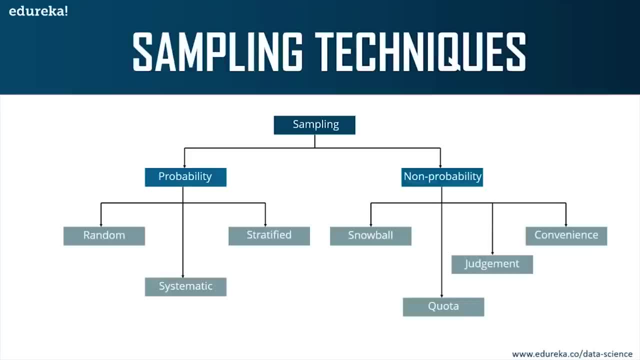 deviation or the variance of a population, then you're going to perform sampling. all right, because it's not reasonable for you to study a large population and find out the mean, median and everything else. so why is sampling performed? you might ask: what is the point of sampling? we can just study the 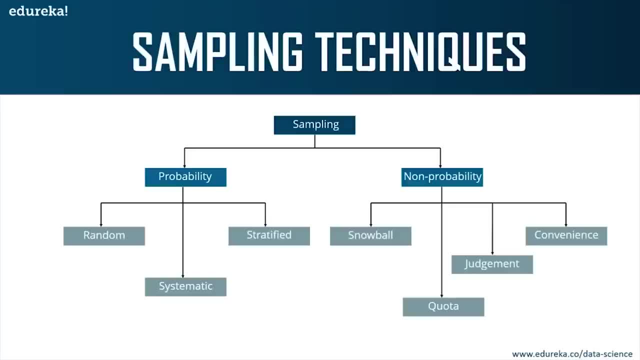 entire population. now, guys, think of a scenario wherein you're asked to perform a survey about the eating habits of teenagers in the US. so at present, there are over 42 million teens in the US and this number is growing as we are speaking right now, correct? is it possible to survey each of these 42 million? 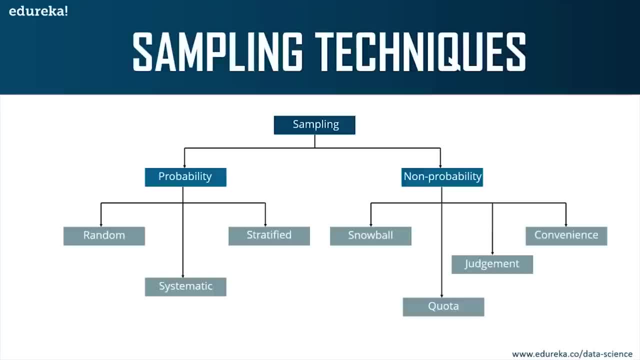 individuals about their health. is it possible? well, it might be possible, but this will take forever to do now. obviously it's not. it's not reasonable to go around knocking each door and asking for what does your teenage son eat? and all of that all right. this is not very. 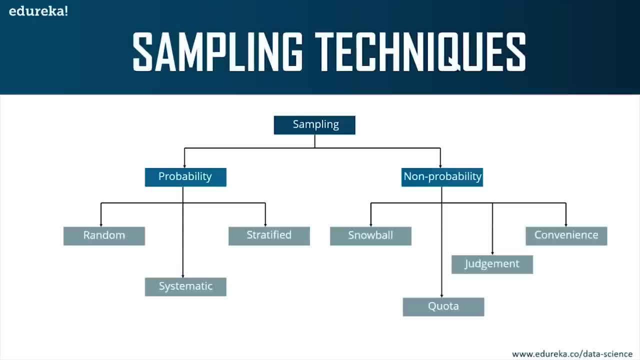 reasonable. that's why sampling is used. it's a method wherein a sample of the population is studied in order to draw inference about the entire population, so it's basically a shortcut to studying the entire population, instead of taking the entire population and finding out all the solutions you're just going to. 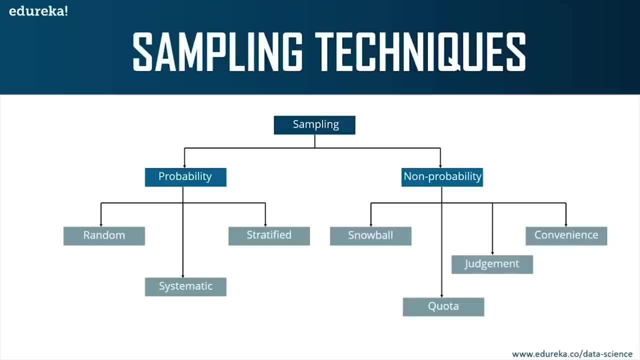 take a part of the population that represents the entire population and you're going to perform all your statistical analysis, your inferential statistic, on that small sample, all right, and that sample basically represents the entire population, all right. So I am sure I have made this clear to you all: what is sample and what is. 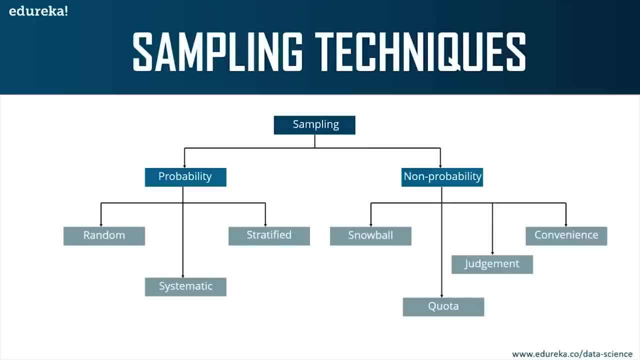 population. Now there are two main types of sampling techniques that I will discuss today. We have probability sampling and non-probability sampling. Now, in this video, we will only be focusing on probability sampling techniques, because non-probability sampling is not within the scope of this video. all right, We'll only discuss the probability part, because we're 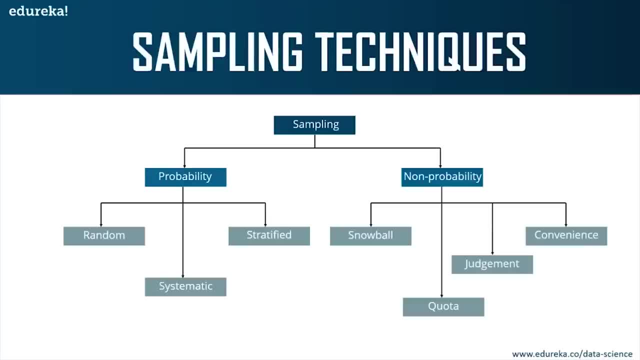 focusing on statistics and probability. correct. Now again, under probability sampling, we have three different types. We have random sampling, systematic and stratified sampling- all right. and just to mention the different types of non-probability samplings, we have snowball, quota judgment and convenient sampling- all right. Now, guys, in this session I'll only be focusing on 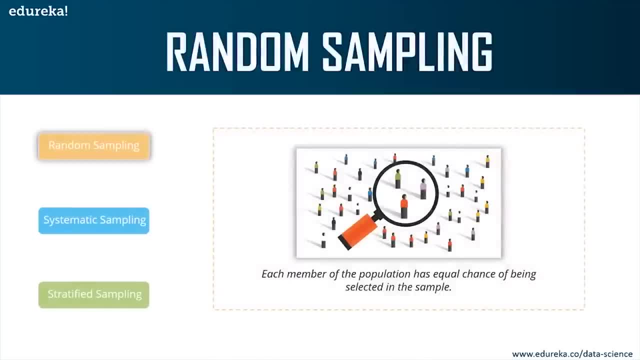 probability. So let's move on and look at the different types of probability sampling. So what is probability sampling? It is a sampling technique in which samples from a large population are chosen by using the theory of probability. all right, So there are three types of probability. 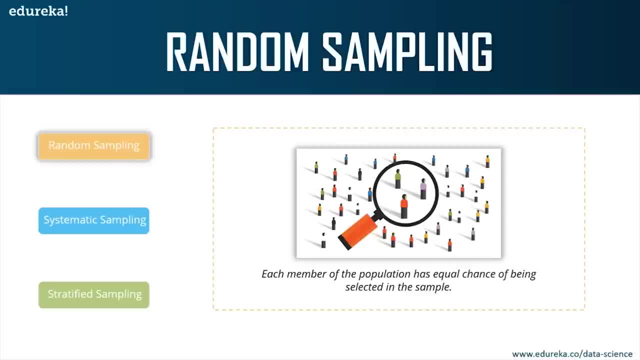 sampling. all right. First we have the random sampling Now. in this method, each member of the population has an equal chance of being selected in the sample, all right. So each and every one of every individual or each and every object in the population has an equal chance of being a part of. 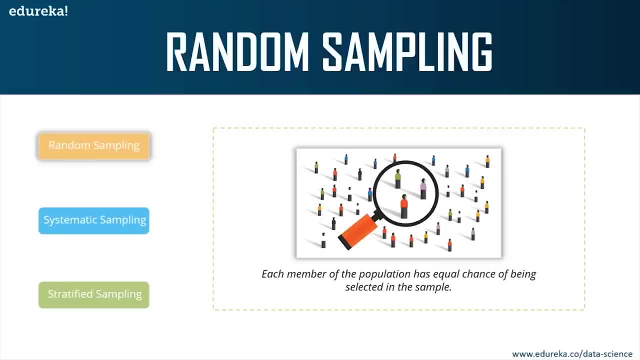 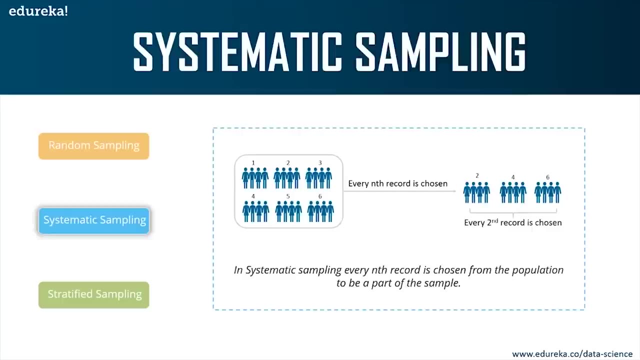 the sample. That's what random sampling is all about. okay, You're randomly going to select any individual or any object, So this way, each individual has an equal chance of being selected correct. Next we have systematic sampling. Now, in systematic sampling, every nth record is chosen. 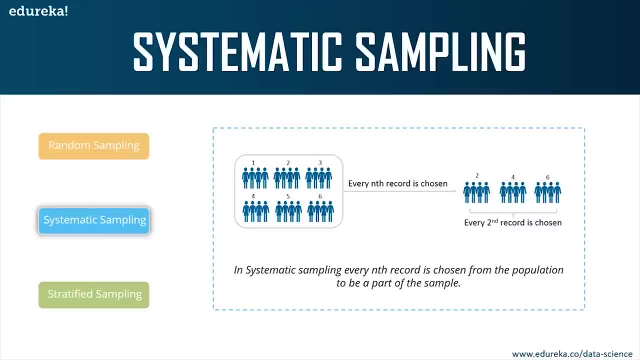 from the population to be a part of the sample. all right, Now refer this image that I've shown over here. Out of these six groups, every second group is chosen as a sample. okay, So every second record is chosen here, and this is how systematic sampling works. 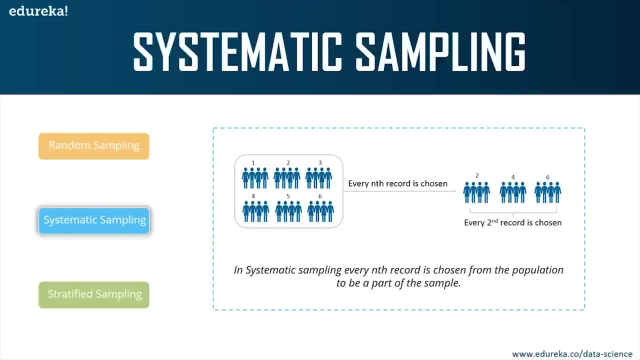 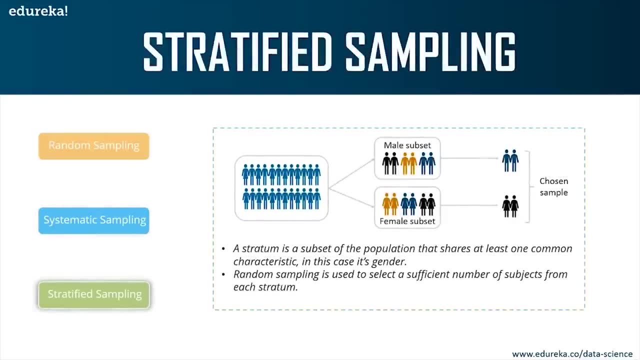 okay, You're randomly selecting the nth record and you're going to add that to your sample. Next we have stratified sampling. Now, in this type of technique, a stratum is used to form samples from a large population. So what is a stratum? 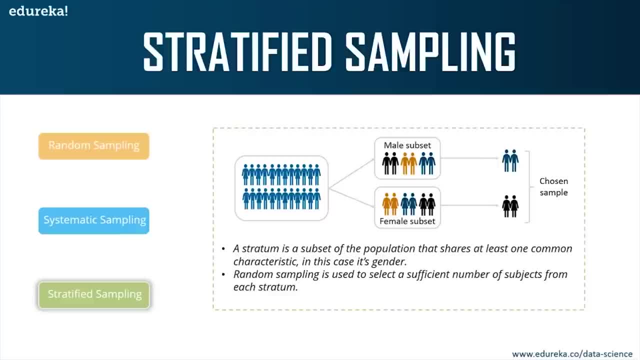 A stratum is basically a subset of the population that shares at least one common characteristics. So let's say that your population has a mix of both male and female. So you can create two stratums out of this. One will have only the male subset and the other will have the female subset. all right, 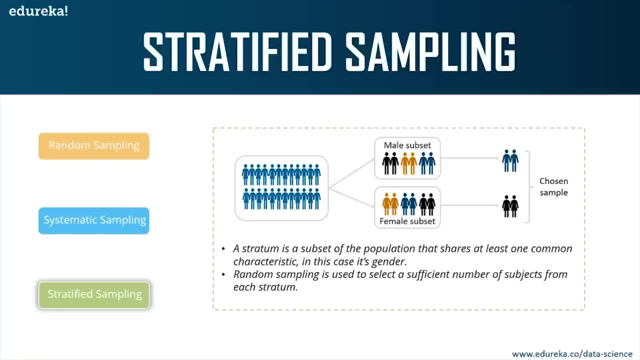 This is what stratum is. It is basically a subset of the population that shares at least one common characteristics. all right, In our example, it is gender. So, after you've created a stratum, you're going to use random sampling on these stratums and you're going to choose a final sample. 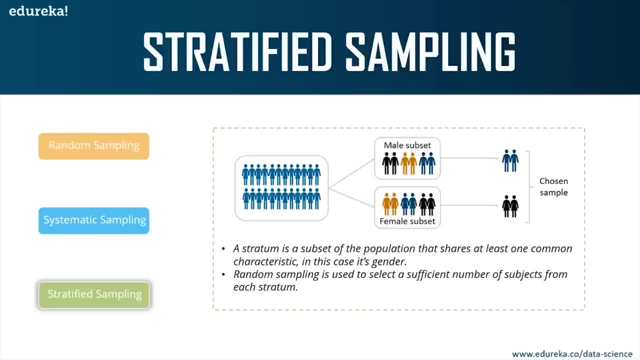 So random sampling, meaning that all of the individuals in each of the stratum will have an equal chance of being selected in the sample, correct? So, guys, these were the three different types of sampling techniques. Now let's move on and look at our next topic, which is the different. 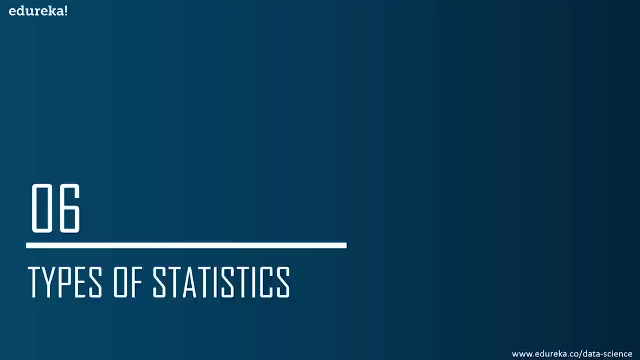 types of statistics. So after this, we'll be looking at the more advanced concepts of statistics. all right, So let's move on and look at our next topic, which is the different types of statistics. So far, we discussed the basics of statistics, which is basically what is statistics. the different 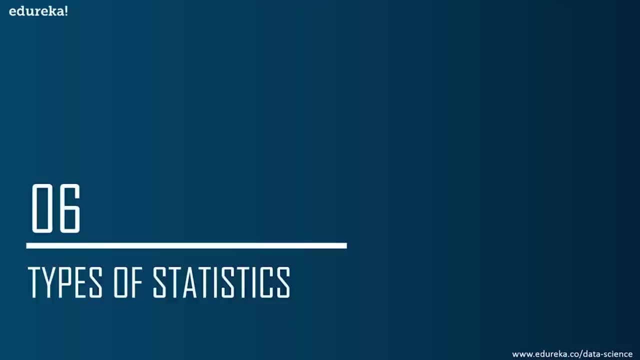 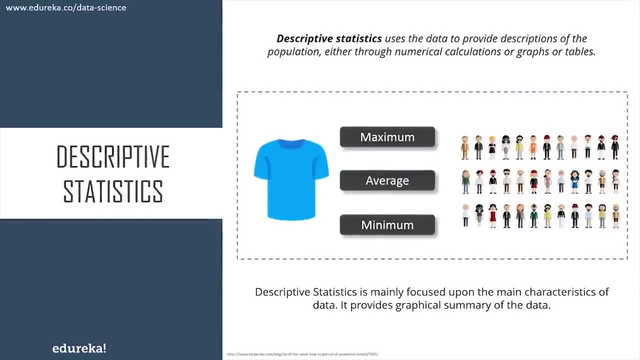 sampling techniques and the terminologies and statistics. all right, Now we look at the different types of statistics. So there are two major types of statistics: descriptive statistics and inferential statistics. In today's session we'll be discussing both of these types of statistics in depth all. 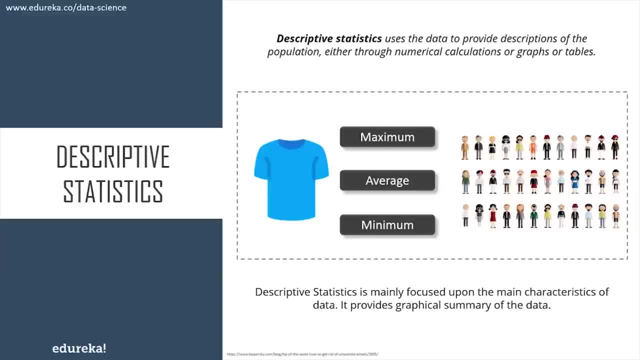 right, We'll also be looking at a demo, which I'll be running in the R language, in order to make you understand what exactly descriptive and inferential statistics is. So, guys, we're just going to look at the basics, so don't worry if you don't have much knowledge. I'm explaining everything from: 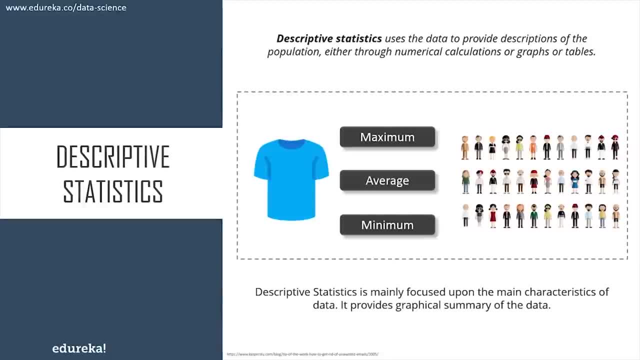 the basic level, all right. So, guys, descriptive statistics is a method which is used to describe and understand the features of specific data set by giving a short summary of the data. okay, So it is mainly focused upon the characteristics of data. It also provides a graphical summary of 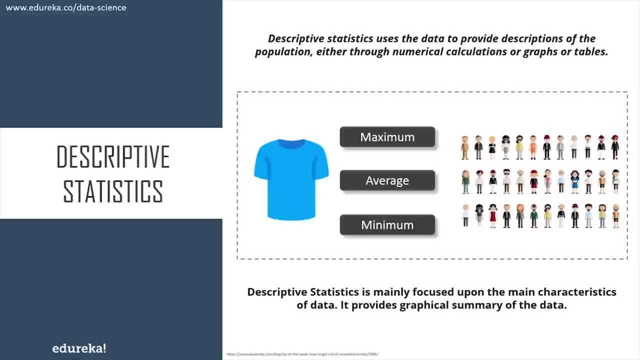 the data. So this is a method which is used to describe and understand the features of specific data. Now, in order to make you understand what descriptive statistics is, let's suppose that you want to gift all your classmates a t-shirt. So to study the average shirt size of a student in a 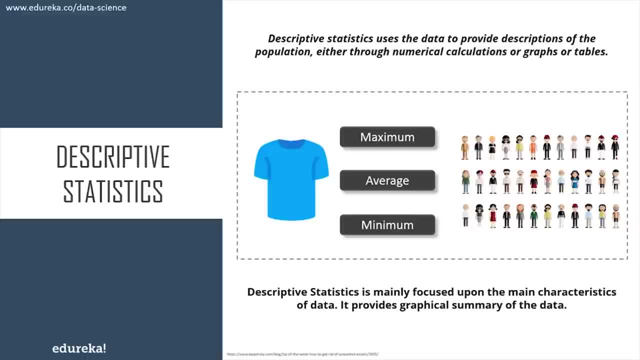 classroom. So if you were to use descriptive statistics to study the average shirt size of students in your classroom, then what you would do is you would record the shirt size of all students in the class and then you would find out the maximum, minimum and average shirt size of the 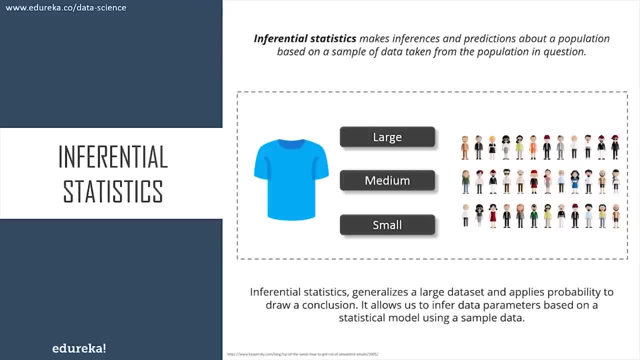 class. Okay. so coming to inferential statistics, inferential statistics makes inferences and predictions about a population based on the sample of data taken from the population. Okay, so in simple words, it generalizes a large data set and it applies probability to draw a conclusion. Okay. 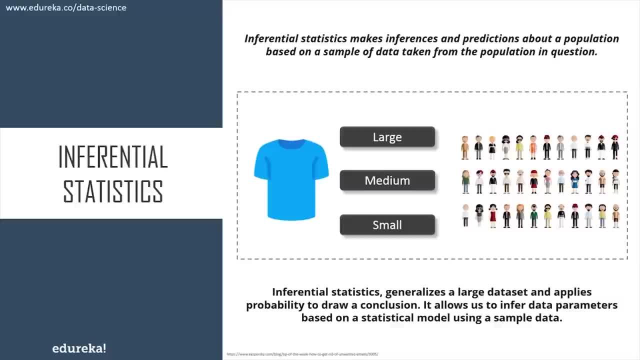 so it allows you to infer data parameters based on a statistical model by using sample data. So if you consider the same example of finding the average shirt size of students in a class, in inferential statistics you will take a sample set of the class, which is basically a few people from the entire class. All right, you already. 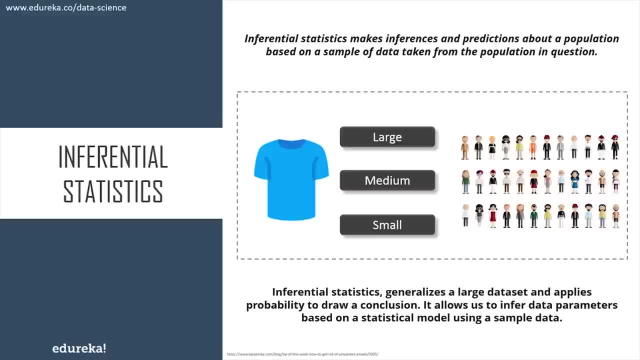 have had grouped the class into large, medium and small. All right, in this method, you basically build a statistical model and expand it for the entire population in the class. So, guys, there was a brief understanding of descriptive and inferential statistics. So that's the difference between. 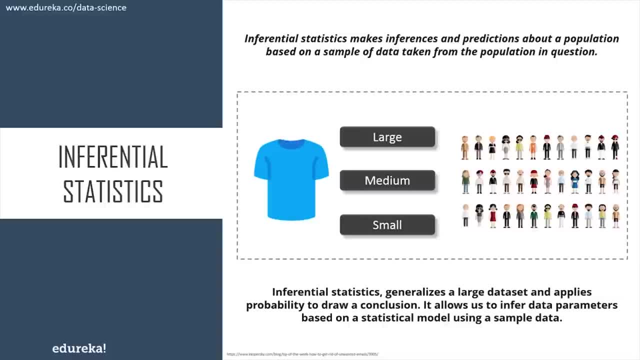 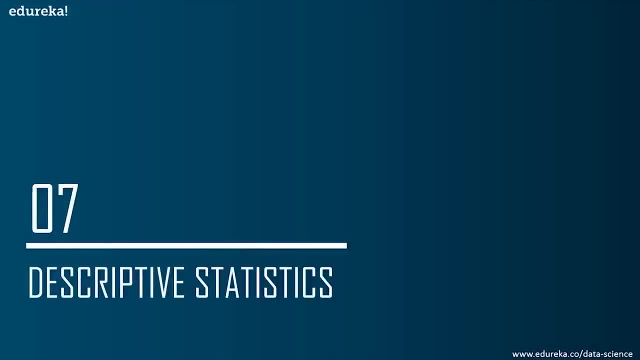 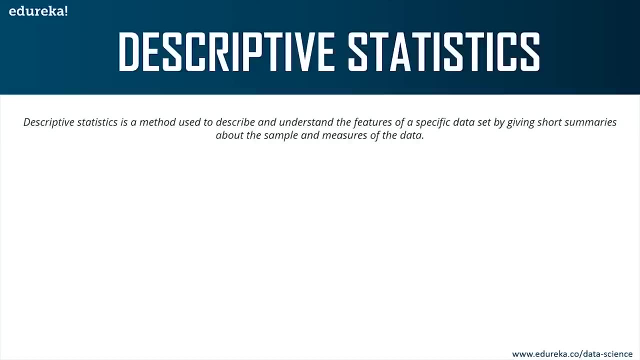 descriptive and inferential statistics. So that's the difference between descriptive and inferential. Now, in the next section, we'll go in depth about descriptive statistics. All right, So let's discuss more about descriptive statistics. So, like I mentioned earlier, descriptive statistics is a method that is used to describe and understand the features of a specific data set. 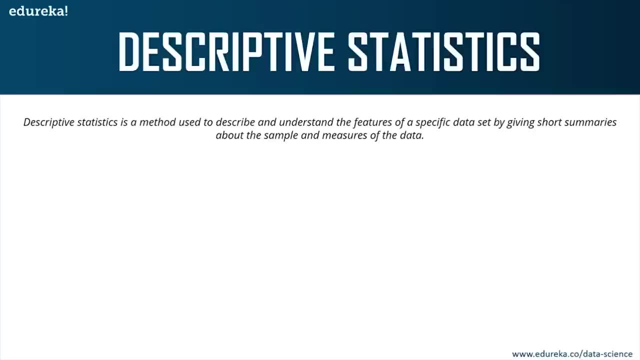 by giving short summaries about the sample and measures of the data. There are two important measures in descriptive statistics. We have measure of central tendency, which is also known as measure of center, and we have measures of variability, This is also known as measures of spread. So measures of center include mean, median and mode. Now, what is measures of? 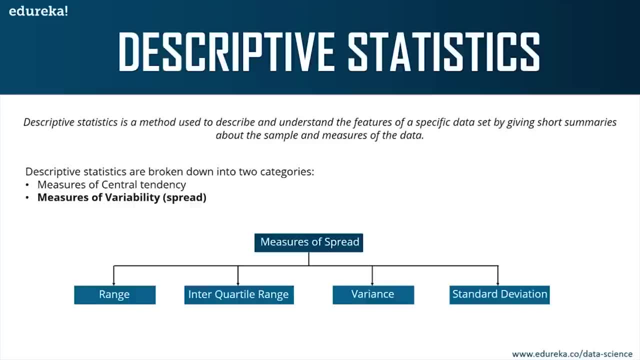 center. Measures of the center are statistical measures that represent the summary of a data set. Okay, the three main measures of center are mean, median and mode. Coming to measures of variability or measures of spread, we have range- interquartile range. We have range- interquartile range. 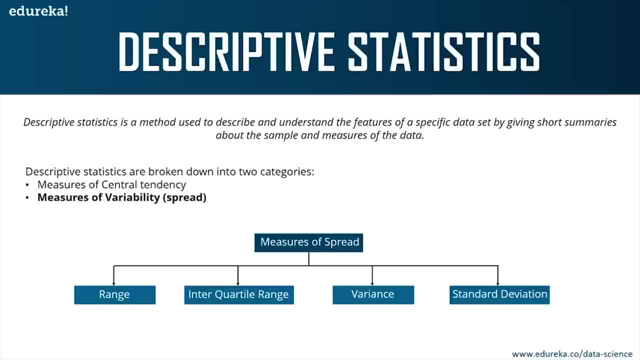 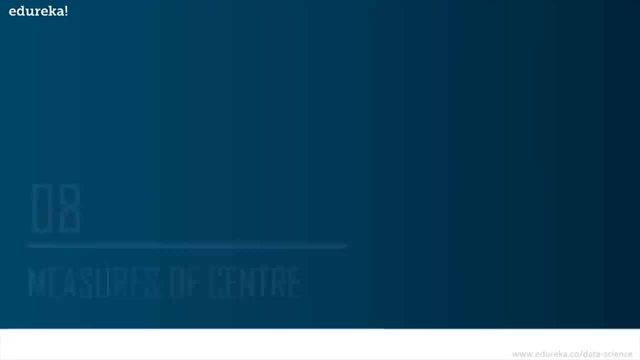 variance and standard deviation. All right, So now let's discuss each of these measures in a little more depth, starting with the measures of center. Now, I'm sure all of you know what the mean is. Mean is basically the measure of the average of all the values in a sample. 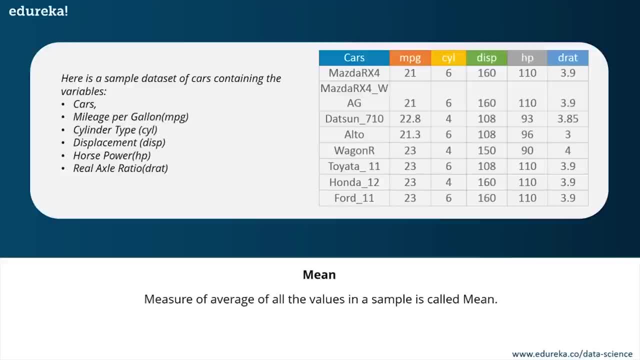 Okay, so it's basically the average of all the values in a sample. How do you measure the mean? I hope all of you know how the mean is measured. If there are 10 numbers and you want to find the mean of these 10 numbers, you can use the mean to measure the average of all the values in a sample. 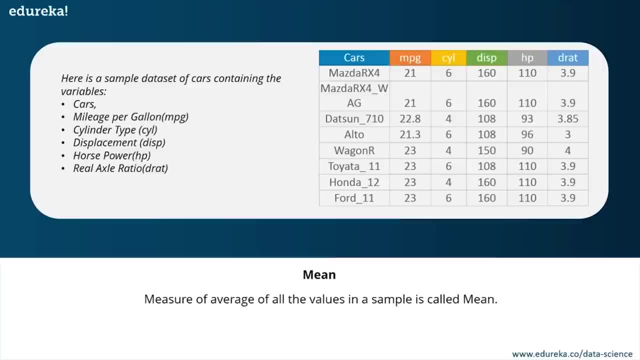 All you have to do is you have to add up all the 10 numbers and you have to divide it by 10.. 10 here represents the number of samples in your data set. All right, since we have 10 numbers, we're going to divide this by 10.. All right, this will give us the average or the mean. So to better. 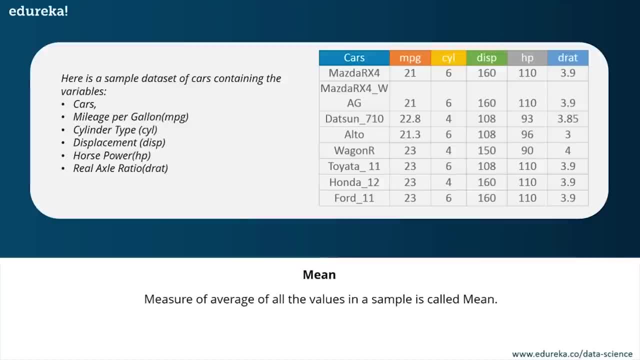 understand the measures of central tendency. let's look at an example Now. the data set over here is basically the cars data set, and it contains a few variables. All right, it has something known as cars. it has mileage per gallon, cylinder type, displacement, horsepower and real axle ratio. 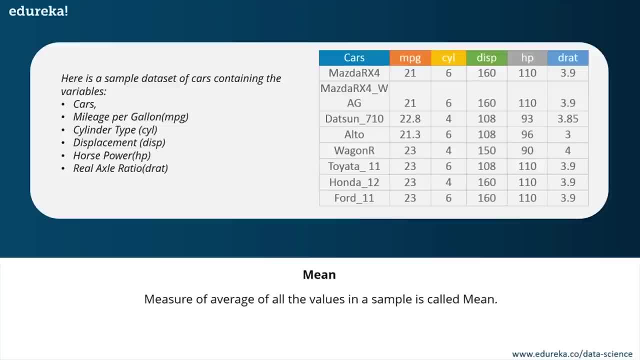 All right, all of these measures are related to cars. Okay, so what you're going to do is you're going to use descriptive analysis and you're going to analyze each of the variables in the sample data set for the mean, standard, deviation, median, more and so on. So let's say that you want. 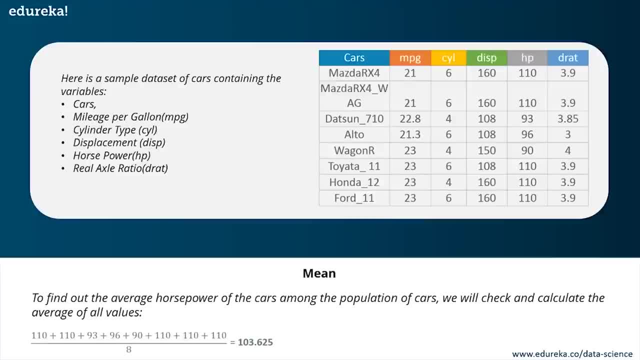 to find out the mean or the average horsepower of the cars among the population of cars. Like I mentioned earlier, what you'll do is you'll check the average of all the values. So in this case, we'll take the sum of the horsepower of each car and we'll divide that by 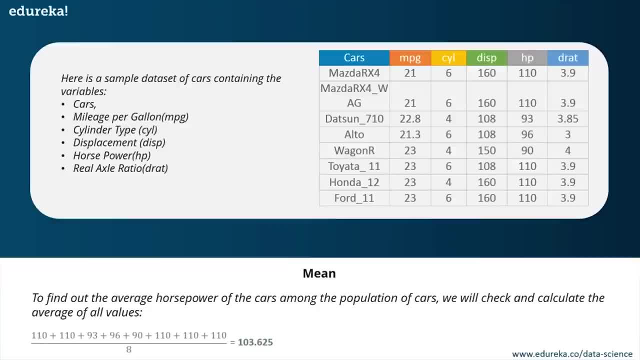 the total number of cars. Okay, that's exactly what I've done here in the calculation part. So this 110 basically represents the horsepower for the first car. All right, similarly, I've just added up all the values of horsepower for each of the cars and I've divided it by 8.. Now, 8 is. 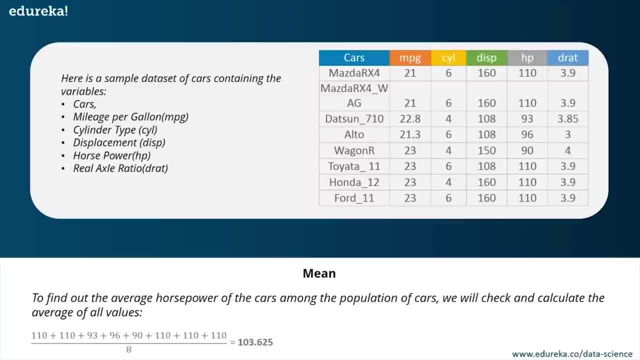 number of cars in our data set. All right, so 103.625 is what our mean is, or the average of horsepower is All right. now let's understand what median is with an example. Okay, so to define median. median is basically a measure of the central value of the sample set. is called the median. All right, you can. 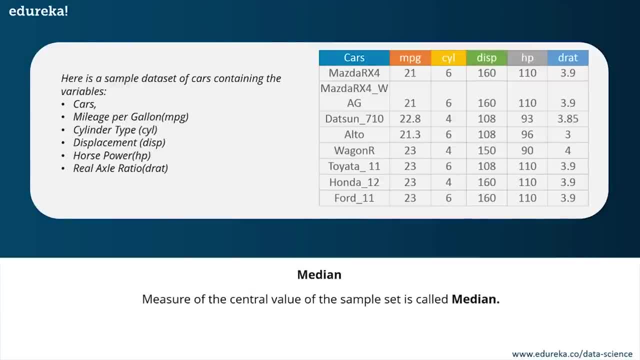 say that it is a middle value. So if you want to find out the center value of the mileage per gallon of cars first, what we'll do is we'll arrange the mpg values in ascending or descending order and choose a middle value. All right in this case, since we have eight values. right, we have. 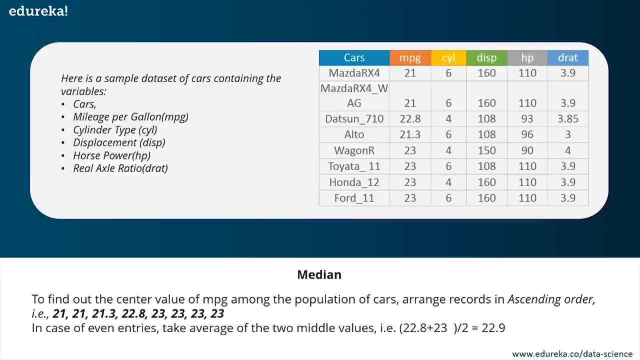 eight values, which is an even entry. So whenever you have even number of data points or samples in your data set, then you're going to take the average of the two middle values. If we had nine values over here, we can easily figure out the middle value and you know, choose that as a. 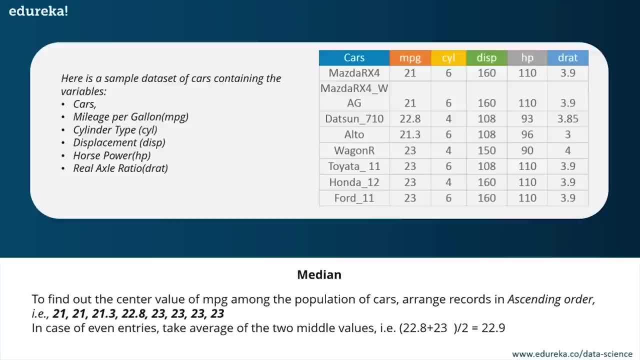 median. But since there are even number of values, we're going to take the average of the two middle values, All right. so 22.8 and 23 are my two middle values and I'm taking the mean of those two and hence I get 22.9, which is my median, All right, lastly, let's look at how mode is calculated. 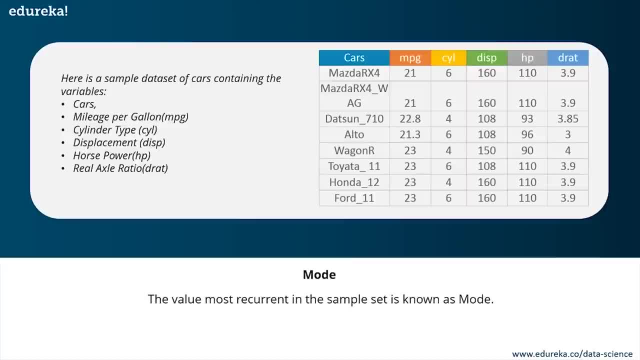 So what is mode? Now, the value that is most recurrent in the sample set is known as mode, or basically the value that occurs most often. Okay, that is known as mode. So let's say that we want to find out the most common type of cylinder among the population. 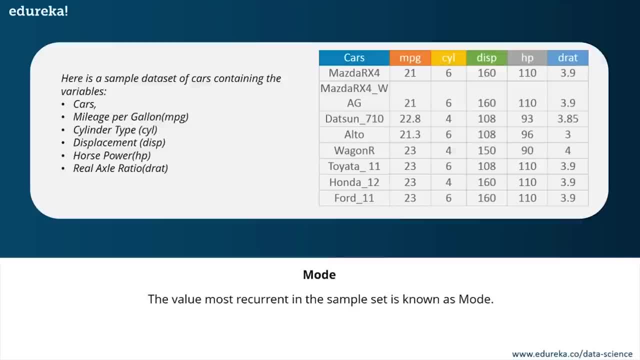 of cars. All we have to do is we will check the value which is repeated the most number of times. Here we can see that the cylinders come in two types. We have cylinder of type four and cylinder of type six, right? So take a look at the data set. you can see that the most recurring value is six. 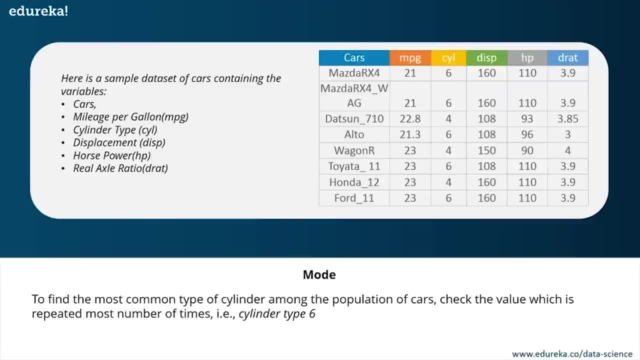 right, We have one, two, three, four and five, We have five, six and we have one, two, three. Yeah, we have three, four type cylinders and five, six type cylinders. So basically, we have three, four type cylinders and we have five, six type cylinders. All right, so our mode is going. 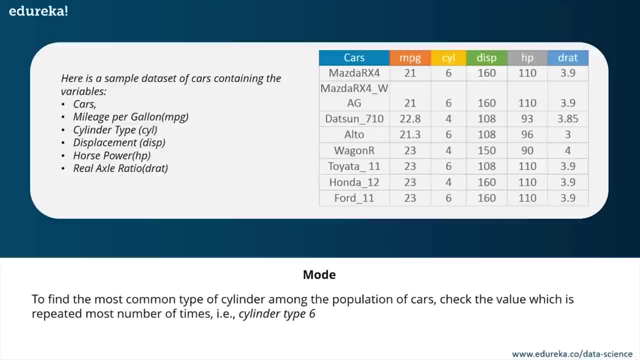 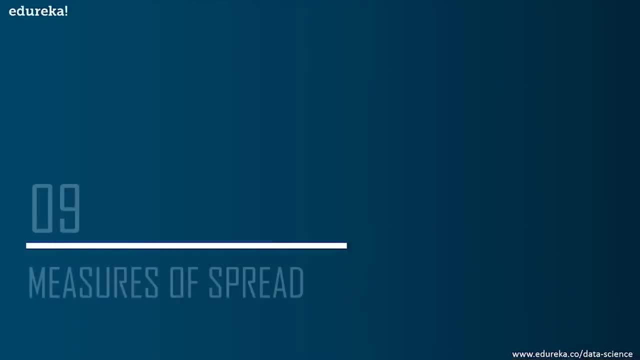 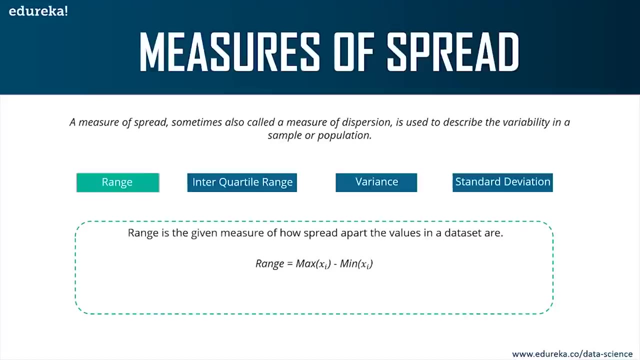 to be six, since six is more recurrent than four. So, guys, those were the measures of the center, or the measures of central tendency. Now let's move on and look at the measures of the spread. All right now, what is the measure of spread? A measure of spread, sometimes also called as measure of 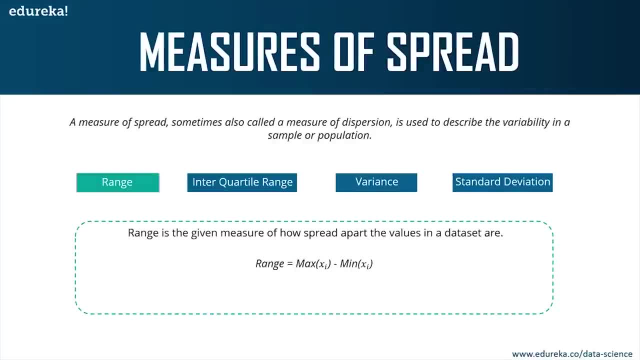 dispersion is used to describe the variability in a sample or population. Okay, you can think of it as some sort of deviation in the sample. All right, so you measure this with the help of the different measure of spreads. We have range, interquartile range, variance and standard deviation. 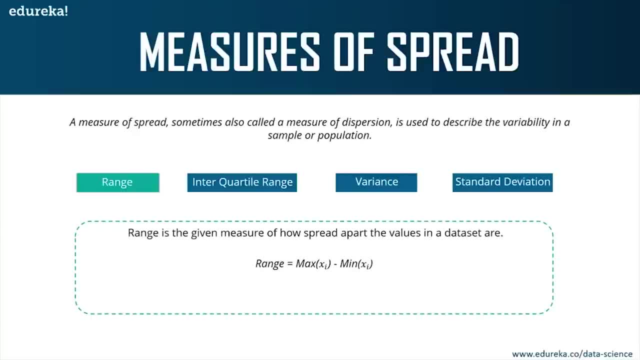 Now, range is pretty self-explanatory, right. It is the given measure of how, spread apart, the values in a data set are. The range can be calculated as shown in this formula. So you're basically going to subtract the maximum value in your data set. 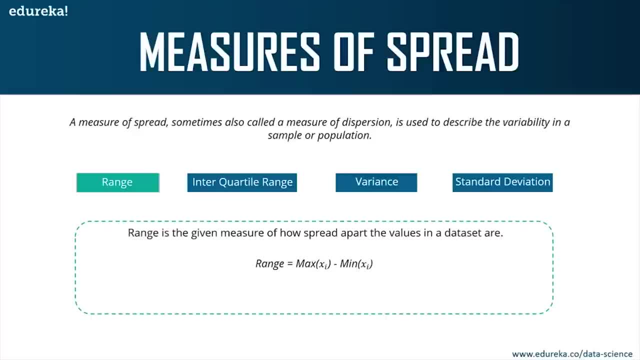 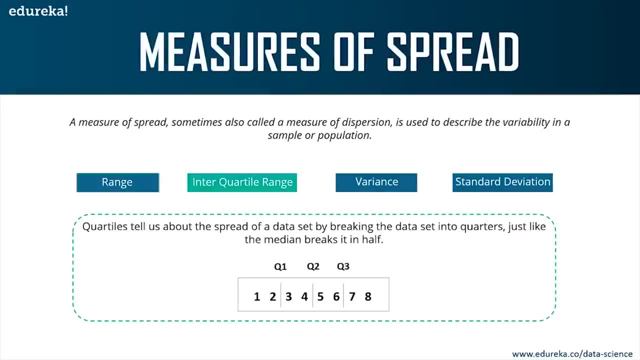 from the minimum value in your data set. That's how you calculate the range of the data. All right. next we have interquartile range. So before we discuss interquartile range, let's understand what a quartile is. All right, so quartiles basically tell us about the spread of a data set. 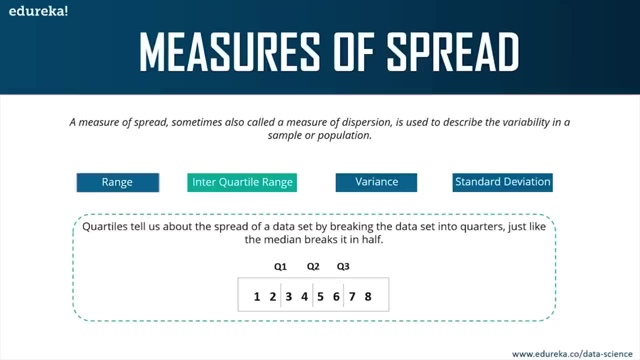 So what is a quartile? A quartile is a set of data sets that are divided into different quartiles. Okay, just like how the median breaks the data into two parts, the quartile will break it into different quartiles. So to better understand how quartile and interquartile are calculated, let's 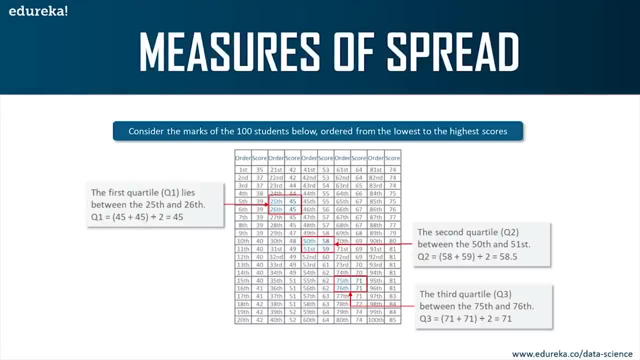 look at a small example Now. this data set basically represents the marks of 100 students, ordered from the lowest to the highest scores. All right, so the quartiles lie in the following ranges: The first quartile is also known as q1.. It lies between the 25th and the 26th observation. 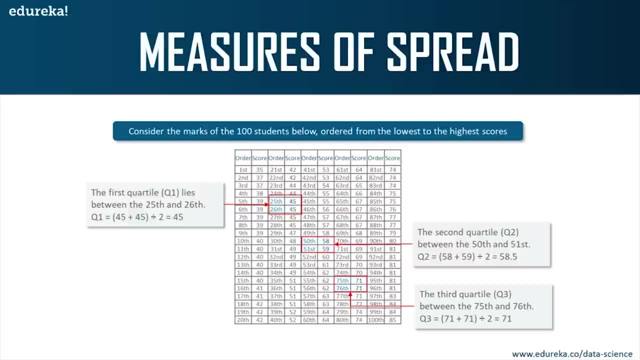 All right. so if you look at this, I've highlighted the 25th and the 26th observation. So how you can calculate q1, or first quartile, is by taking the average of these two values. All right, since both the values are 45, when you add them up and divide them by 2, you'll still get 45.. Now the second. 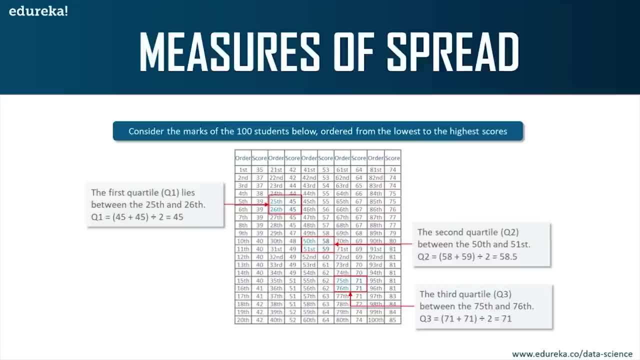 quartile, or q2, is between the 50th and the 51st observation. So you're going to take average of 58 and 59 and you'll get a value of 58.5.. Now, this is my second quarter. The third quartile, or q3, is between the 75th and the 76th observation. 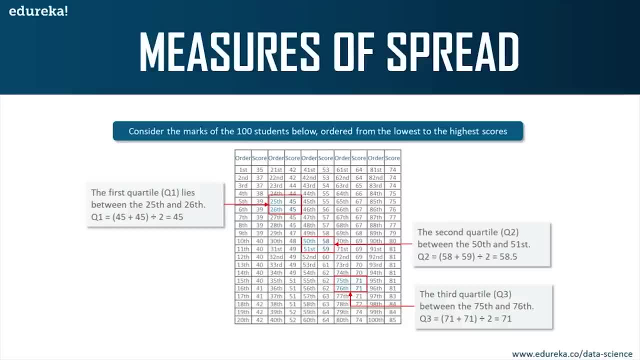 Here again, you'll take the average of the two values, which is the 75th value and the 76th value, All right, and you'll get a value of 71.. All right, so, guys, this is exactly how you calculate the different quartiles. Now let's look at what is interquartile range. 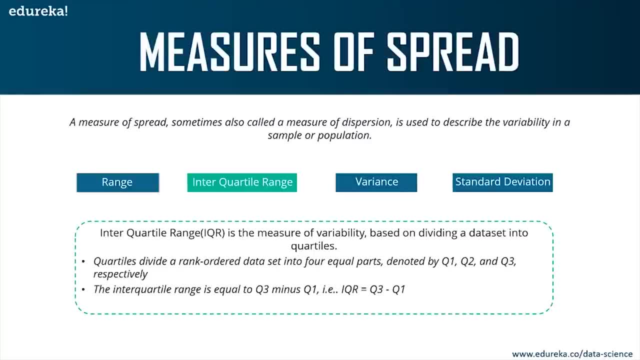 So iqr is the value of the number of students ordered from the lowest to the highest scores. The third quartile, or the interquartile range, is a measure of variability based on dividing a data set into quartiles. Now the interquartile range is calculated by subtracting the q1 from q3. So 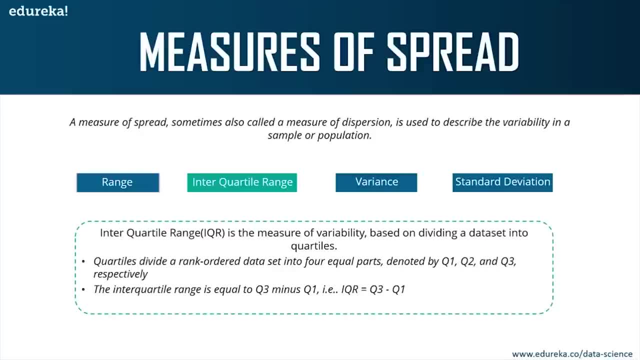 basically, q3 minus q1 is your iqr. So your iqr is your q3 minus q1.. All right now. this is how each of the quartiles are. each quartile represents a quarter, which is 25.. All right, so, guys, i hope all. 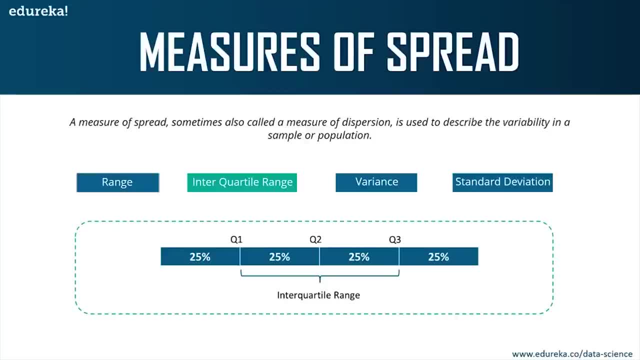 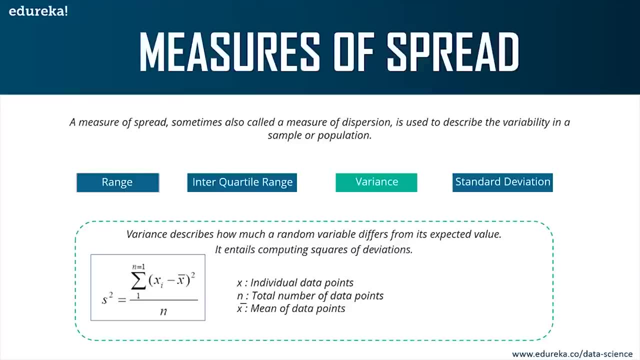 of you are clear with interquartile. All right, let's move on to the next quartile. Now. this is range, and what are quartiles? now let's look at variance. now. variance is basically a measure that shows how much a random variable differs from. 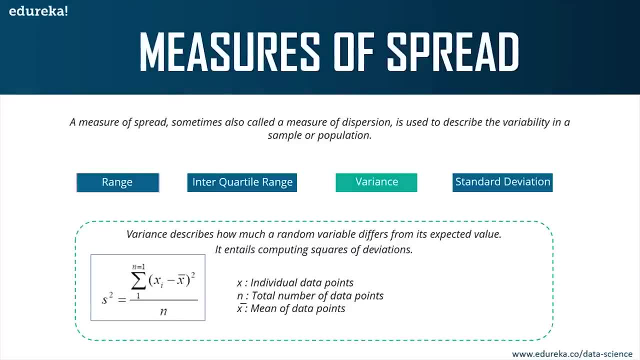 its expected value. okay, it's basically the variance in any variable. now variance can be calculated by using this formula right here: x basically represents any data point in your data set, n is the total number of data points in your data set and x bar is basically the mean of data. 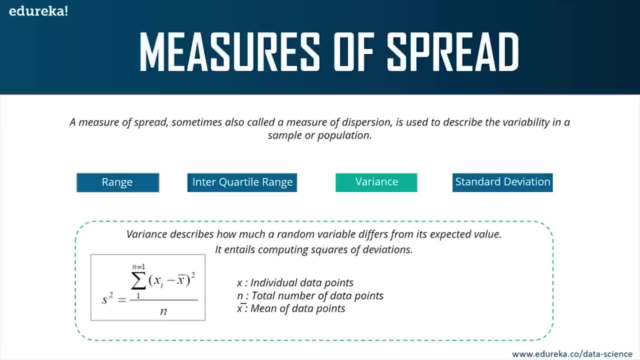 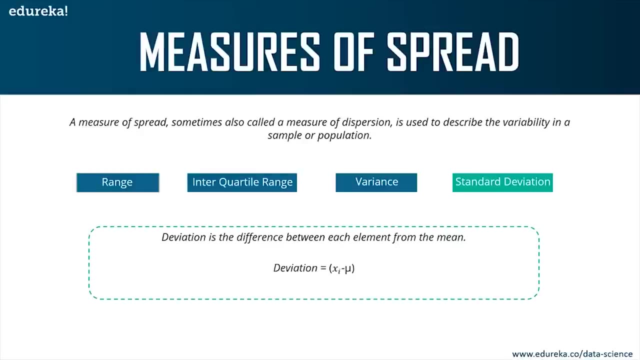 points. all right, this is how you calculate variance. variance is basically, uh, computing the squares of deviations. okay, that's why it says s squared there. now let's look at what is deviation. deviation is just the difference between each element from the mean. okay, so it can be calculated by using. 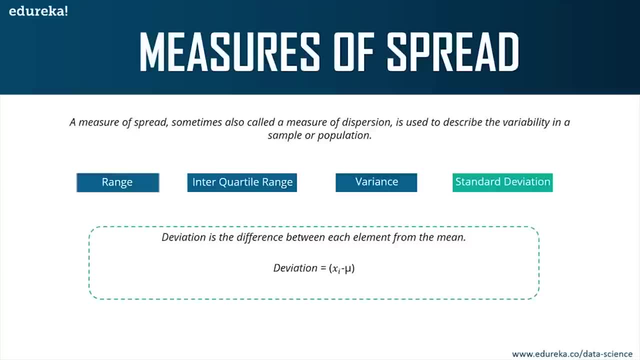 this simple formula, where xi basically represents a data point and mu is the mean of the population. all right, this is exactly how you calculate deviation. now, population variance and sample variance are very specific to whether you're calculating the variance in your population data set or in your sample data set. that's the only difference between. 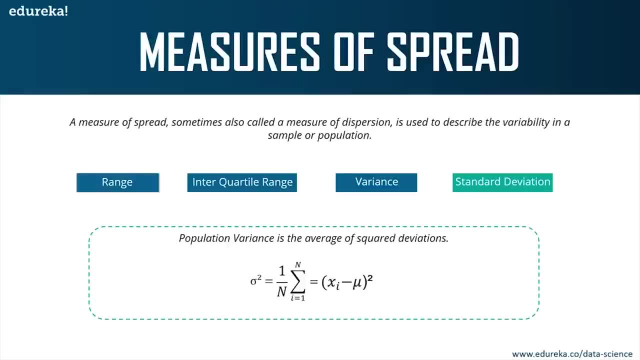 population and sample variance. so the formula for population variance is pretty explanatory. so xi is basically each data point, mu is the mean of the population, n is the number of samples in your data set. all right, now let's look at sample variance. now, sample variance is the average of square. 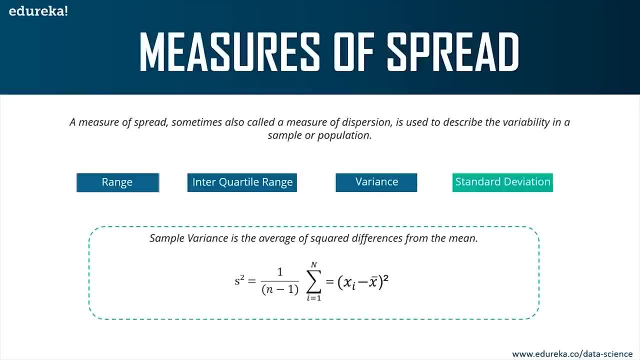 variances from the mean. all right, your xi is any data point or any sample in your data set. x bar is the mean of your sample. all right, it's not the mean of your population, it's the mean of your sample. and if you notice n, here is 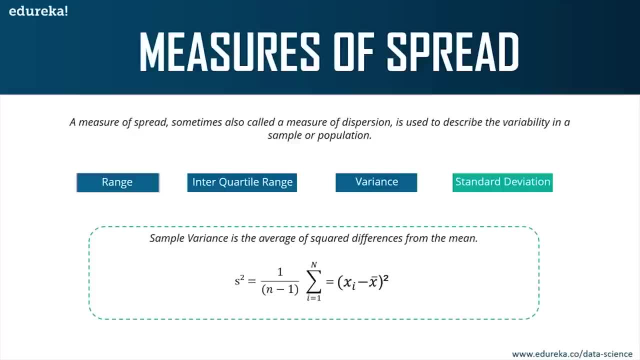 a smaller n. it's the number of data points in your sample and this is basically the difference between sample and population variance. i hope that is clear. coming to standard, deviation is the measure of dispersion of a set of data from its mean. all right, so it's basically the deviation from your mean. 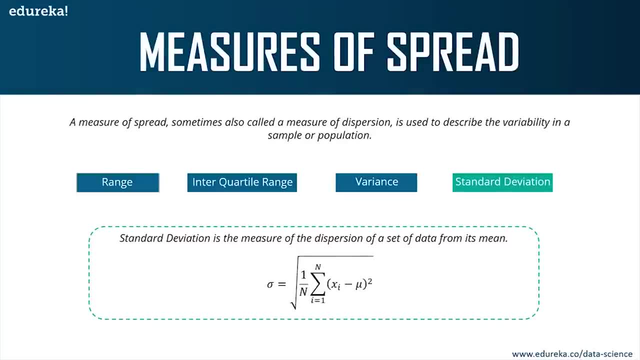 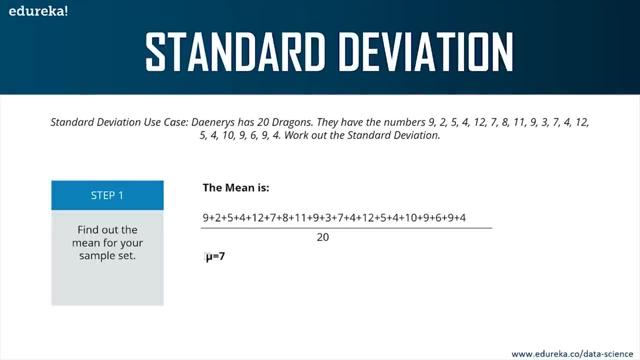 that's what standard deviation is. now, to better understand how the measures of spread are calculated, let's look at a small use case. so let's say daenerys has 20 dragons. they have the numbers 9, 2, 5, 4 and so on, as shown on the screen. what you have to do is you have to work out. 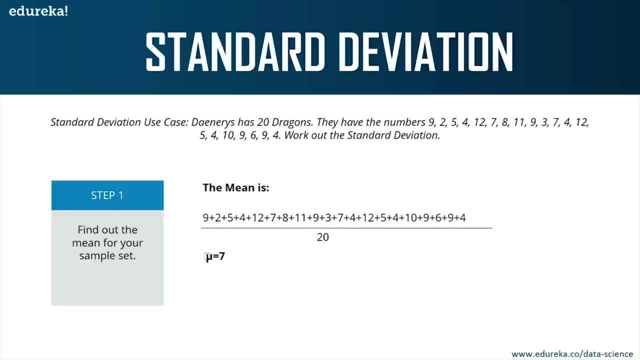 the standard deviation. all right, in order to calculate the standard deviation you need to know the mean, right? so first you're going to find the mean of your sample set. so how do you calculate the mean? you add all the numbers in your data set and divide it by the total number of samples in your data set. so you get a. 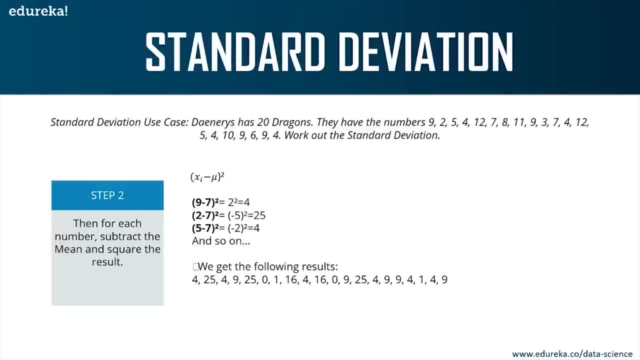 value of 7 here. then you calculate the rhs of your standard deviation formula, all right. so from each data point you're going to subtract the mean and you're going to square that, all right. so when you do that, you'll get the following result: you'll basically get this: 425, 4, 9, 25 and so on. so finally you'll. 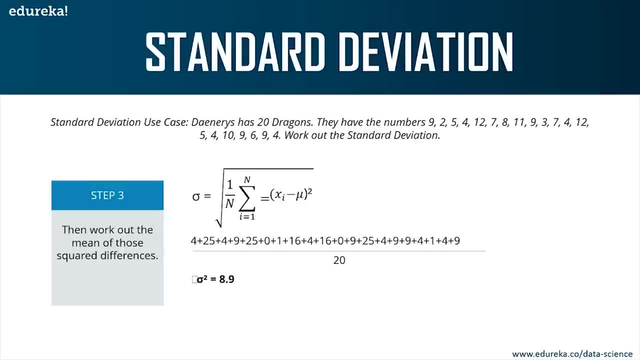 just find the mean of these squared differences. all right. so your standard deviation will come up to 2.983 once you take the square root. so, guys, this is pretty simple. it's a simple mathematic technique. all you have to do is you have to substitute the 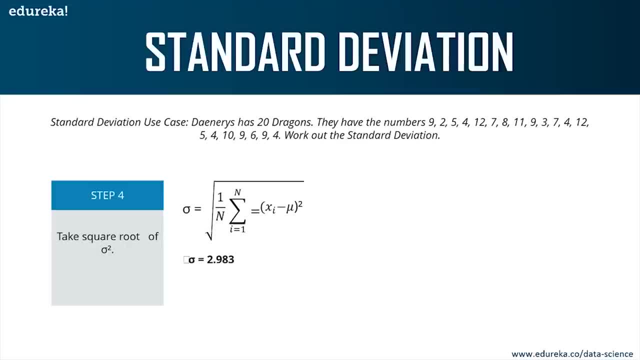 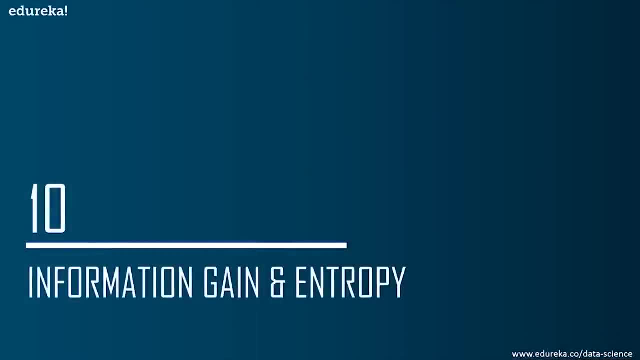 values in the formula. all right, i hope this was clear to all of you. now let's move on and discuss the next topic, which is information gain and entropy. now, this is one of my favorite topics in statistics. it's very interesting, and this topic is mainly involved in machine learning algorithms like 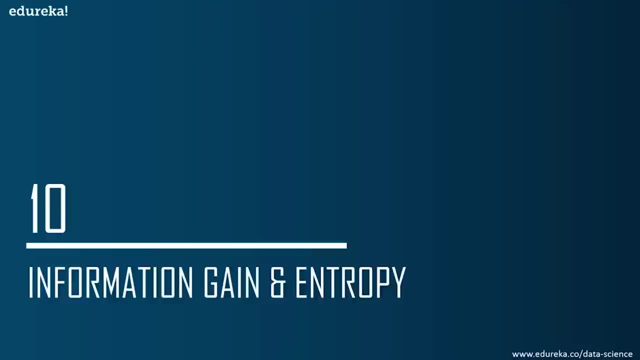 decision trees and random forest. all right, it's very important for you to know how information gain and entropy really work and why they're so essential in building machine learning models. we'll focus on the statistic parts of information gain and entropy and after that we'll discuss a use case and see how. 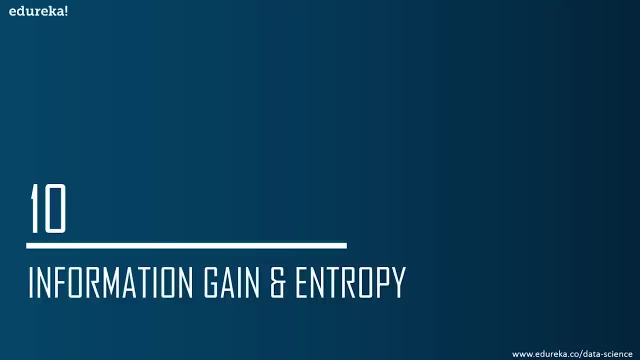 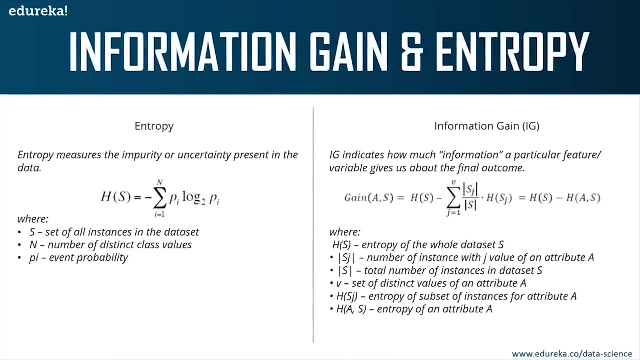 information gain and entropy is used in decision trees. so for those of you who don't know what a decision tree is, it is basically a machine learning algorithm. you don't have to know anything about this. i'll explain everything in depth, so don't worry. now let's look at what exactly entropy and information gain is. 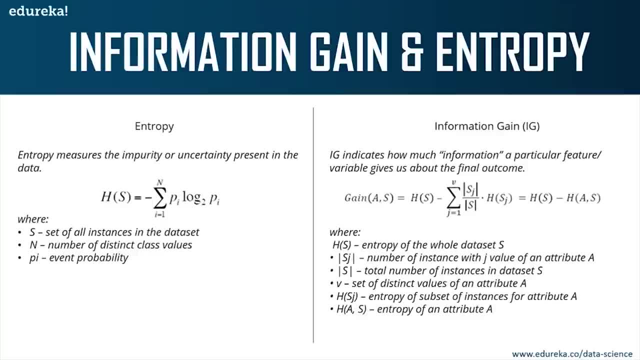 now guys. entropy is basically the measure of any sort of uncertainty that is present in the data. all right, so it can be measured by using this formula. so here s is the set of all instances in the data set, or all the data items in the data set. n. 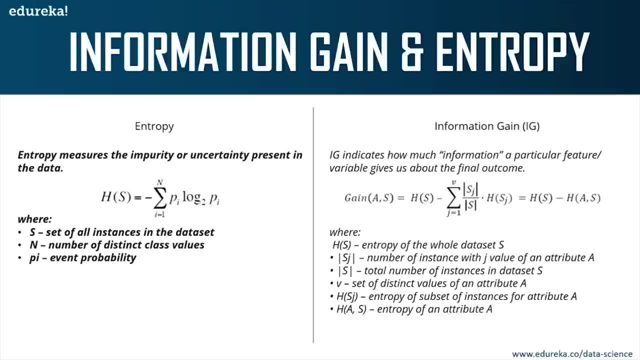 is the different type of classes in your data set. p i is the event probability. now, this might seem a little confusing to y'all, but when we go through the use case you'll understand all of these terms even better. all right, coming to information gain. as the word suggests, information gain. 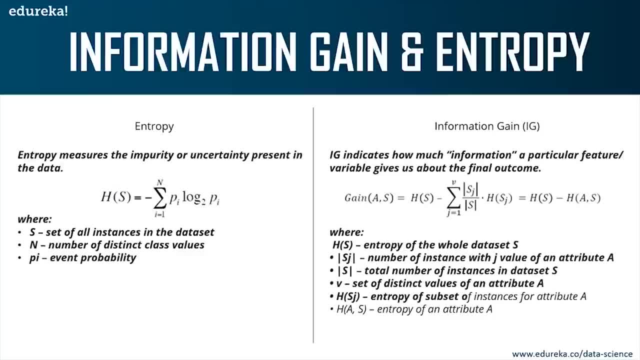 indicates how much information a particular feature or a particular variable gives us about the final outcome. okay, it can be measured by using this formula. so again here, h of s is the entropy of the whole data set s s. j is the number of instances in the data set, s is the total number of instances, with the j value of an. 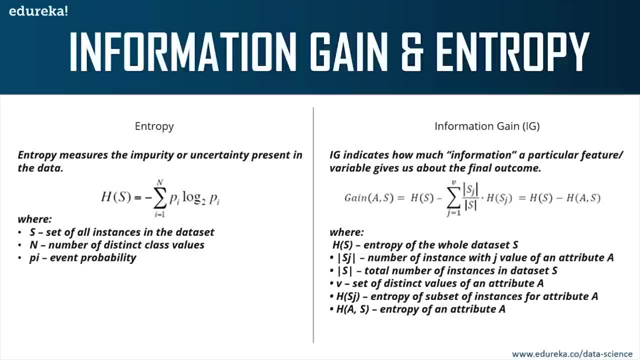 attribute a. s is the total number of instances in the data set, v is the set of distinct values of an attribute a, h of s, j is the entropy of subset of instances and h of a comma. s is the entropy of an attribute a. even though this seems confusing, i'll 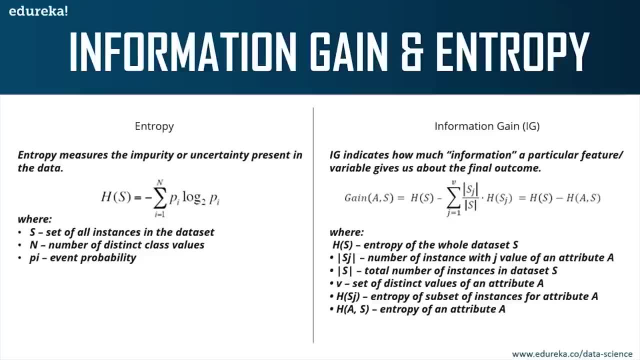 clear out the confusion. all right, let's discuss a small problem statement where we'll understand how information gain and entropy is used to measure the significance of a model. so, like i said, information gain and entropy are very important statistical measures that let us understand the significance of a predictive model. 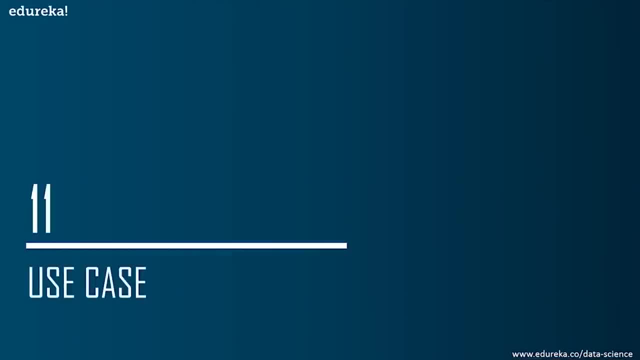 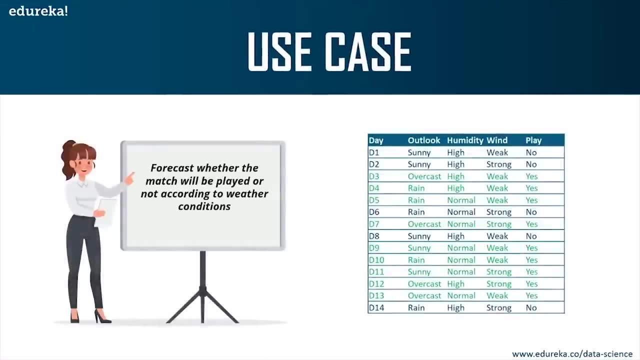 okay, to get a more clear understanding, let's look at a use case. all right, now suppose we're given a problem statement. all right, the statement is that you have to predict whether a match can be played or not by studying the weather conditions. so the predictor variables here are: 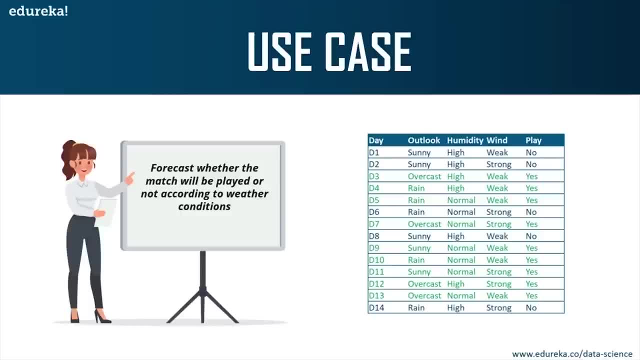 day is also a predictor variable. the target variable is basically play alright. the target variable is the variable that you're trying to predict. okay, now, the value of the target variable will decide whether or not a game can be played alright. so that's why the play has two values. it has no. and yes, no meaning that. 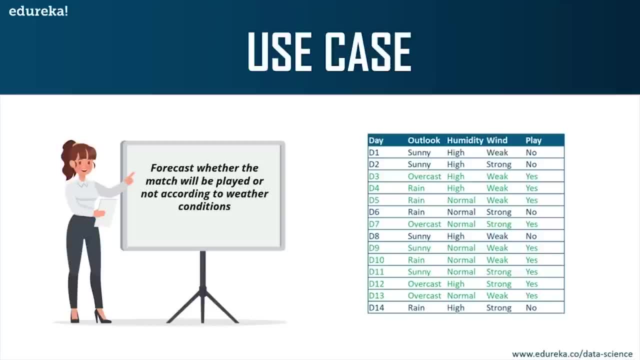 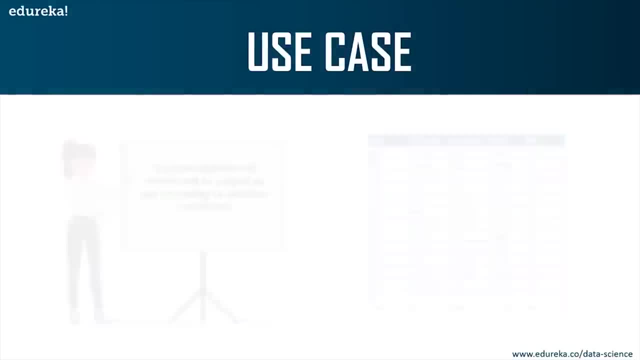 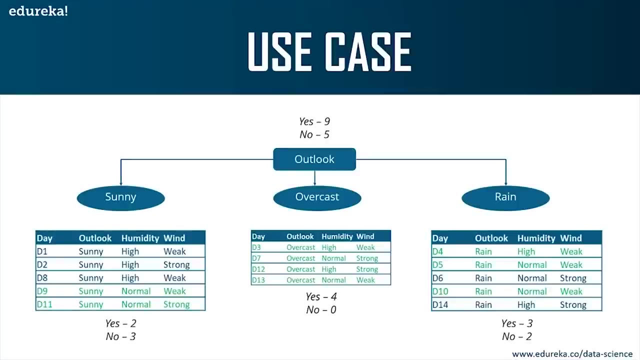 the weather conditions are not good and therefore you cannot play the game. yes, meaning that the weather conditions are good and suitable for you to play the game. alright, so that was a problem statement. I hope the problem statement is clear to all of you now. to solve such a problem, we make use of something known. 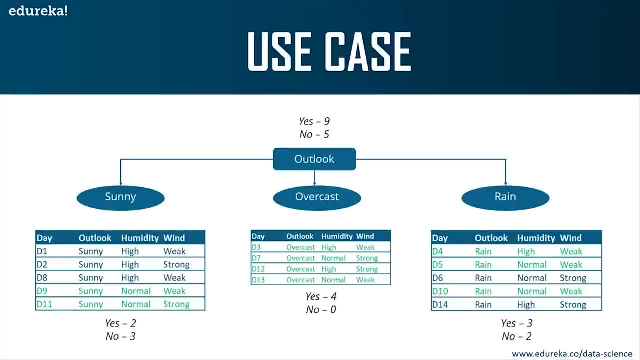 as decision trees. so guys think of an inverted tree and each branch of the tree denotes some decision. alright, each branch is known as the branch node, and at each branch node you're going to take a decision in such a manner that you'll get an outcome at the end of the branch. alright. now this figure here, basically: 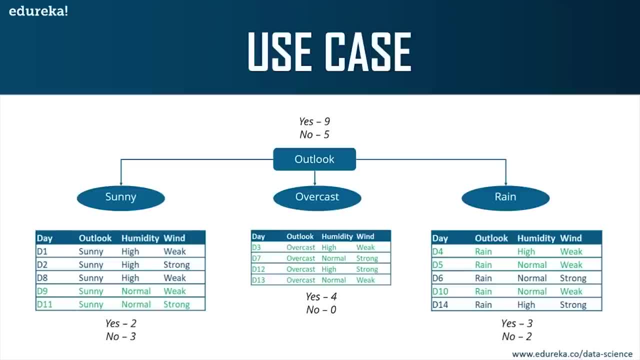 shows you that out of 14 observations, nine observations result in a yes, meaning that out of 14 days, the match can be played only on nine days. alright, so here, if you see, on day one, day two, day eight, day nine and day eleven, the outlook has. 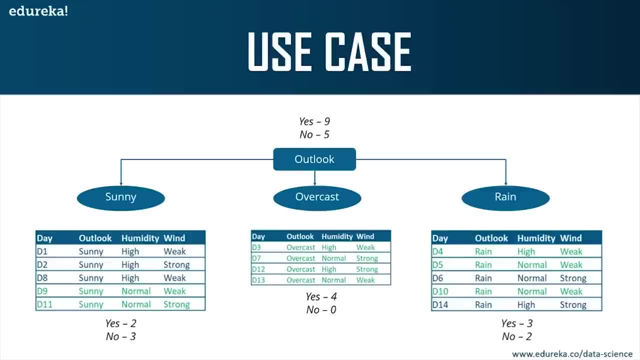 been sunny, alright. so basically, we're trying to cluster our data set depending on the outlook. so when the outlook is sunny, this is our data set. when the outlook is overcast, this is what we have, and when the outlook is rain, this is what we have. alright. so when it is sunny, we have two. 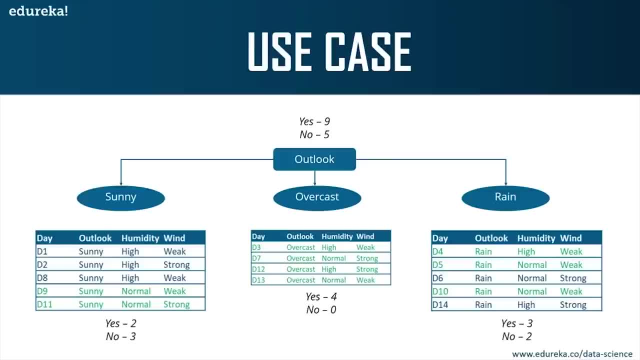 yeses and three no's. okay. when the outlook is overcast, we have all four as yeses, meaning that on the four days when the outlook was overcast, we can play the game alright. now, when it comes to rain, we have three yeses and two no's- alright. 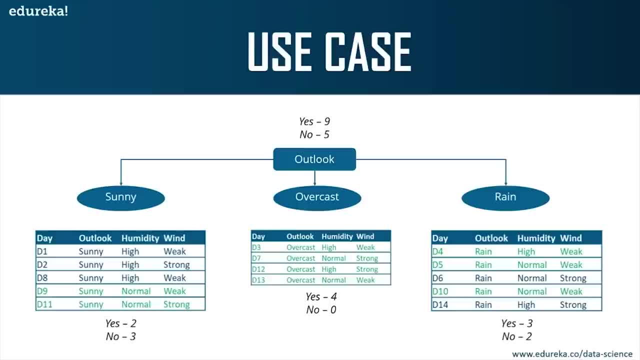 so, if you notice, here the decision is being made by choosing the outlook variable as the root node. okay, so the root node is basically the topmost node in a decision tree. now, what we've done here is we've created a decision tree that starts with the outlook node. alright, then you're splitting the. 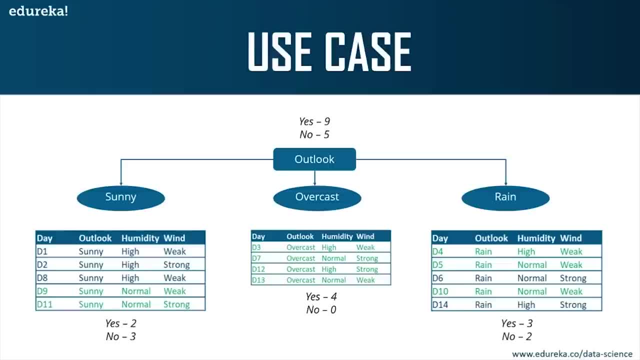 decision tree further depending on other parameters like sunny, overcast and rain. alright, now, like we know, that outlook has three values- sunny, overcast and rain- so let me explain this in a more in-depth manner. okay, so what you're doing here is you're making the decision tree by choosing the outlook variable at the root node, the 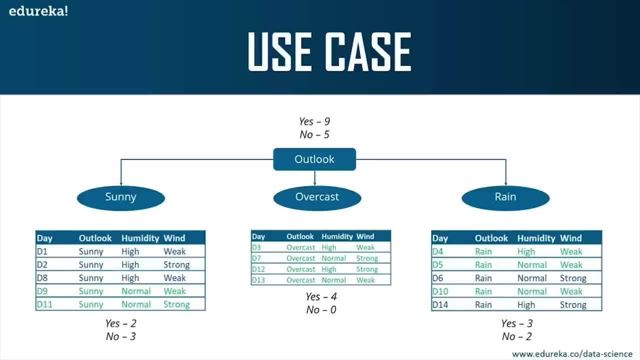 root node is basically the topmost node in a decision tree. now the outlook node has three branches coming out from it, which is sunny, overcast and rain. so basically, outlook can have three values: either it can be sunny, it can be overcast, or it can be rainy. okay, now these three values are assigned to the 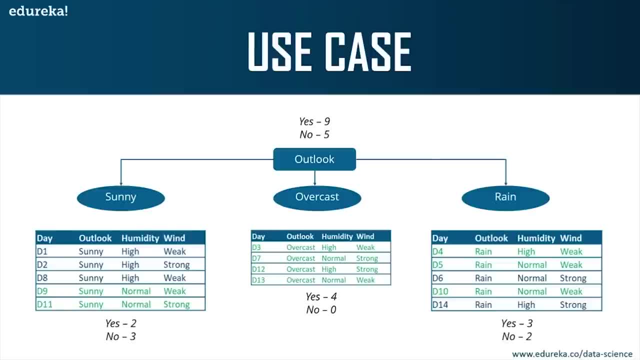 immediate branch nodes, and for each of these values the possibility of play is equal to yes is calculated. so the sunny and the rain branches will give you an impure output, meaning that there is a mix of yes and no. right, there are two yeses here, three no's here there. 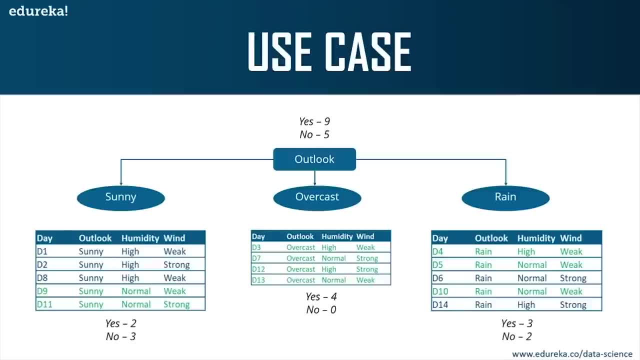 are three yeses here and two no's over here, but when it comes to the overcast variable, it results in a hundred percent pure subset. alright, this shows that the overcast variable will result in a definite and certain output. this is exactly what entropy is used to measure. alright it. 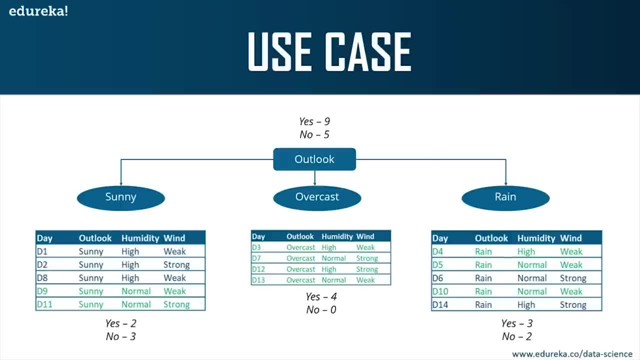 generalizes the impurity or the uncertainty. alright, so the lesser the uncertainty or the entropy of a variable, more significant is that variable. so, when it comes to overcast, there's literally no impurity in the data set. it is a hundred percent pure, subset, right. so we want variables like these in order to build a model. all right, we. 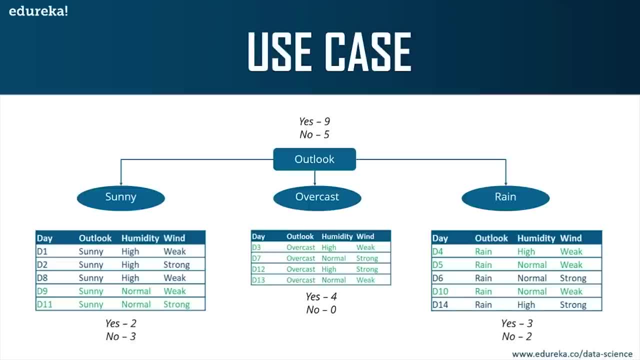 don't always get lucky and we don't always find variables that will result in pure subsets. that's why we have the major entropy, so the lesser the entropy of a particular variable, the most significant that variable will be. so in a decision tree, the root node is assigned the best attribute, so that the decision tree can predict the most precise outcome. 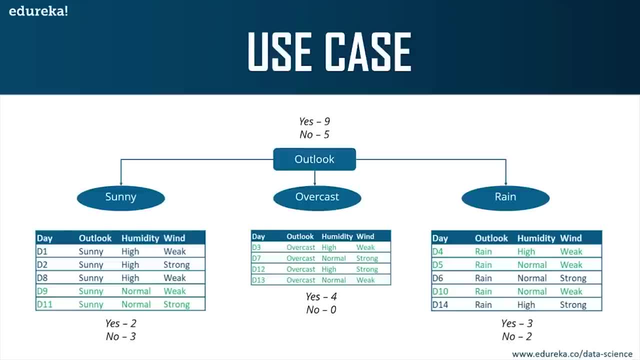 meaning that on the root node, you should have the most significant variable. all right, that's why we've chosen outlook. all right. now some of you might ask me: why haven't you chosen overcast? now, guys, overcast is not a variable, it is a value of the outlook variable. all right, that's why we've 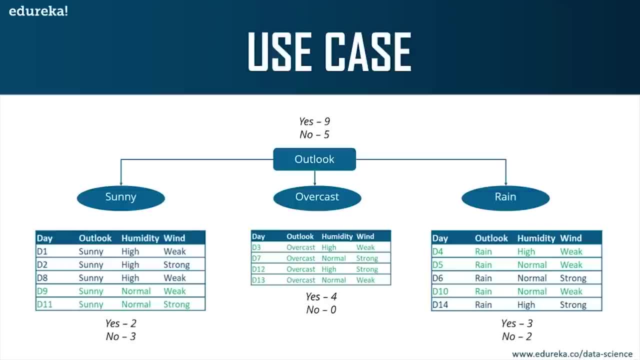 chosen outlook here because it has a 100 pure subset, which is overcast. all right now, the question in your head is: how do i decide which variable or attribute best splits the data? now, right now, i know i looked at the data and i told you that you know, uh, here we have a hundred percent. 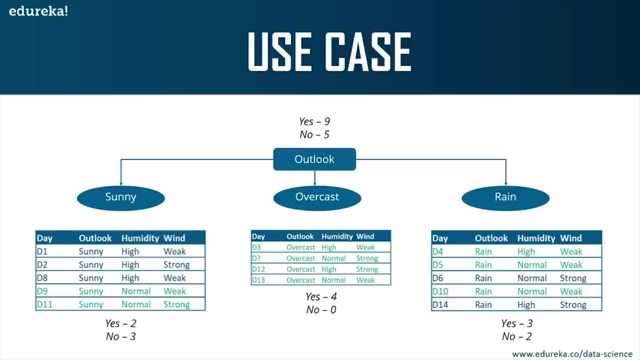 pure subset. but what if it's a more complex problem and you're not able to understand which variable will best split the data? so, guys, when it comes to decision trees, information and gain and entropy will help you understand which variable will best split the data set. all right, or which. 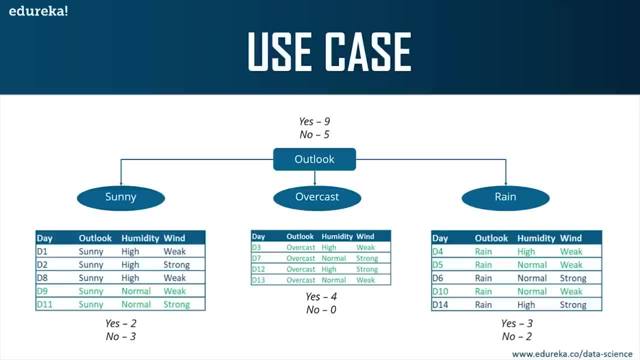 variable you have to assign to the root node, because whichever variable is assigned to the root node, it will best split the data set, and it has to be the most significant variable. all right, so, um, how we can do this is we need to use information gain and entropy. so, from the total of 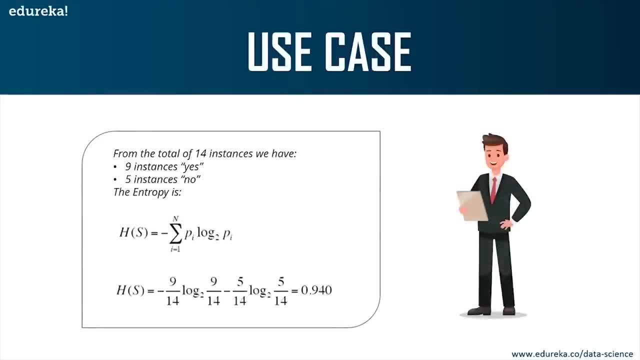 the 14 instances that we saw, 9 of them said yes and 5 of the instances said no, that you cannot play on that particular day. all right, so how do you calculate the entropy? so this is the formula. you just substitute the values in the formula. so when you substitute the values in the formula, you'll get. 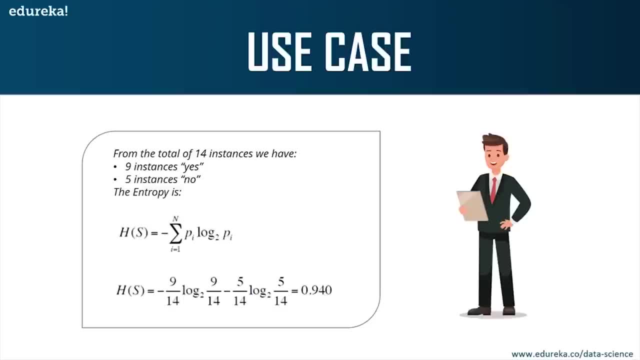 a value of 0.940. all right, this is the entropy, or this is the uncertainty, of the data present in our sample. now, in order to ensure that we choose the best variable for the root node, let us look at all the possible combinations that you can use on the root node. okay, so these are all the possible. 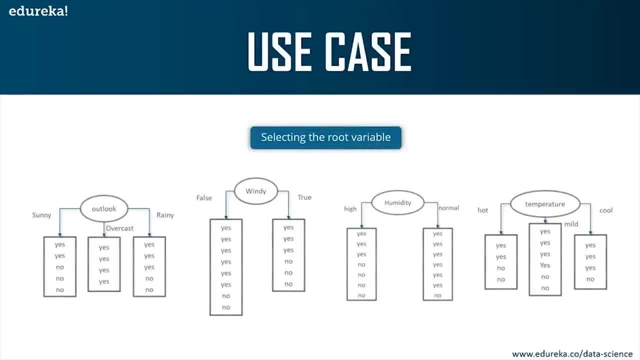 combinations. you can either have outlook, you can have windy, humidity or temperature. okay, these are our four variables, and you can have any one of these variables as your root node, but how do you select which variable best fits the root node? that's what we are going to see, by using information. 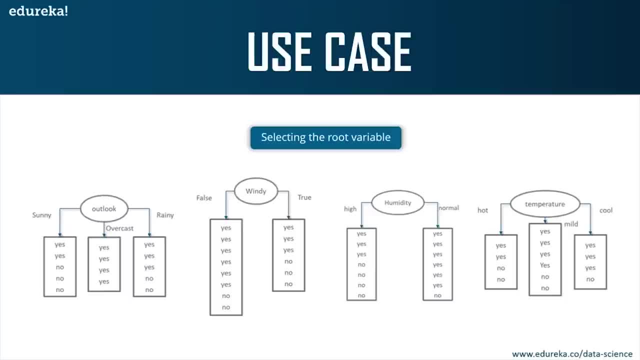 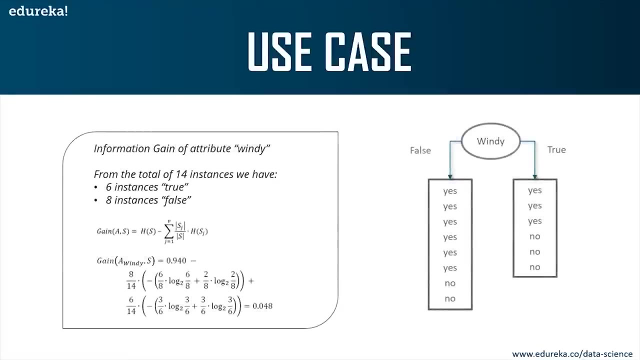 gain and entropy. so, guys, now the task at hand is to find the information gain for each of these attributes. all right, so for outlook, for windy, for humidity and for temperature, we're going to find out the information gain. all right, now. a point to remember is that the variable that results in the highest information 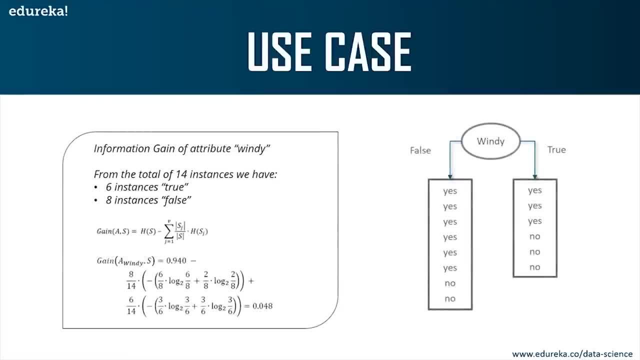 gain must be chosen because it will give us the most precise and output information. all right, so the information gain for attribute windy. we'll calculate that first. here we have six instances of true and eight instances of false. okay, so when you substitute all the values in the formula, 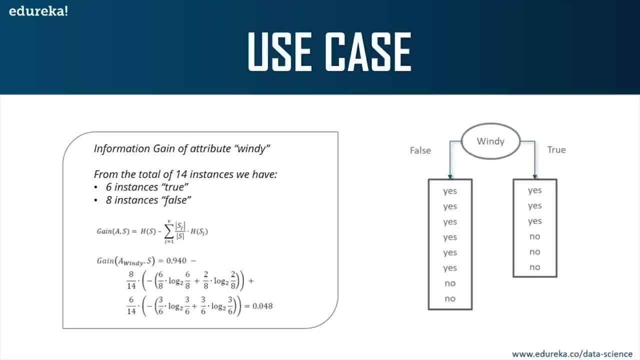 you'll get a value of zero point zero four eight. so we get a value of zero point zero four eight. now, this is a very low value for uh, information gain. all right, so the information that you're going to get from windy attribute is pretty low, so let's calculate the information gain. 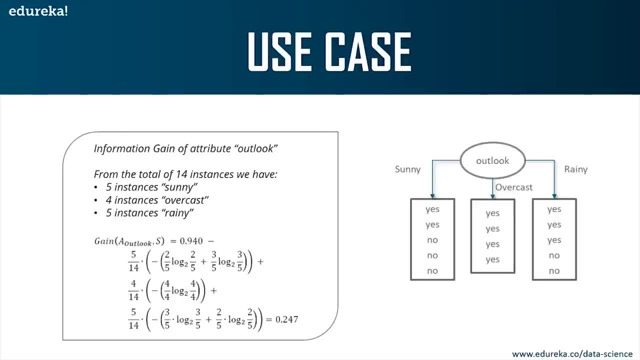 of attribute outlook: all right. so from the total of 14 instances, we have five instances which say sunny, four instances which are overcast and five instances which are rainy. all right for sunny. we have three yeses and two knowns for overcast. we have all the four as 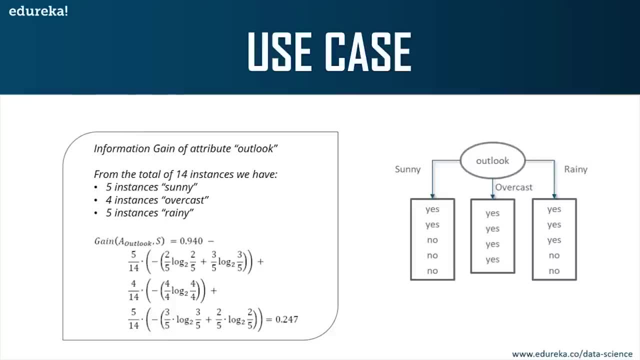 yes for rainy, we have three yes and two nodes. okay, so when you calculate the information gain of the outlook variable, we'll get a value of 0.247. now compare this to the information gain of the windy attribute. this value is actually pretty good. right? we have 0.247, which is a pretty good value. 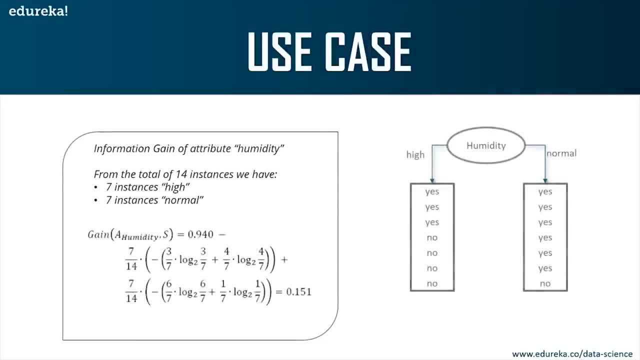 for information gain. now let's look at the information gain of attribute humidity. now over here we have seven instances which say high and seven instances which say normal. right and under the high branch node we have three instances which say yes and the rest four instances which say no. similarly, under the normal branch we have one, two, three, four, five, six, seven. 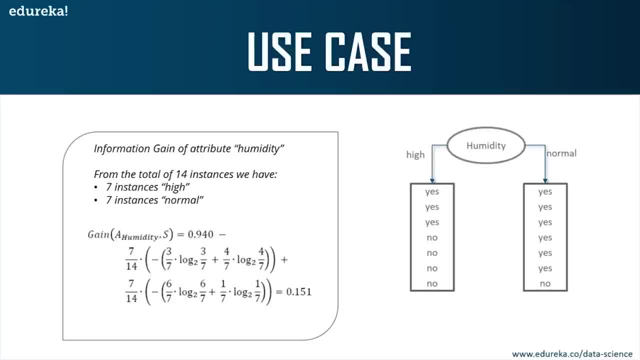 instances which say yes and one instance which says no. all right. so when you calculate the information gain for the humidity variable, you're going to get a value of 0.151. now, this is also a pretty decent value, but when you compare it to the information gain of the attribute, 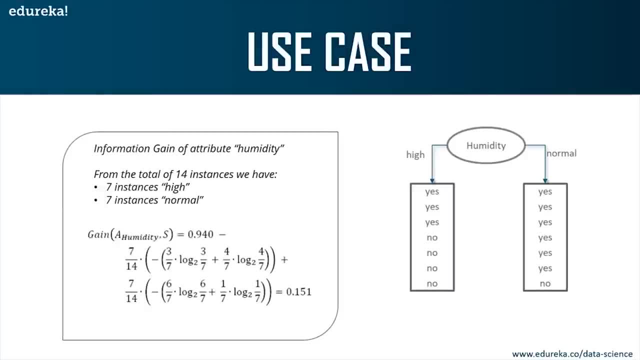 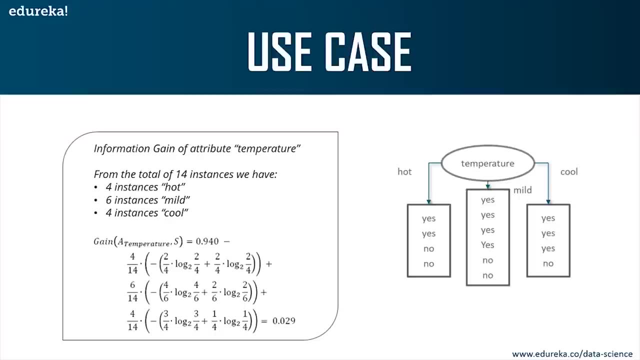 outlook, it is less right now. let's look at the information gain of attribute temperature. all right, so the temperature can hold. repeat. so basically the temperature attribute can hold hot, mild and cool. okay, under hot, we have two instances which says yes and two instances for no. under mild, 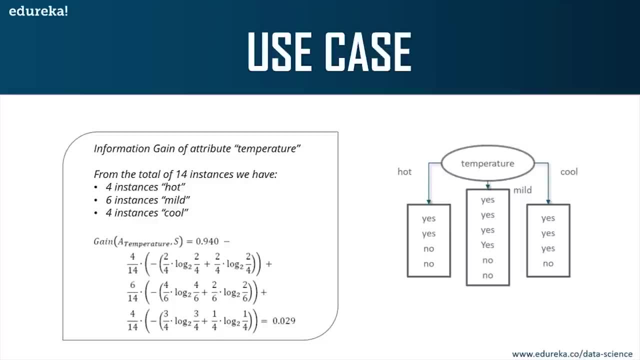 we have four instances of yes and two instances of no, and under cool we have three instances of yes and one instance of no. all right now, when you calculate the information gain of the temperature variable, you will get a value of 0.029, which is again very less. so what you can summarize from: 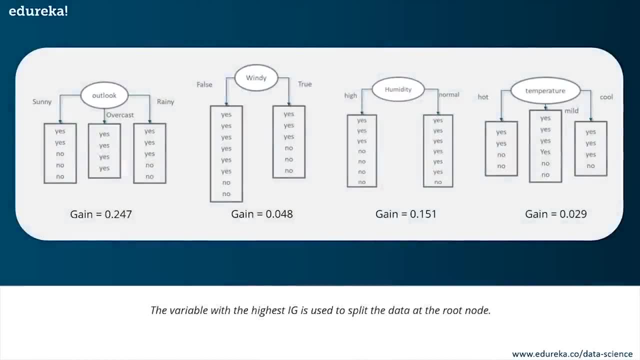 here is: if we look at the information gain for each of these variable, we'll see that for outlook, we have the maximum gain. all right, we have 0.247, which is the highest information gain value, and you must always choose a variable with the highest information gain to split the data at the root. 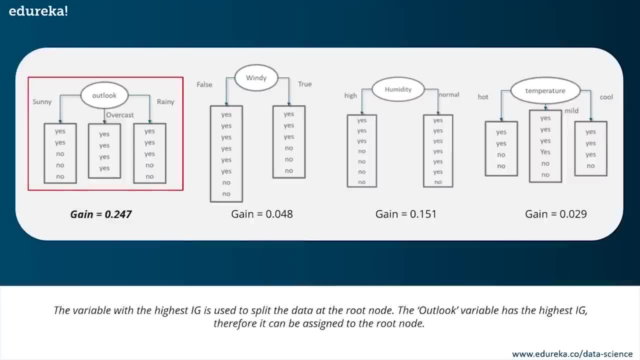 node. so that's why we assign the outlook value to the information gain value, and then we have the variable at the root node. all right, so, guys, i hope this use case was clear. if any of you have doubts, please keep commenting those doubts. now let's move on and look at what exactly a confusion. 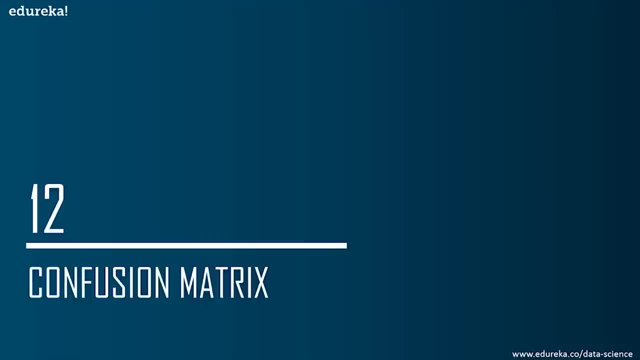 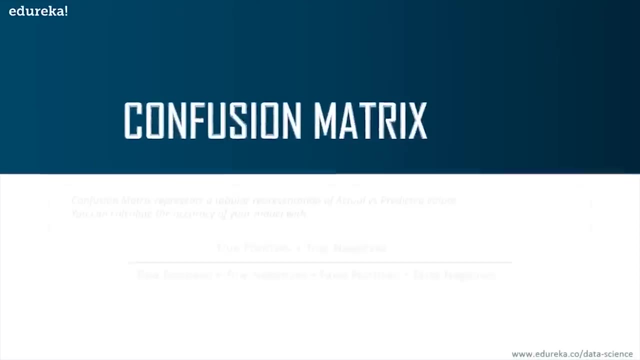 matrix is now the confusion. matrix is the last topic for descriptive statistics. all right, after this, i'll be running a short demo where i'll be showing you how you can calculate mean, median mode and standard deviation variance and all of those values by using r. okay, so let's talk. 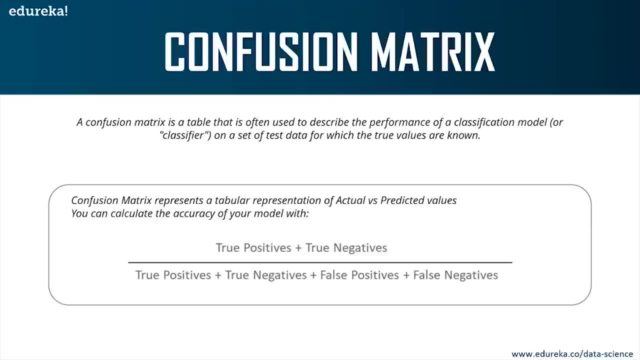 about confusion matrix. now, guys, what is a confusion matrix? now, don't get confused. this is not any complex topic. now, confusion matrix is a matrix that is often used to describe the performance of a model. all right, and this is specifically used for classification models or a classifier, and what it does is it will calculate the accuracy, or it will calculate. 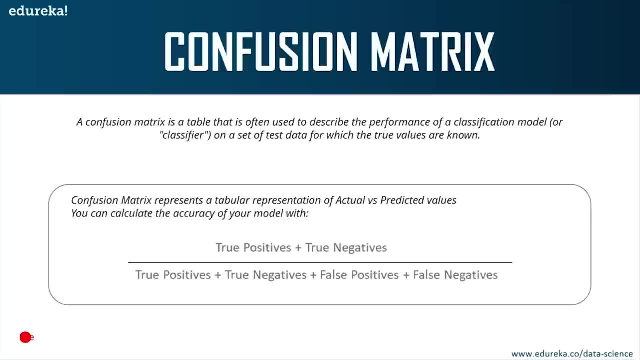 the performance of your classifier by comparing your actual results and your predicted results. all right, so this is what it looks like: true positive plus true negative and all of that. now, this is a little confusing. i'll get back to what exactly true positive, true negative and all of. 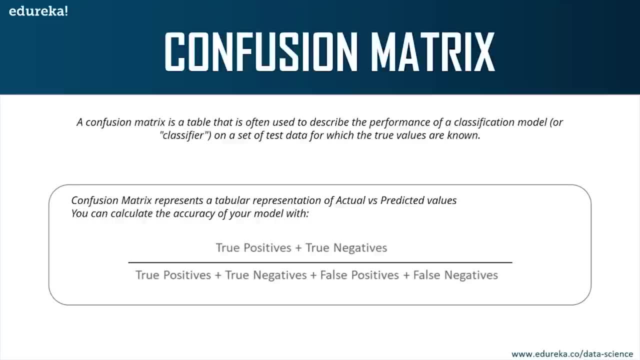 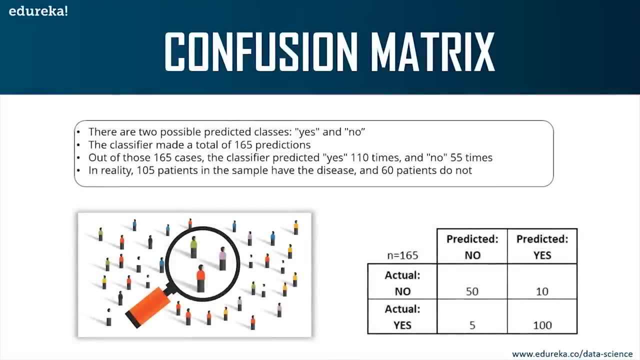 this stands for. for now, let's look at an example and let's try and understand what exactly confusion matrix is. so, guys, i made sure that i put examples after each and every topic because it's important you understand the practical part of statistics. all right, statistics has literally nothing to do. 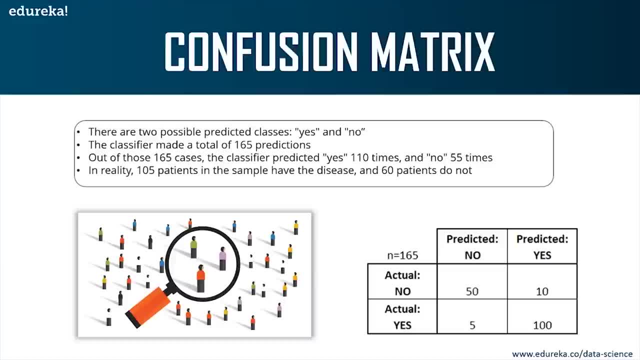 with theory. you need to understand how calculations are made and how you can calculate them, and then you need to understand how calculations are done in statistics. okay, so here, what i've done is: um, now let's look at a small use case. okay, let's consider that you're given data about 165 patients. 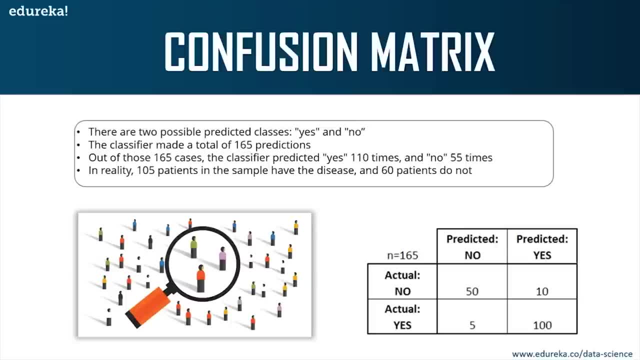 out of which 105 patients have a disease and the remaining 50 patients don't have a disease. okay, so what you're going to do is you'll build a classifier that predicts by using these 165 observations. you'll feed all of these 165 observations to your classifier. 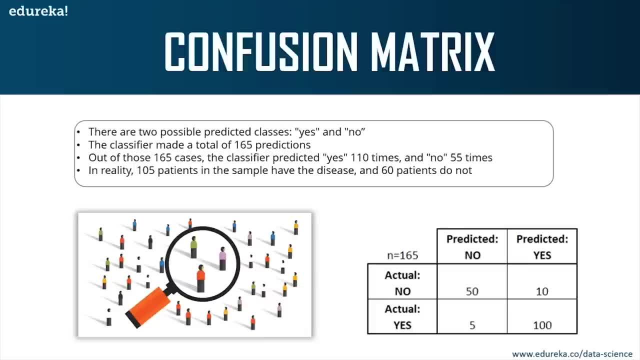 output every time a new patient's detail is fed to the classifier. right now, out of these 165 cases, let's say that the classifier predicted yes 110 times and no 55 times. all right, so yes basically stands for uh- yes, the person has a disease, and no stands for no, the person does not have a disease. 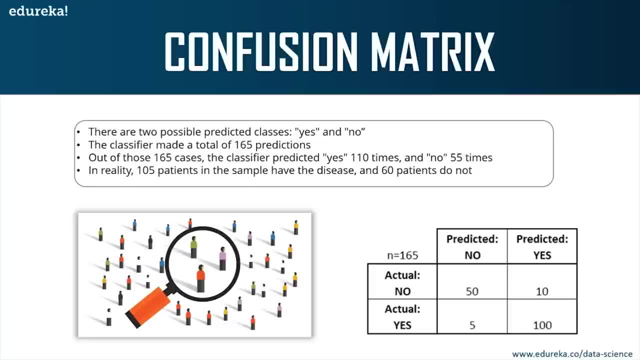 all right, that's pretty self-explanatory, but yeah, so it predicted that 110 times the patient has a disease and 55 times that, no, the patient doesn't have a disease. however, in reality, only 105 patients in the sample have the disease and 60 patients do not have the disease. 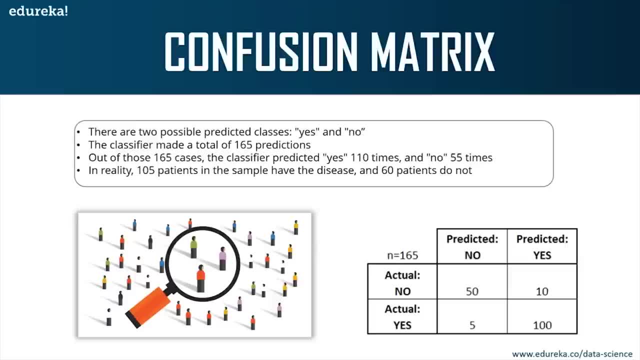 right. so how do you calculate the accuracy of your model? you basically build the confusion matrix. all right, this is how the matrix looks like and basically denotes the total number of observations that you have, which is 165 in our case. actual denotes the actual values in the data. 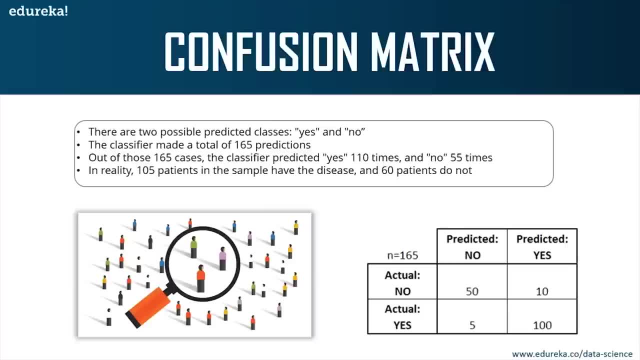 and predicted denotes the predicted values by the classifier, so the actual value is no here and the predicted value is no here. so your classifier was correctly able to classify 50 cases as no. all right, since both of these are no, so 50 it was correctly able to classify but 10 of these cases. it. 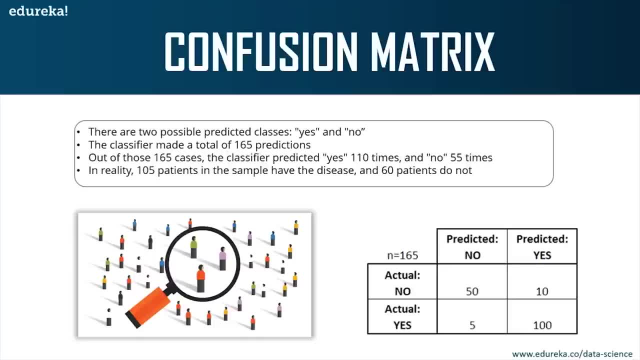 incorrectly classified, meaning that your actual value here is no, but your classifier predicted it as yes. all right, that's why there's 10 over here. similarly, it wrongly predicted that five patients do not have diseases, whereas they actually did have diseases, and it correctly predicted 100 patients, which have the 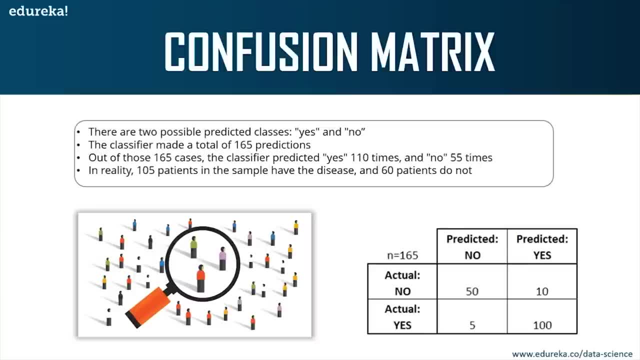 disease. all right, i know this is a little bit confusing, but if you look at these values: no, no, 50, meaning that it correctly predicted 50 values. no, yes means that it wrongly predicted yes for the values that it was supposed to predict. no, all right. now, what exactly is this true? 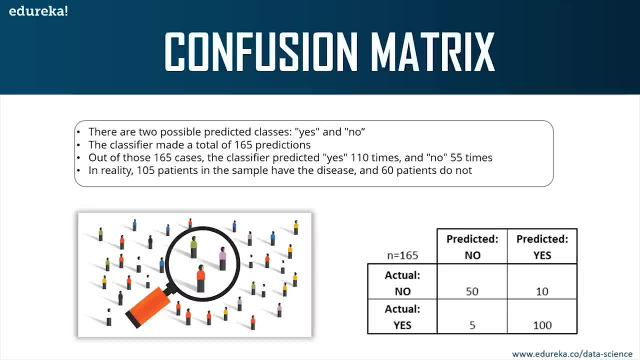 positive, true negative and all of that. i'll tell you what exactly it is so true. positive are the cases in which we predicted a yes and they do not actually have the disease. all right, so it is basically this value. all right, we predicted a yes here, even though they did not have the disease. 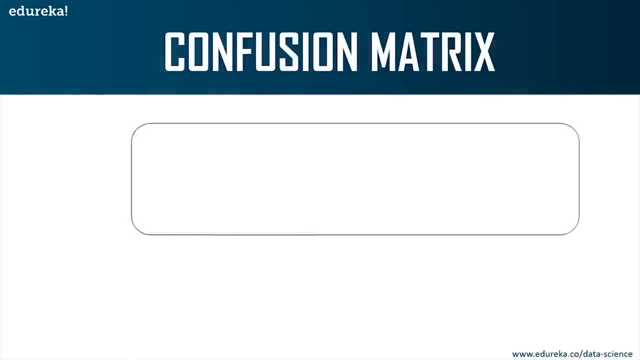 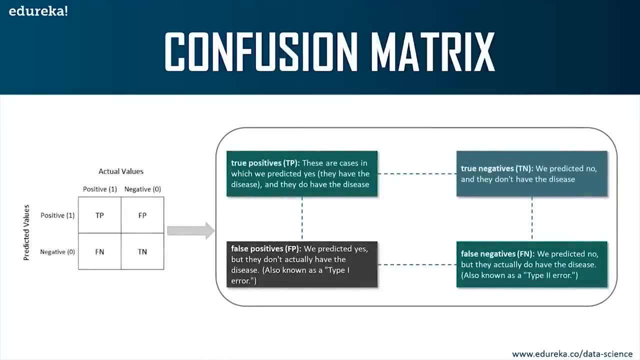 so we have 10 true positives, right. similarly, true negative is we predicted? no, and they don't have the disease, meaning that this is correct. all right. so false negative is false negative is we predicted? yes, but they do not actually have the disease. all right, this is also known as type 1 error. false negative is we predicted? no, but they. 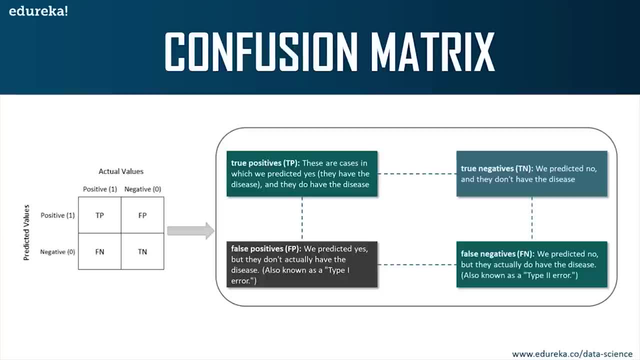 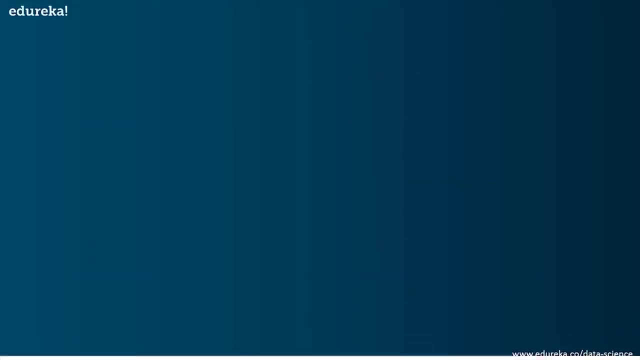 actually do not have the disease. so, guys, basically false negative and true negatives are basically correct classifications, all right. so this was confusion matrix and i hope this concept is clear again. guys, if you have doubts, please comment your doubts in the comment section. so, guys, that was descriptive statistics. now before we go to probability. 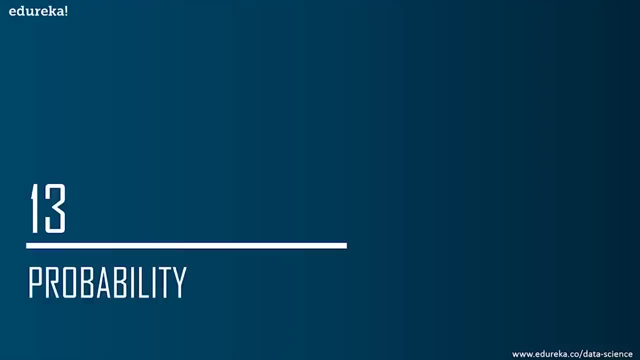 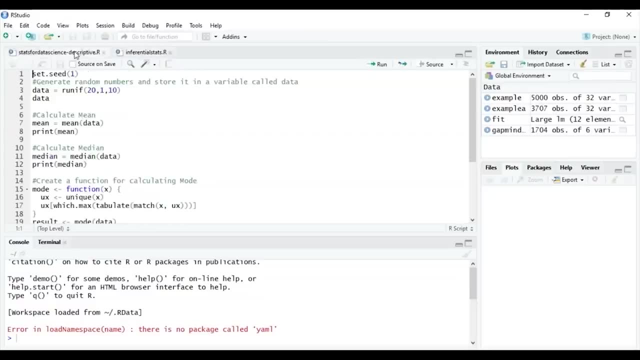 I promised you all that we'll run a small demo in R. All right, we'll try and understand how mean median mode works in R. Okay, so let's do that first. So, guys, again, what we just discussed so far was descriptive statistics. all right, 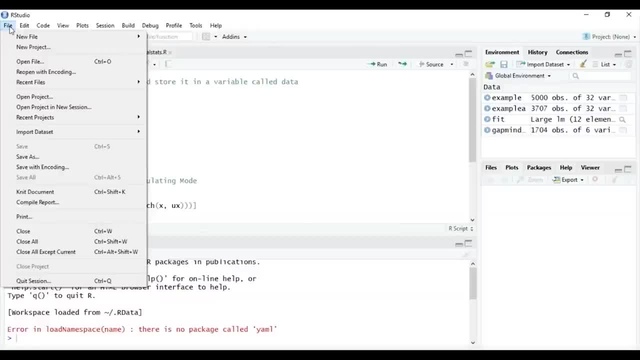 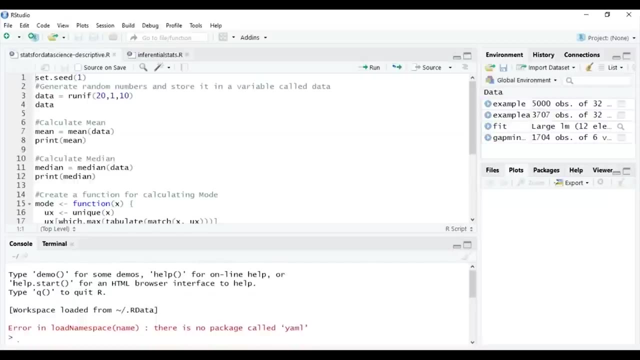 Next we're gonna discuss probability, and then we'll move on to inferential statistics. Okay, inferential statistics is basically the second type of statistics. okay, Now, to make things more clearer for you, let me just zoom in. So, guys, it's always best to perform. 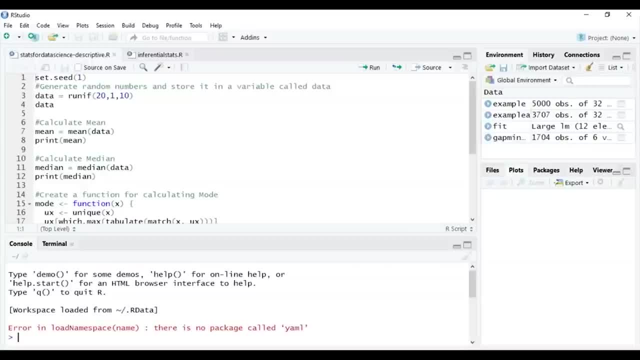 practical implementations in order to understand the concepts in a better way. okay, So here we'll be executing a small demo that'll show you how to calculate the mean, median mode, variance, standard deviation and how to study the variables by plotting a histogram. Okay, don't worry if you don't know what a histogram is. 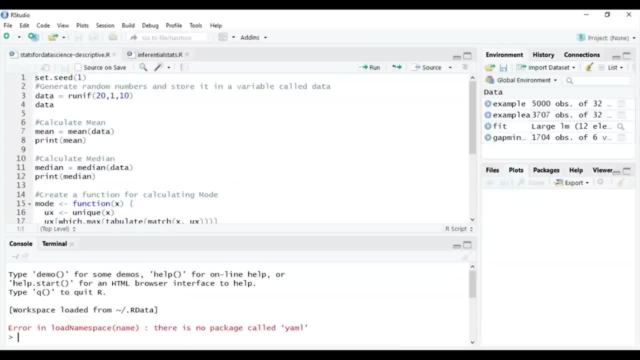 It's basically a frequency plot. There's no big science, There's no math behind it. all right, This is a very simple demo, but it also forms a foundation that every machine learning algorithm is built upon. Okay, you can say that most. 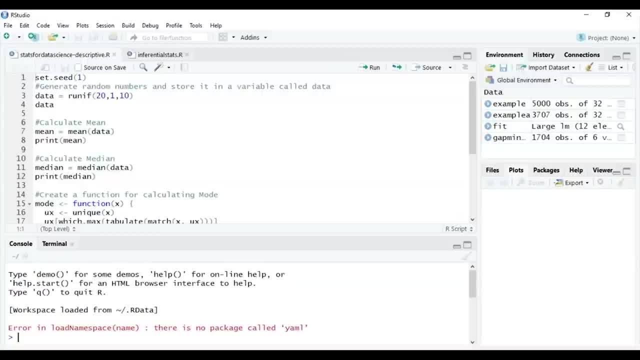 of the machine learning algorithms- actually, all the machine learning algorithms and deep learning algorithms- have this basic concept behind them. Okay, you need to know how mean, median mode and all of that is calculated. So, guys, I'm using the R language to perform this. 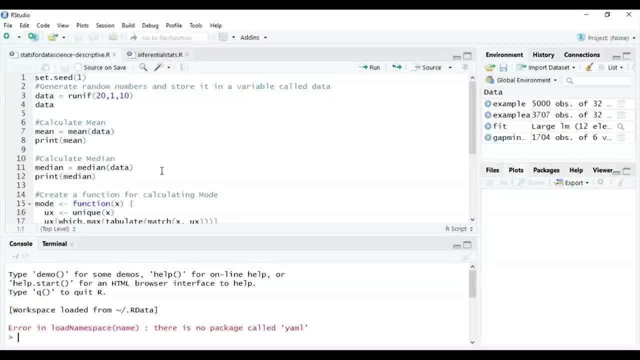 and I'm running this on R studio. For those of you who don't know R language, I will leave a couple of links In the description box. you can go through those videos. So what we're doing is we're randomly generating numbers. 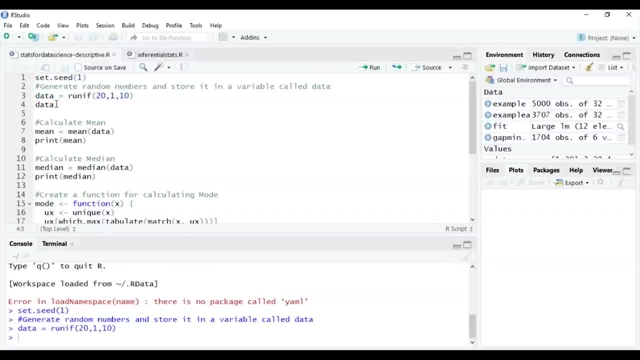 and we're storing it in a variable called data, all right. So if you want to see the generated numbers, just run the line data, all right, This variable basically stores all our numbers, all right. Now what we're gonna do is we're gonna calculate the mean. 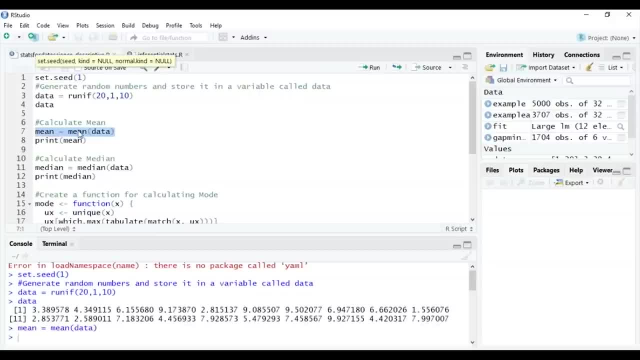 Now all you have to do in R is specify the word mean along with the data that you're calculating. So what we're doing is we're calculating the mean of, And I've assigned this whole thing into a variable called mean, which will hold the mean value of this data. 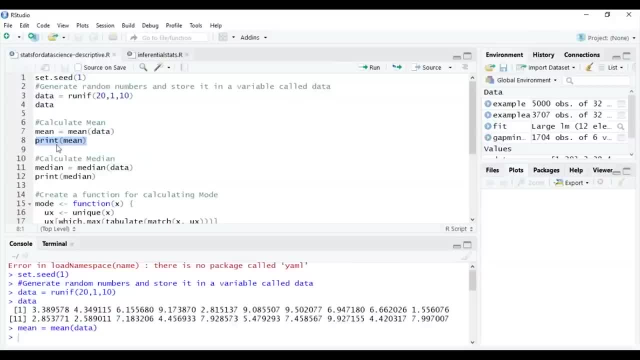 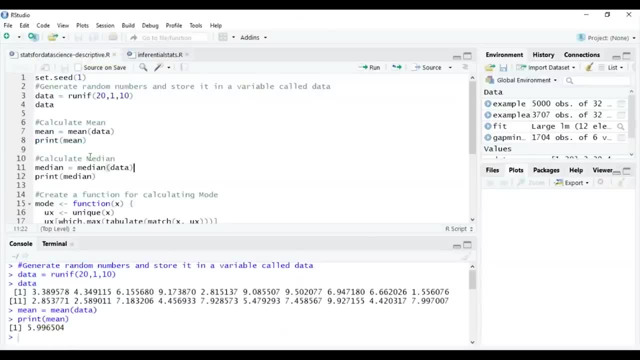 So now let's look at the mean. For that I've used a function called print and mean, All right, so our mean is around 5.99, okay. Next is calculating the median. It's very simple, guys. All you have to do is use a function, median, all right. 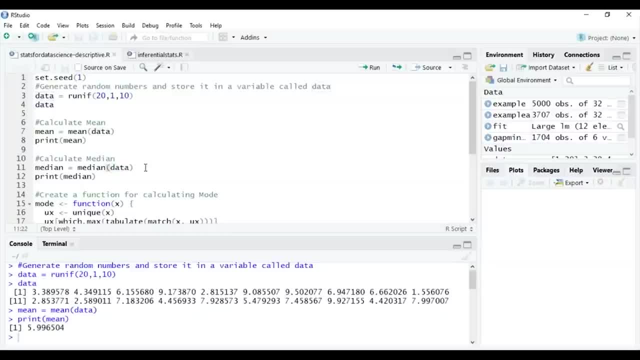 And pass the data. There's a parameter to this function. That's all you have to do. So R provides functions for each and everything. all right, Statistics is very easy when it comes to R, because R is basically a statistical language. okay. 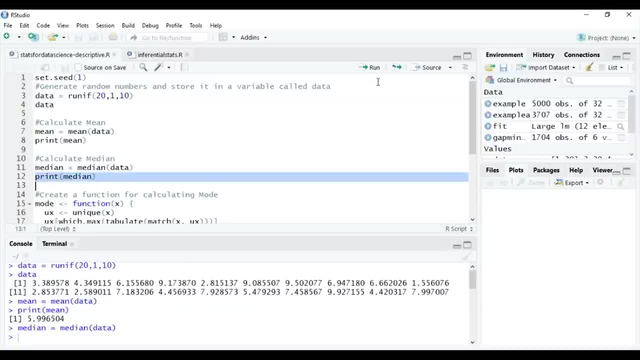 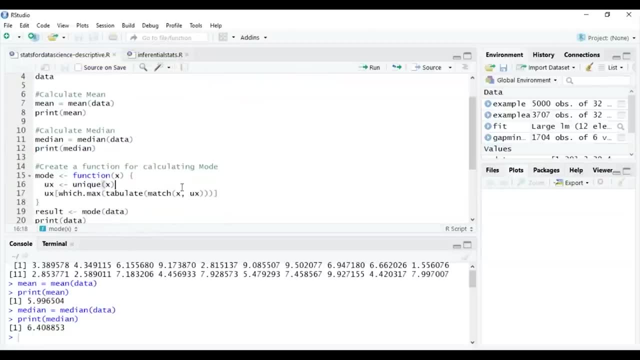 So all you have to do is just name the function, and that function is already built in your R. okay, So your median is around 6.4.. Similarly, we'll calculate the mode. all right, Let's run this function. I've basically created a small function. 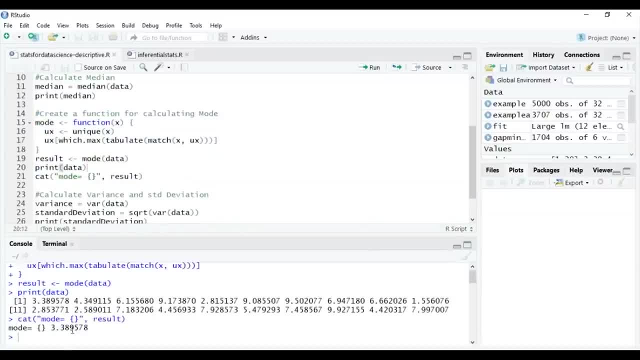 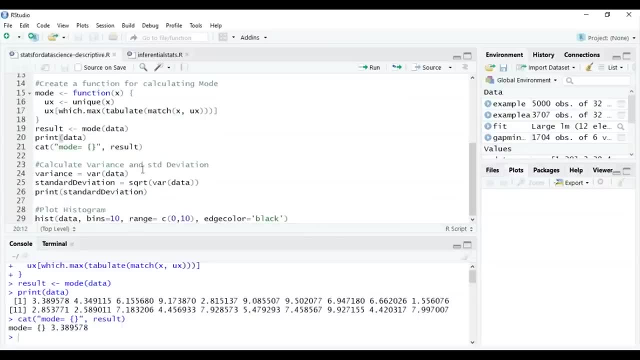 for calculating the mode. So, guys, this is our mode, meaning that this is the most recurrent value right Now. we're gonna calculate the variance and the standard deviation. For that, again, we have a function in R called as var. 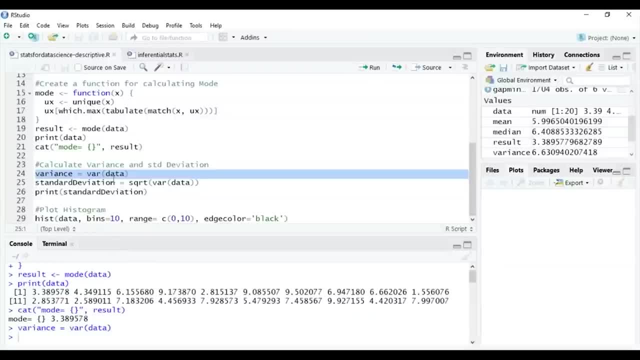 All right, all you have to do is pass the data to that function. okay. Similarly, we'll calculate the standard deviation, which is basically the square root of your variance. right Now. we'll print the standard deviation. right? This is our standard deviation value. 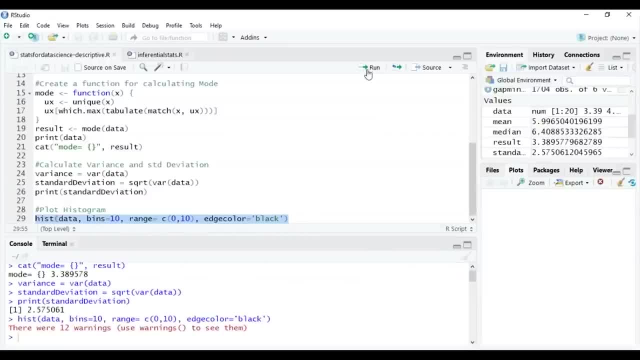 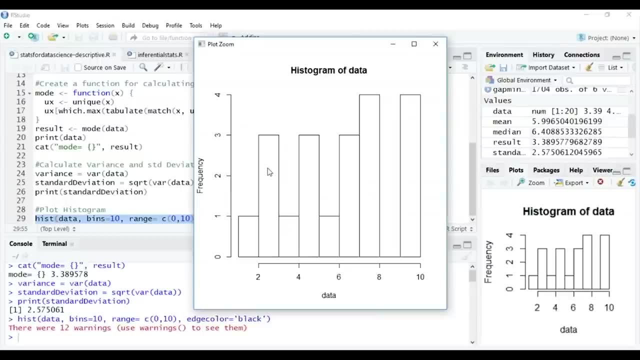 Now, finally, we'll just plot a small histogram. Histogram is nothing, but it's a frequency plot. all right, It'll show you how frequently a data point is occurring. So this is the histogram that we've just created. It's quite simple in R, because R has a lot of packages. 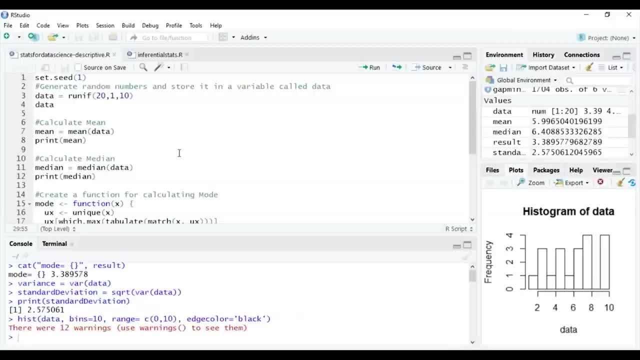 and a lot of inbuilt functions that support statistics. All right, it is a statistical language that is mainly used by data scientists or by data analysts and machine learning engineers, because they don't have to sit and code these functions. All they have to do is they have to mention the name. 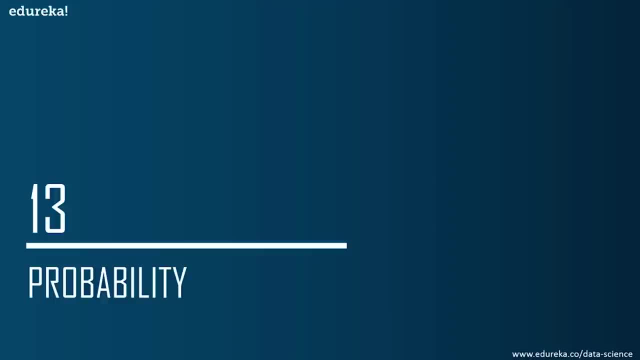 of the function and pass the corresponding parameters. So, guys, that was the entire descriptive statistics module, and now we'll discuss about probability. Okay, so before we understand what exactly probability is, let me clear out a very common misconception. People often tend to ask me this question. 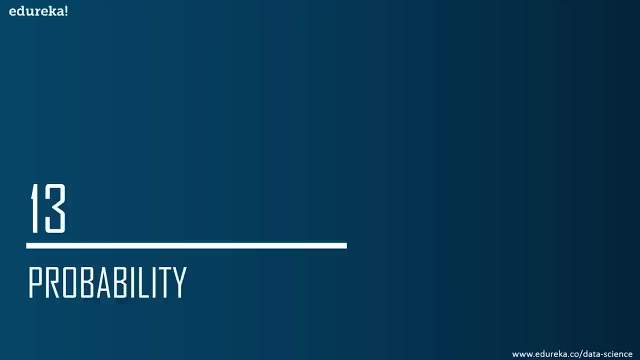 what is the relationship between statistics and probability? So probability and statistics are related fields? all right, So probability is a mathematical method used for statistical analysis. Therefore, we can say that probability and statistics are interconnected branches of mathematics that deal with analyzing the relative frequency of events. 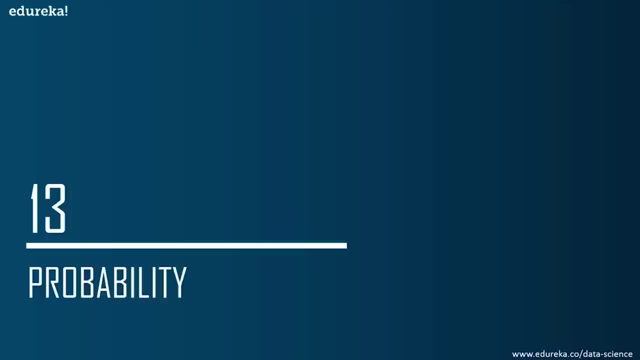 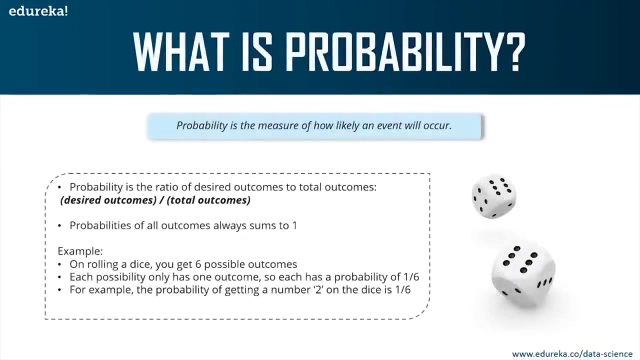 So they're very interconnected fields. and probability makes use of statistics and statistics makes use of probability. All right, they're very interconnected fields. So that is the relationship between statistics and probability. Now let's understand what exactly is probability. So probability is the measure. 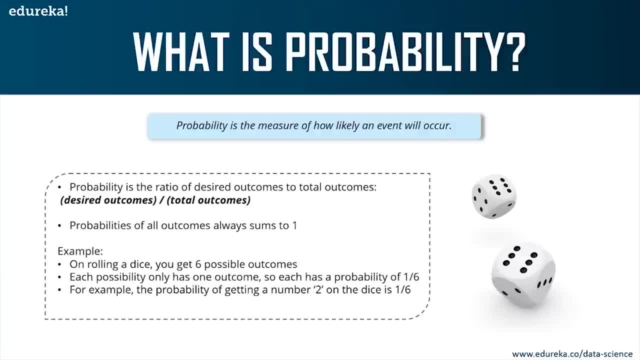 of how likely an event will occur. To be more precise, it is the ratio of desired outcome to the total outcomes. Now, the probability of all outcomes always sum up to one. Now, the probability will always sum up to one. Probability cannot go beyond one. 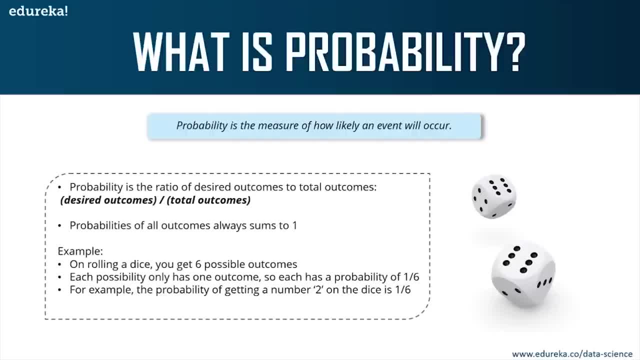 Okay, so either your probability can be zero, or it can be one, or it can be in the form of decimals like 0.52 or 0.55,, or it can be in the form of 0.5,, 0.7,, 0.9,, but its value will always stay. 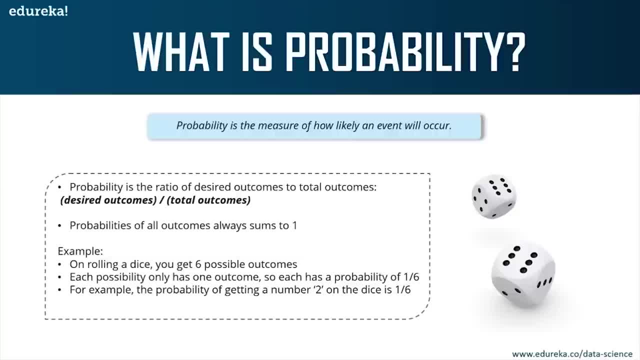 between the range zero and one. okay, Now the famous example of probability is rolling a dice example. So when you roll a dice you get six possible outcomes. right, you get one, two, three, four and five, six phases of a dice. 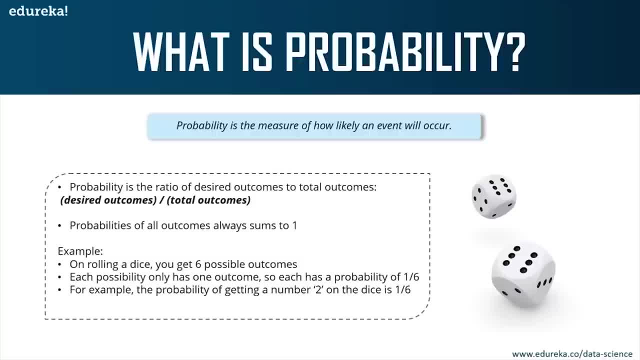 Now, each possibility only has one outcome. So what is the probability that, on rolling a dice, you'll get three? The probability is one by six, right, Because there's only one phase which has the number three on it. Out of six phases, there's only one phase. 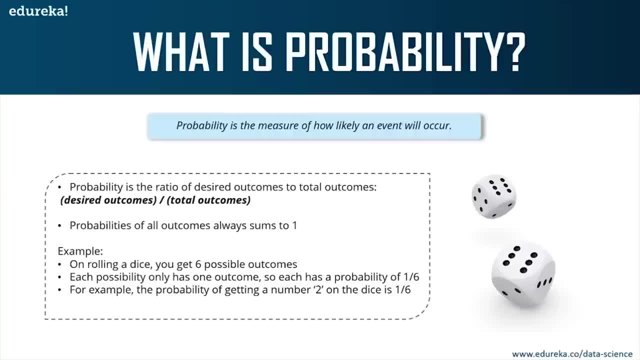 which has the number three. So the probability of getting three when you roll a dice is one by six. Similarly, if you want to find the probability of getting a number five again, the probability is going to be one by six. all right, 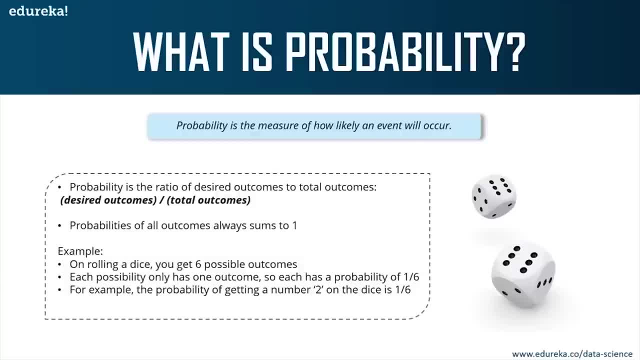 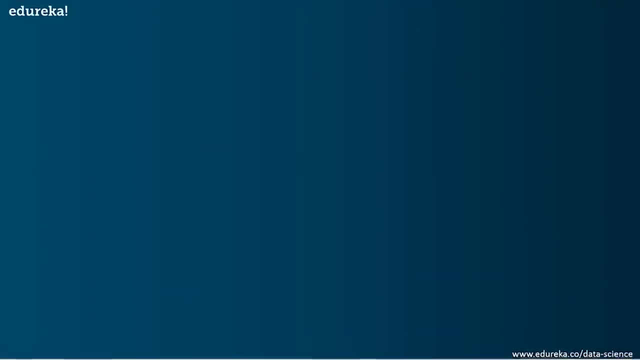 So all of this will sum up to one, all right. So, guys, this is exactly what probability is. It's a very simple concept. We all learned it in eighth standard onwards. right Now, let's understand the different terminologies that are related to probability. 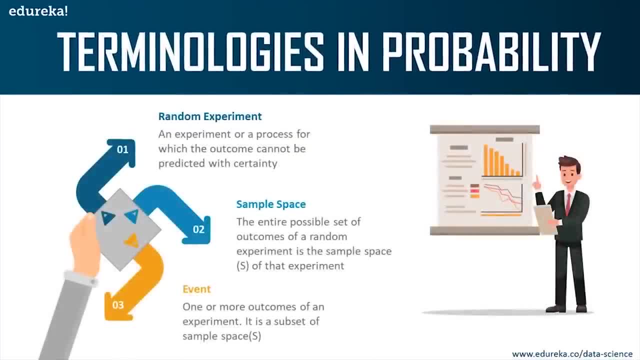 Now, there are three terminologies that you often come across when we talk about probability. We have something known as the random experiment. okay, It's basically an experiment or a process for which the outcomes cannot be predicted with certainty. All right, that's why you use probability. 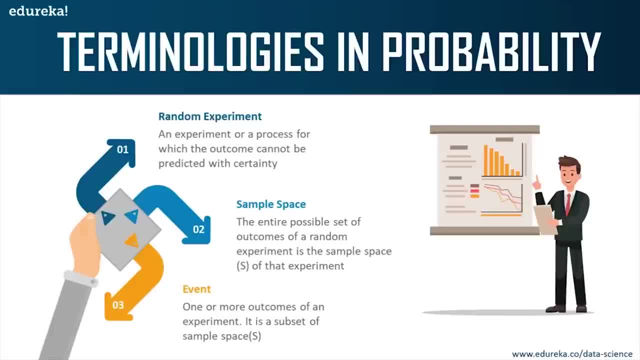 You're going to use probability in order to predict the outcome with some sort of certainty. Sample space is the entire possible set of outcomes of a random experiment. An event is one or more outcomes of an experiment. So if you consider the example of rolling a dice, 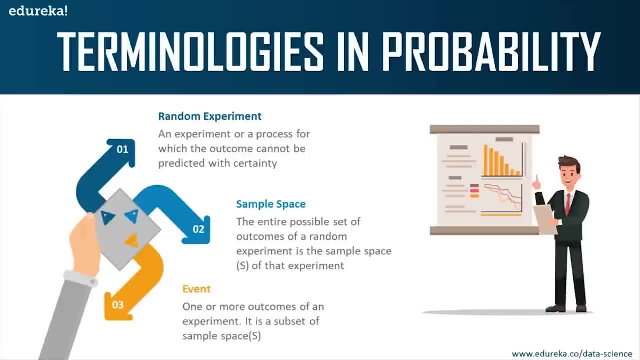 now let's say that you want to find out the probability of getting a two when you roll a dice. okay, So finding this probability is the random experiment. The sample space is basically your entire possibility. okay, So one, two, three, four, five, six phases. 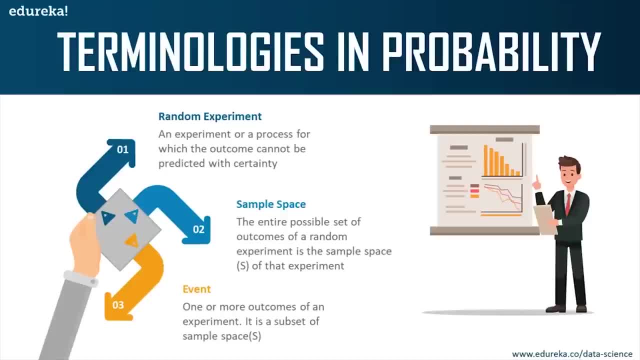 are there and out of that you need to find the probability of getting a two right. So all the possible outcomes will basically represent your sample space. okay, So one to six are all your possible outcomes. This represents your sample space. Now, event is one or more outcome of an experiment. 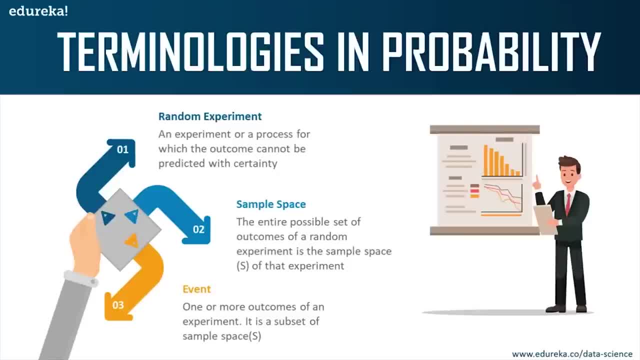 So, in this case, my event is to get a two when I roll a dice, right, So my event is the probability of getting a two when I roll a dice. So, guys, this is basically what random experiment, sample, space and event really means. all right, 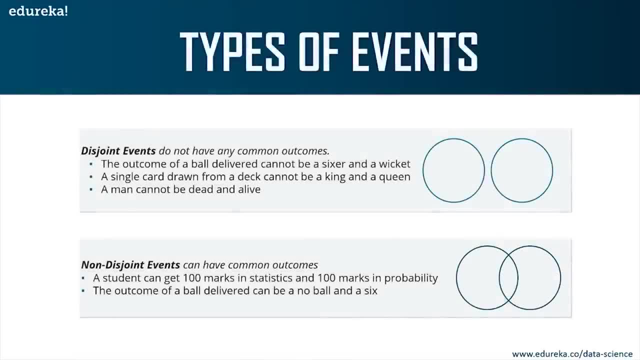 Now let's discuss the different types of events. There are two types of events that you should know about. There is disjoint and non-disjoint events. Disjoint events are events that do not have any common outcome. For example, if you draw a single card from a deck of cards. 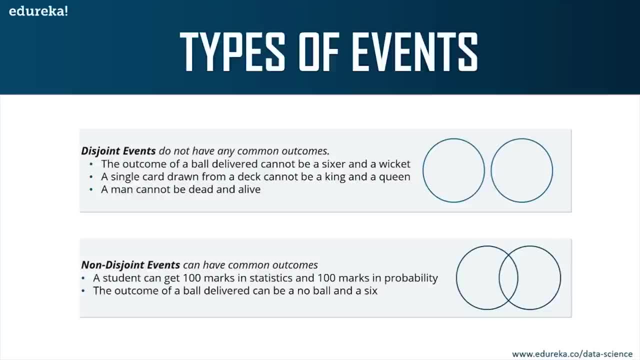 it cannot be a king and a queen, correct? It can either be king or it can be queen. Now, non-disjoint events are events that have common outcome. For example, a student can get 100 marks in statistics and 100 marks in probability, all right. 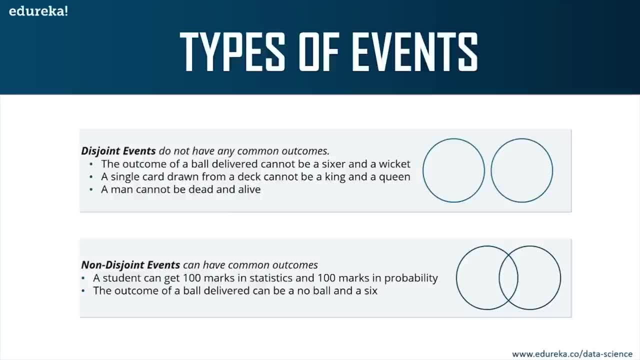 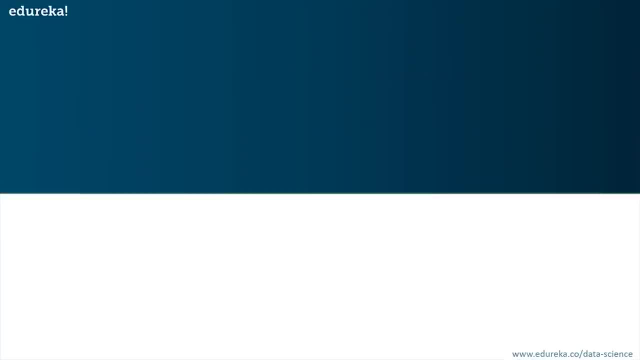 And also the outcome of a ball delivered can be a no ball and it can be a six right. So this is what non-disjoint events are. all right, These are very simple to understand. right Now let's move on and look at the different types. 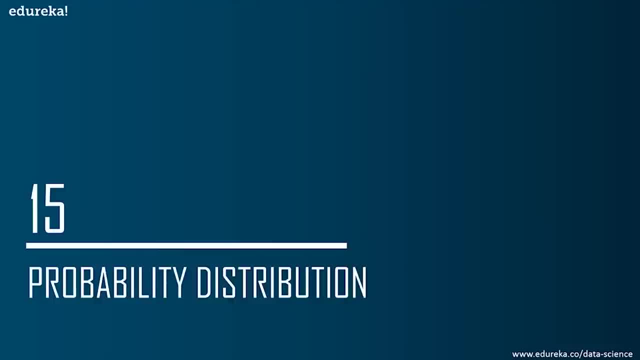 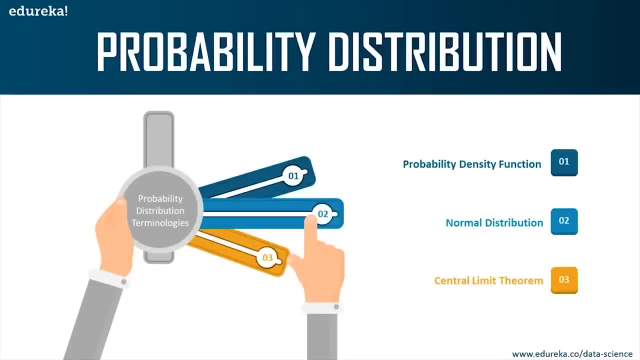 of probability distribution. all right, I'll be discussing the three main probability distribution functions. I'll be talking about probability density function. All right, I'll be talking about probability density function, normal distribution and central limit theorem. okay, probability density function, also known as 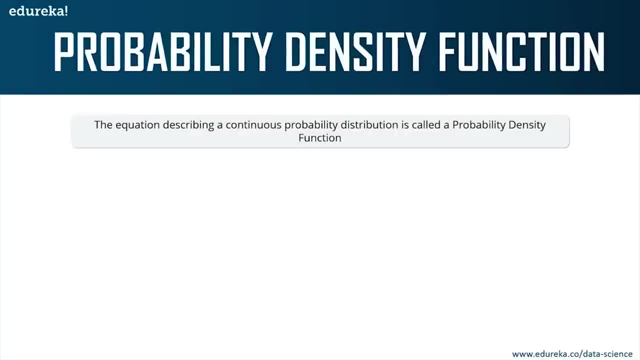 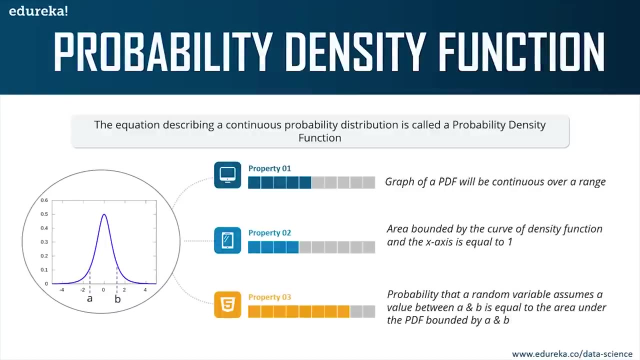 pdf is concerned with the relative likelihood for a continuous random variable to take on a given value. all right, so the pdf gives the probability of a variable that lies between the range a and b. so basically, what you're trying to do is you're going to try and find the probability of a. 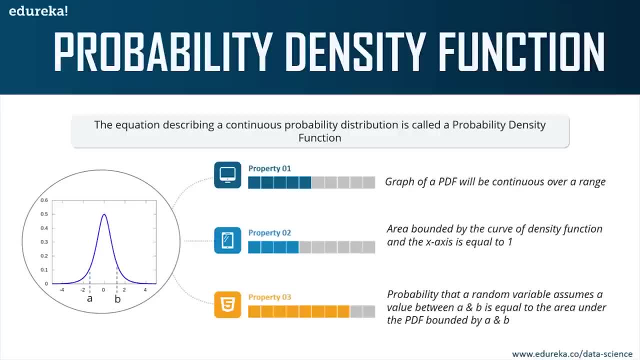 continuous random variable over a specified range. okay, now this graph denotes the pdf of a continuous variable. now, this graph is also known as the bell curve. all right, it's famously called the bell curve because of its shape, and there are three important properties that you need to know. 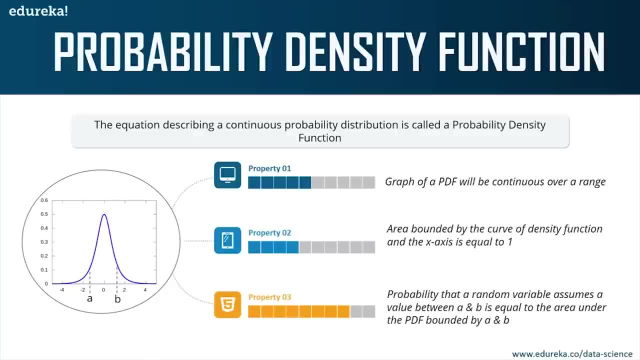 about a probability density function. now the graph of a pdf will be continuous over a range. this is because you're finding the probability that a continuous variable lies between the ranges a and b right. the second property is that the area bounded by the curve of a density function and the x-axis 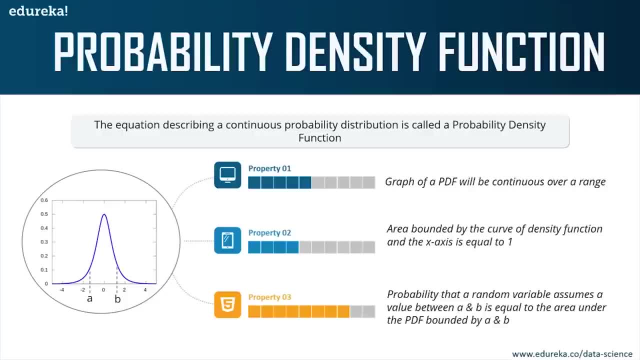 is equal to one. basically, the area below the curve is equal to one. all right, because it denotes probability. again, the probability cannot arrange more than one. it has to be between zero and one property. number three is that the probability that a random variable assumes a value between a and b. 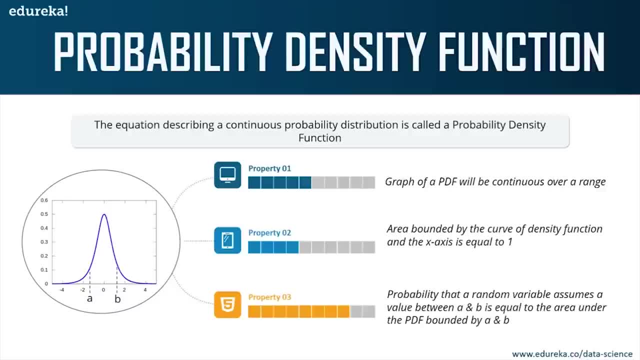 is equal to the area under the pdf bounded by a and b. okay, now, what this means is that the probability value is denoted by the area of the graph. all right, so whatever value that you get here, which is basically one, is the probability that a random variable will lie between the range a and 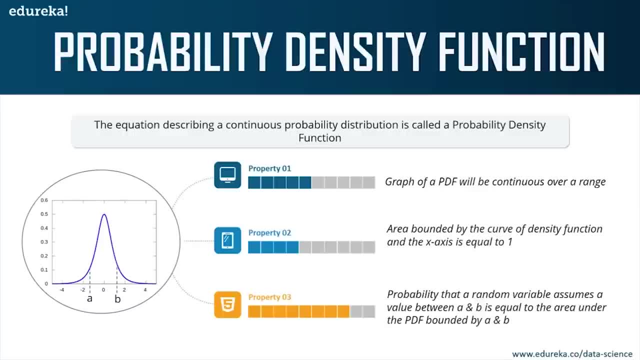 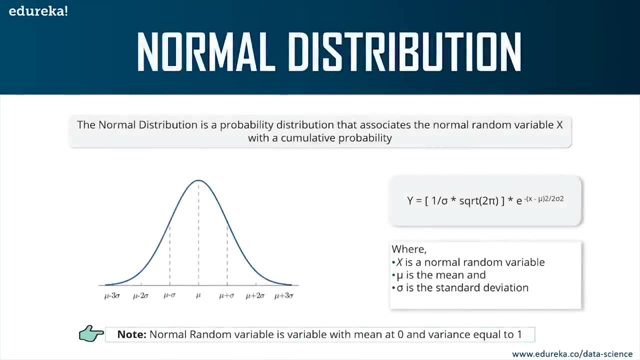 B. all right, so I hope all of you have understood the probability density function. it's basically the probability of finding the value of a continuous random variable between the range a and B. all right, now let's look at our next distribution, which is normal distribution. now, normal distribution. 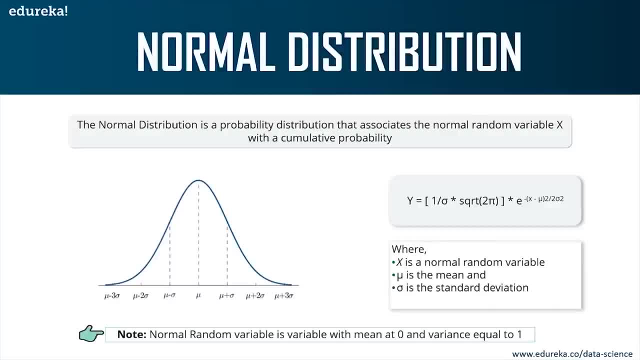 which is also known as the Gaussian distribution, is a probability distribution that denotes the symmetric property of the mean right, meaning that the idea behind this function is that the data near the mean occurs more frequently than the data away from the mean. so what it means to say is that the 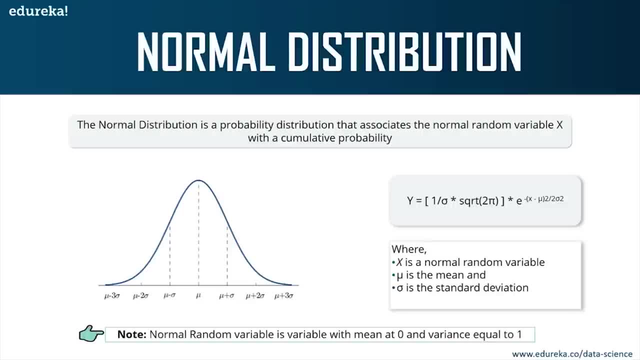 data around the mean. is the data around the mean? is the data around the mean represents the entire data set? okay, so if you just take a sample of data around the mean, it can represent the entire data set. now, similar to the probability density function, the normal distribution appears as a bell curve. all right now. 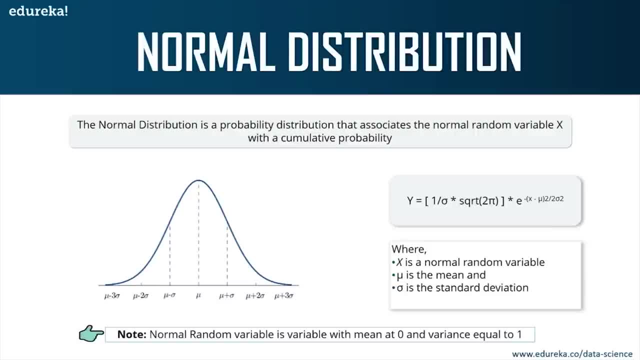 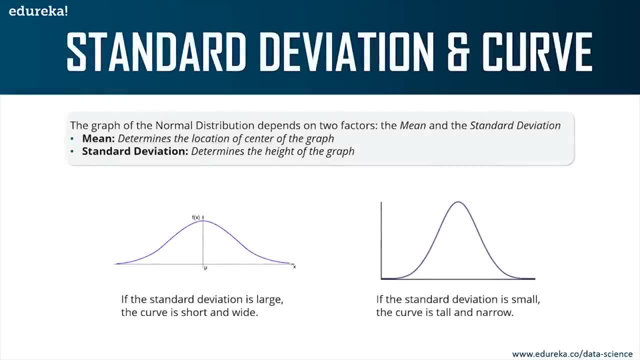 when it comes to normal distribution, there are two important factors. all right, we have the mean of the population and the standard deviation. ok, so the mean and the graph determines the location of the center of the graph right, and the standard deviation determines the height of the graph. 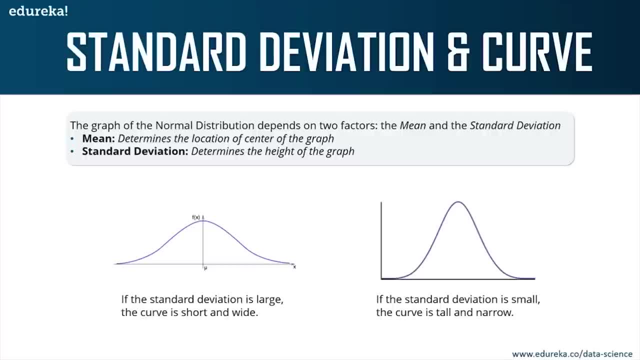 Okay. So if the standard deviation is large, the curve is going to look something like this: Alright, it'll be short and wide, And if the standard deviation is small, the curve is tall and narrow. Alright. So this was it, about normal distribution. 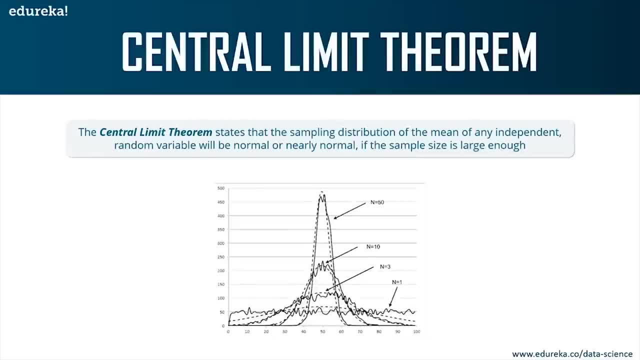 Now let's look at the central limit theory. Now the central limit theory states that the sampling distribution of the mean of any independent random variable will be normal or nearly normal if the sample size is large enough. Now that's a little confusing. Okay, let me break it down for you. 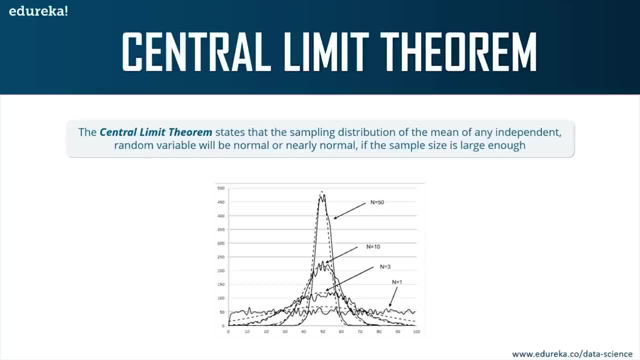 Now, in simple terms, if we had a large population and we divided it into many samples, then the mean of all the samples from the population will be almost equal to the mean of the entire population, Alright Meaning that each of the sample is normally distributed. 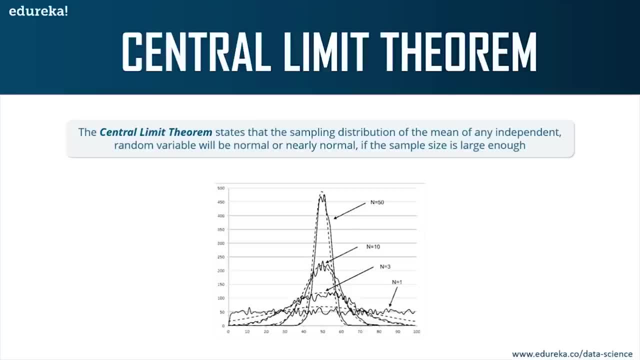 Right, So if you compare the mean of each of the sample, it'll almost be equal to the mean of the population. Alright, So this graph basically shows a more clear understanding of the central limit theorem. Alright, you can see each sample here. 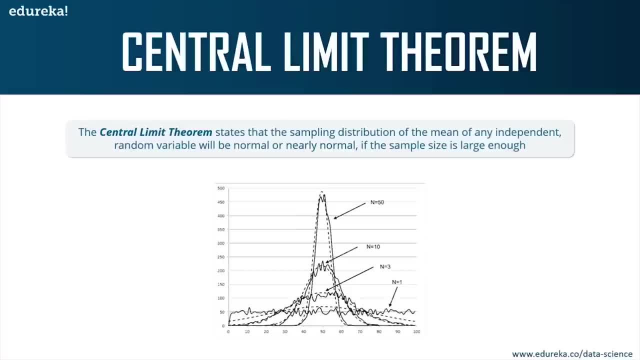 and the mean of each sample is almost along the same line, Right? Okay, so this is exactly what the central limit theorem states. Now, the accuracy, or the resemblance to the normal distribution depends on two main factors, Right? so the first is the number of sample points. 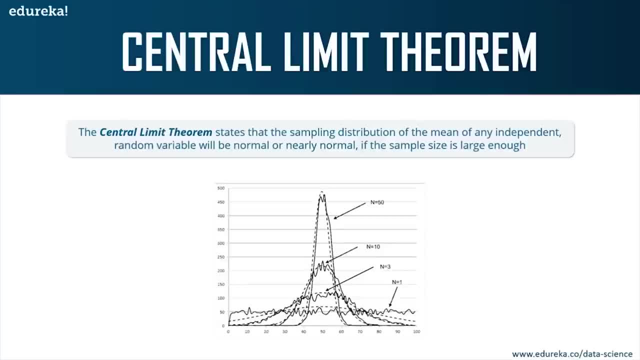 that you consider Alright. And the second is the shape of the underlying population. Alright. Now the shape obviously depends on the standard deviation and the mean of a sample, Correct? So, guys, central limit theorem basically states that each sample will be normally distributed. 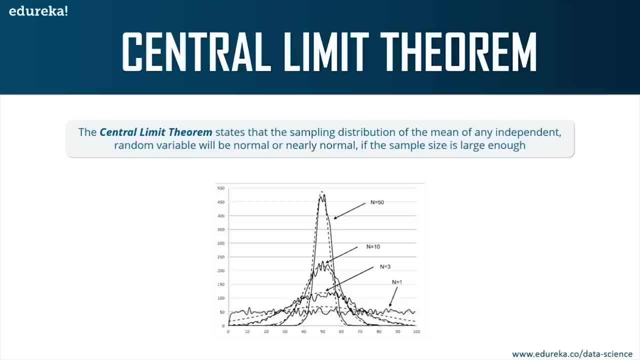 in such a way that the mean of each sample will coincide with the mean of the actual population. Alright, in short terms, that's what central limit theorem states. Alright, and this holds true only for a large data set, Mostly for a small data set. 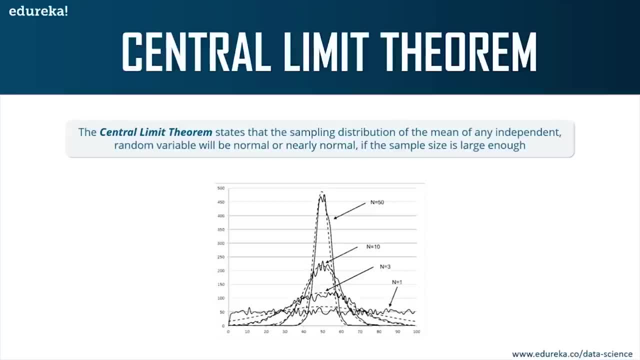 there are more deviations when compared to a large data set, It's because of the scaling factor Right. The smallest deviation in a small data set will change the value very drastically, But in a large data set a small deviation will not matter at all. 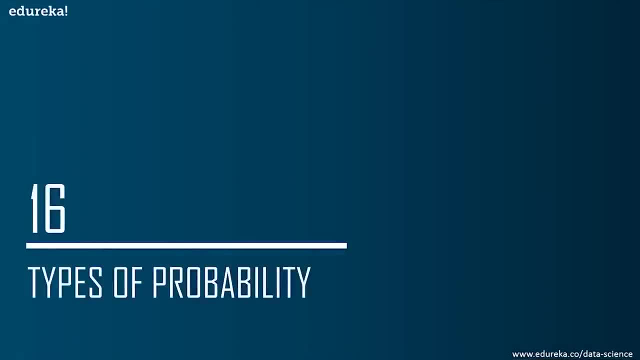 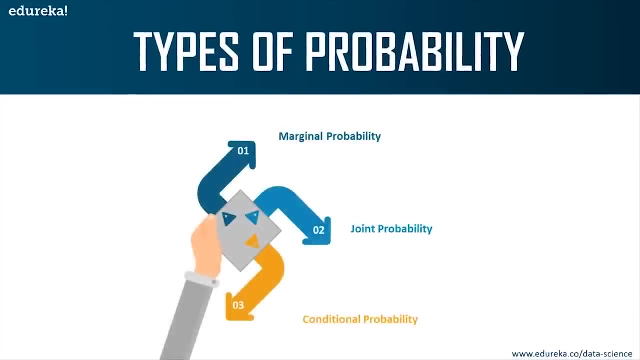 Now let's move on and look at our next topic, which is the different types of probability. Now, this is a important topic because most of your problems can be solved by understanding which type of probability should I use to solve this problem? Right, So we have three important types of probability. 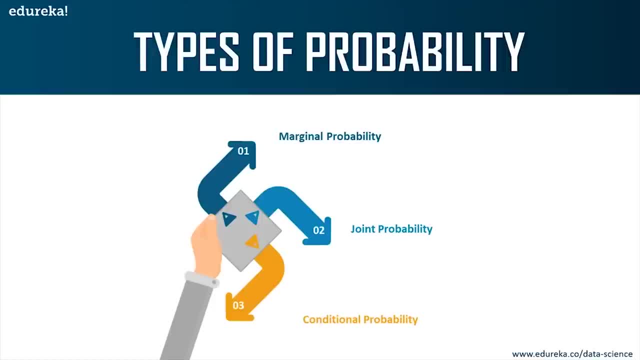 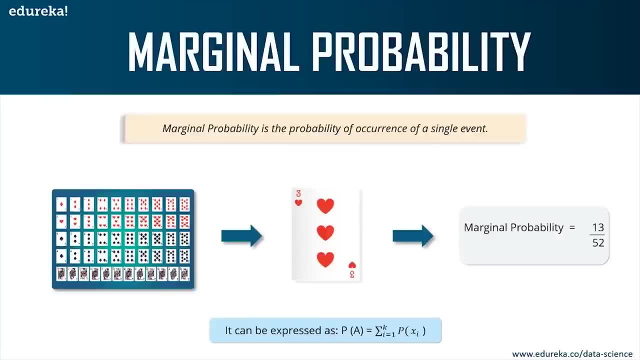 We have marginal, joint and conditional probability. So let's discuss each of these Now. the probability of an event occurring unconditioned on any other event is known as marginal probability or unconditional probability. So let's say that you want to find the probability. 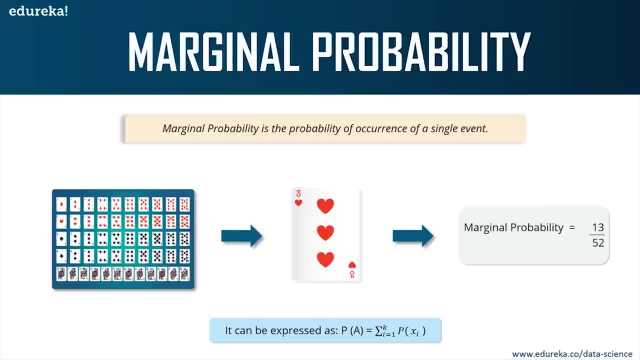 that a card drawn is a heart. Alright, So if you want to find the probability that a card drawn is a heart, the probability will be 13 by 52. Since there are 52 cards in a deck and there are 13 hearts in a deck of cards, 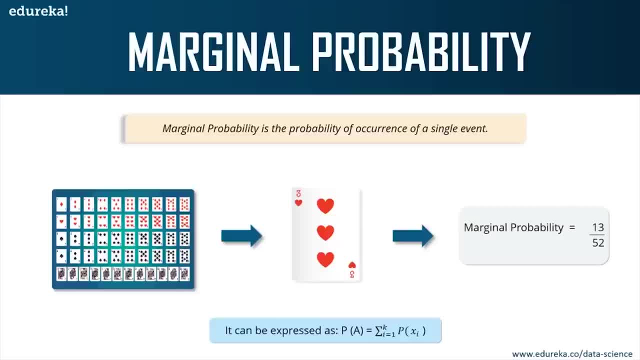 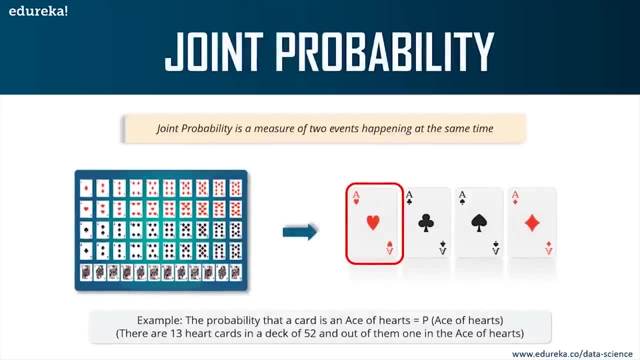 Right, And there are 52 cards in a total deck, So your marginal probability will be 13 by 52.. That's about marginal probability. Now let's understand what is joint probability. Now, joint probability is a measure of two events happening at the same time. 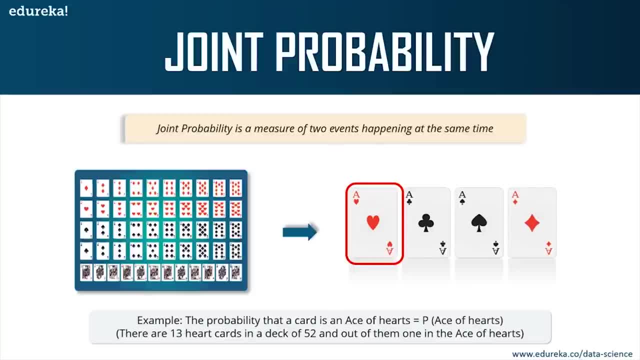 Okay, let's say that the two events are A and B. So the probability of event A and B occurring is the intersection of A and B. So, for example, if you want to find the probability that a card is a heart, that is four and red. 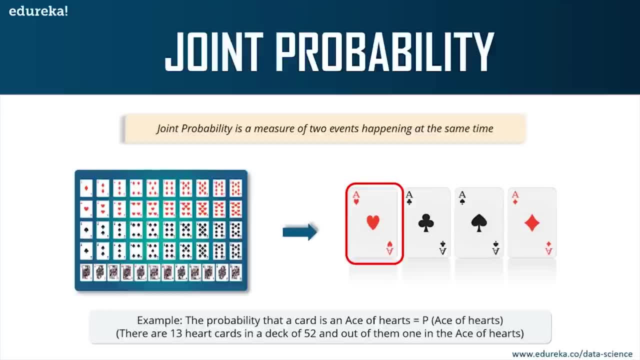 that would be joint probability. Alright, Because you're finding a card that is four and the card has to be red in color. So for the answer, this will be two by 52, because we have one, two in hearts and we have one, two in diamonds. 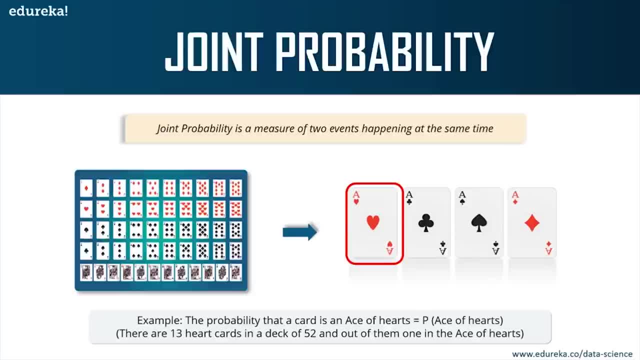 Correct. So both of these are red in color. therefore, our probability is two by 52. And if you further down it, it is one by 26.. Right, So this is what joint probability is all about. Moving on, let's look at. 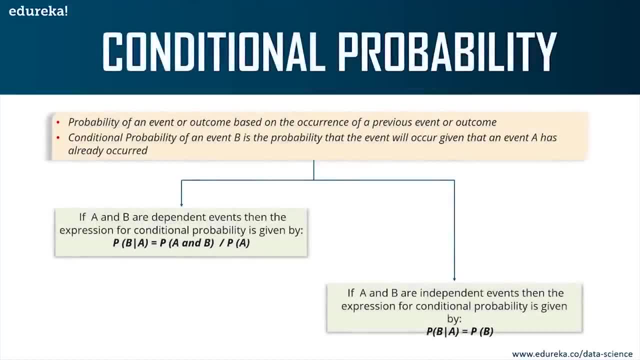 what exactly conditional probability is. So if the probability of an event or an outcome is based on the occurrence of a previous event or an outcome, then you call it as a conditional probability. Okay, So the conditional probability of an event B is the probability that the event will occur. 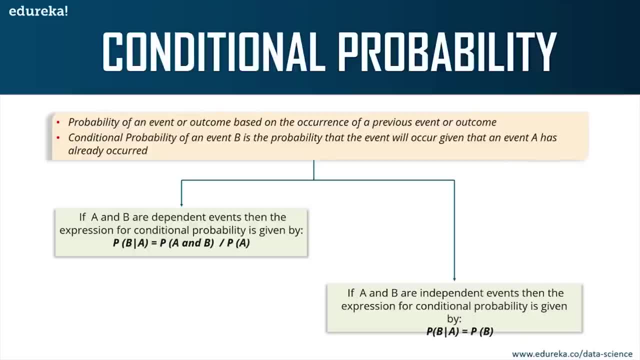 given that an event, A, has already occurred, Right? So if A and B are dependent events, then the expression for conditional probability is given by this. Now, this first term on the left-hand side, which is P, B of A is basically the probability. 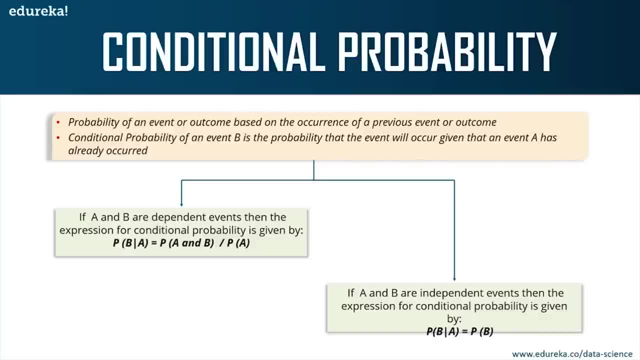 of event B occurring, given that event A has already occurred. All right, So, like I said, if A and B are dependent events, then this is the expression, But if A and B are independent events, then the expression for conditional probability is like this: 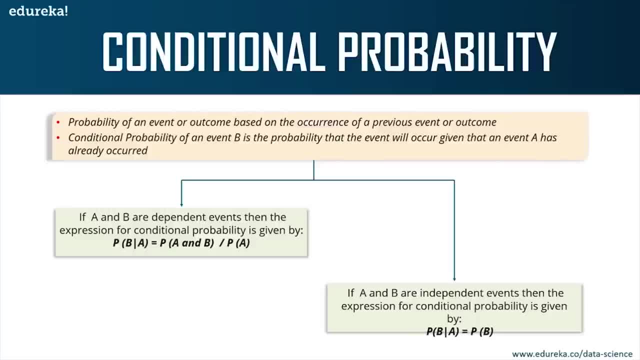 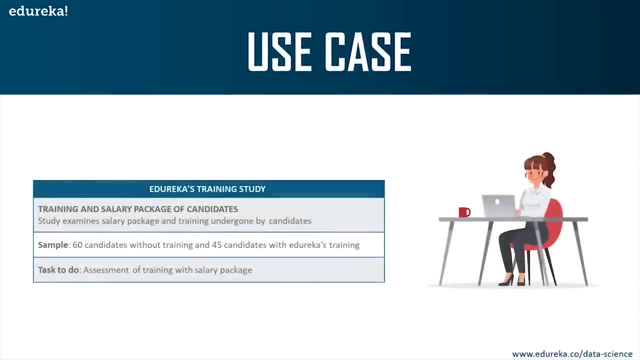 Right. So, guys, P of A and P of B is obviously the probability of A and probability of B, Right Now. let's move on. Now, in order to understand conditional probability, joint probability and marginal probability, let's look at a small use case. 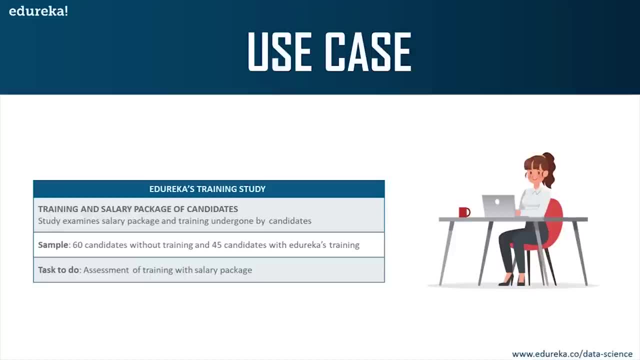 Okay, Now, basically, we're gonna take a data set which examines the salary package and training undergone by candidates. Okay now, in this there are 60 candidates without training and 45 candidates which have enrolled for Edureka's training Right Now. the task here is you have to assess the training. 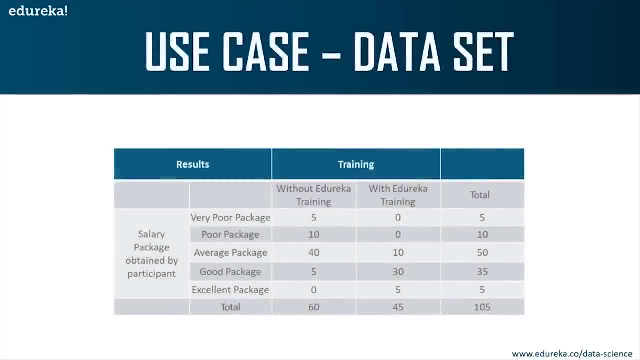 with a salary package. Okay, Let's look at this in a little more depth. So in total, we have 105 candidates, out of which 60 of them have not enrolled for Edureka's training and 45 of them have enrolled for Edureka's training. 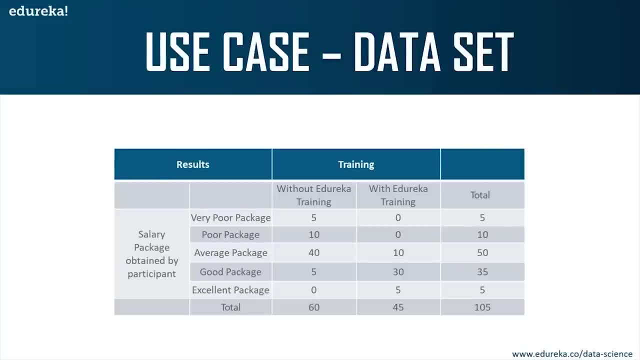 All right, This is a small survey that was conducted and this is the rating of the package or the salary that they got Right. So if you read through the data, you can understand. There were five candidates without Edureka training who got a very poor salary package. 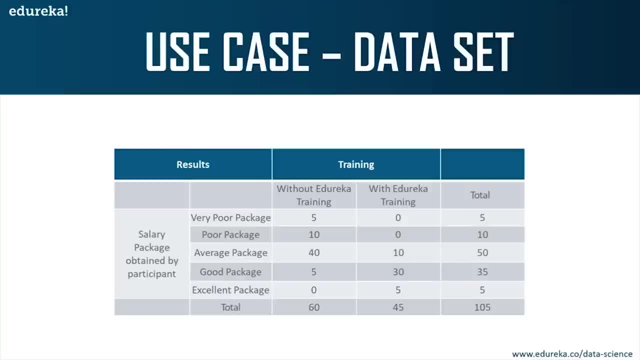 Okay, So basically there are 30 candidates with Edureka training who got a good package, Right? So, guys, basically you're comparing the salary package of a person depending on whether or not they've enrolled for Edureka training, Right? This is our data set. 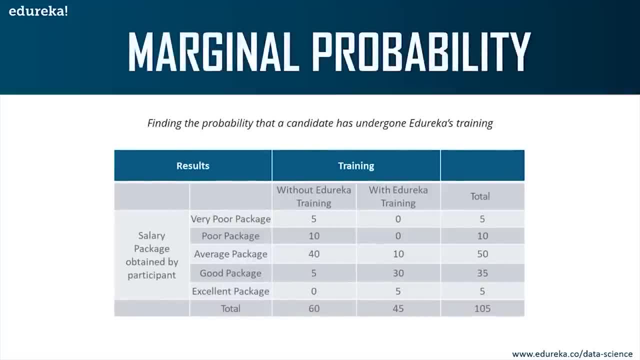 Now let's look at our problem statement. Find the probability that a candidate has undergone Edureka's training Quite simple. Which type of probability is this? This is marginal probability, Right? So the probability that a candidate has undergone Edureka's training. 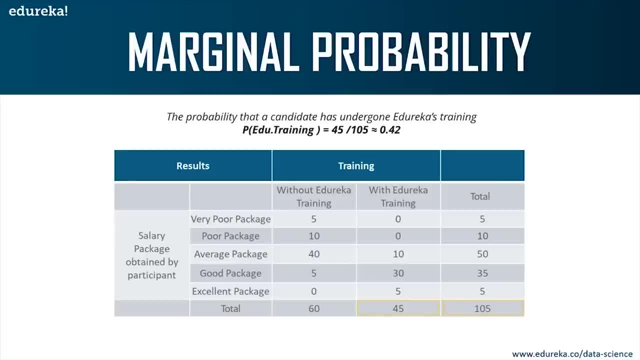 is obviously 45 divided by 105. Since 45 is the number of candidates with Edureka training and 105 is the total number of candidates, So you get a value of approximately 0.42.. All right, That's the probability of a candidate. 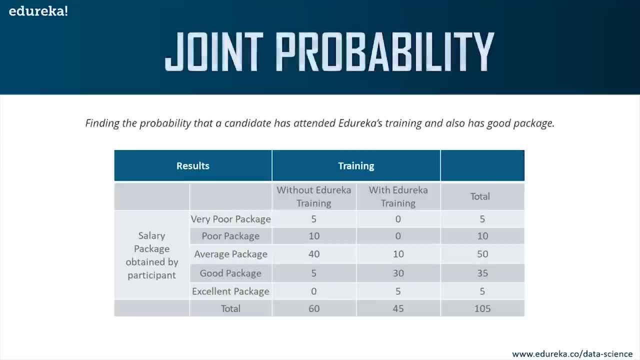 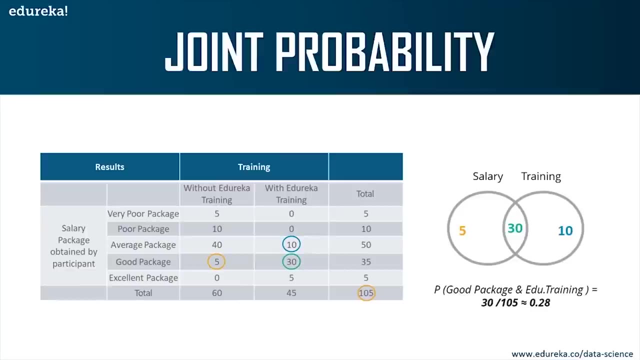 that has undergone Edureka's training. Next question: Find the probability that a candidate has attended Edureka's training and also has good package. Now, this is obviously a joint probability problem, Right? So how do you calculate this Now, since our table is quite formatted? 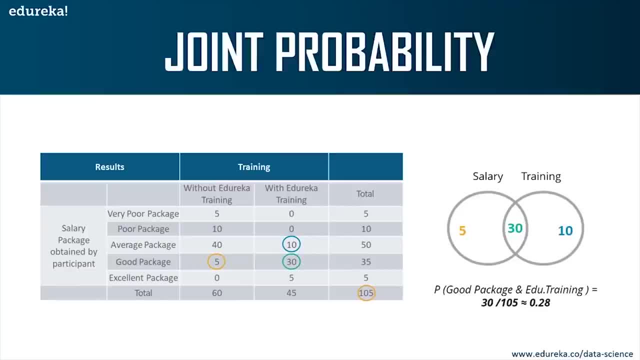 we can directly find that people who have gotten a good package along with Edureka training are 30. Right, So out of 105 people, 30 people have Edureka training and a good package. Right, They're specifically asking for people with Edureka training. 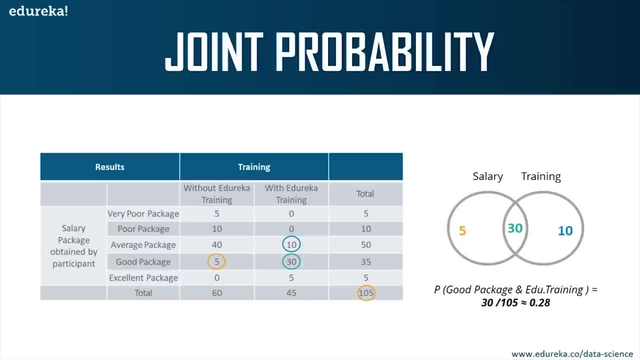 Remember that Right. The question is: find the probability that a candidate has attended Edureka's training and also has a good package, All right. So you need to consider two factors, That is, a candidate who's attended Edureka's training and who has a good package. 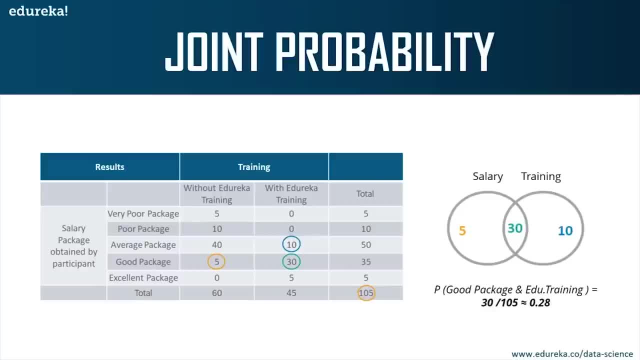 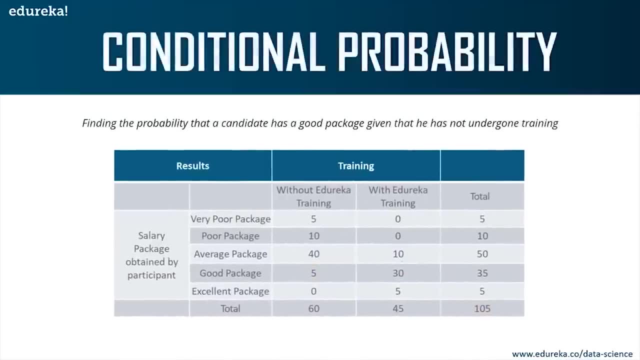 So, clearly, that number is 30.. 30 divided by total number of candidates, which is 105.. Right, So here you get the answer clearly. Next, we have find the probability that a candidate has a good package, given that he has not undergone training. 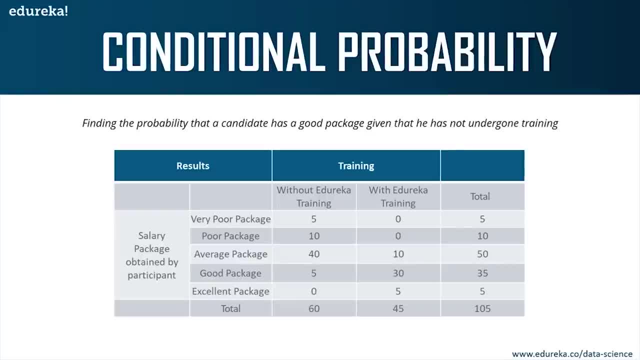 Okay. Now this is clearly conditional probability, because here you're defining a condition. You're saying that you want to find the probability of a candidate who has a good package given that he's not undergone any training. Right, The condition is that he's not undergone any training. 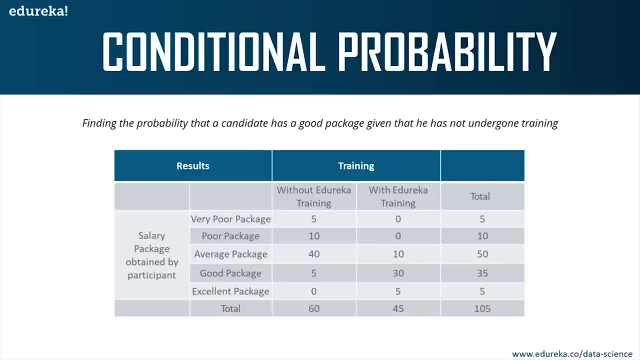 All right. So the number of people who have not undergone training are 60, and out of that, five of them have got a good package Right. So that's why this is five by 60 and not five by 105, because here they've clearly mentioned has a good package. 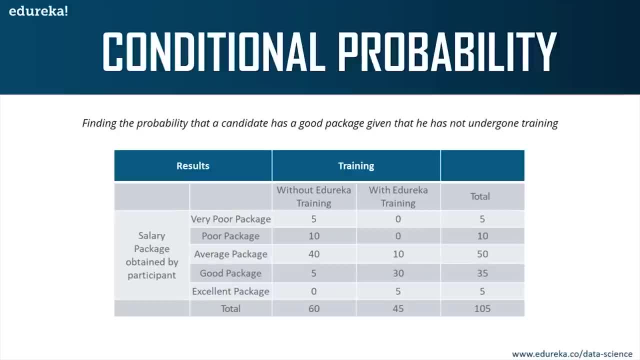 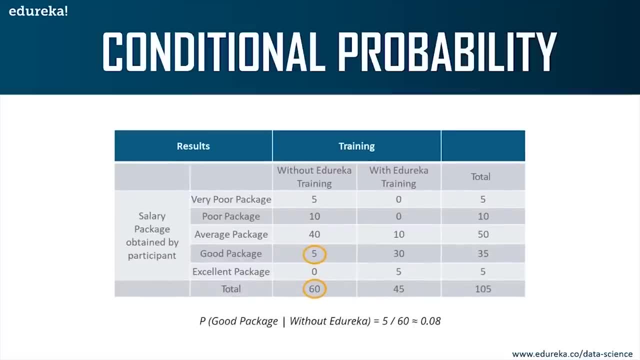 given that he has not undergone training. So you have to only consider people who have not undergone training, Right? So only five people who have not undergone training have gotten a good package, Right? So five divided by 60, you get a probability of around 0.08,. 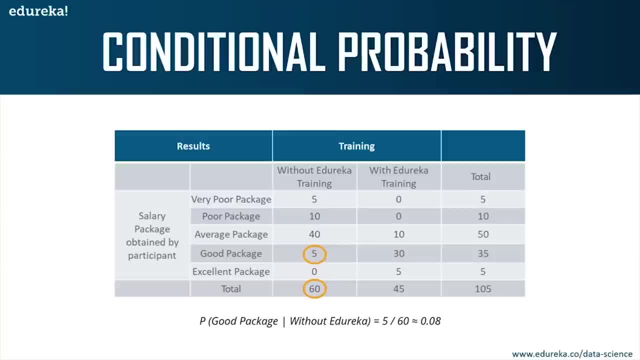 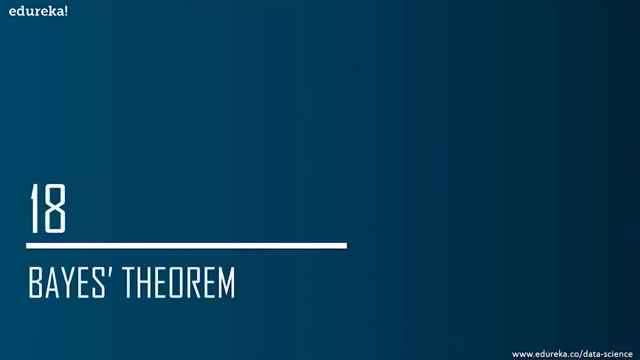 which is pretty low, Right? Okay, So this was all about the different types of probability. Now let's move on and look at our last topic in probability, which is Bayes' theorem. Now, guys, Bayes' theorem is a very important concept. 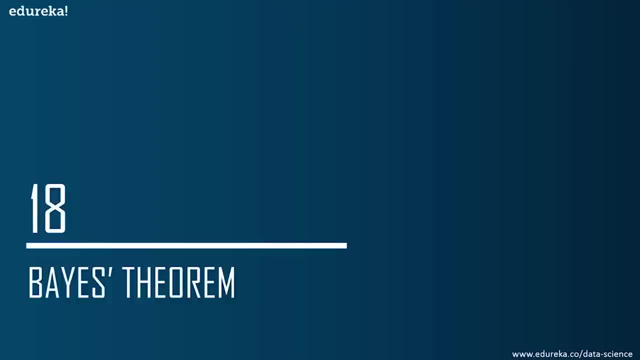 When it comes to statistics and probability. it is majorly used in naive bias algorithm. Those of you who aren't aware, naive bias is a supervised learning classification algorithm and it is mainly used in Gmail spam filtering Right. A lot of you might have noticed that if you open up Gmail, 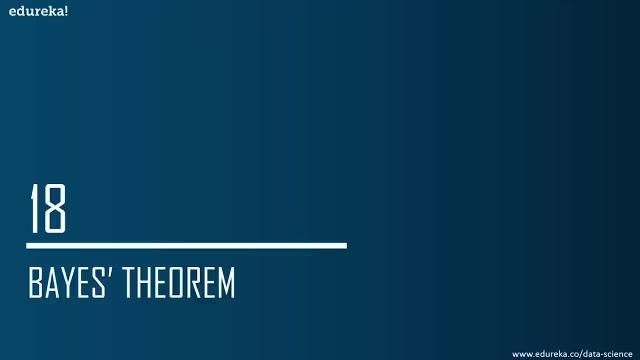 you'll see that you have a folder called spam, Right. All of that is carried out through machine learning, and the algorithm used there is naive bias, Right? So now let's discuss what exactly the Bayes' theorem is and what it denotes. 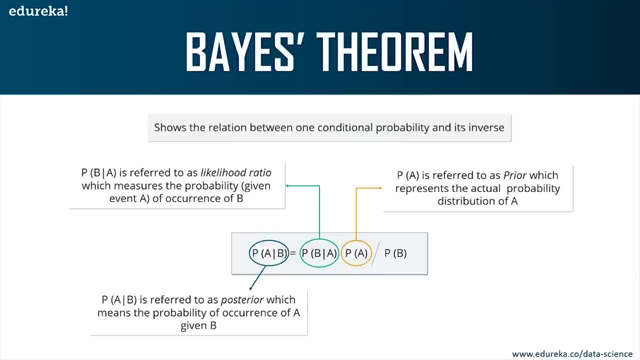 The Bayes' theorem is used to show the relation between one conditional probability and its inverse. All right, Basically it's nothing but the probability of an event occurring, based on prior knowledge of conditions that might be related to the same event. Okay, so mathematically, 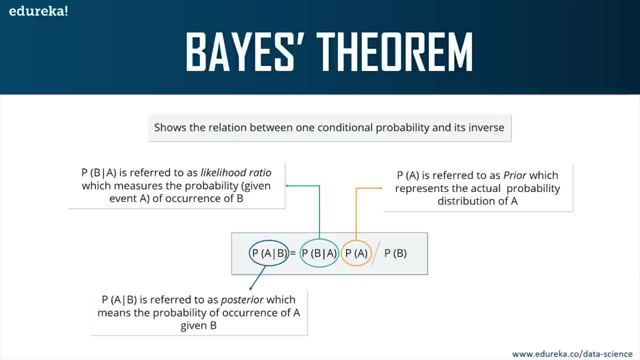 the Bayes' theorem is represented like this: Right, Like shown in this equation. The first term is referred to as the likelihood ratio, which measures the probability of occurrence of event B given an event A. Okay, On the left-hand side is what is known as the posterior. 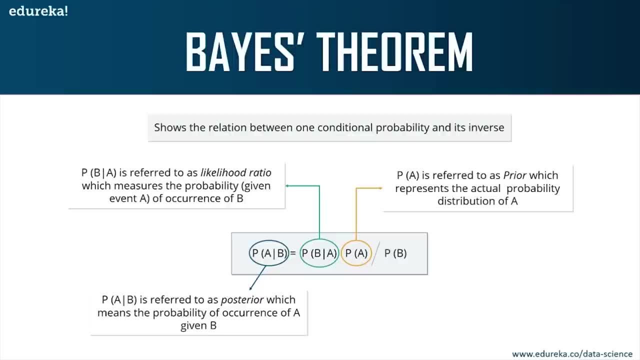 All right, It is referred to as posterior, which means that the probability of occurrence of A given an event B Right. The second term is referred to as the likelihood ratio. All right, This measures the probability of occurrence of B given an event A. 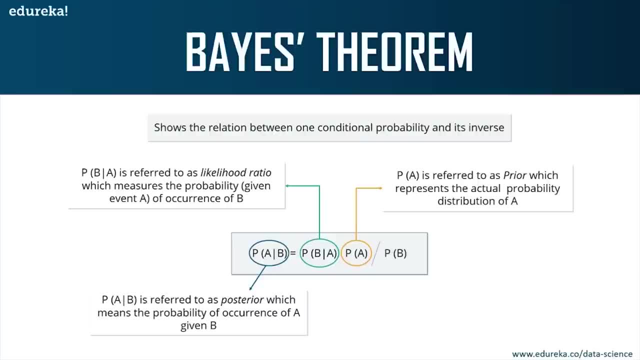 Now P of A is also known as the probability ratio, which refers to the actual probability distribution of A, and P of B is again the probability of B Right. This is the Bayes' theorem. Now, in order to better understand the Bayes' theorem, 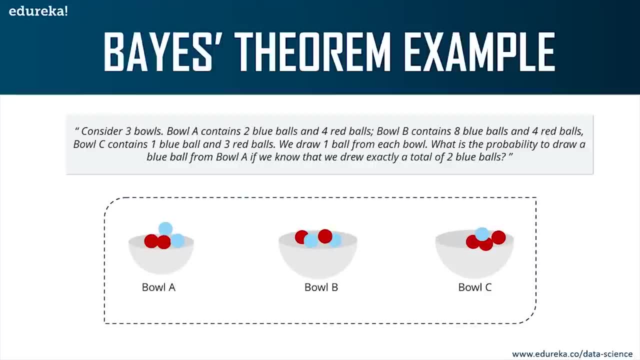 let's look at a small example. Let's say that we have three bowels. We have bowel A, bowel B and bowel C. Okay, bowel A contains two blue balls and four red balls. Bowel B contains eight blue balls and four red balls. 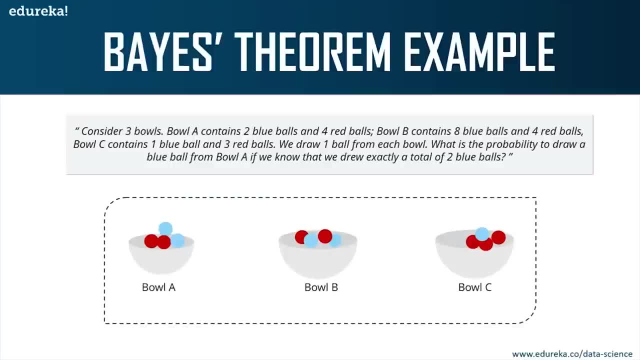 Bowel C contains one blue ball and three red balls. Now, if we draw one ball from each bowel, what is the probability to draw a blue ball from a bowel A if we know that we drew exactly a total of two blue balls? Right? 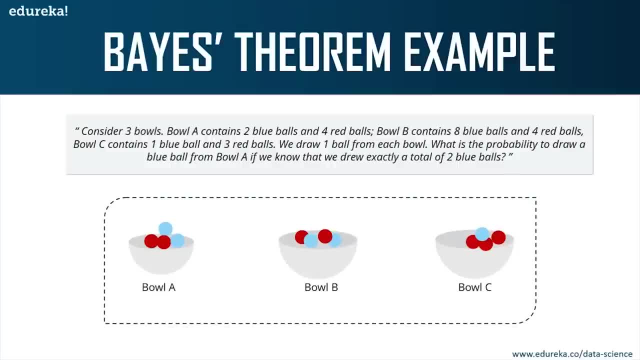 If you didn't understand the question, please re-read it. I shall pause for a second or two, Right? So I hope all of you have understood the question. Okay, now, what I'm gonna do is I'm gonna draw a blueprint for you. 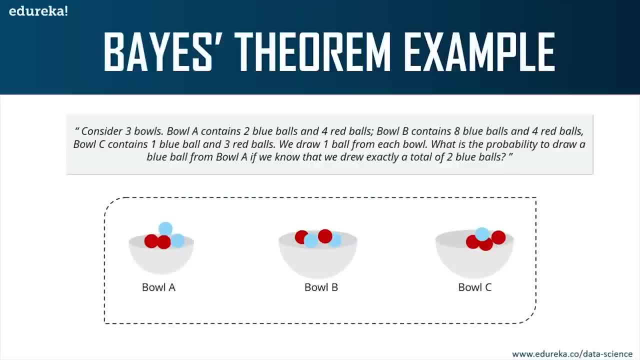 and tell you how exactly to solve the problem. So I'm gonna draw a blueprint for you. I'm gonna tell you how exactly to solve the problem, but I want you all to give me the solution to this problem. Right, I'll draw a blueprint. 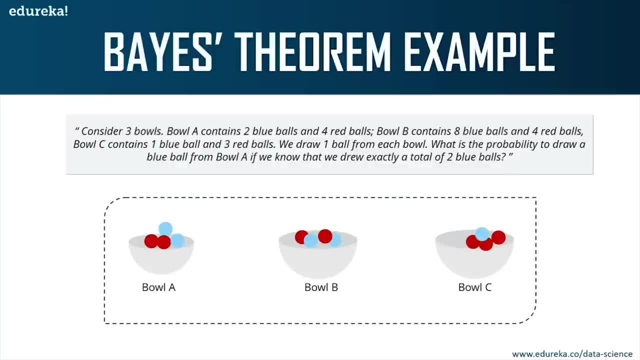 I'll tell you what exactly the steps are, but I want you to come up with a solution on your own Right. The formula is also given to you. Everything is given to you. All you have to do is come up with a final answer. 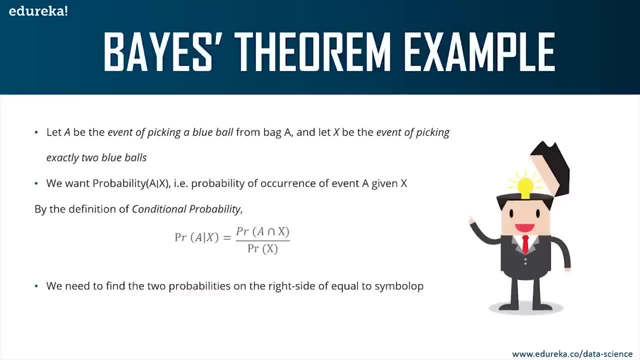 Right, Let's look at how you can solve this problem. So, first of all, what we'll do is: let's consider A. All right, let A be the event of picking a blue ball from bag A, And let X be the event of picking exactly two blue balls. 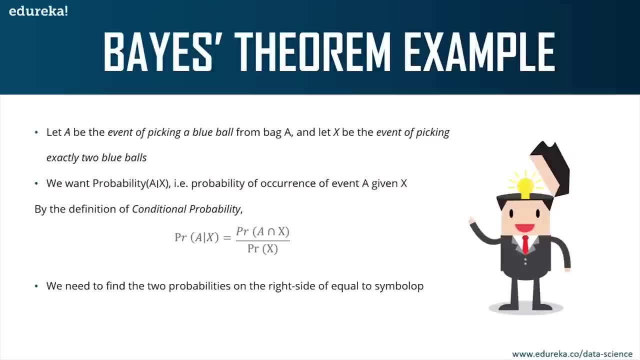 Right, Because these are the two events that we need to calculate the probability of Now. there are two probabilities that you need to consider here. One is the event of picking a blue ball from bag A, And the other is the event of picking exactly two blue balls. 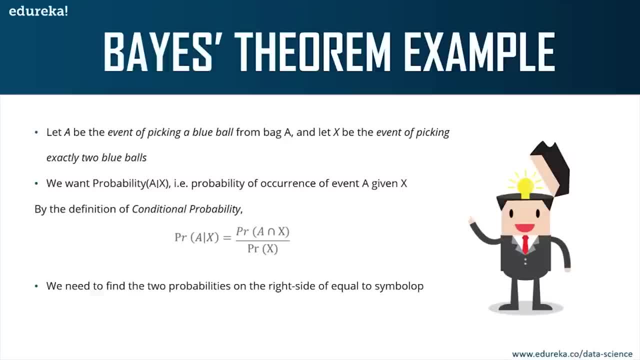 Okay, So these two are represented by A and X respectively. So what we want is the probability of occurrence of event A given X, Which means that, given that we're picking exactly two blue balls, what is the probability that we are picking? 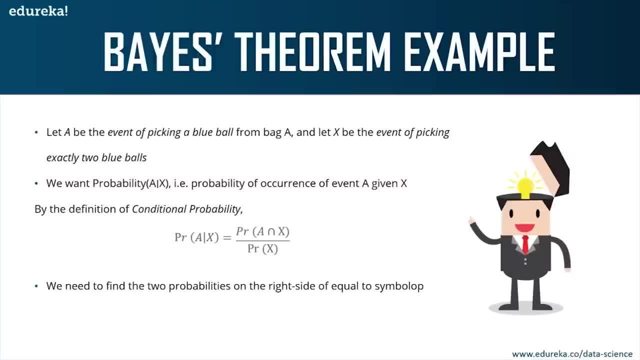 a blue ball from bag A. So, by the definition of conditional probability, this is exactly what our equation will look like, Correct. This is basically occurrence of event A given an event X, And this is the probability of A and X, And this is the probability of X alone. 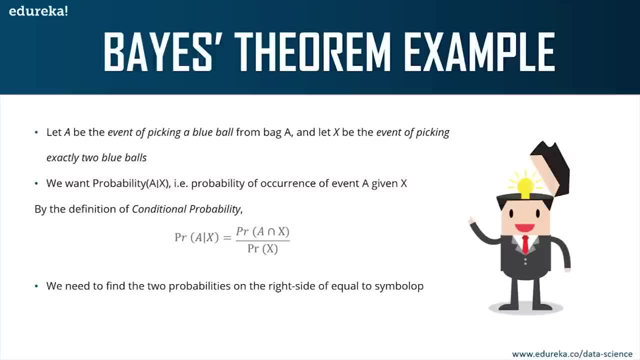 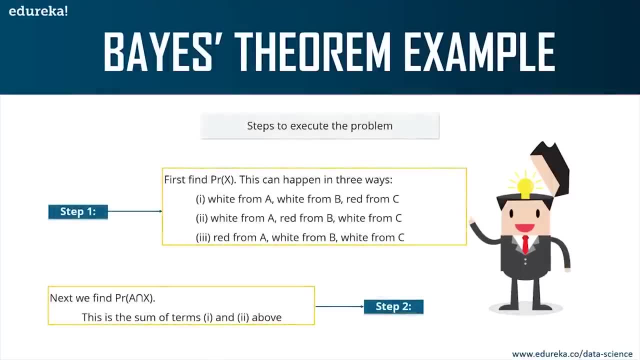 Correct. Now what we need to do is we need to find these two probabilities, which is probability of A and X occurring together and probability of X. Okay, This is the entire solution. So how do you find the probability of X? 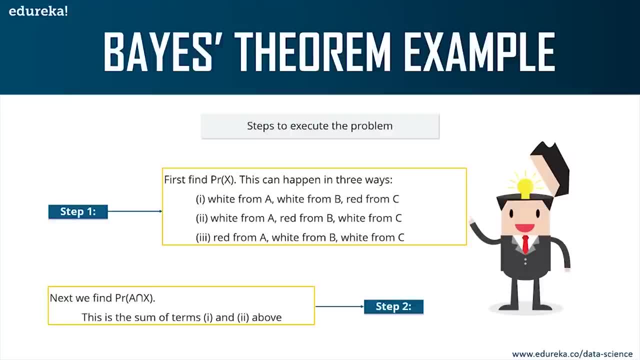 This you can do in three ways. So first is white ball from A, either white from B or red from C. Now, first is to find the probability of X. X basically represents the event of picking exactly two blue balls, Right. 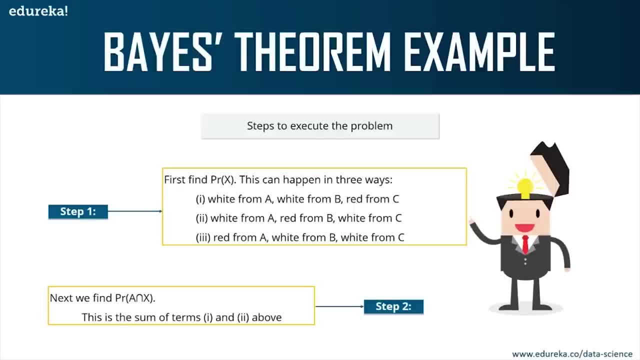 So these are the three ways in which it is possible. So you'll pick one blue ball from bowl A and one from bowl B. In the second case, you can pick one from A and another blue ball from C. In the third case, you can pick a blue ball from bag B. 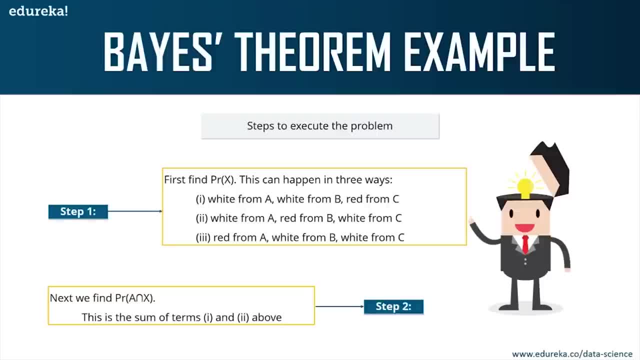 and a blue ball from bag C Right. These are the three ways in which it is possible, So you need to find the probability of each of this. Step two is that you need to find the probability of A and X occurring together. 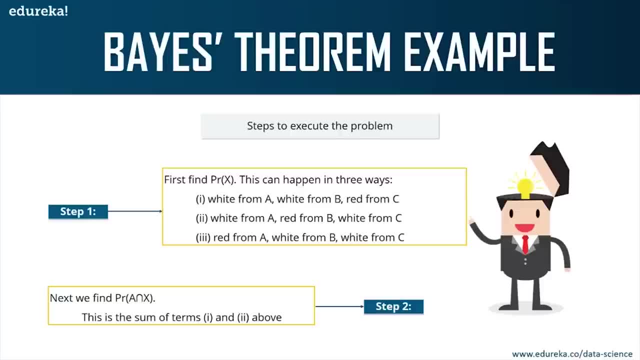 This is the sum of terms one and two. Okay, This is because in both of these events you're picking a ball from bag A, Correct? So, guys, find out this probability and let me know your answer in the comment section. 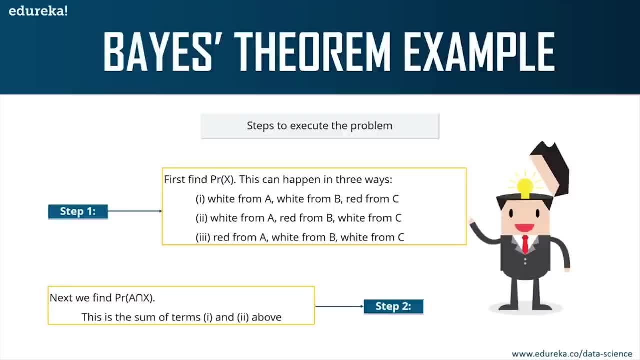 All right, We'll see if you get the answer right. I gave you the entire solution to this. All you have to do is substitute the value Right. If you want a second or two, I'm going to pause on the screen so that you can go through this in a more clearer way. 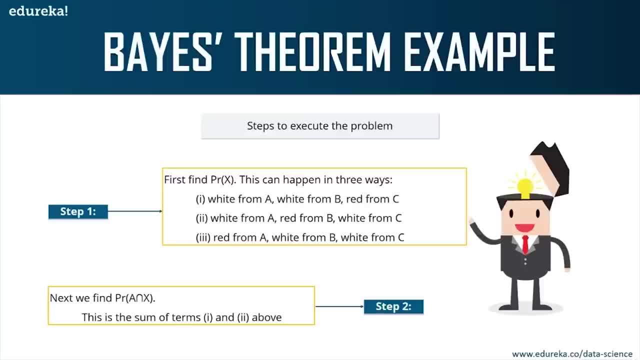 Right, Remember that you need to calculate two probabilities. The first probability that you need to calculate is the event of picking a blue ball from bag A. given that you're picking exactly two blue balls, Okay. The second probability you need to calculate is the event of picking exactly two blue balls. 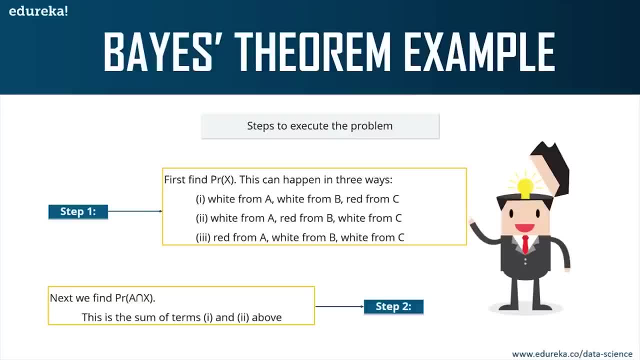 All right, These are the two probabilities you need to calculate. So remember that And this is the solution, All right. So, guys, make sure you mention your answers in the comment section. For now, let's move on and look at our next topic. 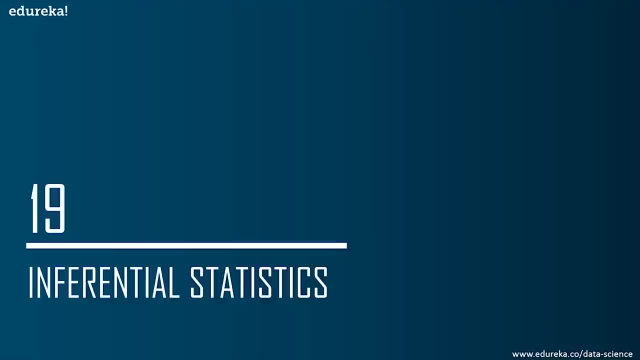 which is the inferential statistics. So, guys, we just completed the probability module. Right Now we'll discuss inferential statistics, which is the second type of statistics. We discussed descriptive statistics earlier, All right, So, like I mentioned earlier, 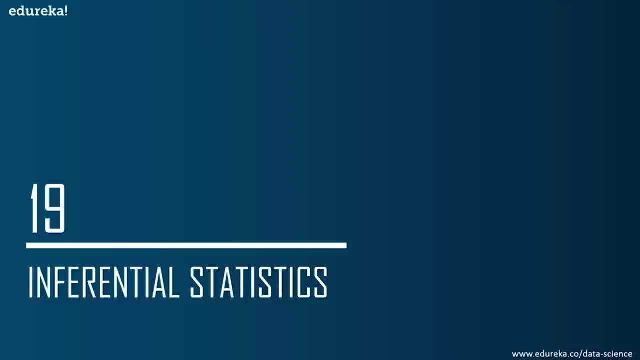 inferential statistics, also known as statistical inference, is a branch of statistics that deals with forming inferences and predictions about a population based on a sample of data taken from the population. All right, And the question you should ask is: how does one form inferences or predictions on a sample? 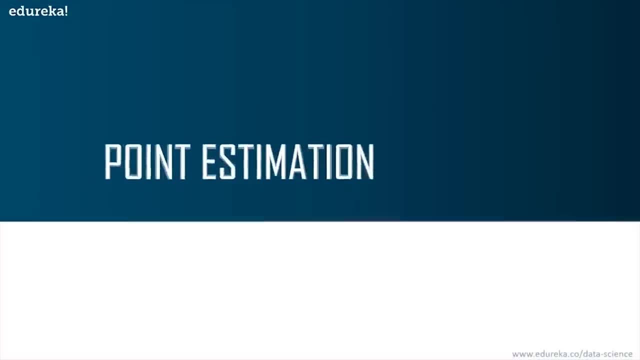 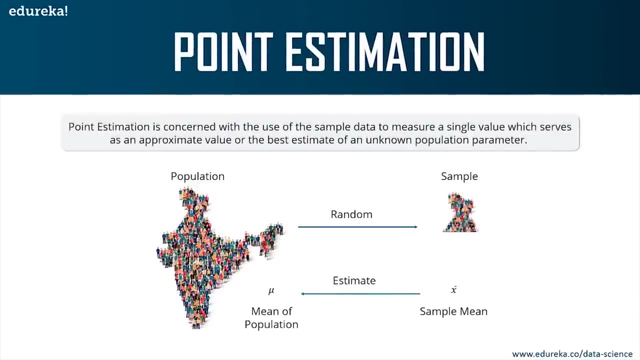 The answer is you use point estimation. Okay, now you must be wondering: what is point estimation? Point estimation is concerned with the use of the sample data to measure a single value which serves as an approximate value or the best estimate of an unknown population parameter. 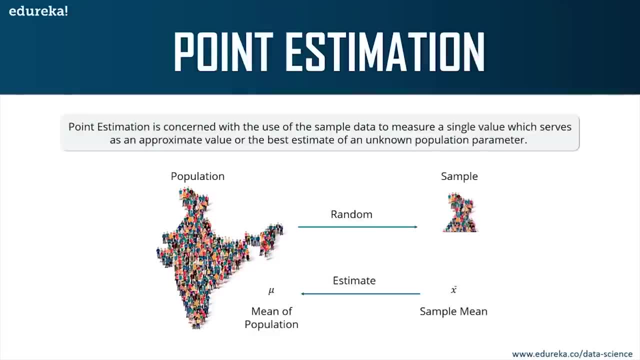 That's a little confusing. Let me break it down to you. For example, in order to calculate the mean of a huge population, what we do is we first draw out the sample of the population, Okay, and then we find the sample mean right. 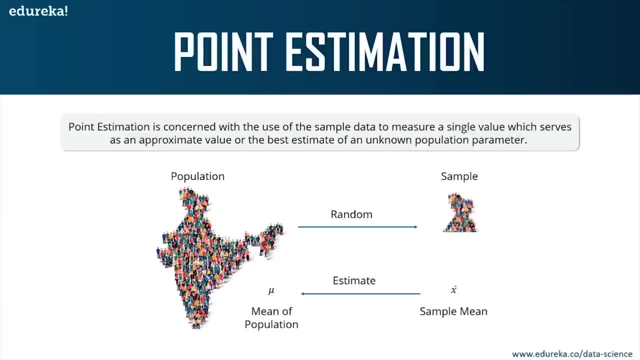 The sample mean is then used to estimate the population mean. This is basically point estimate. You're estimating the value of one of the parameters of the population, right, Basically the mean. you're trying to estimate the value of the mean. This is what point estimation is. 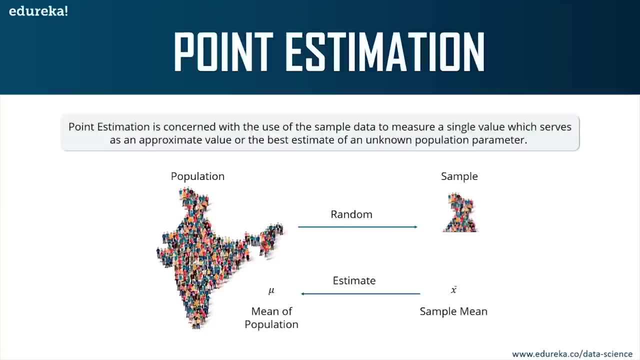 The two main terms in point: estimation. there's something known as the estimator and there's something known as the estimate. Estimator is a function of the sample that is used to find out the estimate. In this example, it's basically the sample mean right. 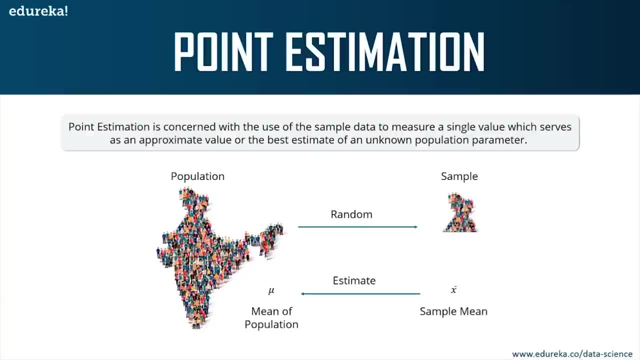 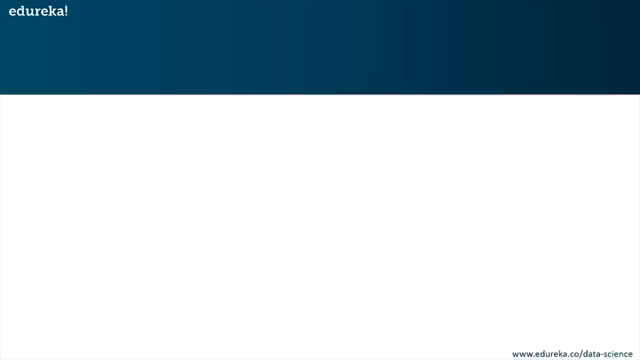 So a function that calculates the sample mean is known as the estimator, and the realized value of the estimator is the estimate. So I hope point estimation is clear. Now, how do you find the estimates? There are four common ways in which you can do this. 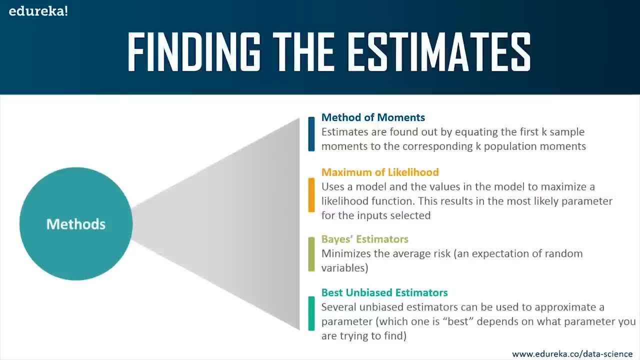 The first one is method of moments. Here what you do is you form an equation in the sample data set and then you analyze a similar equation in the population data set, Like the population mean, population variance and so on. So, in simple terms, what you're doing is: 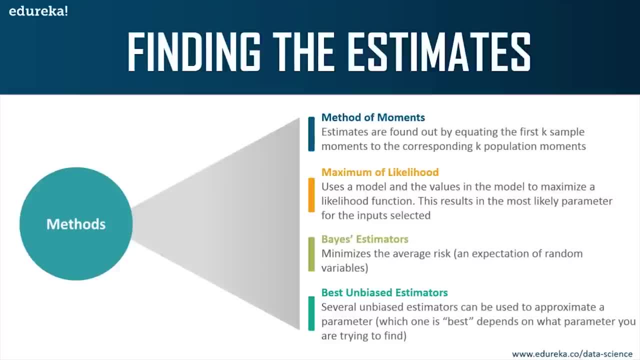 you're taking down some known facts about the population and you're extending those ideas to the sample. all right, Once you do that, you can analyze the sample and estimate more essential or more complex values right. Next we have maximum of likelihood. 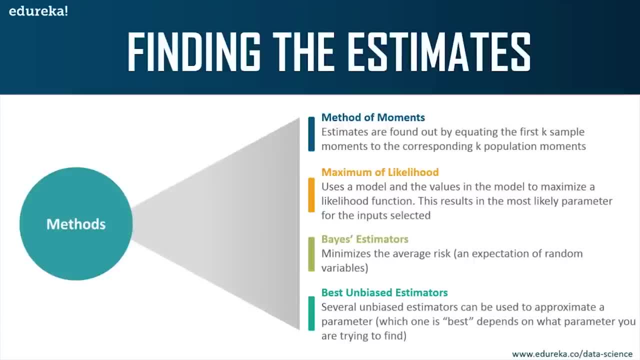 Now, this method basically uses a model to estimate a value. all right, Now, maximum of likelihood is a major based on probability, so there's a lot of probability involved in this method. Next, we have the base estimator. This works by minimizing the errors or the average risk. okay, 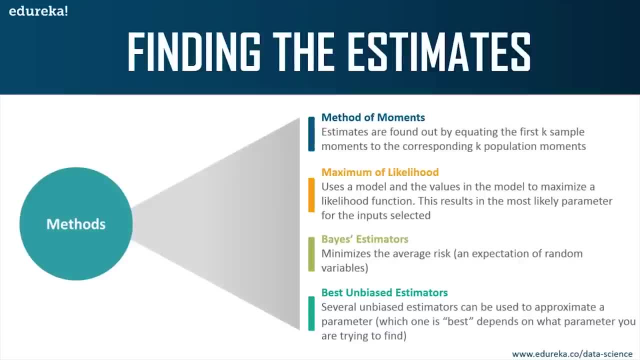 The base estimator has a lot to do with the Bayes Theorem. All right, let's not get into the depth of these estimation methods. Finally, we have the best unbiased estimators. In this method. there are several unbiased estimators that can be used to approximate a parameter. okay, 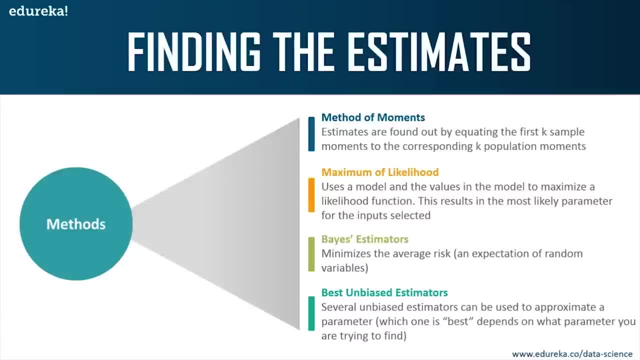 So, guys, these were a couple of methods that are used to find the estimate, but the most well-known method to find the estimate is known as the interval estimation. okay, This is one of the most important estimation methods. all right, this is where confidence interval. 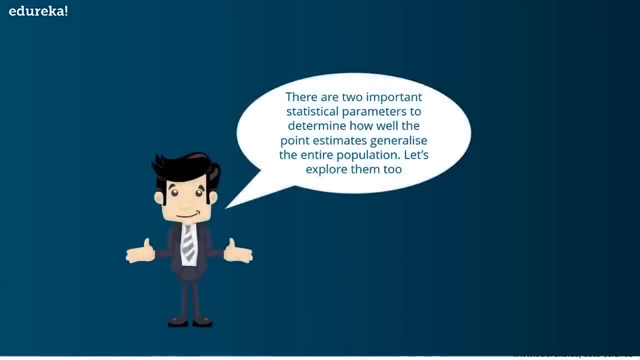 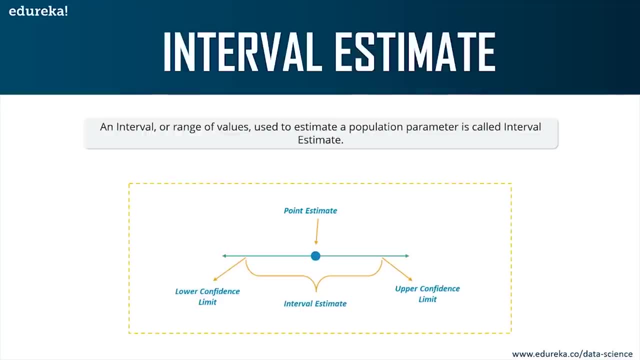 also comes into the picture. right Apart from interval estimation, we also have something known as margin of error. So I'll be discussing all of this in the upcoming slides. So first let's understand what is interval estimate? okay, An interval or range of values. 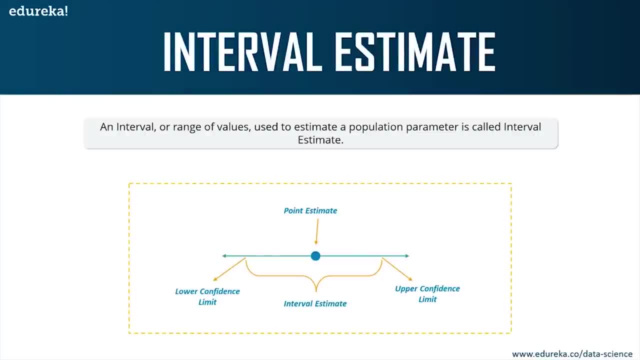 which are used to estimate a population parameter is known as an interval estimation. right, That's very understandable. Basically, what they're trying to say is: you're going to estimate the value of a parameter. let's say you're trying to find the mean of a population. 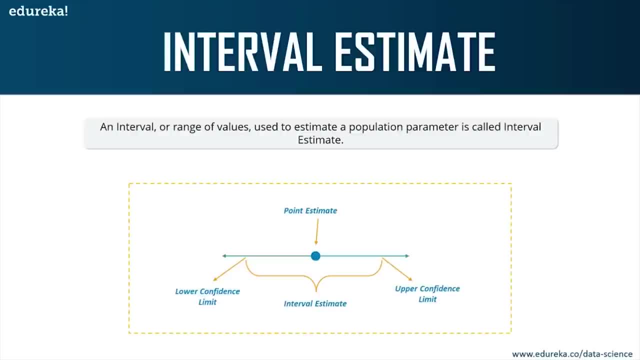 What you're going to do is you're going to build a range and your value will lie in that range or in that interval. All right, so this way your output is gonna be more accurate, because you've not predicted a point estimation. Instead, you have. 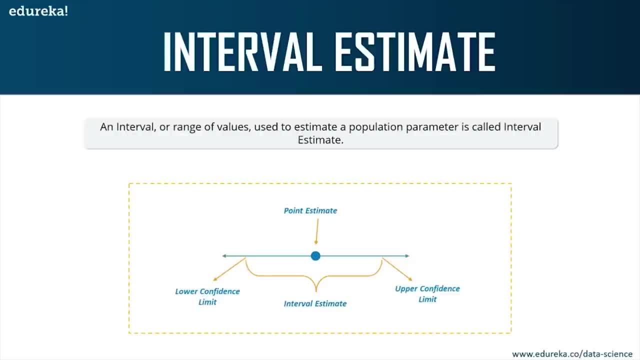 estimated an interval within which your value might occur. right, Okay, now this image clearly shows how point estimate and interval estimate are different. So, as interval estimate is obviously more accurate because you're not just focusing on a particular value or a particular point in order to predict the probability, 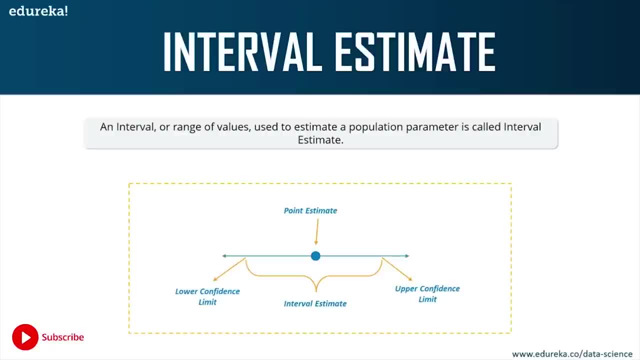 Instead, you're seeing that the value might be within this range between the lower confidence limit and the upper confidence limit. All right, this just denotes the range or the interval. Okay, if you're still confused about interval estimation, let me give you a small example. 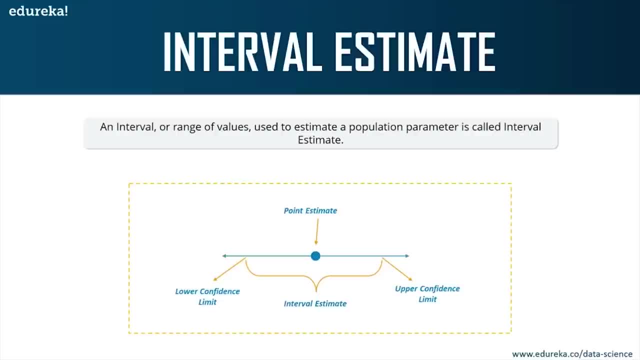 If I stated that I will take 30 minutes to reach the theater- this is known as point estimation- okay, But if I stated that I will take between 45 minutes to an hour to reach the theater, this is an example of interval estimation. 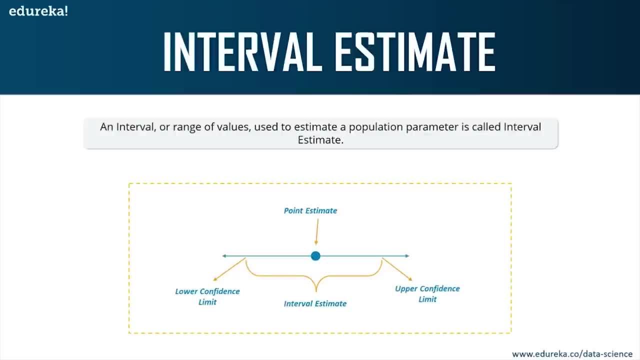 All right, I hope it's clear now. Now, interval estimation gives rise to two important statistical terminologies. One is known as confidence interval and the other is known as margin of error. all right, So, guys, it's important that you pay attention. 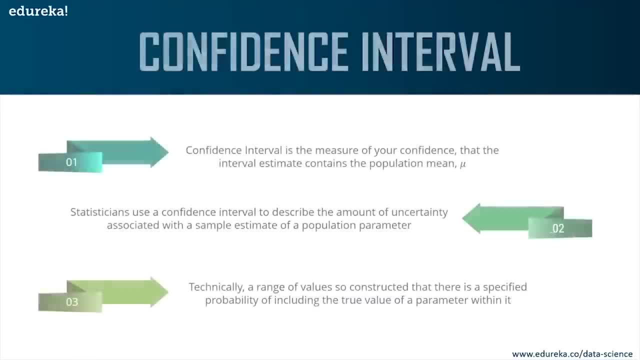 to both of these terminologies. Confidence interval is one of the most significant measures that are used to check how essential a machine learning model is. all right, So what is confidence interval? Confidence interval is the measure of your confidence that the interval estimated contains. 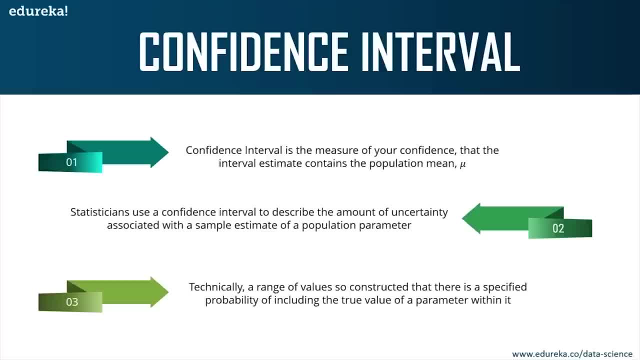 the population parameter or the population mean or any of those parameters. right Now, statisticians use confidence interval to describe the amount of uncertainty associated with a sample estimate of a population parameter. Now, guys, this is a lot of definition. Let me just make you understand confidence interval. 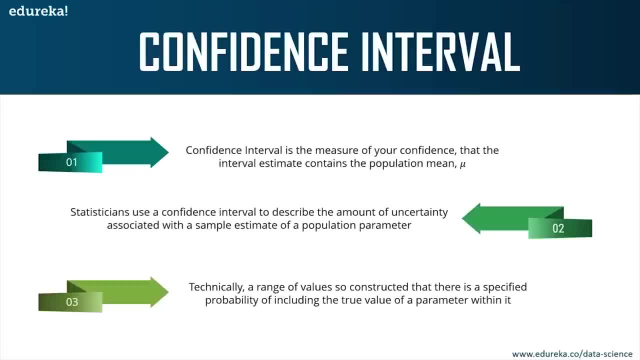 with a small example. Okay, let's say that you perform a survey and you survey a group of cat owners to see how many cans of cat food they purchase in one year. Okay, you test your statistics at the 99% of cat food. 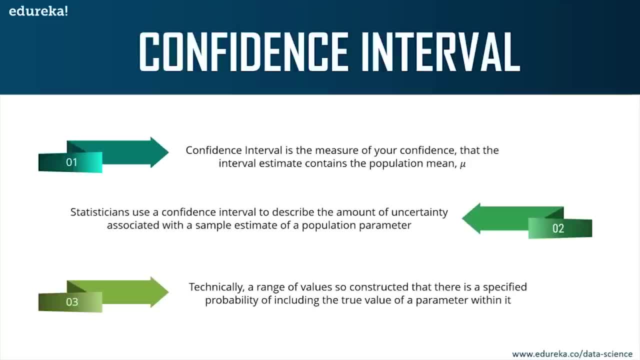 confidence level and you get a confidence interval of 100 comma 200. this means that you think that the cat owners buy between 100 to 200 cans in a year and also, since the confidence level is 99 percent, it shows that you're very confident that the results are correct. okay, i hope all of you. 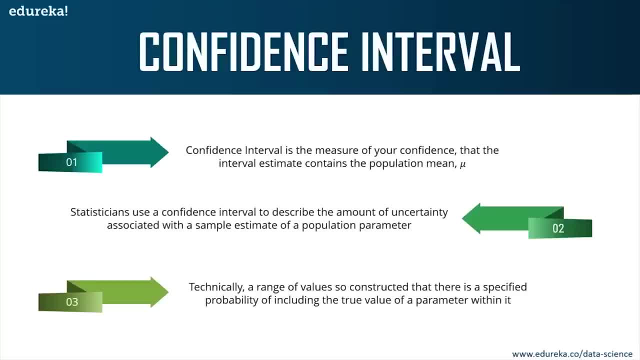 are clear with that right. so your confidence interval here will be 100 and 200 and your confidence level will be 99 percent, right? that's the difference between confidence interval and confidence level. so within your confidence interval your value is going to lie and your confidence level will show how confident you are about your estimation, right? i hope that was clear. 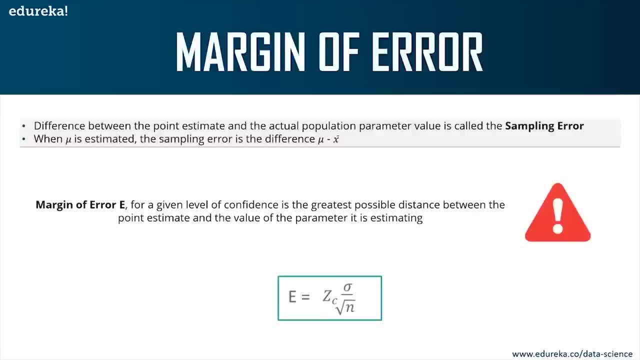 let's look at margin of error now. margin of error for a given level of confidence is the greatest possible distance between the point estimate and the value of the parameter that it is estimating. you can say that it is a deviation from the actual point estimate. right now the margin of error can be calculated. 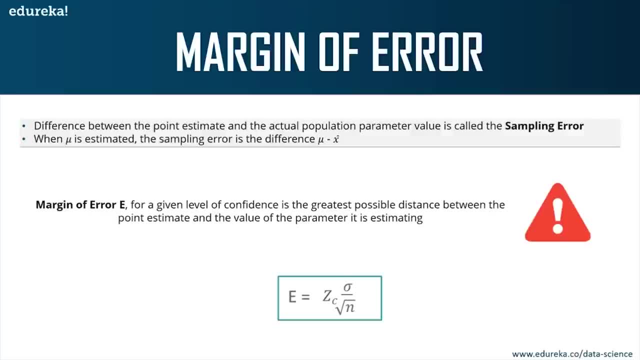 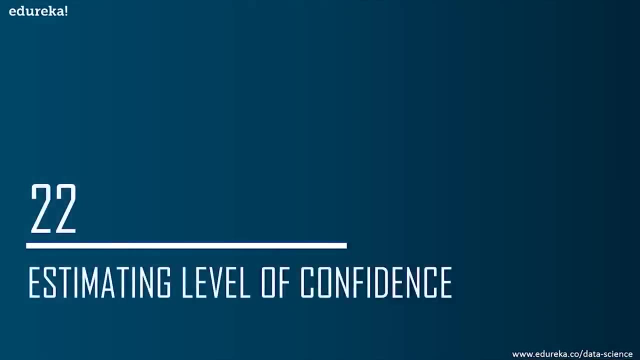 using this formula. now, zc here denotes the critical value or the confidence interval, and this is multiplied by standard deviation, divided by root of the sample size. all right, n is basically the sample size. now let's understand how you can estimate the confidence intervals. so, guys, the level of confidence which is denoted by c, 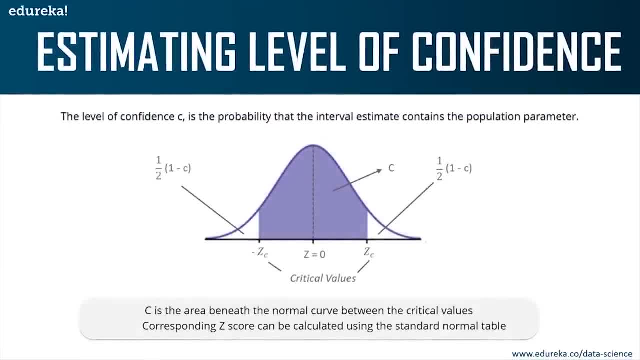 is the probability that the interval estimate contains the population parameter. let's say that you're trying to estimate the mean, all right. so the level of confidence is the probability that the interval estimate contains the population parameter. so this interval between minus zc and zc or the area beneath this, 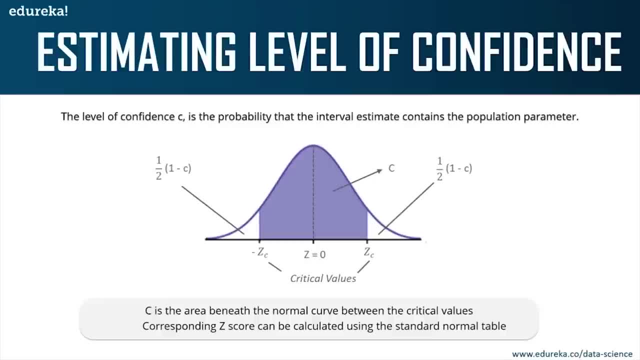 curve is nothing but the probability that the interval estimate contains the population parameter. all right, it should basically contain the value that you are predicting right now. these are known as critical values. this is basically your lower limit and your higher limit confidence level. also, there's something known as the z score. now this score can be: 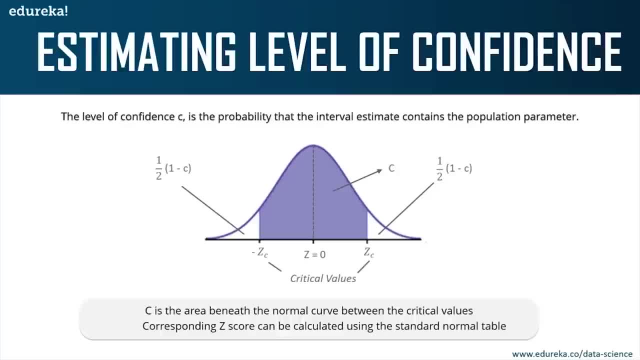 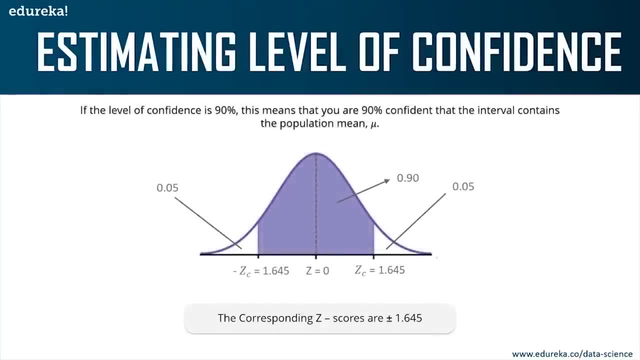 calculated by using the standard normal table. all right, if you look it up anywhere on google, you'll find the z score table or the standard normal table. again, to understand, uh, how this is done, let's look at a small example. okay, let's say that the level of confidence is. 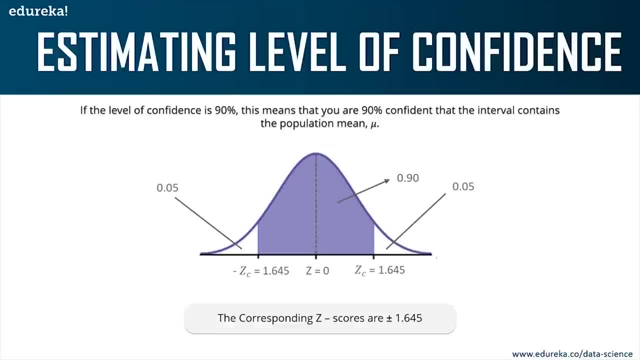 90, that you are 90 percent confident that the interval contains the population, mean, okay, so, uh, the remaining 10 percent, which is out of 100, the remaining 10 percent is equally distributed on these tail regions. okay, so you have 0.05 here and 0.05 over here, right? so on either side of c you'll. 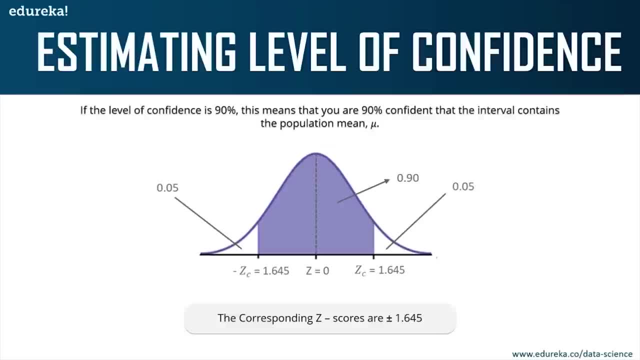 distribute the other left over percentage. now, these, these codes are calculated from the table, as i mentioned before. all right, 1.645 is calculated from the standard normal table. okay, so, guys, this is how you estimate the level of confidence. so, to sum it up, let me tell you the 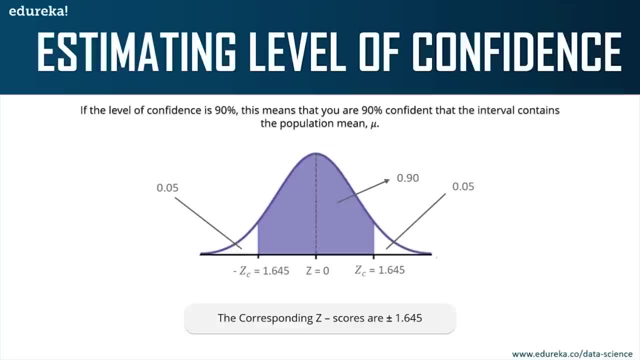 steps that are involved in constructing a confidence interval. first, you'll start by identifying a sample statistic. okay, this is the statistic that you will use to estimate a population parameter. this can be anything like the mean of the sample. next, you will select a confidence level. now the confidence level describes: 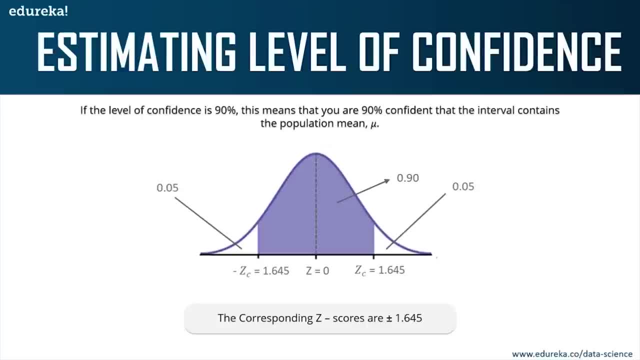 the uncertainty of a sampling method. right after that, you'll find something known as the margin of error. right? we discussed margin of error earlier, so you find this based on the equation that i explained in the previous slide. then you'll finally specify the confidence interval. all right, 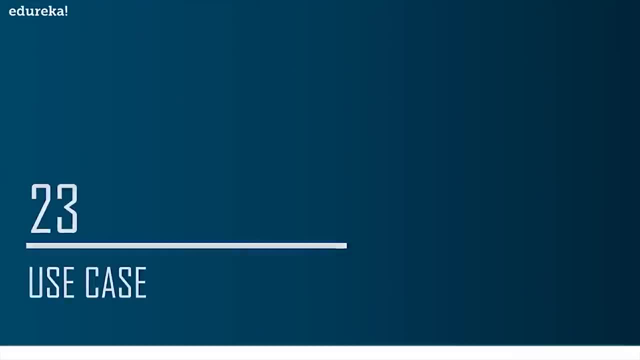 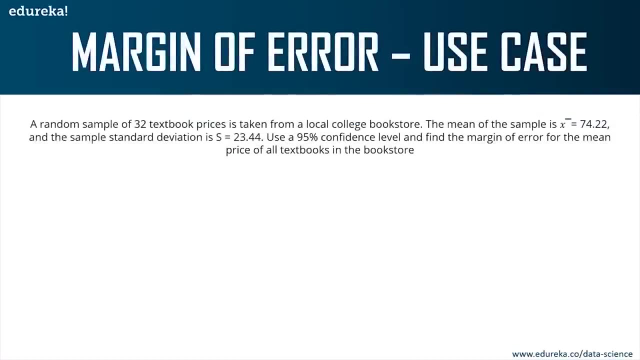 now let's look at a problem statement to better understand this concept. a random sample of 32 textbook prices is taken from a local college bookstore. the main of the sample is so, so and so, and the sample is the number of books that are sold, and the number of books that are sold is the. 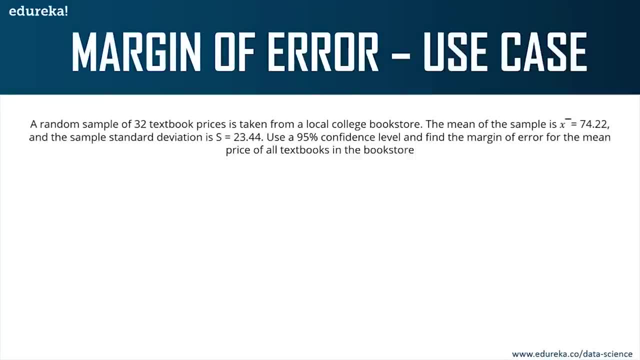 sample standard deviation is this: use a 95 confident level and find the margin of error for the mean price of all textbooks in the bookstore. okay now, this is a very straightforward question. if you want, you can read the question again. all you have to do is you have to just substitute the 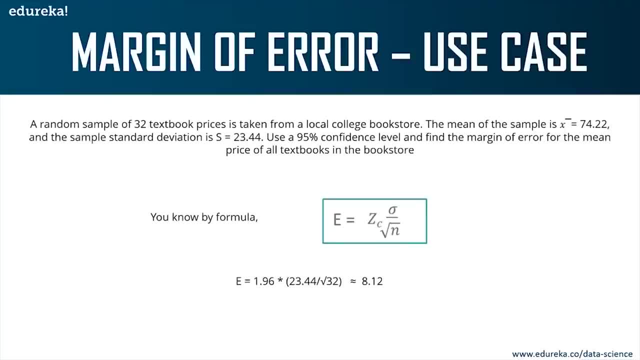 values into the equation. all right, so, guys, we know the formula for margin of error. you take the z score from the table. after that we have deviation, which is 23.44. right, and that's standard deviation. and n stands for the number of samples. here the number. 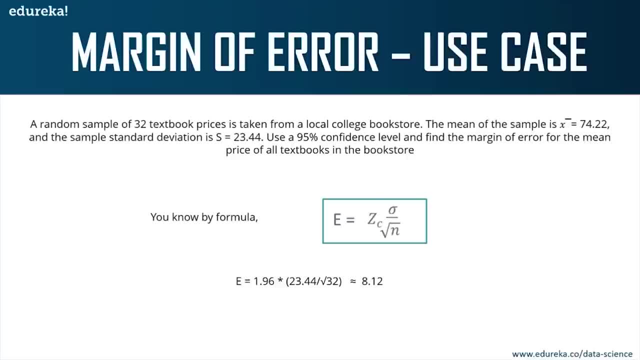 of samples is 32, basically 32 textbooks. so approximately your margin of error is going to be around 8.12. this is a pretty simple uh question. all right, i hope all of you understood this. now that you know the idea behind confidence interval, let's move ahead to one of the most. 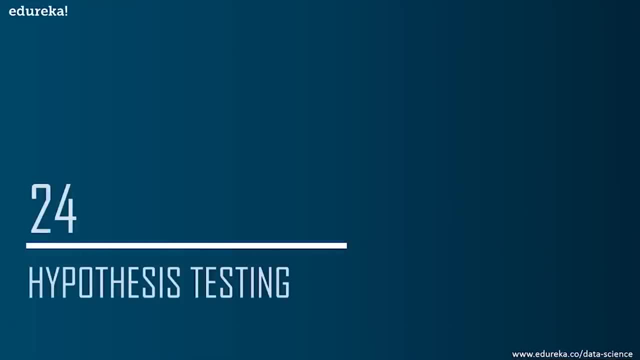 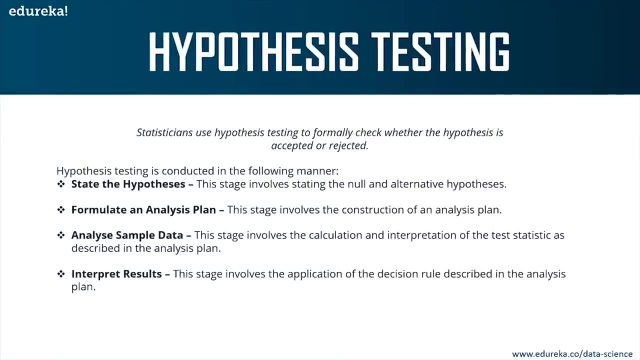 important topics in statistical inference, which is hypothesis testing, right? so basically, statisticians use hypothesis testing to formally check whether the hypothesis is accepted or rejected. okay, hypothesis testing is an inferential statistical technique used to determine whether there is enough evidence in a data sample to infer that a certain condition 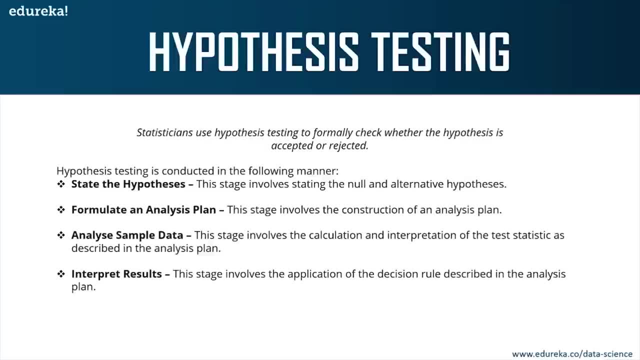 holds true for an entire population. so to understand the characteristics of a general population, we take a random sample and we analyze the properties of the data of the sample right, we test whether or not the identified conclusion represents the population accurately and finally we interpret their results. now, whether or not to accept the hypothesis depends 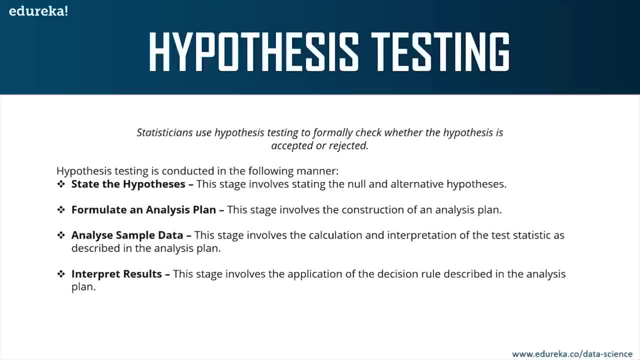 upon the percentage value that we get from the hypothesis. okay, so to better understand this, let's look at a small example. before that, there are a few steps that are followed in hypothesis testing. you begin by stating the null and the alternative hypothesis. all right, i'll tell you what exactly. 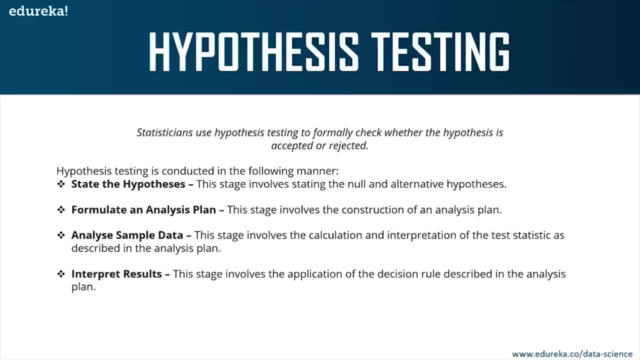 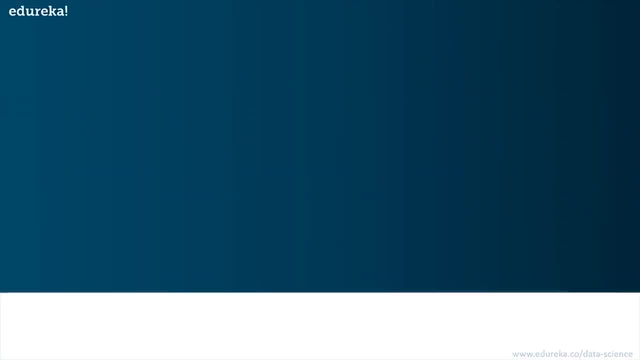 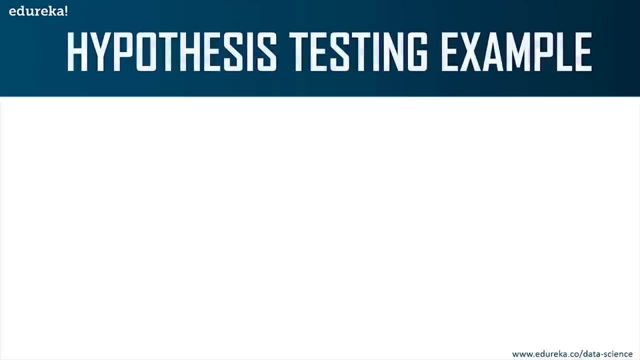 these terms are, and then you formulate an analysis plan, all right. after that you analyze the sample data and finally you can interpret the results right now to understand the entire hypothesis testing, we'll look at a good example. okay, now consider four boys: nick, john, bob and harry. 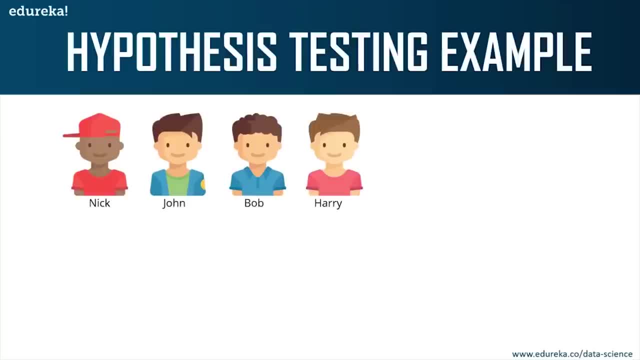 these boys were caught bunking a class and they were asked to stay back at school and clean their classroom as a punishment. right, so what john did is? he said that irico had come to hear you. right, So what John did is he decided that four of them would take turns to clean their classrooms. 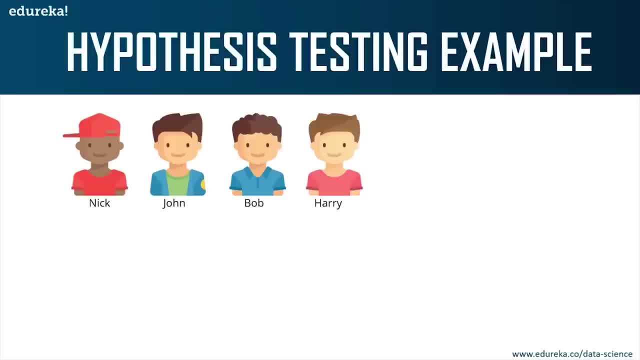 He came up with a plan of writing each of their names on chits and putting them in a bowl. Now, every day they had to pick up a name from the bowl and that person had to clean the class. right, That sounds pretty fair enough. Now it has been three days and everybody's name has come up. 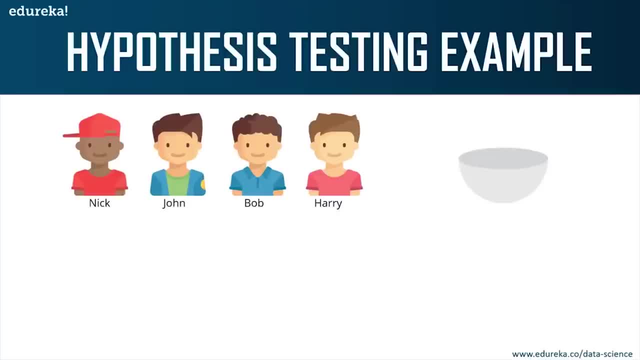 except John's. Assuming that this event is completely random and free of bias, what is the probability of John not cheating, right? What is the probability that he's not actually cheating? This can be solved by using hypothesis testing. okay, So we'll begin by calculating the probability. 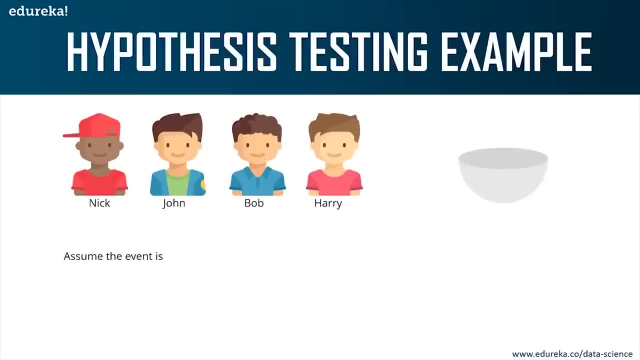 of John not being picked for a day right. So we're going to assume that the event is free of bias. So we need to find out the probability of John not cheating right First. we'll find the probability that John is not picked for a day right. We get three out of four, which is basically: 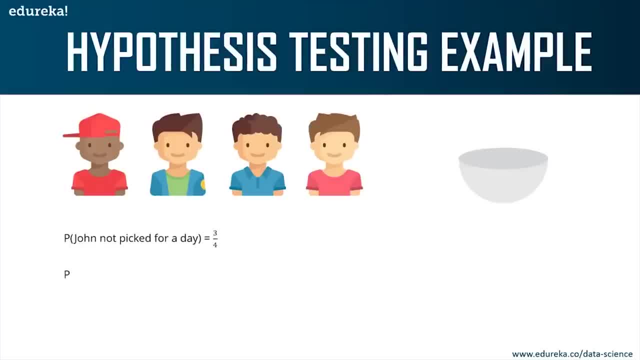 seven, Now 75% is fairly high. So if John is not picked for three days in a row, the probability will drop down to approximately 42%. okay, So three days in a row, meaning that is, the probability drops down. 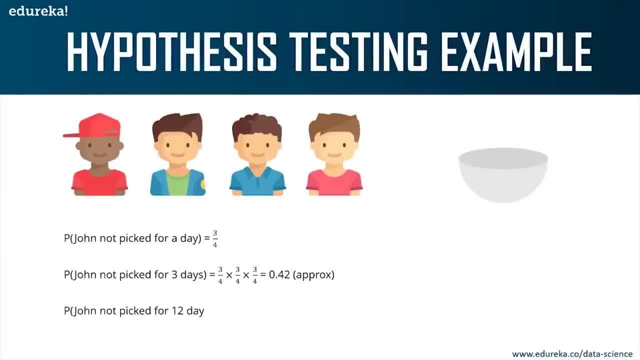 to 42%. Now let's consider a situation where John is not picked for 12 days in a row. The probability drops down to 3.2%. okay, That's, the probability of John cheating becomes fairly high, Right? So in order for statisticians to come to a conclusion, they define what is known as the 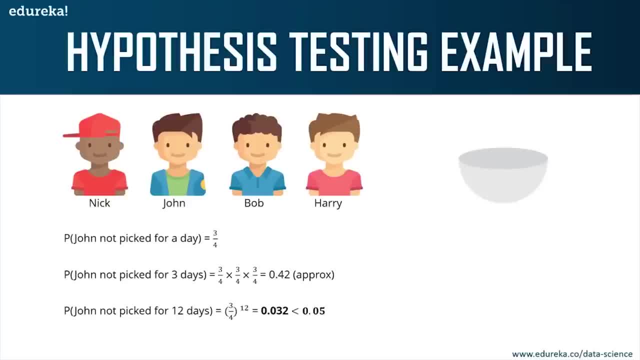 threshold value right. Considering the above situation, if the threshold value is set to 5%, it would indicate that if the probability lies below 5%, then John is cheating his way out of detention, But if the probability is above the threshold value, then John is just lucky and his 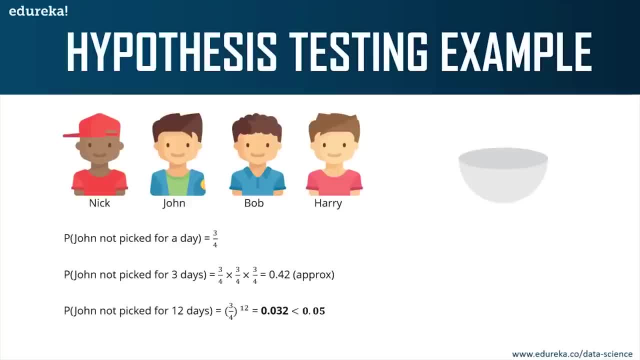 name isn't getting picked. So the probability and hypothesis testing give rise to two important components of hypothesis testing. So the probability and hypothesis testing give rise to two important components of hypothesis testing. So the probability and hypothesis testing give rise to two important components of hypothesis testing, which is null hypothesis. 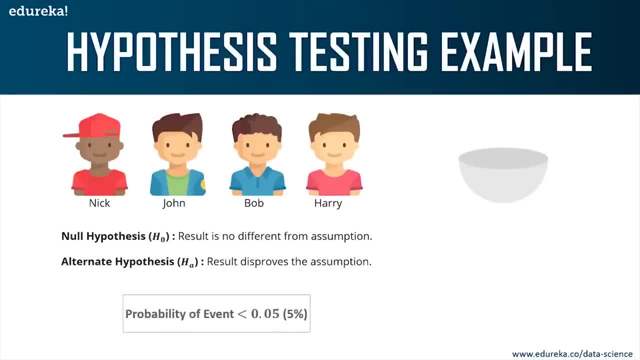 and alternate hypothesis. Null hypothesis is basically approving the assumption. Alternate hypothesis is when your result disapproves the assumption right. Therefore, in our example, if the probability of an event occurring is less than 5%, which it is, then the event is biased. 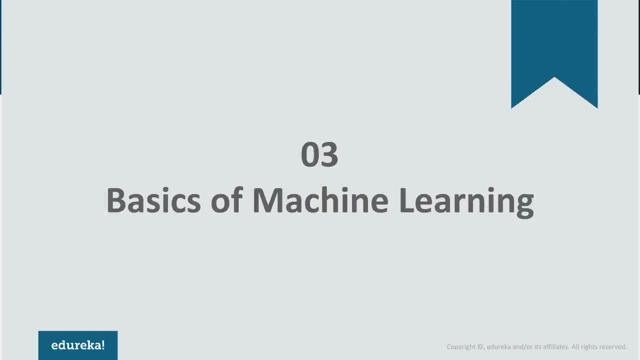 Hence it proves the alternate hypothesis. What is just an Özgörl cours, Pamekha lyrics. Undoubtedly, machine learning is the most in-demand technology in today's market. Its applications range from self-driving cars to predicting deadly diseases such as ALS. 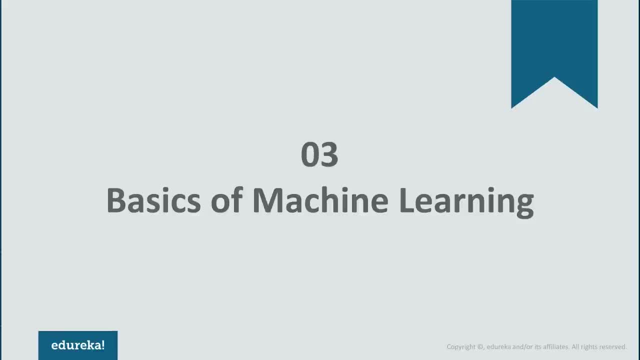 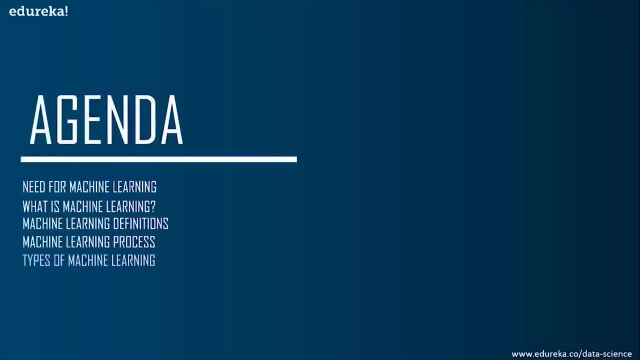 The high demand for machine learning skills is the motivation behind today's session, So let me discuss the agenda with you first. Now we're going to begin the session by understanding the need for machine learning and why it is important. After that, we'll look at what exactly machine learning is, and then we'll discuss a couple of machine learning definitions. 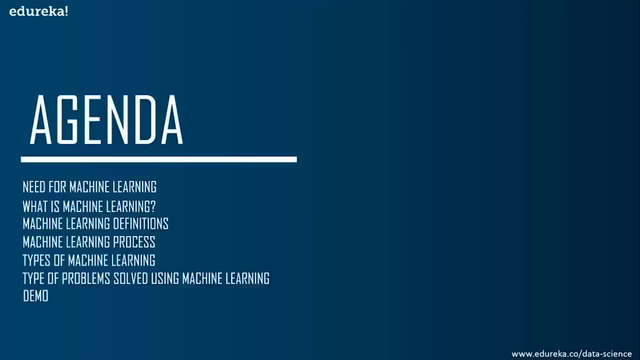 Once we're done with that, we'll look at the machine learning process and how you can solve a problem by using the machine learning process. Next, we'll discuss the types of machine learning, which includes supervised, unsupervised and reinforcement learning. 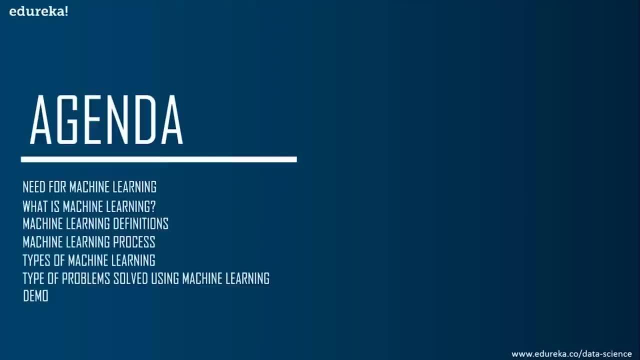 Once we're done with that, we'll discuss the different types of problems that can be solved by using machine learning. Finally, we'll end this session by looking at a demo Where we'll see how you can perform weather forecasting by using machine learning. 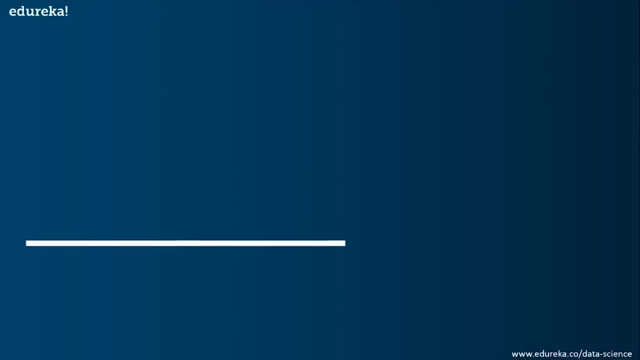 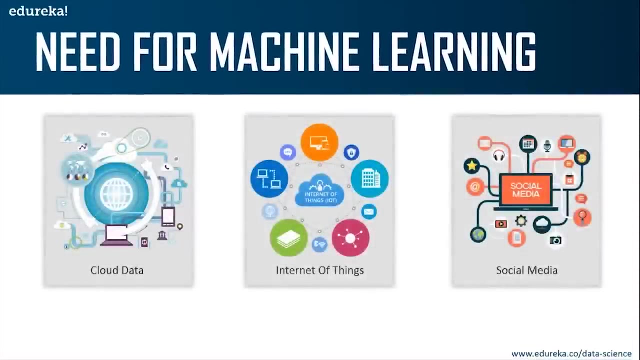 Alright. so, guys, let's get started with our first topic. So what is the importance or what is the need for machine learning Now? ever since the technical revolution, we've been generating an immeasurable amount of data. As per research, we're generating around 2.5 quintillion bytes of data every single day. 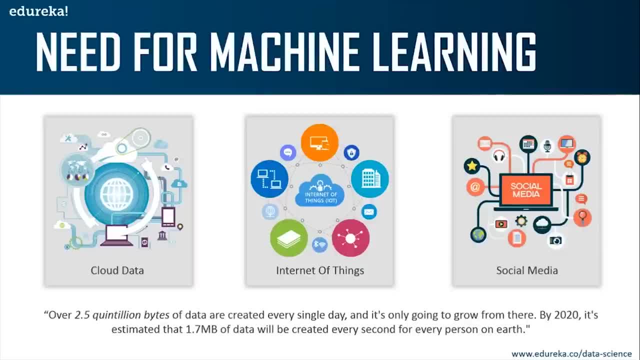 And it is estimated that by 2020, 1.7 MB of data will be created every second for every person on Earth. Now, that is a lot of data. Right now, this data comes from sources such as the cloud, IoT devices, social media and all of that. 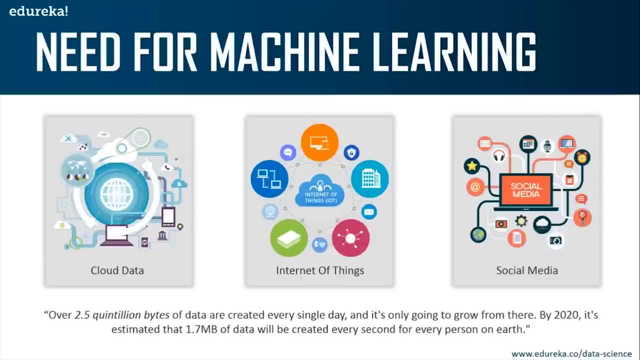 Since all of us are very interested in the Internet right now, we're generating a lot of data. Alright, you have no idea how much data we generate through social media: All the chatting that we do and all the images that we post on Instagram. 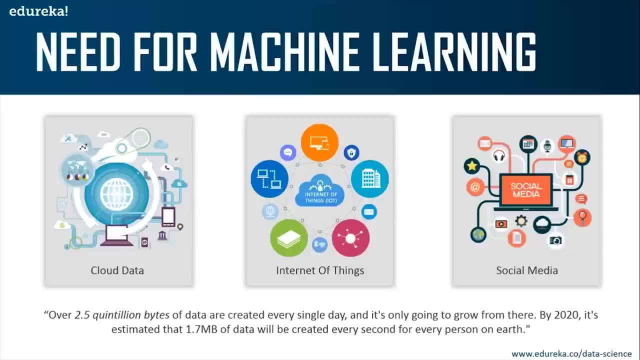 the videos that we watch. all of this generates a lot of data. Now, how does machine learning fit into all of this? Since we're producing this much data, we need to find a method that can analyze, process and interpret this much data. 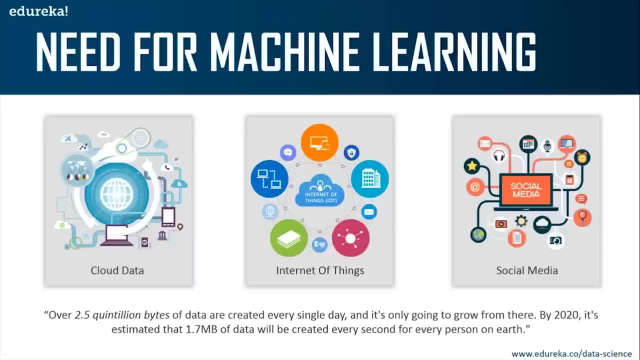 Alright, and we need to find a method that can make sense out of data, And that method is machine learning. Now there are a lot of top-tier companies and data-driven companies, such as Netflix and Amazon, which build machine learning models by using tons of data in order to identify any profitable opportunities. 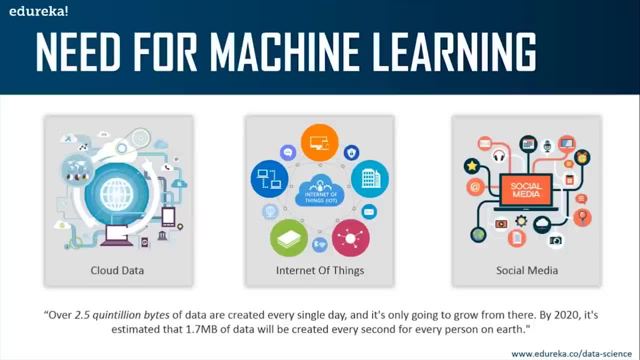 And if they want to avoid any unwanted risks, they make use of machine learning. Alright, so through machine learning, you can predict risks, you can predict profits, you can identify opportunities which will help you grow your business. So now I'll show you a couple of examples wherein machine learning is used. 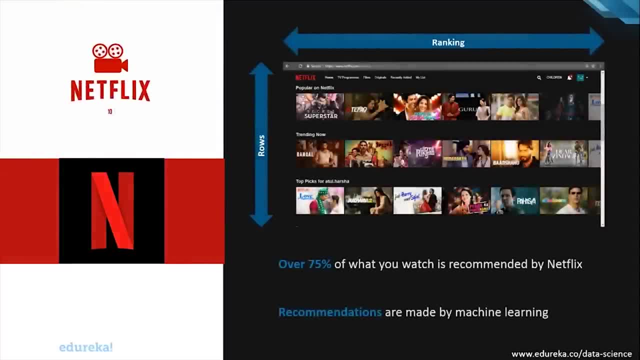 Alright, so I'm sure all of you have binge-watched on Netflix. Now, the most important thing about Netflix is its recommendation engine. Alright, most of Netflix's revenue comes from its recommendation engine, So the recommendation engine basically studies the movie viewing patterns of its users. 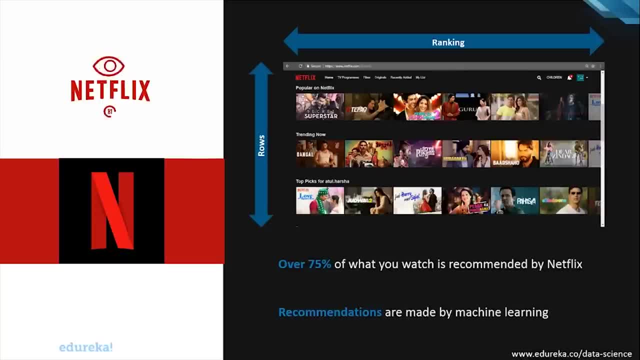 and then recommends relevant movies to them. Alright, it recommends movies depending on users' interests, depending on the type of movies the user watches, and all of that Alright. so that is how Netflix uses machine learning. Next, we have Facebook's auto-tagging feature. 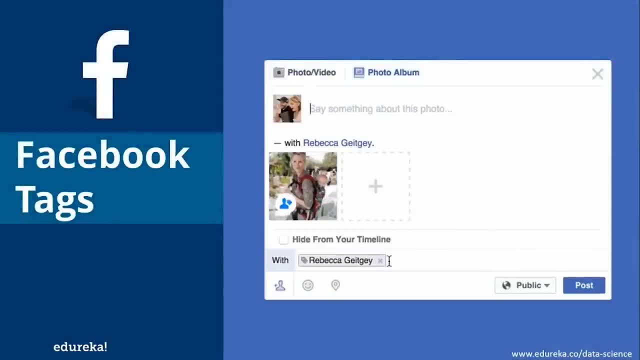 Now, the logic behind Facebook's auto-tagging feature is machine learning and neural networks. I'm not sure how many of you know this, but Facebook makes use of DeepMind face verification system, which is based on machine learning, natural language processing and neural networks. 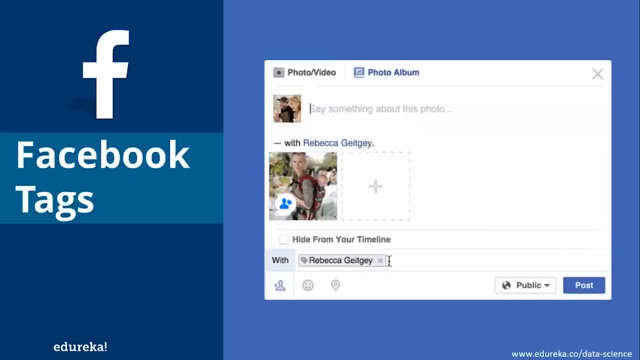 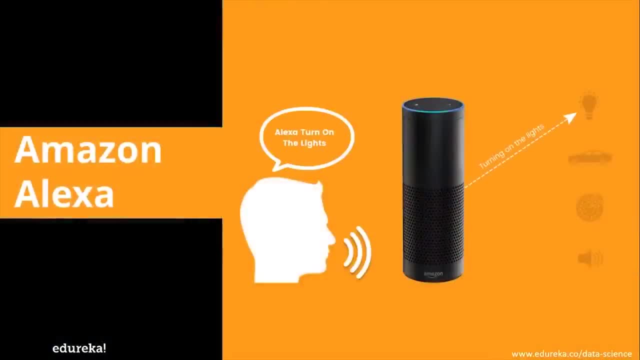 So DeepMind basically studies the facial features in an image and it tags your friends and family. Another such example is Amazon's Alexa. Now, Alexa is basically an advanced level virtual assistant that is based on natural language processing and machine learning. Now it can do more than just play music for you. 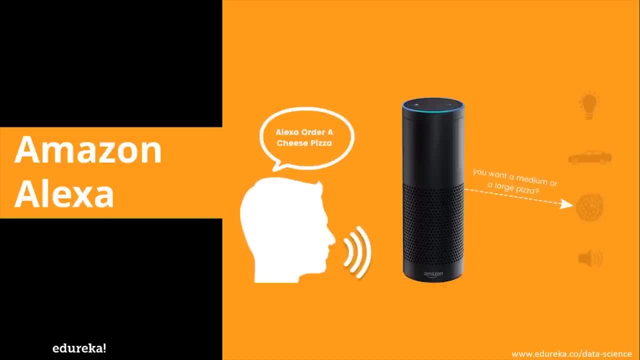 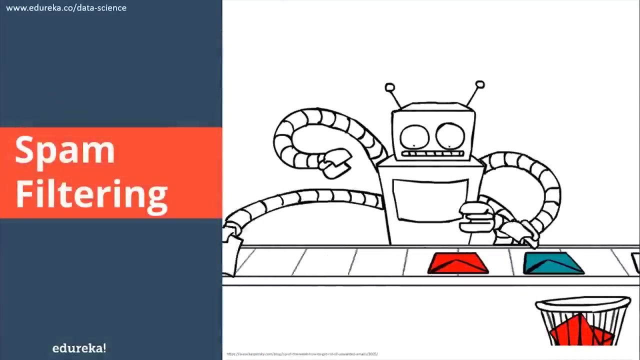 It can book your Uber, it can connect with other IoT devices at your house, it can track your health, it can order food online, and all of that. So data and machine learning are basically the main factors behind Alexa's power. Another such example is the Google spam filter. 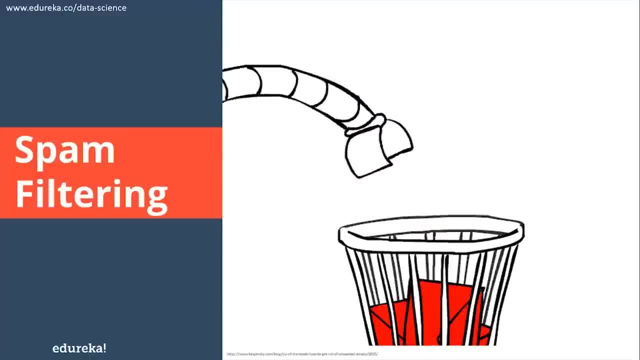 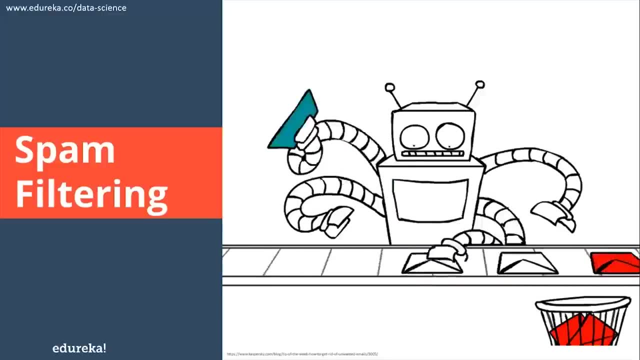 So, guys, Gmail basically makes use of machine learning to filter out spam messages. If any of you just open your Gmail inbox, you'll see that there are separate sections: There's one for primary, there's social, there's spam and there's your general mail. 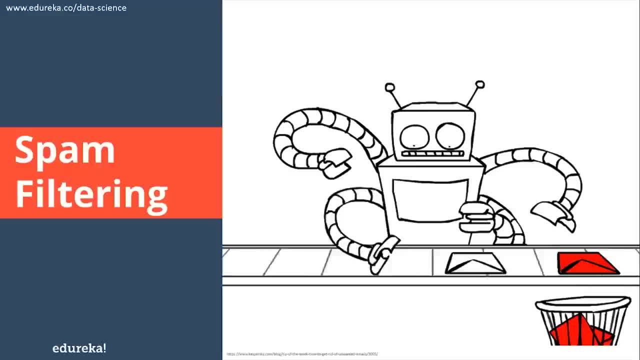 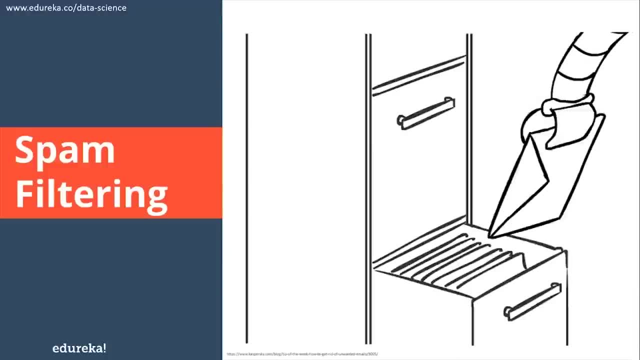 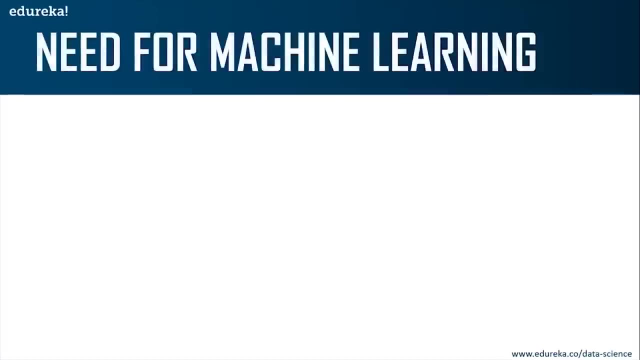 Now, basically, Gmail makes use of machine learning algorithms and natural language processing to analyze emails in real time and then classify them as either spam or non-spam. Now, this is another famous application of machine learning. So, to sum this up, let's look at a few reasons why machine learning is so important. 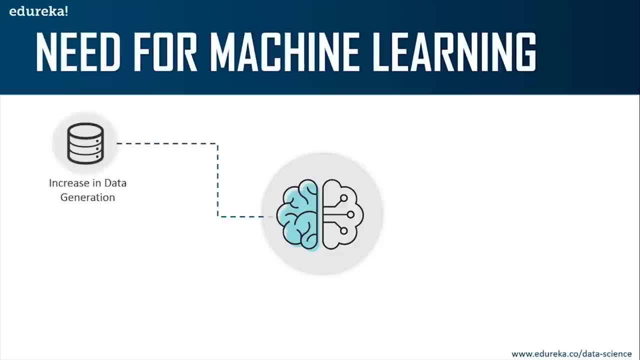 So the first reason is obviously increase in data generation. So, because of excessive production of data, we need a method that can be used to structure, analyze and draw useful insights from data. This is where machine learning comes in. It uses data to solve problems and find solutions to the most complex tasks faced by organizations. 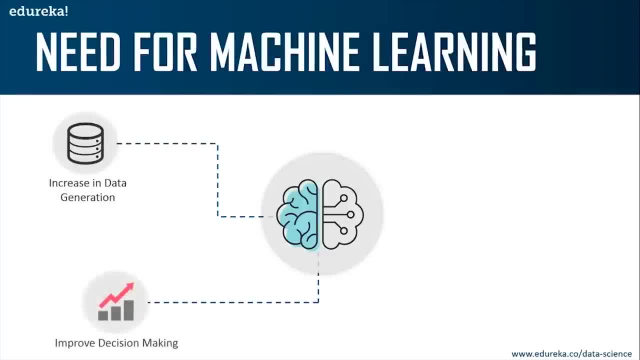 Another important reason is that it improves decision making. So, by making use of various algorithms, machine learning can be used to make better business decisions. For example, machine learning is used to forecast sales. It is used to predict any downfalls in the stock market. 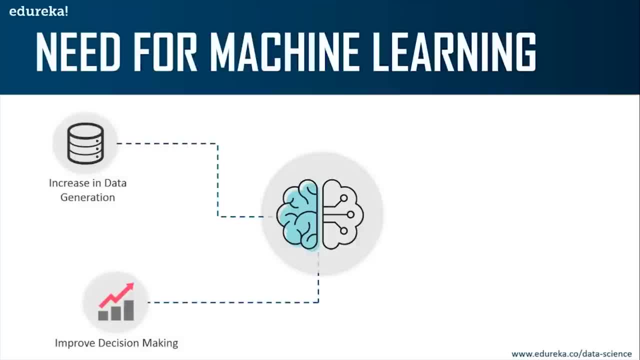 It is used to identify risks, anomalies and so on. Now, the next reason is it uncovers patterns and trends in data. Finding hidden patterns and extracting key insights from data is the most essential part of machine learning. So, by building predictive models, 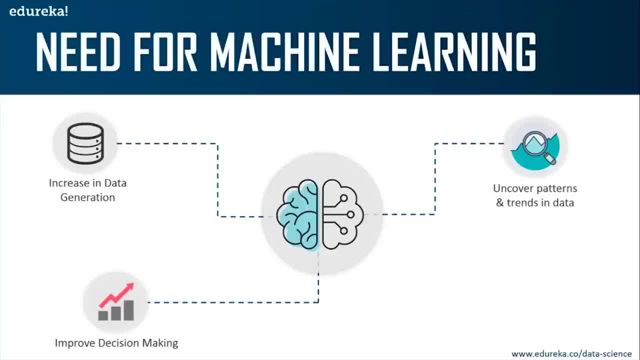 and using statistical techniques, machine learning allows you to dig beneath the surface and explore the data at a minute scale. Now, understanding data and extracting patterns manually will take a lot of days. Now, if you do this through machine learning algorithms, you can perform such computations in less than a second. 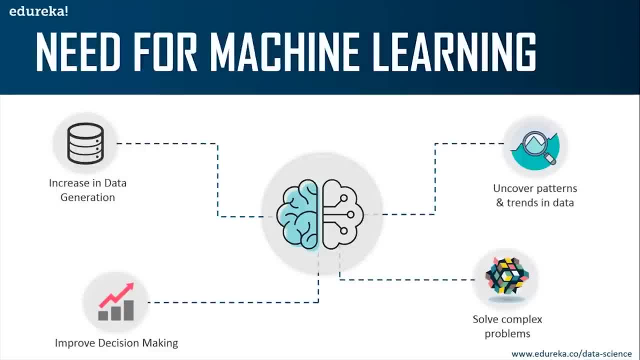 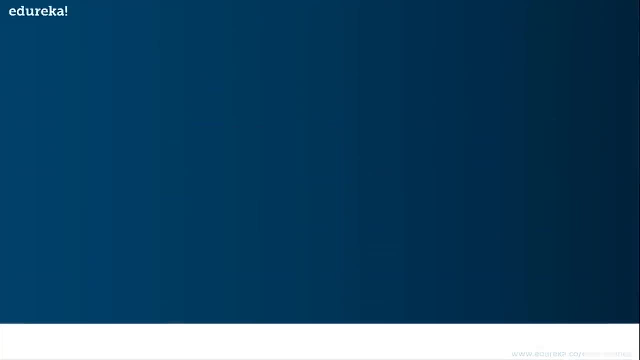 Another reason is that it solves complex problems. So, from detecting genes that are linked to deadly ALS diseases to building self-driving cars and building face detection systems, machine learning can be used to solve the most complex problems. So, guys, now that you know why machine learning is so important, 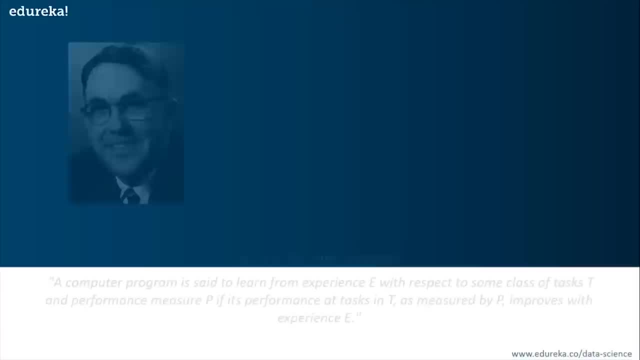 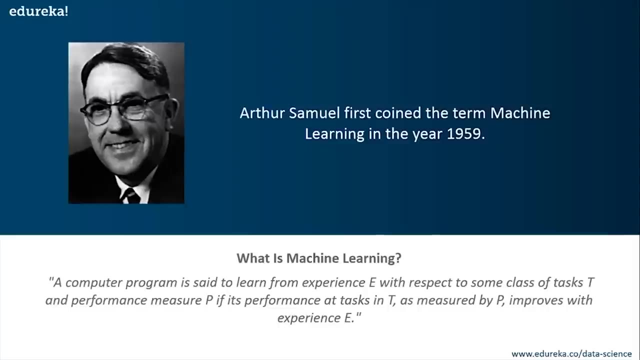 let's look at what exactly machine learning is. The term machine learning was first coined by Arthur Samuel in the year 1959.. Now, looking back, that year was probably the most significant in terms of technological advancements. Guys, if you browse through the net, 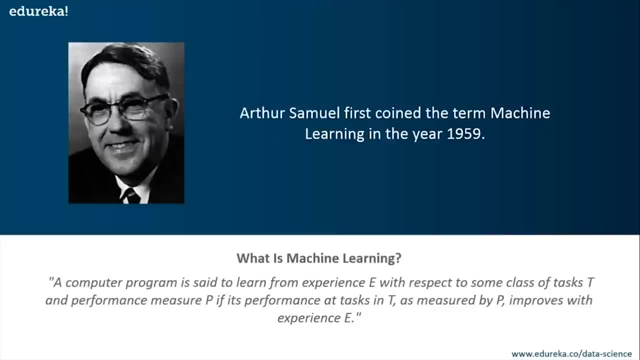 about. what is machine learning? you'll get at least 100 different definitions Now. the first and very formal definition was given by Tom M Mitchell. Now the definition says that a computer program is said to learn from experience. E with respect to some class of task T and performance measure P. 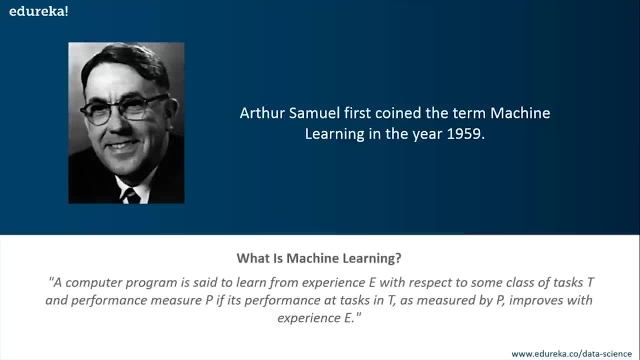 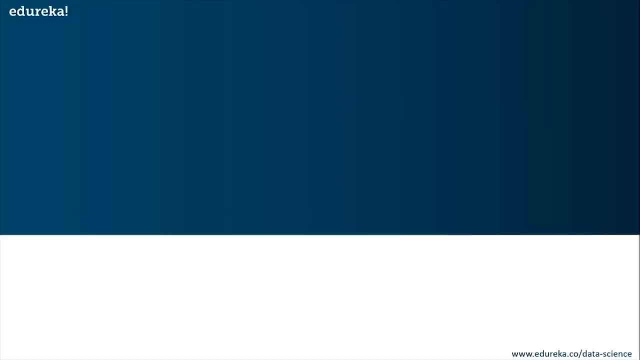 if its performance at task in T, as measured by P, improves with experience E. Alright, Now I know this is a little confusing, so let's break it down into simple words Now. in simple terms, machine learning is a subset of artificial intelligence. 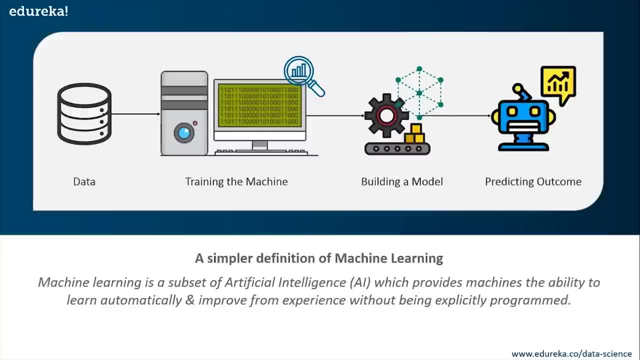 which provides machines the ability to learn automatically and improve from experience without being explicitly programmed to do so. In the sense, it is the practice of getting machines to solve problems by gaining the ability to think. But wait now, how can a machine think or make decisions? 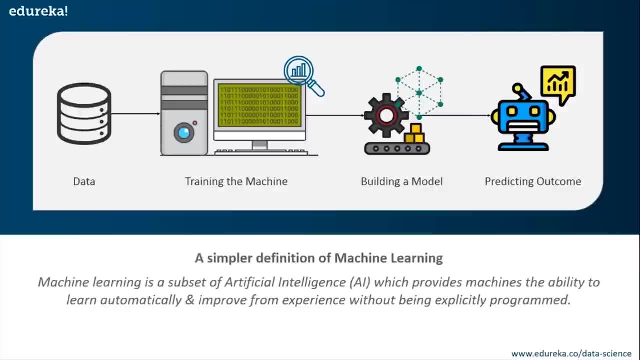 Well, if you feed a machine a good amount of data, it'll learn how to interpret, process and analyze this data by using machine learning algorithms. Okay, Now guys, look at this figure on top. Now, this figure basically shows how a machine learning algorithm 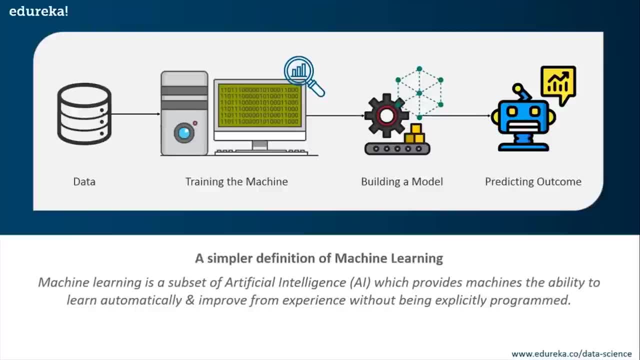 or how the machine learning process really works. So the machine learning process begins by feeding the machine lots and lots of data. Okay, by using this data, the machine is trained to detect hidden insights and trends. Now, these insights are then used to build a machine learning model. 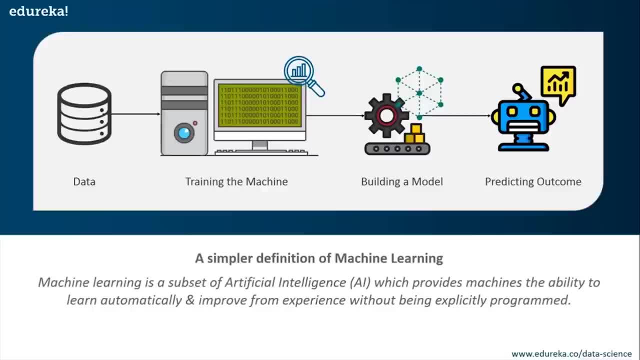 By using an algorithm in order to solve a problem. Okay, So, basically, you're going to feed a lot of data to the machine. The machine is going to get trained by using this data, It's going to use this data and it's going to draw useful insights. 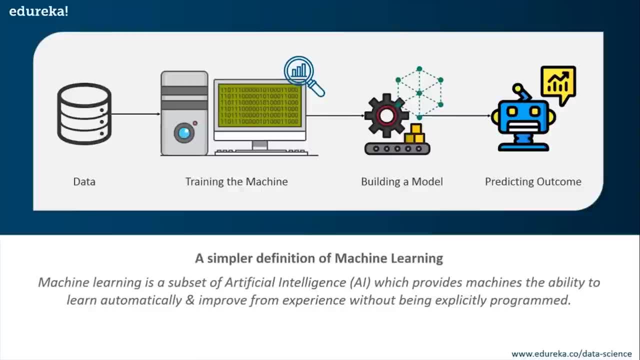 and patterns from it, And then it's going to build a model by using machine learning algorithms. Now this model will help you predict the outcome or help you solve any complex problem or any business problem. So that's a simple explanation of how machine learning works. 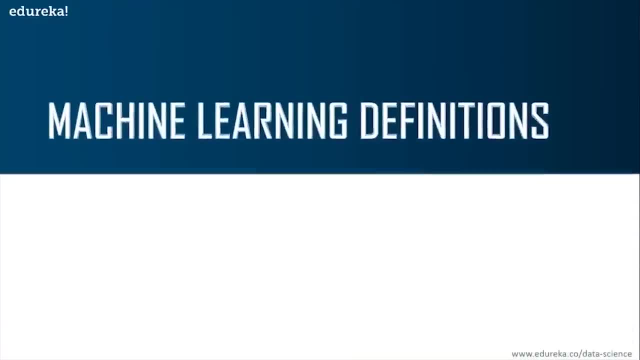 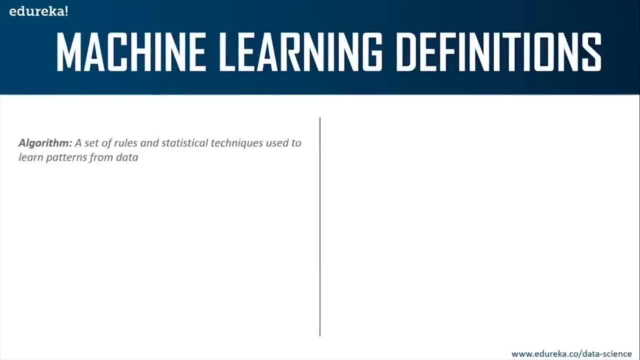 Now let's move on and look at some of the most commonly used machine learning terms. So first of all, we have algorithm. Now this is quite self-explanatory. Basically, algorithm is a set of rules or statistical techniques which are used to learn patterns from data. 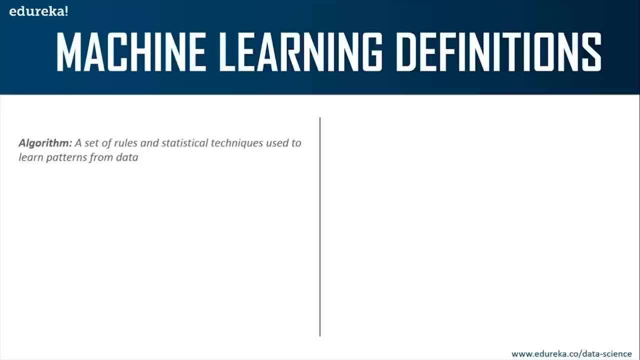 Now, an algorithm is the logic behind a machine learning model. All right, An example of a machine learning algorithm is linear regression. I'm not sure how many of you have heard of linear regression. It's the most simple and basic model of a machine learning algorithm. 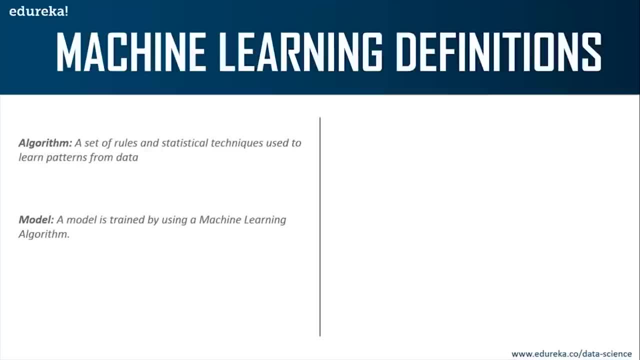 All right. Next we have model. Now model is the main component of machine learning. All right, So model will basically map the input to your output by using the machine learning algorithm and by using the data that you're feeding the machine. 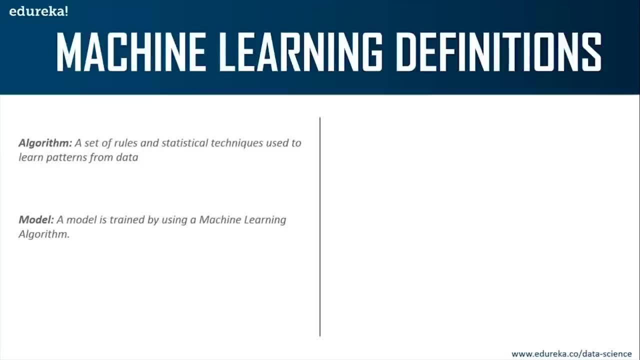 So basically, the model is a representation of the entire machine learning process. So the model is basically fed input, which is a lot of data, and then it will output a particular result or a particular outcome by using machine learning algorithms. Next, we have something known as predictor variable. 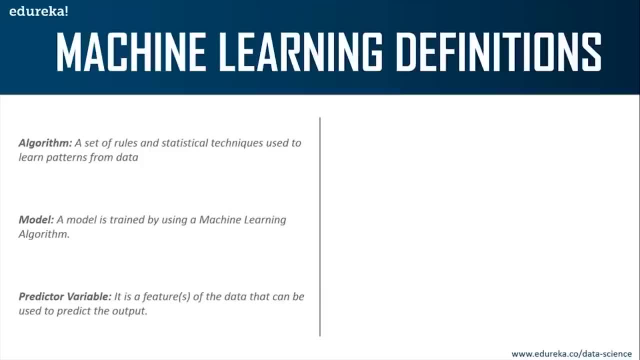 Now, predictor variable is a feature of the data that can be used to predict the output. So, for example, let's say that you're trying to predict the weight of a person depending on the person's height and their age. All right, 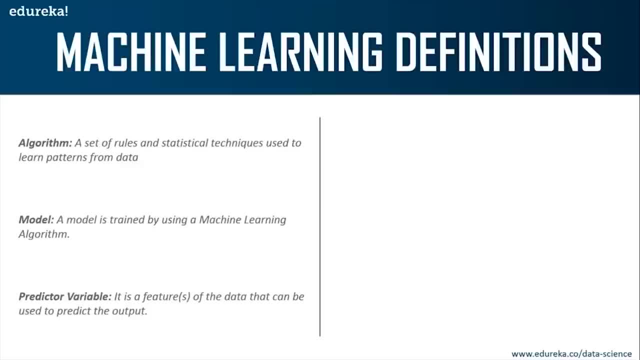 So over here. the predictor variables are your height and your age, because you're using height and age of a person to predict the person's weight, All right. So the height and the age are the predictor variables Now. weight, on the other hand, is the response. 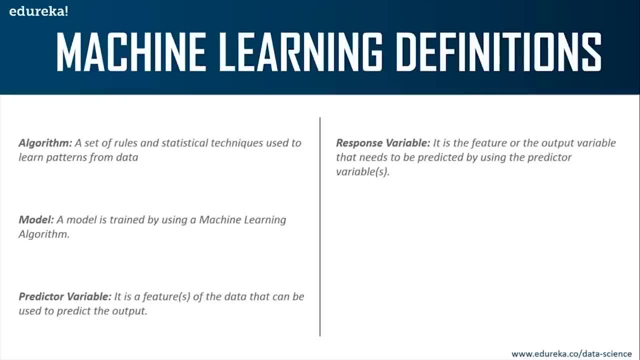 or the target variable. So response variable is a feature, or the output variable that needs to be predicted by using the predictor variables. All right, After that, we have something known as training data. So, guys, the data that is fed to a machine learning model. 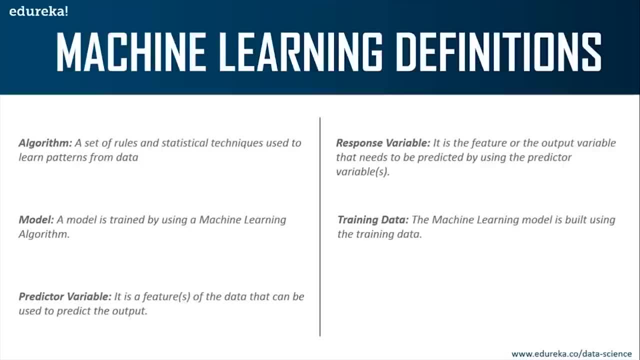 is always split into two parts. First we have the training data and then we have the testing data. Now training data is basically used to build the machine learning model, So usually training data is much larger than the testing data because obviously, if you're trying to train the machine, 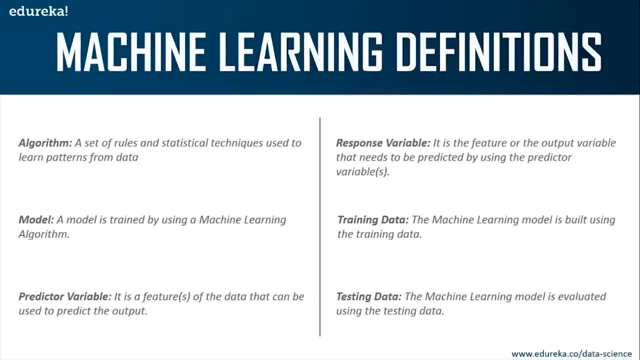 then you're going to feed it a lot more data. Testing data is just used to validate and evaluate the efficiency of the model. All right, So that was training data and testing data. So, guys, these were a few terms that I thought you should know. 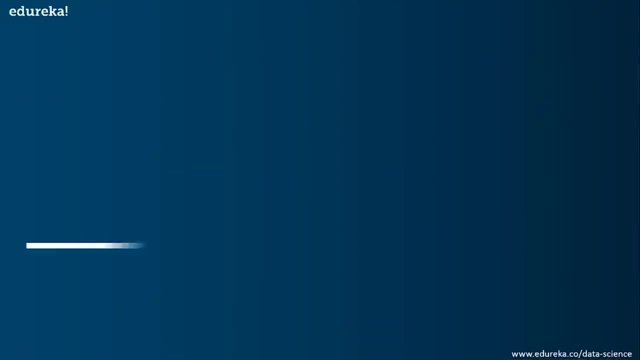 before we move any further. Okay, Now let's move on and discuss the machine learning process. Now this is going to get very interesting because I'm going to give you an example and make you understand how the machine learning process works. So first of all, let's define the different stages. 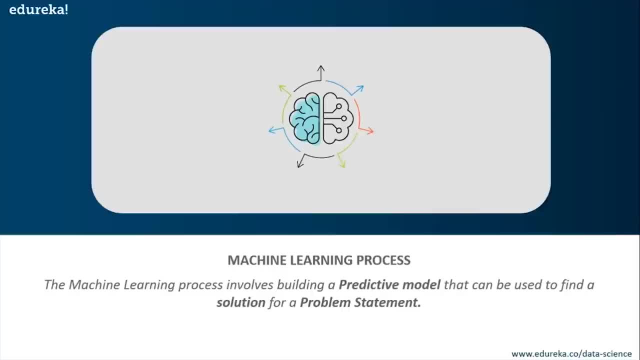 or the different steps involved in the machine learning process. So a machine learning process always begins with defining the objective, or defining the problem that you're trying to solve. Next stage is data gathering, or data collection- Now the data that you need to solve this problem. 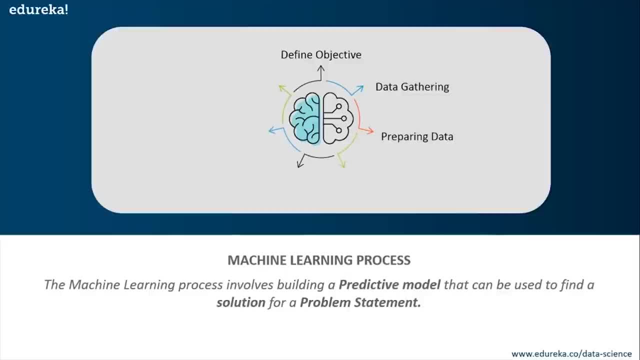 is collected at this stage. This is followed by data preparation or data processing. After that, you have data exploration and analysis, And the next stage is building a machine learning model. This is followed by model evaluation And finally you have prediction or your output. 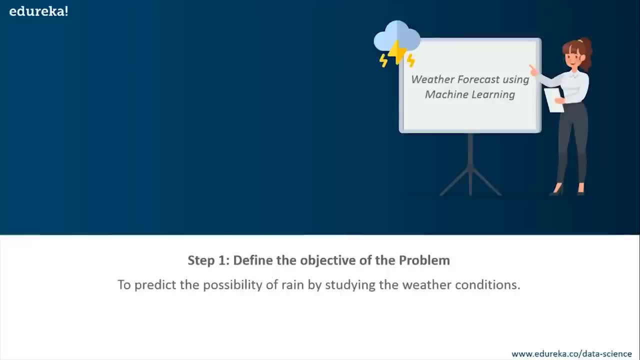 Now let's try to understand this entire process with an example. So our problem statement here is to predict the possibility of rain by studying the weather conditions. So let's say that you're given a problem statement and you're asked to use a machine learning process. 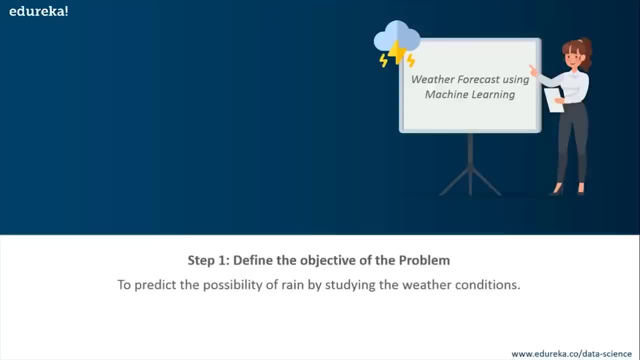 to solve this problem statement. So let's get started. So the first step is to define the objective of the problem statement. Our objective here is to predict the possibility of rain by studying the weather conditions Now, in the first stage of a machine learning process. 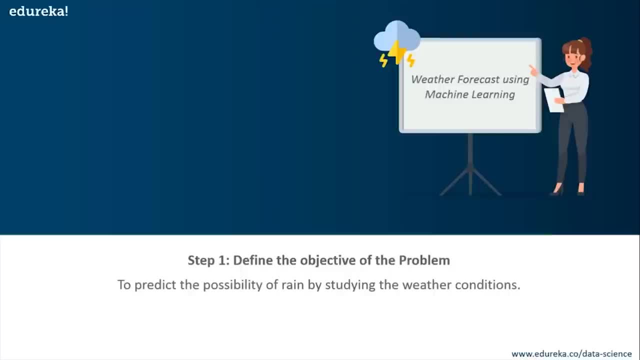 you must understand what exactly needs to be predicted Now. in our case, the objective is to predict the possibility of rain by studying weather conditions, So at this stage, it is also essential to take mental notes on what kind of data can be used to solve this problem. 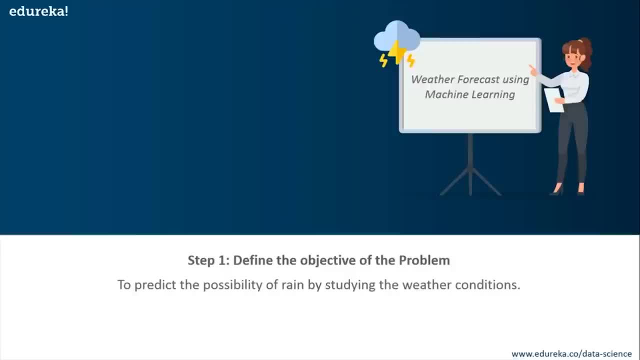 or the type of approach that you can follow to get to the solution. A few questions that are worth asking during this stage is: what are we trying to predict? What are the target features or what are the predictor variables? What kind of input data do we need? 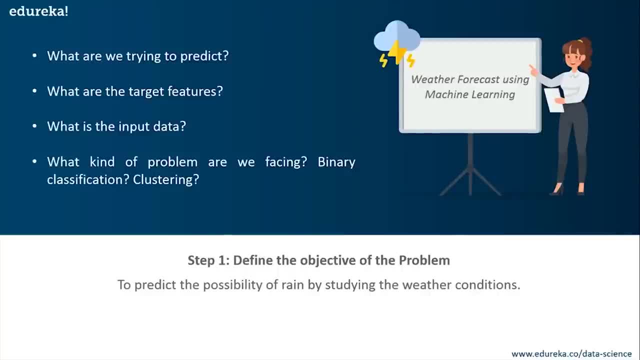 And what kind of problem are we facing? Is it a binary classification problem Or is it a clustering problem? Now, don't worry, if you don't know what classification and clustering is, I'll be explaining this in the upcoming slides. So, guys, this was the first step of a machine learning process. 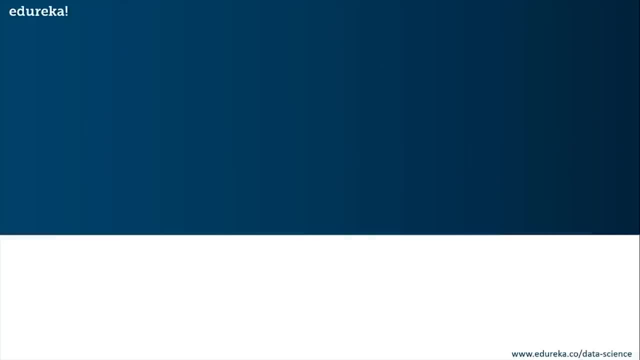 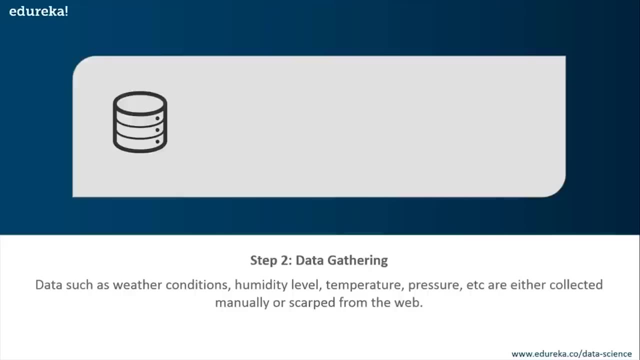 which is define the objective of the problem. All right, now let's move on and look at step number two. So step number two is basically data collection, or data gathering. Now, at this stage, you must be asking questions such as what kind of data is needed to solve the problem? 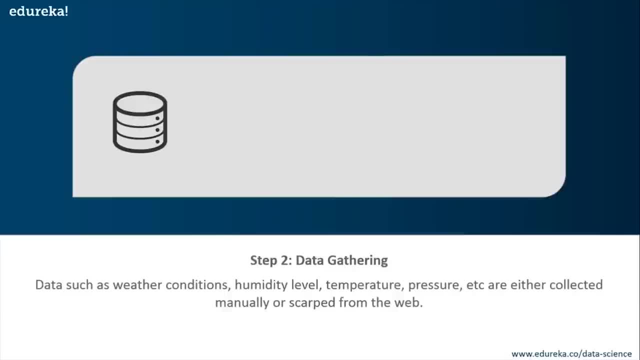 Is the data available And if it is available, how can I get the data? Okay, Once you know the type of data that is required, you must understand how you can derive this data. Data collection can be done manually or by web scraping. 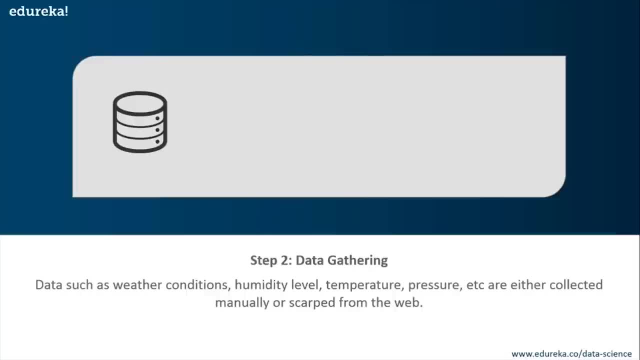 But if you're a beginner and you're just looking to learn machine learning, you don't have to worry about getting the data Okay. There are thousands of data resources on the web. You can just go ahead and download the data sets from websites such as Kaggle. 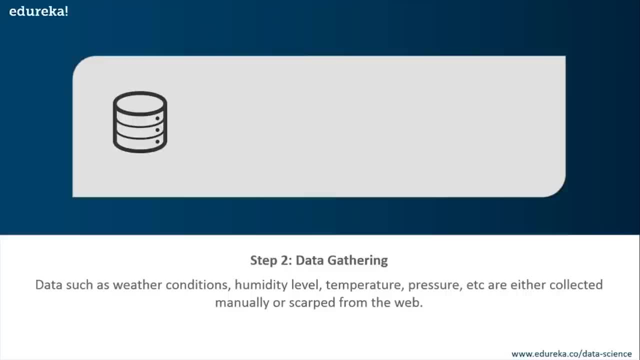 Okay, Now coming back to the problem at hand. the data needed for weather forecasting includes measures such as humidity level, temperature pressure, locality, whether or not you live in a hill station, and so on. So, guys, such data must be collected. 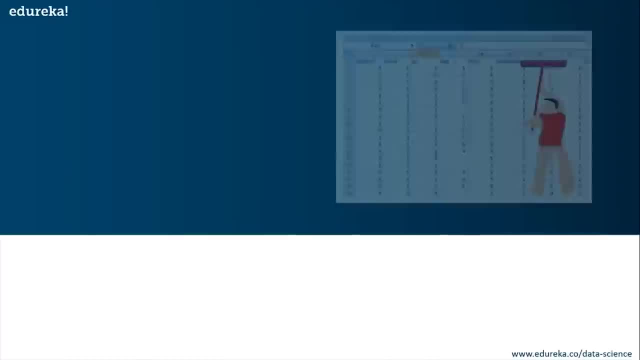 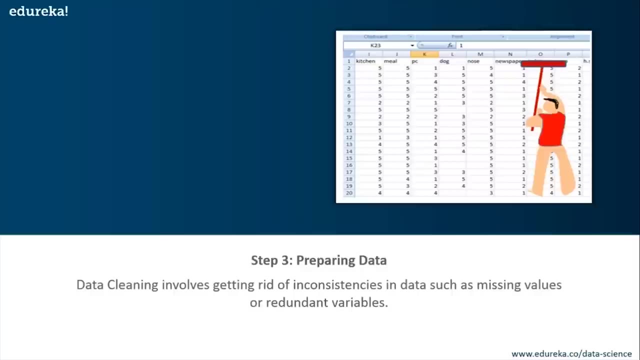 and stored for analysis. Now the next stage in machine learning is preparing your data. The data you collected is almost never in the right format, So, basically, you'll encounter a lot of inconsistencies in the data set. Okay, This includes missing values, redundant variables. 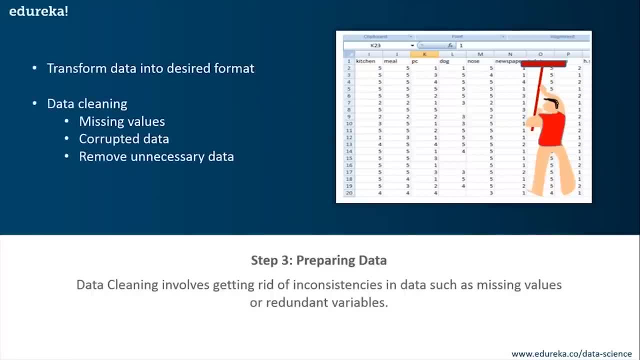 duplicate values and so on. Removing such values is very important because they might lead to wrongful computations and predictions. So that's why, at this stage, you must scan the entire data set for any inconsistencies and you have to fix them at this stage. 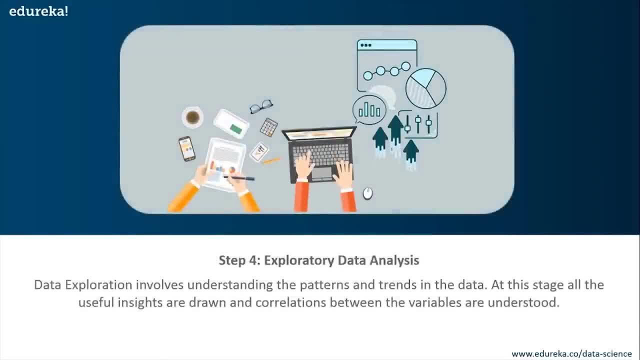 Now the next step is exploratory data analysis. Now, data analysis is all about diving deep into data and finding all the hidden data mysteries. Okay, This is where you become a detective. So EDA, or exploratory data analysis, is like a breakthrough. 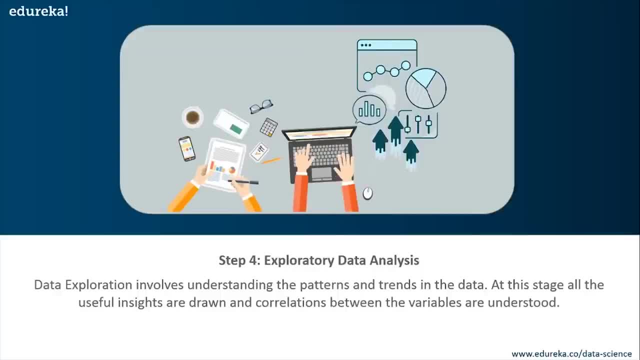 It's the brainstorming of machine learning. Data exploration involves understanding the patterns and the trends in your data. So at this stage all the useful insights are drawn and all the correlations between the variables are understood. So you might ask: what sort of correlations are you talking about? 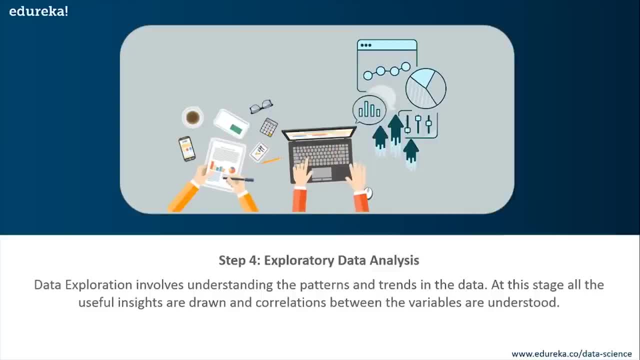 For example, in the case of predicting rainfall, we know that there is a strong possibility of rain if the temperature has fallen low. Okay, So such correlations have to be understood and mapped at this stage. So this stage is followed by stage number five. 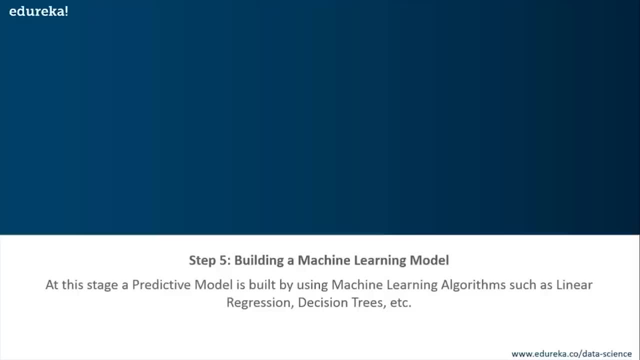 which is building a machine learning model. So all the insights and the patterns that you derive during data exploration are used to build the machine learning model. So this stage always begins by splitting the data set into two parts: training data and the testing data. 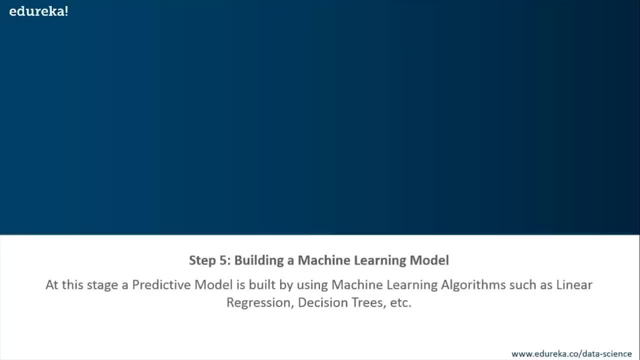 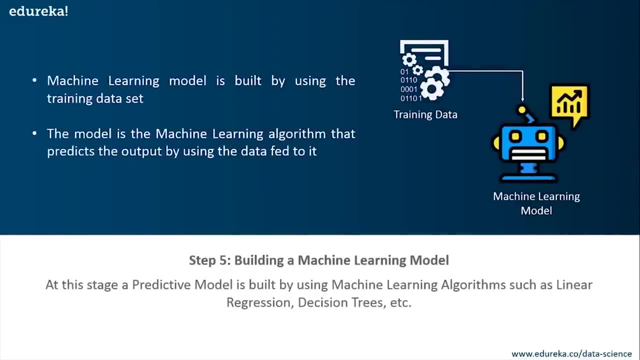 So earlier in this session I already told you what training and testing data is. Now the training data will be used to build and analyze the model, and the logic of the model will be based on the machine learning algorithm that is being implemented. 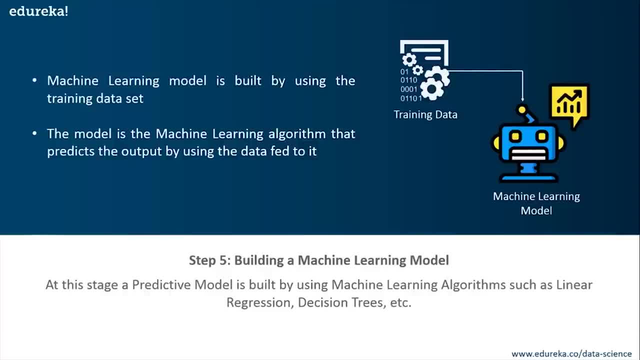 Okay Now, in the case of predicting rainfall, since the output will be in the form of true or false, we can use a classification algorithm like logistic regression. Now, choosing the right algorithm depends on the type of problem you're trying to solve. 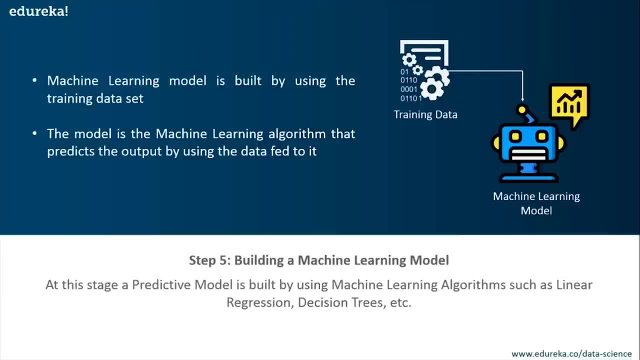 the data set you have and the level of complexity of the problem. So in the upcoming sections we'll be discussing different types of problems that can be solved by using machine learning. So don't worry if you don't know what classification algorithm is. 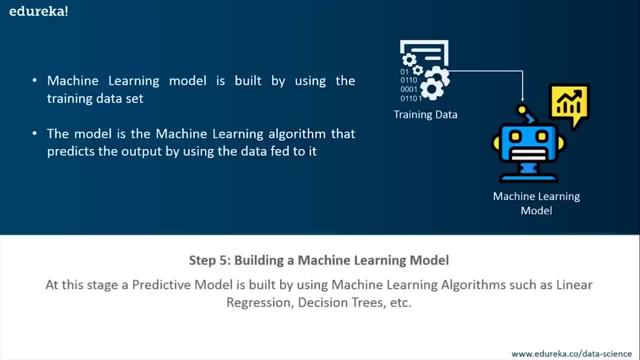 and what logistic regression is Okay. So all you need to know is, at this stage, you'll be building a machine learning model by using machine learning algorithm and by using the training data set. The next step in a machine learning process is model evaluation and optimization. 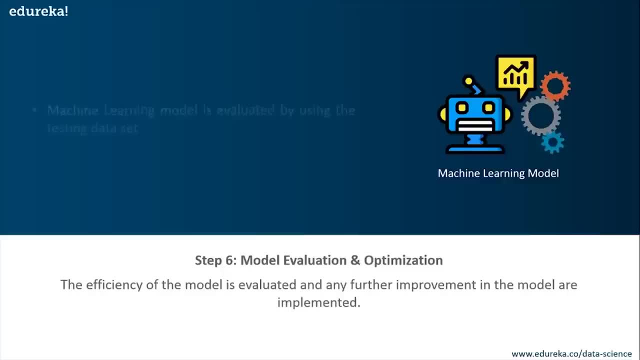 So, after building a model by using the training data set, it is finally time to put the model to a test. Okay, So the testing data set is used to check the efficiency of the model and how accurately it can predict the outcome. 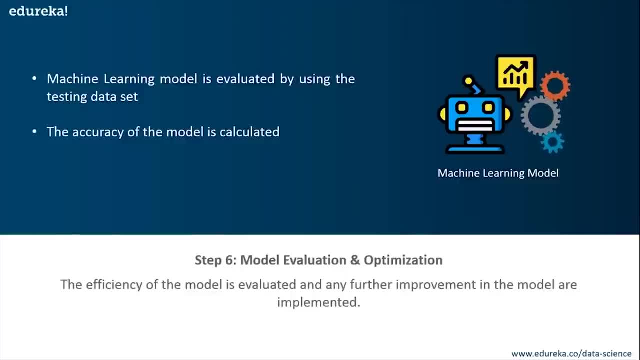 So, once you calculate the accuracy, any improvements in the model have to be implemented in this stage. Okay, So methods like parameter tuning and cross-validation can be used to improve the performance of the model. This is followed by the last stage. 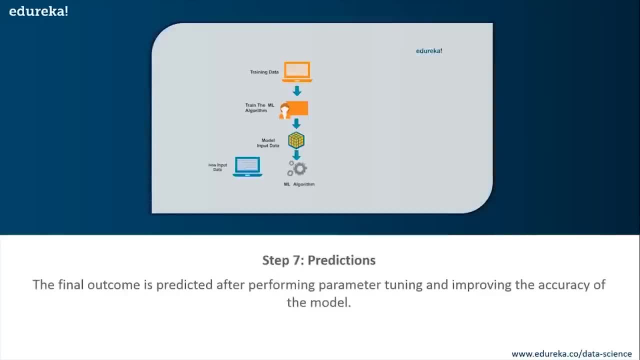 which is predictions. So once the model is evaluated and improved, it is finally used to make predictions. The final output can be a categorical variable or it can be a continuous quantity. In our case, for predicting the occurrence of rainfall, the output will be a categorical variable. 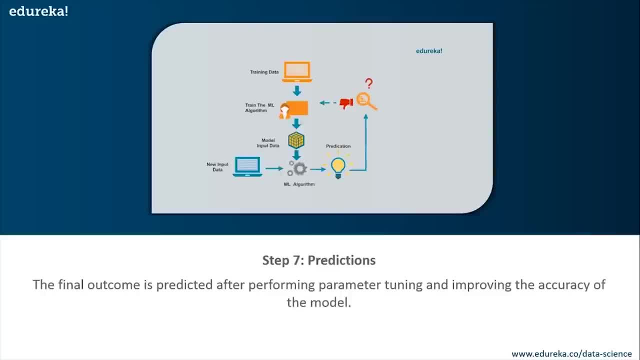 In the sense our output will be in the form of true or false, yes or no. Yes basically represents that it's going to rain, and no will represent that, no, it won't rain. Okay, As simple as that. So, guys, 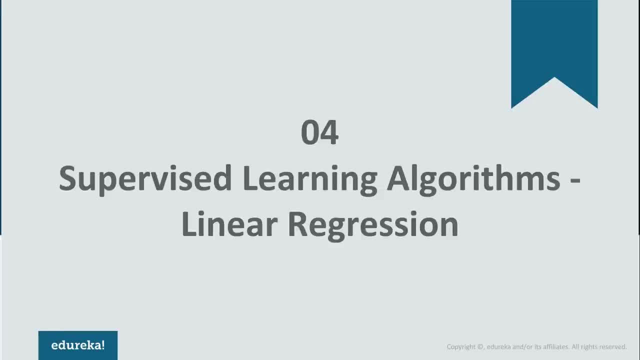 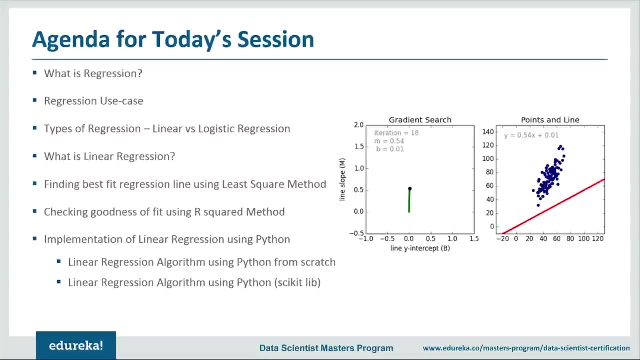 that was the entire machine learning process. A linear regression is one of the easiest algorithm in machine learning. It is a statistical model that attempts to show the relationship between two variables with a linear equation. But before we drill down to linear regression algorithm in depth, 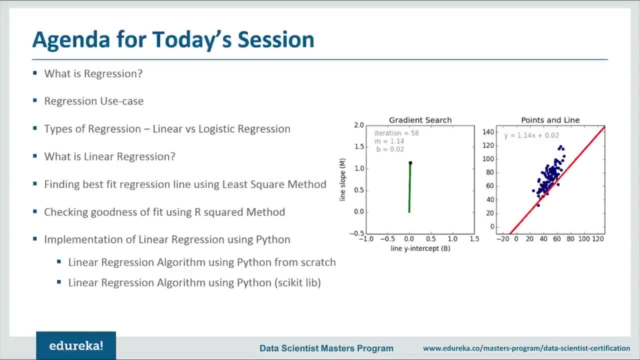 I'll give you a quick overview of today's agenda. So we'll start a session with a quick overview of what is regression, as linear regression is one of a type of regression algorithm. Once we learn about regression, its use case, the various types of it, 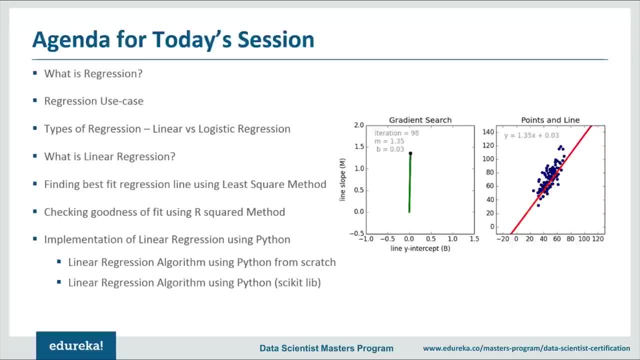 Next we'll learn about the algorithm from scratch, where I'll teach you its mathematical implementation first. Then we'll drill down to the coding part and implement linear regression using Python. in today's session, We'll deal with linear regression algorithm using least square method. 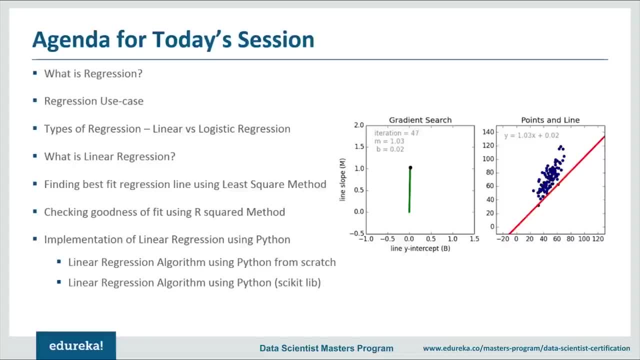 Check its goodness of fit, or how close the data is to the fitted regression line using the R square method, And then, finally, what we'll do will optimize it using the gradient decent method. in the last part, on the coding session, I'll teach you to implement linear regression. 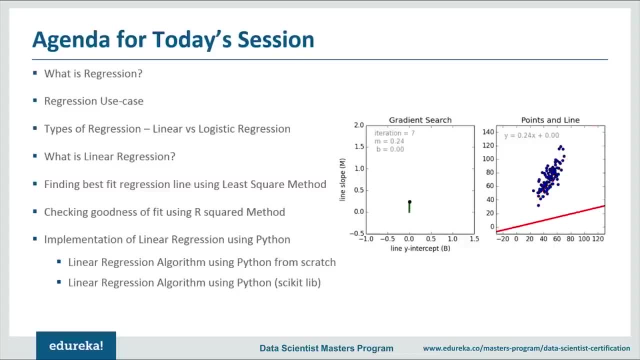 using Python, and the coding session would be divided into two parts. The first part would consist of linear regression using Python from scratch, where you will use the mathematical algorithm that you have learned in this session, and in the next part of the coding session, we'll be using scikit-learn. 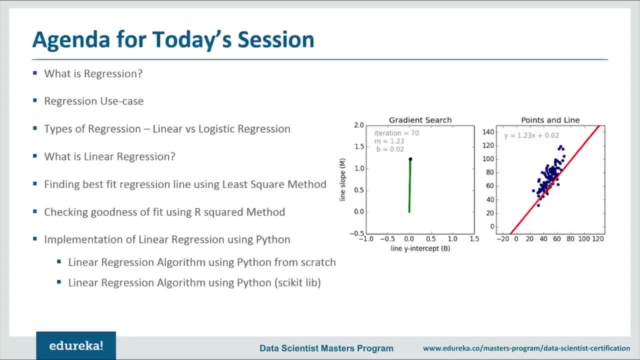 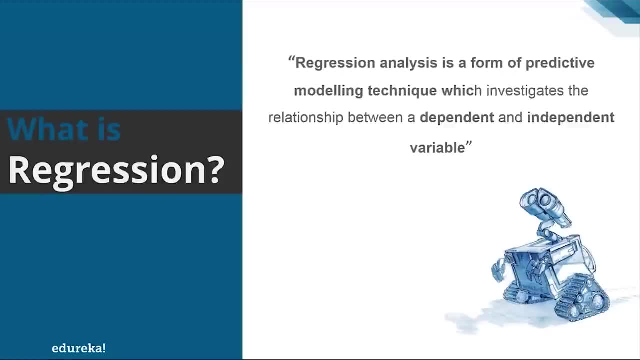 for Derek. implementation of linear regression. All right, I hope the agenda is clear to you guys, All right. So let's begin our session with. what is regression? Well, regression analysis is a form of predictive modeling technique which investigates the relationship between a dependent and independent variable. 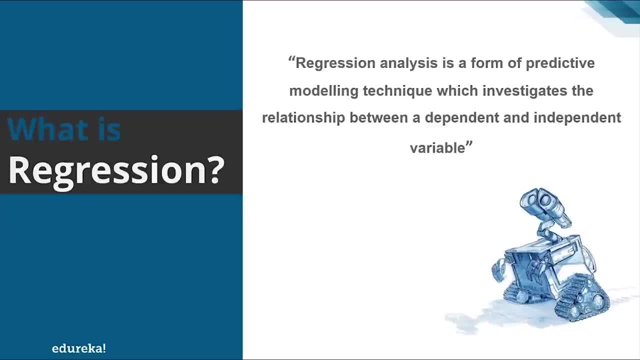 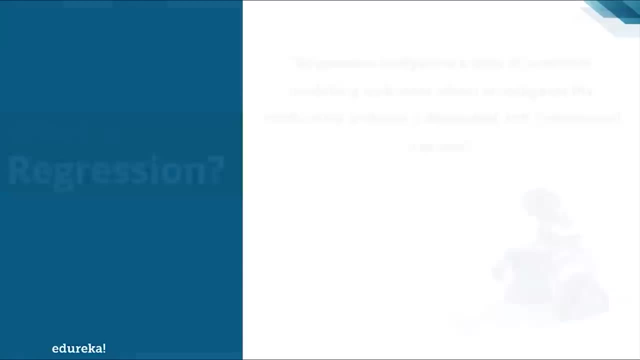 a regression analysis involves graphing a line over a set of data points that most closely fits the overall shape of the data. a regression shows the changes in a dependent variable on the y-axis to the changes in the explanatory variable on the x-axis. fine, Now you'd ask what are the uses of regression? 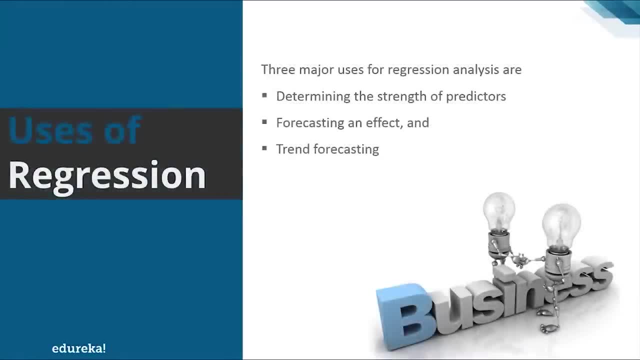 Well, there are major three uses of regression analysis, The first being determining the strength of predicators. the regression might be used to identify the strength of the effect that the independent variables have on the dependent variable. For example, you can ask question like what is the strength of relationship? 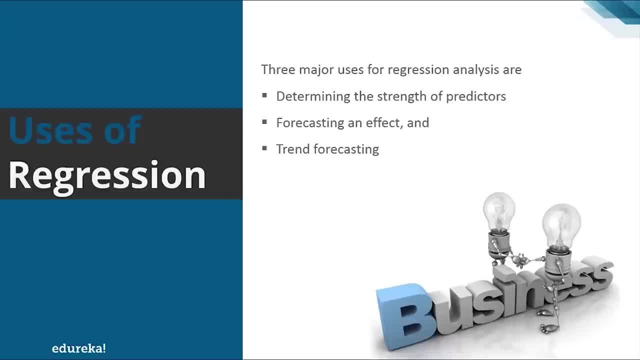 between sales and marketing spending, or what is the relationship between age and income? second, is forecasting an effect in this? the regression can be used to forecast effects or impact of changes. That is, the regression analysis help us to understand how much the dependent variable changes with the change in one or more independent variable. fine, 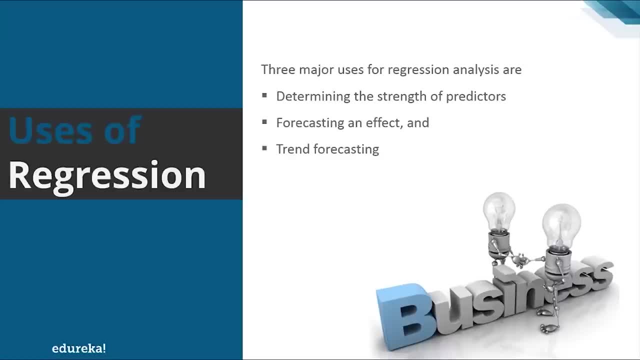 For example, you can ask question like: how much additional sale income will I get for each thousand dollars spent on marketing? third is trend forecasting. in this, the regression analysis predict trends and future values. The regression analysis can be used to get point estimates. in this, you can ask questions like: what will be the price? 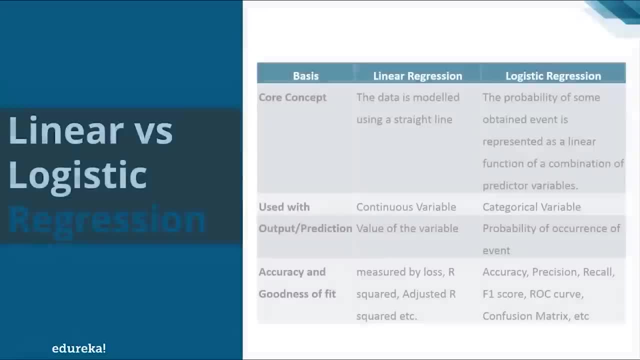 of Bitcoin in next six months, right? So next topic is linear versus logistic regression. by now I hope that you know what a regression is, So let's move on and understand its type. So there are various kinds of regression, like linear regression, logistic regression. 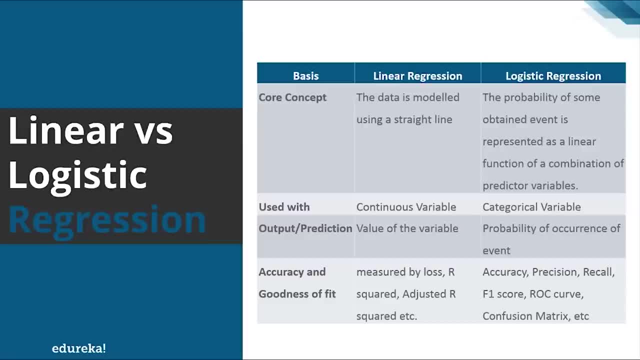 polynomial regression and others, All right, But for this session will be focusing on linear and logistic regression. So let's move on and let me tell you what is linear regression and what is logistic regression. Then what we'll do will compare both of them. 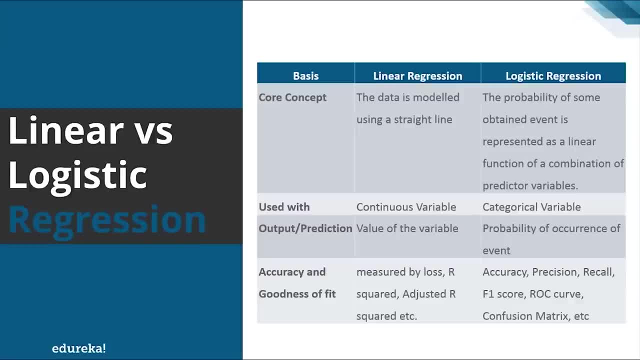 All right. So, starting with linear regression, in simple linear regression We are interested in things like y equal, MX, PC. So what we are trying to find is the correlation between X and Y variable. This means that every value of X has a corresponding value. 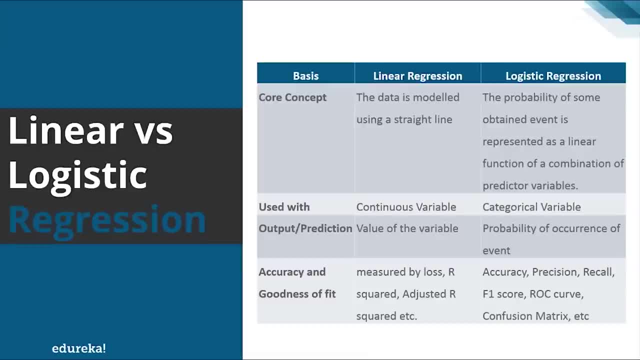 of Y in it. if it is continuous, All right. However, in logistic regression, We are not fitting our data to a straight line like linear regression. instead, what we are doing We are mapping Y versus X to a sigmoid function. in logistic regression, What we find out is: is Y 1 or 0? 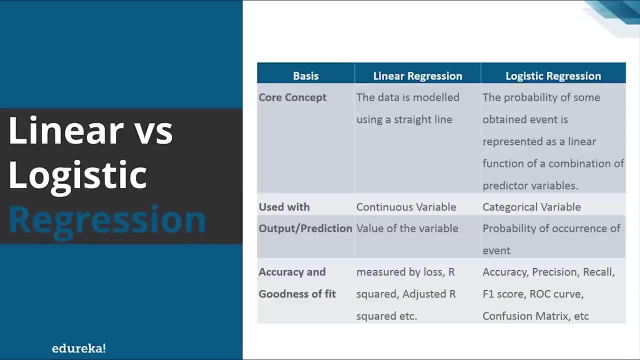 for this particular value of X. So this: we are essentially deciding true or false value for a given value of X. fine, So as a core concept of linear regression, you can say that the data is model using a straight line, where, in the case of logistic regression, 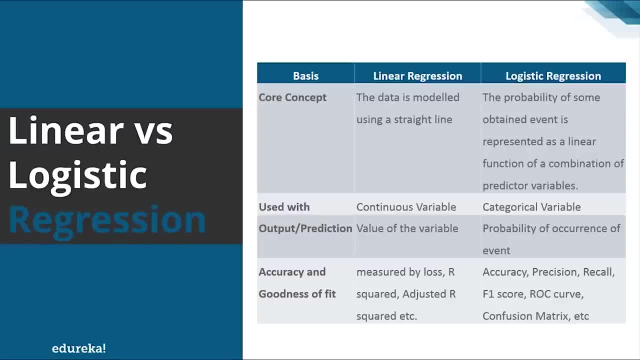 The data is model using a sigmoid function. The linear regression is used with continuous variables. on the other hand, the logistic regression, It is used with categorical variable. the output or the prediction of a linear regression is the value of the variable. on the other hand, the output. 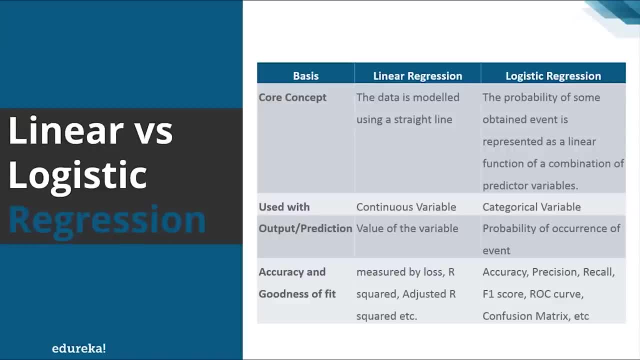 of prediction of a logistic regression is the probability of occurrence of the event. Now, how will you check the accuracy and goodness of fit in case of linear regression, your various methods, like measured by loss, R squared, adjusted R squared, Etc. while in the case of logistic regression you have accuracy, precision, recall. 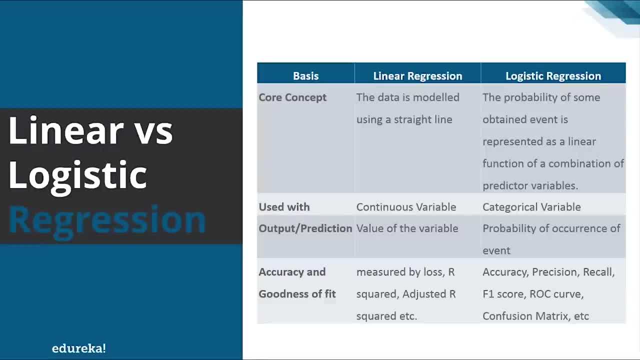 F1 score, which is nothing but the harmonic mean of precision and recall. next is ROC curve for determining the probability threshold for classification, or the confusion Matrix, Etc. There are many, all right. So, summarizing the difference between linear and logistic regression, You can say that the type of function you are mapping, 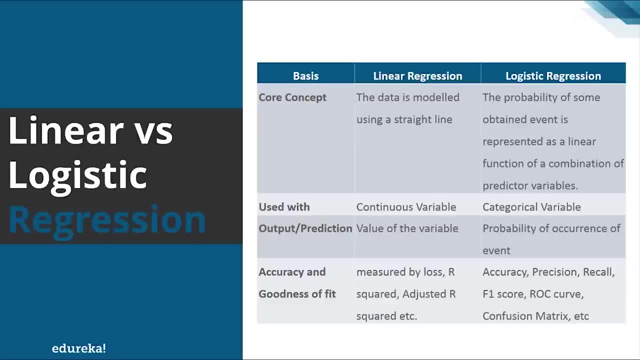 to is the main point of difference between linear and logistic regression. a linear regression Maps a continuous X to a continuous by. on the other hand, a logistic regression Maps a continuous X to the binary Y. so we can use logistic regression to make category or true, false decisions from the data. fine, 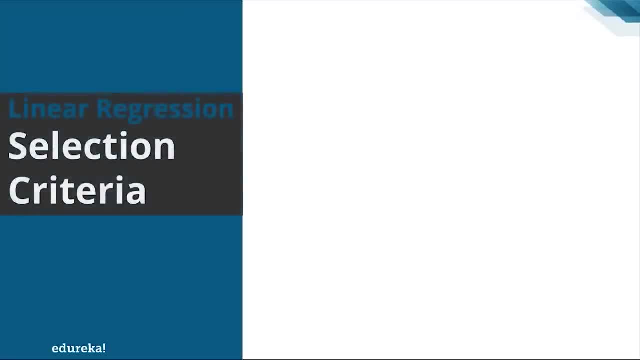 So let's move on ahead. Next is linear regression: selection criteria, or you can say when will you use linear regression? So the first is classification and regression capabilities. regression models predict a continuous variable, such as the sales made on a day, or predict the temperature of a city. that reliance on a polynomial like a straight. 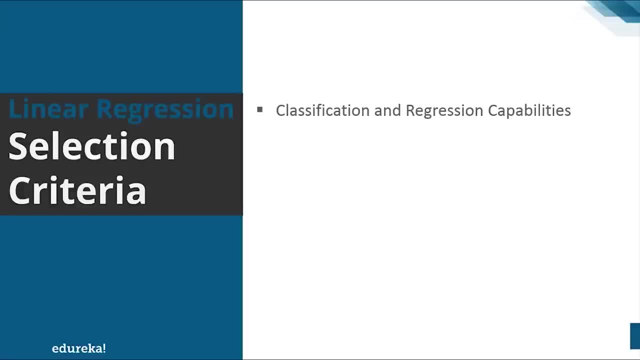 line to fit a data set poses a real challenge when it comes towards building a classification capability. Let's imagine that you fit a line with the training points that you have now. imagine you add some more data points to it. But in order to fit it, what do you have to do? 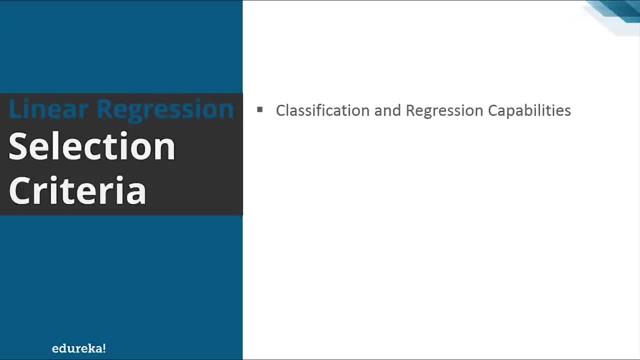 You have to change your existing model, that is, maybe you have to change the threshold itself. So this will happen with each new data point you are to the model. Hence the linear regression is not good for classification models, Fine. Next is data classification, data quality: each missing value removes one data point. 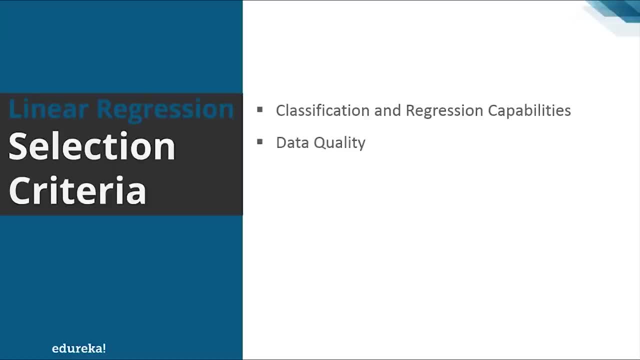 that could optimize the regression and simple linear regression. The outliers can significantly disrupt the outcome. just for now, You can know that if you remove the outliers, your model will become very good. All right. So this is what: data quality. next is computational complexity. 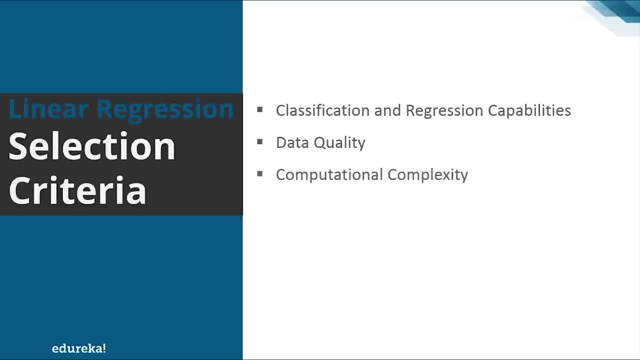 The linear regression is often not computationally expensive as compared to the decision tree or the clustering algorithm. the order of complexity for n training example, and X features usually falls in either big O of n X square or big O of X n. next is comprehensible and transparent. the linear regression are easily comprehensible. 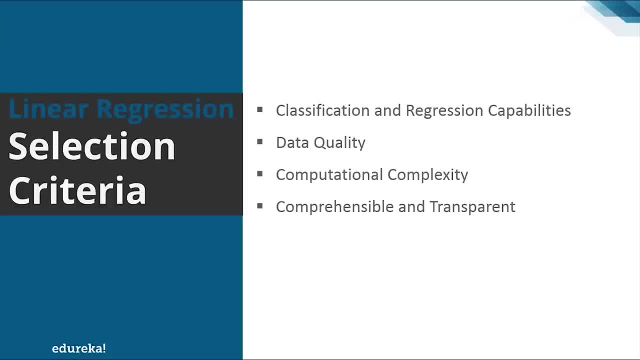 and transparent in nature. They can be represented by a simpler mathematical notation to anyone and can be understood very easily. So these are some of the criteria based on which you will select the linear regression algorithm. All right. Next is: where is linear regression used? first, 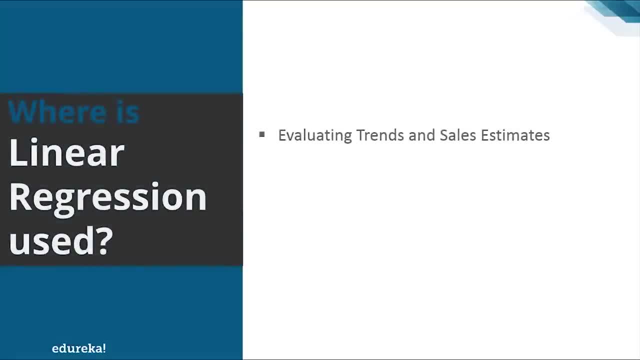 is evaluating Trends and sales estimate. Well, linear regression can be used in business to evaluate Trends and make estimates of forecasts. For example, if a company sale have increased steadily every month for past few years, then conducting a linear analysis on the sales data, with monthly sales on the y-axis. 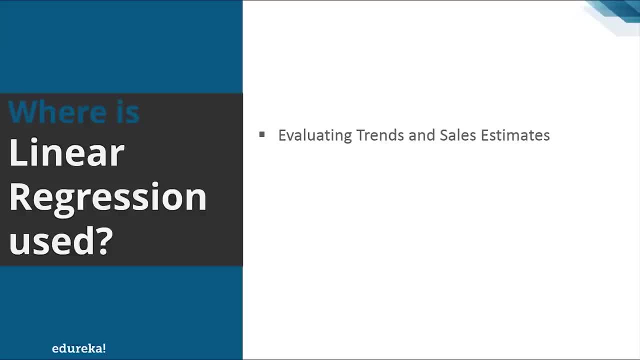 and time on the x-axis. This will give you a line that predicts the upward trends in the sale. after creating the trend line, The company could use the slope of the lines to forecast sale in future months. Next is analyzing the impact of price changes. 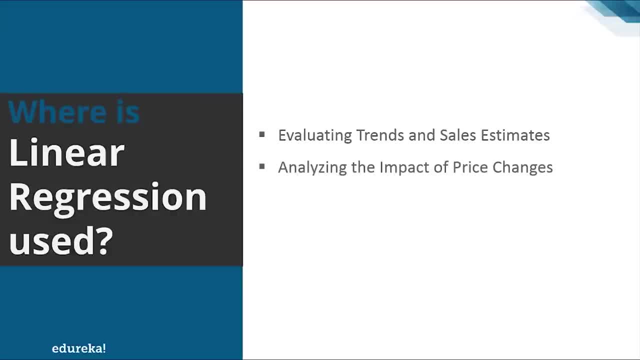 Well, linear regression can be used to analyze the effect of pricing on consumer behavior. For instance, if a company changes the price on a certain product several times, then it can record the quantity itself for each price level and then perform a linear regression with sole quantity as a dependent variable. 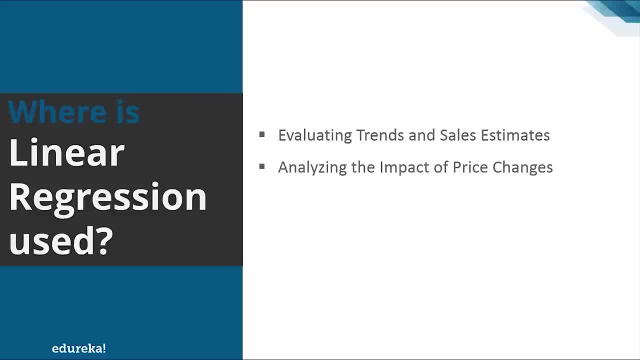 and price as the independent variable. This would result in a line that depicts the extent to which the customer reduce their consumption of the product as the price is increasing. So this result would help us in future pricing decisions. Next is assessment of risk in the financial services and insurance domain. 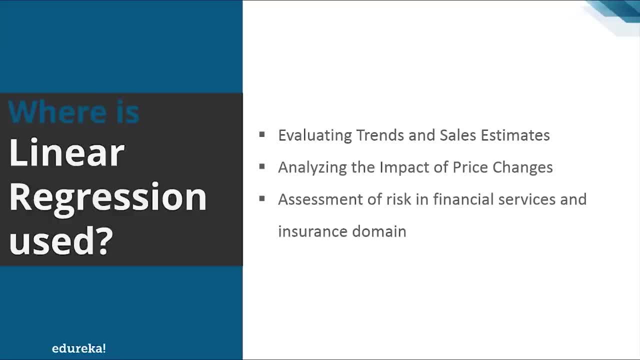 Well, linear regression can be used to analyze the risk. For example, a health insurance company might conduct a linear regression algorithm. How it can do? it can do it by plotting the number of claims per customer against its age, and they might discover that the old customers tend to make more health insurance claim. 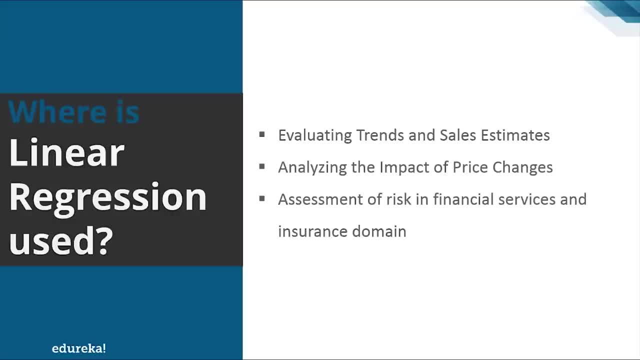 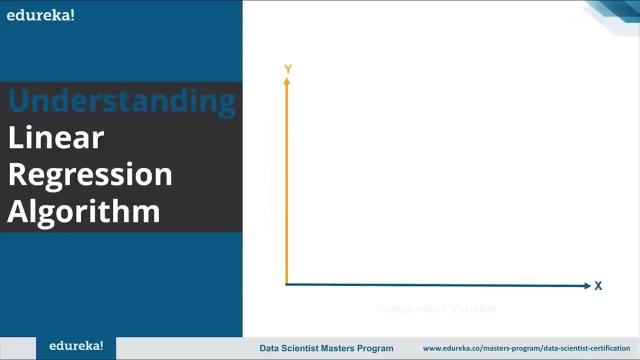 Well, the result of such an analysis might guide important business decisions. All right, So by now you have just a rough idea of what linear regression algorithm is like, what it does, where it is used, when you should use it. All right, Now let's move on and understand the algorithm in depth. 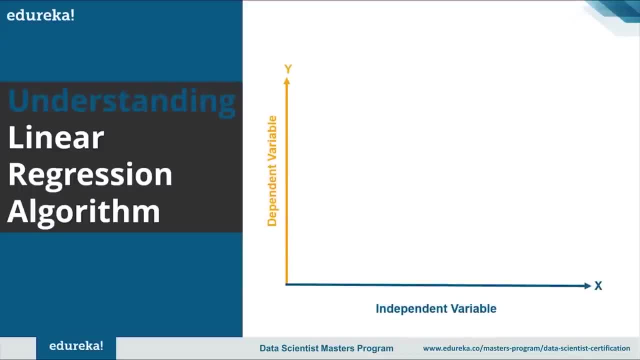 So suppose you have independent variable on the x-axis and dependent variable on the y-axis. All right, Suppose this is the data point on the x-axis. The independent variable is increasing on the x-axis and so does the dependent variable on the y-axis. 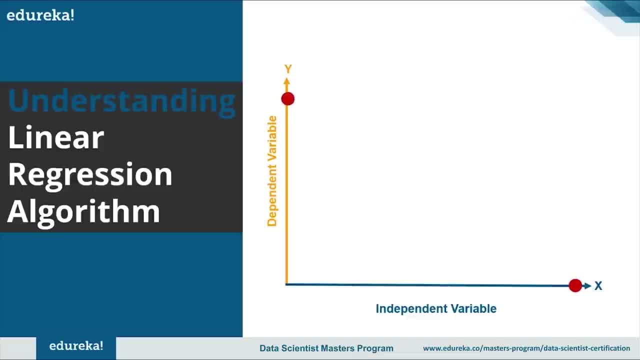 So what kind of linear regression line you would get? you'd get a positive linear regression line, All right, as the slope would be positive. next is suppose you have an independent variable on the x-axis which is increasing and, on the other hand, the dependent variable on the y-axis. 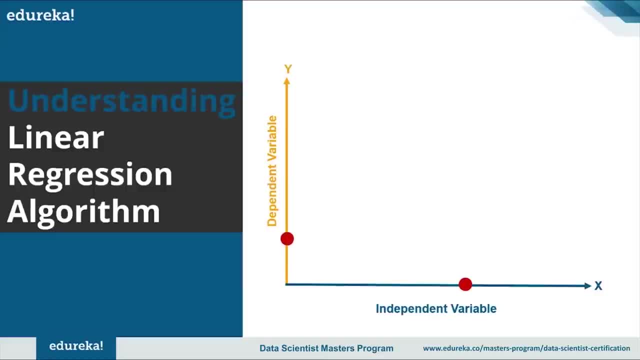 that is decreasing. So what kind of line will you get in that case? You will get a negative regression line in this case, as the slope of the line is negative, and this particular line, that is, line of y equal MX plus C, is a line of linear regression which shows the relationship. 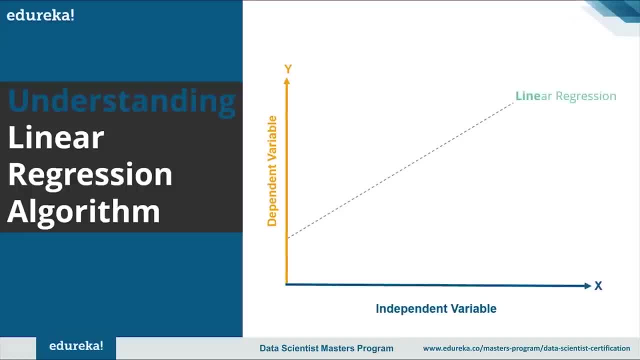 between independent variable and dependent variable, and this line is only known as line of linear regression. Okay, so let's add some data points to our graph. So these are some observation or data points on our graphs. Let's plot some more. Okay, 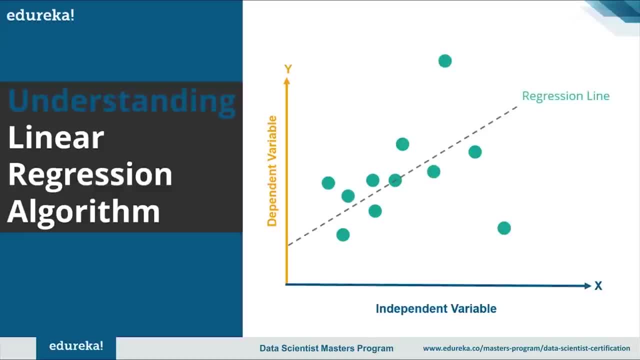 Now all our data points are plotted. now our task is to create a regression line, or the best fit line. All right, Now, once our regression line is drawn, now it's the task of prediction. Now suppose this is our estimated value or the predicted value, and there's our actual value. 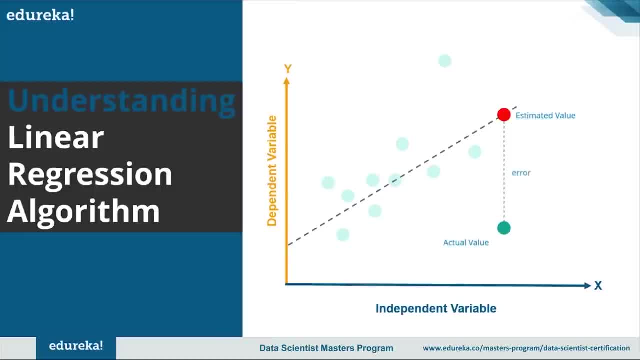 Okay, So what we have to do, our main goal, is to reduce this error, that is, to reduce the distance between the estimated or the predicted value and the actual value. the best fit line would be the one which had the least error or the least difference in estimated value and the actual value. 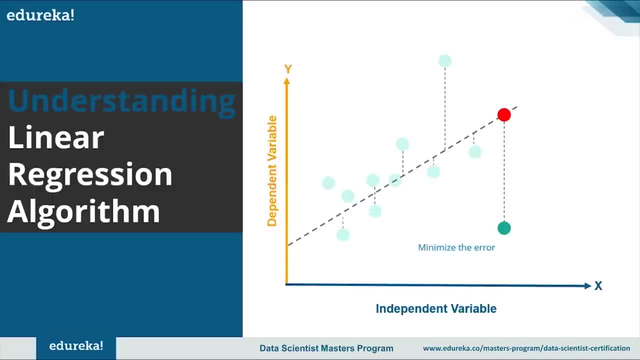 All right. In other words, we have to minimize the error. This was a brief understanding of linear regression algorithm. soon will jump to its mathematical implementation, All right, but for then let me tell you this: suppose you draw a graph with speed on the x-axis and distance covered on the y-axis. 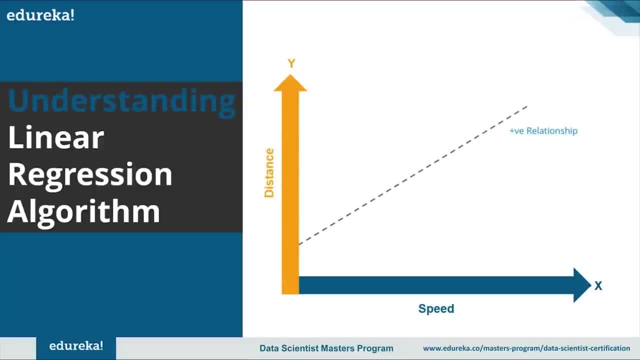 with the time remaining constant. If you plot a graph between the speed traveled by the vehicle and the distance traveled in a fixed unit of time, then you will get a positive relationship. All right, So suppose the equation of line is y equal MX plus C. 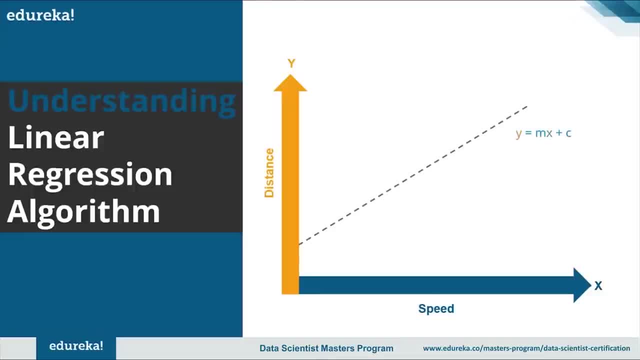 Then, in this case, why is the distance traveled in a fixed duration of time? X is the speed of vehicle, M is the positive slope of the line and C is the y-intercept of the line. All right, Suppose the distance remaining constant. You have to plot a graph between the speed of the vehicle. 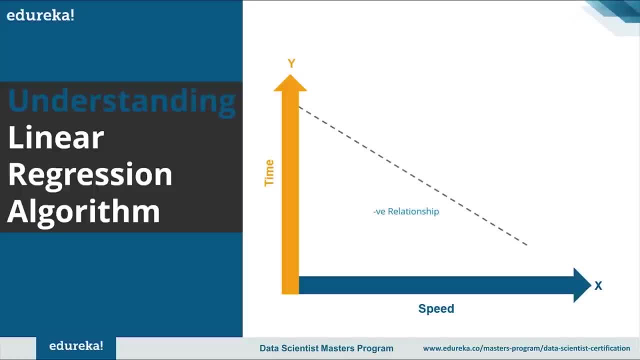 and the time taken to travel a fixed distance, Then in that case you will get a line with a negative relationship. All right, the slope of the line is negative. here The equation of line changes to y equal minus of MX plus C, where Y is the time taken to travel a fixed distance, X is 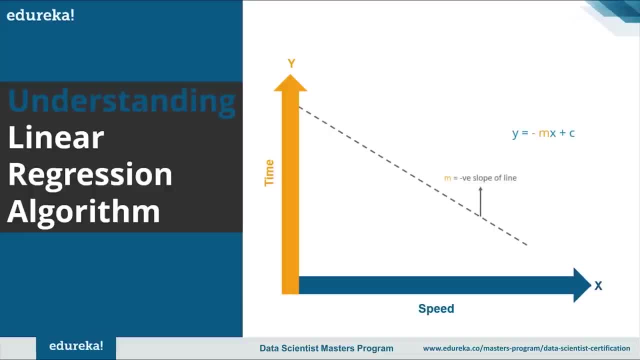 the speed of vehicle. M is the negative slope of the line and C is the y-intercept of the line. All right, Now let's get back to our independent and dependent variable. So in that term, Y is our dependent variable and X, that is our independent variable. 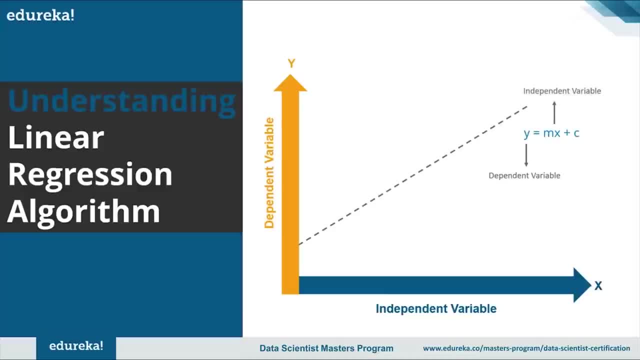 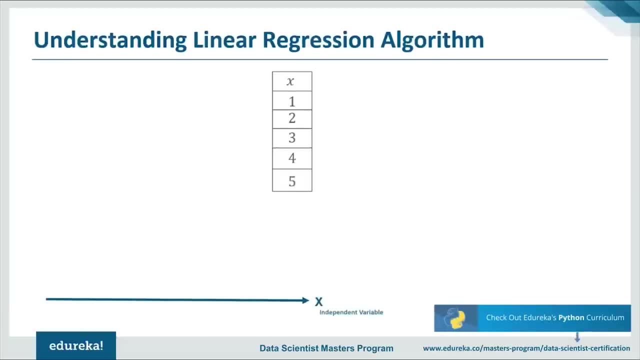 Now let's move on and see the mathematical implementation of the things. All right, So we have X equal 1, 2, 3, 4, 5.. Let's plot them on the x-axis, So 0, 1, 2, 3, 4, 5, 6.. 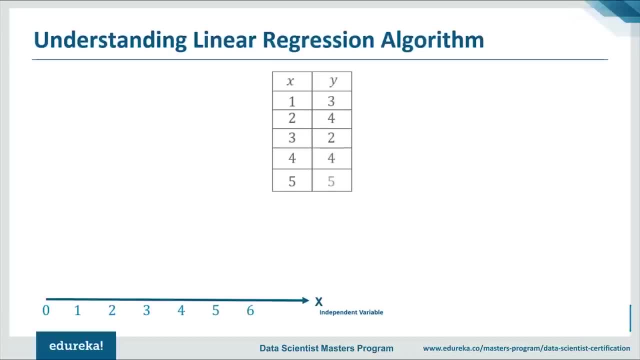 All right, and we have Y as 3, 4, 2, 4, 5.. All right, So let's plot 1, 2, 3, 4, 5 on the y-axis. Now let's plot our coordinates 1 by 1.. 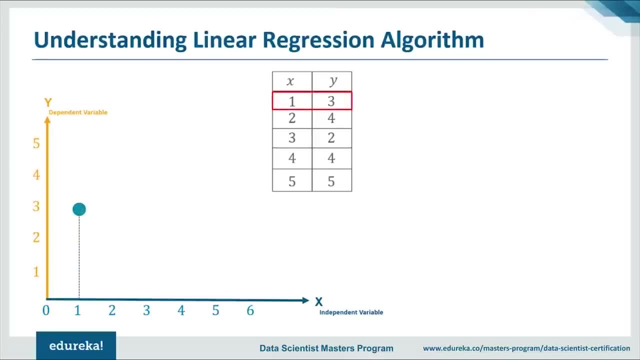 So X equal 1 and y equal 3. So we have here X equal 1 and y equal 3.. So this is our point, 1 comma 3.. So similarly we have 1, 3, 2, 4, 3, 2, 4, 4 and 5, 5.. 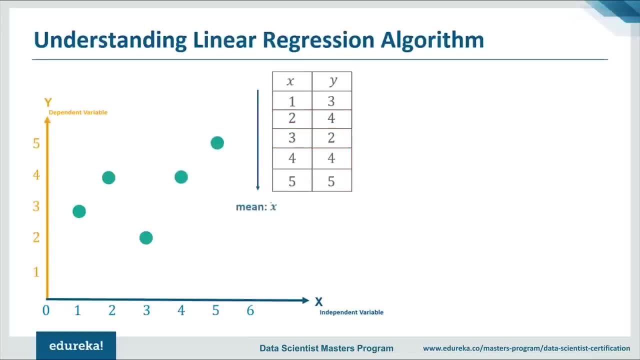 All right, So, moving on ahead, let's calculate the mean of X and Y and plot it on the graph. All right, So mean of X is 1 plus 2 plus 3 plus 4 plus 5, divided by 5, that is 3.. 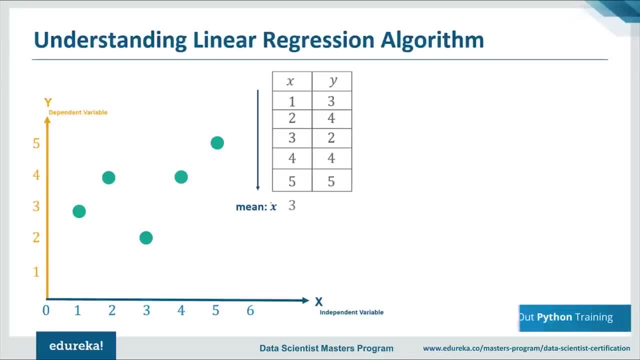 All right. Similarly mean of Y is 3 plus 4 plus 2 plus 4 plus 5, that is 18.. So 18 divided by 5, that is nothing but 3.6.. All right, So next, what we'll do will plot our mean, that is 3 comma 3.6. 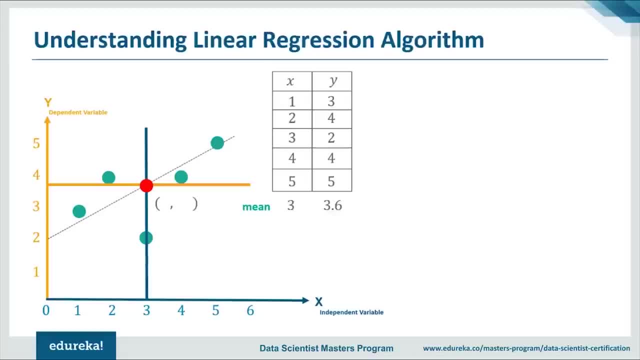 on the graph. Okay, so there's a point 3, comma 3.6.. See, our goal is to find or predict the best fit line using the least square method. All right, So in order to find that, we first need to find the equation. 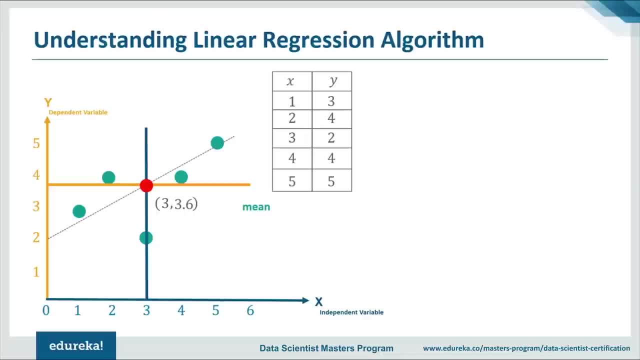 of line. So let's find the equation of our regression line. All right, So let's suppose this is our regression line: Y equal MX plus C. Now we have a equation of line. So all we need to do is find the value of M and C. 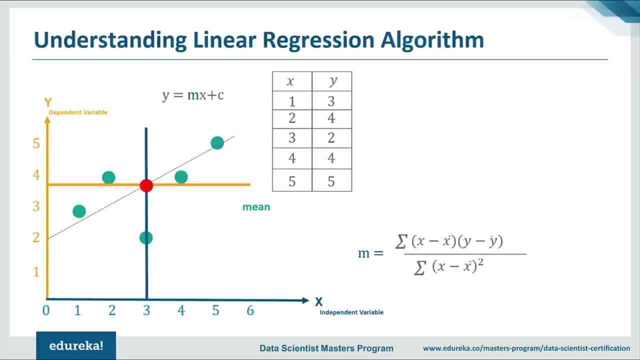 where M equals summation of X minus X bar multiplied by Y minus Y bar. upon the summation of X minus X bar, whole square. Don't get confused. Let me resolve it for you, All right. So moving on ahead as a part of formula. 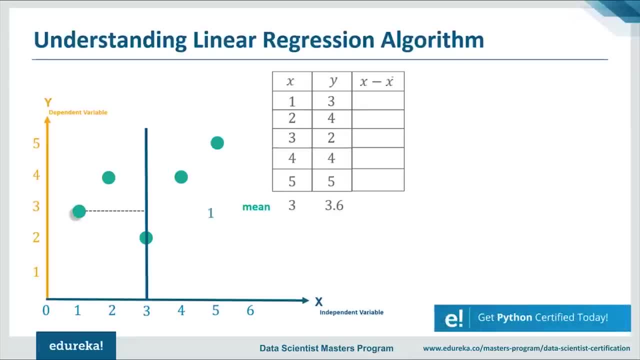 what we are going to do will calculate X minus X bar. So we have X as 1 minus X bar as 3.. All right, So 1 minus 3, that is minus 2. next, We have X equal to minus its mean, 3, that is minus 1.. 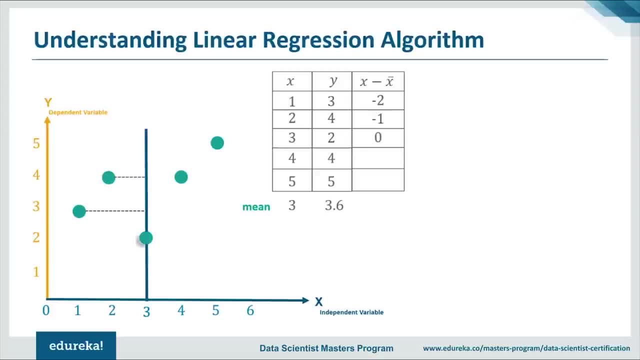 Similarly, We have 3 minus 3, 0, 4 minus 3, 1, 5 minus 3, 2.. All right, So X minus X bar, It's nothing but the distance of all the point through the line Y equal 3. and what does this Y minus Y bar implies? 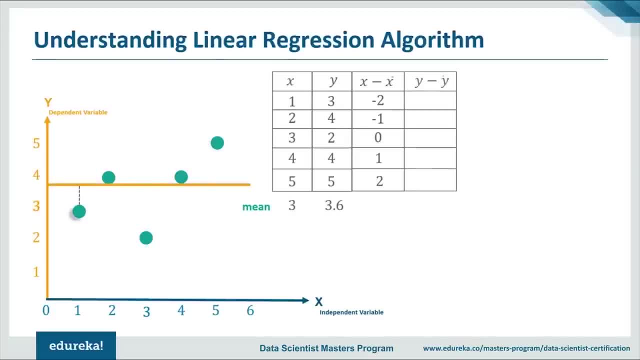 It implies the distance of all the point from the line X equal 3.6.. Fine, So let's calculate the value of Y minus Y bar. So, starting with Y equal 3, minus value of Y bar, that is 3.6.. 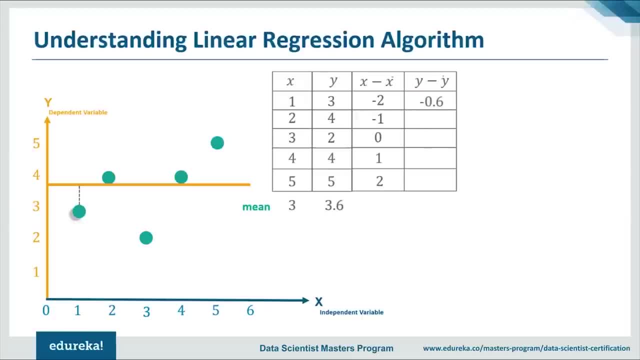 So it is 3 minus 3.6.. How much minus of 0.6. next is 4 minus 3.6.. That is 0.4. next 2 minus 3.6.. That is minus of 1.6.. 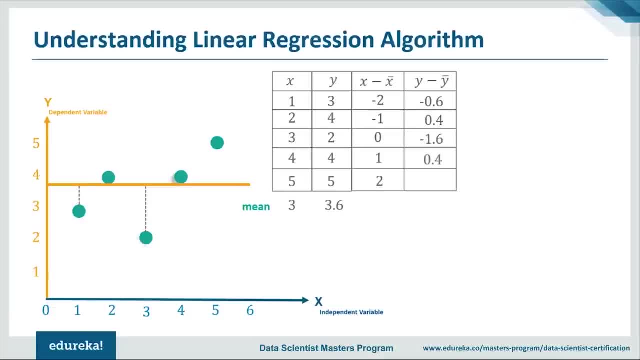 Next is 4 minus 3.6.. That is 0.4. again 5 minus 3.6.. That is 1.4.. All right, So now we are done with Y minus Y bar. fine, Now next we'll calculate X minus X bar whole square. 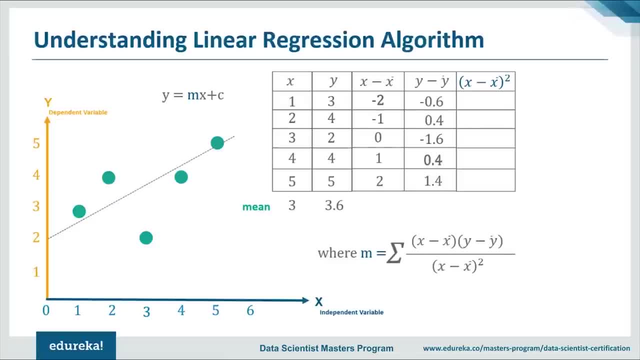 So let's calculate X minus X bar whole square. So it is minus 2 whole square, That is 4 minus 1 whole square, That is 1, 0 square 0, 1 square 1, 2 square 4. fine, 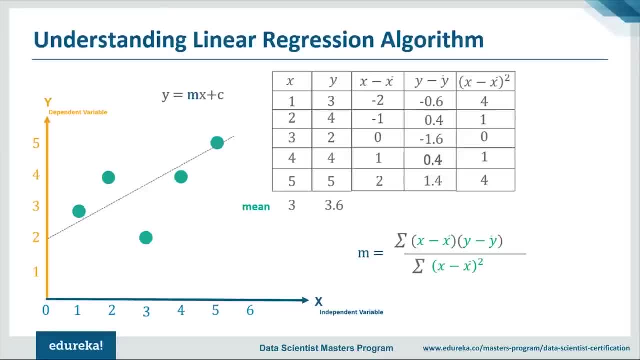 So now in our table We have X minus X bar, Y minus Y bar and X minus X by whole square. Now what we need? we need the product of X minus X bar multiplied by Y minus Y bar. All right, So let's see the product of X minus X bar multiplied by Y minus Y bar. 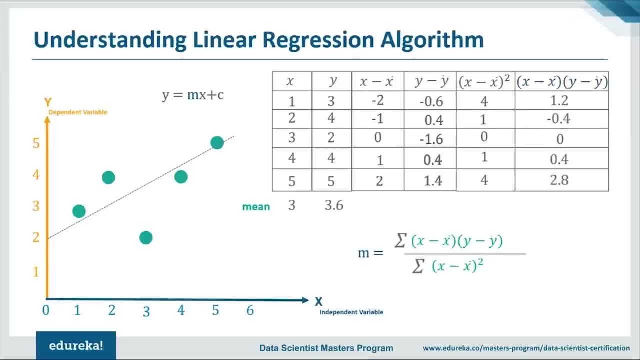 that is minus of 2 multiplied by minus of 0.6.. That is 1.2 minus of 1 multiplied by 0.4.. That is minus of 0.4, 0 multiplied by minus of 1.6.. 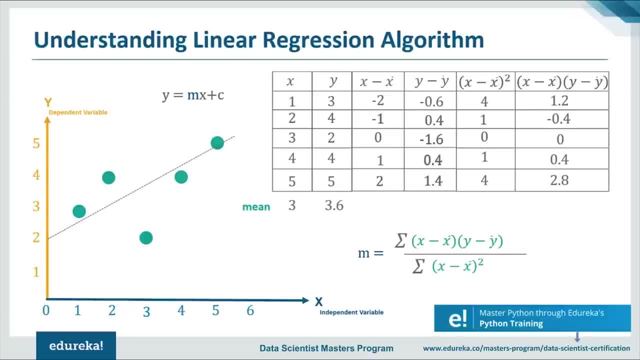 That is 0, 1 multiplied by 0.4.. That is 0.4. and next, 2 multiplied by 1.4.. That is 2.8.. All right, Now almost all the parts of our formula is done. 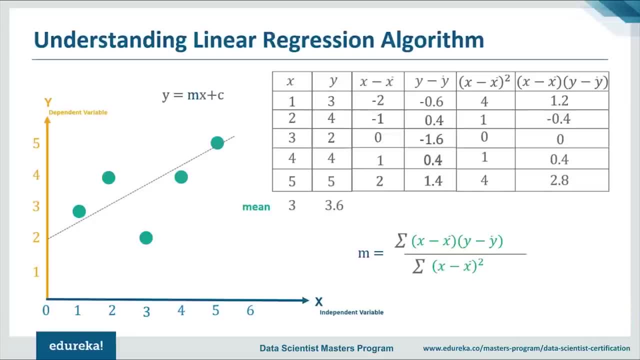 So now what we need to do is get the summation of last two columns, All right. So the summation of X minus X bar whole square is 10, and the summation of X minus X bar multiplied by Y minus Y bar is 4.. 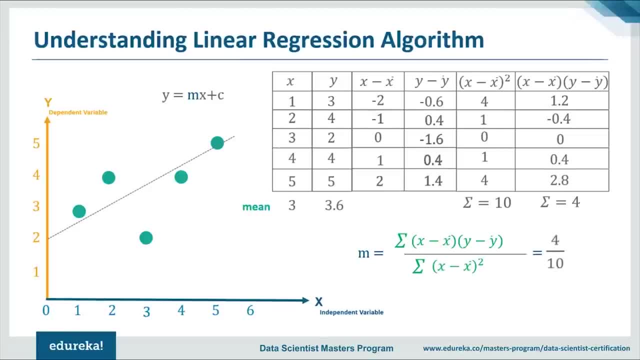 So the value of M will be equal to 4 by 10. fine, So let's put this: value of M equals 0.4 in our line, Y equal MX plus C. So let's fill all the points into the equation and find the value of C. 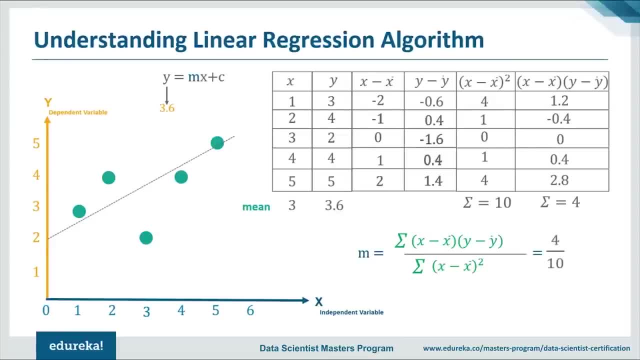 So we have Y as 3.6.. Remember the mean way: M as 0.4, which we calculated just now. X as the mean value of X, that is 3, and we have the equation as: 3.6 equals 0.4. 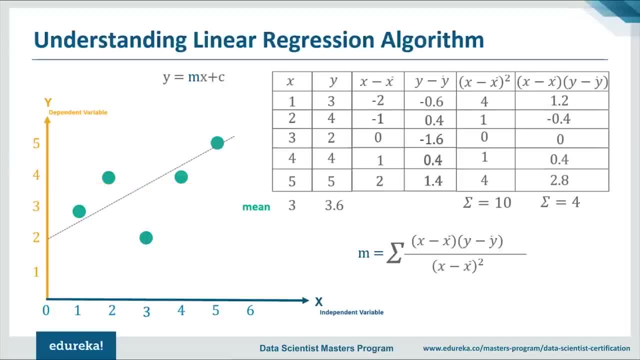 multiplied by 3 plus C. All right, that is 3.6 equal 1.2 plus C. So what is the value of C? That is 3.6 minus 1.2.. That is 2.4.. 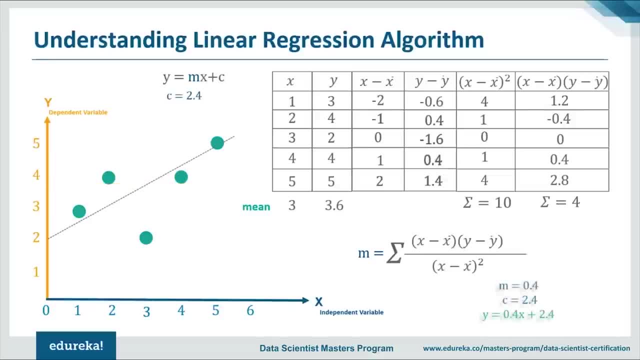 All right. So what we had? we had M equals 0.4 C as 2.4. and then, finally, when we calculate the equation of regression line, what we get is Y equal 0.4 times of X plus 2.4.. 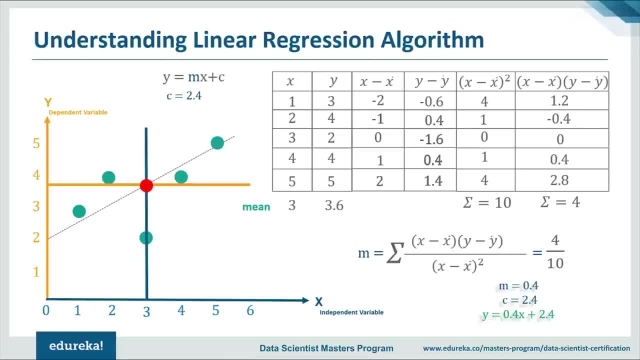 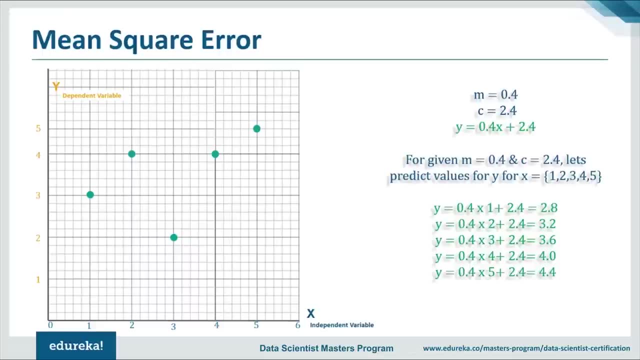 So this is the regression line. All right. So there's how you are plotting your points. This is your actual point. All right, Now for given M equals 0.4 and C equal 2.4.. Let's predict the value of Y for X equal 1, 2, 3, 4 and 5.. 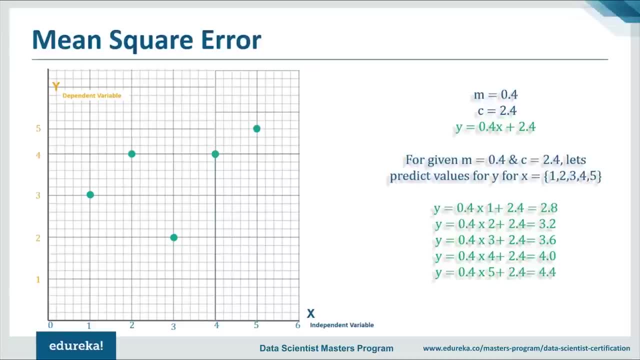 So, when X equal 1, the predicted value of Y will be 0.4 multiplied by 1 plus 2.4.. That is 2.4 plus 2.8. similarly, when X equal 2, predicted value of Y will be 0.4 multiplied by 2 plus 2.4. 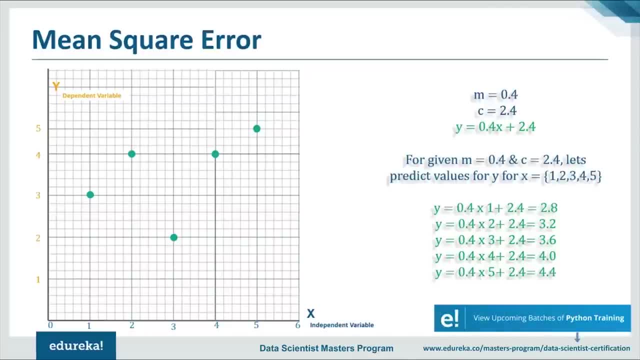 that equals to 3.2.. Similarly, X equal 3- Y will be 3.6. X equal 4- Y will be 4.0. X equal 5- Y will be 4.4.. So let's plot them on the graph. 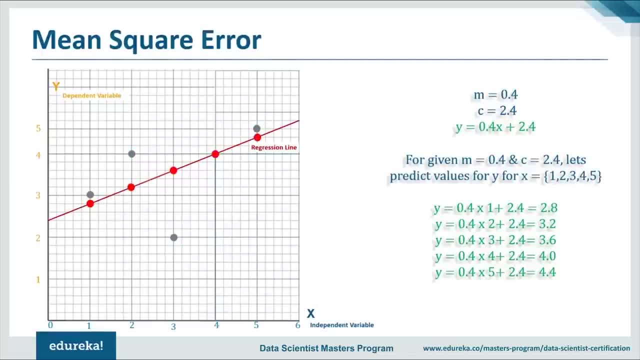 and the line passing through all these predicting point and cutting y-axis at 2.4 is the line of regression. Now your task is to calculate the distance between the actual and the predicted value, and your job is to reduce the distance. All right, or in other words, you have to reduce the error. 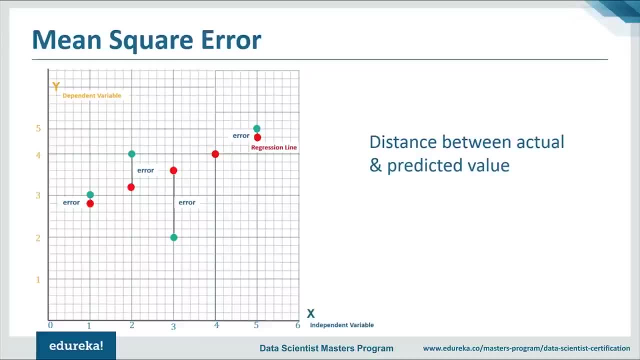 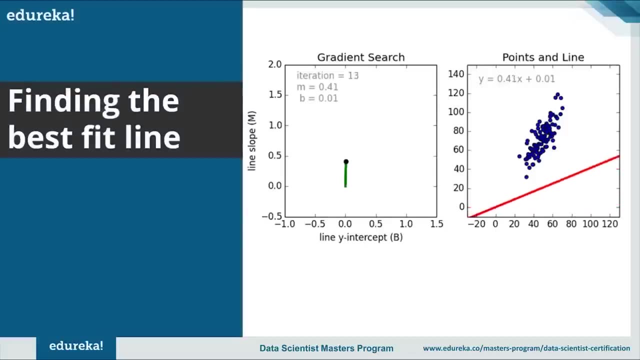 between the actual and the predicted value. the line with the least error will be the line of linear regression or regression line, and it will also be the best fit line. All right, So this is how things work in computer. So what it do, it performs n number of iteration. 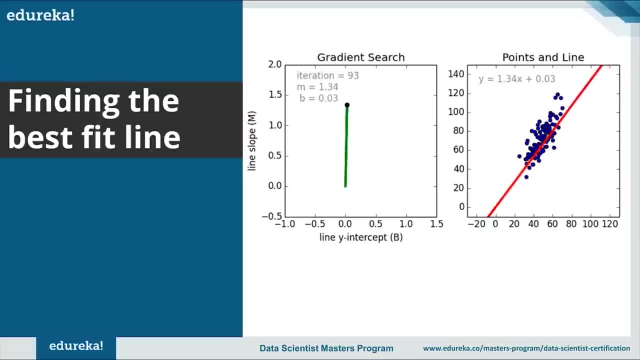 for different values of M. for different values of M, It will calculate the equation of line Y equal MX plus C right. So as the value of M changes, the line is changing. So iteration will start from one All right and it will perform n number of iteration. 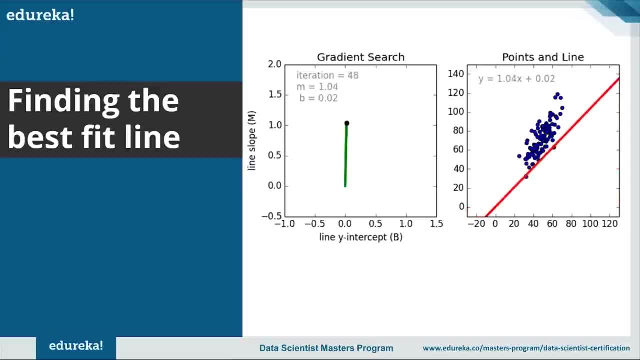 So, after every iteration, what it will do? it will calculate the predicted value according to the line and compare the distance of actual value to the predicted value, and the value of M, for which the distance between the actual and the predicted value is minimum, will be selected as the best fit line. 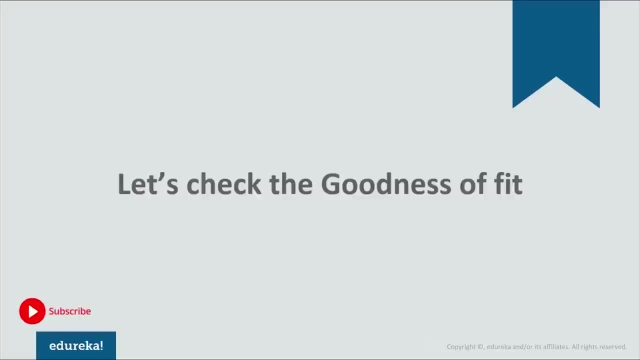 All right, Now that we have calculated the best fit line, now it's time to check the goodness of it, or to check how good a model is performing. So in order to do that, we have a method called R square method. So what is this R square? 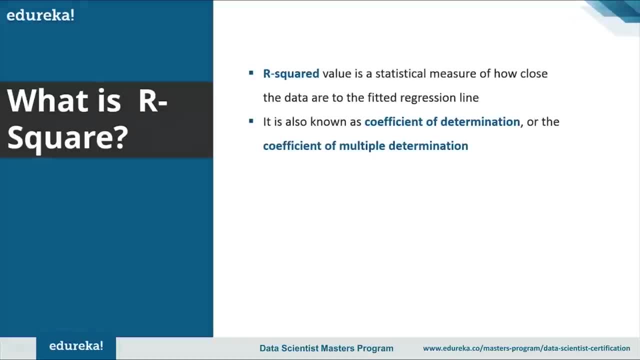 Well, R squared value is a statistical measure of how close the data are to the fitted regression line. in general, It is considered that a higher squared value model is a good model, but you can also have a lower squared value for a good model as well, or a higher squared value. 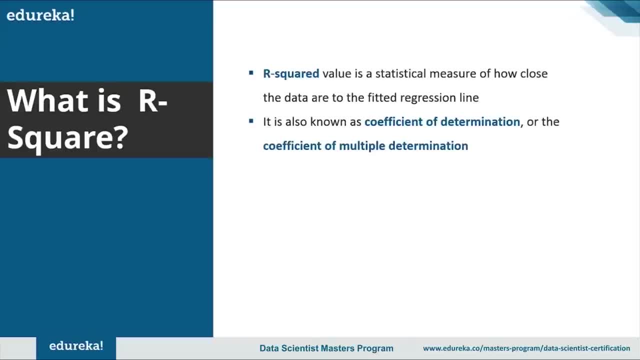 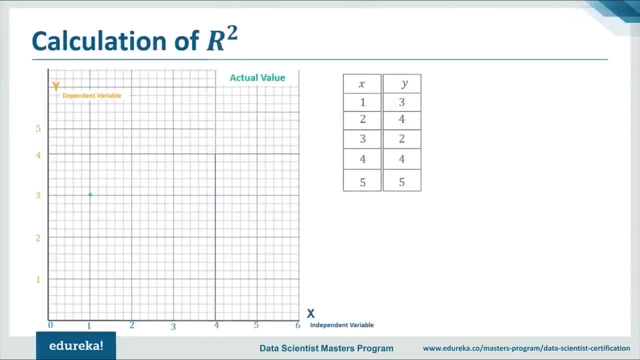 for a model that does not fit at all. All right, It is also known as coefficient of determination or the coefficient of multiple determination. Let's move on and see how R square is calculated. So these are our actual values plotted on the graph. 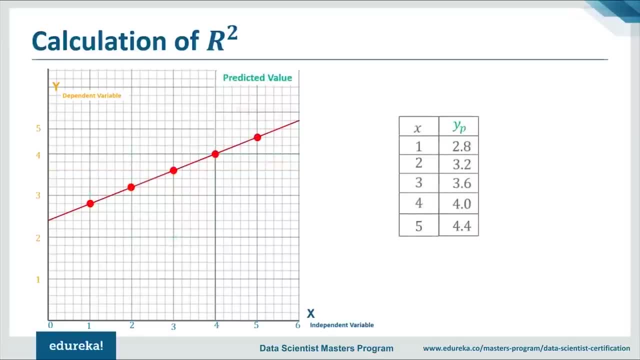 We had calculated the predicted values of Y as 2.8,, 3.2,, 3.6,, 4.0, 4.4.. Remember when we calculated the predicted values of Y for the equation: Y predicted equals 0.4 times of X plus 2.4. 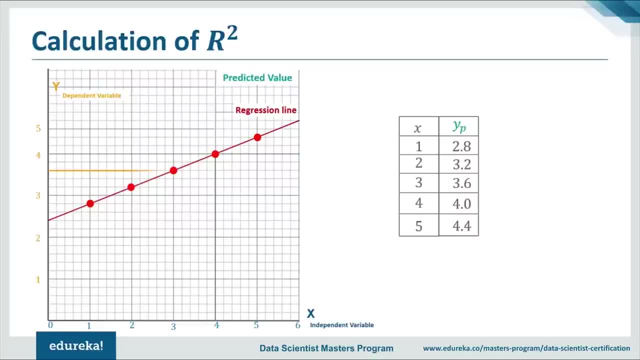 for every X equal 1,, 2,, 3,, 4 and 5.. From there we got the predicted values of Y. All right, So let's plot it on the graph. So these are a point and the line passing through these points are nothing. 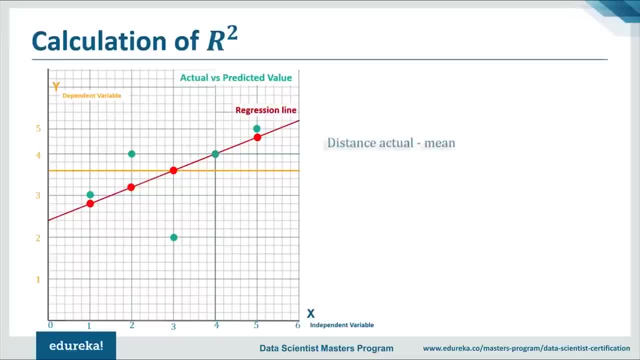 but the regression line, All right. Now what you need to do is you have to check and compare the distance of actual minus mean versus the distance of predicted minus mean, All right. So, basically what you're doing, you're calculating the distance of actual value to the mean. 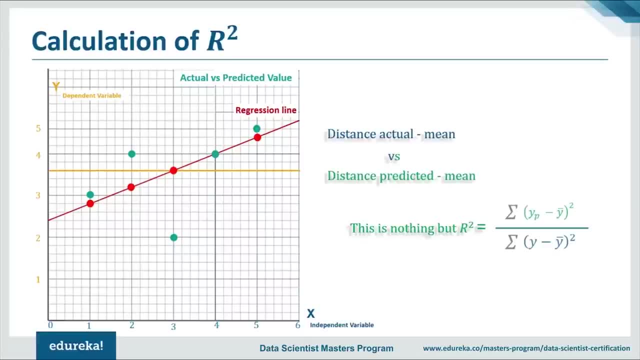 to distance of predicted value to the mean. All right, So there's nothing but R square and mathematically you can represent R square as summation of Y predicted values minus Y bar whole square, divided by summation of Y minus Y bar whole square. 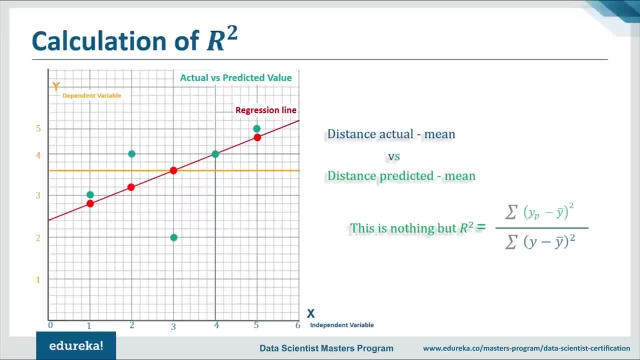 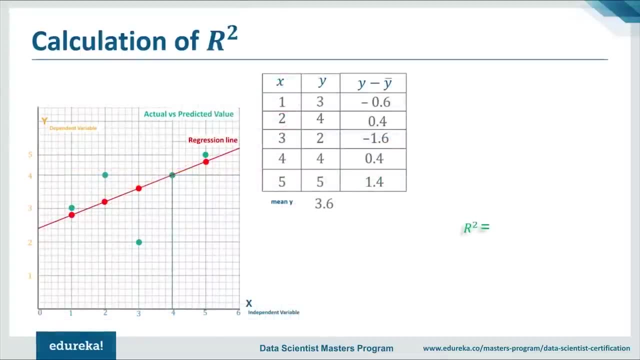 where Y is the actual value, YP is the predicted value and Y bar is the mean value of Y, That is nothing but 3.6.. So remember, this is our formula. So next, what we'll do? we'll calculate Y minus Y bar. 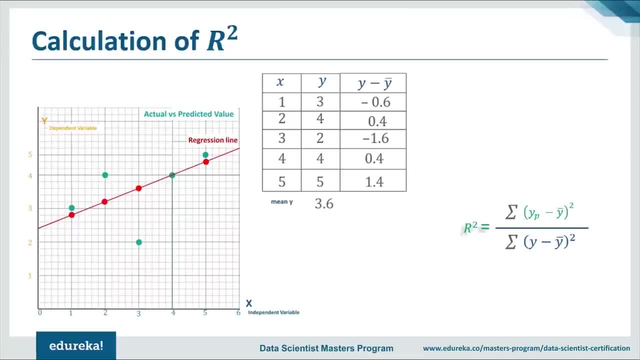 So we have Y as 3, Y bar as 3.6.. So we'll calculate it as 3 minus 3.6.. That is nothing but minus of 0.6.. Similarly for Y equal 4 and Y bar equal 3.6.. 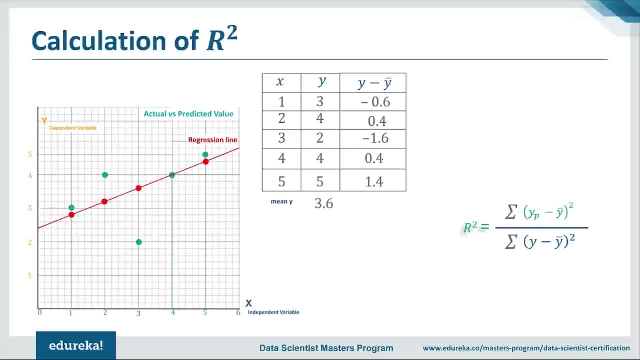 We have Y minus Y bar as 0.4, then 2 minus 3.6.. It is 1.6, 4 minus 3.6, again 0.4, and 5 minus 3.6.. It is 1.4.. 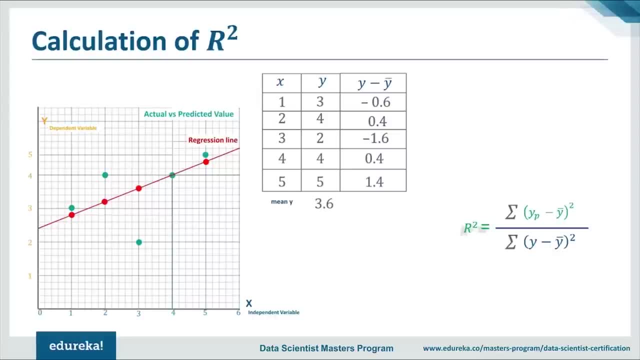 So we got the value of Y minus Y bar. Now what we have to do, We have to take it square. So we have minus of 0.6 square as 0.36, 0.4 square as 0.16, minus of 1.6 square as 2.56, 0.46.. 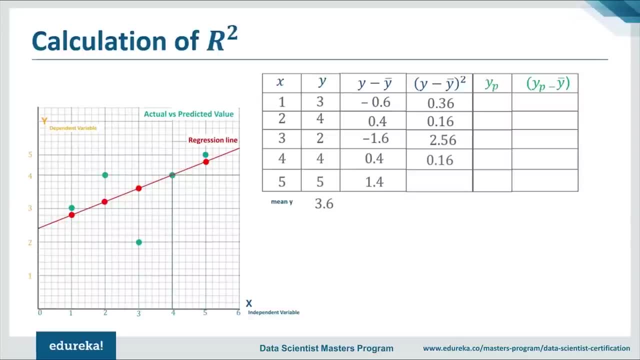 4 square as 0.16 and 1.4 square as 1.96.. Now, as a part of formula, what we need? we need our YP minus Y bar value. So these are YP values and we have to subtract it from the mean of Y. 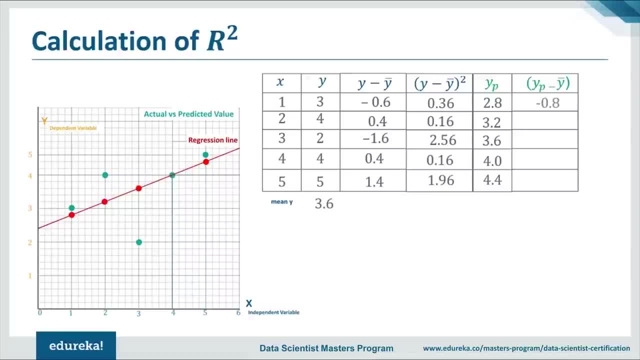 So 2.8 minus 3.6, that is minus 0.8.. Similarly, we'll get 3.2 minus 3.6.. That is 0.4, and 3.6 minus 3.6.. That is 0, 4.0 minus 3.6.. 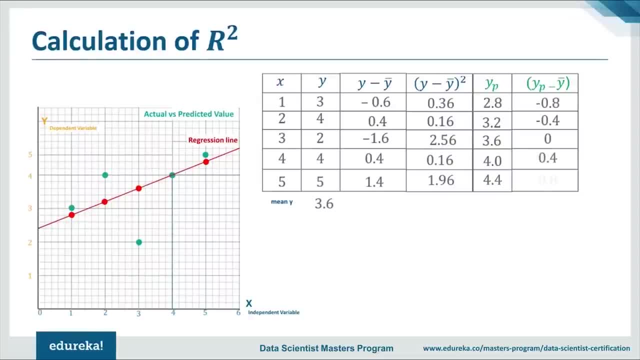 That is 0.4, then 4.4 minus 3.6.. That is 0.8.. So we calculated the value of YP minus Y bar. Now it's our turn to calculate the value of YP minus Y bar whole square. 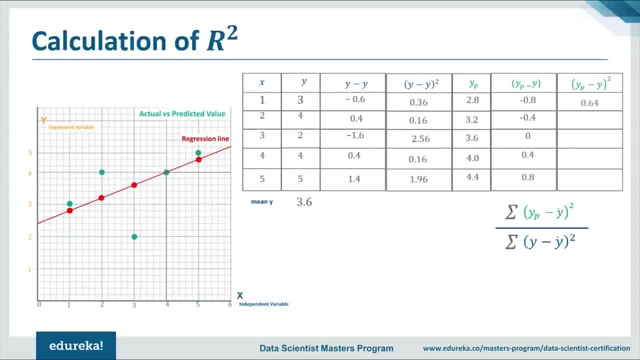 Next, we have minus of 0.8 square as 0.64, minus of 0.4 square as 0.16. 0 square 0, 0.4 square as again 0.16 and 0.8 square as 0.64.. 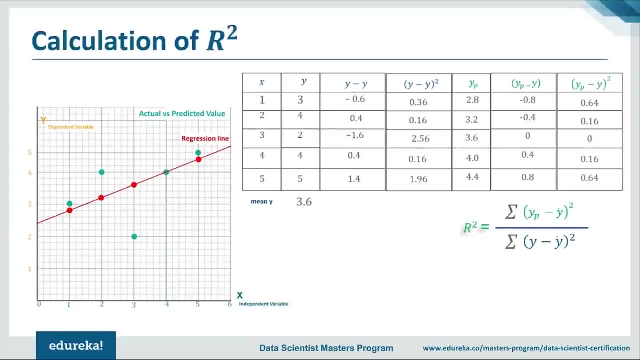 All right, now, as a part of formula, what it suggests? It suggests me to take the summation of YP minus Y bar whole square and summation of Y minus Y bar whole square. All right, let's see. So, on summating Y minus Y bar whole square, what you get is 5.2. 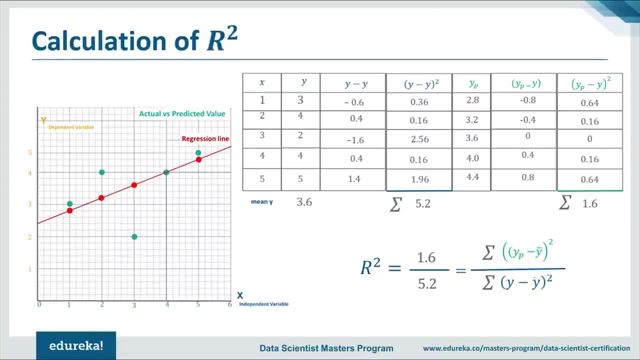 and summation of YP minus Y bar whole square, you get 1.6.. So the value of R square can be calculated as 1.6 upon 5.2. fine, So the result which will get is approximately equal to 0.3.. 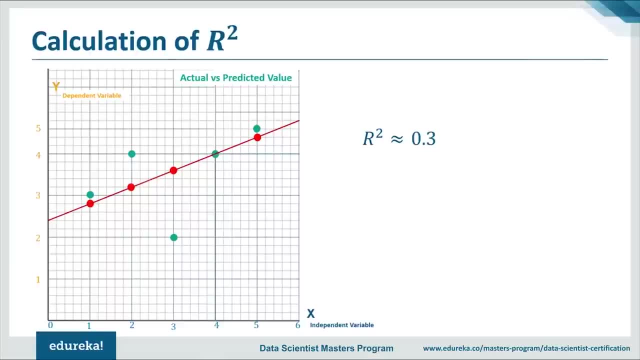 Well, this is not a good fit. All right, so it suggests that the data points are far away from the regression line. All right, So this is how your graph will look like when R square is 0.3, when you increase the value of R square to 0.7.. 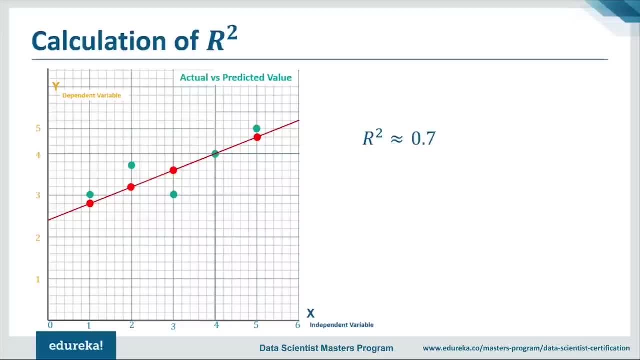 So you'll see that the actual value would lie closer to the regression line when it reaches to 0.9.. It comes more close and when the value approximately equals to 1, then the actual values lies on the regression line itself. For example, in this case, if you get a very low value, 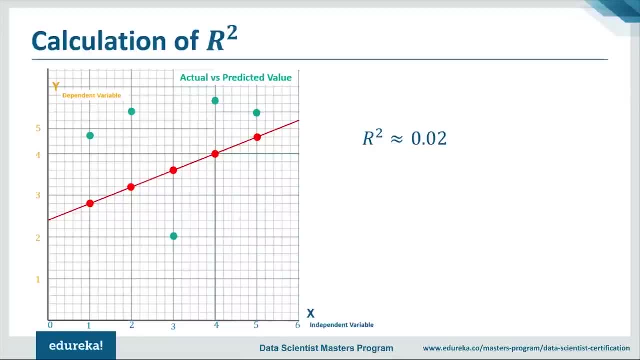 of R square, suppose 0.02.. So in that case, what you'll see? that the actual value is very far away from the regression line, or you can say that there are too many outliers in your data. You cannot forecast anything from the data. 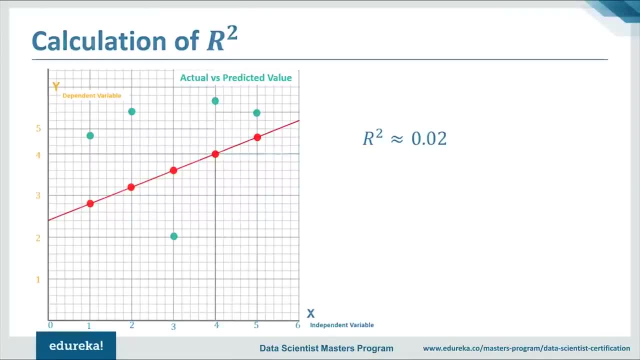 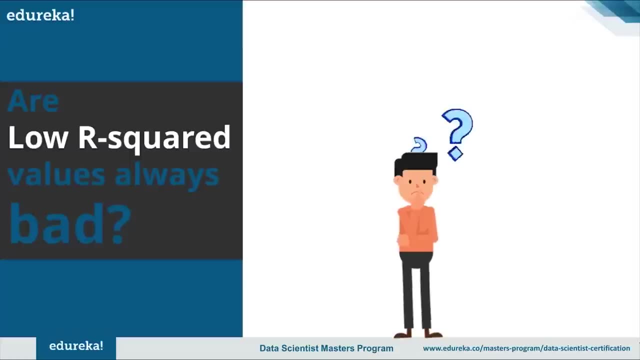 All right, So this was all about the calculation of R square. Now you might get a question: like our low values of R square always bad? Well, in some field it is entirely expected that our R square value will be low, For example, any field that attempts to predict human behavior. 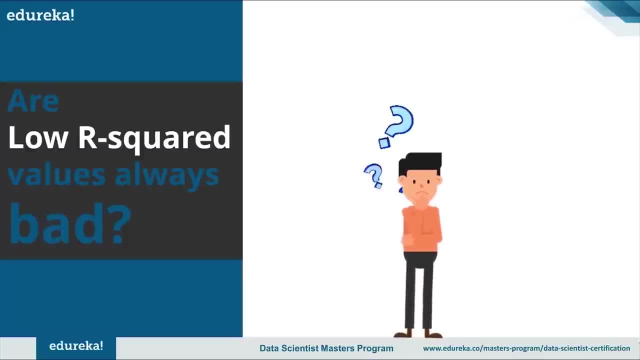 such as psychology, typically has R squared values lower than around 50%, through which you can conclude that humans are simply harder to predict than the physical process. Furthermore, if your R squared value is low but you have statistically significant predicators, then you can still draw important conclusion. 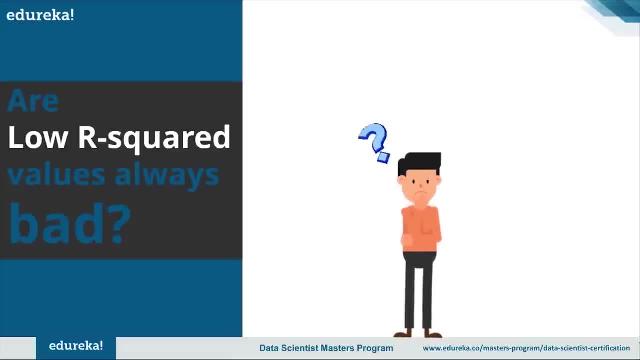 about how changes in the predicator values are associated with the changes in the response value. regardless of the R squared, the significant coefficient still represent the mean change in the response for one unit of change in the predicator, while holding other predicators in the model constant. 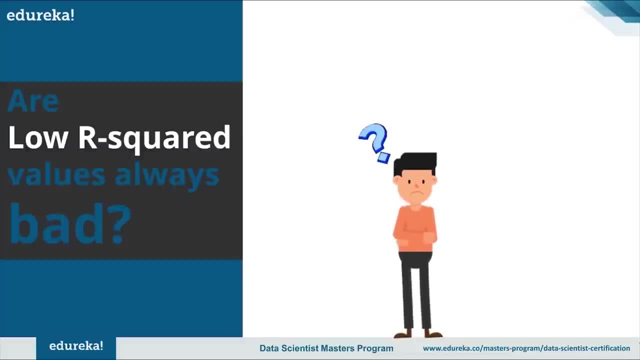 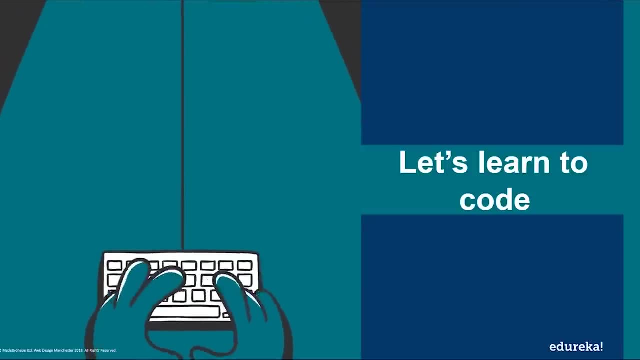 Obviously, This type of information can be extremely valuable. All right, All right. So this was all about the theoretical concept. Now let's move on to the coding part and understand the code in depth. So for implementing linear regression using Python. 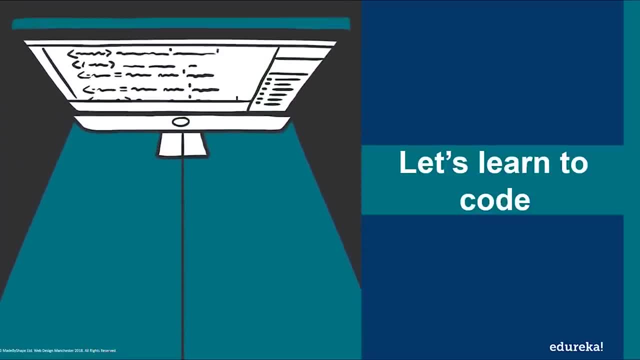 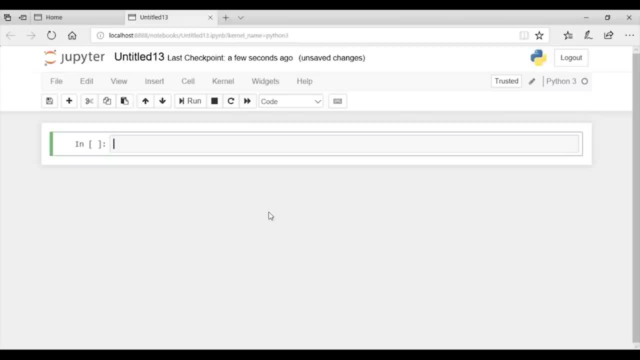 I'll be using anaconda with Jupiter notebook installed on it. So, all right, this is our Jupiter notebook and we are using python 3.0 on it. All right, So we are going to use a data set consisting of head size and human brain of different people. 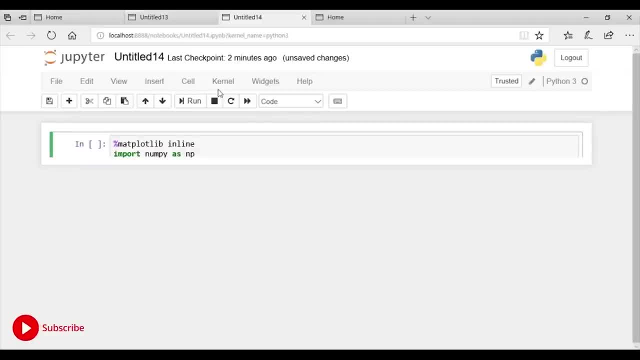 All right. So let's import our data set person matplotlib. in line We are importing numpy as NP, pandas as PD and matplotlib, and from matplotlib We are importing pi, plot of that as PLT. All right, Next we'll import our data head brain dot CSV. 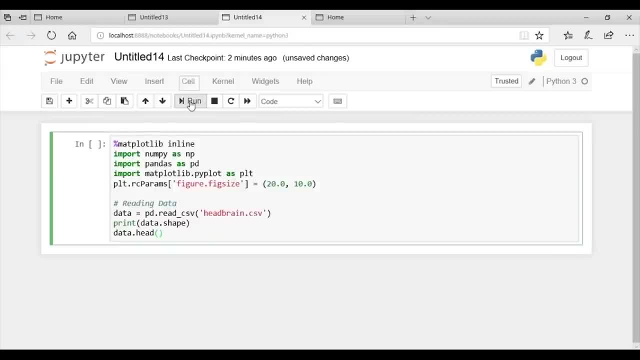 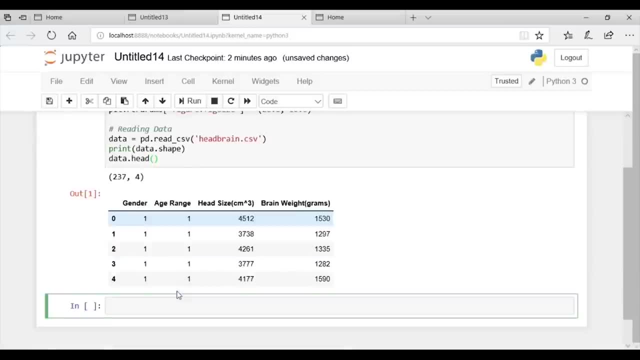 and store it in the data variable. Let's execute the run button and see the output. So this asterisk symbol, it symbolizes that it's still executing. So there's a output. our data set consists of 237 rows and four columns. We have columns as gender, age range, head size. 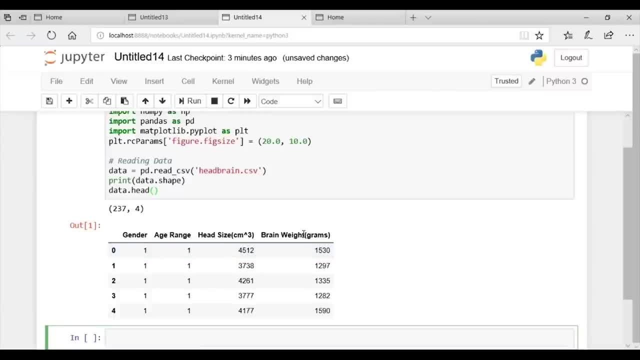 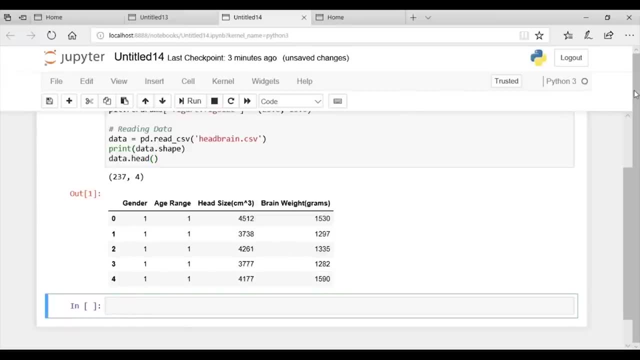 in centimeter cube and brain weights in gram fine. So there's a sample data set. This is how it looks. it consists of all these data set. So now that we have imported our data. So, as you can see, there are 237 values in the training set. 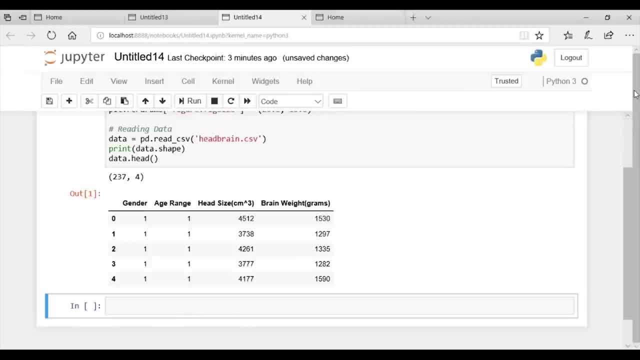 so we can find a linear relationship between the head size and the brain weights. So now, what we'll do will collect X and Y. the X would consist of the head size values and the Y would consist of brain weight values. So, collecting X and Y, let's execute the run. 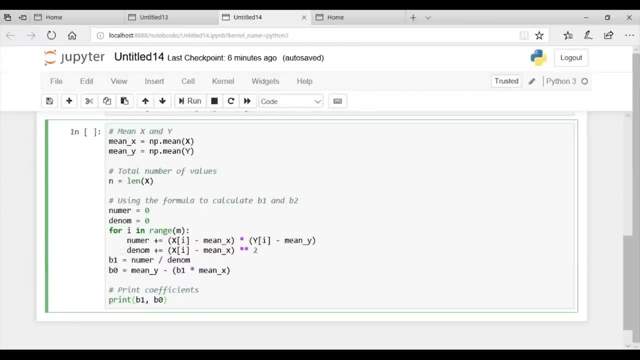 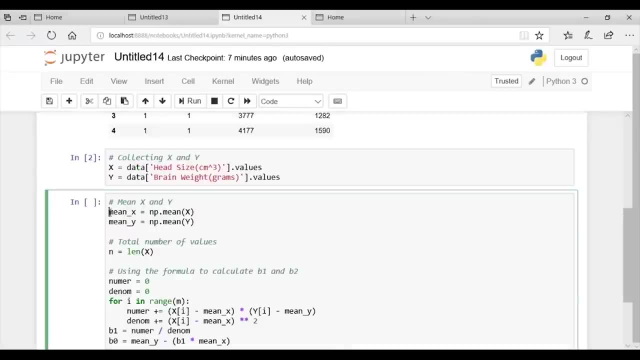 Done. Next, what we'll do. we need to find the values of B1 or B naught, or you can say M and C, So we'll need the mean of X and Y values First of all. what we'll do will calculate the mean of X and Y. 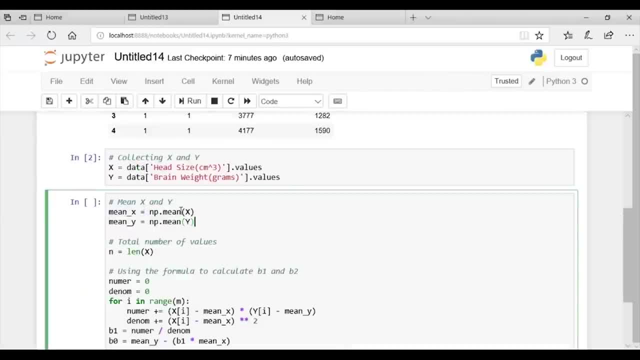 So mean X: equal NP dot mean X. So mean is a predefined function of number. Similarly, mean underscore Y: equal NP dot mean of Y. So what it says, if we'll return, if we'll return the mean values of Y, next we'll check the total number of values. 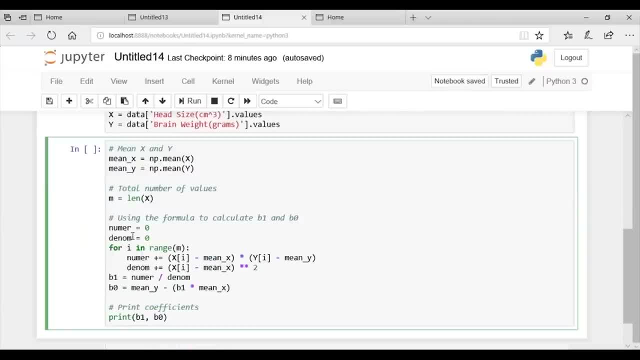 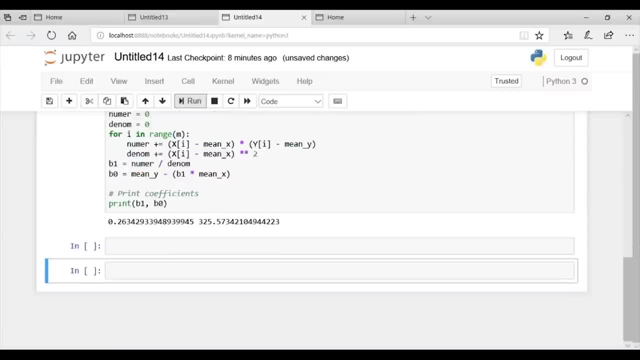 So M equal length of X. All right, then we'll use the formula to calculate the values of B1 and B, naught, or M and C. All right, let's execute the run button and see what is the result. So, as you can see here on the screen, 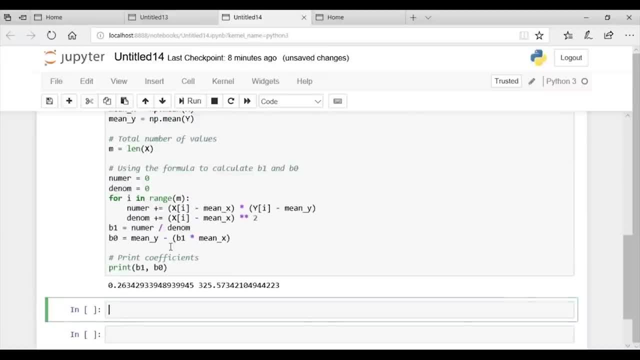 we have got B1 as 0.263 and B naught as 325.57.. All right, So now that we have our coefficient, so comparing it with the equation Y equals MX plus C, you can say that brain weight equals 0.263. 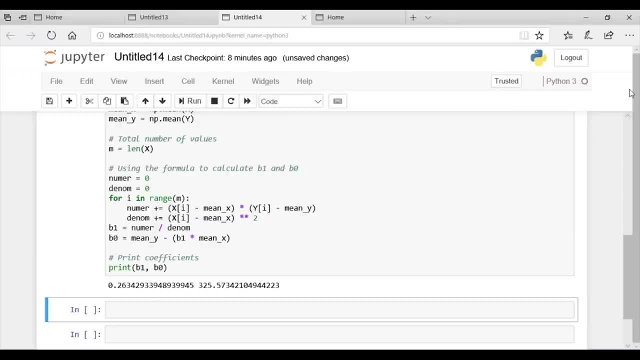 multiplied by head size plus 325.57.. So you can say that the value of M here is 0.263 and the value of C here is 325.57.. All right, So there's our linear model. Now let's plot it and see graphically. 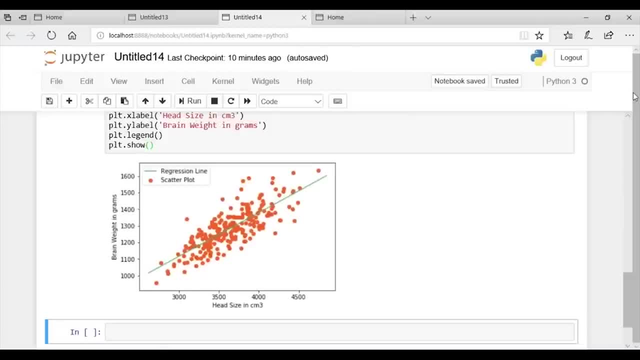 Let's execute it. So this is how our plot looks like. this model is not so bad, but we need to find out how good our model is. So, in order to find it that many methods like root mean square method, the coefficient, or determination, or the R square method, 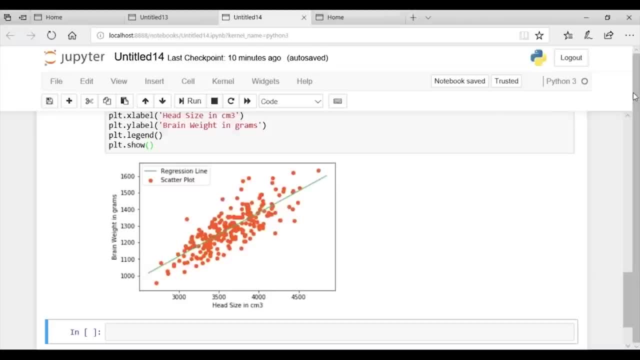 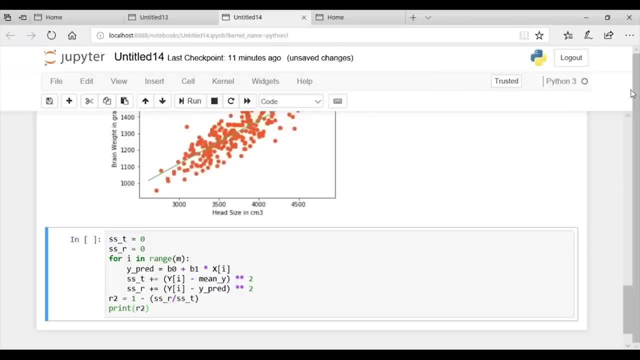 So in this tutorial I have told you about R square method, So let's focus on that and see how good our model is. So let's calculate the R square value. All right here. SS underscore T is the total sum of square. SS underscore R is the total sum of square of residuals. 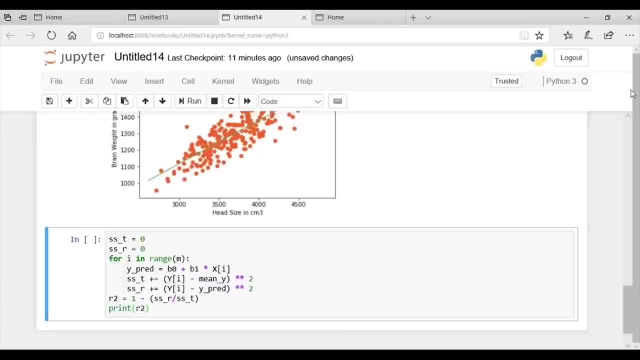 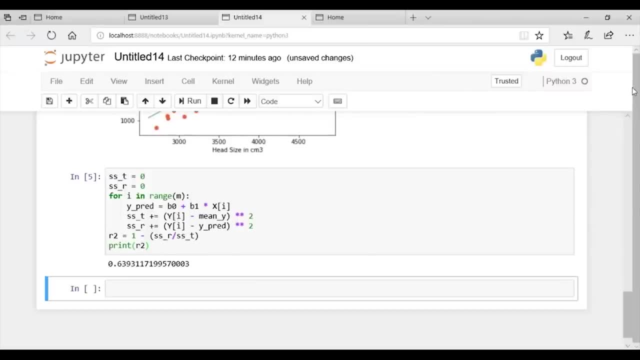 and R square, as the formula is 1 minus total sum of squares upon total sum of square of residuals. All right. next, when you execute it, you will get the value of R square as 0.63, which is pretty, very good Now that you have implemented simple linear regression model. 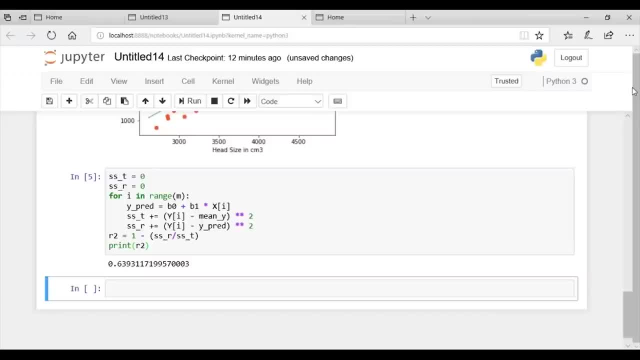 using least square method. Let's move on and see how will you implement the model using machine learning library called scikit-learn. All right, So this scikit-learn is a simple machine learning library in Python. building machine learning model are very easy. 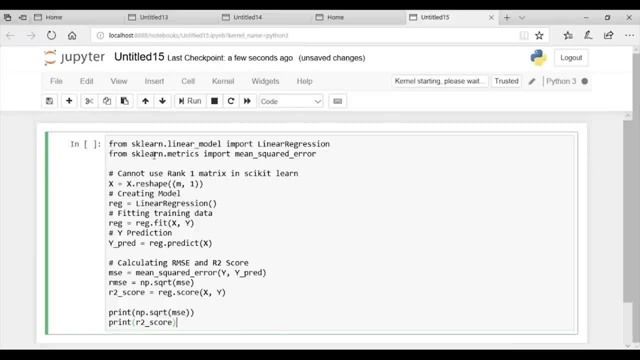 using scikit-learn. So suppose there's a python code. So using the scikit-learn libraries, your code shortens to this length. All right, so let's execute the run button and see you'll get the same R2 score as. 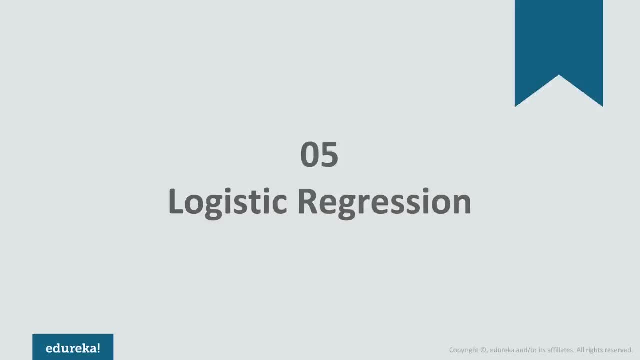 Well, this was all for today's discussion. Most of the entities in this world are related in one way or another. at times, finding relationship between entities can help you take valuable business decisions. Today, I'm going to talk about logistic regression, which is one such approach towards predicting relationships. 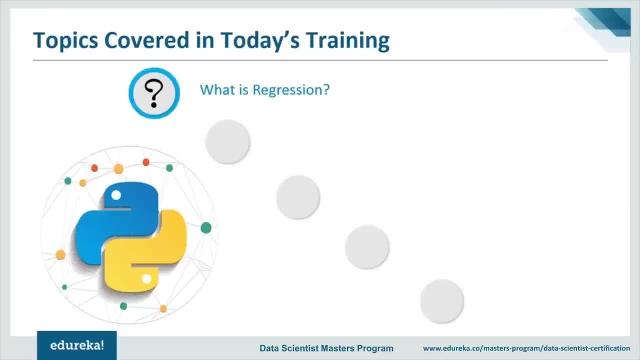 and let us see what all we're going to cover in today's training. So we'll start off the session by getting a quick introduction to what is regression. then we'll see the different types of regression and we'll be discussing the what and why of logistic regression. 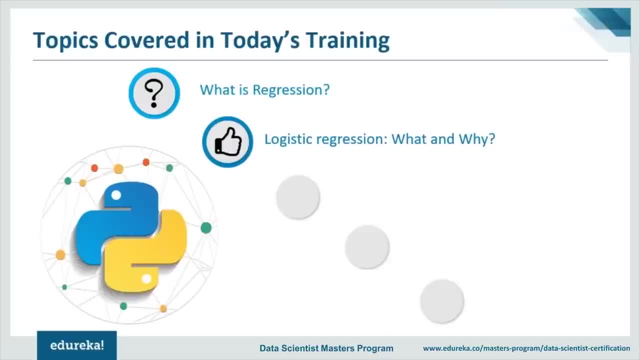 So in this part we'll discuss what exactly it is, where it is used, why it is used and all those things. moving ahead will compare linear regression versus logistic regression, along with the various real-life use cases, And finally, towards the end, I'll be practically implementing logistic regression algorithm. 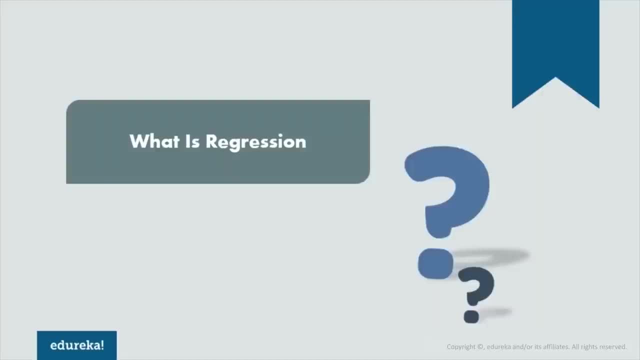 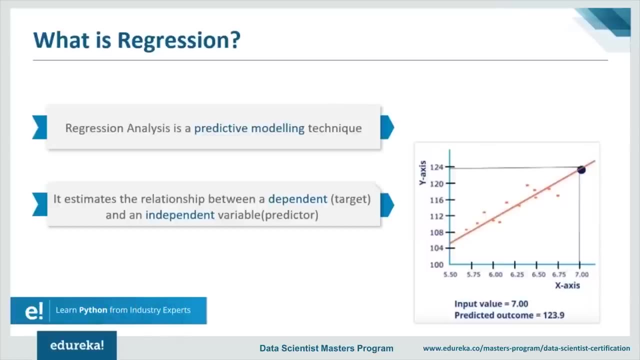 So let's quickly start off with the very first topic. What is regression? now, regression analysis is a predictive modeling technique that always involves predictions. So in this session we'll just talk about predictive analysis and not prescriptive analysis. Now why? because in prescriptive analysis, 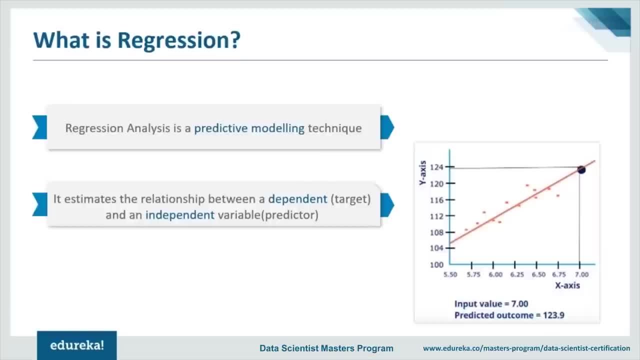 you need to have a good base and a strong hold on the predictive part first. Now it estimates relationship between the dependent variable and an independent variable. So for those of you who are not aware of these terminologies, let me give you a quick summary of it. 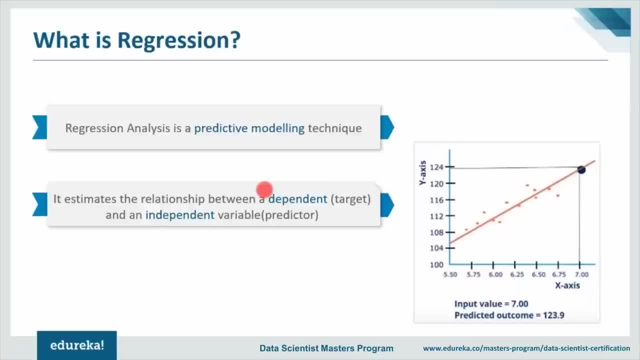 So dependent variable is nothing but a variable which you want to predict. Now let's say, I want to know what will be the sales on 26th of this month. So sales becomes your dependent variable or, you can say, the target variable. Now this dependent variable or target variable are going to depend on a lot of factors. 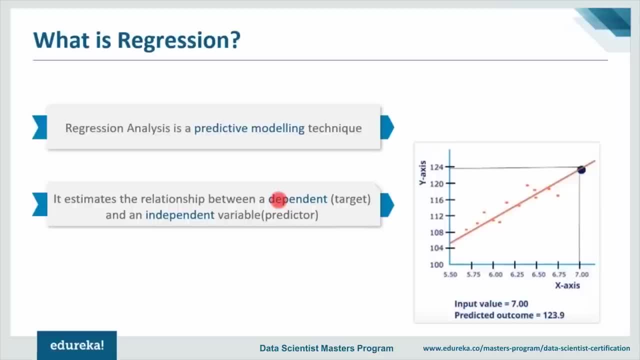 Let's say the number of products you sold till date, or what is the season out there, Is there the availability of product, or how is the product quality, And all these things. So these are the never-ending factors, which are nothing but the different features that leads to sale. 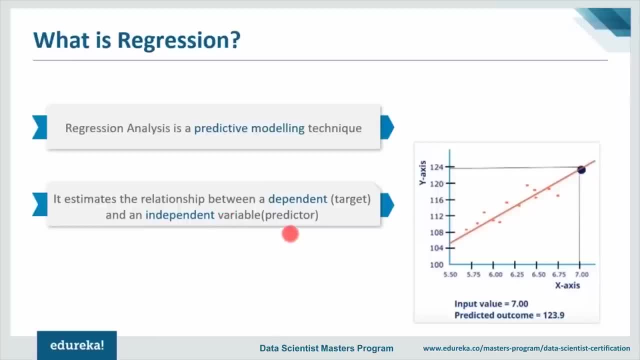 So these variables are called as your independent variable or, you can say, the predictor. Now, if you look at the graph over here, we have some values of X and we have values of Y. Now, as you can see over here, if X increases, the value of Y also increases. 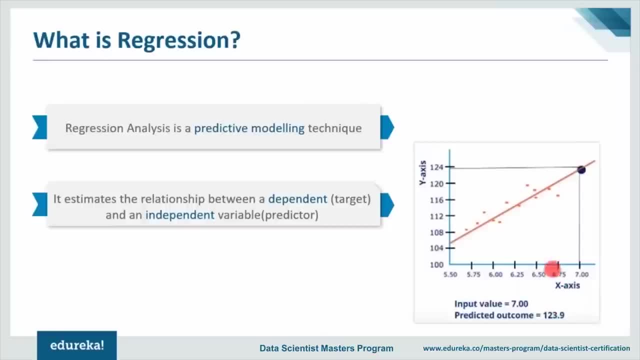 So let me explain you this with an example. Let's say we have data till the value of X which is 6.75, and somebody asks you: what will the value of Y when the value of X increases? This is 7.. So the way which you can do it, or how regression comes into the picture. 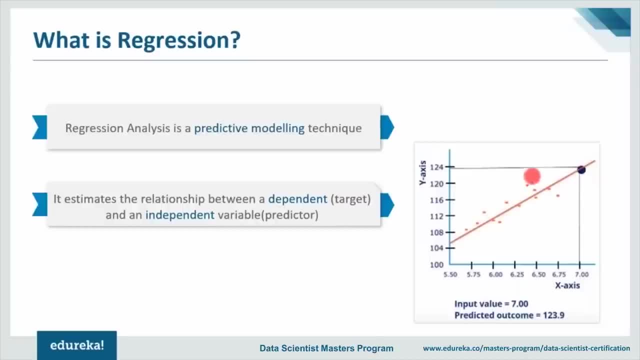 is by fitting a straight line by all these points and getting the value of M and C. So this is straight line, guys, and the formula for the straight line is: Y is equal to MX plus C. So using this, we can try to predict the value of Y. 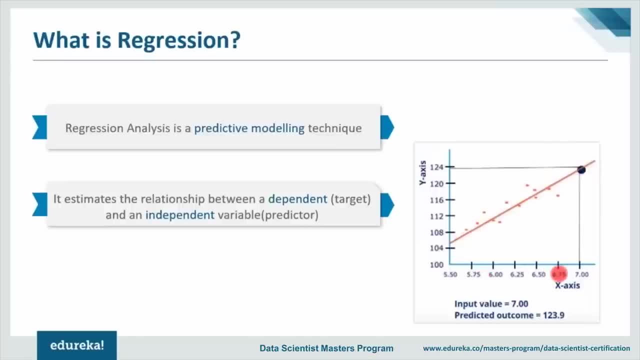 So here, if you notice, the X variable can increase as much as it can, but the Y variable will increase according to X. So Y is basically dependent on your X variable. So for any arbitrary value of X you can predict the value of Y, And this is always done through regression. 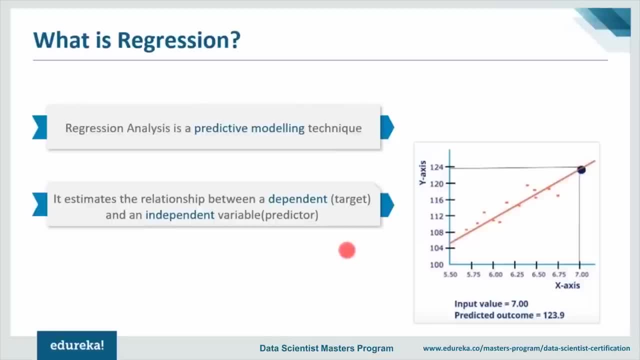 So that is how regression is useful. Now, regression is basically classified into three types: your linear regression, then your logistic regression and polynomial regression. So today we will be discussing logistic regression. So let's move forward and understand the what and why of logistic regression. 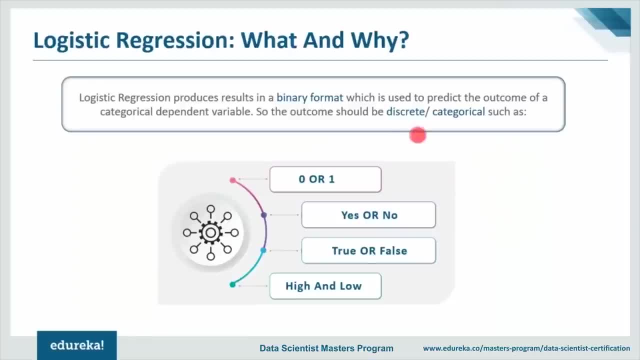 Now this algorithm is most widely used when the dependent variable, or you can say the output, is in the binary format. So here you need to predict the outcome of a categorical dependent variable. So the outcome should be always discrete or categorical in nature. Now by discrete I mean the value should be binary. 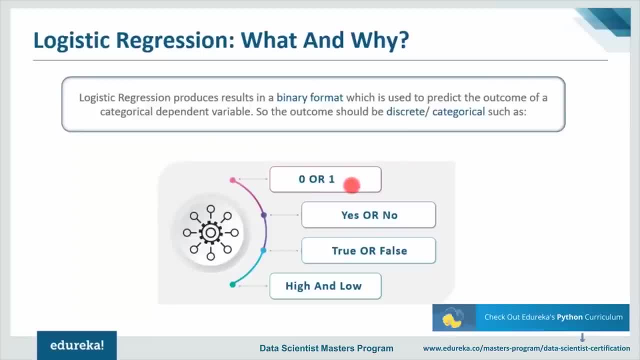 or you can say you just have two values. It can either be 0 or 1.. It can either be yes or no, Either be true or false, or high or low. So only these can be the outcomes. So the value which you need to predict should be discrete. 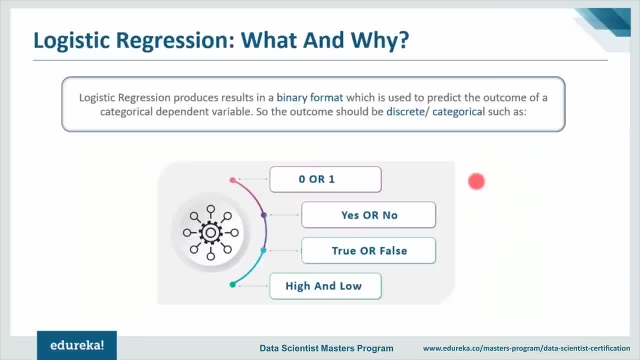 or you can say categorical in nature, Whereas in linear regression we have the value of Y, or you can say: the value you need to predict is in a range. So that is how there is a difference between linear regression and logistic regression. Now you must be having question: why not linear regression? 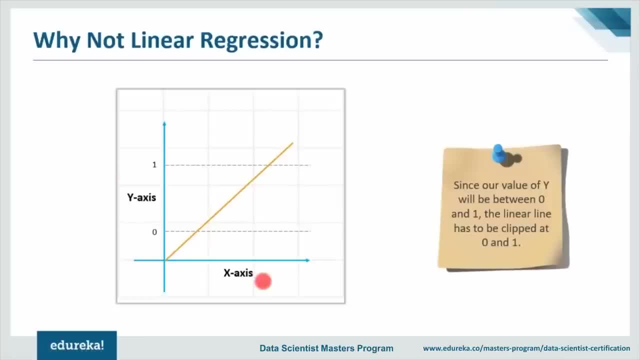 Now, guys, in linear regression, the value of Y, or the value which you need to predict, is in a range, But in our case, as in the logistic regression, we just have two values. It can be either 0 or it can be 1.. It should not entertain the values which is below 0 or above 1.. 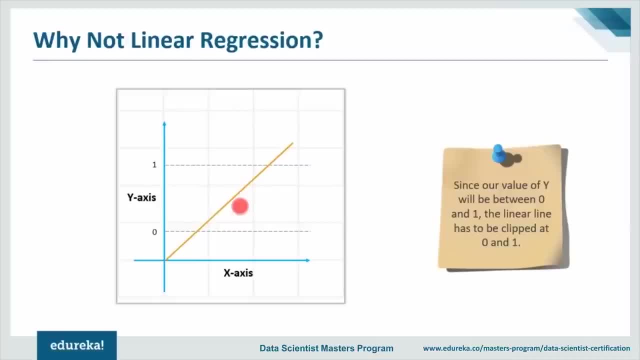 But in linear regression we have the value of Y in the range. So here, in order to implement logistic regression, we need to clip this part, So we don't need the value that is below 0 or we don't need the value which is above 1.. 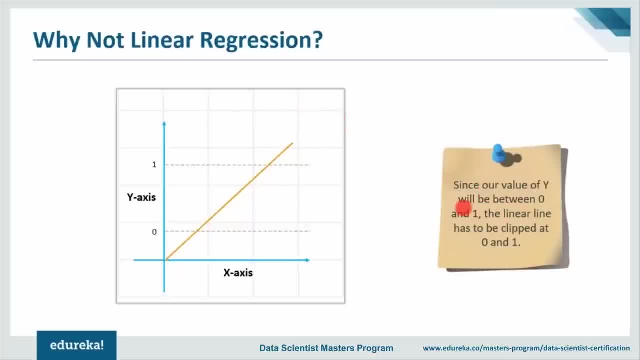 So, since the value of Y will be between only 0 and 1- that is the main rule of logistic regression- the linear line has to be clipped at 0 and 1.. Now, once we clip this graph, it would look somewhat like this: So here you are getting a curve which is nothing but three different straight lines. 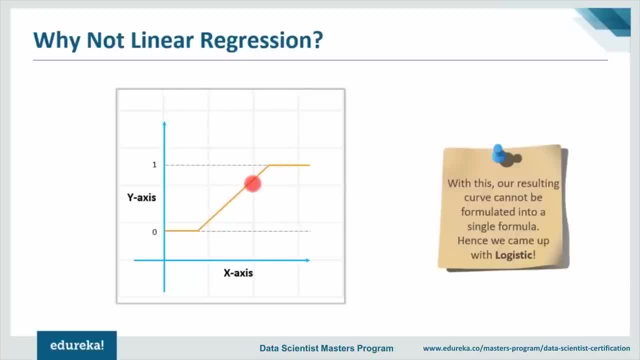 So here we need to make a new way to solve this problem. So this has to be formulated into an equation, and hence we come up with logistic regression. So here the outcome is either 0 or 1, which is the main rule of logistic regression. 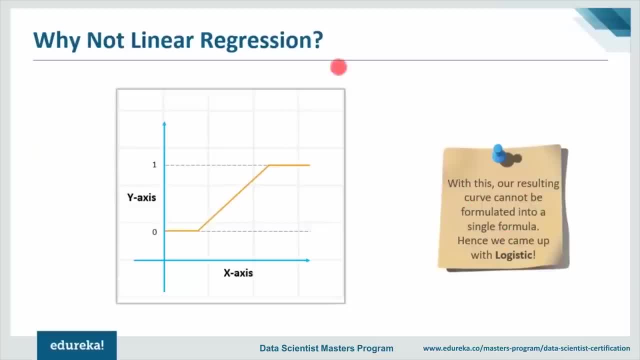 So with this our resulting curve cannot be formulated, so hence our main aim, to bring the values to 0 and 1, is fulfilled. So that is how we came up with logistic regression Now here. once it gets formulated into an equation, it looks somewhat like this: 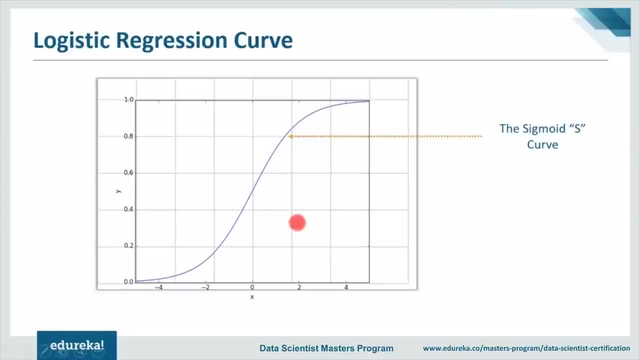 So, guys, this is nothing but a S curve, or you can say the sigmoid curve, or sigmoid function curve. So this sigmoid function basically converts any value from minus infinity to infinity, to your discrete values which a logistic regression wants. or you can say the values which are in binary format, either 0 or 1.. 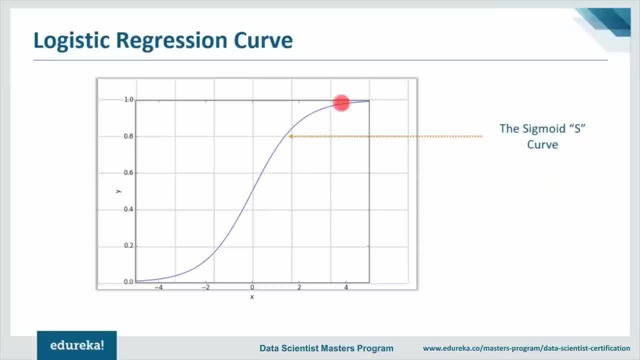 So if you see, here the values are either 0 or 1. And this is nothing but just a transition of it. But, guys, there's a catch over here. So let's say I have a data point that is 0.8.. 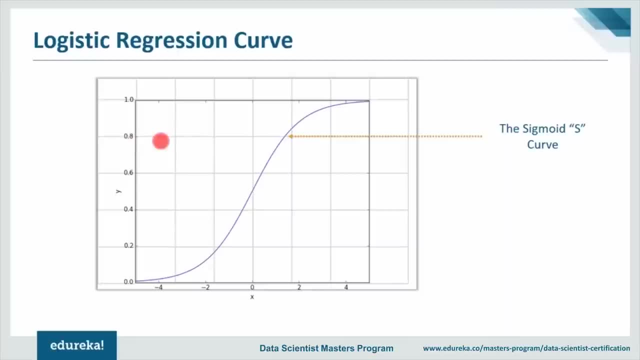 Now, how can you decide whether your value is 0 or 1? Now, here you have the concept of threshold, which basically divides your line. So here threshold value basically indicates the probability of either winning or losing. So here, by winning, I mean the values equals to 1. 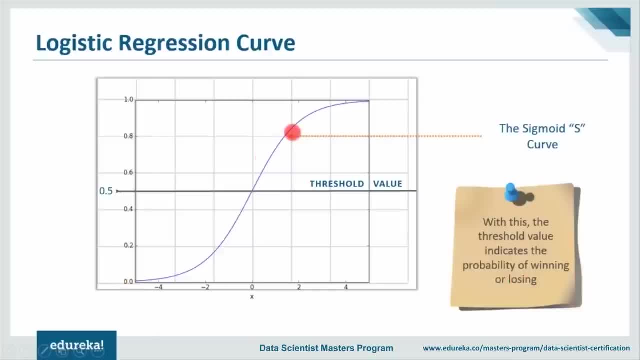 and by losing I mean the values equals to 0. But how does it do that? Let's say I have a data point which is over here. Let's say my cursor is at 0.8.. So here I'll check whether this value is less than my threshold value or not. 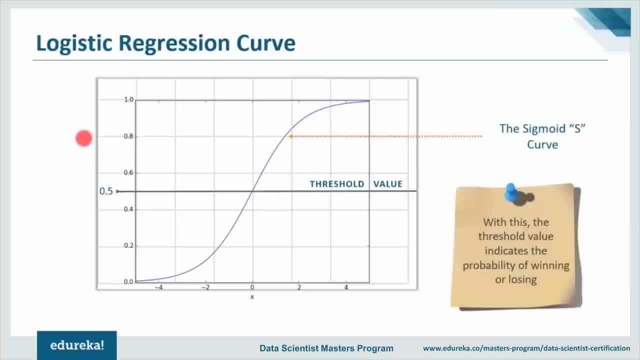 Let's say, if it is more than my threshold value, it should give me the result as 1.. If it is less than that, then should give me the result as 0.. So here my threshold value is 0.5.. Now I need to define that. if my value, let's say 0.8. 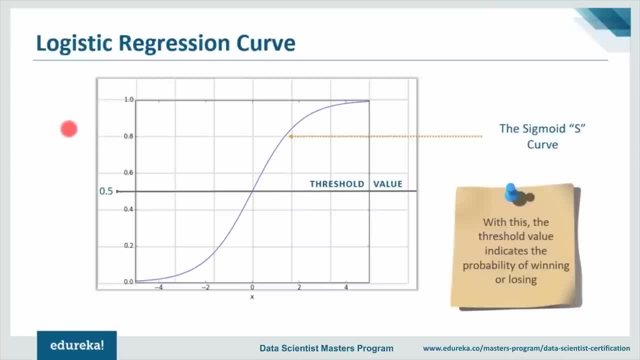 it is more than 0.5, then the value shall be rounded off to 1.. And let's say: if it is less than 0.5- let's say I have a value 0.2- then should reduce it to 0.. 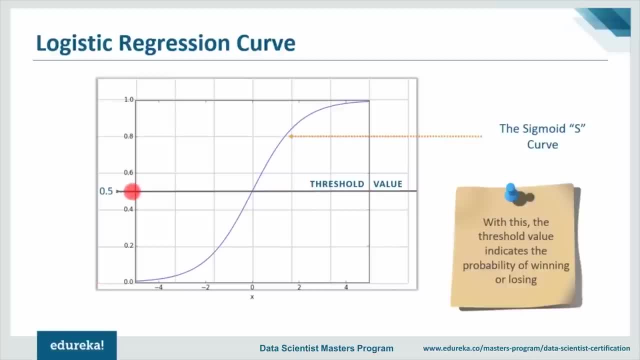 So here you can use the concept of threshold value to find your output. So here it should be discrete, It should be either 0 or it should be 1.. So I hope you caught this curve of logistic regression. So, guys, this is the sigmoid S curve. 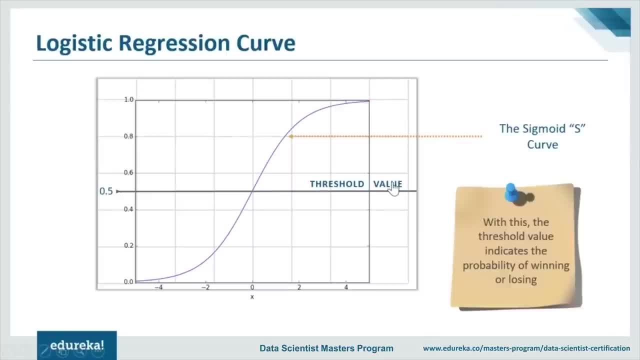 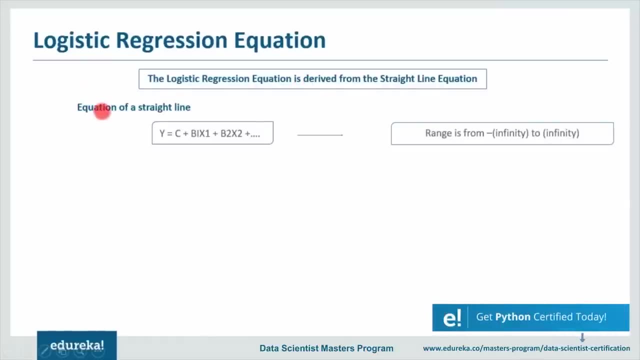 So to make this curve we need to make an equation. So let me address that part as well. So let's see how an equation is formed to imitate this functionality. So over here we have an equation of a straight line which is: y is equals to mx plus c. 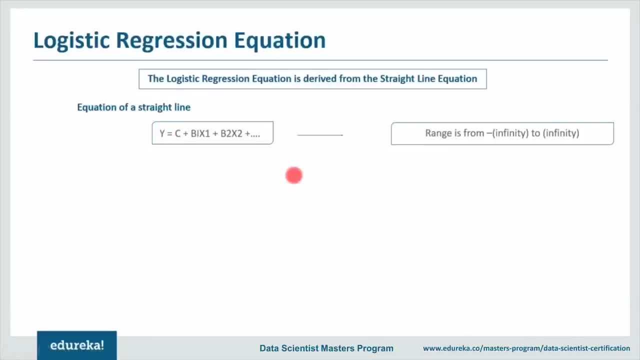 So in this case I just have only one independent variable. But let's say, if we have many independent variable, then the equation becomes m1x1 plus m2x2 plus m3x3 and so on till mnxn. Now let us put in b and x. 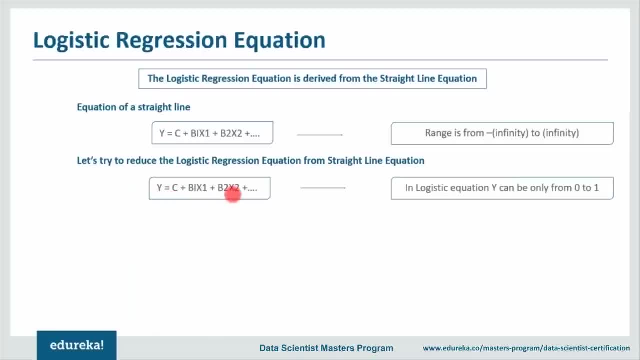 So here the equation becomes: y is equals to b1x1 plus b2x2 plus b3x3, and so on, till bnxn plus c. So, guys, your equation of the straight line has a range from minus infinity to infinity. But in our case- or you can say logistic equation- 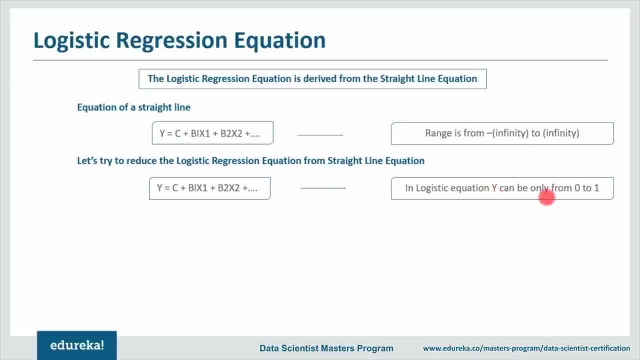 the value which we need to predict, or you can say the y value. it can have the range only from 0 to 1.. So in that case we need to transform this equation. So to do that what we had done, we have just divide the equation by 1 minus y. 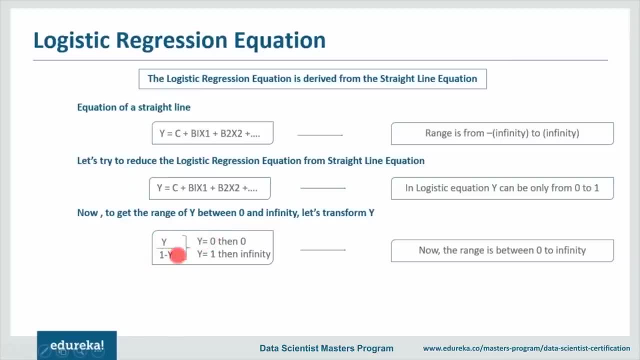 So now our y is equals to 0. So 0 over 1 minus 0, which is equals to 1.. So 0 over 1 is again 0.. And if we take y is equals to 1, then 1 over 1 minus 1, which is 0. 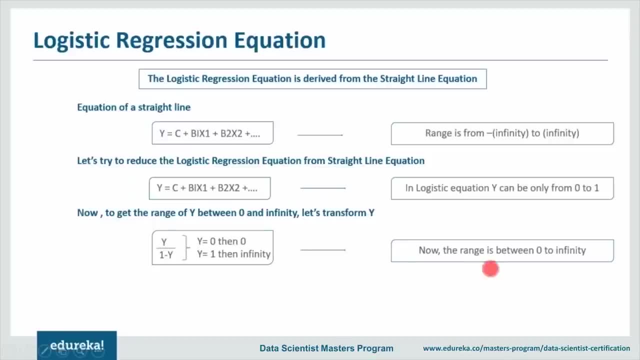 So 1 over 0 is infinity. So here my range is now between 0 to infinity. But again, we want the range from minus infinity to infinity. So for that, what we'll do, we'll have the log of this equation. So let's go ahead and have the logarithmic of this equation. 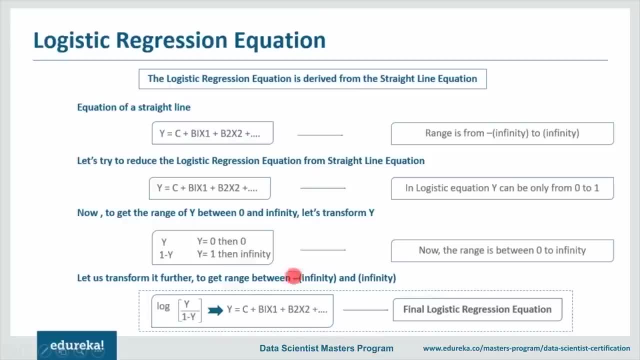 So here we have just transform it further to get the range between minus infinity to infinity. So over here we have log of y over 1 minus 1 and this is your final logistic regression equation. So, guys, don't worry, you don't have to write this formula. 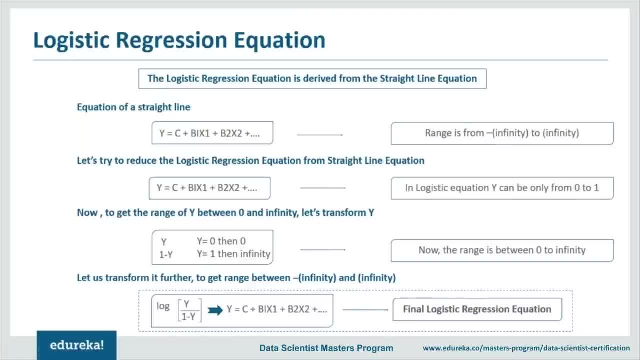 or memorize this formula In Python. you just need to call this function, which is logistic regression, and everything will be automatically for you. So I don't want to scare you with the maths and the formulas behind it, But it's always good to know how this formula was generated. 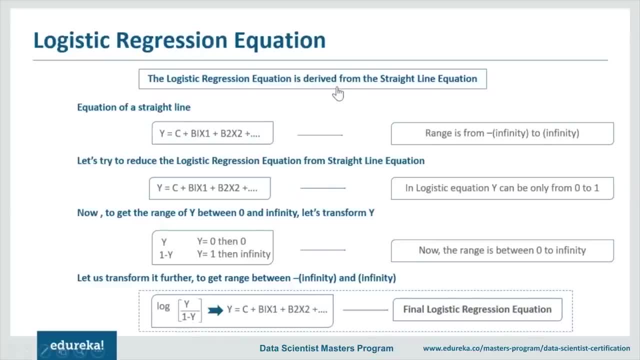 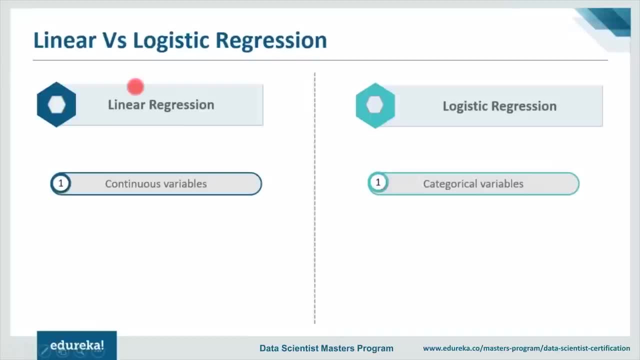 So I hope you guys are clear with how logistic regression comes into the picture. Next let us see what are the major differences between linear regression versus logistic regression. Now, first of all, in linear regression we have the value of y as a continuous variable, or the variable which we need to predict a continuous nature. 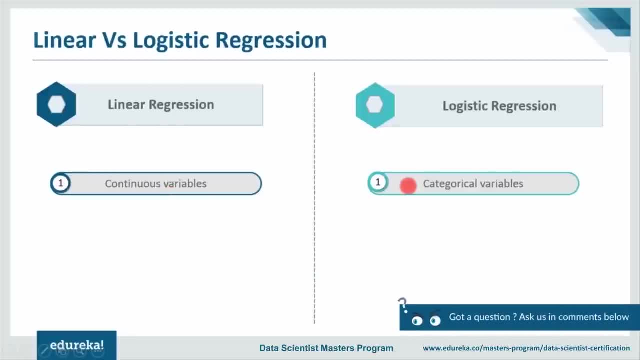 Whereas in logistic regression we have the categorical variable. So here the value which you need to predict should be discrete in nature. It should be either 0 or 1, or it should have just two values to it, For example whether it is raining or it is not raining. 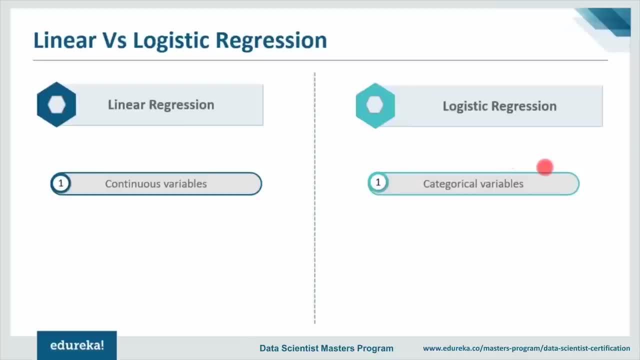 Is it humid outside or it is not humid outside? Now, is it going to snow or it is not going to snow? So these are the few examples where you need to predict, where the values are discrete or you can just predict whether this is happening or not. 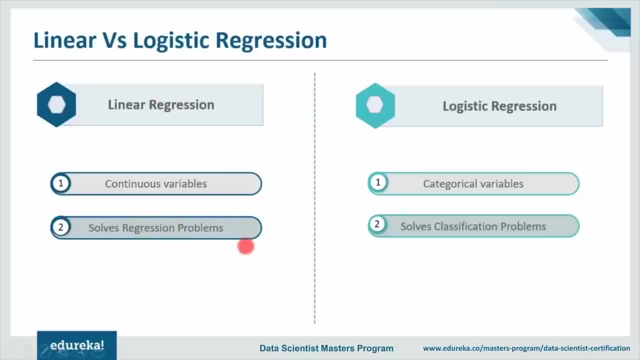 Next, linear regression solves your regression problems. So here you have a concept of independent variable and a dependent variable. So here you can calculate the value of y, which you need to predict using the value of x. So here your y variable, or you can say the value that you need to predict. 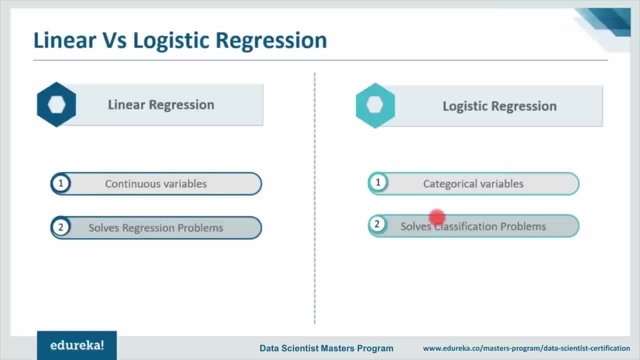 are in a range, But whereas in logistic regression you have discrete values. So logistic regression basically solves your classification problem. So it can basically classify it and it can just give you result, whether this event is happening or not. So I hope it is pretty much clear till now. 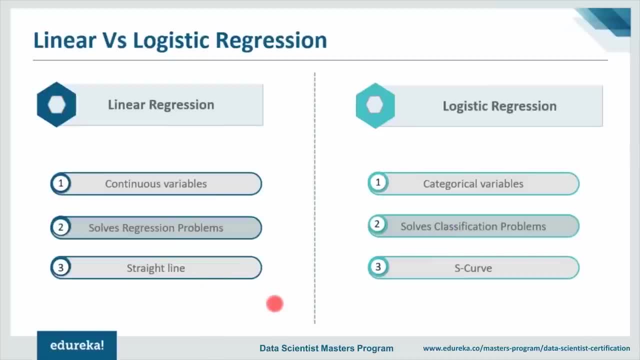 Next, in linear regression, the graph that you have seen is a straight line graph, So over here you can calculate the value of y with respect to the value of x, Whereas in logistic regression the curve that we got was a s curve, or you can say the sigmoid curve. 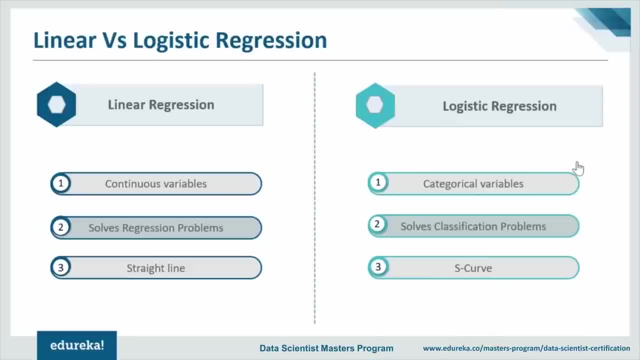 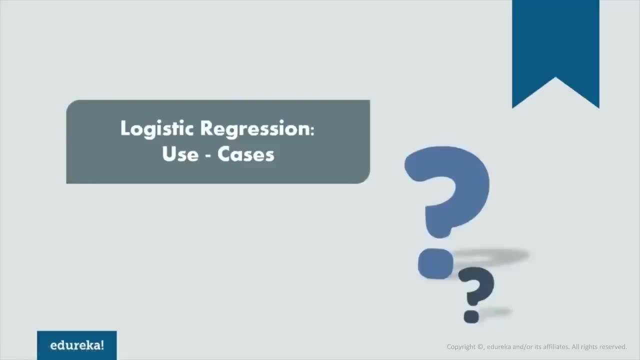 So using the sigmoid function, you can predict your y values. So I hope you guys are clear with the differences between the linear regression and logistic regression. Moving ahead, let us see the various use cases wherein logistic regression is implemented in real life. So the very first is weather prediction. 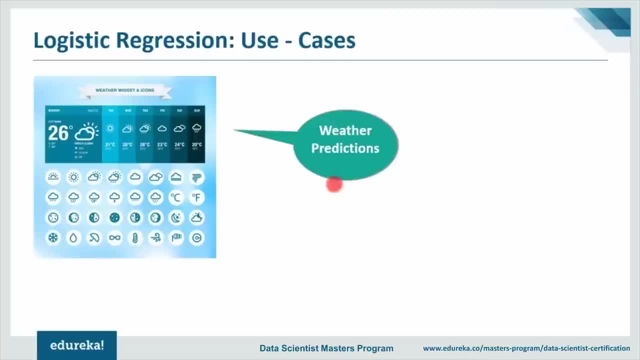 Now, logistic regression helps you to predict your weather. For example, it is used to predict whether it is raining or not, whether it is sunny, is it cloudy or not. So all these things can be predicted using logistic regression, Whereas you need to keep in mind that 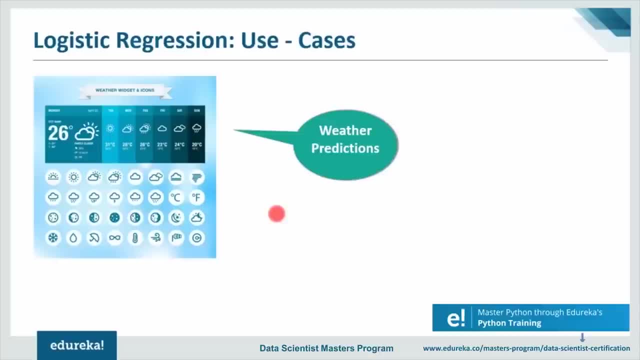 both linear regression and logistic regression can be used in predicting the weather. So in that case, linear regression helps you to predict what will be the temperature tomorrow, Whereas logistic regression will only tell you whether it is going to rain or not, or whether it is cloudy or not. 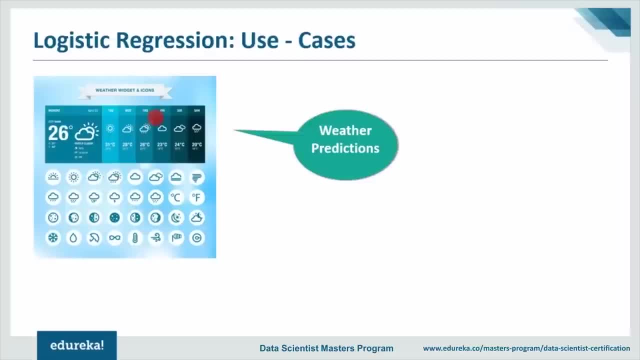 whether it is going to snow or not. So these values are discrete, Whereas if you apply linear regression, you will be predicting things like what is the temperature tomorrow or what is the temperature day after tomorrow and all those things. So these are the slight differences. 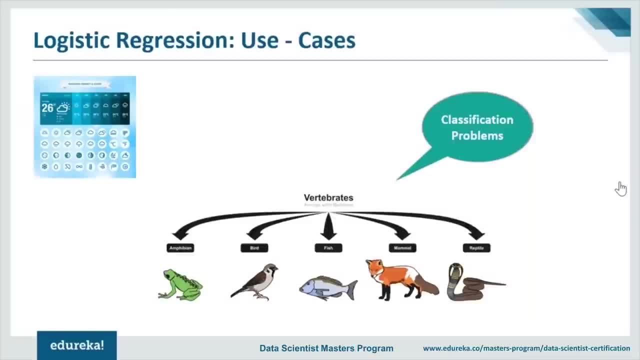 between linear regression and logistic regression. Now moving ahead, we have classification problem. So Python performs multiclass classification. So here it can help you tell whether it is a bird or it is not a bird. Then you can classify different kind of mammals, Let's say whether it is a dog or it is not a dog. 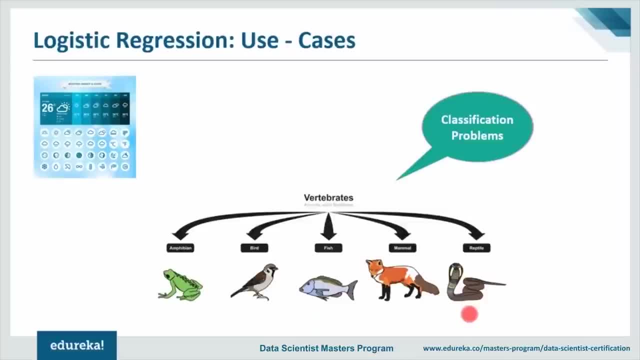 Similarly you can check it for reptile, whether it is a reptile or not a reptile. So in logistic regression it can perform multiclass classification. So this point I have already discussed, that it is used in classification problems. Next, it also helps you to determine: 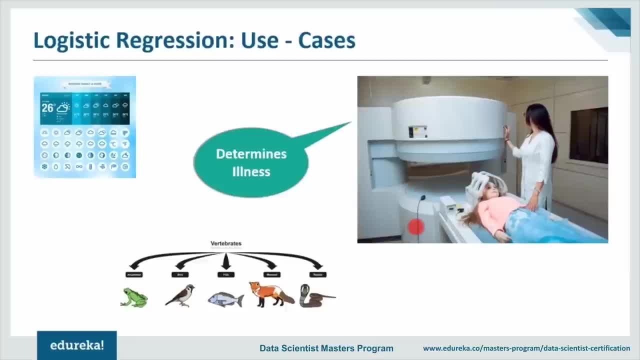 the illness as well. So let me take an example. Let's say a patient goes for routine checkup in hospital. So what doctor will do is it will perform various tests on the patient and will check whether the patient is actually ill or not. 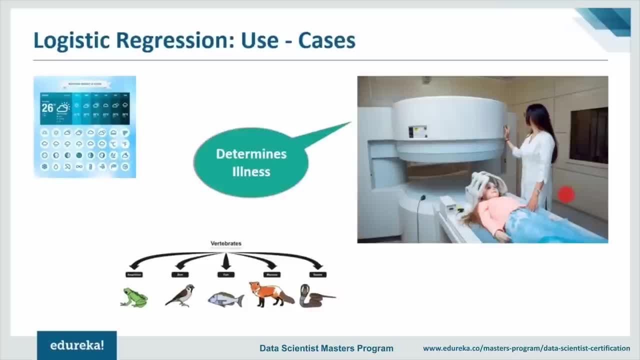 So what will be the features? So doctor can check the sugar level, the blood pressure. then what is the age of the patient? is it very small or is it an old person? then what is the previous medical history of that patient? and all of these features will be recorded by the doctor. 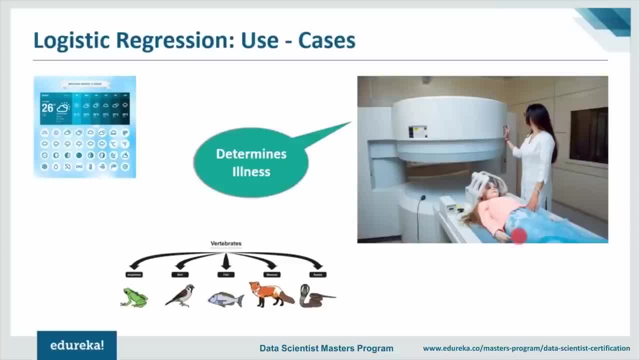 And finally, doctor checks the patient data and determines the outcome of the illness and the severity of illness. So, using all the data, a doctor can identify whether a patient is ill or not. So these are the various use cases in which you can use logistic regression. 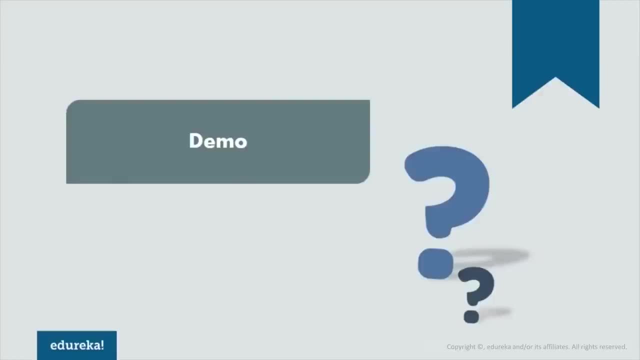 Now, I guess, enough of theory part, So let's move ahead and see some of the practical implementation of logistic regression. So over here I will be implementing two projects wherein I have the data set of a Titanic. So over here we will predict what factors 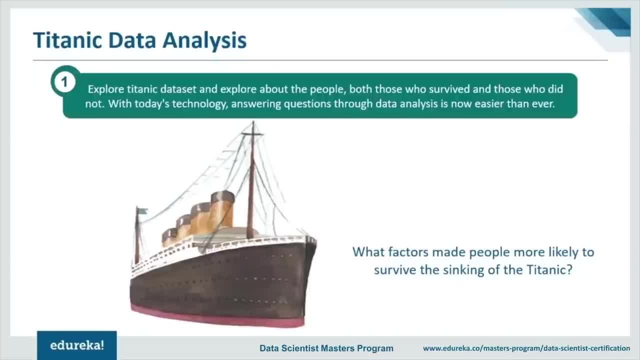 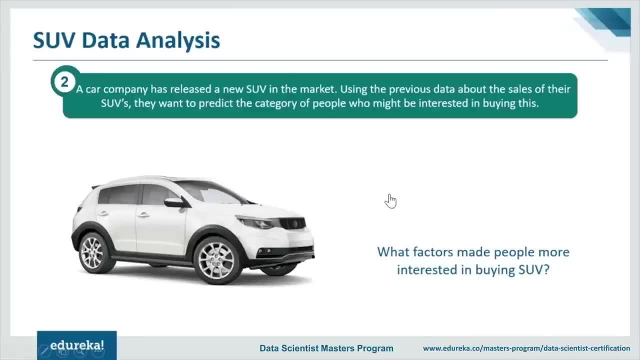 made people more likely to survive the sinking of the Titanic ship, And in my second project we will see the data analysis on the SUV cars. So over here we have the data of the SUV cars, who can purchase it and what factors made people more interested in buying SUV. 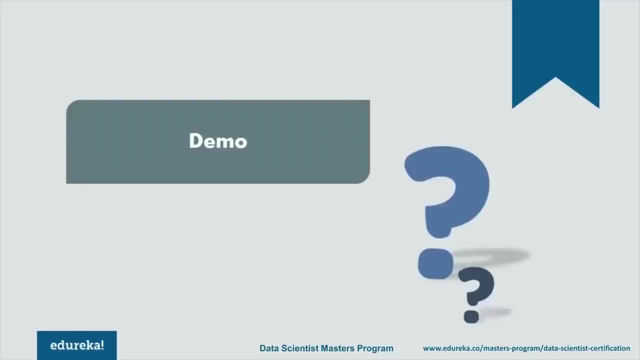 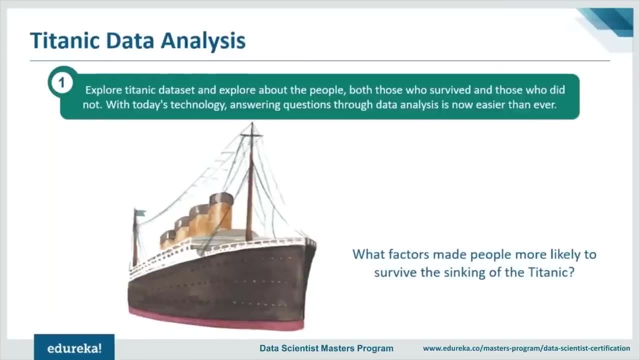 So these will be the major questions as to why you should implement logistic regression and what output will you get by it. So let's start by the very first project, that is, Titanic data analysis. So some of you might know that there was a ship called as Titanic. 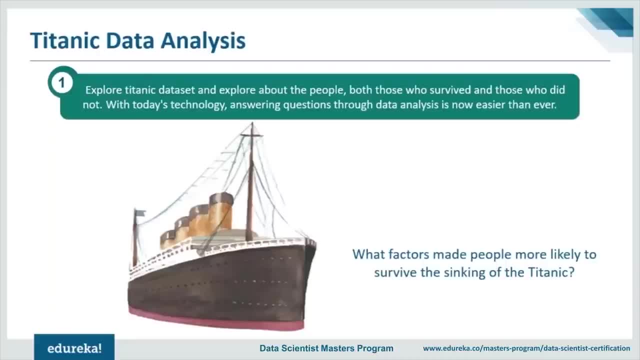 which basically hit an iceberg and it sunk to the bottom of the ocean And it was a big disaster at that time because it was the first voyage of the ship and it was supposed to be really, really strongly built and one of the best ships of that time. 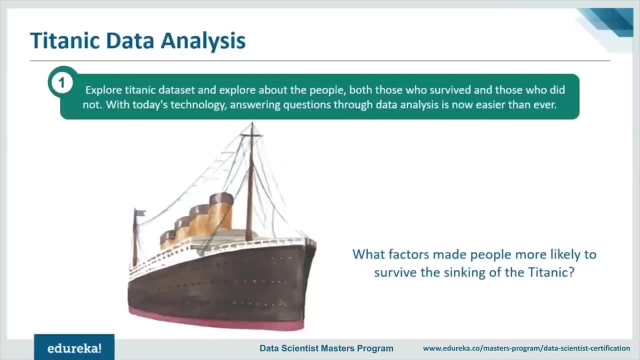 So it was a big disaster of that time and, of course, there is a movie about this as well, So many of you might have watched it. So what we have? we have data of the passengers, those who survived and those who did not survive. 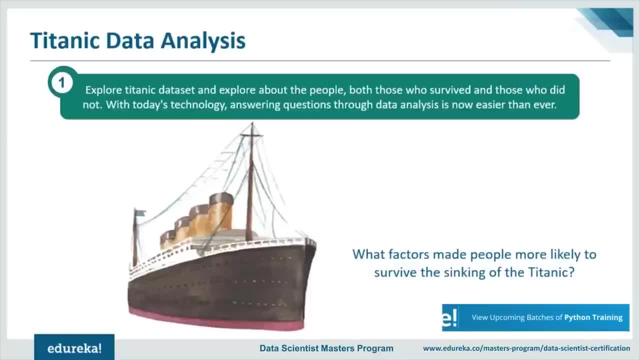 in this particular tragedy. So what you have to do, you have to look at this data and analyze which factors would have been contributed the most to the chances of a person's survival on the ship or not. So, using the logistic regression, we can predict whether the person survived. 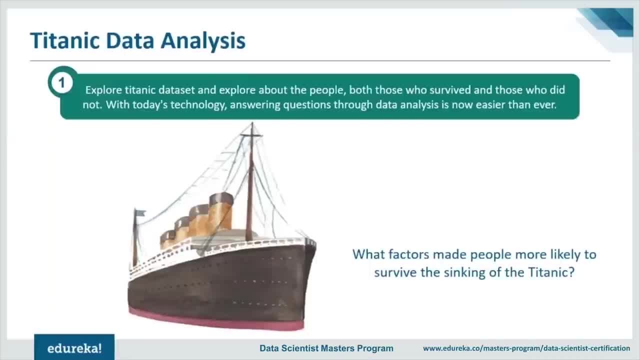 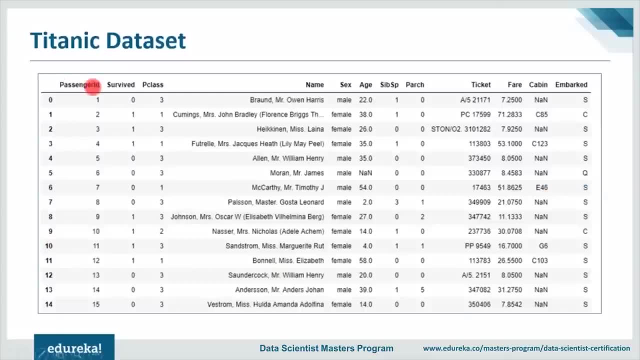 or the person died. Now, apart from this, we'll also have a look with the various features along with that. So first let us explore the data set. So over here we have the index value, Then the first column is passenger ID, Then my next column is survived. 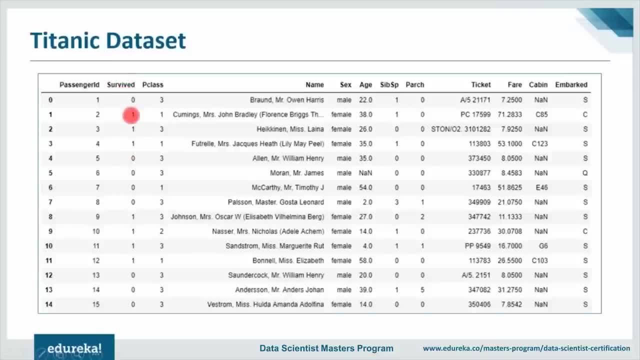 So over here we have two values, a zero and a one. So zero stands for did not survive and one stands for survive. So this column is categorical, where the values are discrete. Next we have passenger class. So over here we have three values. 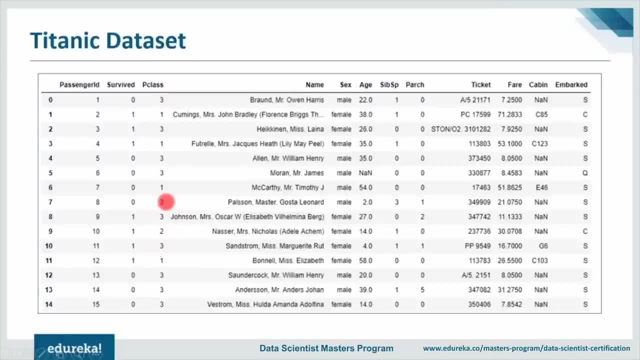 one, two and three. So this basically tells you that whether a passenger is traveling in the first class, second class or third class, Then we have the name of the passenger, We have the sex or you can say the gender of the passenger. 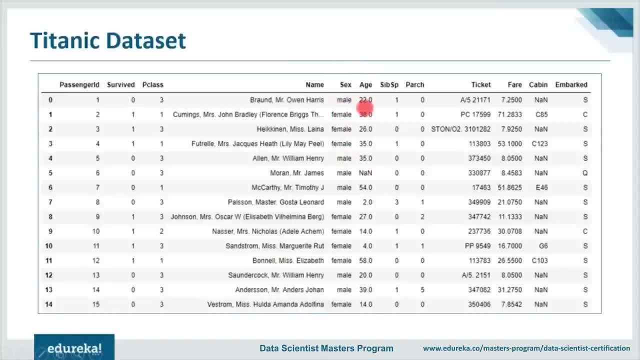 whether the passenger is a male or female. Then we have the age, We have the SibSP, So this basically means the number of siblings or the spouses aboard the Titanic. So over here we have values such as one zero and so on. 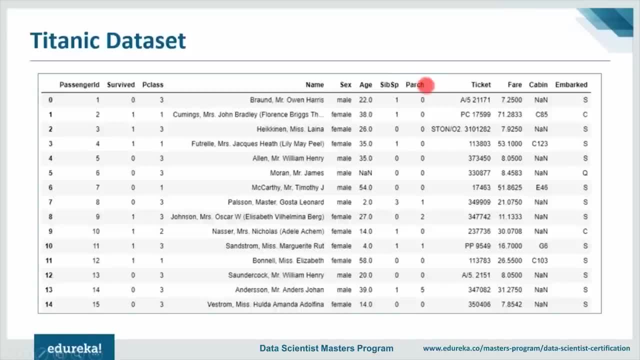 Then we have Parch. So Parch is basically the number of parents or children aboard the Titanic. So over here we also have some values. Then we have the ticket number, We have the fare, We have the cabin number and we have the embarked column. 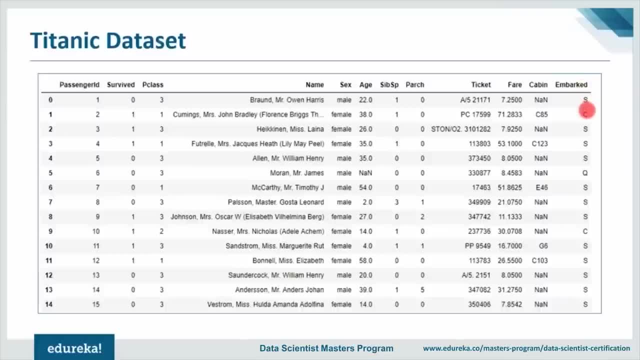 So in my embarked column we have three values. We have S, C and Q. So S basically stands for Southampton, C stands for Cherbourg and Q stands for Kuenstown. So these are the features that we'll be applying our model on. 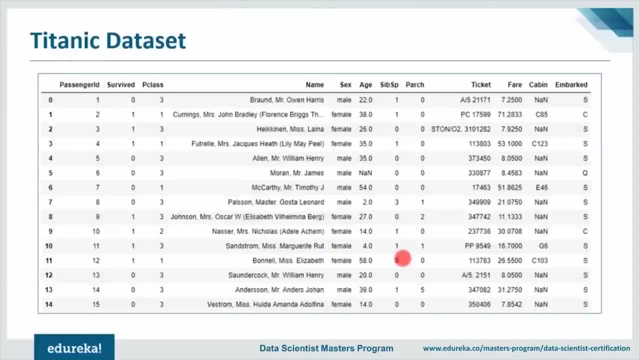 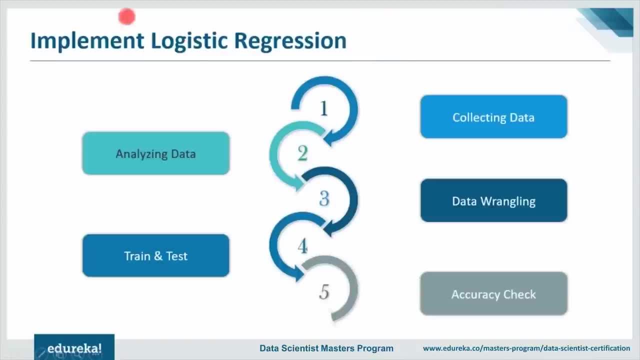 So here we'll perform various steps, and then we'll be implementing logistic regression. So now these are the various steps which are required to implement any algorithm. So first of all, in our case, we are implementing logistic regression. So our very first step, 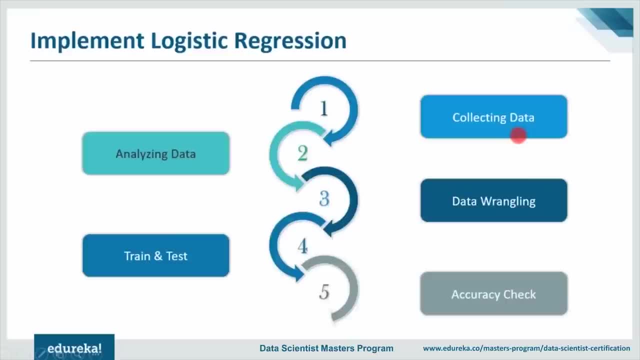 is to collect your data or to import the libraries that are used for collecting your data and then taking it forward, Then my second step is to analyse your data. So over here I can go through the various fields and then I can analyse the data. 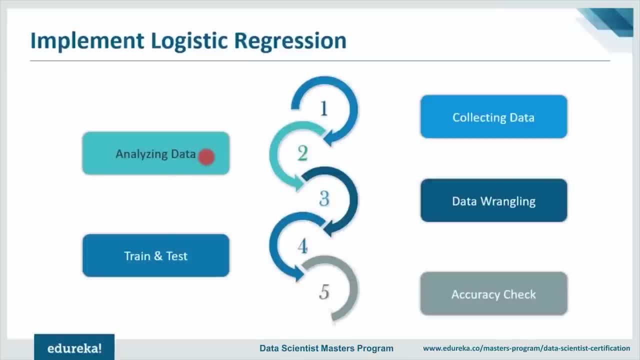 I can check. did the females or children survive better than the males? or did the rich passenger survive more than the poor passenger? or did the money matter, as in who paid more to get into the ship? were they evacuated first? and what about the workers? Does the worker survived? 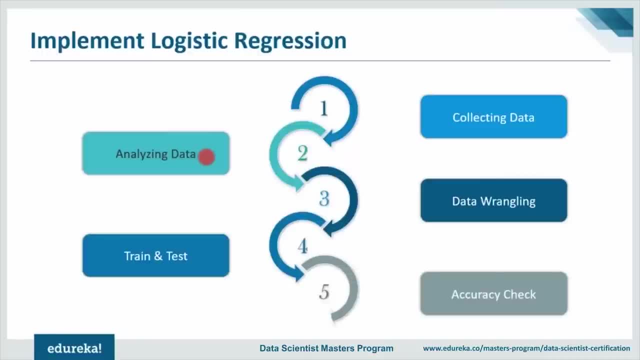 or what is the survival rate if you were the worker in the ship and not just a travelling passenger? So all of these are very, very interesting questions and you would be going through all of them one by one. So in this stage, you need to analyse your data. 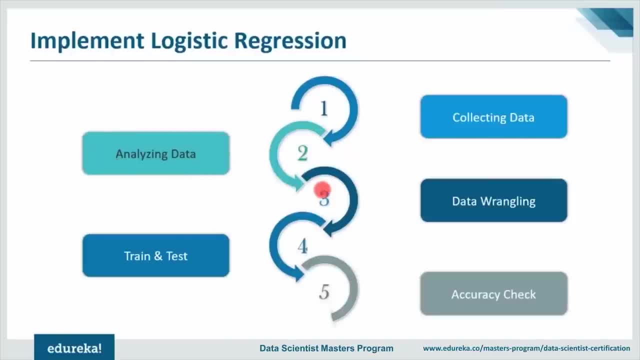 and explore your data as much as you can. Then my third step is to wrangle your data. Now, data wrangling basically means cleaning your data. So over here you can simply remove the unnecessary items or, if you have a null values in the data set. 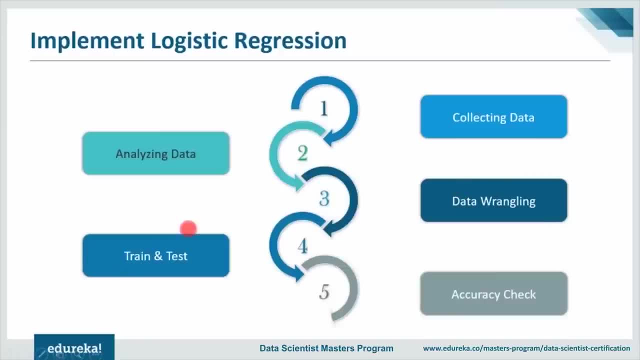 you can just clear that data and then you can take it forward. So in this step you can build your model using the train data set and then you can test it using the test. So over here you will be performing the split, which basically split your data set. 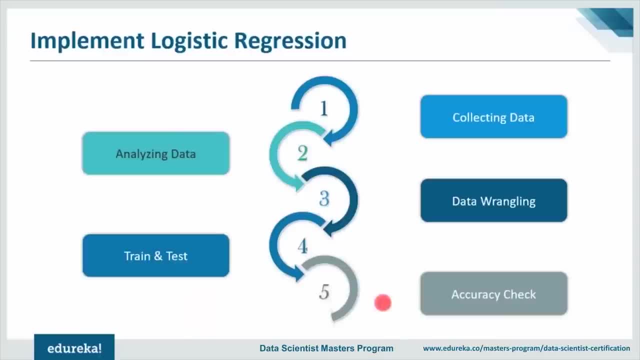 into training and testing data set. and finally, you will check the accuracy So as to ensure how much accurate your values are. So I hope you guys got these five steps that you're going to implement in logistic regression. So now let's go into 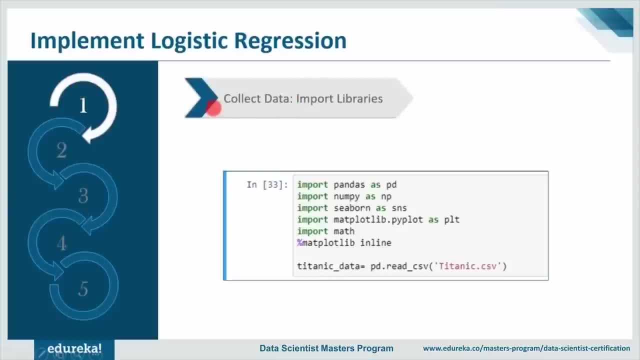 all these steps in detail. So, number one: we have to collect your data, or you can say, import the libraries. So let me just show you the implementation part as well. So I just open my Jupiter notebook and I just implement all of these steps. 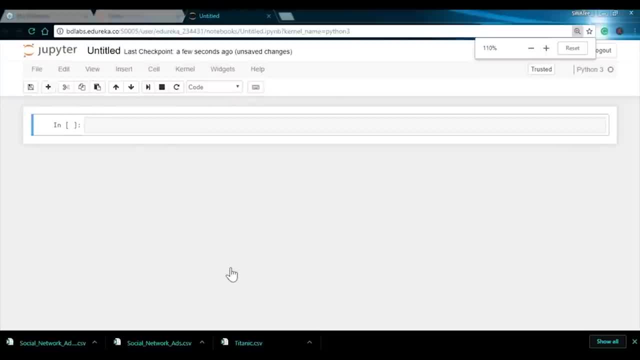 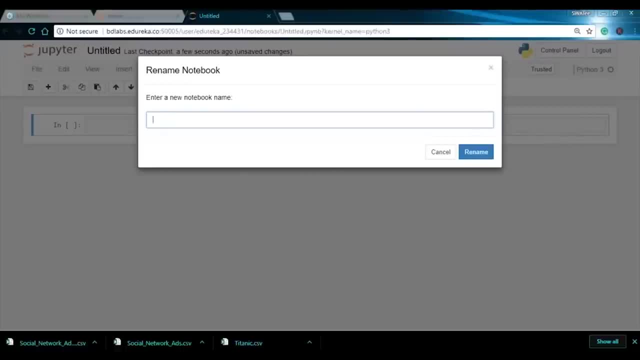 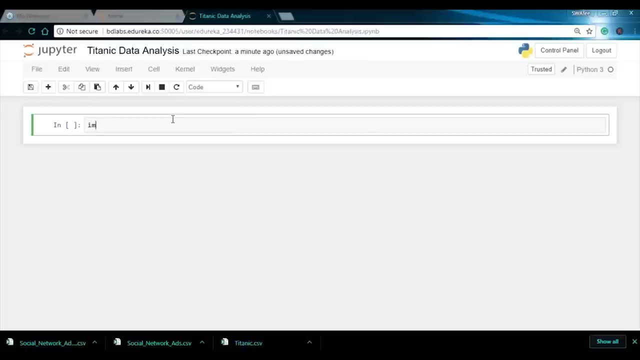 side by side. So, guys, this is my Jupiter notebook. So first let me just rename Jupiter notebook to, let's say, Titanic data analysis. Now our first step was to import all the libraries and collect the data. So let me just import all the libraries first. 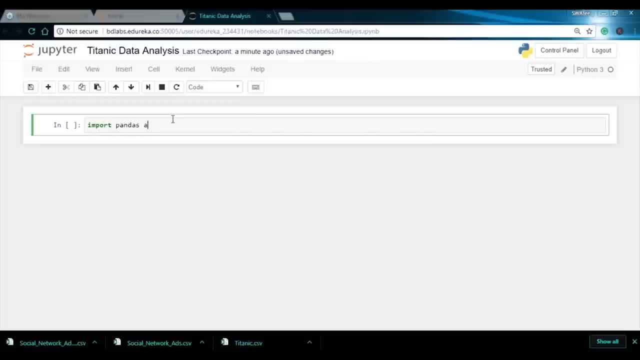 So first of all I'll import pandas, So pandas is used for data analysis. So I'll say import pandas as pd. then I'll say I'll be importing numpy. So I'll say import numpy as np. So numpy is a library in Python. 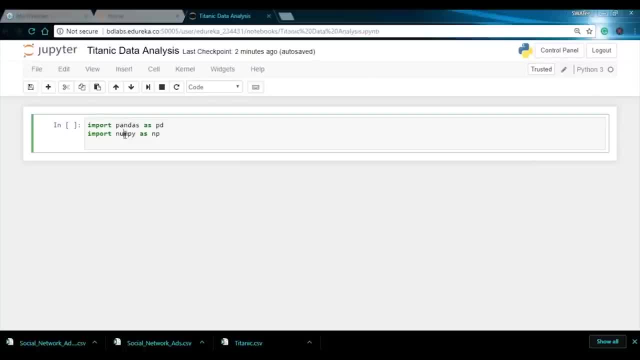 which basically stands for numerical Python, and it is widely used to perform any scientific computation. Next, we'll be importing seaborn, So seaborn is a library for statistical plotting. So I'll say: import seaborn as sns. I'll also import matplotlib, So matplotlib library. 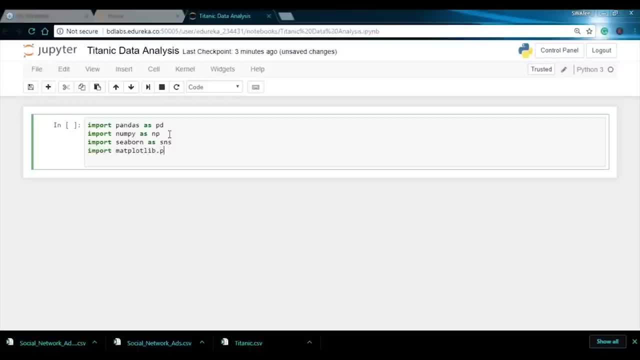 is again for plotting. So I'll say: import matplotlibpyplot as pld. Now to run this library in Jupyter notebook, all I have to write in is %matplotlib inline. Next I'll be importing one module as well, So as to calculate. 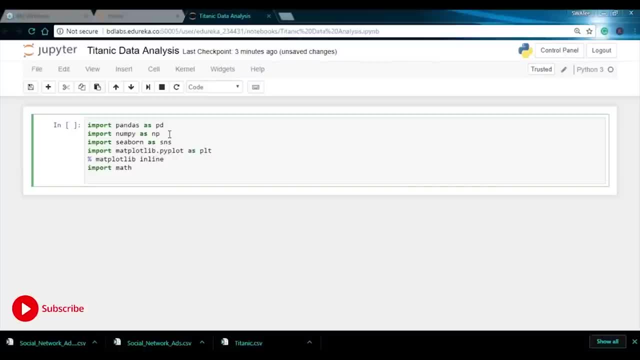 the basic mathematical functions. So I'll say import mats. So these are the libraries that I'll be needing in this Titanic data analysis. So now let me just import my data set. So I'll take a variable, Let's say Titanic data, and using the pandas, 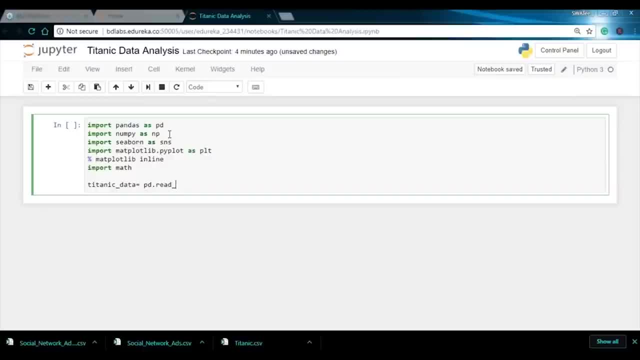 I will just read my CSV, or you can say the data set. I'll write the name of my data set, that is Titaniccsv. Now I have already showed you the data set, So over here let me just print the top 10 rows. 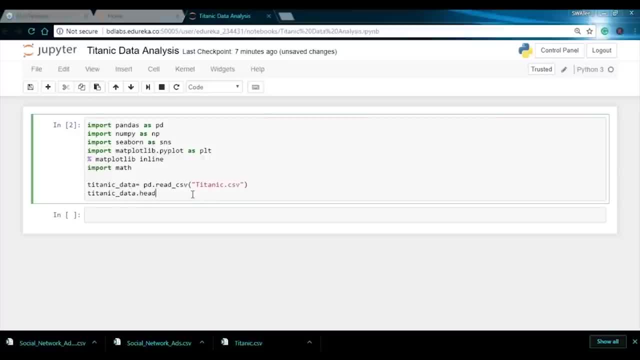 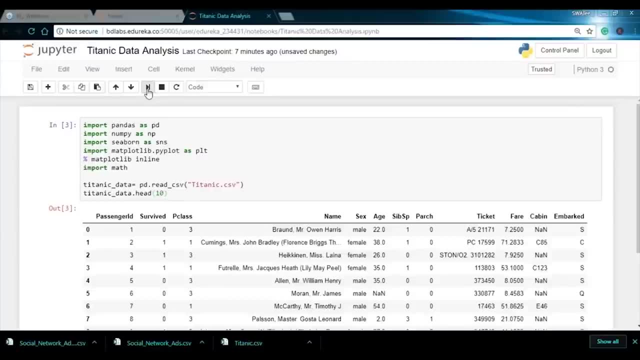 So for that I'll just say I'll take the variable Titanic datahead and I'll say the top 10 rows. So now I'll just run this. So to run this I just have to press shift plus enter, or else you can just 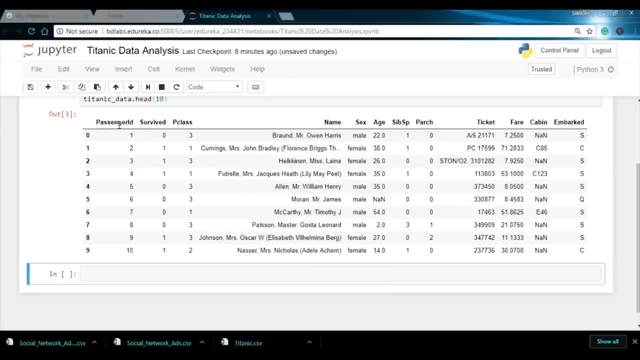 directly click on the cell. So over here I have the index, We have the passenger ID, which is nothing but again the index which is starting from one. Then we have the survived column, which has the categorical values, or you can say the discrete values. 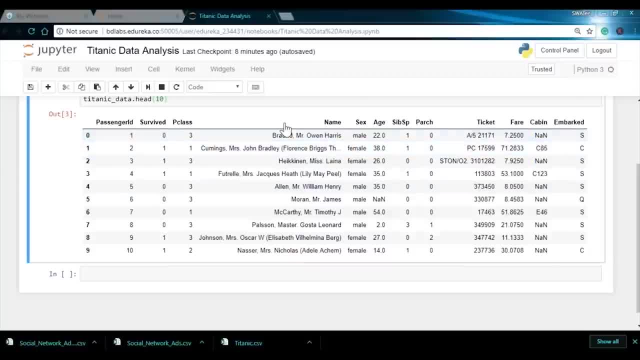 which is in the form of 0 or 1.. Then we have the passenger class. We have the name of the passenger, sex, age and so on. So this is the data set that I'll be going forward with. Next, let us print. 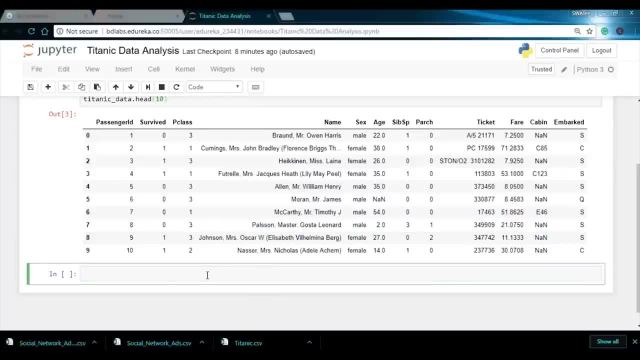 the number of passengers which are there in this original data set. So for that I'll just simply type in print, I'll say number of passengers and using the length function I can calculate the total length. So I'll say length and inside this 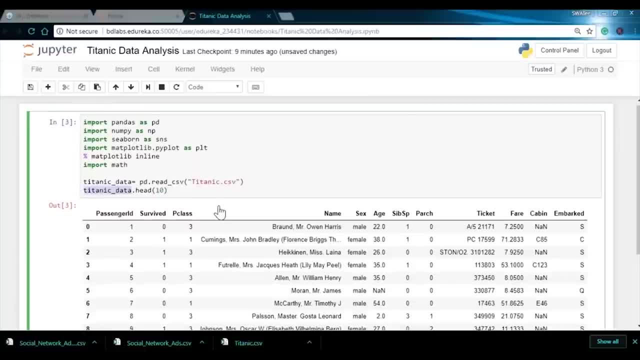 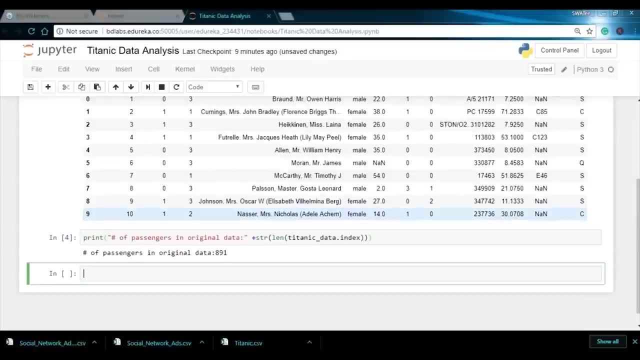 I'll be passing the Titanic data, So I'll just copy it from here. I'll just paste it dot index and next let me just print this one. So here, the number of passengers which are there in the original data set we have is 891.. 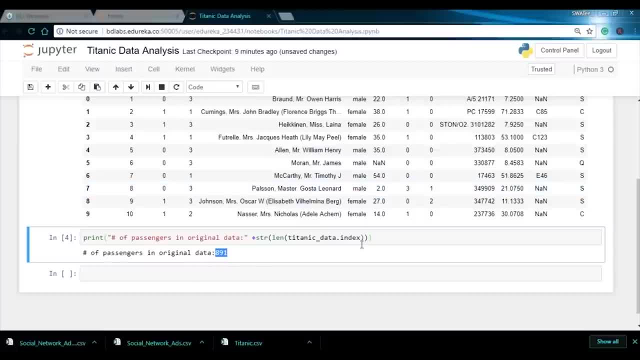 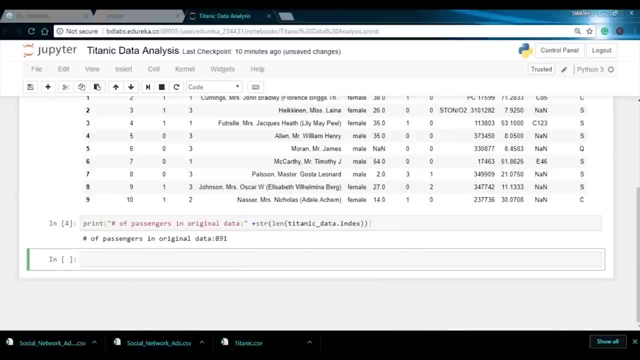 So around this number, we're traveling in the Titanic ship. So over here, my first step is done, where you have just collected data, imported all the libraries and find out the total number of passengers which are traveling in Titanic. So now let me just 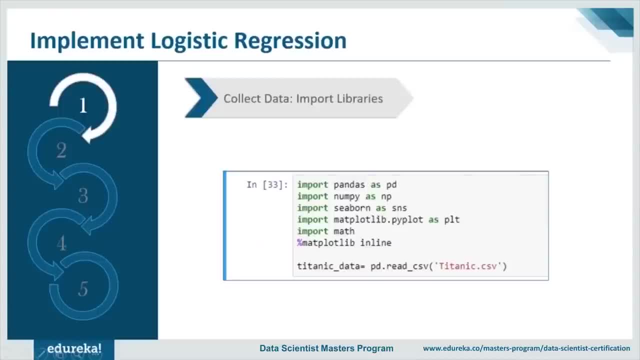 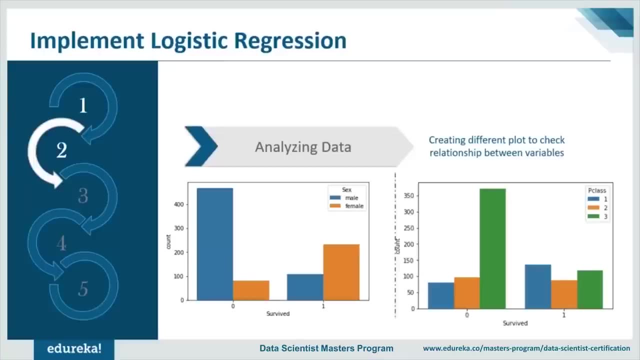 go back to presentation and let's see what is my next step. So we're done. next step is to analyze your data. So over here we'll be creating different plots to check the relationship between variables, as in how one variable is affecting the other. 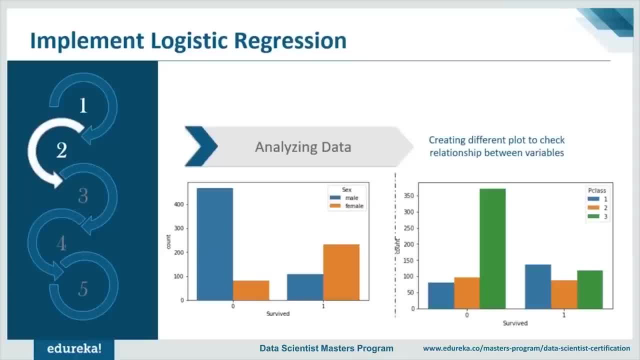 So you can simply explore your data set by making use of various columns, and then you can plot a graph between them. So you can either plot a correlation graph, You can plot a distribution graph. It's up to you guys. So let me just go back. 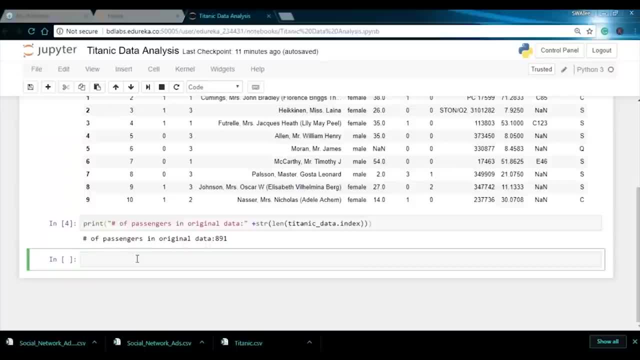 to my Jupiter notebook and let me analyze some of the data Over here. my second part is to analyze data, So I just put this in header 2.. Now to put this in header 2, I have to go on code, click on Markdown. 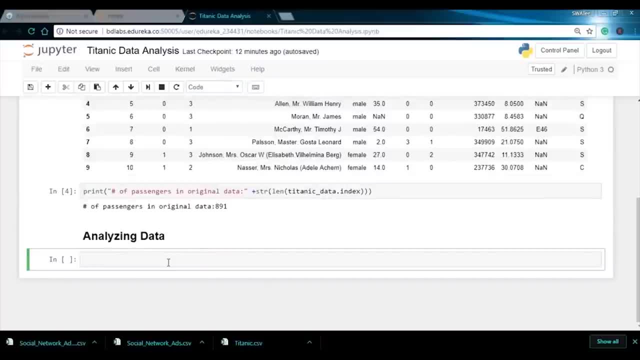 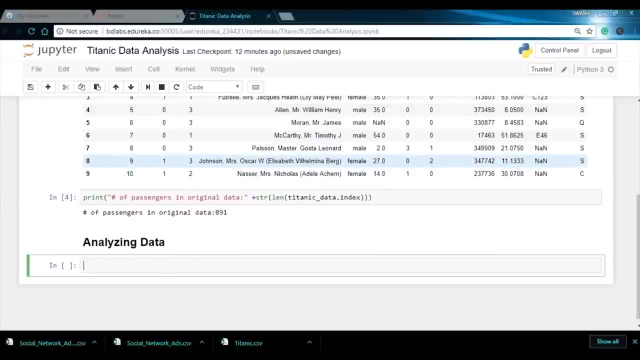 and I just run this. So first let us plot a count plot where you compare between the passengers who survived and who did not survive. So for that I'll be using the seaborn library. So over here I have imported seaborn as SNS. 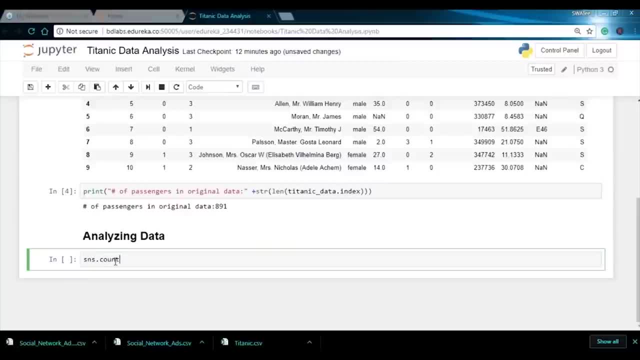 So I don't have to write the whole name. I'll simply say snscountplot. I'll say x is who survived, and the data that I'll be using is the Titanic data, or you can say the name of variable in which you have stored your data set. 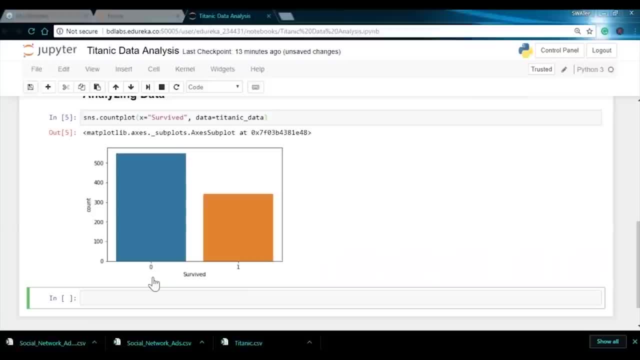 So now let me just run this So over here. as you can see, I have survived column on my x axis and on the y axis I have the count. So 0 basically stands for did not survive and 1 stands for the passengers. 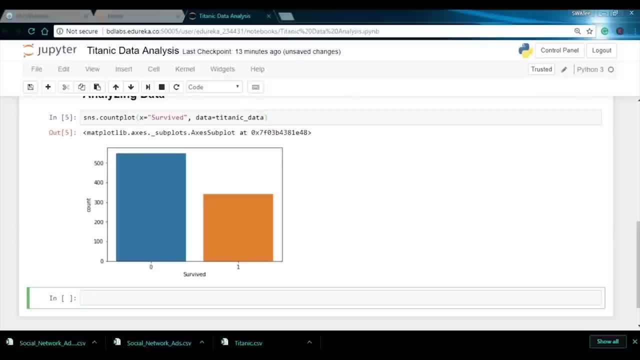 who did survive. So over here you can see that around 550 of the passengers who did not survive and they were around 350 passengers who only survived. So here you can basically conclude that there are very less survivors than non-survivors. 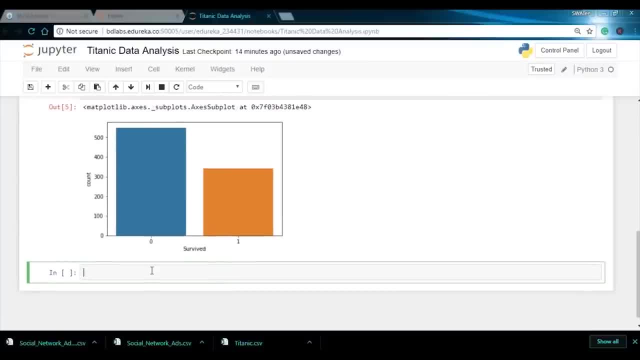 So this was the very first plot. Now let us plot another plot to compare the sex, as to whether, out of all the passengers who survived and who did not survive, how many were men and how many were female. So to do that, I'll simply say: 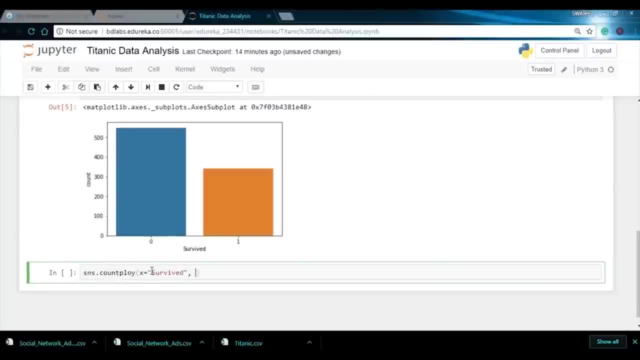 snscountplot and add the hue as sex. So I want to know how many females and how many males survived. Then I'll be specifying the data. So I'm using Titanic data set and let me just run this. Okay, I've done a mistake. 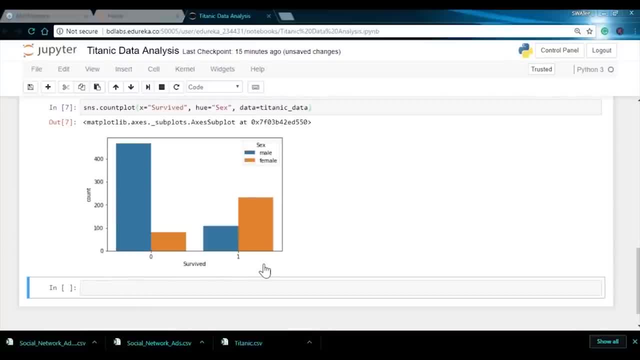 over here. So over here you can see, I have survived column on the x axis and I have the count on the y. Now. orange stands for your male passengers and orange stands for your female. So as you can see, here the passengers. 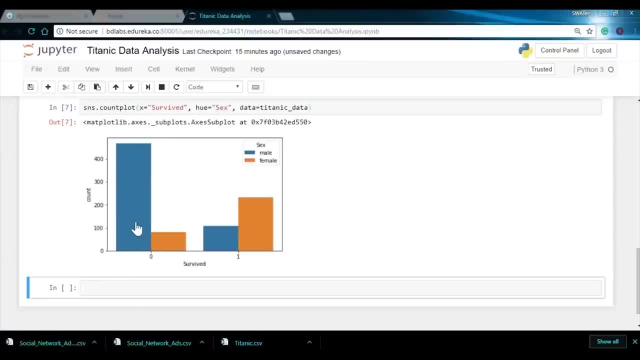 who did not survive. that has a value zero. So we can see that majority of males did not survive And if we see the people who survived here, we can see the majority of females survived. So this basically concludes the gender of the survival rate. 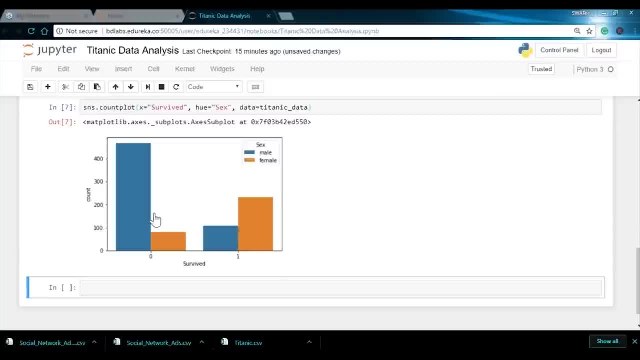 So it appears, on average, women were more than three times more likely to survive than men. Next, let us plot another plot where we have the hue of the class that the passenger was traveling in, whether it was traveling in class one, two or three. 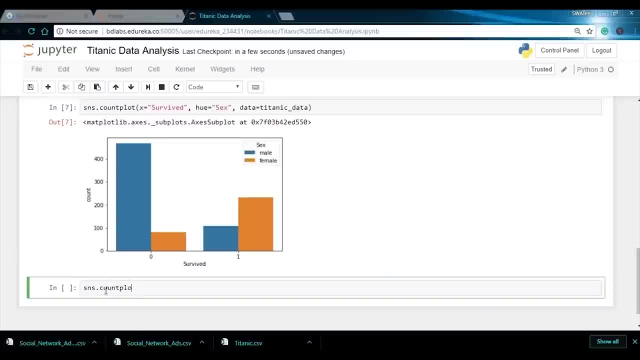 So for that I'll just write the same command. I'll say snscountplot, I'll keep my x axis as sub, only I'll change my hue to passenger class. So my variable is named as p class and the data set that I'll be using. 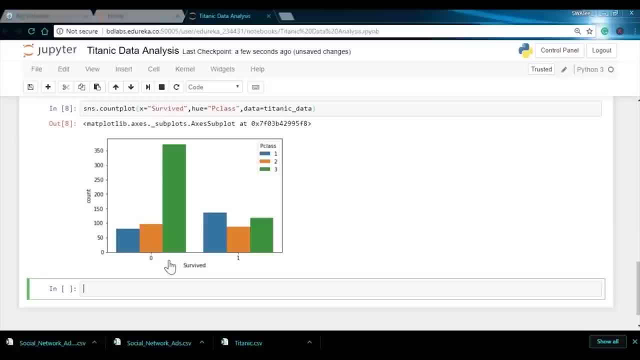 is titanic data, So this is my result. So over here you can see I have blue for first class, orange for second class and green for the third class. So here the passengers who did not survive were majorly of the third class. 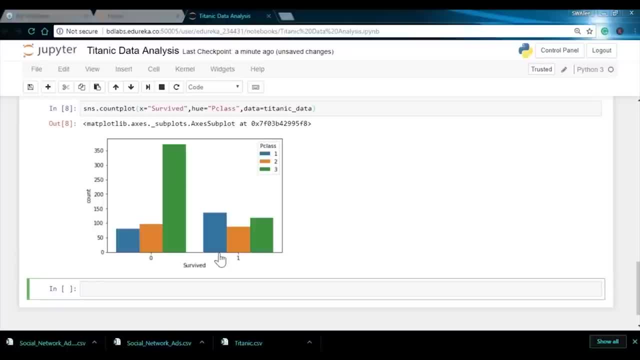 or you can say the lowest class or the cheapest class to get into the Titanic, and the people who did survive majorly belong to the higher classes. So here one and two has more rise than the passenger who were traveling in the third class. So here we have concluded. 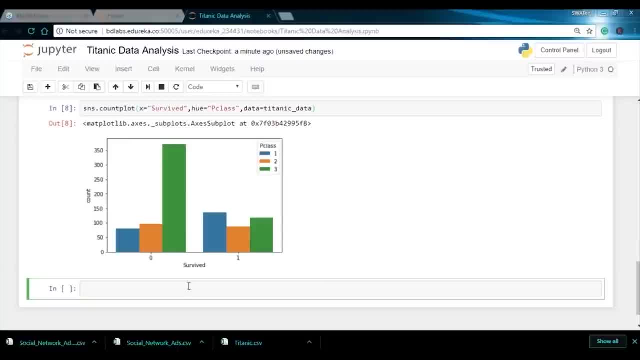 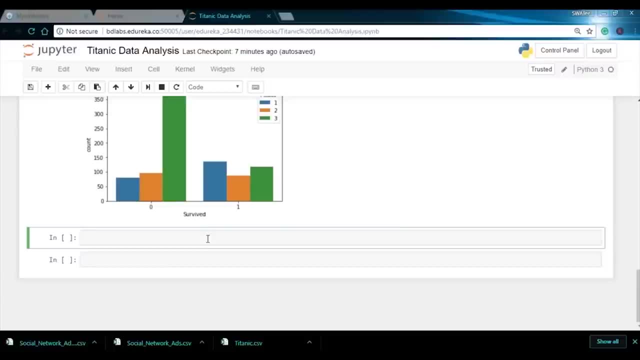 that the passengers who did not survive were majorly of third class, or you can say the lowest class, and the passengers who were traveling in first and second class would tend to survive more. Next, here I can simply use my data, So we'll be using 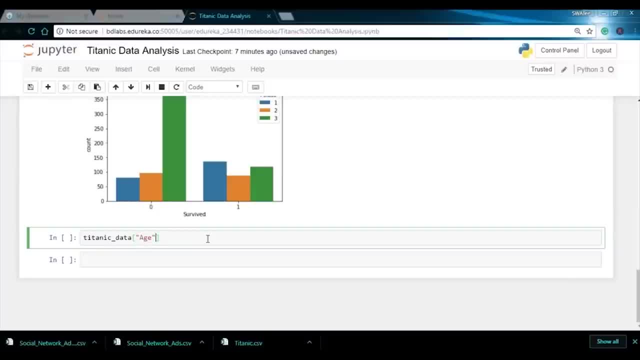 Pandas library. for this I'll declare an array and I'll pass in the column: that is age, So I plot and I want a histogram, So I'll say plot, dot, hist. So you can notice over here that we have more of young passengers. 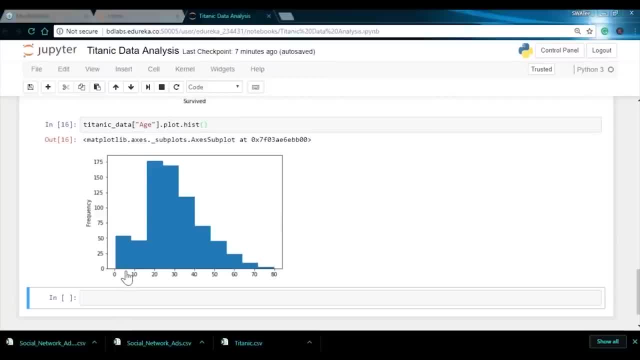 or you can say the children between the ages 0 to 10, and then we have the average age people and if you go ahead, lesser would be the population. So this is the analysis on the age column. So we saw that we have more young passengers. 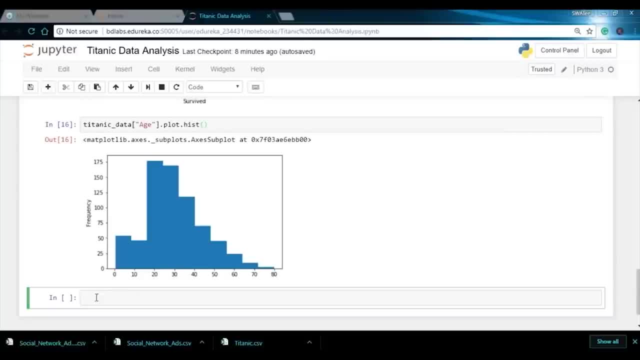 and more mediocre age passengers which are traveling in the Titanic. So next, let me plot a graph of fare as well. So I'll say Titanic data, I'll say fare, and again I'll plot a histogram, So I'll say hist. So here you can see. 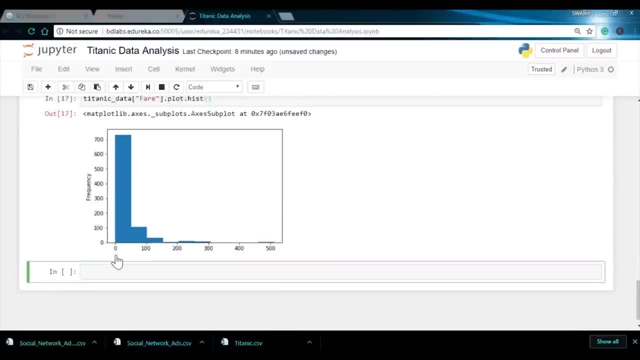 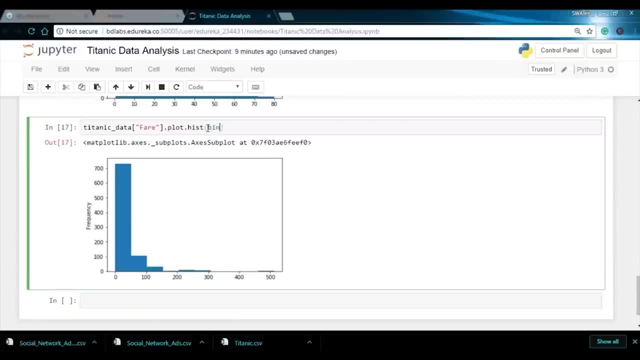 the fare size is between 0 to 100.. Now let me add the bin size so as to make it more clear. So over here I'll say: bin is equals to, let's say, 20, and I'll increase the figure size as well. 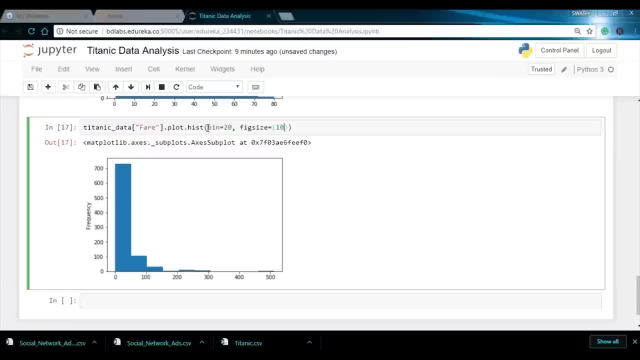 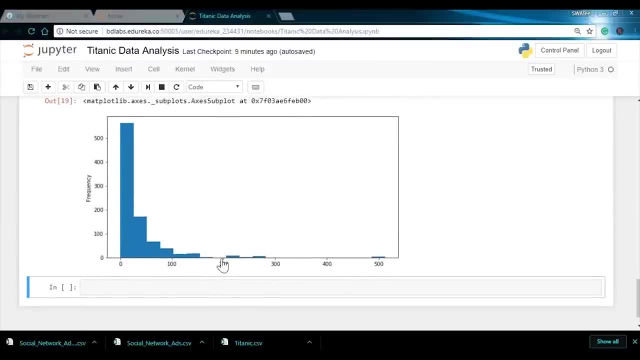 So I'll say the fig size. Let's say I'll give the dimensions as 10 by 5. So it is bins. So this is more clear now. Next, let us analyze the other columns as well. So I'll just type: 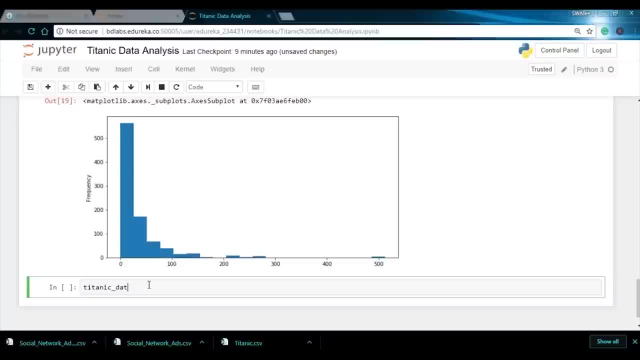 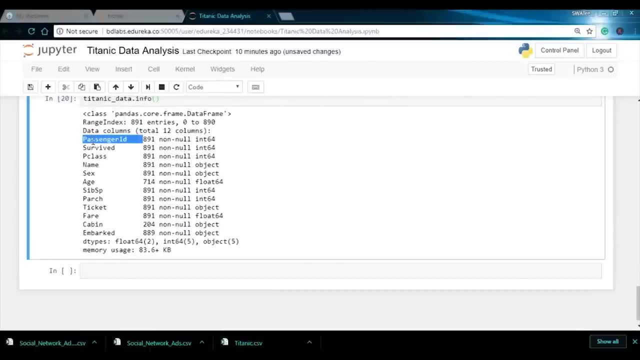 in Titanic data and I want the information as to what all columns are left. So here we have passenger ID, which I guess it's of no use. Then we have see how many passengers survived and how many did not. We also see the analysis on the gender basis. 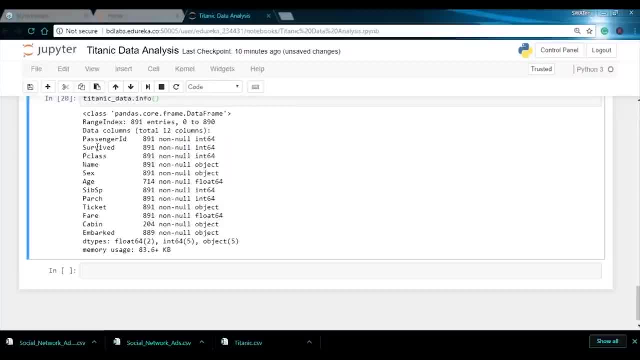 We saw whether female tend to survive more and men tend to survive more. Then we saw the passenger class, whether passenger is traveling in the first class, second class or third class. Then we have the name. So in name we cannot do any analysis. 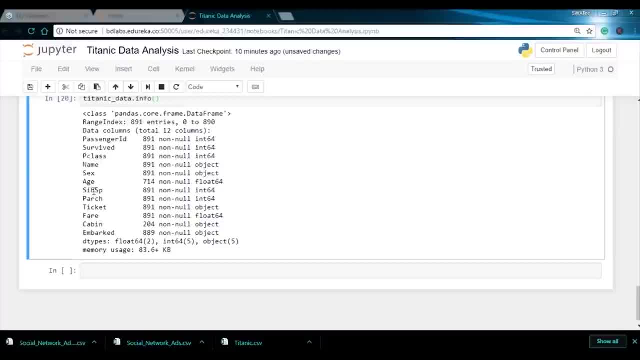 We saw the sex, We saw the age as well. Then we have SibSP, So this stands for the number of siblings, or the spouses, which are aboard the Titanic. So let us do this as well. So I'll say snscountplot. 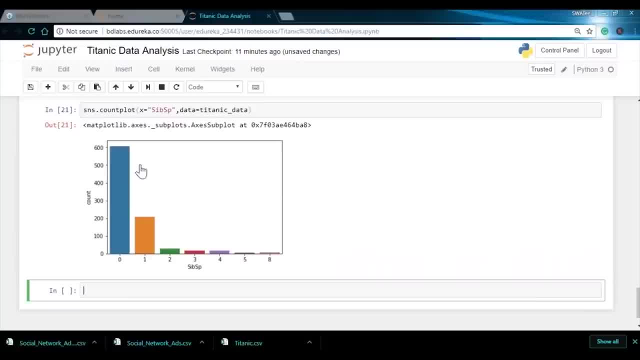 I'll mention x as SibSP so you can see the plot over here. So over here you can conclude that it has the maximum value on zero. So you can conclude that neither a children nor a spouse was on board the Titanic. Now, second most. 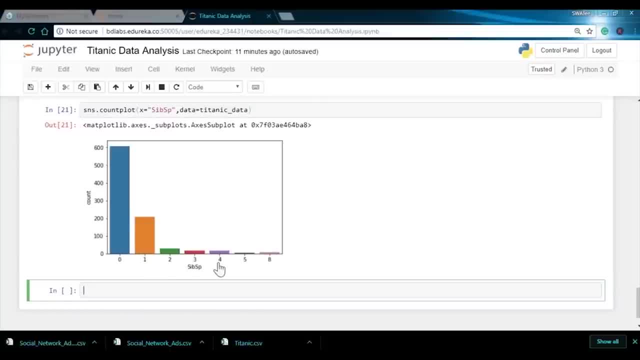 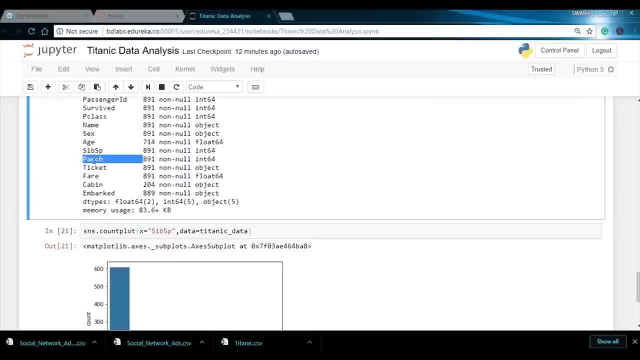 highest value is one and then we have very less values for two, three, four and so on. Next, if I go above, we saw this column as well. Similarly you can do for parj. So next we have parj. or you can say: 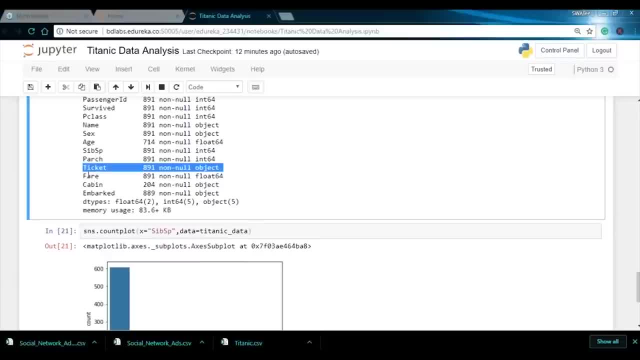 the number of parents. so I don't think so any analysis is required for ticket. Then we have fair, so fair. we have already discussed as in, the people who tend to travel in the first class usually pay the highest fare. Then we have the cabin number. 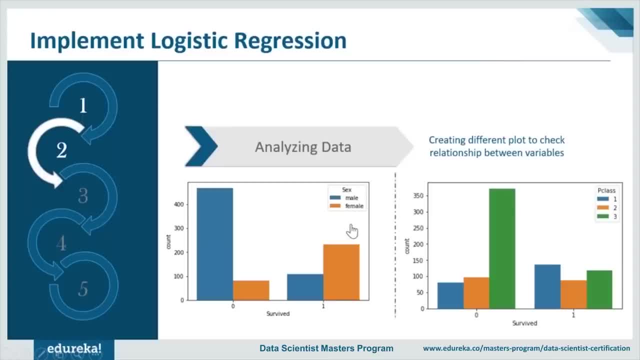 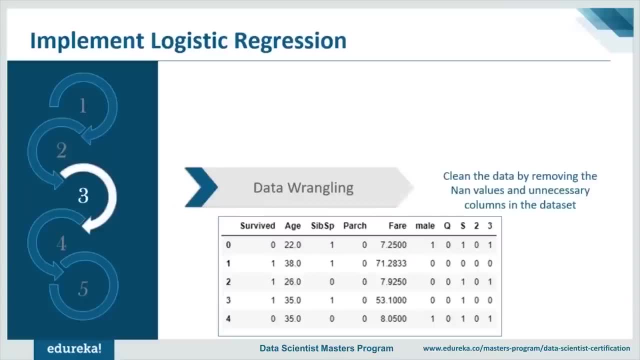 and we have embark. So these are the columns that we'll be doing data wrangling on. So we have analyzed the data and we have seen quite a few graphs in which we can conclude which variable is better than another or what is the relationship they hold. 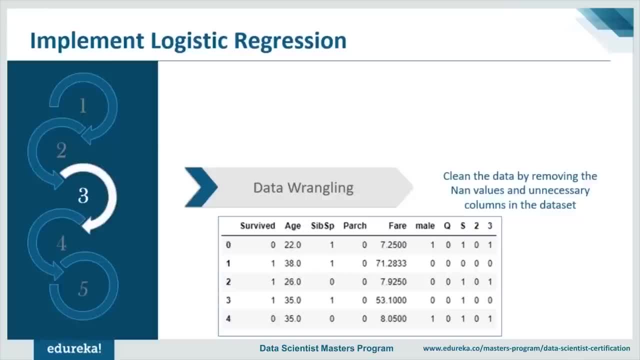 So third step is my data wrangling. So if you have a large data set, you might be having some null values or you can say any and values. So it's very important that you remove all the unnecessary items that are present in your data set. 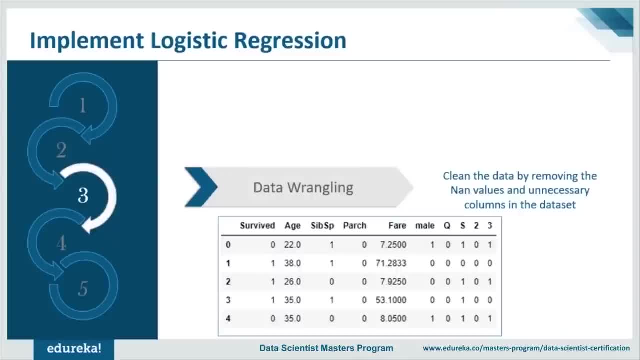 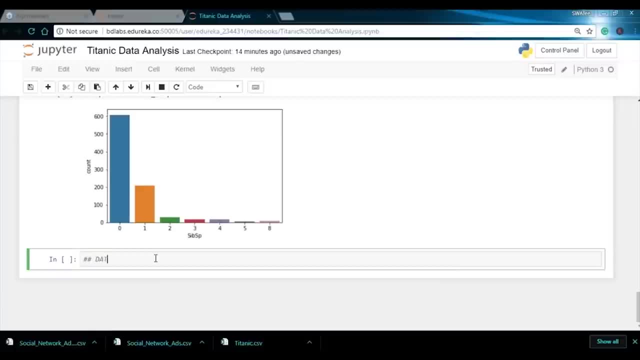 So removing this directly affects your accuracy. So I'll just go ahead and clean my data by removing all the NAN values and unnecessary columns, which has a null value in the data set. So next I'll be performing data wrangling. So first of all, 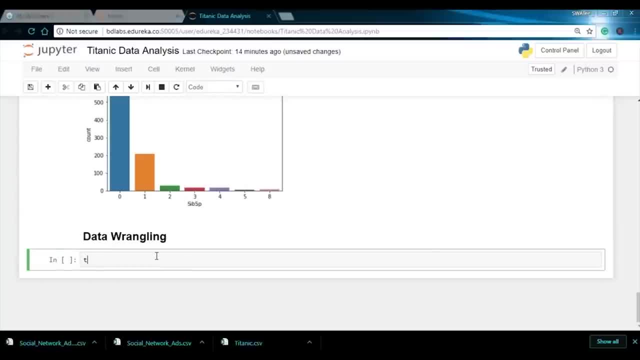 I'll check if my data set is null or not. So I'll say titanic data, which is the name of my data set, and I'll say is null. So this will basically tell me what all values are null and it will return me a boolean result. 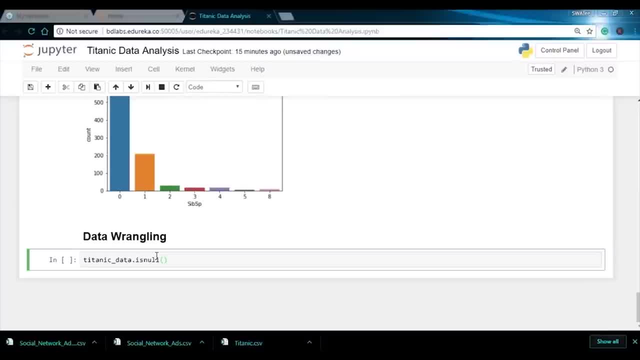 So this basically checks the missing data and your result will be in boolean format. as in, the result will be true or false. So false means if it is not null and true means if it is null. So let me just run this Over here. you can see. 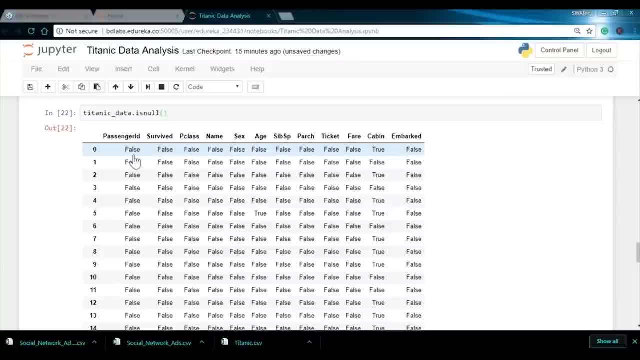 the values as false or true. So false is where the value is not null and true is where the value is not. So over here you can see, in the cabin column we have the very first value, which is null. So we have to do something on this. 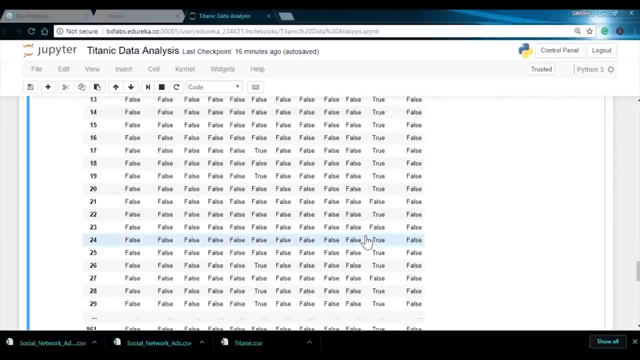 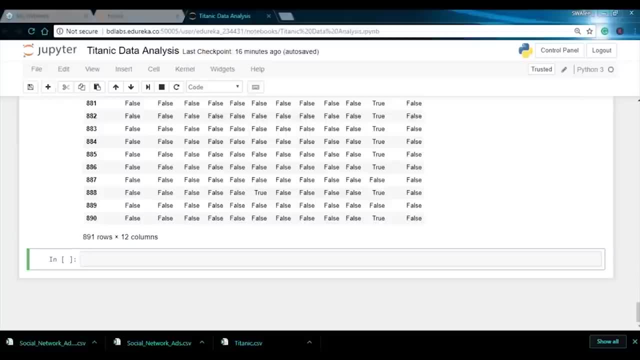 So you can see that we have a large data set, so the counting does not stop and we can actually see the sum of it. We can actually print the number of passengers who have the nan value in each column. So I'll say titanic underscore data. 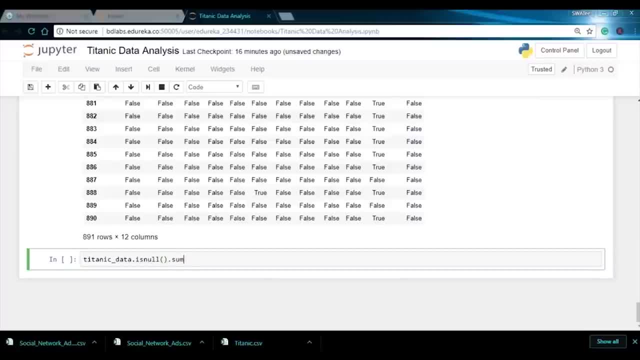 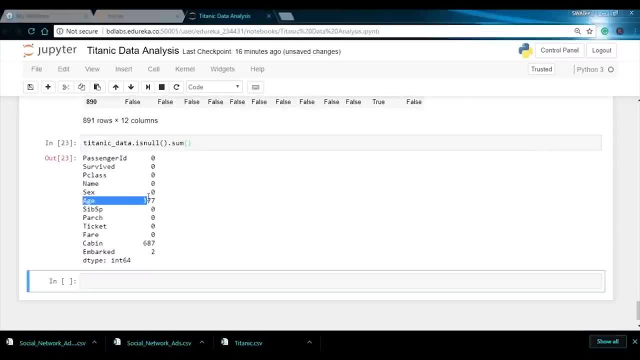 is null and I want the sum of it, So I'll say dot sum. So this will basically print the number of passengers who have the nan values in each column, So we can see that we have missing values in each column. that is, 177.. 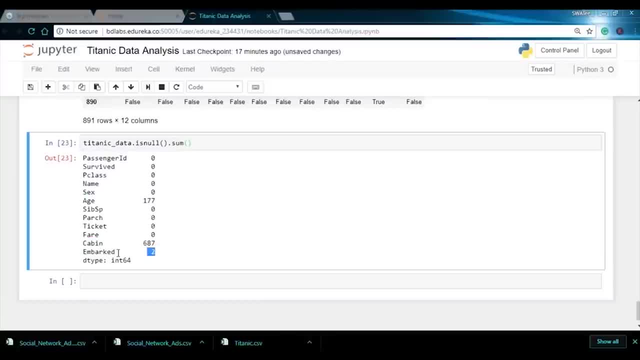 Then we have the maximum value in the cabin column and we have very less in the impact column, that is, 2.. So here, if you don't want to see these numbers, you can also plot a heat map and then you can visually analyze it. So let me just do. 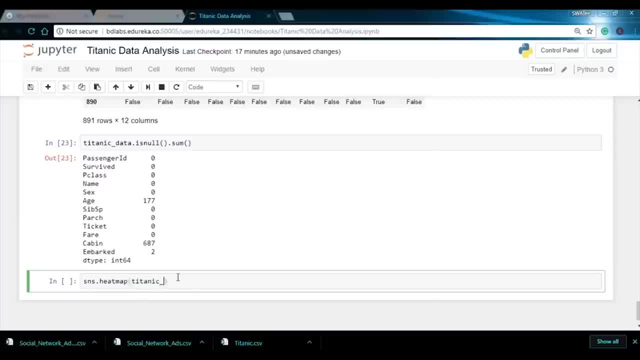 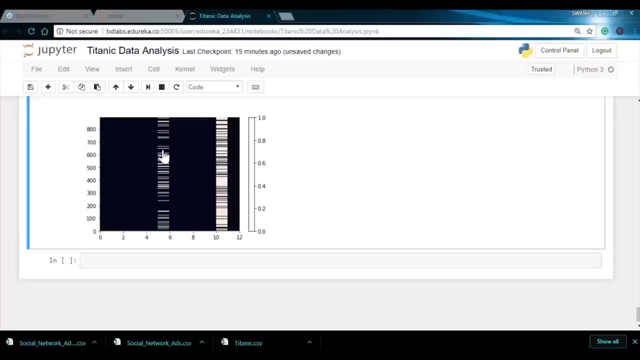 that as well. So I'll say sns dot heat map and say y tick labels false. So I'll just run this. I have already seen that there were three columns in which missing data value was present, So this might be age. So over here almost 20%. 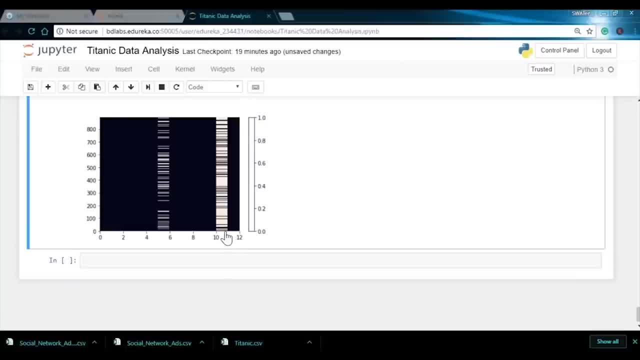 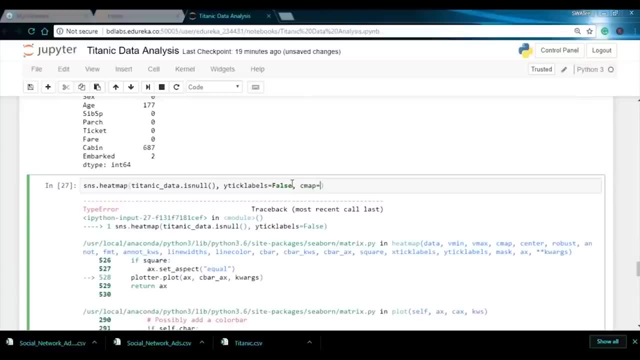 of age column has a missing value. Then we have the cabin columns, So this is quite a large value, and then we have two values for impact column as well. Add a C map for color coding, So I'll say C map. So if I do this, 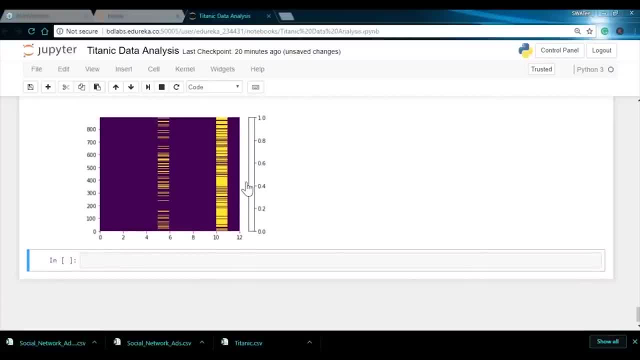 so the graph becomes more attractive. So over here your yellow stands for true or you can say the values are null. So here we have concluded that we have the missing value of age, We have a lot of missing values in the cabin column and we have very less value. 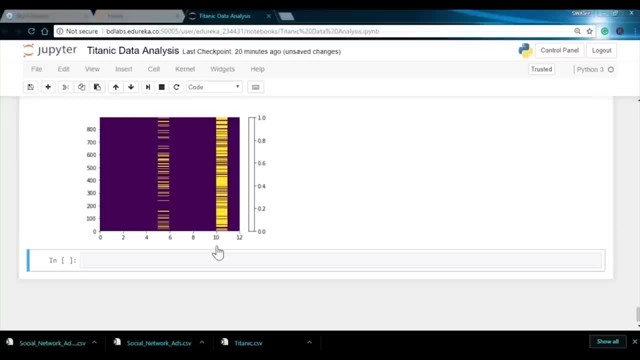 which is not even visible in the embark column as well. So to remove these missing values, you can either replace the values and you can put in some dummy values to it, or you can simply drop the column. So here let us first pick the age column. 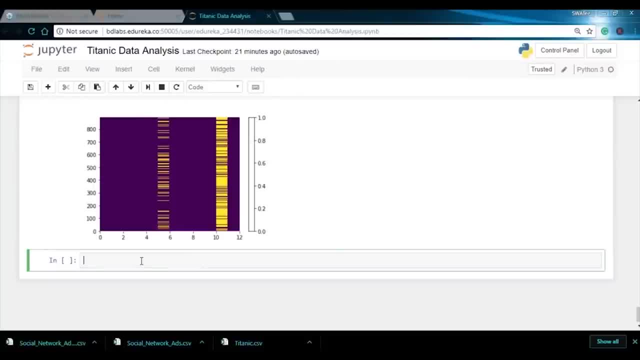 So first let me just plot a box plot and they will analyze with having a column as age. So I'll say sns dot box plot. I'll say X is equals to passenger class, So it's P class. I'll say Y is equals to age. 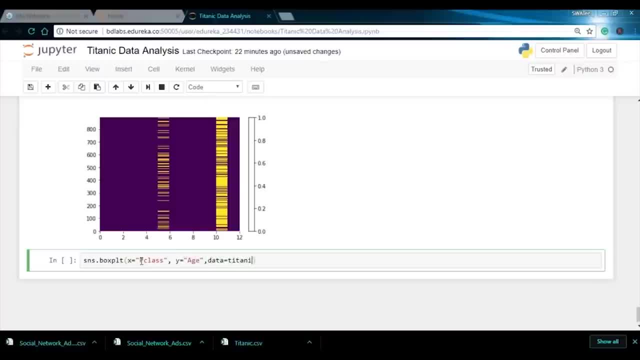 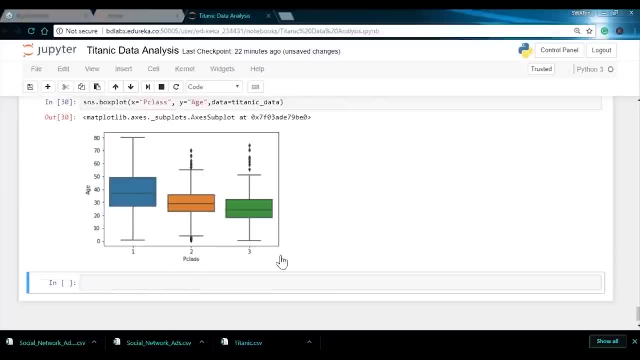 and the data set that I'll be using is Titanic set. So I'll say data is equals to Titanic data. You can see the age in first class and second class tends to be more older, rather than we have it in the third class. Well, that depends. 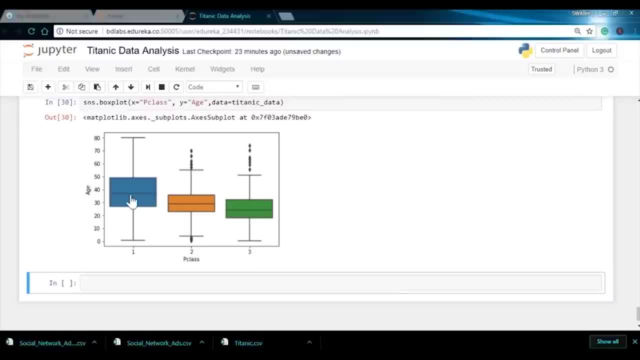 on the experience, how much you earn or might be. there n number of reasons. So here we concluded that passengers who were traveling in class 1 and class 2 what we have in the class 3.. So we have found that we have some missing values in M. 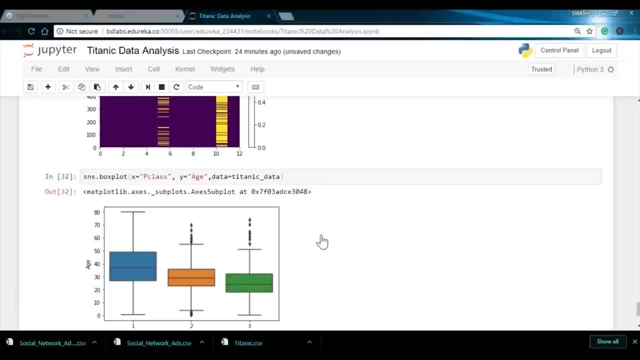 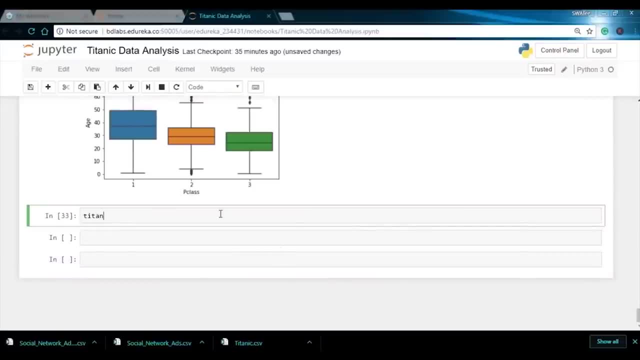 Now one way is to either just drop the column or you can just simply fill in some values to them. So this method is called as imputation. Now to perform data wrangling or cleaning, let us first print the head of the data set. So I'll say: 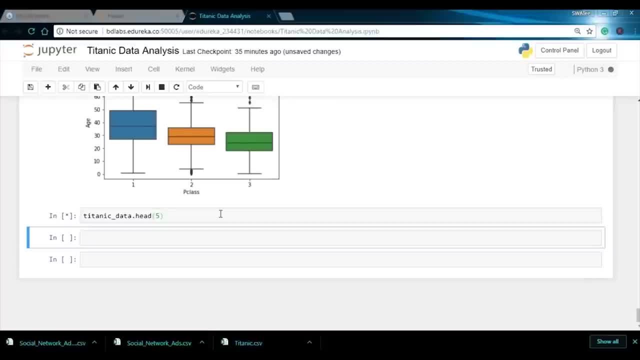 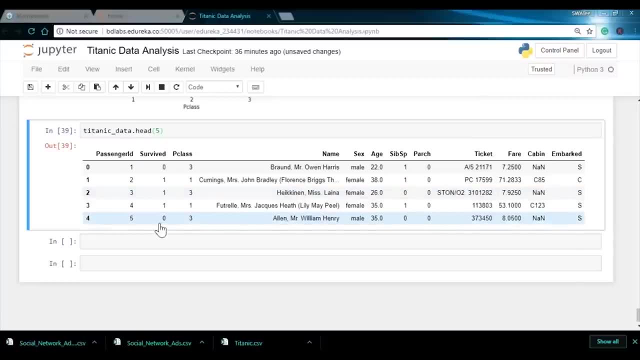 Titanic dot head. so it's Titanic underscore data. Let's say I just want the five rows. So here we have survive, which is again categorical. so in this particular column it can be my y value or the value that I need to predict. Then we have the passenger class. 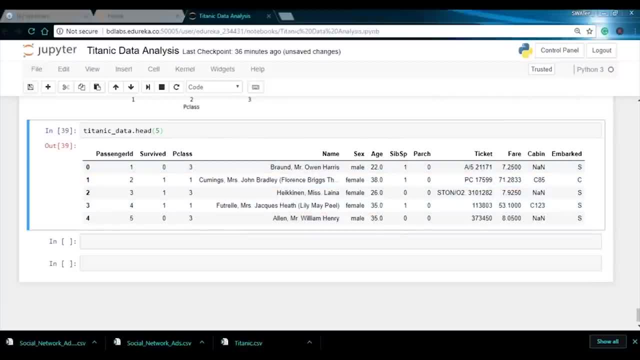 we have the name, then we have ticket number pair: cabin. So over here we have seen that in cabin we have a lot of null values, or you can say the nan values, which is quite visible as well. So first of all, we'll just drop this column. 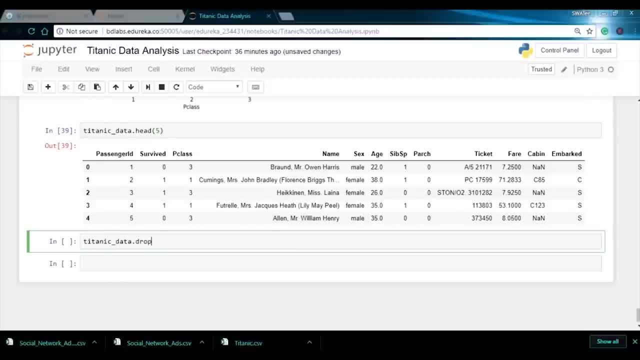 So dropping it, I'll just say Titanic underscore data and I'll simply type in drop and the column which I need to drop. So I have to drop the cabin column. I'll mention the axis equals to 1 and I'll say also to true. 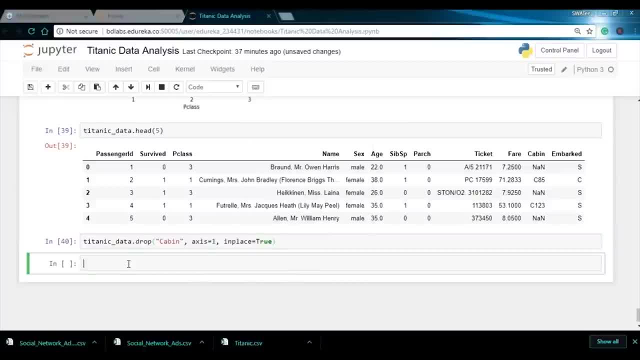 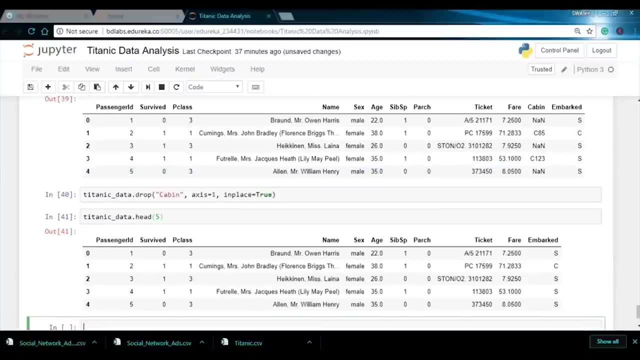 So now again, I'll just print the head and let us see whether this column has been removed from the data set or not. So I'll say: Titanic dot head. So as you can see here, we don't have cabin column anymore. Now you can also. 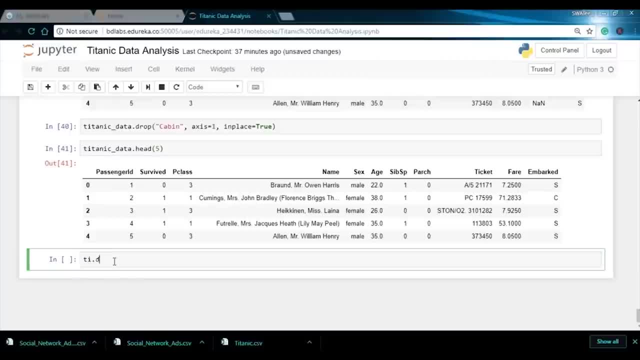 drop the na values. So I'll say: Titanic data dot. drop all the na values. or you can say nan, which is not a number, and I'll say in place, is equals to true Titanic. So over here let me again hit map and let's say: 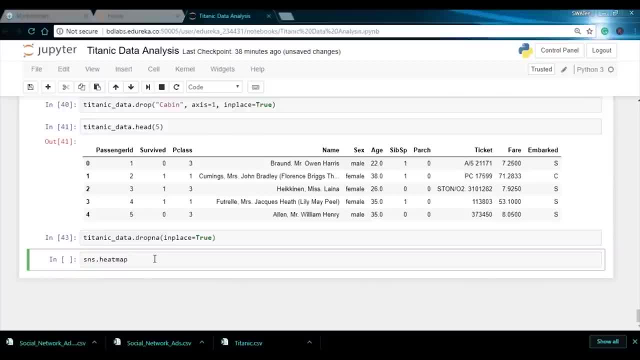 what the values which are before showing a lot of null values. has it been removed or not? So I'll say SNS dot heat map. I'll pass in the data set and check it is null. I'll say y tick labels is equals to false. 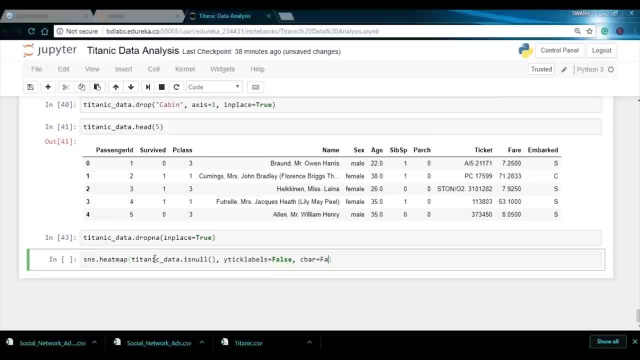 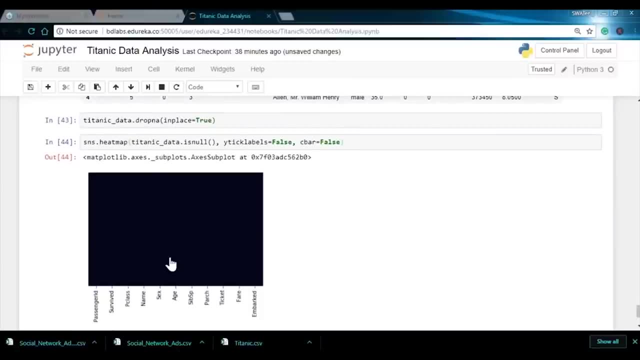 and I don't want color coding. so again I'll say false. So this will basically help me to check whether my values has been removed from the data set or not. So, as you can see here, I don't have any null values. now you can actually. 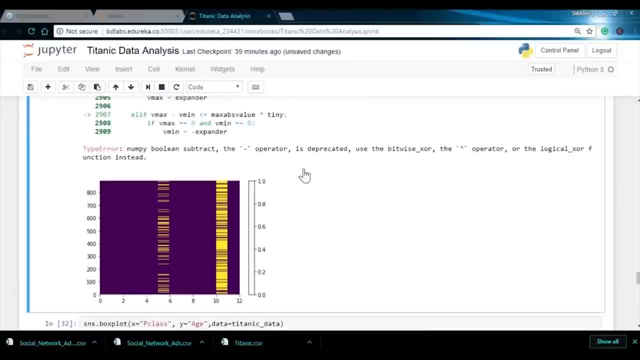 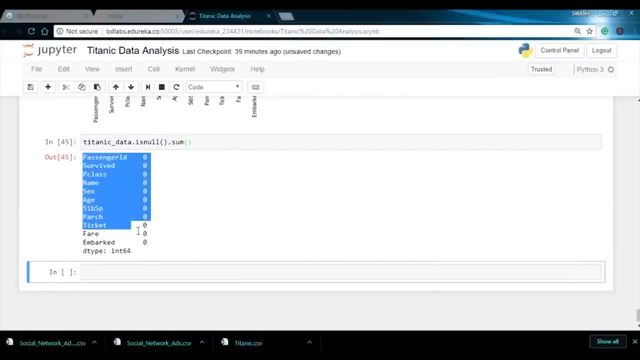 know the sum as well, So I just go above, So I'll just copy this part and I just use the sum function to calculate the sum. So here that tells me that data set is clean, as in, the data set does not contain any null value. 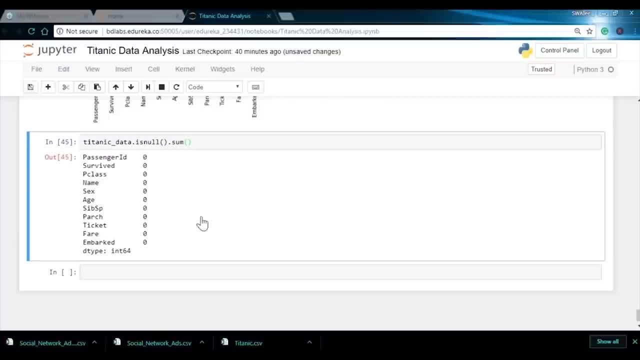 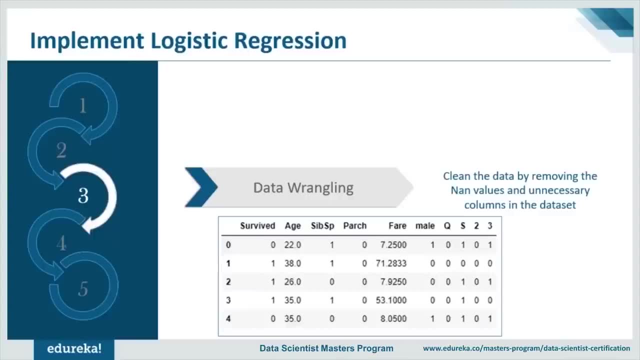 or any any value. So now we have wrangled our data. you can say cleaner data. So here we have done just one step in data wrangling, that is just removing one column out of it. Now you can do a lot of things you can actually fill. 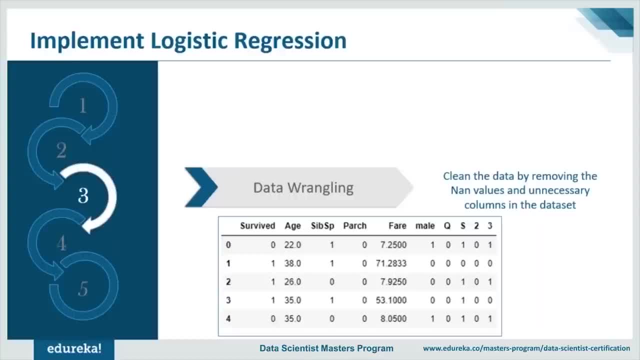 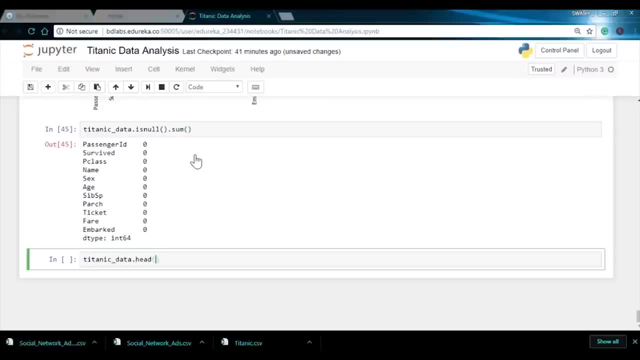 in the values some other values, or you can just calculate the mean and then you can just put in the null values. But now if I see my data set, so I'll say Titanic data dot head. But now if I see over here, I have a lot of string values. 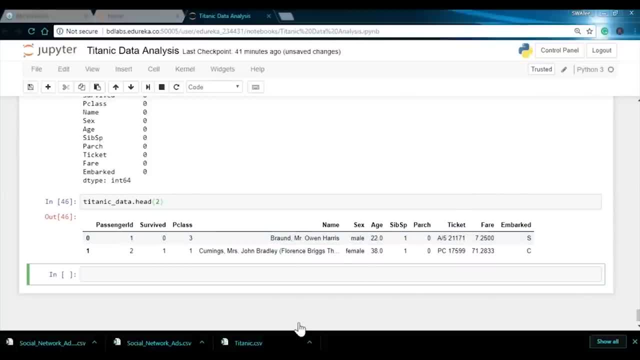 So this has to be converted to categorical variables in order to implement logistic regression. So what we will do, we will convert this to categorical variable into some dummy variables, and this can be done using Pandas, because logistic regression just take two values. So whenever you apply, 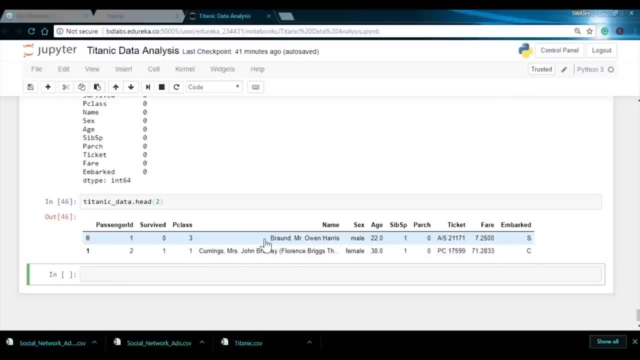 machine learning, you need to make sure that there are no string values present, because it won't be taking these as your input variables. So using string, you don't have to predict anything. But in my case I have the survived columns, so I need to predict. 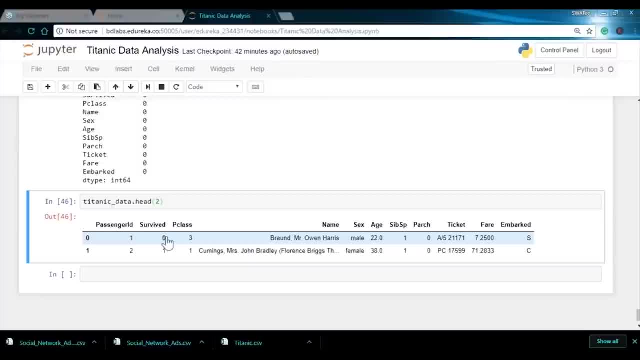 how many people tend to survive and how many did not. So zero stands for did not survive and one stands for survive. So now let me just convert these variables into dummy variables. So I'll just use Pandas and I'll say: pd dot, get dummies. 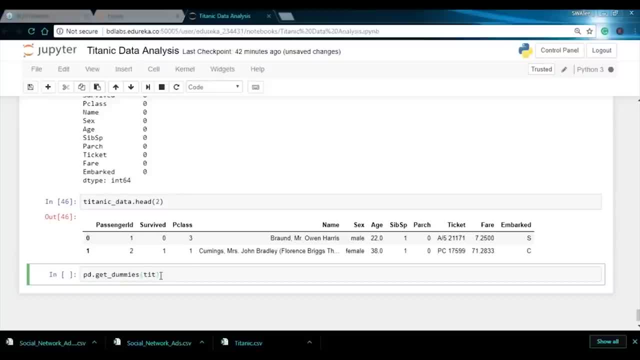 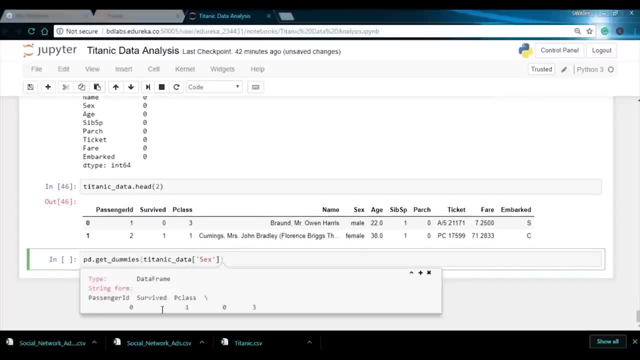 You can simply press tab to auto complete, I'll say Titanic data and I'll pass the string values as six. So you can just simply click on ship plus tab to get more information on this. So here we have the type data frame and we have the passenger. 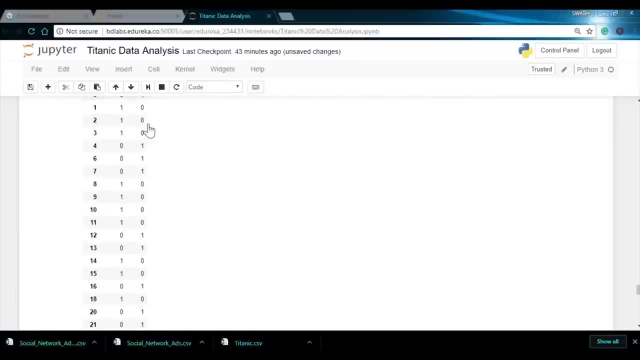 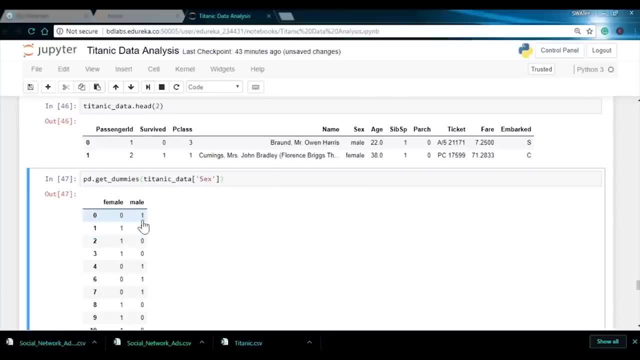 ID survived and passenger class. So if you run this, you'll see that zero basically stands for not a female and one stand for it is a female. Similarly for male, zero stands for it's not male and one stand for male. Now we don't require 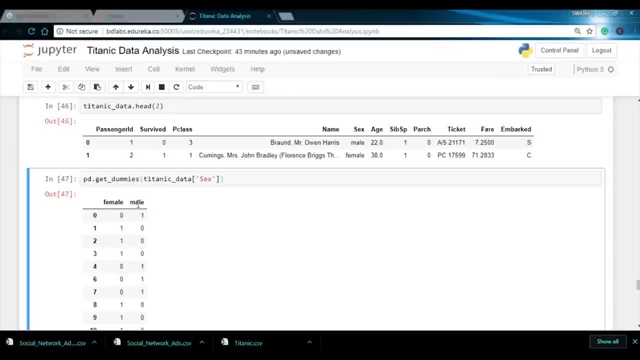 both these columns, because one column itself is enough to tell us whether it's male, or you can say female or not. So let's say, if I want to keep the value of male, I'll say: if the value of male is one, so it is definitely a male. 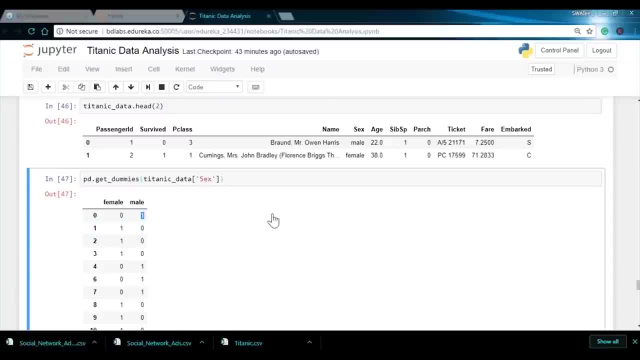 and it is not a female. So that is how you don't need both of these values. So for that I'll just remove the first column. let's say female, so I'll say drop first and true. So over here it has given me just one column. 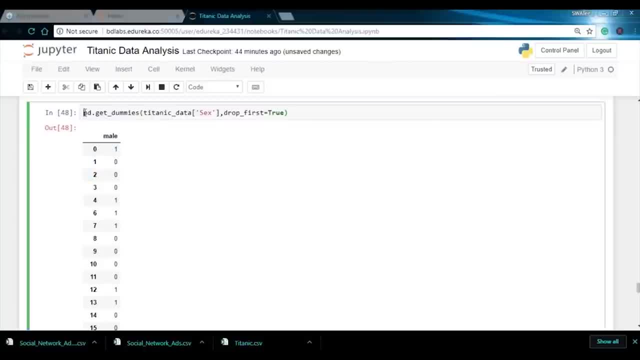 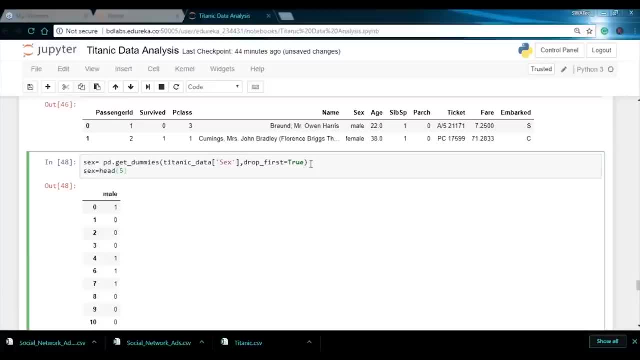 which is male and has the value zero and one. Now let me just set this as a variable. let's say sex. So over here I can say sex dot head, and I'll just want to see the first. sorry, it's dot. So this is how my data 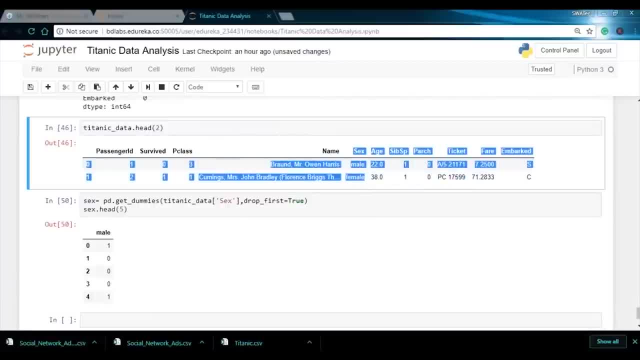 looks like Now here we have done it for sex. then we have the numerical values in age, we have the numerical values in spouses, then we have the ticket number, we have the fare and we have embarked as well. So in embarked the values are in S, C and Q. 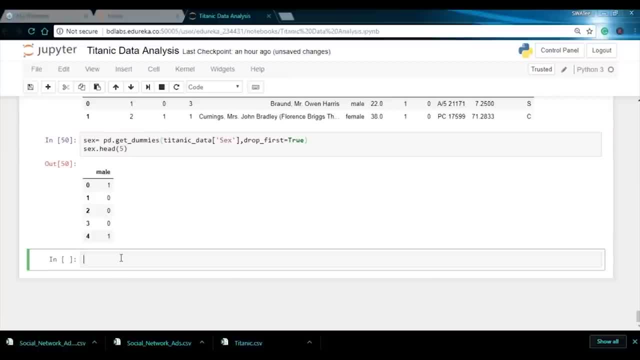 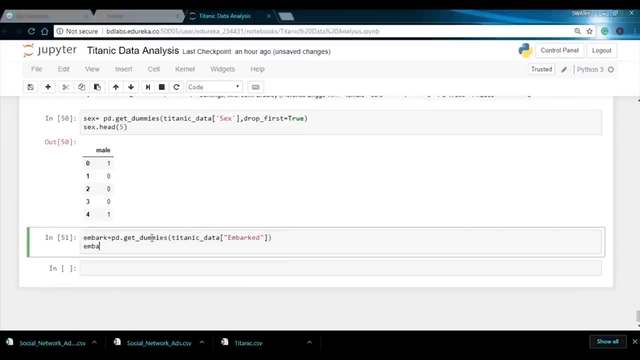 So here also we can apply this get dummy function. So let's say I'll take a variable. let's say embark, I'll use the pandas library, I'll enter the column name that is embarked. Let me just print the head of it. 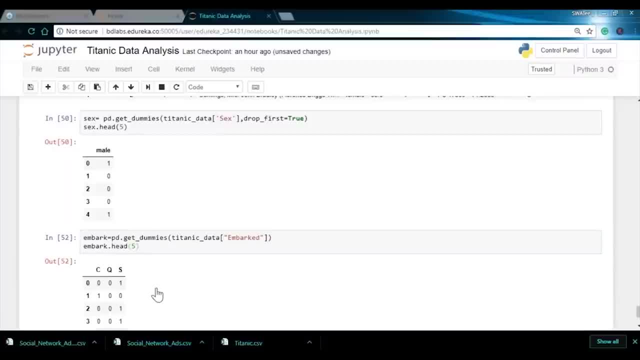 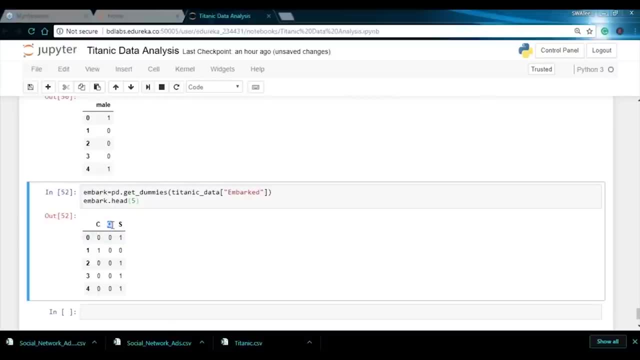 So I'll say embarked dot head. So over here we have C, Q and S. Now here also we can drop the first column, because these two values are enough, whether the passenger is either traveling for Q, that is, Kuenstown, S for Southam, and if both. 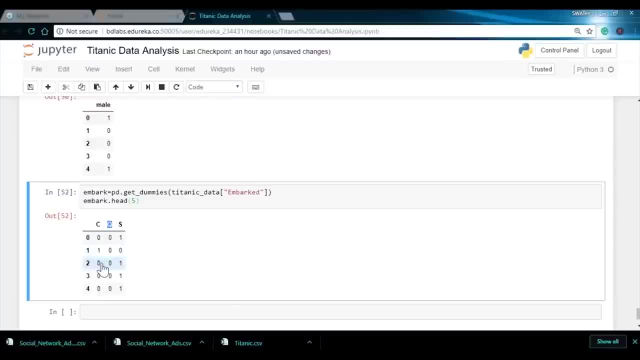 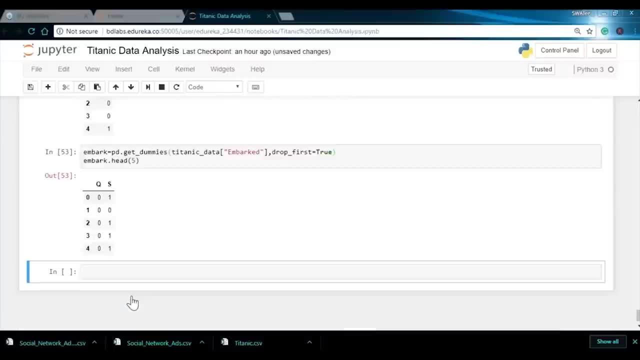 the values are zero, then definitely the passenger is from Cherbourg. that is the third value. So you can again drop the first value. So I'll say drop and true. Let me just run this. So this is how my output looks like Now. similarly, you can: 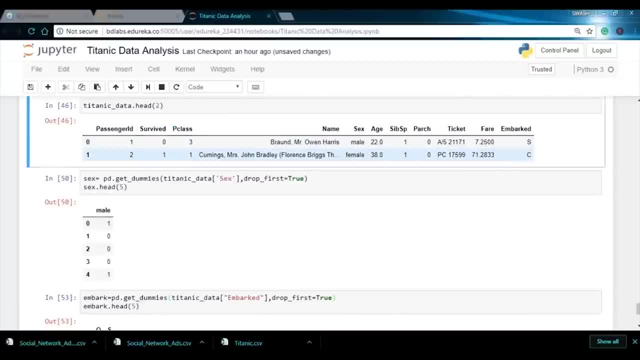 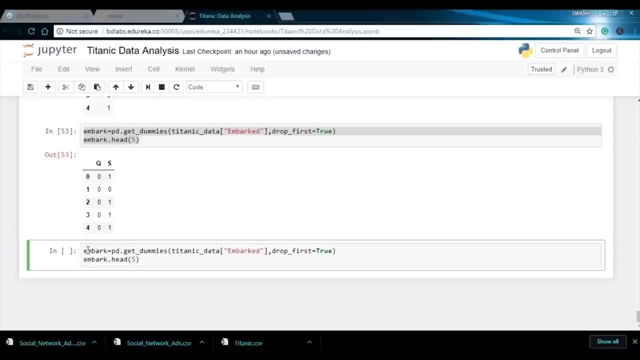 do it for passenger class as well. So here also we have three classes: one, two and three. So I'll just copy the whole statement. So let's say I want the variable name, let's say PCL. I'll pass in the column name, that is P class. 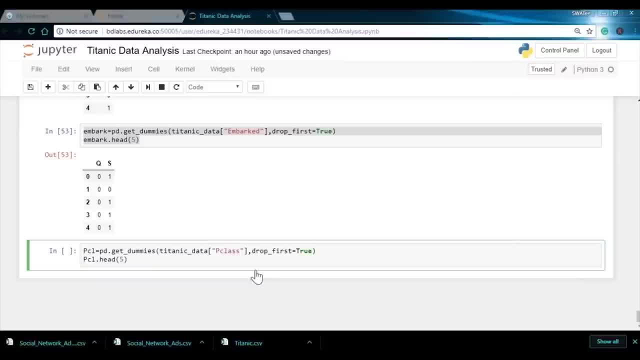 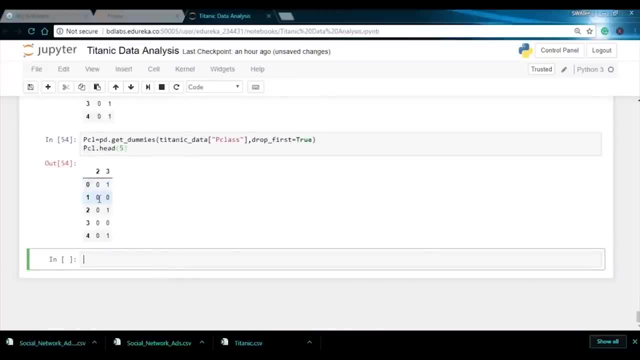 and I'll just drop the first column. So here also the values will be one, two or three, and I'll just remove the first column. So here we just left with two and three. So if both the values are zero, then definitely the passengers traveling. 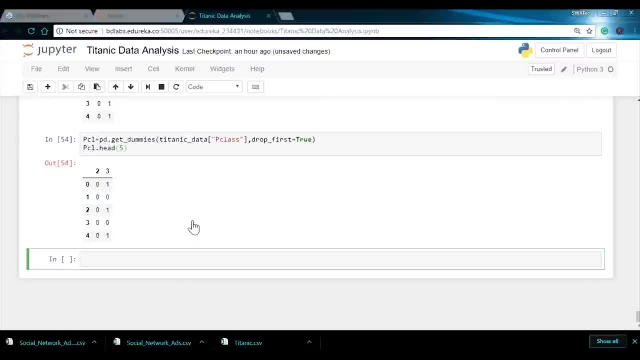 in the first class. Now we have made the values as categorical. Now my next step would be to concatenate all these new rows into a data set. Or you can say Titanic data. using the Pandas will just concatenate all these columns. So I'll say pconcat. 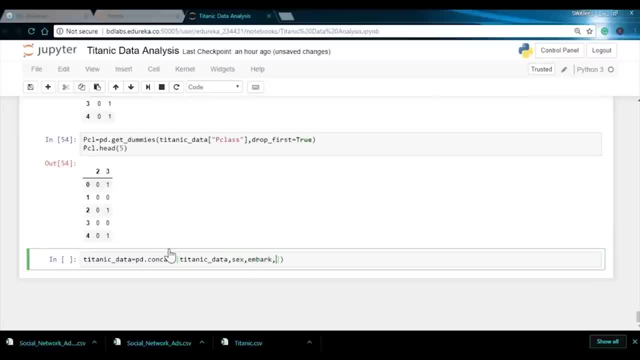 and I'll say we have to concatenate sex, We have to concatenate Embark and PCL, and then I'll mention the access to one. I'll just run this. Okay, I need to print the head, So over here you can see that these columns. 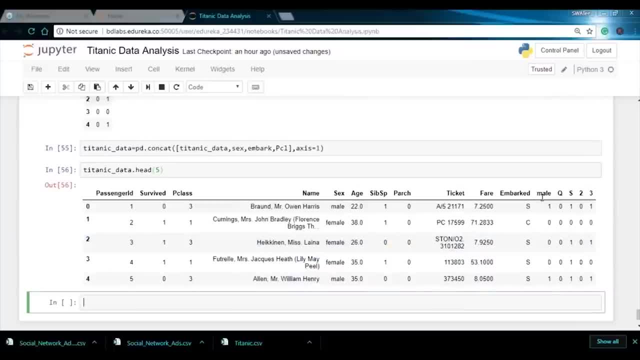 have been added over here. So we have the male column, which basically tells whether a person is male or it's a female. Then we have the Embark, which is basically Q and S. So if it's traveling from Kuenstown, the value would be one. 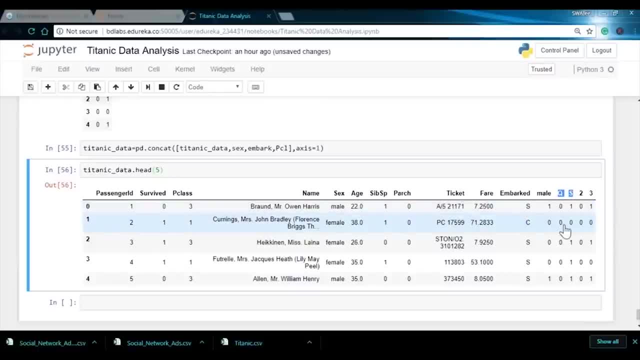 else it would be zero. And if both of these values are zero, it is definitely traveling from Cherbourg. Then we have the passenger class as two and three. So if the value of both these is zero, then the passengers traveling in class one. So I hope you got. 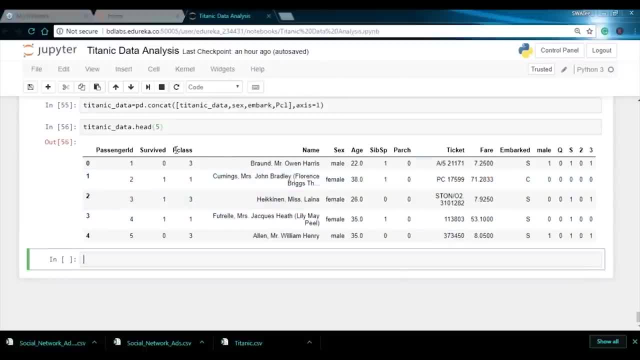 this till now. Now these are the irrelevant columns that we have it over here, So we can just drop these columns. We'll drop in P class the Embark column and the sex column. So I'll just type in Titanic data dot drop and I'll mention the. 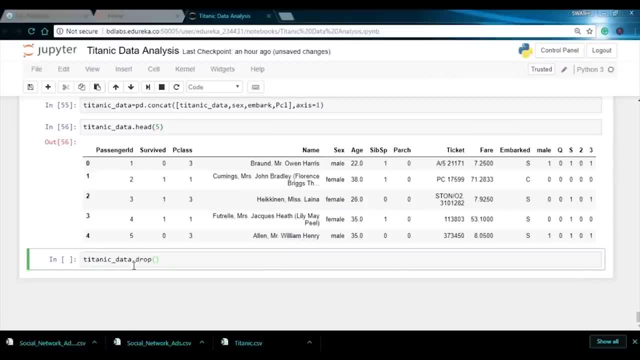 columns that I want to drop. So I'll say I'll even delete the passenger ID, because it's nothing but just the internal index value, which is starting from one. So I'll drop this as well. Then I don't want name as well. 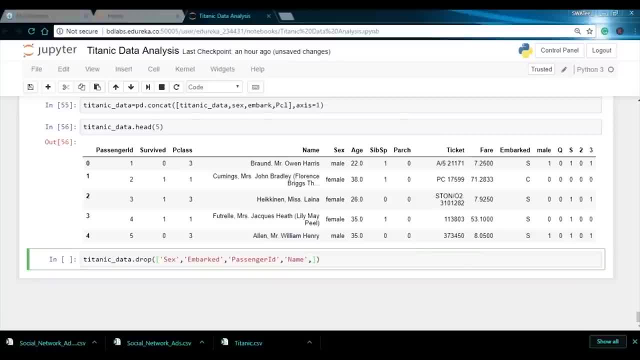 So I'll delete name as well. Then what else we can drop? We can drop the ticket as well, And then I'll just mention the axis and I'll say: in place is equals to true. Okay, So my column name starts from uppercase. 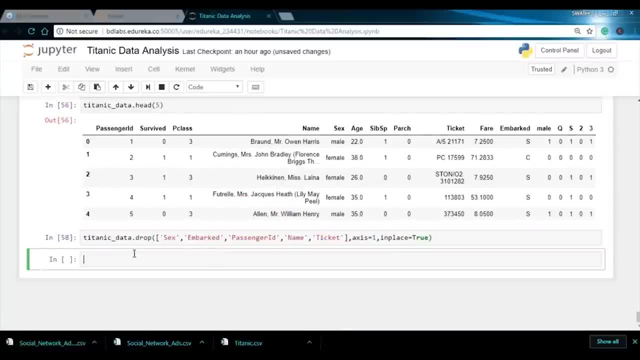 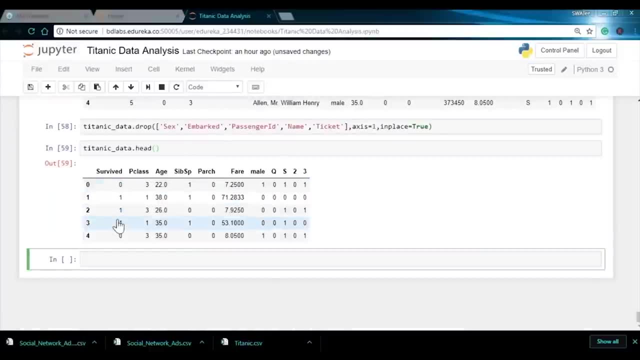 So these has been dropped. Now let me just print my data set again. So this is my final data set. guys, We have the survived column, which has the value zero and one. So I'm going to change the value zero and one. then we have 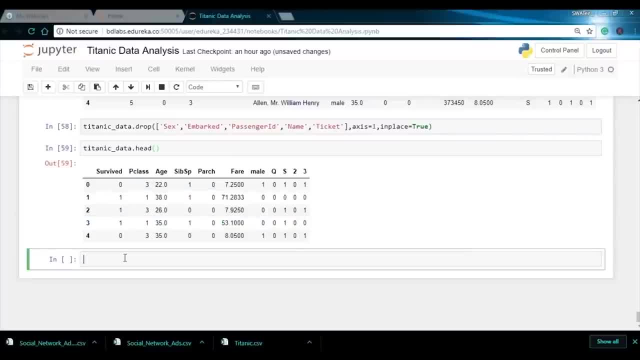 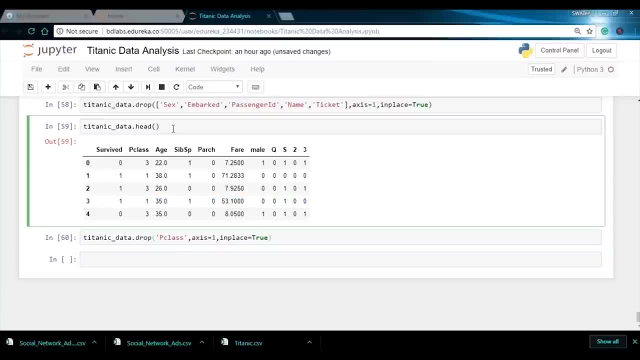 the passenger class. Oh, we forgot to drop this as well, So, no worries, I'll drop this again. So now let me just run this Over here. We have the survive, We have the age, We have the Sib SP. 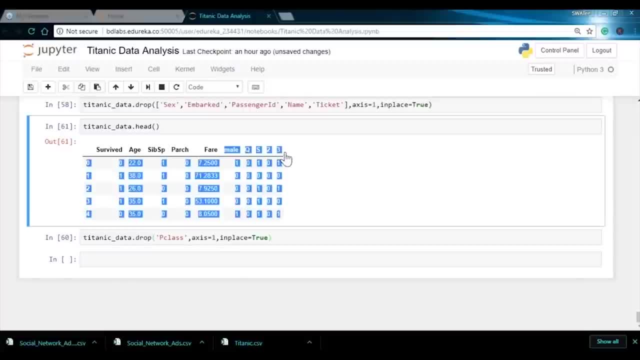 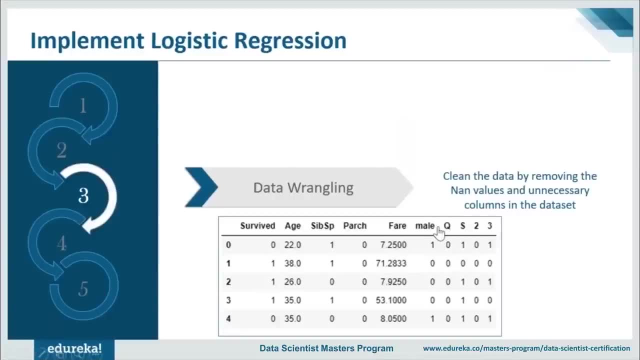 We have the parts, We have fair meal, and these we have just converted. So here we have just performed data wrangling, or you can say clean the data, and then we have just converted the values of gender to mail. Then we have just then embarked to Q&S. 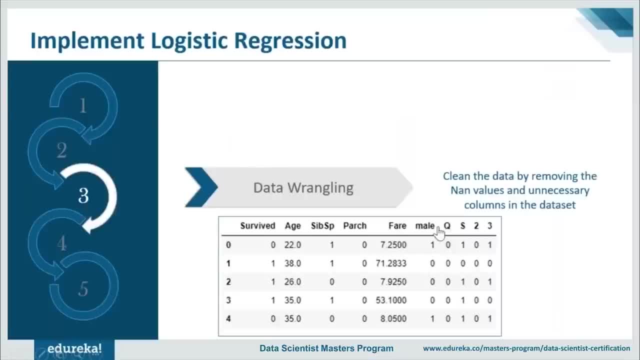 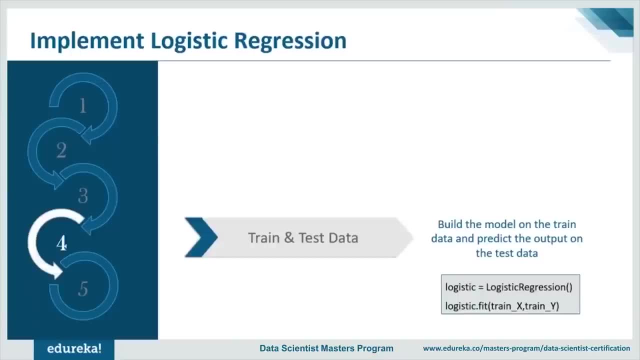 and the passenger class to two and three. So this was all about my data running or just cleaning the data. Then my next step is training and testing your data. So here we will split the data set into train subset and test subset, and then what we'll do. 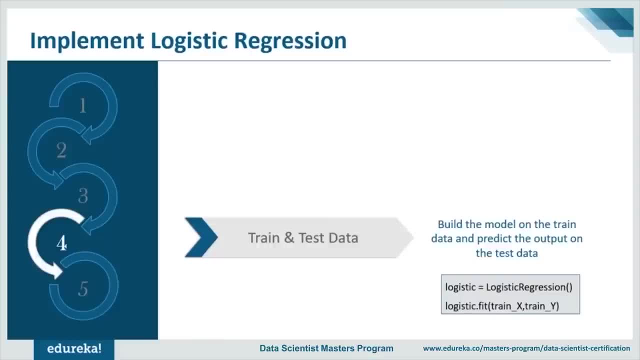 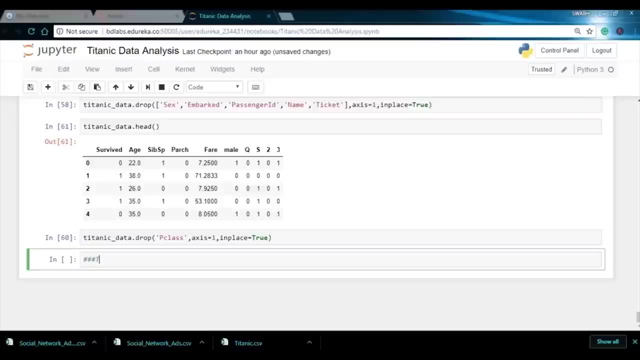 will build a model on the train data and then predict the output on your test data set. So let me just go back to Jupiter and let us implement this as well Over here. I need to train my data set, So I'll just put this: 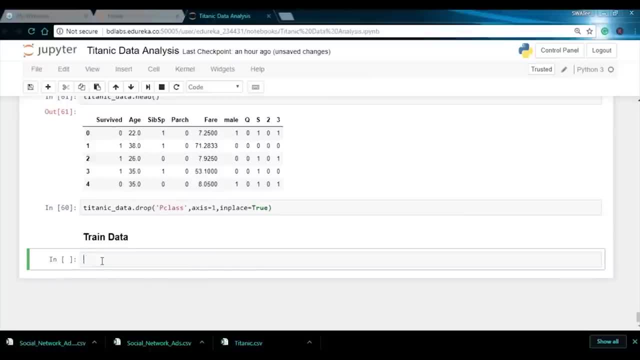 in deep heading three. So over here I need to train my data set. So over here you need to define your dependent variable and independent variable. So here my Y is the output, or you can say the value that I need to predict. 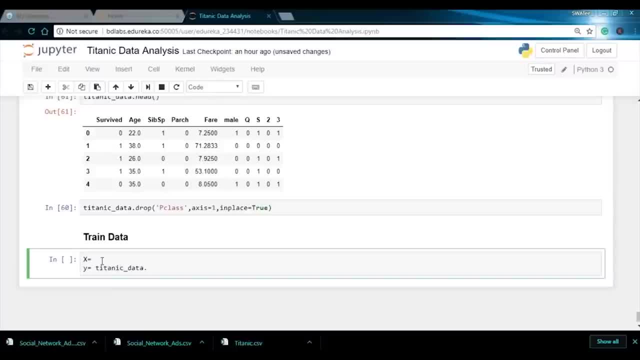 So over here I'll write Titanic data. I'll take the column which is survive. So, basically, I have to predict this column, whether the passenger survived or not, and, as you can see, we have the discrete outcome, which is in the form of zero and one and rest. 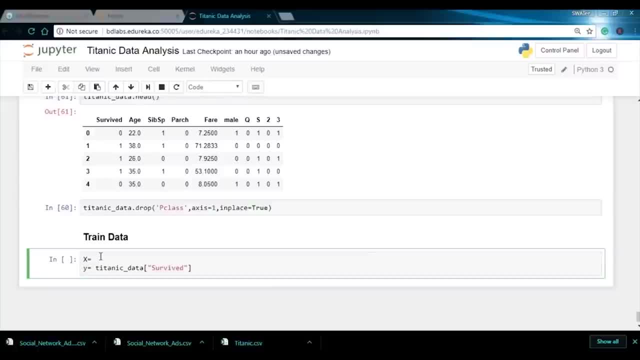 all the things. we can take it as a features or you can say independent variable. So I'll say Titanic data set, Data not drop. So we'll just simply drop this, survive and all the other columns will be my independent variable. So everything else. 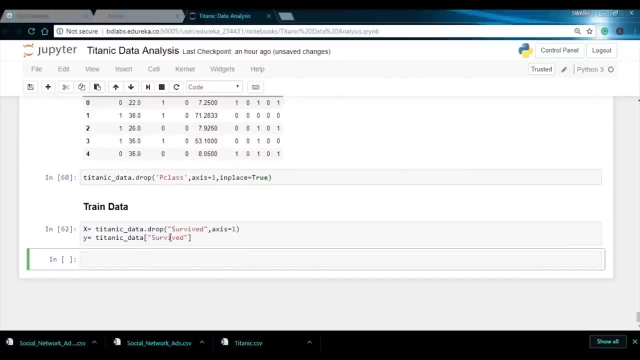 are the features which leads to the survival rate. So once we have defined the independent variable and the dependent variable, next step is to split your data into training and testing subset. So for that we'll be using sklearn. I just type in from sklearn: 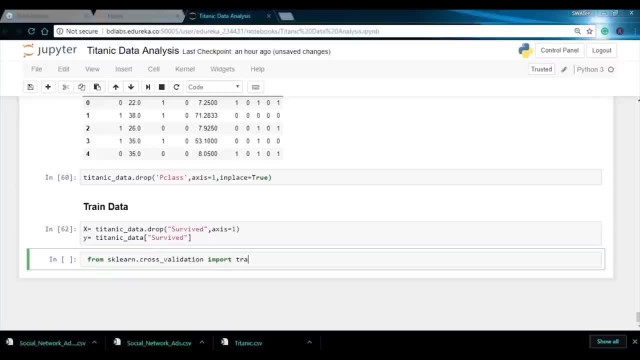 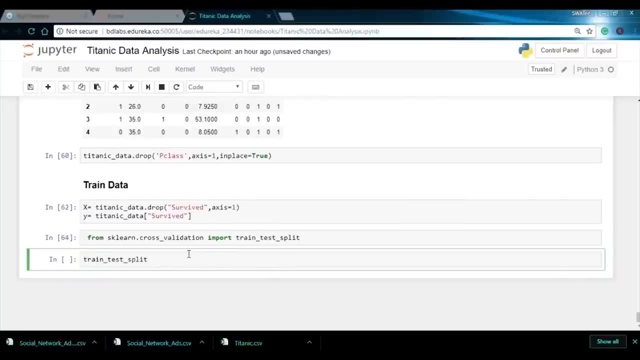 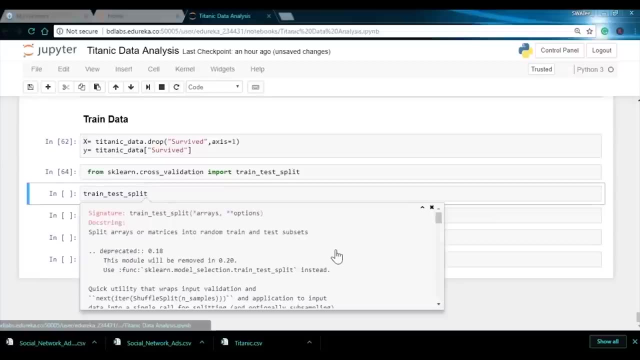 cross validation: import train test split. Now here, if you just click on shift and tab, you can go to the documentation and you can just see the examples over here. I'll click on plus to open it and then I just go to examples and see how you can. 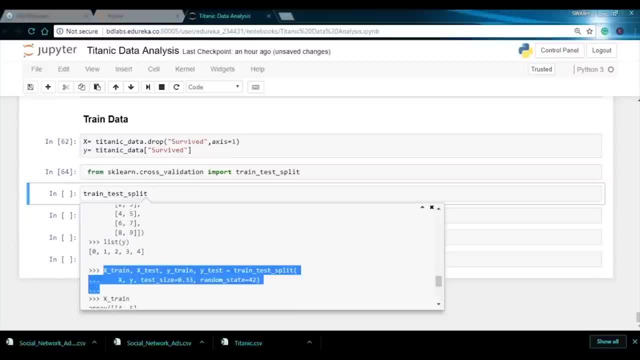 split your data. So over here you have X train, X test, Y train, Y test and then, using this train test split, you can just pass in your independent variable and dependent variable and just define a size and a random state to it. So let me just copy this: 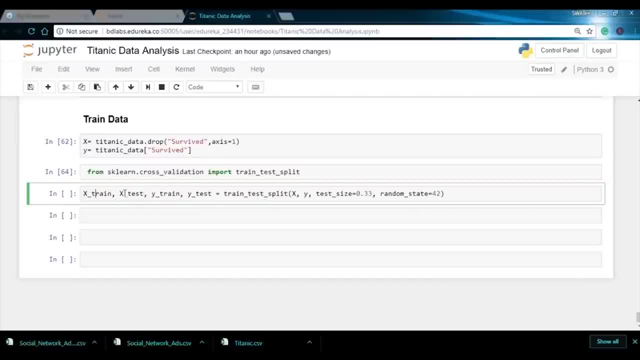 and I'll just paste it over here: Over here we'll train test, then we have the dependent variable, train and test, and using the split function we'll pass in the independent and dependent variable and then we'll set a split size. So let's say: 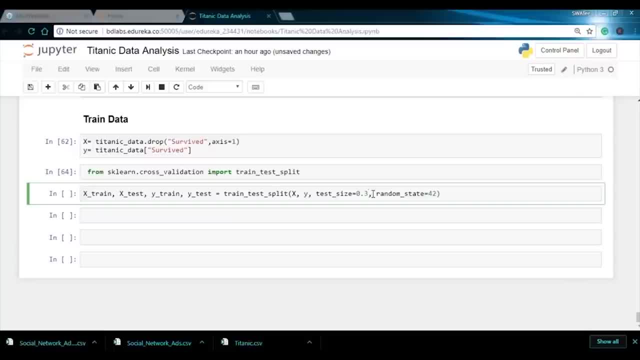 I'll put it at 0.3. so this basically means that your data set is divided in 0.3, that is, in 70: 30 ratio, and then I can add any random state to it. So let's say I'm applying one. 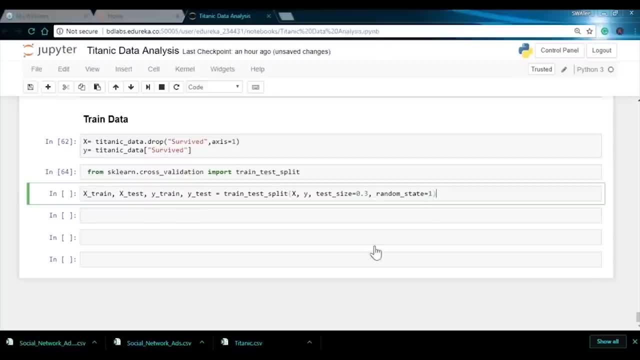 this is not necessary. if you want the same result as that of mine, you can add the random state. So this will basically take exactly the same sample every time. Next, I have to train and predict by creating a model. So here logistic regression will grab from the 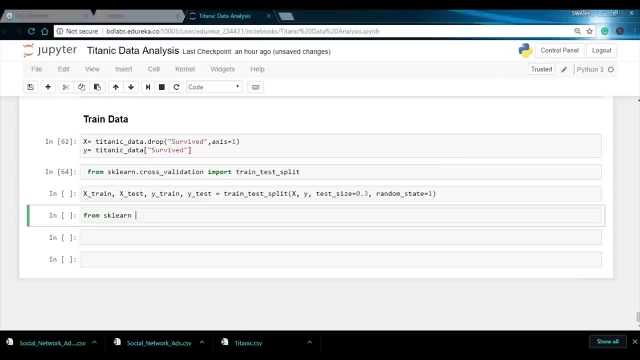 linear regression. So next I'll just type in from sklearnlinearmodel import logistic regression. Next I'll just create the instance of this logistic regression model. So I'll say log model is equals to logistic regression. Now I just need to fit my model. 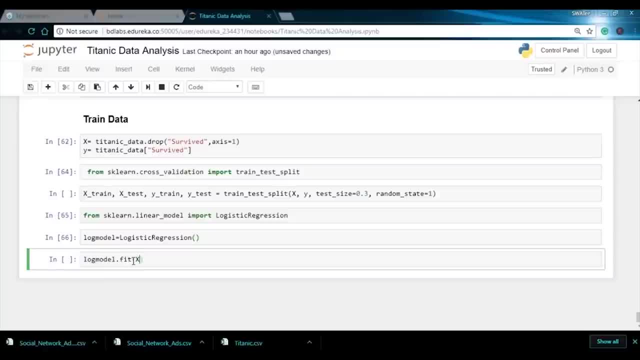 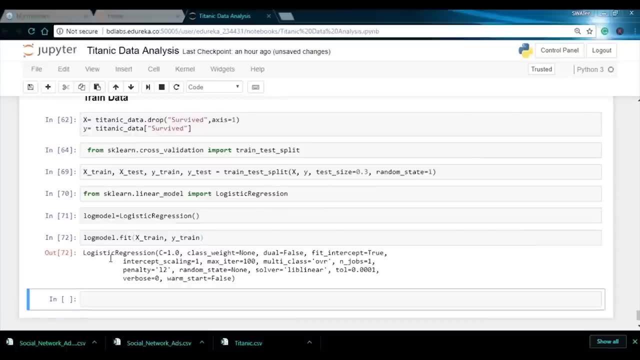 so I'll say logmodelfit and I'll just pass in my x train and y train. Alright, so here it gives me all the details of logistic regression. So here it gives me the class, weight, dual fit, intercept and all those things. 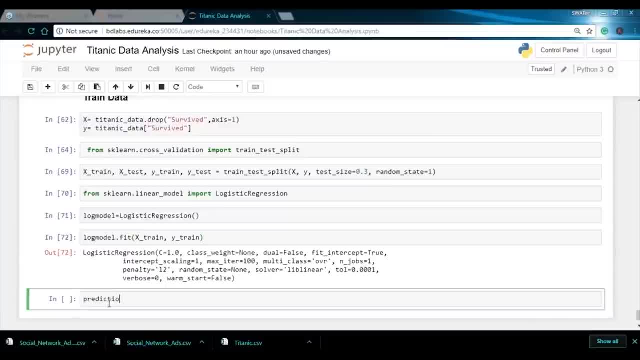 Then what I need to do. I need to make prediction. So I'll take a variable- let's say predictions, and I'll pass on the model to it. So I'll say logmodelpredict and I'll pass in the value that is xtest. 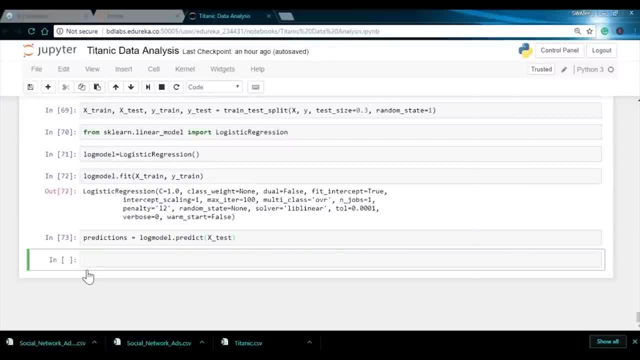 So here we have just created a model. fit that model, and then we had made predictions. So now to evaluate how my model has been performing, so you can simply calculate the accuracy, or you can also calculate a classification report. So don't worry guys, I'll be showing. 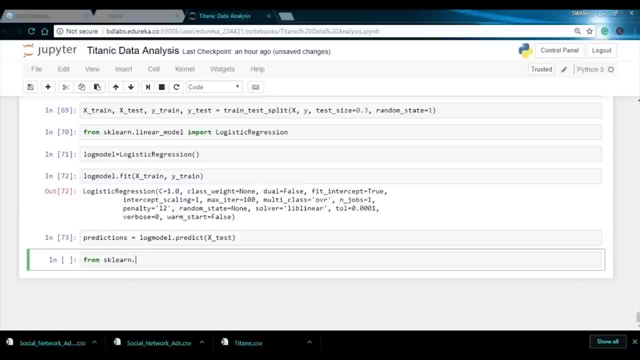 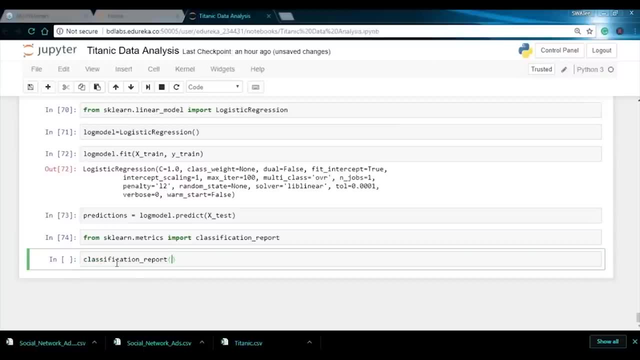 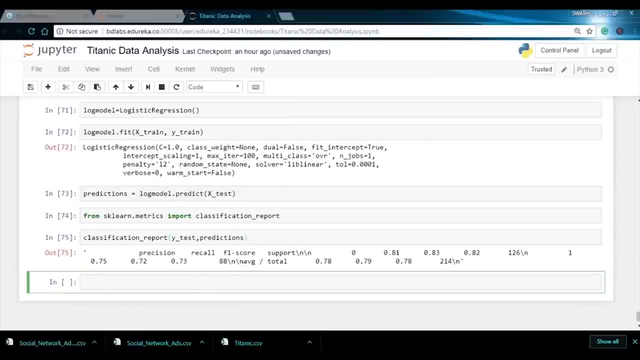 both of these methods. So I'll say from sklearnmetrics import classification report. So over here I'll use classification report and inside this I'll be passing in ytest and the predictions. So, guys, this is my classification report. So, guys, this is my classification report. 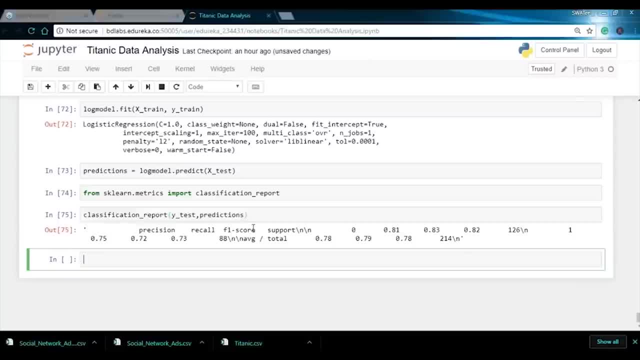 So over here I have the precision, I have the recall, we have the F1 score and then we have support. So here we have the value of precision as 75, 72 and 73, which is not that bad. Now, in order to calculate the accuracy as well. 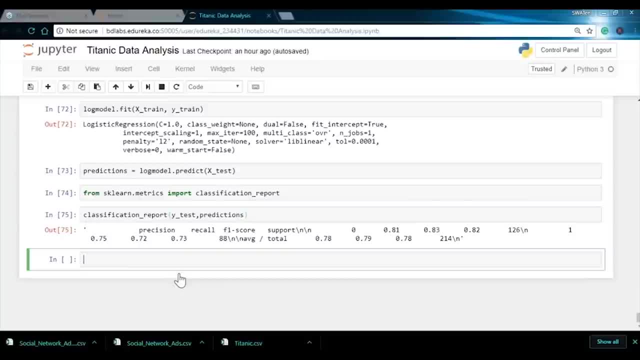 you can also use the concept of confusion matrix. So if you want to print the confusion matrix, I'll simply say: from sklearnmetrics, import confusion matrix first of all, and then we'll just print this. So here my function has been imported successfully, so I'll just 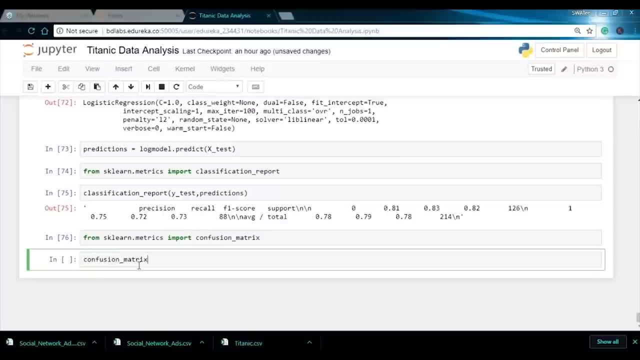 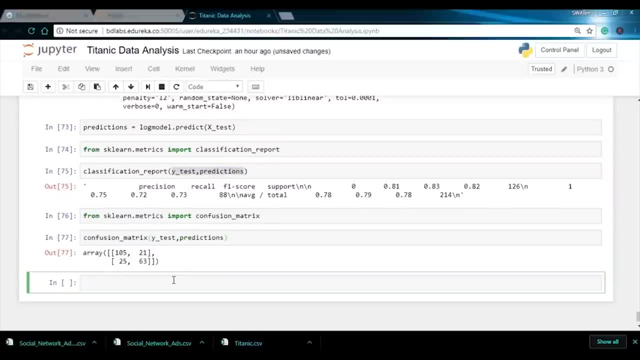 say confusion matrix, and I'll again pass in the same variables, which is ytest and predictions. So I hope you guys already know the concept of confusion matrix. So I'll just tell you in a brief what confusion matrix is all about. So confusion matrix. 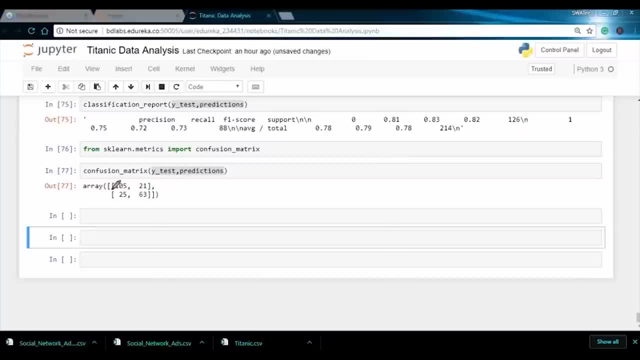 is nothing but a two by two matrix which has four outcomes. This basically tells us that how accurate your values are. So here we have the column as predicted no, predicted y, and we have actual no and actual yes. So this is the concept of confusion matrix. 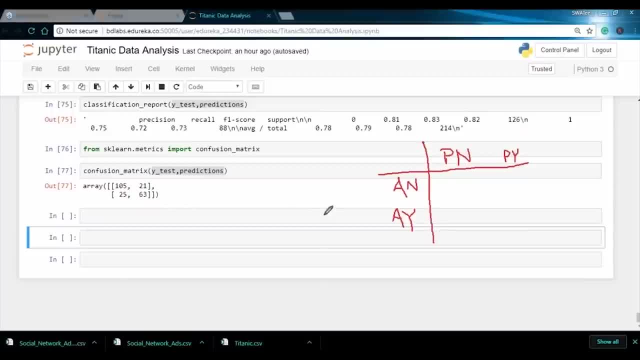 So here let me just feed in these values which we have just calculated. So here we have 105, 105,, 21,, 25 and 63.. So as you can see, here we have got four outcomes. Now 105 is the value. 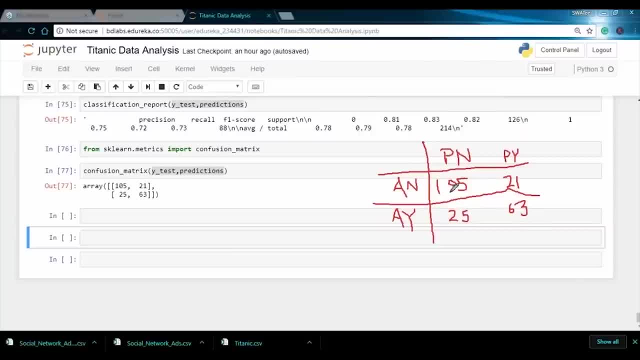 where our model has predicted no and in reality it was also a no. So here we have predicted no and an actual no. Similarly, we have 63 as a predicted yes. So here the model predicted yes and actually also it was a yes. So, in order to calculate, 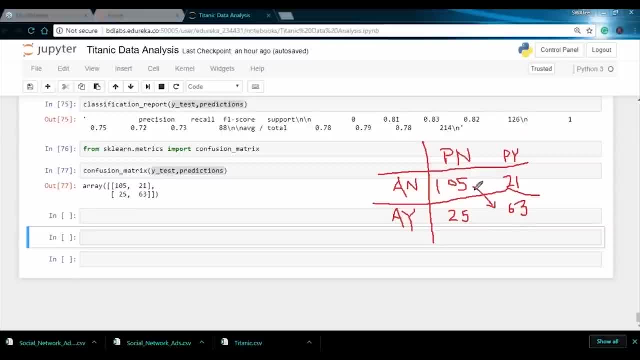 the accuracy. you just need to add the sum of these two values and divide the whole by the sum. So here these two values tells me where the model has actually predicted the correct output. So this value is also called as true negative. This is called 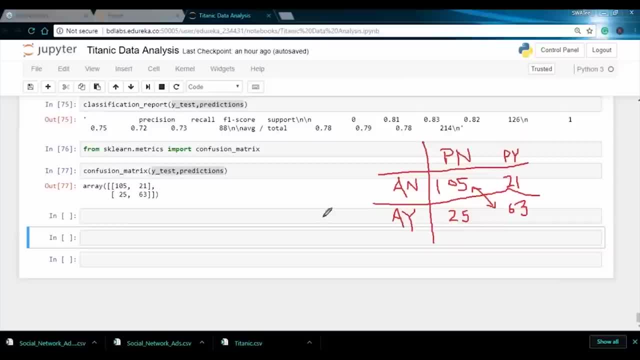 as false positive, This is called as true positive and this is called as false negative. Now, in order to calculate the accuracy. so in Python you can just import accuracy score function and you can get the results from that. So I'll just do that as well. 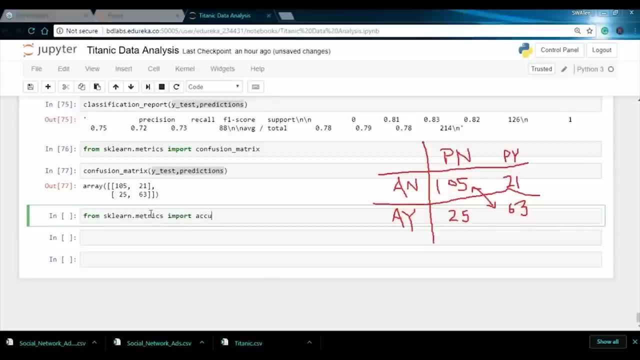 So I'll say from sklearnmetrics import accuracy score and I'll simply print the accuracy and I'll pass in the same variables, that is, ytest and predictions. So over here. it tells me the accuracy as 78, which is quite good. So over here. 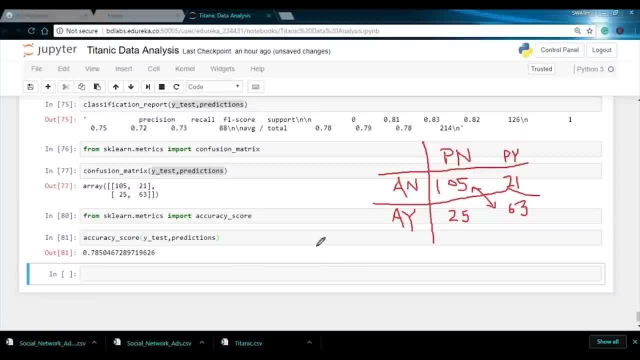 if you want to do it manually, you have to plus these two numbers, which is 105 plus 63. Almost 168, and then you have to divide it by the sum of all the four numbers, So 105 plus 63 plus 21, plus 25.. 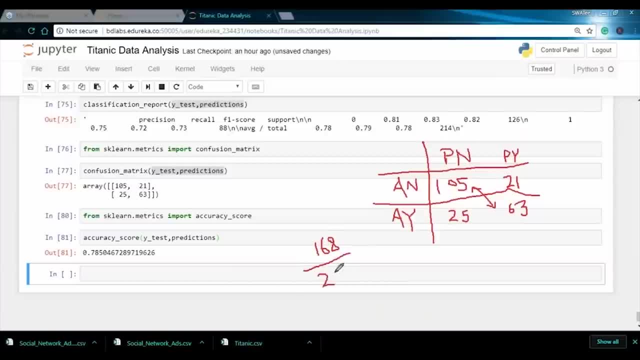 So this gives me a result of 214.. So now, if you divide these two number, you will get the same accuracy, that is 78%, or you can say 0.78.. So that is how you can calculate the accuracy. So now let me. 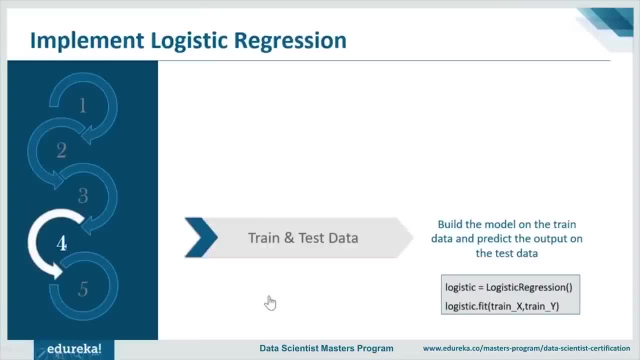 just go back to my presentation and let's see what all we have covered till now. So here we have first split our data into train and test subset And then predicted the output on the test data set, and then my fifth step is to check the accuracy. 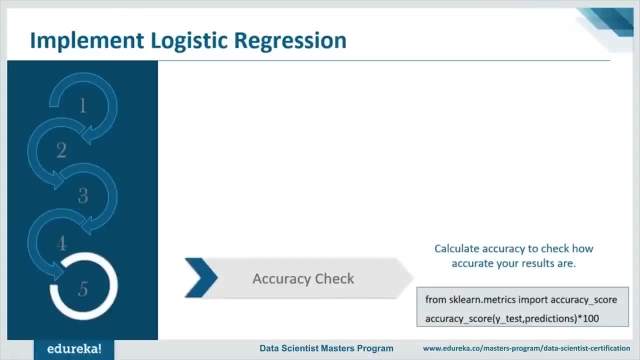 So here we have calculated accuracy to almost 78%, which is quite good. You cannot say that accuracy is bad. So here it tells me how accurate your results are. So here my accuracy score defines that, and hence we got a good accuracy. So now moving ahead. 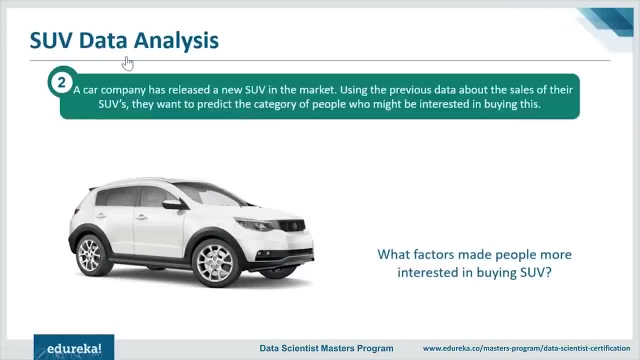 let us see the second project, that is, SUV data analysis. So in this, a car company has released new SUV in the market, and when they do this data about the sales of their SUV, they want to predict the category of people who might be interested in buying this. 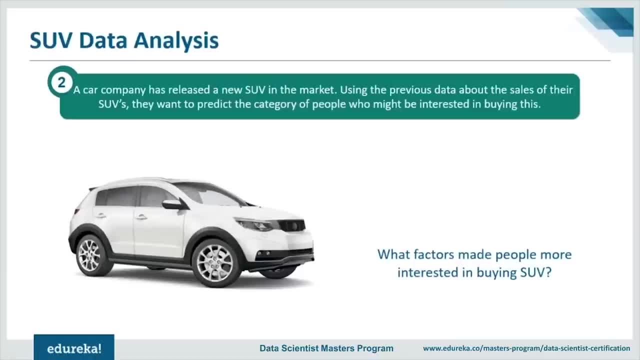 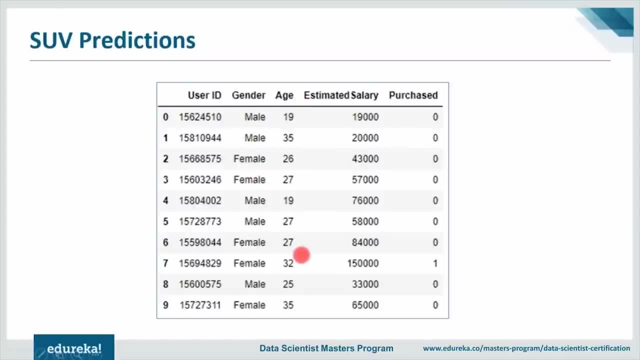 So, using the logistic regression, you need to find what factors made people more interested in buying this SUV. So for this, let us see a data set where I have user ID, I have gender as male and female, Then we have the age, we have the estimated. 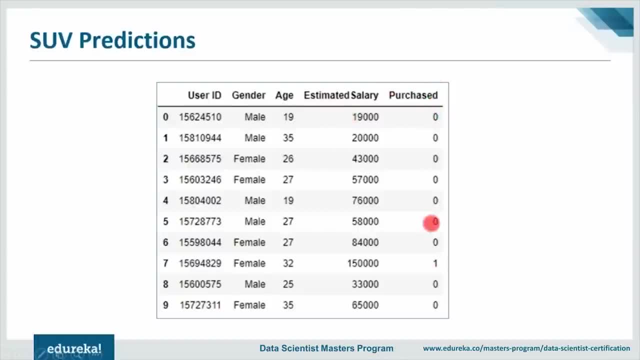 salary. and then we have the purchase column. So this is my discrete column, or you can say the categorical column. So here we just have the value that is used to predict whether a person can actually purchase a SUV or not. So, based on these factors, 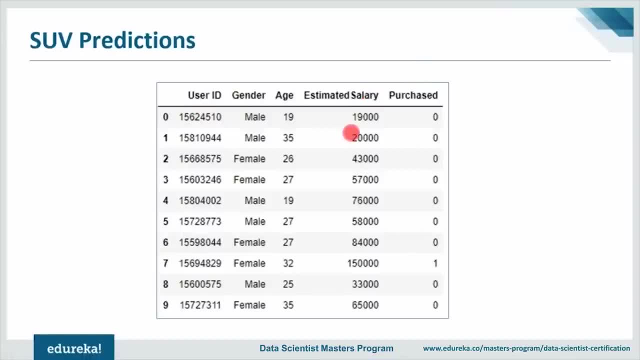 we will be deciding whether a person can actually purchase a SUV or not. So we know the salary of a person, we know the age and using these, we can predict whether a person can actually purchase a SUV or not. So let me just go to my Jupyter notebook. 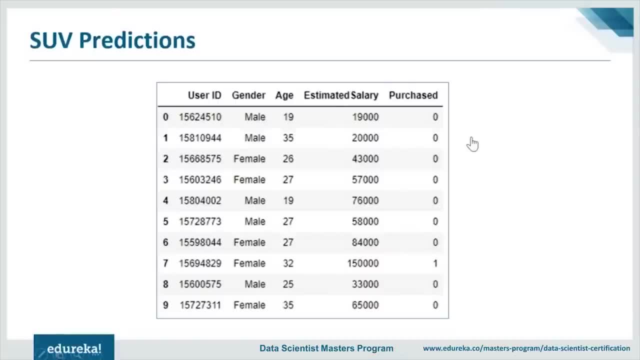 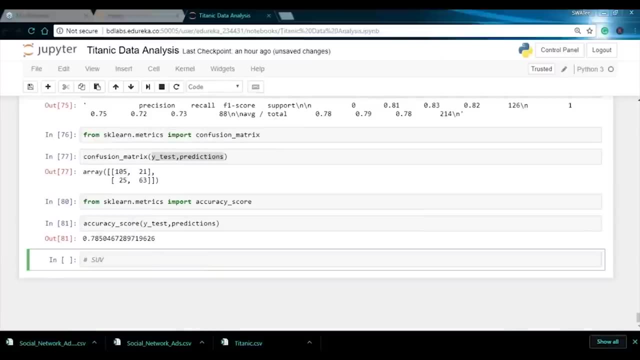 and let us implement logistic regression. So, guys, I will not be going through all the details of data cleaning and analyzing the part, So that part I'll just leave it on you. So just go ahead and practice as much as you can. The next project: 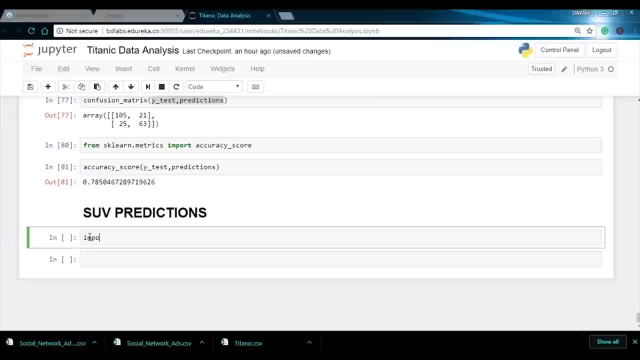 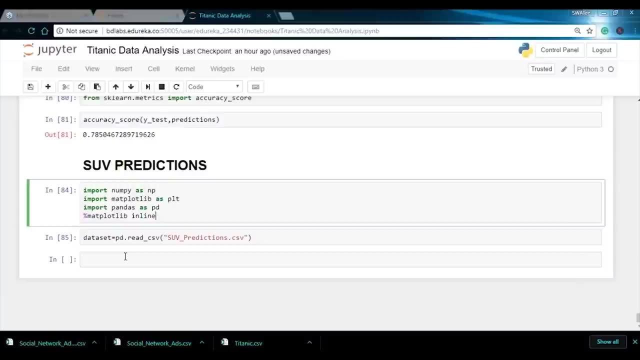 is SUV predictions, All right. So first of all I have to import all the libraries. So I say import numpy as np and similarly I'll do the rest of it. All right. So now let me just print the head of this data set. 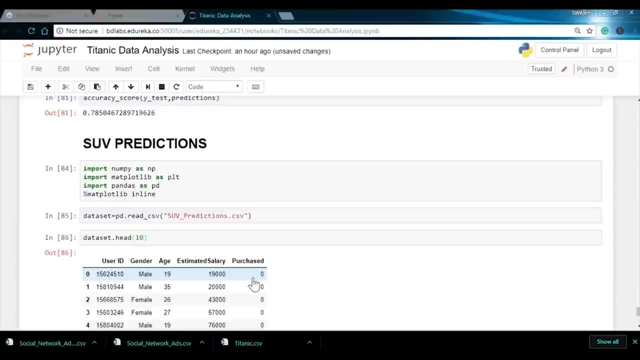 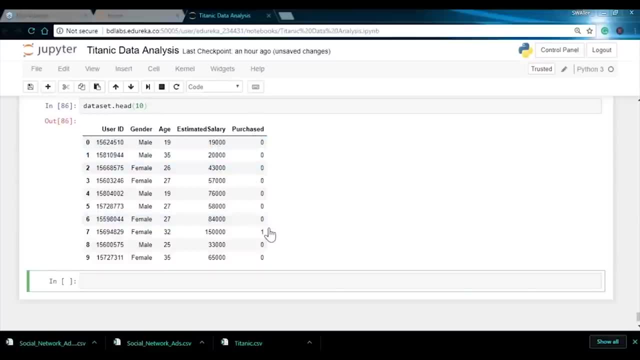 So this we've already seen- that we have columns as user ID, We have gender, we have the age, we have the salary and then we have to specify whether the person can actually purchase a SUV or not. So now it is just simply go on to the algorithm. 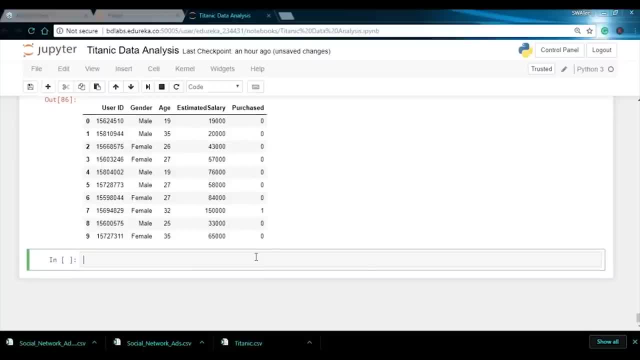 part, So we'll directly start off with the logistic regression or how you can train a model. So for doing all those things, we first need to define your independent variable and dependent variable. So in this case, I want my X. that is an independent variable. 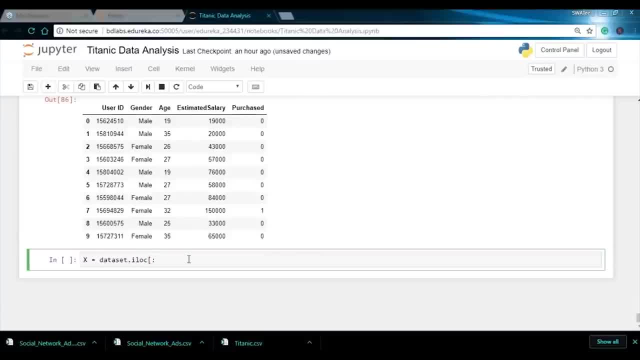 I said data set, dot I lock. So here I'll be specifying all the rows. So colon basically stands for that and in the columns I want only two and three dot values. So here should fetch me all the rows and only the second and third column. 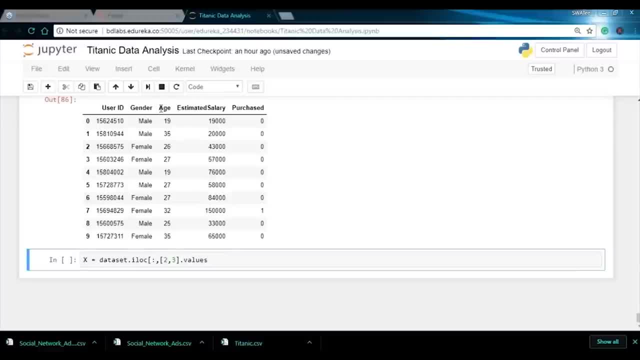 which is age and estimated salary. So these are the factors which will be used to predict the dependent variable that is purchase. So here my dependent variable is purchase and independent variable is of age and salary. So I'll say: data set, dot, I lock, I'll have all the rows. 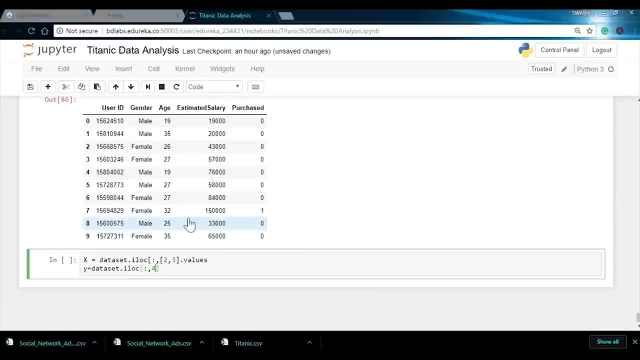 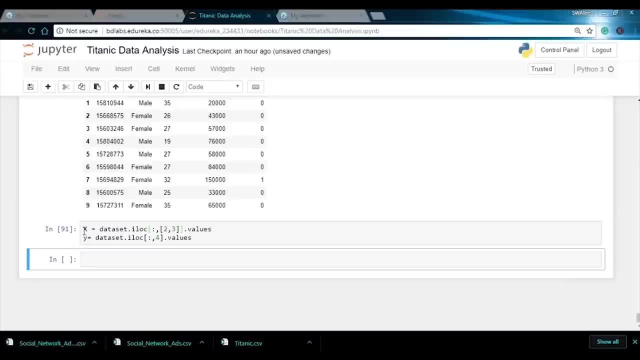 and I just want fourth column, that is, my purchased column, dot values. All right, So I've just forgot one one square bracket over here, All right, So over here I have defined my independent variable and dependent variable. So here my independent variable. 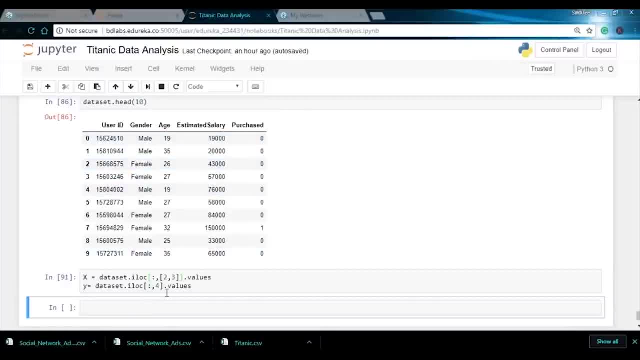 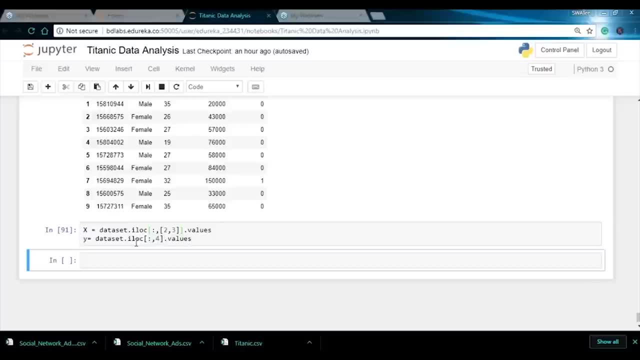 is age and salary, and dependent variable is the column purchase. Now you must be wondering: what is this? I lock function, So I love. function is basically an indexer for Pandas data frame and it is used for integer based indexing. I can also say: 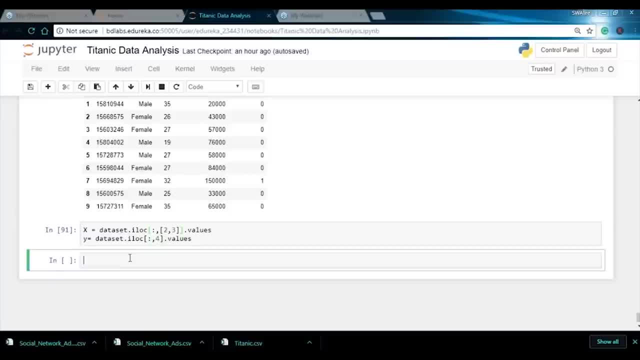 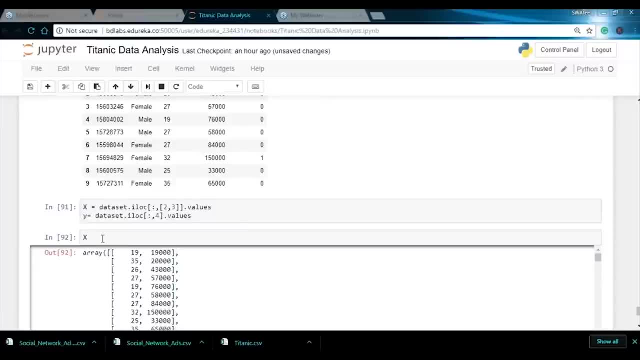 selection by index. Now let me just print these independent variables and dependent variable. So if I print the independent variable, I have the age as well as the salary. Next let me print the dependent variable over here, You can see, I just 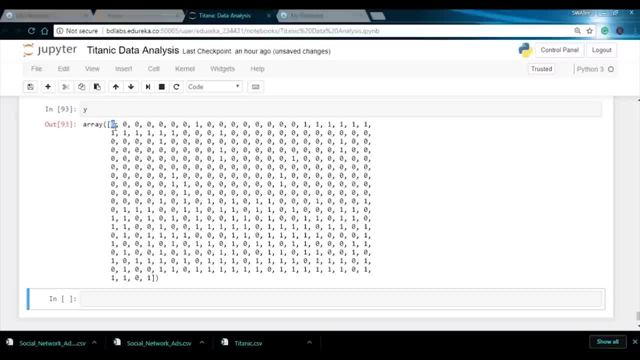 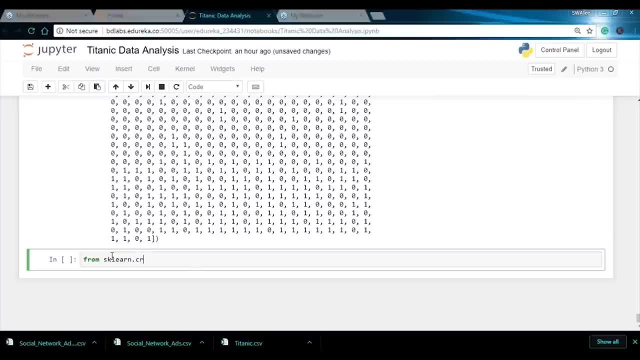 have the values in 0 and 1.. So 0 stands for did not purchase. next, Let me just divide my data set into training and test subset, So I'll simply write in from sklearn dot cross, split dot cross, validation, import train test. 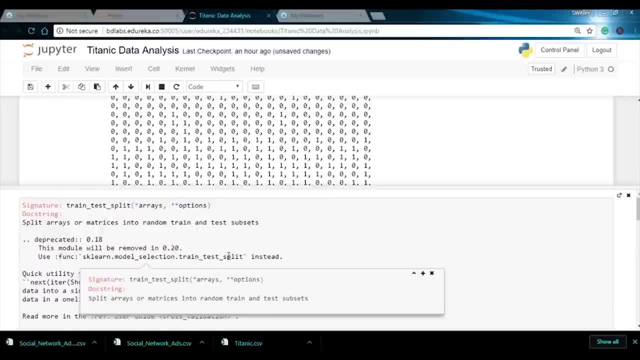 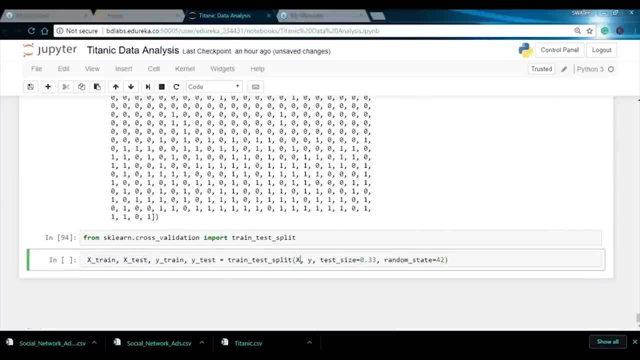 Next I just press shift and tab and over here I'll go to the examples and just copy the same line. So I'll just copy this and remove the points. Now I want the text size to be, let's say, 25.. 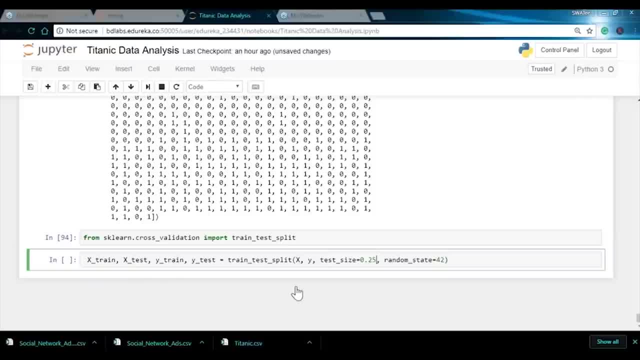 So I have divided the train and tested in 7525 ratio. Now let's say I'll take the random set as 0. So random state basically ensures the same result. or you can say the same samples taken whenever you run the code. 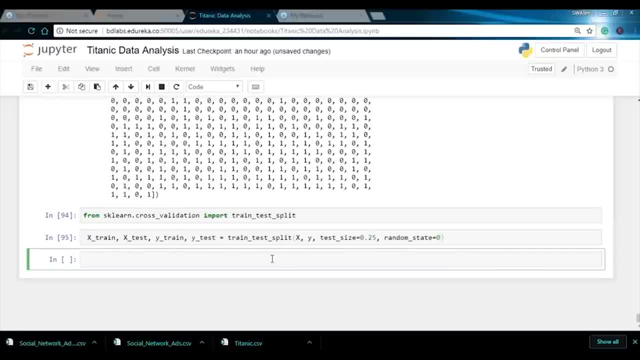 So let me just run this. Now you can also scale your input values for better performing, and this can be done using standard scalar, So let me do that as well. So I'll say: from sklearn dot pre-processing import standard scalar. Now. 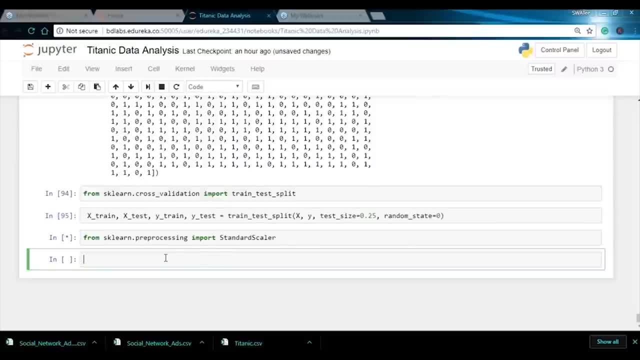 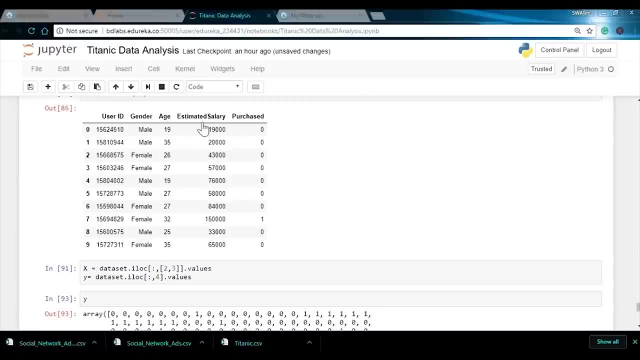 let's say, from sklearn dot pre-processing import standard scalar. Now, why do we scale it? Now, if you see our data set, we are dealing with large numbers, Well, although we are using a very small data set. So, whenever you're working, 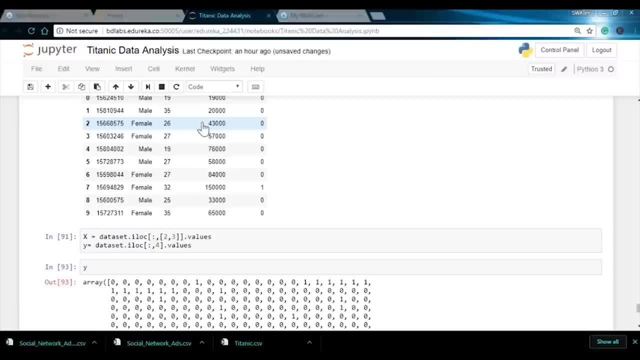 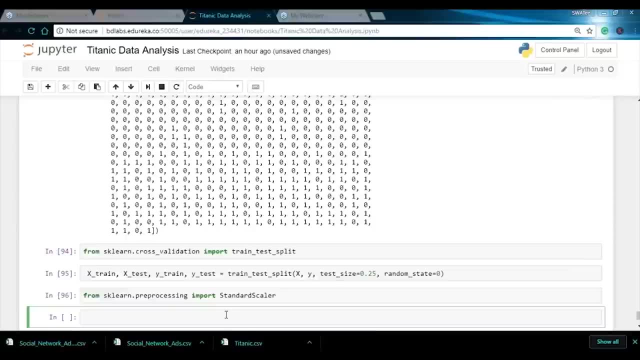 in a broad environment. you'll be working with large data set where you'll be using thousands and hundred thousands of tuples, So their scaling down will definitely affect the performance by a large extent. So here let me just show you how you can scale down. 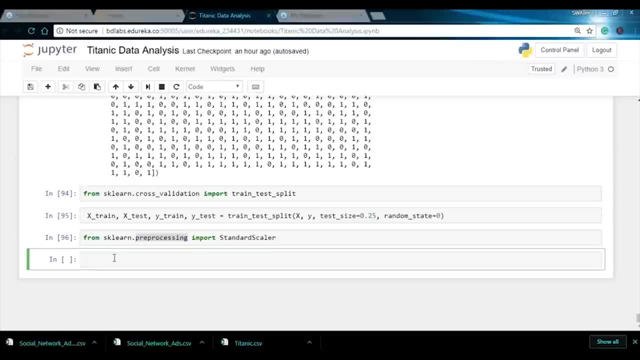 these input values and then the pre-processing contains all your methods and functionality to scale down for test, as well as a training data set. So I'll first make an instance of it. So I'll say standard scalar, then I'll have extreme. I'll say 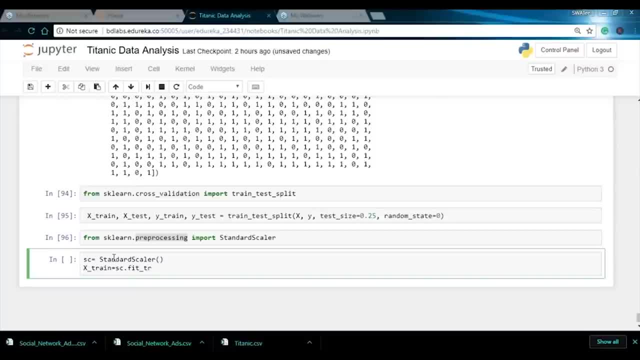 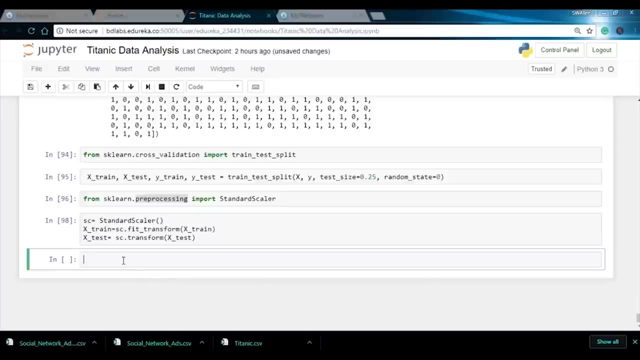 sc dot fit, fit, underscore transform, I'll pass in my extreme variable, And similarly I can do it for test, wherein I'll pass the X test. All right Now. my next step is to import logistic regression, So I'll simply apply logistic regression. 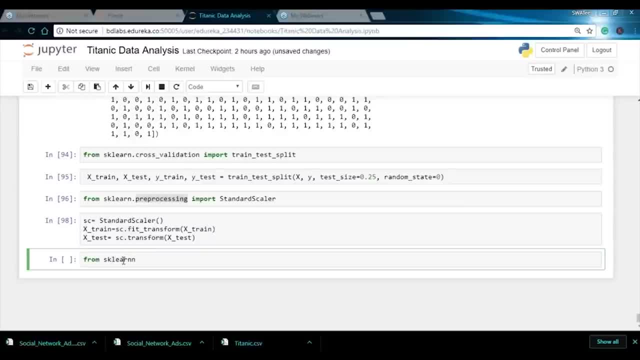 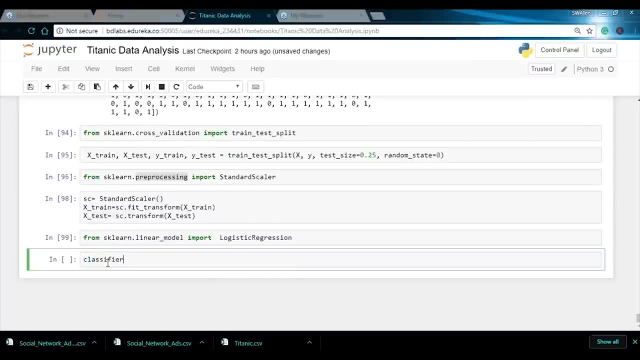 by first importing it. So I'll say: from sklearn, from sklearn dot. linear model import logistic regression. Over here I'll be using classifier, So I'll say: classifier dot is equals to logistic regression. So over here I'll just make an instance of it. 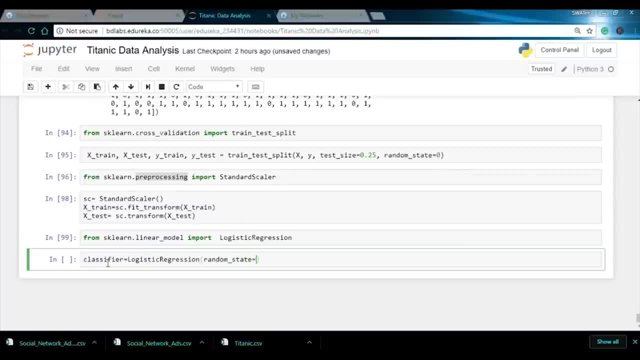 So I'll say logistic regression, and over here I'll just pass in the random state, which is zero, And now I'll simply fit the model and I'll simply pass in extreme and y-train. So here it tells me all the details. 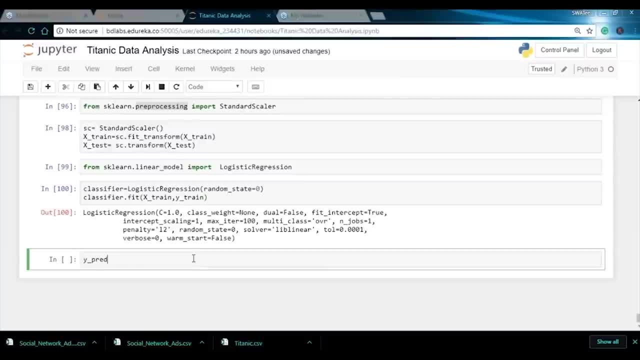 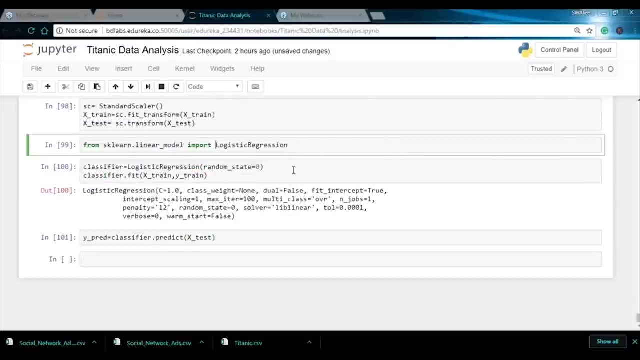 of logistic regression. Then I have to predict the value. So I'll say y-pred is equals to classifier, then predict function and then I just pass in X test. So now we have created the model, We have scaled down our input values. 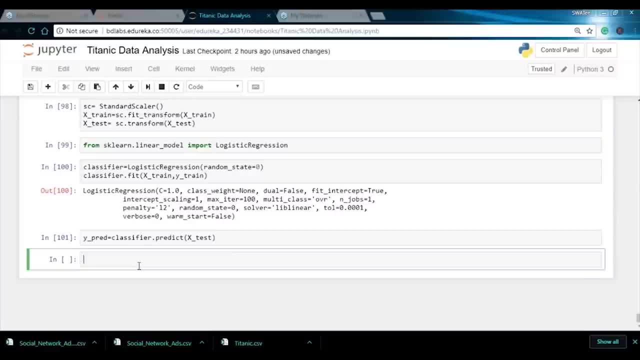 Then we have applied logistic regression, We have predicted the values and we want to know the accuracy. First we need to import accuracy scores. So I'll say, from sklearnmetrics, import accuracy score and using this function we can calculate the accuracy. or you can manually. 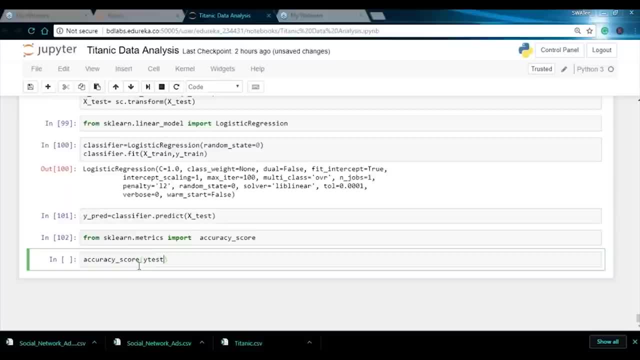 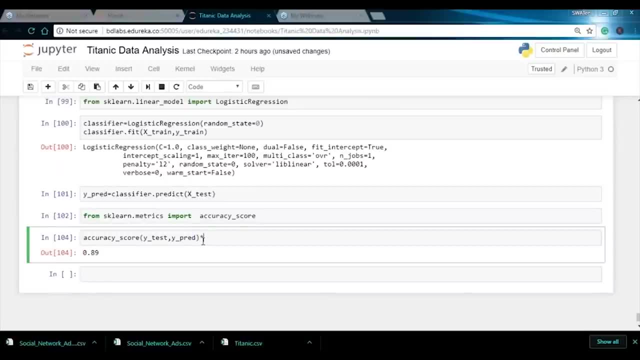 do that by creating a confusion matrix. So I'll just pass in my y-test and my y-predicted, All right, So over here I get the accuracy as 89%. So we want to know the accuracy in percentage. So I just have. 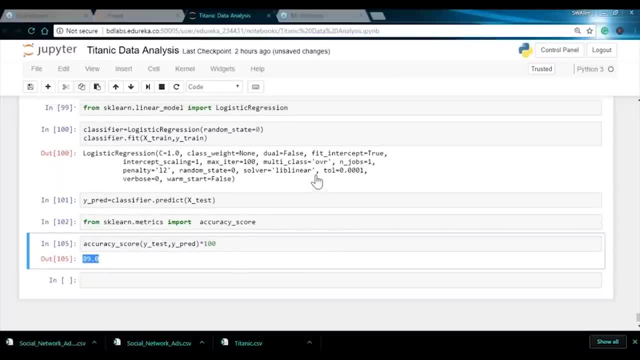 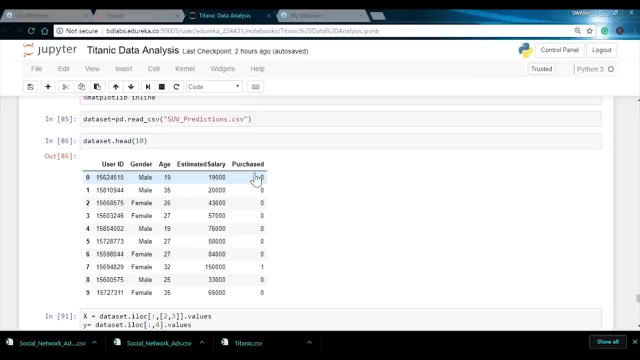 to multiply it by 100 to 99%. So I hope you guys are clear with whatever I have taught you today. So here I have taken my independent variables as age and salary, and then we have calculated that how many people can purchase the SUV, and then we have 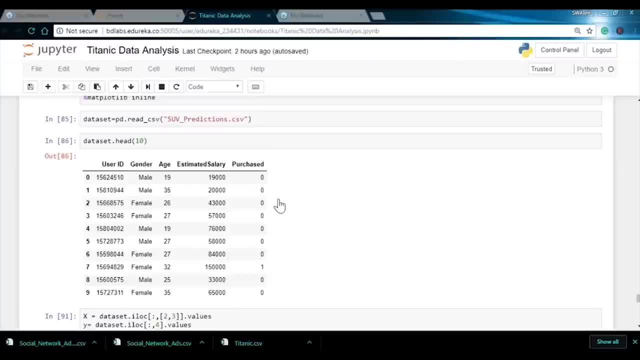 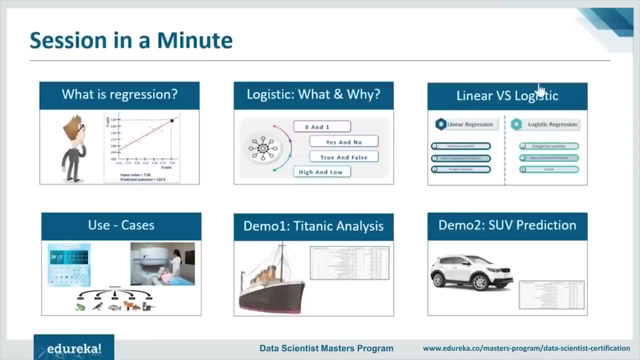 calculated our model by checking the accuracy. So over here we get the accuracy as 89, which is great. All right, guys, that is it for today, So I'll just discuss what all we have covered in today's training. First of all, 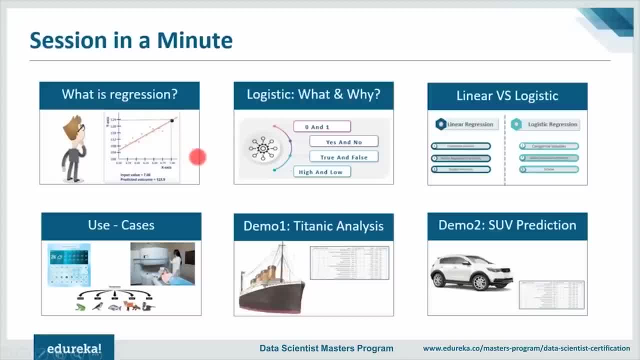 we had a quick introduction to what is regression and where regression is actually used. Then we have understood and got into the details of what and why of logistic regression. I've compared linear versus logistic regression. We have also seen the various use cases where you can implement. 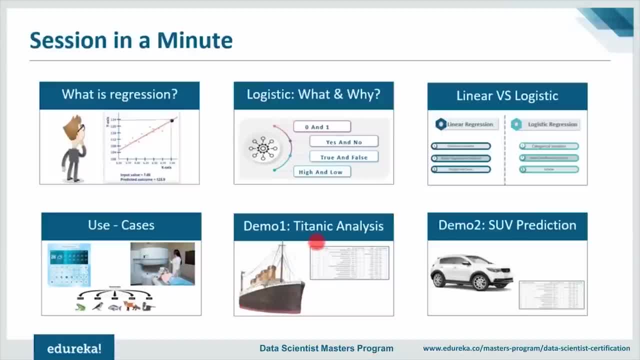 logistic regression in real life. and then we have picked up two projects, that is, titanic data analysis and SUV prediction. So over here we have seen how you can collect your data, analyze your data, then perform modeling on that data, train the data. 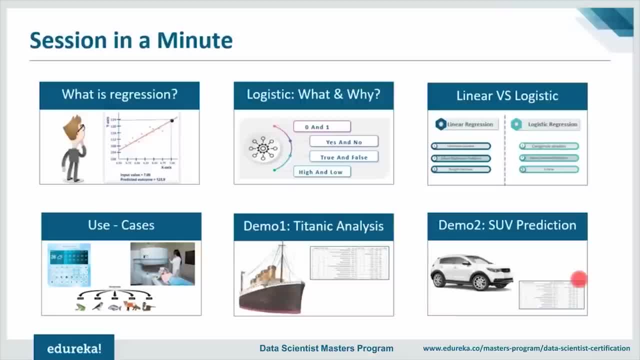 test the data and then finally, you have calculated the accuracy. So in your SUV prediction you can actually analyze, clean your data and you can do a lot of things. So you can just go ahead, pick up any data set and explore it as much as you can. 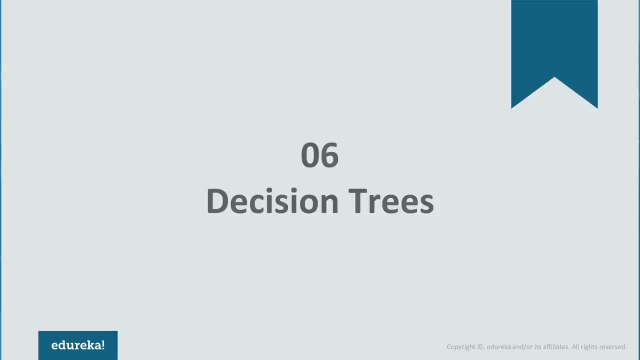 Open your eyes and see around, You will find dozens of applications of machine learning which you are using and interacting with in your daily life. Be it be using the face detection algorithm in Facebook or getting the recommendation for similar products from Amazon, Machine learning is applied almost everywhere. 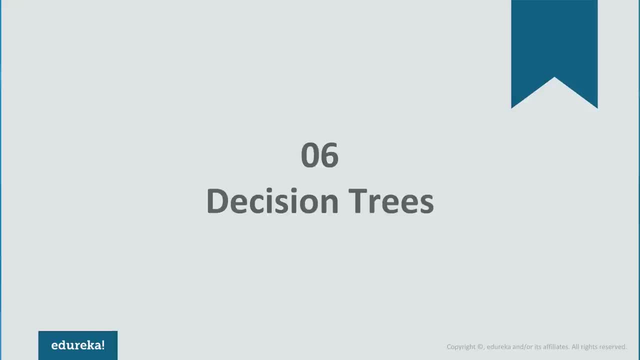 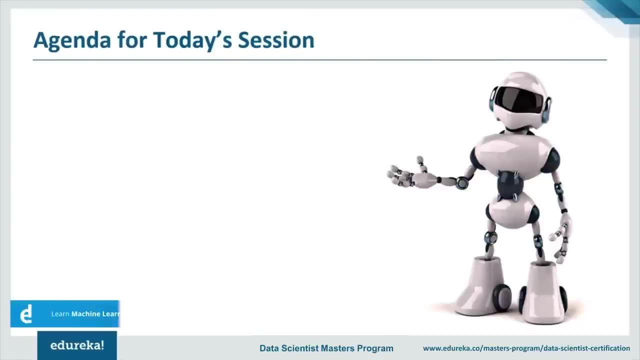 So hello and welcome all to this YouTube session. Today we will learn about how to build a decision tree. This session is designed in a way that you get most out of it, Alright, so this decision tree is a type of classification algorithm which comes under: 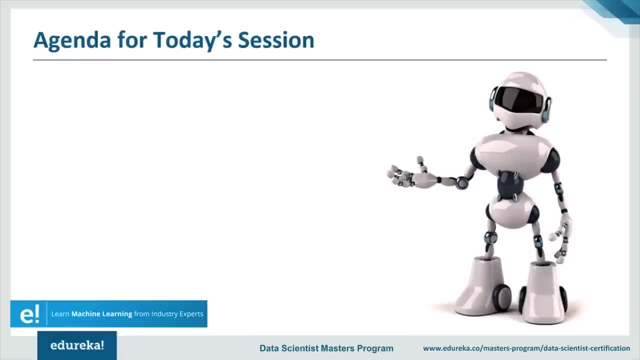 the supervised learning technique. So, before learning about decision tree, I'll give you a short introduction to classification, where we'll learn about what is classification, what are its various types, where it is used or what are its use cases. Now, once you get, 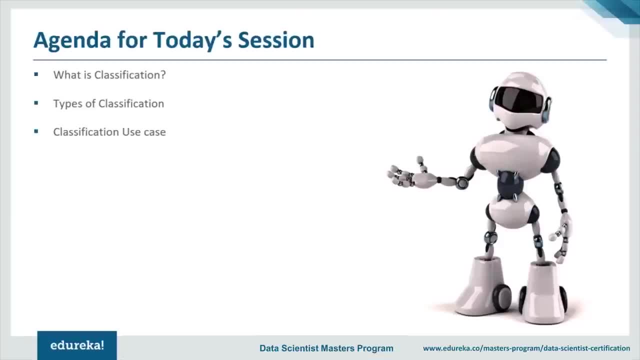 your fundamental clear, we'll jump to the decision tree part Under this. first of all, you mathematically create a decision tree from scratch. Then, once you get your concepts clear, we'll see how you can write a decision tree classifier from scratch. 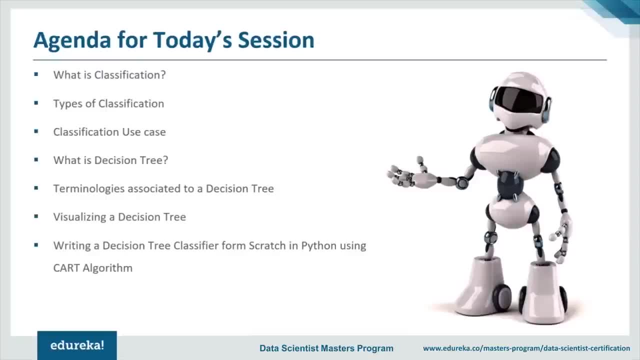 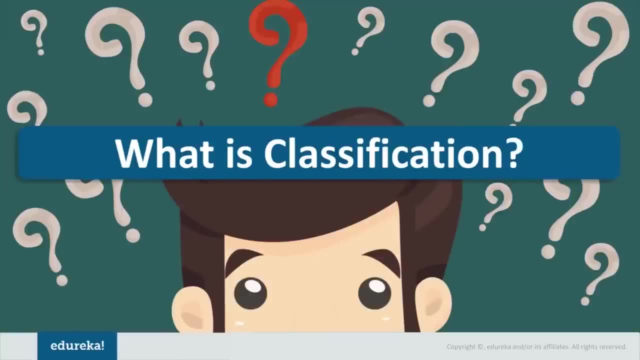 in Python using the cart algorithm. Alright, I hope the agenda is clear to you guys. What is classification? I hope every one of you must have used Gmail, So how do you think the mail is getting classified: as a spam or not a spam mail? 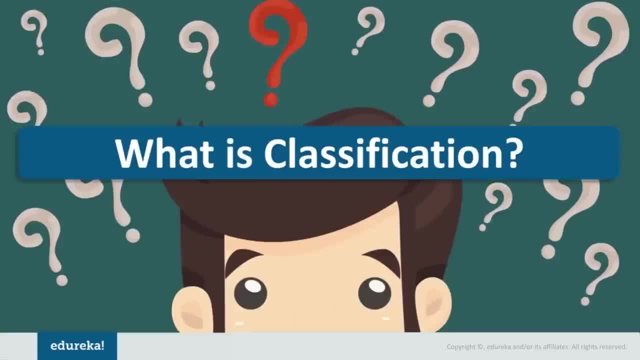 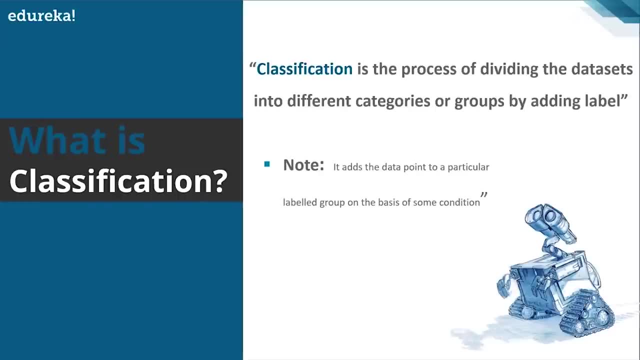 Well, there's nothing but classification. So what it is? Well, classification is a process of adding different categories or groups by adding label. In other way, you can say that it is a technique of categorizing the observation into different category. So basically, 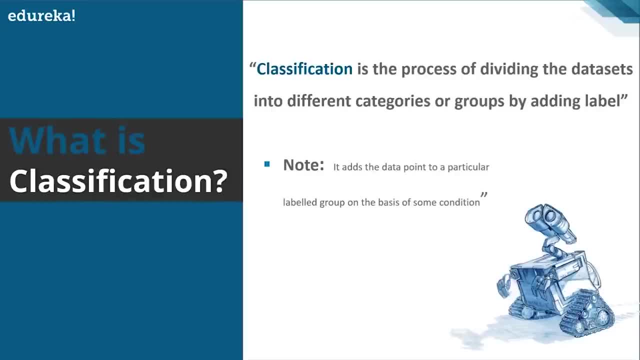 what you're doing is you're taking the data, analyzing it and, on the basis of some condition, you finally divide into various categories. Now why do we classify it? Well, we classify it to perform predictive analysis on it, Like when you get the mail. 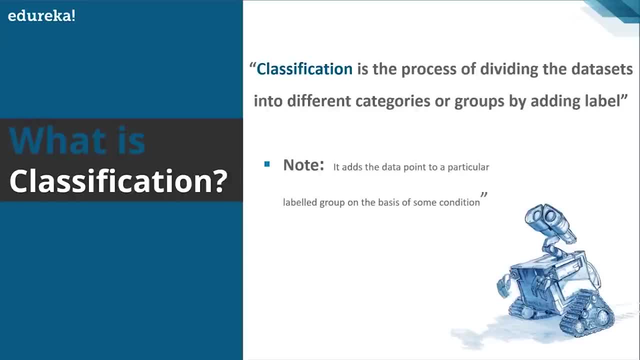 the machine predicts it to be a spam or not a spam mail And on the basis of that prediction, it will send a spam mail to the respective folder. In general, this classification algorithm handle questions like: is this data belongs to A category or B category? 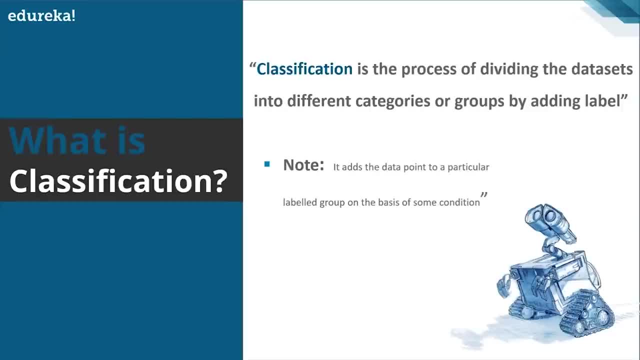 Like: is this a male or is this a female? Something like that. Now the question arises: where will you use it? Well, you can use this for fraud detection or to check whether the transaction is genuine or not. Suppose I'm using 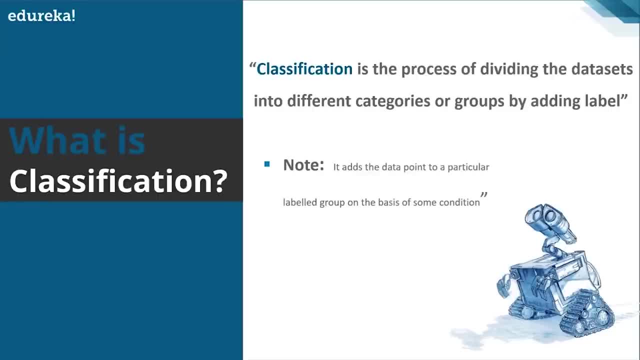 a credit card here in India. Now, due to some reason, I had to fly to Dubai. Now, if I'm using the credit card over there, it will send a notification alert regarding my transaction. They would ask me to confirm about the transaction. 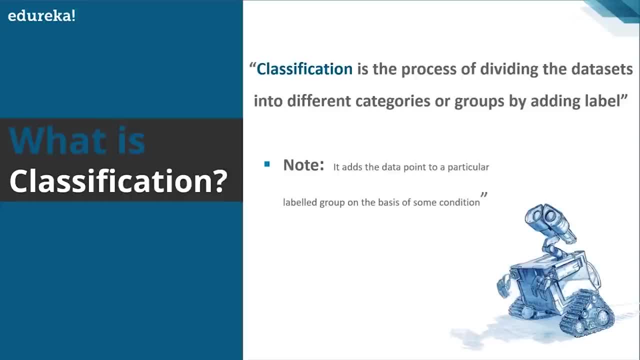 So there's also kind of predictive analysis, as the machine predicts that something fishy is in the transaction, as 24 hour ago I made the transaction using the same credit card in India And 24 hour later, the same credit card is being used. 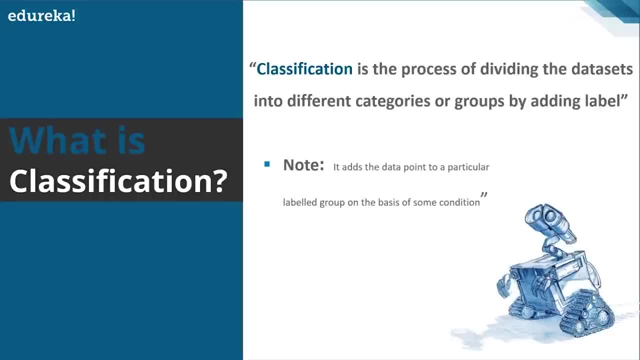 for the payment in Dubai. So the machine predicts that something fishy is going on in the transaction. So, in order to confirm it, it sends you a notification alert. Well, this is one of the use case of classification. You can even use it. 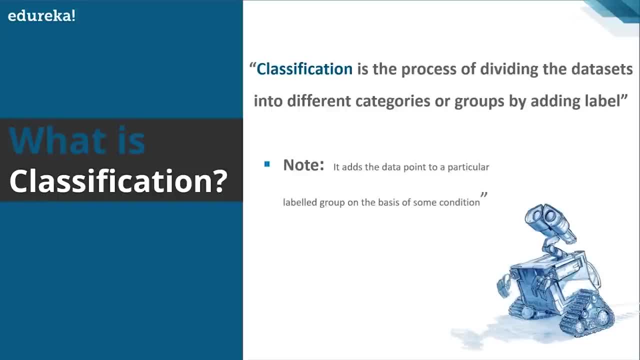 to classify different items, like fruits, on the basis of its taste, color, size or weight. A machine well trained, using the classification algorithm can easily predict the class or the type of fruit whenever new data is given to it. Not just the fruit, it can be any item. 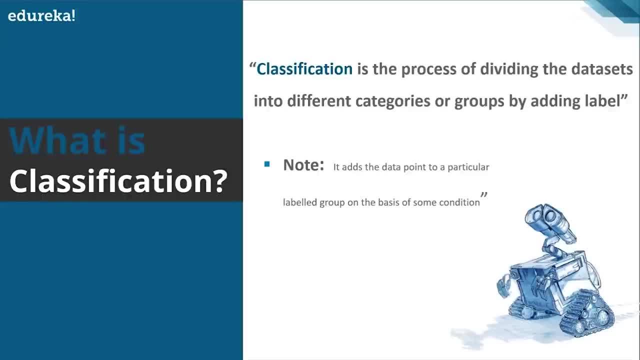 It can be a car, it can be a house, it can be a sign board or anything. Have you noticed that while you visit some sites or you try to login into some, you get a picture capture for that right Where you have to identify? 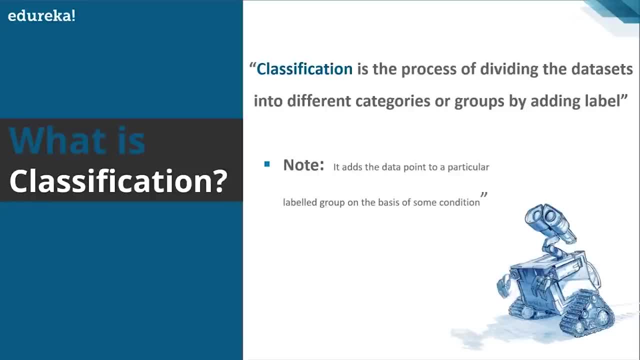 whether the given image is of a car or it's of a pole or not, You have to select it. For example, there are 10 images and you're selecting three images out of it. So in a way, you're training the machine. 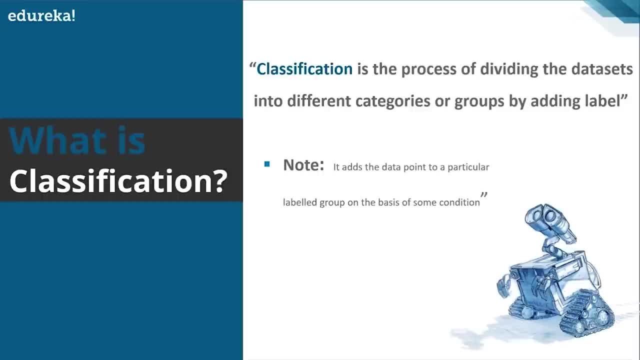 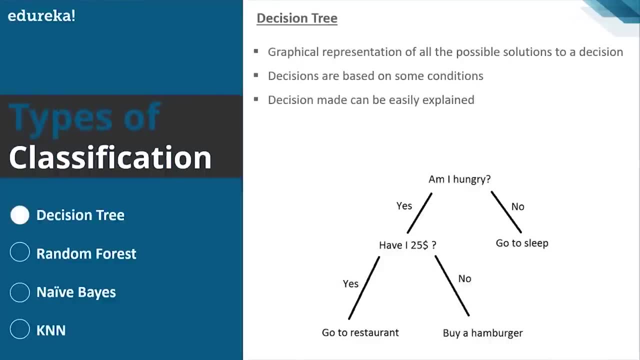 right. You're telling that these three are the picture of a car and rest are not. So who knows? you're training it for something big, right? So, moving on ahead, let's discuss the types of classification, All right. 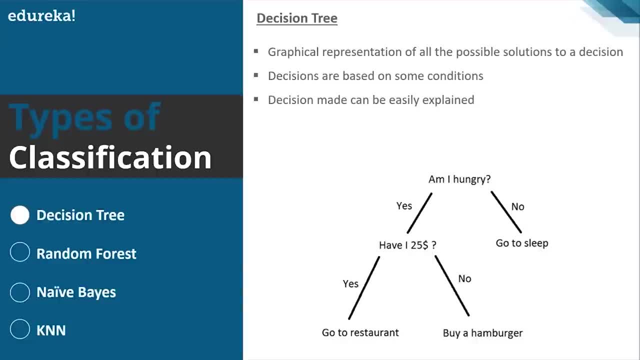 So, whether a given person is a male or a female, the machine had to be trained first. all right, But there are multiple ways to train the machine and you can choose any one of them. Just for predictive analytics, there are many different techniques. 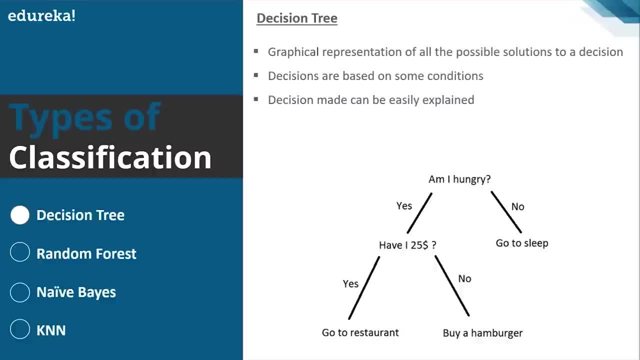 but the most common of them all is the decision tree, which we'll cover in depth in today's session. So as a part of classification algorithm, we have decision tree: random forest neighbors, k nearest neighbor. logistic regression, linear regression. 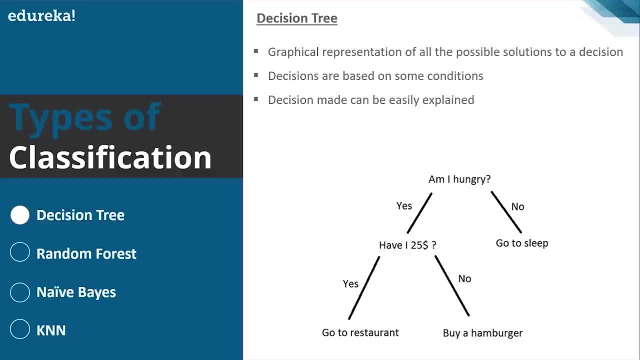 support vector machines and so on. There are many. Let's take a look at a few of them, Starting with decision tree. A decision tree is a graphical representation of all the possible solution to a decision, The decisions which are made. they can be explained. 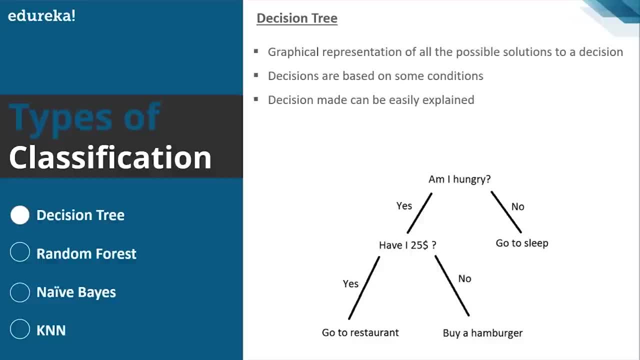 very easily. For example, here is a task which says that: should I go to a restaurant or should I buy a hamburger? You're confused on that, So for that, what you'll do? you'll create a decision tree for it. 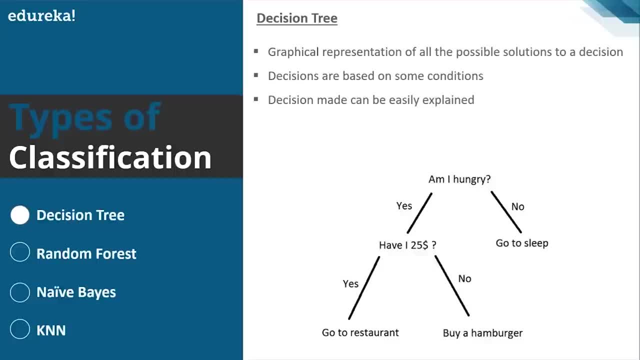 Starting with the root node will be: first of all, you'll check whether you're hungry or not. All right, If you're hungry and you have $25, then you'll decide to go to restaurant. And if you're hungry and you don't have $25,. 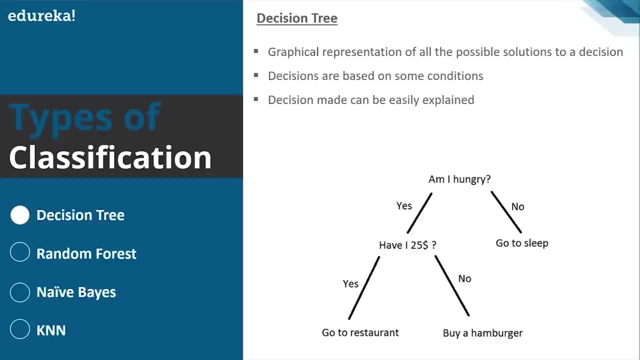 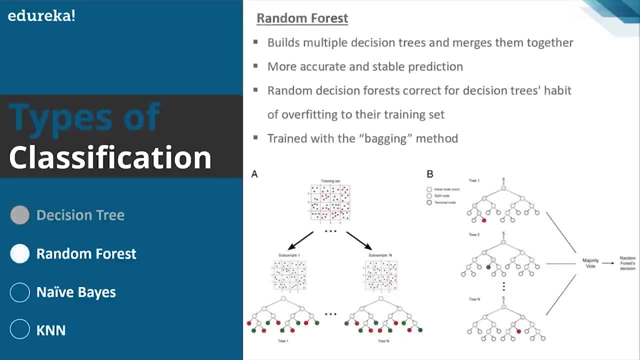 then you'll just go and buy a hamburger, That's it All right. So this is about decision tree. Now, moving on ahead, let's see what is a random forest. Well, random forest build multiple decision trees and merges them together. 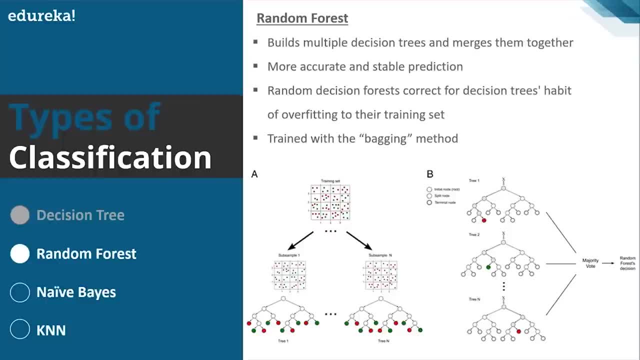 to get a more accurate and stable prediction. All right. Most of the time, random forest is trained with a bagging method. The bagging method is based on the idea that the combination of learning model increases the overall result. If you're combining. 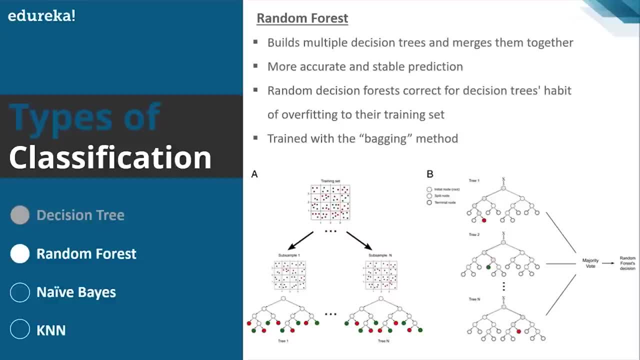 the learning from different models and then clubbing it together. what it will do? it will increase the overall result, Fine. Just one more thing: If the size of your data set is huge, then in that case one single decision tree would lead. 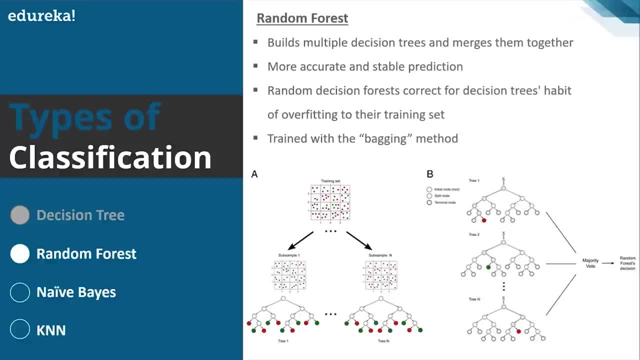 to an overfit model. Same way, like a single person might have its own perspective on the complete population, as the population is very huge, Right. However, if we implement the voting system and ask different individual to interpret the data, then we would be able. 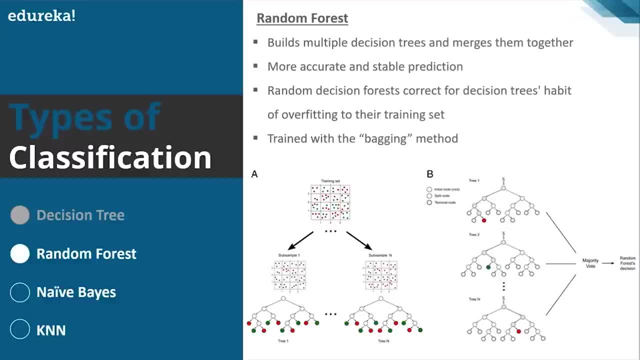 to cover the pattern in a much meticulous way. Even from the diagram you can see that in section A we have a large training data set. What we do? we first divide our training data set into N subsamples, All right, And we create a decision tree. 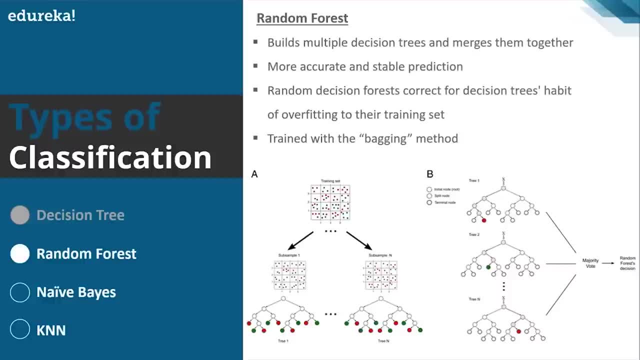 for each subsample. Now, in the B part, what we do? we take the vote out of every decision made by every decision tree And finally, we club the vote to get the random forest decision. Finally, we take the vote to get the random forest decision. 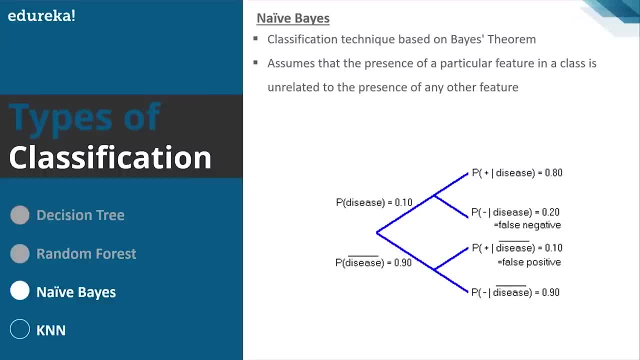 Is that fine? Let's move on ahead. Next we have name bias. So name bias is a classification technique which is based on Bayes theorem. It assumes that presence of any particular feature in a class is completely unrelated to the presence of any other feature. 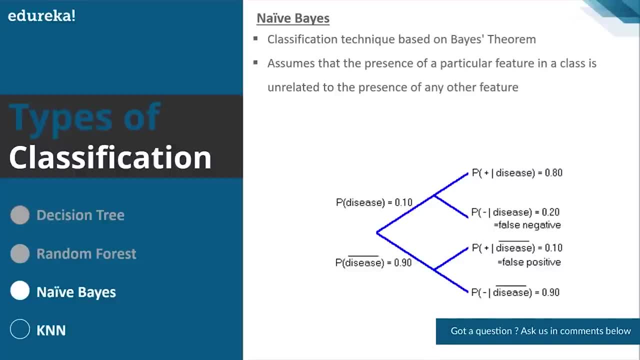 Name bias is simple and easy to implement algorithm And due to its simplicity, this algorithm might outperform more complex model when the size of the data set is not large enough. All right, A classical use case of name bias is a document classification. 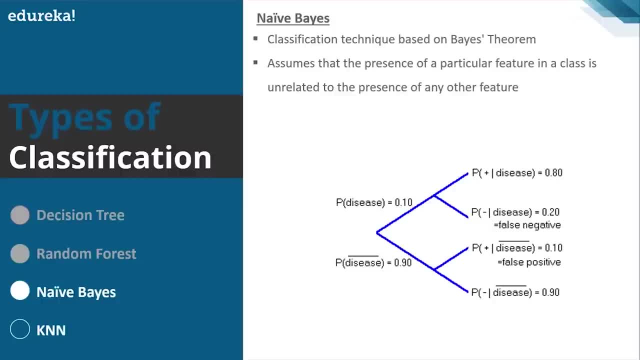 In that what you do? you determine whether a given text corresponds to one or more categories. In the text case, the features used might be the presence or absence of any keyword. So this was about name. From the diagram you can see that. 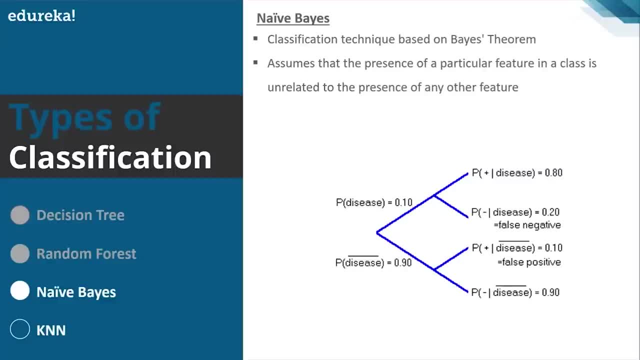 using name bias. we have to decide whether we have a disease or not. First, what we do, we check the probability of having a disease and not having the disease right. Probability of having a disease is 0.1. And probability 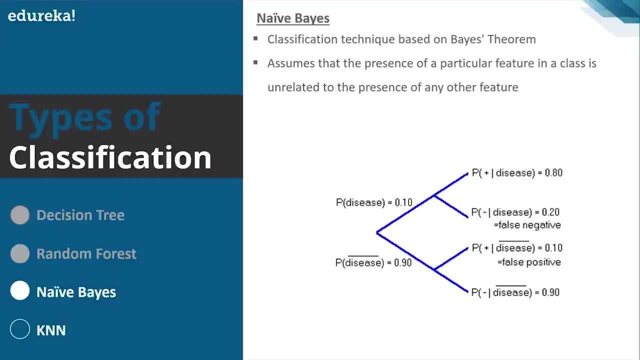 of not having a disease is 0.9.. Okay, First let's see when we have disease and we go to doctor. All right, So when you visited the doctor and the test is positive, so probability of having a positive test when you're having a disease. 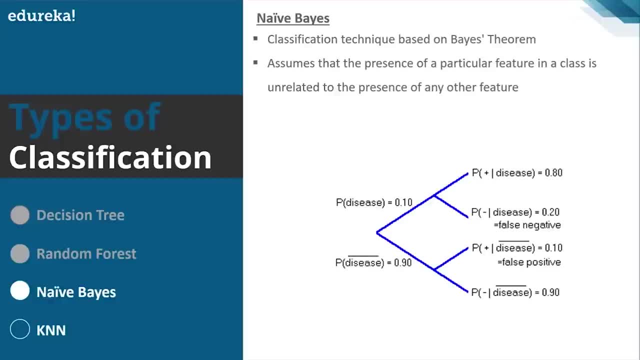 is 0.80 and probability of a negative test when you already have a disease that is 0.20.. This is also a false negative statement as the test is detecting negative but you still have the disease right. So it's a false negative statement. 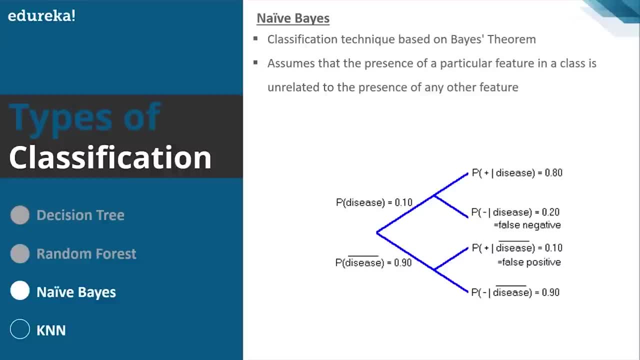 Now let's move ahead when you don't have the disease at all. So probability of not having a disease is 0.9.. And when you visit the doctor and the doctor is like, yes, you have the disease, but you already know. 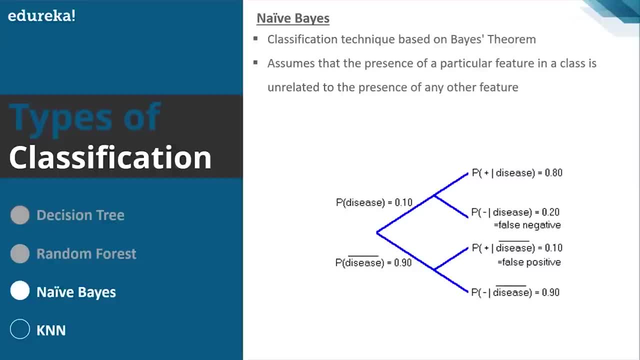 that you don't have the disease. So it's a false positive statement. So probability of having a disease when you actually know there is no disease is 0.1, and probability of not having a disease when you actually know there is no disease. 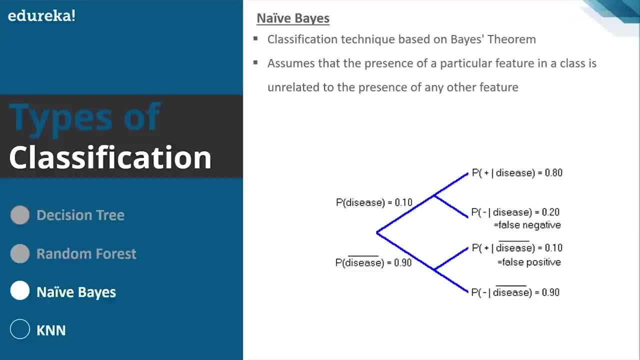 So and the probability of not having a disease is 0.90.. Fine, It is same, as probability of not having a disease in the test is showing the same result, the true positive statement. So it is 0.9.. All right. 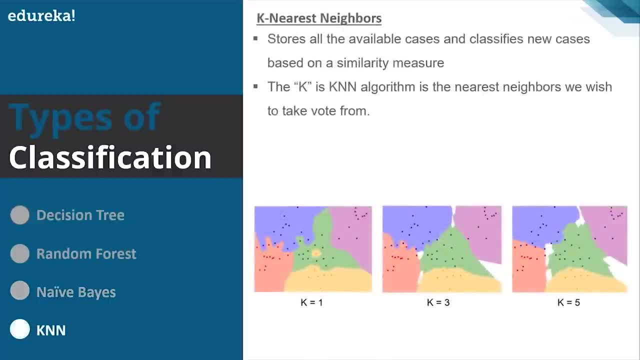 So let's move on ahead and discuss about K and N algorithm. So this K and N algorithm, or the K nearest neighbor, it stores all the available cases and classifies new cases based on this similarity measure, The K in the K and N algorithm. 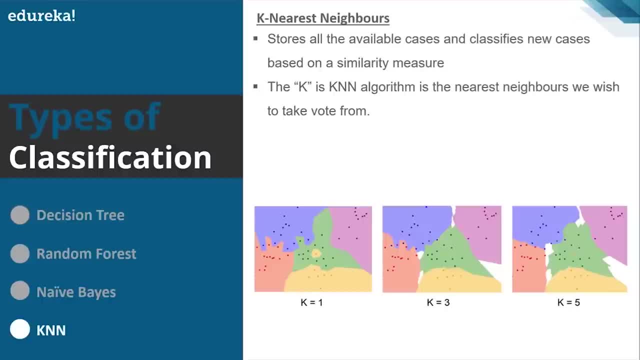 is the nearest neighbor we wish to take vote from. For example, if K equal one, then the object is simply assigned to the class of that single nearest neighbor. From the diagram you can see the difference in the image when K equal one. 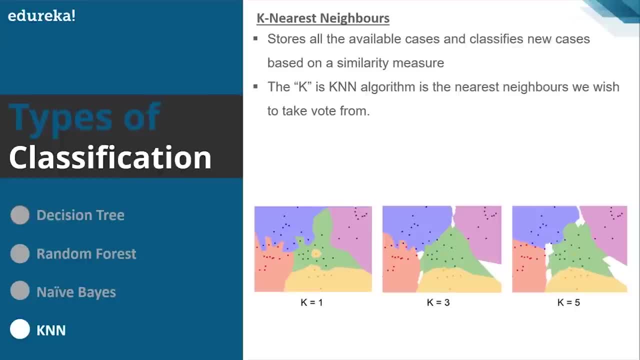 K equal three and K equal five Right. Well, the modern systems are now able to use the K nearest neighbor for visual pattern recognition to scan and detect hidden packages in the bottom bin of a shopping cart. at the checkout, If an object is detected, 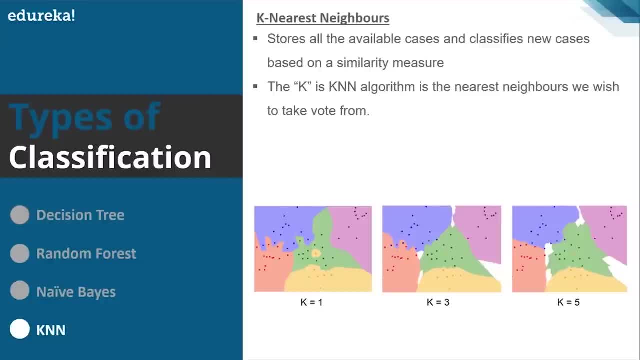 which matches exactly to the object in the shopping cart. then the object is automatically added to the customer's bill, While this automated billing practice is not used extensively at this time, but the technology has been developed and is available for use If you want. 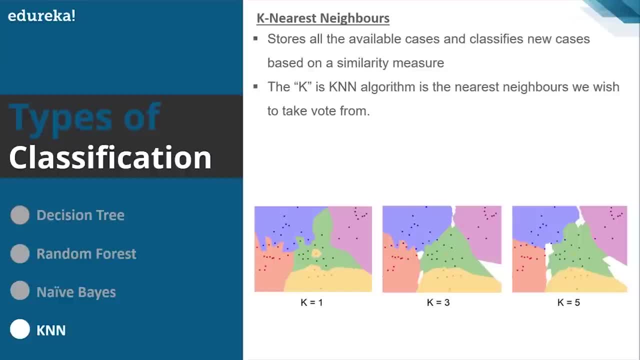 you can just use it. And yeah, one more thing: K nearest neighbor is also used in retail to detect patterns in the credit card users. Many new transactions scrutinizing software application use K and N algorithms to analyze registered data and spot unusual pattern that indicates. 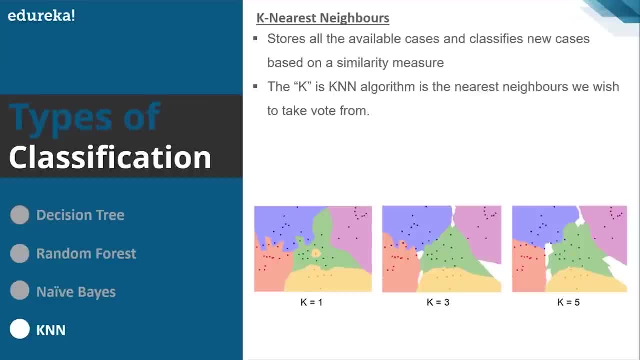 suspicious activity. For example, if registered data indicates that a lot of customers' information is being entered manually rather than through automated scanning and swapping, then in that case this could indicate that the employees who are using the register are in fact stealing customers'. 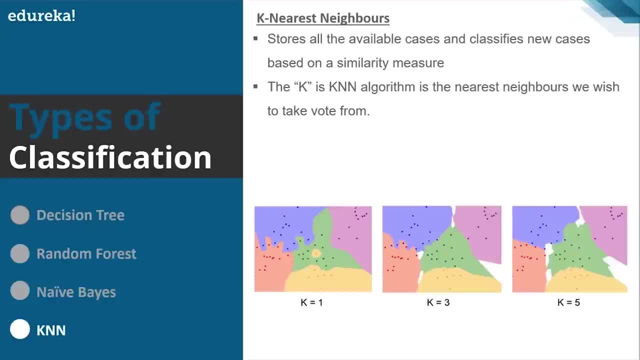 personal information, Or if a registered data indicates that a particular good is being returned or exchanged multiple times, this could indicate that employees are misusing the return policy to take returns right. So this was about K and N algorithm, since our main focus for this session. 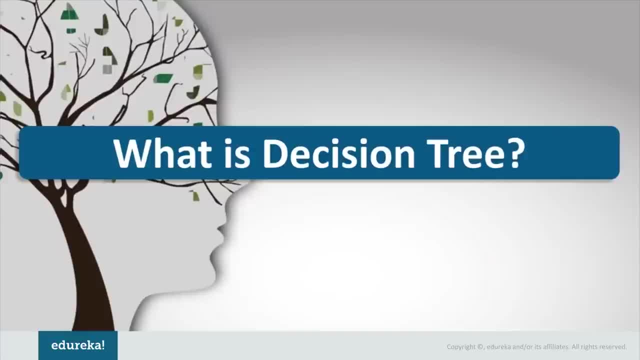 will be on decision tree. So, starting with, what is decision tree? but first let me tell you why do we choose decision tree to start with. Well, these decision tree are really very easy to read and understand. It belongs to one of the few models. 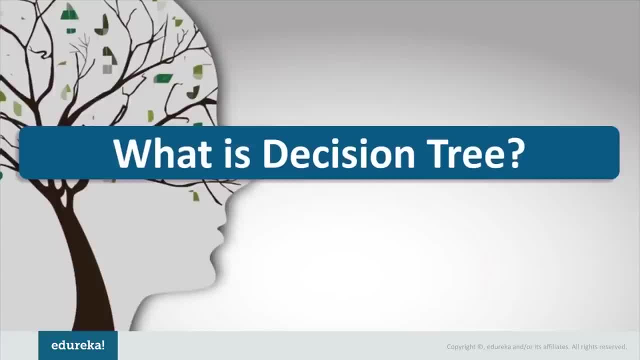 that are interpretable, where you can understand exactly why the classifier has made that particular decision right. Let me tell you a fact: that for a given data set, this algorithm performs better than that. It's like you cannot say that decision tree is better. 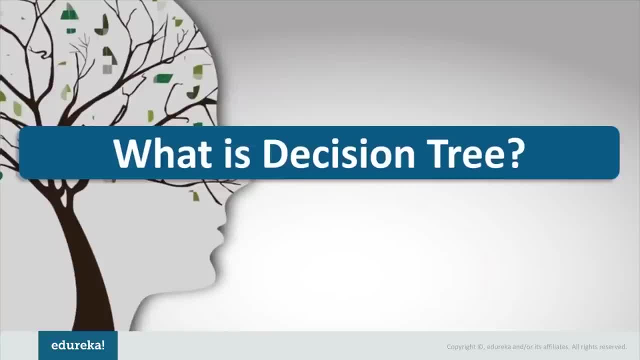 than name bias, or name bias is performing better than decision tree. It depends on the data set right. You have to apply hidden trial method with all the algorithms one by one and then compare the result. The model which gives the best result is the model. 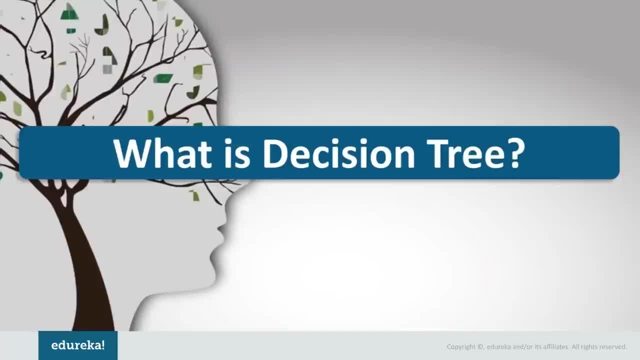 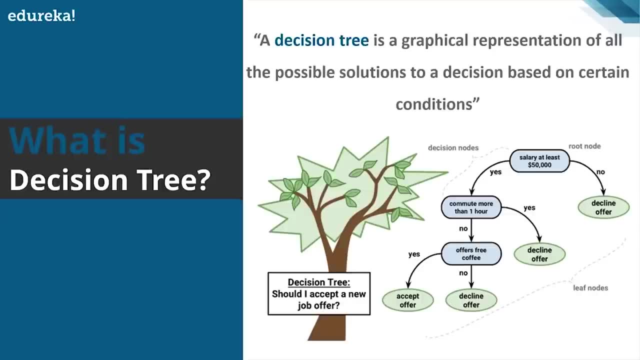 which you can use it for better accuracy for your data set. All right, So let's start with. what is decision tree? Well, a decision tree is a graphical representation of all the possible solution or decision based on certain conditions. Now you might be wondering: 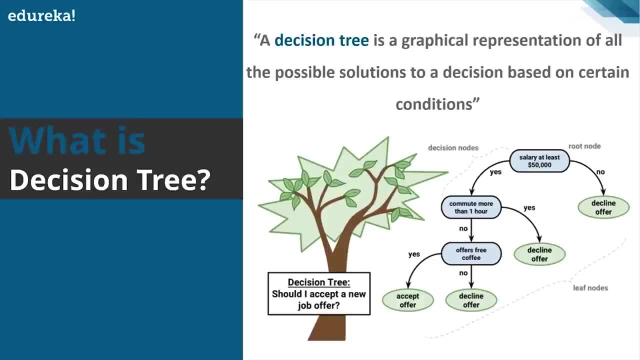 why this thing is called as decision tree. Well, it is called so because it starts with a root and then branches off to a number of solution, just like a tree, right? Even the tree starts from a root and it starts growing its branches once it gets bigger. 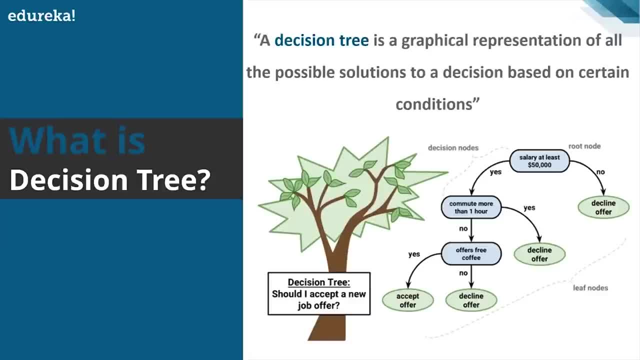 and bigger. Similarly, in a decision tree, it has a root which keeps on growing with increasing number of decision and the conditions. Now you might be wondering why this is called a decision tree, but most of you must have used it, Remember. 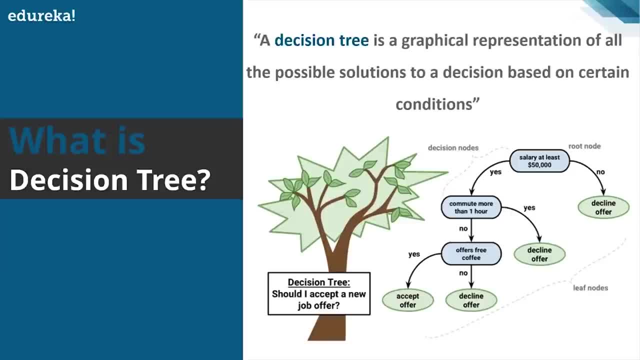 whenever you dial the toll-free number of your credit card company, it redirects you to his intelligent computerized assistant, where it asks you questions like press 1 for English or press 2 for Hindi, press 3 for this, press 4 for that. 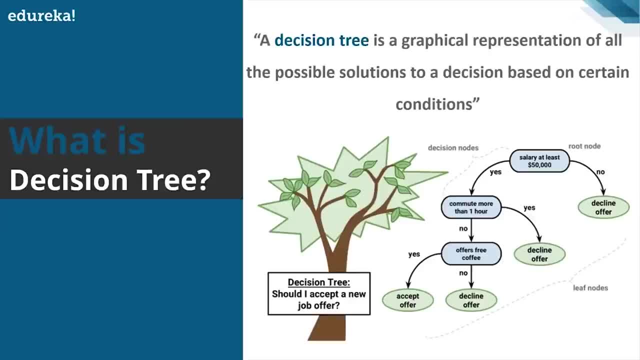 right Now. once you select 1, now again, it redirects you to a certain set of questions like press 1 for this, press 1 for that and similarly right. So this keeps on repeating until you finally get to the right person. 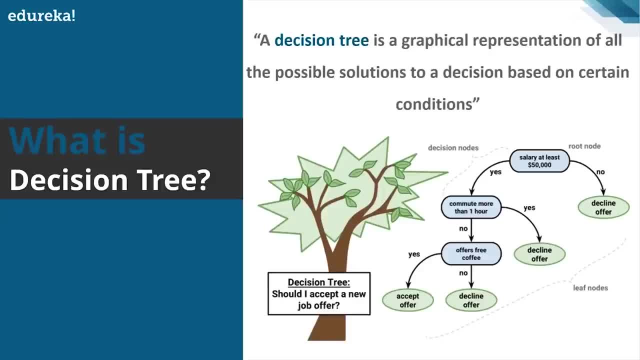 right Now. it's not like it's a blackmail hell, but what the company was actually doing, it was just using a decision tree to get you to the right person. Alright, I'd like you to focus on this particular image for a moment. 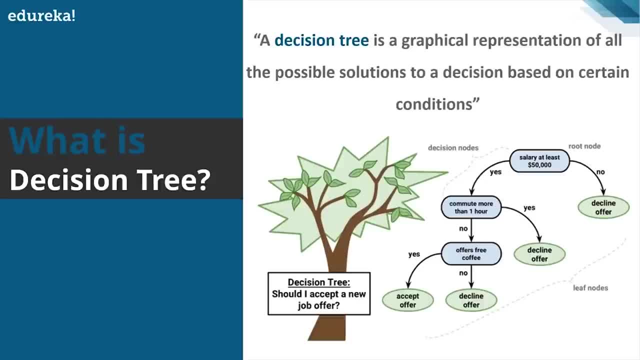 On this particular slide, you can see image where the task is. should I accept a new job offer or not? Alright, so you have to decide that. but that what you did? you created a decision tree starting with the base condition or the root node. 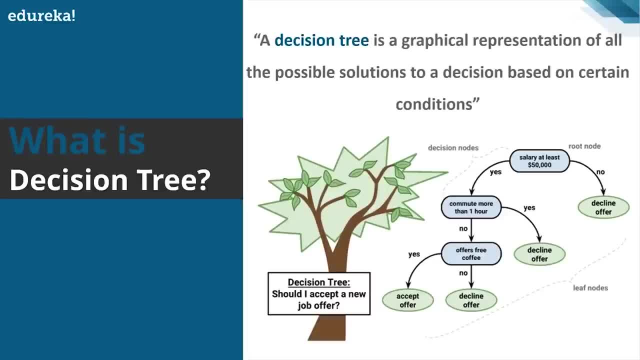 was that the basic salary is not at all accepting the offer. alright, So if your salary is greater than $50,000, then you will further check whether the commute is more than one hour or not. If it is more than one hour, 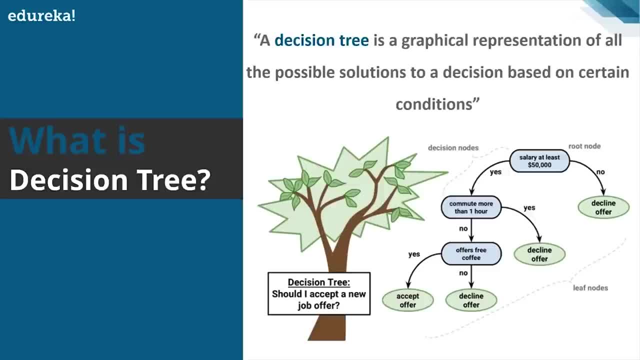 you will just decline the offer. If it is less than one hour, then you are getting closer to accepting the job offer. Then further, what you'll do? you will check whether the company is offering free coffee or not. right, If the company is not offering. 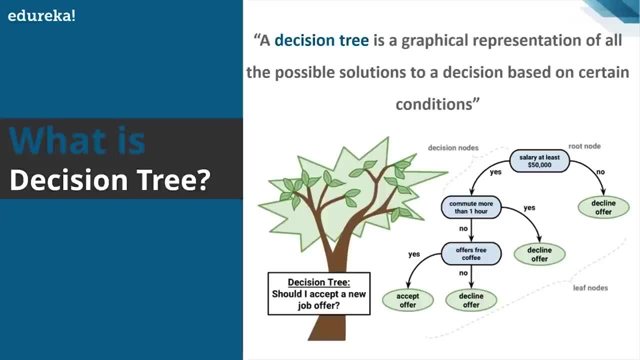 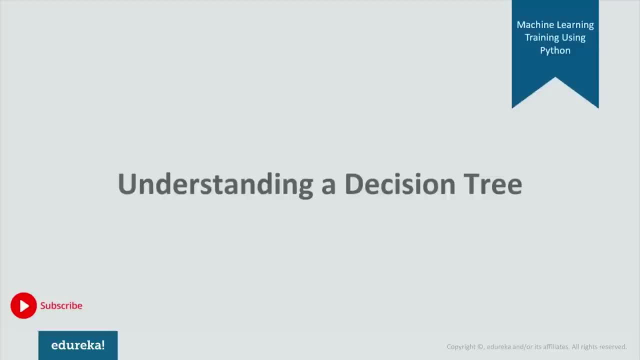 the free coffee, then you will just decline the offer, and if it is offering the free coffee, then yeah, you will happily accept the offer, right? So this is an example of a decision tree. Now let's move ahead and understand a decision tree. 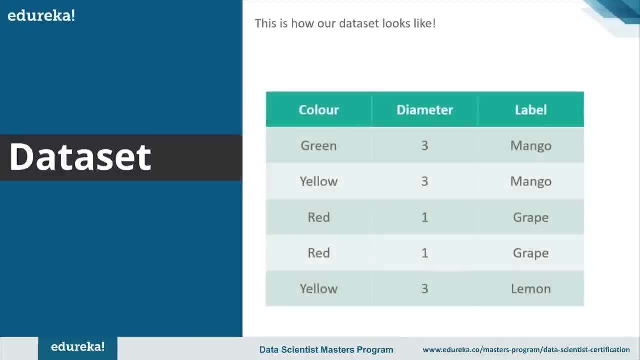 Well, here is a sample data set that I'll be using it to explain you about the decision tree, alright. In this data set, each row is an example and the first two columns provide features or attributes. that describes the data and the last column. 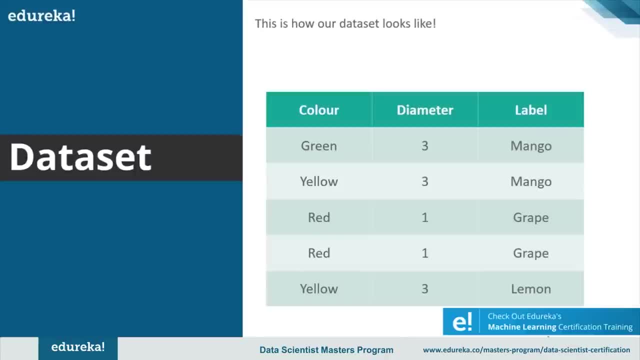 gives the label or the class we want to predict and, if you like, you can just modify this data by adding additional features and more example, and our program will work in exactly the same way. Now this data set is pretty straightforward, except for one thing. 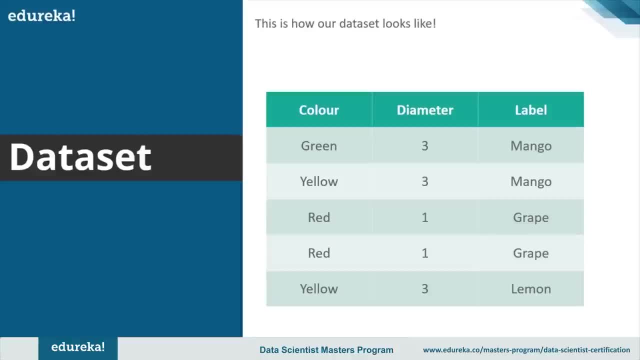 I hope you have noticed that it is not perfectly separable. Let me tell you something more about that, as in the second and fifth examples, they have the same features but different labels. both have yellow as their color and diameter as three, but the labels are mango. 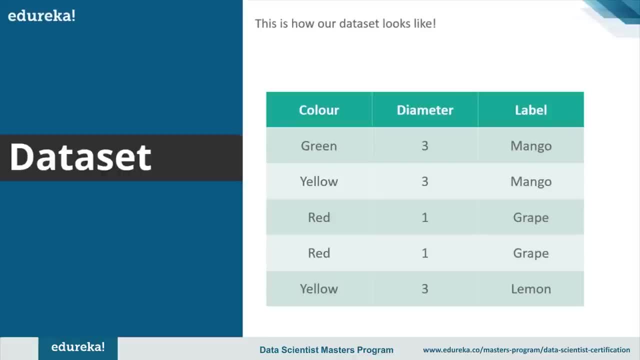 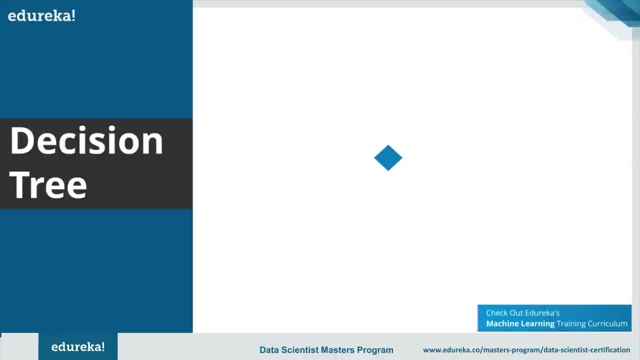 and lemon, right. Let's move on and see how decision tree handles this case. Alright, in order to build a tree, the SCART algorithm stands for classification and regression tree algorithm. Alright, let's see a preview of how it works. 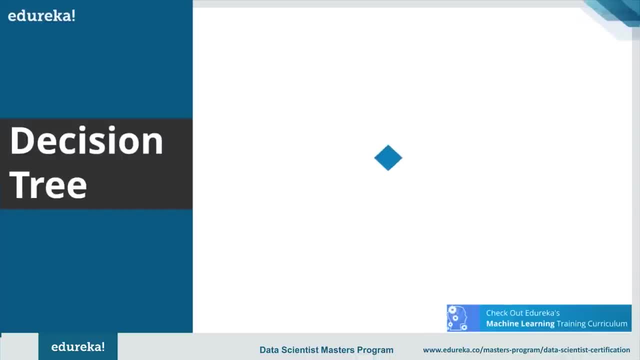 Alright, to begin with, we'll add a root node for the tree and all the nodes receive a list of rows as input and the root will receive the entire training data set. Now each node will ask true and false question about one of the feature. 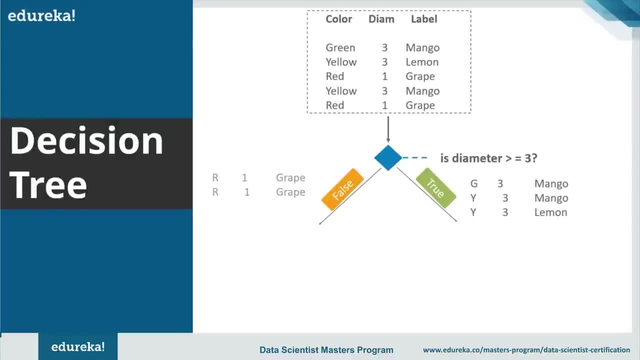 and in response to that question, will split or partition the data set into two different subsets. These subsets will be used in order to determine which of the two nodes is the best and which is the worst. Now let's look at the distribution of the labels. 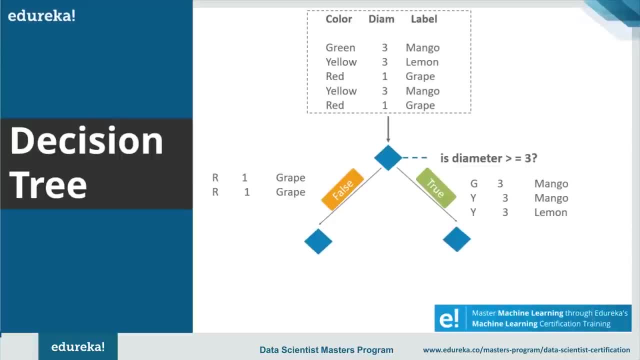 at each node. For example, the input of this node contains only one single type of label, So we could say that it's perfectly unmixed. There is no uncertainty about the type of label, as it consists of only grapes, right? So 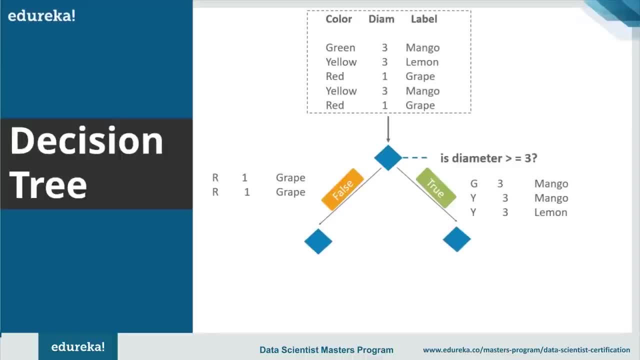 we would ask another question to further drill it down. right, But before that we need to understand which question to ask and when. and to do that we need to quantify how much question helps to unmix the label and we can quantify the amount. 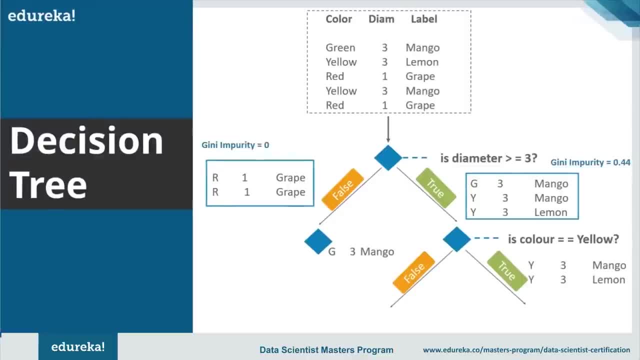 of uncertainty at a single node using a metric called Gini impurity, and we can quantify how much a question reduces that uncertainty using a concept called information gain. We'll use these to select the best question to ask at each point, and then what we'll do. 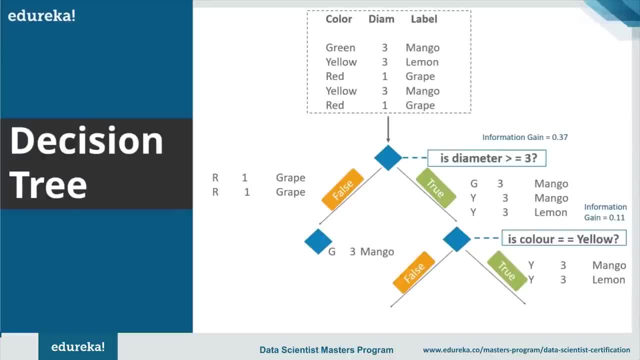 is. we'll iterate the steps will recursively build the tree on. each of the new node, will continue dividing the data until there are no further question to ask and finally we reach to our leaf. All right, All right, So this was about decision tree. 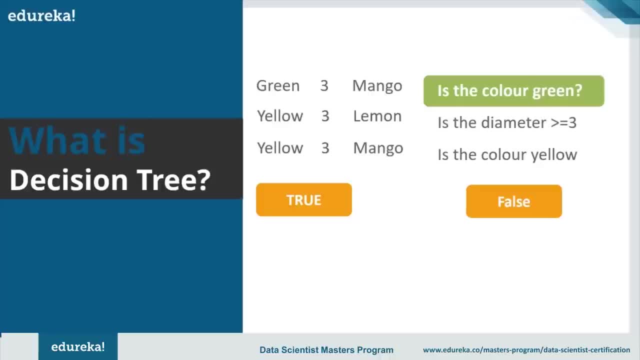 So, in order to create a decision tree, First of all, what you have to do, you have to identify different set of questions that you can ask to a tree, like: is this color green and what will be these question? these question will be decided by your data set. 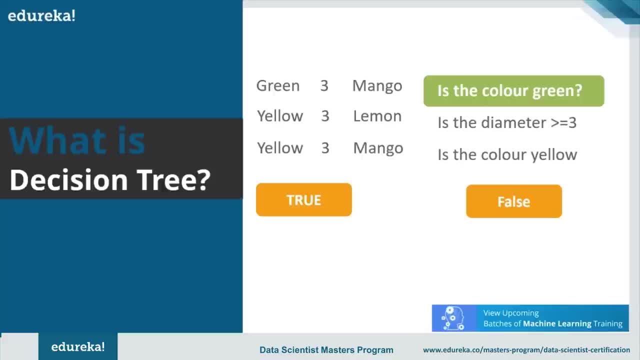 like. is this color green? Is this color yellow? Right Questions resembles to your data set. Remember that. All right. So if my color is green, then what it will do. it will divide into two parts. First, the green mango will be in the true 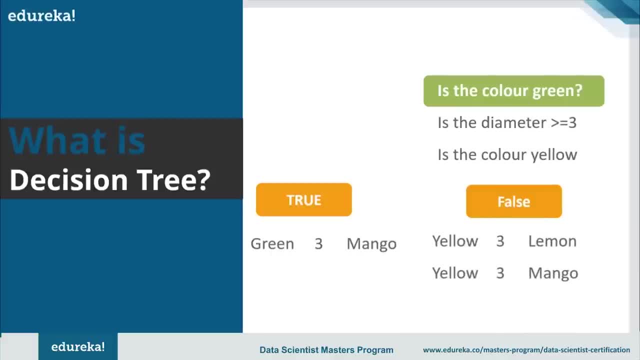 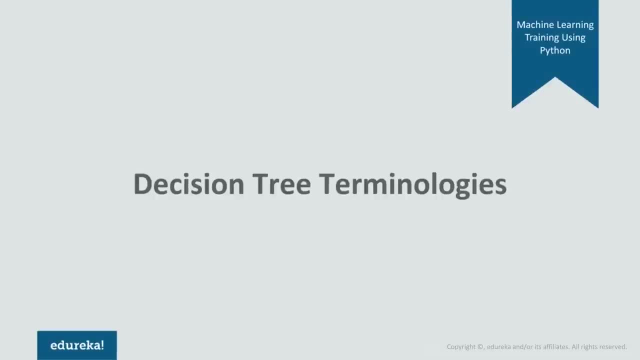 while on the false we have lemon and the mango. All right If the color is green, or the diameter is greater than or equal to three, or the color is yellow. decision tree terminologies. So, starting with root node, root node is the base node of a tree. 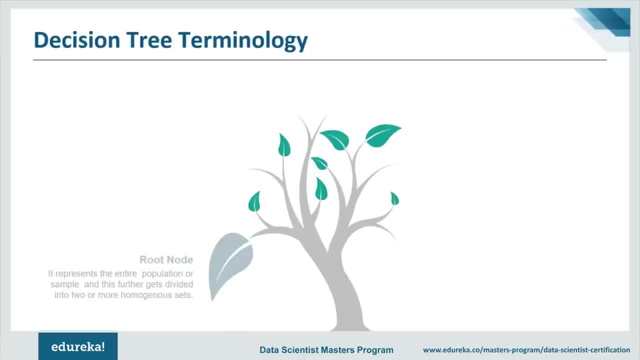 The entire tree starts from a root node. In other words, it is the first node of a tree. It represents the entire population or sample, and this entire population is further segregated or divided into two or more homogeneous set, Fine. Next is the leaf node. 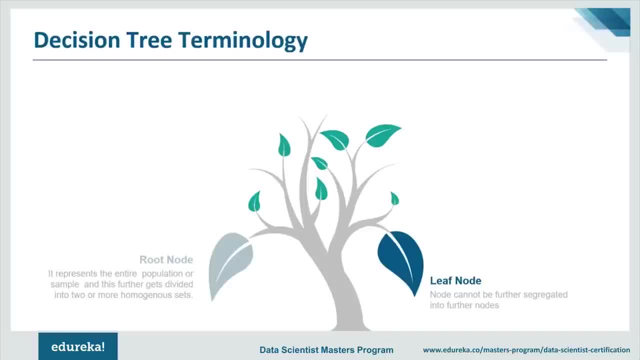 Well, leaf node is the one when you reach at the end of the tree, Right That is. you cannot further segregated down to any other level. That is the leaf node. Next is splitting. Splitting is dividing your root node or your node into different sub part. 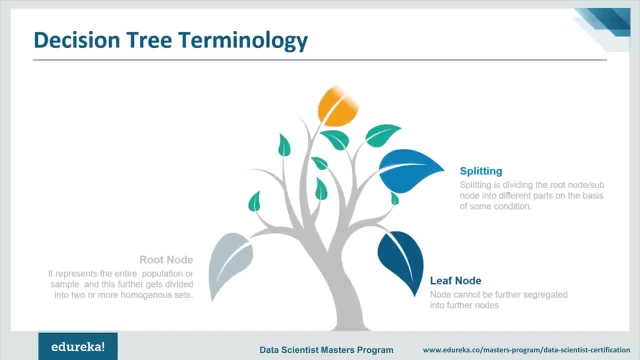 on the base node or some condition. Alright, Then comes the branch or the sub tree. Well, this branch or sub tree gets formed when you split the tree. Suppose, when you split a root node, it gets divided into two branches or two sub trees. 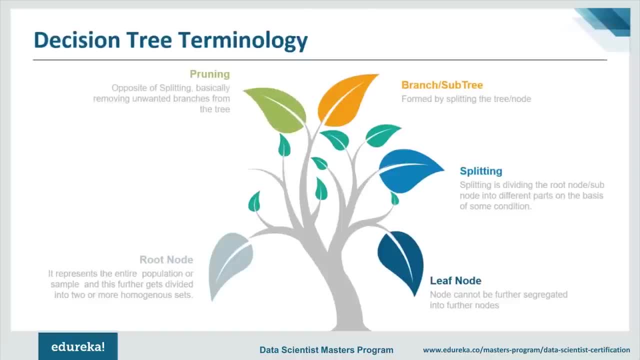 Right. Next is the concept of pruning. Well, you can say that pruning is just opposite of splitting. What we are doing here, we are just removing the sub node of a decision tree. We will see more about pruning later in this session. Alright. 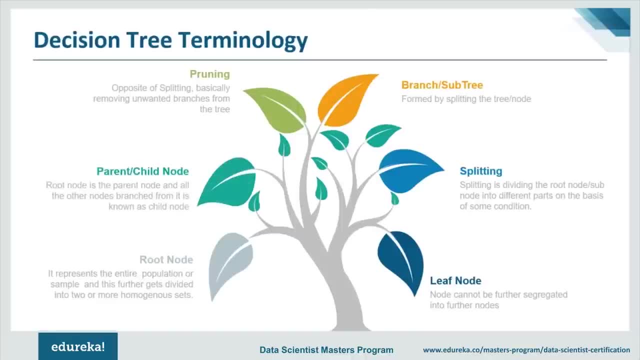 Let's move on ahead. Next is parent or child. Well, first of all, root node is always the parent node and all other nodes associated with that is known as child node. Well, you can understand it in a way that all the top node belongs to a parent node. 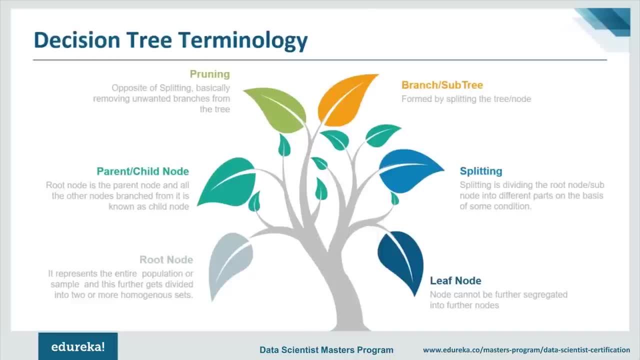 and all the bottom node which are derived from a top node is a child node. The node producing a further node is a child node and the node which is producing it is a parent node. Simple concept, right? Let's use the cart algorithm and design. 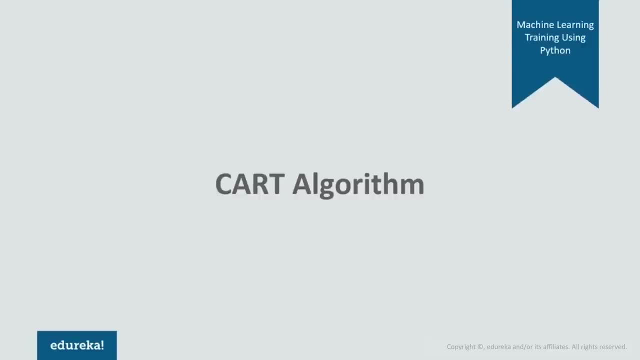 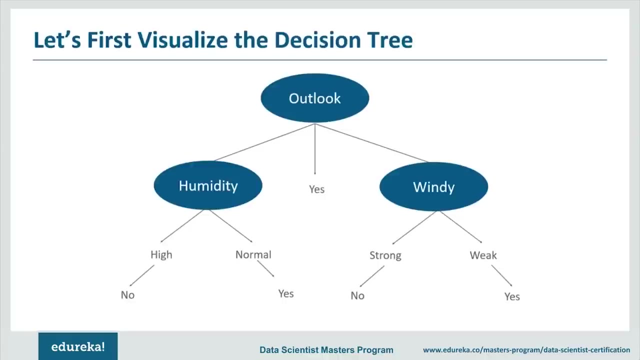 a tree manually. So, first of all, what you will do: you would decide which question to ask and when. So how will you do that? So let's first of all visualize the decision tree. So this is the decision tree which we will be creating. 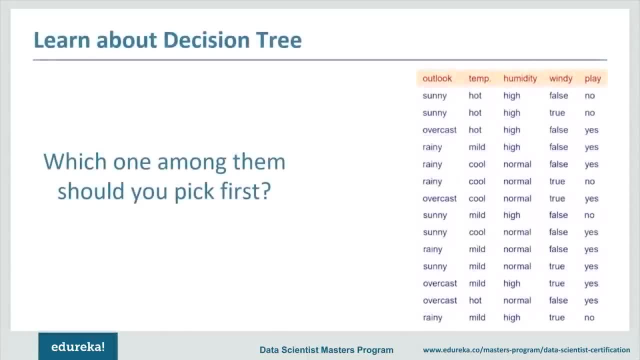 manually. Alright, First of all, let's have a look at the data set. You have outlook, temperature, humidity and windy as your different attribute. on the base of that, you have to predict that, whether you can play or not. So which one among them should you pick first? 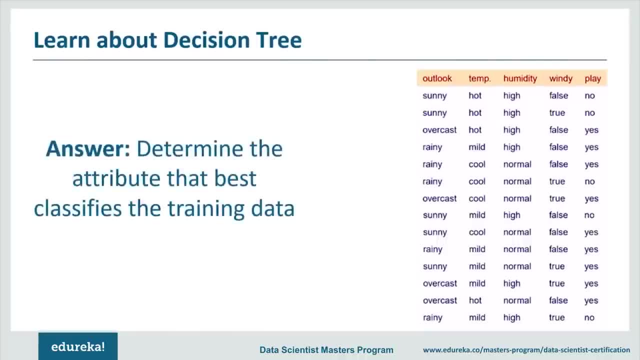 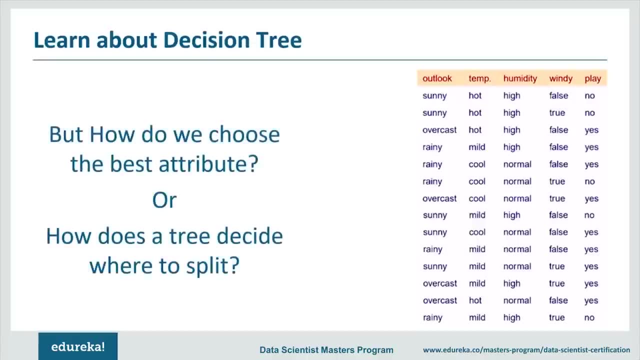 Answer: Determine the best attribute that classifies the training data. Alright, So how will you choose the best attribute? or how does a tree need to split, or how the tree will decide its root node? Well, before we move on and split a tree, there are some terminologies. 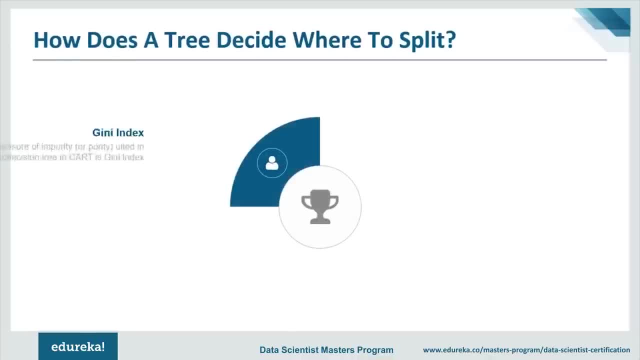 that you should know, Alright, First being the gene index. So what is this gene index? This gene index is the measure of impurity or purity used in building a decision tree in cart algorithm, Alright. Next is information gain. This information gain: 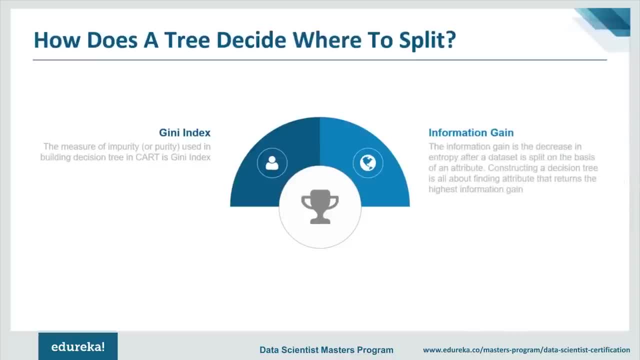 is the decrease in entropy after data set is split on the basis of an attribute. Constructing a decision tree is finding an attribute that returns the highest information gain- Alright, So you'll be selecting the node that would give you the highest information gain. 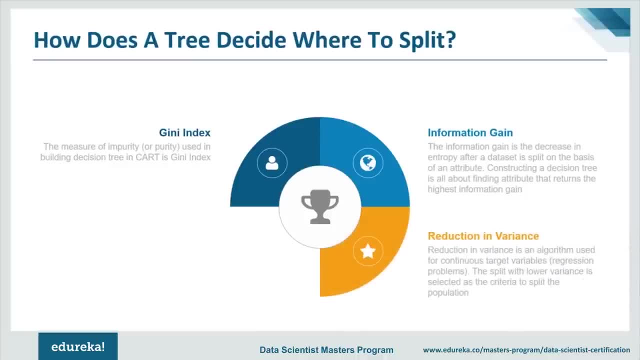 Alright. Next is reduction in variance. This reduction in variance is an algorithm which is used for continuous target variable or regression problems. The split with lower variance is selected as a criteria to split the population. See in general term. what do you mean by variance? 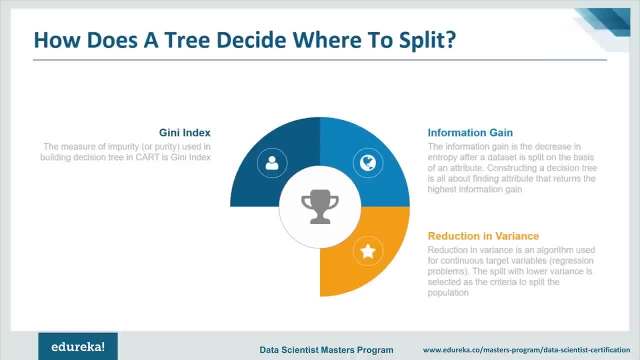 Variance is how much your data is varying. Right So, if your data is less impure, as the variation would be less as all the data are most similar. Right So there's also a way of splitting a tree that split with lower variance. 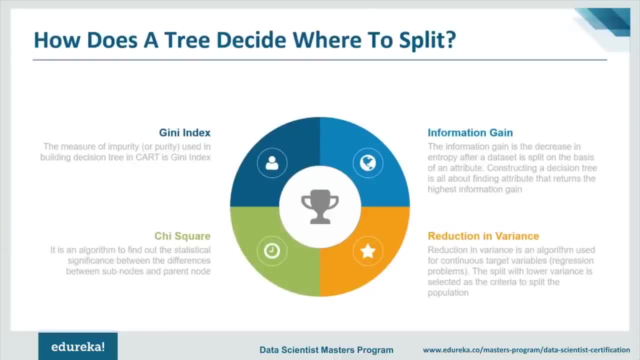 is selected as a criteria to split the population, Alright. Next is the G square. G square: It is an algorithm which is used to find out the statistical significance between the differences between sub nodes and the parent nodes. Fine, Let's move ahead. 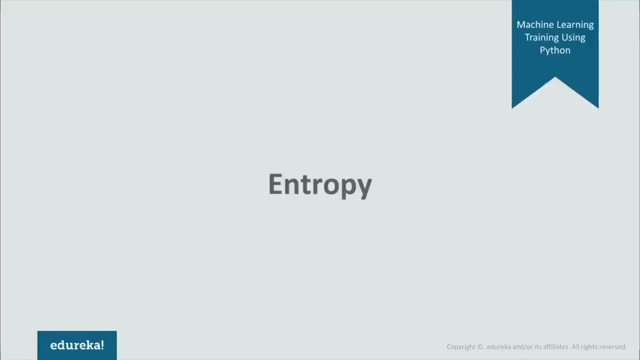 Now The main question is: how will you decide the best attribute? for now, Just understand: the attribute with the highest information gain is considered the best. Yeah, I know your next question might be like: what is this information? But before we move on and see what exactly, 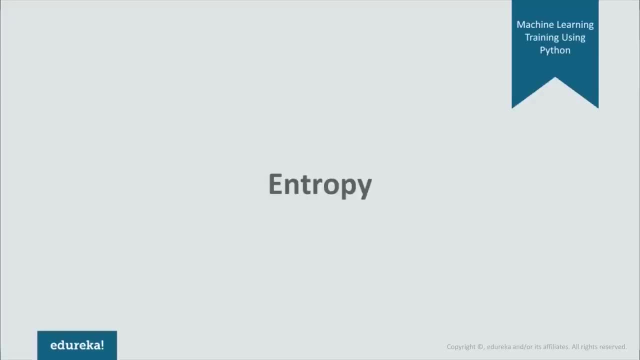 information gain is. let me first introduce you to a term called entropy, because this term will be used in calculating the information gain will. entropy is just a metric which measures the impurity of something, or in other words, you can say that it's the first step to do before you solve. 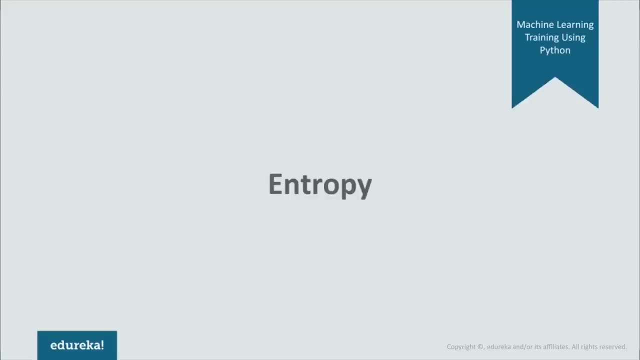 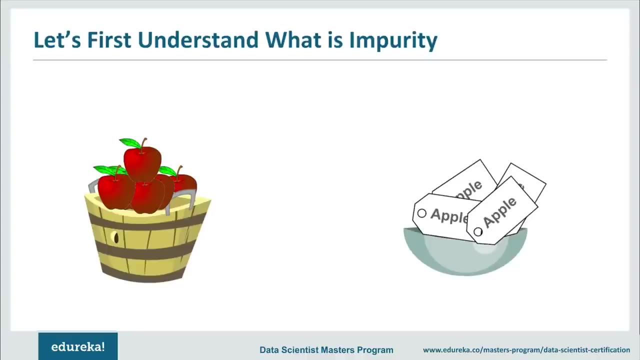 the problem of a decision tree, as I mentioned. to understand what is impurity, Suppose you have a basket full of apples and another bowl which is full of same label which says apple. Now, if you are asked to pick one item from each basket and ball, 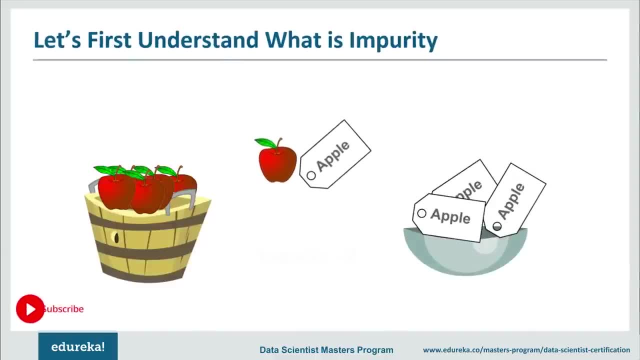 then the probability of getting the apple and its correct label is one. So in this case you can say that impurity is zero. All right, Now what if there are four different fruits in the basket and four different labels in the ball? then the probability 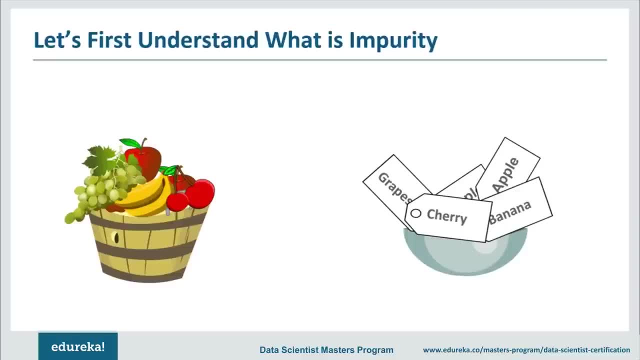 of matching the fruit to a label is obviously not one, Nothing less than that. Well, it could be possible that I picked banana from the basket and when I randomly picked the label from the ball, it says a cherry. Any random permutation and combination can be possible. 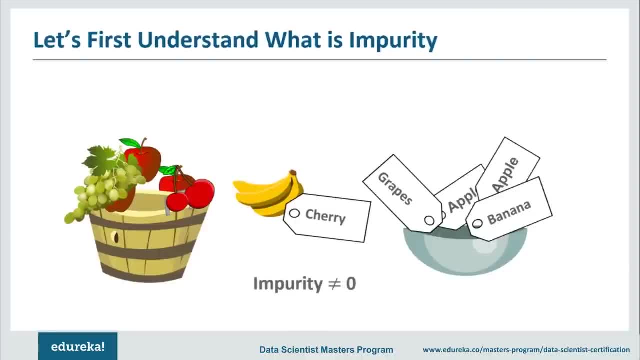 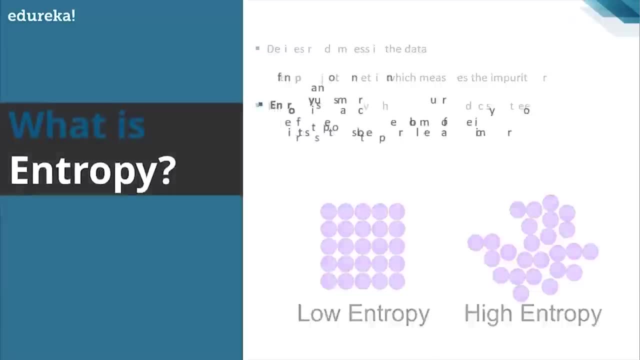 So in this case I would say that impurity is non-zero. I hope the concept of impurity is clear. So, coming back to entropy, As I said, entropy is the measure of impurity. From the graph on your left you can see that. 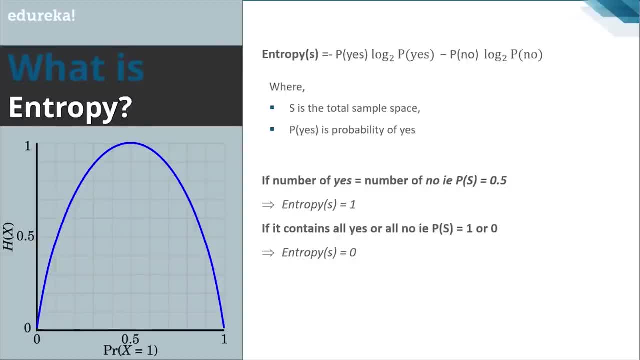 as the probability is zero or one. that is, either they are highly impure or the value of entropy is zero. and when the probability is 0.5, then the value of entropy is maximum. Well, what is impurity? Impurity is the degree. 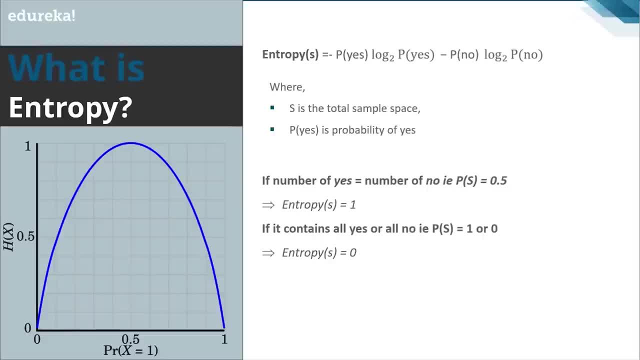 of randomness, how random a data is. So if the data is completely pure, in that case the randomness equals zero. or if the data is completely impure, even in that case, the value of impurity will be zero. Question like: why is it that the value of entropy? 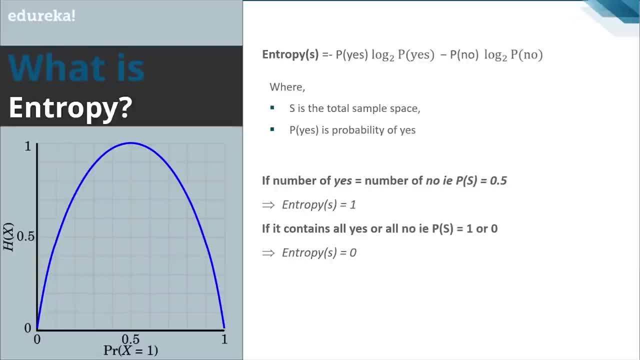 is maximum at 0.5 might arise in your mind, right. So let me discuss about that Mathematically. as you can see here on the slide, the mathematical formula of entropy is minus a probability of yes. Let's move on and see what this graph 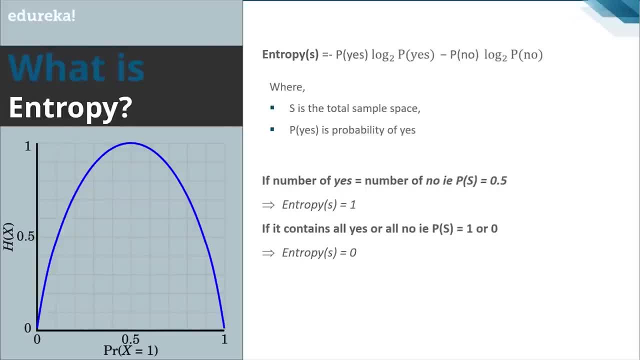 has to say mathematically, Suppose S is our total sample space and it's divided into two parts- yes and no, like in our data set, the result for playing was divided into two parts, either yes or no, which we have to predict, either we have to play. 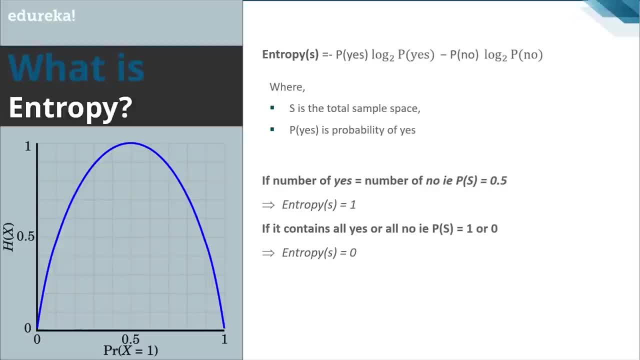 or not right. So for that particular case you can define the formula of entropy as entropy of total sample space equals negative of probability of yes multiplied by log of probability of yes with a base 2 minus probability of no multiplied by log of probability of no. 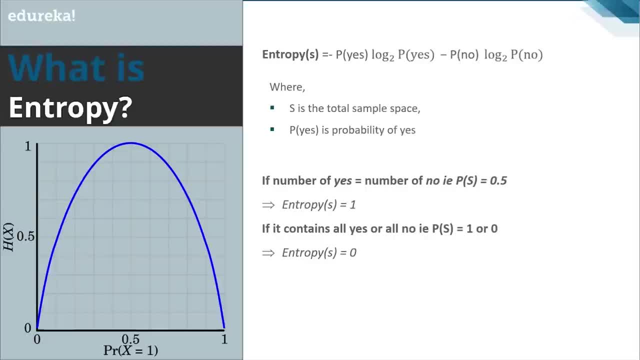 with base 2, where S is your total sample space and P of yes is the probability of yes and P of no is the probability of no. Well, if the number of yes equal number of no- that is, probability of S- equals 0.5 right. 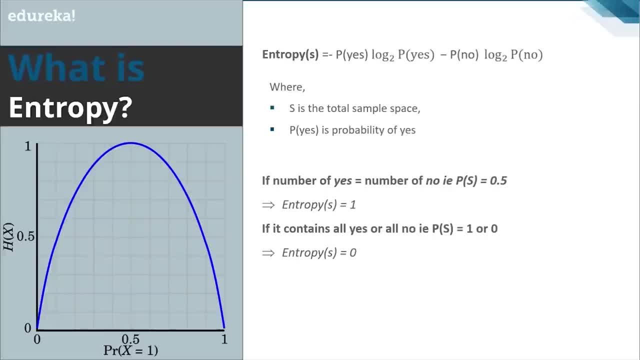 Since you have equal number of yes and no, In this case value of entropy will be one. just put the value over there. All right, Let me just move to the next slide. I'll show you this, All right. Next is if it contains: 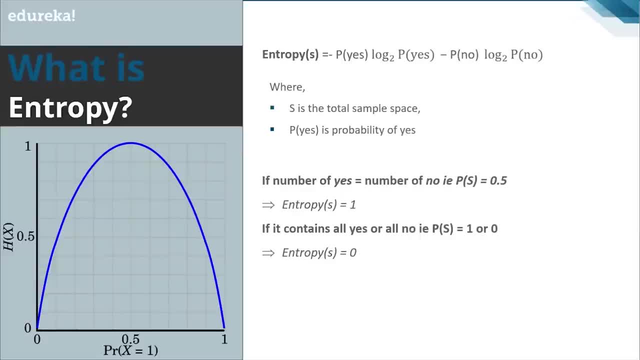 all yes or all no. that is, probability of a sample space is either one or zero, then in that case entropy will be equal to zero. Let's see it mathematically one by one. So let's start with the first condition, where the probability was 0.5.. 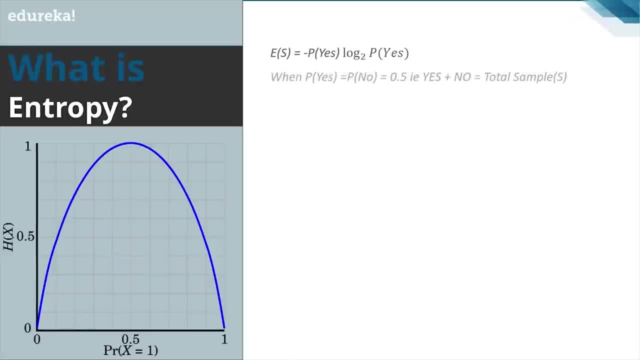 So this is our formula for entropy, right? So this is our formula. If we discuss that when the probability of yes equal probability of no, that is, in our data set We have equal number of yes and no. All right, So probability of yes equal. 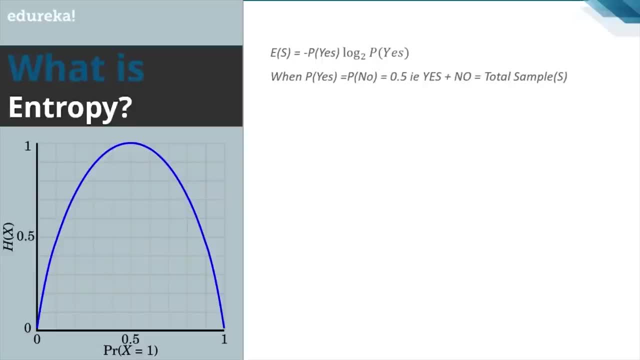 probability of no and that equals 0.5. or in other words, you can say that yes plus no equal to total sample space. All right, since the probability is 0.5.. So when you put the values in the formula, you get something. 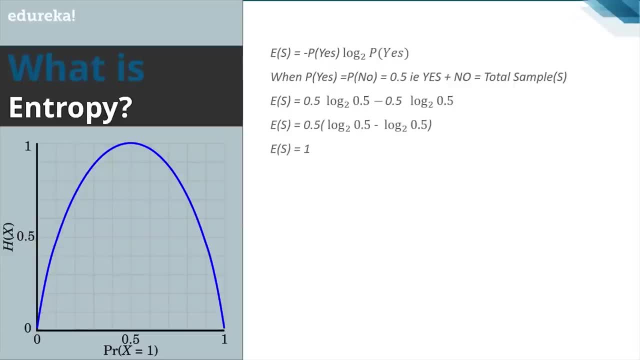 like this, and when you calculate it, you will get the entropy of the total sample space. let's see for the next case. What was the next case? Either you have total yes or you have total no. So if you have total yes, let's see the formula. 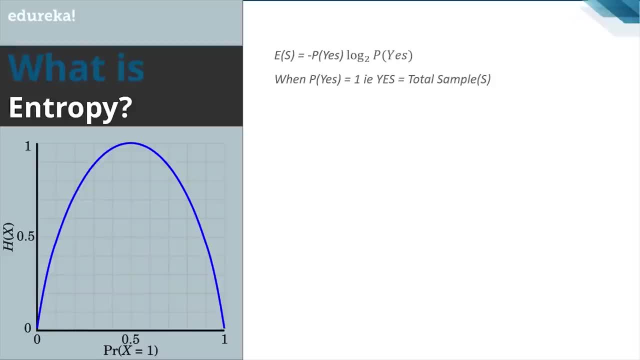 when we have total yes. So you have all yes and 0. no fine. So probability of yes equal 1 and yes as the total sample space, obviously. So in the formula when you put that thing up, you will get entropy of sample space. 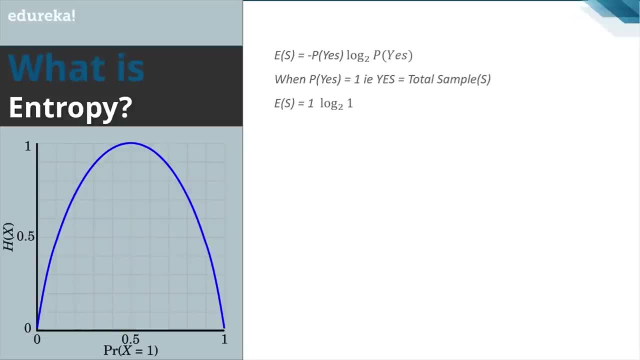 equal negative times of 1 multiplied by log of 1, as the value of log 1 equals 0. So the total sampling will result to 0. similarly is the case with no. even in that case you'll get the entropy of total sample space. 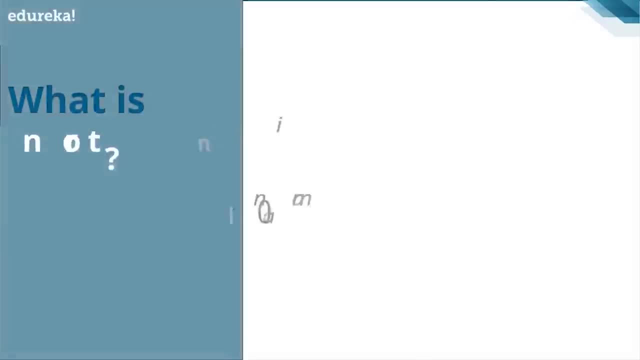 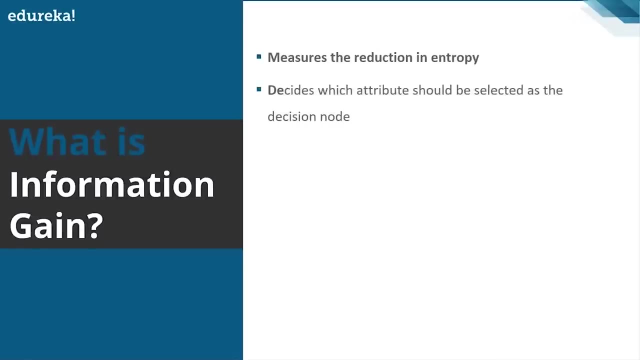 as 0.. So this was all about entropy. All right. Next is, what is information gain? Well, information gain what it does. it measures the reduction in entropy. It decides which attribute should be selected as the decision node. If S is our total, 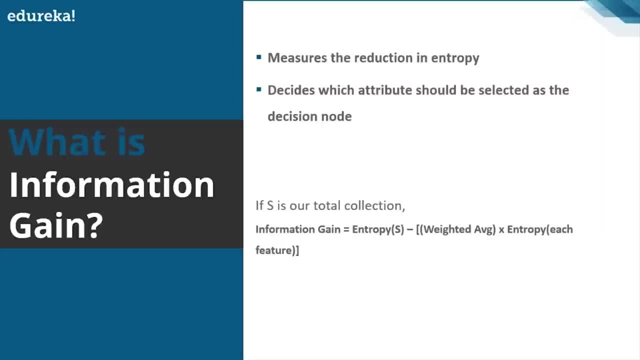 collection. then information gain equals entropy, which we calculated just now. that minus 1 multiplied by entropy of each feature. Don't worry, We'll just see how to calculate it with an example. Let's manually build a decision tree for our data set. 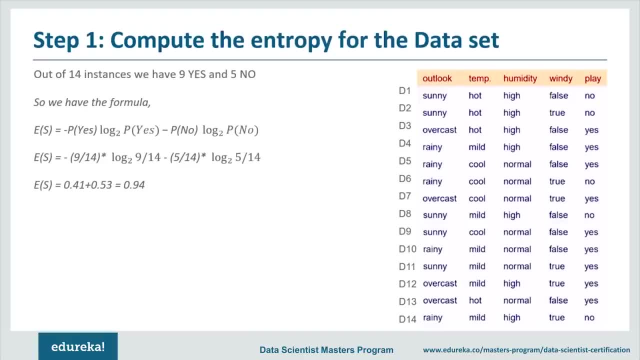 So there's our data set, which consists of 14 different instances, out of which we have nine yes and five no. All right, So we have the formula for entropy, just put over that, since nine years. so total probability of yes equals 9 by 14. 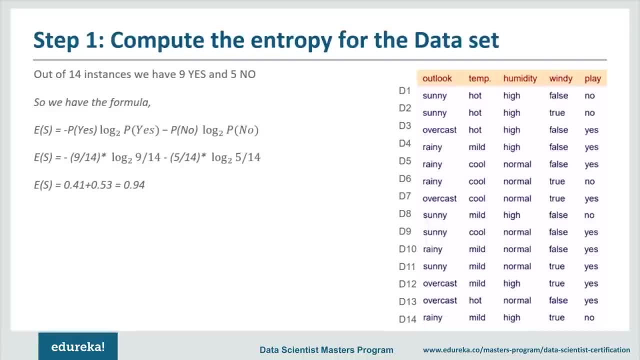 and total probability of no equals 5 by 14, and when you put up the value, you get the value of entropy as 0.94.. All right, So this was your first step, that is, compute the entropy for the entire data set. All right. 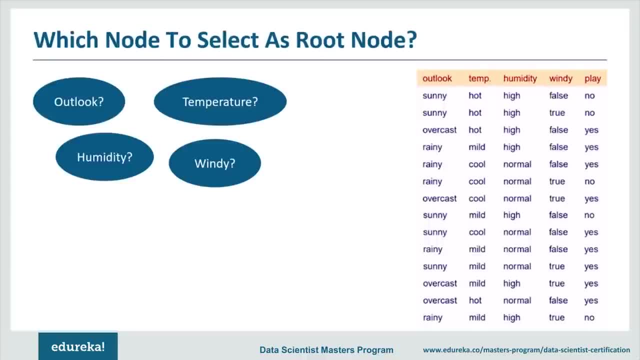 Now you have to select that out of Outlook: temperature, humidity and windy. which of the node should you select as the root node? big question, right? How will you decide that this particular node should be chosen at the base node and on the base of that only? 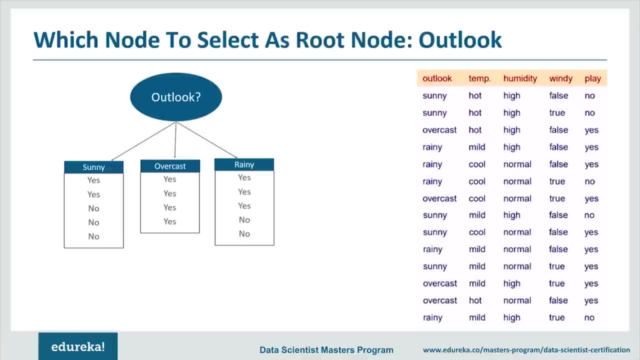 I'll be creating the entire tree. how you'll select that, let's see. so you have to do it for all of the different nodes, So starting with Outlook. so Outlook has three different parameters: sunny, overcast and rainy. So first of all, select how many number of yes. 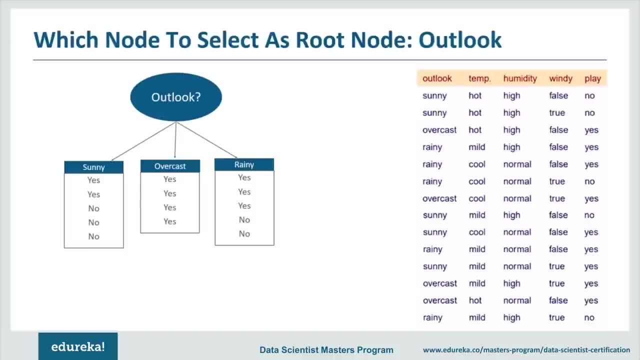 and no are there in the case of sunny, like when it is sunny, how many number of yes and how many number of nose are there? So, in total, we have two years and three nose. in case of Sunny, in case of overcast, We have all yes. 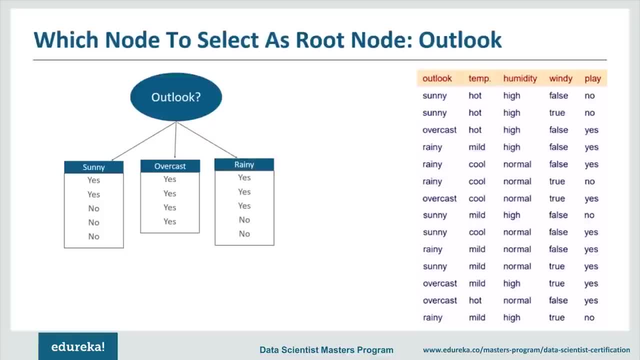 So if it is overcast, then we'll surely go to play. It's like that, All right. And next it is rainy, then total number of yes equal three and total number of no equals two. fine, Next, what we do? we calculate the entropy. 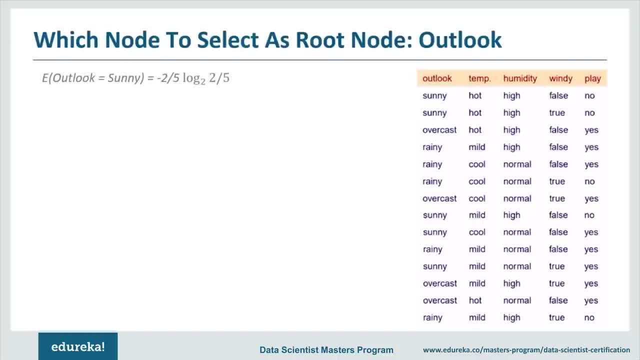 for each feature. for here We are calculating the entropy when Outlook equals sunny. First of all, we are assuming that Outlook is our root node and for that we are calculating the information gain for it. All right, So in order to calculate the information gain, 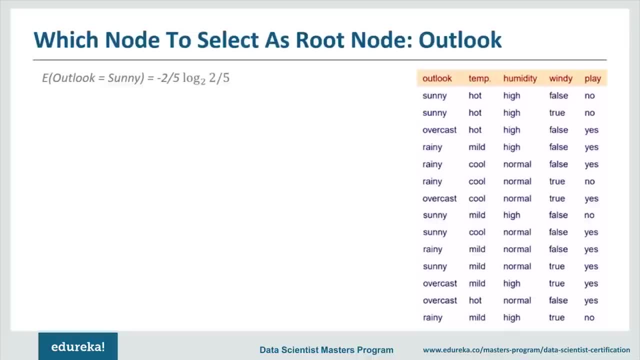 remember the formula. It was entropy of the total sample space minus weighted average, multiplied by entropy of each feature. All right, So what we are doing here? we are calculating the entropy of Outlook when it was sunny. So total number of yes, when it was sunny. 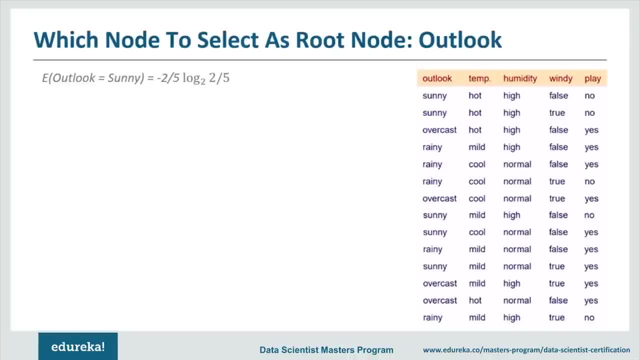 was two and total number of no that was three. fine, So let's put up in the formula, since the probability of yes is two by five and the probability of no is three by five, So you will get something like this. All right, So you are getting. 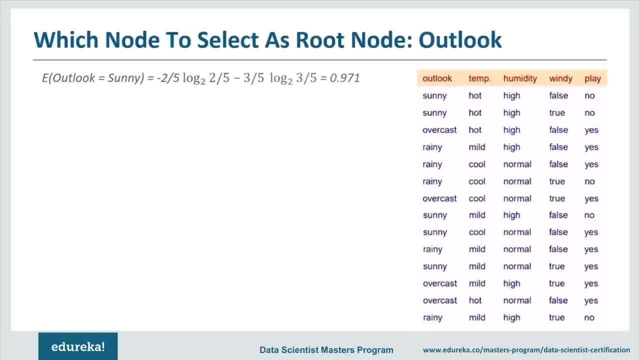 the entropy of Sunny as 0.971. fine. Next you will calculate the entropy for overcast. when it was overcast, Remember, it was all yes, right? So the probability of yes equal one, and when you put over that you'll get the value. 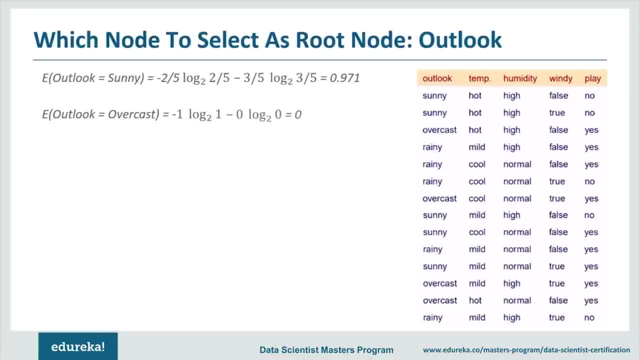 of entropy as zero, fine. and when it was rainy rainy has three yes and two nose. So probability of yes in case of Sunny is three by five and probability of no in case of Sunny is two by five. and when you add the value of probability of yes, 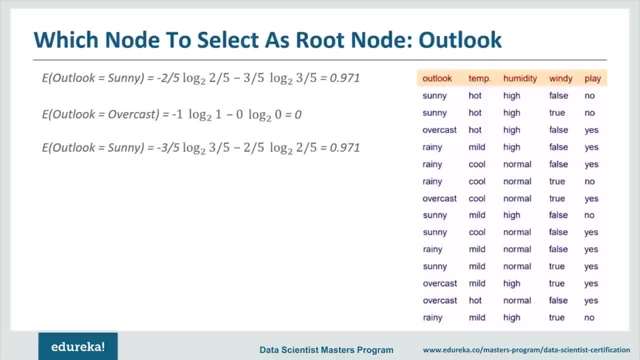 and probability of no to the formula. You get the entropy of Sunny as 0.971. fine, Now you have to calculate how much information you are getting from Outlook. that equals weighted average, All right. So what was this weighted average? total number of yes and total number. 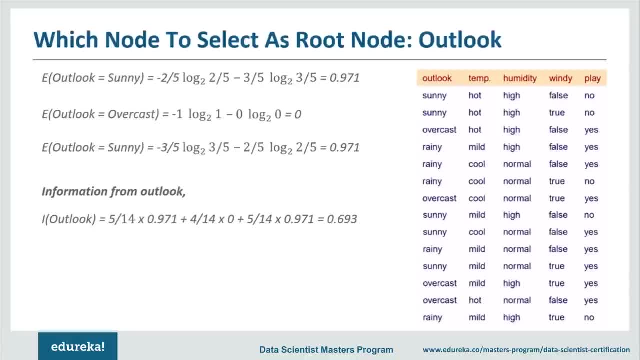 of no fine. So information from Outlook equals five by 14. from where does this five came over? We are calculating the total number of sample space within that particular Outlook. when it was sunny, right? So in case of Sunny, there was two yes and three nose. 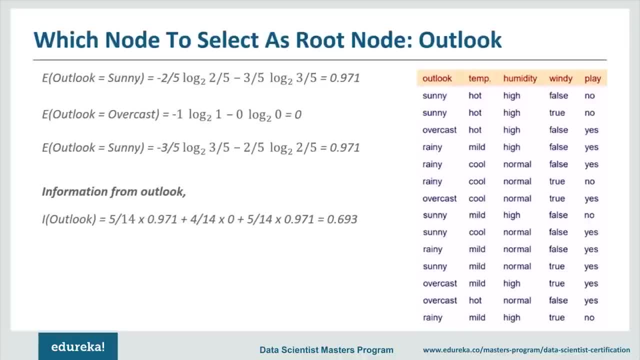 All right, So weighted average for Sunny would be equal to five by 14.. All right, Since the formula was five by 14, multiplied by entropy of each feature. All right, So, as calculated, the entropy for Sunny is 0.971, right. 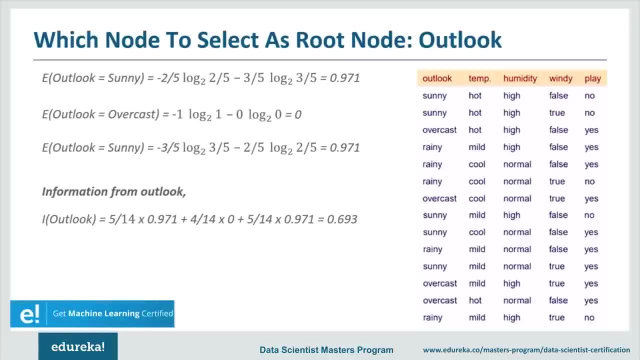 So what we'll do will multiply 5 by 14 with 0.971, right? Well, this was a calculation for information. when Outlook equals Sunny, but Outlook even equals overcast and rainy. for, in that case, What we'll do again, 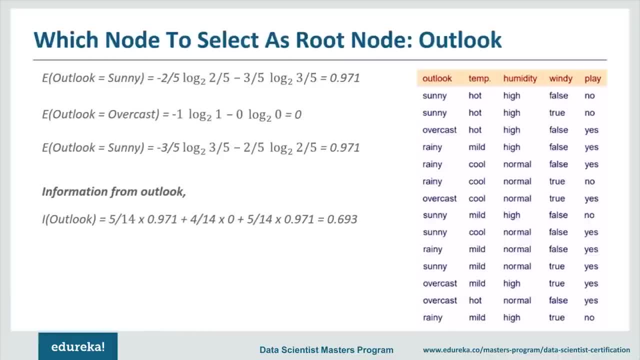 Similarly will calculate for everything, for overcast and Sunny. for overcast weighted averages, 4 by 14, multiplied by its entropy, That is 0, and for Sunny It is same as for 14, three years and two knows, multiplied by its entropy, That is 0.971. 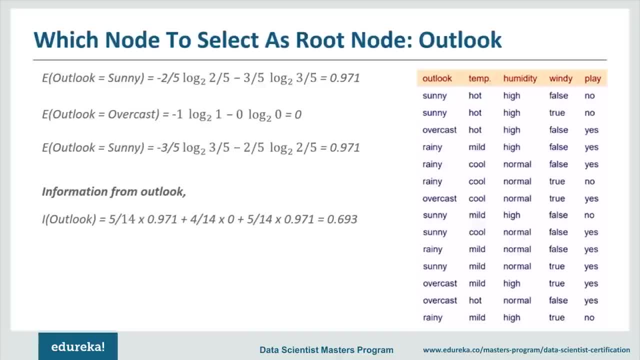 and finally, will take the sum of all of them, which equals to 0.693, right. Next we'll calculate the information gained. this: what we did earlier was information taken from Outlook. Now we are calculating what is the information we are gaining from Outlook right now. 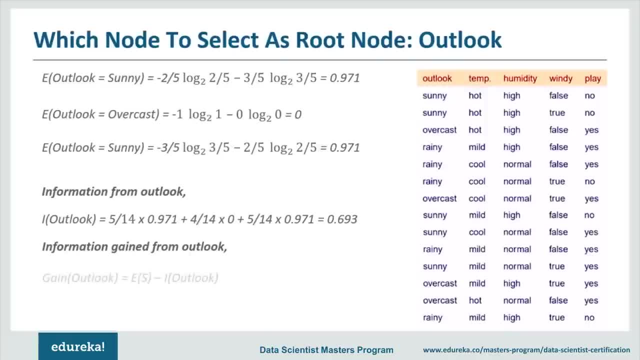 this information gain. that equals to total entropy minus the information that is taken from Outlook. All right, So what we're going to do is we're going to calculate. so total entropy- We had 0.94, minus information We took from Outlook- is 0.693.. 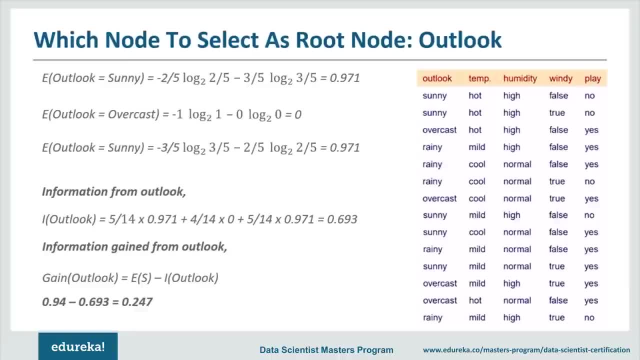 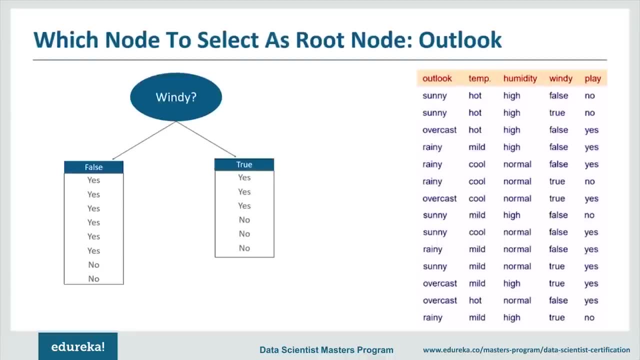 So the value of information gained from Outlook results to 0.247.. All right, So next, what do we have to do? Let's assume that Wendy is our root node. So Wendy consists of two parameters, false and true. Let's see how many yes. 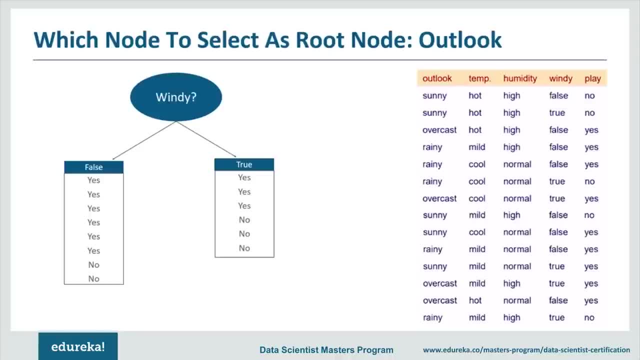 and how many knows are there in case of true and false. So when Wendy has false as its parameter, then in that case it has six yes and two no. Let's see how many no's. and when it has true as its parameter, it has three yes. 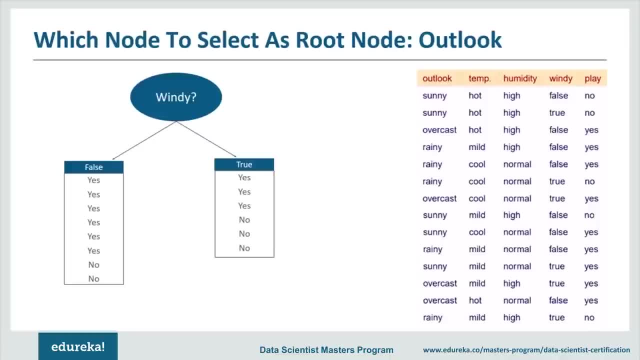 and three no's. All right, So let's move ahead and similarly calculate the information taken from Wendy and finally calculate the information gained from Wendy. All right, So, first of all, what we'll do will calculate the entropy of each feature, starting with Wendy, equal true. 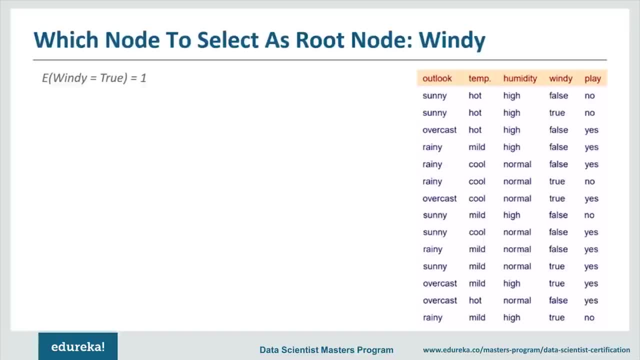 So in case of true, we had equal number of yes and equal number of no. We'll remember the graph when we had the probability of yes and no and for that case the entropy equals one. So we can directly write entropy of true when it's Wendy. 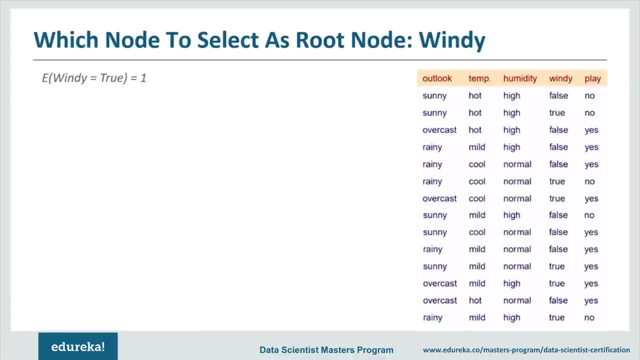 is one, as we had already proved it, when probability equals 0.5, the entropy is the maximum that equals to one, All right. Next is entropy of false when it is Wendy, All right. So similarly, just put the probability of yes and no. 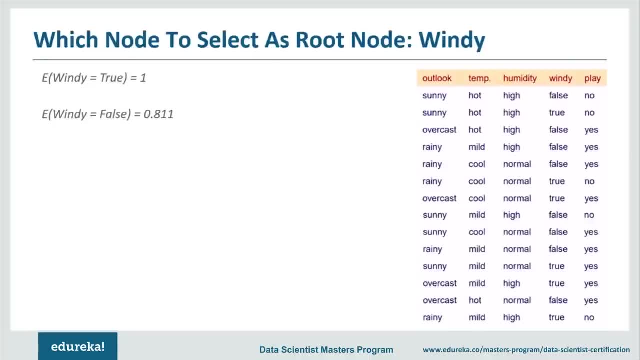 in the formula and then calculate the result, since you have six yes and probability of no as two by eight. All right, So when you will calculate it, you will get the entropy of false as 0.811.. All right, Now let's calculate. 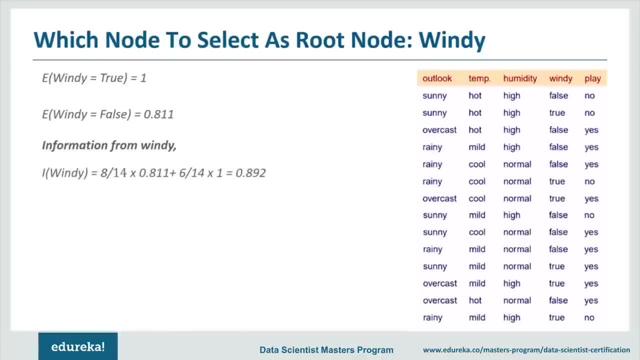 the information from Wendy. So total information collected from Wendy equals information taken when Wendy equal true, plus information taken when Wendy equal false. So we'll calculate the weighted average for each one of them and then we'll sum it up to finally get the total information. 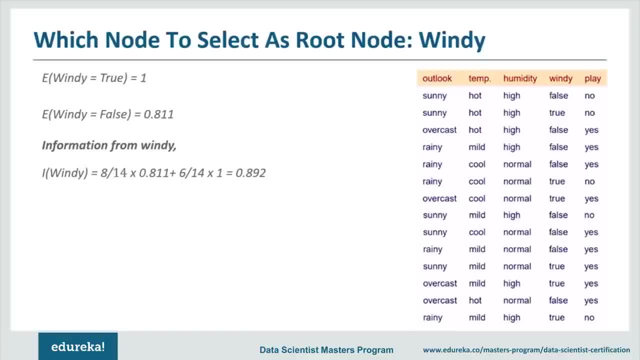 taken from Wendy. So in this case it equals to 8 by 0.811 plus 6 by 14 multiplied by 1.. What is this 8?? 8 is total number of yes and no in case when Wendy equals false. 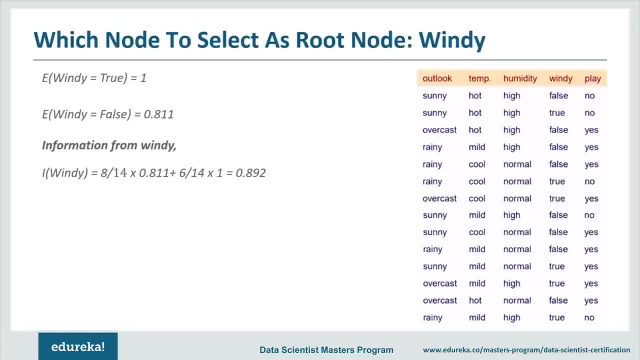 right. So when it was false. so total number of yes, that equals to 6, and total number of no, that equal to 2, that sum ups to 8.. All right, So. that is why the weighted average results to 8 by 14.. 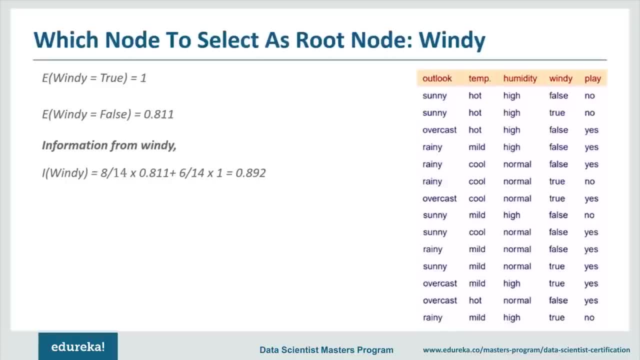 Similarly, information taken when Wendy equals true equals to 3 plus 3, that is, 3 yes and 3 no equals 6 plus 14 multiplied by 1. that is entropy of true, All right. so it is 8 by 14 multiplied by 0.811. 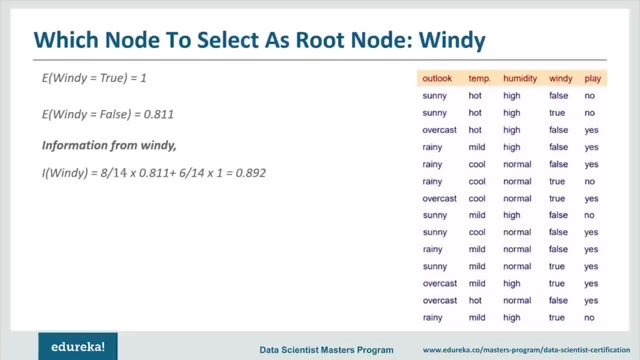 plus 6 by 14, multiplied by 1, which results to 0.892.. This is information taken from Wendy. All right, Now, how much information you are gaining from Wendy. So for that, what you'll do. so, total information gained from Wendy. 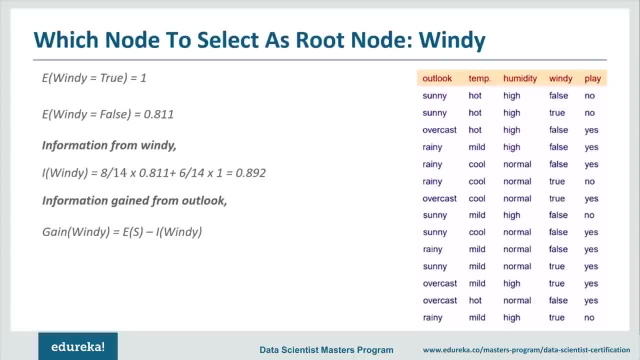 that equals to total entropy minus information taken from Wendy. All right, that is 0.94 minus 0.892. that equals to 0.048.. So 0.048 is the information gained from Wendy. Similarly, we calculated for the rest. 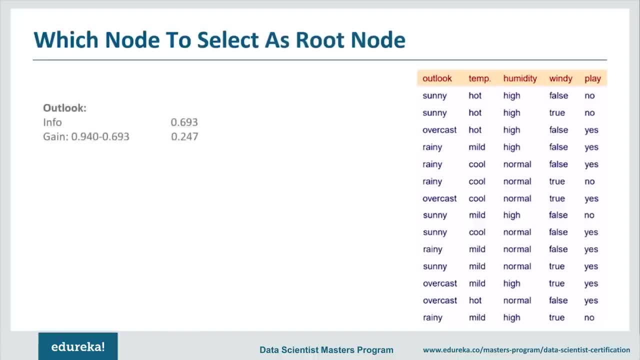 too. So for Outlook, as you can see, the information was 0.693 and its information gain was 0.247. in case of temperature, the information was around 0.911 and the information gain that was equal to 0.029 in case. 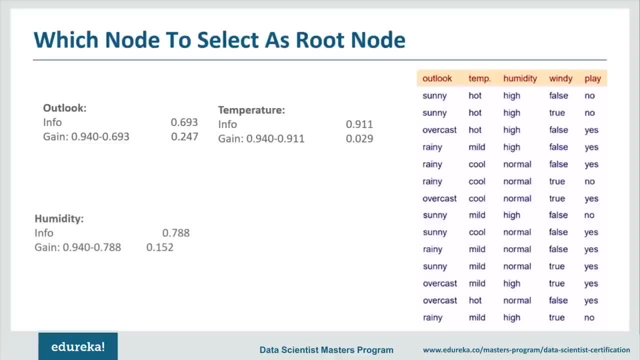 of humidity, the information gain was 0.152 and in the case of Wendy, the information gain was 0.48. so what we'll do will select the attribute with the maximum fine. Now we are selected Outlook as our root node, and it is further. 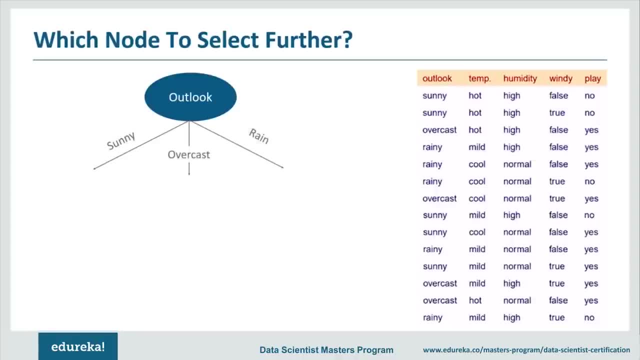 subdivided into three different parts: sunny, overcast and rain. So in case of overcast, we have seen that it consists of all. yes, so we can consider it as a leaf node, But in case of sunny and rainy, it's doubtful as it consists. 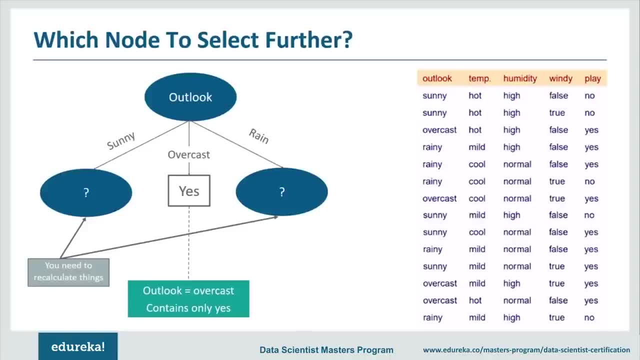 of both yes and both no, So you need to recalculate the things right again. all right, You have to again select the attribute which is having the maximum information gain. All right, So there's how your complete tree will look like, all right. 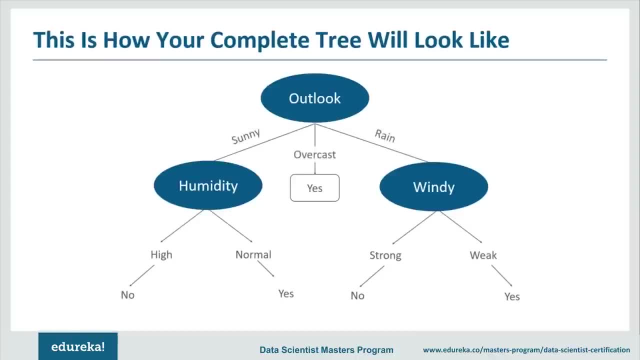 So let's see when you can play. so you can play when Outlook is overcast. all right, In that case you can always play if the Outlook is sunny. You will further drill down to check the humidity condition. all right, If the humidity is normal. 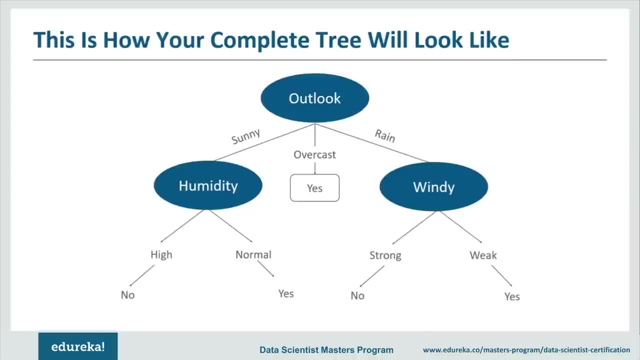 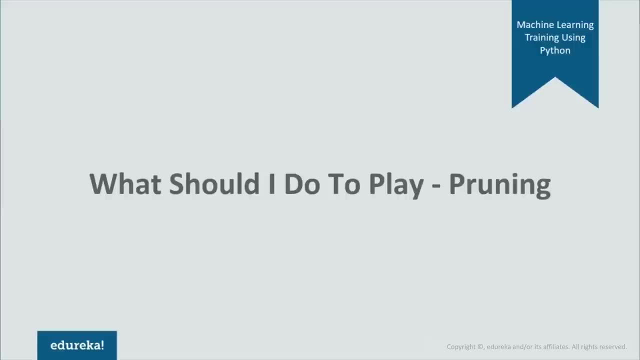 you can check whether it's windy or not. If it has a weak wind, then you'll go and offer play, but if it has strong wind, then you won't play right. So there's how your entire decision tree would look like at the end. 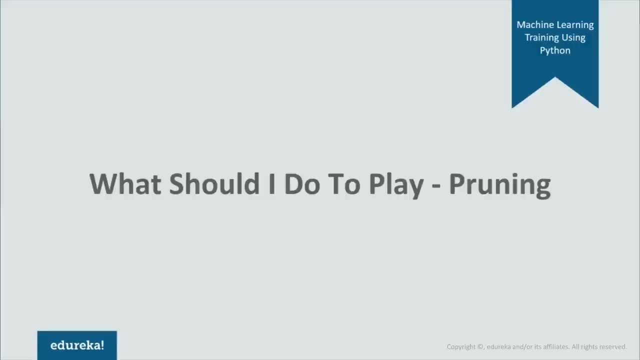 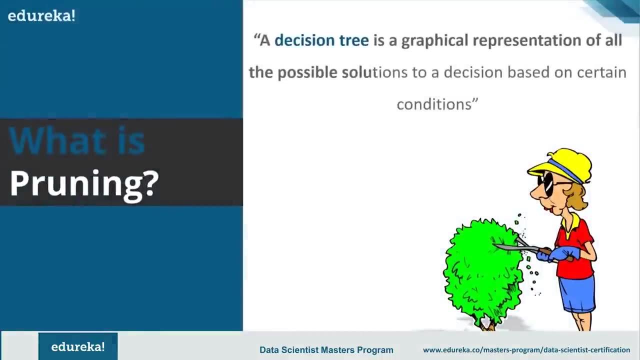 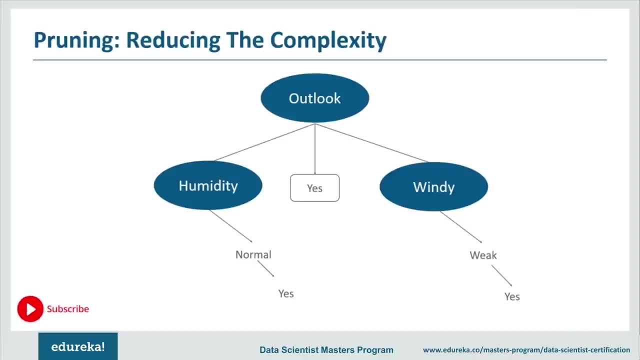 Now comes the concept of pruning says that: what should I do to play? Well, you have to do pruning. pruning will decide how you will play. What is this pruning? Well, this pruning is nothing but cutting down the nodes of the tree in order to 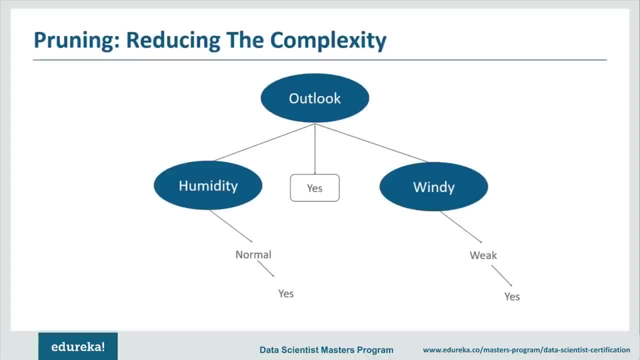 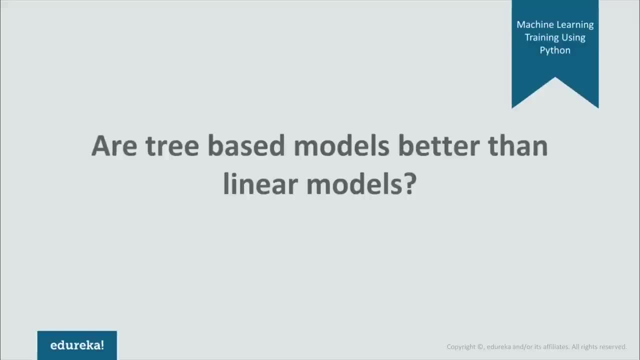 make the tree look like city. all right, As here. you can see on the screen that it's showing only the result, for yes, that is, it's showing all the result, which says that you can play. before we drill down to a practical session, a common question. 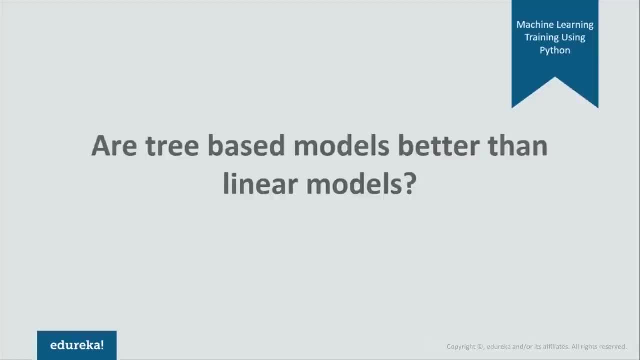 might come in your mind. you might think that a tree based model better than linear model, right? Some people have this question in their mind, and well, there's a valid question to will. actually, as I said earlier, you can use any algorithm. It depends on the type of problem. 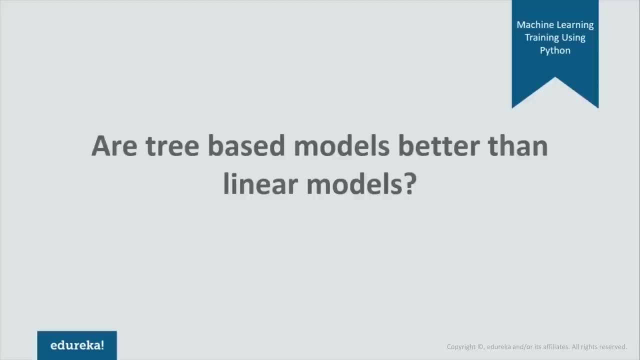 you're solving. Let's look at some key factor which will help you to decide which algorithm to use and when. so the first point being, if the relationship between dependent and independent variable is well approximated by a linear model, then linear regression will outperform tree based model. 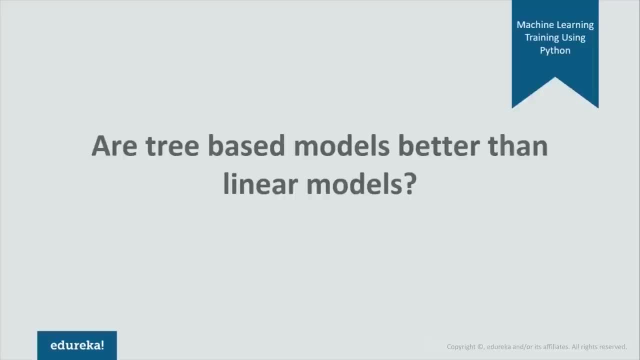 second case: if there is a high relationship between dependent and independent variables, a tree model will outperform a classical regression model. and third case: if you need to build a model which is easy to explain to people, a decision tree model will always do better than a linear model. 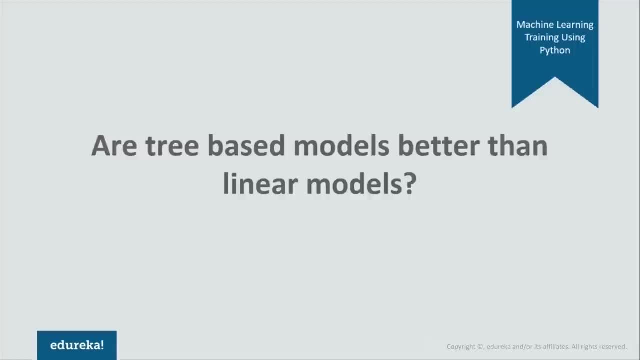 as the decision tree models are simpler to interpret than linear regression, alright, Now let's move on ahead and see how you can write a decision tree classifier from scratch in Python using the cart algorithm. alright, for this, I'll be using Python 3.0 installed on it. 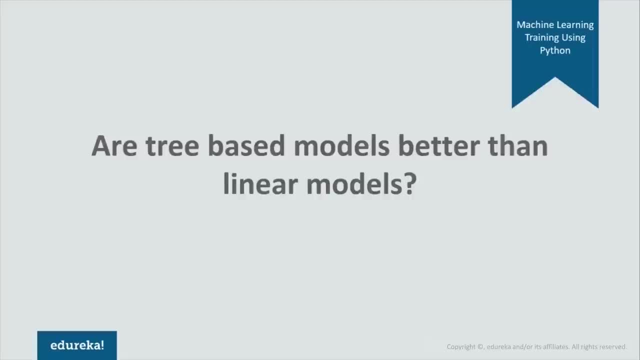 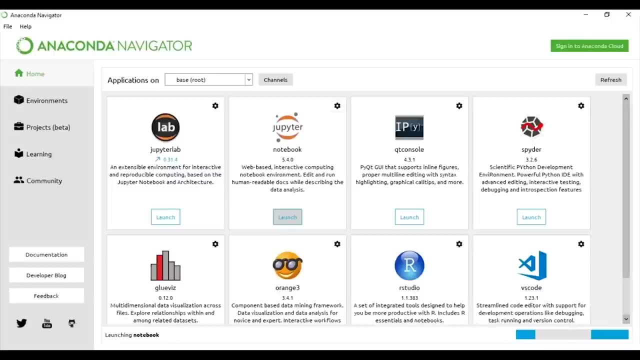 alright, so let's open the anaconda and the Jupiter notebook. where is that? so there's an anaconda navigator and I'll directly jump over to Jupiter notebook and hit the launch button. I guess everyone knows that Jupiter notebook is a web-based interactive computing notebook environment. 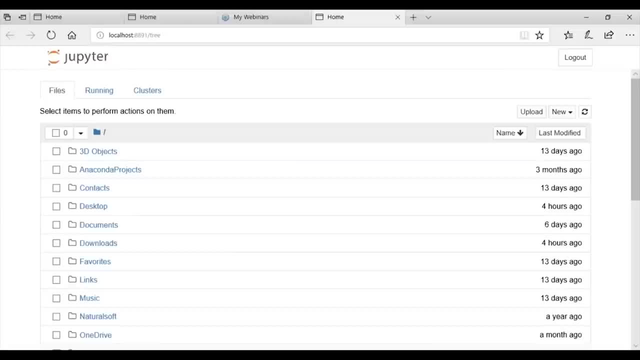 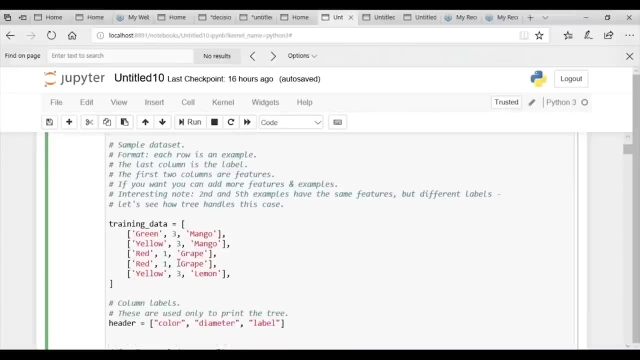 where you can run your Python codes. so my Jupiter notebook. it opens on my local host double eight nine one. so I'll be using this Jupiter notebook in order to write my decision tree classifier using Python. for this decision tree classifier, I have already written the set of codes. 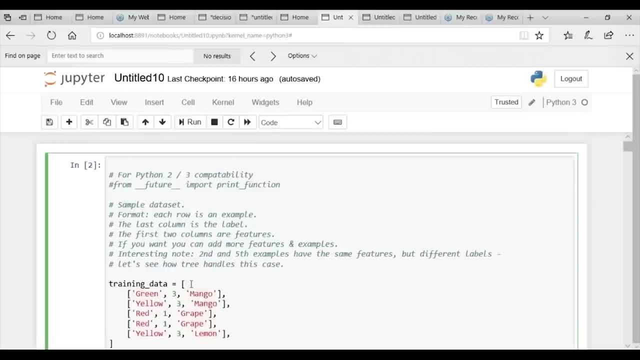 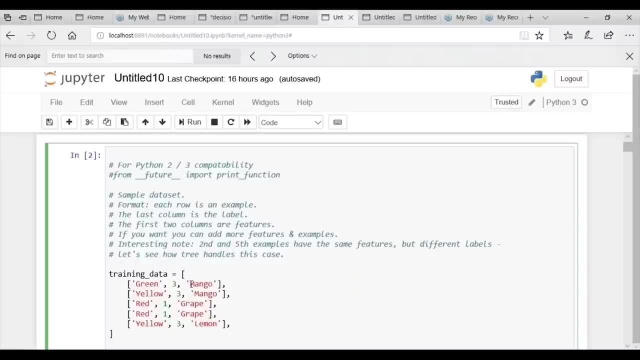 let me explain you just one by one. so we'll start with initializing our training data set. so there's a sample data set for which each row is an example. the last column is a label and the first two columns are the features. if you want, you can add. 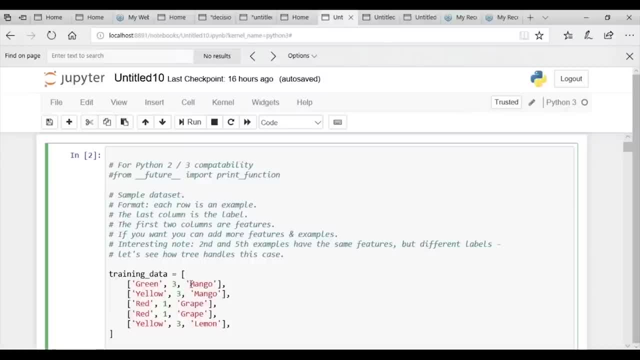 some more features and example for your practice. interesting fact is that this data set is designed in a way that the second and the fifth example have almost the same features, but they have different labels. alright, this tree handles this case, as you can see here, both of them. 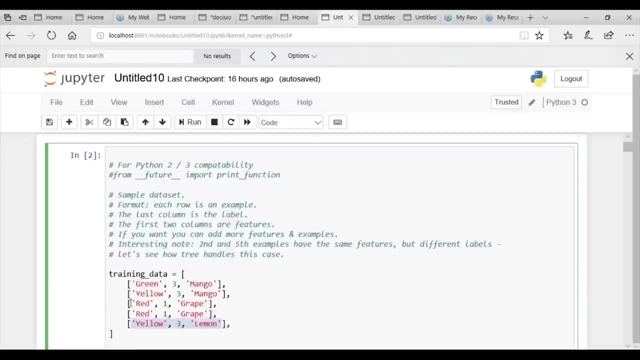 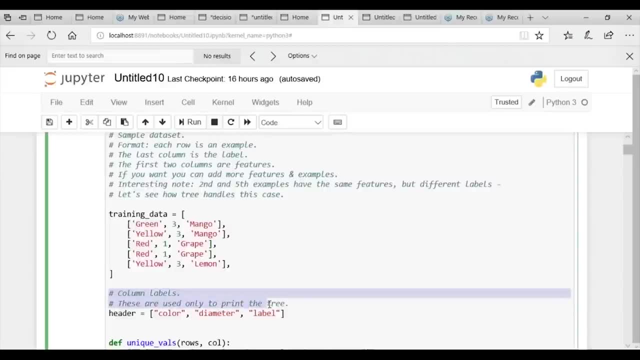 the second and the fifth column have the same features. what the different is? just their label, right. so let's move ahead. so this is our training data set. next, what we are doing: we are adding some column labels so they are used only to print the trees. fine, 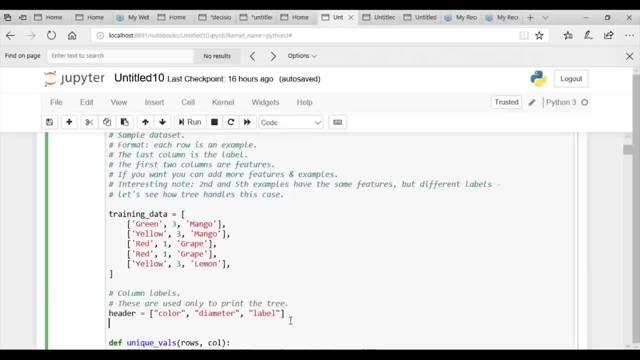 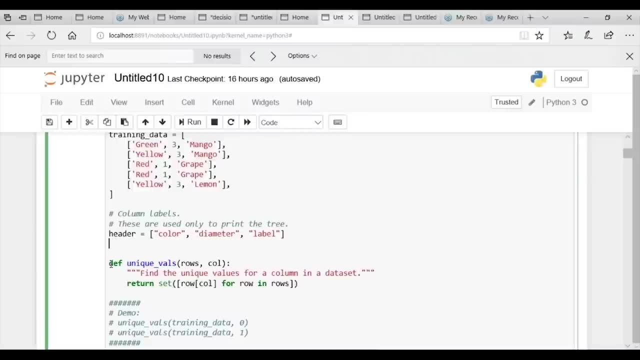 so what we'll do, we'll add header to the columns, like the first column is of color, second is of diameter and third is a label column. alright, next, what we'll do? we'll define a function as unique values, in which we'll pass the rows. so this function. 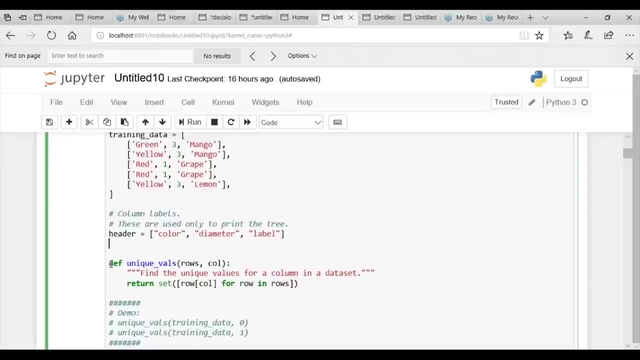 what it will do: it will find the unique values for a column in the data set. so there's an example for that. so what we are doing here: we are passing training data as our row and column number as 0. so what we are doing? we are finding. 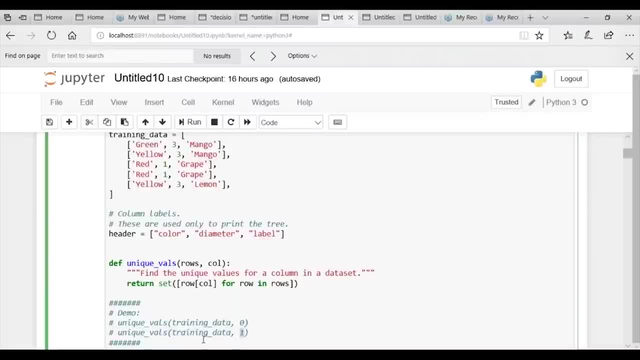 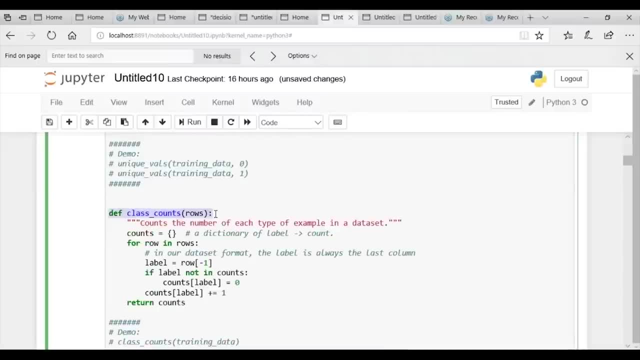 unique values in terms of color and in this, since the row is training data and the column is one. so what we are doing here? so we are finding the unique values in terms of diameter fine. so this is just an example. so what it does, it counts the number. 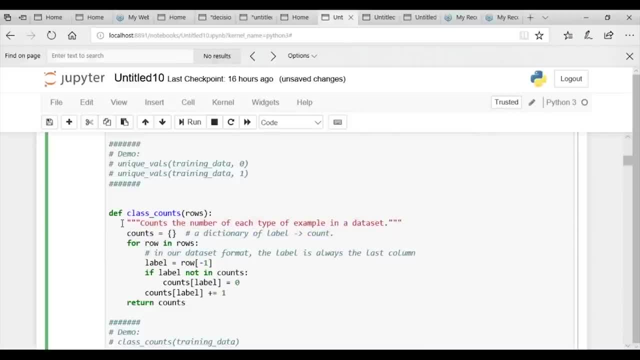 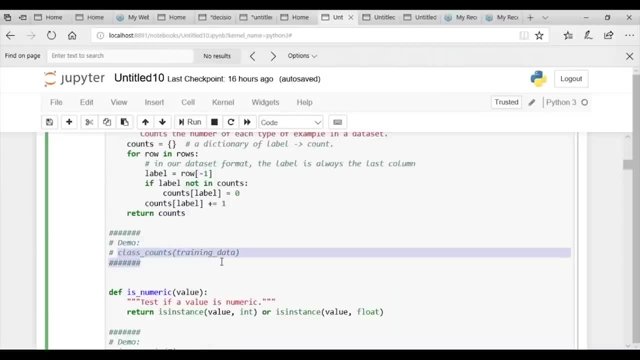 of each type of example within data set. so in this function, what we are basically doing, we are counting the number of each type, for example, in the data set, or what we are doing we are counting the unique values for the label in the data set as a sample. 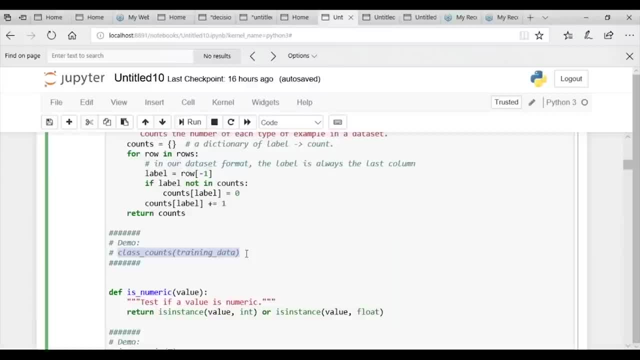 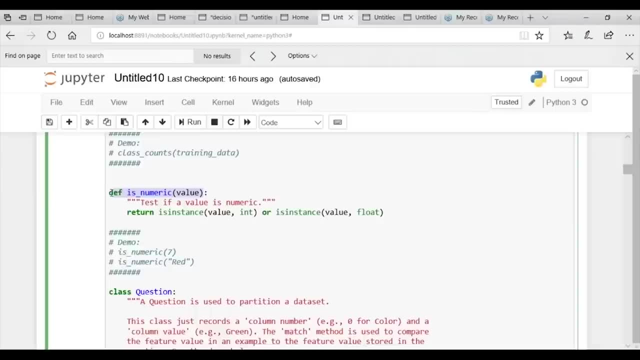 you can see here, we can pass that entire training data set to this particular function as class underscore count. what it will do? it will find all the different types of label within the training data set. as you can see here, the unique label in this function is numeric. 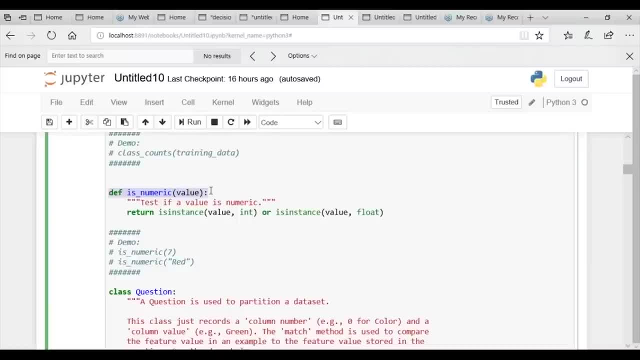 and will pass a value into it. so what it will do? it will just test if the value is numeric or not and it will return if the value is an integer or a float, for example. you can see is numeric, we are passing 7, so it has an integer. 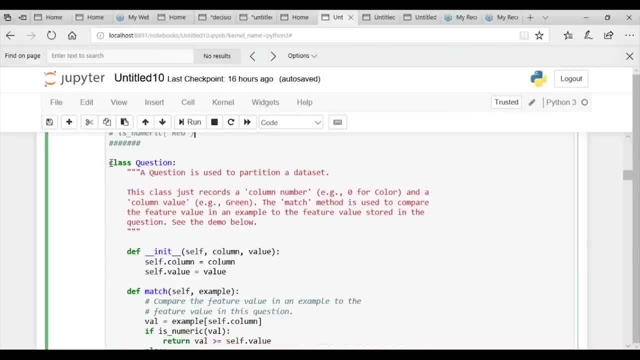 so it will return an int value and, if you are passing red, it's not a numeric value, right? so, moving on ahead, we'll define a class named as question. so what this question does. this question is used to partition the data set this class, what it does. 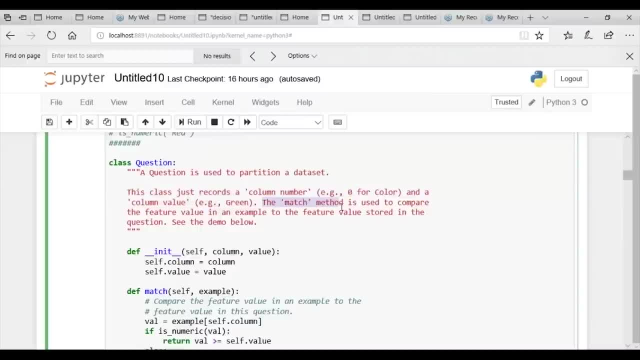 it will define a parameter for color- alright- and a column value, for example, green. next, what we are doing? we are defining a match method which is used to compare the feature value in the example to the feature value stored in the question. let's see how. first of all, 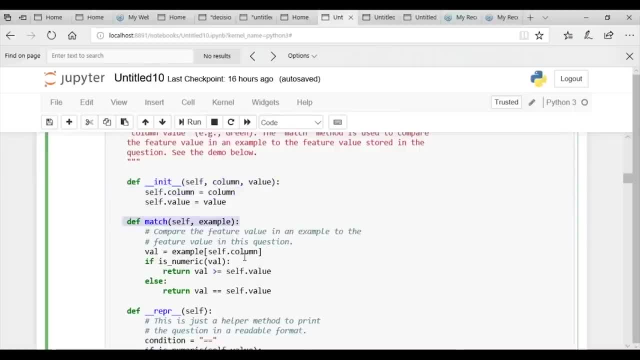 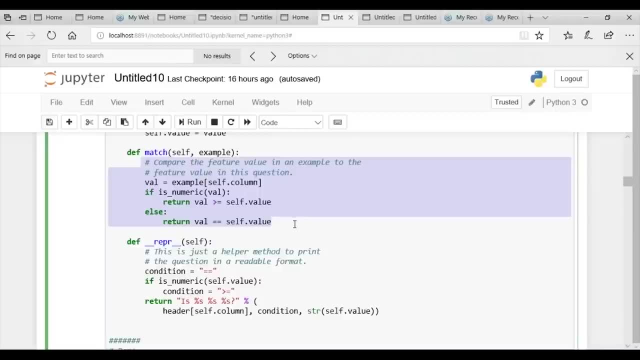 what we are doing. we are defining an init function and inside that we are passing the self column and the value as parameter. so next, what we do, we define a function as match what it does. it compares the feature value in an example, which is just a helper method. 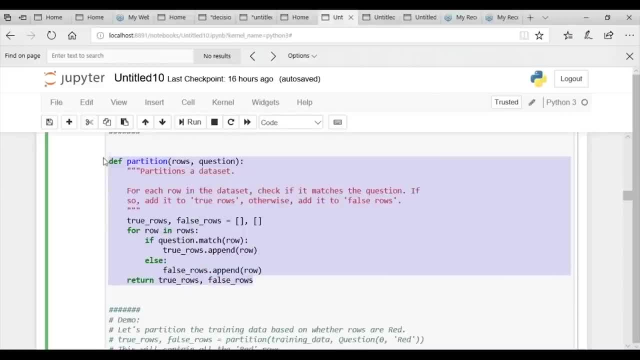 to print the question in a readable format. next, what we are doing? we are defining a function partition. well, this function is used to partition the data set. each row in the data set. it checks if it matches the question or not. if it does so, it adds it. 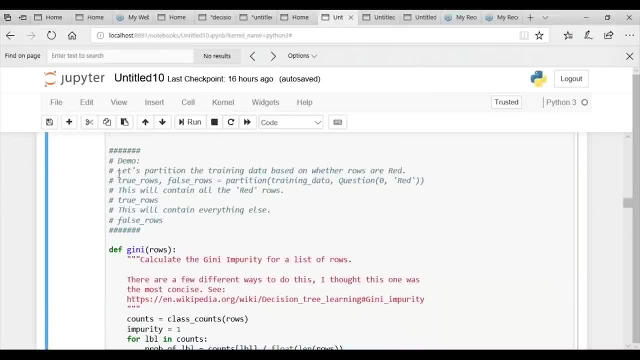 to the true rows or if not, then it adds to the false rows. alright, for example, as you can see here, let's partition the training data set based on whether the rows are red or not. here we are calling the function question. it will assign all the red rows. 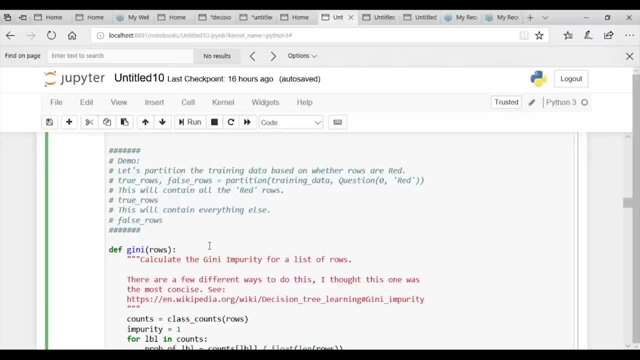 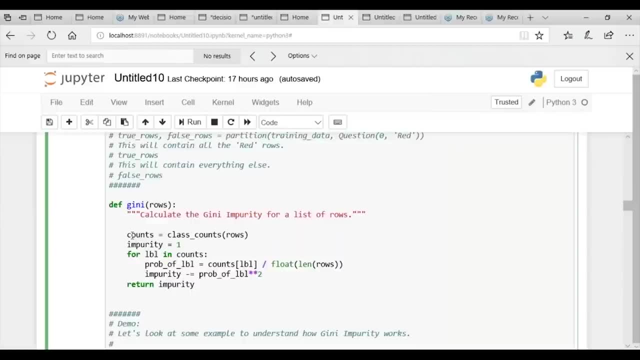 to true underscore rows and everything else will be assigned to false underscore rows. fine, next, what we will do, we will define a geny impurity function and inside that we will pass the list of rows. so what it will do, it will just calculate the geny impurity. 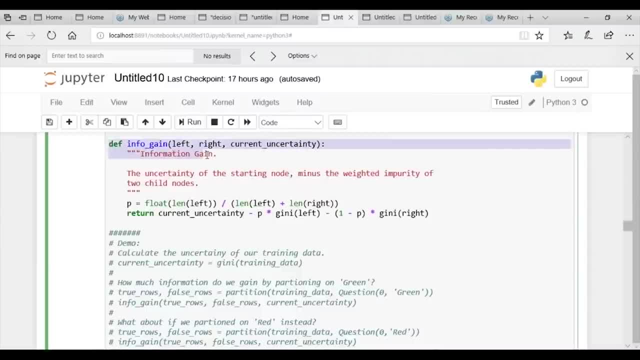 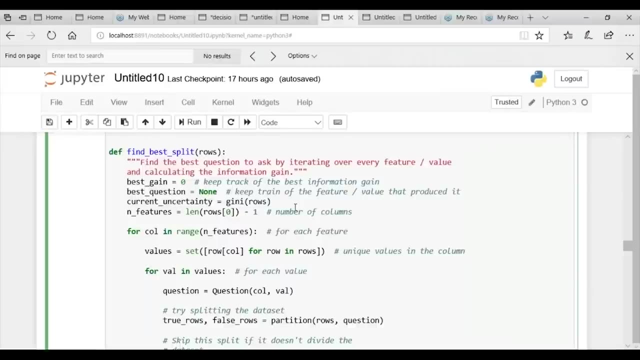 for the list of rows. next, what we are doing here? we are defining a function as information gain. so what this information gain function does? it calculates the information gain using the uncertainty of the starting node minus the weighted of the child node. the next function is find the best split. 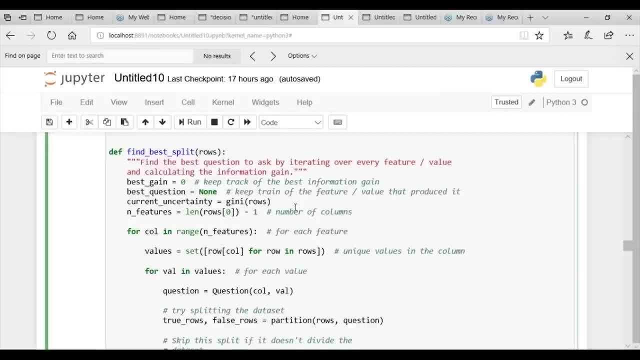 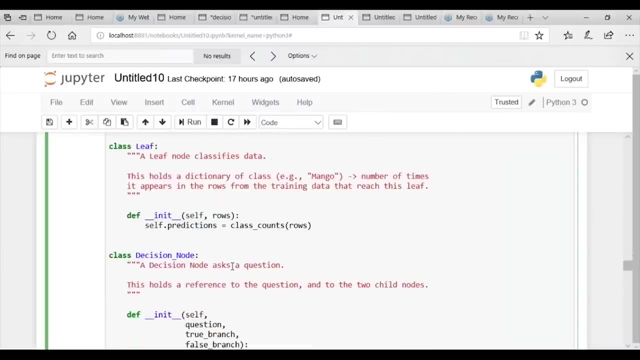 well, this function is used to find the best question to ask by iterating over every feature or value and then calculating the information gain. for the detail explanation on the code, you can find the code in the description given below. alright, next we will define a class as leaf. 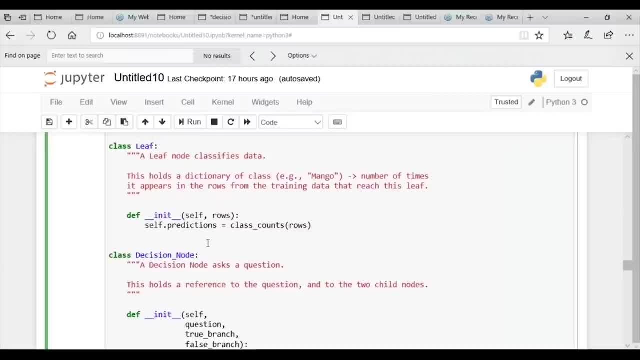 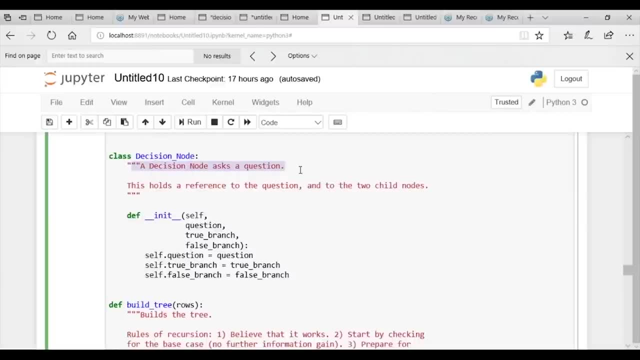 for classifying the data. it holds a dictionary of class like mango. for how many times it appears in the row? so this decision node, it will ask a question. this holds a reference to the question and the two child nodes. on the basis of it, you are deciding. 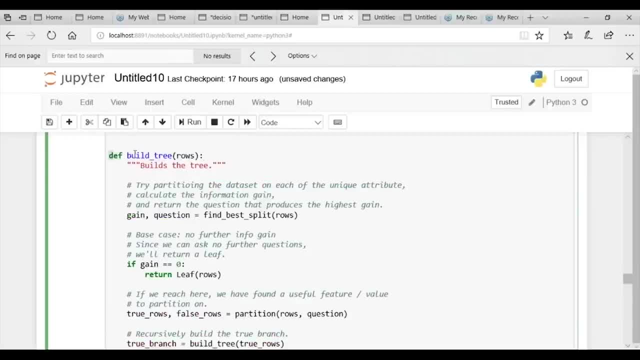 which node to add further to which branch. alright, so next, what we are doing, we are defining a function of build tree and inside that we are passing our number of rows. so this is the function that is used to build a tree. so, initially, what we did, we defined 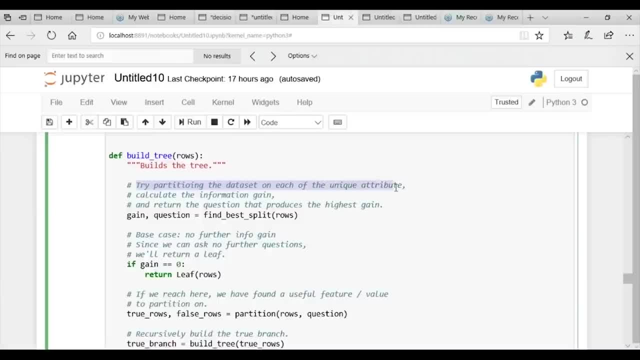 all the various function that we will be using in order to build a tree. so what we are doing here, we are partitioning the data set, calculating the information gain, and then what this is returning? it is returning the question that is, producing the highest gain. alright, now 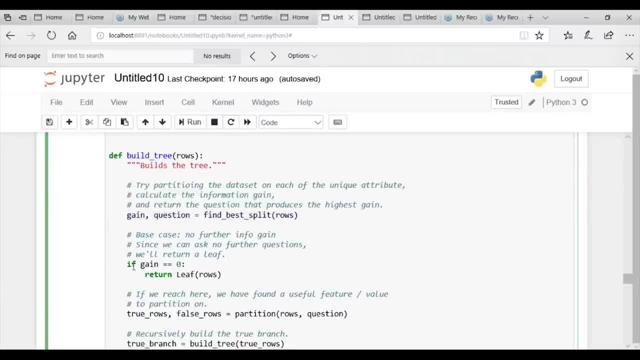 if gain equals zero, return leaf rows. so what it will do? so if we are getting no for the gain, that is, gain equals zero, then in that case, since no further question could be asked, so what it will do is so what it will do: it will return. 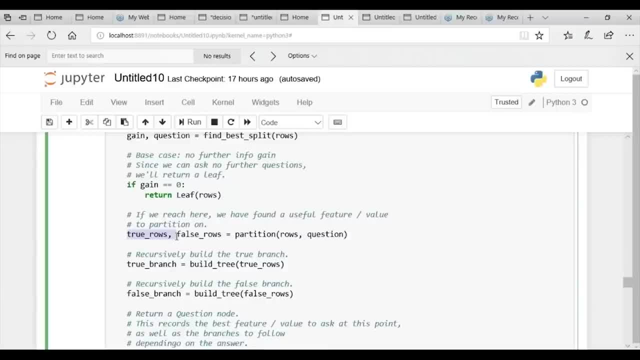 a leaf. fine now, true underscore rows or false underscore rows, equal partition with rows, and the question. so if we are reaching till this position, then you have already found a feature or value which will be used to partition the data set. then what you will do, you will recursively. 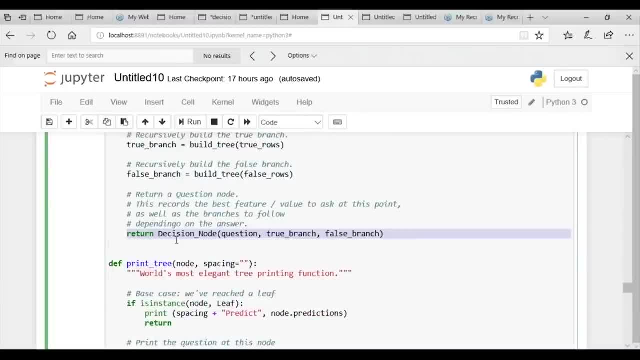 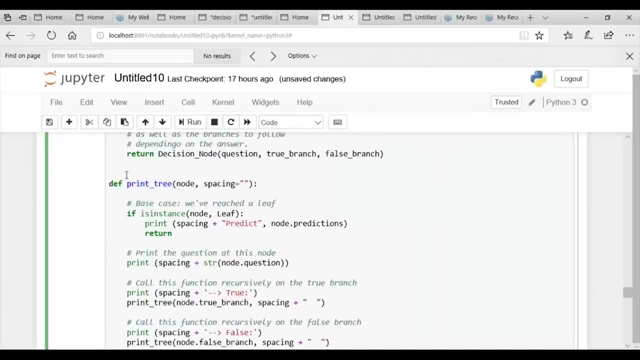 build the true branch and similarly recursively build the false branch. so return decision underscore node and inside that will be passing question: true branch node. now this question node. this records the best feature or the value to ask at this point. fine, now that we have built our tree. 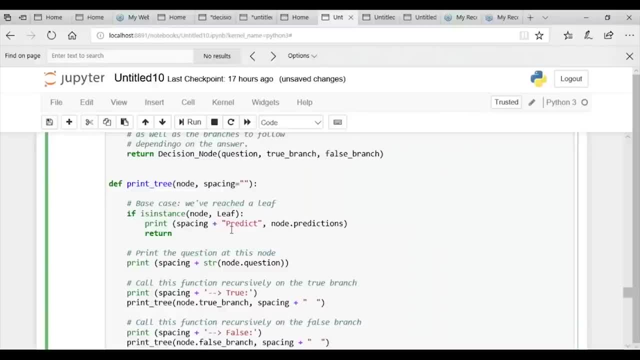 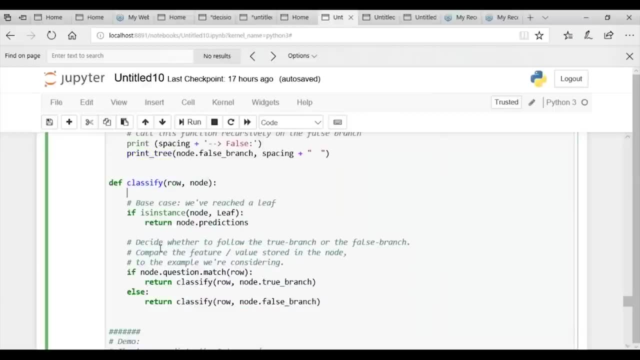 next, what we will do, we will define a print underscore tree function which will be used to print the tree. fine, so, finally, what we are doing in this particular function that we are printing our tree next is the classify function, which will use it to decide whether to follow the true branch. 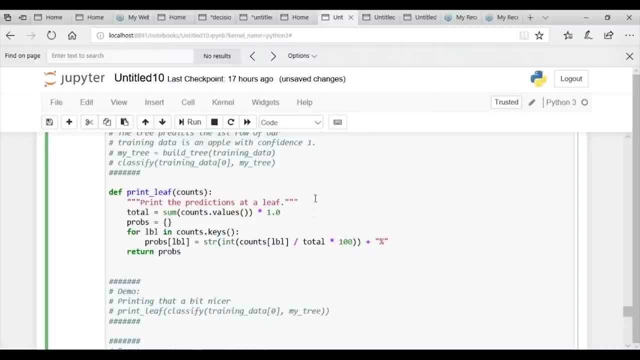 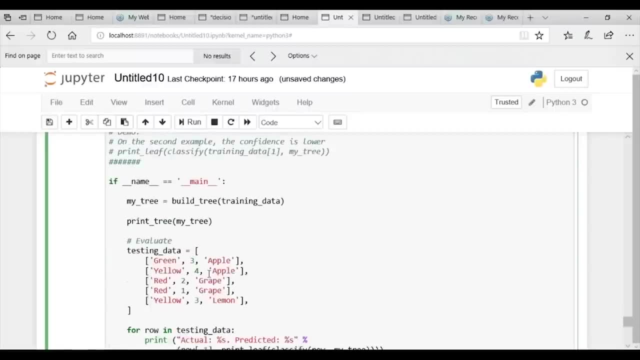 or the false branch, and then compare to the feature of values stored in the node to the example, and finally print the prediction and leave. so let's execute it and see. okay, so this is our testing data. all right, so we printed our leaf as well. now that we have 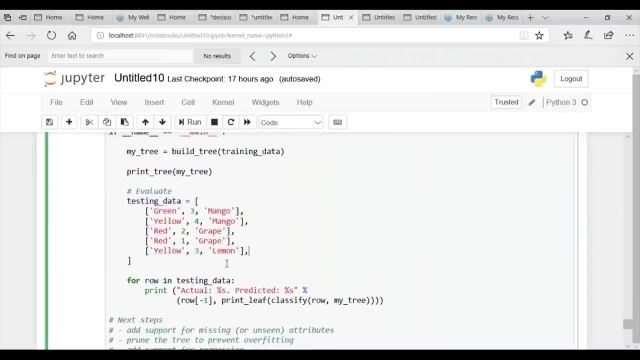 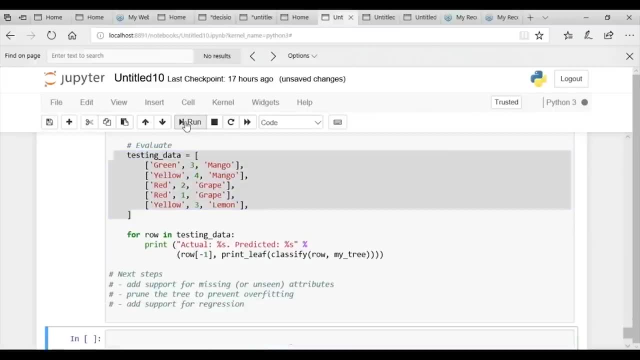 trained our algorithm with our training data set. now it's time to test it. so this is our testing data set. so let's finally execute it and see what is the result. so this is the result you will get. so first question which is asked by the algorithm: 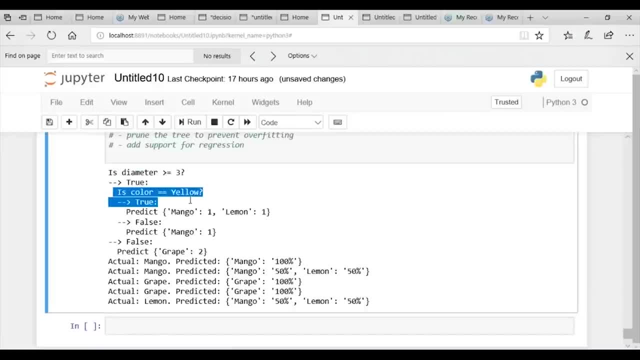 is is diameter greater than equal to 3? if it is true, then it will further ask if the color is yellow again, if it is true, then it will predict mango as one and lemon with one. all right, and in case it is false, then it will just. 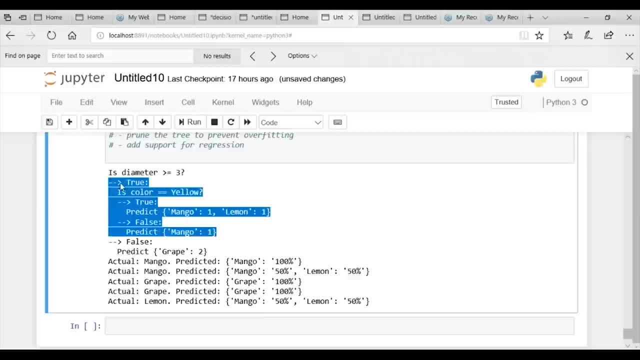 predict the mango. now, this was the true part. now next coming to: if diameter is not greater than or equal to 3, then in that case it's false and what it will do? it will just predict the grape. fine, okay, so this was all about the coding part. 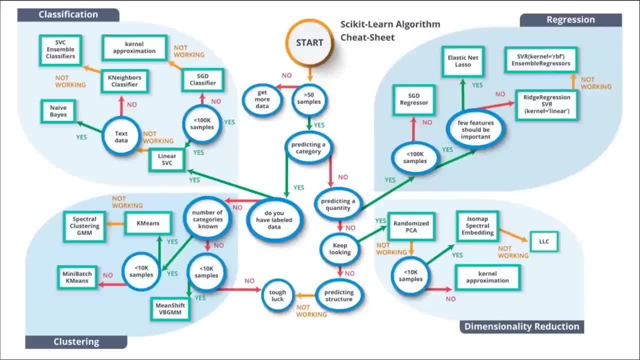 let me just show you one more thing. now there's a scikit-learn algorithm cheat sheet which explains you which algorithm you should use and when. all right, it's built in a decision tree format. let's see how it is built. so, first condition: it will check. 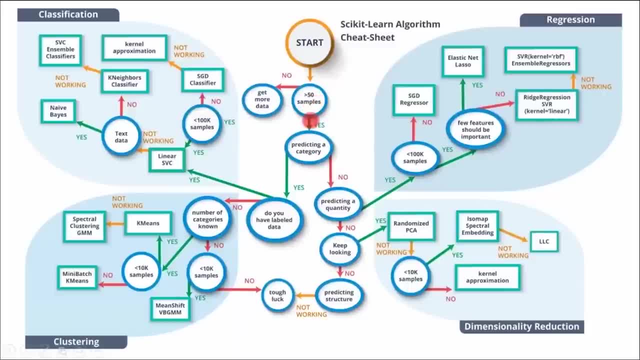 whether you have 50 samples or not. if your samples are greater than 50, then it will move ahead. if it is less than 50, then you need to collect more data. if your sample is greater than 50, then you have to decide whether you want to predict. 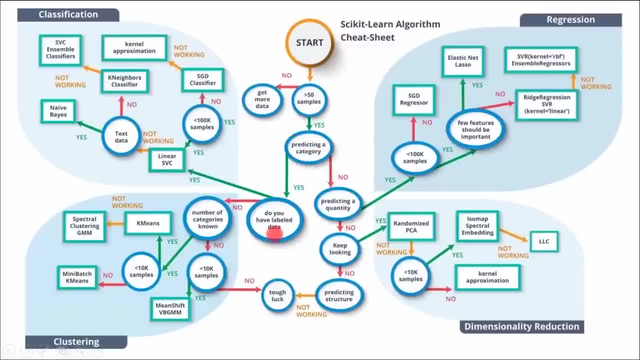 a category or not. if you want to predict a category, then further you will see that whether you have label data or not. if you have label data, then that would be a classification algorithm problem. if you don't have the label data, then it would be a clustering problem. 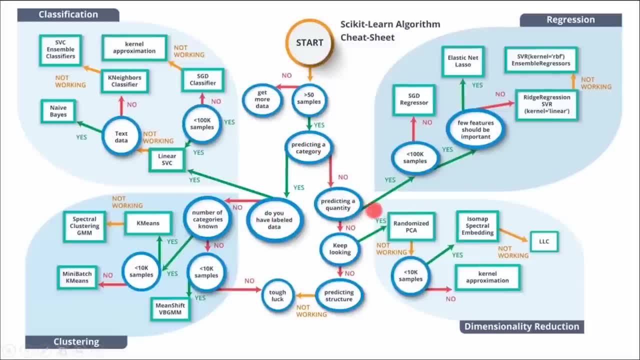 now, if you don't want to predict a category, then what do you want to predict? predict a quantity? well, if you want to predict a quantity, then in that case it would be a regression problem. if you don't want to predict a quantity and you want to keep, 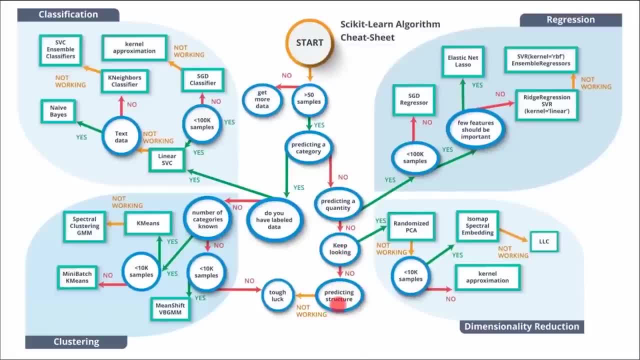 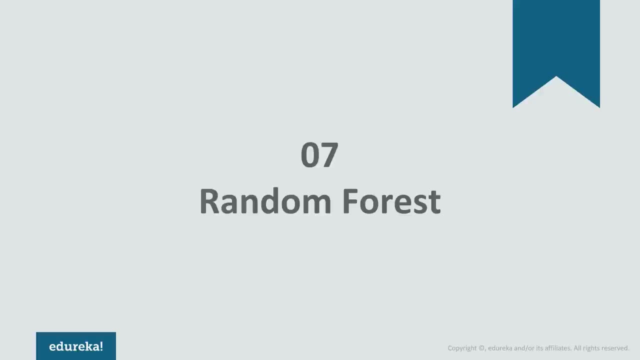 looking further, then in that case you should go for dimensionality reduction problems. and still, if you don't want to predict a quantity, then you should keep going. so let's go to the second part. I hope this decision tree session clarifies all your doubt over decision tree. 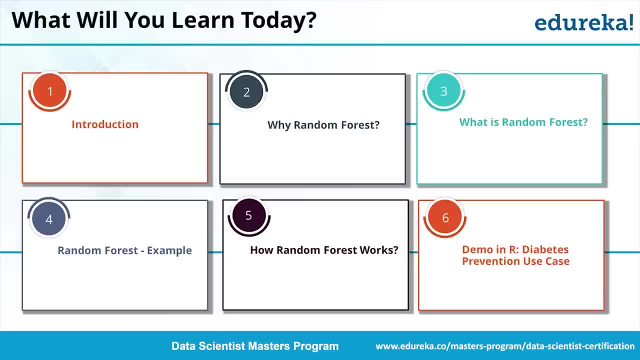 algorithm. let's begin this tutorial by looking at the topics that we'll be covering today. so first of all, we'll start away by getting a brief introduction of random forest and then we'll go as to So. once we understand its need at first place, then we'll go on to learn more about what is random forest and we'll also look at various fascinating examples of random forest so that we get a very clear understanding of it. 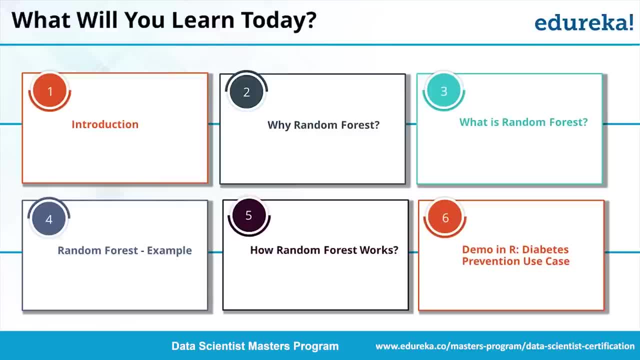 So further. we'll also delve inside into understand the working of random forest, as to how exactly random forest works. We'll also watch out the random forest algorithm step by step, right so that you're able to write any piece of code, any domain specific algorithm on your own. 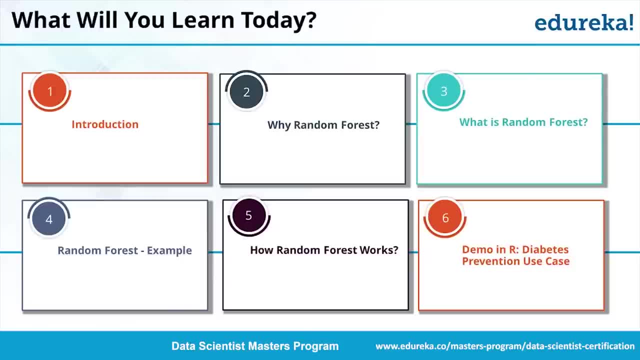 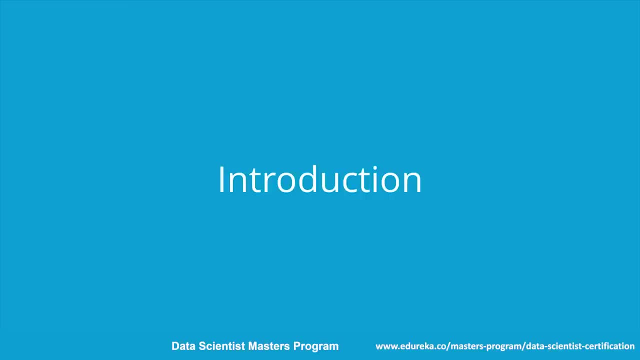 Now I personally believe that any learning is really incomplete if it's not put into application. So for its completion, we'll also. We'll also implement random forest in R with a very simple use case, that is diabetes prevention. So let's get started with the introduction then. 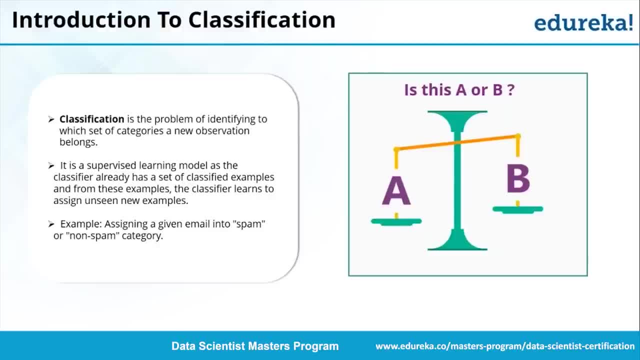 Now, random forest is actually one of the classifiers which is used for solving classification problems Now, since some of you might not be really aware of what classification is. so let's quickly understand classification first, and then we'll try to relate it to the random forest. 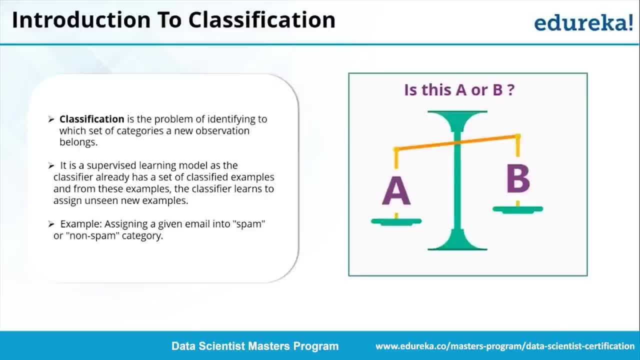 So basically, classification is a machine learning technique in which you already have predefined categories under which you can classify your data. So it's nothing but a supervised learning model where you already have a data based on which you can train your machine right, So your machine actually learns from this data. 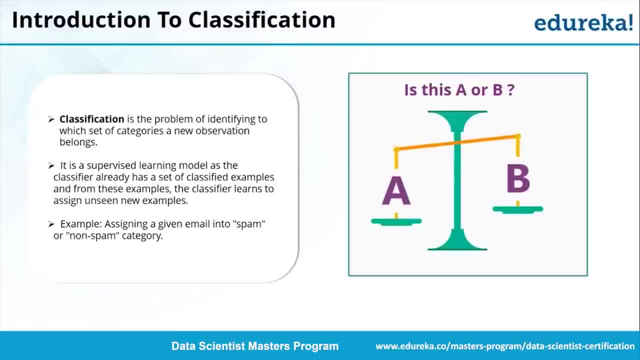 So, whatever all that predefined data that you already have, it actually works as a fuel for your machine, right? So let's say, for an example, ever wondered how your Gmail gets to know about the spam emails and filters it out from the rest of the genuine emails? any guesses? all right, I 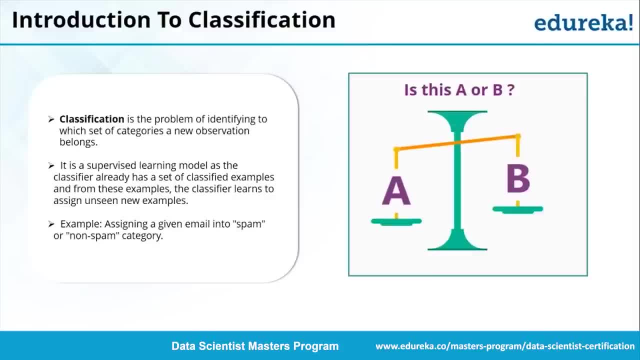 will give you a hint. try to think something on the line that: what would it actually look for? what can be the possible parameters based on which you can decide, or read: this is a genuine email or this is a spam email. so there are certain parameters that your classifier will actually look for, like 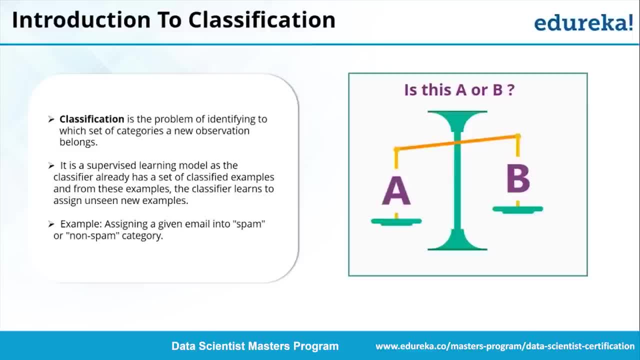 the subject line or the text or the HTML tags and also the IP address of the source. from where is this mail getting from? so it will analyze all these variables and then it will classify them into this spam or the genuine folder. so let's say, for an example, if your subject line states like mad or cute or pretty, 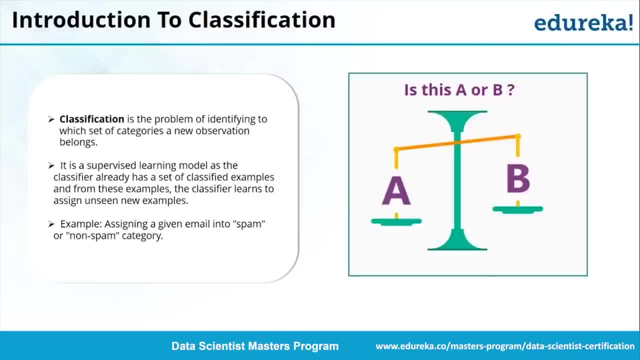 and some other absurd keywords. your classifier is smart enough and it's trained in such a manner that it will get to know: all right, this is a spam email, and it will automatically filter it out from your genuine emails. so that is how your classifier works, basically. so that's pretty much about the classification now. 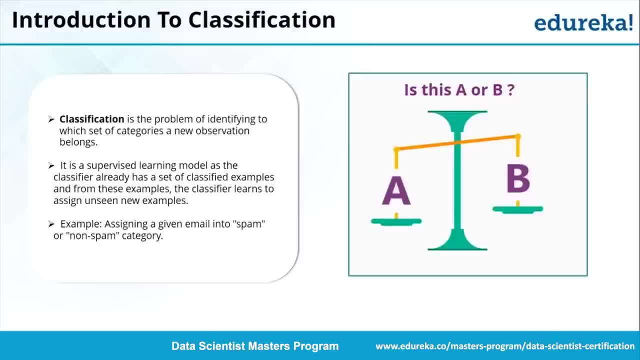 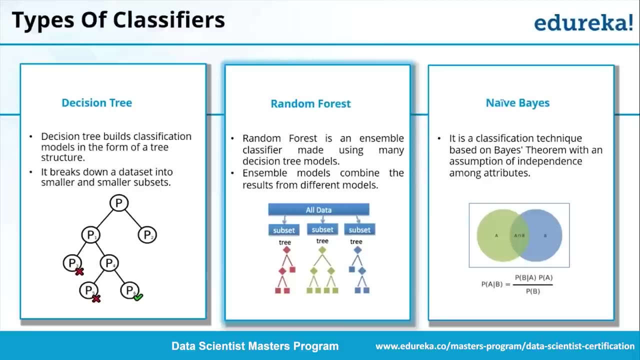 let's move forward and see what all ways can be there through which you can actually perform classification. so we have three classifiers, namely decision tree, random forest and name base. right, so speaking briefly about decision tree at first. so decision tree actually splits your entire data set in this structure. 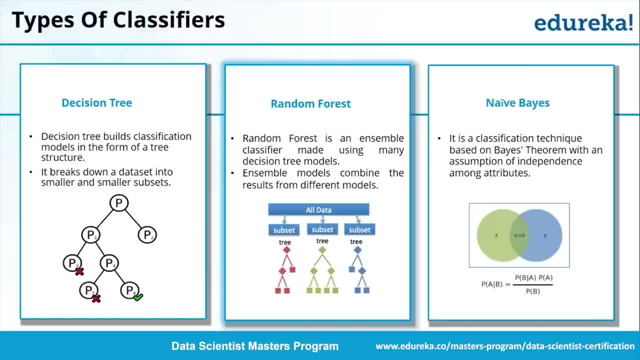 of a tree and it makes decision at every node and hence called decision tree. so no big bang theory, right? so you have certain data set. there are certain nodes at each node. it will further split into the child nodes and at each node it will make a decision. 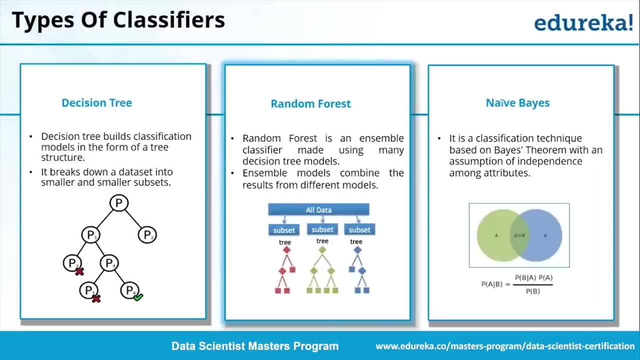 so final decision will be in the form of positive and negative right. so let's say, for an example, you want to purchase a car, right? so what wall will be the parameters? let's say, I go and I want to purchase a car and I will keep certain. 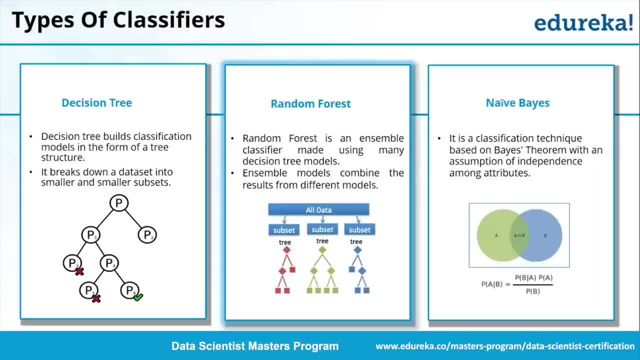 parameters. in my mind, that would be: what exactly is my income, what is my budget, what is the particular brand that I want to go for, what is the mileage of the car, what is the wedding number, what is the break-in? properly and finally, in a form of aprogram or visa right. so the final decision will be in the form of positive and 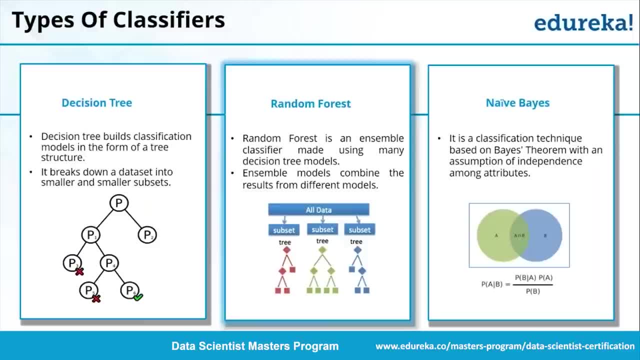 capacity of the car and so and so forth, right, so I made my decision based on all these parameters, right? and that is how you make decisions. and further, if you really want to know more about decision tree as to how it exactly works, you can also check out our decision tree tutorial as well. so let's begin now to 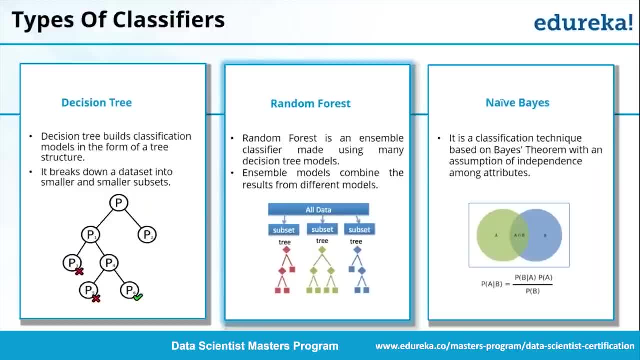 the random forest now. so random forest is an ensemble classifier actually. now let's understand what this word ensemble means. so ensemble methods actually use multiple machine learning algorithms to obtain better predictive performance. so, particularly talking about random forest, so random forest uses multiple decision trees for prediction, right? so you are assembling a lot of decision trees to. 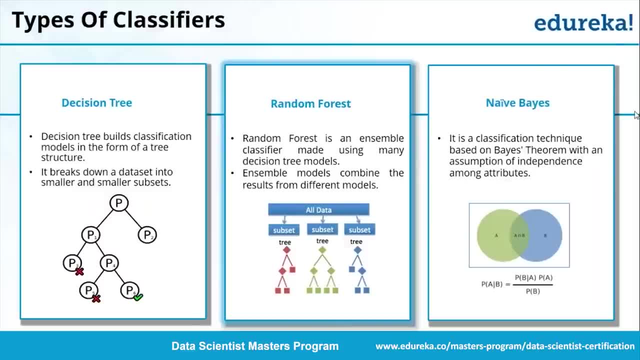 come up to your final outcome, as you can also look here in the image that your entire data set is actually further split into three subsets, right, and each subset further leads to a particular decision tree. so here you have three decision trees and each decision tree will lead to a certain 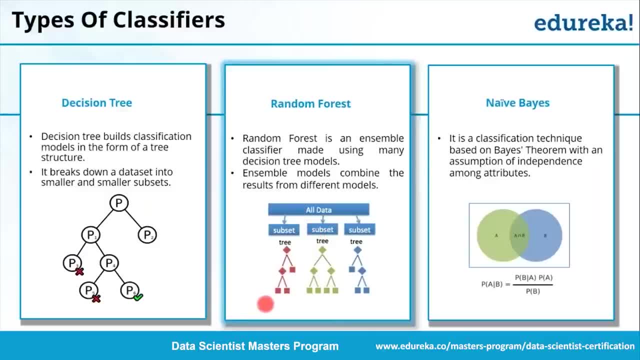 outcome. now, what random forest will do is it will compile the results from all the decision trees and then it will lead to a final outcome. right, so it's compilation of all the multiple decision trees. that's all about the random forest. now let's see what lies there in naive base. 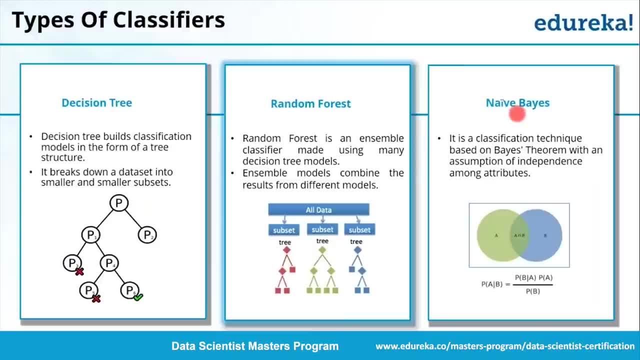 right. so naive base is very famous classifier which is made on a very famous rule called Bayes theorem. you might have studied about naive Bayes theorem in your 10 standard as well, so let's just see what Bayes theorem describes. so Bayes theorem actually describes the probability of an event based on certain prior. 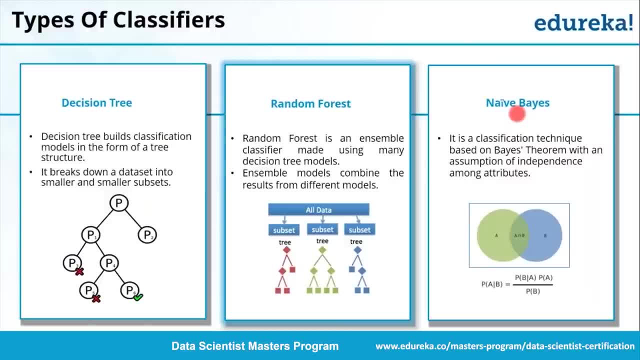 knowledge of conditions that might be related to the event, right? so, for example, if cancer is related to age, right. so then person's age can be used to more accurately assess probability of having the cancer than without having the knowledge of age. so if you know the age then it will become handy in. 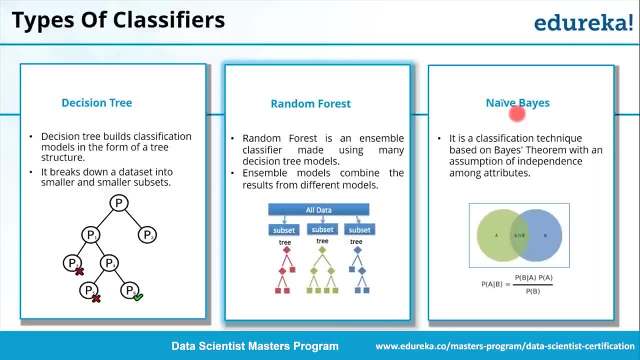 predicting the occurrence of cancer for a particular person, right? so the outcome of first event is is actually affecting your final outcome, isn't it? yeah, so this is how naive base classifier actually works. so that was all to give an overview of naive base classifier and this all pretty much about the types of classifiers. now we'll 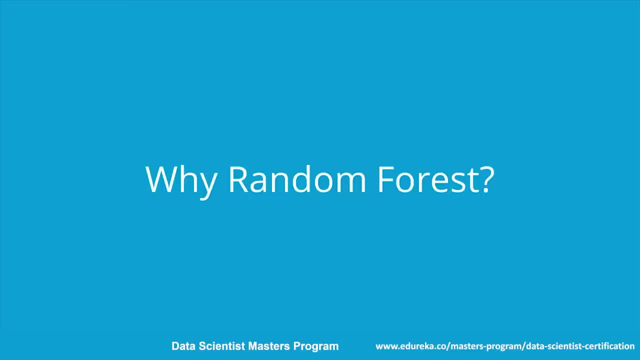 try to find out the answer to this particular question as to why we need random forest. fine, so, like human beings, learn from the past experiences, so, unlike human beings, a computer does not have experiences. then how does machine takes decisions? where does it learn from? well, a computer system actually learns. 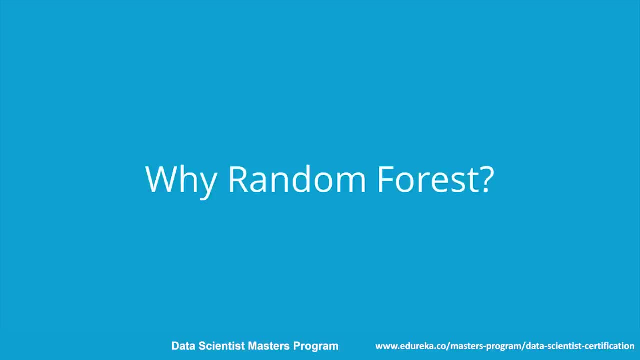 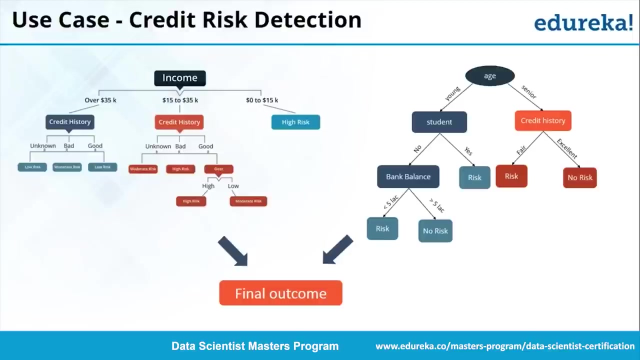 from the data, which represents some past experiences of an application domain. so now let's see how random forest helps in building up the learning model with a very simple use case of credit risk detection. Now, needless to say that credit card companies have a very nested interest. 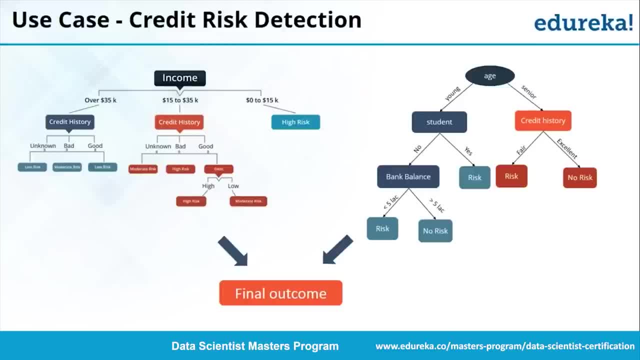 in identifying financial transactions that are illegitimate and criminal in nature. and also, I would like to mention this point- that, according to the Federal Reserve Payments Study, Americans used credit cards to pay for 26.2 billion purchases in 2012, and the estimated loss due to 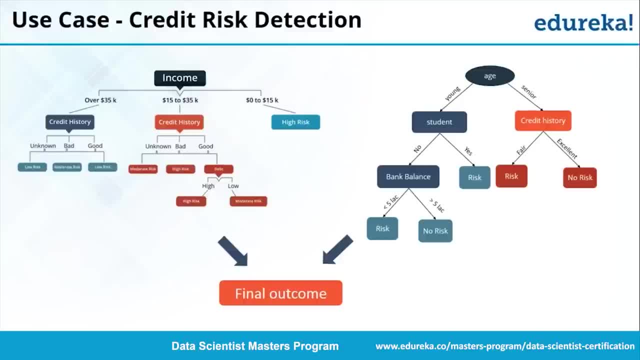 unauthorized transactions. that here was US 6.1 billion dollars. Now, in the banking industry, measuring risk is very critical because the stakes are too high. so the overall goal is actually to figure out who all can be fraudulent before too much financial damage has been done. So for this, 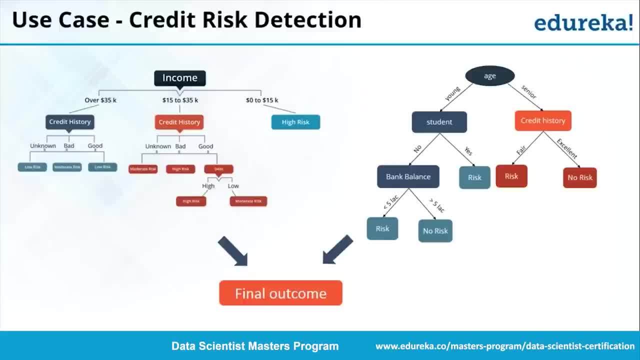 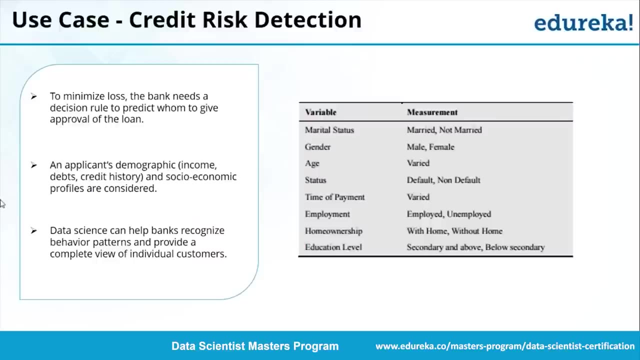 a credit card company receives thousands of applications for new cards, and each application contains information about an applicant Right. so so here as you can see that, from all those applications, what we can actually figure out is our predictor variables, like: what is the marital status of the person, what is the gender, 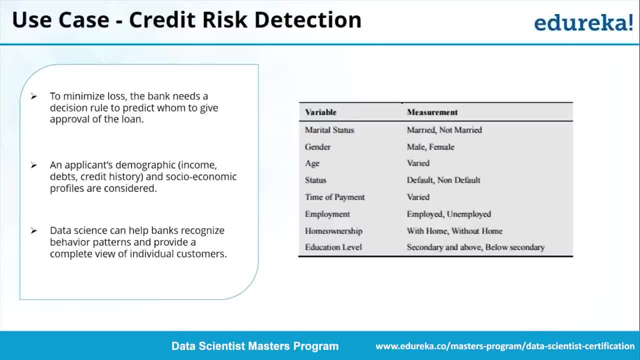 of the person, what is the age of the person and the status, which is actually whether it is a default pair or a non default pair. So default payments are basically when payments are not made in time and according to the agreement signed by the agreement. 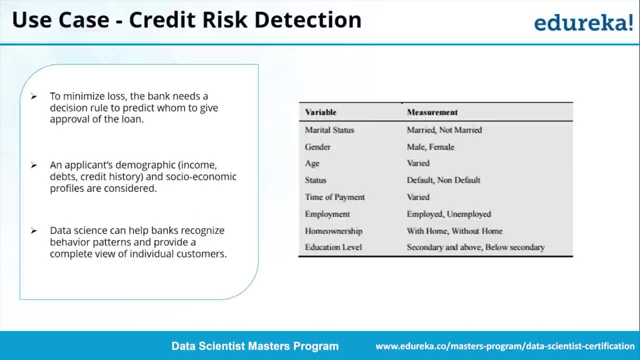 the card holder. so now that account is actually set to be in the default, so you can easily figure out the history of the particular card holder from this. then we can also look at the time of payment, whether he has been a regular payer or a non-regular one. what is the source of income? 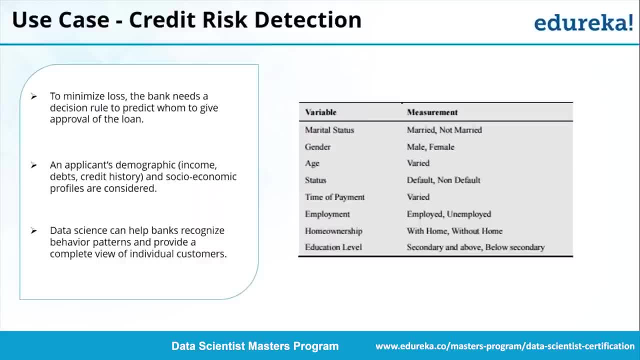 for that particular person and so and so forth. so to minimize loss, the bank actually needs certain decision rule to predict whether to approve a particular loan of that particular person or not. now, here is where the random forest actually comes into the picture right now. let's see how random forest can actually help us in this particular scenario. now we have 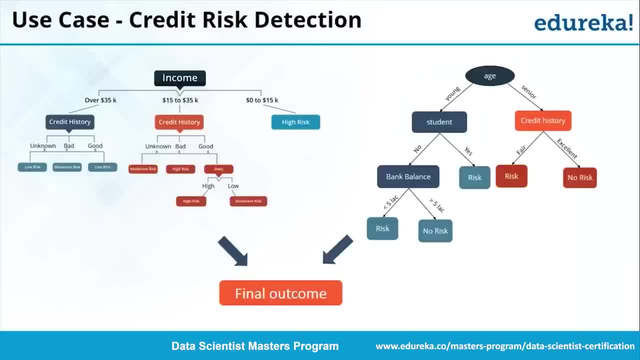 taken randomly two parameters out of all the predictive variables that we saw previously. now we have taken two predictive variables here. the first one is the income and the second one is the age right, and similarly, parallelly, two decision trees have been implemented upon those predicted variables. now let's first assume the case of the income variable. 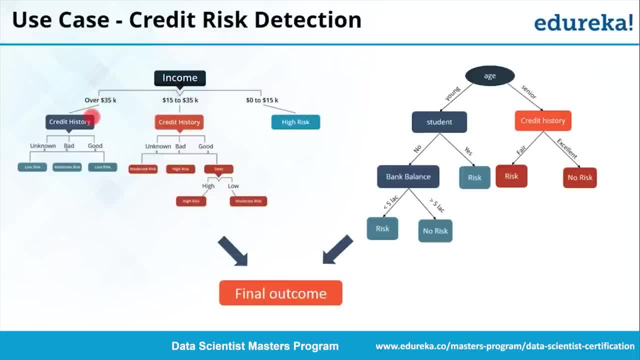 right. so here we have divided our income into three categories, the first one being the person earning over thirty five thousand dollars. second, from fifteen to thirty five thousand dollars. the third one earning in the range of zero to fifteen thousand dollars. now, if a person is earning over thirty five thousand dollars, which is a pretty good income, pretty decent. so now we'll. 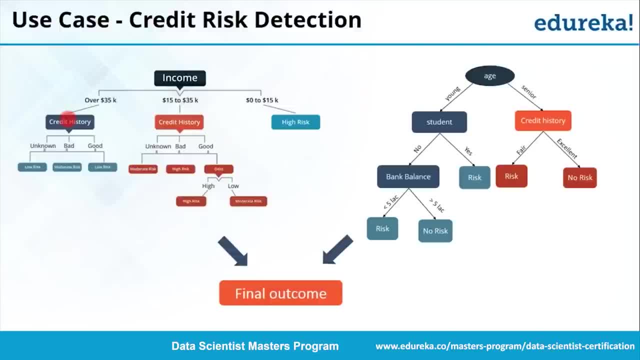 check out for the credit history. now here the probability is that if a person is earning a good amount, then there is very low risk that he won't be able to pay back already earning goods. so the probability is that his application of loan will get approved right. so there is actually low risk. 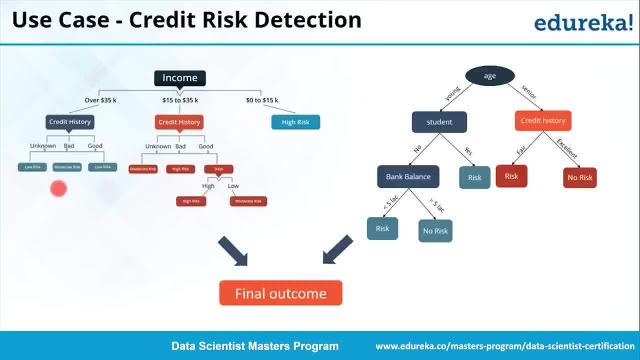 or moderate risk, but there's no real issue of higher risk as such. we can approve the applicant's request here. now let's move on and watch out for the second category, where the person is actually earning from fifteen to thirty five thousand dollars right now. here the person may or may not pay back. 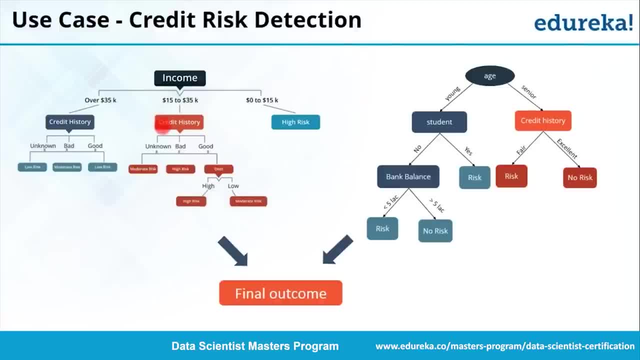 so in such scenarios we'll look for the credit history as to what has been his previous history. now, if his previous history has been bad, like he has been a defaulter in the previous transactions, we'll definitely not consider approving his request and he'll be at the 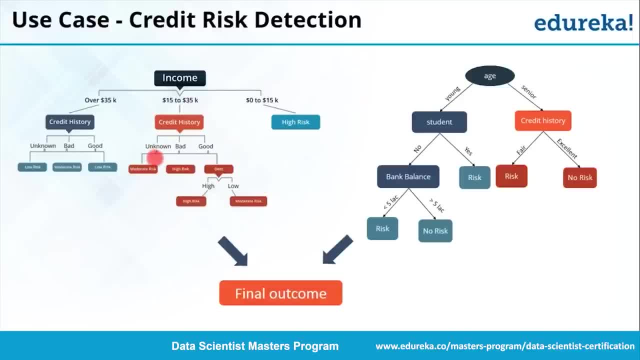 high risk end, which is not good for the bank. if the previous history of that particular applicant is really good, then we will. just to clarify our doubt, we'll consider another parameter as well, that will be our depth. now, if he's already in really high depth, then the risks again increases. 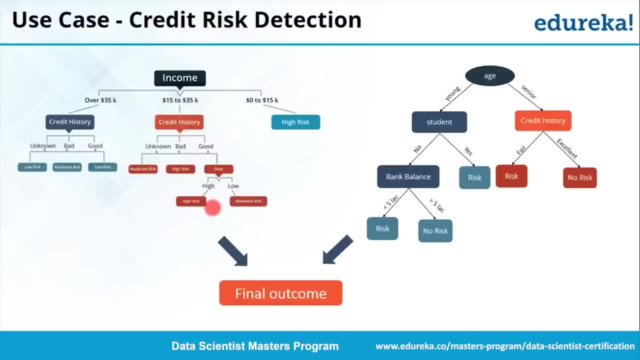 and there are chances that he might not change in the future. so here we'll not accept the request of the person having high depth. if the person is in the lower depth and he has been a good pair in his past history, then there are chances that he might pay back and we can consider approving the request of this particular applicant. now let's. 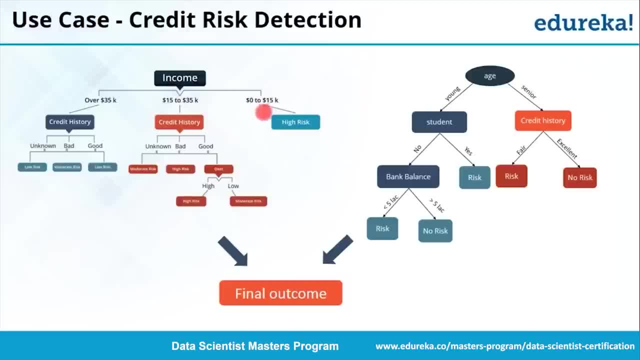 look at the third category, which is a person earning from zero to fifteen thousand dollars. now, this is something which actually raises i pro, and this person will actually lie in the category of high risk. all right, so the probability is that his application of loan will probably get rejected. 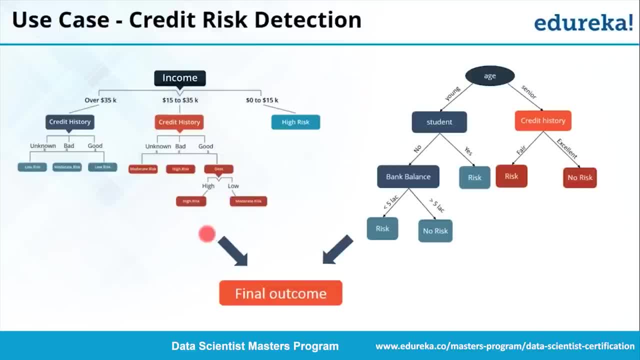 now we'll get one final outcome from this income parameter. right now, let us look at our second variable, that is, age, which will lead into the second decision tree. now let us say: if the person is young, right, so now we'll look forward to if it is a student. now, if it is a student, then the chances are high that he won't be able. 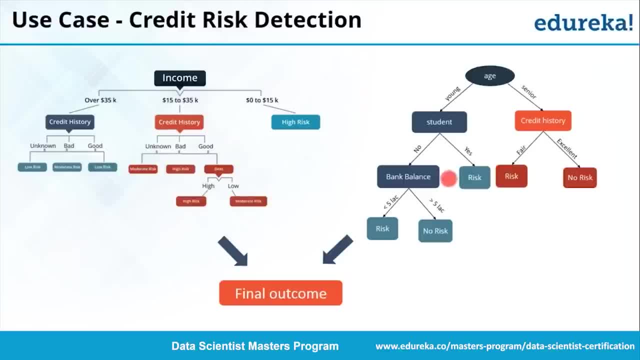 to repay back because he has no earning source right. so here the risks are too high and the probability is that his application of loan will get rejected. fine now, if the person is young and he's not a student, then we'll probably go on and look for another variable, that is, bank balance. 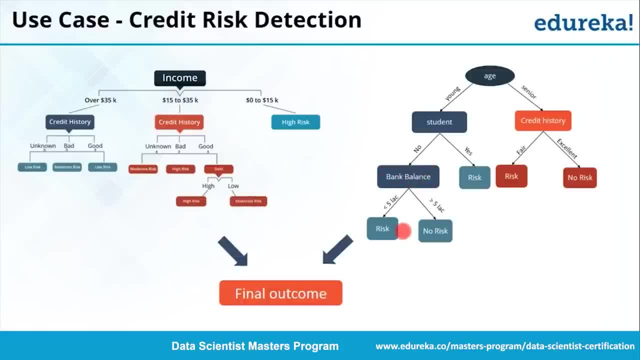 now let's look if the bank balance is less than five lakhs. so again, the risk arises and the probability is that his application of loan will get rejected. now, if the person is young, he's not a student and he has a bank balance of greater than five lakhs, 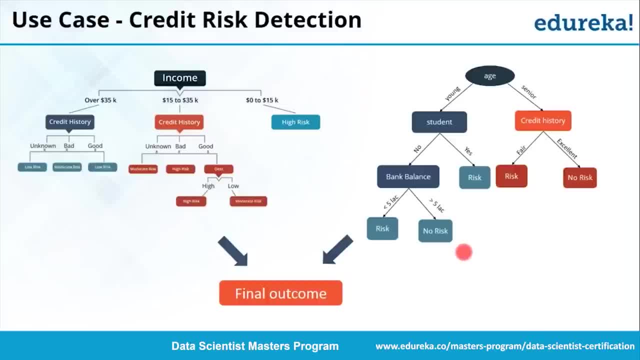 he's got a pretty good and stable bank balance, then the probability is that his own of application will get approved of now. let us take another scenario: if he's a senior, right? so if he's a senior, will probably go and check out for his credit history. how well has he been in his previous? 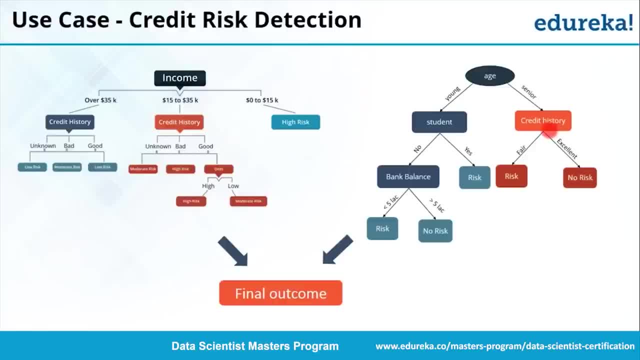 transactions, what kind of a person he is like, whether he is a defaulter or he is a non-defaulter. now, if he is a very fair kind of person in his previous transactions, then again the risk arises and the probability of his application getting rejected actually increases right now. if he has 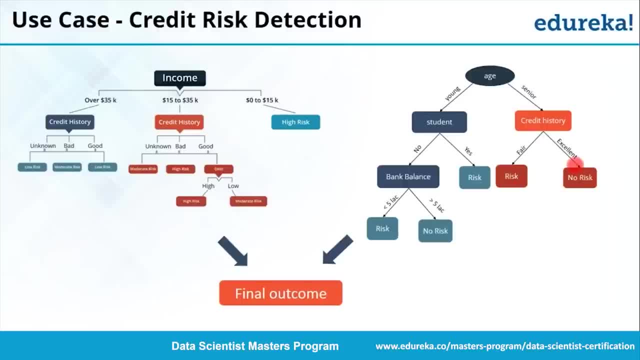 been an excellent person as per his transactions in the previous history. so now, again here, there is least risk and the probabilities that his application of loan will get approved. so now here. these two variables, income and age, have led to two different decision trees: right and these two. 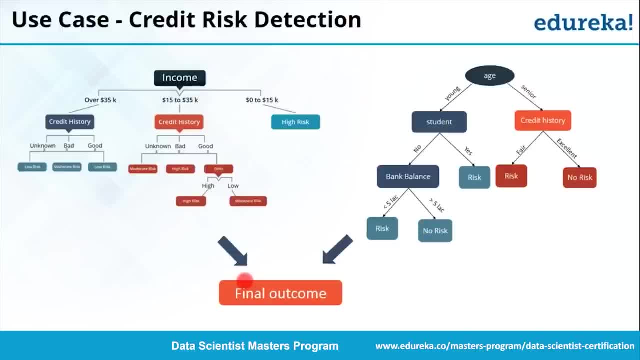 different decision trees actually led to two different results. now, what random forest does is it will actually compile these two different results from these two different decisions decision trees and then finally, it will lead to a final outcome. that is how random forest actually works right? so that is actually the motive of the random forest. 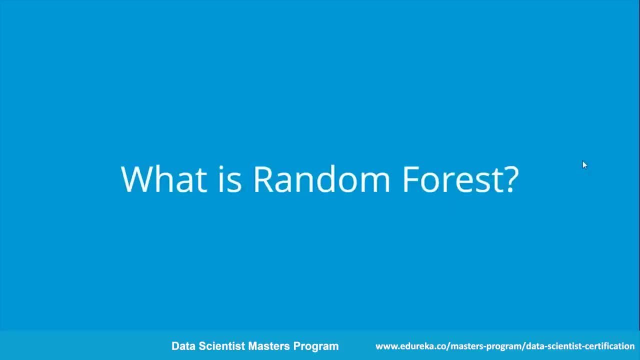 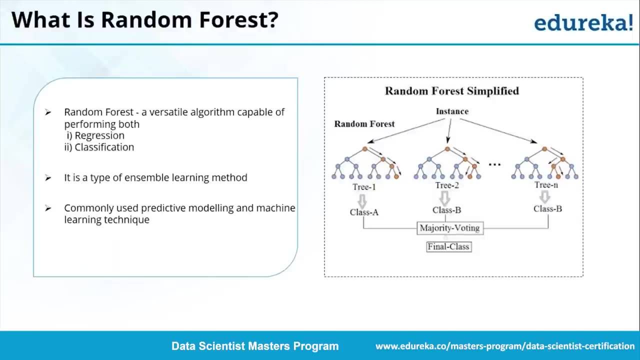 now let us move forward and see what is random forest. right, you can get an idea of the mechanism from the name itself: random forest. so a collection of trees is a forest. that's why called forest, probably, and here also the trees are actually- because being trained on subset. 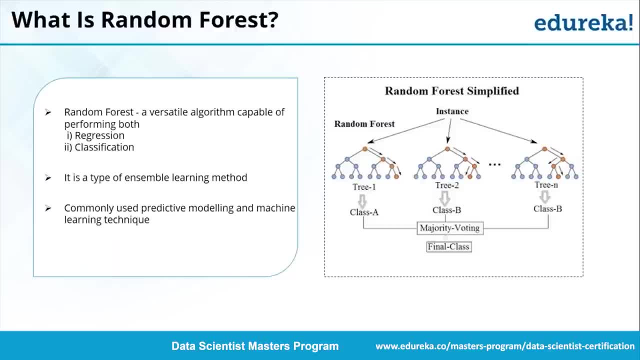 which are being selected at random, and therefore they are called random forests. so a random forest is a collection or an ensemble of decision trees. right here, a decision tree is actually built using the whole data set, considering all features, but actually in random forest only a fraction of the number of rows is selected, and that too at 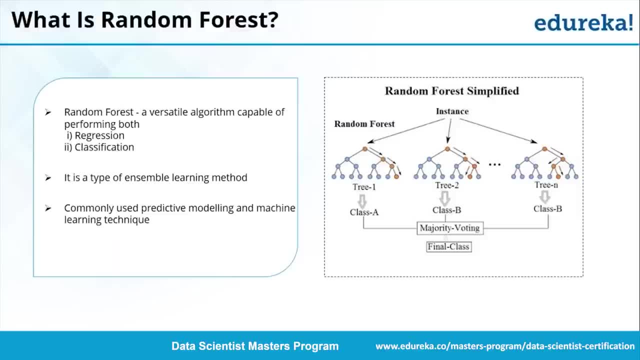 random and a particular number of features, which are actually selected at random, are trained upon. that is how the decision trees are built upon, right? so, similarly, a number of decision trees will be grown and each decision tree will result into a certain final outcome, and random forest will do nothing but actually just compile the results of all those decision trees to bring. 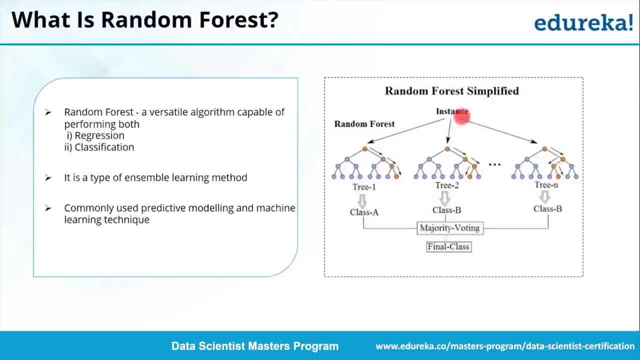 out the final result. as you can see in this particular figure that a particular instance actually has resulted into three different decision trees. right, so now, tree one results a final outcome called class a, and tree two results into class b. similarly, tree three results into class b. so random forest will compile the results of all these decision trees and it will 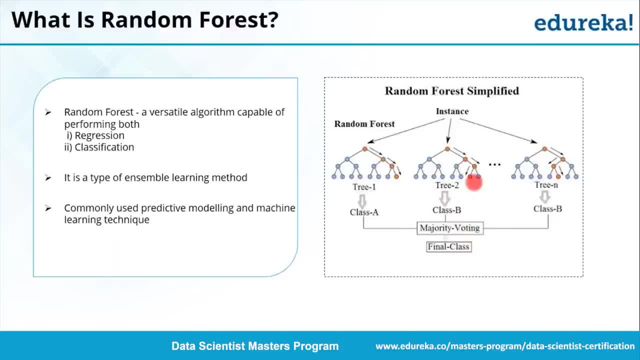 go by the call of the majority voting now, since here two decision trees have actually voted into the favor of the class b, that is, decision tree two and three. therefore, the final outcome will be in the favor of the class b. and that is how random forest actually works. upon now one really beautiful. 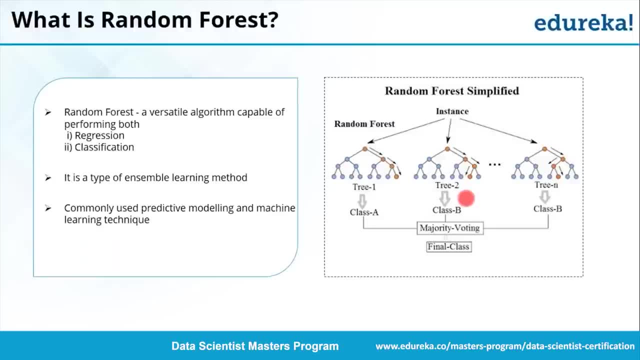 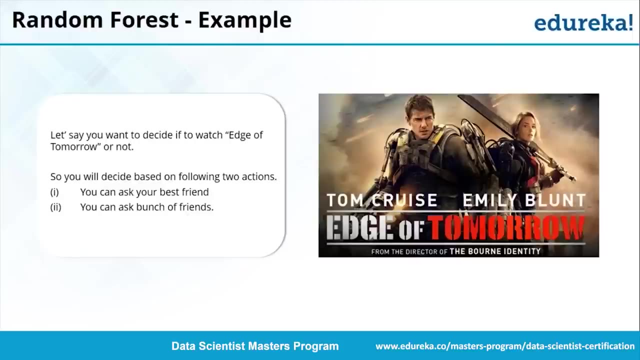 thing about this particular algorithm is that it is one of the versatile algorithms which is capable of performing both regression as well as classification. now let's try to understand random forest further with a very beautiful example. all right, this is my favorite one. so let's say: you want. 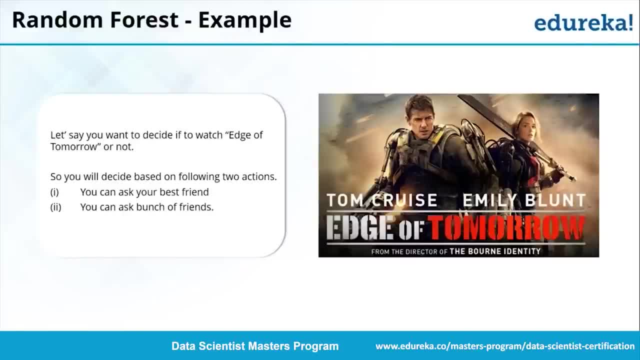 to decide if you want to watch edge of tomorrow or not, right? so in this particular scenario, you will have two different actions to take. in this particular scenario, you will have two different actions to work upon. either you can just straight away go to your best friend, ask him about all. 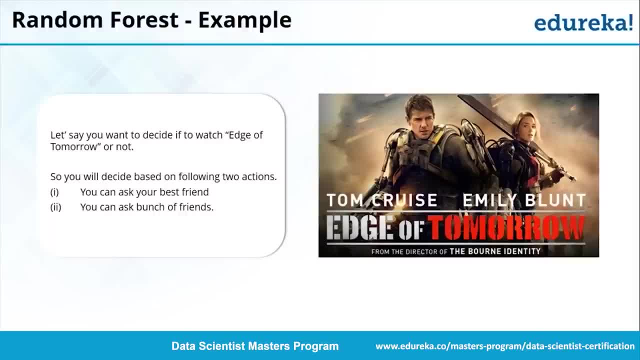 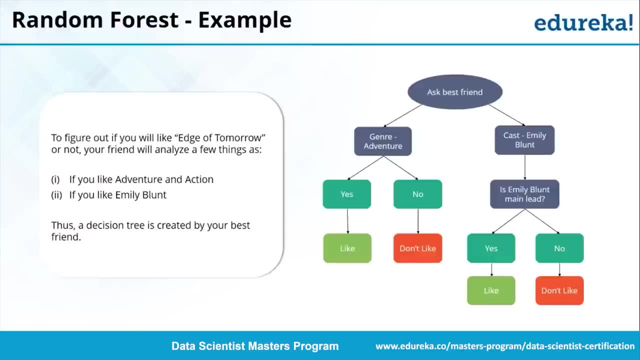 right, whether should i go for edge of tomorrow or not? will i like this movie? or you can ask a bunch of friends and take their opinion consideration and then, based on the final result, you can go out and watch edge of tomorrow, right? so now let's just take the first scenario, so where you go to. 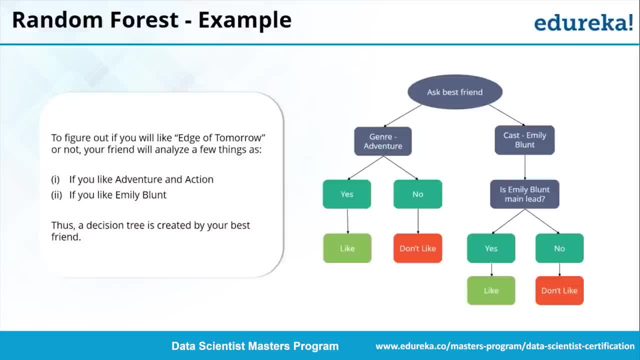 your best friend ask about whether you should go out to watch edge of tomorrow or not. so your friend will probably ask you a certain questions, like the first one being here, jonna. so so let's say your friend asks you if you really like the adventurous kind of movies or 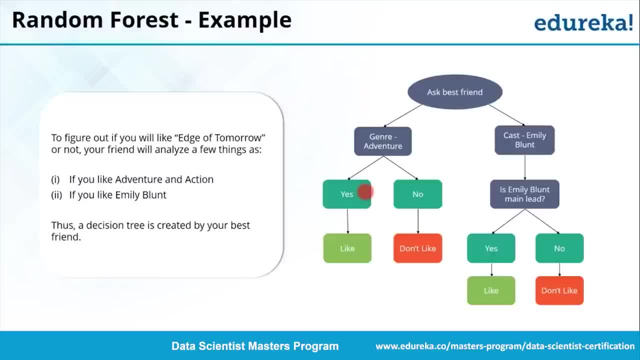 not. so you say yes, definitely, i would love to watch adventure kind of movie. so the probabilities that you will like edge of tomorrow as well, since edge of tomorrow is also a movie of adventure and sci-fi kind of genre, right? so let's say you do not. 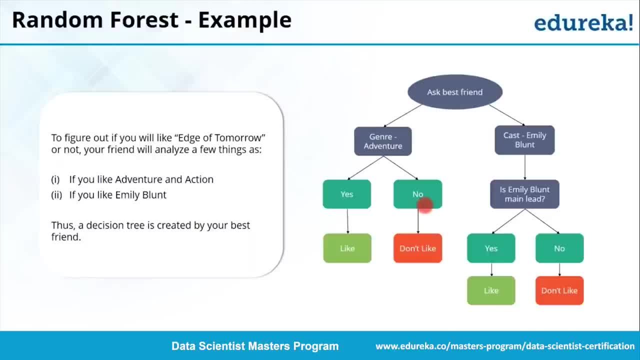 like the adventure genre movie. so then again, the probability reduces that you might really not like edge of tomorrow. right? so from here you can come to a certain conclusion. right, let's say, your best friend puts you into another situation where he'll ask you: all right, do you like emily blunt? and you say, definitely, i like emily blunt. 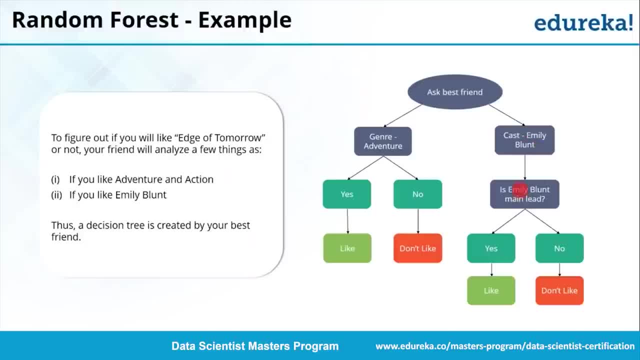 and then he puts another question to you: do you like emily blunt to be in the main lead? and you say yes, and again the probability arises that you will definitely like edge of tomorrow as well, because edge of tomorrow's has the Emily Blunt in the 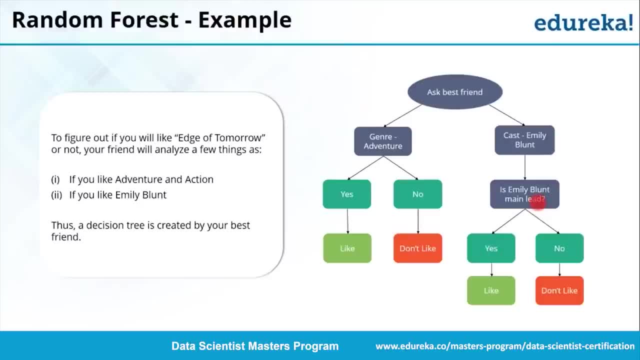 main lead cast. so and if you say, oh, I do not like Emily Blunt, then again the probability reduces that you would like edge of tomorrow too, right? so this is one way where you have one decision tree and your final outcome. your final decision, will be based on your one decision tree, or you can say your final. 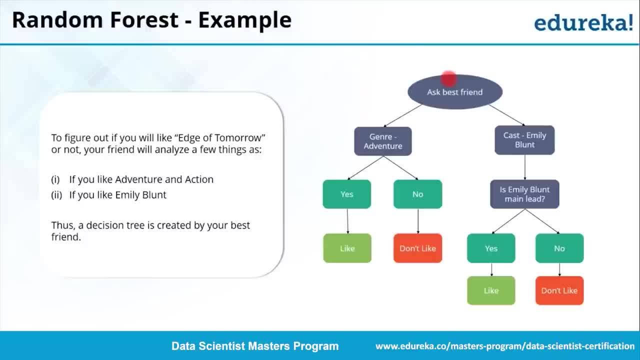 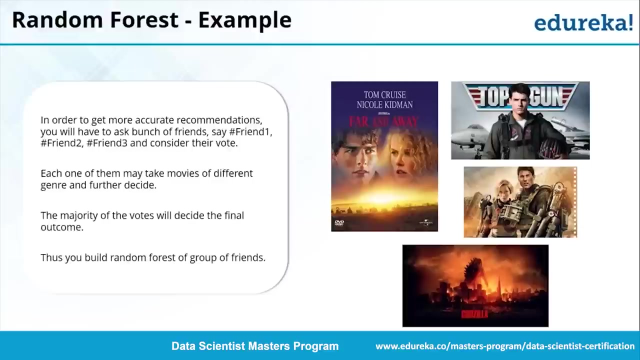 outcome will be based on just one friend. now, definitely, you're not really convinced. you want to consider the options of your other friends also so that you can make very precise and crisp decision. right, you go out and you approach some other bunch of friends of yours. so now, let's say you go to three of your friends and you ask them the same. 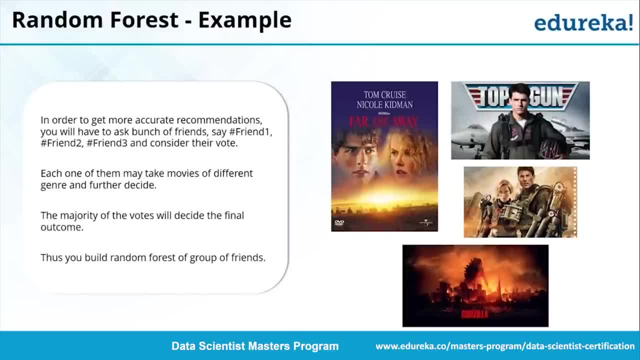 question you whether I would like to watch edge of tomorrow or not. so you go to an approach three of your friends- friend one, friend two and friend three. now you will consider each of theirs vote and then you will. your decision now will be dependent on the compiled results of all of your three friends, right? 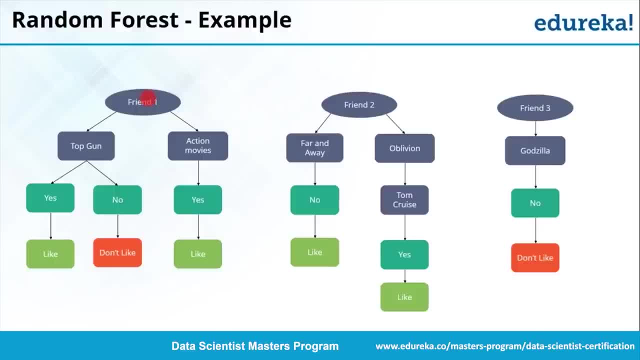 now here. let's say you go to your first friend and you ask him whether you would like to watch edge of tomorrow or not. and your first friend puts you to one question: did you like Top Gun? and you say yes, definitely, I did like the movie Top Gun. then the probability is that you would. 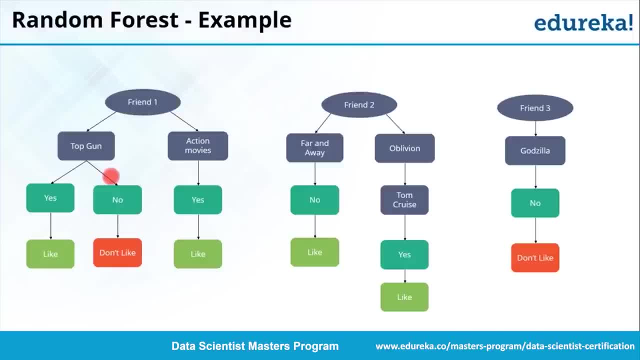 like edge of tomorrow as well, because Top Gun is actually a military action drama, which also Tom Cruise. so now again the probability arises that, yes, you will like edge of tomorrow as well. and if you say, no, I didn't like Top Gun, then again the chances are that you wouldn't like edge of tomorrow. right, and then another. 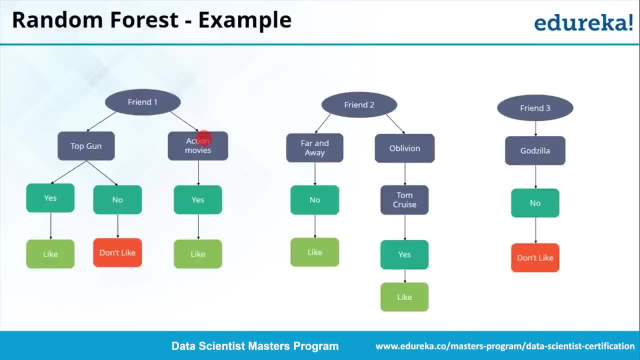 question that he puts you across is that: do you really like to watch action movies? and you say yes, I would love to watch them, then again, the chances are that you would like to watch edge of tomorrow. so from your friend one, you can come to one conclusion now here, since the ratio of liking the movie to don't like is 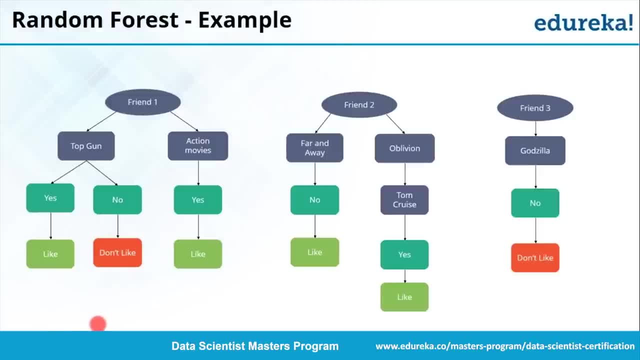 actually two is to one. so the final result is actually: you would like edge of tomorrow. now you go to your second friend and you ask the same question. so now your second friend asks you, did you like far and away when we went out and the last time when we? or? 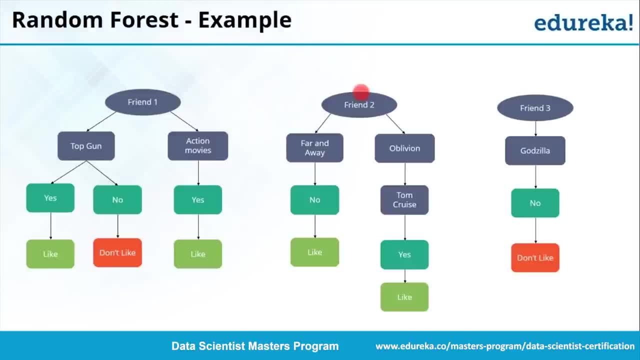 watched it and you say, no, I really didn't like far and away. then you would say: then you are definitely going to like edge of tomorrow. why it is so? because far and away is actually- since most of you might not be knowing it so far and away is genre of romance and it revolves around a girl and a guy falling 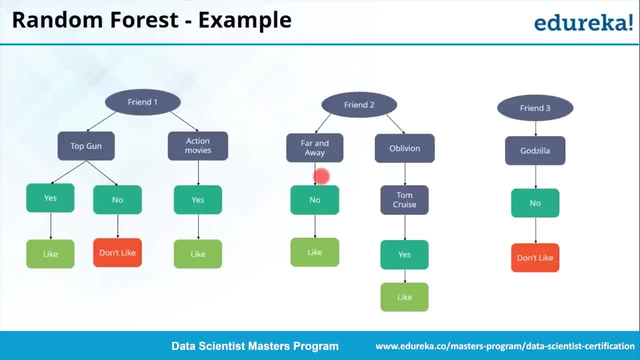 in love with each other and so on. so the probability is that you wouldn't like edge of tomorrow. so he asks you another question: did you like Oblivion and do you like the movie Top Gun? you really like to watch Tom Cruise and you say yes. again, the probability is. 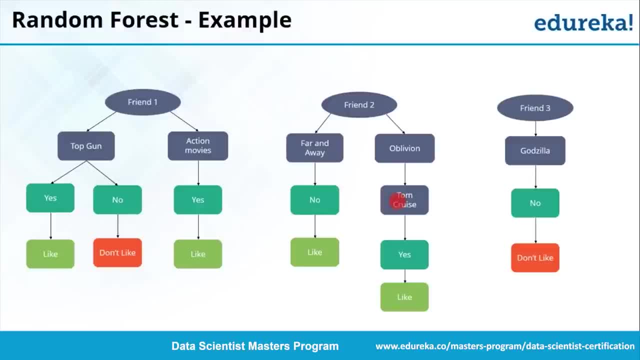 that you would like to watch edge of tomorrow, and why? because Oblivion, again, is a science fiction casting Tom Cruise, full of strange experiences, and where Tom Cruise is the savior of the mankind. well, that is the same kind of plot in edge of tomorrow as well. so here it is pure yes that you would. 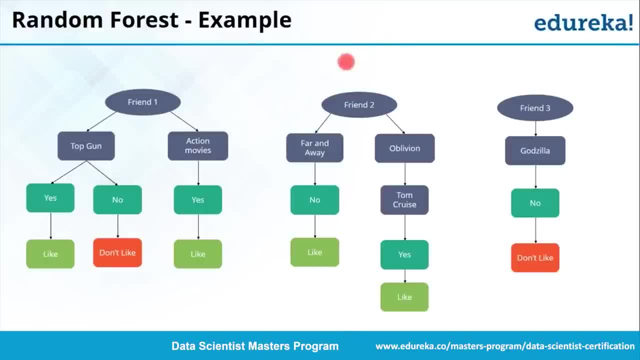 like to watch edge of tomorrow. so you get another second decision from your second friend. now you go to your third friend and ask him. so probably your third friend is not really interested in having any sort of conversation with you, so it just simply asks you, did you like Godzilla and you? 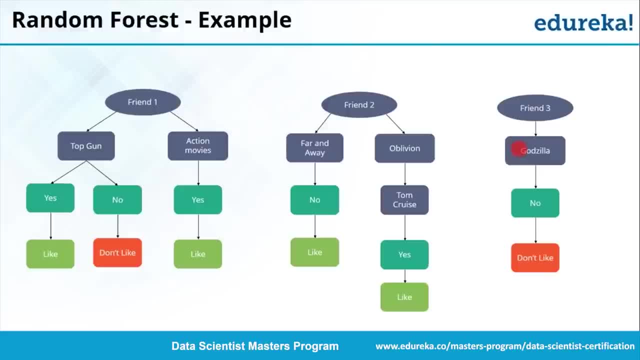 say no, I didn't like Godzilla. so you say definitely you wouldn't like edge of tomorrow. why so? because Godzilla is also actually a science fiction movie from the adventure genre. so now you've got three results from three different decision trees from three different friends. now you compile the results of 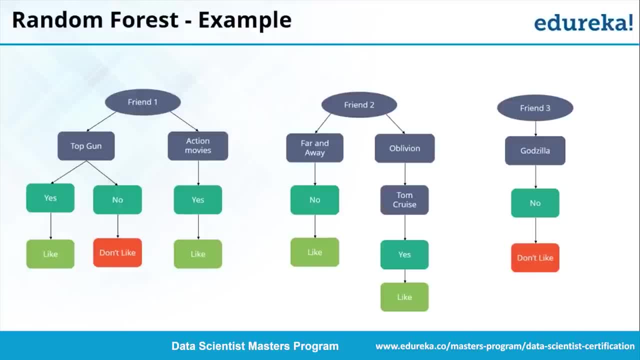 all those friends and then you make a final call that, yes, would you like to watch edge of tomorrow or not? so this is some very real time and very interesting example where you can actually implement random forests into ground reality. now let us look at various domains where random forest is actually used. so 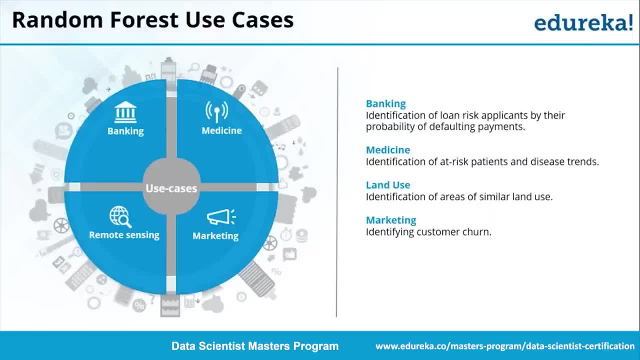 because of its diversity, random forest is actually used in various diverse domains. So, be it banking, be it medicine, be it land use, be it marketing, name it- and random forest is there. So in banking, particularly, random forest is being actually used to make it out whether the applicant 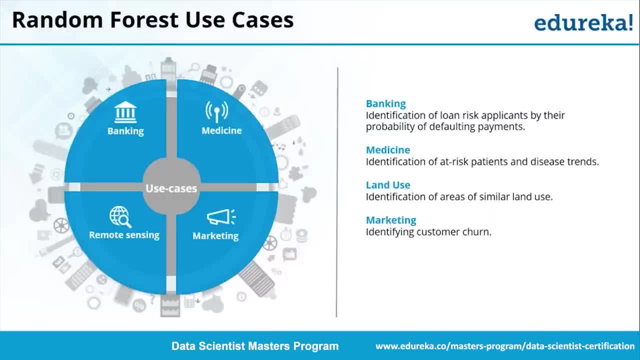 will be a defaulted pair or it will be non-defaulted one, so that it can accordingly approve or reject the applications of loan. So that is how random forest is being used in banking. Talking about medicine, random forest is widely used in medicine field to predict beforehand. 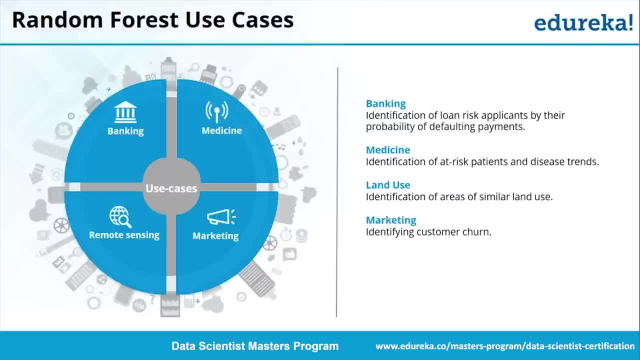 what is the probability if a person will actually have a particular disease or not. So it's actually used to look at the various disease trends. Let's say you want to figure out what is the probability that a person will have diabetes or not, and so what would you do? 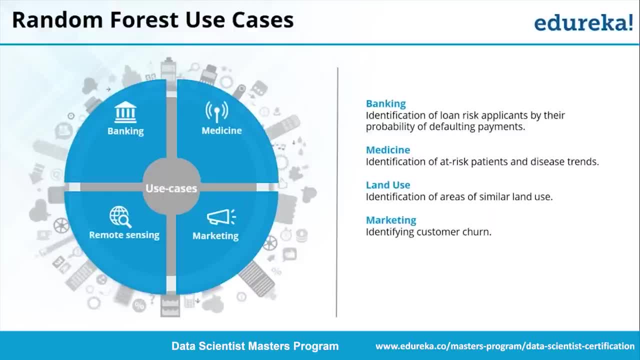 You'll probably look at the medical history of the patient and then you will see: all right, this has been the glucose concentration. what was the BMI? what was the insulin levels in the patient in the past previous three months? what is the age of this particular person? 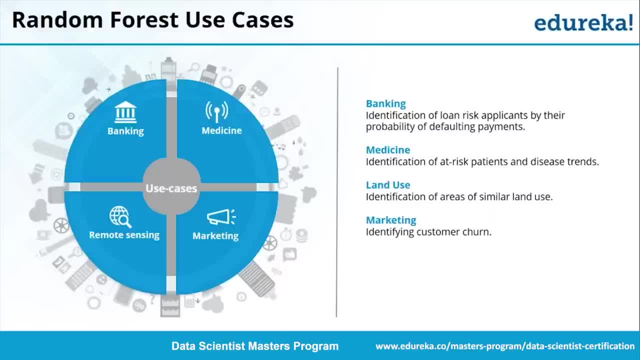 and you will make different decision trees based on each one of these predicted variables and then you'll finally compile the results of all those variables and then you'll make a final decision as to whether the person will have diabetes in the near future or not. That is how random forest will be used in medicine sector. 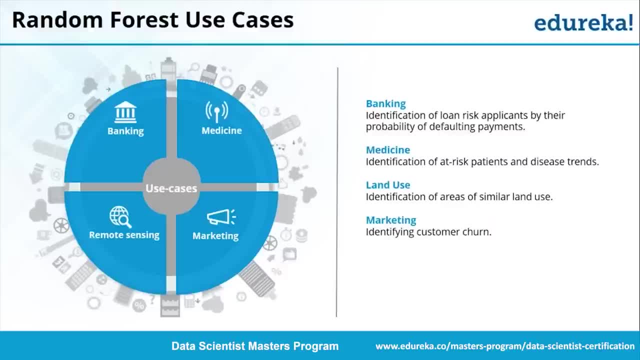 Now, random forest is also actually used to find out the land use. For example, I want to set up a particular industry in certain area, So what would I probably look for? I look for what is the vegetation over there, what is the urban population over there, right? 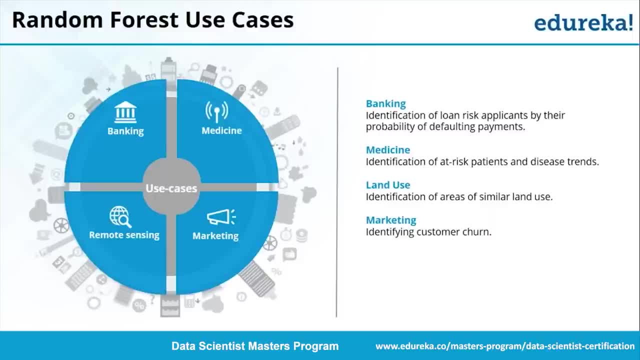 and how much is the distance from the nearest modes of transport, like from the bus station or the railway station, And accordingly, I will split my parameters and I will make decision on each one of these parameters And finally, I'll compile my decision of all these parameters and that will be my final outcome. 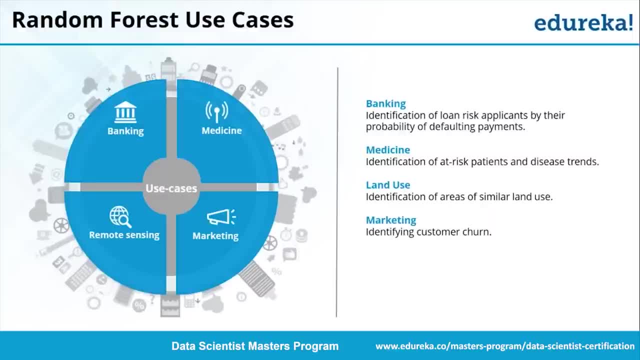 So that is how I'm finally going to predict whether I should put my industry at this particular location or not, right? So these three examples have actually been of majorly around classification problem, because we are trying to classify whether or not We're actually trying to classify whether or not. 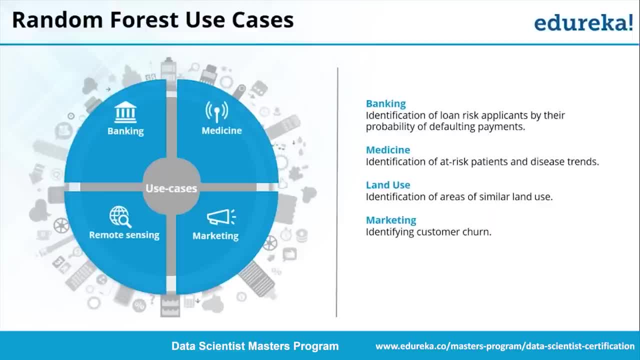 We're actually trying to answer this question, whether or not, right Now. let's move forward and look how marketing is revolving around random forest. So particularly in marketing, we try to identify the customer churn. So this is particularly the regression kind of problem. 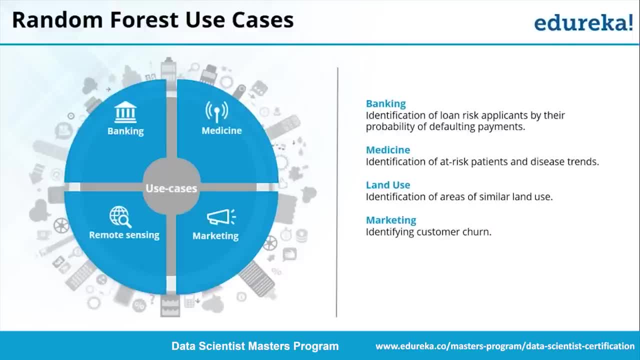 right now how let's see So customer churn is nothing, but actually the number of people which are actually, or the number of customers who are losing out, So who are going out of your market. You want to identify what will be your customer churn in near future. 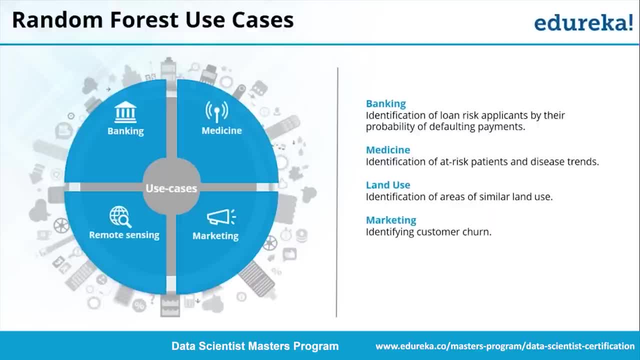 So most of the e-commerce industries are actually using this, like Amazon, Flipkart, et cetera. So they particularly look at your each behavior as to what has been your past history, what has been your purchasing history, what do you like based on your activity? 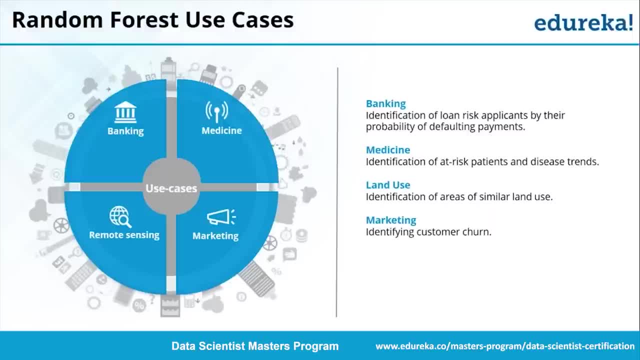 around certain things, around certain ads, around certain discounts or around certain kind of materials. right, If you like a particular top, you're actually going to like it. If you like a particular top, you're actually going to like it. 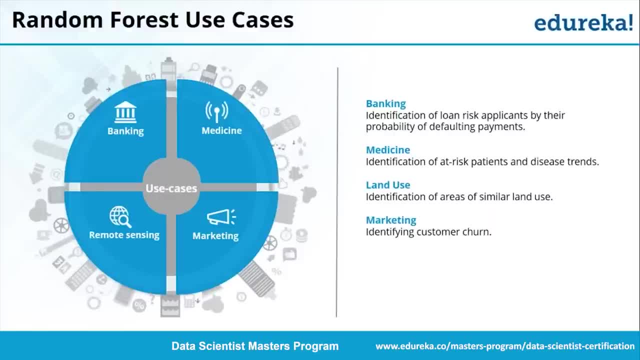 If you like a particular top, you're actually going to like it. Your activity will be more around that particular top. So that is how they track each and every particular move of yours, and then they try to predict whether you will be moving out or not. 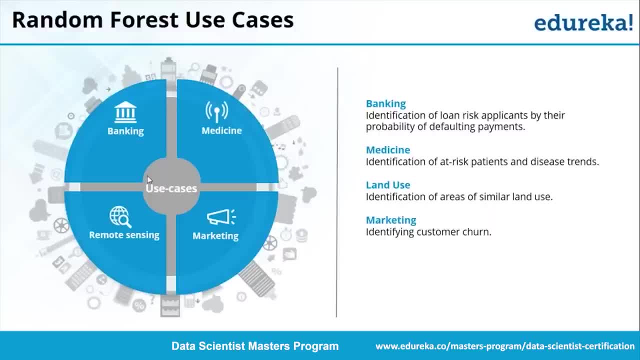 So that is how they identify the customer churn. So these all are various domains where random forest is used, and this is not the only list, So there are numerous other examples which actually are using random forest. That makes it so special actually. 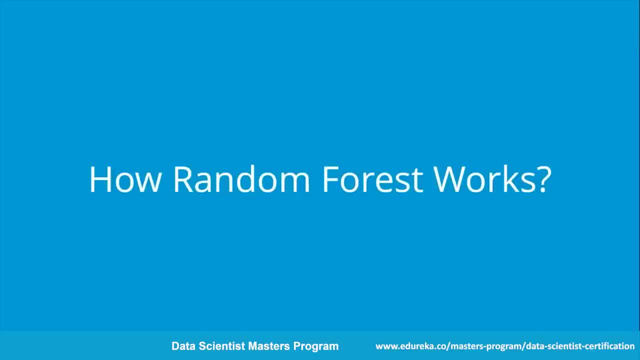 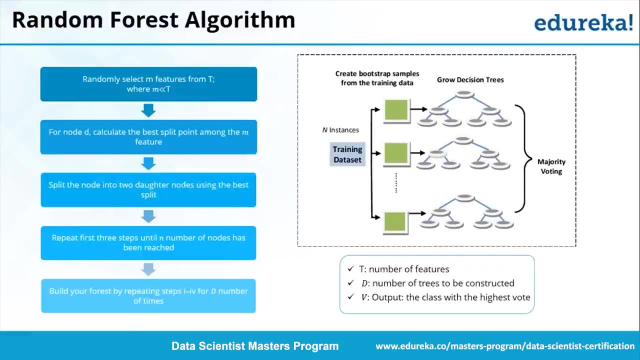 Now let's move forward and see how random forest actually works, right? So let us start with the random forest algorithm first. Let's just see it step by step as to how random forest algorithm works. So the first step is to actually select certain M features from T where M is less than T. 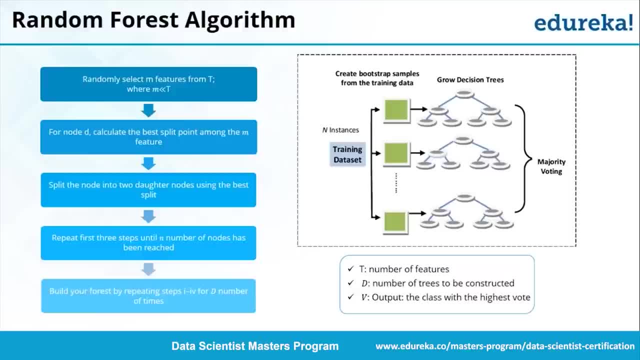 So here, T is the total number of the predicted variables that you have in your data set, and out of those total predicted variables you will select some randomly, some few, a few features out of those. Now why we are actually selecting a few features only. 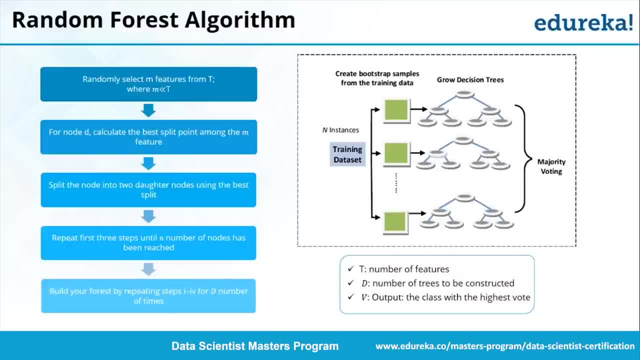 the reason is that if you will select all the predicted variables, or the total predicted variables, then each of your decision tree will be same. So your model is not actually learning something new. It is learning the same previous thing, because all those decision trees will be similar, right? 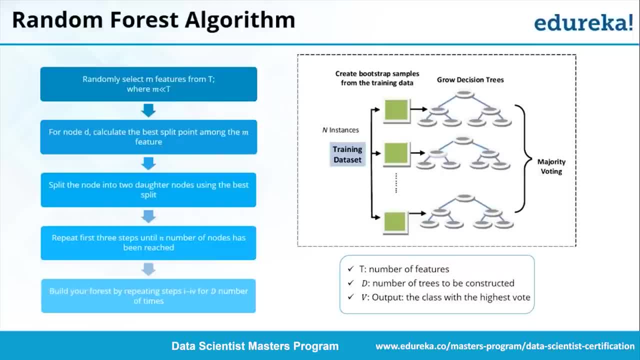 Now if you actually split your predicted variables and you select randomly a few predicted variables only, let's say there are 14 total number of variables and out of those you'll randomly pick just three right? So every time you will get a new decision tree. 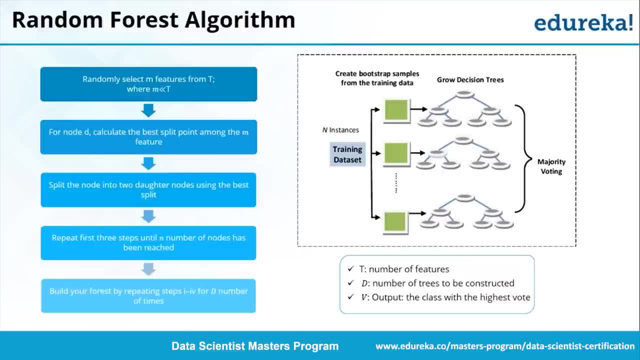 so there will be variety, right. So the classification model will be actually much more intelligent than the previous one. Now it has got varied experiences, so definitely it will make different decisions each time and then, when you will compile all those different decisions, it will be a new, more accurate. 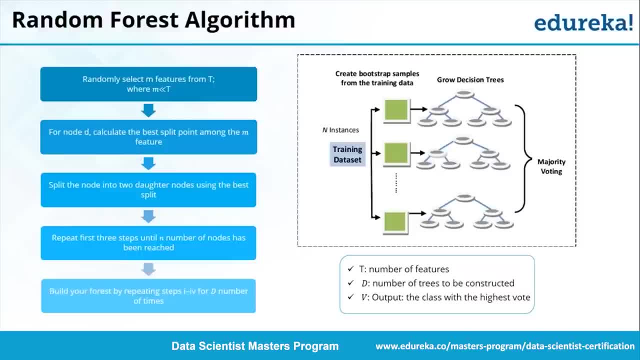 and efficient result right. So the first important step is to select certain number of features out of all the features. Now let's move on to the second step. Let's say, for any node D, Now the first step is to calculate the best split at that point, 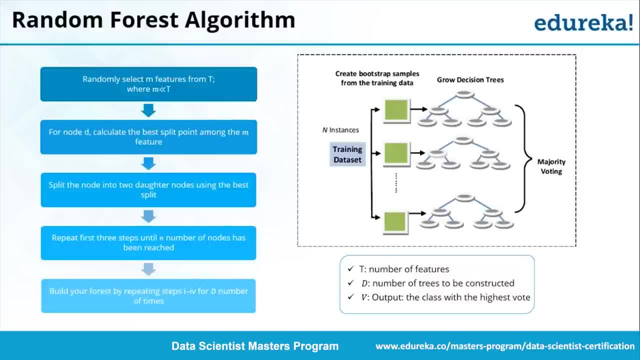 So you know that decision tree, how decision tree is actually implemented. So you pick up the most significant variable, right, And then you will split that particular node into further child nodes. That is how the split takes place, right. So you will do it for m number of variables. 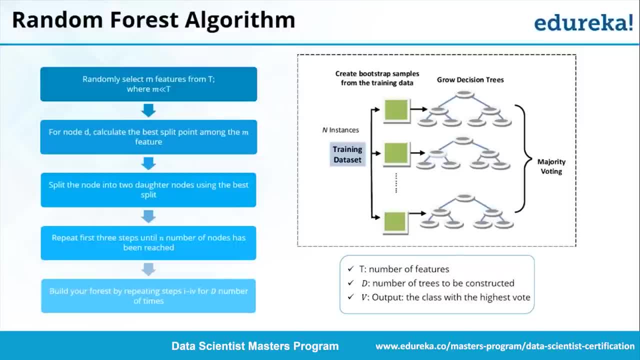 that you've selected. Let's say you have selected three, so you will implement the split at all those three nodes in one particular decision tree, right? The third step is split up the node into two daughter nodes. So now you can split your root node. 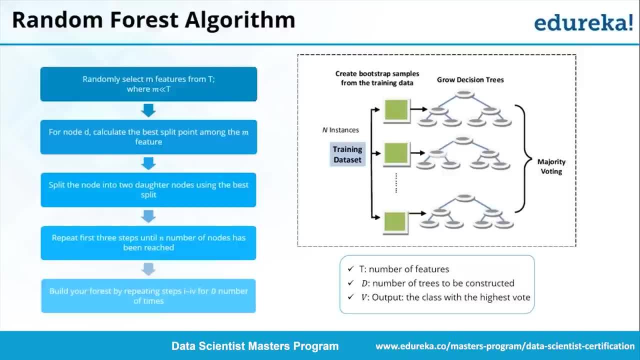 into as many nodes as you want to, but here we'll split our node into two daughter nodes as to this or that. so it will be an answer in terms of this or that, right. Our fourth step will be to repeat all these three steps. 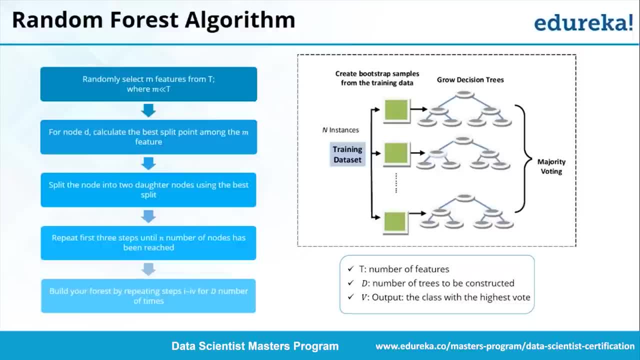 that we've done previously and we'll repeat all this splitting until we have reached all the n number of nodes right. So we need to repeat until we have reached till the leaf nodes of our decision tree. That is how we will do it right. 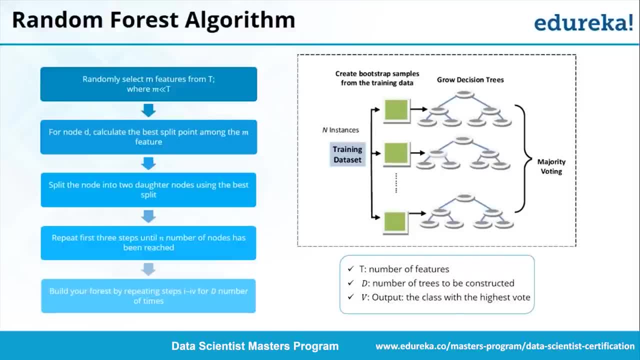 Now, after these four steps, we will have our one decision tree. but random forest is actually about multiple decision trees. So here our fifth step will come into the picture, which will actually repeat all these previous steps for d number of times. Now here, d is the d number of decision trees. 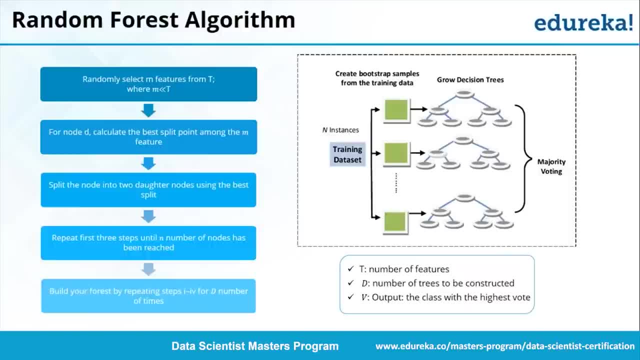 Let's say I want to implement five decision trees, So my fifth step will be to implement all the previous steps five times. So here the iteration is for five number of times. right Now, once I have created these five decision trees, still my task. 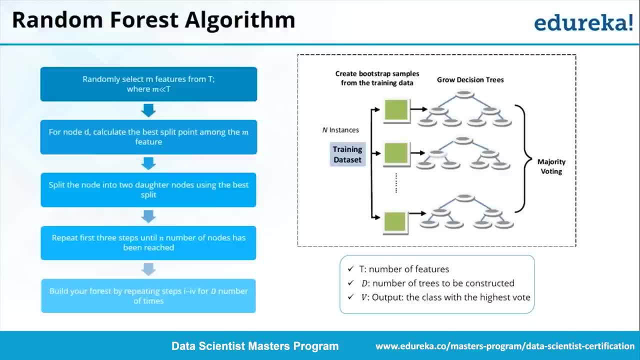 is not complete yet. Now my final task will be to compile the results of all these five different decision trees, and I will make a call on the majority voting right Here. as you can see in this picture, I had n different instances. 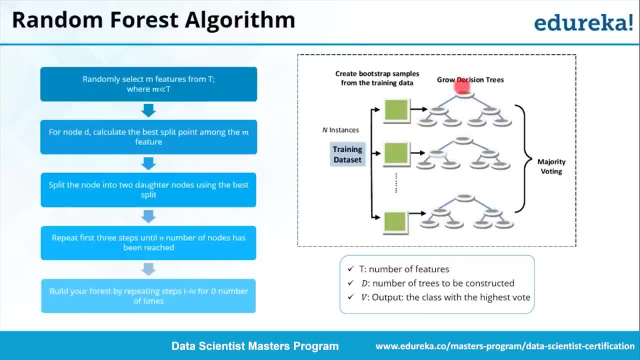 Then I've created n different decision trees And finally I will compile the result of all these n different decision trees and I will take my call on the majority voting. So whatever my majority votes say really doesn't matter. So I will compile the results of all these n different decision trees and I will make a call on the majority voting. 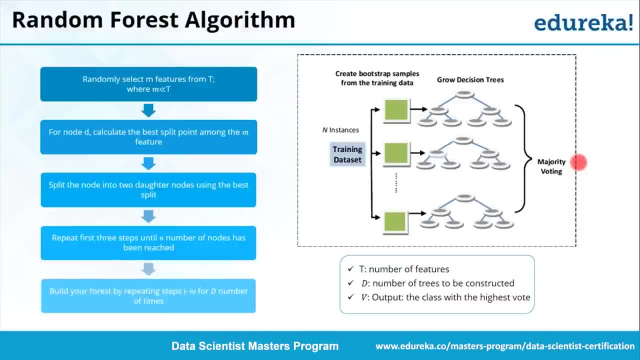 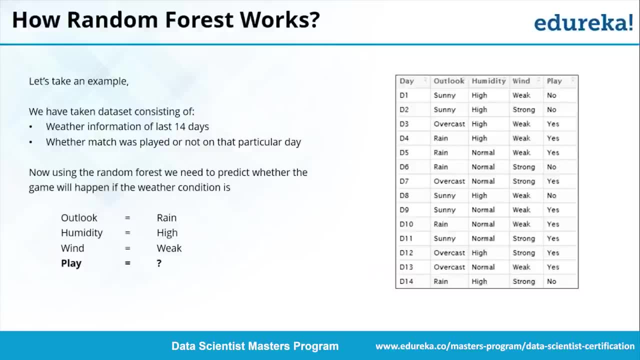 that will be my final result. so this is basically an overview of the random forest algorithm, how it actually works. let's just have a look at this example to get much better understanding of what we have learnt. so let's say, I have this data set which consists of four different instances, right? so basically, 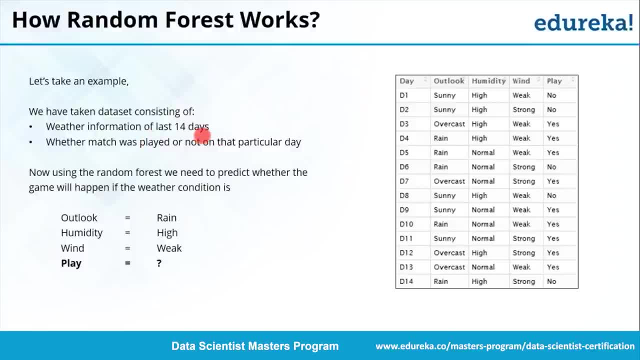 it consists of the weather information of previous 14 days, right from d1 till d14, and this basically outlook: humidity and wind. this basically gives me the weather condition of those 14 days and finally, I have play, which is my target variable, where the match did take place on that particular day or not right now. 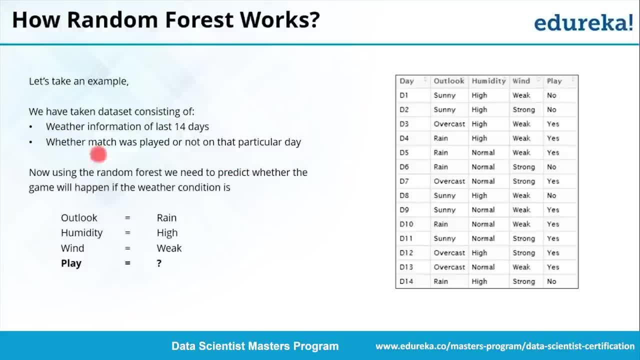 my main goal is to find out whether the match will actually take place. if I have following these weather conditions with me on any particular day- let's say the outlook is rainy that day and humidity is high- you can see that the weather condition is very high and the humidity is very high. 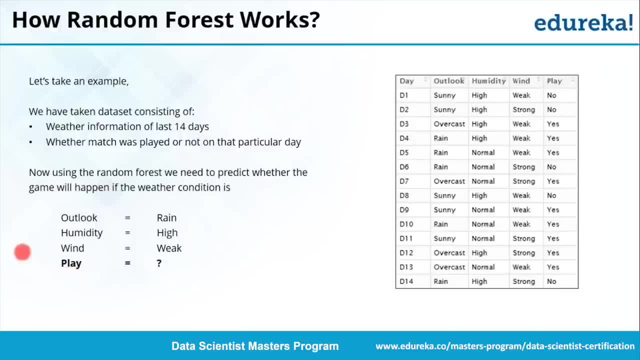 and the wind is very weak, so now I need to predict whether I will be able to play the match that day or not. all right, so this is a problem statement. fine, now let's see how random forest is used in this to sort it out. now, here the first. 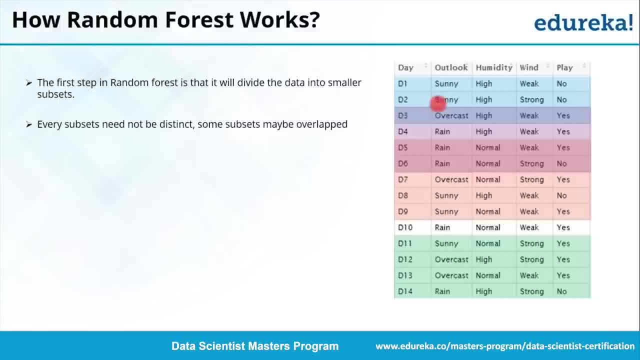 step is to actually split my entire data set into subsets. here I have split my entire 14 variables into further smaller subsets. right now these subsets may or may not overlap. like there is certain overlapping between d1 till d3 and d3 till d6, right, so there is an overlapping. 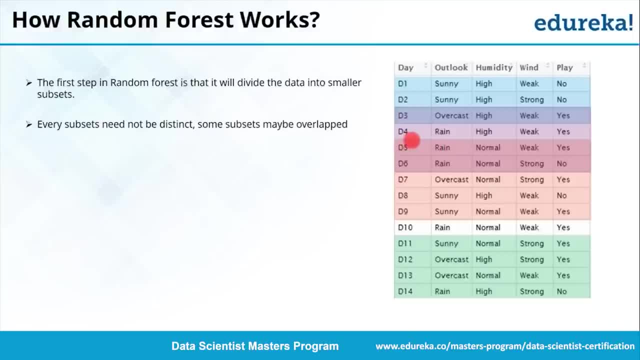 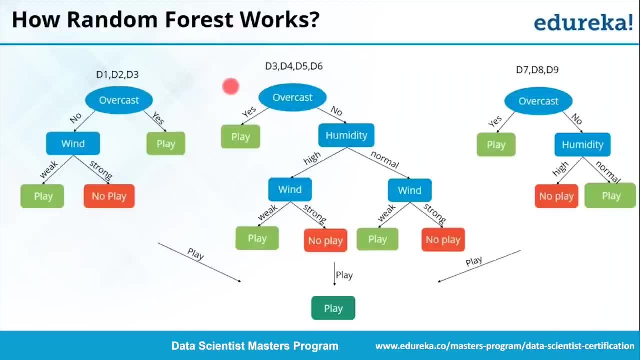 of d3. so it might happen that there might be overlapping. so you need not really worry about the overlapping, but you have to make sure that all those subsets are actually different, right? so here I have taken three different subsets. my first subset consists of d1 till d3. my second subset consists of d3 till d6. 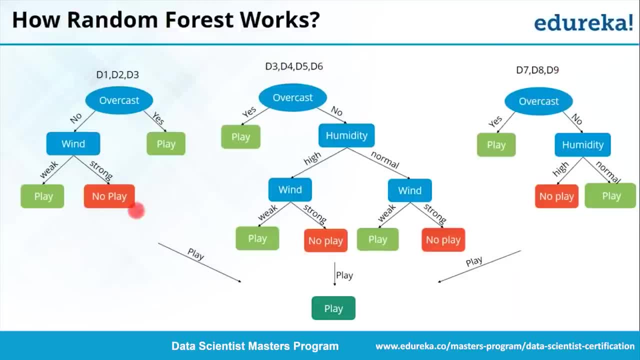 and my third subset consists of d7 till d now. now I will first be focusing on the first subset now here. let's say that particular day the outlook was overcast. fine, if yes, it was overcast, then the probability is that the match will take place. so overcast is basically when your weather is too cloudy. so if that is the 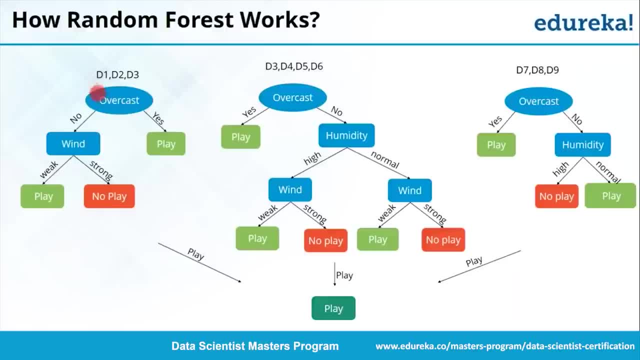 condition, then definitely the match will take place now- let's say it wasn't overcast- then you will consider the second most probable option, that will be the wind, and you will make a decision based on this now whether wind was weak or strong. if it was weak, then you will definitely go out and play the match. 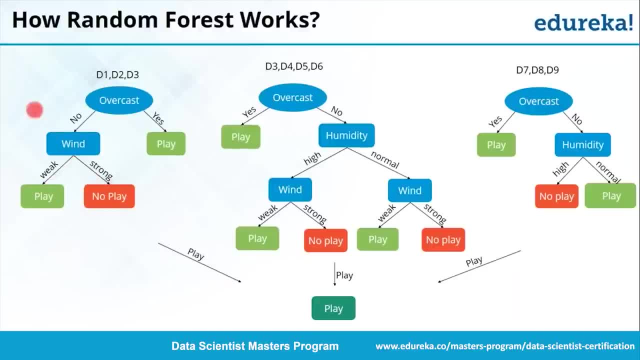 else you would not. so now the final outcome out of this decision tree will be play, because here the ratio between the play and no play is 2 is to 1. so we get to a certain decision from a first decision tree. now let us look at the 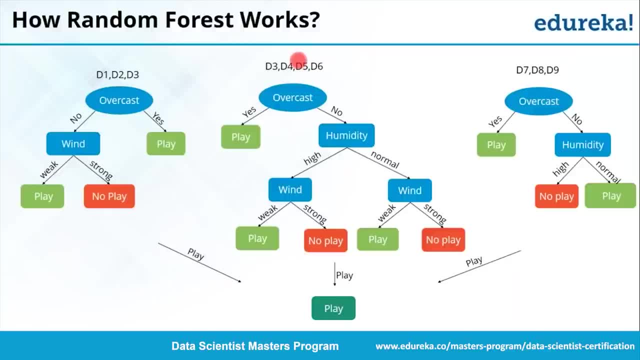 second subset now, since second subset has different number of variables, so that is why this decision tree is absolutely different from what we saw in a first set subset. so let's say, if it was overcast then you will play the match, if it isn't the overcast, then you would go and look out for humidity. now, further it. 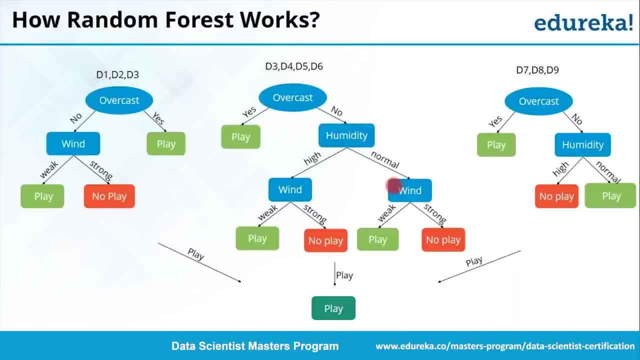 will get split into two, whether it was high or normal. now we'll take the first case. if the humidity was high and wind was weak, then you will play the match. else, if humidity was high but wind was too strong, then you would not go out and play the match. right now let us look at the second daughter node of humidity. if 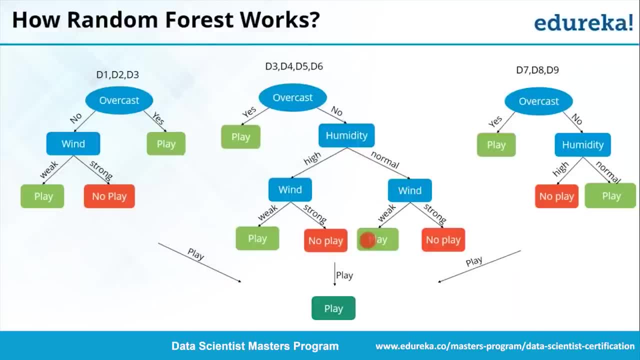 the humidity was normal and the wind was weak, then you will definitely go out and play the match. else you won't go out and play the match. so here, if you look at the final result, then the ratio of plays to no play is 3 is to 2. then again the 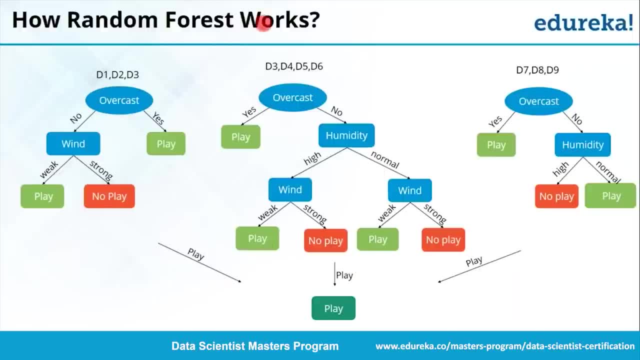 final outcome is actually play right. so from second subset we get the final decision of play. now let us look at our third subset, which consists of d7 till d9. here, if again the overcast is yes, then you will play a match. else you will go and check out for humidity and if the humidity is, 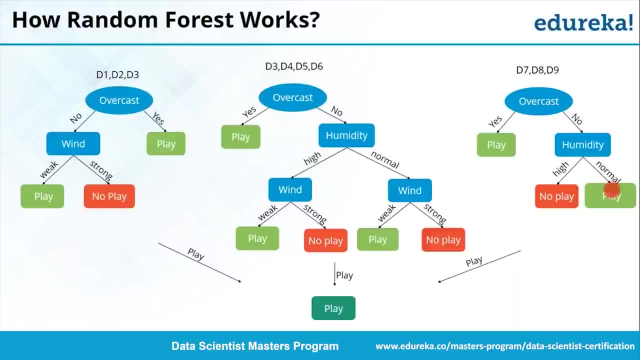 really high, then you won't play the match, else you will play the match again. the probability of playing the matches- yes, because the ratio of no play is 2- is to 1. right, so, three different subsets, three different decision trees, three different outcomes and one final outcome after compiling all the results from these three. 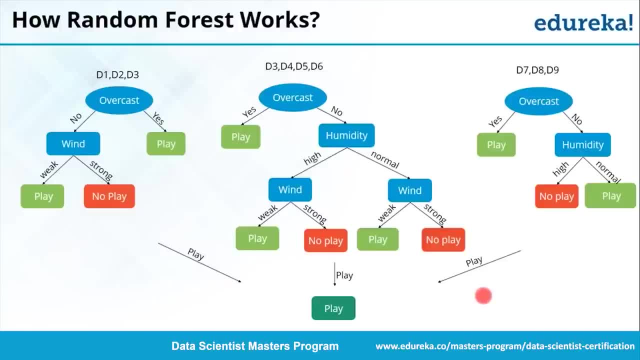 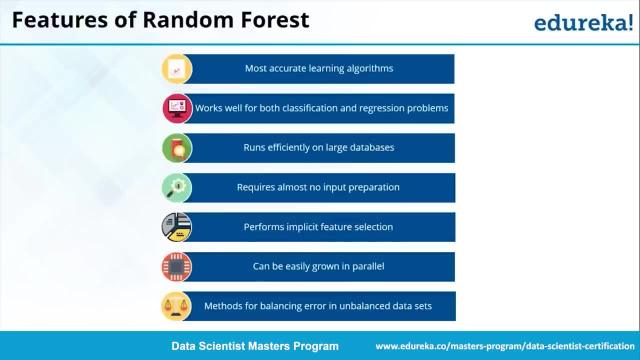 different decision trees. all right, so I hope this gives a better perspective, a bit understanding of random forest, like how it really works. all right, so now let's just have a look at various features of random forest, right? so the first and the foremost feature is that it is one of the most accurate learning. 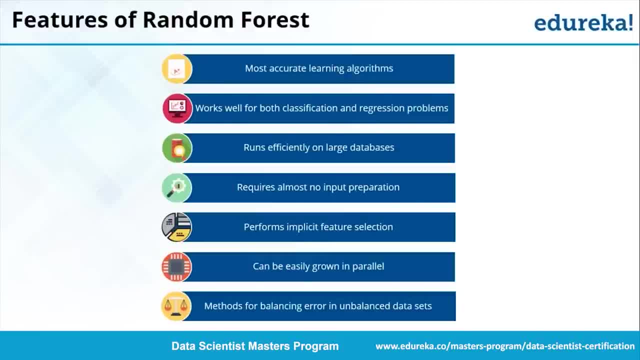 algorithms right. so why it is so? because single decision trees are actually prone to having high variance or high bias and, on the contrary, actually random forest it averages the entire variance across the decision trees. so let's say, if the variances say X for decision tree, but 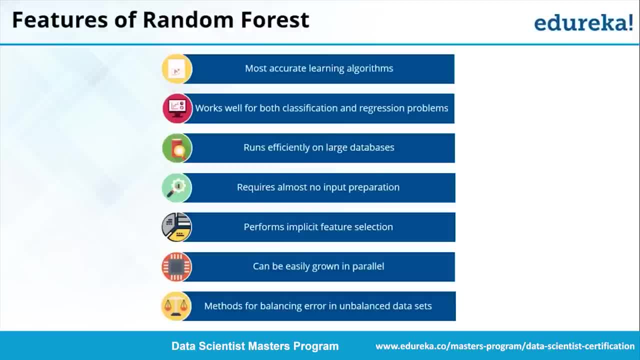 for random forests. let's say we have implemented n number of decision trees- παdалі, so my entire variance gets averaged upon and my final variance actually becomes x upon n. so that is how the entire variance actually goes down as compared to other algorithms right now. second most important feature is that it works well for both. 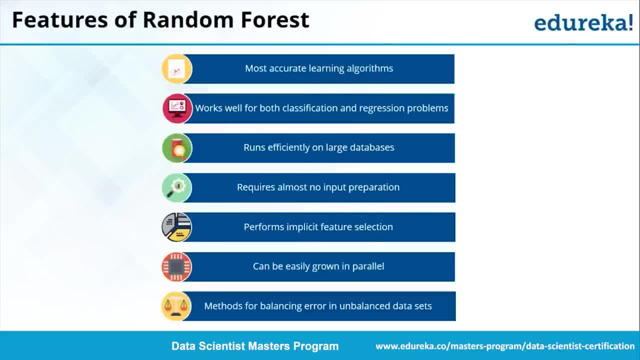 classification and regression problems and by far i have come across, this is one and the only algorithm which works equally well for both of them, be it classification kind of problem or a regression kind of problem. right then, it really runs efficient on large databases. so basically, it's really scalable even if you work for the lesser amount of database or if you work for 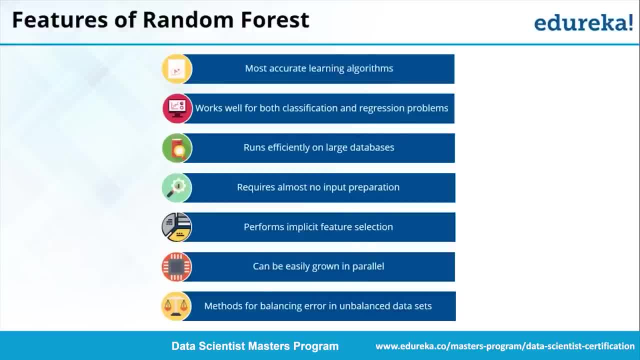 really huge volume of data, right, so that's a very good part about it. then the fourth most important point is that it requires almost no input preparation. now, why am i saying this? is because it has got certain implicit methods which actually take care and remove all the outliers and all the missing data, and you really 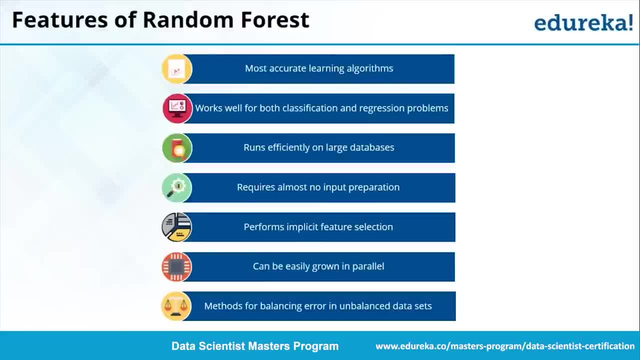 don't have to take care about all that thing while you are in the stages of input preparation. so random forest is all here to take care of everything else, and next is it performs implicit feature selection, right? so while we are implementing multiple decision trees. so it has got. 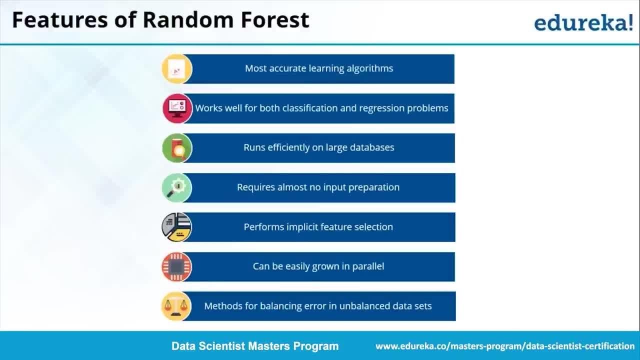 implicit method which will implement multiple decision trees. so it has got implicit method which will automatically pick up some random features out of all your parameters and then it will go on and implementing different decision trees. so, for example, if you just give one simple command, that all right, i want to implement 500 decision trees, no matter how so random forest. 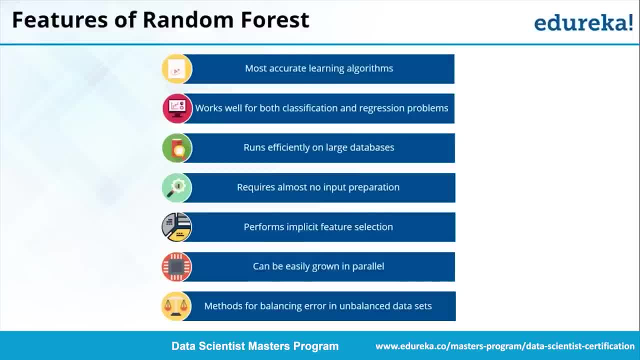 will automatically take care and it will implement all those 500 decision trees, and those all 500 decision trees will be different from each other, and this is because it has got implicit methods. and this is because it has got implicit methods which will automatically collect different parameters itself out of all the variables that you have. 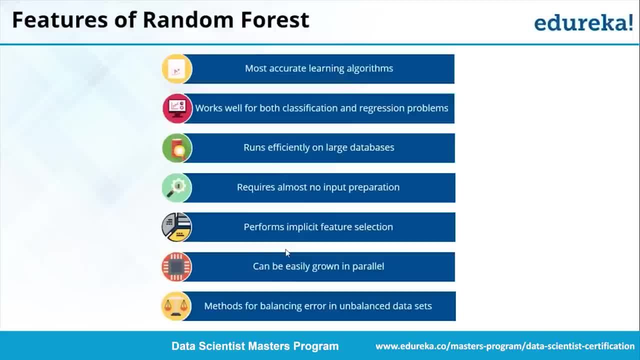 right, then it can be easily grown in parallel. why it is so? because we are actually implementing multiple decision trees and all those decision trees are running, or all those decisions trees are actually getting implemented parallelly. so if you say i want thousand trees to be implemented, so all those thousand trees are getting implemented parallelly. 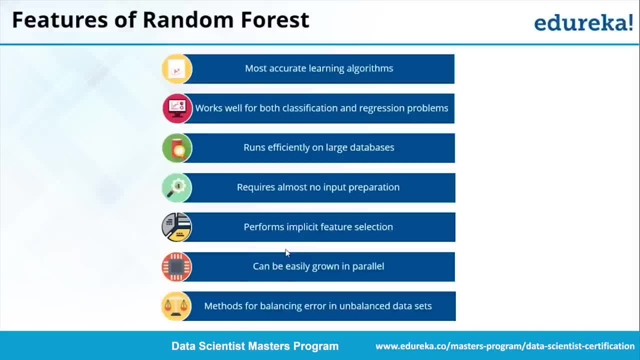 so that is how the competition time reduces down right. and the last point is that it has got methods for balancing error in unbalanced data sets. now what exactly unbalanced data sets are? let me just give you an example of that. so let's say you're working on a data set, fine, and you create: 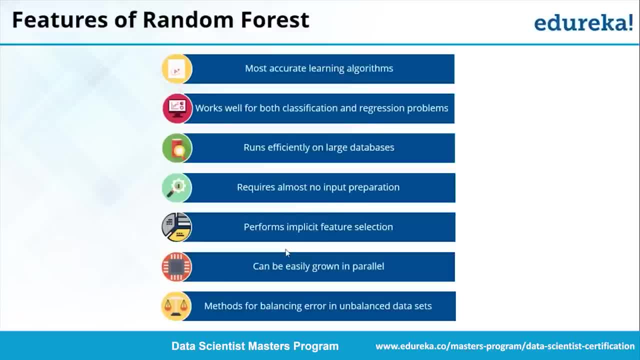 a random forest model and get 90 accuracy immediately. fantastic, you think right, so now we are going to you start diving deep. you go a little deeper and you discovered that 90% of that data actually belongs to just one class. damn, your entire data set, your. 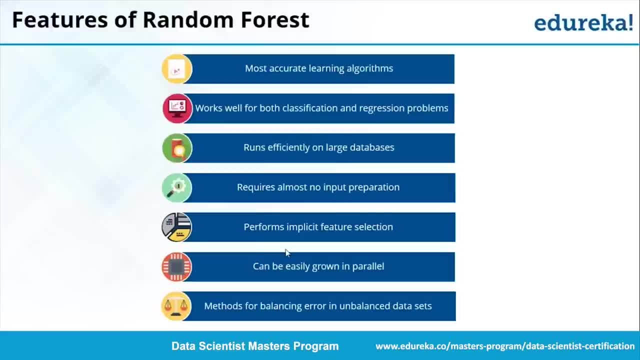 entire decision is actually biased to just one particular class. so random forest actually takes care of this thing and it is really not biased towards any particular decision tree or any particular variable or any class. so it has got methods which looks after it and there does all the balance of errors in. 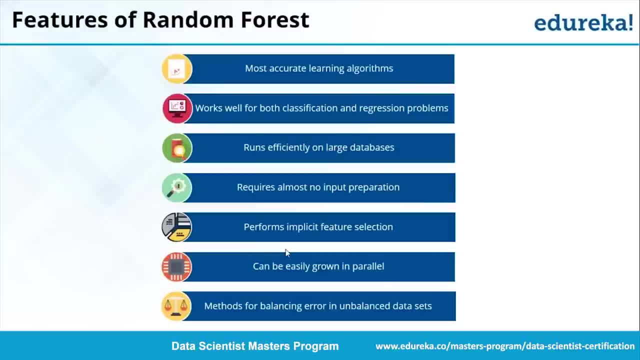 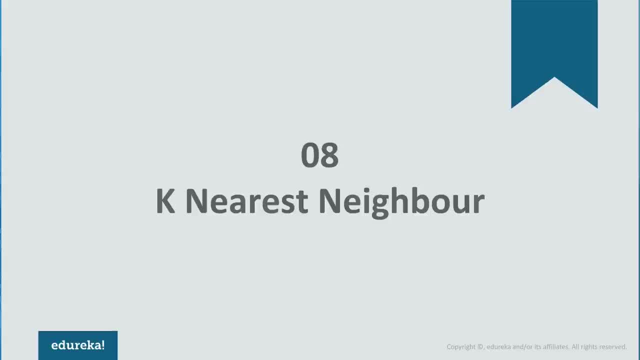 your data sets. so that's pretty much about the features of random forests. k-nearest neighbor is a simple algorithm which uses entire data set in its training phase. whenever a prediction is required for unseen data, what it does is it searches through the entire training data set for k most similar instances. 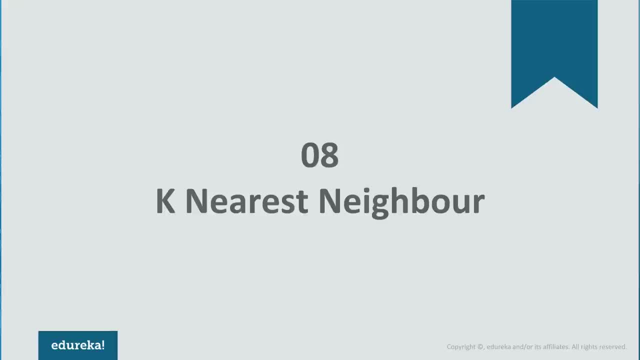 and the data set is then used to predict the data set and the data set is used to predict. the data with the most similar instance is finally returned as the prediction. so hello and welcome all to this YouTube session, and in today's session we'll be dealing with KNN algorithm. so, without dealing any further, 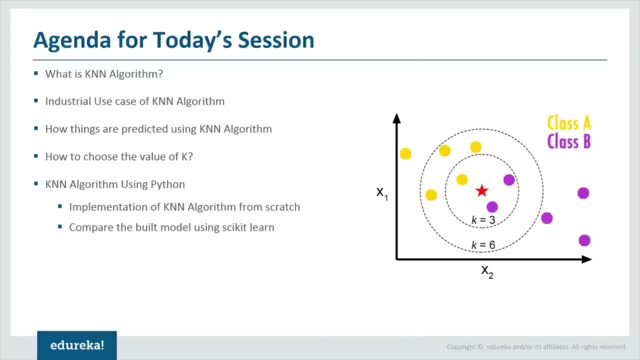 let's move on and discuss agenda for today's session. so we'll start our session with what is KNN, where I'll brief you about the topic and we'll move ahead to see what its popular use cases or how the industry is using KNN for. 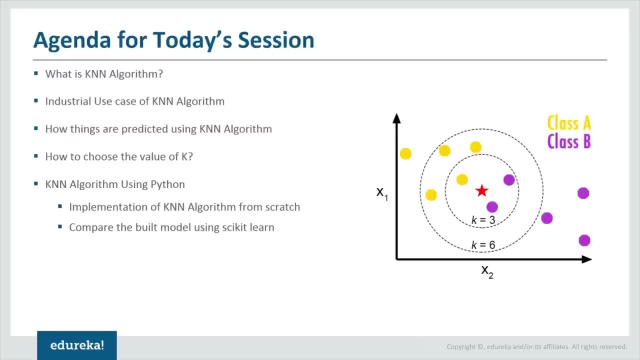 their benefit. once we are done with it, we will drill down to the working of algorithm in depth. while learning the algorithm, you will also understand the significance of K- or what does this case stands for- in the nearest neighbor algorithm, and then we'll see how the prediction is made using KNN algorithm. 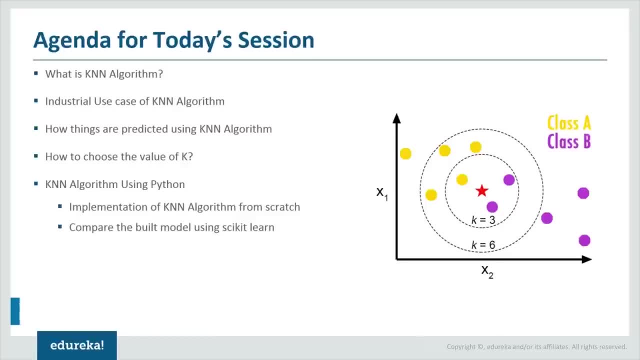 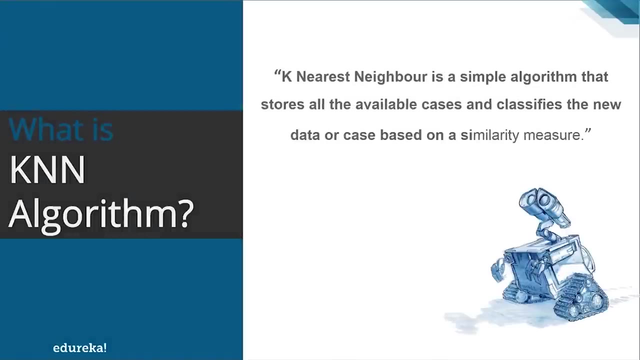 manually or mathematically. all right now, once we are done with the theoretical concept, we'll start the practical or the demo session, where we'll learn how to implement KNN algorithm using python. so let's start our session. so, starting with, what is KNN algorithm? well, k-nearest neighbor is a simple algorithm that stores all the 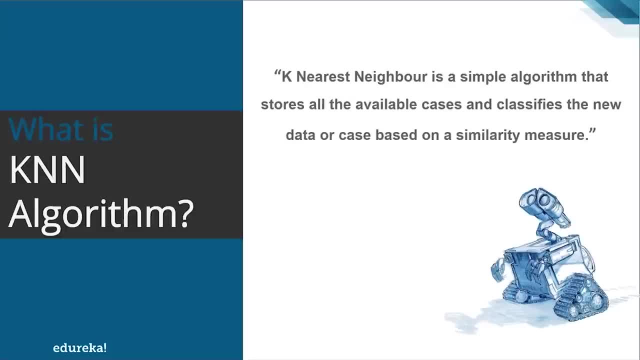 available cases and classify the new data or case based on a similarity measure. it suggests that if you are similar to your neighbors, then you are one of them right. for example, if Apple looks more similar to banana, orange or melon rather than a monkey, rat or a cat, then most likely Apple belong. 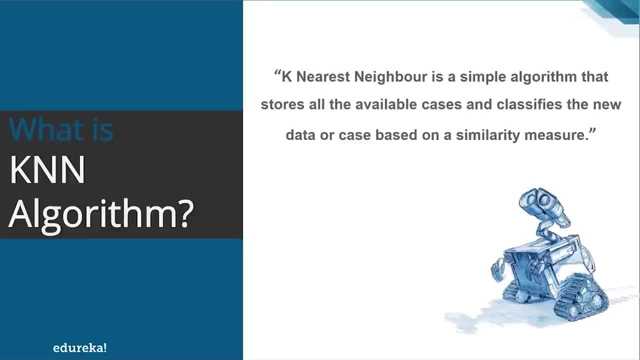 to the group of fruits. alright. well, in general, KNN is used in search application where you're looking for similar items, that is, when your task is some form of fine items similar to this one. then you call this search as a k and search. but what is this k in KNN? well, this K denotes the 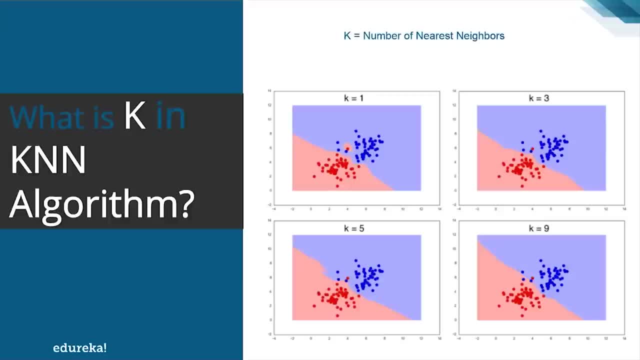 number of nearest neighbor which are voting new data or the testing data. For example, if K equal 1, then the testing data are given the same label as the closest example in the training set. Similarly, if K equal 3, the labels of the three. 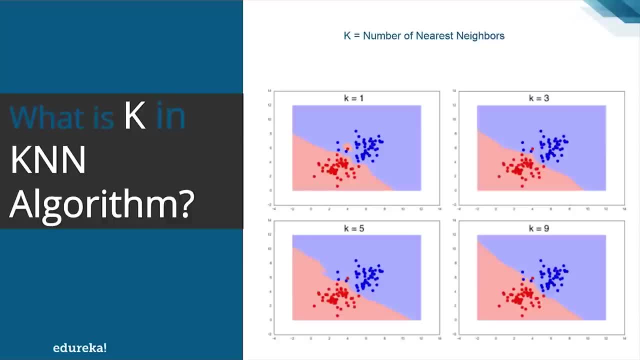 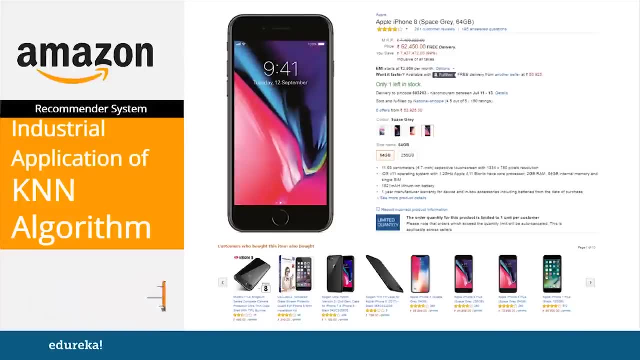 closest classes are checked and the most common label is assigned to the testing data. So this is what a KN-KN algorithm means. So, moving on ahead, let's see some of the example of scenarios where KNN is used in the industry. So let's see the industrial application of KNN algorithm starting. 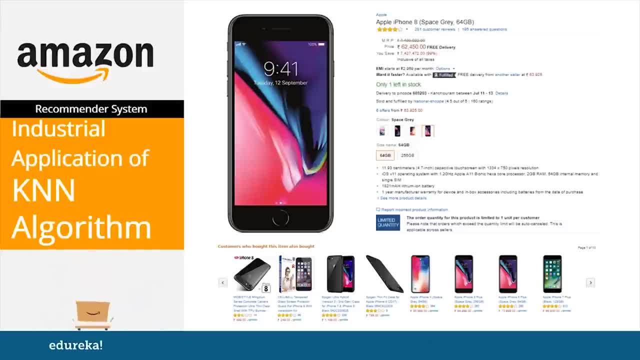 with recommender system. Well, the biggest use case of KNN search is a recommender system. This recommender system is like an automated form of a shop counter guy. When you ask him for a product, not only shows you the product but also suggests you or displays you a relevant set of products. 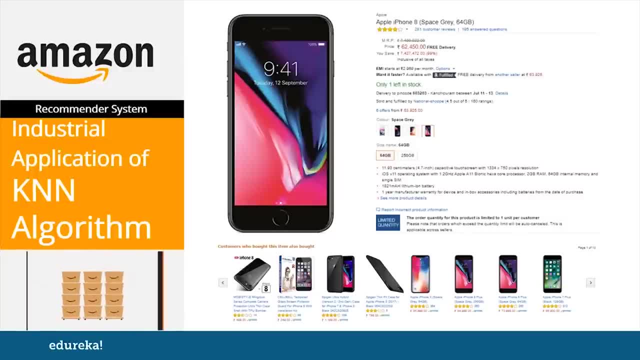 which are related to the item you're already interested in buying. This KNN algorithm applies to recommending products, like in Amazon, or for recommending media, like in case of Netflix, or even for recommending advertisement to display to a user. If I am not wrong, almost all of you must. 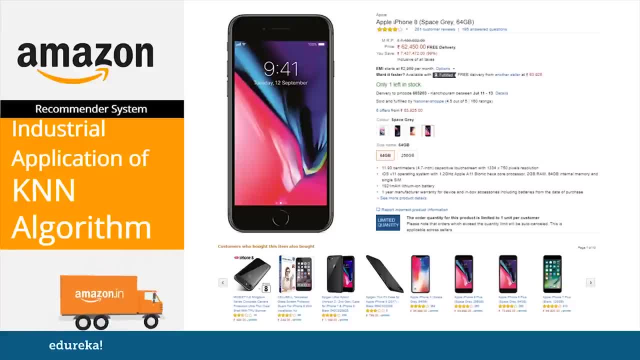 have used Amazon for shop counter guy. So if you are using a product like a shop counter guy, right? so just to tell you, more than 35% of Amazoncom's revenue is generated by its recommendation engine. So what's their strategy? Amazon uses recommendation as a targeted marketing. 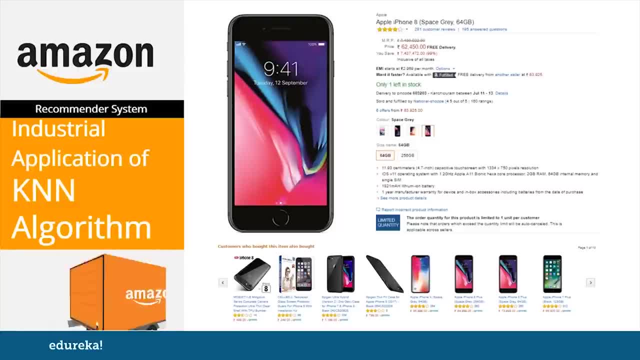 tool. in both the email campaigns and on most of its website pages, Amazon will recommend many products from different categories based on what you have browsed, and it will pull those products in front of you which you are likely to buy, Like the frequently bought together option that comes. 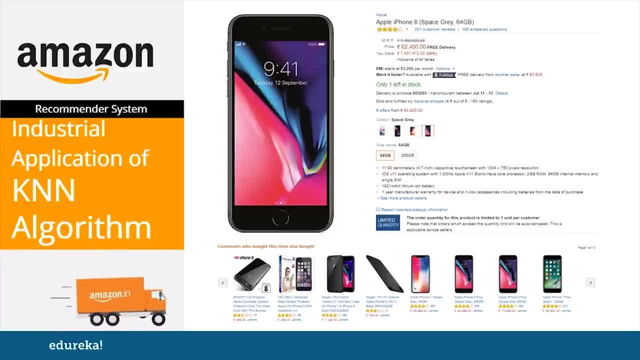 at the bottom of the product page to tempt you into buying the combo. Well, this recommendation has generated a lot of revenue from Amazon. So what's their strategy? Well, the recommendation is just one main goal, that is, increase average order value, or to upsell and cross-sell customers. 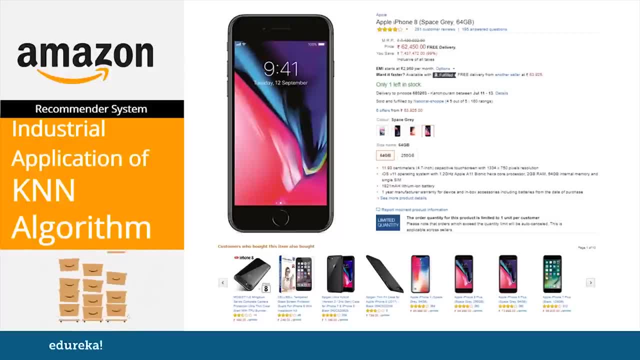 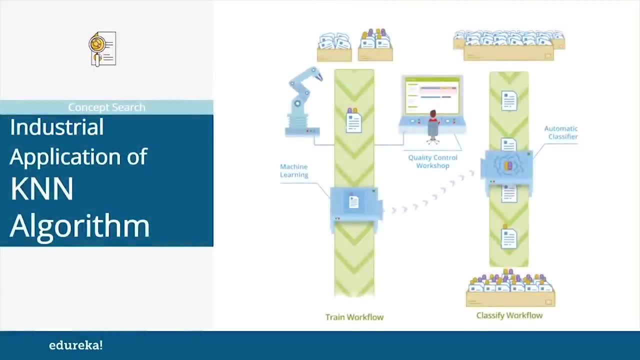 by providing product suggestion based on items in the shopping cart or based on the product they are currently looking at on-site. So next industrial application of KNN algorithm is concept search, or searching semantically similar documents and classifying documents containing similar topics. So, as you know, the data on the internet is increasing exponentially every single. 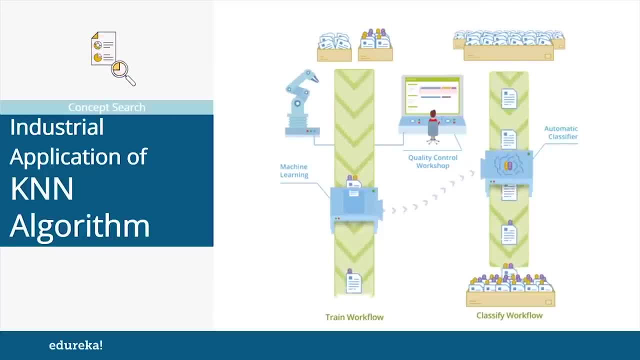 second, There are billions and billions of documents on the internet. Each of the documents on the internet contains multiple concepts that could be a potential concept. Now there's a situation where the main problem is to extract concept from a set of documents, as each page could. 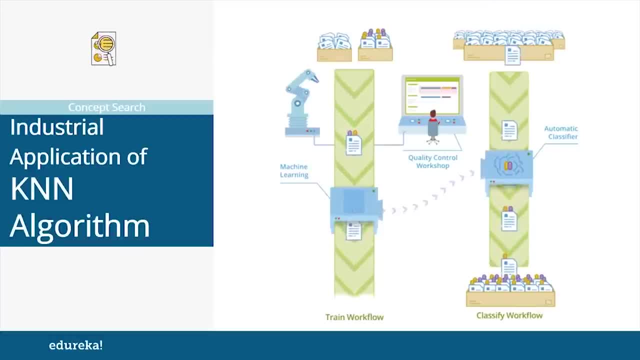 have thousands of combination that could be potential concepts. An average document could have millions of concept. Combine that to the vast amount of data on the web. Well, we are talking about an enormous amount of data set and sample. So what we need here? we need to find a concept. 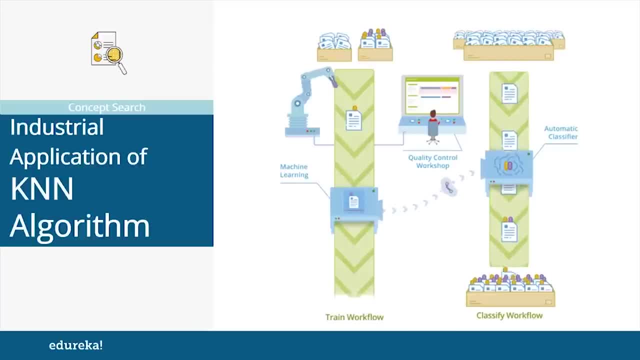 from the enormous amount of data set and samples. right, So for this purpose, we'll be using KNN algorithm. More advanced example could include handwriting detection like an OCR, or image recognition or even video recognition. All right, So now that you know various use cases of KNN. 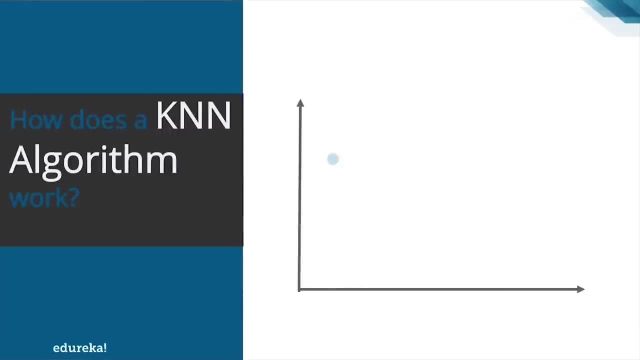 algorithm. let's proceed and see how does it work. So how does a KNN algorithm work? Let's start by plotting these blue and orange point on our graph. So these blue points, they belong to class A, and the orange ones, they belong to class B. Now you get a star as a new point and your task is to 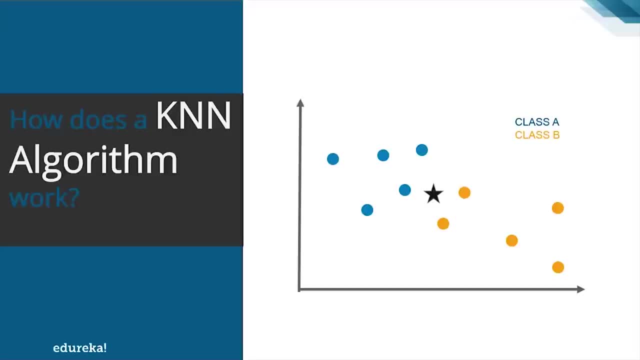 predict whether this new point is going to be a new point or not. So let's start by plotting this point. It belongs to class A or it belongs to class B. So to start the prediction, the very first thing that you have to do is select the value of K. Just as I told you, K in KNN algorithm refers to. 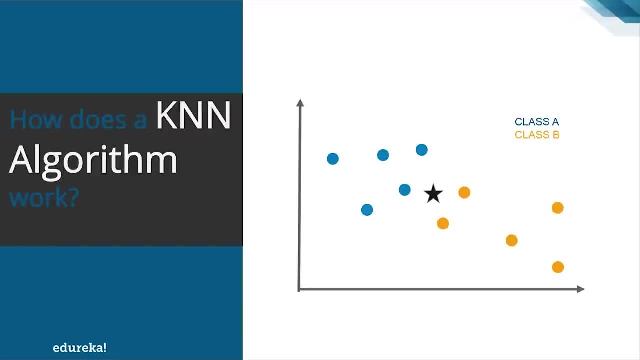 the number of nearest neighbors that you want to select, For example. in this case, K equal 3.. So what does it mean? It means that I'm selecting three points which are the least distance to the new point. Or you can say: I'm selecting three different points which are closest to the star. Well at this. 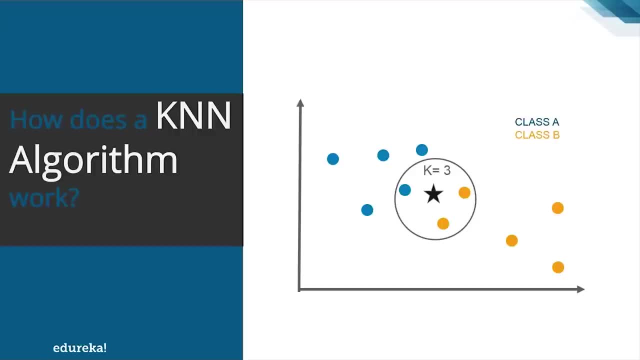 point of time, you can ask: how will you calculate the least distance? So, once you calculate the distance, you'll get one blue and two orange points, which are closest to the star Now, since in this case, as we have a majority of orange points, so you can say that for. 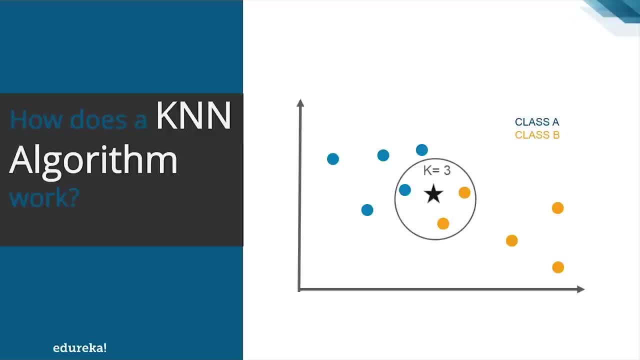 K equal 3, the star belongs to class B, Or you can say that the star is more similar to the orange points Moving on ahead. Well, what if K equal to 6.? Well, for this case, you have to look for six different points which are closest to the star. So, in this case, after calculating the distance, we 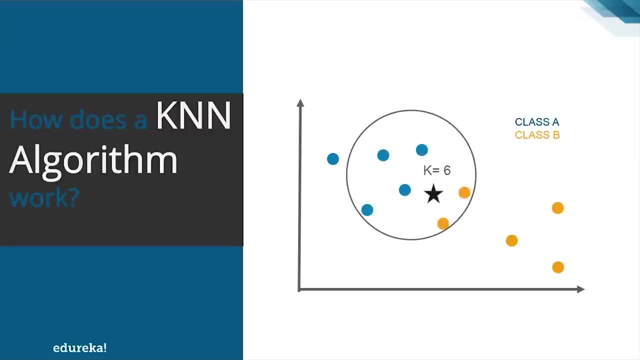 find that we have four blue points which are closest to the star. So in this case, after calculating the distance, we find that we have four blue points and two orange points which are closest to the star. Now, as you can see that the blue points are in majority, So you can say that for K equals 6. 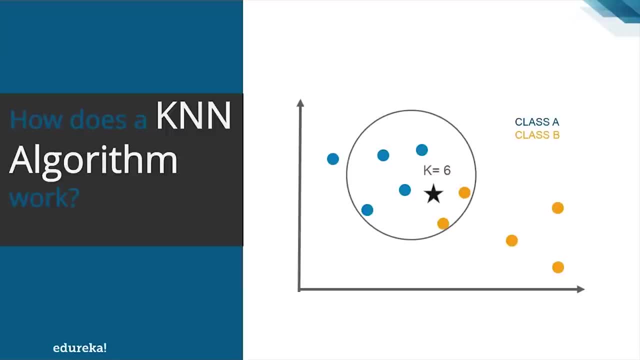 the star belongs to class A, Or the star is more similar to blue points. So by now I guess you know how a K-NN algorithm work and what is the significance of K in K-NN algorithm. So how will you choose the value of K? So, keeping in mind this, K is the most important parameter in K-NN. 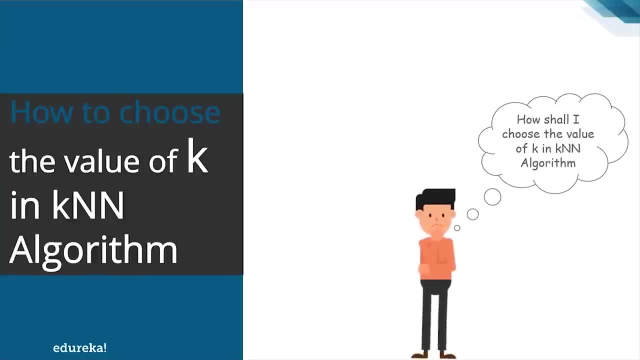 algorithm. So let's see, when you build a K nearest neighbor classifier, how will you choose the value of K? Well, you might have a specific value of K, So you might have a specific value of K, So you might have a specific value of K in mind. or you could divide up your data and use something like cross. 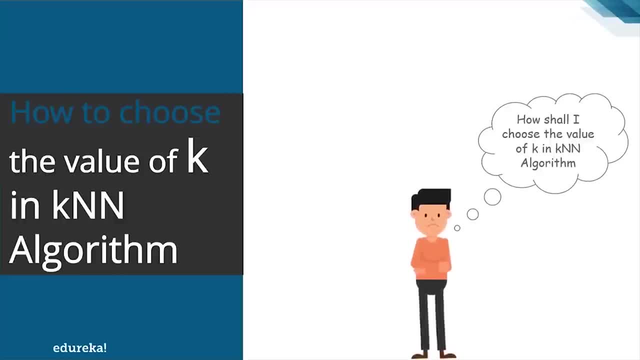 validation technique to test several values of K in order to determine which works best for your data. For example, if N equals 1000 cases, then in that case the optimal value of K lies somewhere in between 1 to 19.. But yes, unless you try it, you cannot be sure of it. So you know how the 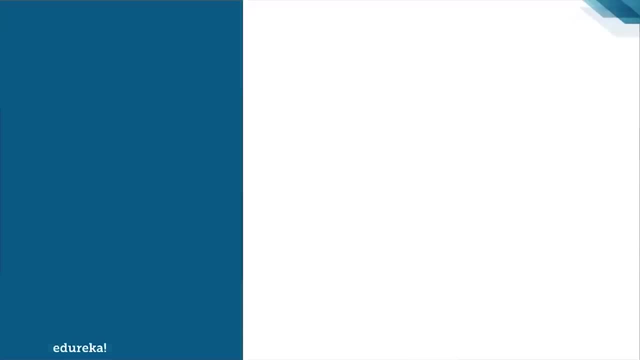 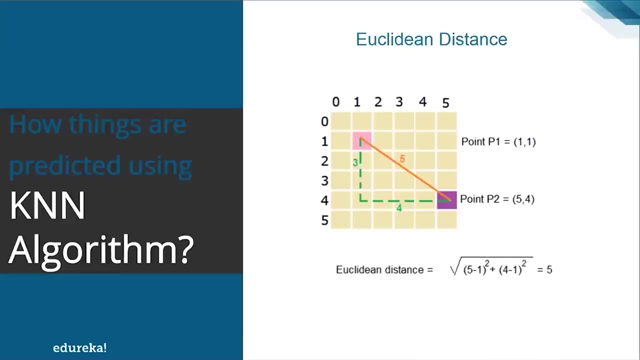 algorithm is working on a higher level. Let's move on and see how things are predicted using K-NN algorithm. Remember I told you: the K-NN algorithm uses the least distance measure in order to find a. K-NN algorithm uses the least distance measure in order to find a. 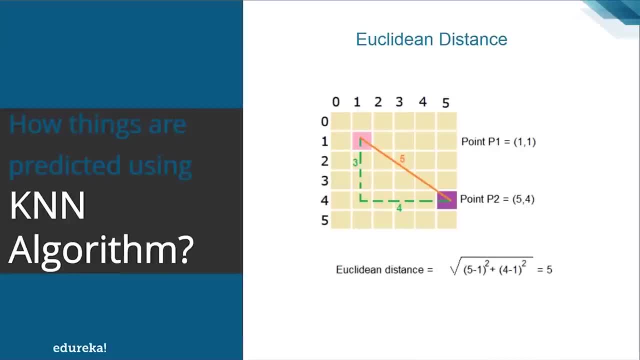 K-NN algorithm uses the least distance measure in order to find a nearest neighbors. So let's see how these distances calculated. Well, there are several distance measures which can be used, so, to start with, I'll mainly focus on Euclidean distance in Manhattan distance in this session. So what is this Euclidean distance? well, 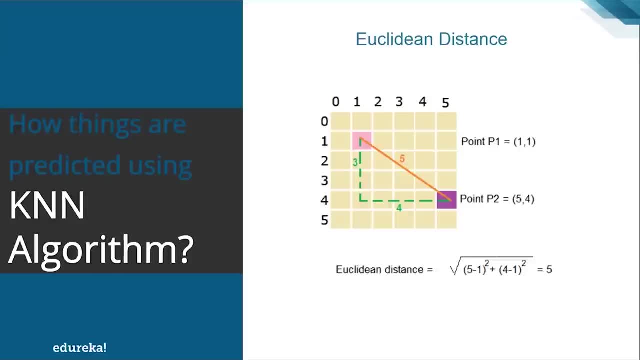 this Euclidean distance is defined as the square root of the sum of difference between a new point x and an existing point y. So, for example, here we have point p 1 and p 2. point p 1 is 1: 1 and point p. 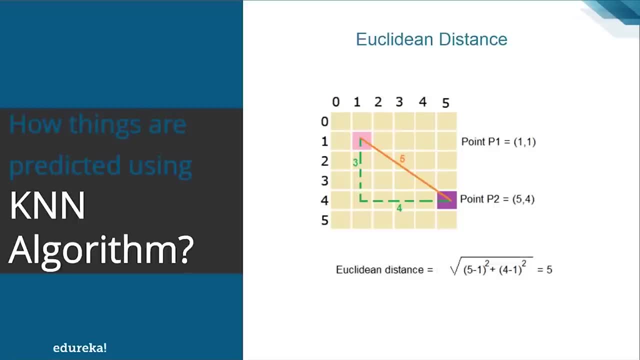 So what is the Euclidean distance between both of them? so you can say that Euclidean distance is a direct distance between two points. So what is the distance between the point P1 and P2? so we can calculate it as 5 minus 1 whole square plus 4 minus 1 whole square and we can root it over which. 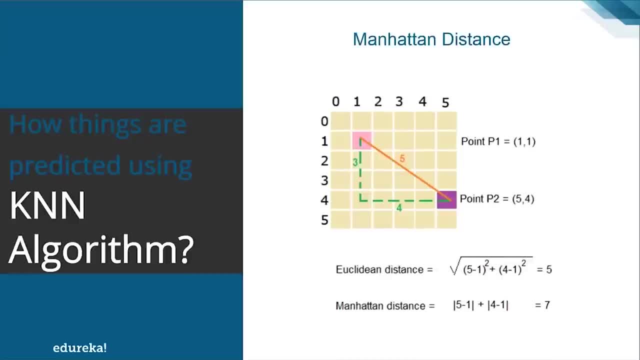 results to 5.. So next is the Manhattan distance. Well, this Manhattan distance is used to calculate the distance between real vector using the sum of their absolute difference. In this case, the Manhattan distance between the point P1 and P2 is mod of 5 minus 1, plus mod value of 4 minus 1. 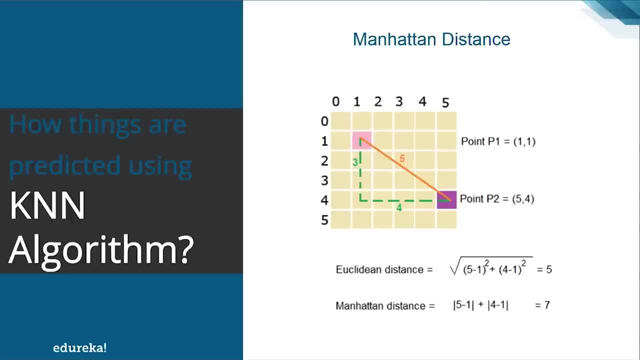 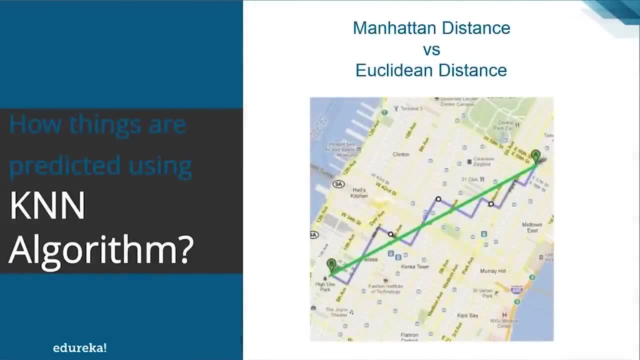 which results to 3 plus 4, that is 7.. So this slide shows the difference between Euclidean and Manhattan distance from point A to point B. So Euclidean distance is nothing but the direct or the least possible distance between A and B, whereas the Manhattan distance is a distance between A and. 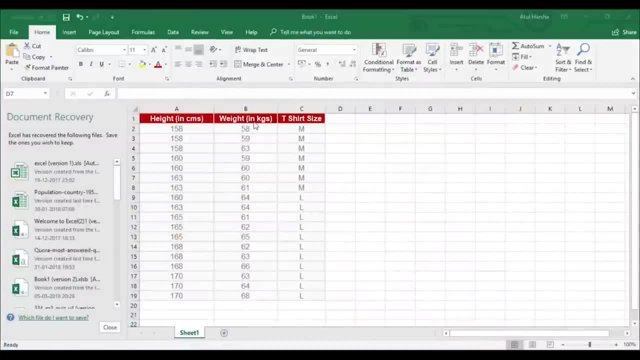 B, measured along the axis at right angle. Let's take an example and see how things are predicted using K-NN algorithm, Or how the K-NN algorithm is working. Suppose we have a data set which consists of height, weight and t-shirt size of some customers. Now, when a new customer come, we only have his height and weight. 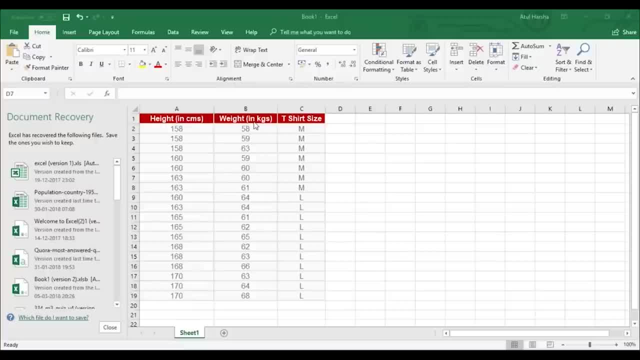 as the information. Now our task is to predict what is the t-shirt size of that particular customer, So for this we'll be using the K-NN algorithm. So, the very first thing, what we need to do, we need to calculate the Euclidean distance. So, now that you have a new data of height, 161 centimeter and 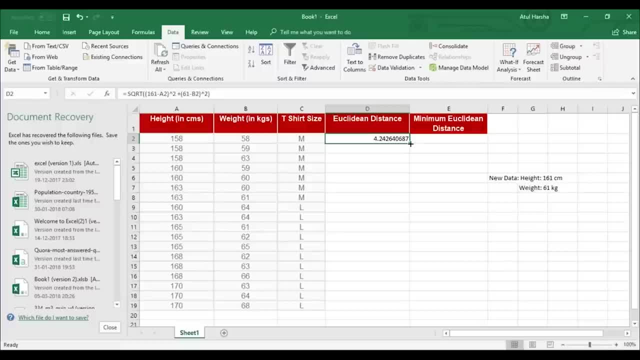 weight as 61 kg. The first thing that we'll do is we'll calculate the Euclidean distance, which is nothing but the square root of 161 minus 158 whole square, plus 61 minus 58 whole square, and square root of that is 4.24.. Let's drag and drop it. So these are the various Euclidean distance of other points Now. 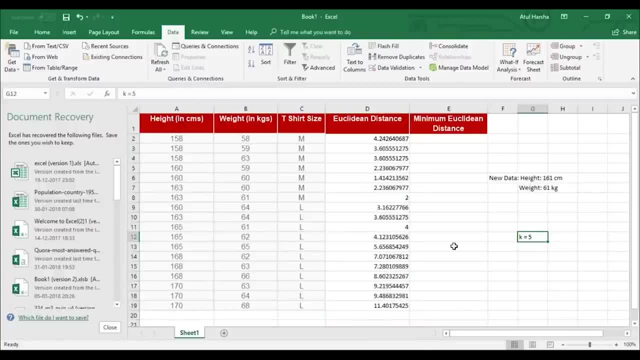 let's suppose K equal to 5. then the algorithm, what it does? it searches for the 5 customer closest to the new customer. That is more similar to the new data in terms of its attribute. For K equal 5, let's find the top 5 minimum Euclidean distance. 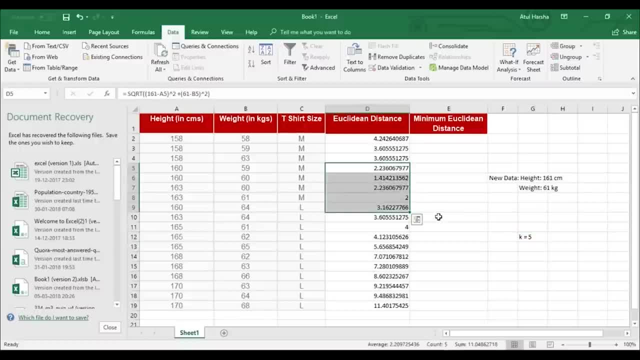 So these are the distance which we are going to use: 1, 2, 3, 4 and 5.. So let's rank them in the order: First this is second, this is third, then this one is 4 and again this one is 5.. So this is our order. 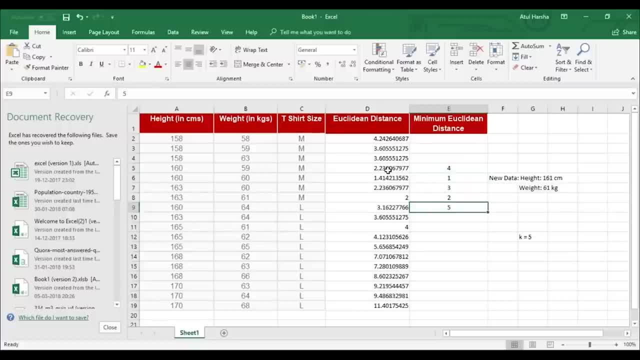 So for K equal 5, we have 4 t-shirts which come under size M and one t-shirt which comes under size L. So obviously best guess or the best prediction for the t-shirt- size of height, 161 centimeter and weight 61 kg- is M. Or you can say that our new customer 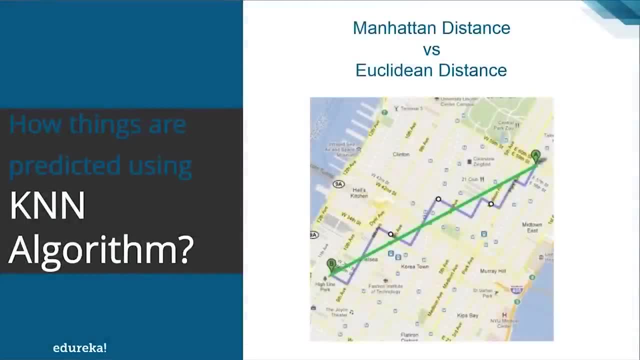 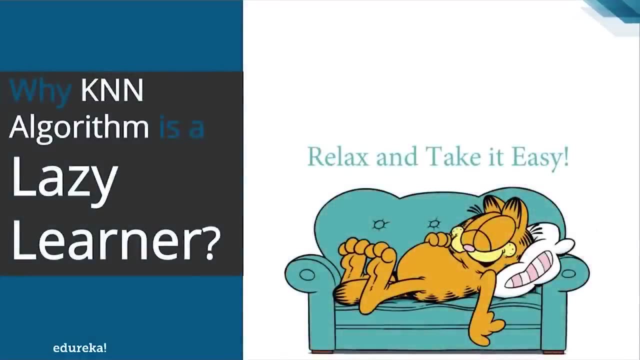 Return to size M. Well, this was all about the theoretical session, But before we drill down to the coding part, let me just tell you why people call K and N as a lazy learner. Well, K and N for classification is a very simple algorithm, but that's not why they are called lazy. K and N is a. 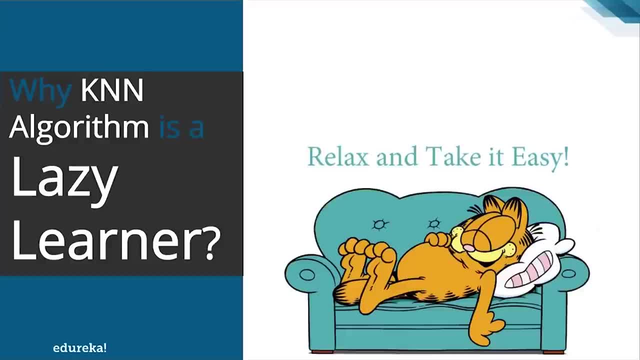 lazy learner because it doesn't have a discriminative function from the training data, But what it does? it memorizes the training data. There is no learning phase of the model and all of the work happens at the time of prediction is requested. So, as such, there's the reason why K and N is often. 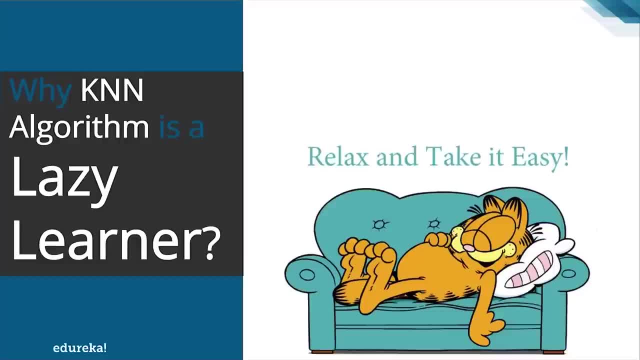 referred to as lazy learner. So let's say that we have a training data. So let's say that we have a learning algorithm. So this was all about the theoretical session. Now let's move on to the coding part. So for the practical implementation of the hands-on part, I'll be using the artist. 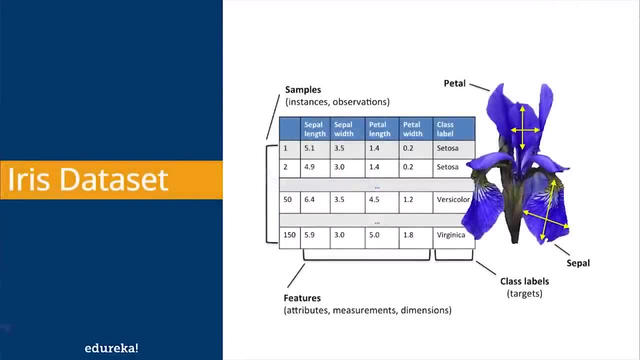 data set. So this data set consists of 150 observation. We have four features and one class label. The four features include the sepal length, the sepal width, petal length and the petal width, whereas the class label decides which flower belongs to which category. So this was the 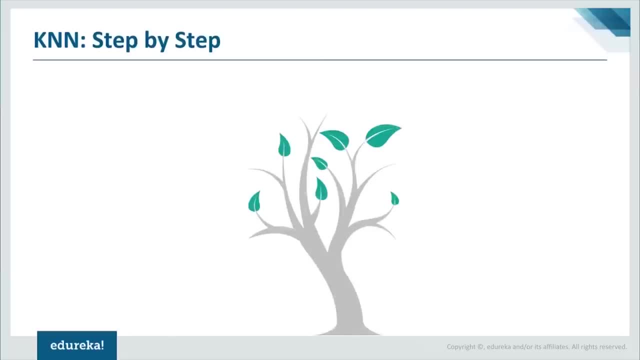 description of the data set which we are using. Now let's move on and see what are the step-by-step solution to perform a K and N algorithm. So first we'll start by handling the data. What we have to do? we have to open the data set from. 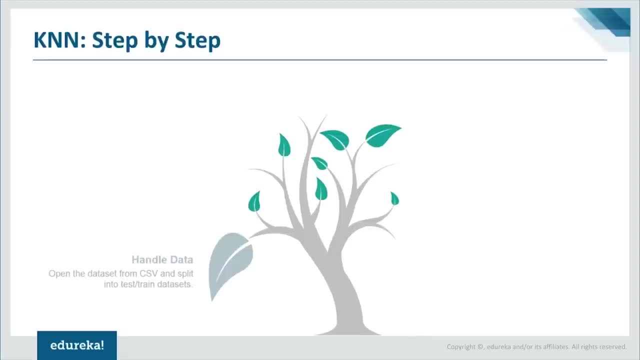 the CSV format and split the data set into train and test part. Next we'll check the similarity where we have to calculate the distance between two data instances. Once we calculate the distance, next we'll look for the neighbor and select K neighbors which are having the least distance. 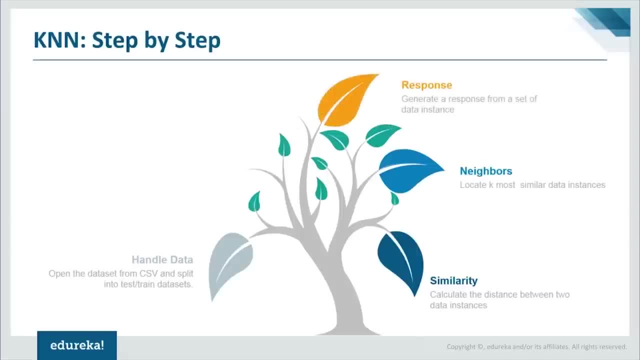 from a new point. Now, once we get our neighbor, then we'll generate a response from a set of data instances. So this will decide whether the new point belongs to class A or class B. Finally, we'll create the accuracy function and in the end we'll tie it all together in the main. 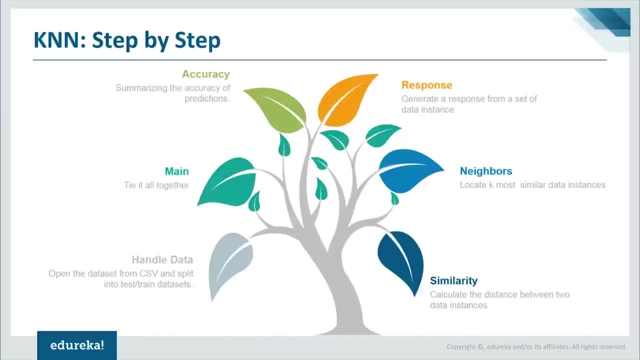 function. So let's start with our code For implementing K and N algorithm using Python. I'll be using Jupyter Notebook, Python 3.0 installed on it. Now let's move on and see how K and N algorithm can be implemented using Python. So there's my Jupyter Notebook, which is a web-based 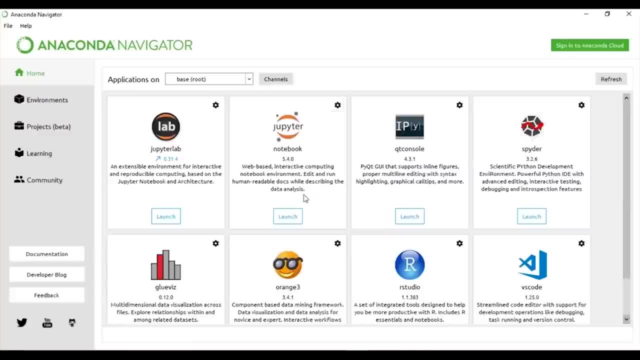 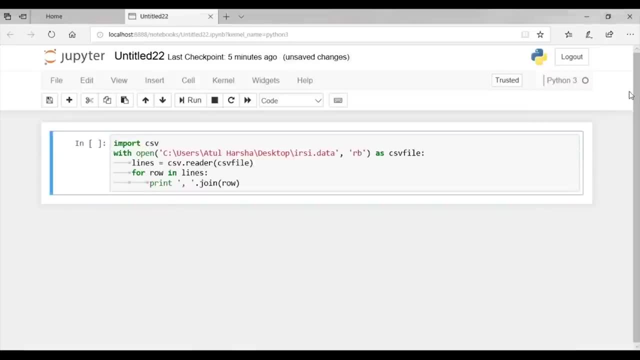 interactive computing notebook environment with Python 3.0 installed on it. So the launch? yeah, it's launching. So there's our Jupyter Notebook and we'll be writing our Python codes on it. The next thing that we need to do is load our file. Our data is in CSV format without a header line. 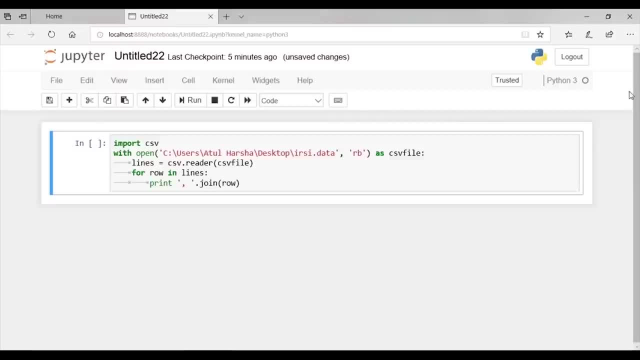 or any code. We can open the file, the open function, and read the data line using the reader function in the CSV module. So let's write a code to load our data file. Let's execute the run button. So once you execute the run button, you can see the entire training data set as the output. 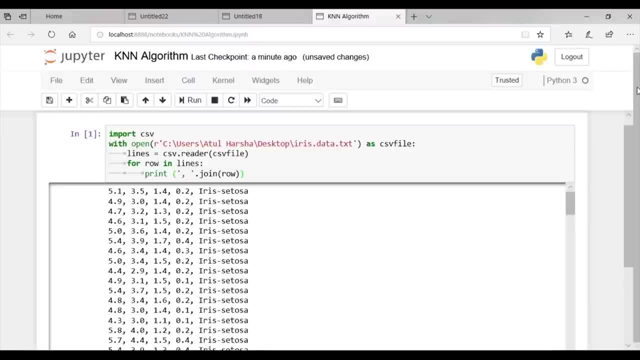 Next, we need to split the data into a training data set that K and N can use to make prediction and a test data set that we can use to evaluate the accuracy of the model. So we first need to convert the flower measure that were loaded as string into numbers that we 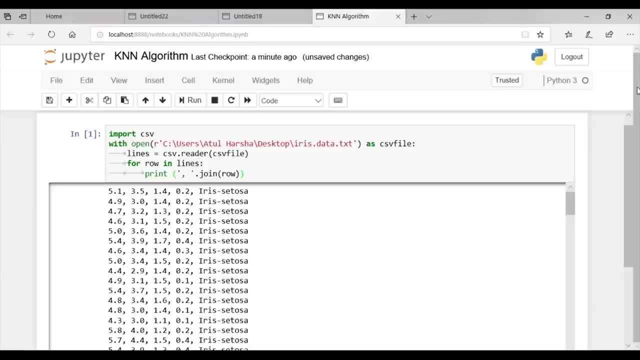 can work. Next, we need to split the data set randomly to train and test. A ratio of 67 is to 33 for test is to train is a standard ratio which is used for this purpose. So let's define a function as load data set that loads a CSV with a provided file name and split it randomly into. 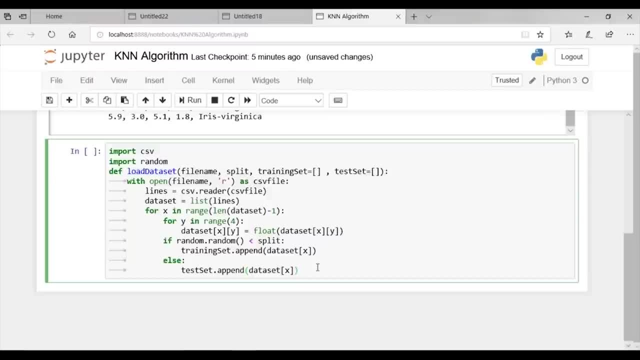 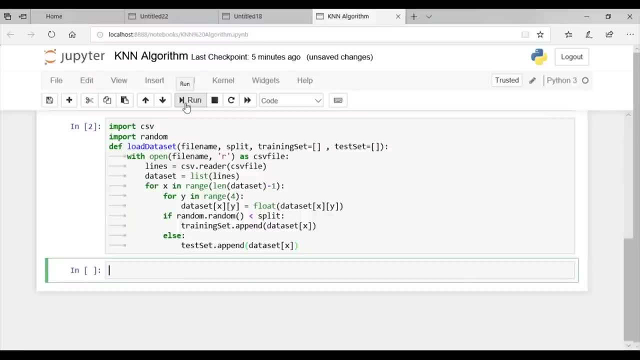 training and test data set using the provided split ratio. So this is our function: load data set, which is using file name, split ratio, training data set and testing data set as its input. All right, so let's execute the run button and check for any errors. So it's executed with zero. 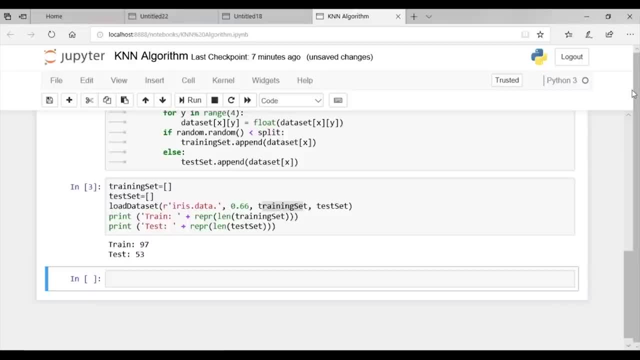 errors. Let's test this function. So there's our training set testing set. load data set. So this is our function: load data set and inside that we are passing our file iris data with a split ratio of 0.66 and training data set and test data set. Let's see what our training data set and test. 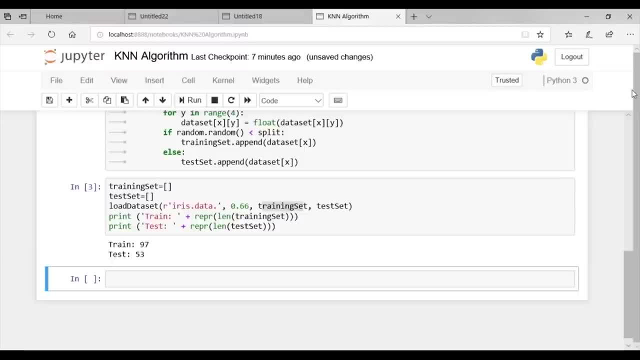 data set it's dividing into. So it's giving a count of training data set and testing data set. the total number of training data set it has split into is 97 and total number of test data set we have is 53. So total number of training data set we have here is 97 and total number 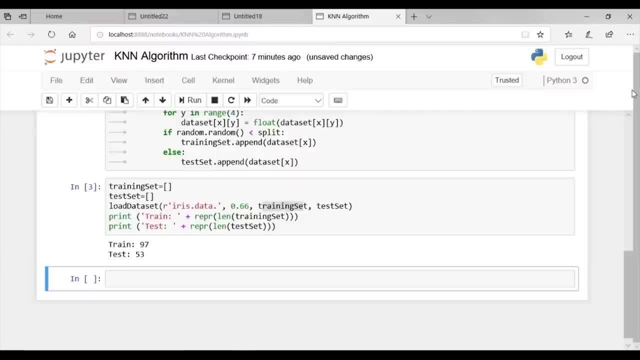 of test data set we have here is 53.. All right, Okay, so our function- load data set- is performing well. So let's move ahead to step two, which is similarity. So, in order to make prediction, we need to calculate the similarity between any two given data instances. This is needed. 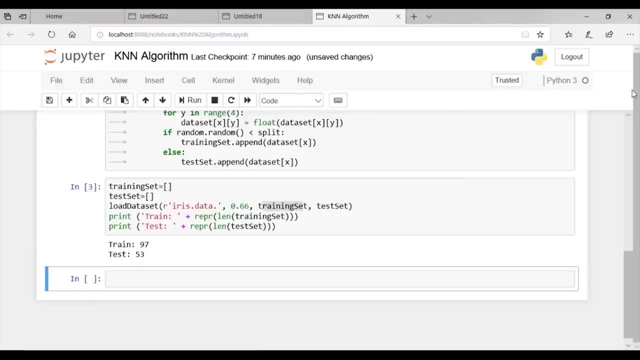 so that we can locate the K most similar data instances in the training data set and in turn make a prediction. given that all four flower measurement are numeric and have same unit, We can directly use the Euclidean distance measure, which is nothing but the square root. 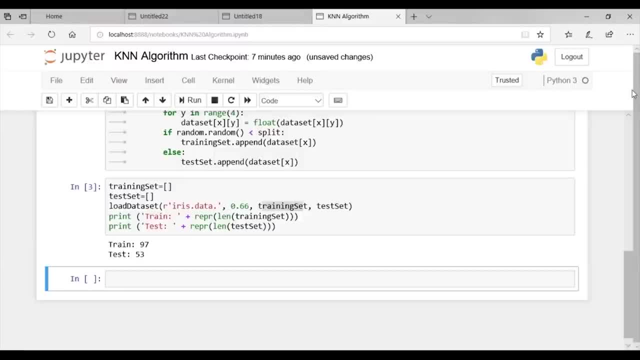 of the sum of squared differences between two arrays of the number. given that all the four flower measurements are numeric and have same unit, We can directly use the Euclidean distance measure, which is nothing but the square root of the sum of squared difference between two arrays of the number. Additionally, we want to control which field to include. 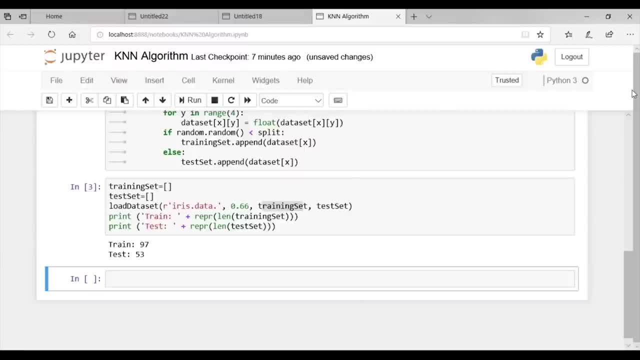 in the distance calculation. So specifically, we only want to include first four attribute. So our approach will be to limit the Euclidean distance to a fixed length. All right, so let's define our Euclidean function. So this is our Euclidean distance function, which takes: 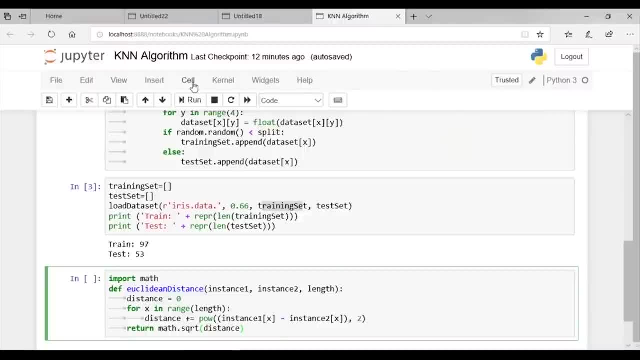 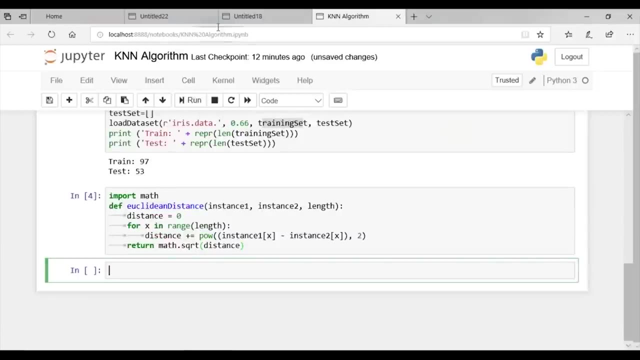 instance one, instance two and length as parameters. instance one and instance two are the two points of which you want to calculate the Euclidean distance, whereas this length, and they know that how many attributes you want to include. Okay, so there's our Euclidean function. Let's execute it. It's executing fine, without any errors. Let's test the function. 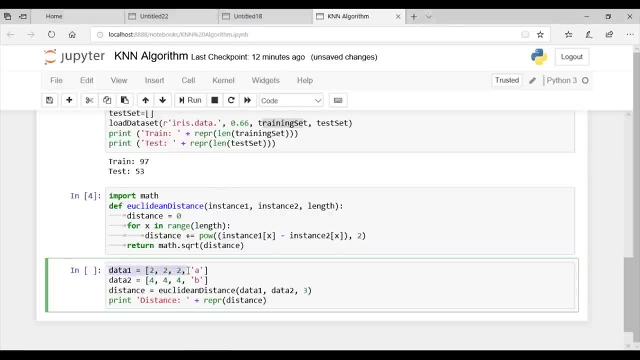 suppose the data one or the first instance consists of data point as 2 to 2 and it belongs to class A, Data to consist of 444 and it belongs to class B. So when we calculate the Euclidean distance of data 1 to data 2 and what we have to do, we have to consider only first three features. 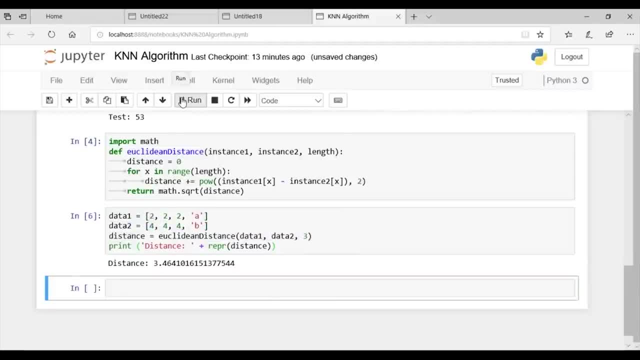 of them. All right, so let's print the distance. as you can see here, the distance comes out to be 3.464.. All right, so this is nothing but the square root of 4 minus 2, whole square. So this distance is nothing but the Euclidean distance and it is calculated as square root. 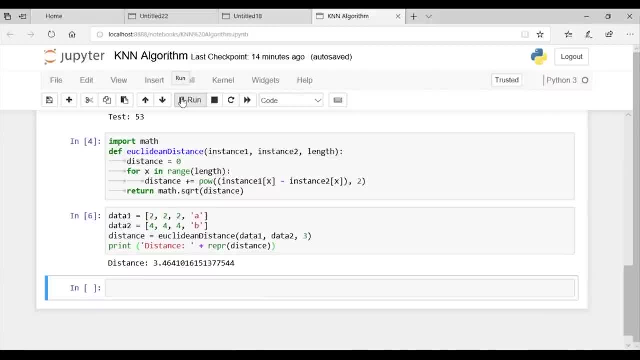 of 4 minus 2 whole square, plus 4 minus 2 whole square, that is nothing but 3 times of 4 minus 2 whole square, That is 12, and square root of 12 is nothing but 3.464.. All right, so now that we have. 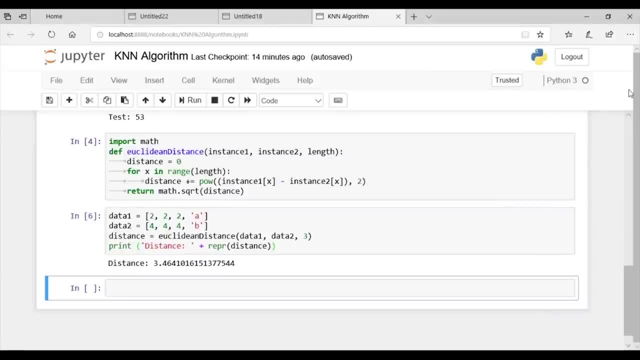 calculated the distance. now we need to look for K nearest neighbors. now that we have a similarity measure, we can use it to collect the K most similar instances for a given unseen instance. Well, this is a straightforward process of calculating the distance for all the instances. 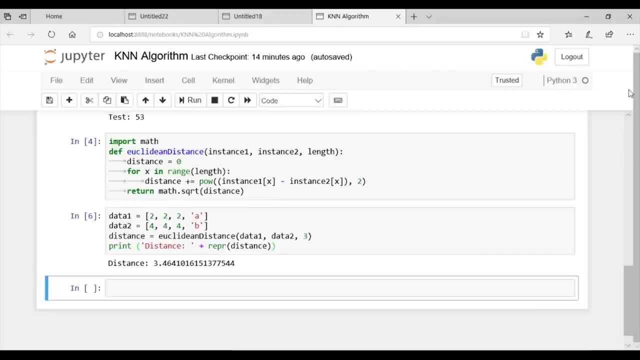 and selecting a subset with the smallest distance value. and now what we have to do? we have to select the smallest distance values, So for that, we'll be defining a function as get neighbors. So for that, what we'll be doing, we'll be defining a function as get neighbors. 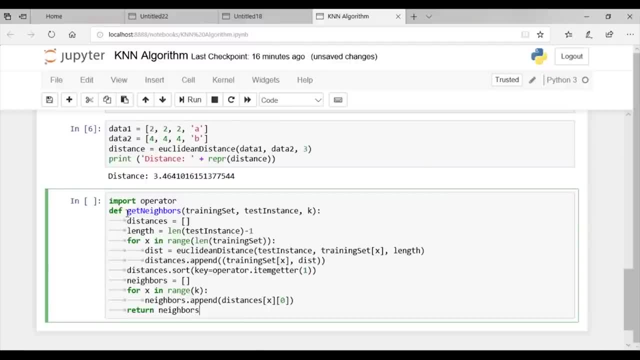 What it will do. it will return the K most similar neighbors from the training set for a given test instance. All right, so this is how our get neighbors function look like. it takes training data set and test instance and K as its input. here The K is nothing. 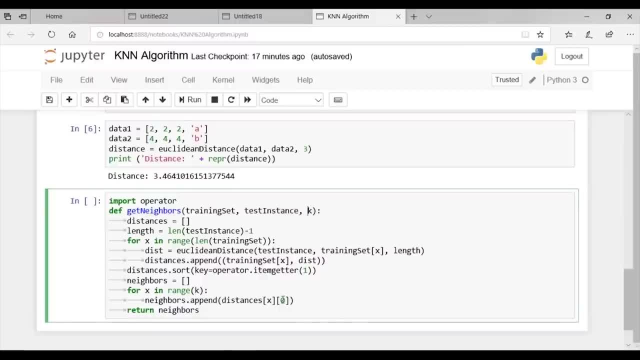 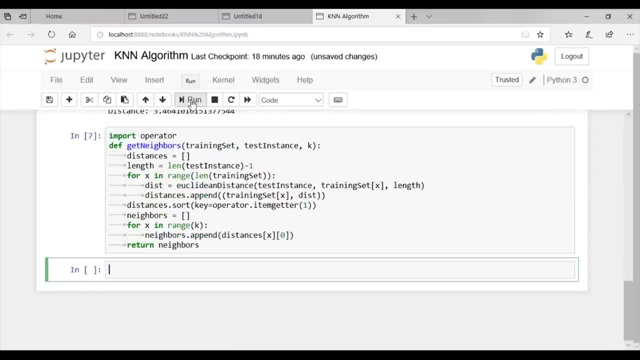 but the number of nearest neighbor you want to check for. All right, so basically, what you'll be getting from this get neighbors function is K different points having least Euclidean distance from the test instance. All right, let's execute it. So the function. 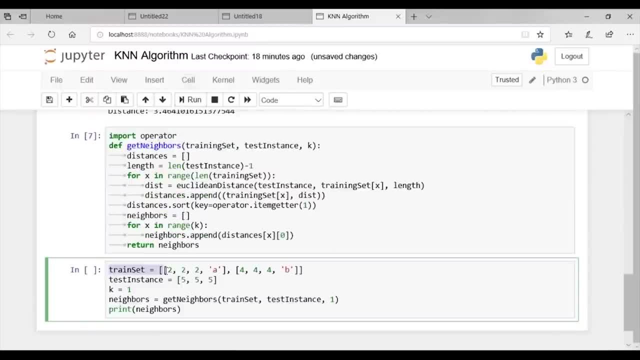 executed without any errors, So let's test our function. So suppose the training data set includes the data like 2, 2, 2 and it belongs to Class A, and other data includes 4, 4, 4 and it belongs to Class B, and our testing instances 555 or 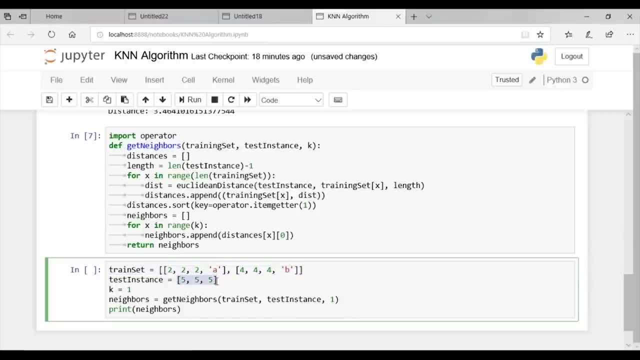 now we have to predict whether this test instance belongs to Class A or it belongs to Class B. All right. for K equal 1, we have to predict its nearest neighbor and predict whether this test instance it will belong to Class A or will it belong to Class B, All right, so let's 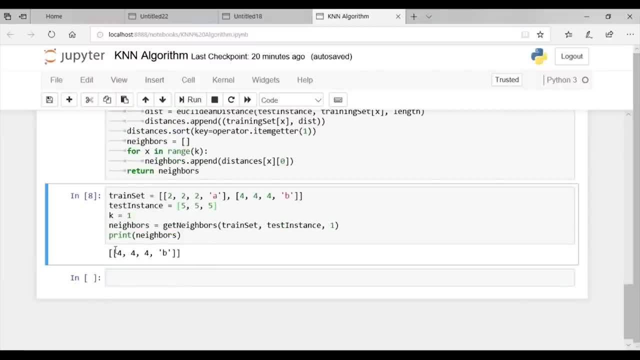 execute the run button. All right. So in executing the run button, you can see that we have output as 4, 4, 4 and B. Our new instance, 555, is closest to point 4, 4, 4, which belongs to Class B. All right Now. 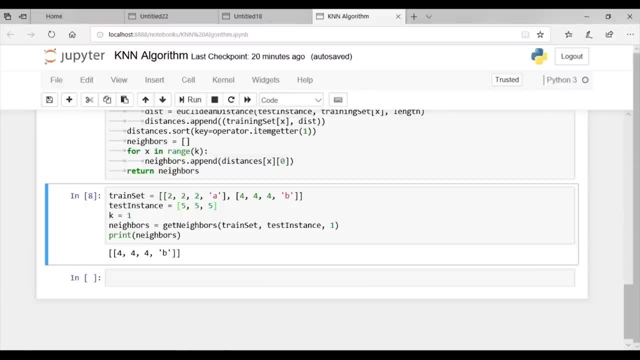 once you are located the most similar neighbor for a test instance, next task is to predict a response based on those neighbors. So how we can do that? Well, we can do this by allowing each neighbor to vote for the class attribute and take the majority vote as a prediction. 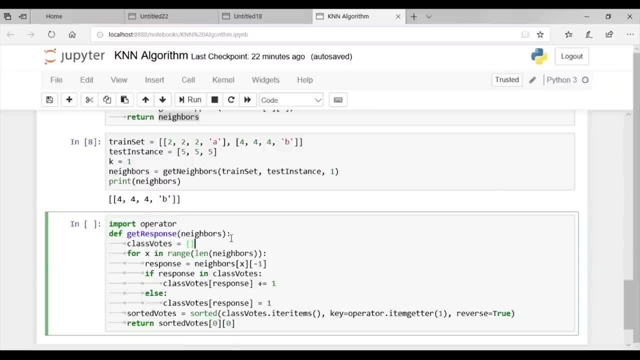 Let's see how we can do that. So we have a function as get response, which takes neighbors as the input. Well, this neighbor was nothing but the output of this get neighbor function. The output of get neighbor function was nothing but the output of this get neighbor function. 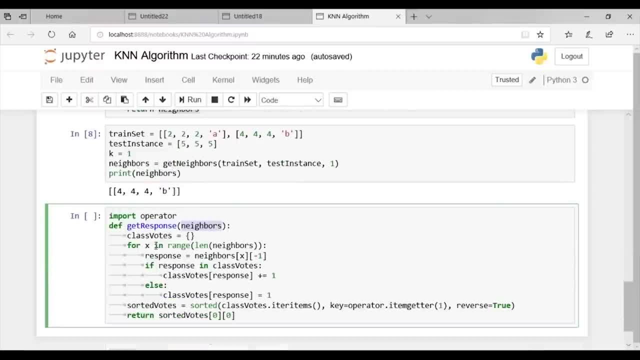 The output of get neighbor function was nothing, but the output of this get neighbor function. The output of get neighbor function was nothing, but the output of this get neighbor function will be fed to get response. All right, let's execute the run button. It's executed. Let's. 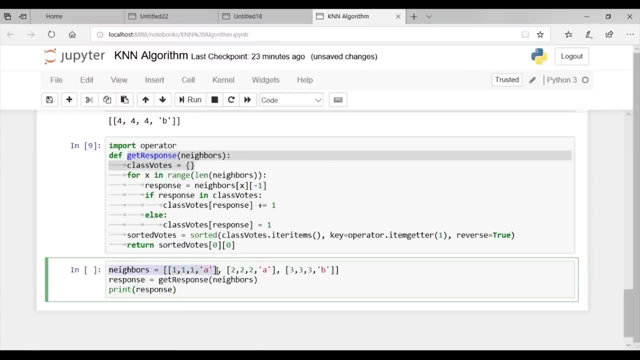 move ahead and test our function. get response. So we have a neighbor. as 1, 1, 1, it belongs to Class A. 2, 2, 2, it belongs to Class A. 3, 3, 3, it belongs to Class B. So this response what? 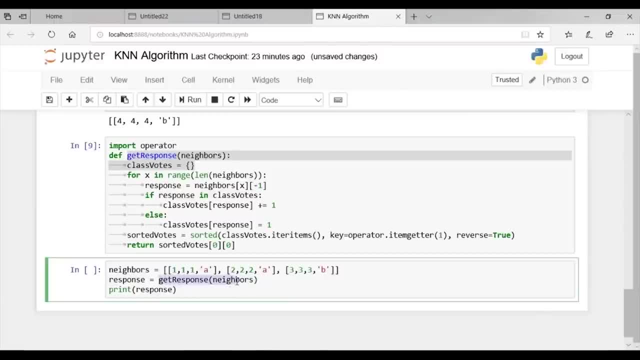 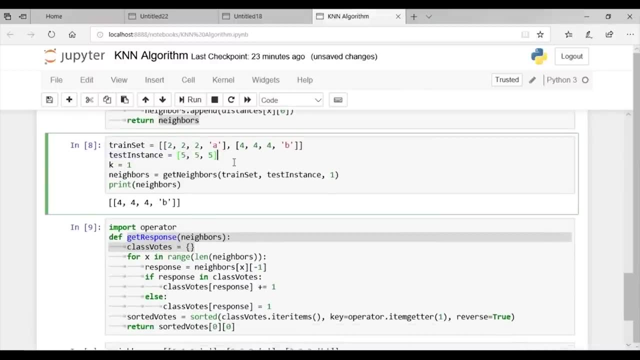 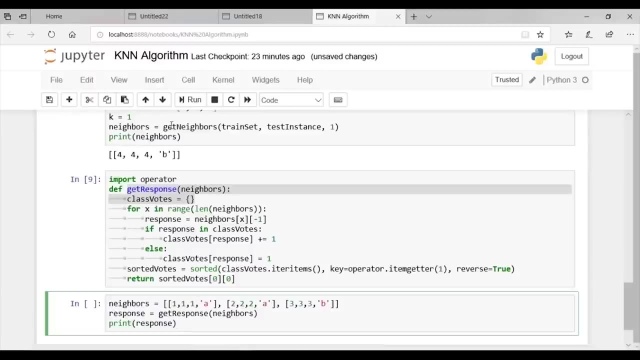 it will do will store the value of get response by passing this neighbor value. All right, So what we want to check is we want to predict whether that test instance 555, it belongs to Class A or Class B When the neighbors are 1, 1, 1 A, 2, 2, 2 A and 3, 3, 3 B. So let's check our response Now that we have created all. 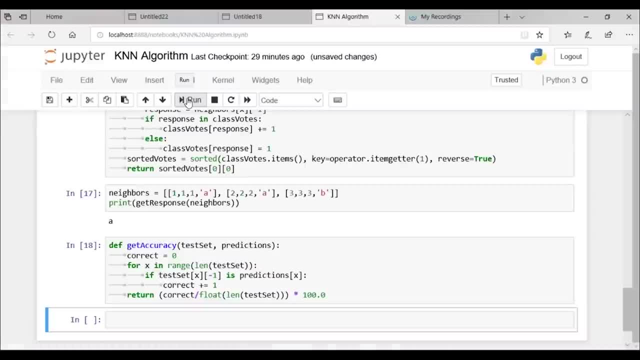 the different function which are required for a canon algorithm. So important main concern is how to evaluate the accuracy of the prediction, and easy way to evaluate the accuracy of the model is to calculate a ratio of the total correct prediction to all the prediction made. So for this I'll be defining function as get accuracy and inside that I'll be passing my 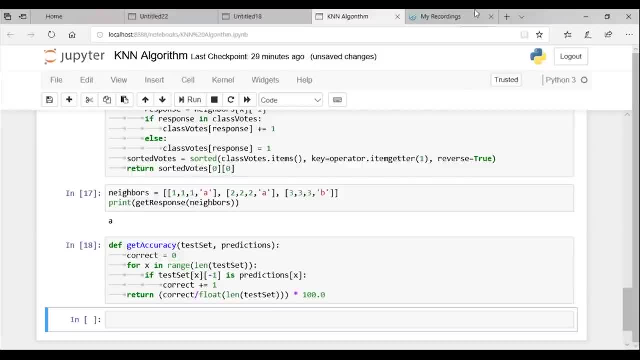 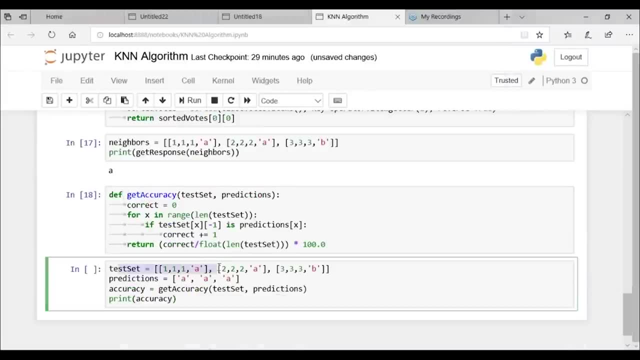 test data set and the predictions get accuracy function, check it, execute it without any error. let's check it for a sample data set. So we have our test data set as 1, 1, 1, which belongs to Class A, 2, 2, 2, which again belongs. 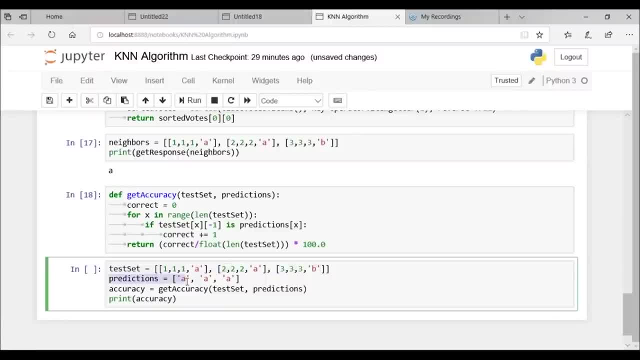 to Class 3, 3, 3, which belongs to Class B, and my predictions is: for first test data, It predicted that it belongs to Class A, which is true. for next, it predicted that belongs to Class A, which is again true. and for the next, again, it predicted that it belongs to 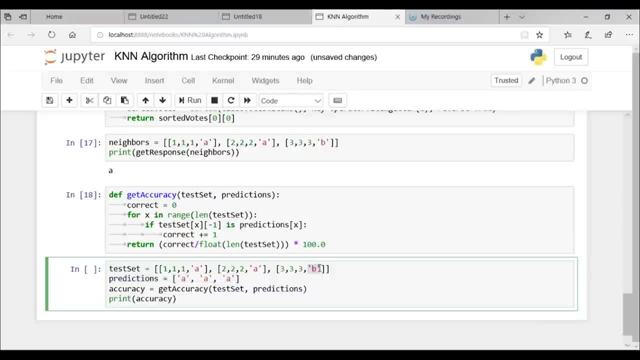 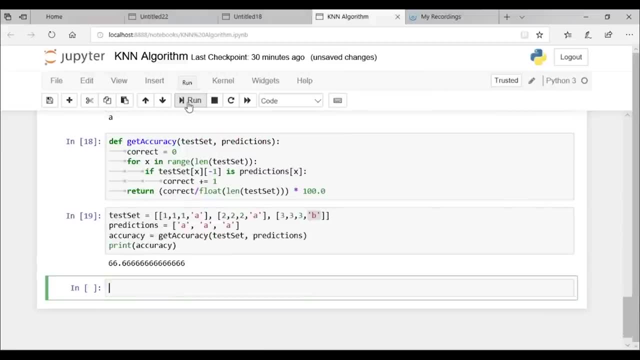 Class A, which is false in this case because the test data belongs to Class B. All right, So in total, we have two correct prediction out of three. All right, So the ratio will be 2 by 3, which is nothing but 66.66.. So our accuracy rate is 66.66.. So now that you 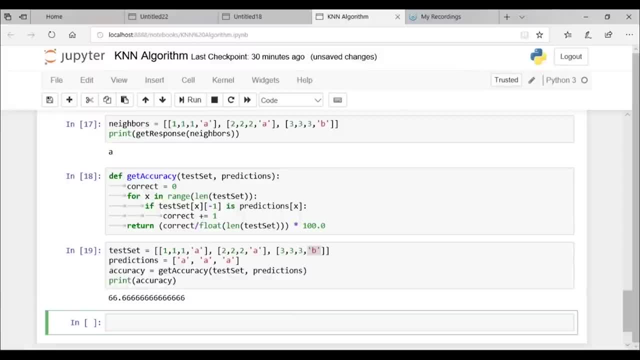 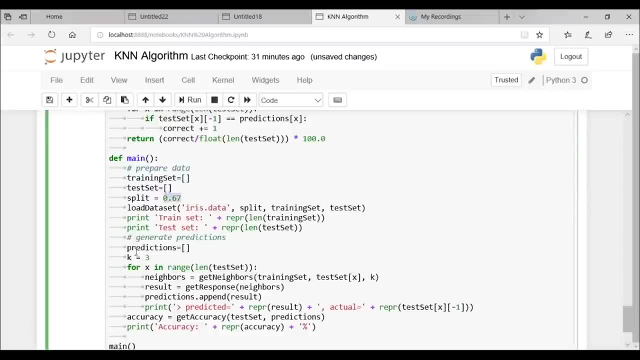 have created all the function that are required for K&N algorithm. let's compile them into one single main function. All right, So there's our main function, and we are using iris data set with a split of 0.67 and the value of K is 3.. Let's see what is the accuracy score. 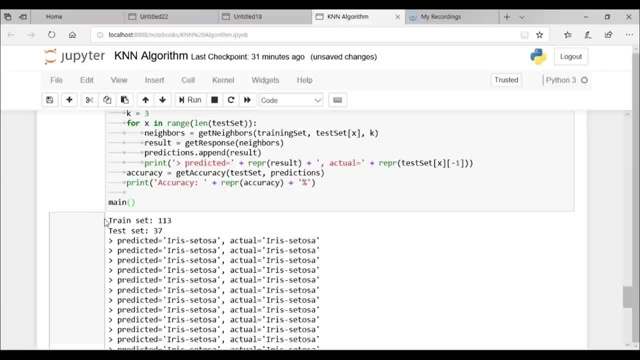 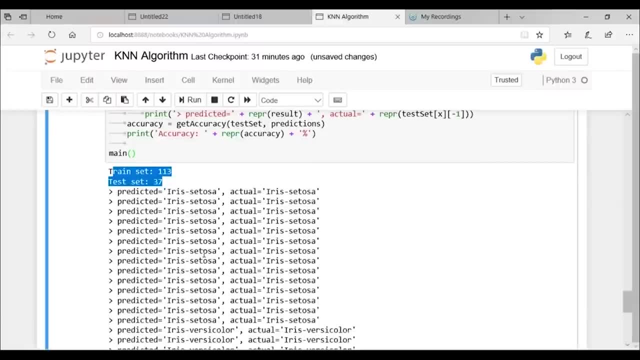 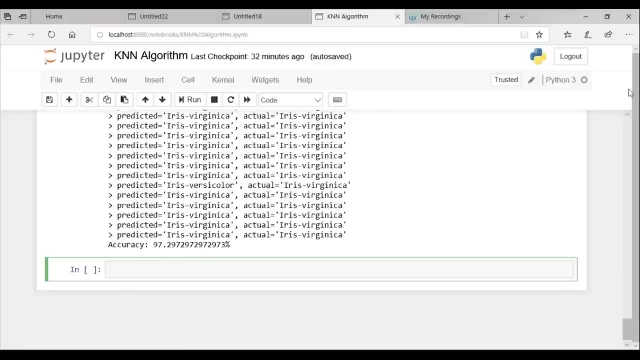 of this check how accurate our model is. So in training data set we have 113 values and in the test data set we have 37 values, And these are the predicted and the actual values of the output. Okay, So in total we got an accuracy of 97.29%, which is really very good. All right, So I hope the concept 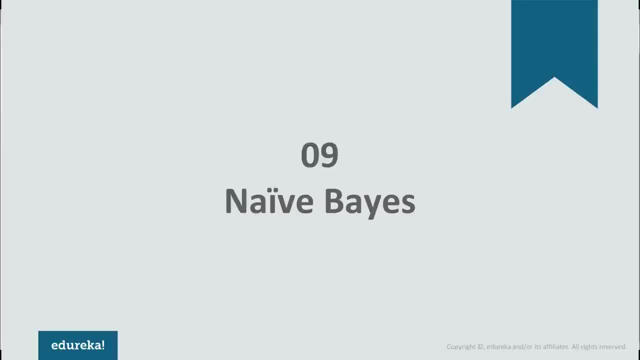 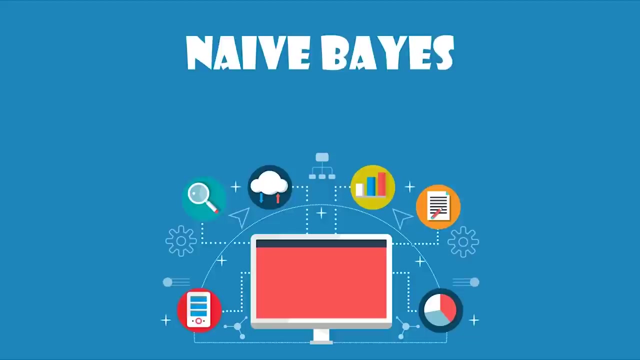 of this K&N algorithm is clear to you guys. In a world full of machine learning and artificial intelligence surrounding almost everything around us, classification and prediction is one of the most important aspects of machine learning. So before moving forward, let's have a quick look at the agenda. 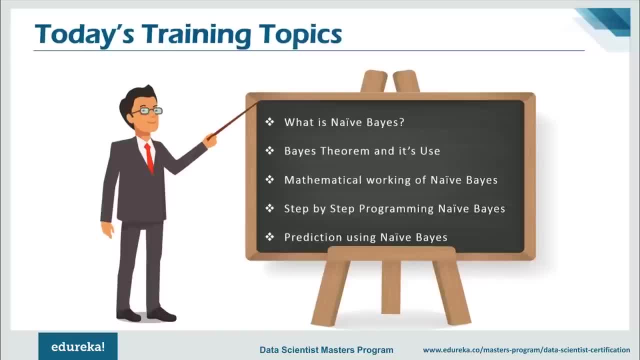 I'll start off this video by explaining you guys what exactly is naive bias. Then we'll understand what is Bayes Theorem, which serves as a logic behind the naive bias algorithm. moving forward, I'll explain the steps involved in the naive bias algorithm one by one, and 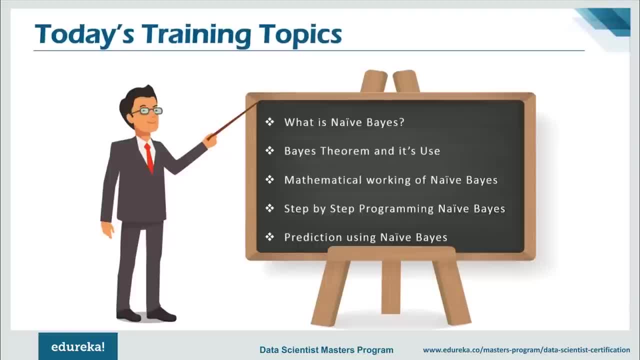 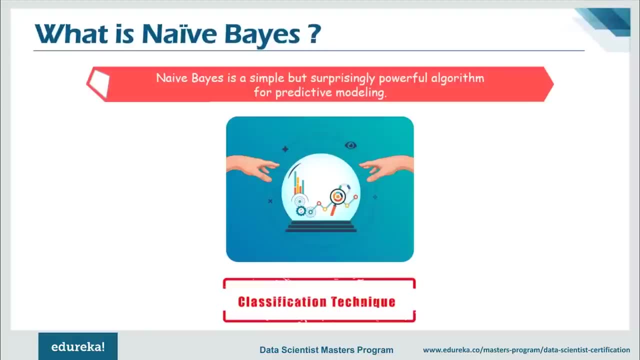 finally, I'll finish off this video with a demo on the naive bias using the sklearn package. Now, naive bias is a simple but surprisingly powerful algorithm from predictive analysis. It is a classification technique based on Bayes Theorem With an assumption of independence among predictors. It comprises of two parts, which 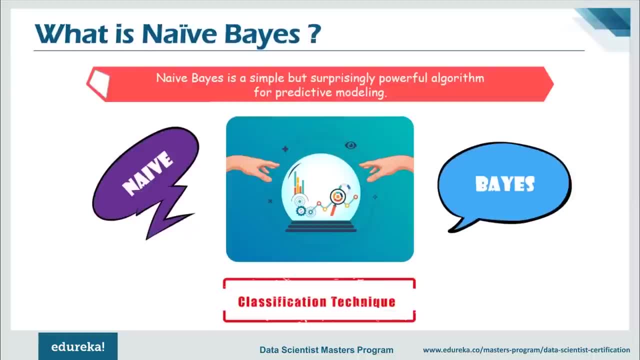 is naive and bias. In simple terms, naive bias classifier assumes that the presence of a particular feature in a class is unrelated to the presence of any other feature, Even if these features depend on each other or upon the existence of the other features. all of these properties independently contribute to the probability whether a fruit is an apple. 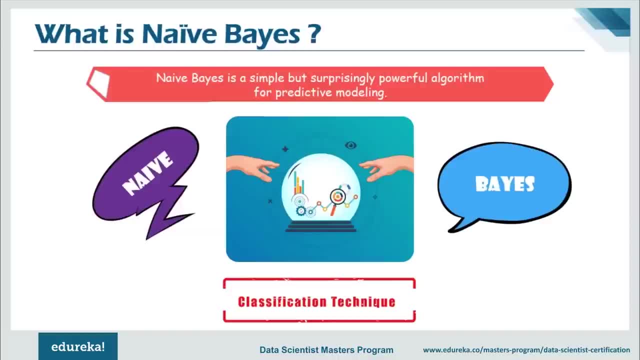 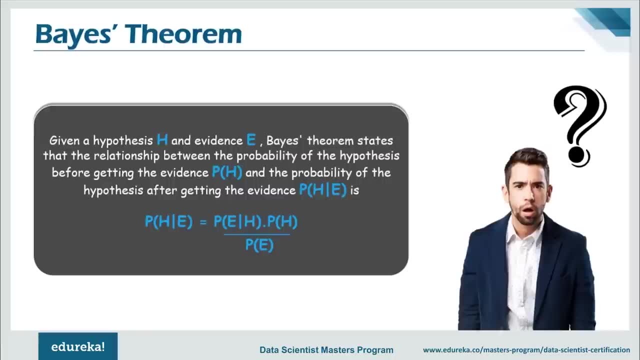 or an orange or a banana, So that is why it is known as naive. Now, naive based model is easy to build and particularly useful for very large data sets. In probability theory and statistics, Bayes Theorem, which is alternatively known as the Bayes law or the Bayes rule, describes the probability of an event based 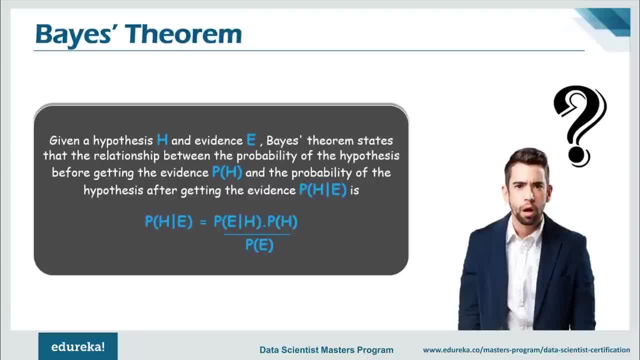 on prior knowledge of the conditions that might be related to the event. Now, Bayes Theorem is a way to figure out conditional probability. The conditional probability is the probability of an event happening, given that it has some relationship to one of the conditions or more other events. For example, your probability of getting a parking space. 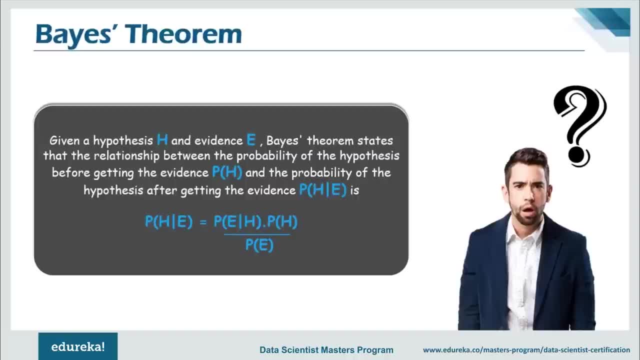 is connected to the time of the day you park, where you park and what conventions are you going on at that time. Bayes Theorem is slightly more nuanced. In a nutshell, it gives you an actual probability of an event, given information about the tests. 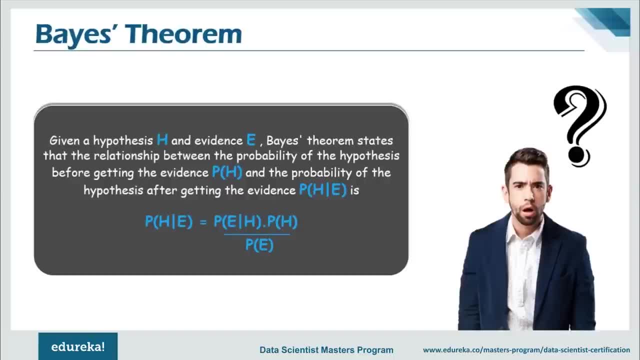 Now, if we look at the definition of Bayes Theorem, we can see that, given a hypothesis H and the evidence E, Bayes Theorem states that the relationship between the probability of the hypothesis before getting the evidence, which is the P, and the probability 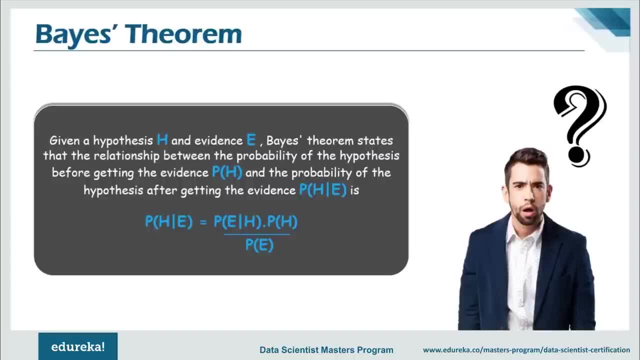 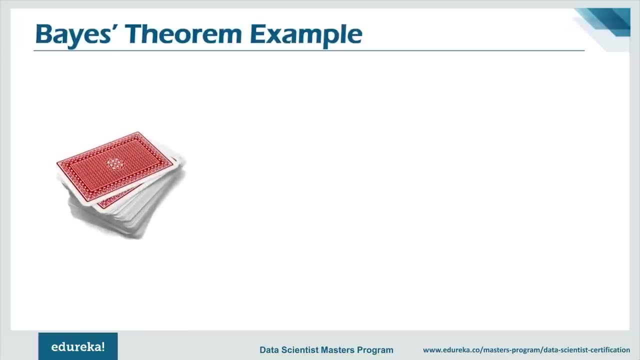 of the hypothesis after getting the evidence, that is, P is defined as probability of E given H into probability of H divided by probability of E. It's rather confusing, right? So let's take an example to understand this theorem. So suppose I have a deck of cards. 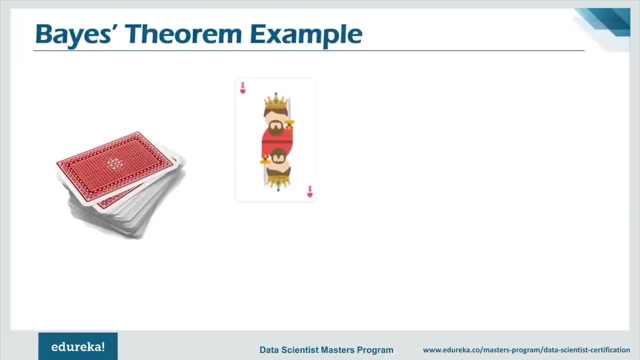 and if a single card is drawn from the deck of playing cards, the probability that the card is a king is 4 by 52. Since there are four kings in a standard deck of 52 cards. Now if king is an event, this: 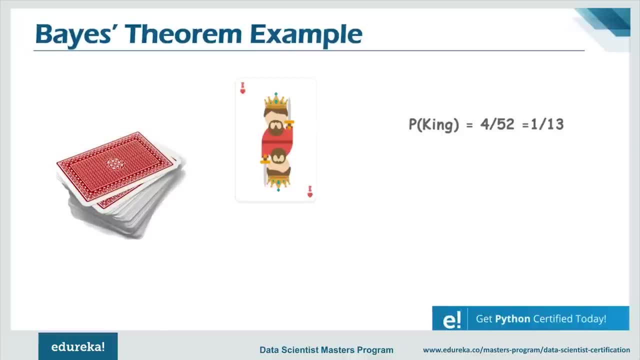 card is a king, the probability of king is given as 4 by 52, that is equal to 1 by 13.. Now if the evidence is provided- for instance, someone looks at the card- that the single card is a face card, The probability of king, given that it's a face, can be calculated. 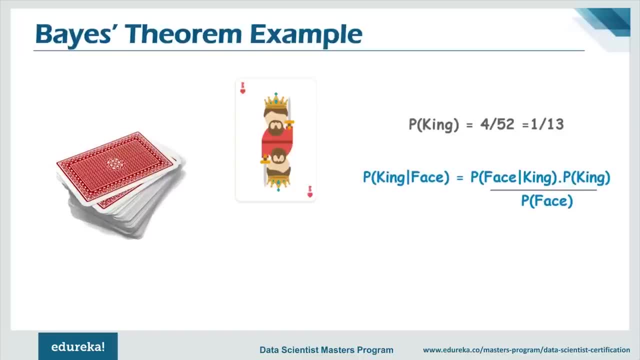 using the Bayes Theorem. by this formula Now, since every king is also a face card, each face card, the probability of face- given that it's a king, is equal to one. and since there are three face cards in each suit, that is, the jack, king and queen, the probability of the face card is equal to. 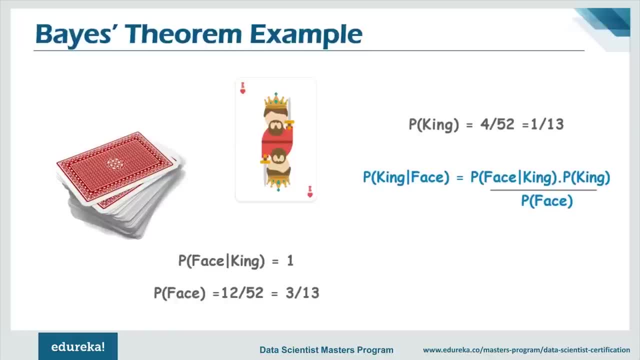 12 by 52, that is, 3 by 30. now, using Bayes theorem, we can find out the probability of king, given that it's a face. so our final answer comes to 1 by 3, which is also true. so if you have a deck of cards, 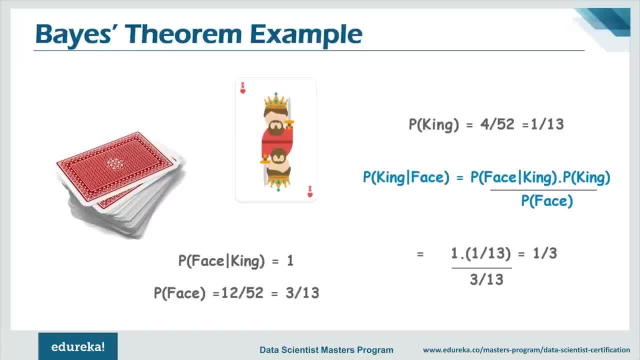 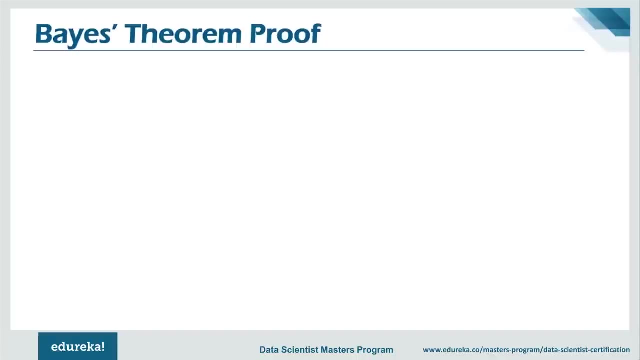 which has having only faces. now there are three types of faces, which are the jack, king and queen. so the probability that it's a king is 1 by 3. now this is the simple example of how Bayes theorem works. now if we look at the proof as in how this Bayes theorem evolved. so here we have probability. 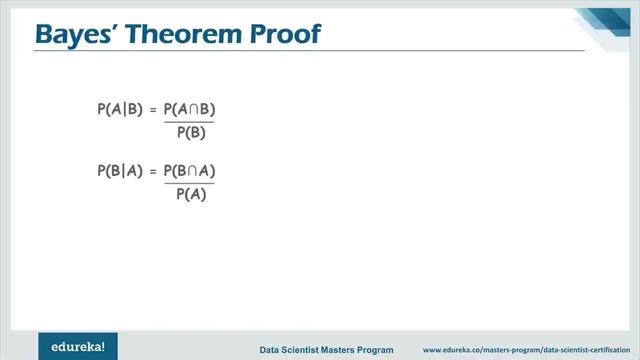 of a given b and probability of b given a. now for a joint probability distribution over the sets a and b: the probability of a intercalated probability of a intercalated probability of a intercalated probability of a intersection b. the conditional probability of a given b is defined as the probability of a. 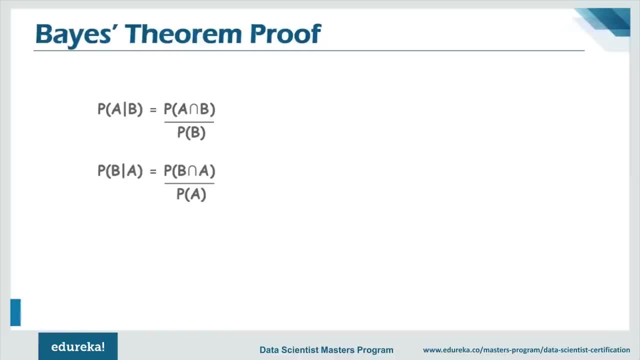 intersection b divided by probability of b, and similarly, probability of b given a is defined as probability of b intersection a divided by probability of a. now we can equate probability of a intersection b and probability of b intersection a, as both are the same thing. now from. 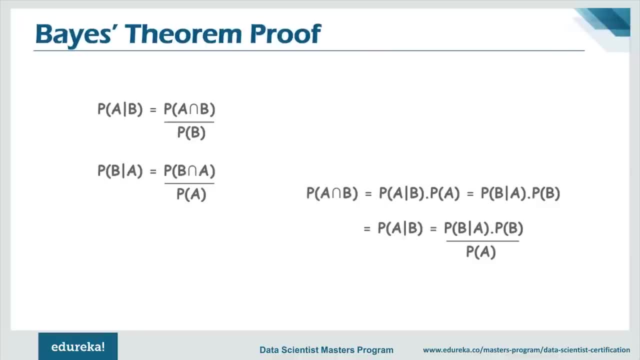 this method, as you can see, we get our final Bayes theorem proof, which is: the probability of a given b equals probability of b given a into probability of b divided by the probability of a. now, while this is the equation that applies to any probability distribution over the events a and b, 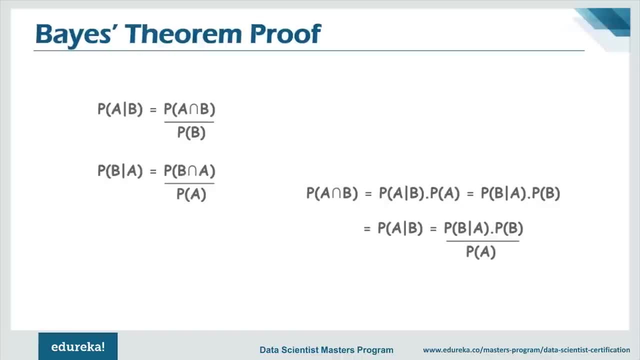 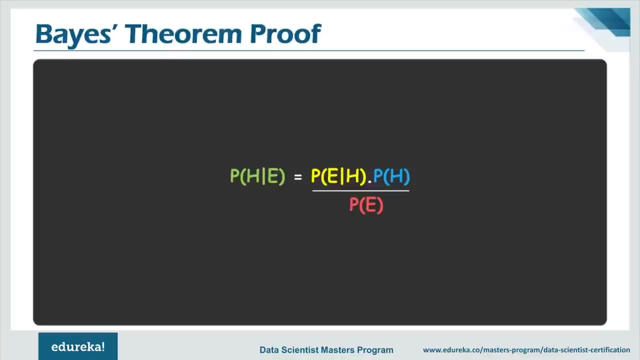 it has a particular nice interpretation in case where a is represented as the hypothesis h and b is represented as some observed evidence e. in that case the formula is p of h, given e is equal to p of e, given h into probability of b and b is represented as some observed evidence e in that. 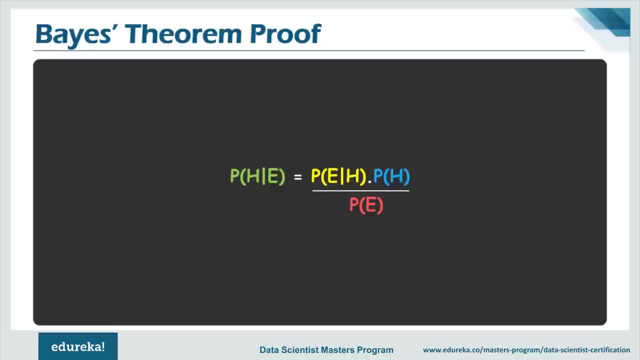 case probability of h divided by probability of e. now this relates the probability of hypothesis before getting the evidence, which is p of h, to the probability of the hypothesis after getting the evidence which is p of h, given e. for this reason p of h is known as the prior probability, while p of h 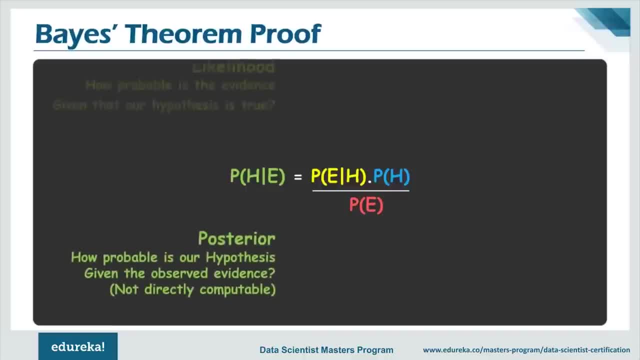 given e is known as the posterior probability and the factor that relates the two is known as the likelihood ratio. now, using this terms, Bayes theorem can be rephrased as the procedure: probabilitybar probability equals the probability of b来� Ven, the prior probability times the likelihood ratio. 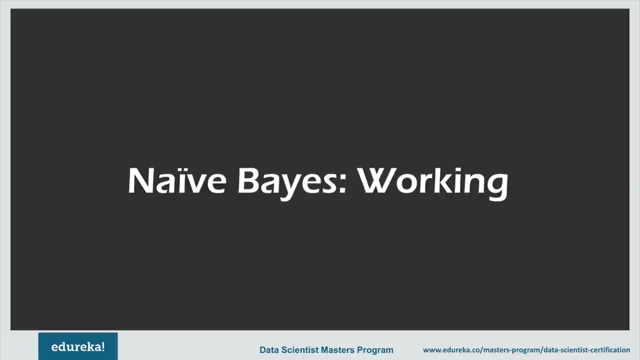 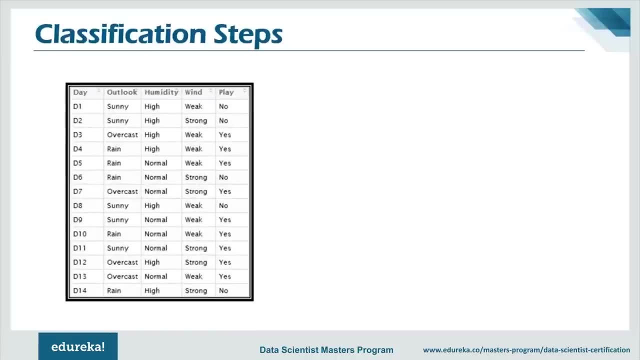 So now that we know the maths which is involved behind the Bayes theorem, let's see how we can implement this in a real life scenario. So suppose we have a data set in which we have the outlook, the humidity, and we need to find out whether we should play. 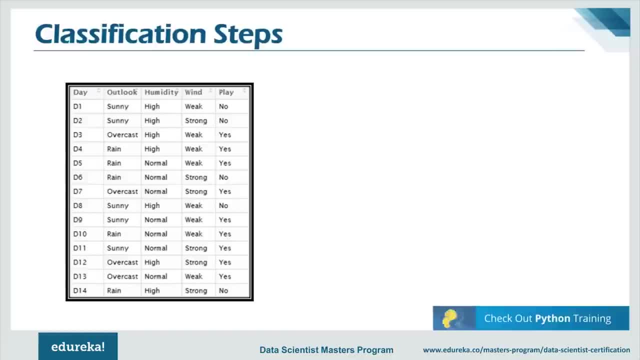 or not on that day. So the outlook can be sunny, overcast, rain and the humidity are high, normal, and the wind are categorized into two features, which are the weak and the strong winds. The first of all. we'll create a frequency table. 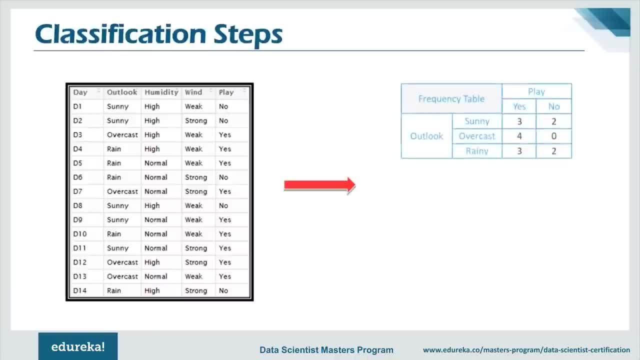 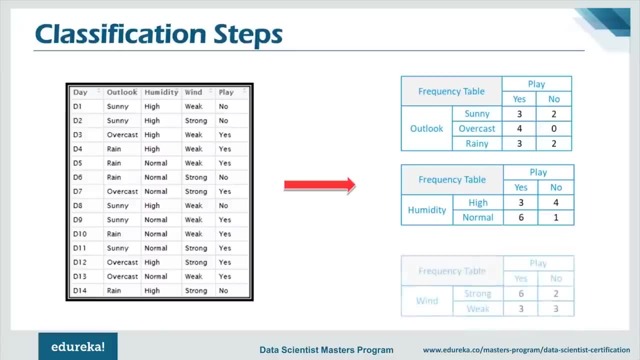 using each attribute of the data set. So the frequency table for the outlook looks like this: We have sunny, overcast and rainy. The frequency table of humidity looks like this and the frequency table of wind looks like this: We have strong and weak for wind. 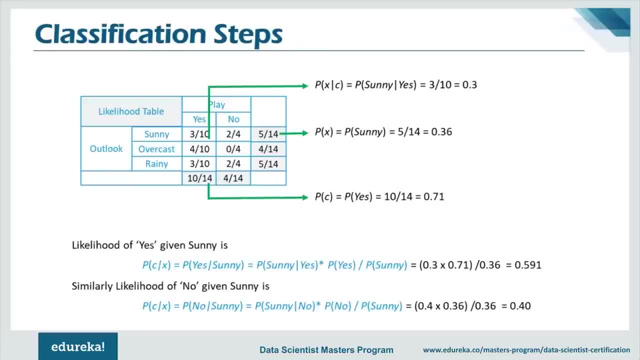 and high and normal ranges for humidity. So for each frequency table we will generate a likelihood table now. Now the likelihood table contains the probability of a particular day. Suppose we take the sunny and we take the play as yes and no. So the probability of sunny, given that we play, yes, 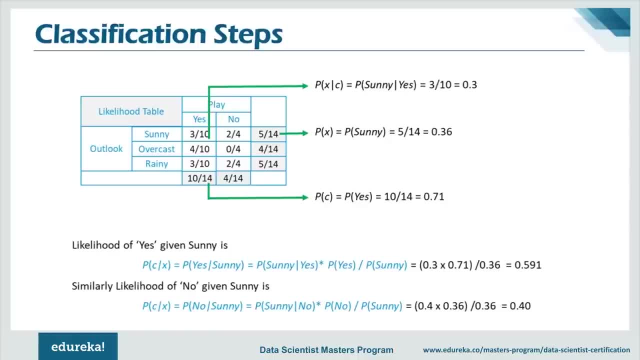 is three by 10, which is 0.3.. The probability of X, which is the probability of sunny, is equal to five by 14.. Now, these are all the terms which are just generated from the data which we have here. 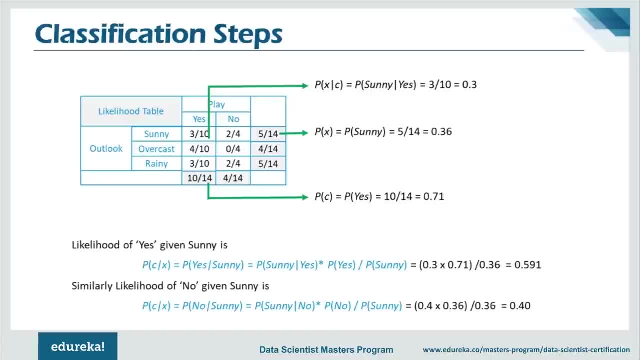 And finally, the probability of yes is 10 out of 14.. So if we have a look at the likelihood of yes, given that it's a sunny, we can see using Bayes' theorem, it's the probability of sunny given yes into probability of yes divided by the probability of sunny. 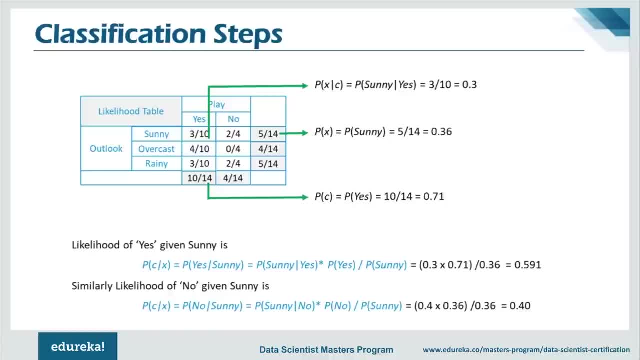 So we have all the values here calculated. So if we put that in our Bayes' theorem equation, we get the likelihood of yes as 0.59.. Similarly the likelihood of no can also be calculated here, It's 0.40. 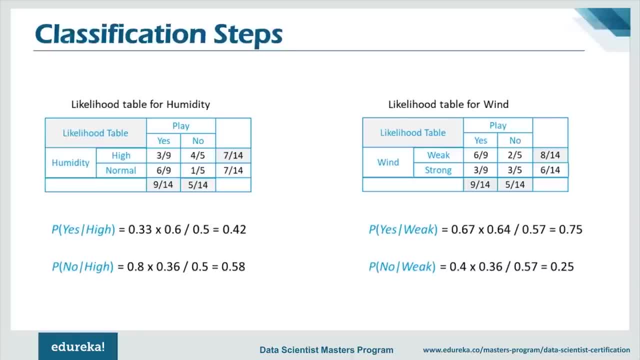 Now, similarly, we are going to create the likelihood table for both the humidity and the wind. So, for humidity, the likelihood for yes, given the humidity is high, is equal to 0.42.. And the probability of playing no, given the wind is high, is 0.58. 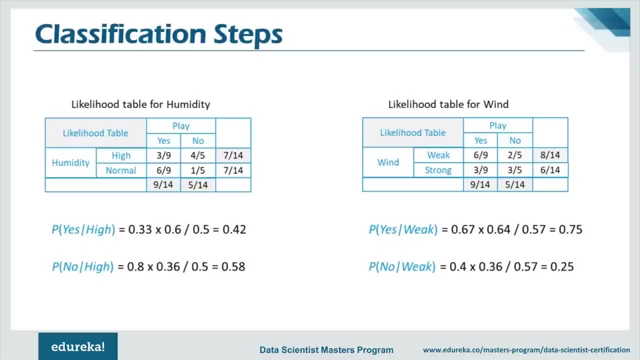 Now, similarly, for table wind, the probability of yes, given that the wind is weak, is 0.75.. And the probability of no, given that the wind is weak, is 0.25.. Now suppose we have, let's say, the probability of no. 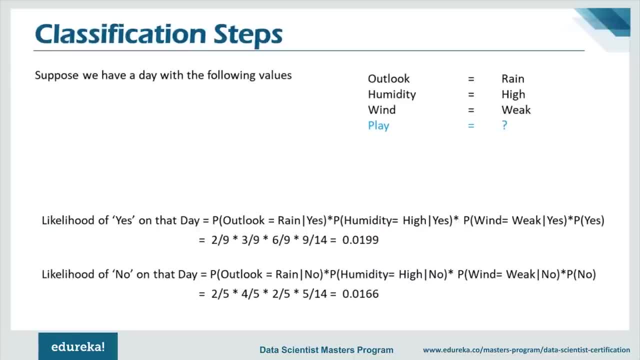 given that the wind is weak, is 0.25.. And the probability of day which has high rain, which has high humidity, and the wind is weak. So should we play or not Now? so for that we use the Bayes theorem here again. 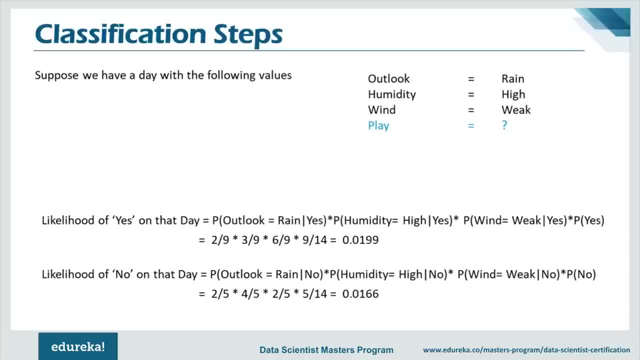 So the likelihood of yes on that day is equal to the probability of outlook rain, given that it's a yes, into probability of humidity, given that it's a yes, and the probability of wind that is weak, given that we are playing. yes. 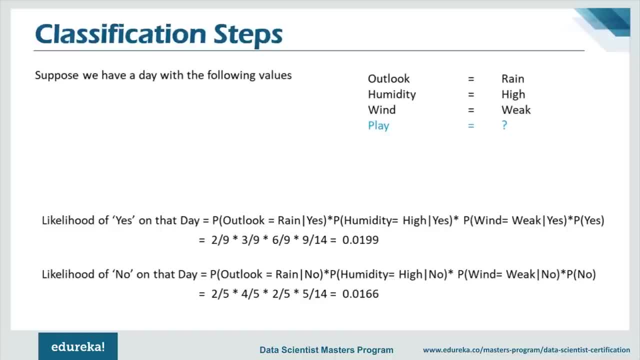 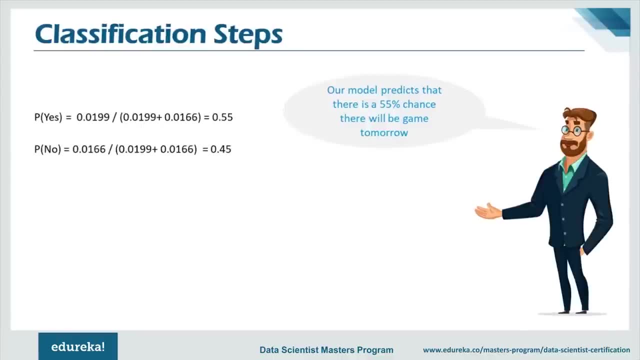 into the probability of yes, which equals to 0.00.. 0.019 and similarly, the likelihood of no on that day is equal to 0.016. now, if we look at the probability of yes for that day of playing, we just need to divide it with the likelihood sum. 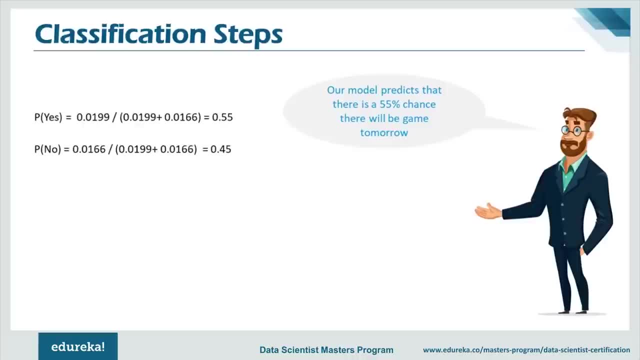 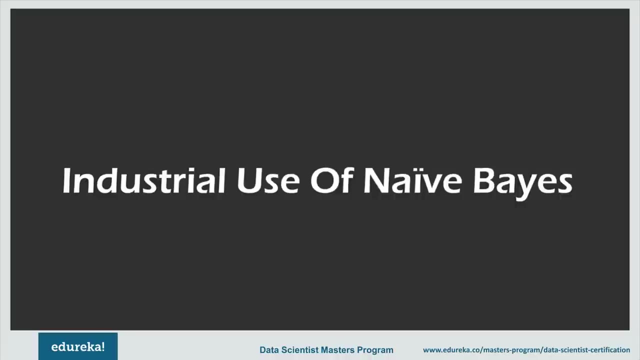 of both the yes and no. so the probability of playing tomorrow, which is yes, is 0.5, whereas the probability of not playing is equal to 0.45. now, this is based upon the data which we already have with us. so now that you have an idea of what exactly is naive bias, how it works, 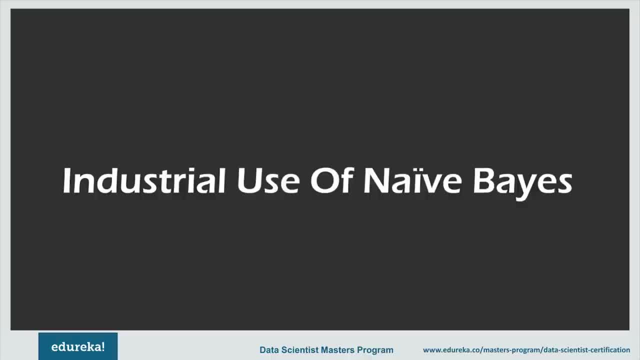 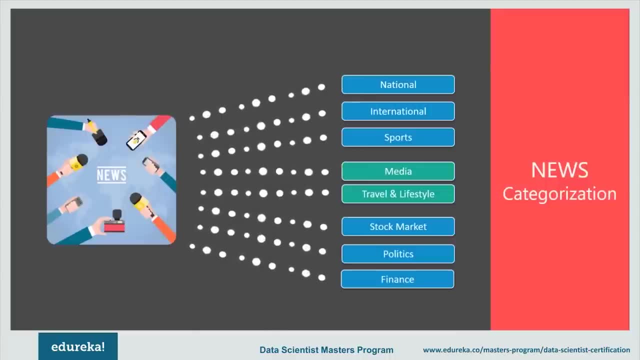 and we have seen how it can be implemented on a particular data set. let's see where it is used in the industry now, starting with our first industrial use case, which is news categorization, or we can use the term text classification to broaden the spectrum of this algorithm. 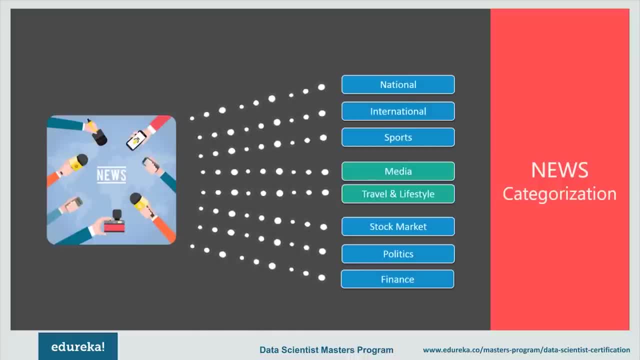 news in the web are rapidly growing in the era of information age, where each news site has its own different layout and categorization for grouping news. now, these heterogeneity of layout and categorization cannot always satisfy individual users need so remove these heterogeneity and classifying the news articles according to the 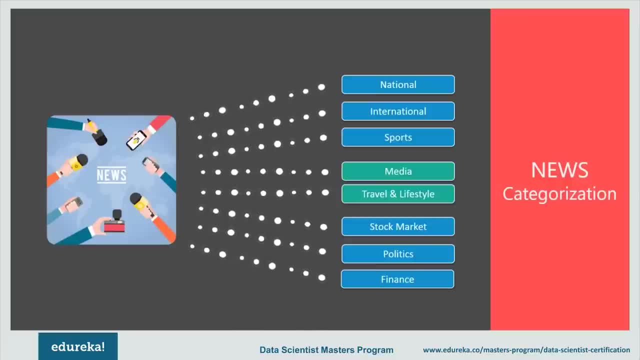 user preference is a formidable task. companies use web crawler to extract useful text from stml pages- the news articles- and each of these news articles is then tokenized. now you, these tokens are nothing but the categories of the news. now, in order to achieve better classification result, we remove the less significant words, which are the stop words, from the documents. 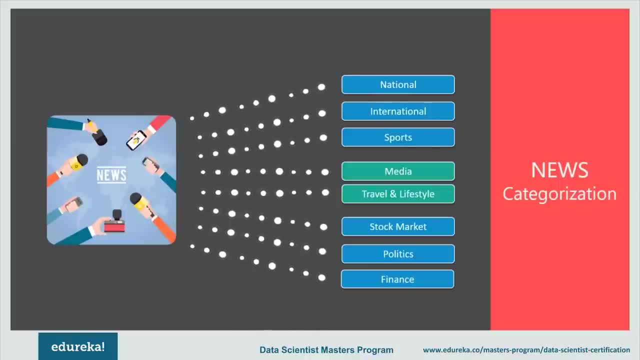 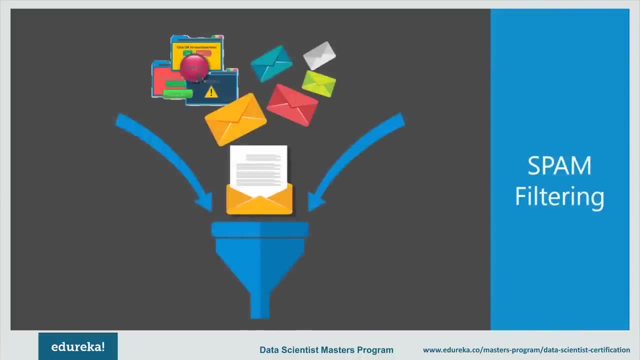 or the articles, and then we apply the naive bias classifier for classifying the news contents based on the news code. now this is by far one of the best examples of naive bias classifier, which is spam filtering. now it's the naive bias classifier are a popular statistical technique for. 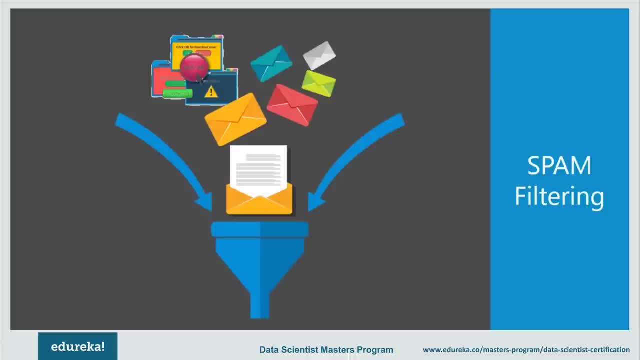 email filtering. they typically use bag of words features to identify the spam email and an approach commonly used in tax classification as well. now it works by correlating the use of tokens but the spam and the non spam emails, and then the base theorem which i explained earlier is used to calculate the probability that an email is are not a. 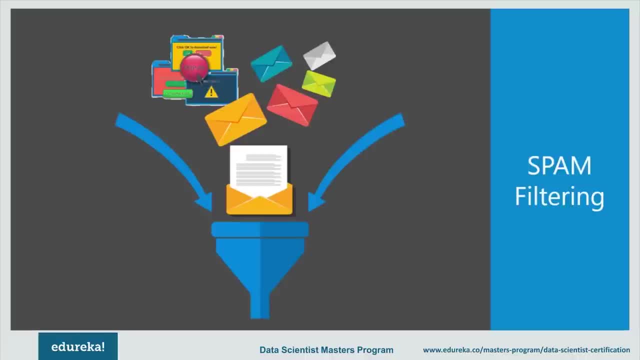 spam, so naive bias. spam filtering is a baseline technique for dealing with spam that can tailor itself to the emails need of an individual user and give low false positive spam detection rates that are generally acceptable to users. it is one of the oldest ways of doing spam filtering, with its roots in the 1990s. 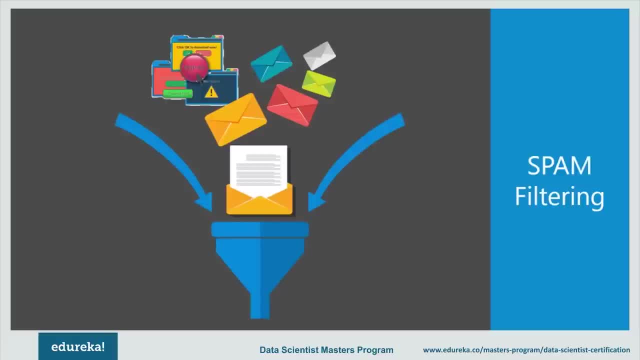 particular words have particular probabilities of occurring in spam email and in legitimate email as well. for instance, most emails users will frequently encounter the word lottery or the lucky draw is spam email, but will seldom see it in other emails. the filter doesn't know these probabilities in advance and must be trained so it can build them up. to train the filter, the 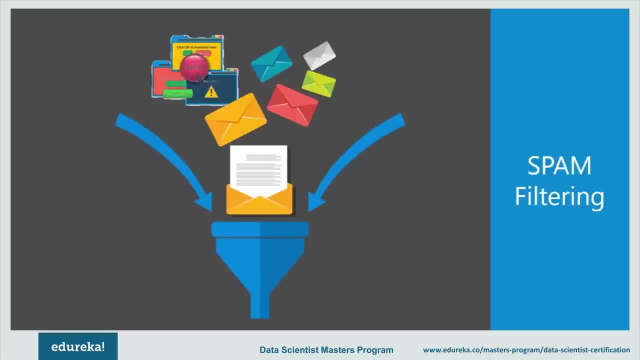 user must manually indicate whether a new email is spam or not. for all the words in each training email, the filter will adjust the probability that each word will appear in a spam or legitimate email in the database. now, after training, the word probabilities, also known as the likelihood functions, are used to compute. 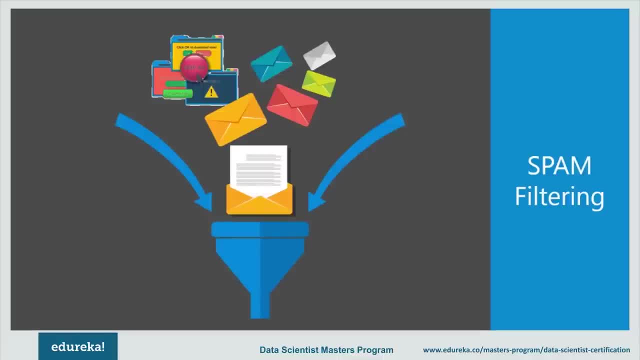 the probability that an email with a particular set of words and, as it belongs to either category, each word in the email contributes the email spam probability. this contribution is called the posterior probability and is computed again using the Bayes theorem. then the email spam probability is computed over all the words in the email and if the total exceeds a certain 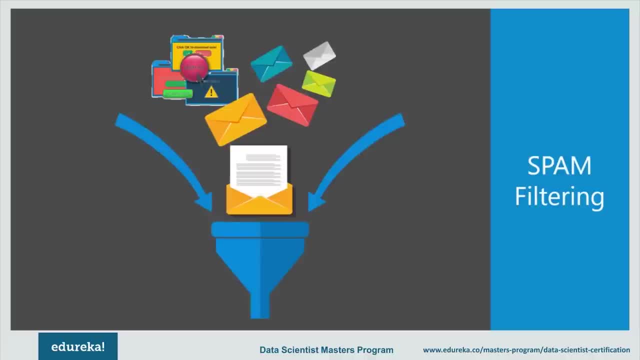 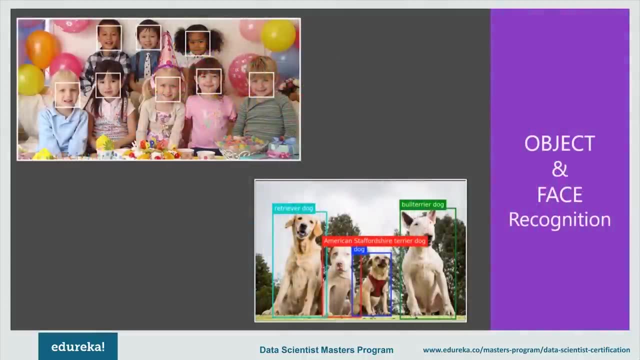 threshold, say 90 or 95 percent, the filter will mark the email as spam. now, object detection is the process of finding instances of real-world objects such as faces, bicycles and buildings in images of video. now, object detection algorithm typically use abstracted features and learning algorithm to recognize instance. 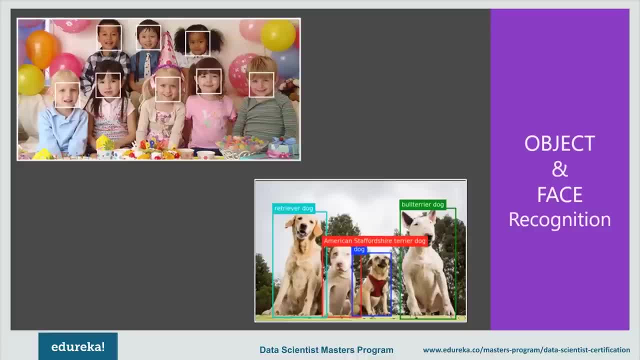 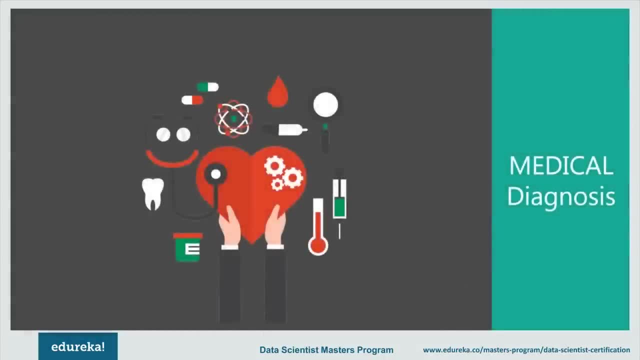 of an object category. here again, name bys plays an important role of categorization and classification of object. now, medical area produces increasingly voluminous amount of electronic data, which are becoming more and more complicated. the produce medical data have certain characteristics that make the analysis very challenging and attractive as well. Among all the different approaches, the naive bias. 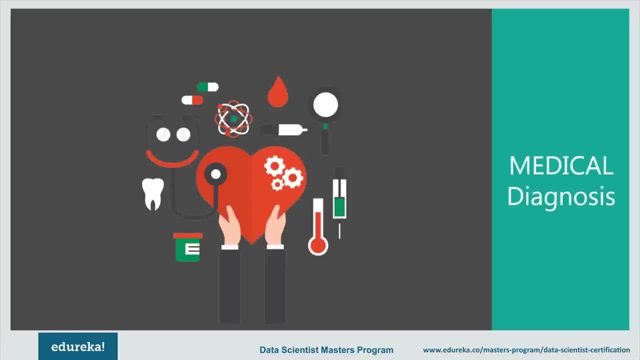 is used. it is the most effective and the efficient classification algorithm and has been successfully applied to many medical problems. Empirical comparison of naive bias versus five popular classifiers on 15 medical data sets shows that naive bias is well suited for medical application and has high performance in most of the examined medical problems. Now, in the past, various statistical 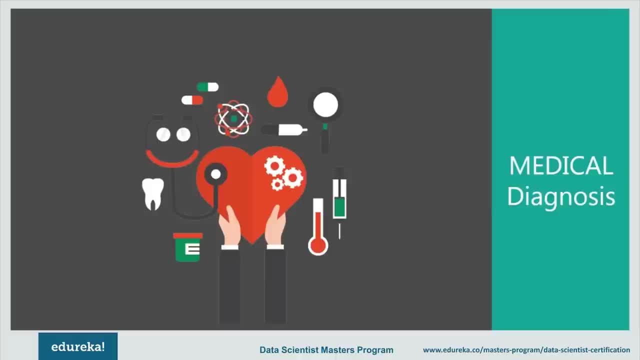 methods have been used for modeling in the area of disease diagnosis. These methods require prior assumptions and are less capable of dealing with massive and complicated non-linear and dependent data. One of the main advantages of naive bias approach, which is appealing to physicians, is that all the available information is used to explain the decision. This explanation seems to be natural. 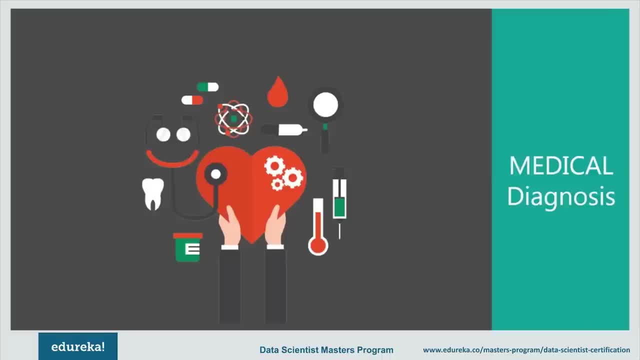 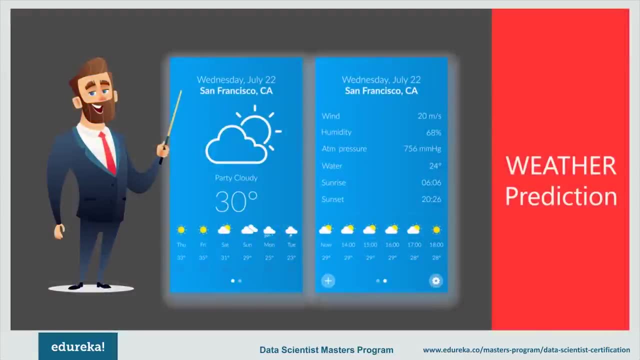 for medical diagnosis and for medical analysis. The main advantage of the naive bias approach is that it is very close to the way how physicians diagnose patients. Now, weather is one of the most influential factor in our daily life to an extent that it may affect the economy of a country that. 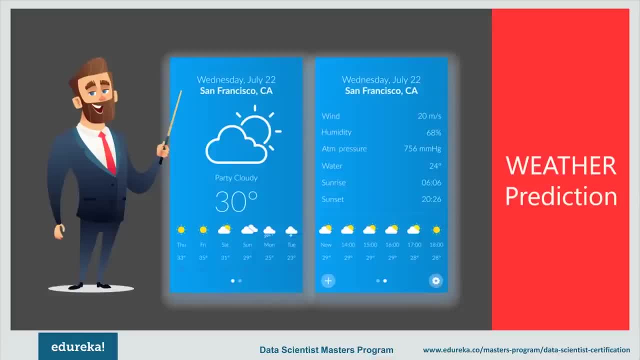 depends on occupation, like agriculture. Therefore, as a counter measure to reduce the damage caused by uncertainty in weather behavior, there should be an efficient way to predict the weather. Now. weather projecting has been challenging problem in the meteorological department since years. Even after the technology comes into play, it is still very difficult to predict the weather. 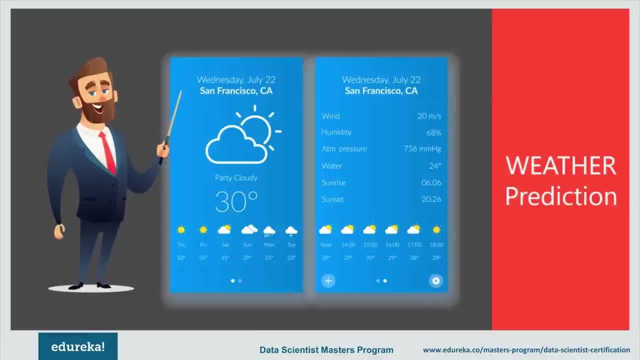 Even after the technology comes into play, it is still very difficult to predict the weather. Even after the technology comes into play, it is still very difficult to predict the weather. The accuracy in prediction of weather has never been sufficient, Even in current date. this domain 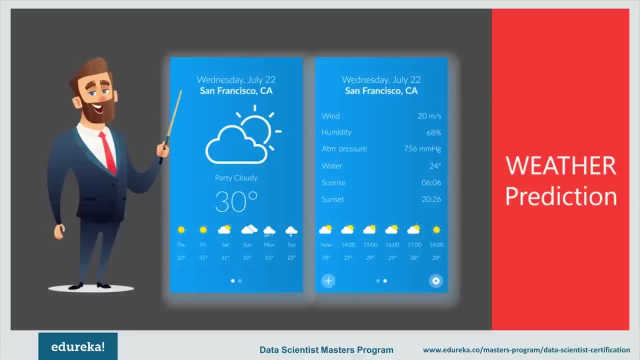 remains as a research topic in which scientists and mathematicians are working to produce a model or an algorithm that will accurately predict the weather. Now, a bias in approach based model is created by where posterior probabilities are used to calculate the likelihood of each class label for input data instance, and the one with the maximum likelihood is considered as the resulting output. 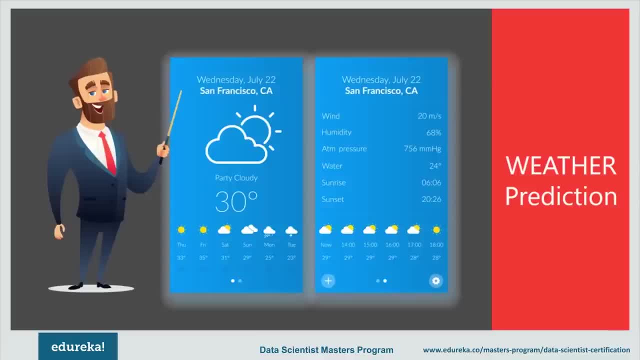 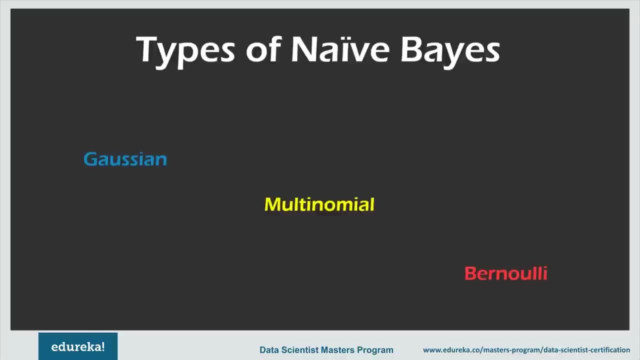 Now, earlier we saw a small implementation of this algorithm as well, where we predicted whether we should play or not, based on the data which we have collected earlier. Now there is a Python library which is known as scikit-learn. It helps to build naive bias and model in Python. Now there are three. 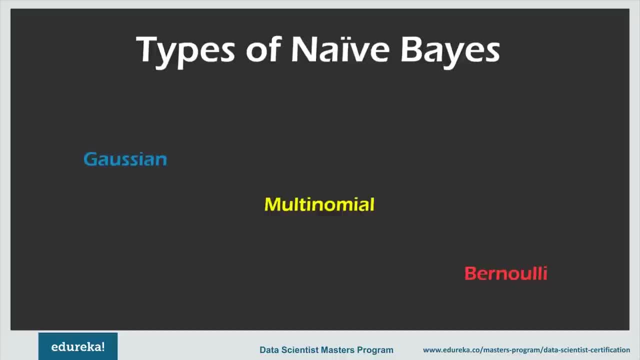 types of naive bias model under scikit-learn library. The first one is the Gaussian. It is used in classification and it assumes that the feature follow a normal distribution. The next we have is multinomial. It is used for discrete counts, For example. let's say we have a text classification. 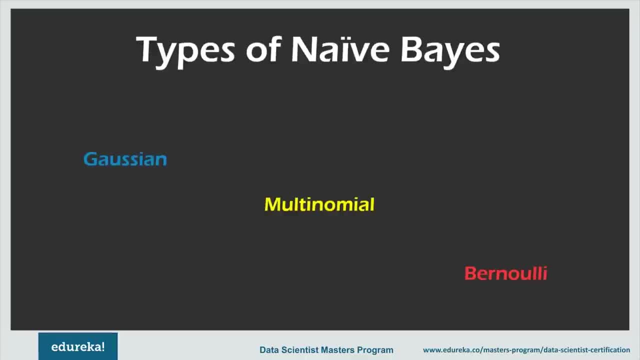 problem, and here we consider Bernoulli trials, which is one step further, and instead of word occurring in the document, we have count how often word occurs in the document. You can think of it as in the number of times outcomes number is observed in the given number of trials And 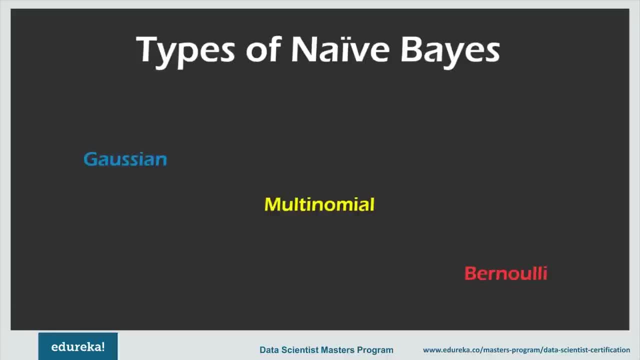 finally, we have the Bernoulli type of naive bias. The binomial model is useful if your feature vectors are used to calculate the number of times outcomes number is observed in the given number of trials. And finally, we have the Bernoulli type of naive bias. The binomial model is useful if your feature vectors 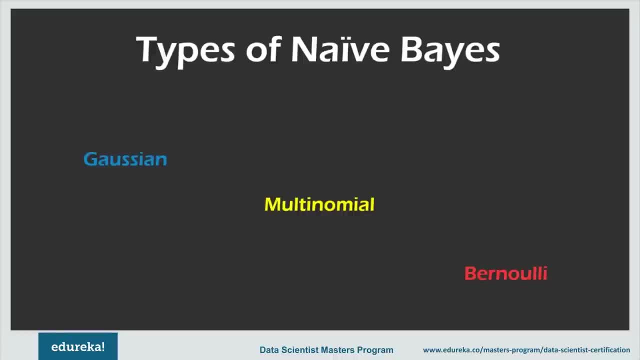 are binary Bag of words model where the ones and the zeros are words occur in the document and the words which do not occur in the document respectively. Based on your data set, you can choose any of the given discussed model here, which is the Gaussian, the. 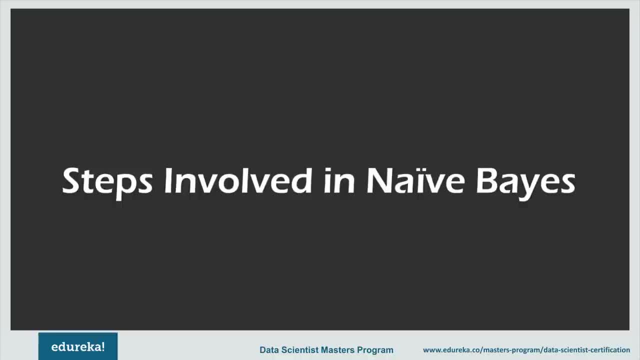 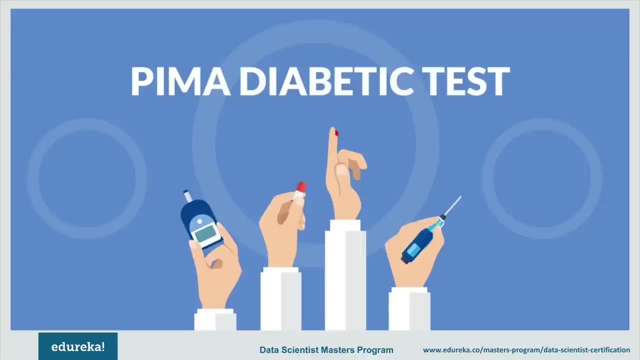 multinomial or the Bernoulli. So let's understand how this algorithm works and what are the different steps one can take to create a Bayesian model and use naive bias to predict the output. So here, to understand better, we are going to predict the onset of 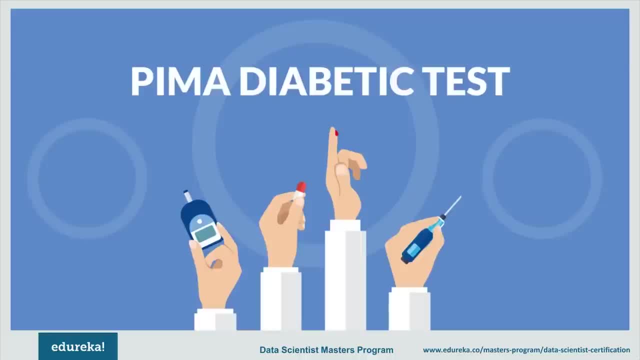 diabetes. Now this problem comprises of 768 observations of medical details for Pima Indian patients. The record describes instantaneous measurement taken from the patients, such as their age, the number of times pregnant and the blood workgroup. Now all the patients are women aged 21 and older and all the attributes are numeric and the 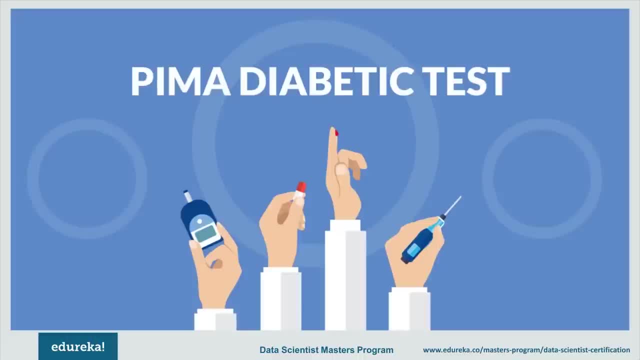 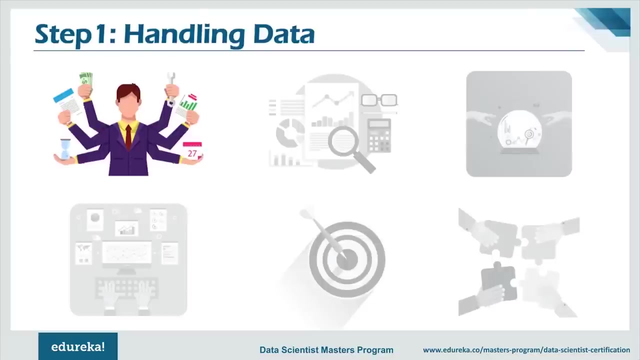 the units vary from attribute to attribute. Each record has a class value that indicate whether the patient suffered or an onset of diabetes within five years, or the measurements. Now these are classified as zero. Now I've broken the whole process down into the following steps. The first step is: 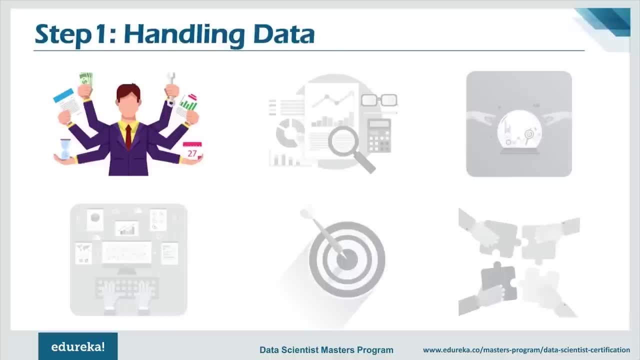 handling the data, in which we load the data from the CSV file and split it into training and test data sets. The second step is summarizing the data, in which we summarize the properties in the training data sets so that we can calculate the probabilities and make predictions. Now the third step comes is 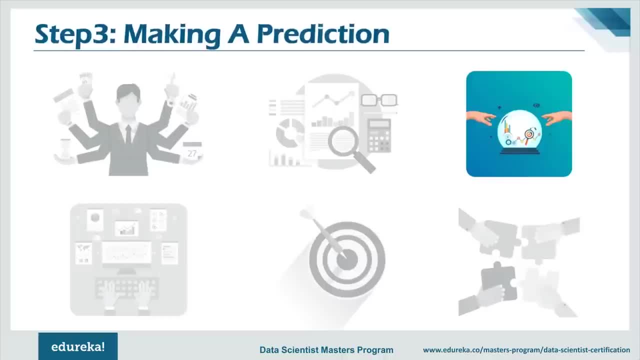 making a particular prediction, We use the summaries of the data set to generate a single prediction and after that we generate predictions given a test data set and a summarized training data sets. And finally, we evaluate the accuracy of the predictions made for a test data set as a percentage correct. 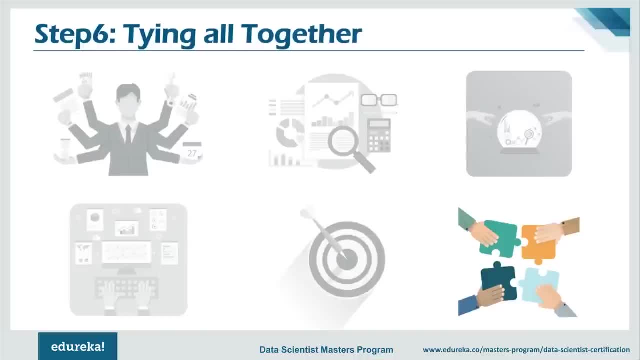 out of all the predictions made And finally we tie it together and form our own model of nape-wise classifier. Now the first thing we need to do is load our data. The data is in the CSV format without a header line or any quotes. We can open the file with the open function and read the data lines. 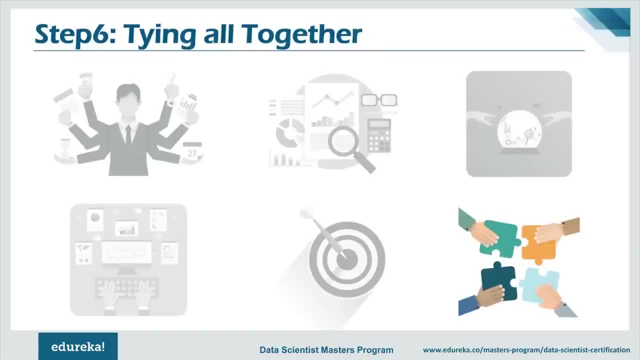 using the read functions in the CSV module. Now we also need to convert the attributes that were loaded as strings into numbers so that we can work with them. So let me show you how this can be implemented Now. for that, you need to install a. 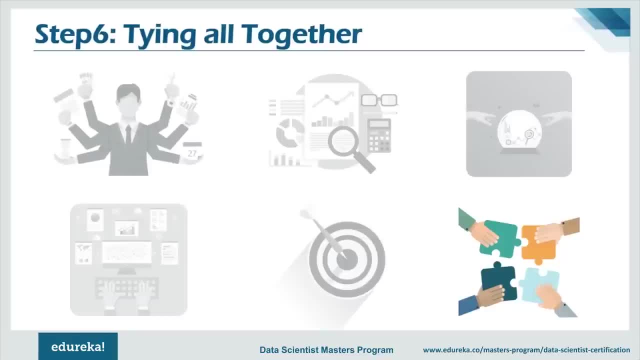 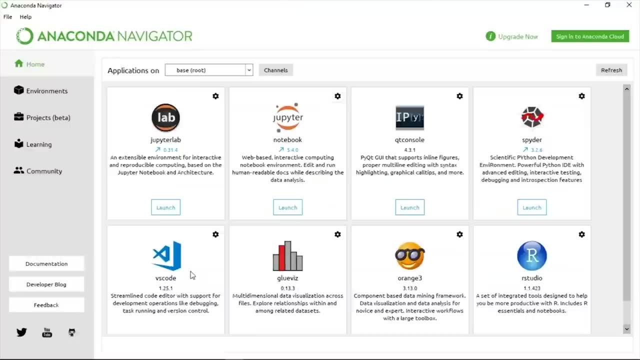 Python on your system and use the Jupyter Notebook or the Python shell. Here I'm using the Anaconda Navigator, which has all the things required to do programming in Python. We have the Jupyter Lab, we have the Notebook, we have the Qt console. even we have RStudio as well. So what you need to do is just 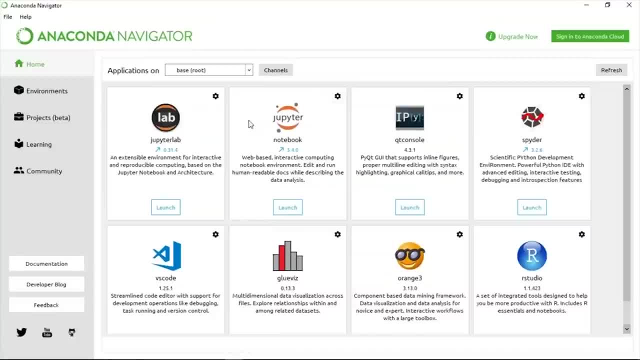 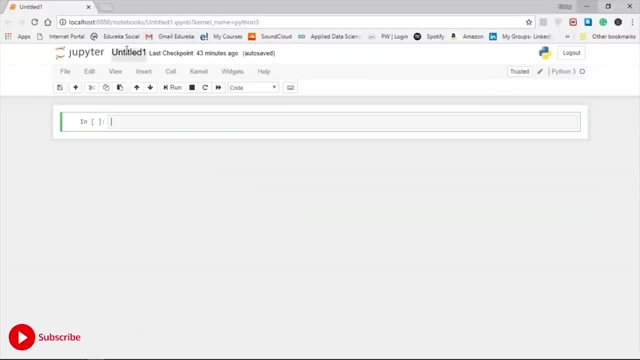 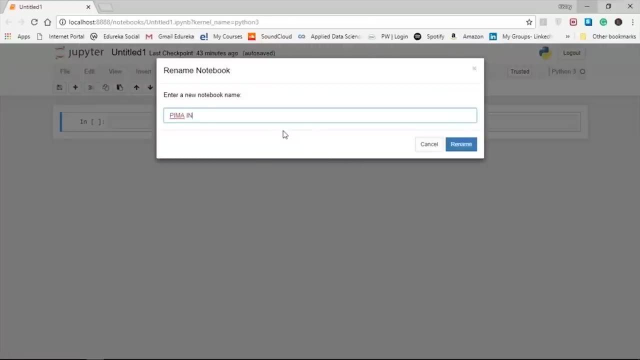 install the Anaconda Navigator. It comes with the pre-installed Python also, So the moment you click launch on the Jupyter Notebook, it will take you to the Jupyter homepage in a local system and here you can do programming in Python. So let me just rename it as Pima, India, diabetes. 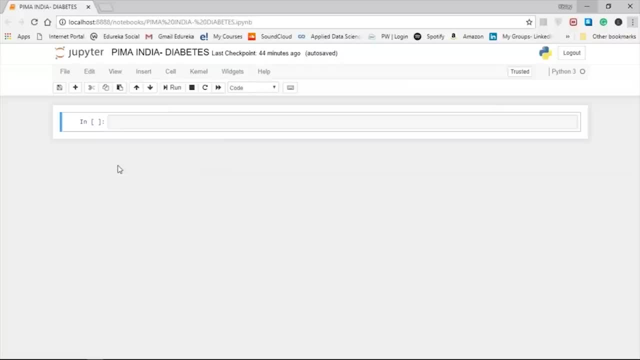 So first we need to load the data set. So I'm creating here a function: load CSV. Now, before that, we need to import certain CSV, the math and the random methods. So, as you can see, I've created a load CSV function which will take the Pima Indian diabetes. 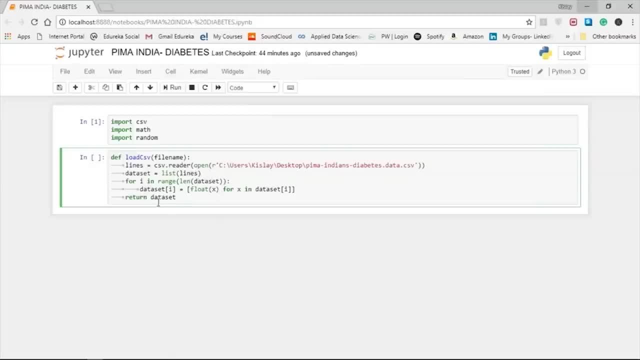 data dot CSV file using the CSV dot reader method, and then we are converting every element of that data set into float. originally, all the elements are in string, but we need to convert them into float for all calculation purposes now. next we need to split the data into training data sets that naive bias can. 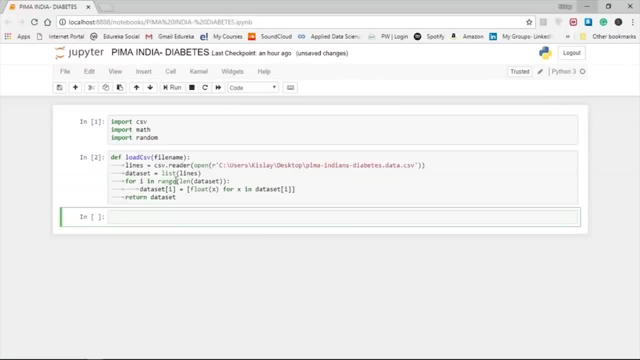 use to make the prediction and test data set that we can use to evaluate the accuracy of the model. we need to split the data set randomly into training and testing data set in the ratio of usually, which is 70 to 30, but for this example I am going to use 67 and 33. now, 70 and 30 is a common ratio for testing. 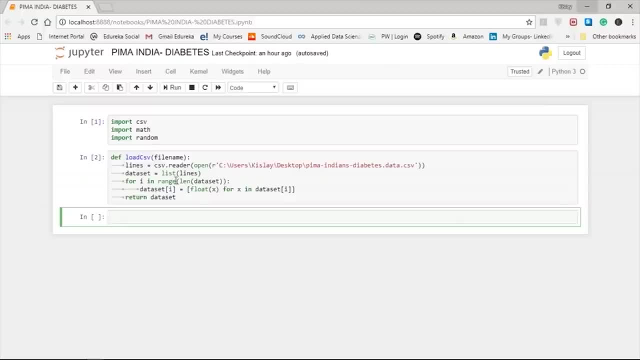 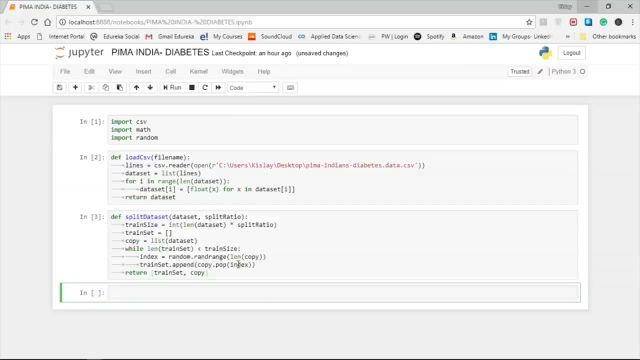 algorithms so you can play around with this number. so this is our split data set function. now. the naive bias model is comprised of summary of the data in the training data set. now. this is our split data set function. now. the naive bias model is comprised of summary of the data in the training data set. now this: 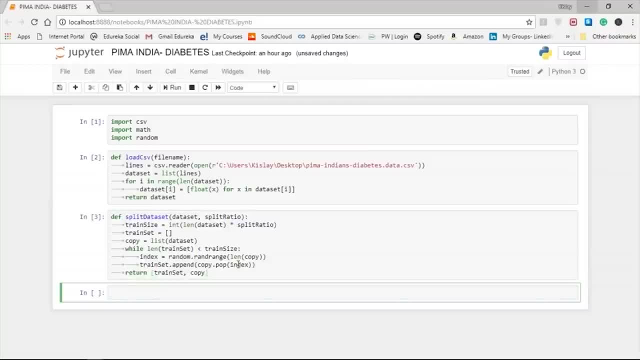 summary is then used while making predictions. now, the summary of the training data collected involves the mean, the standard deviation of each attribute by class value. now, for example, if there are two class values and seven numerical attributes, then we need a mean and the standard deviation for each of. 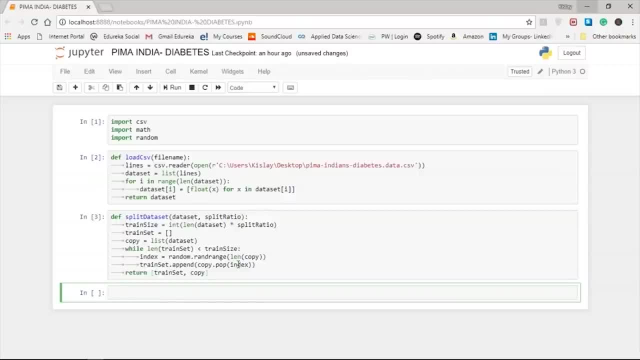 these seven attributes and the class value which makes it the 14 attribute summaries. so we can break the preparation of this summary down into the following subtasks, which are the separating data by class, calculating mean, calculating standard deviation, summarizing the data sets and summarizing attributes by class. so the first task is to separate the 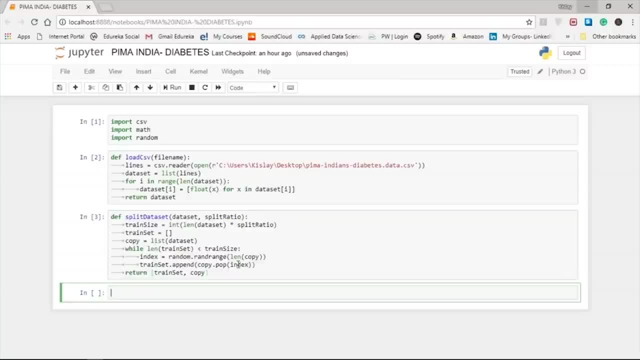 training data. set instances by class value so that we can calculate statistics for each class. we can do that by creating a map of each class value to a list of instances that belong to the class and sort the entire data set of instances into the appropriate list. now the separate by class function just does. 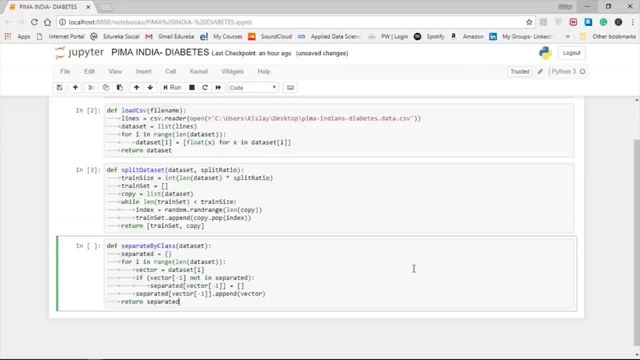 the same thing in the same way for each class. this separate by class function. so, as you can see, the function assumes that the last attribute is the class value. the function returns a map of class value to the list of data instances. next we need to calculate the mean of each attribute for a class value. 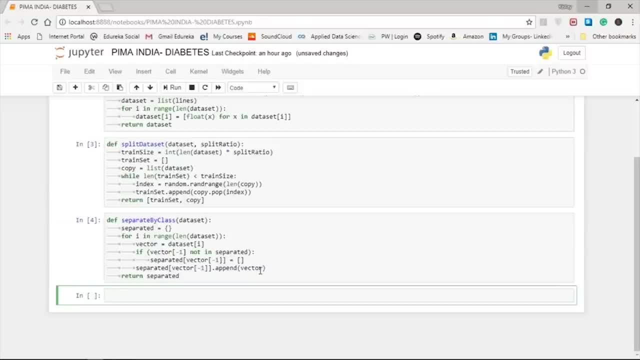 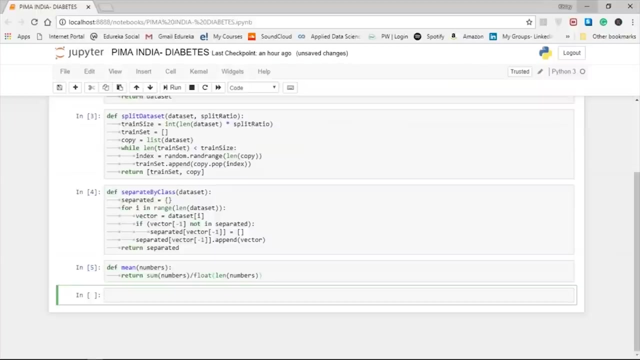 now the mean is the central middle or the central tendency of the data, and we use it as the middle of our Gaussian distribution when calculating the probabilities. so this is our function for mean. now we also need to calculate the standard deviation of each attribute for a class value. now standard deviation. 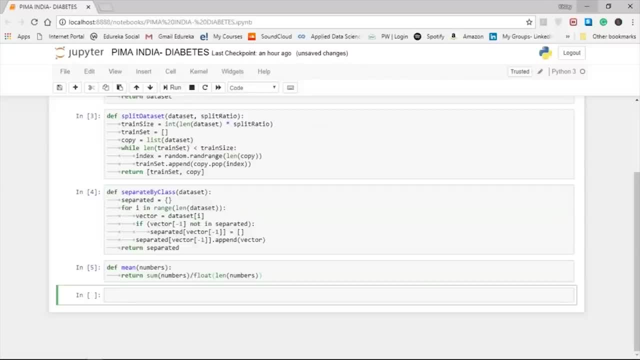 is calculated as a square root of the variance and the variance is calculated as the average of the square differences for each attribute value. from the mean now, one thing to note that here is that we are using n minus 1 method, which subtracts 1 from the number of attributes values when calculating the. 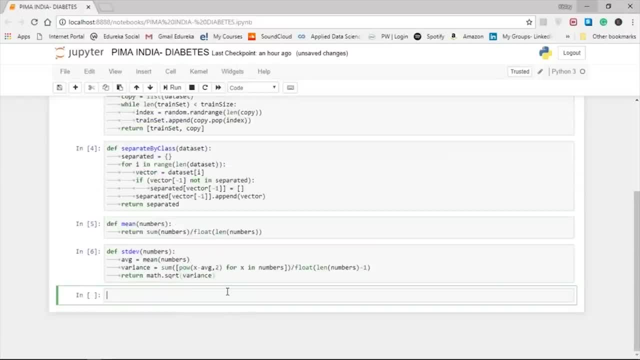 variance. now that we have the tools to summarize the data for a given list of instances, we can calculate the mean and standard deviation for each attribute. now, that's if function groups the values for each attribute across our data instances into their own lists so that we can compute the mean and standard deviation values for each. 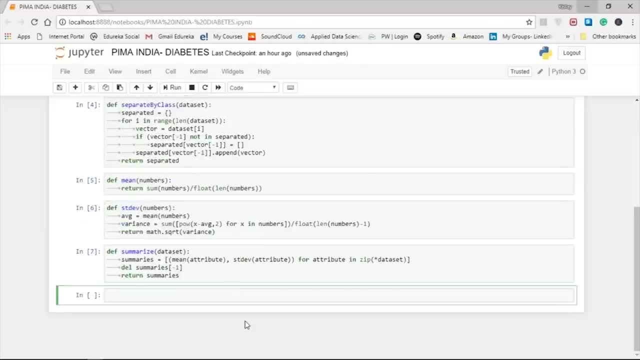 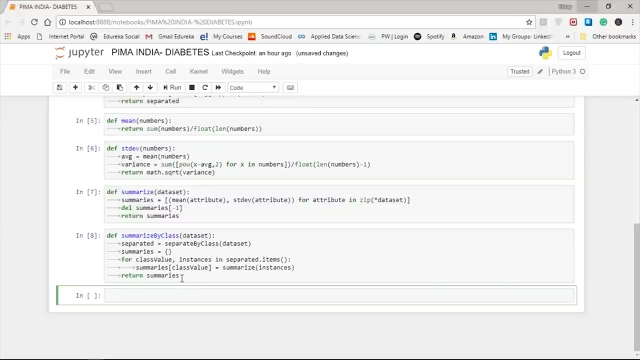 attribute. now. next comes the summarizing attributes by class. we can pull it all together by first separating our training data sets into instances growth by class, then calculating the summaries for each attribute. now we are ready to make predictions using the summaries prepared from our training data. making predictions involve calculating the probability that a given data 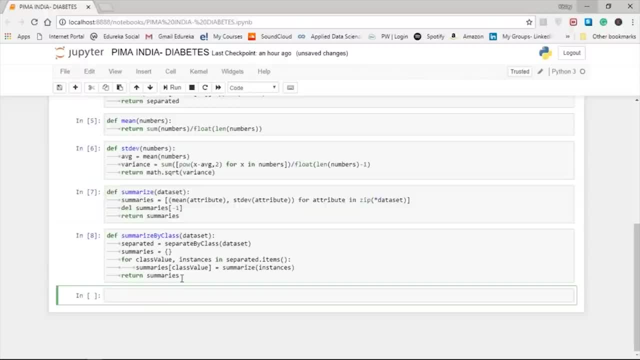 instance belong to each class, then selecting the class with the largest probability as a prediction. now we can divide this whole method into four tasks, which are the calculating Gaussian probability density function, calculating cost probability, making a prediction and then estimating the accuracy. now, to calculate the Gaussian probability density function, we use the 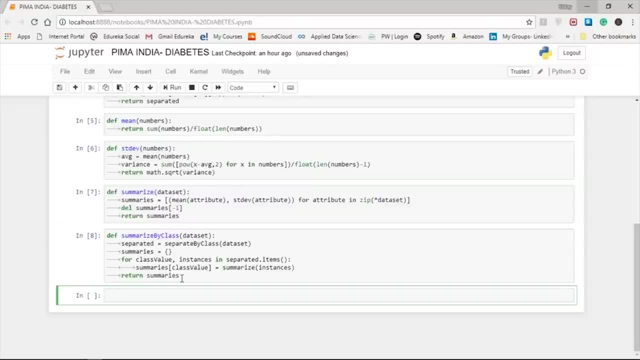 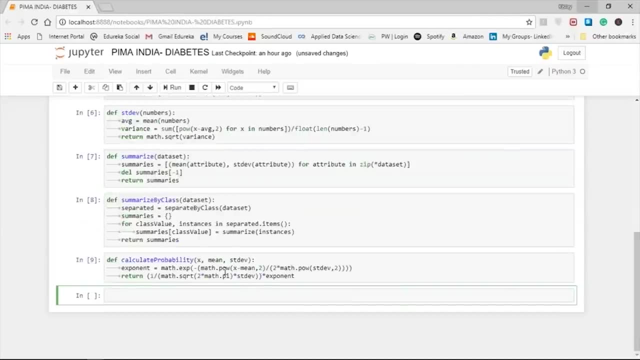 Gaussian function to estimate the probability of a given attribute value, given the node mean and the standard deviation of the attribute estimated from the training data. As you can see, the parameters are X, mean and the standard deviation. Now in the calculate probability function we calculate the exponent first. 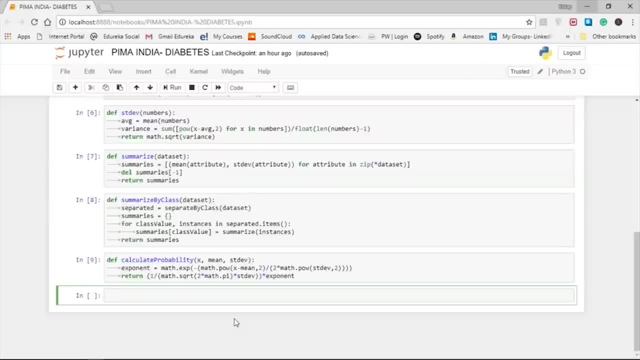 then calculate the main division. This lets us fit the equation nicely into two lines. Now the next task is calculating the class probabilities. Now that we can calculate the probability of an attribute belonging to a class, we can combine the probabilities of all the attributes values for a data instance. 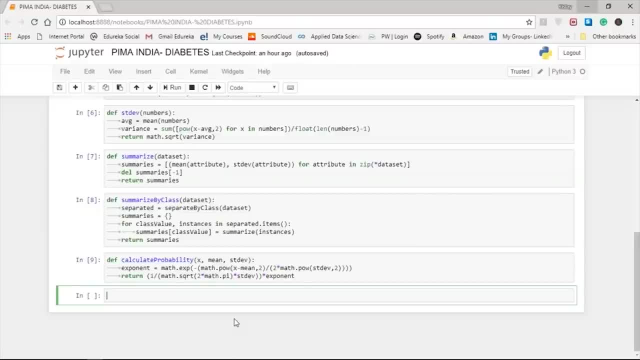 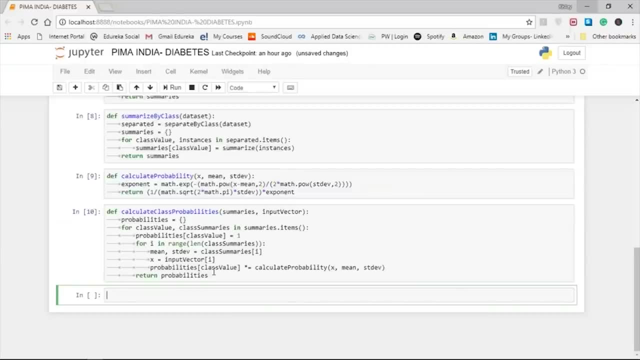 and come up with a probability of the entire data instance belonging to the class. So now that we have calculated the class probabilities, it's time to finally make our first prediction. Now we can calculate the probability of the data instance belonging to each class value. 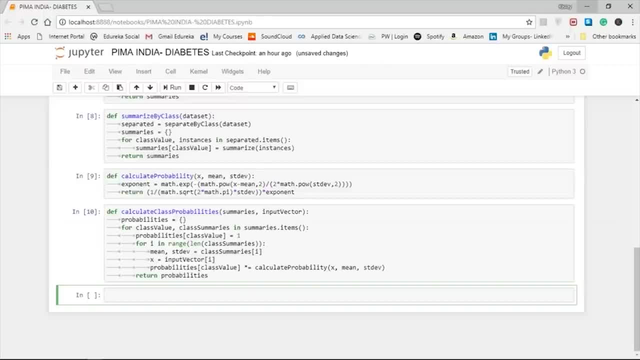 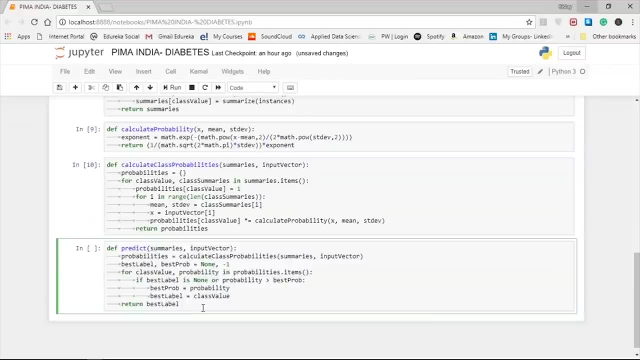 and we can look for the largest probability and return the associated class. And for that we are going to use this function predict, which uses the summaries and the input vector, which is basically all the probabilities which are being input for a particular label. 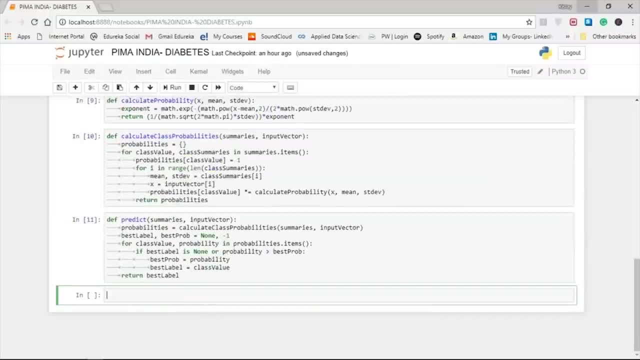 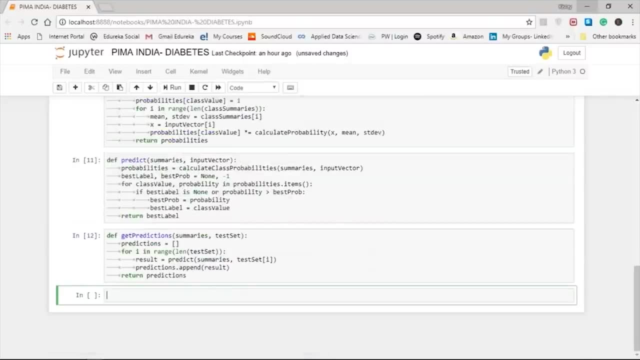 Now, finally, we can estimate the accuracy of the model by making predictions for each data instances in our test data. For that we use the getPredictions method. Now, this method is used to calculate the predictions based upon the test data sets and the summary of the training data set. 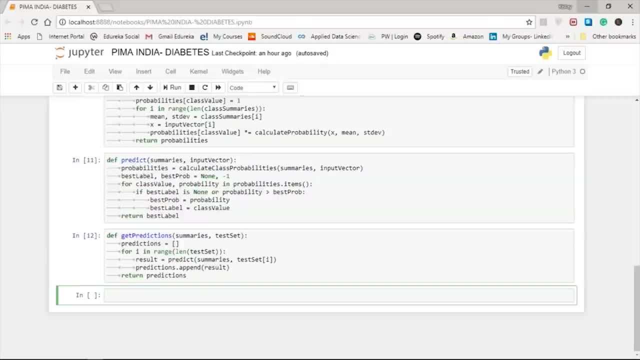 Now the predictions can be compared to the class values in our test data set, and classification accuracy can be calculated as an accuracy ratio between the zeros and the 100%. Now the getAccuracy method will calculate this accuracy ratio. Now, finally, to sum it all up, 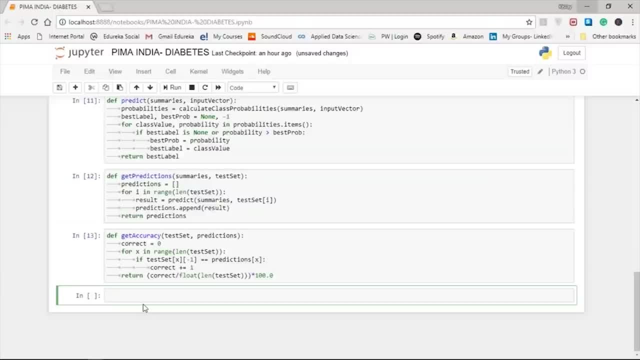 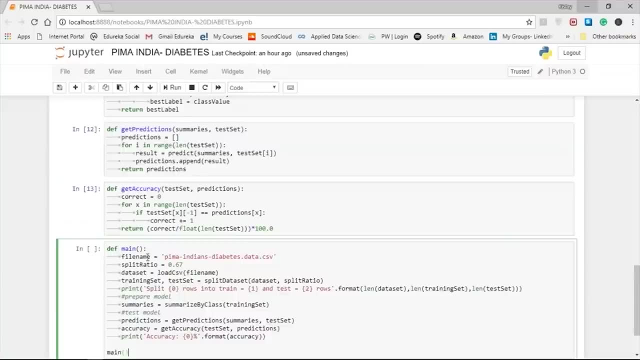 we define our main function. We recall all these methods which we have defined earlier, one by one, to get the accuracy of the model which we have created. So, as you can see, this is our main function, in which we have the file name, we have defined the split ratio, we have the data set. 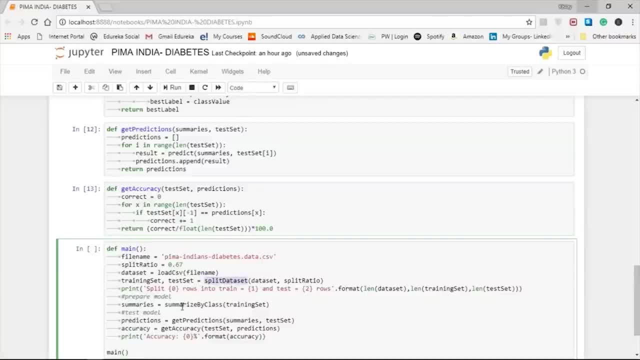 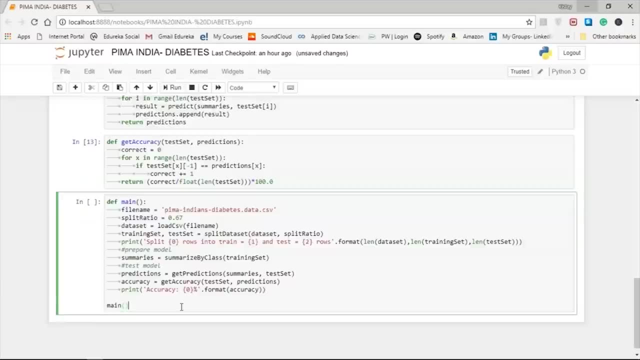 we have the training and test data set. We are using the split data set method. Next, we are using the summarizeByClass function. We are using the getPrediction and the getAccuracy method as well. So, guys, as you can see, the output of this one gives us. 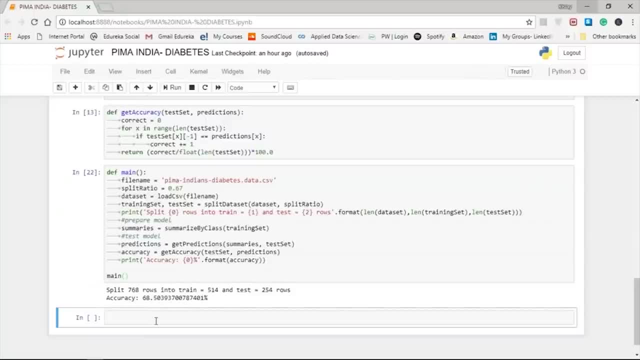 that we are splitting the 768 rows into 514,, which is the training, and 254,, which is the test data set rows, And the accuracy of this model is 68%. Now we can play with the amount of training and test data sets which are to be used here. 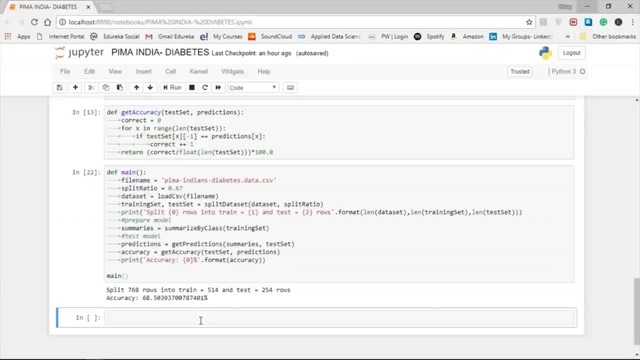 So we can change the split ratio to 70s to 30,, 80s to 20 to get different sort of accuracy. So suppose I change the split ratio from 0.67 to 0.8.. So, as you can see, we get the accuracy of 62%. 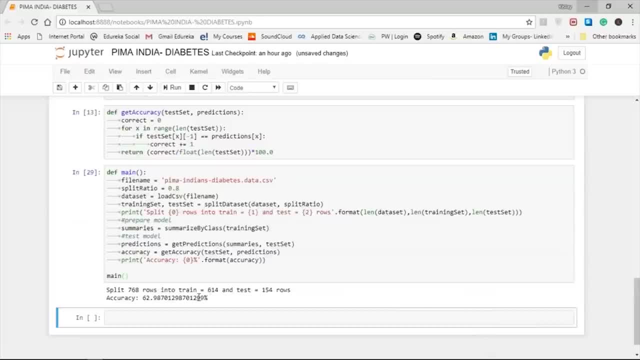 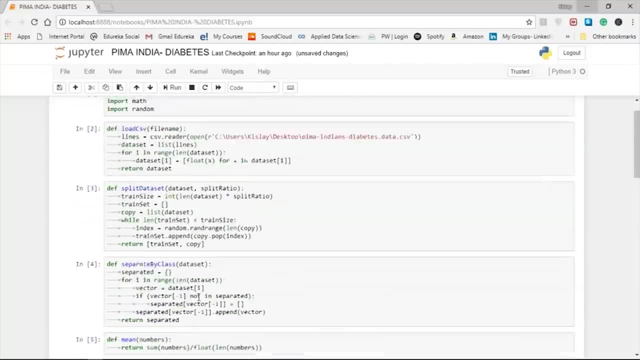 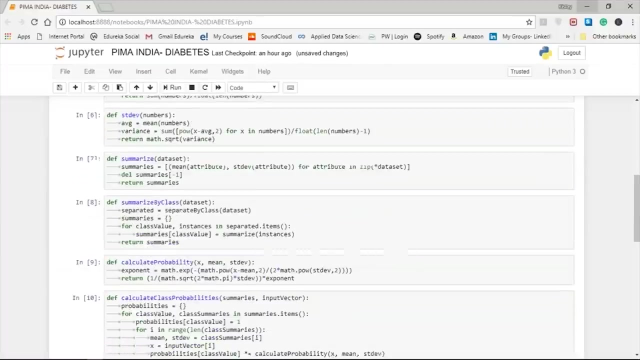 So splitting it into 0.67 gave us a better result, which was 68%. So this is how you can do this, How you can implement a naive bias caution classifier. These are the step-by-step methods which you need to do in case of using the naive bias classifier. 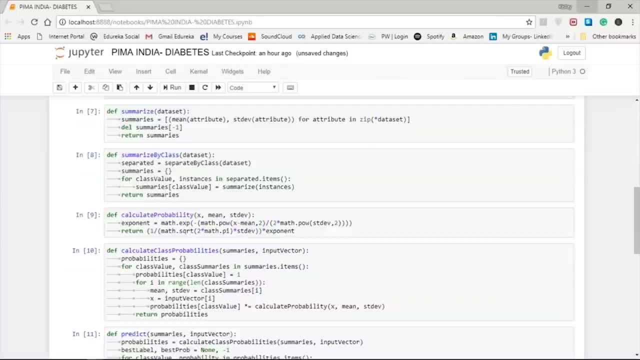 But don't worry, we do not need to write all this many lines of code to make a model. This is where the scikit-learn library comes into picture. The scikit-learn library has a predefined method or I'll say, a predefined function of naive bias. 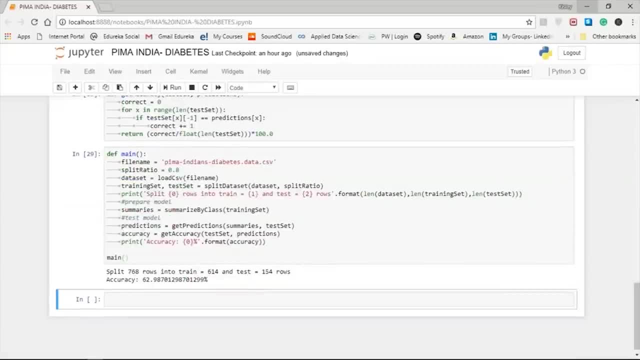 which converts all of these lines of course into a model which converts all of these lines of course into a model which converts all of these lines of course into a model To merely just two or three lines of course. So let me just open another Jupyter notebook. 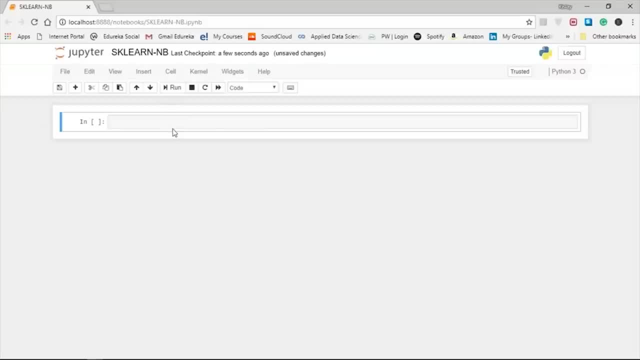 So let me name it as sklearn-naive-bias. Now here we are going to use the most famous data set, which is the iris data set. Now, the iris flower data set is a multivariate data set introduced by the British statistician and biologist Roland Fisher. 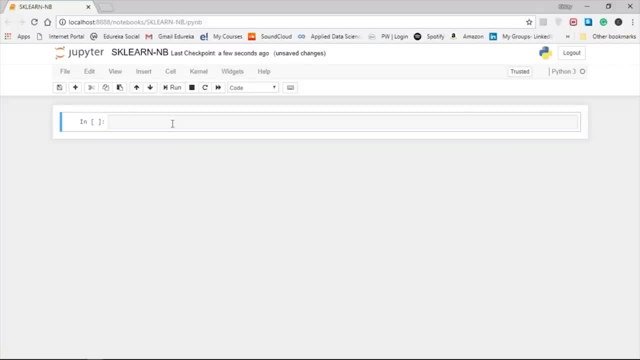 And based on this Fisher's linear discriminant model, this data set became a typical test case for many statistical classification techniques in machine learning. So here we are going to use the Gaussian NB model, which is already available in the sklearn, As I mentioned earlier. 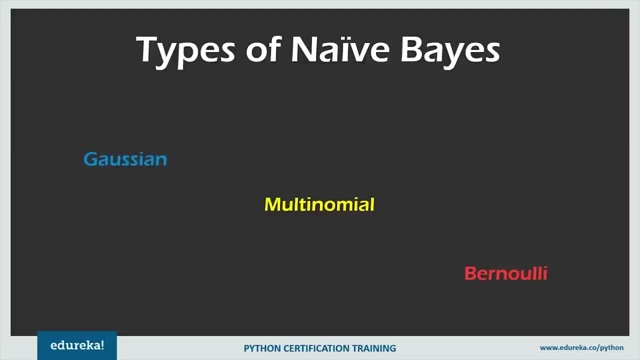 there were three types of nave bias, which are the Gaussian multinomial and the Bernoulli. So here we are going to use the Gaussian NB model, which is already present in the sklearn library, which is the scikit-learn library. So first of all, what we need to do is import. 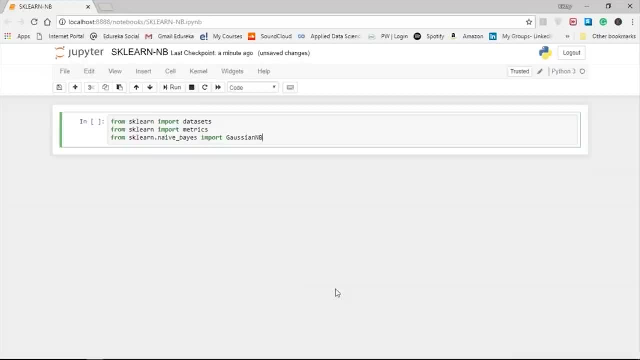 the sklearn data sets and the metrics. So, first of all, what we need to do is import the sklearn data sets and the metrics, and we also need to import the Gaussian NB. now, once all these libraries are loaded, we need to load the data set, which is the iris data set. the next, what? 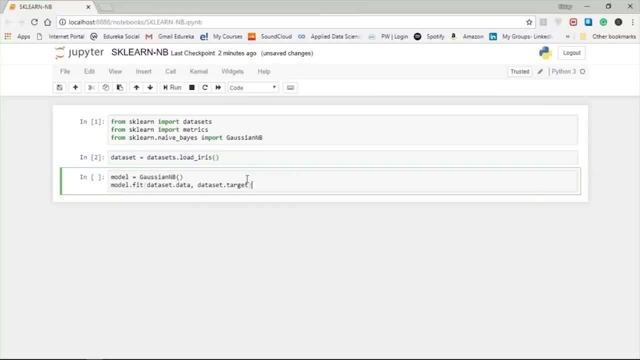 we need to do is fit a naive bias model to this data set. so, as you can see, we have so easily defined the model, which is the Gaussian NB, which contains all the programming which I just showed you earlier, all the methods which are taking the input, calculating the mean, the standard deviation, separating it by 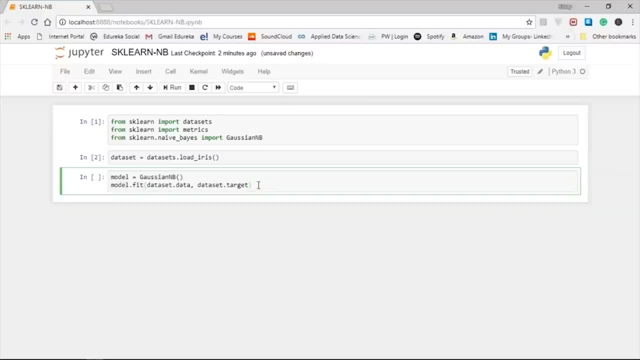 class. then finally, making predictions and calculating the prediction accuracy. all of these comes under the Gaussian NB method, which is inside, already present in the sklearn library. we just need to fit it according to the data set which we have here. so next, if we print the model, we see, which is the Gaussian NB. 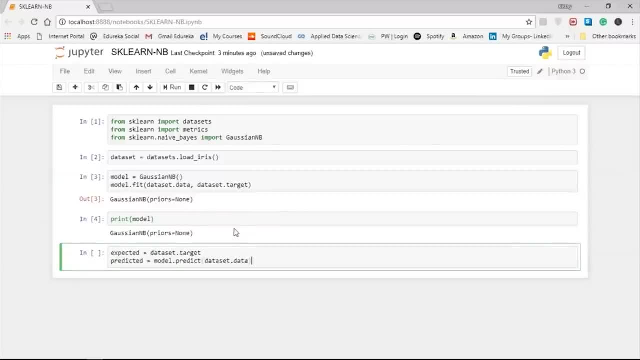 model now. next, what we need to do is make the predictions, so the expected output is data set, dot target and the predicted is using the predicted model. and the model we are using is the Gaussian NB. here now to summarize the model which is created: we calculate the confusion matrix and the 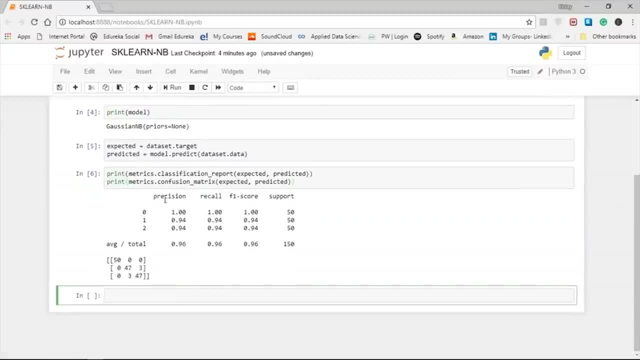 classification report. so, guys, as you can see the classification report, we have the precision of 0.96, we have the recall of 0.96, we have the f1 score and the support and, finally, if we print our confusion matrix, as you can see, it gives us this output. so, as you can see, using the Gaussian, 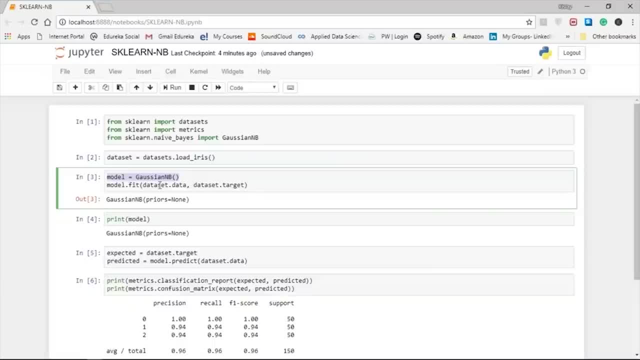 envy method, just putting it in another model and using any of the data set. fitting the model which you created into a particular data set and getting the desired output is so easy with the scikit-learn library. so, guys, this is it. I hope you understood a lot about the naive bias classifier, how it is used. 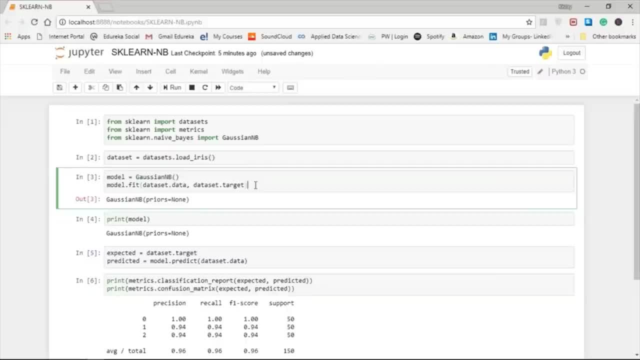 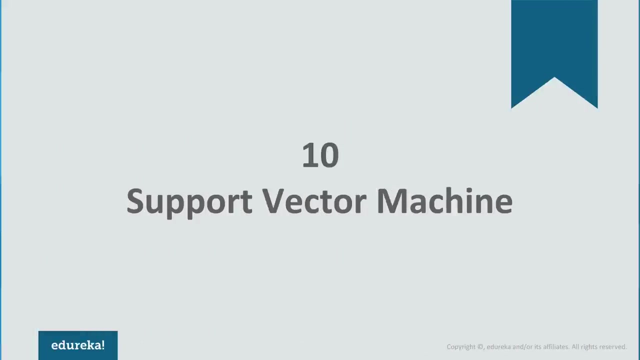 where it is used and what are the different steps involved in the classification technique and how the scikit-learn makes all of those techniques really easy to implement. in any data set which we have, SVM or support vector machine is one of the most effective machine learning. 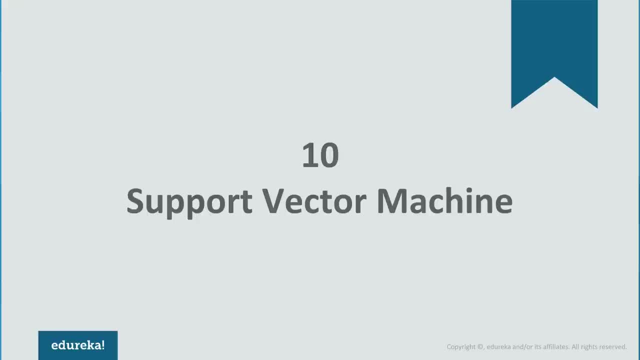 classifier, and it has been used in various fields, such as face recognition, cancer classification and so on. today's session is dedicated to how SVM works, the various features of SVM and how it is used in the real world. so, without any further ado, let's take a look at the 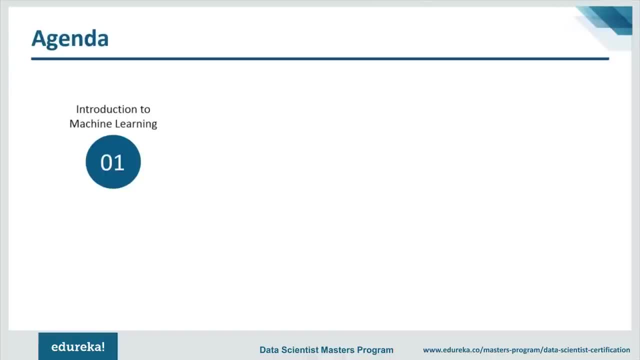 agenda for today. we're going to begin the session with an introduction to machine learning and the different types of machine learning. next we'll discuss what exactly support vector machines are, and then we'll move on and see how SVM works and how it can be used to classify linearly separable data. we'll also 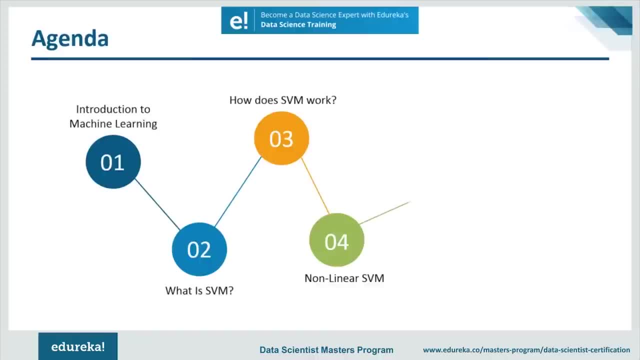 briefly discuss about how nonlinear SVMs work, and then we'll move on and look at the use case of SVM in colon cancer classification. and finally we'll end the session by running a demo where we'll use SVM to predict whether a patient is suffering from a heart disease or not. okay, so that. 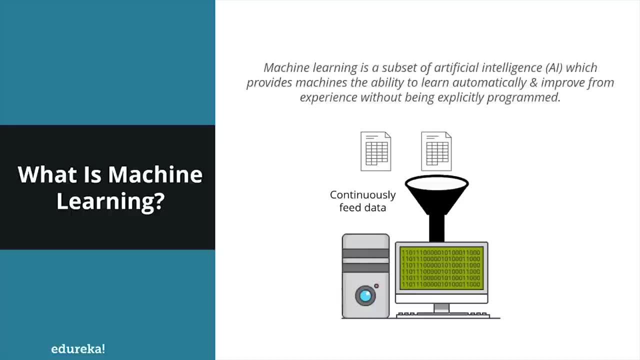 was the agenda. let's get started with our first topic. so what is machine learning? machine learning is a science of getting computers to act by feeding them data and letting them learn a few tricks on their own. okay, we're not going to explicitly program the machine. instead, we're going to feed it data and 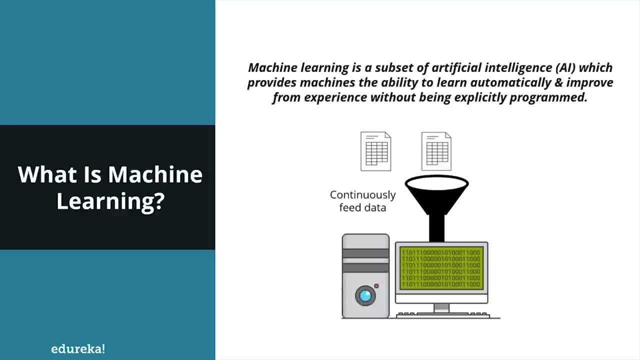 let it learn. the key to machine learning is the data. machines learn just like us humans. we humans need to collect information and data to learn. similarly, machines must also be fed data in order to learn and make decisions. so let's say that you want a machine to predict the value of a 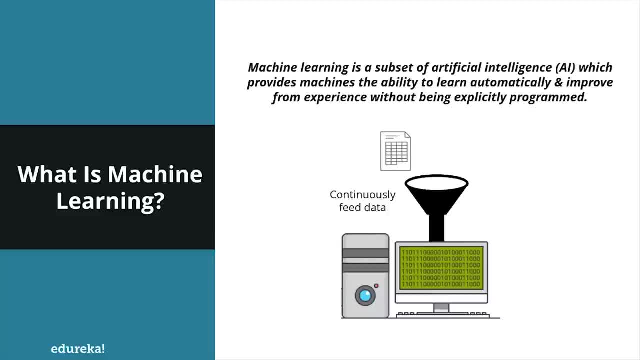 stock. all right. in such situations, you just feed the machine with relevant data, after which you develop a model which is used to predict the value of the stock. now, one thing to keep in mind is the more data you feed the machine, the better it'll learn and make more accurate predictions. so let's get started. 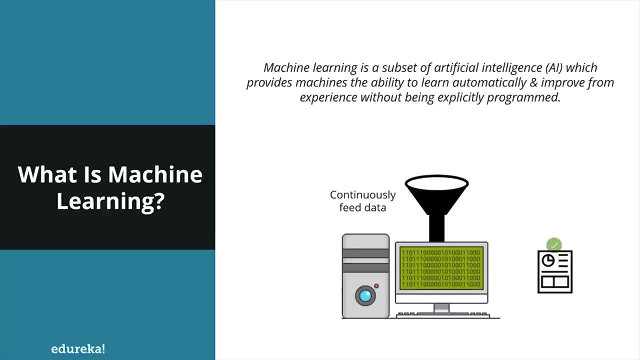 obviously, machine learning is not so simple. in order for a machine to analyze and get useful insights from data, it must process and study the data by running different algorithms on it. all right, and today we'll be discussing about one of the most widely used algorithm, called the support vector. 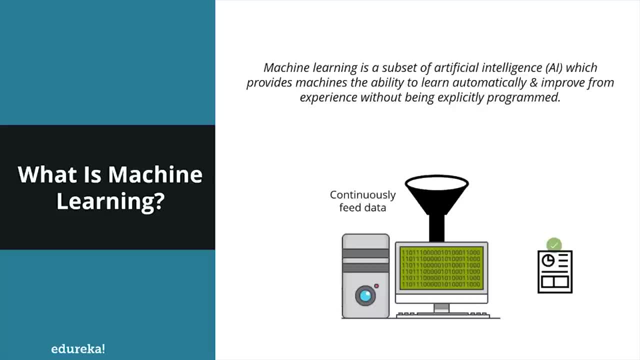 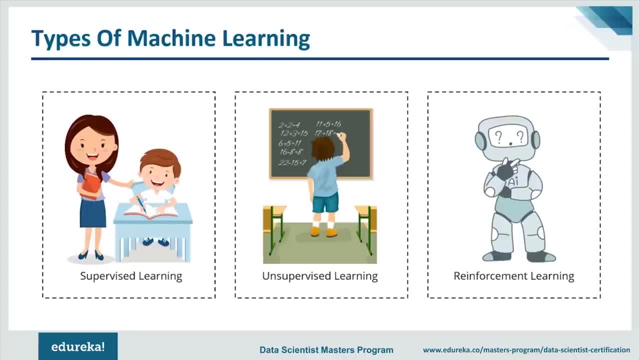 machine. okay, now that you have a brief idea about what machine learning is, let's look at the different ways in which machines learn. first, we have supervised learning. in this type of learning, the machine learns on the guidance. all right, that's why it's called supervised learning now at school. 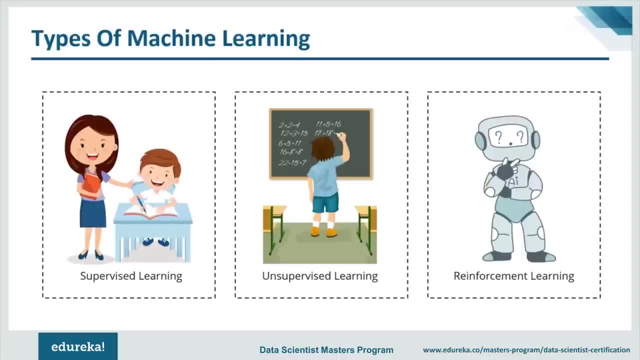 our teachers guided us and taught us. similarly, in supervised learning machines learn by feeding them label data and explicitly telling them: hey, this is the input and this is how the output must look. okay. so, guys, the teacher in this case is a training data. next we have unsupervised learning. here 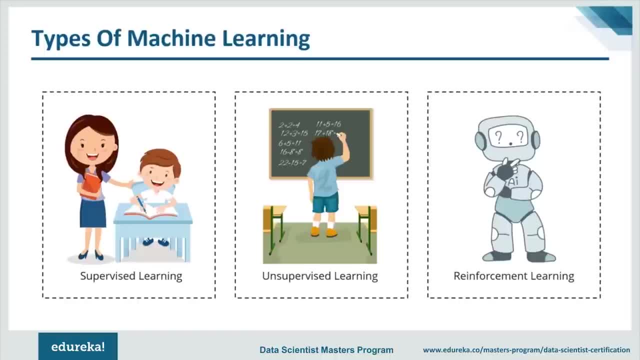 the data is not labeled and there is no guide of any sort. okay, the machine must figure out the data set given and must find hidden patterns in order to make predictions about the output. an example of unsupervised learning is an adult like you and me. we don't need a guide to help. 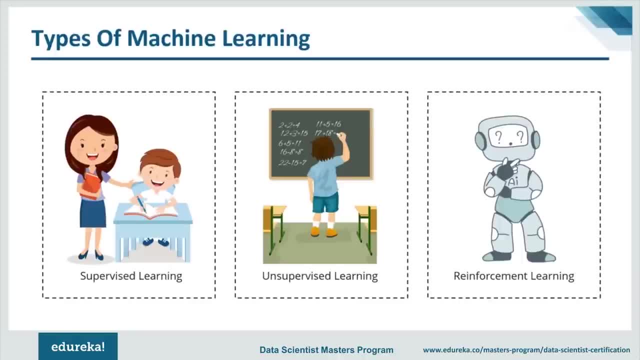 us with our daily activities. we figure things out on our own, without any supervision. all right. that's exactly how unsupervised learning work. finally, we have reinforcement learning. let's say you were dropped off at an isolated island. what would you do now? initially, you'd panic and you'd be unsure of what. 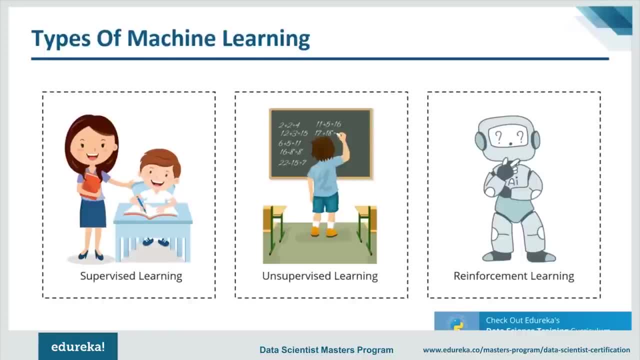 to do, where to get food from, how to live and all of that. but after a while you will have to adapt. you must learn how to live in the island, adapt to the changing climate, learn what to eat and what not to eat. you're basically following the hit and trial concept because you're new to the 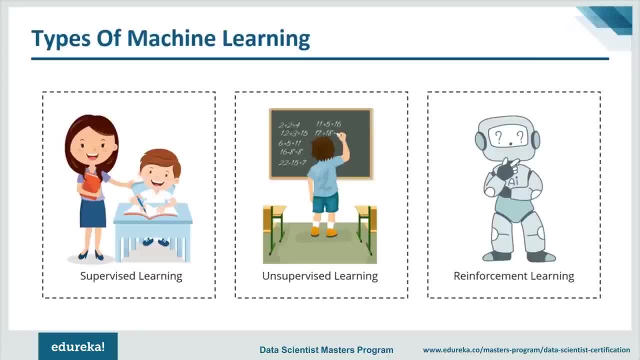 surrounding, and the only way to learn is experience, and then learn from your experience. this is exactly what reinforcement learning is. it is a learning method wherein an agent interacts with its environment by producing actions and discovers errors or rewards- all right- and once it gets ready to predict the new data presented to it. now, in our case, the agent was you. 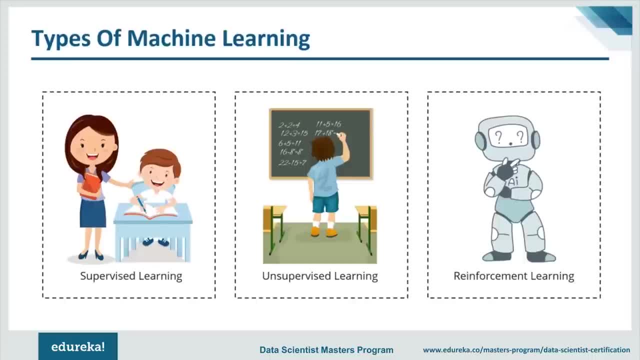 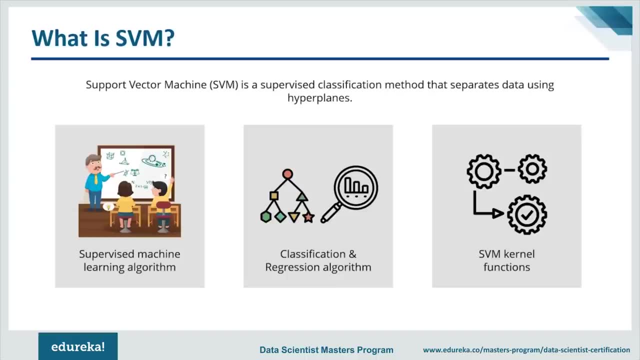 basically stuck on the island and the environment was the island. all right, okay, now let's move on and see what SVM algorithm is all about. so, guys, SVM, or support vector machine, is a supervised learning algorithm which is mainly used to classify data into different classes. now, unlike most algorithms, SVM makes use. 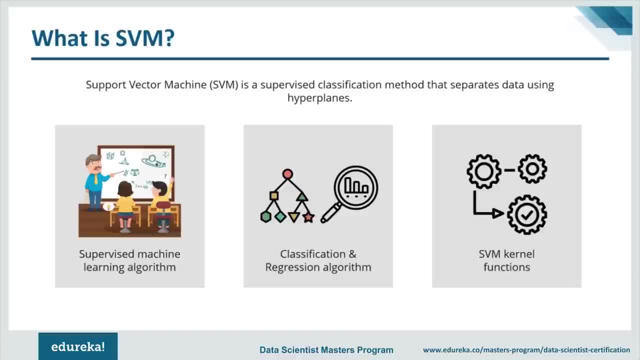 of a hyperplane which acts like a decision boundary between the various classes. in general, SVM can be used to generate multiple separating hyperplanes so that the data is divided into segments- okay- and each of these segments will contain only one kind of data. it's mainly used for classification purpose. 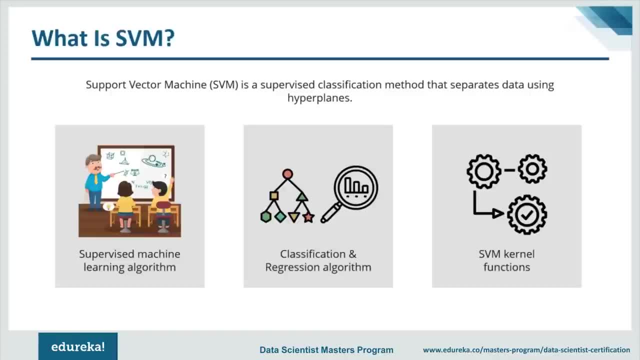 wherein you want to classify a data into two different segments depending on the features of the data. now, before moving any further, let's discuss a few features of SVM. like I mentioned earlier, SVM is a supervised learning algorithm. this means that SVM trains on a set of label data. SVM studies the label training data and then classifies any. 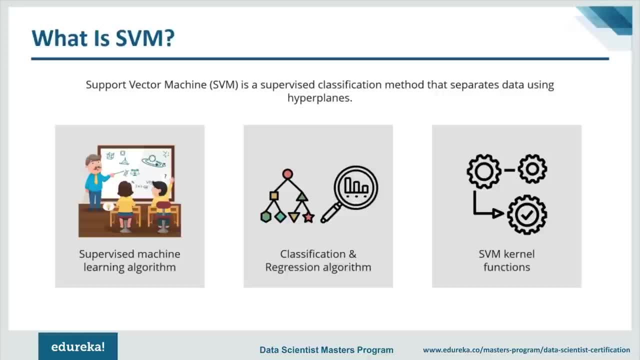 new input data, depending on what it learned in the training phase. a main advantage of support vector machine is that it can be used for both classification and regression problems. all right now, even though SVM is mainly known for classification, the SVR, which is the support vector regressor, is used. 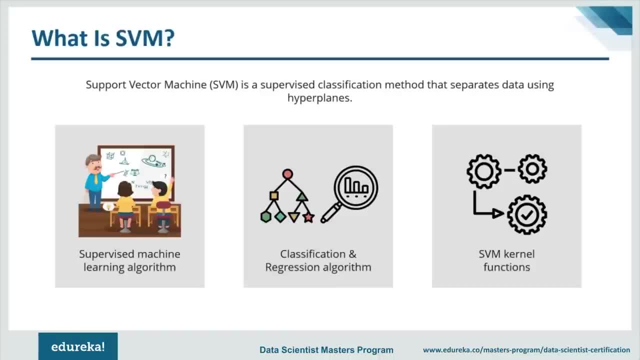 for regression problems. all right, so SVM can be used both for classification and for regression. now, this is one of the reasons why a lot of people prefer SVM, because it's a very good classifier and, along with that, it is also used for regression. okay, another feature is the SVM kernel functions SVM can be used for. 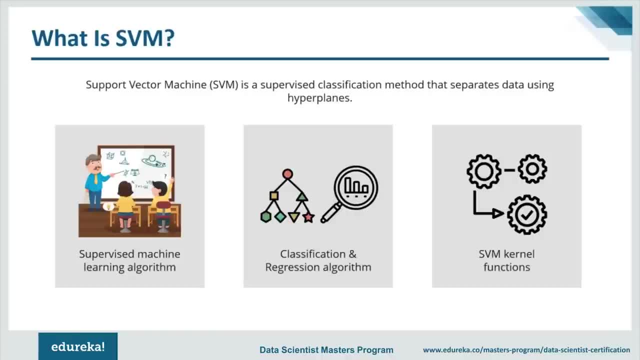 classifying nonlinear data by using the kernel trick. the kernel trick basically means to transform your data into another dimension so that you can easily draw a hyperplane between the different segments of the data, so that you can easily draw a hyperplane between the different classes of the data. all right, nonlinear data is basically data which. 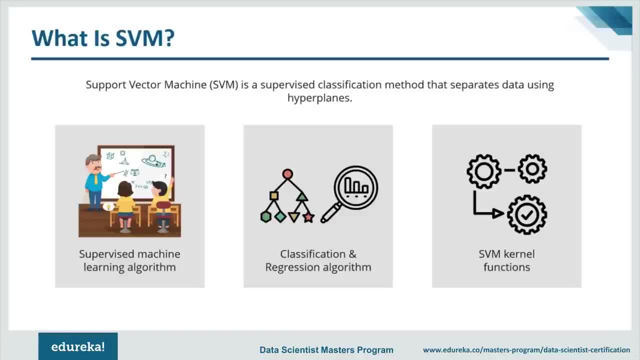 cannot be separated with a straight line. all right, so SVM can even be used on nonlinear data sets. you just have to use the kernel functions to do this. all right. so, guys, I hope you all are clear with the basic concepts of SVM. now let's move on and look at how SVM works. so there's an order to understand how. 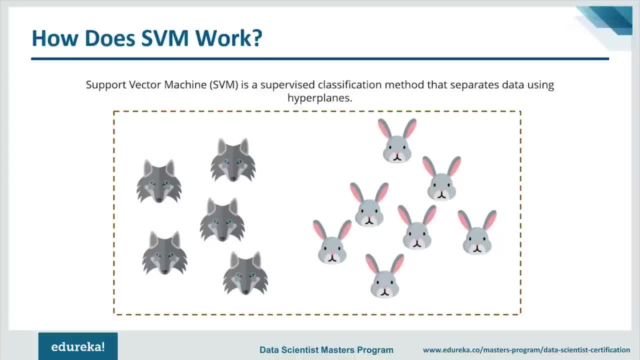 SVM works. let's consider a small scenario now for a second. pretend that you own a farm. okay, and let's say that you have a and you want to set up a fence to protect your rabbits from the pack of wolves. okay, But where do you build your fence? One way to get around the problem is to build a classifier based on. 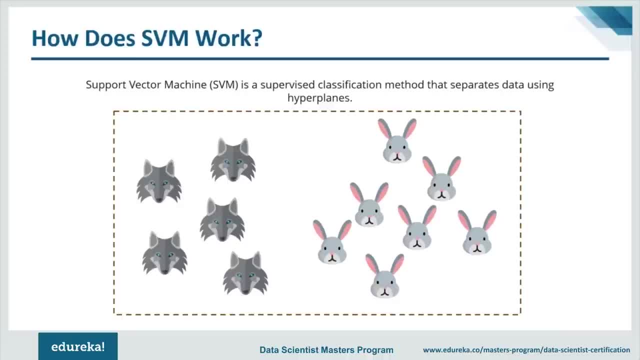 the position of the rabbits and wolves in your pasture. So what I'm telling you is you can classify the group of rabbits as one group and draw a decision boundary between the rabbits and the wolves, all right. So if I do that and if I try to draw a decision boundary between the rabbits, 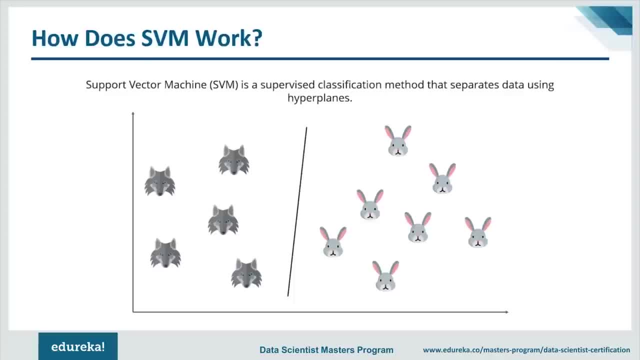 and the wolves. it looks something like this: okay, Now you can clearly build a fence along this line. In simple terms, this is exactly how SVM works. It draws a decision boundary, which is a hyperplane between any two classes, in order to separate them or classify them. Now I know you're. 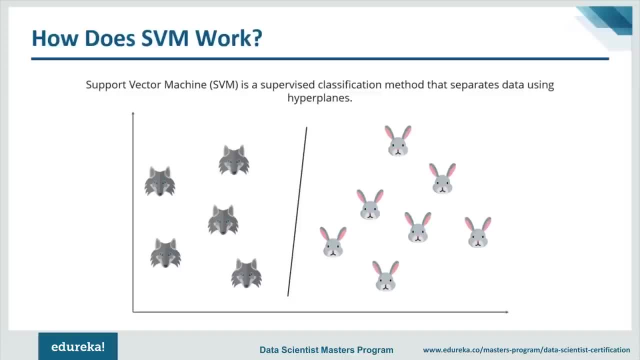 thinking: how do you know where to draw a hyperplane? The basic principle behind SVM is to draw a hyperplane that best separates the two classes. In our case, the two classes are the rabbits and the wolves. So you start off by drawing a random hyperplane and then you check the distance between the 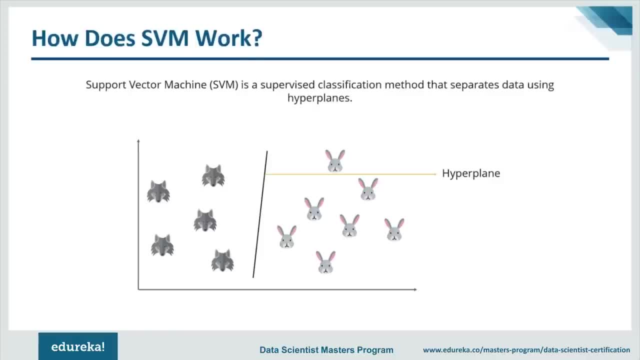 hyperplane and the closest data points from each class. These closest or nearest data points to the hyperplane are known as support vectors, and that's where the name comes from: support vector machine. So, basically, the hyperplane is drawn based on these support vectors. So, guys, an optimum. 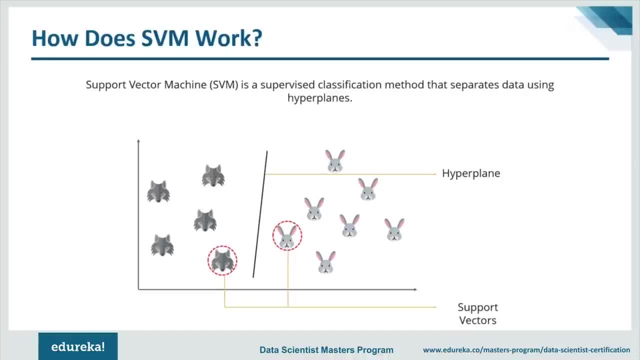 hyperplane will have a maximum distance from each of these support vectors. all right, So basically, the hyperplane which has the maximum distance from each of these support vectors is called a maximum distance from the support vectors is the most optimum hyperplane And this distance between 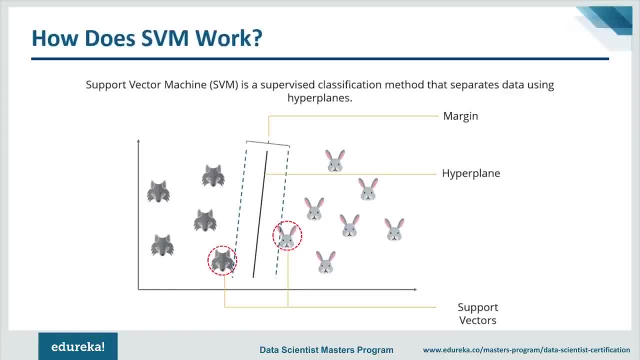 the hyperplane and the support vectors is known as the margin. all right, So to sum it up, SVM is used to classify data by using a hyperplane, such that the distance between the hyperplane and the support vectors is maximum. So basically, your margin has to be maximum. all right, That way you know that. 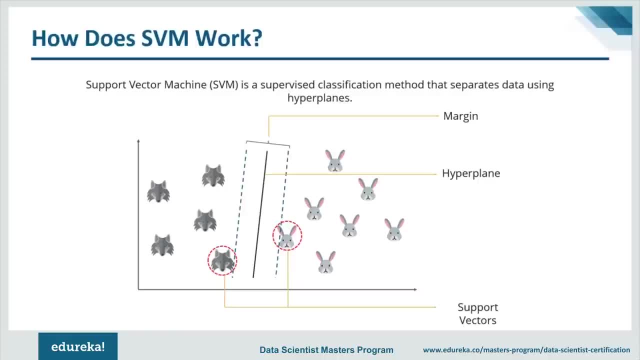 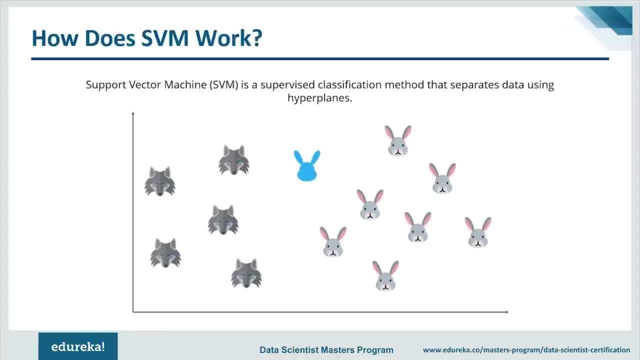 you're actually separating your classes. all right, Because the distance between the two classes is maximum. okay, Now let's try to solve a problem. So let's try to solve a problem. So let's try to solve a problem. okay. So let's say that I input a new data point. okay, This is a new data point. And now I 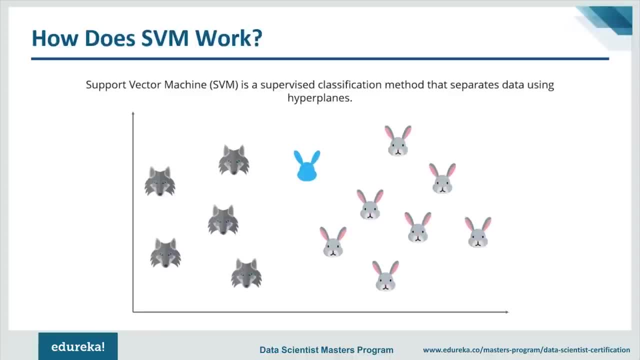 want to draw a hyperplane such that it best separates the two classes. okay, So I start off by drawing a hyperplane like this and then I check the distance between the hyperplane and the support vectors. okay, So I'm trying to check if the margin is maximum for this hyperplane. But what if I draw 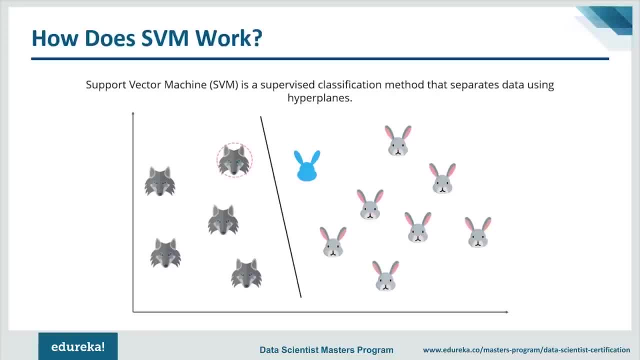 a hyperplane which is like this: all right. Now I'm going to check the support vectors over here, The distance from the support vectors, and for this hyperplane it's clear that the margin is more all right. When you compare the margin of the previous one to this hyperplane, it is more So. 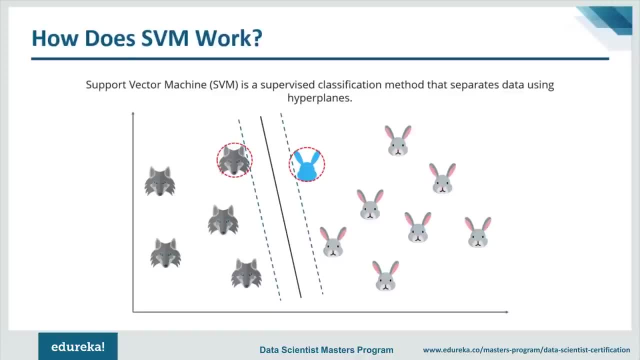 the reason why I'm choosing this hyperplane is because the distance between the support vectors and the hyperplane is maximum in this scenario. okay, So, guys, this is how you choose a hyperplane. You basically have to make sure that the hyperplane has a maximum margin. all right, It has to best. 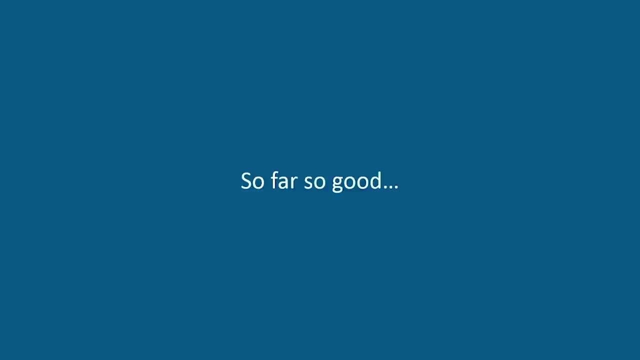 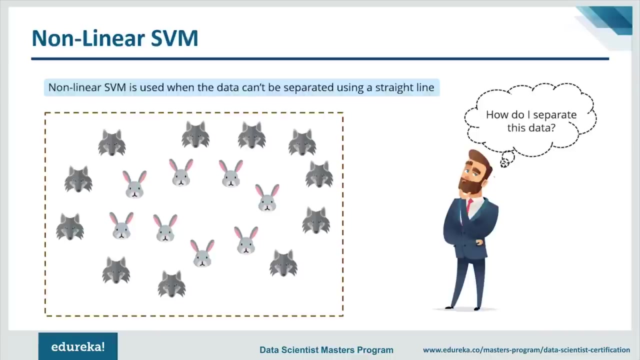 separate the two classes. So far, it was quite easy. Our data was linearly separable, which means that you could draw a straight line to separate the two classes. all right, But what will you do if the data set is like this? You possibly can't draw a hyperplane like this. all right, It doesn't. 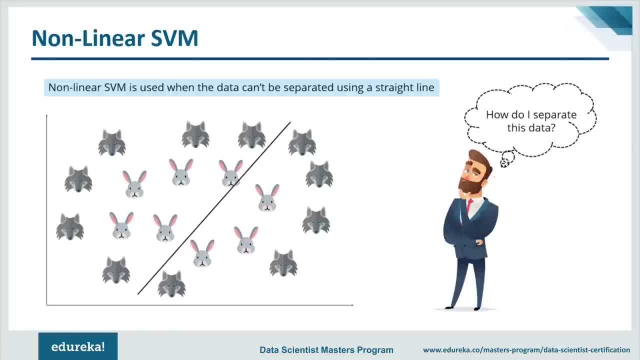 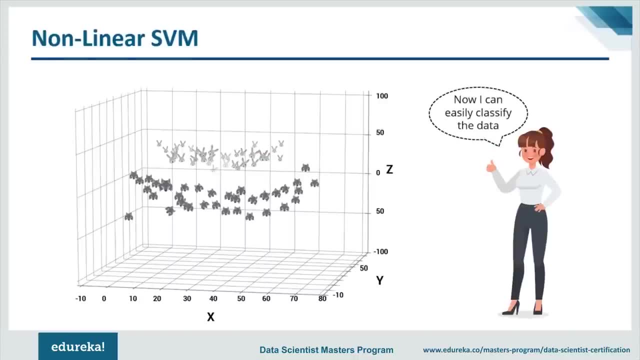 separate the two classes at all. So what do you do in such situations? Now? earlier in the session I mentioned how a kernel can be used to transform data into another dimension that has a clear dividing margin between the classes of data. All right, So kernel functions offer the user this option of transforming nonlinear spaces into. 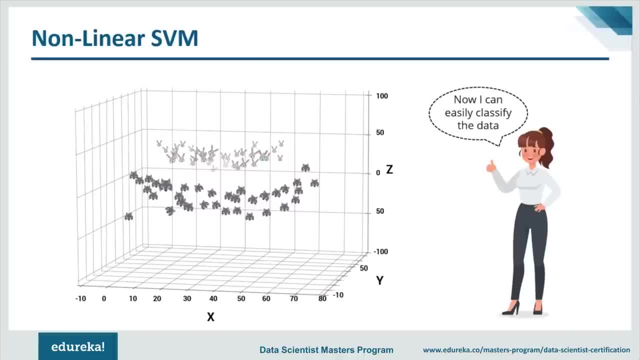 linear ones. Nonlinear data set is the one that you can't separate using a straight line. all right, In order to deal with such data sets, you're going to transform them into linear data sets and then use SVM on them. okay, So a simple trick would be to transform the two variables x and y into a new. 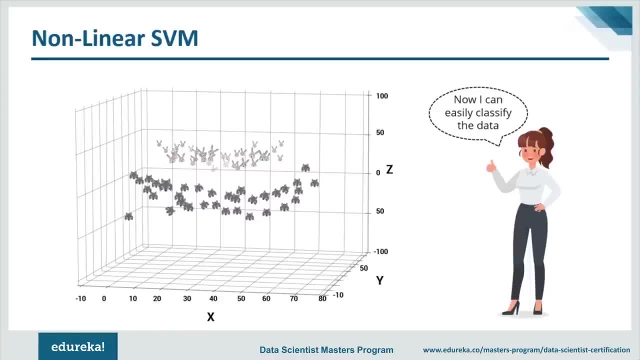 feature space involving a new variable called z. all right, So, guys, I'm going to show you how to do this. So first, I'm going to show you how to do this. So, guys, so far we were plotting our data on two-dimensional space, correct, We were only using 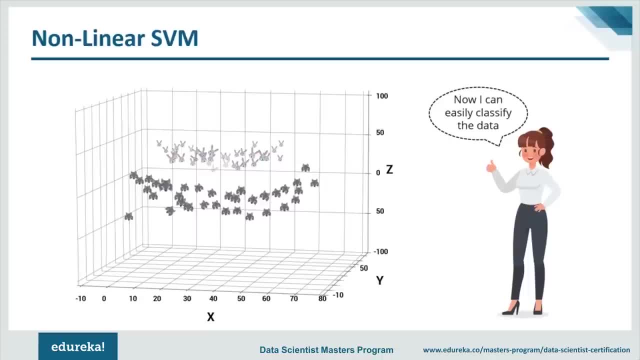 the x and the y-axis, So we had only those two variables, x and y. Now, in order to deal with this kind of data, a simple trick would be to transform the two variables x and y into a new feature space involving a new variable called z. okay, So we're basically visualizing the data on a. 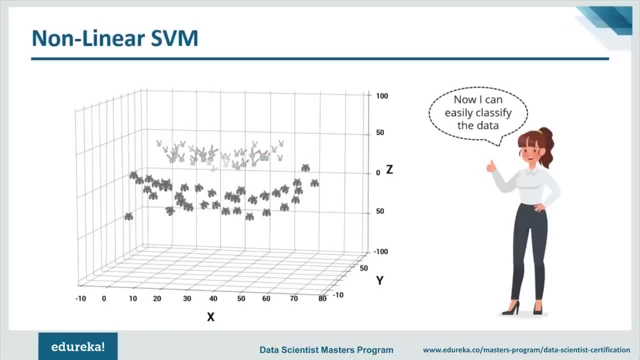 three-dimensional space. Now, when you transform the 2D space into a 3D space, you can clearly see a dividing margin between the two classes of data. all right, Now you can go ahead and separate the two classes by drawing the best hyperplane between them. okay, That's exactly what we discussed in the 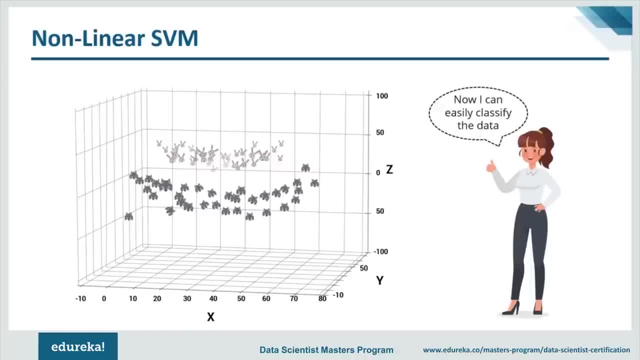 previous slides. So, guys, why don't you try this yourself? Try drawing a hyperplane which is the most optimum for these two classes. all right, So, guys, I hope you have a good understanding about nonlinear SVMs. Now let's look at a real-world use case of support vector machines. So, guys, 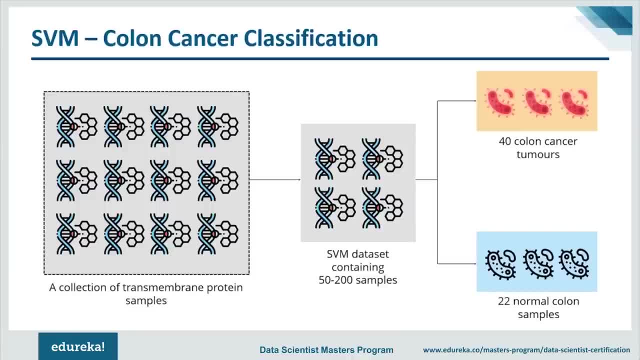 SVM as a classifier has been used in cancer classification since the early 2000s. So there was an experiment held by a group of professionals who applied SVM in a colon cancer tissue classification. So the data set consisted of about 2,000 transmembrane protein samples and only about 50 to 200 gene samples were input into. 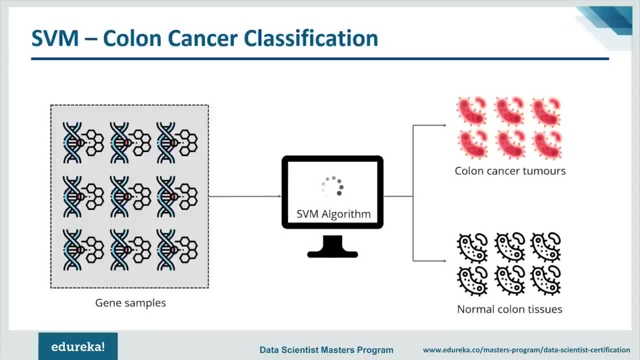 the SVM classifier. Now, this sample, which was input into the SVM classifier, had both colon cancer tissue samples and normal colon tissue samples. All right Now. the main objective of the study was to classify gene samples based on whether they are cancerous or not. okay, So SVM was trained using the 50 to 200 samples in order. 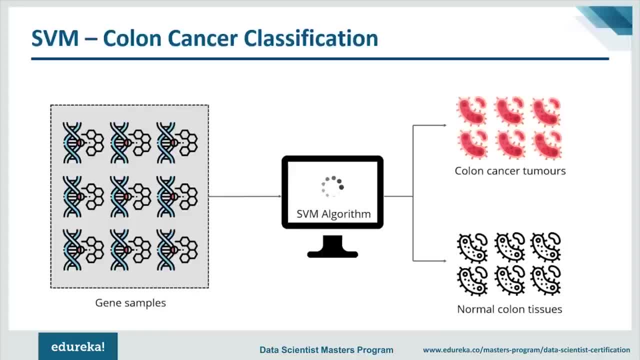 to discriminate between non-tumor from tumor specimens. So the performance of the SVM classifier was very accurate for even a small data set. all right, We had only 50 to 200 samples and even for the small data set, SVM was pretty accurate with its results. Not only that, its performance was. 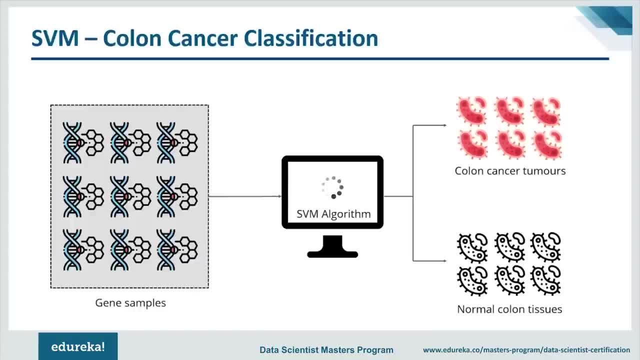 similar to other classification algorithms like Naive Bayes, and in each case SVM outperformed Naive Bayes. So after this experiment, it was clear that SVM classified the data more effectively and it worked exceptionally good with small data sets. 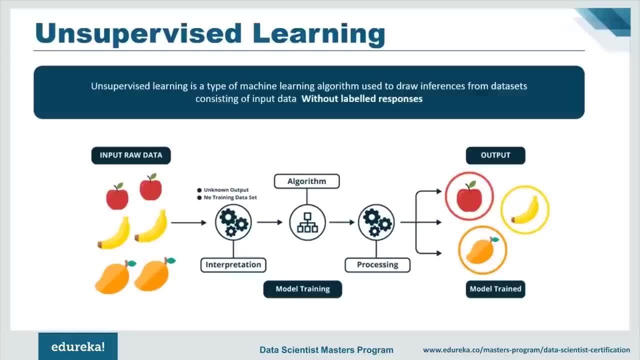 Let's go ahead and understand what exactly is unsupervised learning. So sometimes the given data is unstructured and unlabeled, so it becomes difficult to classify the data into different categories. So unsupervised learning helps to solve this problem. This learning is used. 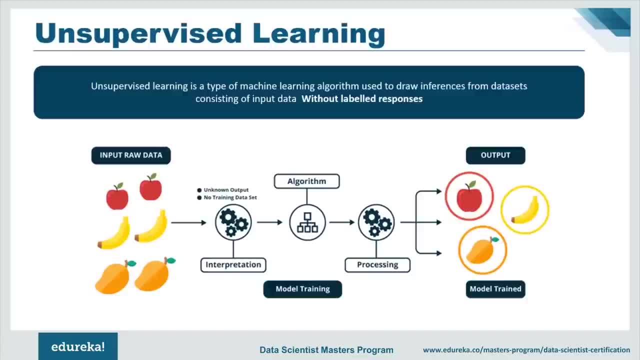 to cluster the input data in classes on the basis of their statistical properties. So, example, we can cluster different bikes based upon their speed limit, their acceleration or the average that they are giving. So unsupervised learning is a type of machine learning algorithm used to draw. 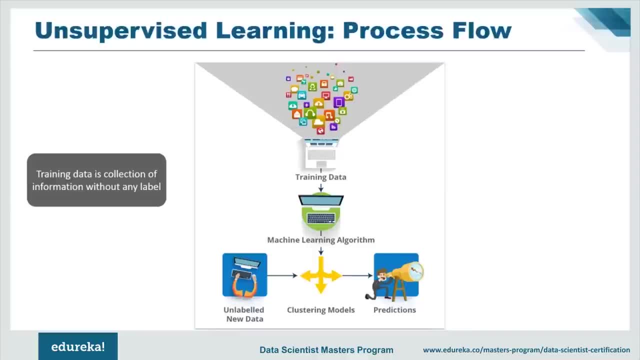 inferences from data sets consisting of input data without labeled responses. So if you have a look at the flow or the process flow of unsupervised learning, so the training data is a collection of information without any label. We have the machine learning algorithm and then we 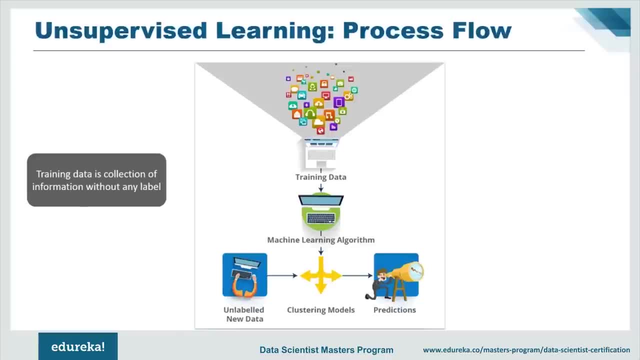 have the clustering models. So what it does is that it distributes the data into different clusters And, again, if you provide any unlabeled new data, it will make a prediction and find out to which cluster that particular data or the data set belongs to, or the particular. 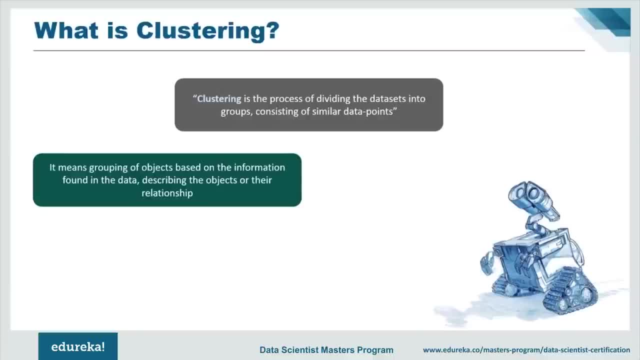 data point belongs to. So one of the most important algorithms in unsupervised learning is clustering. Let's understand exactly what is clustering. So clustering, basically, is the process of dividing the data sets into groups consisting of similar data points. It means grouping of objects based 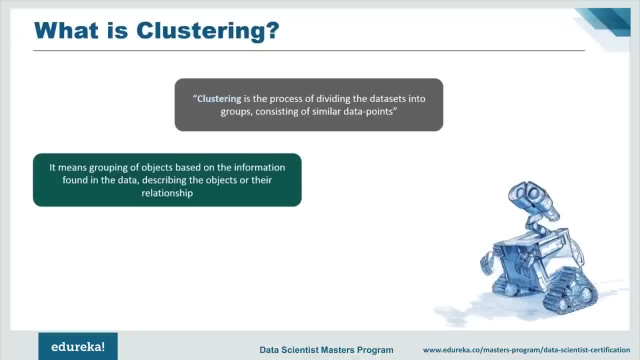 on the information found in the data describing the objects or their relationships. So clustering models focus on identifying groups of similar records and labeling records according to the group to which they belong. Now, this is done without the benefit of prior knowledge about the groups and their characteristics. So, and in fact, we may not even know exactly how. 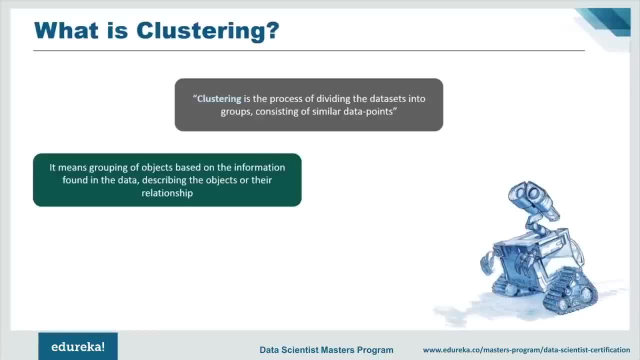 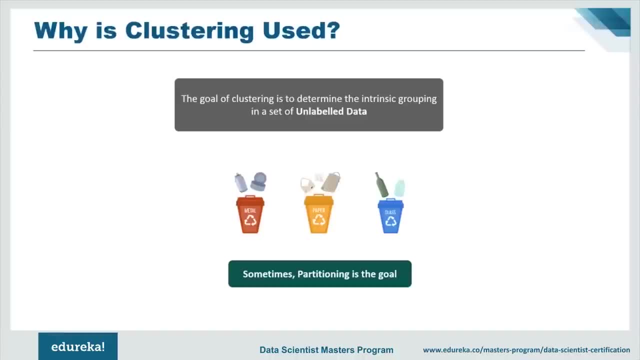 many groups are there to look for. Now, these models are often referred to as unsupervised learning models, since there's no external standard by which to judge the model's classification performance. There are no right or wrong answers to these models, And if we talk about why, 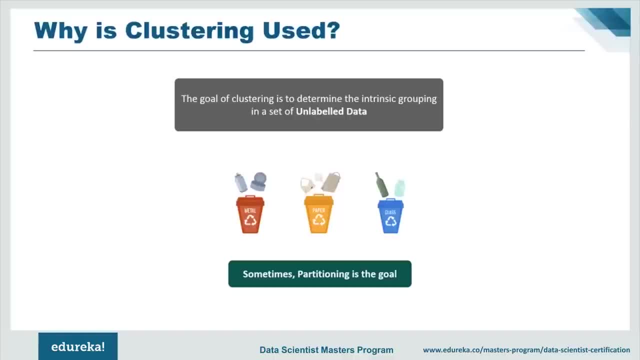 clustering is used. so the goal of clustering is to determine the intrinsic group in a set of unlabeled data. Sometimes the part of the data set is used to determine the intrinsic group in a set of unlabeled data. Sometimes the part of the data set is used to determine the intrinsic. 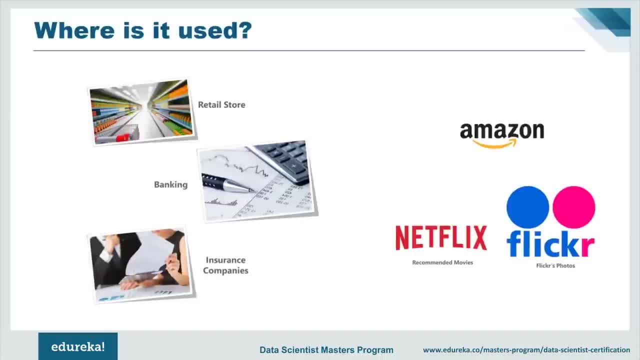 group in a set of unlabeled data. Sometimes the part of the data set is used to determine the intrinsic group in a set of unlabeled data, And so that's why clustering is used in the industry, And if you have a look at the various use cases of clustering in the 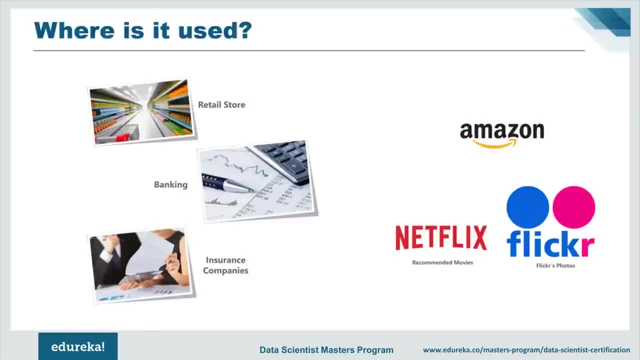 industry. so, first of all, it's being used in marketing, So discovering distinct groups and customer databases, such as customers who make a lot of long distance calls, customers who use internet more than calls. They're also used in insurance companies, like identifying groups of corporation insurance policyholders. 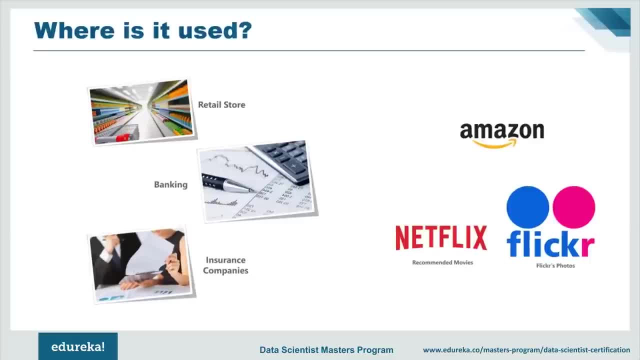 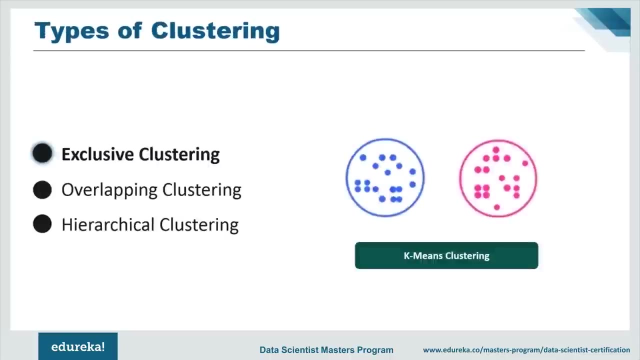 with high average claim rate. farmers crash cops, which is profitable. They are used in seismic studies and define probable areas of oil or gas exploration based on seismic data, And they're also used in the recommendation of movies, if you'd say. They're also used in Flickr photos. 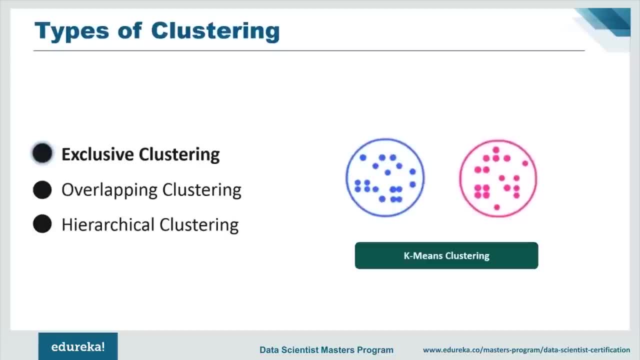 They're also used by Amazon for recommending the product, which category it lies in. So basically, if we talk about clustering, there are three types of clustering. So first of all we have the exclusive clustering, which is the hard clustering. So here an item belongs exclusively to one cluster, not several clusters. 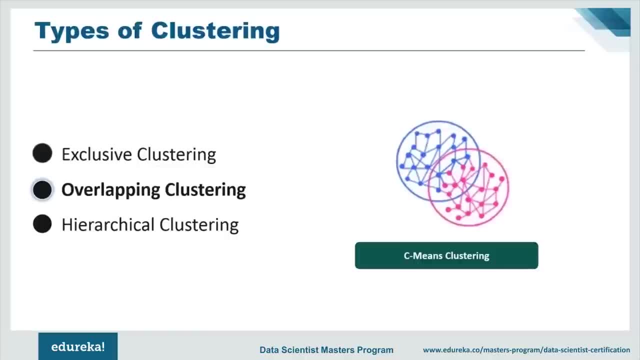 And the data point belong exclusively to one cluster. So an example of this is the K-mean clustering. So K-mean clustering does this exclusive kind of clustering. So secondly, we have overlapping clustering, So it is also known as soft clusters in this. 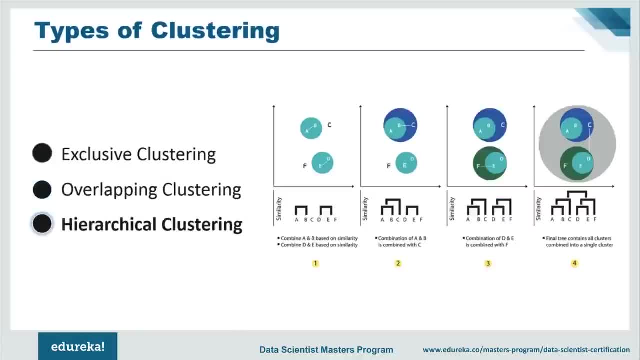 An item can belong to multiple clusters as its degree of association with each cluster is shown. And, for example, we have fuzzy or the C-means clustering, which is being used for overlapping clustering, And finally we have the hierarchical clustering, So when two clusters have a parent-child relationship or a tree-like structure. 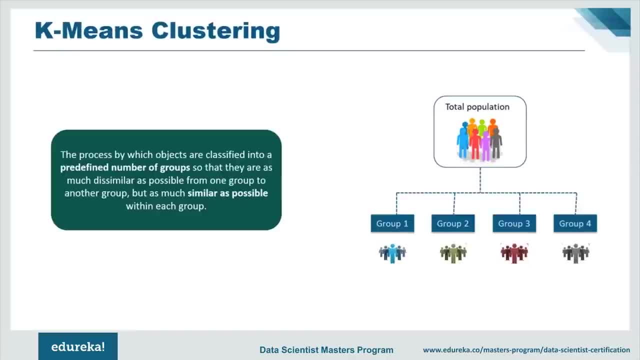 then it is known as hierarchical cluster. So, as you can see here from the example, we have a parent-child kind of relationship in the cluster given here. So let's understand what exactly is K-means clustering. So K-means clustering is an algorithm whose main goal is to group similar elements of data points into a cluster. 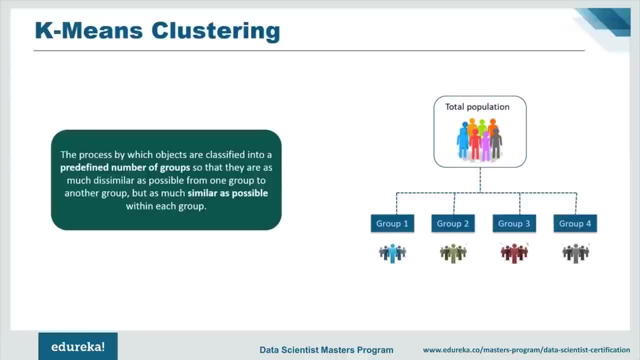 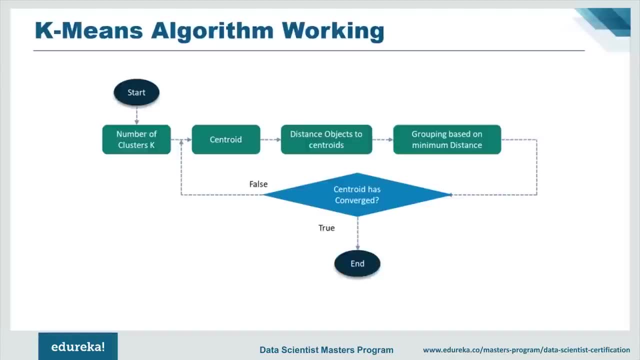 And it is the process by which objects are classified into a predefined number of groups so that they are as much dissimilar as possible from one group to another group, but as much as similar or possible within each group. Now, if you have a look at the algorithm working here, you're right. 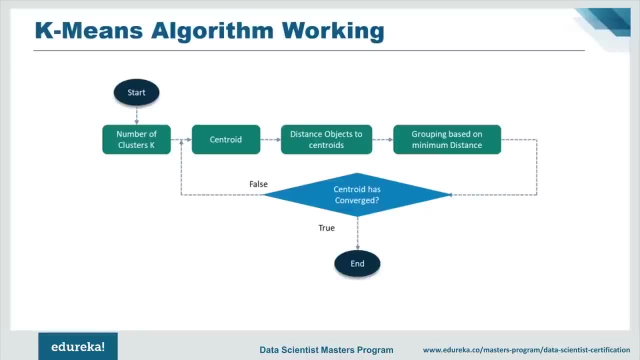 So first of all it starts with identifying the number of clusters, which is K. Then again we find the centroid, We find the distance objects to the distance, object to the centroid, distance of objects to the centroid. Then we find the grouping based on the minimum distance. 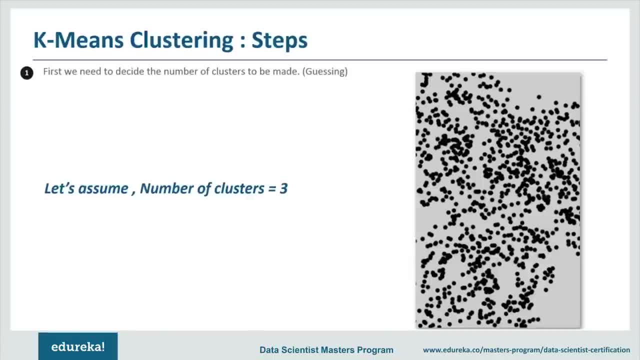 Has the centroid converged? If true, then we make a cluster. If false, we then again find the centroid. repeat all of the steps again and again. So let me show you how exactly clustering works With an example here. So first we need to decide the number of clusters to be made. 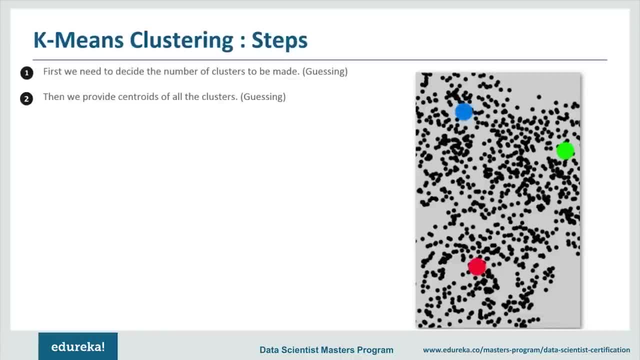 Now, another important task here is how to decide the number of clusters, or how to decide the number of clusters, We'll get into that later. So first let's assume that the number of clusters we have decided is three. So after that, then we provide the centroid for all the clusters. which is guessing? 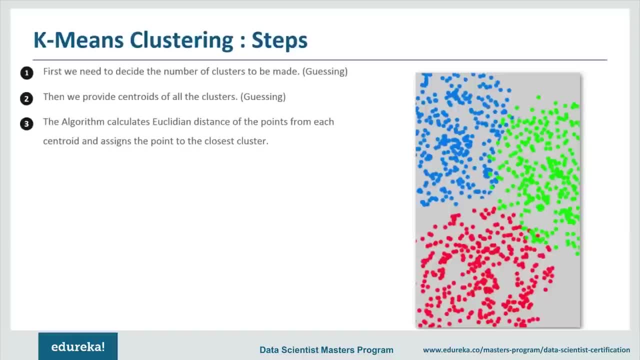 The algorithm calculates the Euclidean distance of the point from each centroid and assigns the data point to it, To the closest cluster. Now, Euclidean distance, all of you know, is the square root of the distance, the square root of the square of the distance. 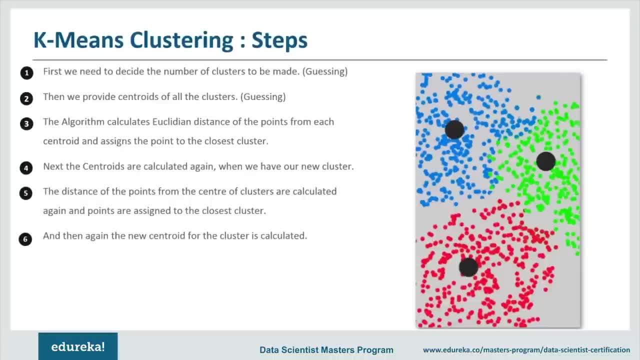 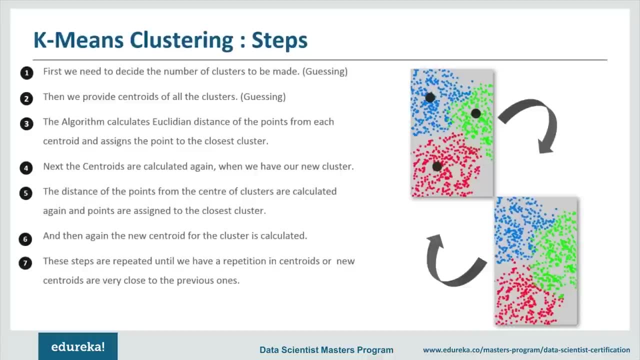 So next, when the centroid is calculated again, we have our new clusters for each data point, Then again the distance from the points to the new clusters are calculated, And then again the points are assigned to the closest cluster, And then again we have the new centroid is calculated. 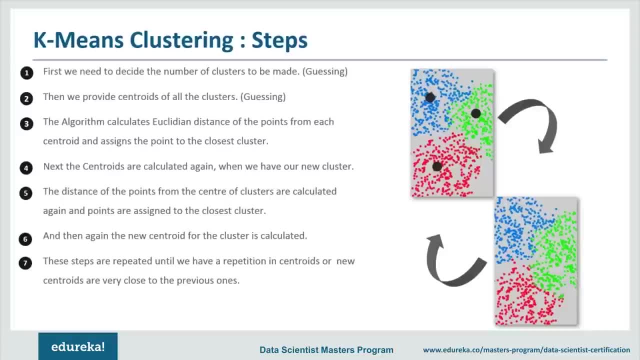 Now these steps are repeated. until we have a repetition, The centroid or the new centroid are very close to the very previous ones. So until and unless our output gets repeated or the outputs are very, very close enough, we do not stop this process. 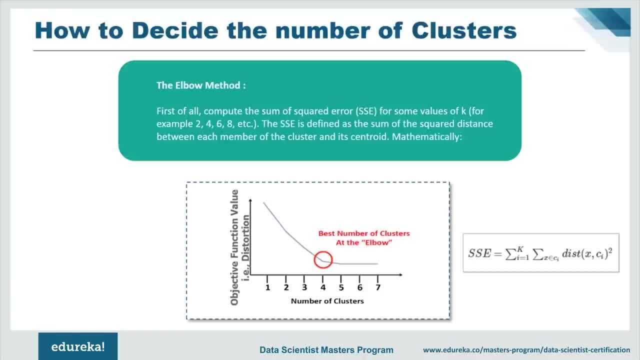 We keep on calculating the Euclidean distance of all the points to the centroid, Then we calculate the new centroid, And that is how K-means clustering works basically. So an important part here is to understand how to decide the value of K or the number of clusters. 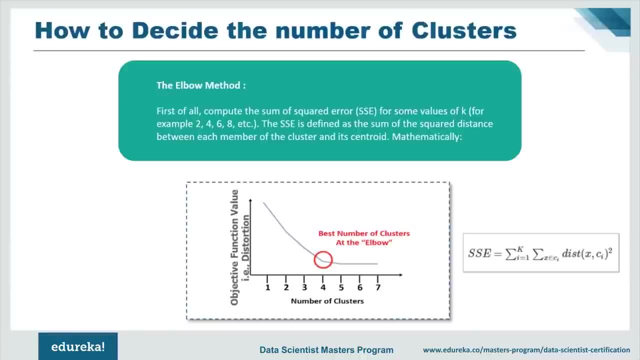 because it does not make any sense if you do not know how many clusters you're going to make. So to decide the number of clusters we have the Elbow method. So let's assume first of all compute the sum squared. error, which is the SSE for some value of K. 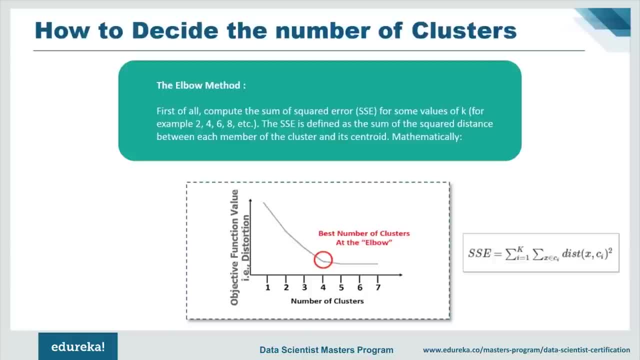 For example, let's take 2,, 4,, 6 and 8.. Now the SSE, which is the sum squared error, is defined as the sum of the squared distance between each number member of the cluster and its centroid. Mathematically, it is given by the equation which is provided here: 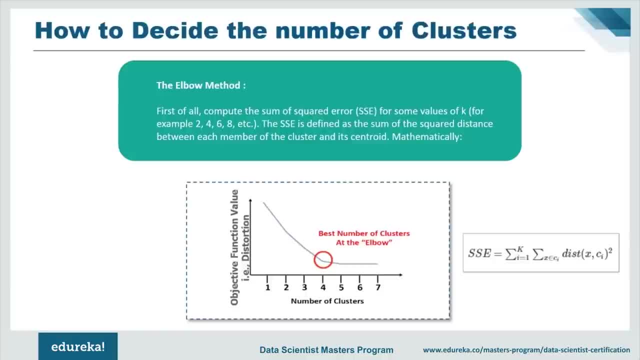 And if you plot the K against the SSE, you will see that the error decreases as K gets large. Now, this is because the number of cluster increases. they should be smaller, So the distortion is also smaller. Now, the idea of the Elbow method is to choose the K at which the SSE decreases abruptly. 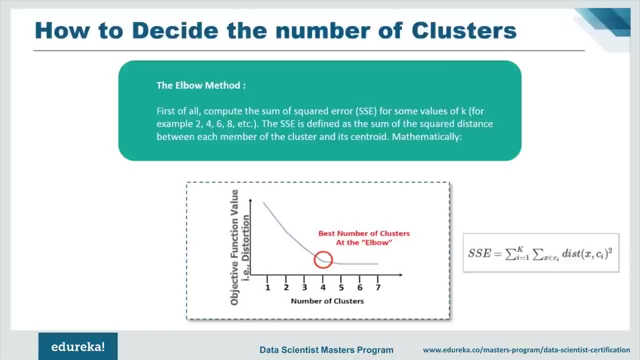 So for example here, if we have a look at the figure given here, we see that the best number of cluster is at the Elbow. So as you can see here, the graph here changes abruptly after the number 4.. So for this particular example we're going to use 4 as the number of cluster. 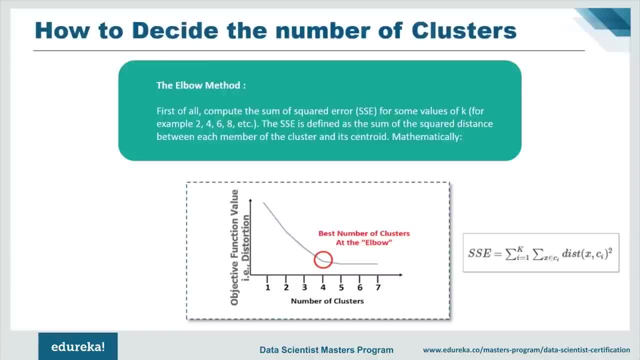 So, first of all, while working with K-means clustering, there are two key points to know. First of all, be careful about where you start. So choosing the first center at random, choosing the second center that is far away from the first center. 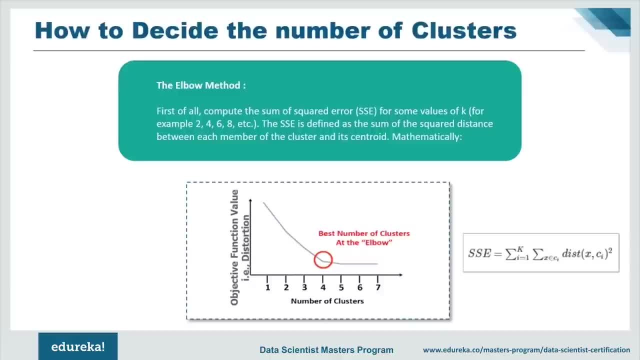 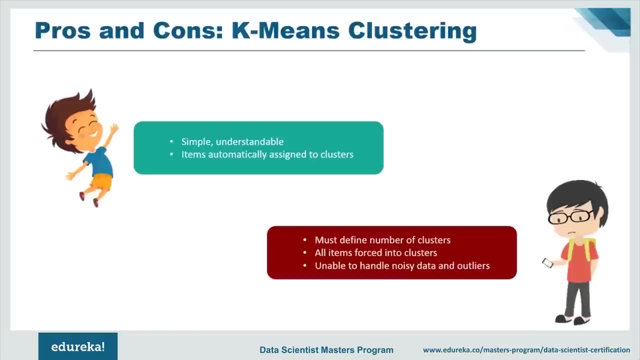 Similarly, choosing the nth center at random. Choose the nth center as far away as possible from the closest of all the other centers. And the second idea is to do as many runs of K-means, each with different random starting points, so that you get an idea of where exactly and how many clusters you need to make. 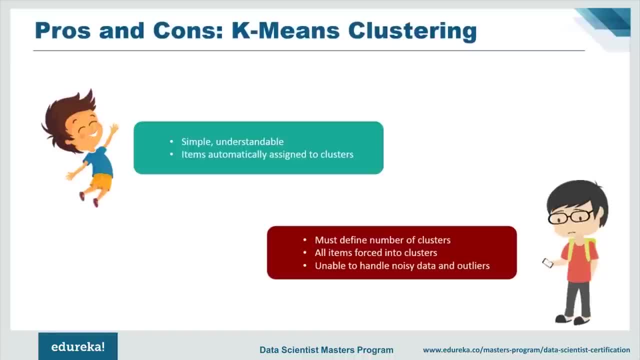 and where exactly the centroid lies and how the data is getting converged. Now, K-means is not exactly a very good method, So let's understand the pros and cons of K-means clustering. We know that K-means is simple and understandable. 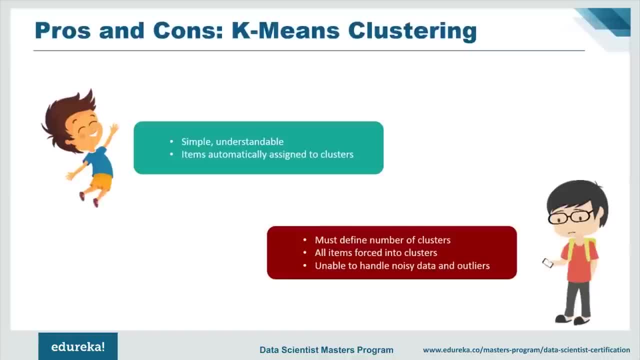 Everyone learns it at the first go- The items automatically assigned to the clusters. Now if we have a look at the cons, So first of all one needs to define the number of clusters. This is a very heavy task, as if we have 3,, 4 or if we have 10 categories. 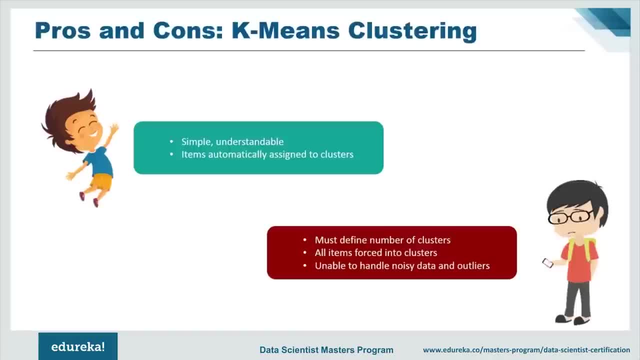 and if we do not know what the number of clusters are going to be, it's very difficult for anyone to guess the number of clusters. Now, all the items are forced into the clusters, Whether they actually belong to any other cluster or any other category. 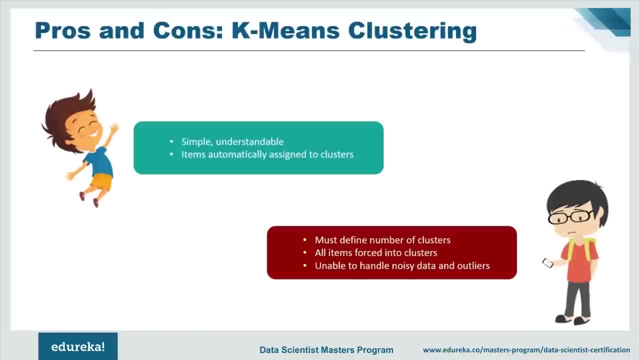 they are forced to lie in that other category in which they are closest to. Now this again happens because of the number of clusters, with not defining the correct number of clusters or not being able to guess the correct number of clusters And, most of all, it's unable to handle the noisy data and the outliners. 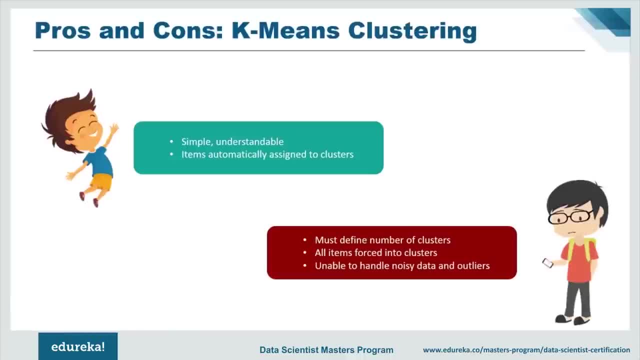 because, anyways, machine learning engineers and data scientists have to clean the data, But then again it comes down to the analysis, what they are doing and the method that they are using. So typically people do not clean the data for k-means clustering. 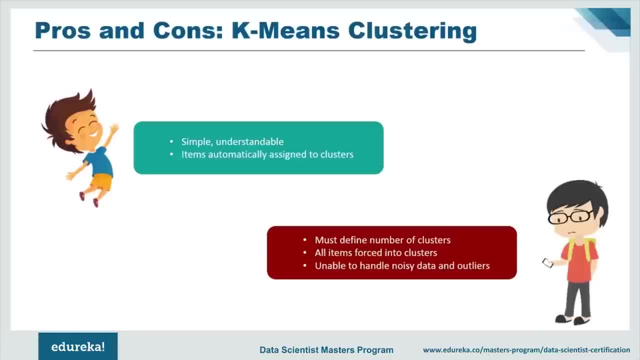 Even if they clean, sometimes there are noisy and outliners data which affect the whole model. So that was all for k-means clustering. So what we're going to do is now use k-means clustering for the movie data set. So we have to find out the number of clusters and divide it accordingly. 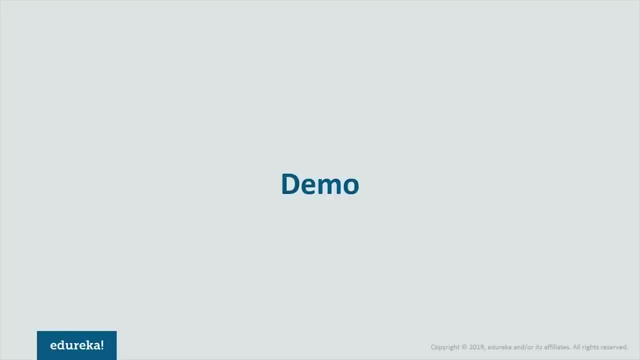 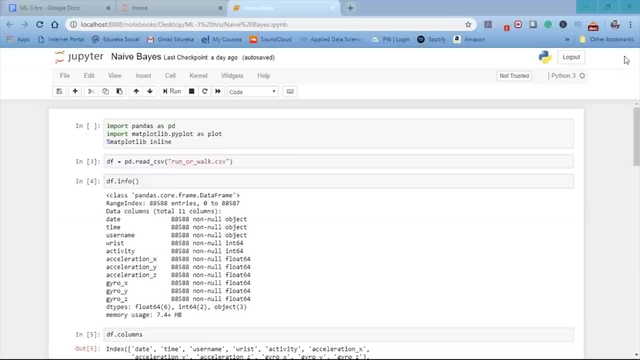 So the use case is that, first of all, we have a data set of 5000 movies and what we want to do is group them, group the movies into clusters based on the Facebook likes. So, guys, let's have a look at the demo here. 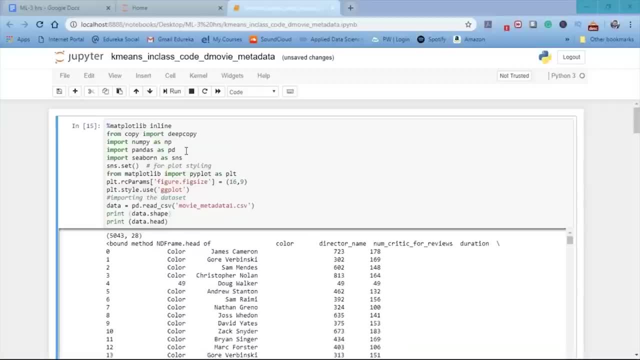 So, first of all, what we're going to do is import DeepCopy, NumPy, Panda, Seaborn, the various libraries which we're going to use now, And from MapRotLib. we're going to use PyPlot and we're going to use this ggplot. 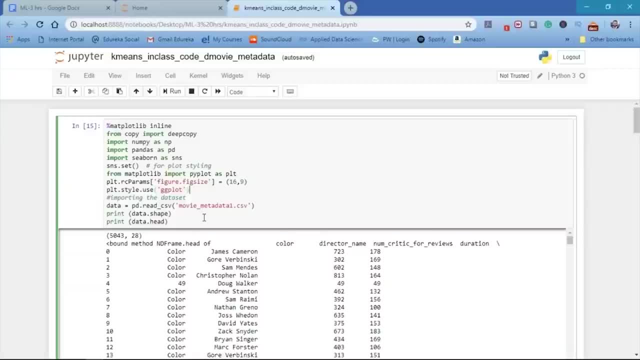 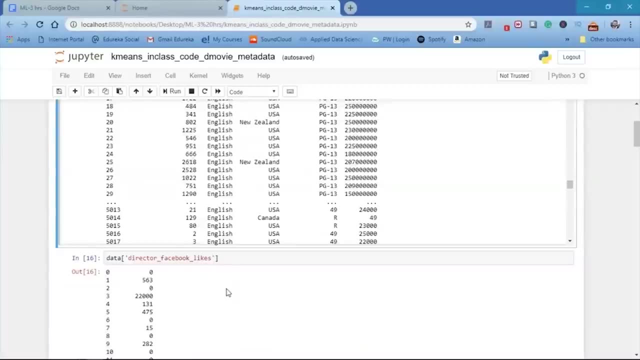 And next, what we're going to do is import the data set and look at it. We're going to look at the shape of the data set. So if you have a look at the shape of the data set, we can see that it has 5043 rows with 28 columns. 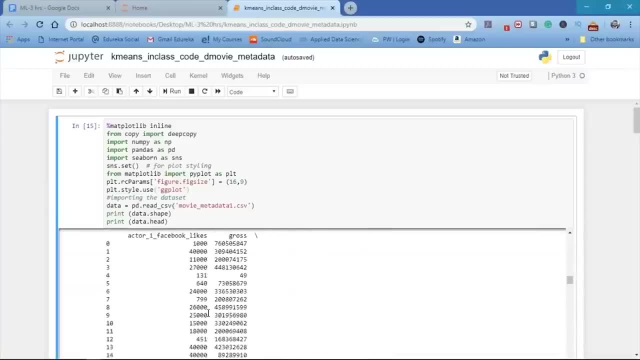 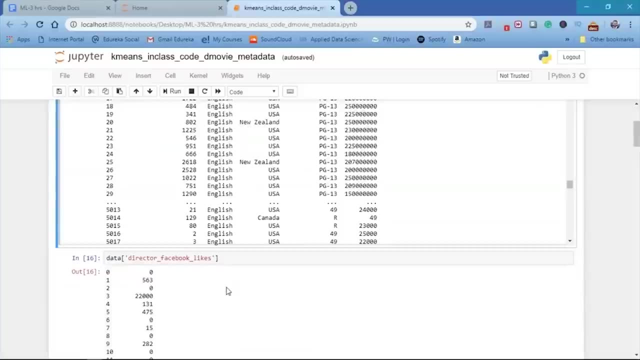 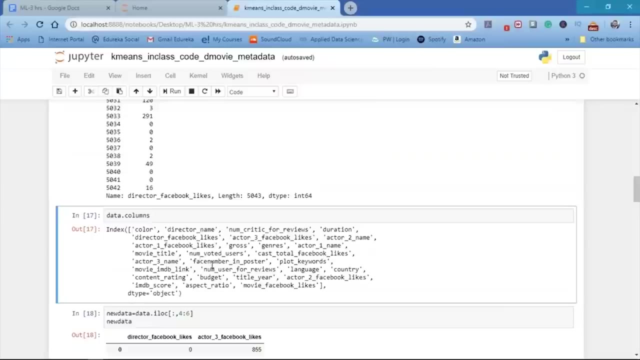 And if you have a look at the head of the data set, we can see it has 5043 data points. So what we're going to do is place the data points in the plot. We take the director Facebook likes and we have a look at the data columns. 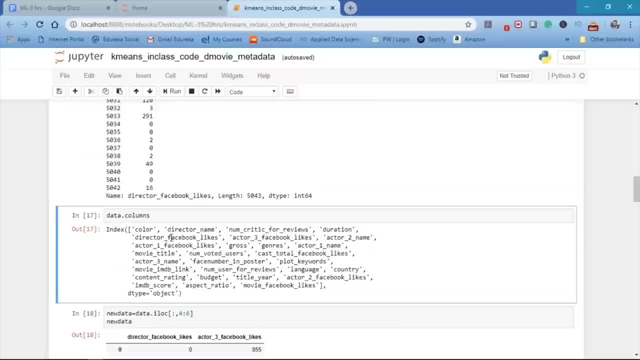 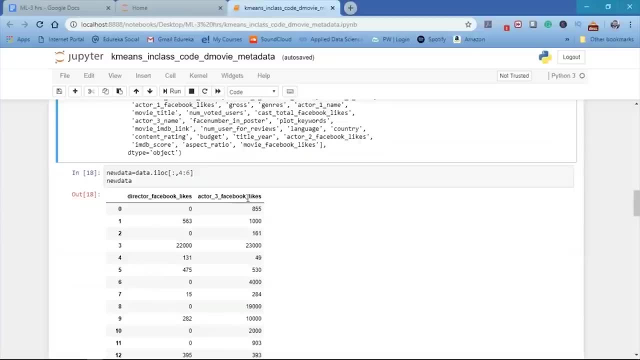 We have face number and poster cast. total Facebook likes- director Facebook likes. So what we have done here now is taking the director Facebook likes and the actor three Facebook likes Right. So we have 5043 rows and two columns. 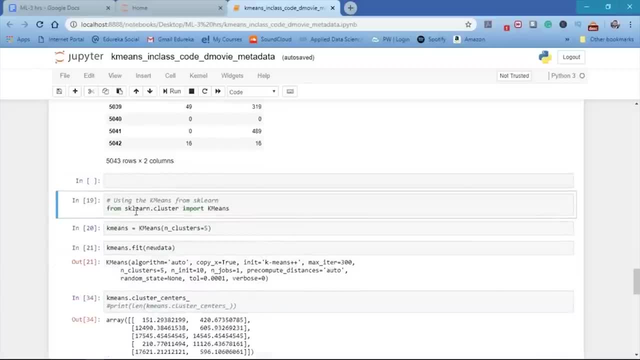 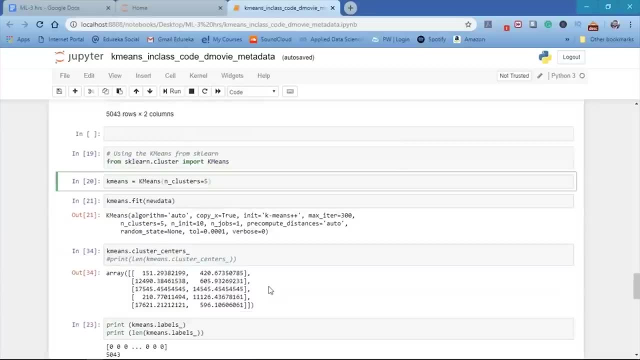 Now using the k-means from sklearn, what we're going to do is import it. first. We're going to import k-means from sklearncluster. Remember, guys, sklearn is a very important library in Python for machine learning- And the number of clusters. what we're going to do is provide as five. 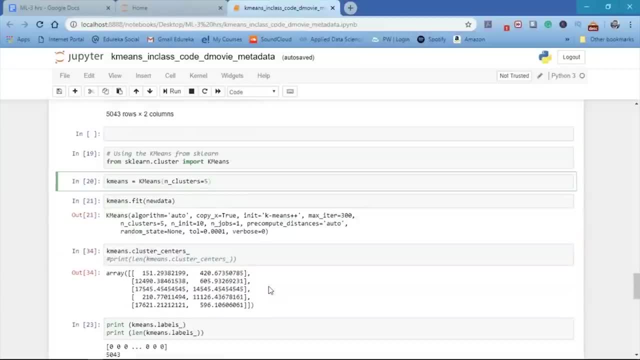 Now this again: the number of clusters depends upon the sse, which is the sum squared errors, or we're going to use the elbow method, So I'm not going to go into the details of that again. So we're going to fit the data into the k-meansfit. 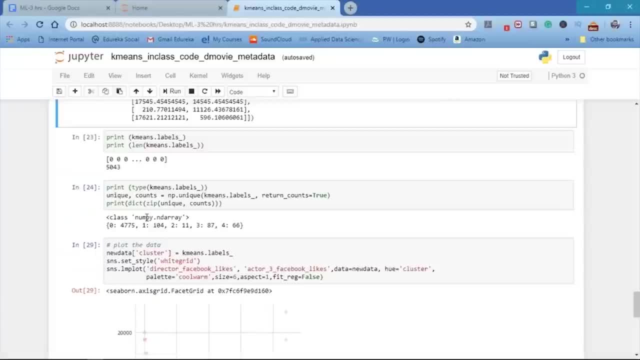 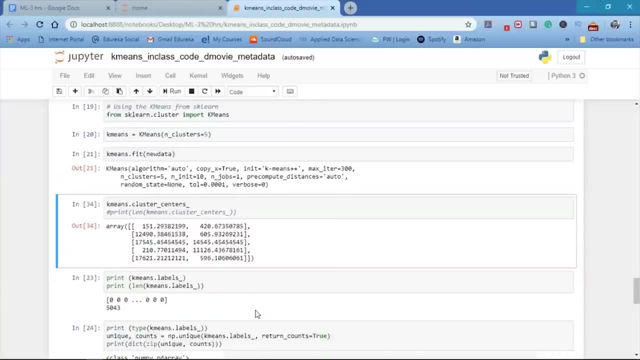 And if we find the cluster centers, then for the k-means and print it. so what we find is an array of five clusters And if we print the label of the k-means cluster, Now next, what we're going to do is plot the data. 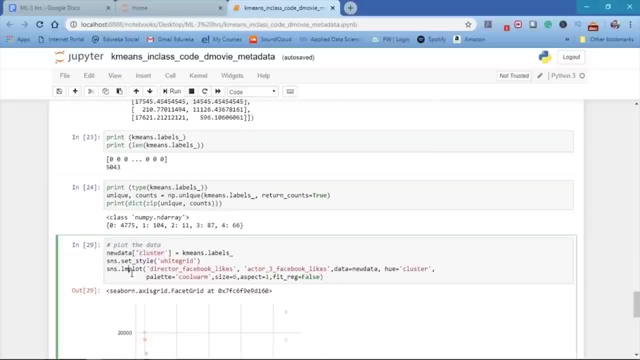 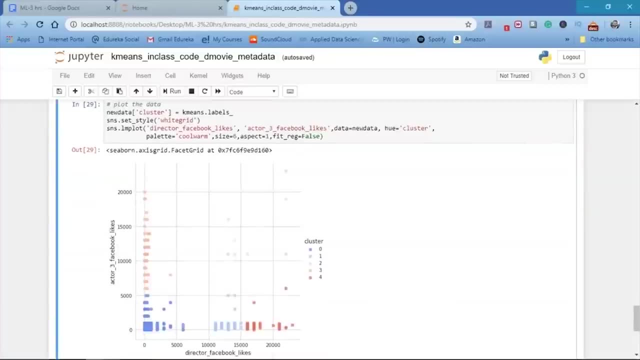 which we have with the clusters, with the new data clusters which we have found, And for this we're going to use the seaborn And, as you can see here we have plotted the data into the grid And you can see, here we have five clusters. 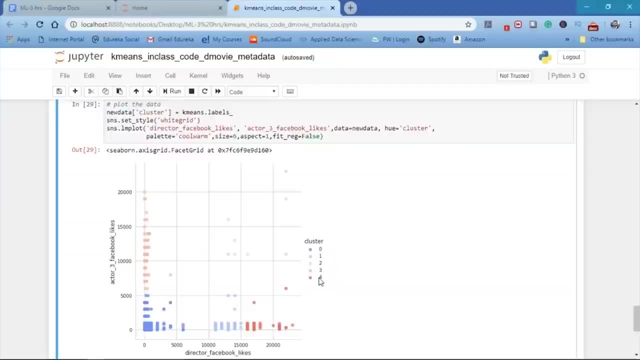 So probably, what I would say is that the cluster three and the cluster zero are very, very close, So it might depend. See, that's exactly what I was going to say is that, initially, the main challenge in k-means clustering is to define the number of centers which are the k. 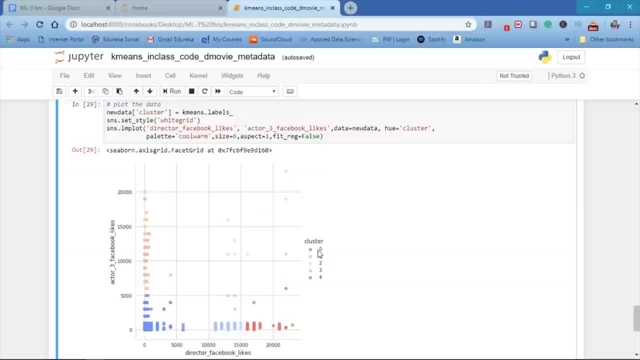 So, as you can see here, the third center and the zeroth cluster, the third cluster and the zeroth cluster- are very, very close to each other. So, guys, it probably could have been in one another cluster, And the another disadvantage was that we do not exactly know. 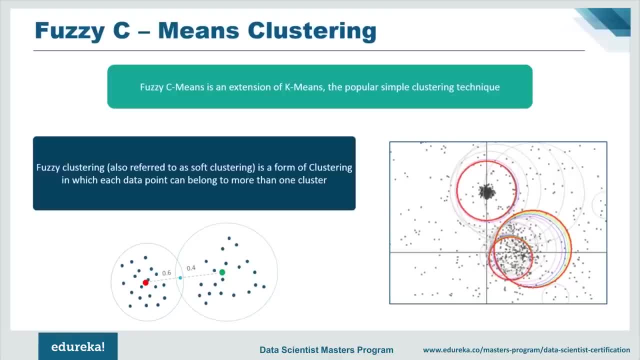 how the points are to be arranged, So it's very difficult to follow. It's very difficult to force the data into any other cluster, which makes our analysis a little different. It works fine, but sometimes it might be difficult to code in the k-means clustering. 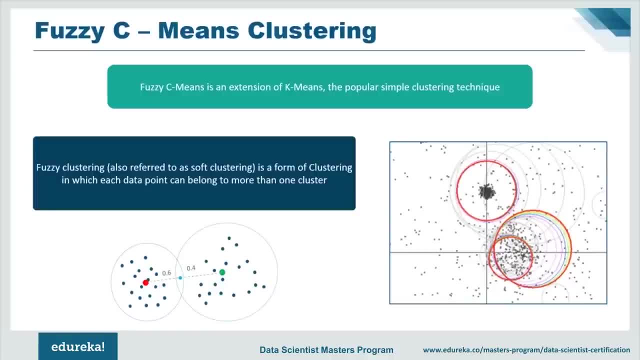 Now let's understand what exactly is c-means clustering? So the fuzzy c-means is an extension of the k-means clustering, the popular simple clustering technique. So fuzzy clustering, also referred to as soft clustering, is a form of clustering in which each data point 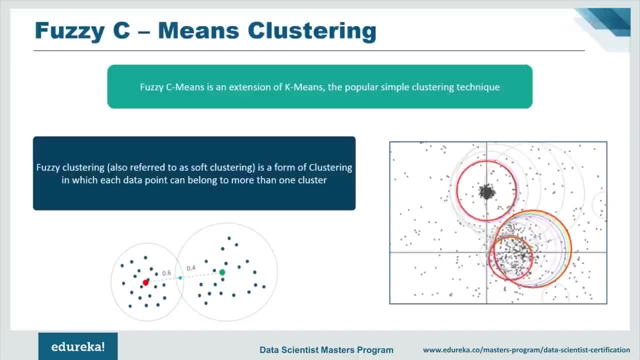 belongs to more than one cluster. So k-means tries to find the hard clusters, where each point belongs to one cluster, whereas the fuzzy c-means discovers the soft clusters. In a soft cluster, any point can belong to more than one cluster at a time, with a certain affinity value towards each. 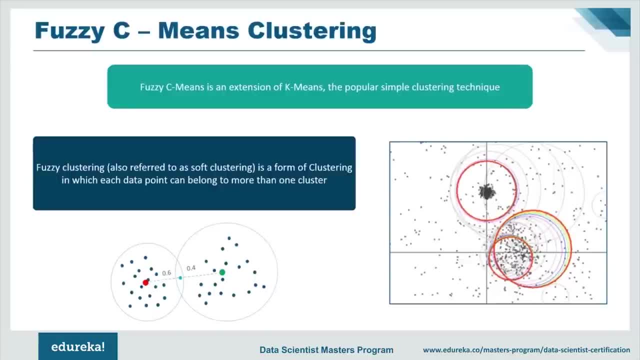 Fuzzy c-means assigns the degree of membership, which ranges from 0 to 1, to an object to a given cluster. So there is a stipulation that the sum of fuzzy membership of an object to all the cluster it belongs to must be equal to 1.. 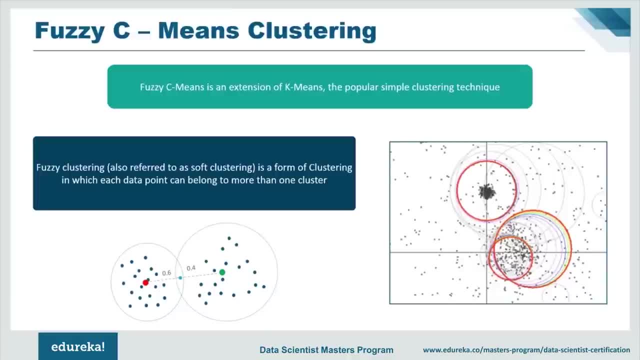 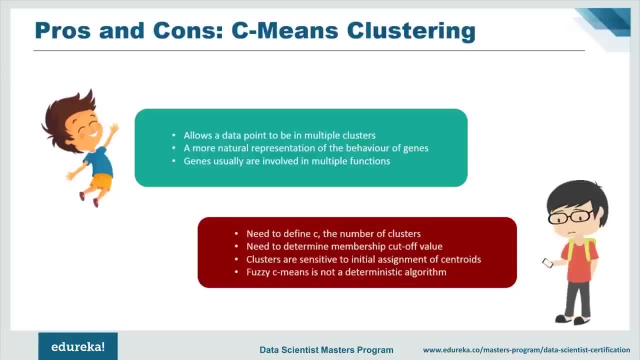 So the degree of membership of this particular point to both of these clusters are 0.6 and 0.4.. And if we add up we get 1.. So that is one of the logic behind the fuzzy c-means. And this affinity is proportional to the distance. 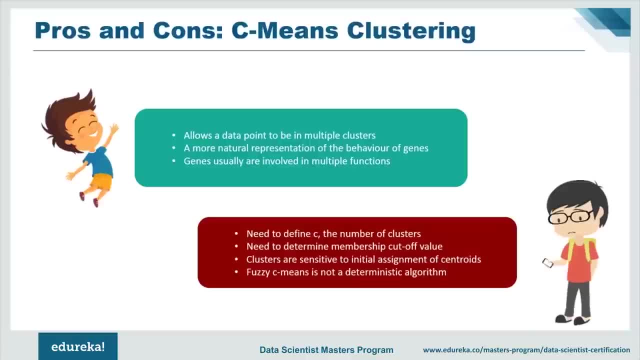 from the point to the centroid of the cluster. Now, then again, we have the pros and cons of fuzzy c-means. So, first of all, it allows a data point to be in multiple clusters. That's a pro. It's a more neutral representation of the behavior of genes. 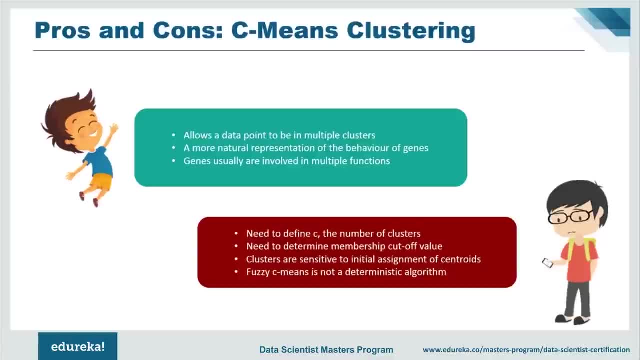 Genes usually are involved in multiple functions, So it is a very good type of clustering when we're talking about genes And again, if we talk about the cons, again we have to define c, which is the number of clusters same as k. 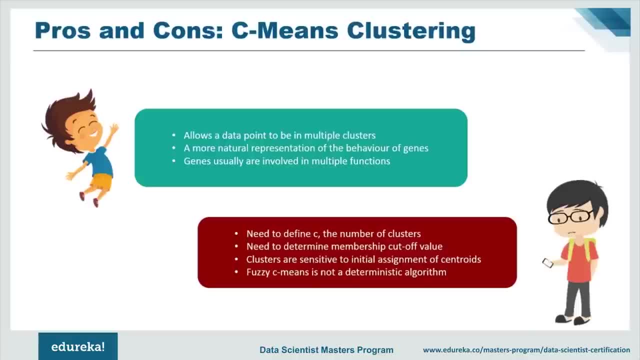 Next we need to determine the membership cutoff value also. So that takes a lot of time and it's time consuming, And the clusters are sensitive to initial assignment of centroid. So a slight change or a deviation from the centroid is going to result in a very different kind of 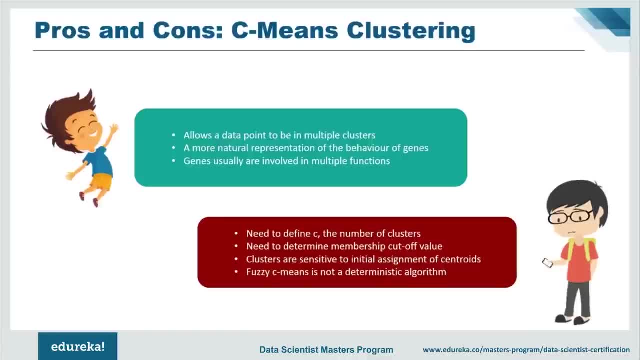 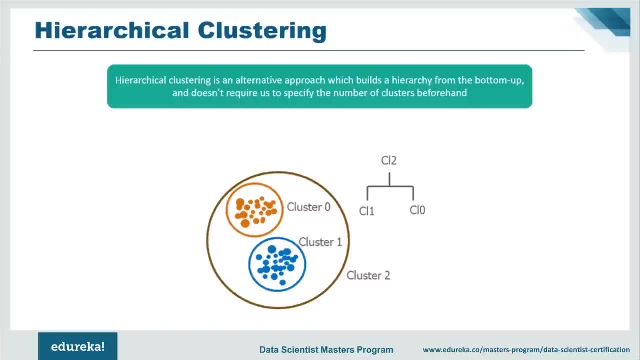 you know a funny kind of output we get from the fuzzy c-means. And one of the major disadvantages of c-means clustering is that there's a non-deterministic algorithm, So it does not give you a particular output, as in such. 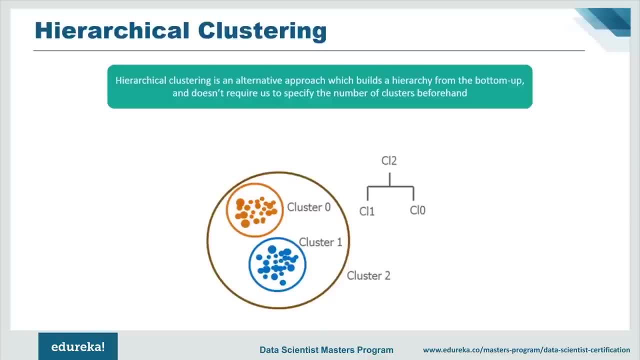 That's that. Now let's have a look at the third type of clustering, which is the hierarchical clustering. So hierarchical clustering is an alternative approach which builds a hierarchy from the bottom up or the top to bottom and does not require to specify the number of clusters beforehand. 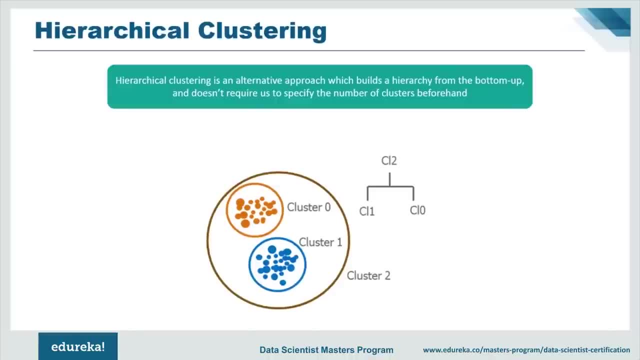 Now the algorithm works as in: first of all, we put each data point in its own cluster, identify the closest two clusters and combine them into one more cluster. Repeat the above step till the data points are in a single cluster. Now there are two types of hierarchical clustering. 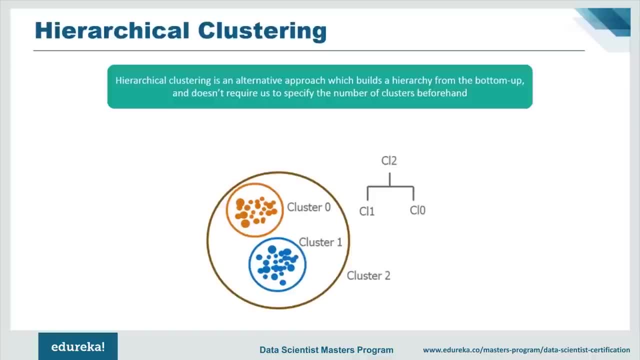 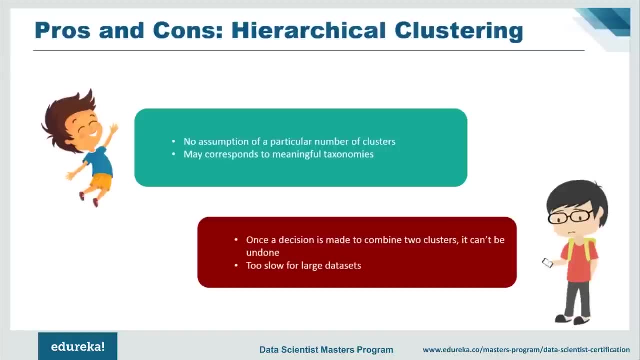 One is agglomerative clustering and the other one is division clustering. So agglomerative clustering builds the dendrogram from bottom level, while the division clustering it starts all the data points in one cluster, the root cluster. Now again, hierarchical clustering also has some sort of pros and cons. 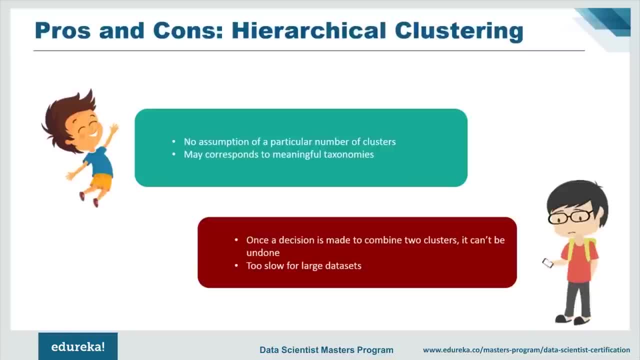 So, in the pros, though, no assumption of a particular number of clusters is required and it may correspond to meaningful taxonomies, Whereas if we talk about the cons, once a decision is made to combine two clusters, it cannot be undone, And one of the major disadvantages- 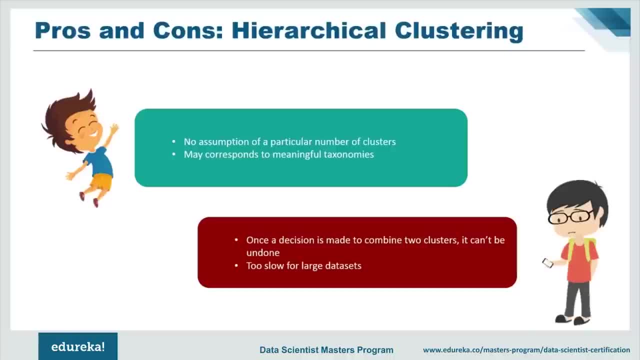 of these hierarchical clustering is that it becomes very slow if we talk about very, very large data sets, And nowadays, I think every industry are using large data sets and collecting large amounts of data. So hierarchical clustering is not the apt or the best method. 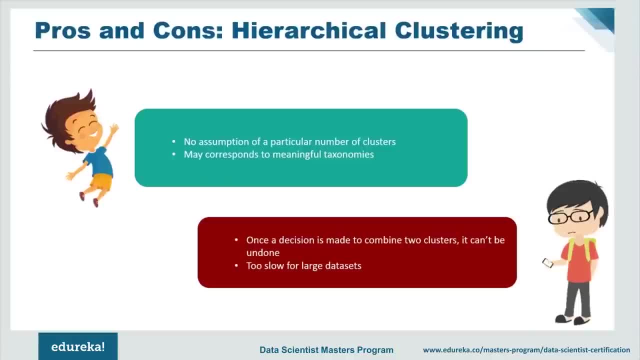 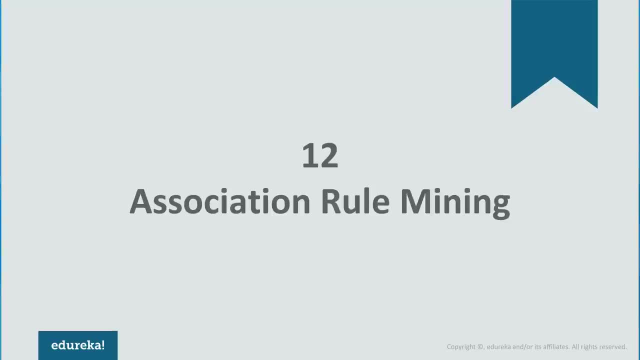 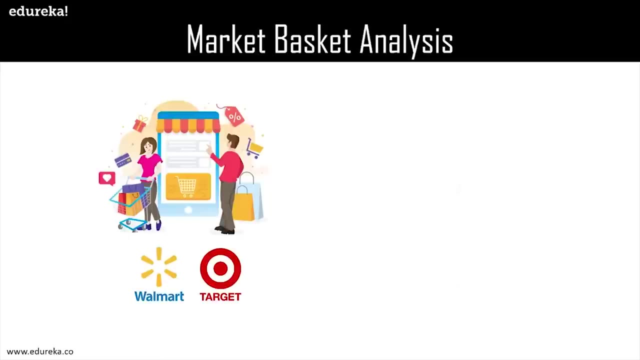 someone might need to go for. So there's that, Hello everyone, and welcome to this interesting session on a priori algorithm. Now, many of us have visited retail shops such as Walmart or Target for our household needs, Or let's say that we are planning to buy a new iPhone from Target. 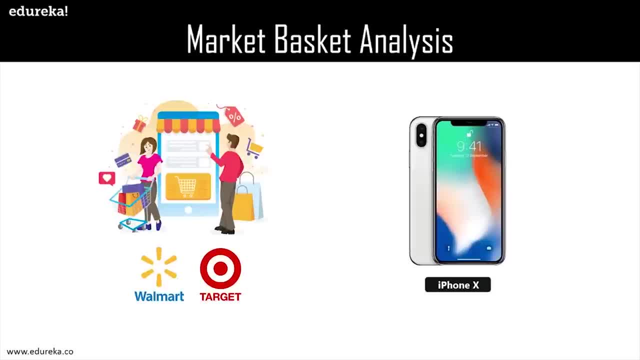 What we would typically do is search for the model by visiting the mobile section of the store and then select the product and head towards the billing counter. But in today's world, the goal of the organization is to increase the revenue. Can this be done by just pitching one product at a time to the customer? 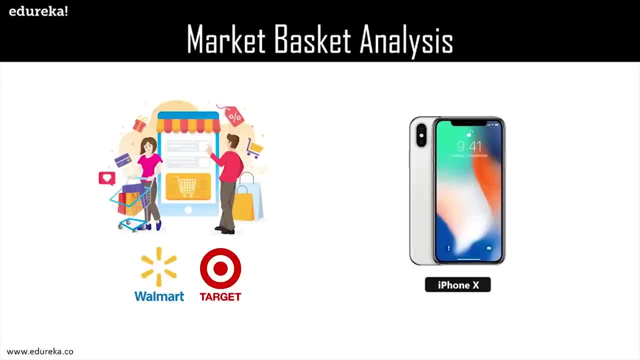 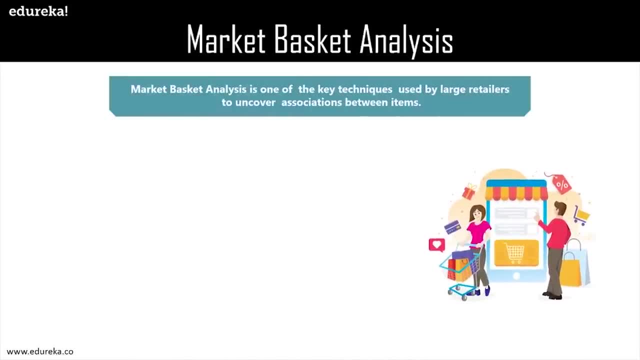 Now the answer to this is clearly no. Hence organization began mining data relating to frequently bought items, So market basket analysis is one of the key techniques used by large retailers to uncover associations between items. Now examples could be: the customers who purchase bread have a 60% likelihood to also purchase jam. 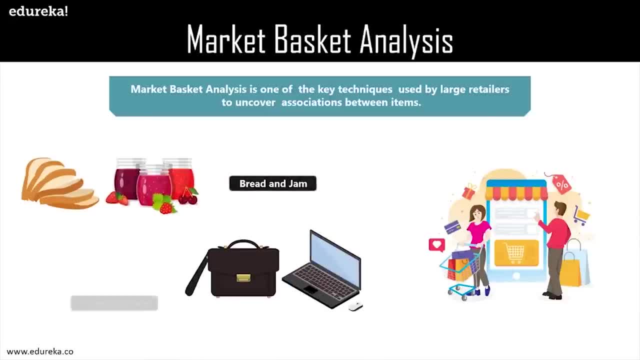 Customers who purchase laptops are more likely to purchase laptop bags as well. They try to find out associations between different items and products. They also try to find out which products can be sold together, which gives assisting in the right product placement. Typically, it figures out what products are being bought together. 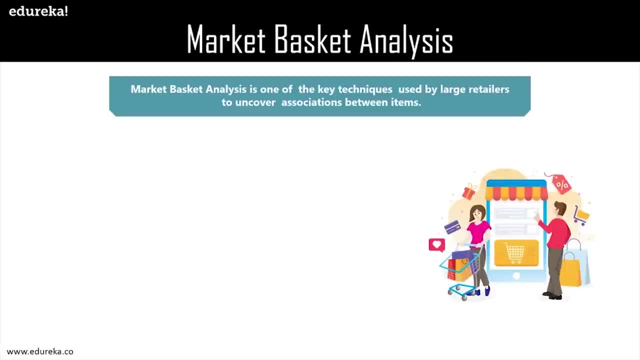 and organizations can place products in a similar manner. For example, people who buy bread also tend to buy butter right, And the marketing team at retail stores should target customers who buy bread and butter and provide an offer to them so that they buy a third item, suppose eggs. 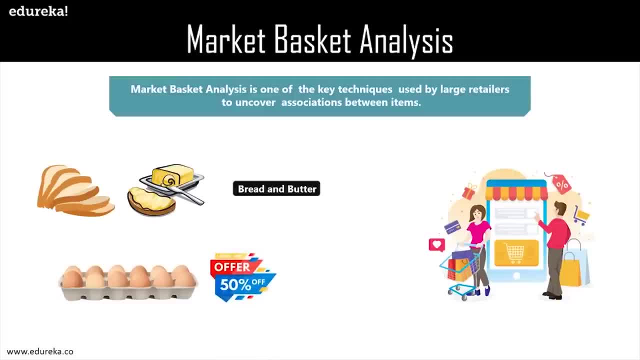 So if a customer buys bread and butter and sees a discount offer on eggs, he will be encouraged to spend more and buy the eggs, And this is what market basket analysis is all about. This is what we are going to talk about in this session. 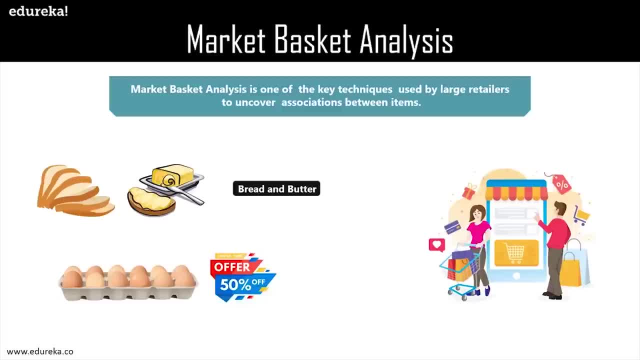 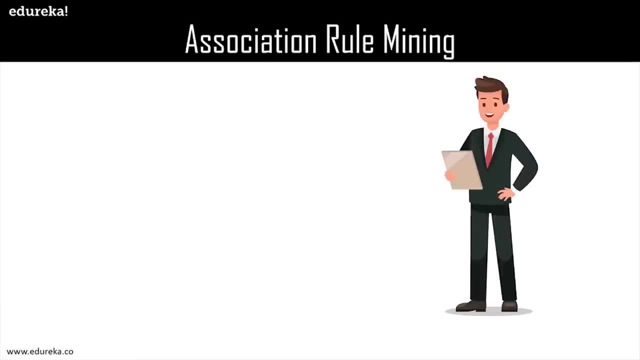 which is association rule, mining and the a priori algorithm. Now association rule can be thought of as an if-then relationship. Just to elaborate on that, we have come up with a rule. Suppose if an item A is being bought by the customer. 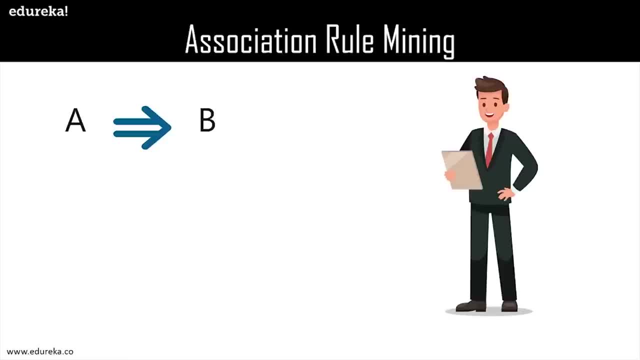 then the chances of item B being picked by the customer 2 under the same transaction ID is found out. You need to understand here that it's not a casualty, rather it's a co-occurrence pattern that comes to the force. Now there are two elements to this rule. 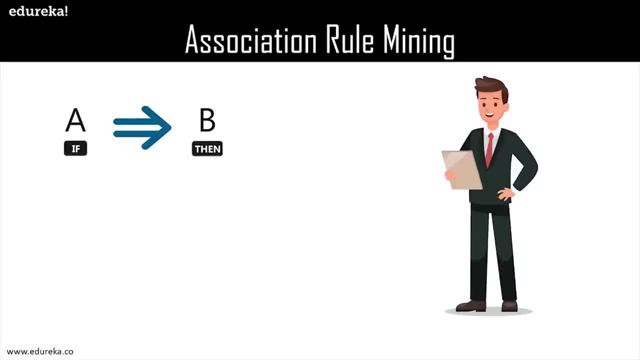 First is the if and second is the then. Now, if is also known as antecedent. This is an item or a group of items that are typically found in the item set, And the later one is called antecedent, The consequent. 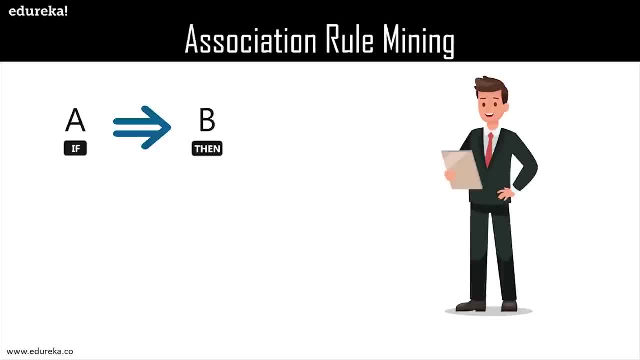 This comes along as an item with an antecedent group, or the group of antecedents are purchased. Now, if you look at the image here, A arrow B, it means that if a person buys an item A, then he will also buy an item B. 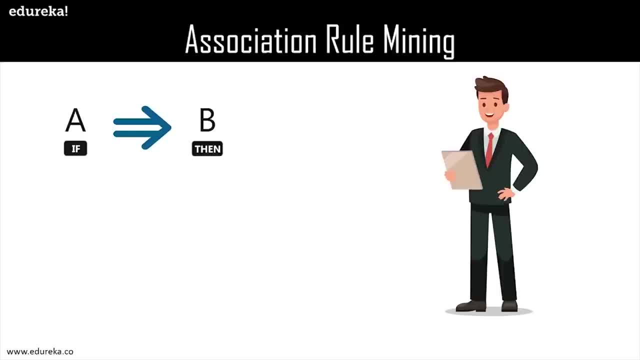 Or he will most probably buy an item B. Now, the simple example that I gave you about the bread and butter and the eggs is just a small example. But what if you have thousands and thousands of items? If you go to any professional data scientist, 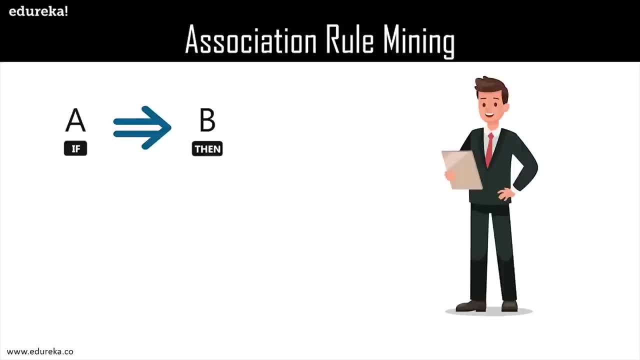 with that data. you can just imagine how much of profit you can make if the data scientist provides you with the right examples and the right placement of the items, which you can do, And you can get a lot of insights. That is why association rule mining is a very good algorithm. 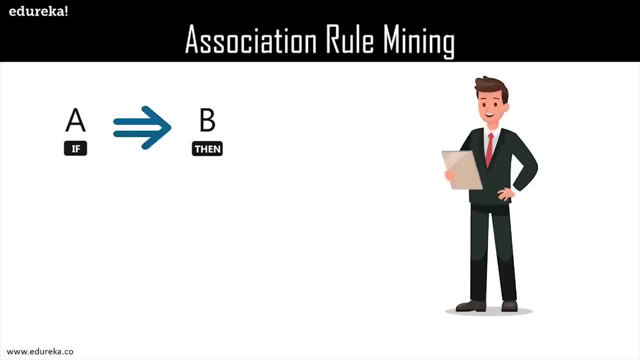 which helps the business make profit. So let's see how this algorithm works. So association rule mining is all about building the rules, And we have just seen one rule: that if you buy A, then there is a slight possibility or there is a chance. 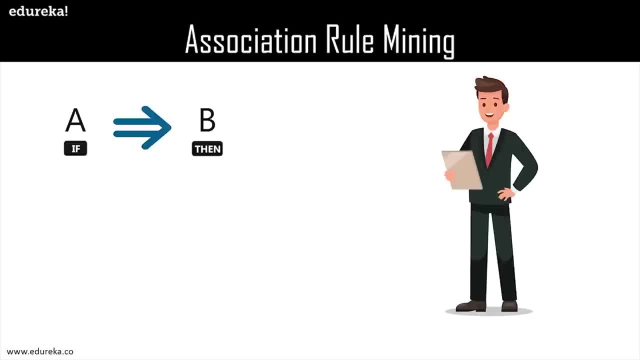 that you might buy B also. This type of relationship, in which we can find the relationship between these two items, is known as single cardinality. But what if the customer who bought A and B also wants to buy C? Or if a customer who bought A, B and C also wants to buy D? 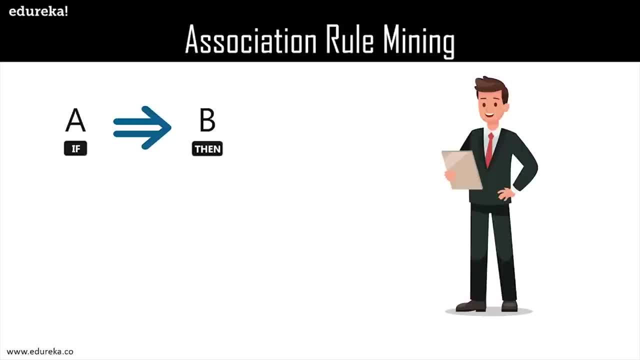 Then in these cases the cardinality usually increases and we can have a lot of competition for the combination around these data. And if you have around 10,000 or more than 10,000 data or items, just imagine how many rules you're going to create for each product. 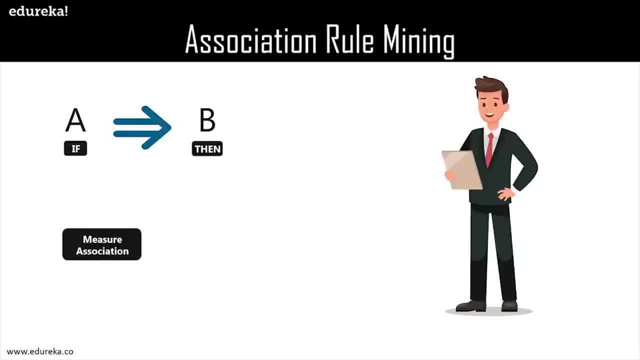 That is why association rule mining has such measures, so that we do not end up creating tens of thousands of rules. Now that is where the a priori algorithm comes in. But before we get into the a priori algorithm, let's understand what's the maths behind it. 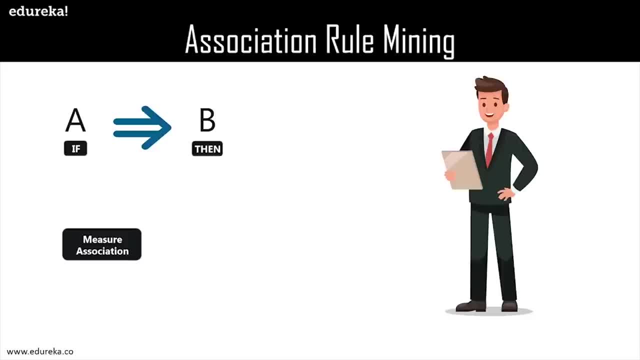 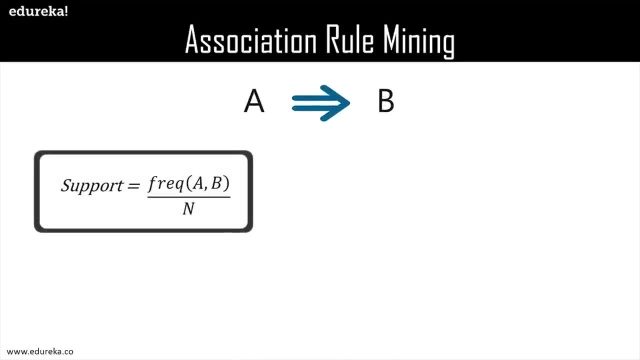 Now there are three types of matrices which help to measure the association We have: support, confidence and lift. So support is the frequency of item A or the combination of item A or B. It's basically the frequency of the items which we have bought. 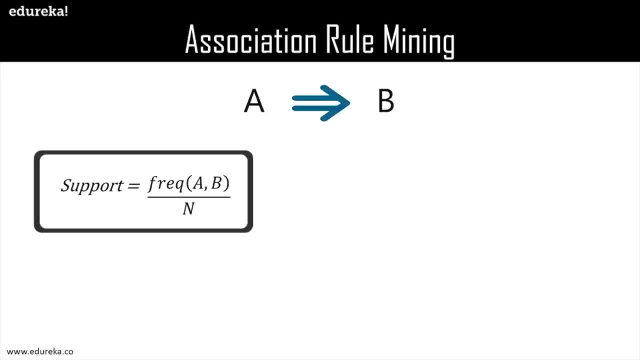 and what are the combination of the frequency of the item we have bought. So with this, what we can do is filter out the items which have been bought less frequently. This is one of the measures which is support. Now, what confidence tells us. So confidence gives us how often the items A and B occur together. 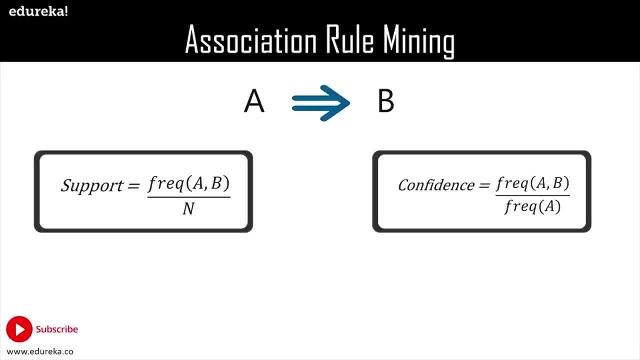 given the number of times A occur. Now this also helps us solve a lot of other problems, because if somebody is buying A and B together and not buying C, we can just rule out C at that point of time. So this solves. another problem is that we obviously do not need to analyze. 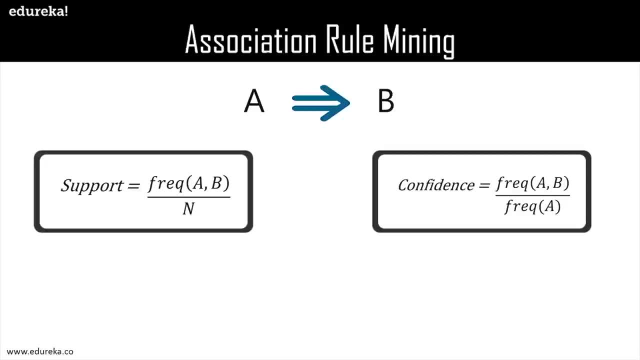 the products which people just buy barely. So what we can do is, according to the sales, we can define our measurement, We can define the minimum support and confidence And when you have set these values, we can put these values in the algorithm and we can filter out the data and we can create different rules. 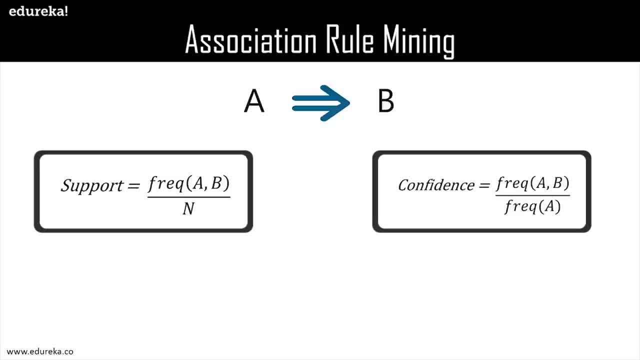 And suppose, even after filtering you have like 5000 rules and for every item we create these 5000 rules. So that's practically impossible. So for that we need the third calculation, which is the lift. So lift is basically the strength of any rule. 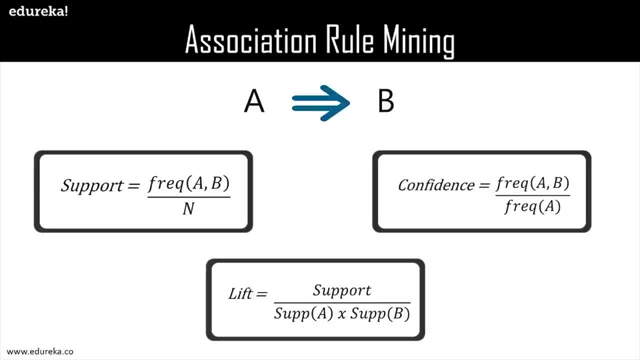 Now let's have a look at the denominator of the formula given here And, if you see, here we have the independent support values of A and B. So this gives us the independent occurrence probability of A and B And obviously there's a lot of difference between. 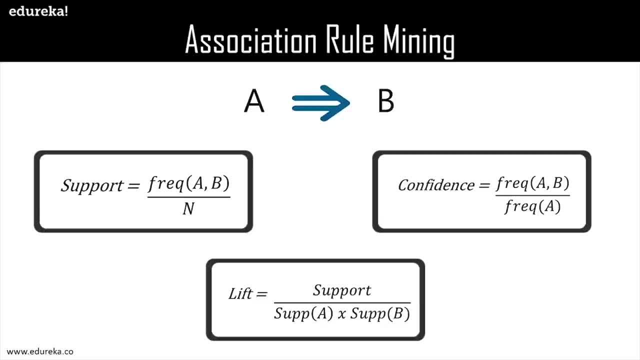 the random occurrence and association. And if the denominator of the lift is more, what it means is that the occurrence of randomness is more, rather than the occurrence because of any association. So lift is the final verdict where we know whether we have to spend time on this particular rule. 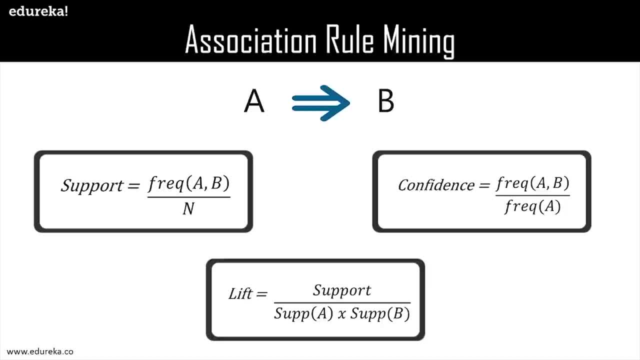 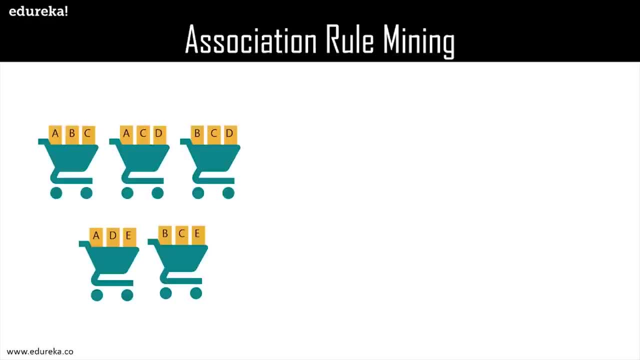 what we have got here or not. Now let's have a look at a simple example of association rule mining. So suppose we have a set of items A, B, C, D and E and a set of transactions- T1, T2, T3, T4 and T5. 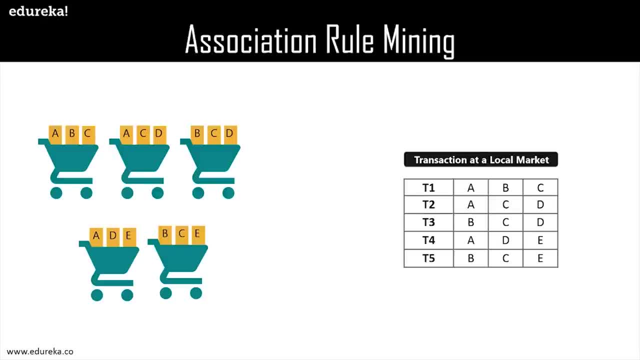 And, as you can see, here we have the transactions T1, in which we have A, B, C, T2, A C D, T3, B C, D, T4, A D, C, D. 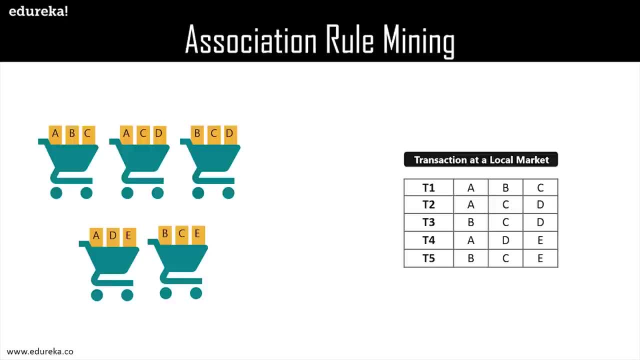 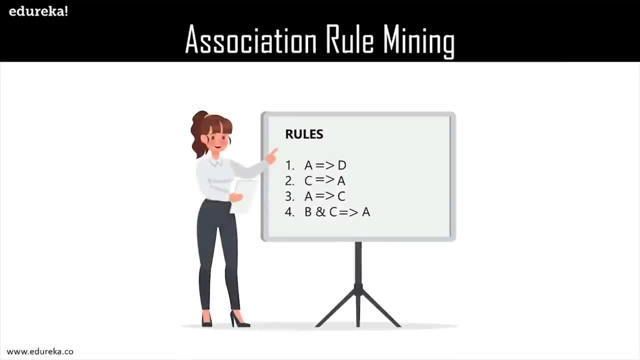 T4, A, D, E and T5, B, C, E. Now what we generally do is create some rules or association rules, such as: A gives T or C gives A, A gives C, B and C gives A. What this basically means is that if a person buys A, 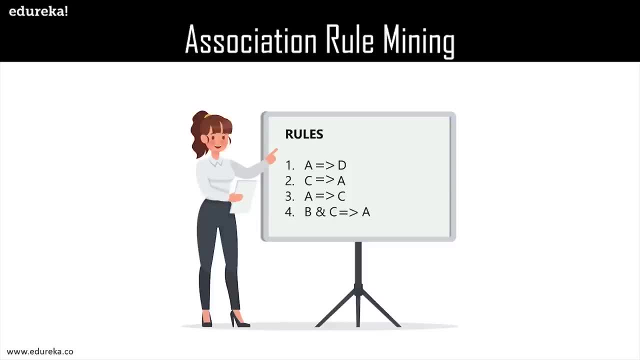 then he is most likely to buy D. And if a person buys C, then he is most likely to buy A. And if you have a look at the last one, if a person buys B and C, he is most likely to buy the item A as well. 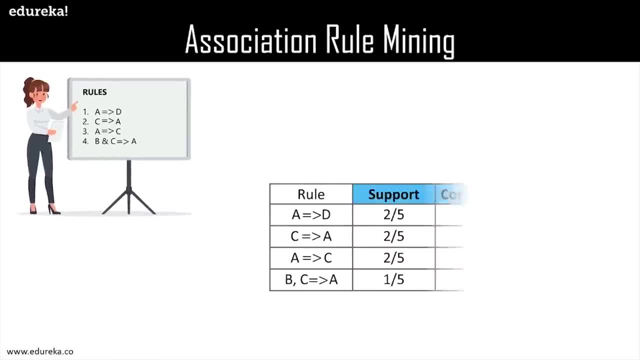 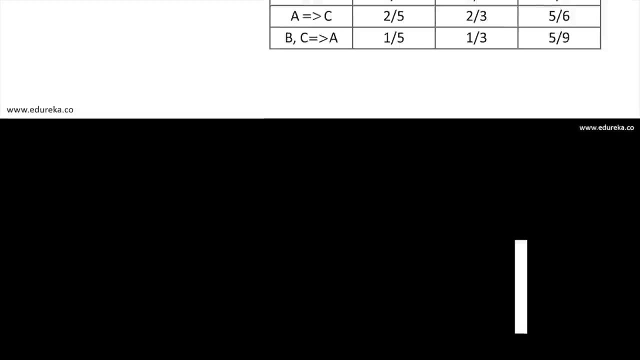 Now, if we calculate the support, confidence and lift using these rules, as you can see here in the table, we have the rule and the support, confidence and the lift values. Now let's discuss about a priori. So a priori algorithm uses the frequent item sets. 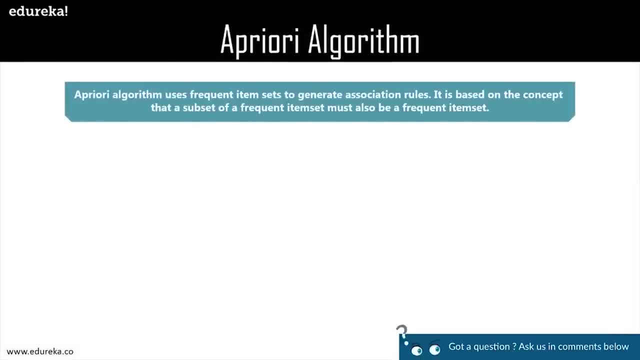 to generate the association rule, And it is based on the concept that a subset of a frequent item set must also be a frequent item set itself. Now this raises the question: what exactly is a frequent item set? So a frequent item set is an item set whose support value 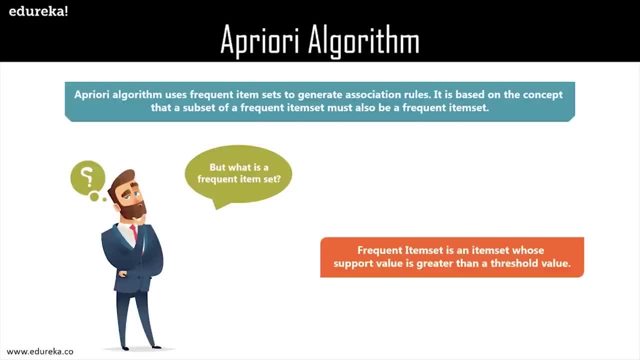 is greater than the threshold value. Just now we discussed that the marketing team, according to the sales, have a minimum threshold value for the confidence as well as the support. So frequent item set is that item set whose support value is greater than the threshold value already specified. 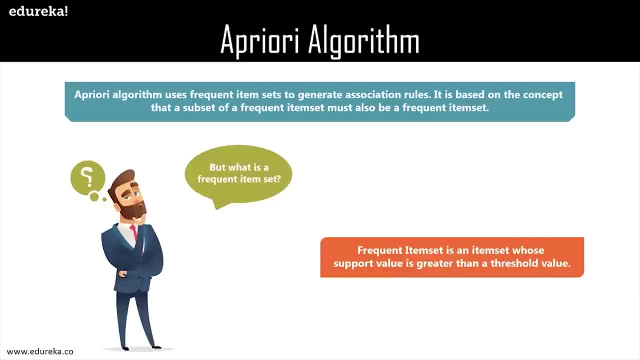 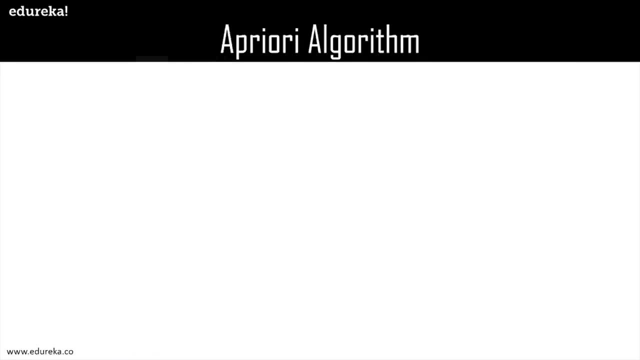 For example, if A and B is a frequent item set, then A and B should also be frequent item sets individually. Now let's consider the following. Let's consider the following transaction. to make the things a little easier, Suppose we have transactions 1,, 2,, 3,, 4, 5 and these items are there. 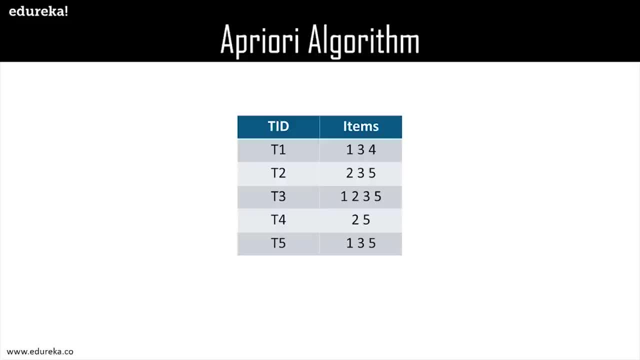 So T1 has 1,, 3 and 4.. T2 has 2,, 3 and 5.. T3 has 1,, 2,, 3, 5. T4, 2, 5 and T5, 1,, 3 and 5.. 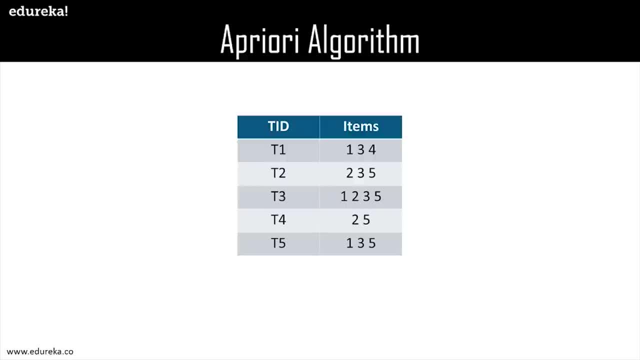 Now the first step is to build a list of item sets of size 1 by using this transactional data, And one thing to note here is that the minimum support count which is given here is 2.. So let's suppose it's 2.. 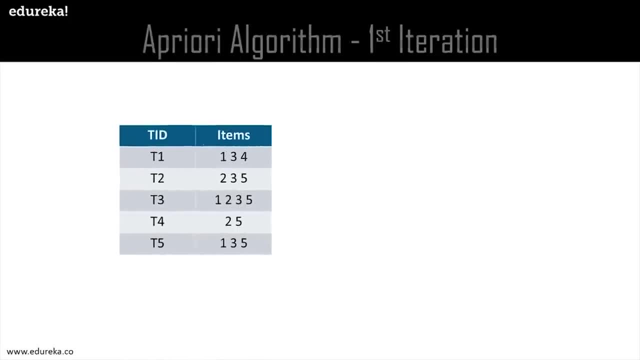 So the first step is to create item sets of size 1 and calculate their support values. So, as you can see, here we have the table C1 in which we have the item sets 1,, 2,, 3,, 4, 5. 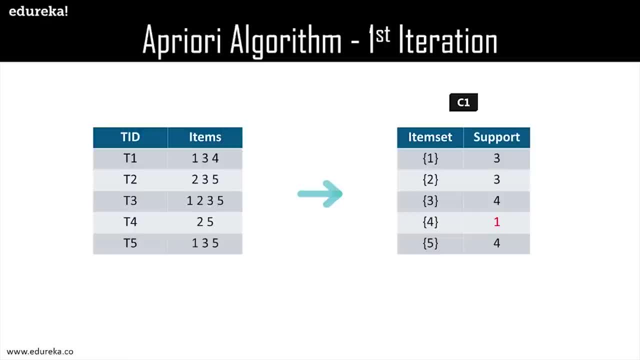 and the support values. If you remember the formula of support, it was frequency divided by the total number of occurrence. So, as you can see here, for the item set 1, the support is 3.. As you can see here, the item set 1 appears in T1, T3 and T5. 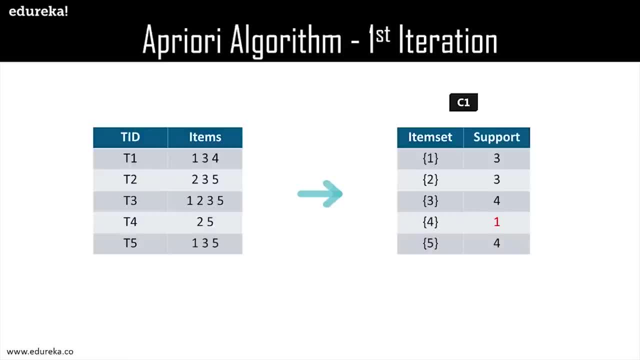 So, as you can see, the frequency is 1,, 2 and 3.. Now, as you can see here, the item set 4 has a support of 1, as it occurs only once in transaction 1.. But the minimum support value is 2,. 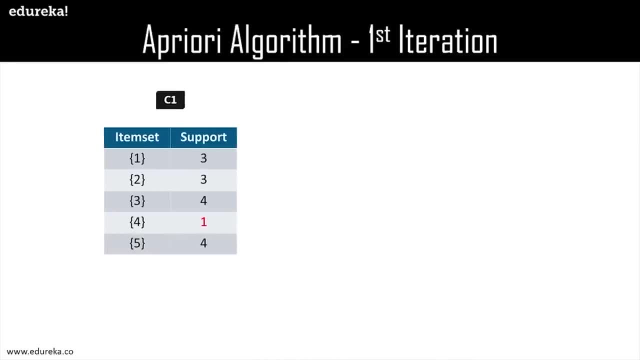 that's why it's gonna be eliminated. So we have the final table, which is the table F1, in which we have the item sets 1, 2, 3 and 5 and we have the support values 3, 3,, 4 and 4.. 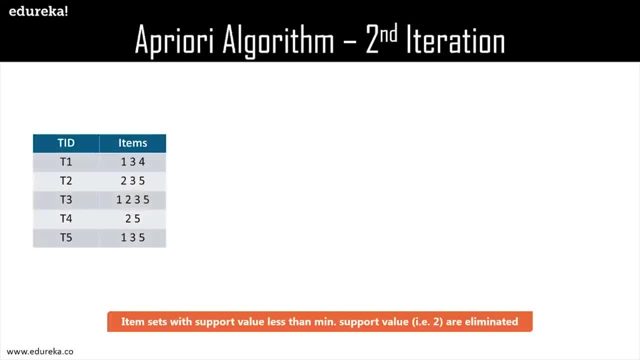 Now the next step is to create item sets of size 2 and calculate their support values. Now all the combination of the item sets in the F1, which is the final table in which we discarded the 4, are going to be used for this iteration. 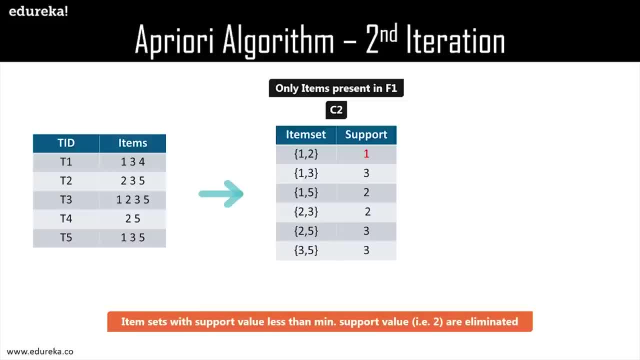 So we get the table C2.. So, as you can see, here we have 1, 2,, 1, 3, 1, 5, 2, 3,, 2, 5 and 3, 5.. 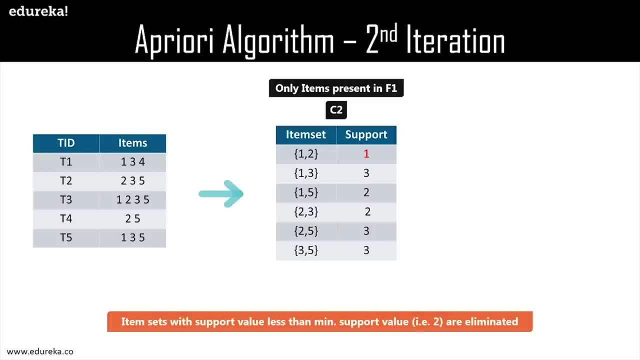 Now if you calculate the support here again, we can see that the item set 1, 2 has a support of 1, which is again less than the specified threshold. So we're gonna discard that. So if we have a look at the table F2,. 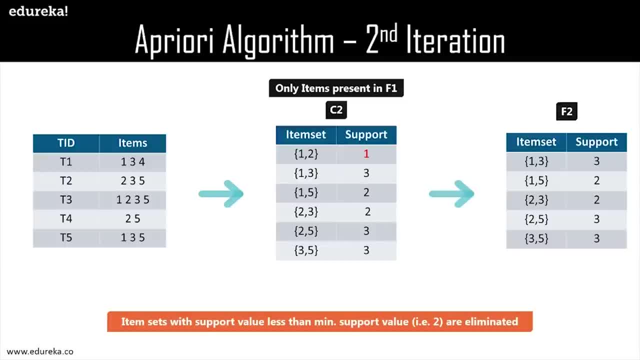 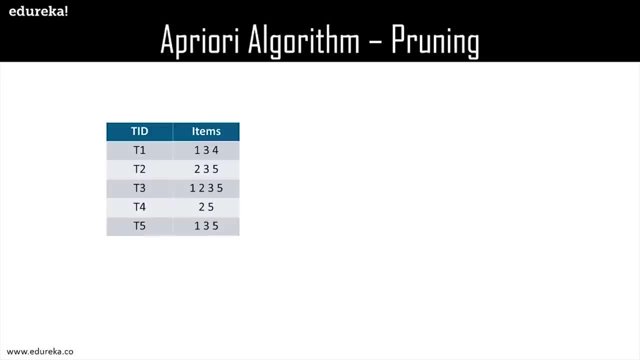 we have 1, 3, 1, 5, 2, 3, 2, 5 and 3, 5.. Again, we're gonna move forward and create the item set of size 3 and calculate their support values. 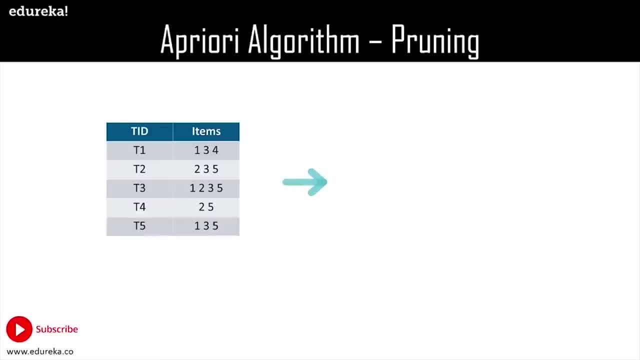 Now all the combinations are gonna be used from the item set F2 for this particular iterations. Now, before calculating support values, let's perform pruning on the data set. Now, what is pruning? Now, after the combinations are being made, we divide C3 item sets to check if there is another subset. 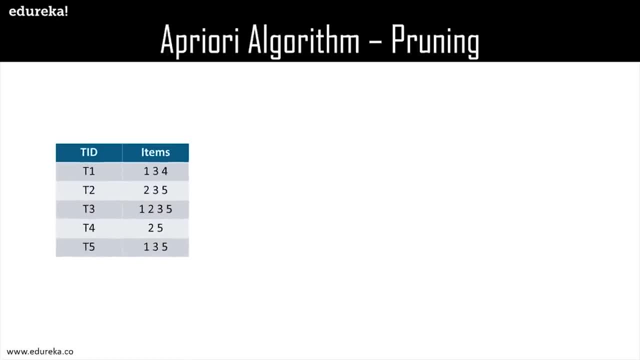 whose support is less than the minimum support value. That is what frequent item set means. So if we have a look here, the item sets we have is 1, 2, 3, 1, 2, 1, 3, 2, 3. 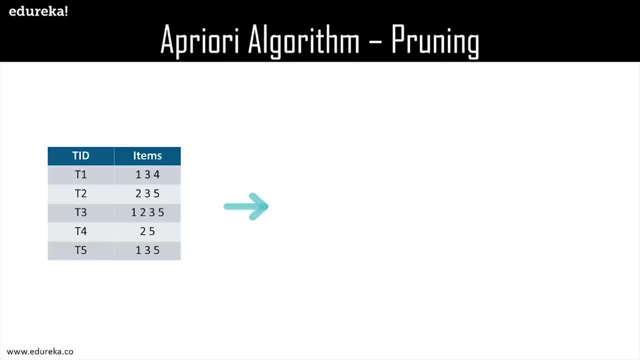 for the first one, Because, as you can see here, if we have a look at the subsets of 1, 2, 3, we have 1, 2 as well. So we are going to discard this whole item set. 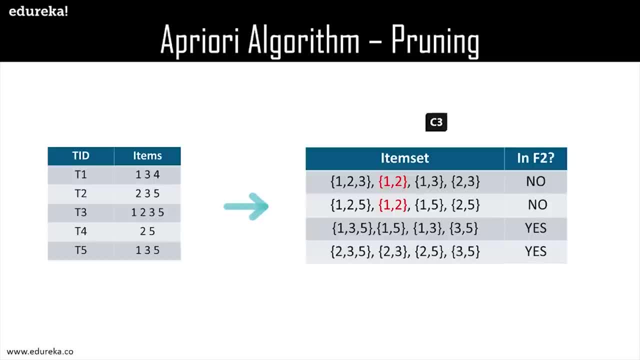 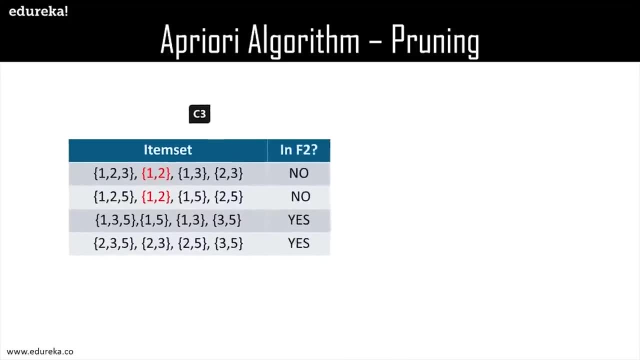 Same goes for the second one. We have 1,, 2, 5.. We have 1, 2 in that, which was discarded in the previous set or the previous step. That's why we're gonna discard that also, Which leaves us with only two factors. 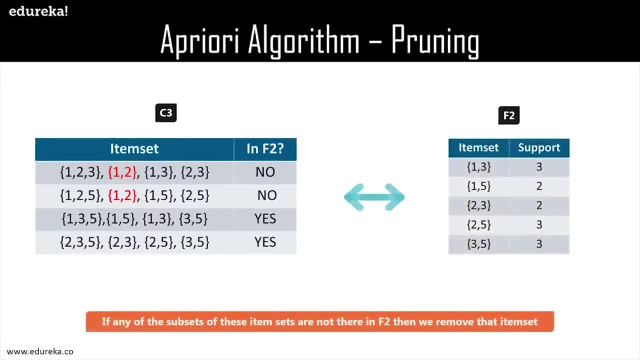 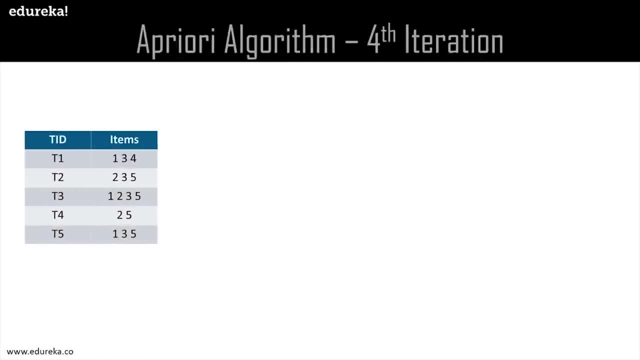 which is 1,, 3, 5 item set and the 2,, 3, 5.. And the support for this is 2 and 2 as well. Now, if we create the table C4 using four elements, we're gonna have only one item set. 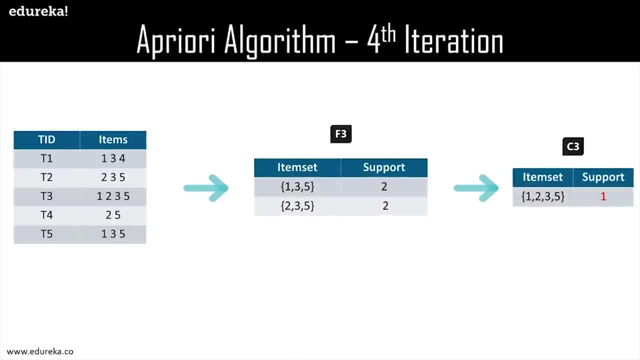 which is 1,, 2,, 3, and 5.. And if we have a look at the table here- the transaction table 1,, 2,, 3, and 5- appears only 1.. So the support is 1.. 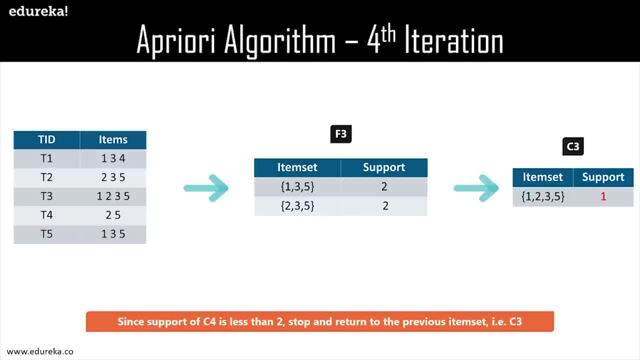 And since C4, the support of the whole table C4 is less than 2, so we're gonna stop here and return to the previous item set, that is, C3.. So the frequent item sets are 1, 3, 5 and 2, 3, 5.. 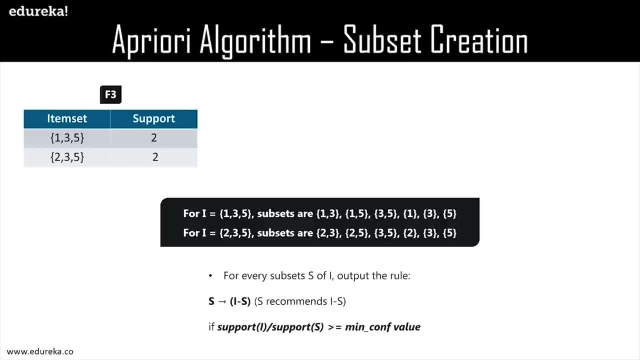 Now, let's assume our minimum confidence value is 60%. For that we're gonna generate all the non-empty subsets for each frequent item set. Now for i equals 1,, 2,, 3,, 5,, which is the item set. 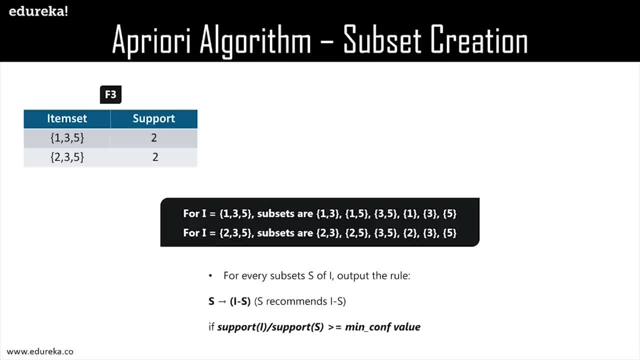 we get the subset 1, 3,, 1,, 5,, 3,, 5,, 1,, 3, and 5.. Similarly for 2,, 3,, 5, we get 2,, 3,, 2,, 5,, 3,, 5,, 2,, 3, and 5.. 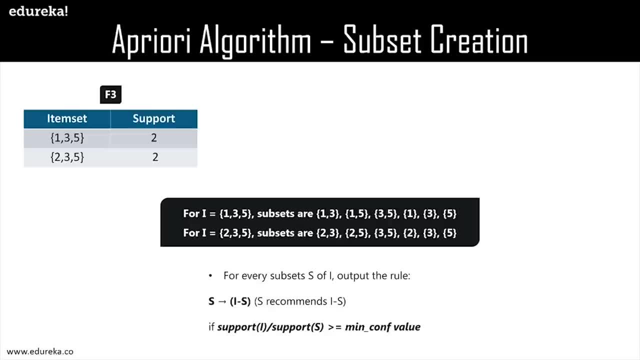 Now this rule states that for every subset S of i, the output of the rule gives something like S gives i to S. That implies S recommends i of S, And this is only possible if the support of i divided by the support of S is greater than equal to the minimum confidence value. 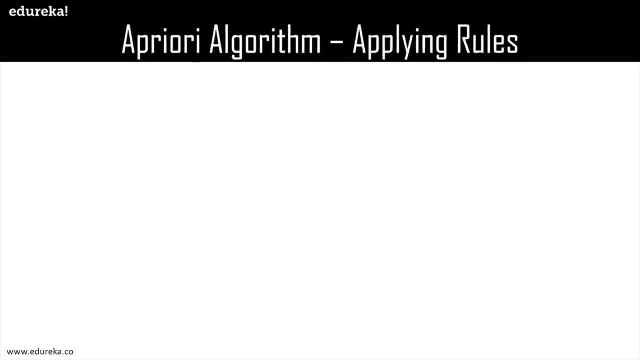 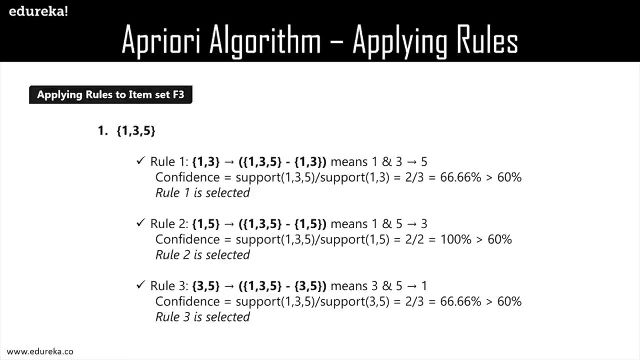 Now applying these rules to the item set of F3, we get rule 1, which is: 1, 3 gives 1, 3, 5 and 1, 3.. It means 1 and 3 gives 5.. 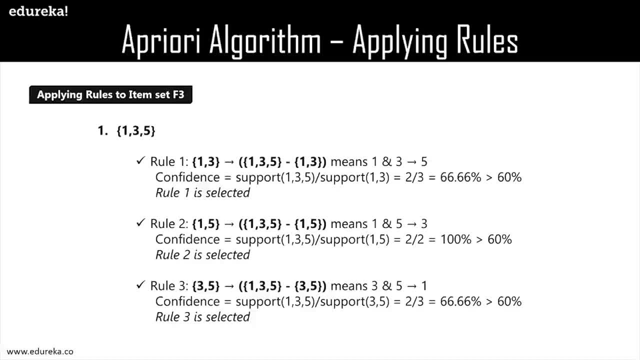 So the confidence is equal to the support of 1, 3, 5 divided by the support of 1, 3.. That equals 2 by 3, which is 66% and which is greater than the 60%. So the rule 1 is selected. 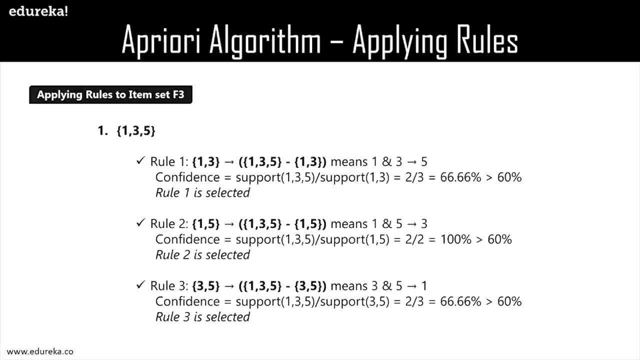 Now, if we come to rule 2, which is 1, 5, it gives 1, 3, 5 and 1, 5.. It means, if we have 1 and 5, it implies we also gonna have 3.. 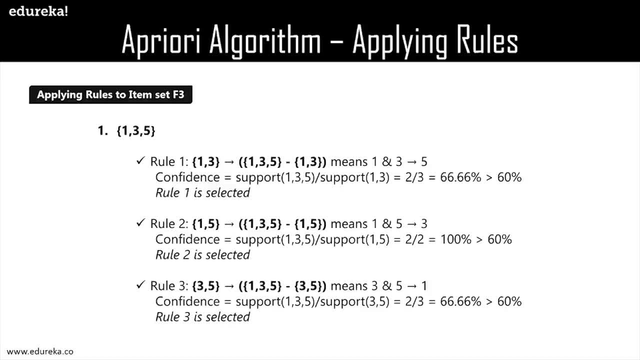 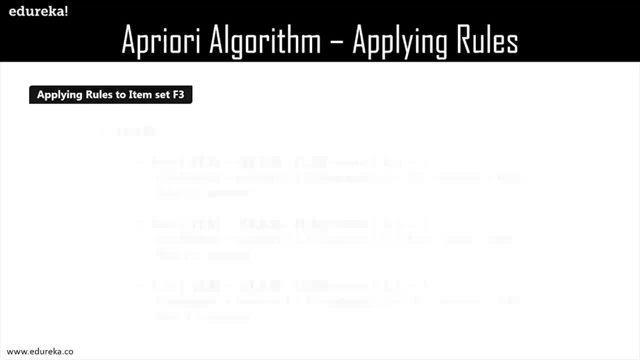 Now, if we calculate the confidence of this one, we're gonna have support 1, 3, 5 divided by support 1, 5, which gives us 100%, which means rule 2 is selected as well. But again, if we have a look at rule 5 and rule 6 over here, 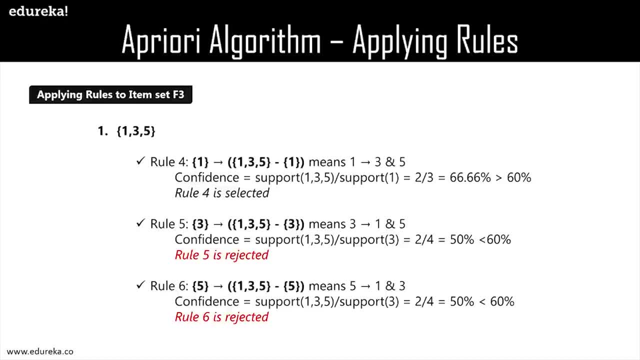 similarly, if we select 3 gives 1,, 3,, 5 and 3, it means if we have 3,, we also get 1 and 5.. So the confidence for this comes at 50%, which is less than the given 60% target. 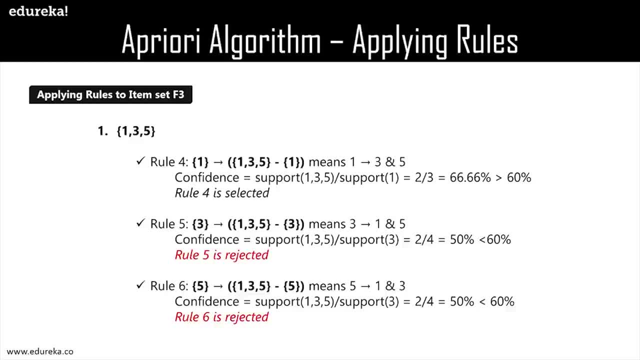 So we're gonna reject this rule, And same goes for the rule number 6.. Now, one thing to keep in mind here is that although the rule 1 and rule 5 look a lot similar, they are not. So it really depends what's on the left-hand side of the arrow. 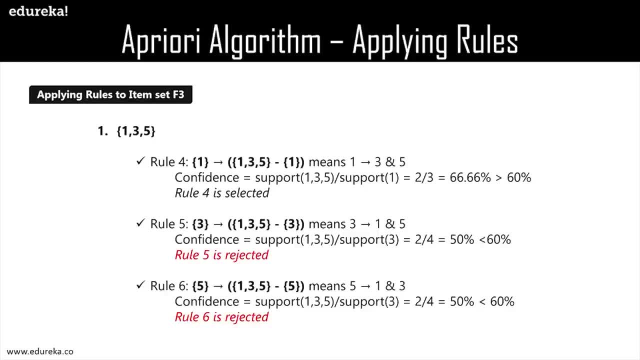 and what's on the right-hand side of the arrow? It's the if-then possibility. I'm sure you guys can understand what exactly these rules are and how to proceed with these rules. So let's see how we can implement the same in Python, right? 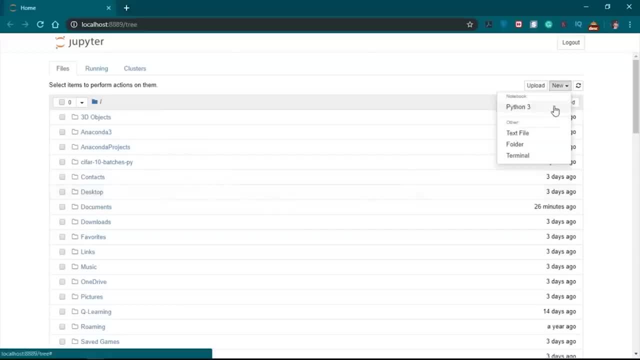 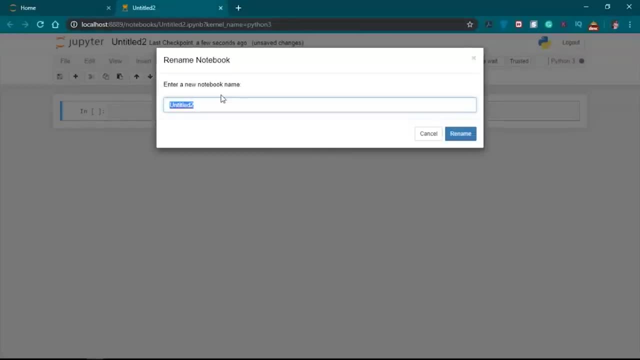 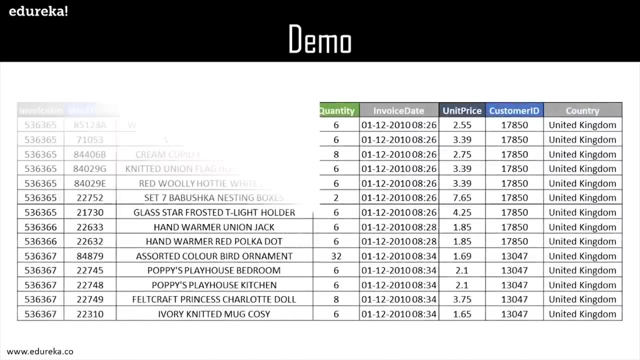 So for that, what I'm gonna do is create a new Python file, and I'm going to use the Jupyter Notebook. You're free to use any sort of IDE. I'm gonna name it as Apriori. So the first thing what we're gonna do is 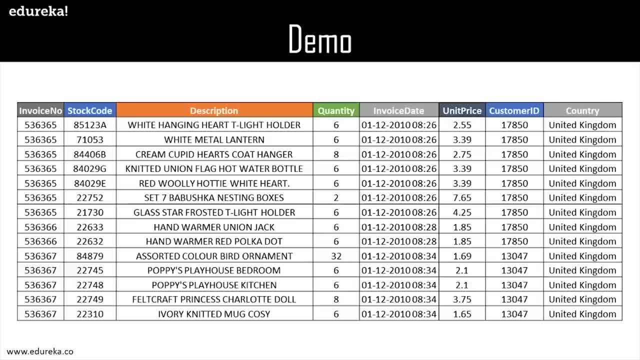 we'll be using the online transactional data of a retail store for generating association rules. So, firstly, what we need to do is get the Pandas and MLX10 libraries imported and read the file. So, as you can see, here we are using the 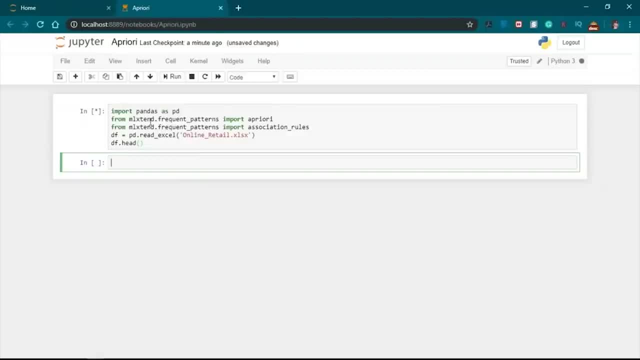 online-retailxlsx format file And from MLX10, we're gonna import Apriori and association rules. It all comes under MLX10.. So, as you can see, here we have the invoice, the stock code, the description, the quantity. 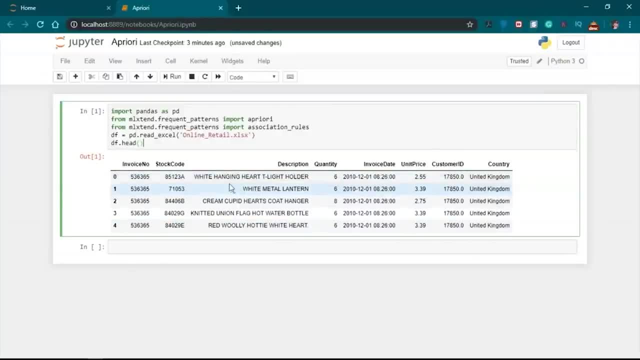 the invoice data, unit price, customer ID and the country. Now, next in this step, what we're going to do is do data cleanup, which includes removing the spaces from some of the descriptions, and drop the rules that do not have invoice numbers. 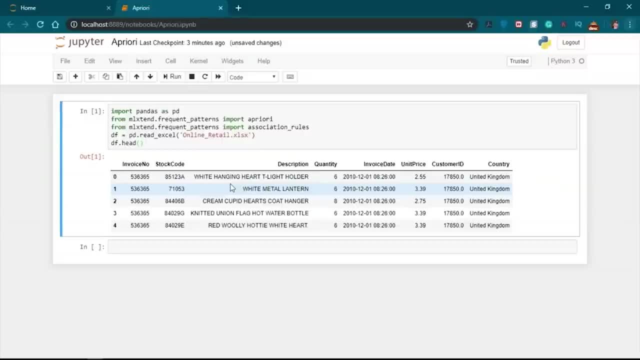 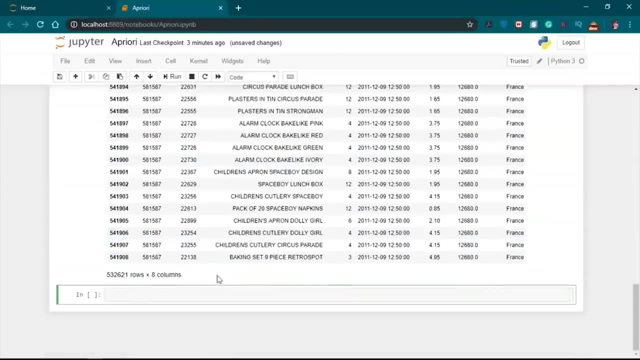 and remove the credit card transactions, because that is of no use to us. So, as you can see here the output in which we have like 532,000 rows with eight columns. So after the cleanup we need to consolidate the items into one transaction per row with each product. 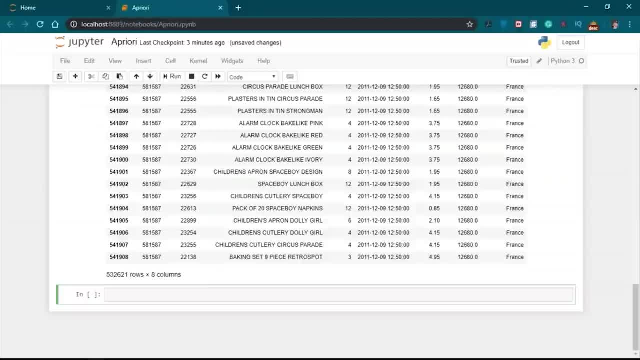 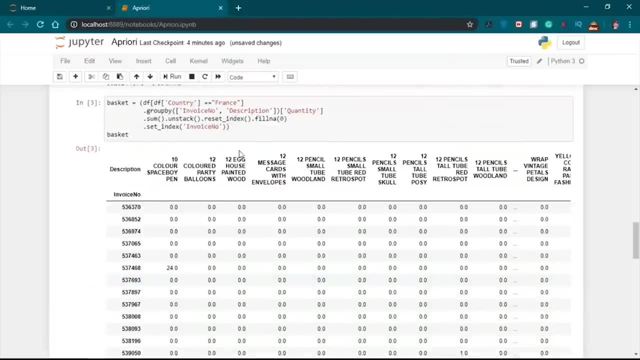 For the sake of keeping the data set small, we are only looking at the sales for France. So, as you can see here we have excluded all the other sales. We are just looking at the sales for France. Now there are a lot of zeros in the data. 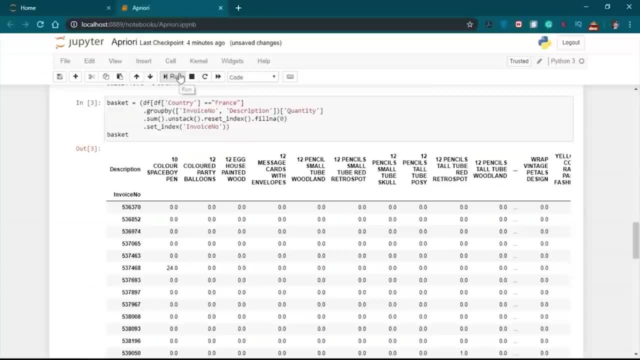 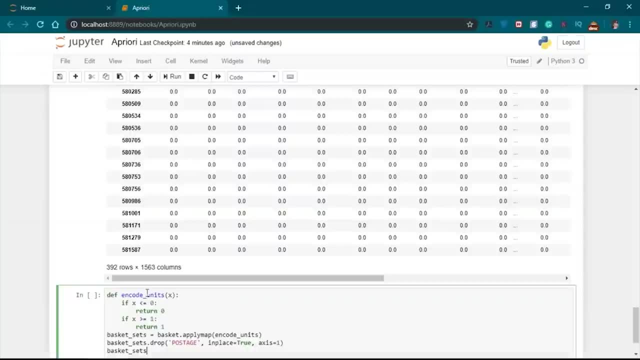 but we also need to make sure any positive values are converted to one and anything less than zero is set to zero. So, as you can see, here we are still 392 rows. We're going to encode it and see Check again, Now that you have structured the data properly. 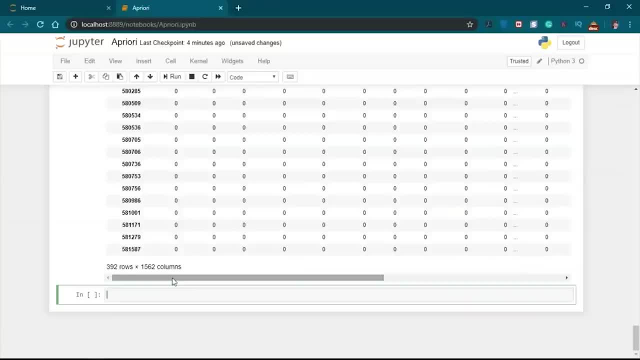 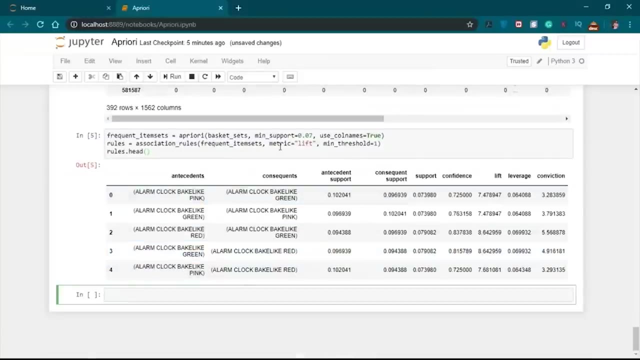 in this step, what we're going to do is generate frequent item sets that have support at least 7%. Now, this number is chosen so that you can get close enough and generate the rules with the corresponding support, confidence and lift. So again, as you can see here, the minimum support is 0.7.. 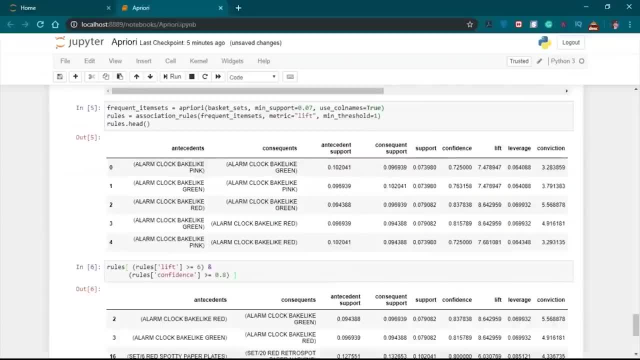 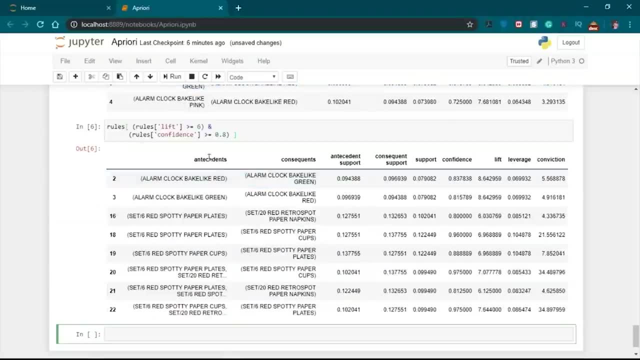 Now what if we add another constraint on the rules, such as the lift is greater than 6 and the confidence is greater than 0.8?? So, as you can see, here we have the left-hand side and the right-hand side of the association rule. 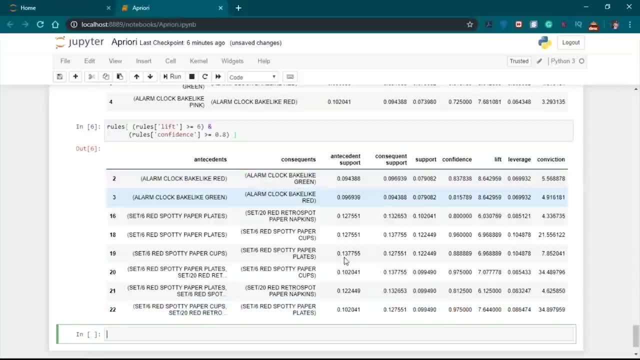 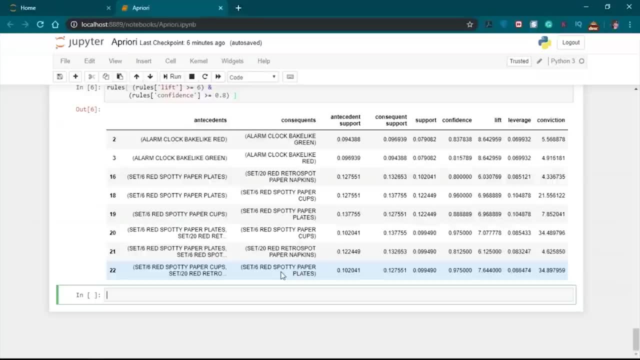 which is the antecedent and the consequence. We have the support, We have the confidence, the lift, the leverage and the conviction. So, guys, that's it for this session. That is how you create association rules using the Apriori algorithm. 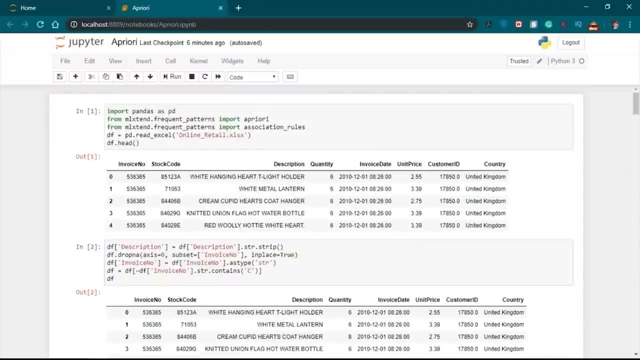 which helps a lot in the marketing business. It runs on the principle of market basket analysis, which is exactly what big companies like Walmart- you have Reliance and Target- do. Even Ikea does it, And I hope you got to know what exactly is association rule mining. 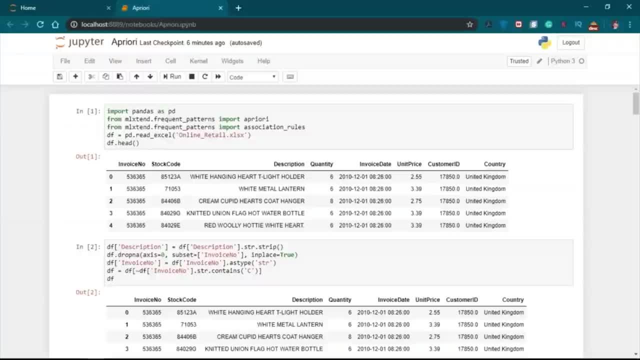 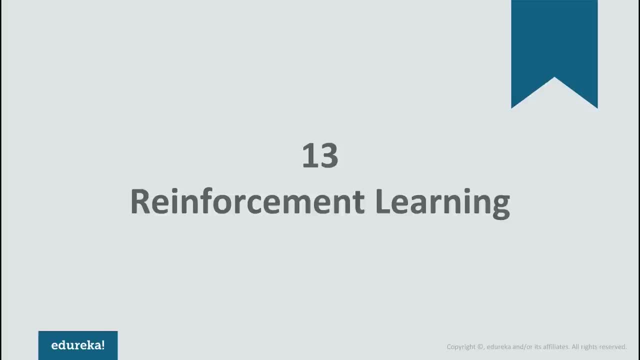 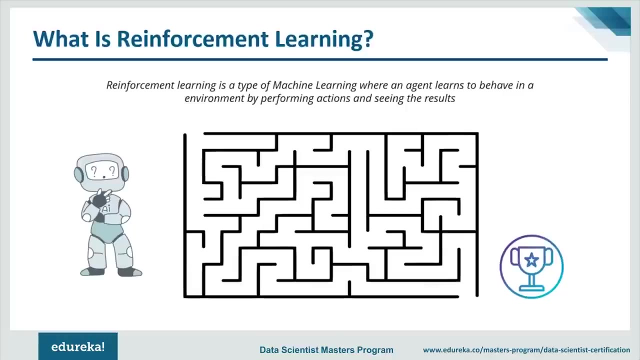 what is lift confidence and support And how to create association rules. So, guys, reinforcement learning is a part of machine learning, where an agent is put in an environment and he learns to behave in this environment by performing certain actions. Okay, so it basically performs actions. 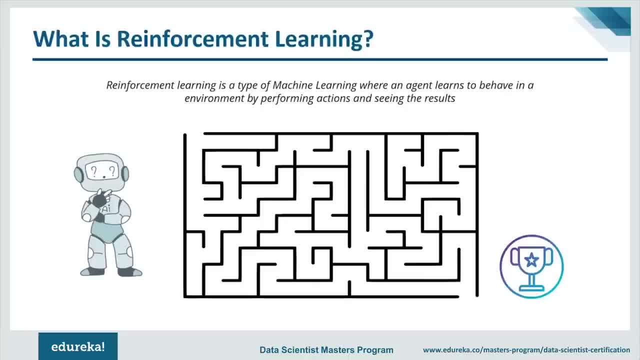 and it either gets the rewards on the actions or it gets a punishment and observing the reward which it gets from those actions. Reinforcement learning is all about taking an action in appropriate action in order to maximize the reward in a particular situation. So, guys, in supervised learning, 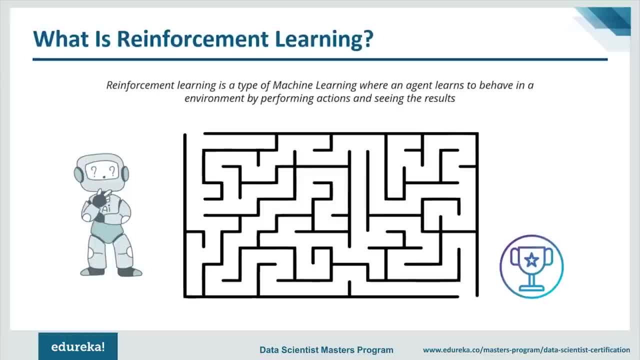 the training data comprises of the input and the expected output, And so the model is trained with the expected output itself. But when it comes to reinforcement learning, there is no expected output. Here the reinforcement agent decides what actions to take in order to perform a given task. 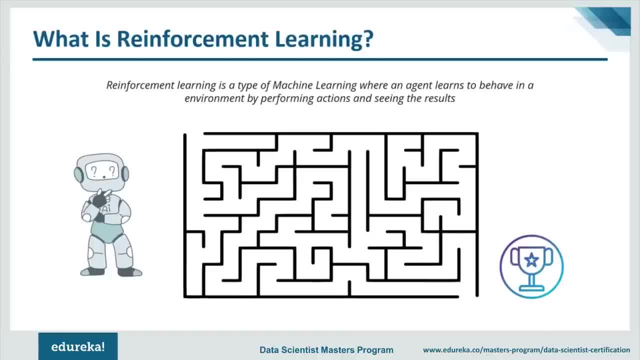 In the absence of a training data set, it is bound to learn from its experience itself. All right, so reinforcement learning is all about an agent who's put in an unknown environment and he's going to use a hit and trial method in order to figure out the environment. 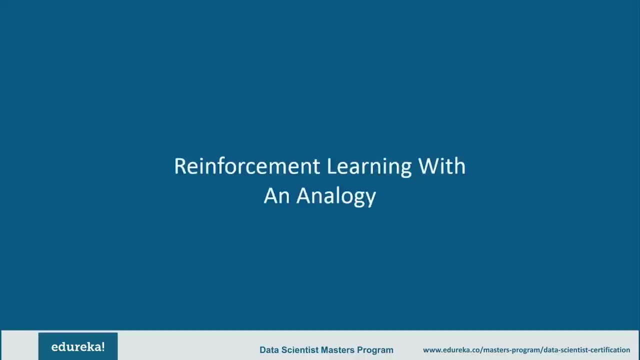 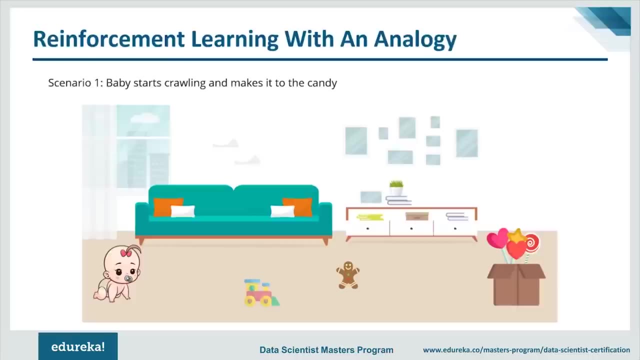 and then come up with an outcome. Okay, now let's look at reinforcement learning with an analogy. So consider a scenario wherein a baby is learning how to walk. This scenario can go about in two ways, Now. in the first case, the baby starts walking. 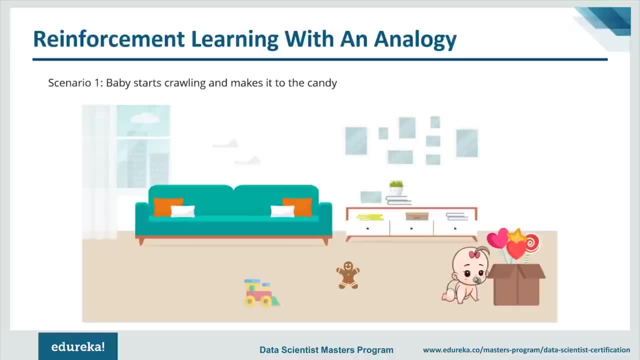 and makes it to the candy. Here, the candy is basically the reward it's going to get. So, since the candy is the end goal, the baby is happy, it's positive. Okay, so the baby is happy and it gets rewarded a set of candies. 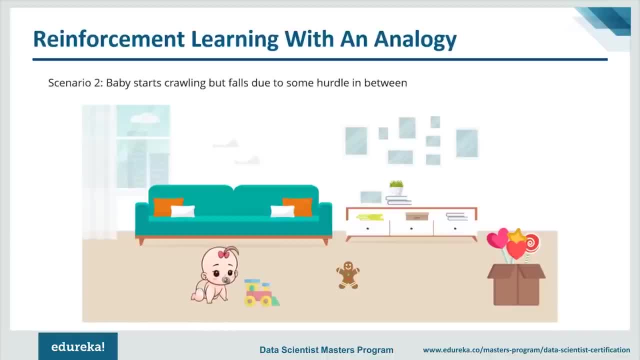 Now another way in which this could go is that the baby starts walking but falls due to some hurdle in between. The baby gets hurt and it doesn't get any candy and obviously the baby is sad. So this is a negative reward, Okay, or you can say this is a setback. 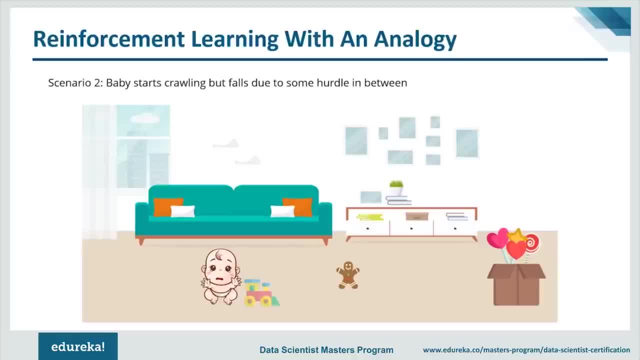 So, just like how we humans learn from our mistakes by trial and error, reinforcement learning is also similar. Okay, so we have an agent which is basically the baby and a reward which is the candy over here, Okay, and with many hurdles in between. 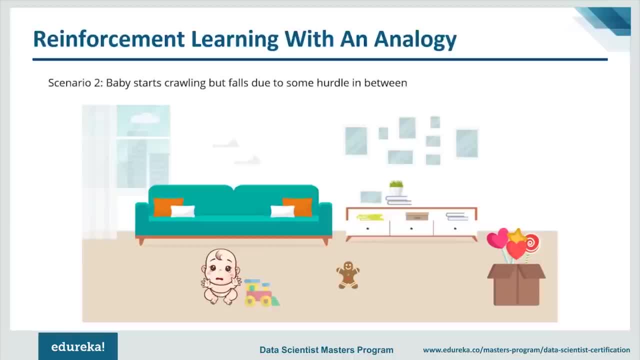 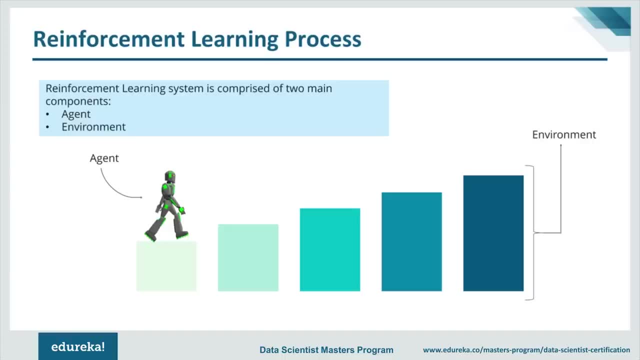 the agent is supposed to find the best possible path to reach the reward. So, guys, I hope you all are clear with the reinforcement learning. Now let's look at the reinforcement learning process. So, generally, a reinforcement learning system has two main components. Alright, the first is an agent. 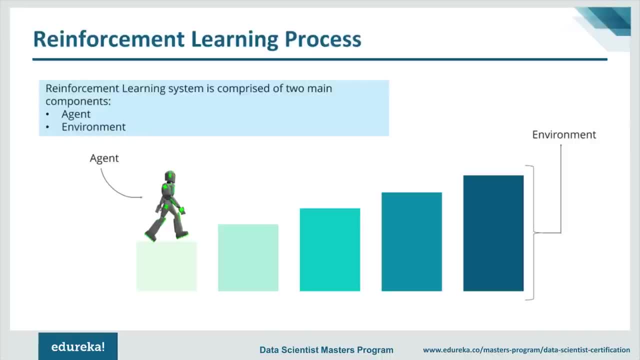 and the second one is an environment. Now, in the previous case, we saw that the agent was a baby and the environment was a living room wherein the baby was crawling. Okay, the environment is the setting that the agent is acting on and the agent over here represents. 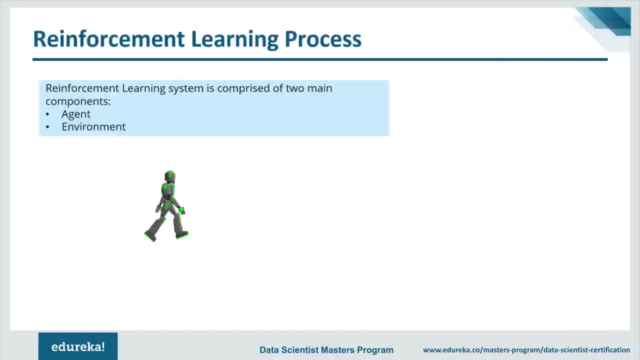 the reinforcement learning algorithm. So, guys, the reinforcement learning process starts when the environment sends a state to the agent, and then the agent will take some actions based on the observations. In turn, the environment will send the next state and the respective reward back to the agent. 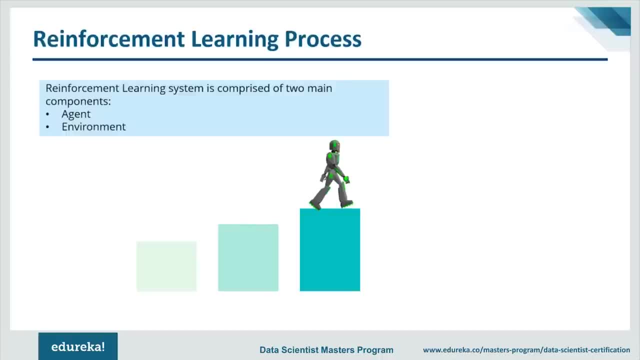 The agent will update its knowledge with a reward returned by the environment, and it uses that to evaluate its previous action. So, guys, this loop keeps continuing until the environment sends a terminal state, which means that the agent has accomplished all his tasks and he finally gets the reward. 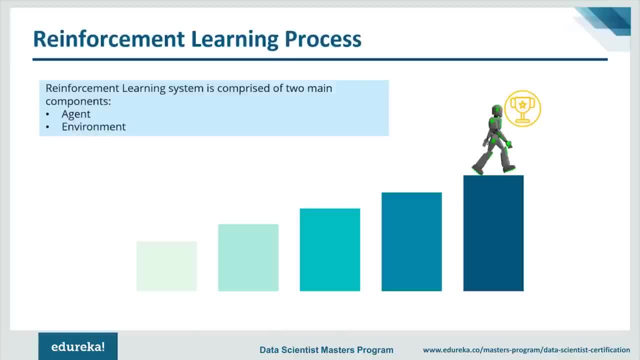 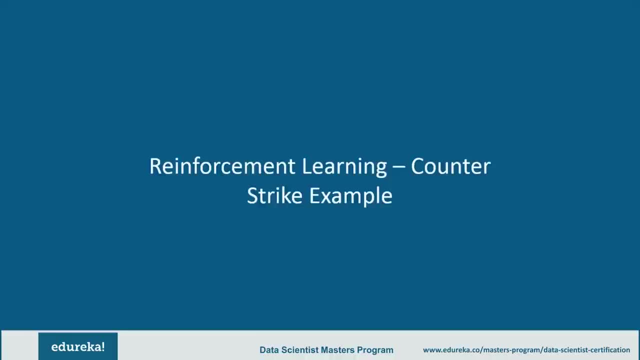 Okay, this is exactly what was depicted in this scenario, So the agent keeps climbing up ladders until he reaches his reward. To understand this better, let's suppose that our agent is learning to play Counter Strike. Okay, so let's break it down. 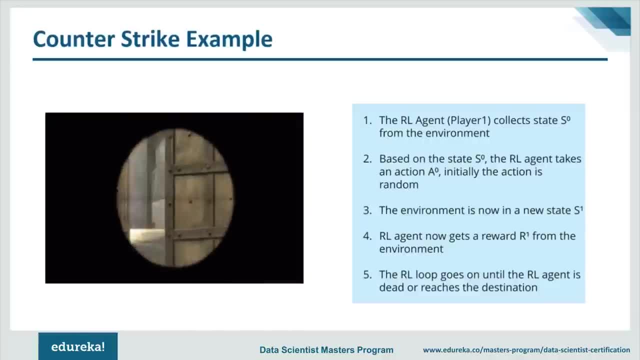 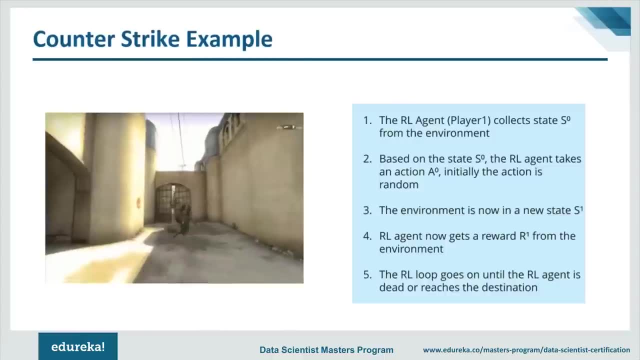 Now, initially, the RL agent, which is basically the player, player one, let's say, it's the player one who is trying to learn how to play the game. He collects some state from the environment. Okay, this could be the first state of Counter Strike. 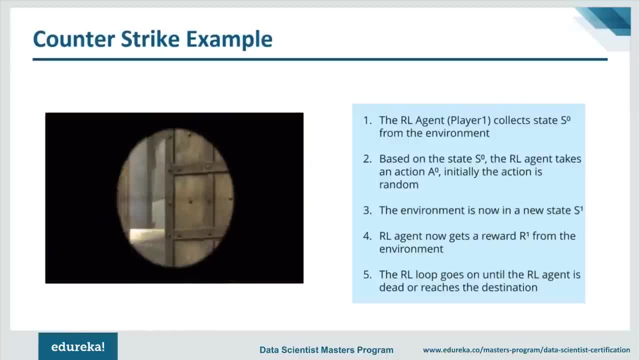 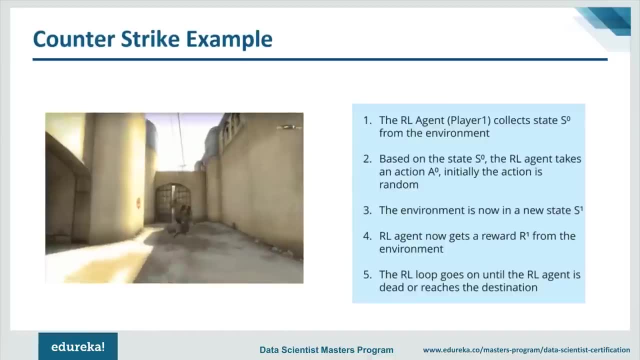 Now, based on this state, the agent will take some action. Okay, and this action can be anything that causes a result. So if the player moves left or right, it's also considered as an action. Okay, so initially the action is going to be random. 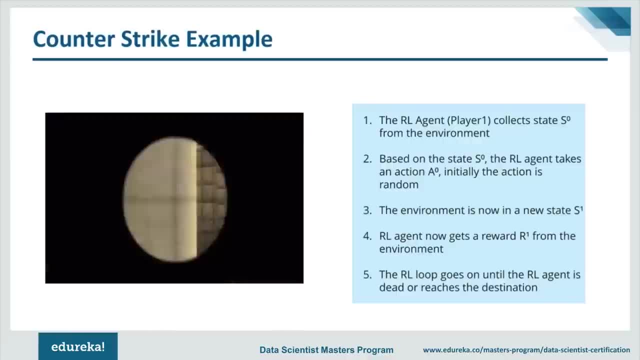 because obviously, the first time you pick up Counter Strike, you're not going to be a master at it, So you're going to try with different actions and you're just going to pick up a random action in the beginning. Now the environment is going to give a new state. 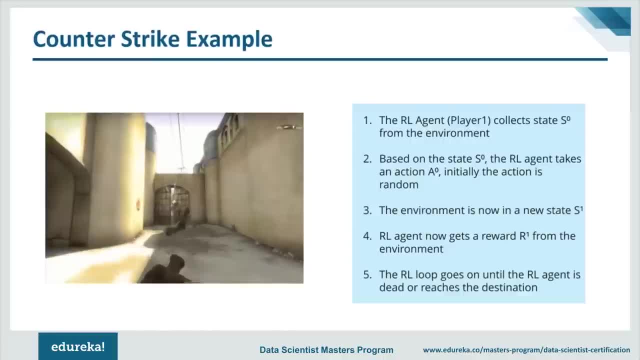 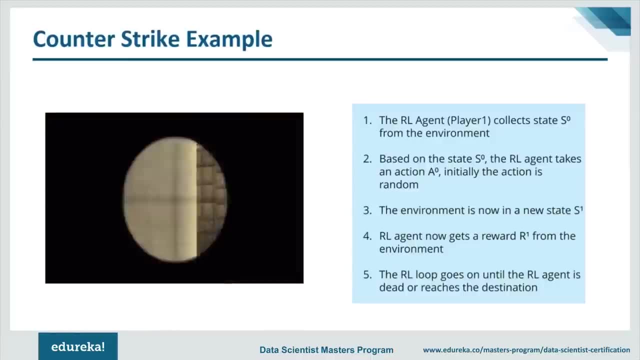 So after clearing that, the environment is now going to give a new state to the agent or to the player. So maybe he's crossed stage one Now he's in stage two. So now the player will get a reward- R1- from the environment because it cleared stage one. 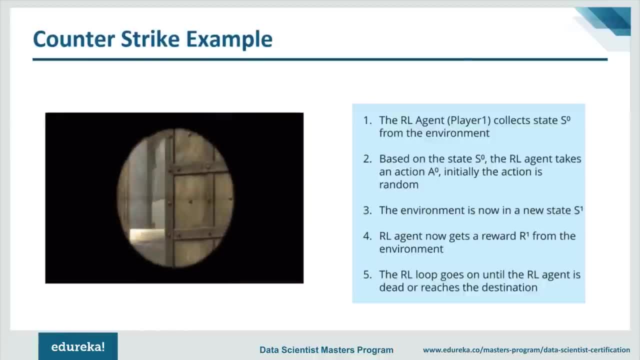 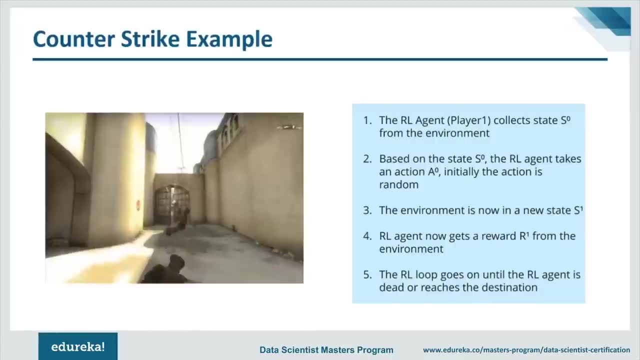 So this reward can be anything. It can be additional points or coins or anything like that, Okay. so basically, this loop keeps going on until the player is dead or reaches the destination- Okay- and it continuously outputs a sequence of states, actions and rewards. 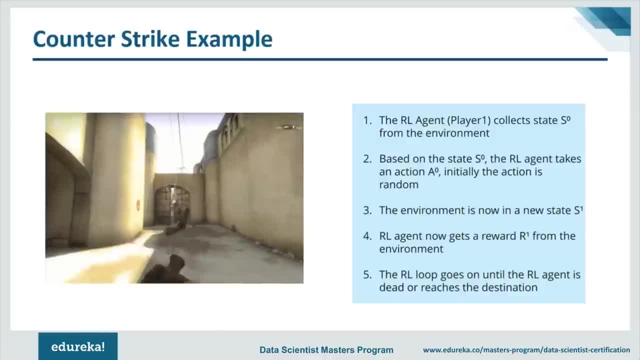 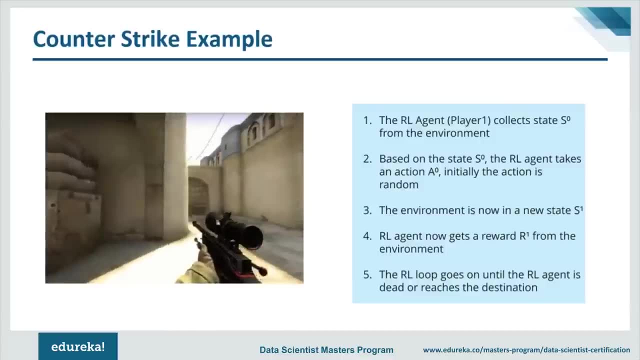 So, guys, this was a small example to show you how reinforcement learning process works. So you start with an initial state and once the player clears that state, he gets a reward. After that, the environment will give another stage to the player and after it clears that state, 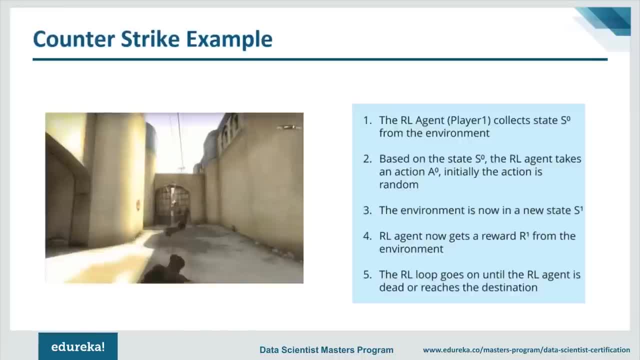 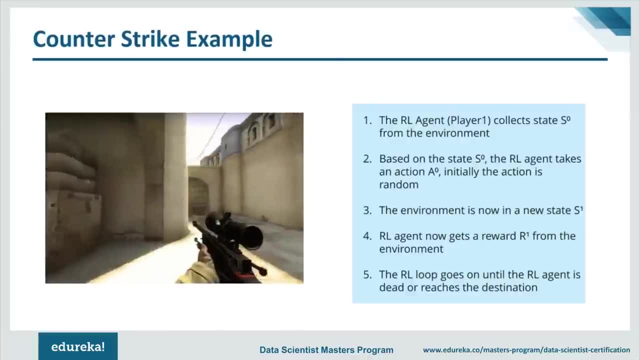 it's going to get another reward, and it's going to keep happening until the player reaches his destination. All right, So, guys, I hope this is clear. Now let's move on and look at the reinforcement learning definitions. So there are a few concepts that you should be aware of. 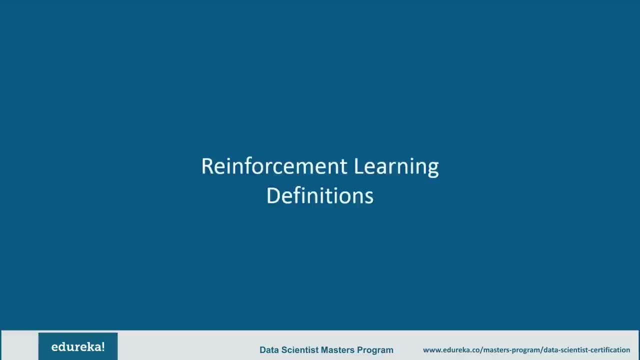 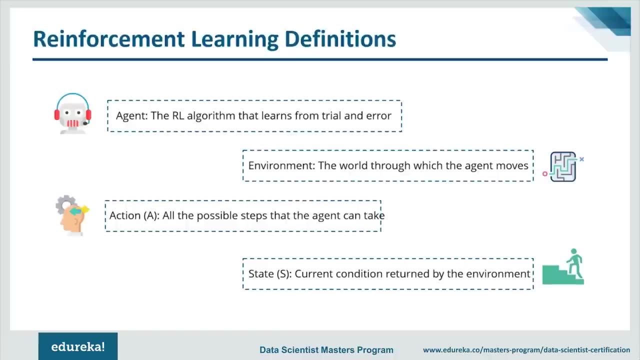 while studying reinforcement learning, Let's look at those definitions over here. So first we have the agent. Now an agent is basically the reinforcement learning algorithm that learns from trial and error. Okay, so an agent takes actions like, for example, a soldier in Counter-Strike navigating through the game. 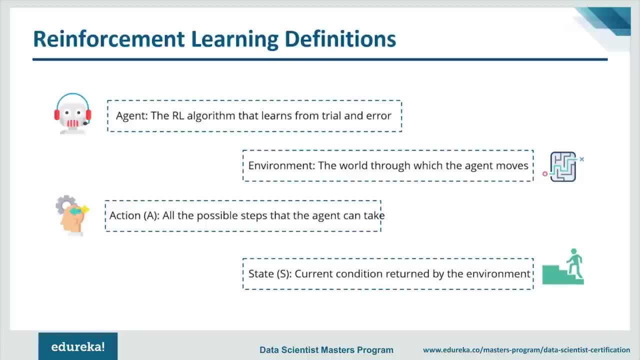 That's also an action. Okay, if he moves left, right or if he shoots at somebody, that's also an action Okay. so the agent is responsible for taking actions in the environment. Now, the environment is the whole Counter-Strike game. 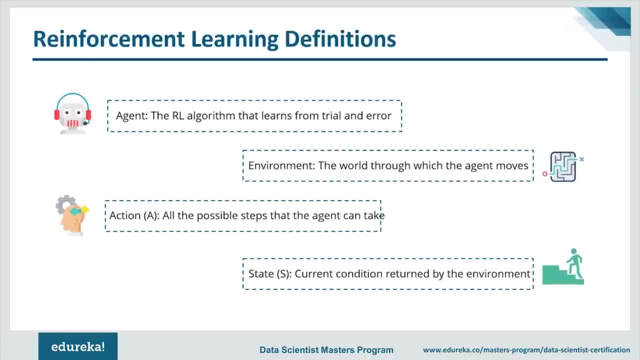 Okay, so it's basically the world through which the agent moves. the environment takes the agents current state and action as input and it returns the agents reward and its next state as output. All right, Next we have action. now all the possible steps that an agent can take are called actions. 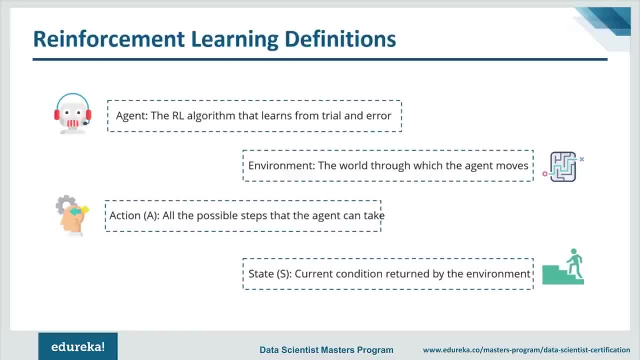 So, like I said, it can be moving right, left or shooting or any of that. All right. then we have state. now, state is basically the current condition returned by the environment. So, whichever state you are in, if you are in state one or if you're in state to, that represents your current condition. 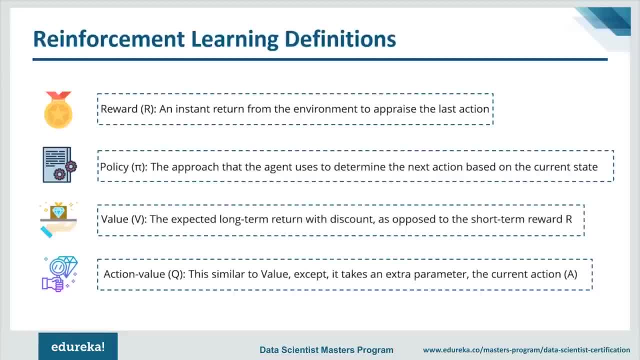 All right. Next we have reward. a reward is basically an instant return from the environment to appraise your last action. Okay, so it can be anything like coins or it can be additional points. So basically, a reward is given to an agent after it clears the specific stages. 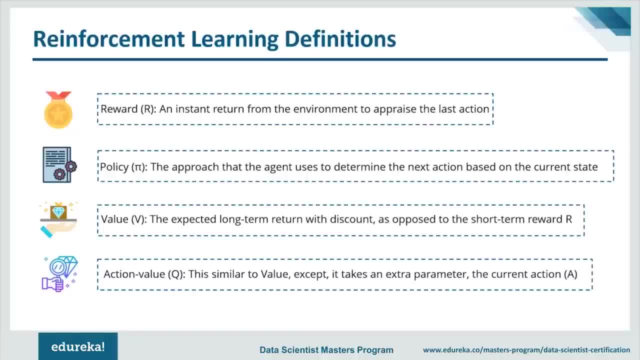 Next we have policy. policy is basically the strategy that the agent uses to find out his next action based on his current state. Policy is just the strategy with which you approach the game. Then we have value. Now value is the expected long-term return with discount. 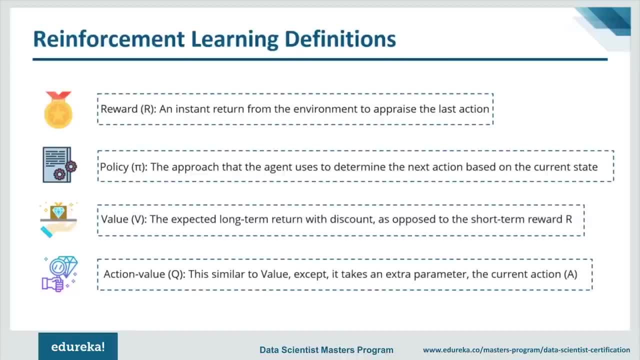 So value and action value can be a little bit confusing for you right now, but as we move further you'll understand what I'm talking about. Okay, So value is basically the long-term return that you get with discount. Okay, discount, I'll explain in the further slides. 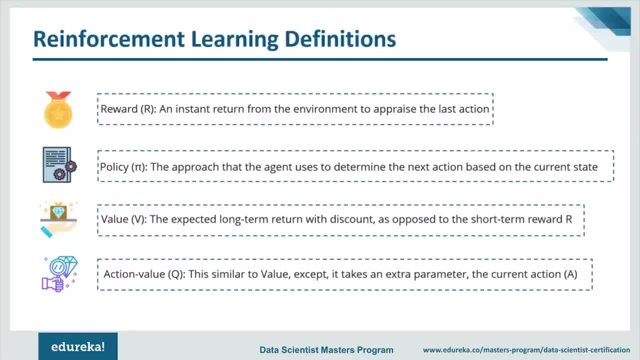 Then we have action value. Now, action value is also known as Q value. Okay, It's very similar to value, except that it takes an extra parameter, which is the current action. So, basically, here you'll find out the Q value, depending on the particular action that you took. 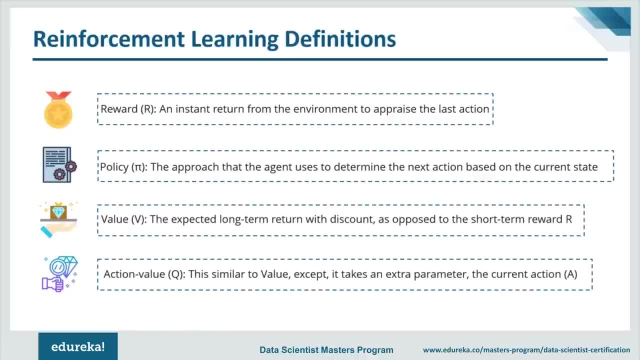 All right. So, guys, don't get confused with value and action value. We look at examples in the further slides and you'll understand this better, Okay, So, guys, make sure that you're familiar with these terms, because you'll be seeing a lot of these terms in the further slides. 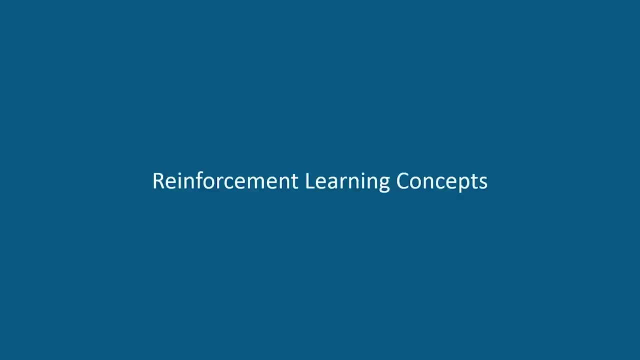 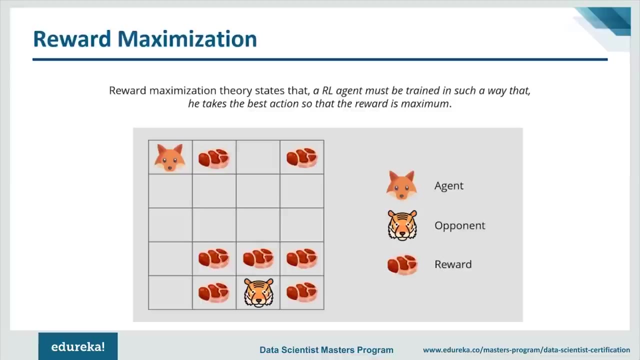 All right Now, before we move any further, I'd like to discuss a few more concepts. Okay, So first we'll discuss the reward maximization. So, if you have haven't already realized it, the basic aim of the RL agent is to maximize the reward. 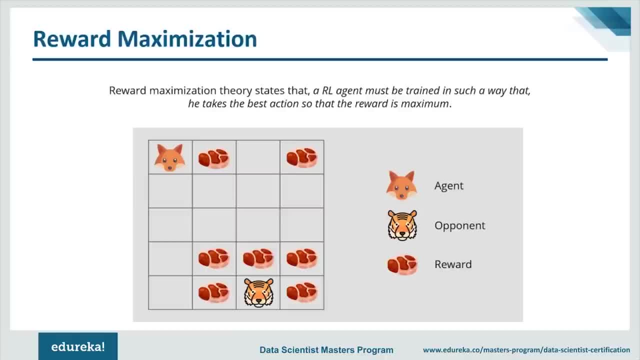 Now, how does that happen? Let's try to understand this in depth. So the agent must be trained in such a way that he takes the best action so that the reward is maximum, because the end goal of reinforcement learning is to maximize your reward based on a set of actions. 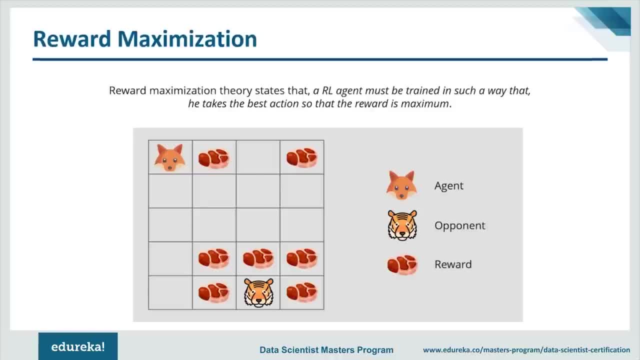 So let me explain this with a small game. Now in the figure you can see there is a Fox, There's some meat and there's a tiger. So our agent is basically the Fox and his end goal is to eat the maximum amount of meat. 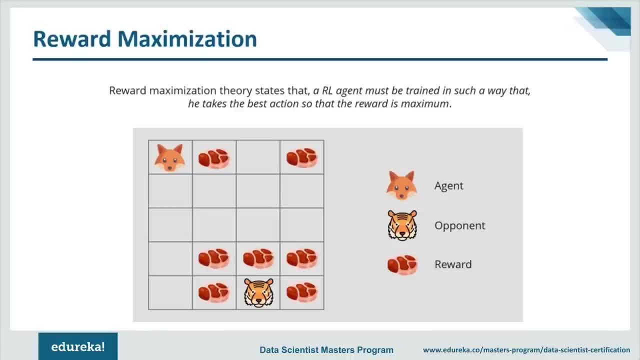 before being eaten by the tiger. Now, since the Fox is a clever fellow, he eats the meat that is closer to him, rather than the meat which is closer to the tiger. Now, this is because the closer he is to the tiger, the higher are his chances of getting killed. 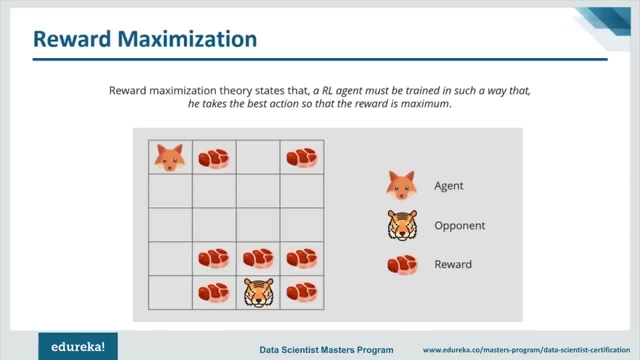 So, because of this, the rewards which are near the tiger, even if they are bigger meat chunks, they will be discounted. So this is exactly what discounting means. So our agent is not going to eat the meat chunks which are closer to the tiger because of the risk. 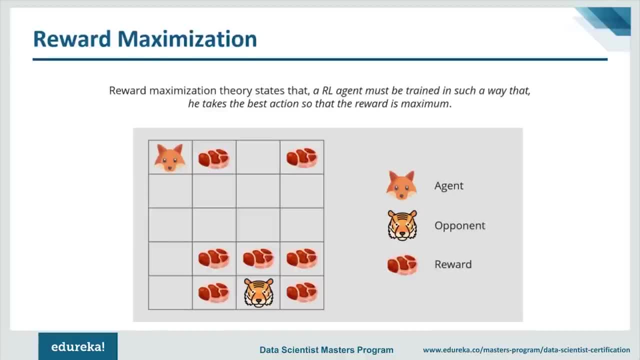 Now, even though the meat chunks might be larger, he does not want to take the chances of getting killed. This is called discounting. This is where you discount because you improvise and you just eat the meat which are closer to you, instead of taking risks and eating the meat. 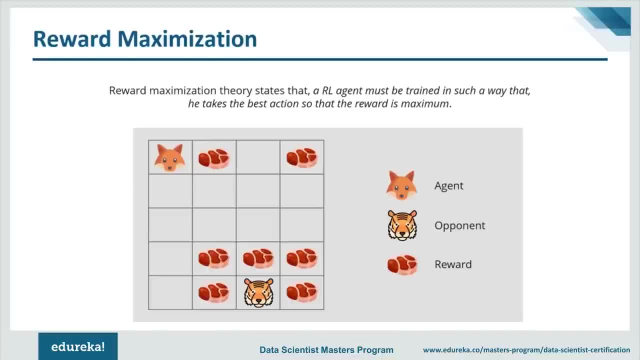 which are closer to your opponent. Now the discounting of reward works based on a value called gamma. We'll be discussing gamma in our further slides, But, in short, the value of gamma is between 0 and 1. So the smaller the gamma. 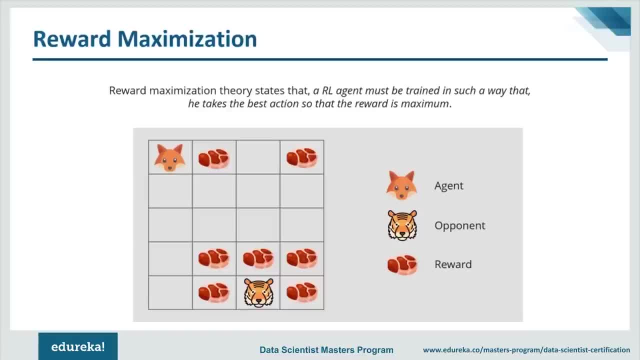 the larger is the discount value. So if the gamma value is lesser, it means that the agent is not going to explore and he's not going to try and eat the meat chunks which are closer to the tiger. But if the gamma value is closer to 1,. 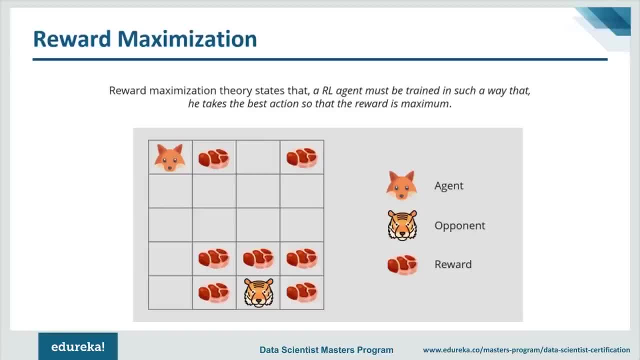 it means that our agent is actually going to explore and it's going to try and eat the meat chunks which are closer to the tiger. Now I'll be explaining this in depth in the further slides, So don't worry if you haven't got a clear concept yet. 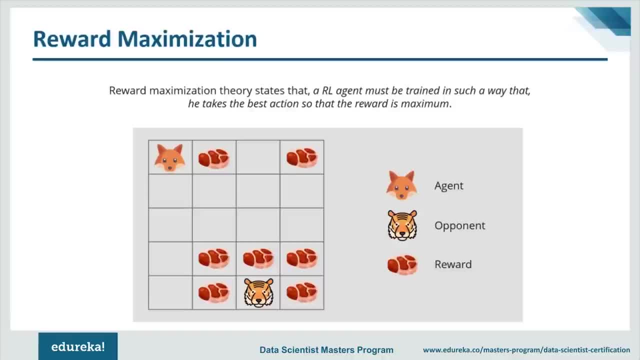 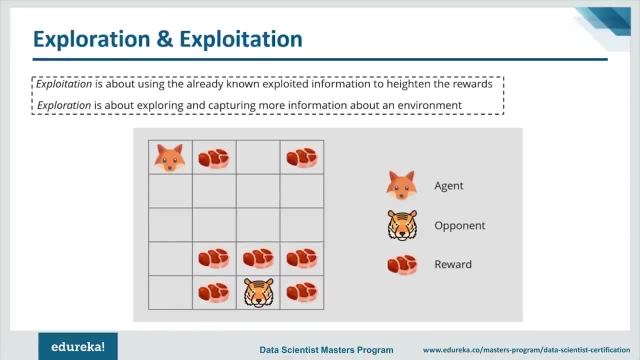 But just understand that reward maximization is a very important step when it comes to reinforcement learning, because the agent has to collect maximum rewards by the end of the game. All right, Now let's look at another concept, which is called exploration and exploitation. So exploration, like the name suggests. 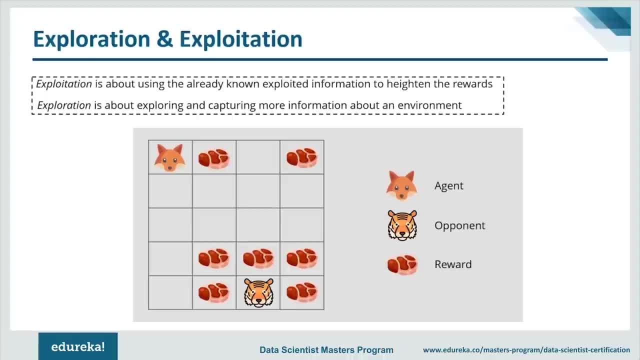 is about exploring and capturing more information about an environment. On the other hand, exploitation is about using the already known, exploited information to heighten the rewards. So guys, consider the fox and tiger example that we learned and we discussed Now here. the fox eats only the meat chunks. 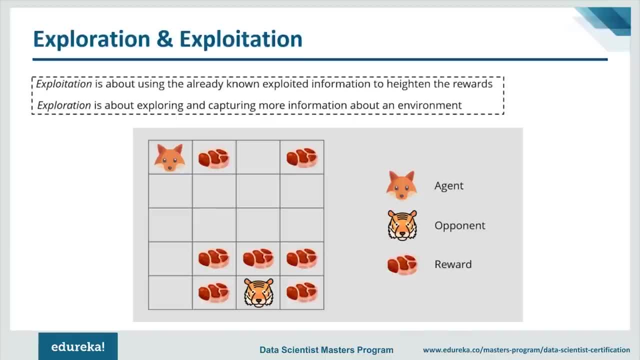 which are close to him, but he does not eat the meat chunks which are closer to the tiger. Okay, even though they might give him more rewards, he does not eat them. If the fox only focuses on the closest rewards, he will never reach the big chunks of meat. 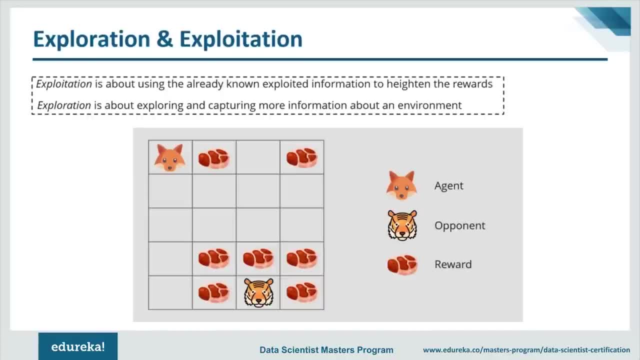 Okay, this is what exploitation is about. You're just going to use the currently known information and you're going to try and get rewards based on that information. But if the fox decides to explore a bit, it can find the bigger reward, which is the big chunks of meat. 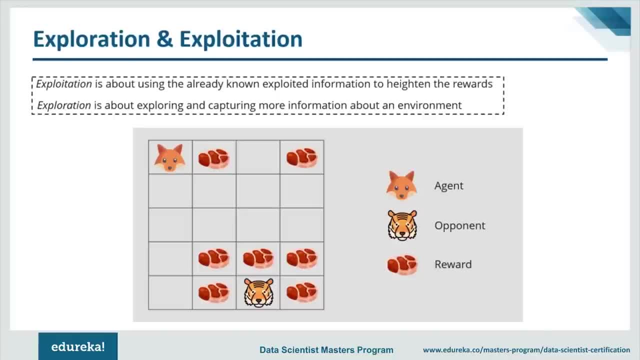 This is exactly what exploration is, So the agent is not going to stick to one corner. Instead, he's going to explore the entire environment and try and collect bigger rewards. All right, So, guys, I hope you all are clear with exploration and exploitation. 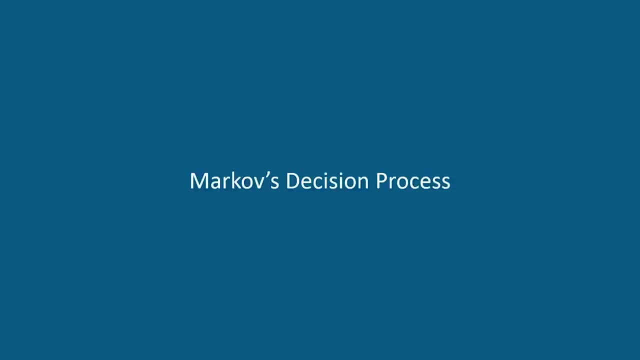 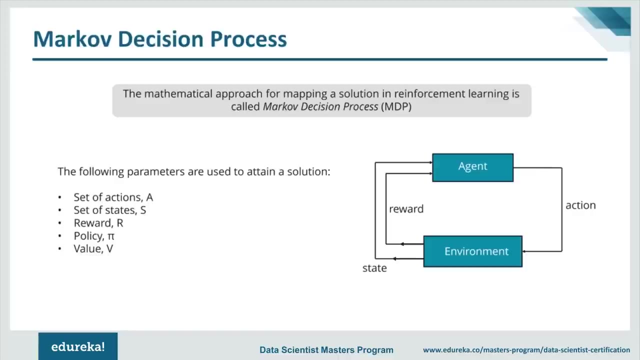 Now let's look at the Markov's decision process. So, guys, this is basically a mathematical approach for mapping a solution in reinforcement learning. In a way, the purpose of reinforcement learning is to solve a Markov problem. Markov decision process. 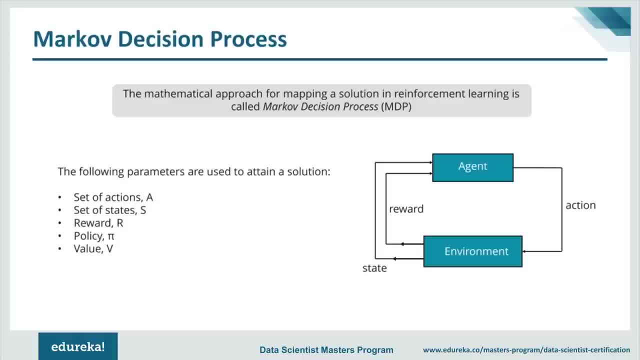 Okay, so there are a few parameters that are used to get to the solution. So the parameters include the set of actions, the set of states, the rewards, the policy that you're taking to approach the problem and the value that you get. 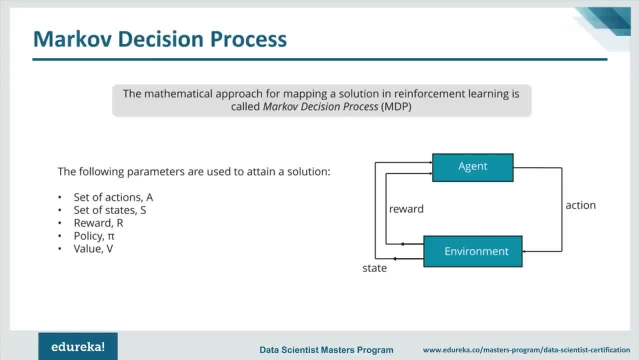 Okay. so to sum it up, the agent must take an action A to transition from a start state to the end state S. While doing so, the agent will receive a reward R for each action that he takes. So, guys, a series of actions taken by the agent. 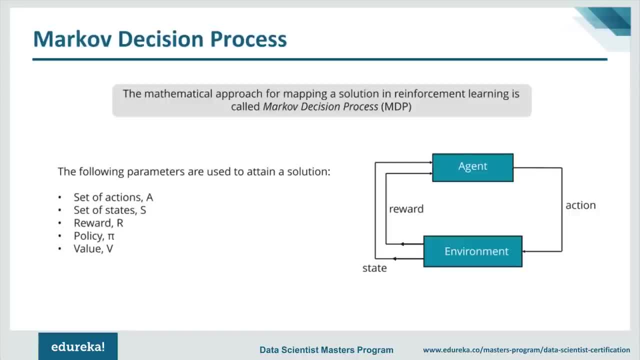 define the policy, or it defines the approach, and the rewards that are collected define the value. So the main goal here is to maximize the rewards by choosing the optimum policy. All right now let's try to understand this with the help of the shortest path problem. 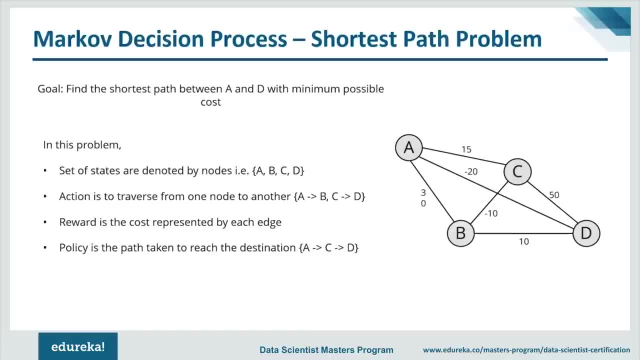 I'm sure a lot of you might have gone through this problem when you were in college. So, guys, look at the graph over here. So our aim here is to find the shortest path between A and D with minimum possible cost. So the value that you see on each of these edges- 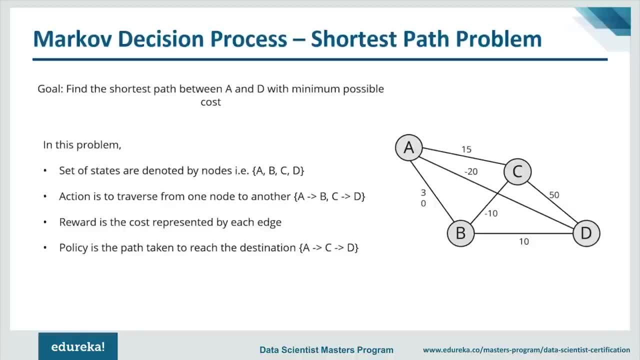 basically denotes the cost. So if I want to go from A to C, it's going to cost me 15 points. Okay, so let's look at how this is done Now, before we move and look at the problem. in this problem, the set of states are denoted. 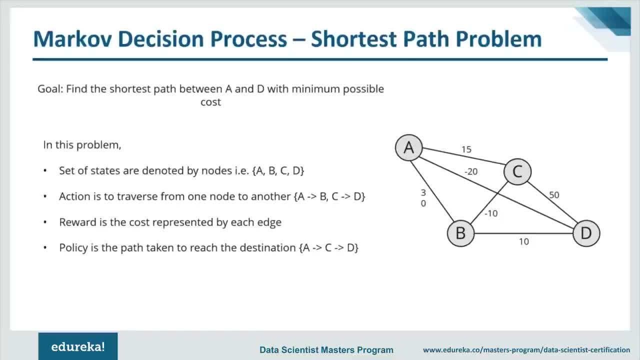 by the nodes, which is A, B, C, D, and the action is to traverse from one node to the other. So if I'm going from A to B, that's an action. Similarly, A to C, that's an action. 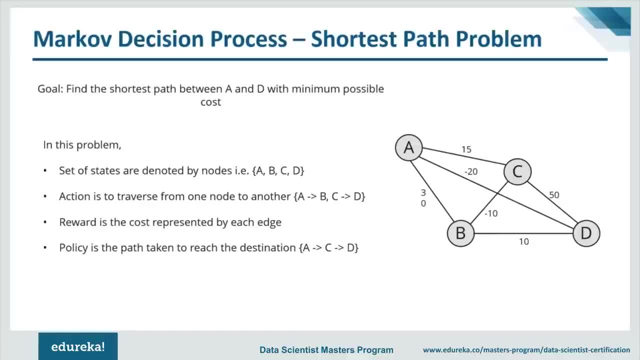 Okay, the reward is basically the cost, which is represented by each edge over here. All right, now. the policy is basically the path that I choose to reach the destination. So let's say I choose A, C, D. Okay, that's one policy. 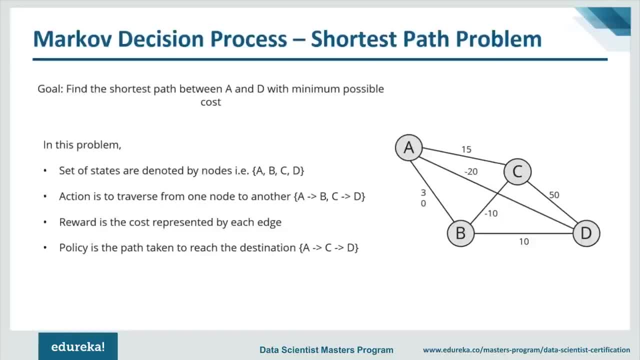 In order to get to D, I'm choosing A, C, D, which is a policy. Okay, it's basically how I'm approaching the problem. So, guys, here you can start off at node A and you can take baby steps to your destination. 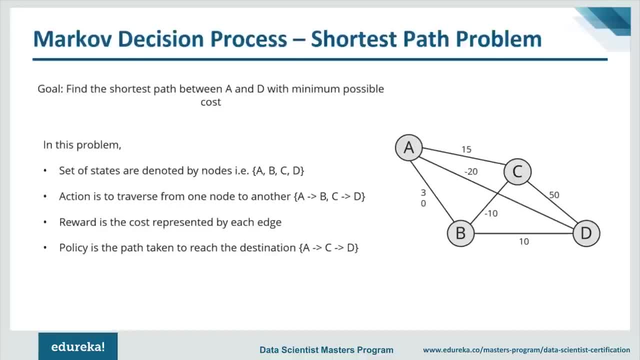 Now, initially you're clueless, so you can just take the next possible node which is visible to you. So, guys, if you're smart enough, you're going to choose A to C instead of A B, C D or A B D. 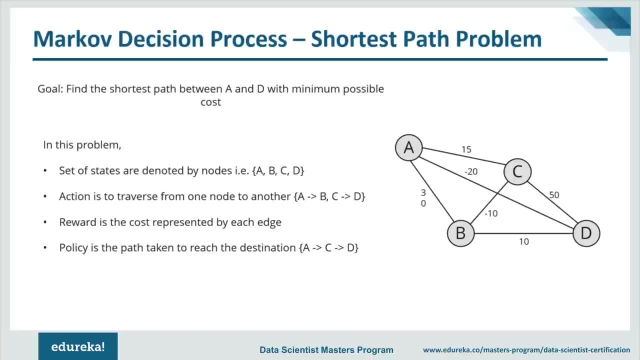 All right. So now, if you're at node C, you want to traverse to node D. You must again choose a wise path. All right, you just have to calculate which path has the highest cost or which path will give you the maximum rewards. 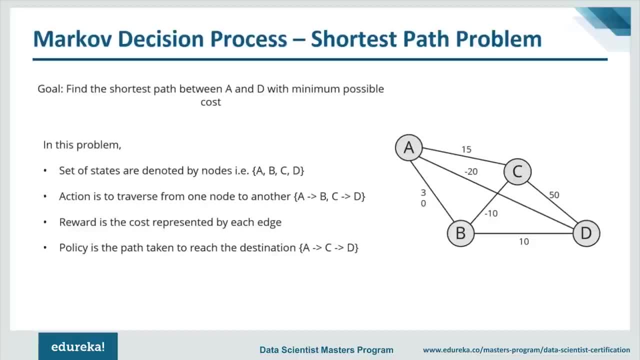 So, guys, this is a simple problem. We're just trying to calculate the shortest path between A and D by traversing through these nodes. So if I traverse from A, C, D, it gives me the maximum reward. Okay, it gives me 65,. 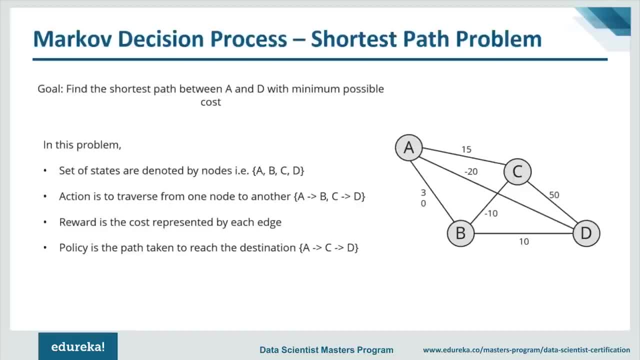 which is more than any other policy would give me Okay. so if I go from A B D, it would be 40. When you compare this to A C D, it gives me more rewards. So obviously I'm going to go with A C D. 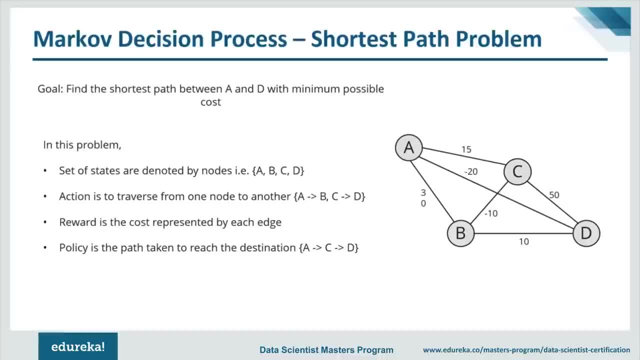 Okay. so, guys, it was a simple problem in order to understand how Markov decision process works, All right. so, guys, I want to ask you a question: What do you think I did here? Did I perform exploration or did I perform exploitation? 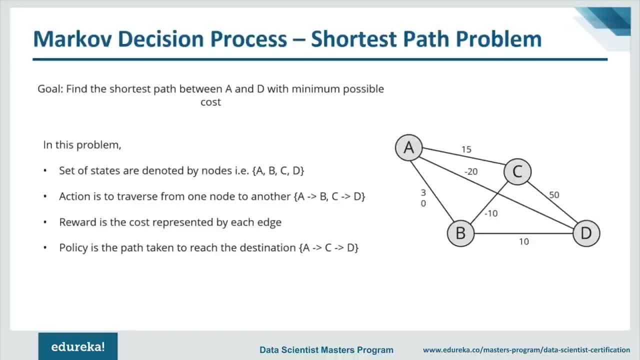 Now the policy for the above example is of exploitation, because we didn't explore the other nodes. Okay, we just selected three nodes and we traverse through them. So that's why this is called exploitation. We must always explore the different nodes so that we can find a more optimal policy. 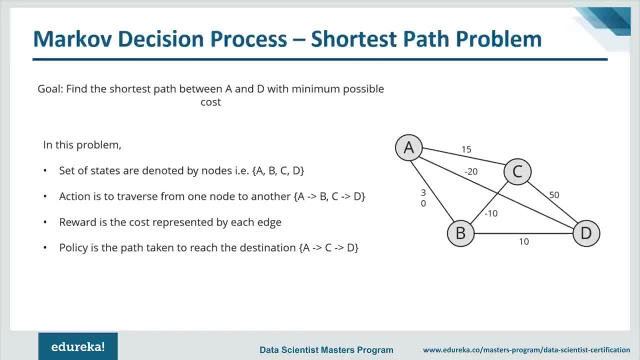 But in this case obviously A C D has the highest reward and we're going with A C D. But generally it's not so simple. There are a lot of nodes, There are hundreds of nodes to traverse and there are like 50, 60 policies. 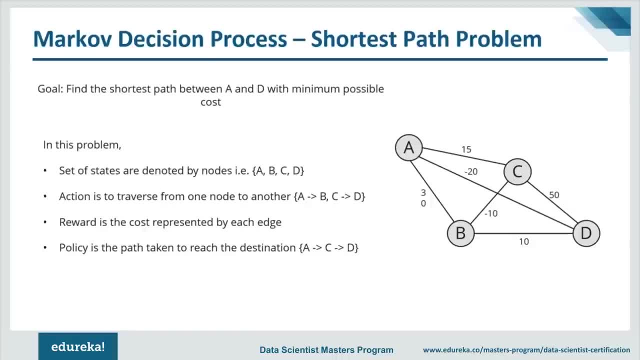 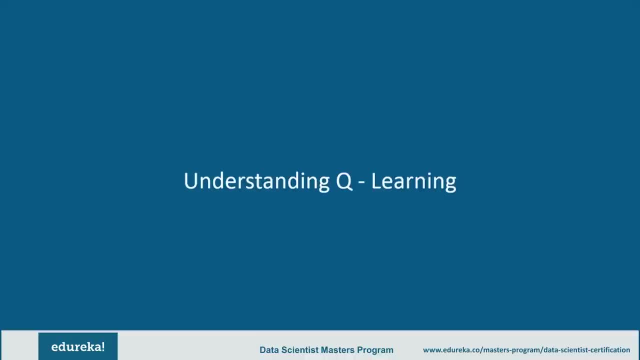 Okay, 50,, 60 different policies. So you make sure you explore through all the policies and then decide on an optimum policy which will give you a maximum reward. So, guys, before we perform the hands-on process for the hands-on part, 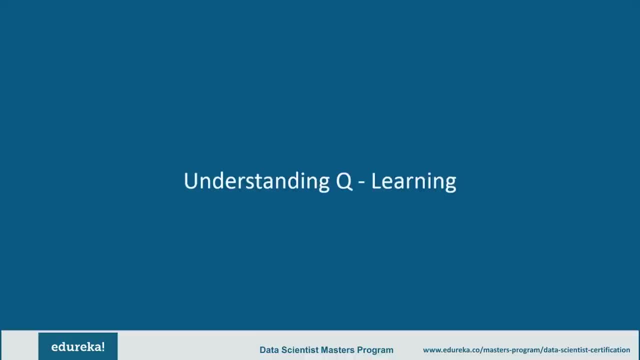 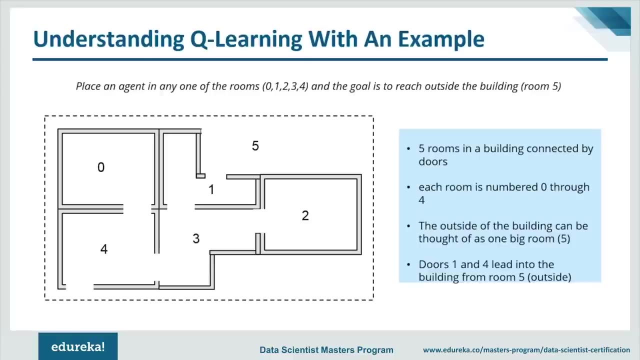 let's try to understand the math behind our demo. Okay, so in our demo we'll be using the Q learning algorithm, which is a type of reinforcement learning algorithm. Okay, it's simple. It just means that you have to take the best possible actions. 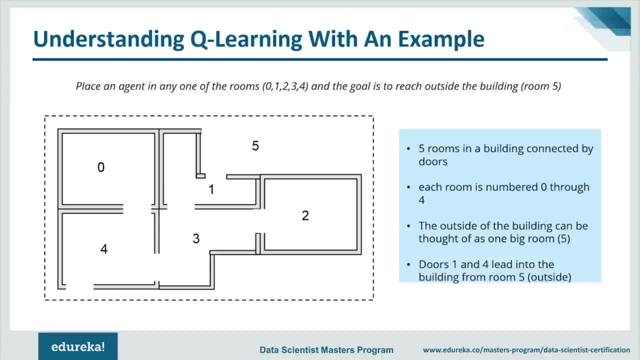 to reach your goal or to get the most rewards. All right, let's try to understand this with an example. So, guys, this is exactly what will be running in our demo, So make sure you understand this properly. Okay, so our goal here is: 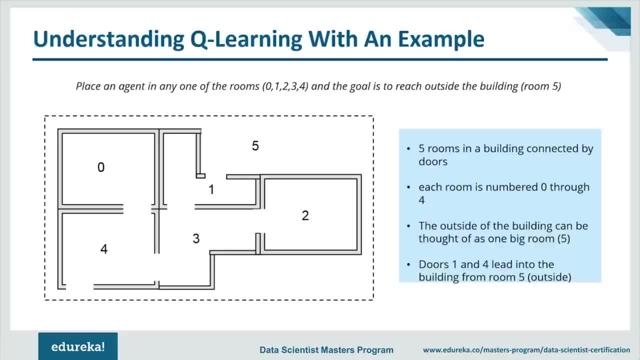 we're going to place an agent in any one of the rooms, Okay, so basically, these squares. you see, here are rooms, Okay. 0 is a room. 4 is a room. 3 is a room. 1 is a room. 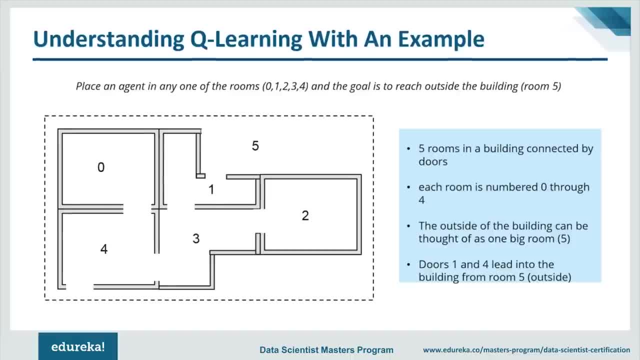 and 2 is a room. 5 is also a room. It's basically a way outside the building, All right, so what we're going to do is we're going to place an agent in any one of these rooms and the goal is to reach outside the building. 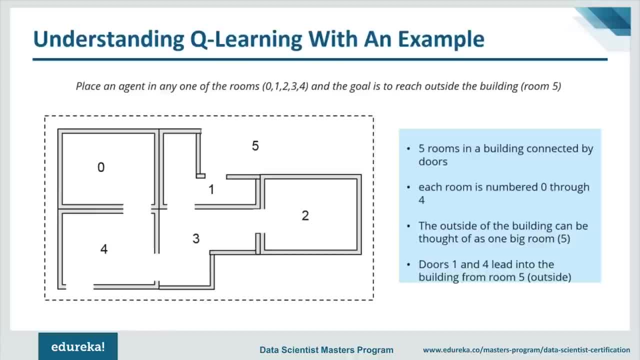 Okay, outside the building is room number 5.. Okay, so these empty spaces are basically doors, which means that you can go from 0 to 4.. You can go from 4 to 3,, 3 to 1,, 5 to 5,. 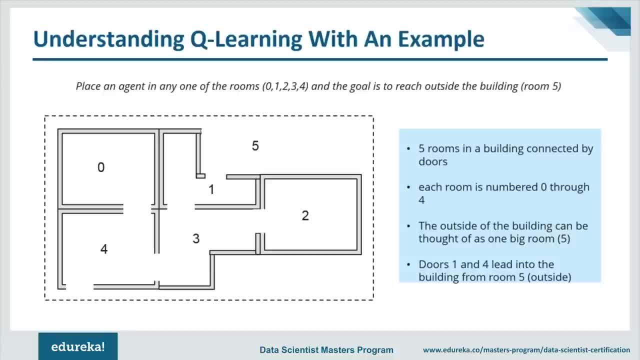 and similarly 3 to 2, but you can't go from 5 to 2 directly. All right, so there are certain set of rooms that don't get connected directly. Okay, so, like I've mentioned here, each room is numbered from 0 to 4. 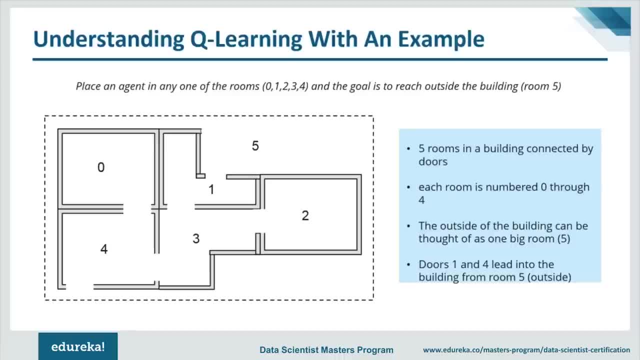 and the outside of the building is numbered as 5.. And one thing to note here is: room 1 and room 4 directly lead to room number 5.. All right, so room number 1 and 4 will directly lead out to room number 5.. 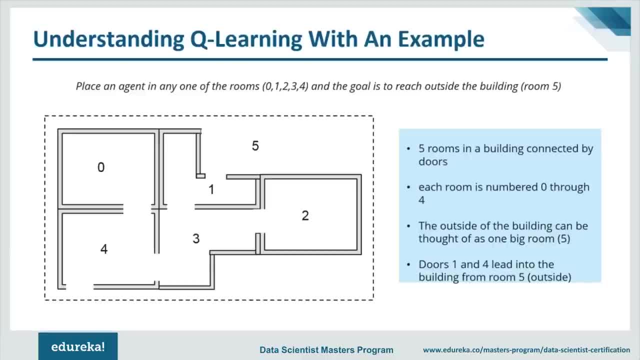 So, basically, our goal over here is to get to room number 5.. Okay, to set this room as a goal, we'll associate a reward value to each door. Okay, don't worry, I'll explain what I'm saying. So if you represent these rooms in a graph, 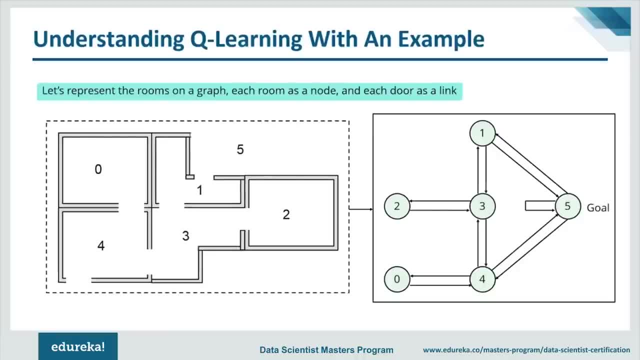 this is how the graph is going to look, Okay. so, for example, from 2, you can go to 3, and then 3 to 1,, 1 to 5,, which will lead us to our goal. These arrows represent the link between the doors. 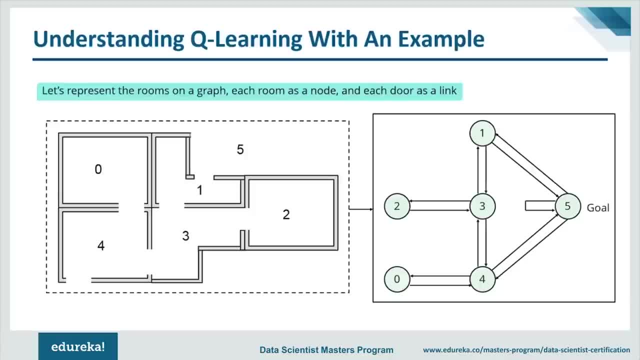 All right, this is quite understandable. Now our next step is to associate a reward value to each of these doors. Okay, so the rooms that are directly connected to our end room, which is room number 5, will get a reward of 100. 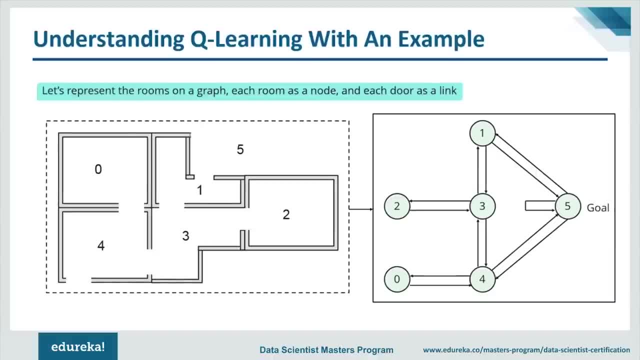 Okay, so basically, our room number 1 will have a reward 5.. Now, this is obviously because it's directly connected to 5.. Similarly, 4 will also be associated with a reward of 100, because it's directly connected to 5.. 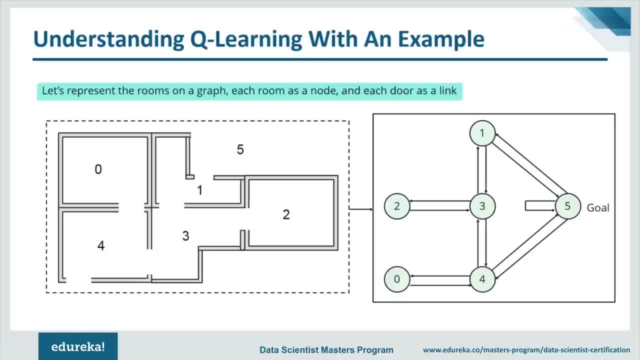 Okay, so if you go out from 4, it'll lead to 5.. Now the other nodes are not directly connected to 5.. So you can't directly go from 0 to 5.. Okay, so for this we'll be assigning a reward of 0.. 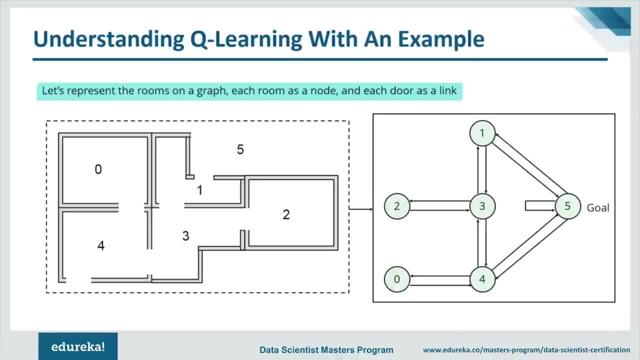 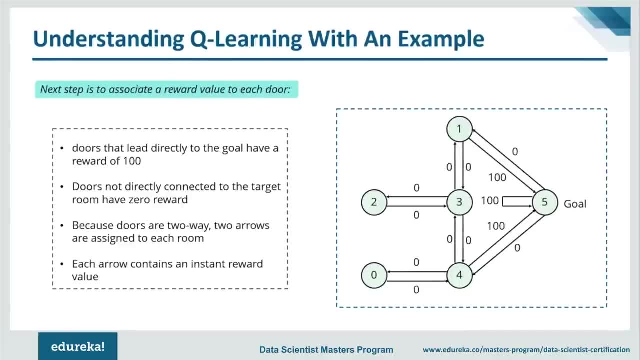 So, basically, other doors not directly connected to the target room have a 0 reward. Okay, now, because the doors are two-way, the two arrows are assigned to each room. Okay, you can see two arrows assigned to each room. So, basically, 0 leads to 4. 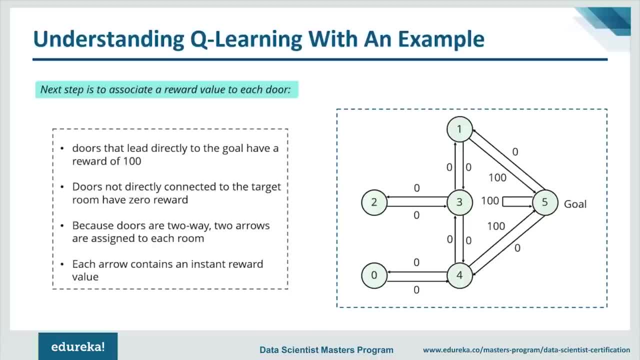 and 4 leads back to 0.. Now we've assigned 0, 0 over here because 0 does not directly lead to 5. But 1 directly leads to 5 and that's why you can see 100 over here. 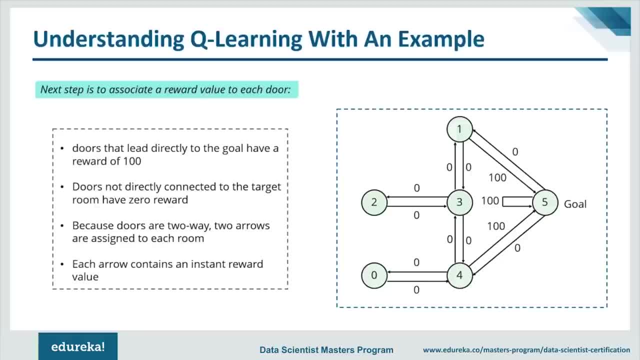 Similarly, 4 directly leads to our goal state, and that's why we've assigned 100 over here, And obviously 5 to 5 is 100 as well. So here all the direct connections to room number 5 are rewarded 100. 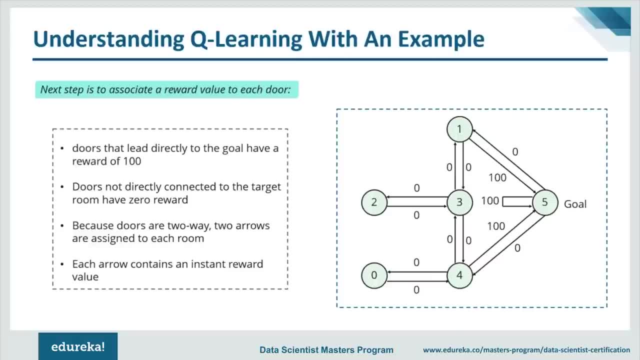 and all the indirect connections are rewarded: 0.. So, guys, in Q-learning, the end goal is to reach the state with the highest reward, so that the agent arrives at the goal. Okay, so let me just explain this graph to you in detail. 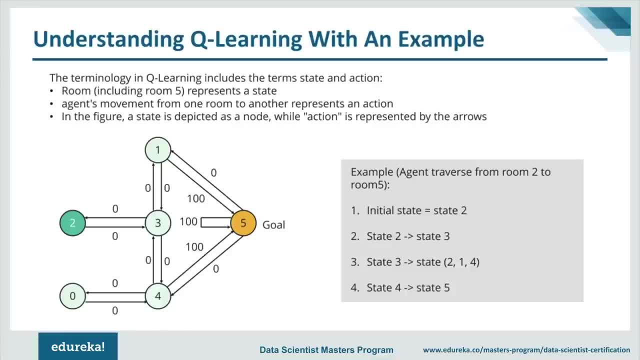 Now these rooms over here labeled 1,, 2,, 3 to 5, they represent the state an agent is in. So if I state 1,, it means that the agent is in room number 1.. Similarly, the agent's movement. 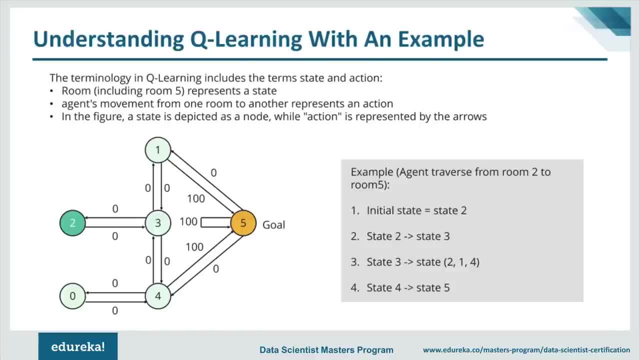 from one room to the other represents the action. Okay, so if I say 1 to 3, it represents an action, Alright, So basically, the state is represented as node and the action is represented by these arrows. Okay, so this is what this graph is about. 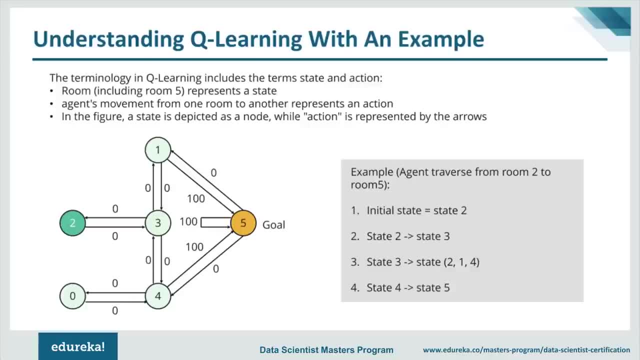 These nodes represent the rooms and these arrows represent the actions. Okay, let's look at a small example. Let's set the initial state to 0.. So my agent is placed in room number 2 and he has to travel all the way to room number 5.. 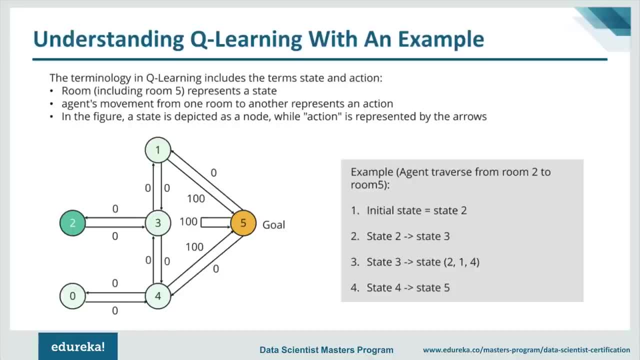 So if I set the initial state to 2, he can travel to state 3.. Okay, from 3, he can either go to 1, or he can go back to 2, or he can go to 4.. If he chooses to go to 4,, 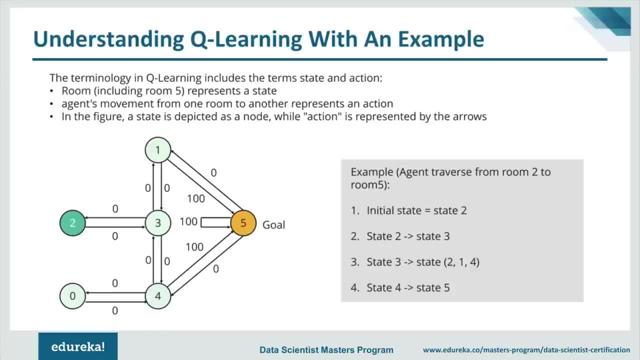 it will directly take him to room number 5.. Okay, which is our end goal, And even if he goes from room number 3 to 1, it will take him to room number 5.. So this is how our algorithm works. 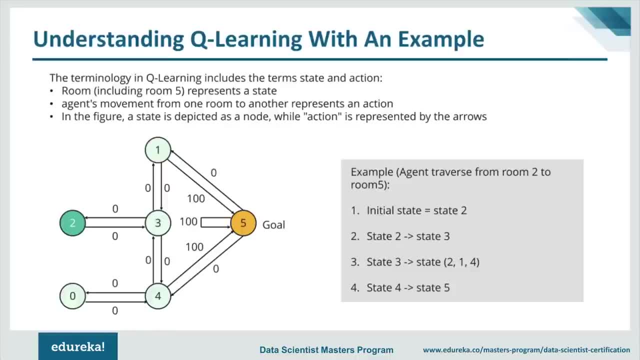 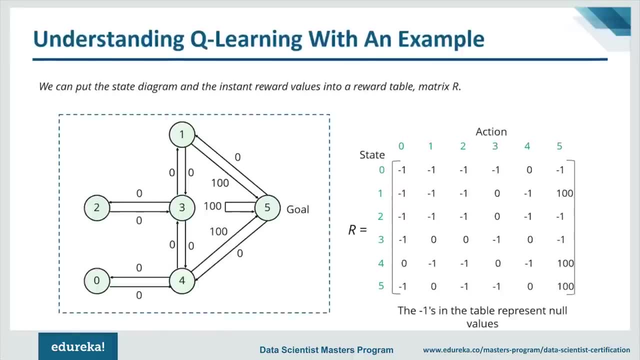 It's going to traverse different rooms in order to reach the goal room, which is room number 5.. Now let's try and depict these rewards in the form of a matrix. Okay, because we'll be using this R matrix or the reward matrix. 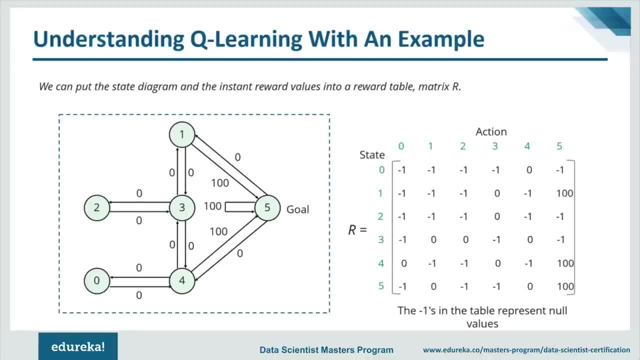 to calculate the Q value or the Q matrix. Okay, we'll see what the Q value is in the next step, But for now, let's see how this reward matrix is calculated. Now, the minus 1s that you see in the table. 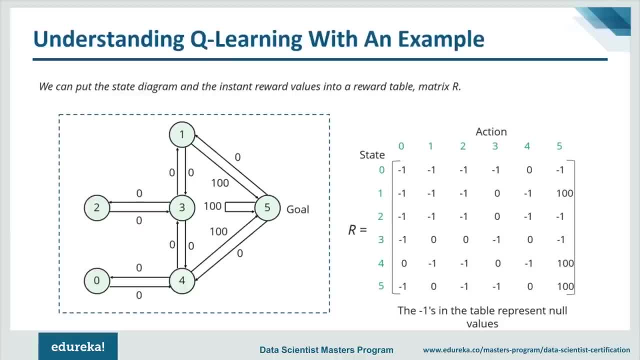 they represent the null values. Now these minus 1 basically means that wherever there is no link between nodes, it's represented as minus 1.. So 0 to 0 is minus 1.. 0 to 1, there is no link. 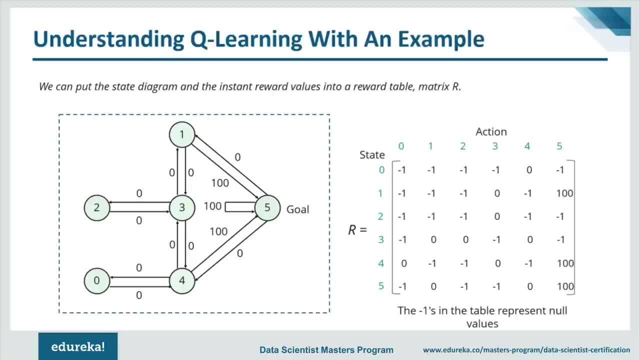 Okay, there's no direct link from 0 to 1.. So it's represented as minus 1.. Similarly, 0 to 2, also there is no link. You can see there's no line over here, So this is also minus 1.. 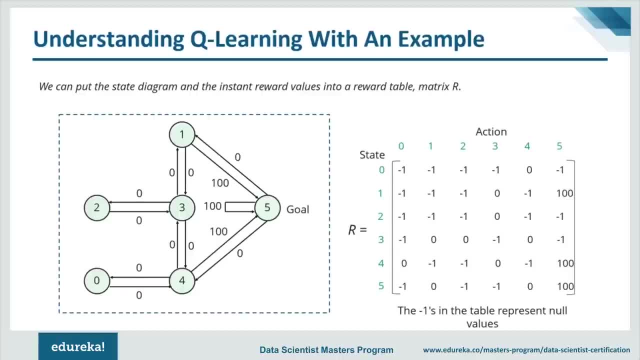 But when it comes to 0 to 4, there is a connection and we have numbered it 0 because the reward for a state which is not directly connected to the goal is 0. But if you look at this, 1,, 5,- 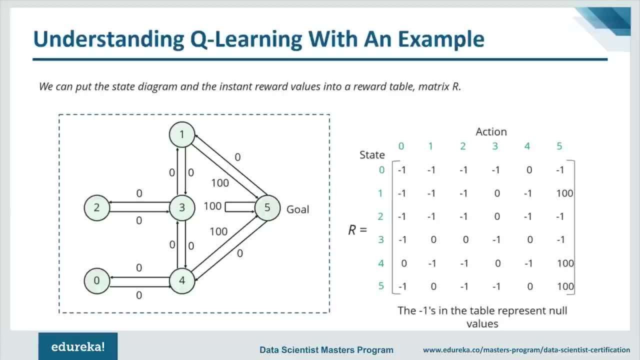 which is basically traversing from node 1 to node 2, you can see, the reward is 100.. Okay, that's basically because 1 and 5 are directly connected and 5 is our end goal. So any node which is directly connected to our goal state. 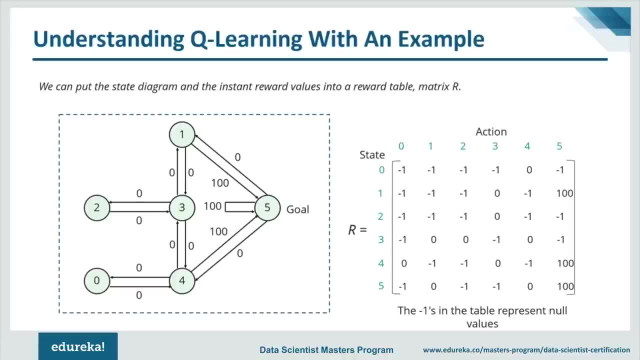 will get a reward of 100.. Okay, that's why I've put 100 over here. Similarly, if you look at the fourth row over here, I've assigned 100 over here. This is because from 4 to 5, there is a direct connection. 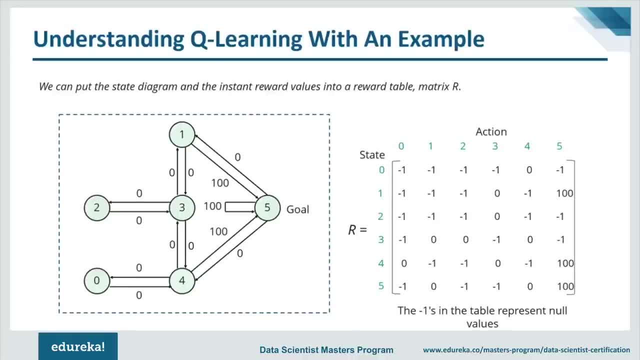 There's a direct connection which gives them a 100 reward. Okay, you can see, from 4 to 5, there is a direct link. Okay, so from room number 4 to room number 5, you can go directly. That's why there's a 100 reward over here. 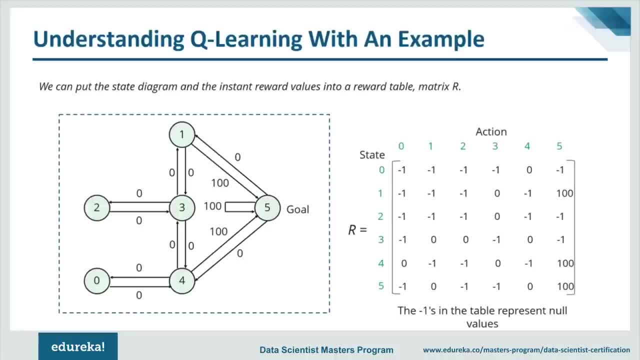 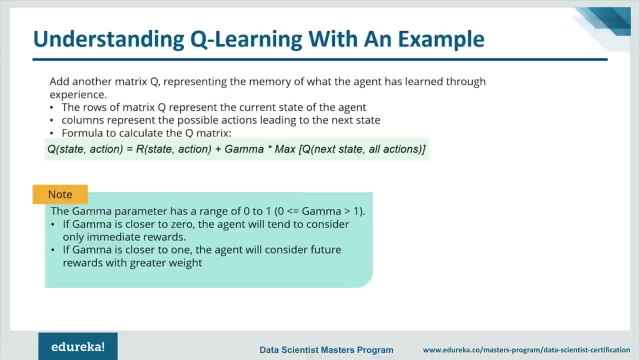 So, guys, this is how the reward matrix is made. Alright, I hope this is clear to you all. Okay, now that we have the reward matrix, we need to create another matrix called the Q matrix. Okay, here you'll store all the Q values that we'll calculate. 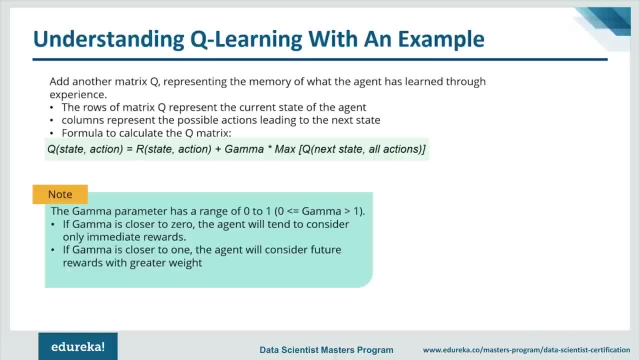 Now, this Q matrix basically represents the memory of what the agent has learned through experience. Okay, so once he traverses from one room to the final room, whatever he's learned is stored in this Q matrix In order for him to remember that the next time he traverses. 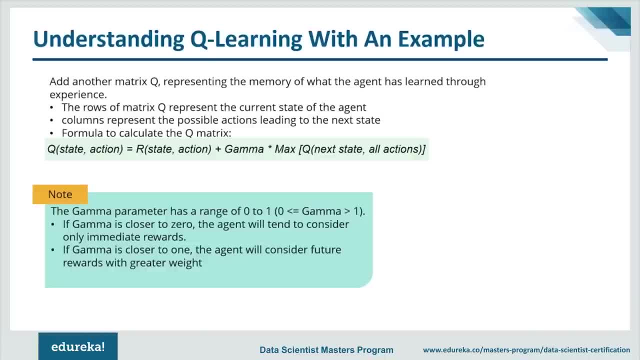 we use this matrix. Okay, it's basically like a memory. So, guys, the rows of the Q matrix will represent the current state of the agent, The columns will represent the possible actions And to calculate the Q value, you use this formula. 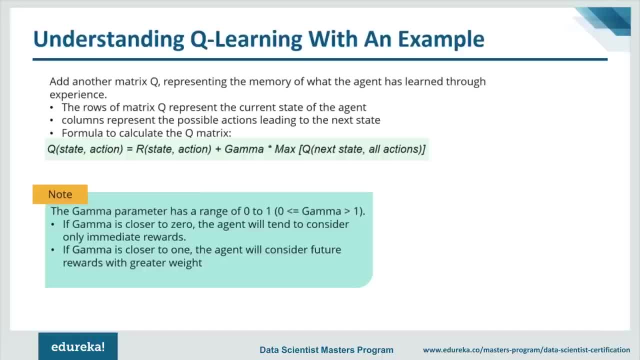 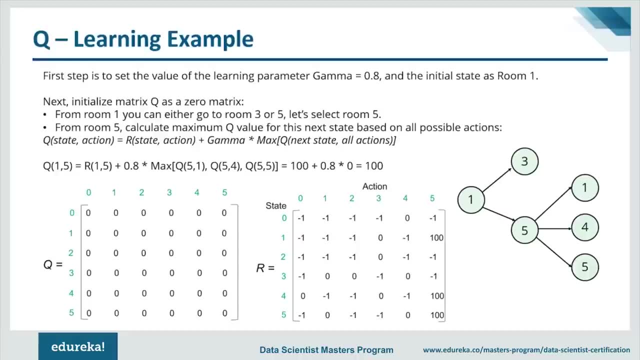 Alright, I'll show you what the Q matrix looks like, But first let's understand this formula. Now, this Q value we're calculating because we want to fill in the Q matrix. Okay, so this is basically our Q matrix, over here. 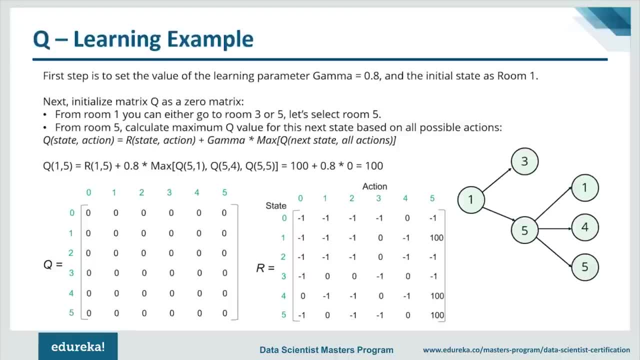 Actually it's all zero, but as the agent traverses from different nodes to the destination node, this matrix will get filled up, Okay. so basically, it will be like a memory to the agent. He'll know that, okay, when he traversed using a particular path. 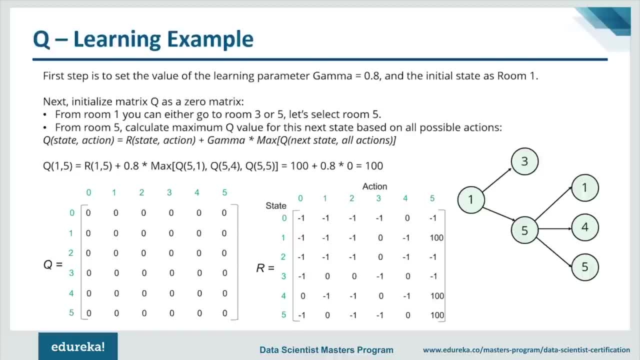 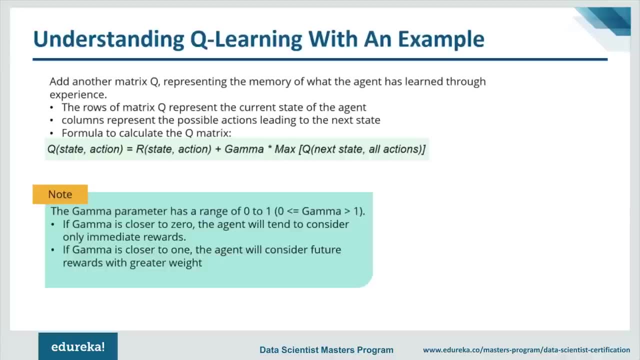 he found out that his value was maximum or his reward was maximum over here, So next time he'll choose that path. This is exactly what the Q matrix is. Okay, let's go back Now, guys. don't worry about this formula for now. 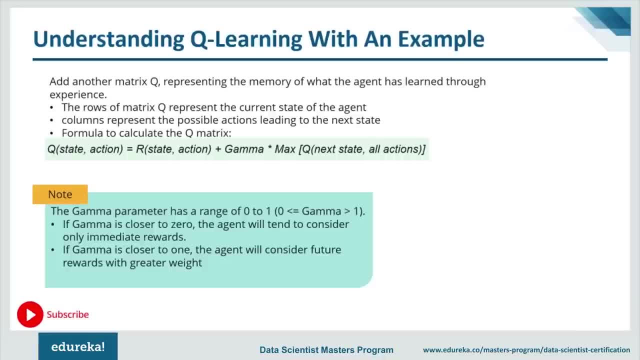 because we'll be implementing this formula in an example in the next slide. Okay, so don't worry about this formula for now, But here just remember that this Q basically represents the Q matrix, The R represents the reward matrix and the gamma is a gamma value. 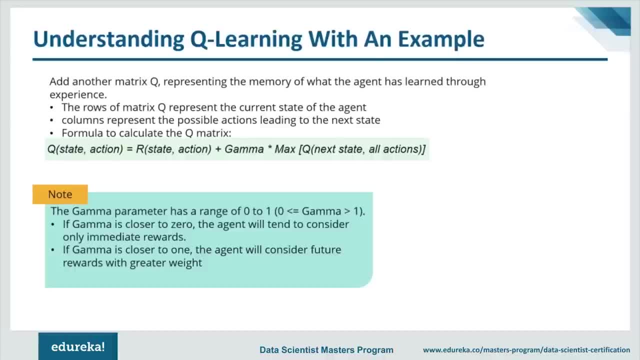 which I'll talk about shortly, And here you're just finding out the maximum from the Q matrix. So basically, the gamma parameter has a range from zero to one, So you can have a value of 0.1,, 0.3,, 0.5,, 0.8. 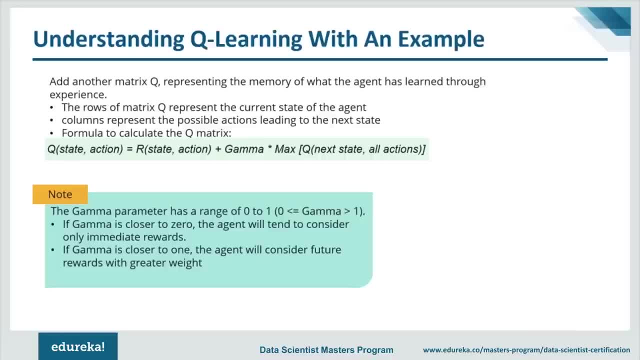 and all of that. So if the gamma is closer to zero, it means that the agent will consider only the immediate rewards, which means that the agent will not explore the surrounding. Basically, it won't explore different rooms, It'll just choose a particular room. 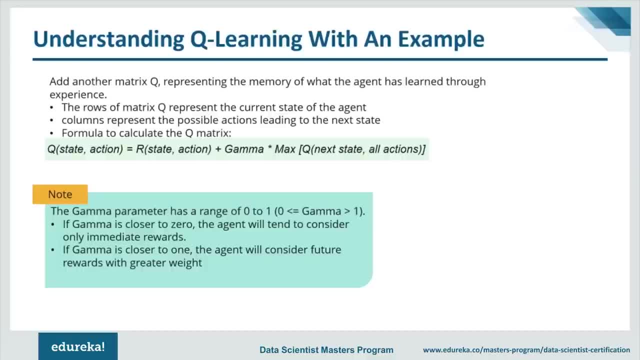 and then it'll try sticking to it. But if the value of gamma is high, meaning that if it's closer to one, the agent will consider future rewards with greater weight- This means that the agent will explore all the possible approaches or all the possible policies. 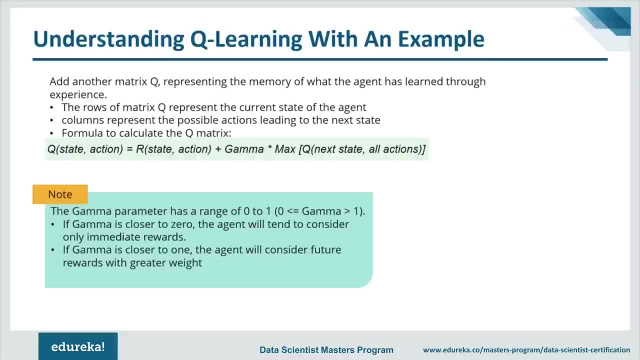 in order to get to the end goal. So, guys, this is what I was talking about when I mentioned exploitation and exploration. All right, so if the gamma value is closer to one, it basically means that you're actually exploring the entire environment and then choosing an optimum policy. 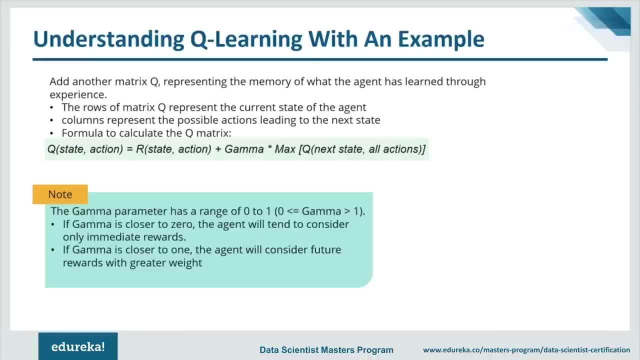 But if your gamma value is closer to zero, it means that the agent will only stick to a certain set of policies and it'll calculate the maximum reward based on those policies. Now, next, we have the Q learning algorithm that we're going to use to solve this problem. 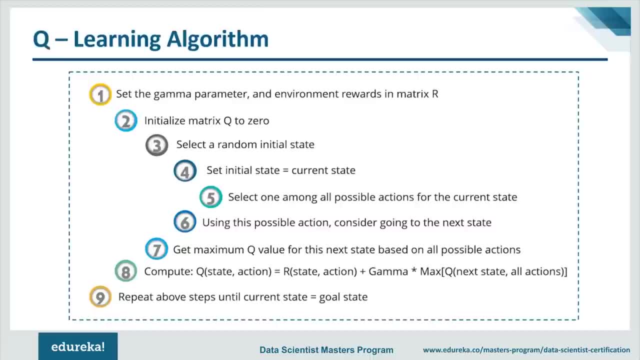 So, guys, now this is gonna look very confusing to y'all, So let me just explain this with an example. Okay, we'll see what we're actually going to run in our demo, We'll do the math behind it and then I'll tell you what this Q learning algorithm is. 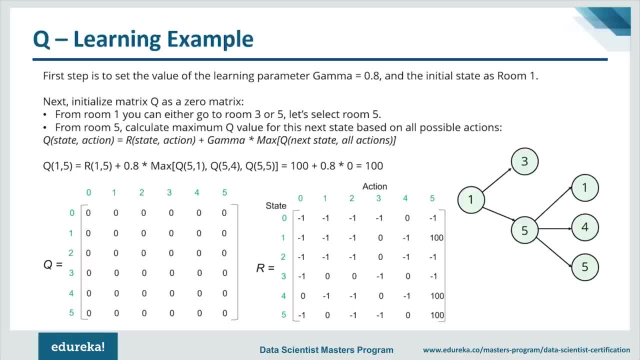 Okay, you'll understand it as I'm showing you the example. So, guys, in the Q learning algorithm, the agent learns from his experience. Okay, so each episode, which is basically when the agent starts traversing from an initial room to the end goal. 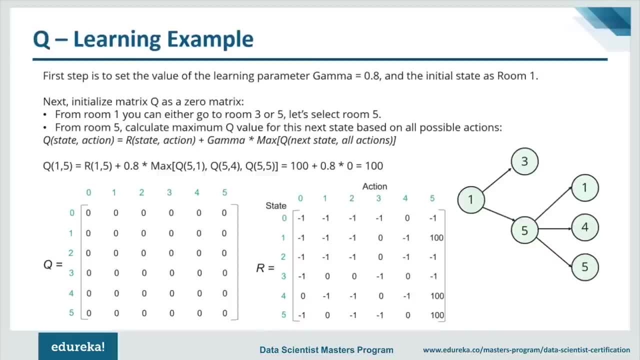 is equivalent to one training session, And in every training session the agent will explore the environment, it'll receive some reward until it reaches the goal state, which is five. So, guys, the purpose of training is to enhance the brain of our agent. 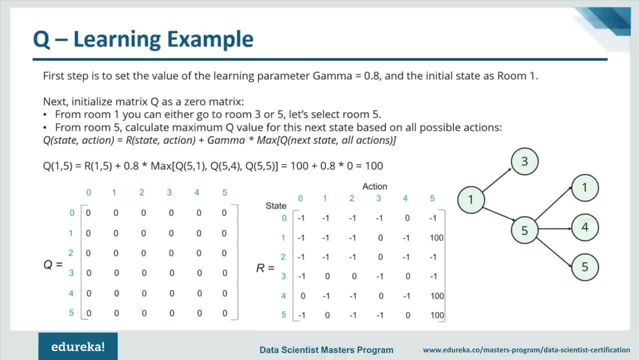 Okay, only if he knows the environment very well will he know which action to take. And this is why we calculate the Q matrix. Okay, in Q matrix, we're just going to calculate the value of traversing from every state to the end state. 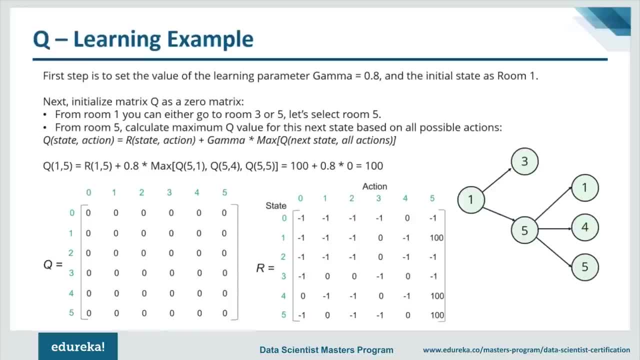 from every initial room to the end room. Okay, so when we calculate all the values, or how much reward we're getting from each policy that we take, we know the optimum policy that'll give us the maximum reward. Okay, that's why we have the Q matrix. 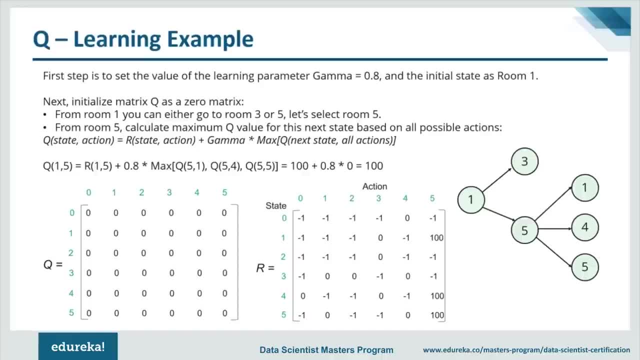 This is very important because the more you train the agent and the more optimum your output will be. So basically, here, the agent will not perform exploitation. Instead, he'll explore around and go back and forth through the different rooms and find the fastest route to the goal. 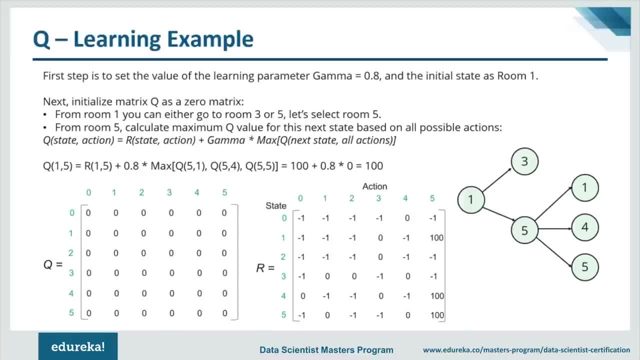 All right. now let's look at an example. Okay, let's see how the algorithm works. Okay, let's go back to the previous slide, And here it says that the first step is to set the gamma parameter. Okay, so let's do that. 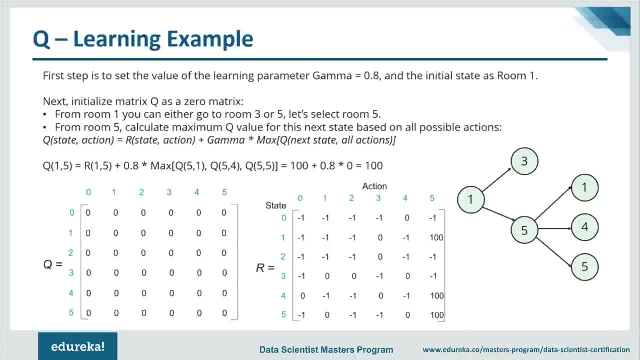 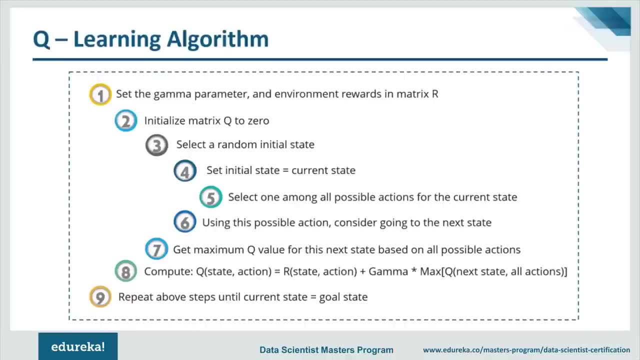 Now the first step is to set the value of the learning parameter, which is gamma, And we've randomly set it to 0.8.. Okay, the next step is to initialize the matrix Q to zero. Okay, so we've set matrix Q to zero over here. 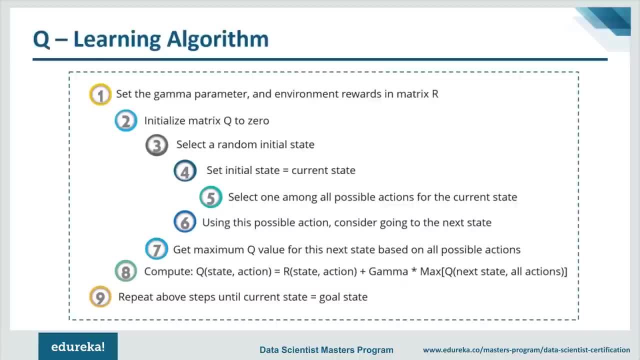 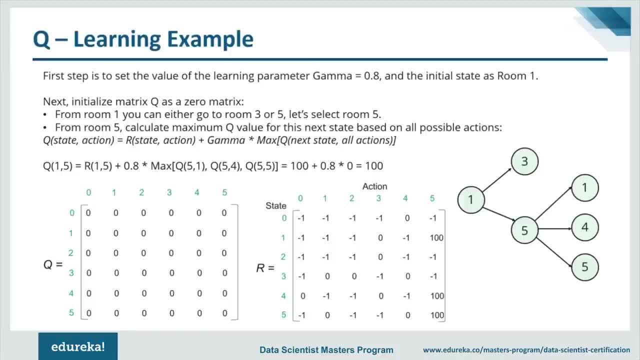 And then we'll select the initial stage. Okay. the third step is select a random initial state, And here we've selected the initial state as room number one. okay, So after you initialize the matrix Q as a zero matrix from room number one. 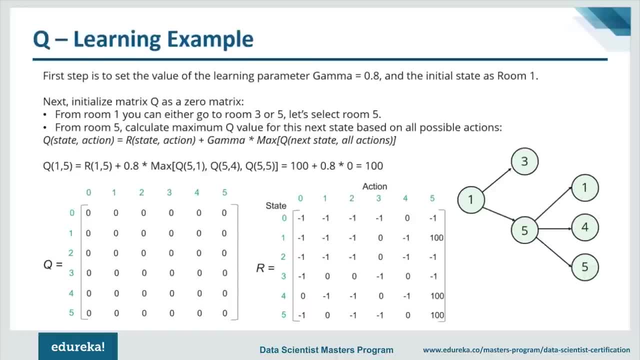 you can either go to room number three or room number five. So if you look at the reward matrix you can see that from room number one you can only go to room number three or room number five. The other values are minus one here. 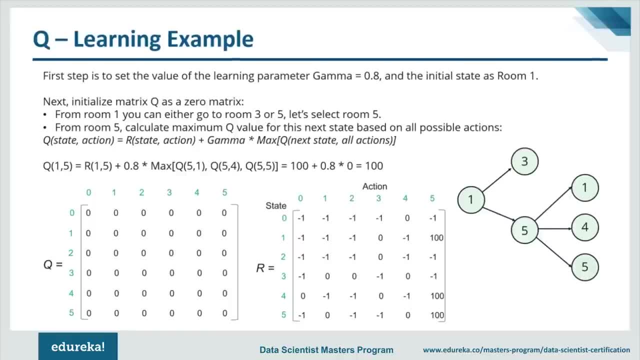 which means that there is no link from one to zero, one to one, one to two and one to four. So the only possible actions from room number one is to go to room number three and to go to room number five. all right, 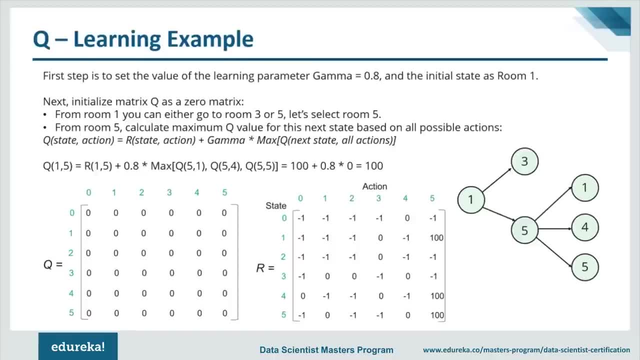 Okay, so let's select room number five. Okay, so from room number one, you can go to three and five, And we have randomly selected five. You can also select three, But, for example, let's select five over here. Now from room five, you're going to calculate. 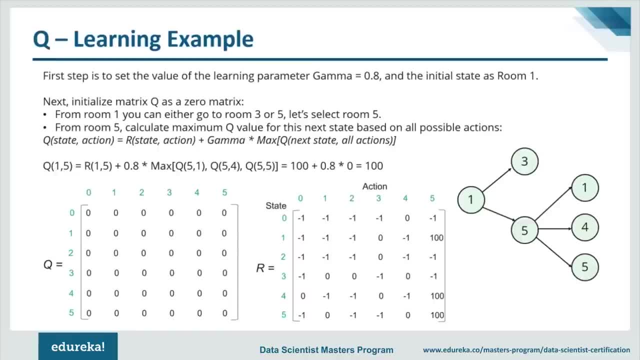 the maximum Q value for the next state based on all possible actions. So, from room number five, the next state can be room number one, four or five. So you're going to calculate the Q value for traversing five to one, five to four. 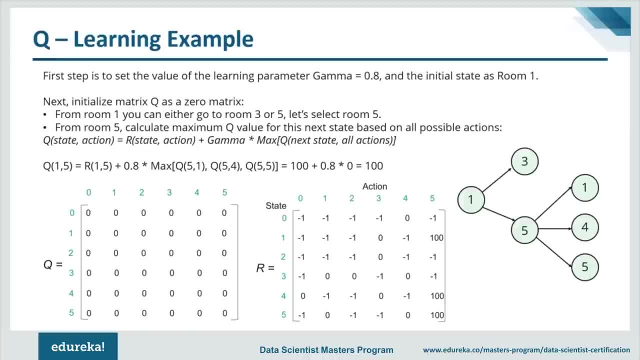 five to five and you're going to find out which has the maximum Q value, And that's how you're going to compute the Q value. So let's implement our formula. Okay, this is the Q learning formula. So right now we're traversing from room number one. 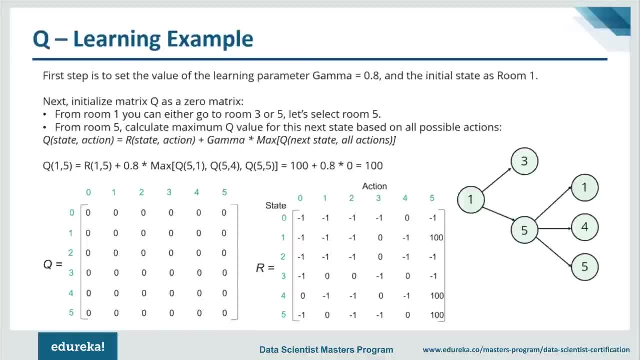 to room number five. Okay, this is our state. So here I've written Q, one comma five. Okay, one represents our current state, which is room number one. Okay, our initial state was room number one And we are traversing to room number five. 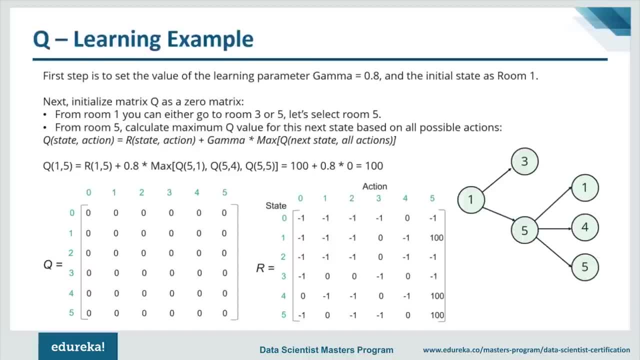 Okay, it's shown in this figure, room number five. Now for this we need to calculate the Q value. Next, in our formula it says reward matrix, state and action. So the reward matrix for one comma five. let's look at one comma five. 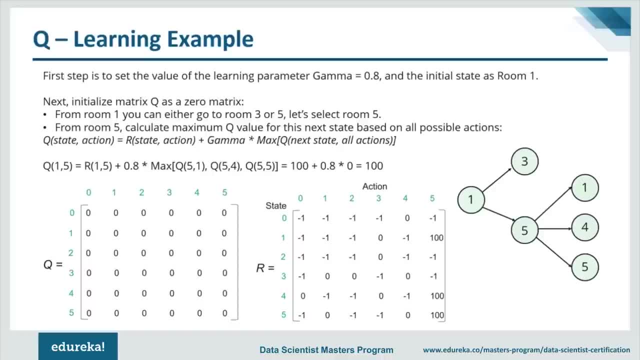 One comma five corresponds to 100.. Okay, so our reward over here will be 100.. So our one comma five is basically 100.. Then you're going to add the gamma value. Now, the gamma value, we've initialized it to 0.8.. 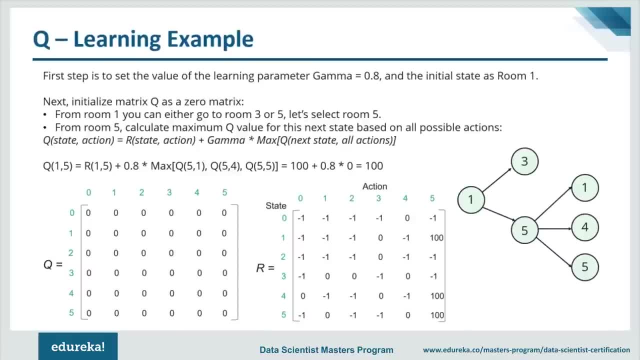 So that's what we've written over here, And we're going to multiply it with the maximum value that we're going to get for the next state, based on all possible actions. Okay, so from five, the next state is one, four and five. 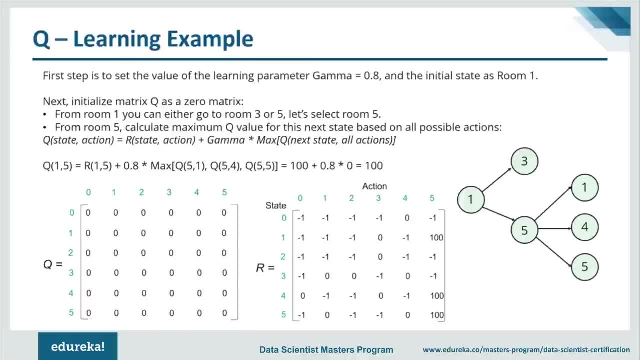 So if you traverse from five to one- that's what I've written over here- Five to four, you're going to calculate the Q value of five to four and five to five. Okay, that's what I mentioned over here. So Q five, comma one. 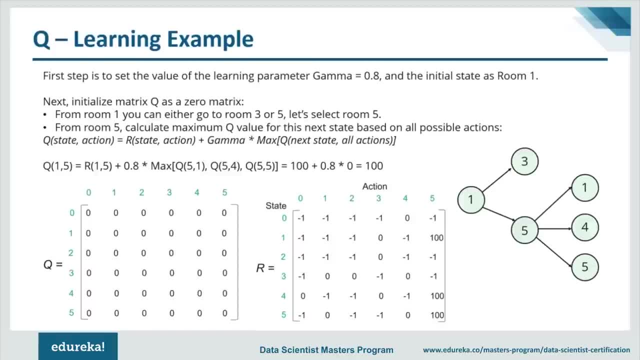 five comma four and five comma five are the next possible actions that you can take from state five. So our one comma five is 100.. Okay, because from the reward matrix you can see that one comma five is 100.. Zero comma five is 100.. 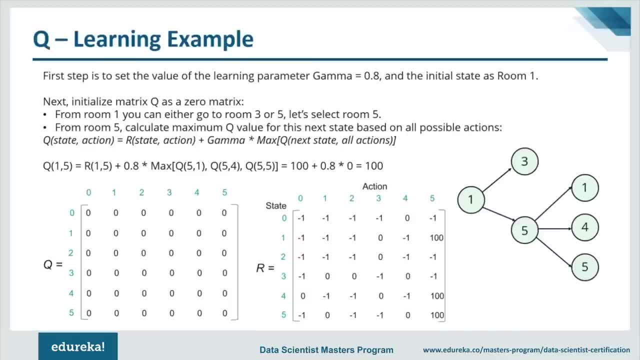 Zero. point eight is the value of gamma. After that we'll calculate Q of five comma one, five comma four and five comma five. Like I mentioned earlier that we're going to initialize matrix Q as zero matrix, So we're setting the value as zero. 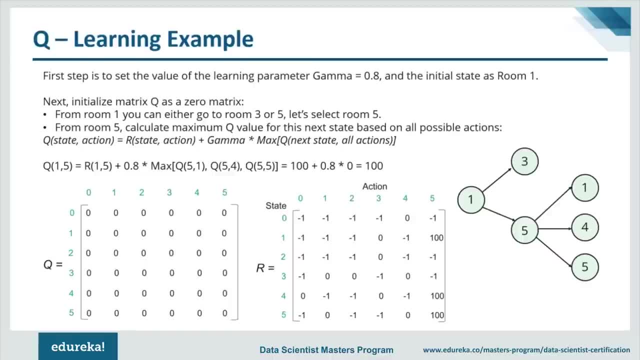 because initially, obviously, the agent doesn't have any memory of what is happening. Okay, so he's just starting from scratch. That's why all these values are zero. So Q of five comma one will obviously be zero. Five comma four will be zero. 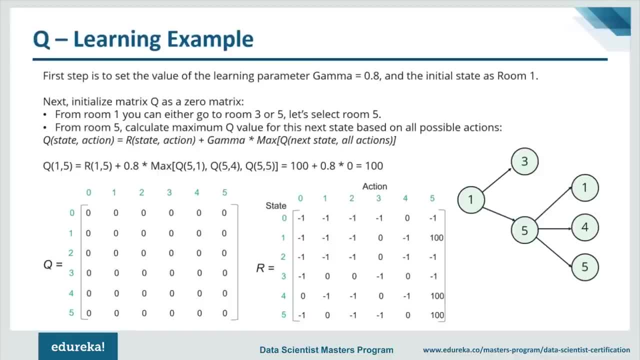 and five comma five will also be zero, And to find out the maximum between these, it's obvious that it's obviously zero. So when you compute this equation you'll get 100.. So the Q value of one comma five is 100. 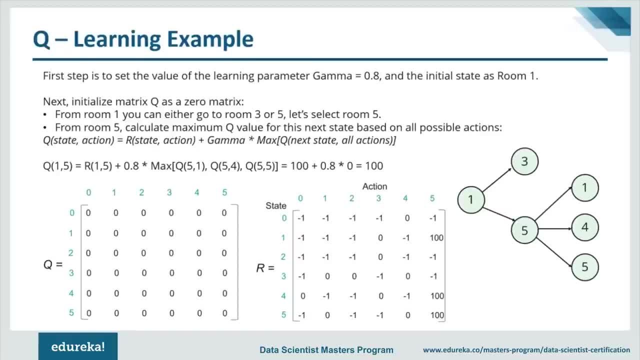 So if our agent goes from room number one to room number five, he's going to have a maximum reward or Q value of 100.. All right, Now in the next slide you can see that I've updated the value of Q of one comma five. 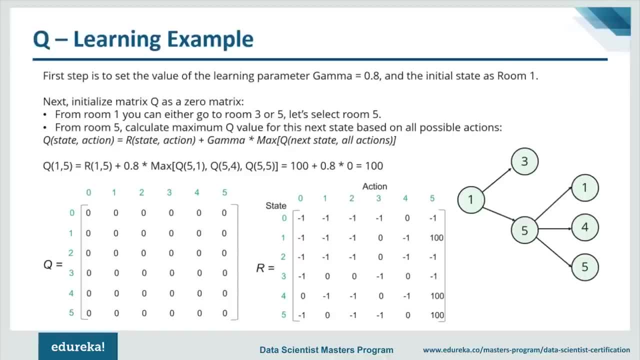 Okay, it's set to 100.. All right Now. similarly, let's look at another example so that you understand this better. So, guys, this is exactly what we're going to do in our demo. We're only going to be coded. 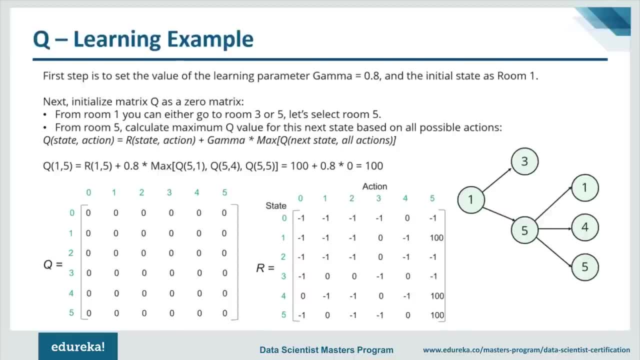 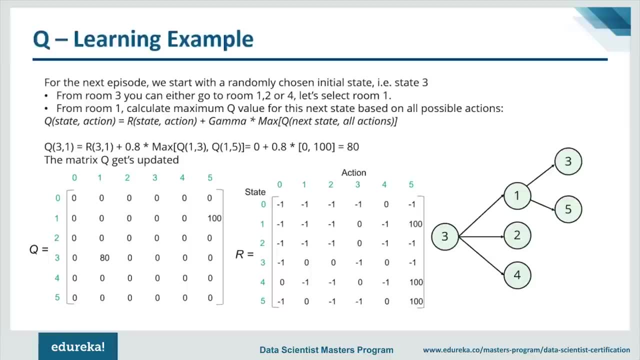 Okay, I'm just explaining our code right now. I'm just telling you the math behind it. All right, Now let's look at another example. Okay, This time we'll start with a randomly chosen initial state. Let's say that we've chosen state three. 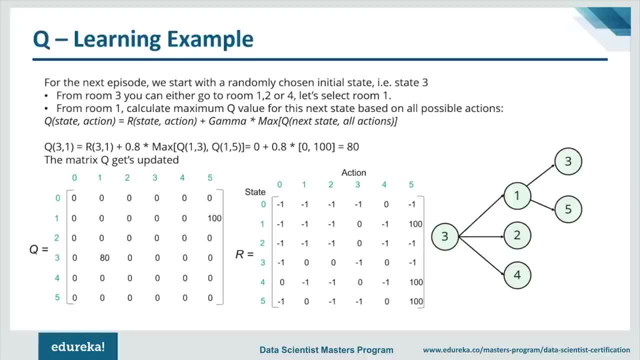 Okay, So from room three you can either go to room number one, two or four Randomly. we'll select room number one And from room number one you're going to calculate the maximum Q value for the next state, based on all possible actions. 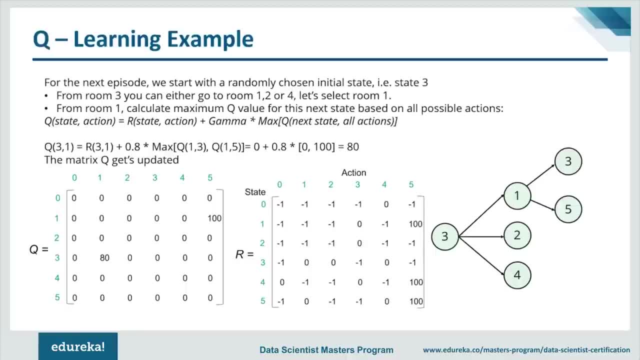 So the possible actions from one is to go to three and to go to five. Now, if you calculate the Q value using this formula, so let me explain this to you once again Now. Q three comma one basically represents that we're in room number three. 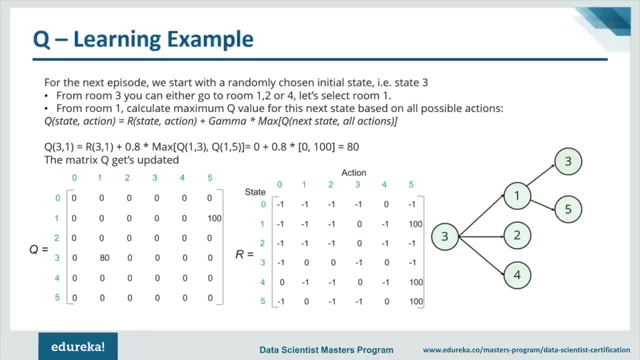 and we're going to room number one. Okay, So this represents our action. Okay, So we're going from three to one, which is our action, and three is our current state. Next, you'll look at the reward of going from three to one. 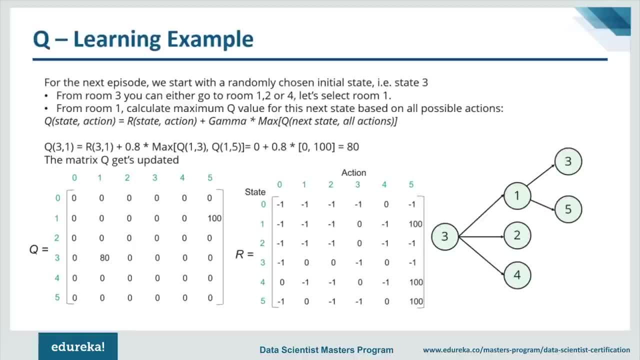 Okay, If you go to the reward matrix, three comma one is zero. Okay, Now we have a direct link between three and five. Okay, So that's why the reward here is zero. So the value here will be zero After that. 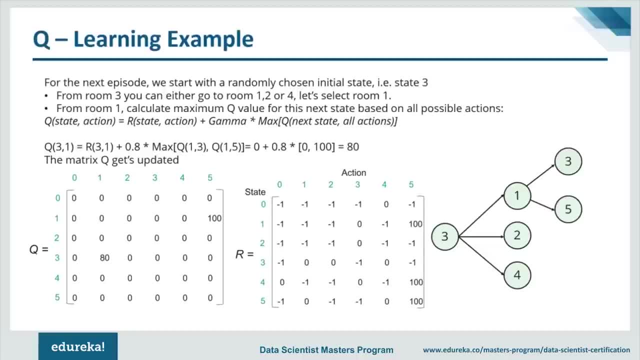 we have a gamma value which is 0.8.. And then we're going to calculate the Q max of one comma three and one comma five. Out of these, whichever has the maximum value, we're going to use that Okay. 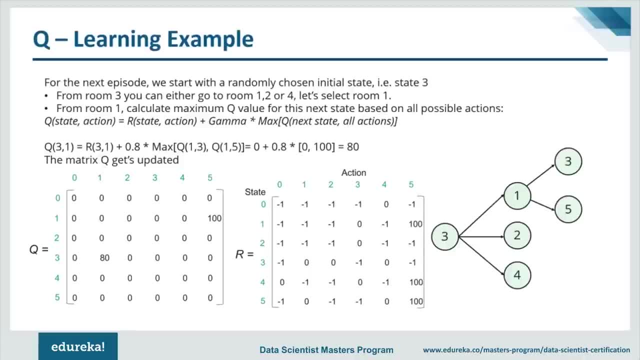 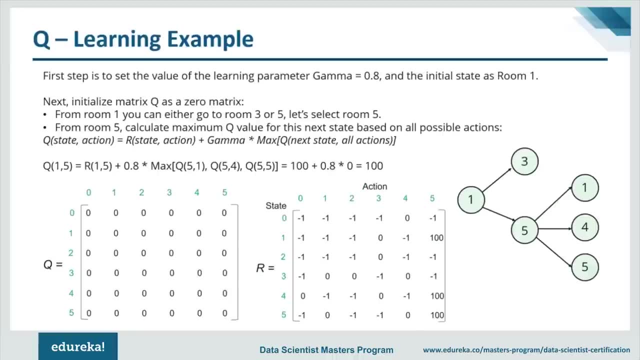 So Q of one comma three is zero. All right, It's zero. You can see here one comma three is zero and one comma five. If you remember, we just calculated one comma five in the previous slide. Okay, So here I'm going to put 100. 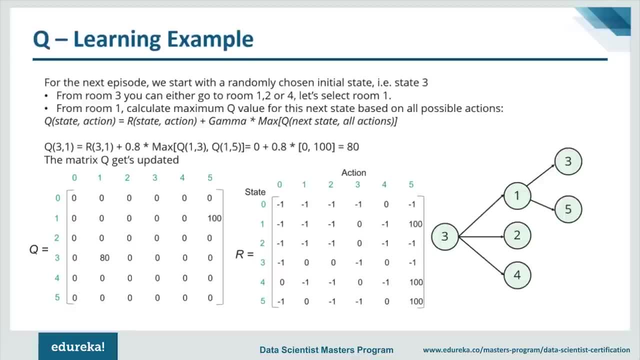 So the maximum here is 100.. So 0.8 into 100 will give us 80.. So that's the Q value we're going to get if you traverse from three to one. Okay, I hope that was clear. So now we've traversed from room number three. 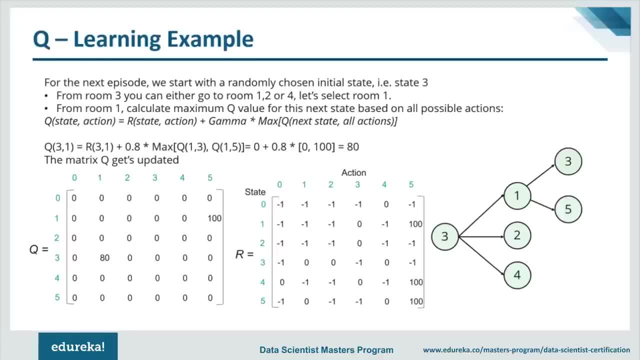 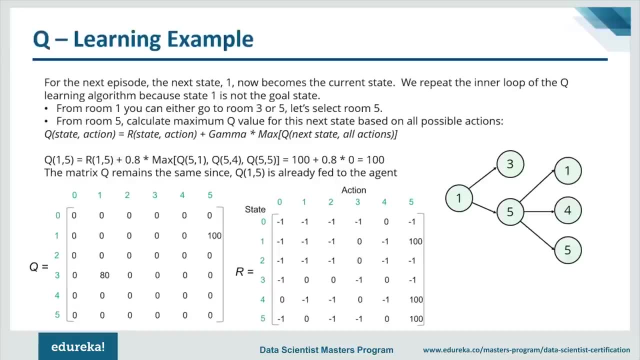 to room number one with a reward of 80.. Okay, But we still haven't reached the end goal, which is room number five. So for our next episode, the state will be room number one. So, guys, like I said, we'll repeat this inner loop. 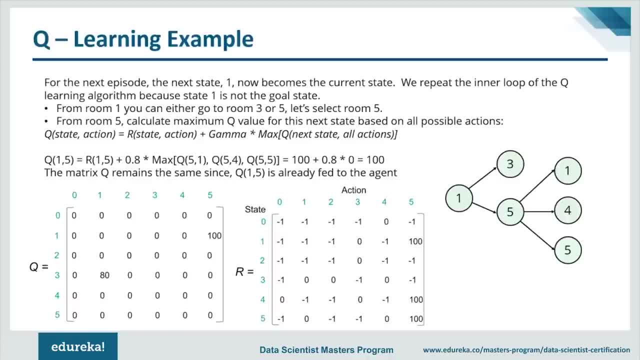 because room number one is not our end goal. Okay, Our end goal is room number five. So now we need to figure out how to get from room number one to room number five. So from room number one you can either go to three or five. 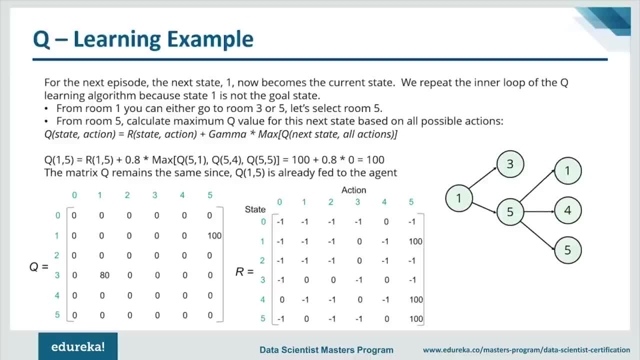 That's what I've drawn over here. So if we select five, we know that is our end goal. Okay, So from room number five, then you have to calculate the maximum Q value for the next possible actions. So the next possible actions from five. 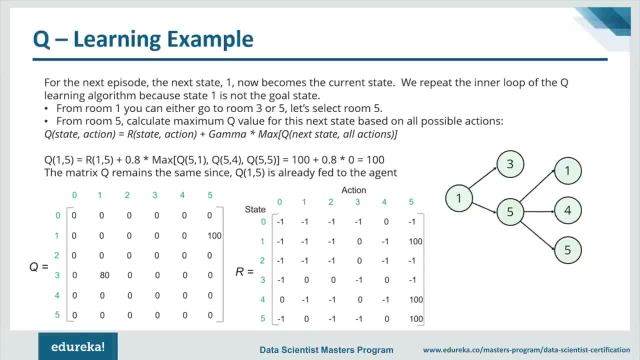 is to go to room number one, room number four or room number five. So you're going to calculate the Q value of five to one, five to four and 5 to 5 and find out which is the maximum Q value here. 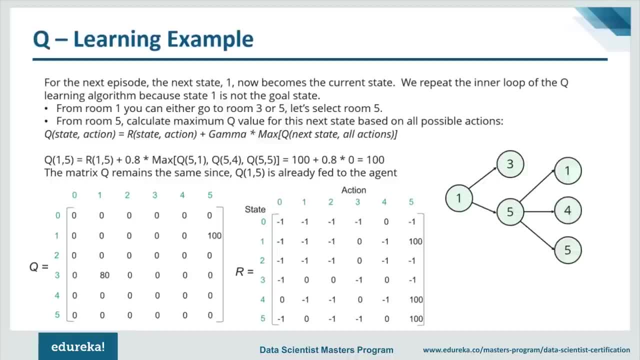 and you're going to use that value. All right, So let's look at the formula now. Now again, we're in room number 1 and we want to go to room number 5.. Okay, so that's exactly what I've written here: Q 1, 5.. 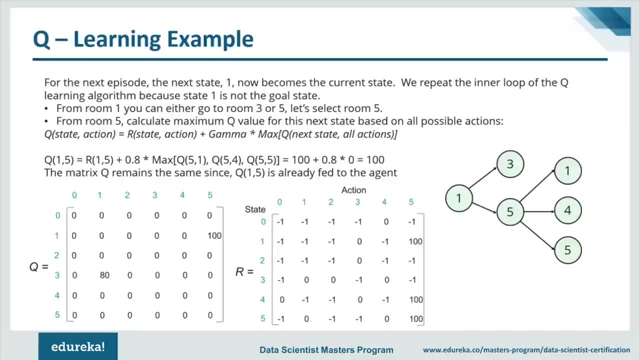 Next is the reward matrix, So reward of 1, 5, which is 100.. All right, then we've added the gamma value, which is 0.8, and then we're going to find the maximum Q value from 5 to 1,, 5 to 4 and 5 to 5.. 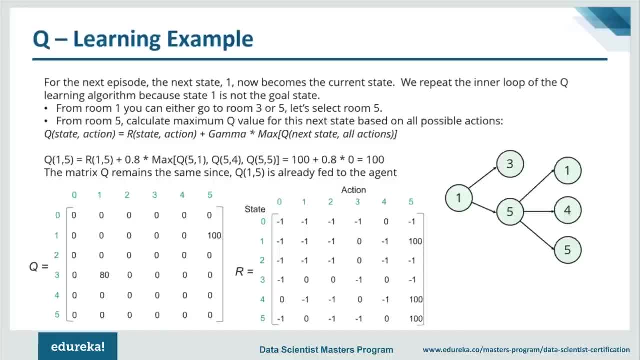 So this is what we're performing over here. So 5, 1, 5, 4 and 5, 5 are all 0. This is because we initially set all the values of the Q matrix as 0. So you get a 100 over here. 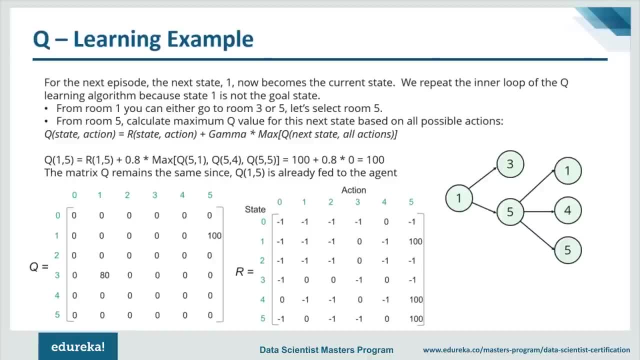 and the matrix remains the same, because we already had calculated Q 1, 5.. So the value of 1, 5 is already fed to the agent. So when he comes back here he knows that, okay, he's already done this before. 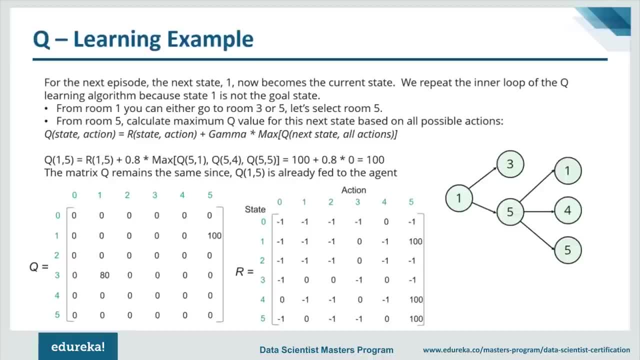 Now he's going to try and implement another method. Okay, he's going to try and take another route or another policy. So he's going to try to go from different rooms and finally land up in room number 5.. So, guys, this is exactly how our code runs. 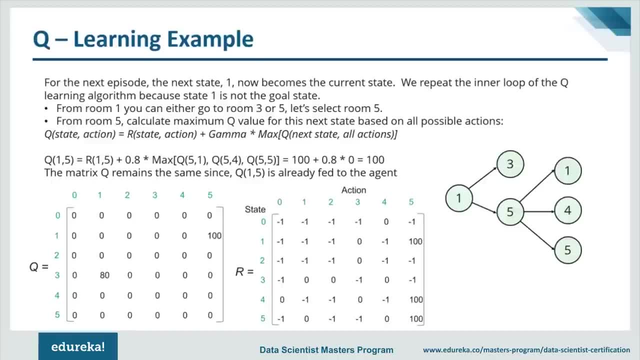 We're going to traverse through each and every node because we want an optimum policy. Okay, an optimum policy is attained only when you traverse through all possible actions. Okay, so if you go through all possible actions that you can perform, only then will you understand which is the best action. 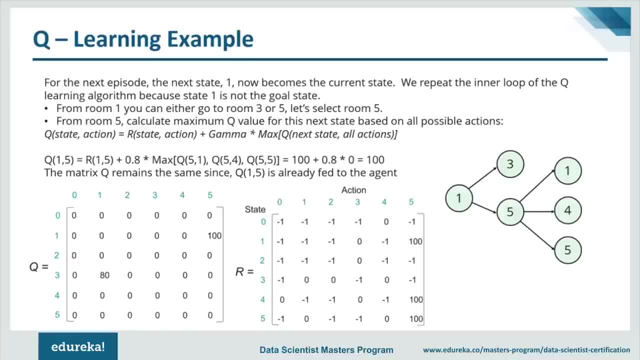 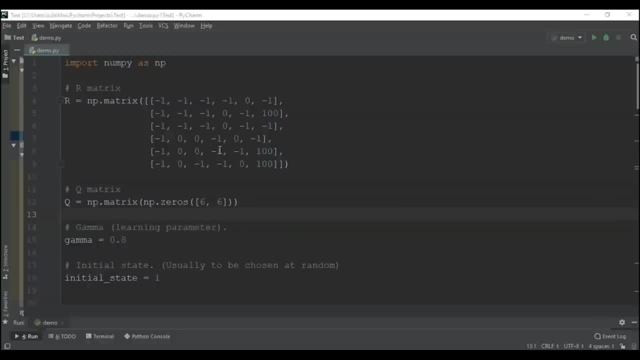 which will lead us to the reward. I hope this is clear. Now let's move on and look at our code. So, guys, this is our code and this is executed in Python, and I'm assuming that all of you have a good background in Python. 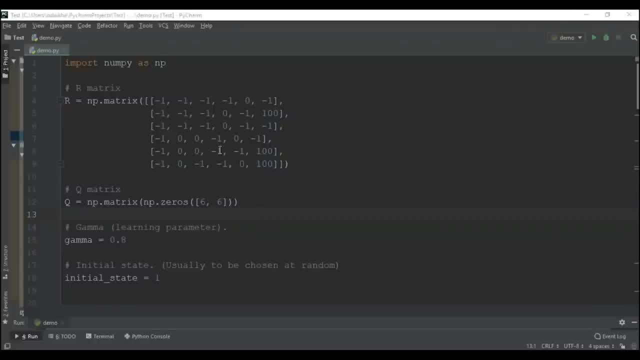 Okay, if you don't understand Python very well, I'm going to leave a link in the description. You can check out that video on Python and then maybe come back to this later. Okay, but I'll be explaining the code to you anyway. 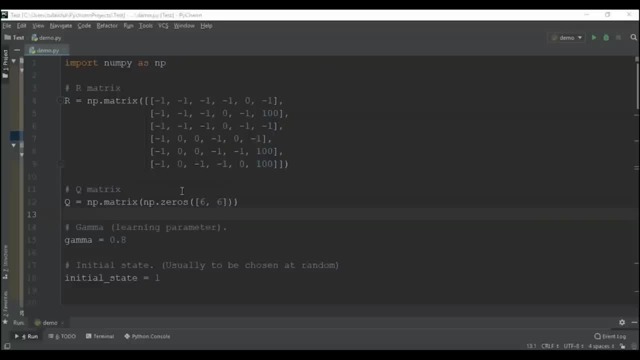 but I'm not going to spend a lot of time explaining each and every line of code, because I'm assuming that you know Python, Okay, so let's look at the first line of code over here. So what we're going to do is we're going to import NumPy. 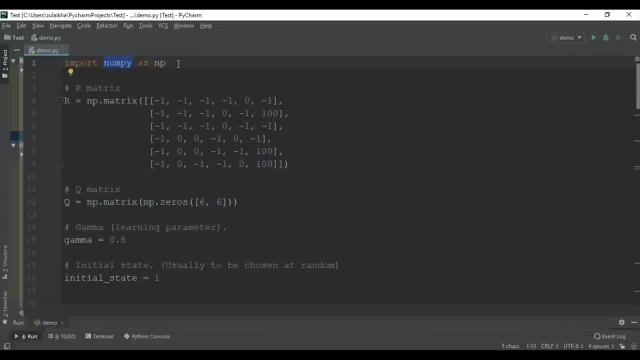 Okay, NumPy is basically a Python library for adding support for large multidimensional arrays and matrices, and it's basically for computing mathematical functions. Okay, so first we're going to import that, After that we're going to create the R matrix. 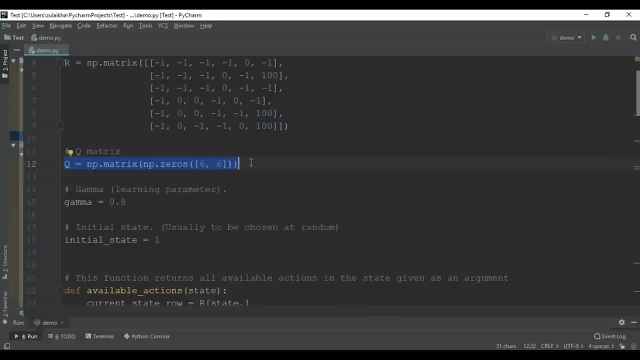 Okay, so this is the R matrix. Next, we're going to create a Q matrix and it's a six into six matrix, because obviously we have six states, starting from zero to five. Okay, and we're going to initialize the value to zero. 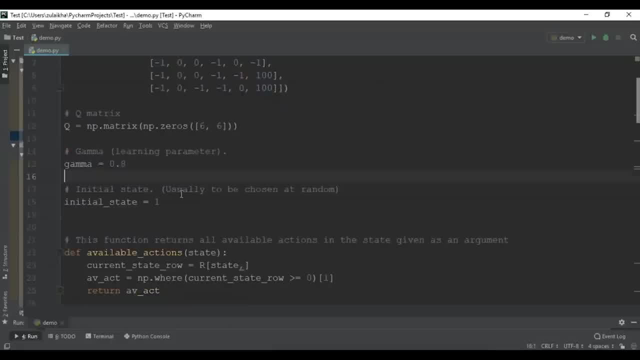 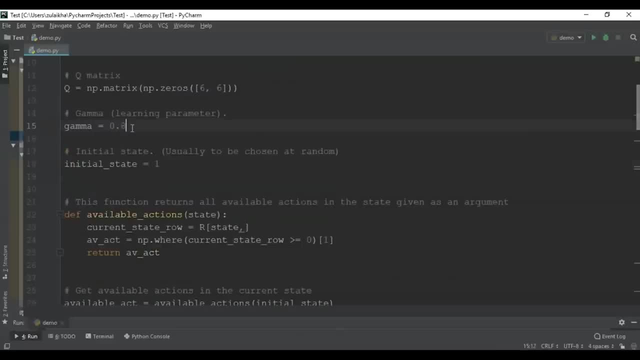 So, basically, the Q matrix is going to be initialized to zero over here, All right. after that we're setting the gamma parameter to 0.8.. So, guys, you can play with this parameter and, you know, move it to 0.9. 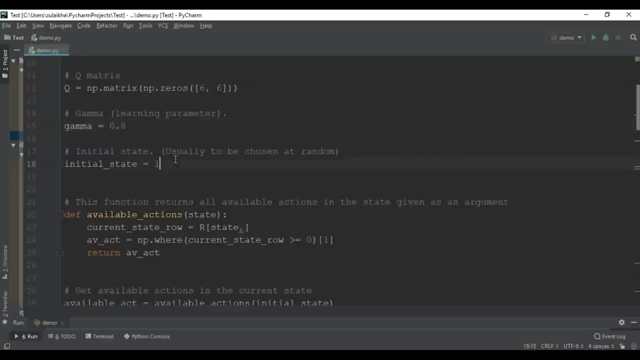 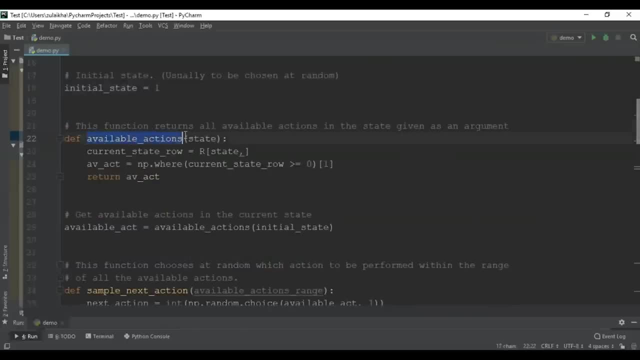 or move it lower to 0.8.. Okay, you can see what happens then. Then we'll set an initial stage. Okay, initial stage is set as one. After that we're defining a function called available actions. Okay, so basically, what we're doing here is: 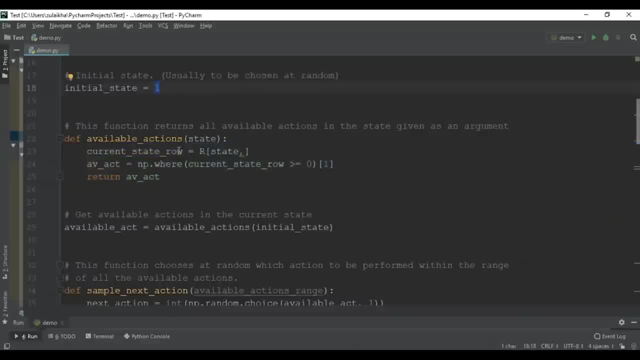 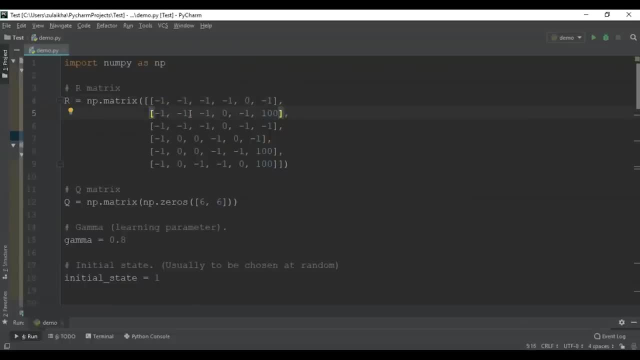 since our initial state is one, we're going to check our row number one. Okay, this is our row number one. Okay, this is row number zero, This is row number one, and so on. So we're going to check the row number one. 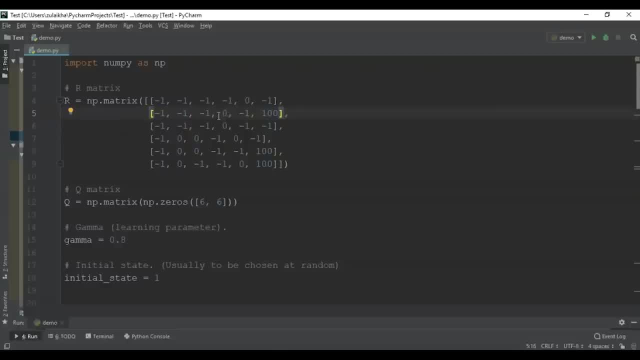 and we're going to find the values which are greater than or equal to zero, because these values basically represent the nodes that we can travel to. Now, if you select minus one, you can't traverse to minus one. Okay, I explained this earlier. 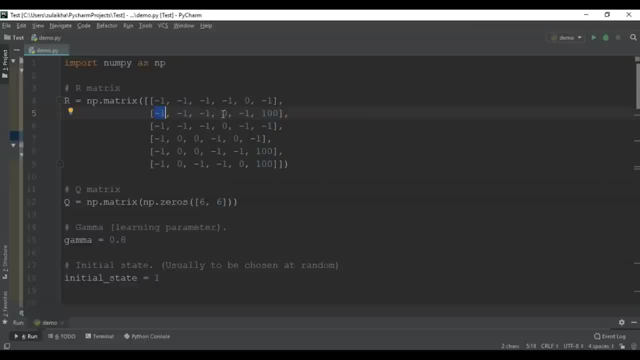 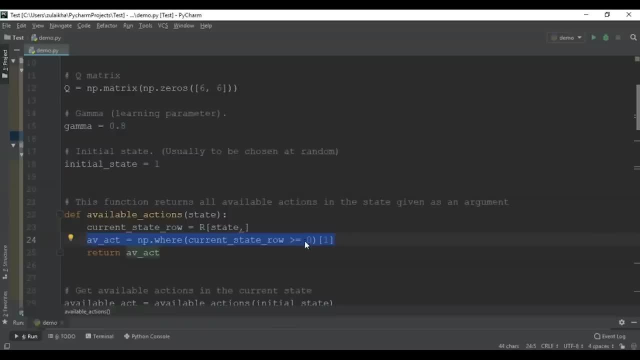 The minus one represents all the nodes that we can't travel to, but we can travel to these nodes, Okay. so basically, over here we're checking all the values which are equal to zero or greater than zero. These will be our available actions. 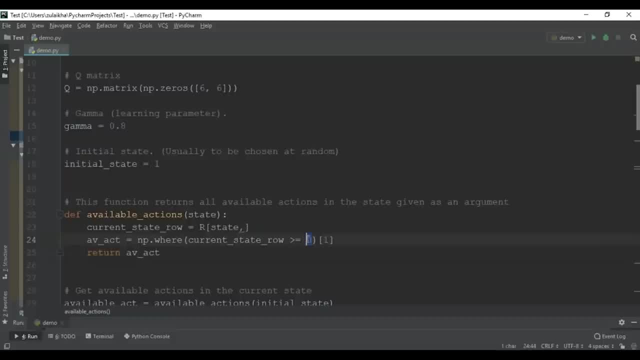 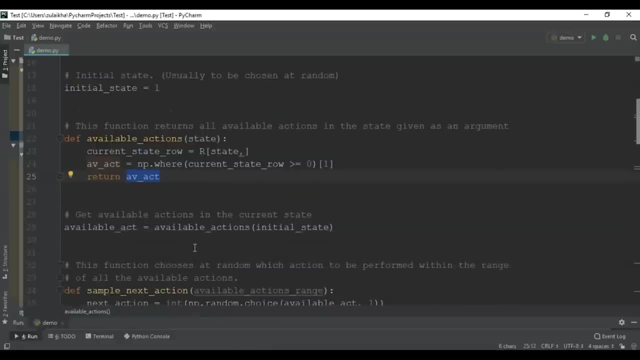 So if our initial state is one, we can travel to other states whose value is equal to zero or greater than zero, And this is stored in this variable called available act. All right now, this will basically get the available actions in the current state. 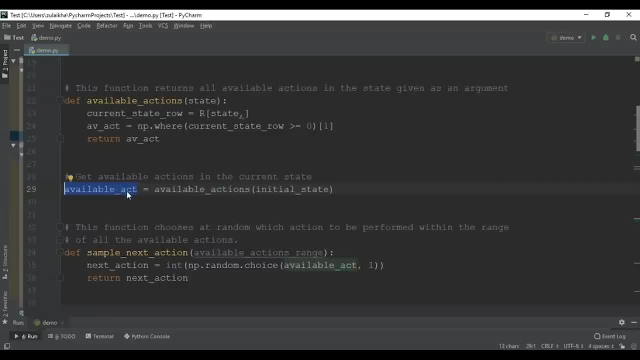 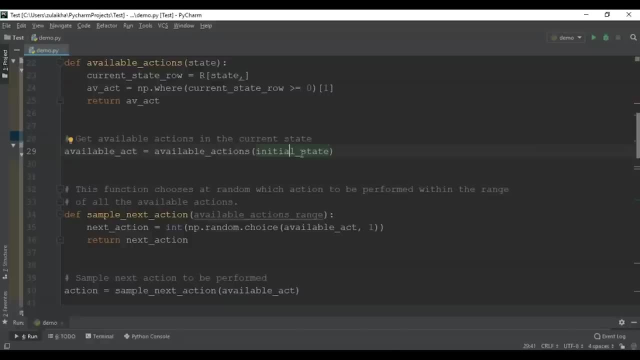 Okay, so we're just storing the possible actions in this available act variable over here. So basically over here, since our initial state is one we're going to find out, the next possible states we can go to. Okay, that is stored in the. 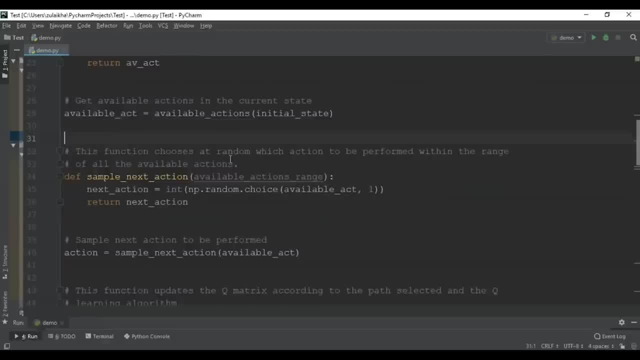 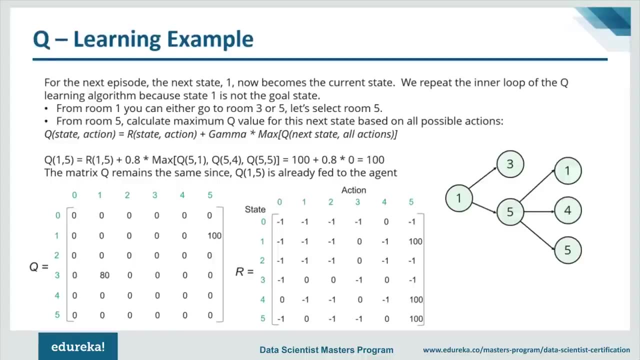 the available act variable. Now, next is this function chooses at random which action to be performed within the range, So if you remember over here. so, guys, initially we are in stage number one. Okay, our available actions is to go to stage number three. 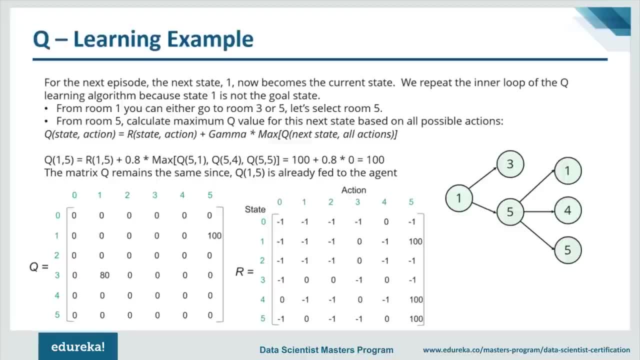 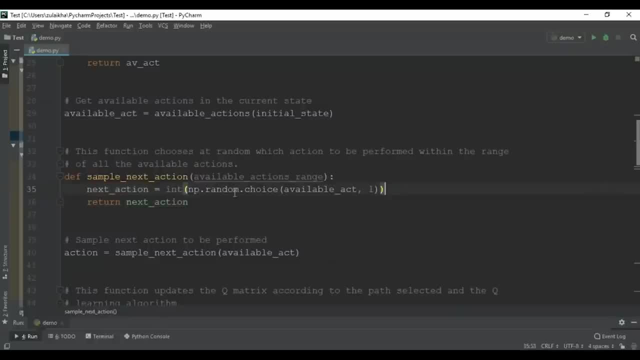 or stage number five, Sorry, room number three or room number five. Okay, now, randomly, we need to choose one room, So for that we're using this line of code: Okay, so here we're randomly going to choose one of the actions from the available act. 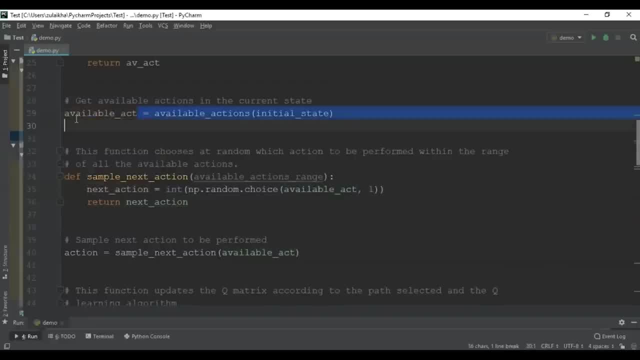 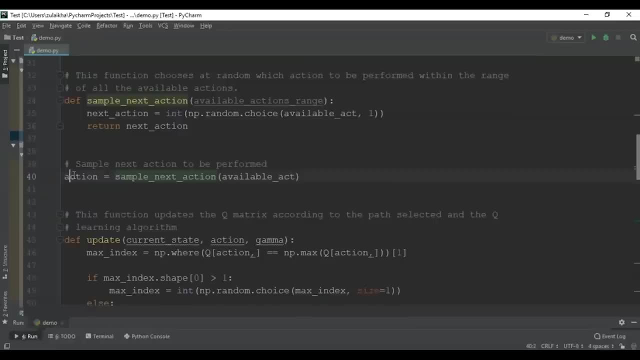 This available act, like I said earlier, stores all our possible actions Okay, from the initial state Okay. so once it chooses an action, it's going to store it in next action. So, guys, this action will represent the next available action to take. 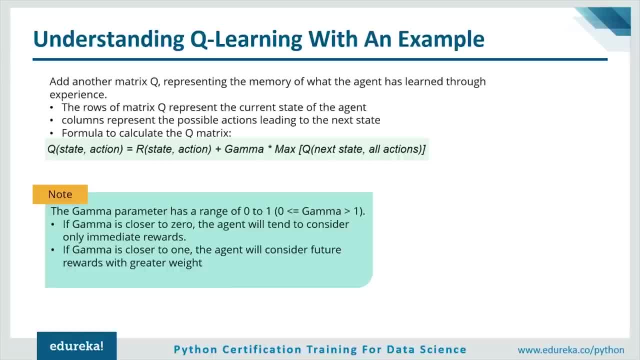 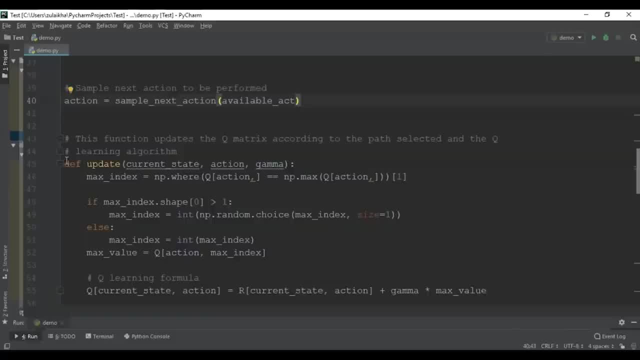 Now, next is our Q matrix. Remember this formula that we used? So, guys, this formula that we use is what we're going to calculate in the next few lines of code. So, in this block of code, we're just executing and computing the value of Q. 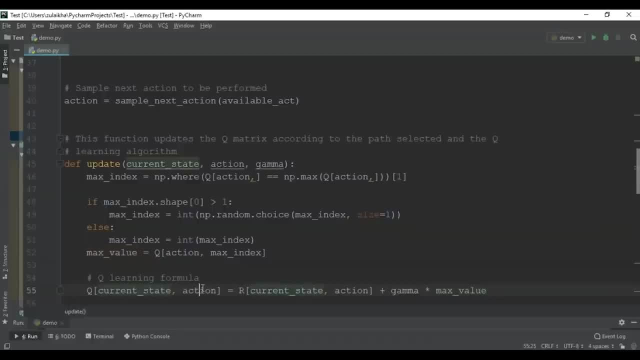 Okay, this is our formula for computing the value of Q- Current state comma action, our current state comma action- gamma- into the maximum value. So here, basically, we're going to calculate the maximum index, meaning that we're going to check which of the possible actions 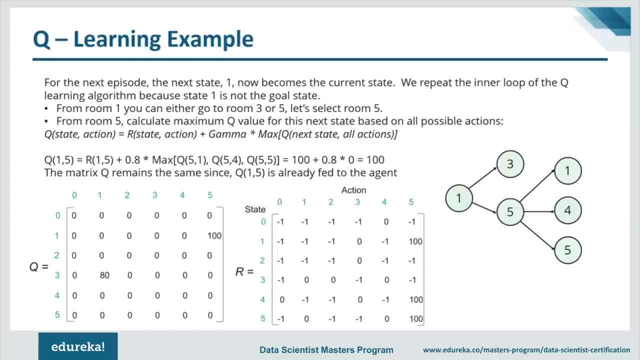 will give us the maximum Q value. All right, if you remember in our explanation over here, this value over here: max Q of five comma one, five comma four and five comma five. we had to choose a maximum Q value that we get from these three. 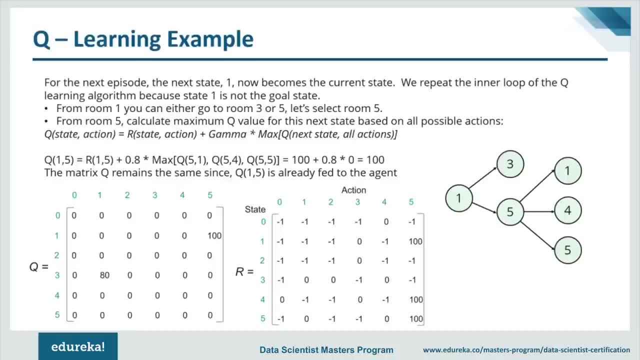 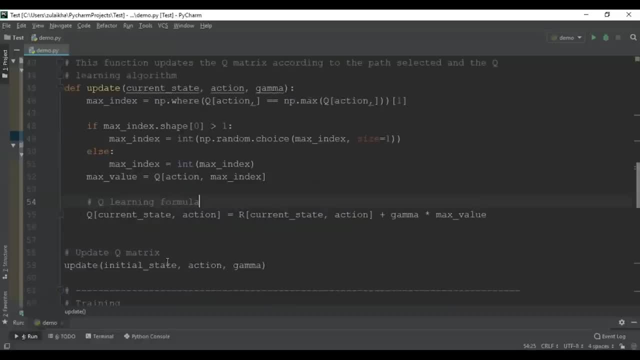 So basically, that's exactly what we're doing in this line of code: We're calculating the index which gives us the maximum value. After we finish computing the value of Q, we'll just have to update our matrix. After that, we'll be updating the Q value. 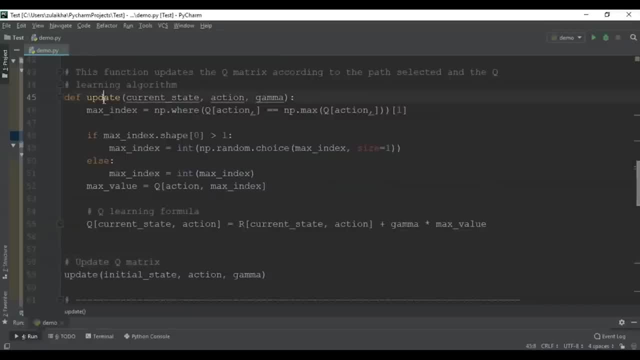 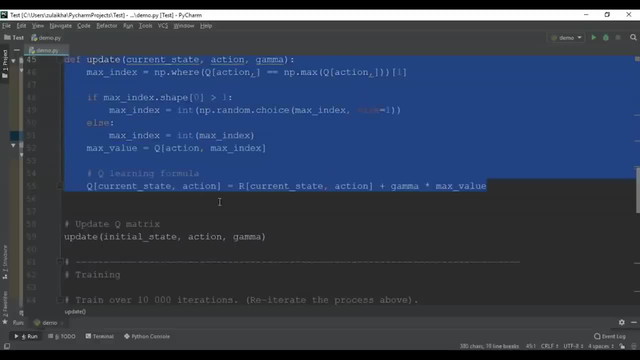 and we'll be choosing a new initial state. Okay, so this is the update function that is defined over here. Okay, so I've just called the function over here. So, guys, this whole set of code will just calculate the Q value. 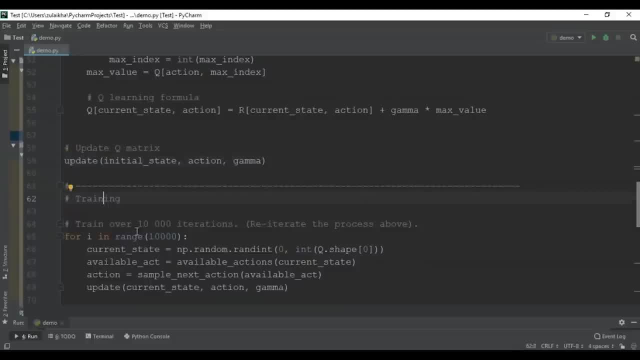 Okay, this is exactly what we did in our examples. After that we have the training phase. So, guys remember, the more you train an algorithm, the better it's going to learn. Okay, so over here I've provided around 10,000 iterations. 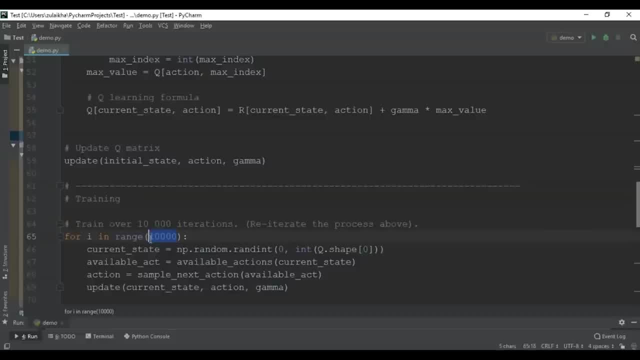 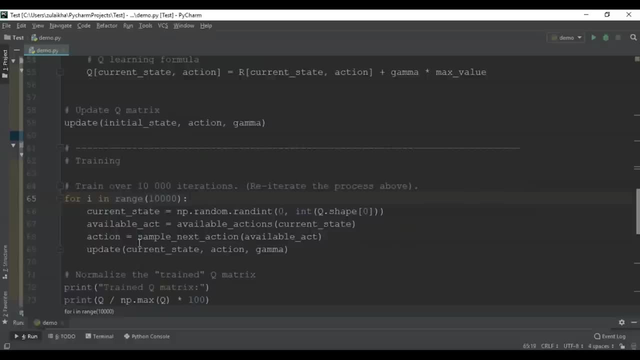 Okay, so my range is 10,000 iterations, meaning that my agent will take 10,000 possible scenarios and it'll go through 10,000 iterations to find out the best policy. So here, exactly what I'm doing is I'm choosing the current state randomly. 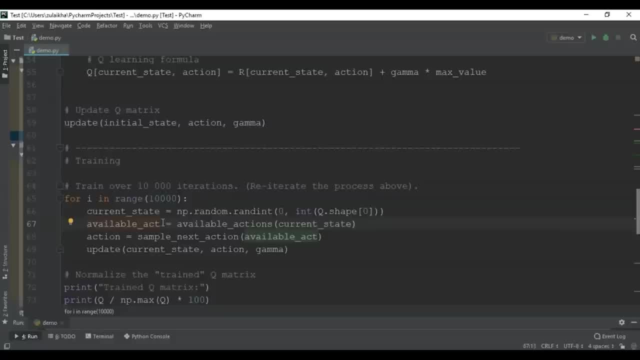 After that I'm choosing the available action from the current state, So either I can go to stage three or state five. Then I'm calculating the next action and then I'm finally updating the value in the Q matrix And next we just normalize the Q matrix. 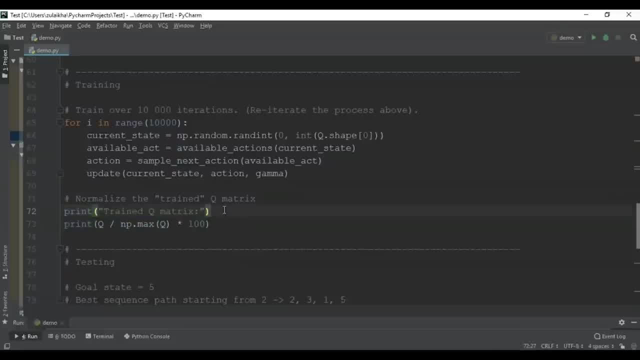 So sometimes in our Q matrix the value might exceed- Okay, let's say it exceeded to 500, 600. So that time you want to normalize the matrix, Okay, we want to bring it down a little bit. Okay, because larger numbers 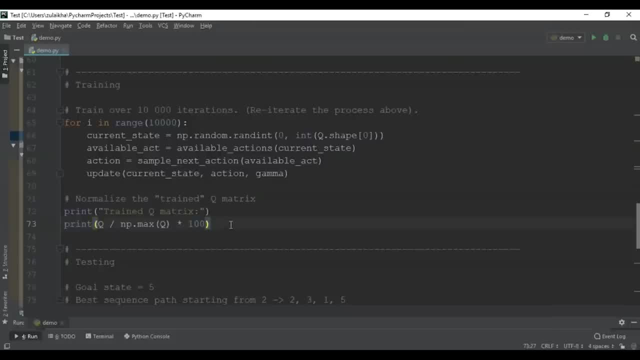 we won't be able to understand And computation will be very hard on larger numbers. That's why we perform normalization. You're taking your calculated value and you're dividing it with the maximum Q value into 100, all right, So you're normalizing it over here. 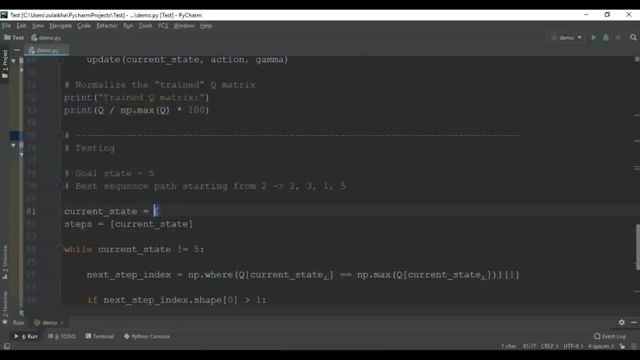 So, guys, this is the testing phase. Okay, here you'll just randomly set a current state and you won't give in any other data, because you've already trained a model. Okay, you're going to give a current state, Then you're going to tell your agent that. 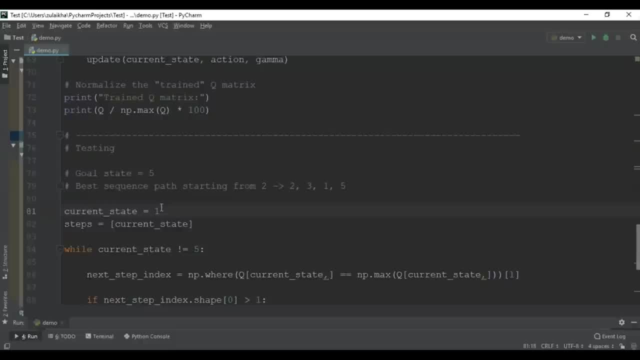 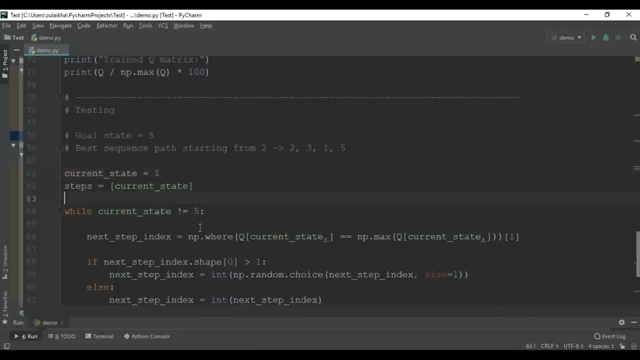 listen, you're in room number one. Now you need to go to room number five. Okay, so he has to figure out how to go to room number five, because we've trained him now. all right, So here we've set the current state to one. 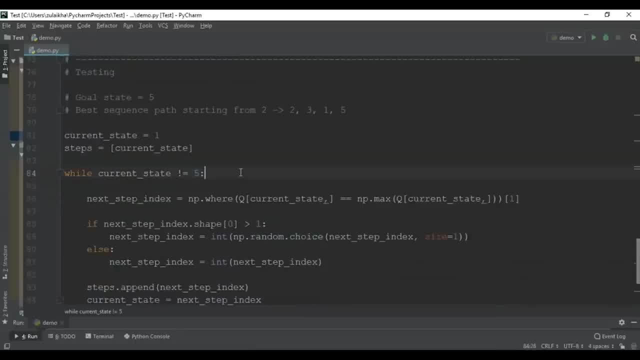 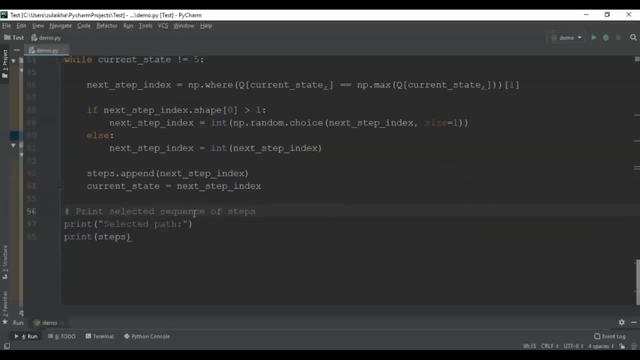 and we need to make sure that it's not equal to five, because five is the end End goal. So, guys, this is the same loop that we executed earlier, So we're going to do the same iterations again. Now, if I run this entire code, let's look at the result. 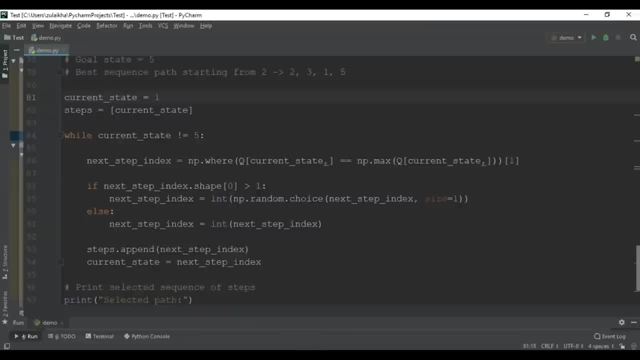 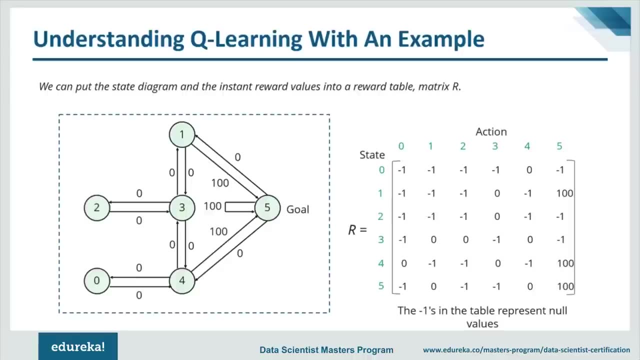 So our current state here we've chosen as one: Okay, and if we go back to our matrix, you can see that there is a direct link from one to five, which means that the route that the agent should take is one to five. 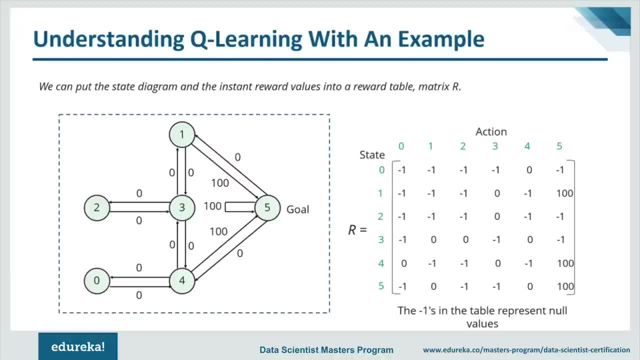 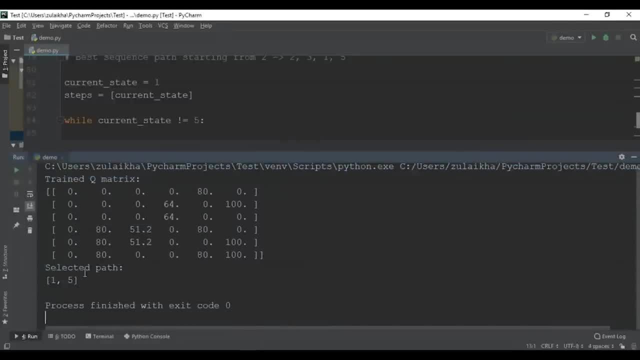 Okay, directly it should go from one to five, because it'll get the maximum reward, like that. Okay, let's see if that's happening. So, if I run this, it should give me a direct path from one to five. Okay, that's exactly what happened. 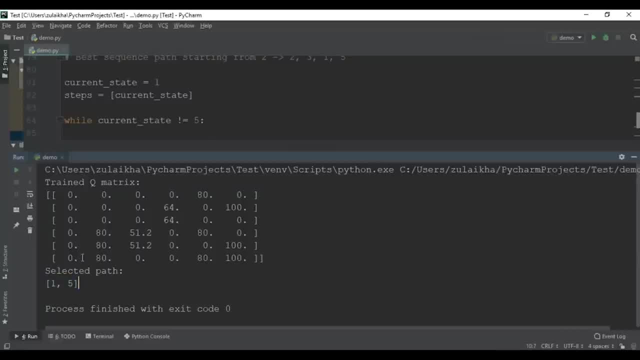 So this is the selected path. So directly from one to five it went, and it calculated the entire queue matrix for me. So, guys, this is exactly how it works. Now let's try to set the initial stage as, let's say, two. 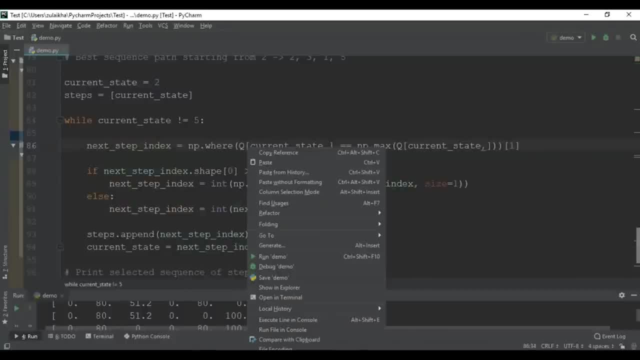 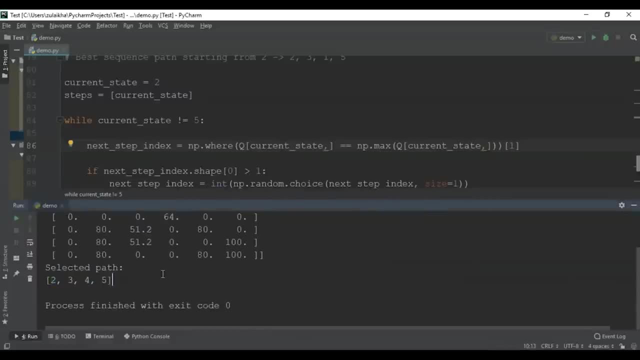 So if I set the initial stage as two and if I try to run the code, let's see the path that it gives. So the selected path is two, three, four, five. Now it chose this path because it's giving us the maximum reward from this path. 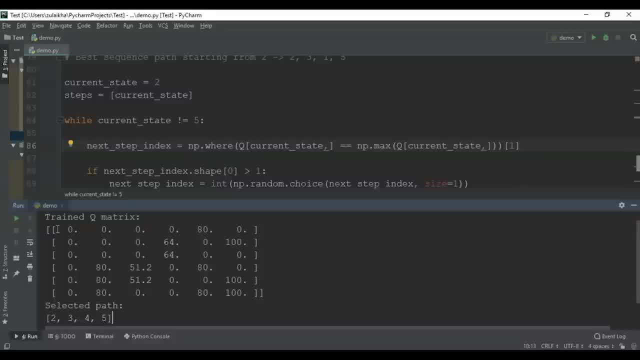 Okay, this is the queue matrix that it calculated and this is the selected path. All right, so, guys, with this we come to the end of this demo. So, basically, what we did was we just placed an agent in a room- random room- and we asked it to traverse through. 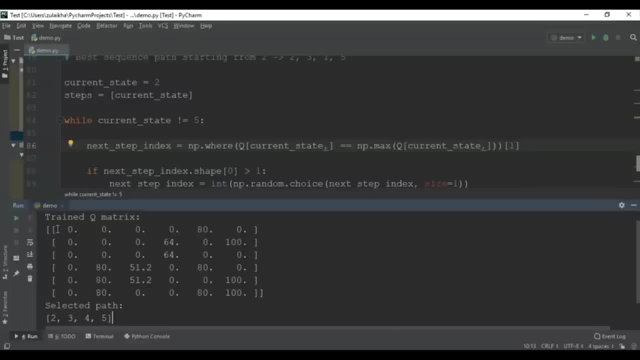 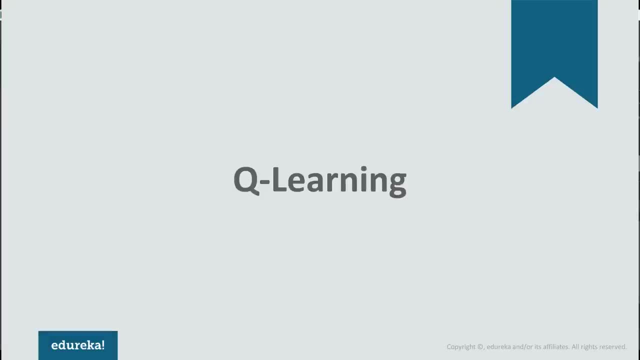 and reach to the end room, which is room number five. So, basically, we trained our agent and we made sure that it went through all the possible paths to calculate the best path. Now, for a robot, an environment is a place where it has been put to use. 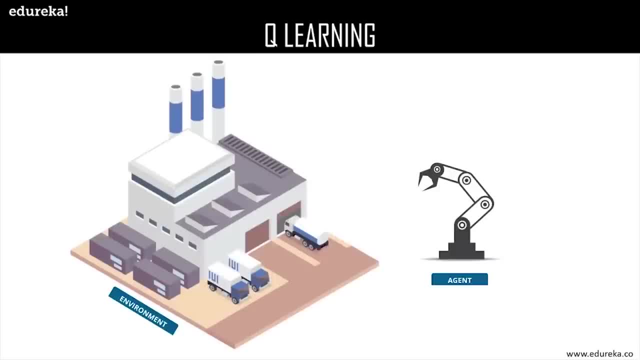 Now remember, this robot is itself the agent. For example, an automobile factory where a robot is used to move materials from one place to another. Now, the task we discussed just now have a property in common. Now, these tasks involve an environment. 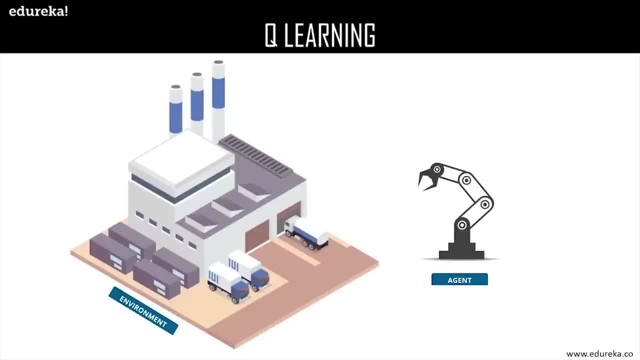 and expect the agent to learn from the environment. Now this is where traditional machine learning fails, and hence the need for reinforcement learning. Now it is good to have an established overview of the problem that is to be solved using the queue learning or the reinforcement learning. 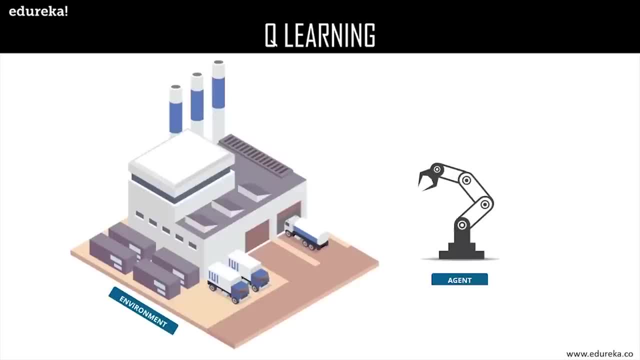 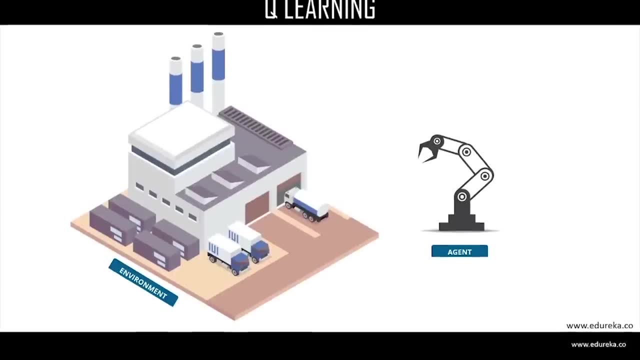 So it helps to define the main components of a reinforcement learning solution, that is, the agent environment, action, rewards and states. So let's suppose we are to build a few autonomous robots for an automobile building factory. Now these robots will help the factory personnel. 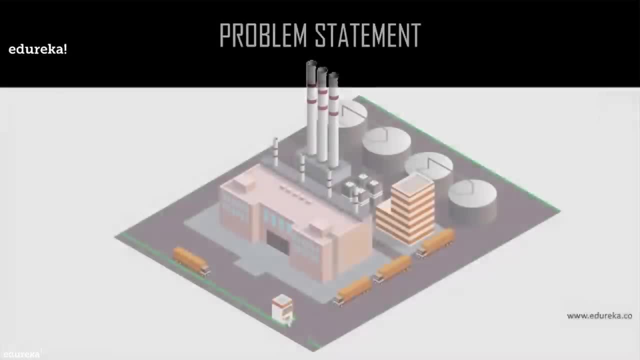 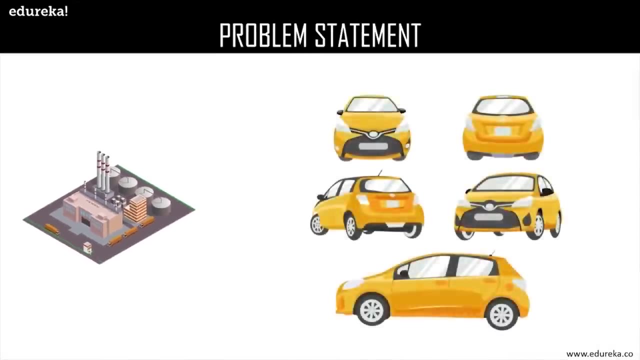 by conveying them the necessary power, like the engine and the other parts that they would need in order to build the car. Now these different parts are located at nine different positions within the factory warehouse. The car parts include these: chassis, wheels, dashboard. 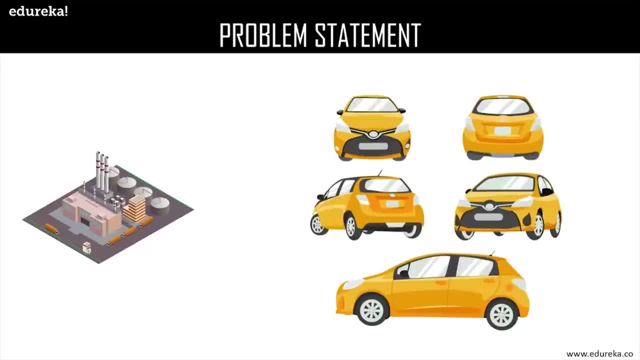 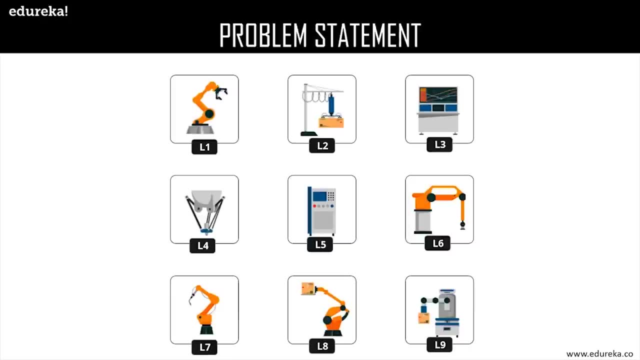 the engine and so on, and the factory workers have prioritized the location that contains the body or the chassis to be the top most. but they have provided the priorities for other locations as well, which we'll look into at the moment. Now, these locations within the factory: 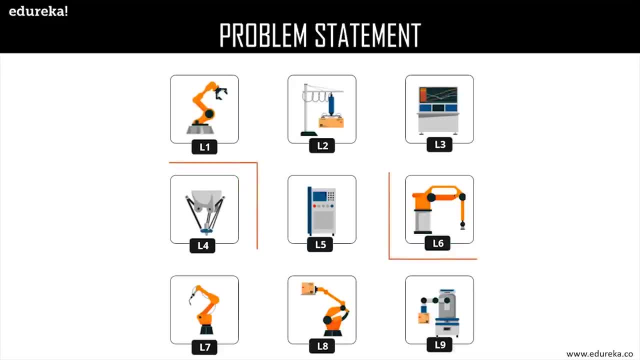 somewhat like this. so, as you can see, here we have l1, l2, l3, all of these stations. now, one thing you might notice here that there are little obstacle present in between the locations. so l6 is the top priority location that contains the chassis for preparing the car bodies. now the task is to enable 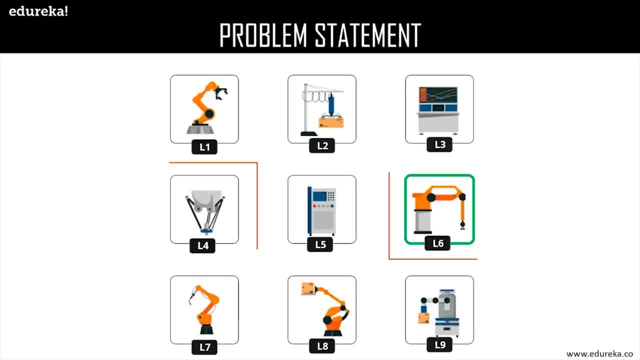 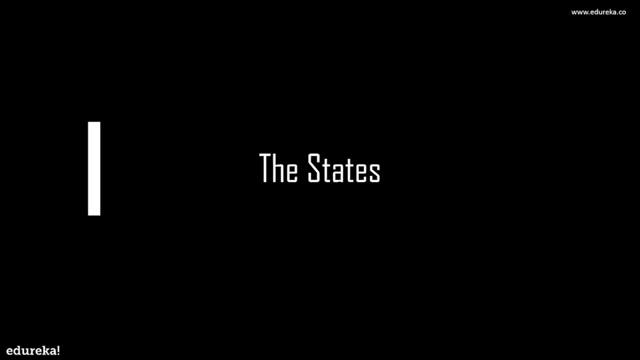 the robots so that they can find the shortest route from any given location to another location on their own. now the agents in this case are the robots. the environment is the automobile factory warehouse. so let's talk about the states. so the states are the location in which a particular 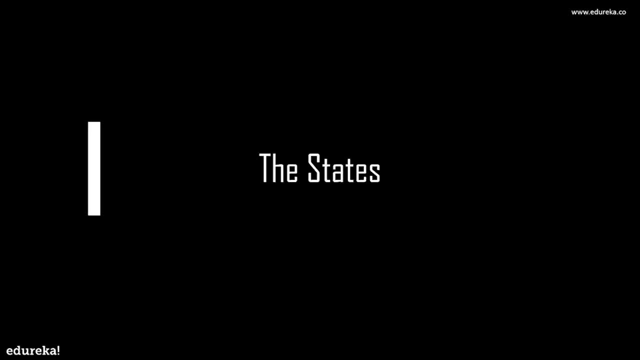 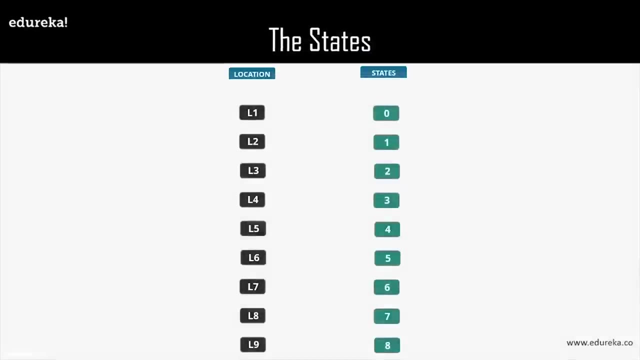 robot is present in the particular instance of time, which will denote its states. now, machines understand numbers rather than letters, so let's map the location codes to number. so, as you can see here, we have mapped location l1 to the state 0, l2 and 1 and so on. we have l8 as state 7. 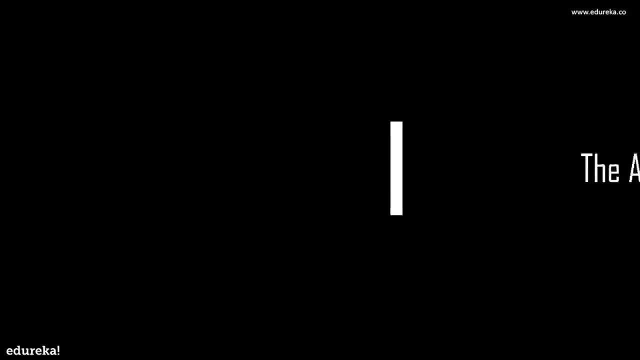 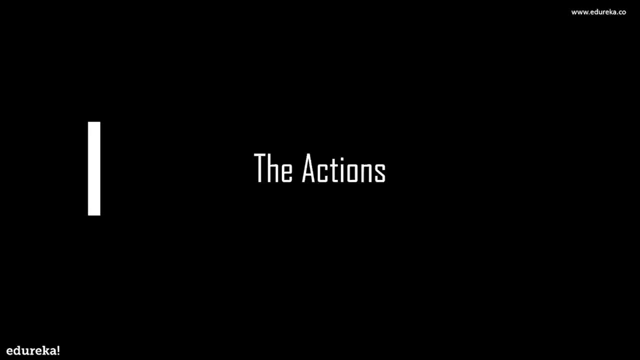 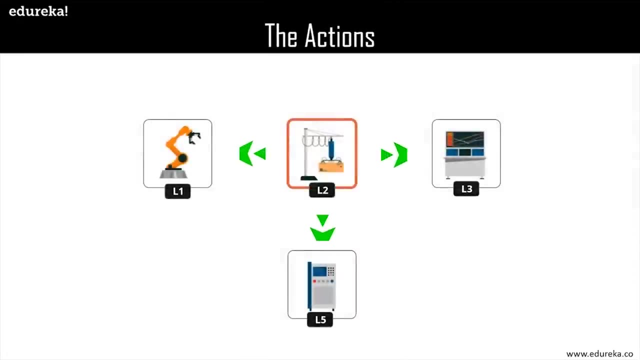 the action will be the direct location that a robot can go from a particular location. right, consider a robot that is at l2 location and the direct locations to which it can move are l5, l1 and l3. now, the figure here may come in handy to visualize this. now, as you might have already, 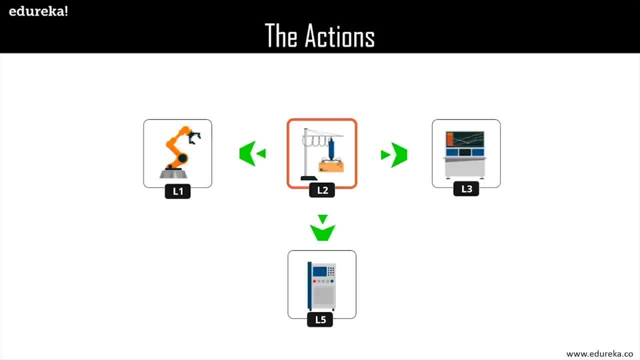 guessed, the set of actions here is nothing but the same thing. you can see here. the action will be the direct location that a robot can go from a set of all possible states of the robot. for each location, the set of actions that a robot can take will be different. for example, the set of actions will change if the robot is in l1 rather than l2. 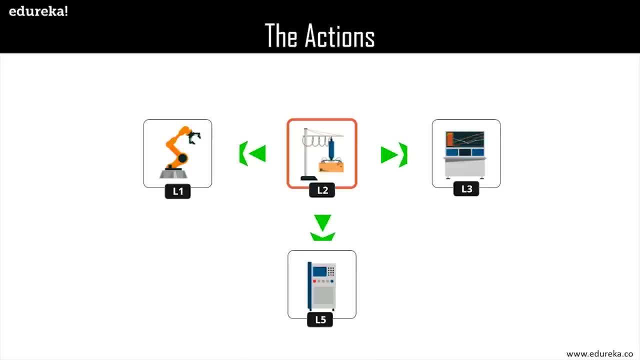 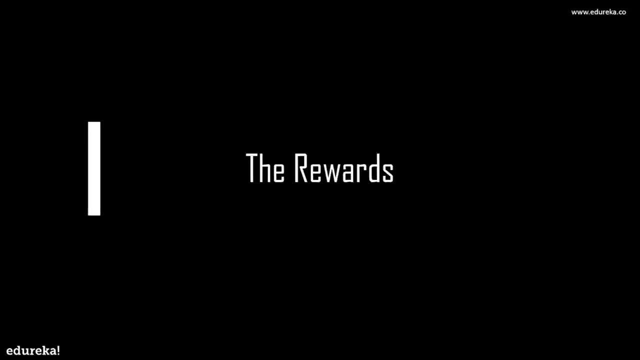 so if the robot is in l1, it can only go to l4 and l2 directly. now that we are done with the states and the actions, let's talk about the rewards. so the states are basically 0, 1, 2, 3, 4. 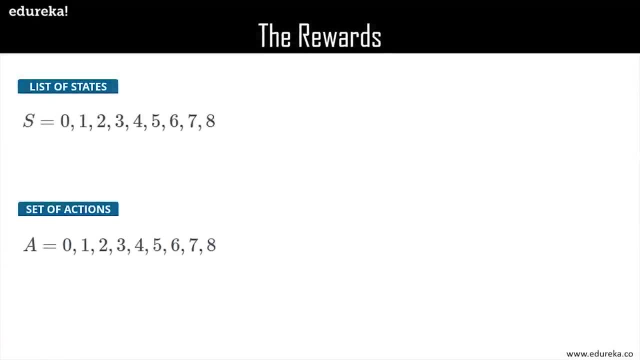 and the actions are also 0, 1, 2, 3, 4, up till 8. now the rewards are basically 0, 1, 2, 3, 4 and the actions rewards now will be given to a robot if a location, which is the state, is directly reachable from a. 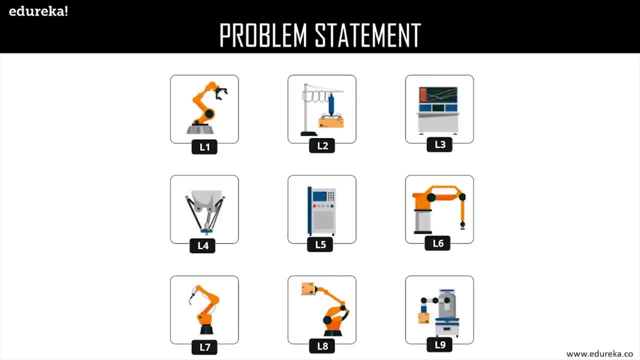 particular location. so let's take an example. suppose l9 is directly reachable from l8, right? so if a robot goes from l8 to l9 and vice versa, it will be rewarded by 1, and if a location is not directly reachable from a particular location, we do not give any reward. a reward of 0. now the 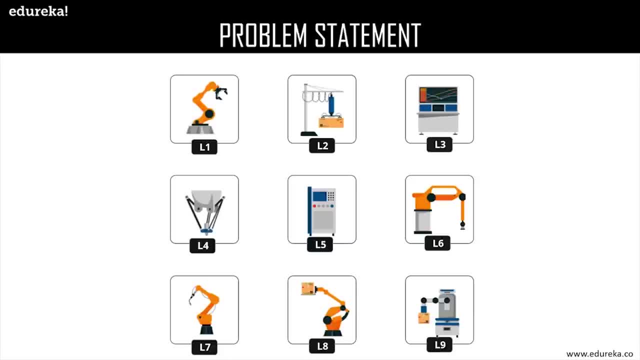 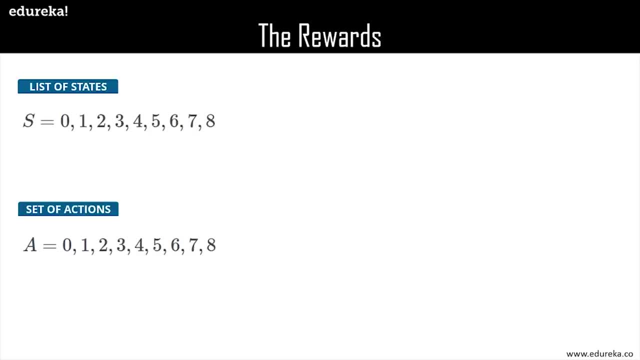 reward is just a number here and nothing else. it enables the robots to make sense of the movements, helping them in deciding what locations are directly reachable and what are not. now, with this queue, we can construct a reward table which contains all the reward values, mapping between all. 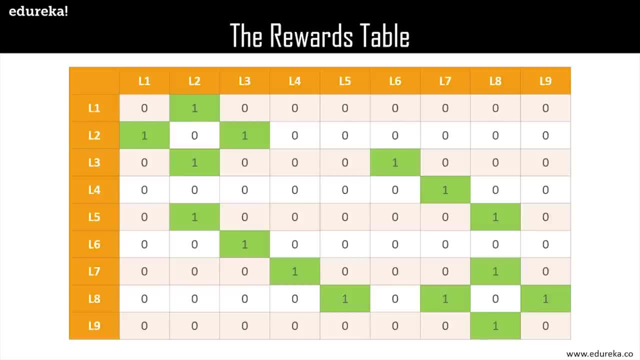 possible states. so, as you can see here in the table, the positions which are marked green have a positive reward and as you can see here we have all the possible rewards that a robot can get by moving in between the different states. now comes an interesting decision. now remember that the 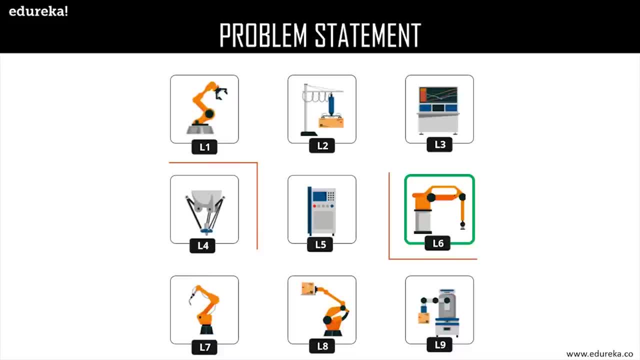 factory administrator prioritizes the rewards that the robot can get by moving in between the places in the process, so in this case we can see that the factory administrator is выше. the new position and the goal area is the target area. within this block, the new position equals the. 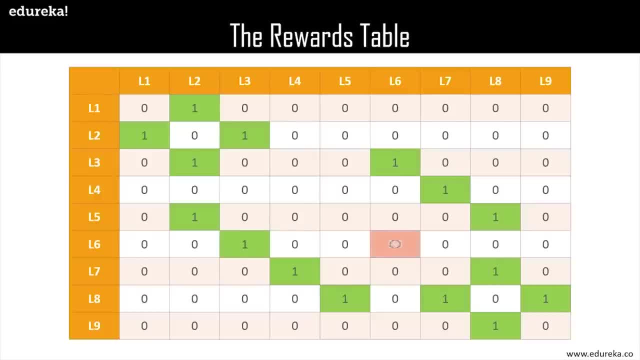 target area. so what we need to do is to add a reward in every classí equation of top 하나�. ımız like to do this without religiosity, and we just create these requirements as a concealer in. so simply find the room of reward in пой teki. so let's add 999 to the corndog box. 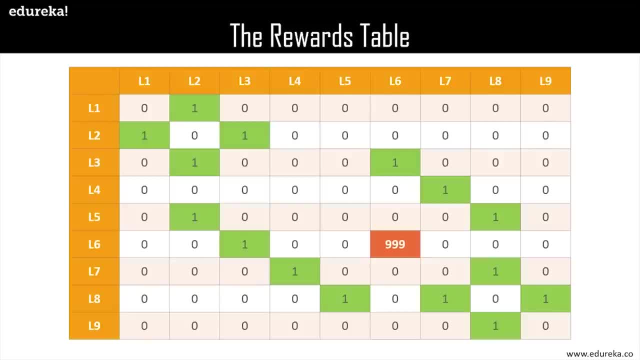 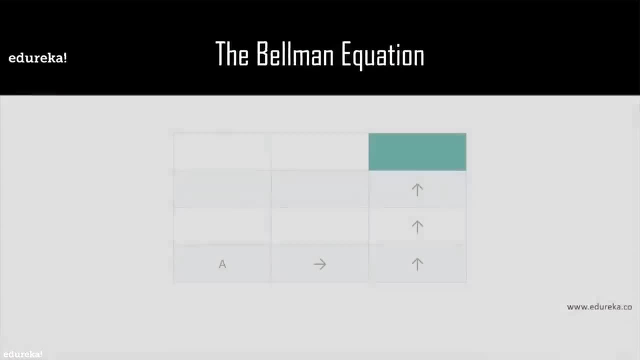 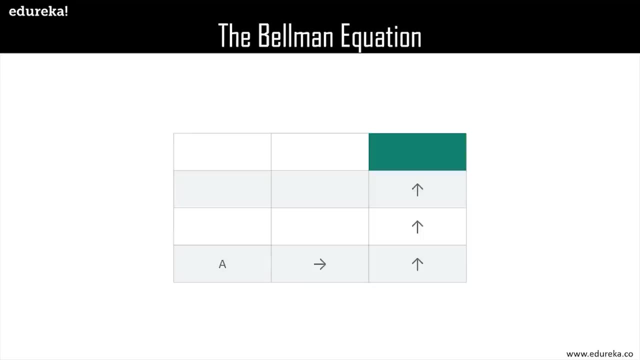 an x some of the fundamental concepts that prevail in the world of reinforcement learning and queue learning. so first of all we'll start with the bellman equation. now consider the following square of rooms, which is analogous to the actual environment from our original problem, but without the barriers. now suppose a robot needs to go to the room marked in the green from its 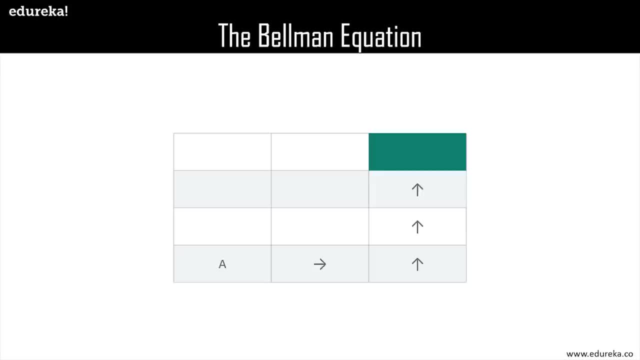 current position, a, using the specified direction. now, how can we enable the robot to do this programmatically? one idea would be introduce some kind of a footprint which the robot will be able to follow. now, here, a constant value is specified in each of the rooms which will come. 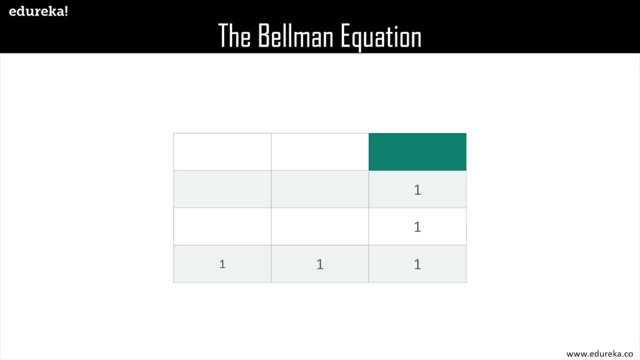 along the robot's way if it follows the direction specified above now. in this way, if it starts at location a, it will be able to scan through this constant value and will move accordingly. but this will only work if the direction is prefixed and the robot always starts at the location a now. 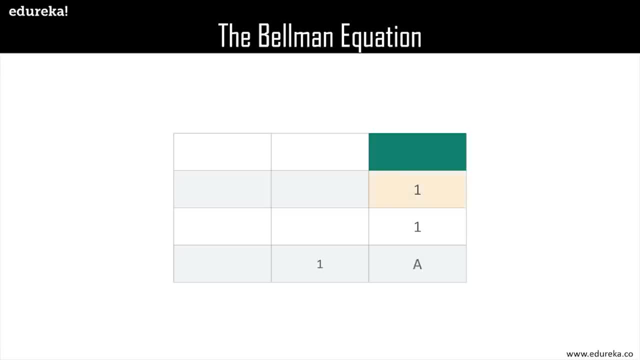 consider the robot starts at this location a. now consider the robot starts at this location a. now consider the robot starts at this location a, rather than its previous one. now, the robot now sees footprints in two different directions. it is therefore unable to decide which way to go in order to get the destination which. 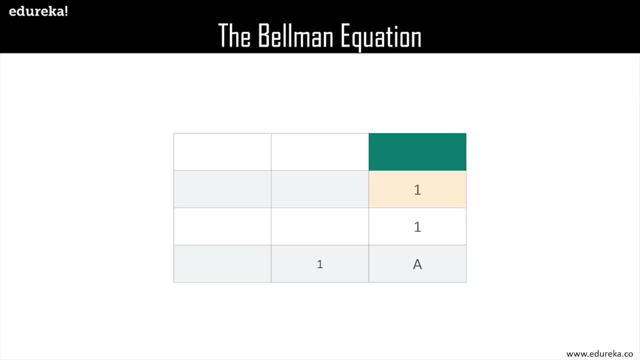 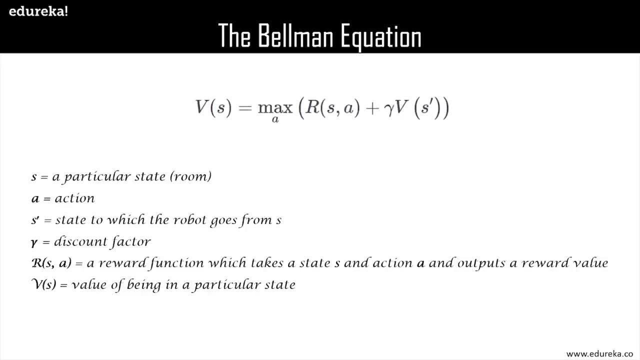 is the green room. it happens primarily because the robot does not have a way to remember the directions to proceed. so our job now is to enable the robot with the memory. now, this is where the Bellman equation comes into play. so, as you see here, the main reason of the Bellman equation is: 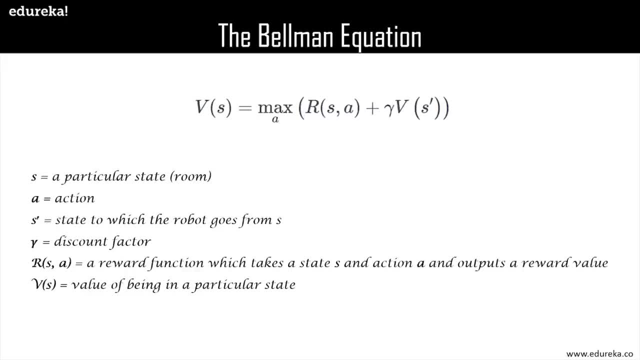 to enable the robot with the memory. that's the thing we're going to use. so the equation goes something like this: V of s gives maximum a R of s comma a plus gamma of V s dash, where s is a particular state which is a room, a is the action moving between the rooms. s dash is the state to. 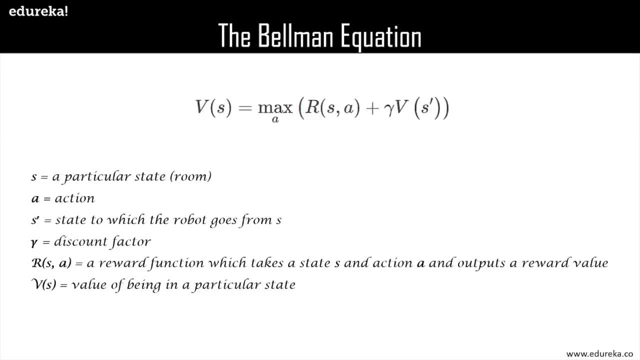 which the robot goes from. s and gamma is the discount factor- now we'll get into it in a moment- and obviously R of s, comma a, is a reward function which takes a state- s- and action a, and outputs the reward. now, V of s is the value of being in a particular state. 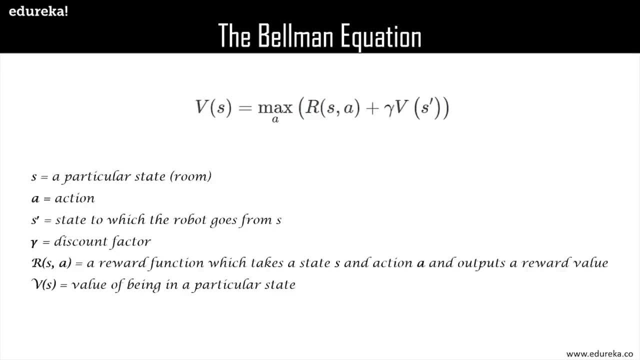 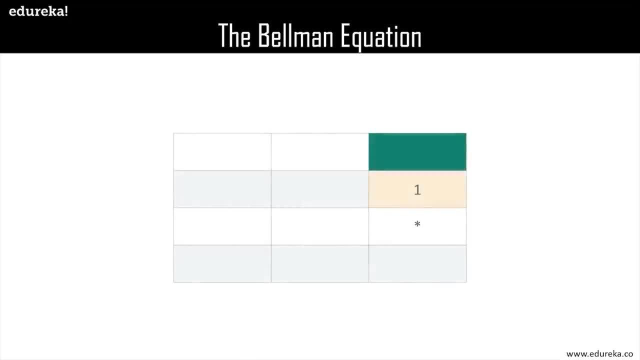 which is the footprint. now we consider all the possible actions and take the one that yields the maximum value. now there is one constraint, however, regarding the value footprint. that is the room marked in the yellow just below the green room. it will always have the value of one to denote that. 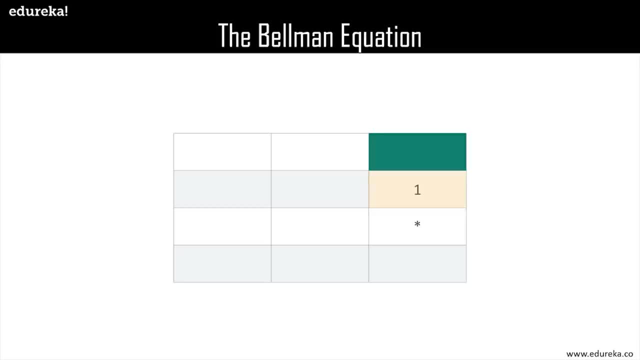 is one of the nearest room, adjacent to the green room. now, this is also to ensure that a robot gets a reward when it goes from a yellow room to the green room. let's see how to make sense of the equation which we have here. so let's assume a discount factor of 0.9. as we remember, gamma is 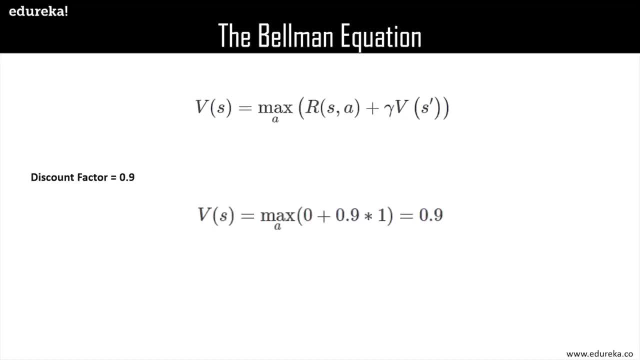 the discount value or the discount factor. so let's take it 0.9. now for the room which is marked just below the one, or the yellow room, which is the asterisk mark for this room, what will be the V of s? that is, the value of being in a particular state. so for this V of s would be something like: 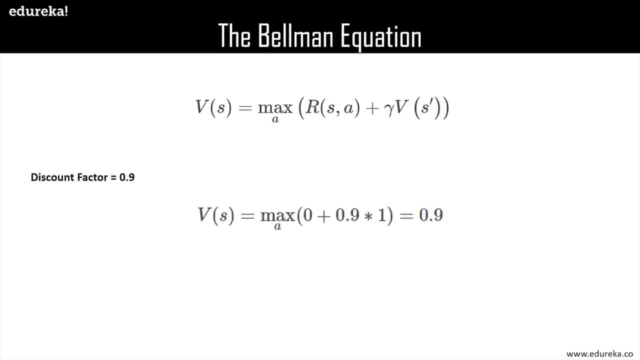 a dash, dash 1, the amount of a is going to be 0.9 and the amount of a is going to be zero. so the value of being in the yellow room is 0.9 and the maximum of a will take 0, which is the initial of. 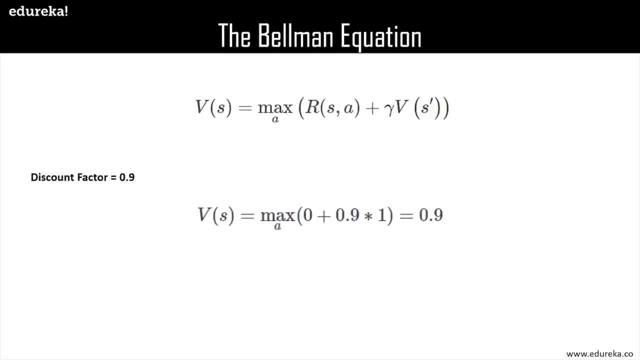 r s comma a plus 0.9, which is gamma, into 1, that gives us 0.9. now here the robot will not get any reward for going to a state marked in yellow, hence the r? s comma a is 0 here, but the robot knows the. 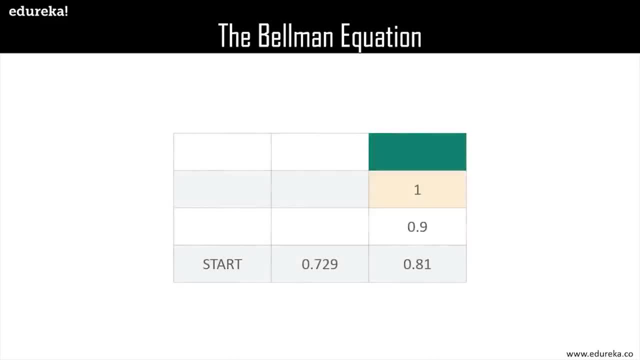 value of being in the yellow room 0.9, then again, if we put 0.9 in this equation, we get 0.81, then 0.729, and then we again reach the starting point. so this is how the table looks, with some value footprints computed from the: 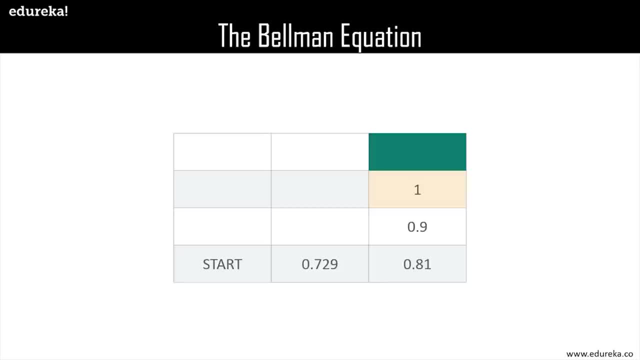 bellman equation. now, a couple of things to notice here is that the max function helps the robot to always choose the state that gives it the maximum value of being in that state. now the discount factor gamma notifies the robot about how far it is from the destination. this is typically specified. 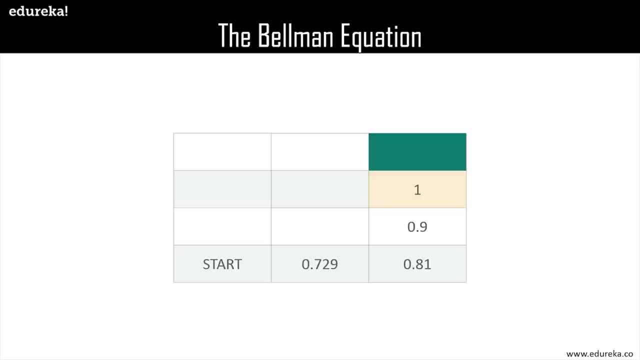 by the developer of the algorithm that would be installed in the robot. now the other states can also be given their respective values in a similar way. so, as you can see here, the boxes adjacent to the green one have one, and if we move away from one, we get 0.9, 0.81, 0.729 and finally we reach 0.66. 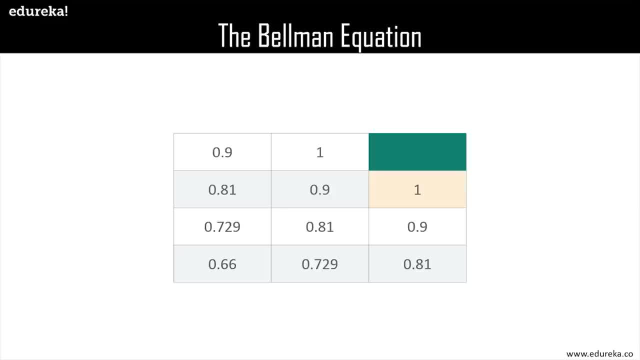 now the robot is also able to set the value of 0.9 and 0.729 and finally we reach 0.66. now the robot now can proceed its way through the green room utilizing these value footprints, even if it's dropped at any arbitrary room in the given location. now, if a robot lands up in the highlighted sky, 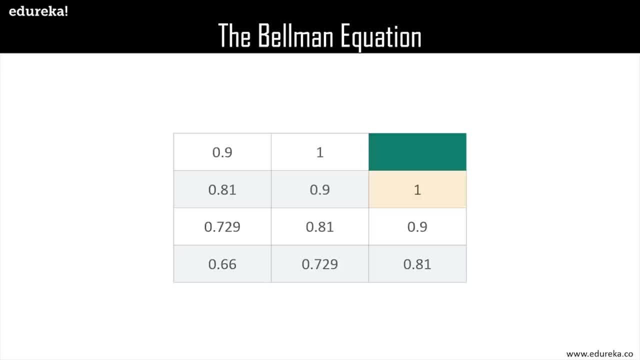 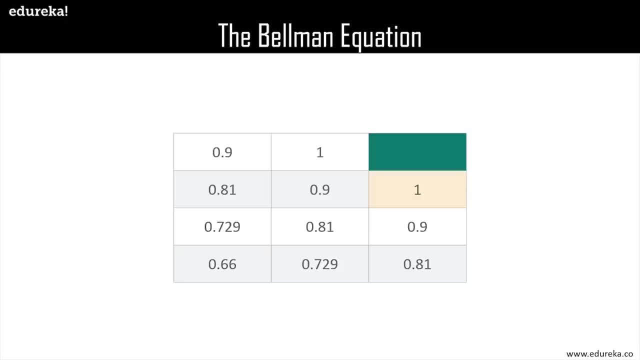 of reinforcement, and the equation is one of the key equations in the world of reinforcement learning and of reinforcement learning and Q learning. so, if we think realistically, our surroundings do not always work in the way we expect. there is always a bit of stochasticity involved in it, but this 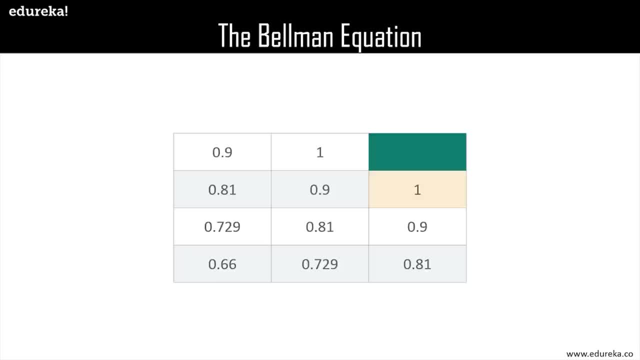 applies to robot as well. sometimes it might so happen that the robots machinery got corrupted. sometimes the robot may come across some hindrance on its way which may not be known to it beforehand. right and sometimes, even if the robot knows that it needs to take the right turn, it will not. so how? 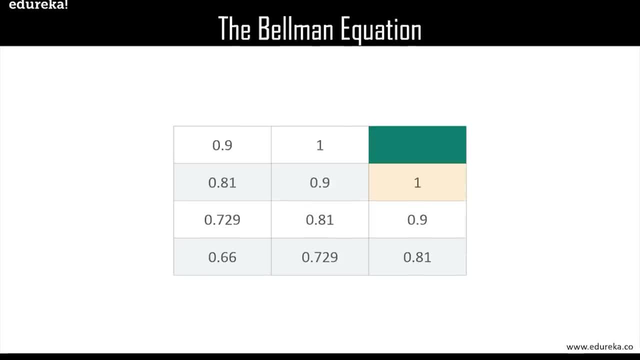 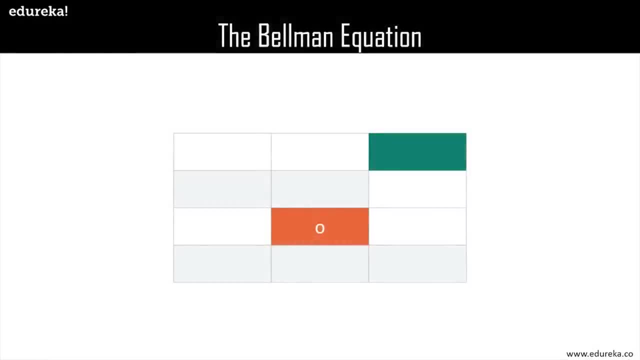 right and sometimes, even if the robot knows that it needs to take the right turn, it will not. so how do we introduce the stochasticity in our case now? here comes the mark of decision process. now consider: the robot is currently in the red room and it needs to go to the green room now. 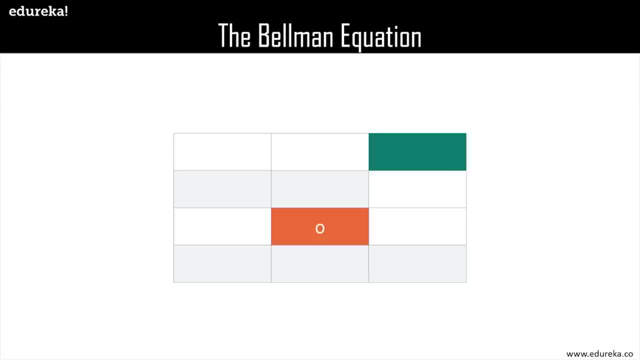 let's now consider the robot has a slight chance of dysfunctioning and might take the left or the right or the bottom turn, instead of taking the upper turn, in order to get to the green room from where it is now, which is the red room. now the question is: how do we enable the robot to handle? 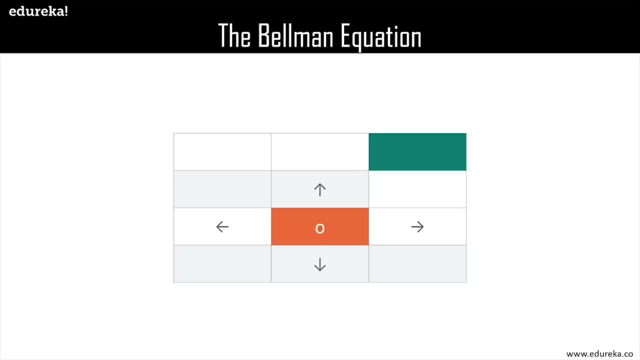 the red room. now the question is: how do we enable the robot to handle this when it is unable to do so when it is out in the given environment right now? this is a situation where the decision making regarding which turn is to be taken is partly random and partly under the control of the robot. 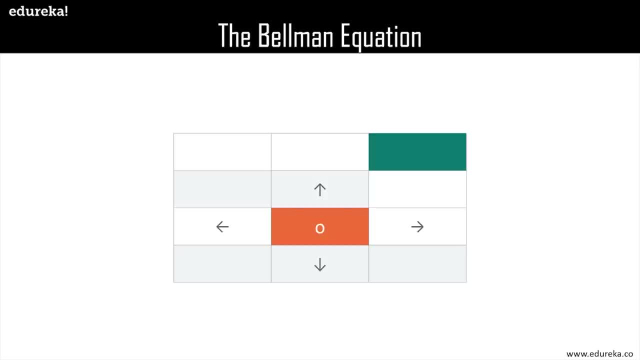 now partly random, because we are not sure when exactly the robot might dysfunctional, and partly under the control of the robot, because it is still making a decision of taking a turn right on its own and with the help of the program embedded into it. so a mark of decision process is a discrete time. 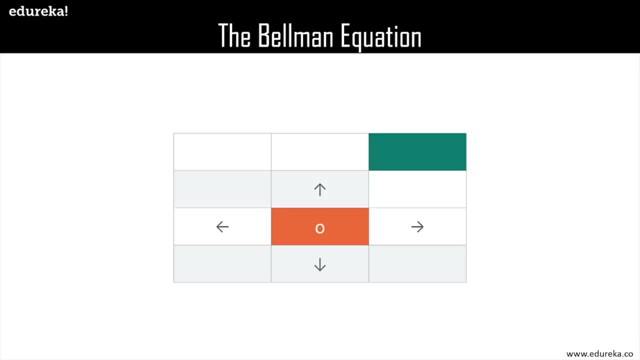 process. it provides a mathematical framework for modeling decision making in situations where the outcomes are partly random and partly under control of the decision maker. now we need to give this concept a mathematical shape, most likely an equation, which then can be taken further. now you might be surprised that we can do this with the help of the bellman equation, with a few minor 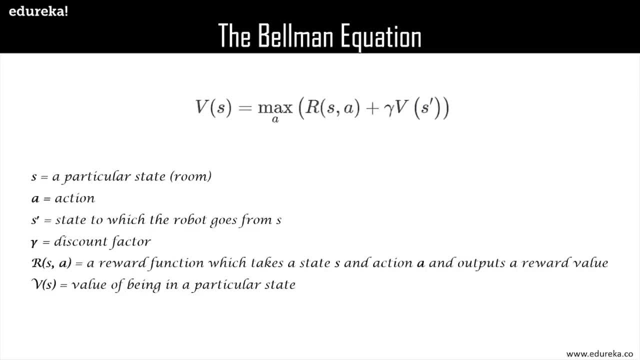 tweaks. so if we have a look at the original bellman equation, v of x is equal to maximum of r s comma a plus gamma v of s dash. what needs to be changed in the above equation so that we can introduce some amount of randomness here, as long as we are not sure when the robot might not take? 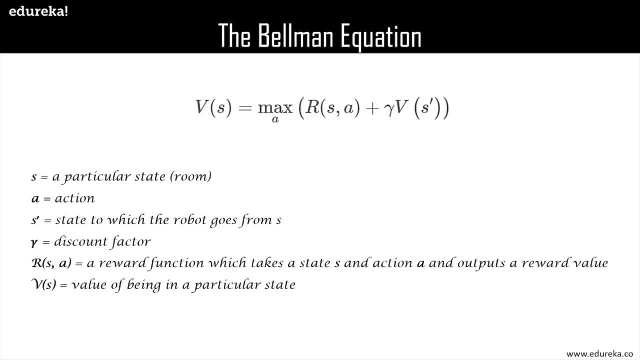 the expected turn. we are then also not sure in which room it might end up, in, which is nothing but the room it moves from its current room. at this point, according to the equation, we are not sure of the s dash, which is the next state, or the room, but we do know. 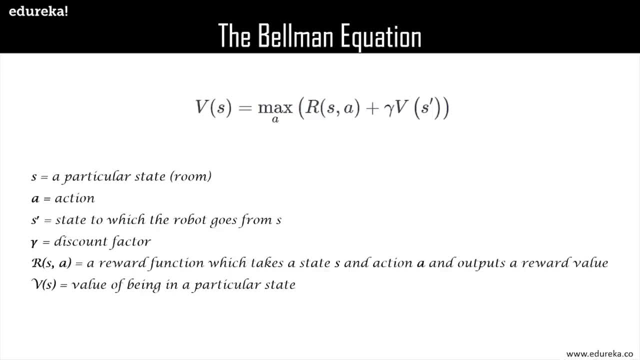 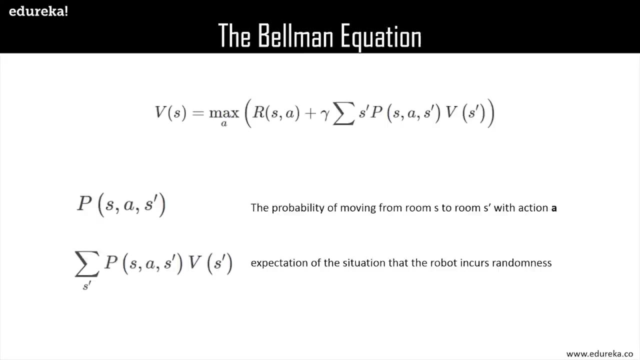 all the probable turns the robot might take now. in order to incorporate each of these probabilities into the above equation, we need to associate a probability with each of the turns to quantify the robot if it has got any explicit chance of taking this turn now. if we do so, we get p s is. 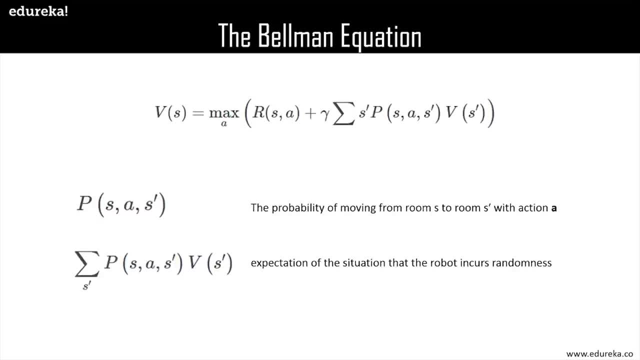 equal to maximum of r s comma a plus gamma into summation of s dash, p s comma a, comma s dash into v of s dash. now the p? s a and s dash is the probability of moving from room s to s dash with the action a and the submission here is the expectation of the situation that the robot 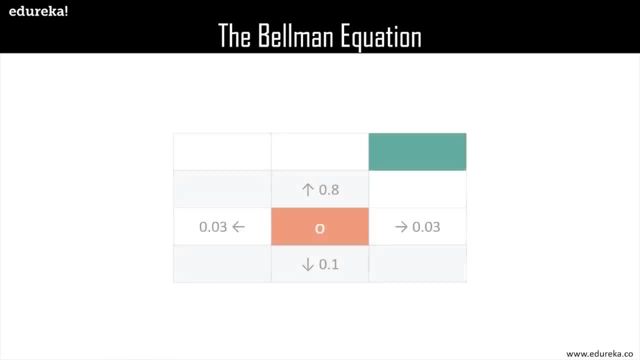 incurs, which is the randomness. now let's take a look at this example here. so when we associate the probabilities to each of these terms, we essentially mean that there is an 80 chance that the robot will take the upper turn. now, if we put all the required values in our equation, we get 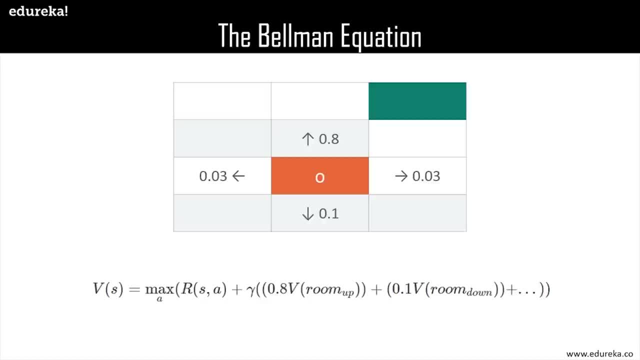 v of s is equal to maximum of r of s comma a, plus gamma of 0.8 into v of room up plus 0.1 into v of room down, 0.03 into room of v of room left plus 0.03 into v of room right now. note that the value. 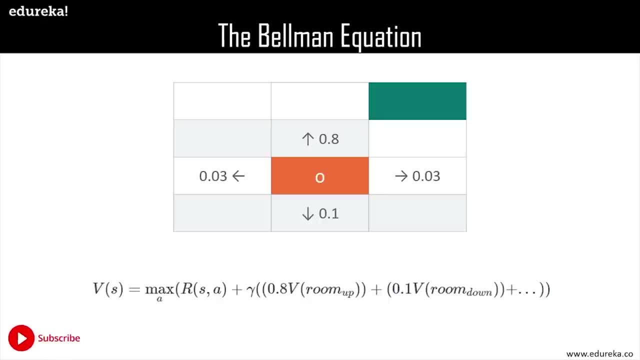 footprints will not change due to the fact that we are incorporating stochastically here. but this time we will not calculate those value footprints. instead we will let the robot to figure it out. now, up until this point, we have not considered about rewarding the robot for its 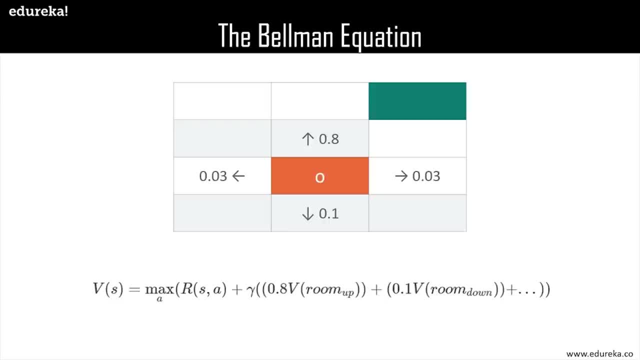 action of going into a particular room. we are only rewarding the robot when it gets to the destination. now, ideally, there should be a reward for each action the robot takes to help it better assess the quality of the actions. but the rewards need not to be always be the same, but it is much. 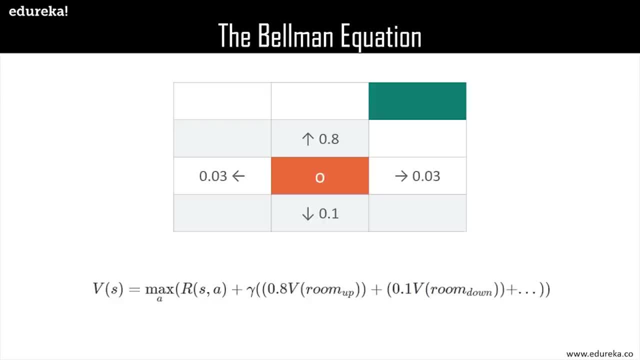 better than having some amount of reward for the actions than having no rewards at all. right, and this idea is known as the living penalty. in reality, the reward system can be very complex, and particularly modeling sparse rewards is an active area of research in the domain of reinforcement. 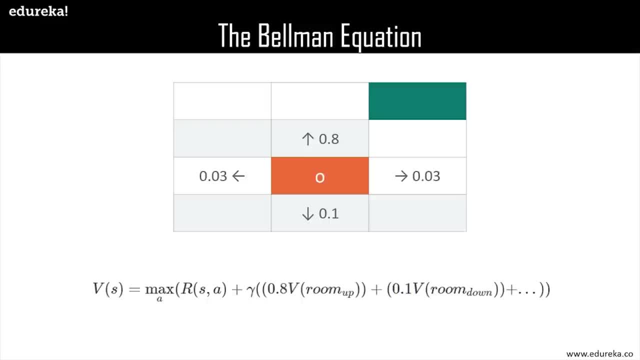 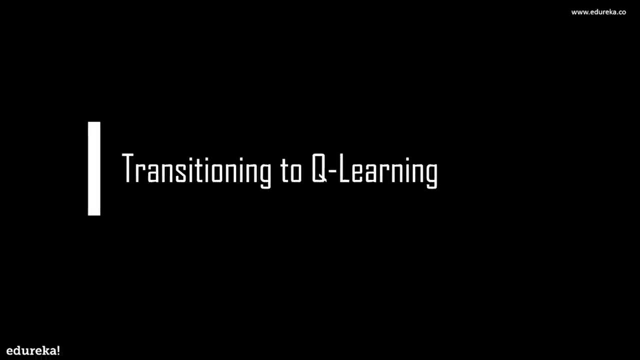 learning. so by now we have got the equation which we have is. so what we're going to do is now transition to q learning. so this equation gives us the value of going to a particular state, taking the stochasticity of the environment into account. now we have also learned very 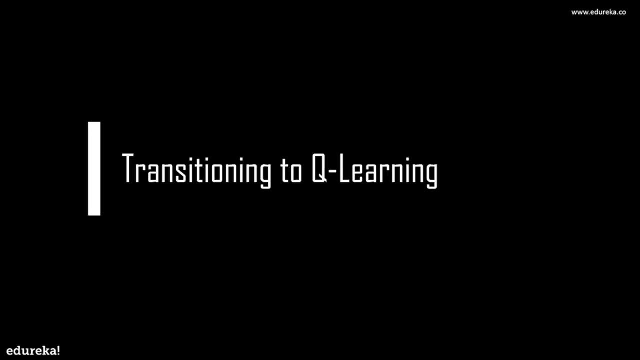 briefly about the idea of living penalty, which deals with associating each move of the robot with a reward. so q learning possesses an idea of assessing the quality of an action that is taken to move to a state, rather than determining the possible value of the state which is being moved to. 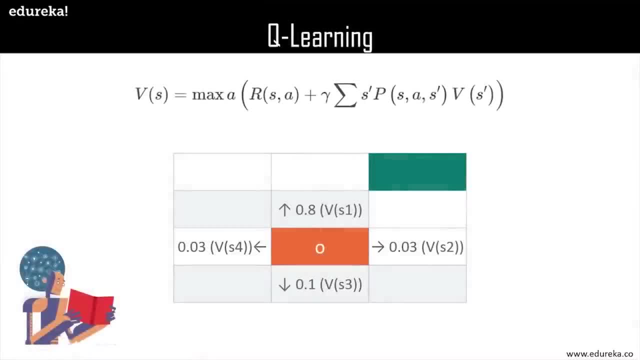 so earlier we had 0.8 into v of s 1, 0.03 into v of s 2, 0.1 into v of s 3 and so on. now, if we incorporate the idea of assessing the quality of the action for moving to a certain state, so the environment with the agent and the quality of the 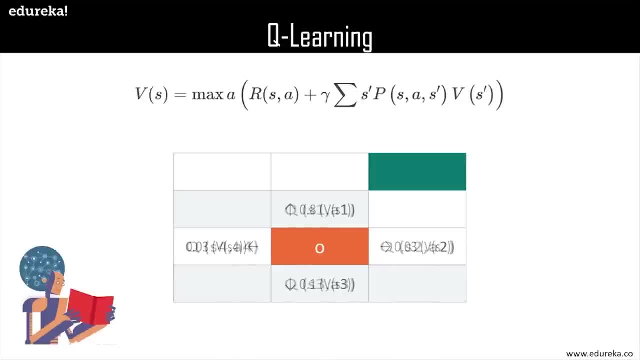 action will look something like this. so instead of 0.8 v of s 1, we'll have q of s 1 comma a 1. we'll have q of s 2, comma a 2. q of s 3. now the robot now has four different states to choose from. 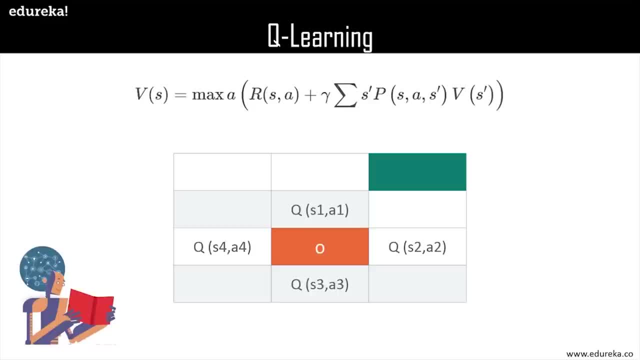 and along with that there are four different actions, also for the current state it is in. so how do we calculate q of s comma a? that is the cumulative quality of the possible actions the robot might take. so let's break it down now from the equation: v of s equals maximum of a r s comma a plus gamma summation: s dash, p, s a, s dash. 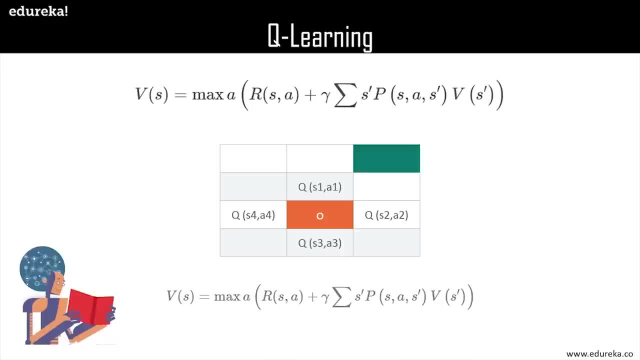 into v of s dash. if we discard the maximum function, we have r? s of a plus gamma and plus b of s, minus b of s, squared into summation p and v. now, essentially in the equation that produces v of s, we are considering all possible actions and all possible states from the current 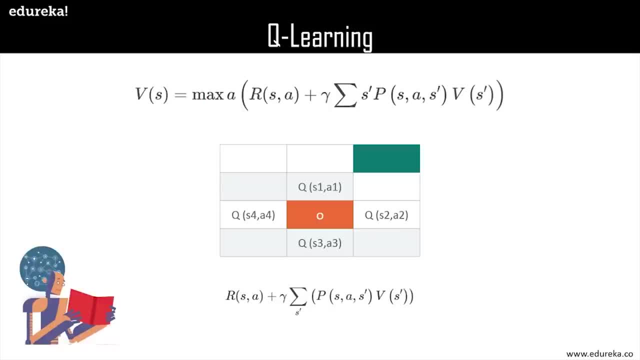 state that the robot is in, and then we are taking the maximum value caused by taking a certain action and the equation produces a value footprint which is for just one possible action. in fact we can think of it as the quality of the action. so to rs comma, a plus comma of summation p and v, now that we have got an equation to quantify the 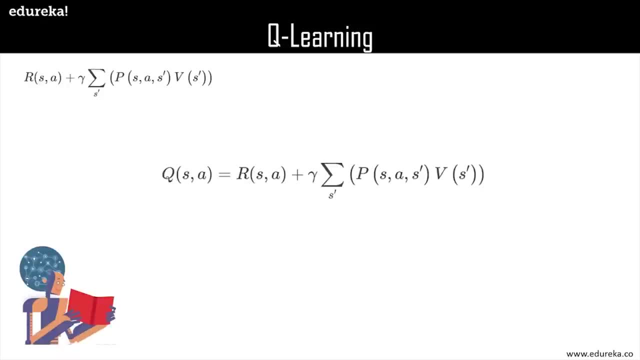 quality of a particular action. we are going to make a little adjustment in the equation. we can now say that v of s is the maximum of all the possible values of q of s comma a right. so let's utilize this fact and replace v of s dash as a function of q, so q s comma a becomes. 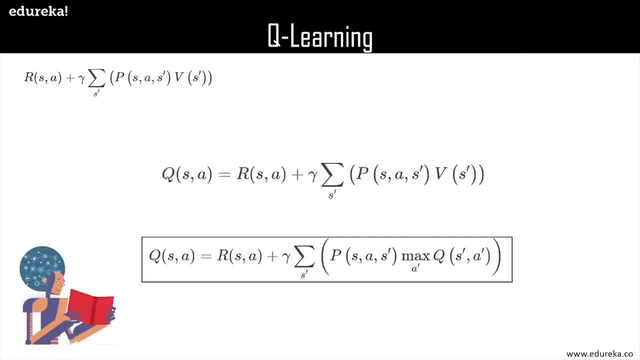 r of s comma, a plus comma of summation, p, s, a, s dash and maximum of the q s dash, a dash. so the equation of v is now turned into an equation of q, which is the quality. but why would we do that now? this is done to ease our calculations, because now we have only one function. 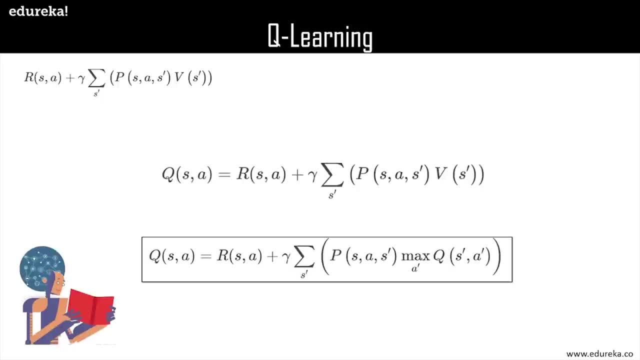 q, which is also the core of the dynamic programming language. we have only one function q to calculate, and we have only one function q to calculate and we have only one function q to calculate. and r of s comma a is a quantified metric which produces reward of moving to a certain state. 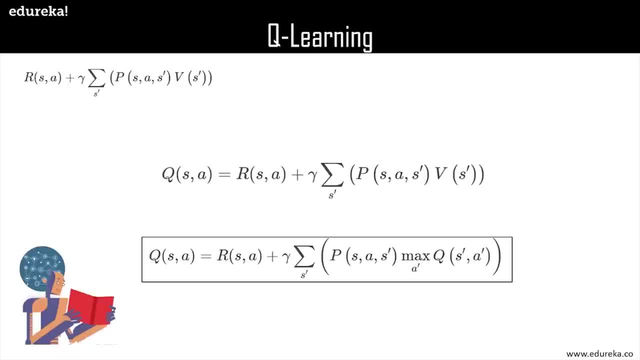 now the qualities of the actions are called the q values, and from now on we will refer to the value footprints as the q values. an important piece of the puzzle is the temporal difference. now, temporal difference is the component that will help the robot calculate the q values with. 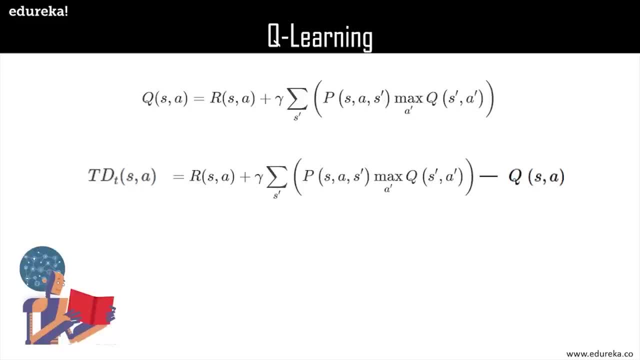 respect to the changes in the environment over time. so consider: our robot is currently in the marked state and it wants to move to the upper state. one thing to note that here is that the robot already knows the q value of making the action. that is, moving to the upper state and we 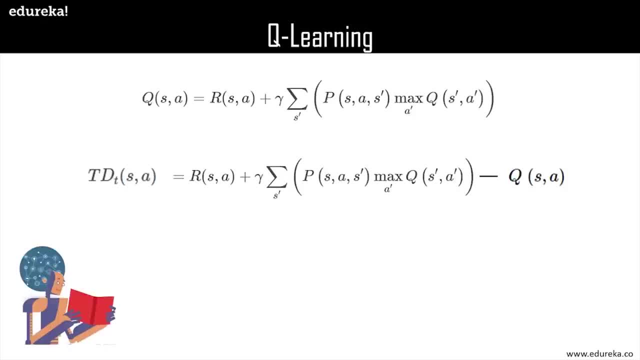 know that the environment is stochastic in nature and the reward that the robot will get after moving to the upper state might be different from an earlier observation. so how do we capture this change, the real difference? we calculate the new q s, comma a with the same formula and subtract the previously known q, and here we can see that our representation of q as r in the state systemалась in. the second step for us is right now. we need to transfer the 기�aan brain in the state systemapolis q to the stochastic state. we already know that. the robot knows that there is a value of p with the inversion statements. 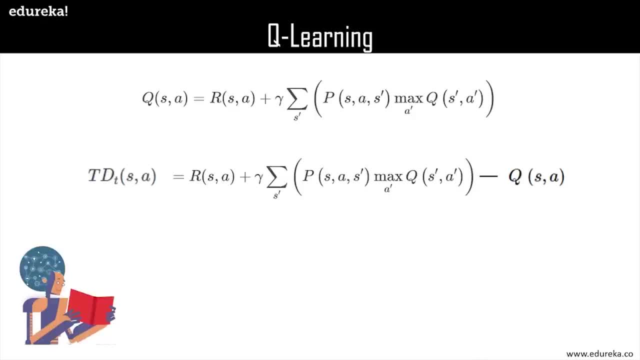 q sa from it. so this will in turn give us the new qa. now the equation that we just derived gives the temporal difference in the q values, which further helps to capture the random changes in the environment which may impose. now the new q s comma a is updated as the following: so qt of s comma a. 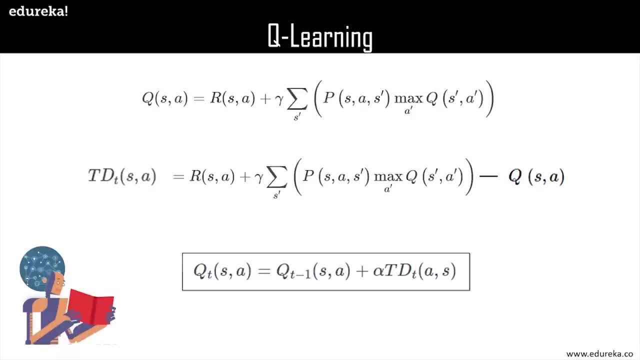 is equal to qt minus one s comma a plus alpha tdt of a comma s. now here alpha is the learning rate, which controls how quickly the robot adapts to the random changes imposed by the environment. the qt s comma a is the current state q value and the qt minus one s comma a is the previously. 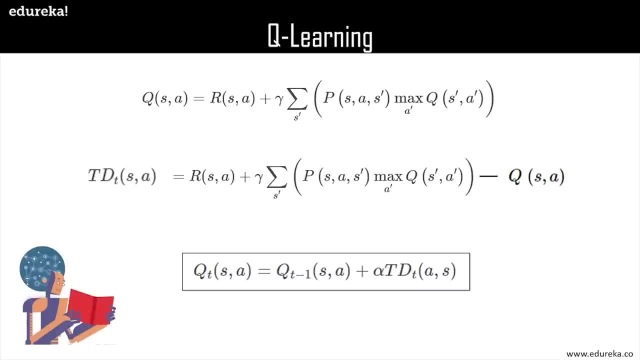 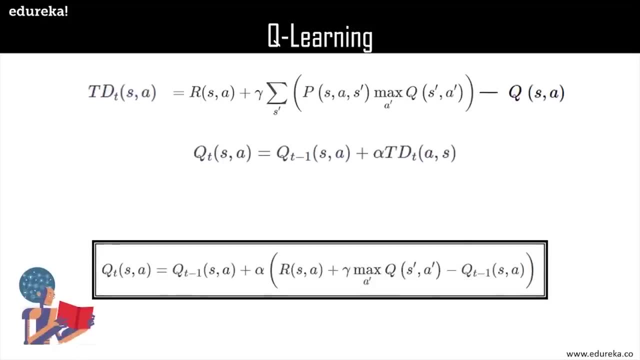 recorded q value. so if we replace the tds comma a with its full form equation we should get: qt of s comma a is equal to qt minus 1 of s comma a plus alpha into r of s comma a plus gamma. maximum of q s dash a dash minus q. 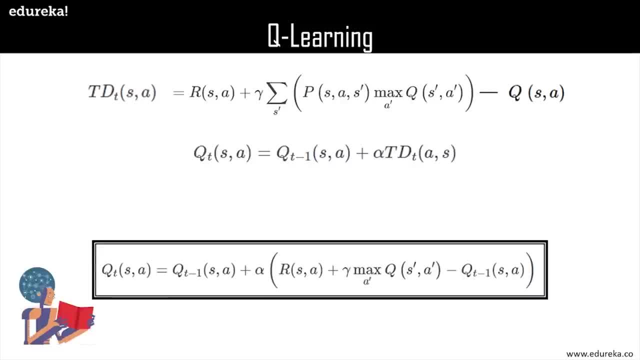 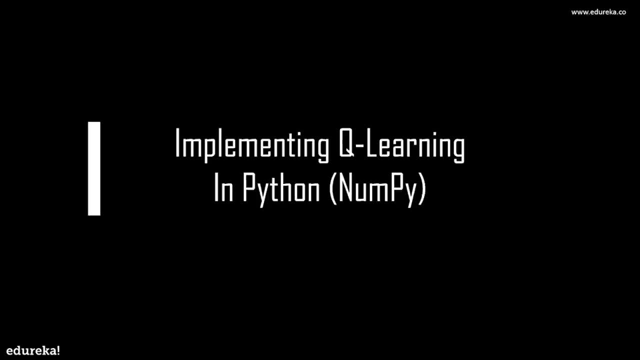 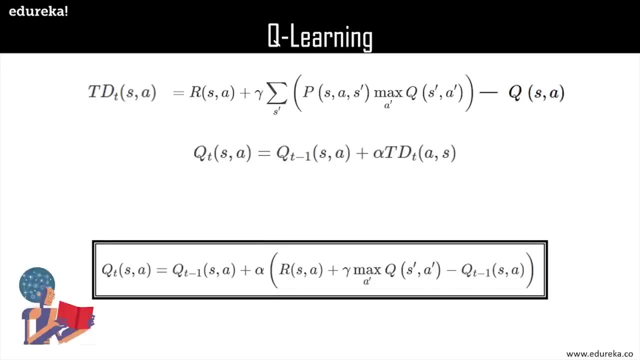 t minus 1 s comma a. now that we have all the little pieces of q learning together, let's move forward to its implementation part. now this is the final equation of q learning, right, so let's see how we can implement this and obtain the best path for any robot to take now to implement the 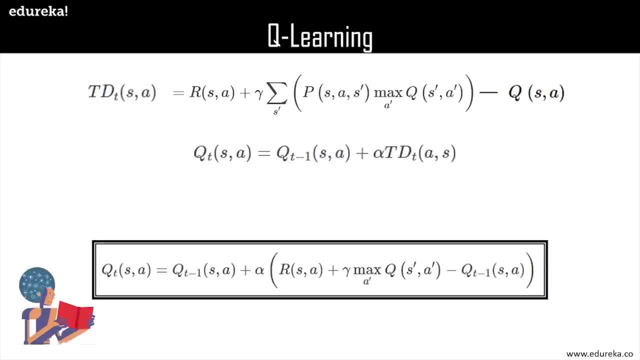 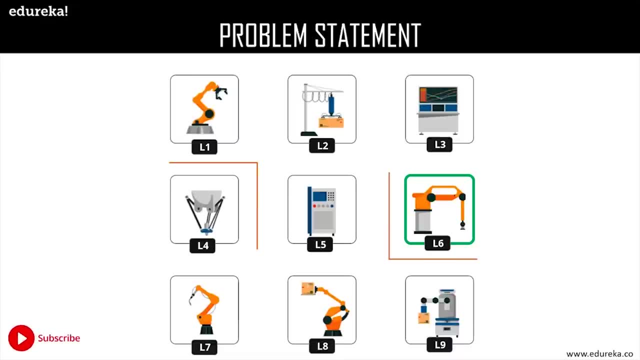 algorithm. we need to understand the warehouse location and how that can be mapped to different states. so let's start by recollecting the sample environment. so, as you can see here we have l1, l2, l3 till l9 and, as you can see here, we have certain borders also. so first of all, let's map each of the 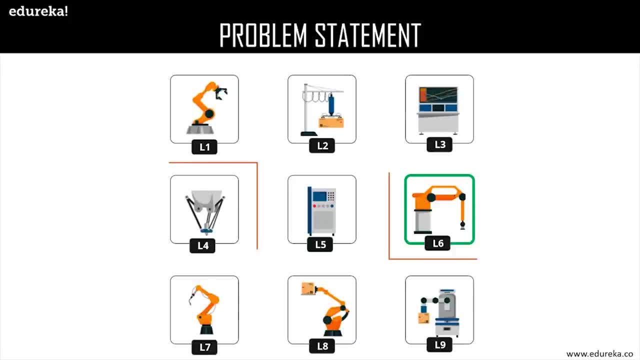 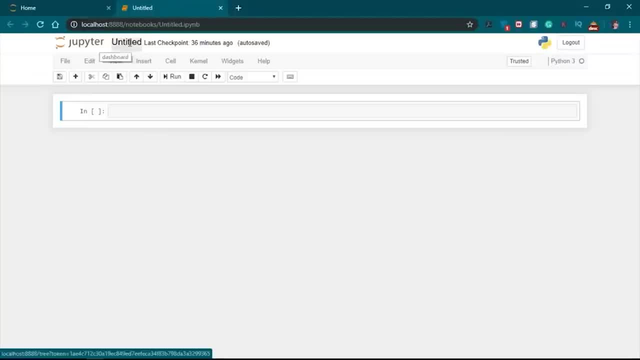 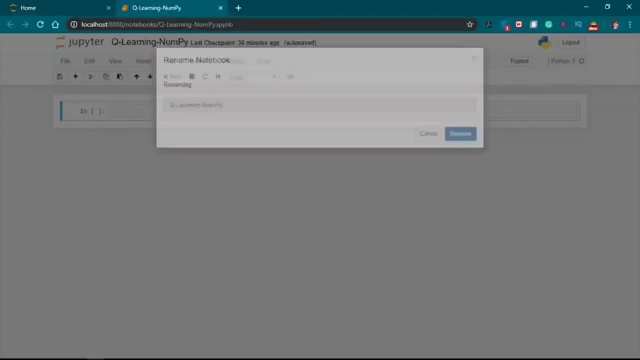 locations in the warehouse to numbers or the states, so that it will ease our calculations, right? so what i'm going to do is create a new python 3 file in the jupyter notebook and i'll name it as q learning numpy. okay, so let's define. 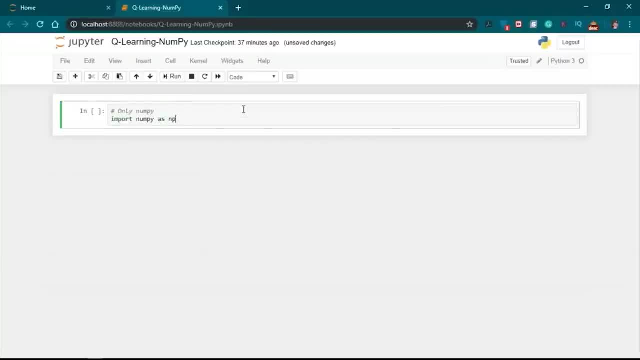 the states. but before that, what we need to do is import numpy- because we're going to use numpy for this purpose- and let's initialize the parameters, that is, the gamma and alpha parameters. so let's initialize the parameters, that is, the gamma and alpha parameters, and let's initialize. 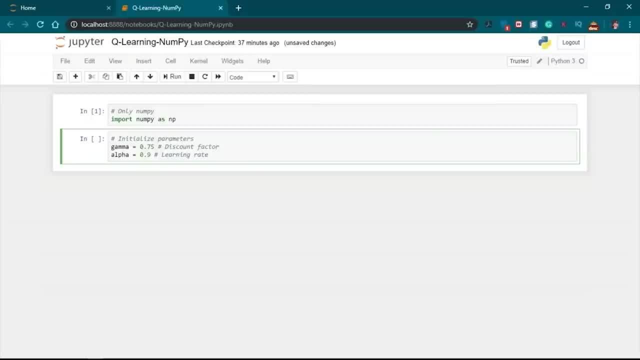 the parameters, that is, the gamma and alpha parameters. and let's initialize. so gamma is 0.75, which is the. so gamma is 0.75, which is the discount factor, whereas alpha is 0.9, which is the learning rate. now, next, what we're going to do is define the states and map it to numbers. so, as i mentioned, 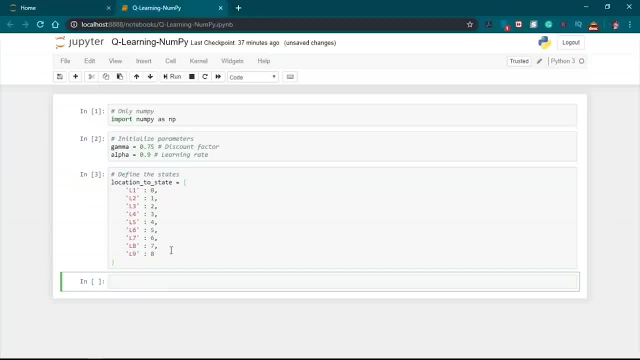 earlier. l1 is 0 and till n line. we have defined the states in the numerical form. now the next step is to define the actions, which is, as mentioned above, represent the transition to the next state. so, as you can see, here we have an array of actions, from 0 to 8. 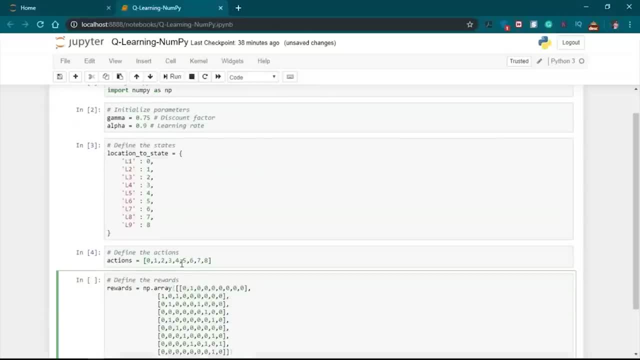 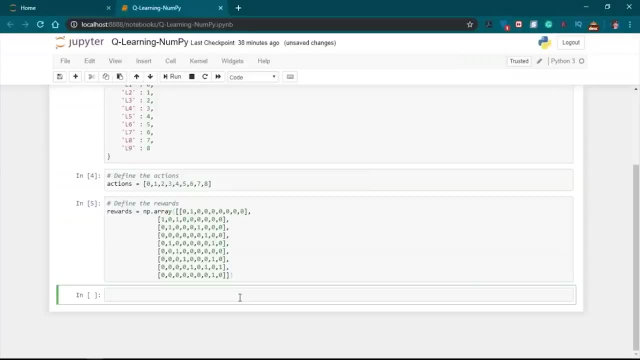 now what we're going to do is define the reward table. so, as you can see, it's the same matrix that we created just now, that i showed you just now. now, if you understood it correctly, there isn't any real barrier limitation, as depicted in the image. 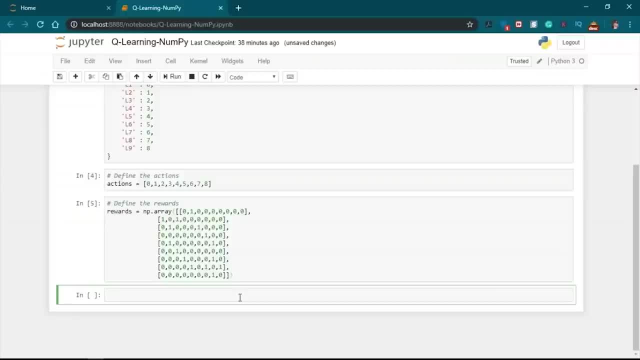 for example, the transition l4 to l1 is allowed, but the reward will be 0. to discourage that path or in tough situation, what we do is add a minus one there so that it gets a negative reward. now in the above code snippet, as you can see here, we took each of the states and put ones in the respective 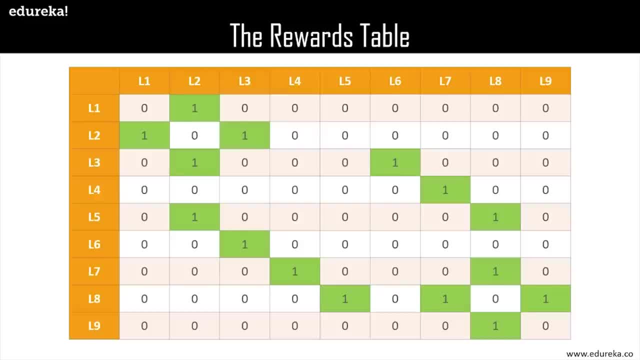 state that are directly reachable from the certain state. now, if we refer to that reward table once again which we created, the above early construction will be easy to understand. but one thing to note here is that we did not consider the top priority location l6 yet. we would also need an inverse. 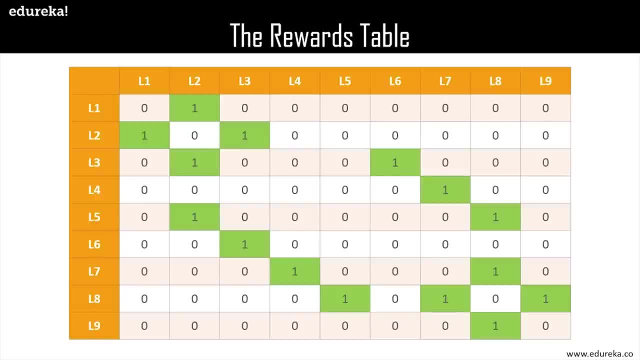 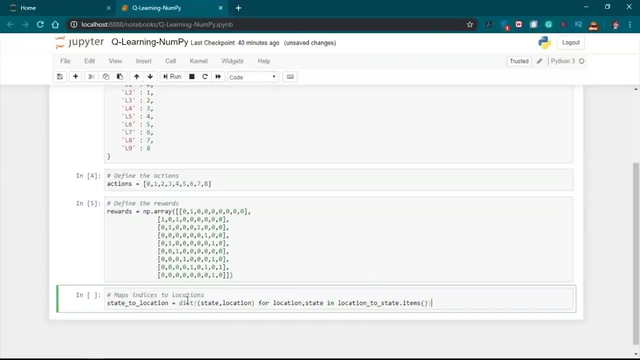 mapping from the states back to its original location, and it will be cleaner when we reach to other depths of the algorithms. so for that, what we're going to do is have the inverse map, location, state to location. we will take the distinct state and location and convert it back. 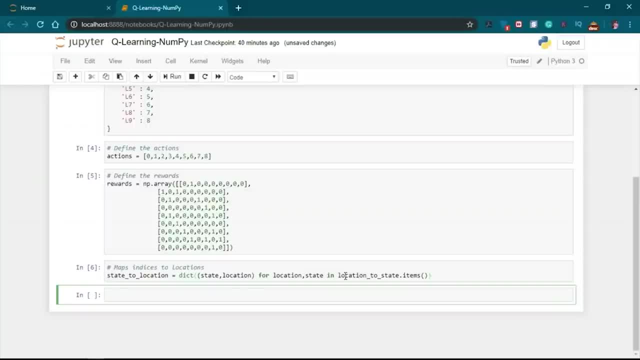 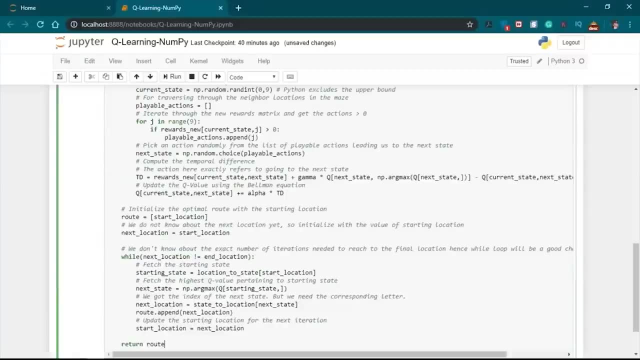 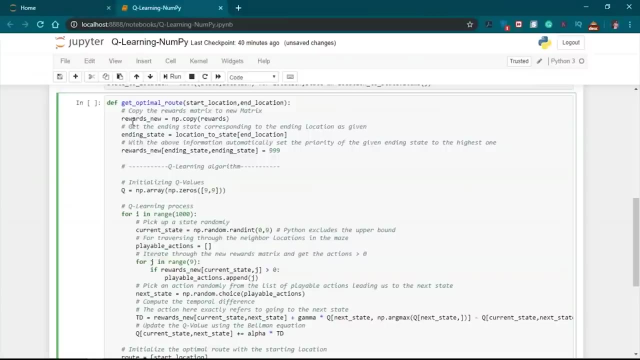 now what we'll do is we'll now define a function, get optimal, which is the get optimal root, which will have a start location and an end location. don't worry, the code is big, but i'll explain you each and every bit of the code. now, the get optimal. 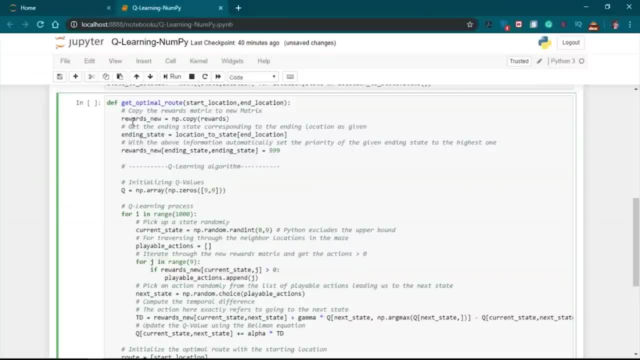 root function will take two arguments, the starting location in the warehouse and the end location in the warehouse respectively, and it will return the optimal root for reaching the end location from the starting location in the form of an ordered list containing the letters. so we'll start by defining the function by initializing the q values to be all zeros. 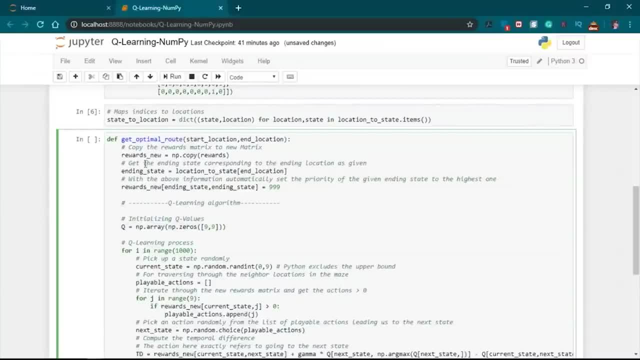 so, as you can see, here, we have given the q values to be zero, but before that, what we need to do is copy the reward matrix to a new one. so this is the rewards, new, and next again. what we're going to do is get the ending state corresponding to the ending location. 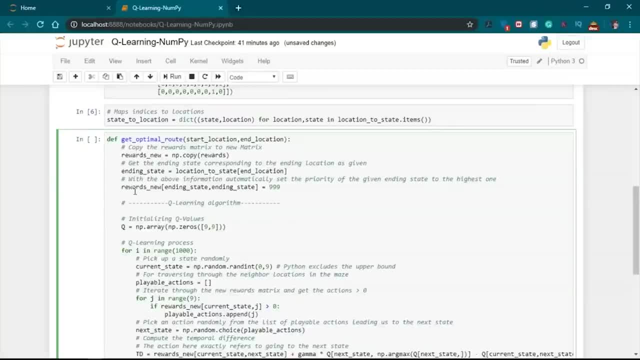 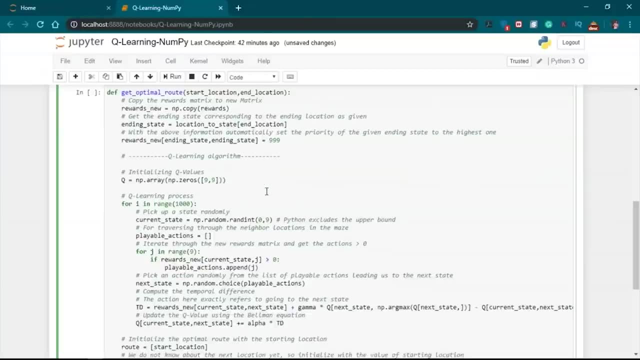 and with this information, automatically we'll set the priority of the given ending state to the highest one. that we are not defining it now, but we'll automatically set the priority of the given ending state as 999. so what we're going to do is initialize the q values to be 0 and in the q, 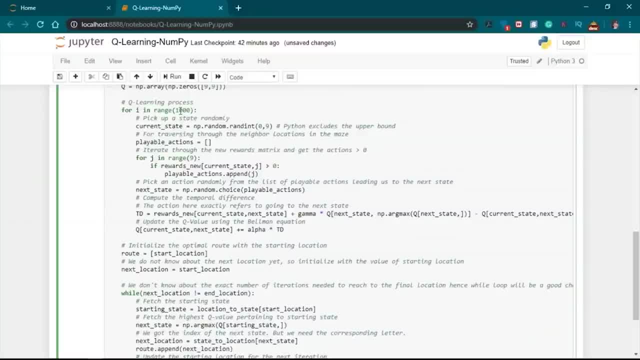 learning process. what you can see here: we are taking i in range 1000 and we're going to pick up a state randomly. so we're going to use the nprandom rand int and for traversing through the neighbor location in the same maze, we're going to iterate through the new reward matrix and get the actions which are greater than. 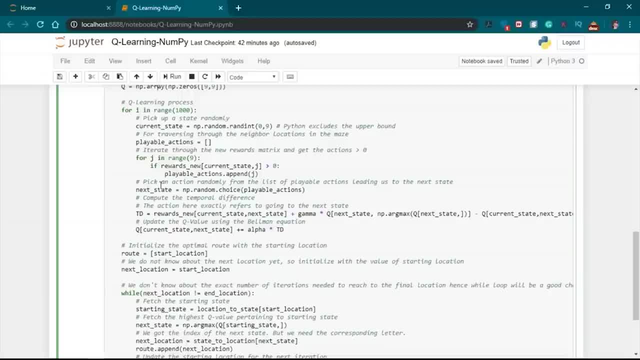 0 and after that, what we're going to do is pick an action randomly from the list of the playable actions in years to the next state. we're going to compute the temporal difference, which is td, which is the rewards plus gamma, into the q of next state and we'll take npargmax of q of next state. 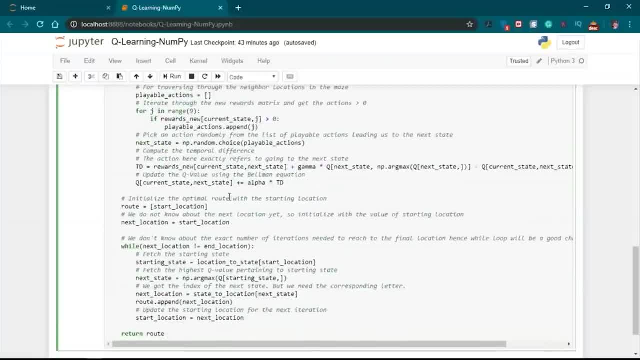 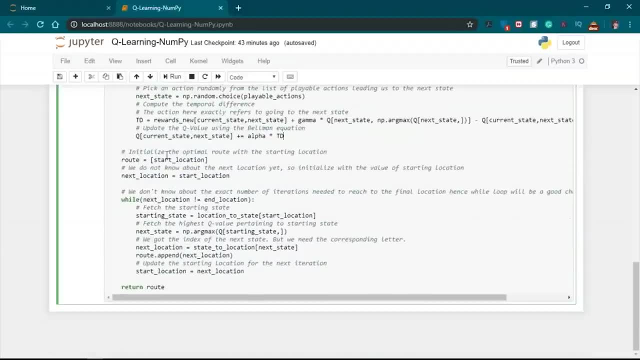 of the current state. we're going to then update the q values using the bellman equation. as you can see, here we have the bellman equation and we're going to update the q values and after that we're going to initialize the optimal route with the starting location. now here we do not know. 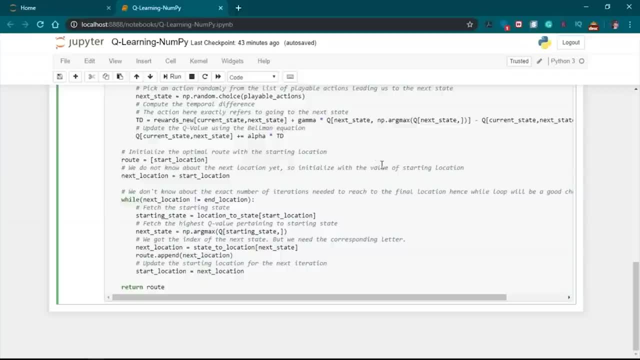 what the next location yet, so initialize it with the value of the starting location, which again, is the random location. now, we do not know what the exact number of iterations needed to reach to, while low will be a good choice for the iteration. so we're going to fetch the starting state. fetch. 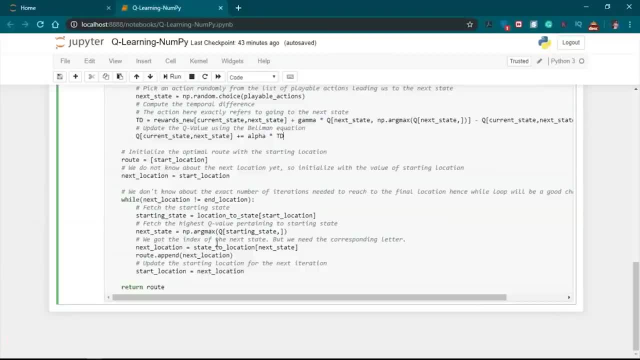 the highest q value penetrating to the starting state. we go to the index of the next state, but we need the corresponding letter, so we're going to use that state to location function we just mentioned there and after that we're going to update the starting location for the next iteration. 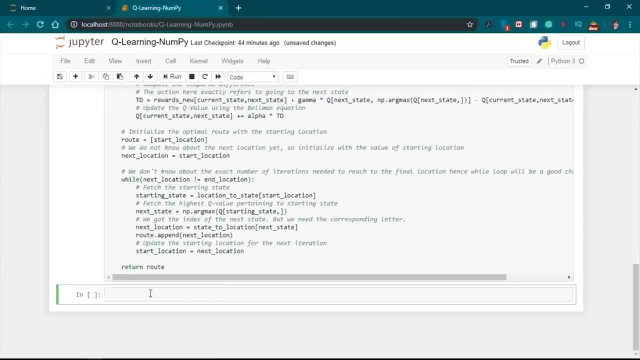 and finally we'll return the root. so let's take the starting location of n line and the end location of l1 and see what part do we actually get. so, as you can see here, we get l9, l8, l5, l2 and l1. 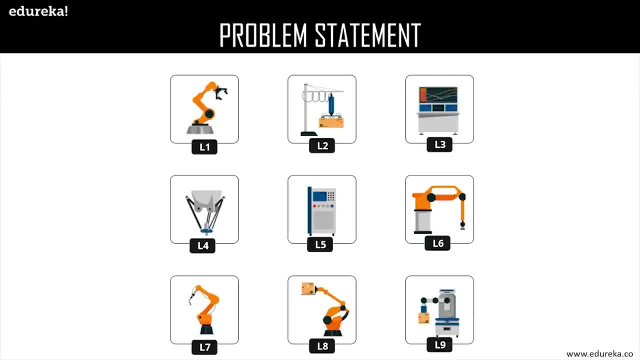 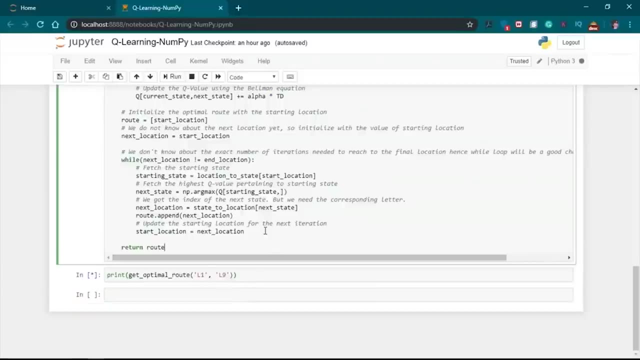 and if you have a look at the image here we have, if we start from l9 to l1, we got l8, l5, l2, l1, l8, l5, l2, l1. that would yield us the maximum value or the maximum reward for the robot. so now we have come to. 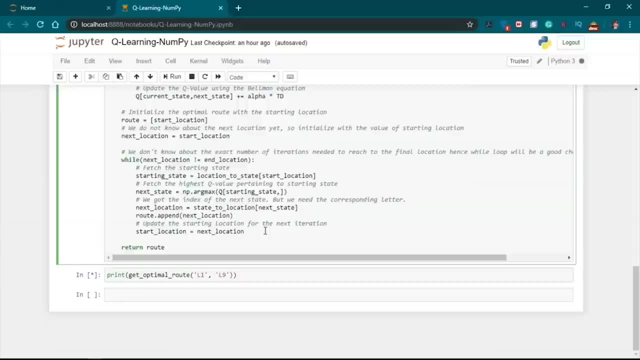 the end of our learning session and i hope you got to know what exactly is q learning, with the analogy all the way, starting from the number of rooms, and i hope the example which i took, the analogy which i took, was good enough for you to understand q learning, understand the bellman. 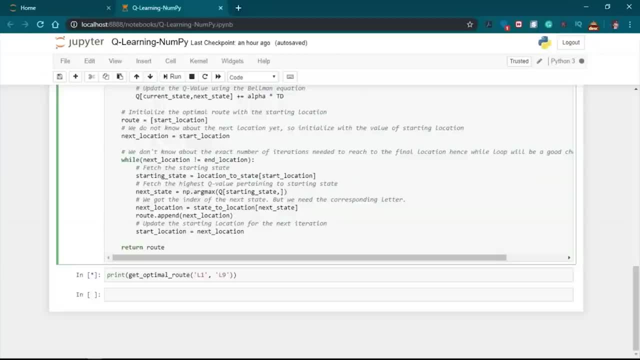 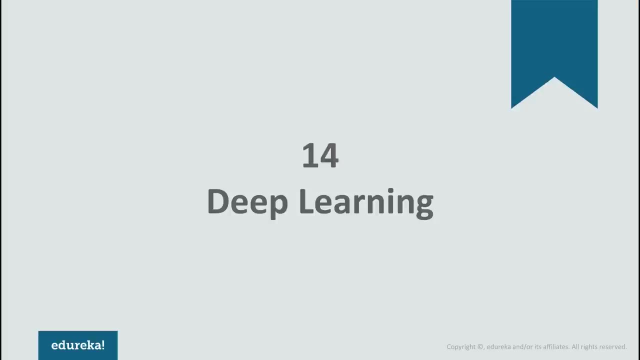 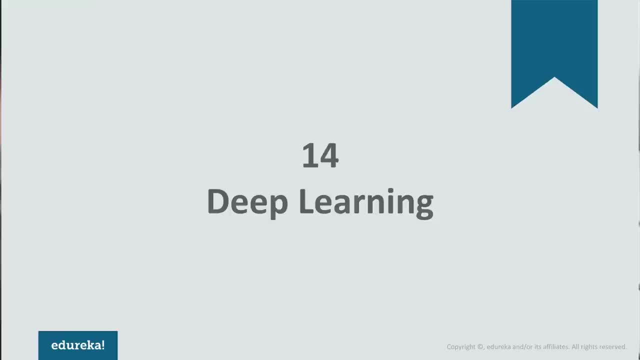 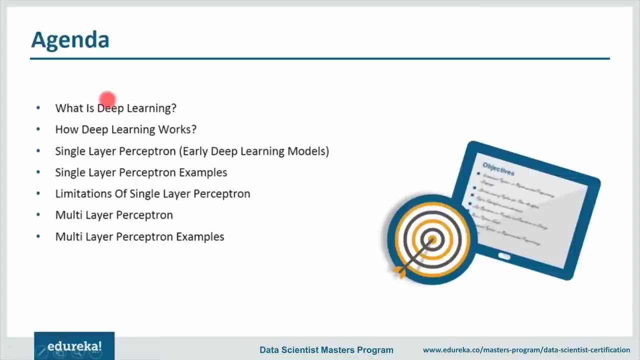 welcome to today's session on deep learning tutorial with tensorflow. so let us move forward and have a look at the agenda for today. so this is the agenda for today. guys, we'll understand what exactly is deep learning and how it works. so we'll look at the motivation behind deep learning and 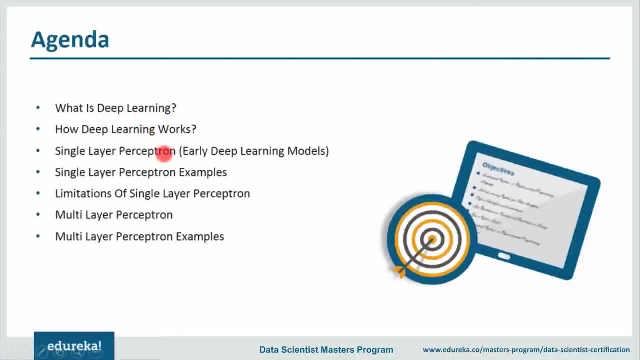 how it actually evolved. then we'll focus on single layer perceptron, which are nothing but the early deep learning models. we'll also look at various examples of single layer perception. and guys, when we talk about perceptron, these are nothing but the artificial neurons. and what are neurons? neurons? 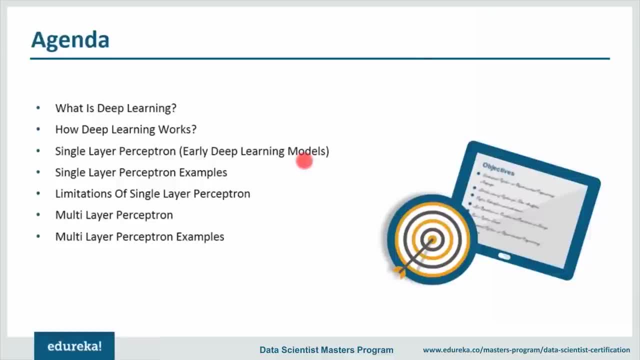 are your brain cells. then we'll also understand the limitations of single layer perceptron that led to the evolution of multi-layer perceptron. we'll understand how multi-layer perception overcame those limitations and we'll also look at various examples of multi-layer perception. in the beginning, 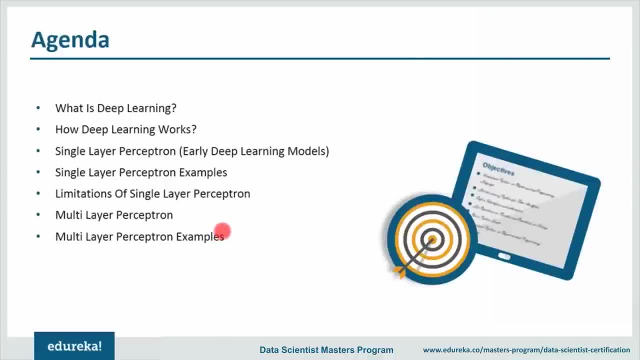 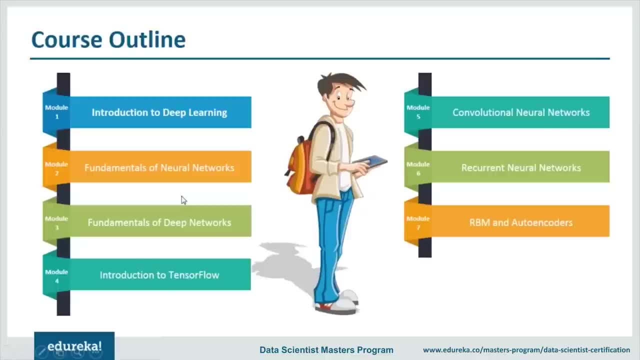 i'll be also talking about the core structure, how the course is structured, what all topics will be covered in, what all modules. so let us move forward and see how the course is structured. what are the modules? so this is how our course looks like. we'll start with the introduction to deep learning. 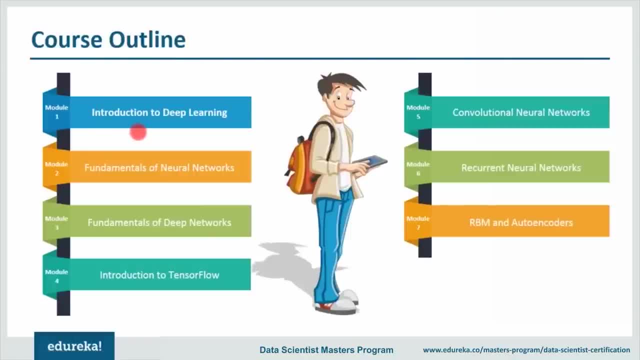 that is how deep learning evolved. what were the algorithms that were present before deep learning? then we'll understand the fundamentals of neural networks. neural networks are nothing but the networks that try to mimic your brain. then we'll understand the fundamentals of deep networks. deep networks are nothing but complex neural networks, or you can even say that these are subsets of 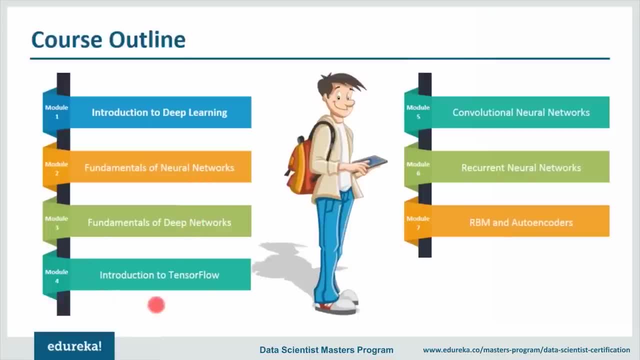 neural networks. then we'll introduce you to tensorflow, which is nothing but a library of python for deep learning. then we'll focus on various types of neural networks. first is convolutional neural networks, that is used for image recognition. then we'll focus on recurrent neural networks and 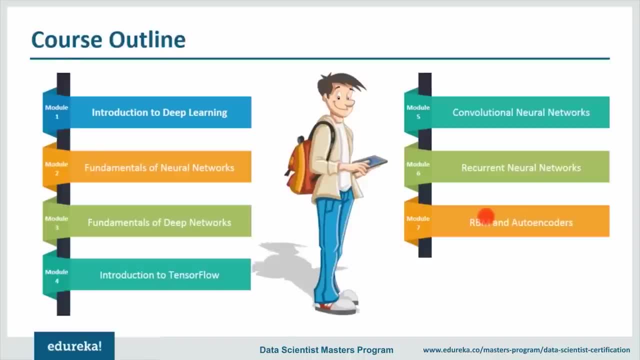 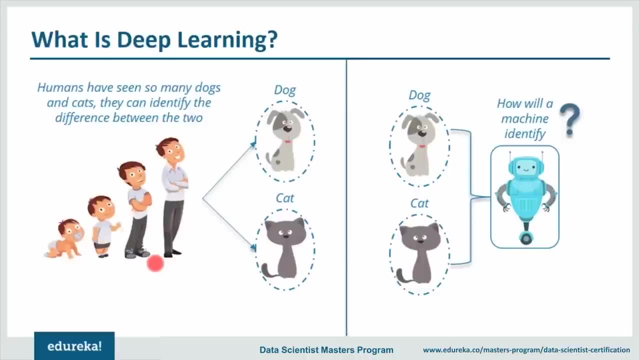 then finally, rbm and auto encoders. so this is how our course will be structured. so, guys, we'll move forward now and understand what exactly is deep learning and how it works. so, guys, let us understand deep learning with an analogy. so how do you think our brain is able to identify the difference? 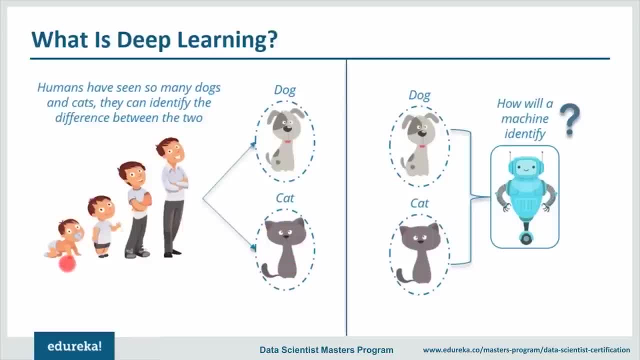 between a dog and a cat. so the reason is, since the day we are born, we are actually seeing different types of cats and dogs in our day-to-day life and because of that we are able to identify the difference or spot the difference between the two, that is, dog and a cat. 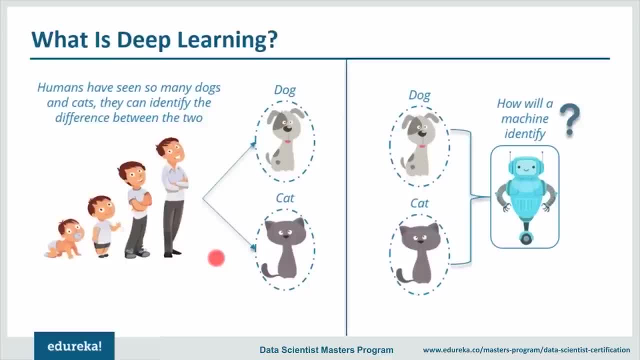 even if we see different types of cats and dogs, we still know which is a cat and which is a dog. so this is because we have seen a lot of cats and dogs in our entire life. but what if i want a machine to do that task for me? 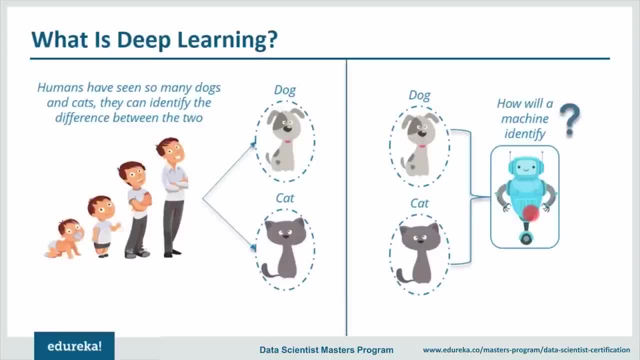 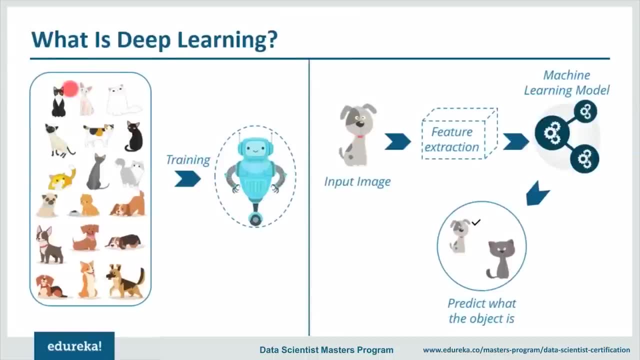 so how will a machine identify whether the given image is of a dog or a cat? so one way of doing this is we can train our machine to a lot of images, a lot of images of different cats and dogs, that is, different breeds of cats and dogs. and then what will happen once our training is done? 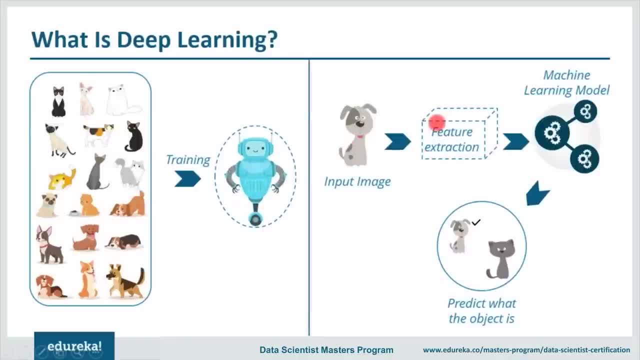 we can provide it with an input image, then we'll manually extract certain features, features like nose, whiskers, colors, edges, it can be anything, the important features, which actually helps us in classifying whether the input image is a cat or a dog. then we make a machine learning. 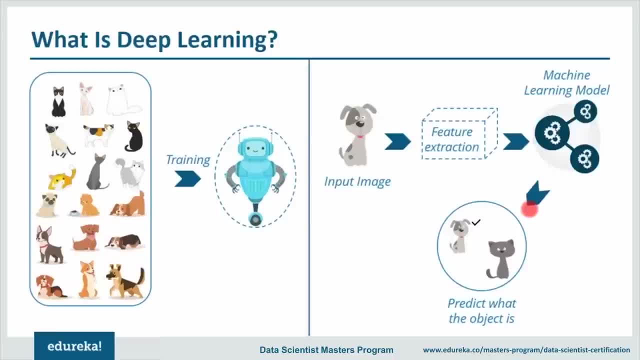 model. with that and once it is done, our machine learning model is able to predict whether the input image is of a cat or a dog. but if you notice here, one very big disadvantage with this is we have to manually extract features, features such as nose whiskers, all those features we have to manually extract it. 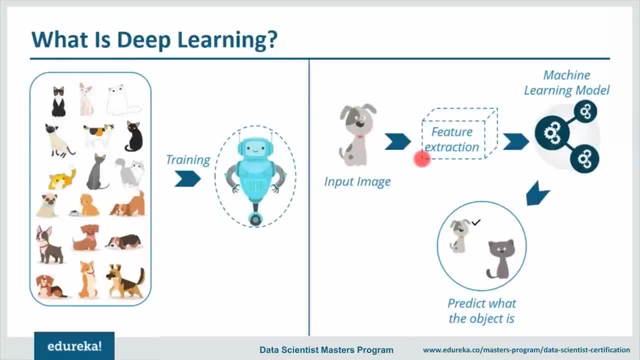 and provide it to our machine learning model. and trust me guys, in every scenario it is not possible. if you have large number of inputs, you cannot do that. you cannot manually extract the features or basically, you can say columns which are important to you, for you, in order to predict what the object is right. and that led to the 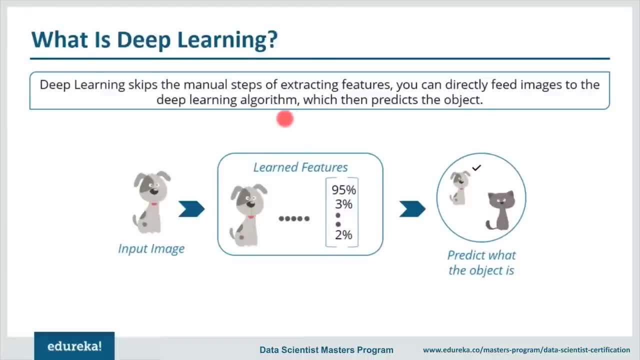 evolution of deep learning. so what happens in deep learning? we skip the manual step of feature extraction. so what we do? we directly take the input image and feed it to our deep learning algorithm. and because of that, what happens? whatever features are we already manually provided. apart from that, there 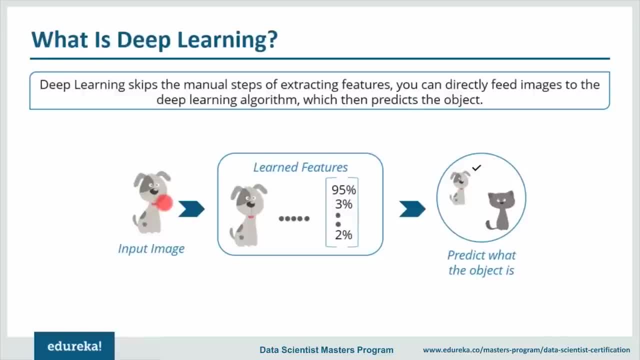 might be many other features which are important. for example, if our features don't include the length of the neck, and that is one of the major feature in order to identify or classify whether it is a cat or a dog, now what will happen? our algorithm will automatically determine that feature and will take 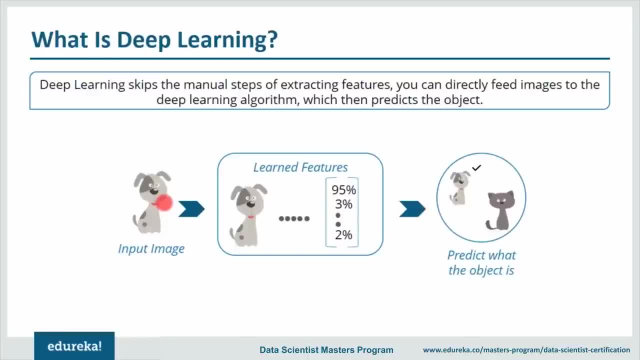 into consideration and then it will classify whether the input image is a cat or a dog. so what happens here? we provide an input image of a dog and then it will automatically learn certain features, even if we don't provide it with those features, and after that it will give us the probability and 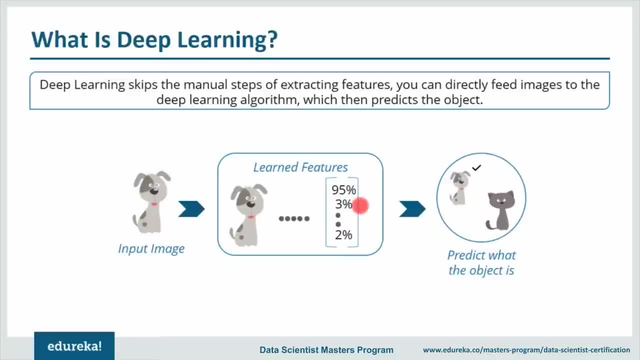 according to this particular scenario, it says 95% chances of being a dog, 3% chances of some other animals. similarly, 2% chances of some other animals. so since the highest probability goes with the dog, so the prediction says that the object or the input image is 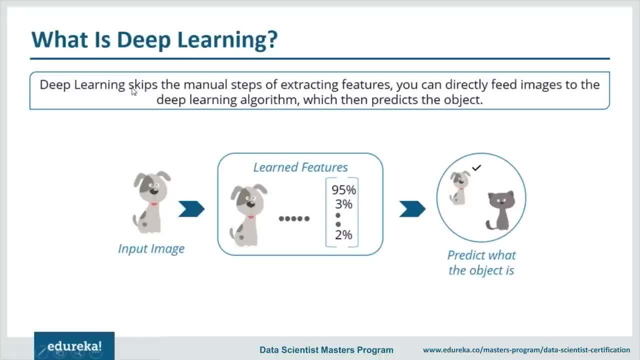 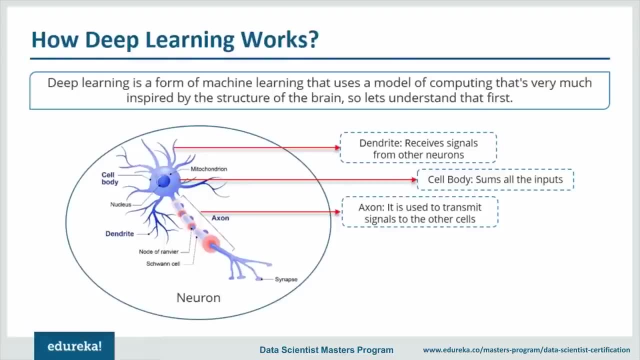 nothing but a dog. fine guys. so we'll move forward and we'll understand how exactly deep learning works. so the motivation behind deep learning is nothing but the human brain, as we have seen in the previous analogy as well. what we are trying to do, we are trying to mimic the human brain. we are trying 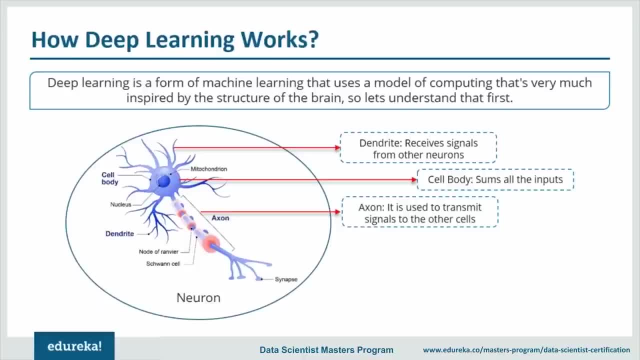 to mimic the way we think, the way we take decisions, the way we solve problems. we are trying to make sure that we have a system that can mimic our own brain. so obviously the motivation for deep learning has to be our brain and how our brain work with the help of our brain. 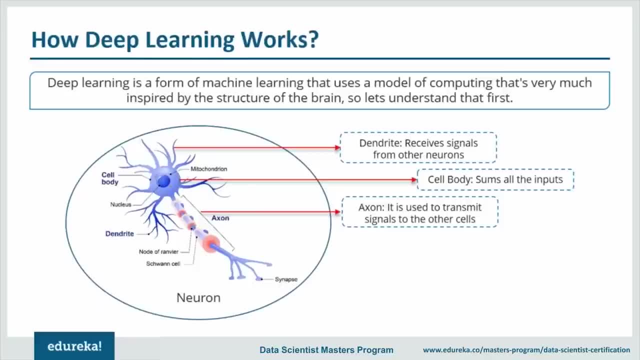 cells, which we call neuron. now let us understand how a neuron works, and let me tell you guys, this is what we think how a neuron works. this is what our studies tell us. so yeah, so these are called dendrites. so dendrites receive signals from other neurons and then it passes those signals. 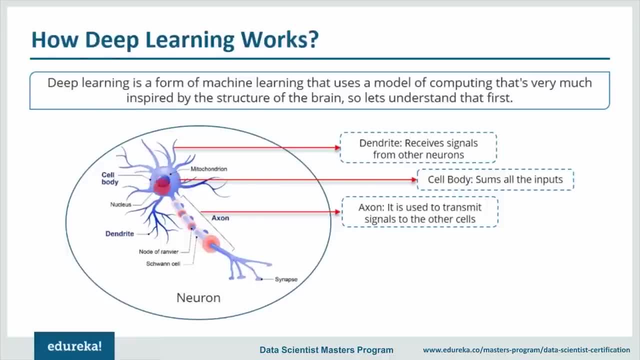 to the cell body. now, this cell body is where we perform certain function. it can be a Sigma function, that's what we believe. we believe it performs Sigma function. that is nothing but sums all the inputs. then, through exon, what happens? these signals are fired to the next neuron, and the next neuron is present at some distance, and that distance is. 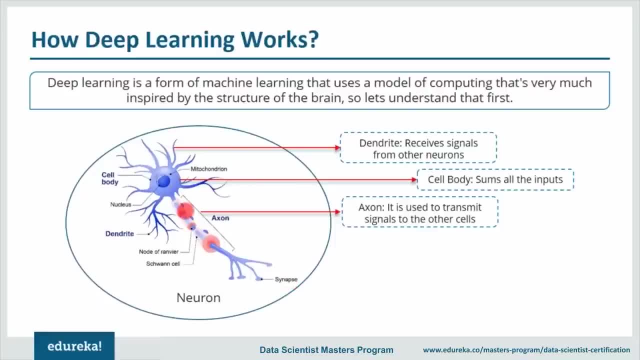 nothing but synapse. So it fires only when the signals coming from the cell body exceeds a particular limit. then only the cell or this neuron will fire the signals to the next neuron. and this is how the neuron at the brain cell works, and we take the same process forward and we try to create 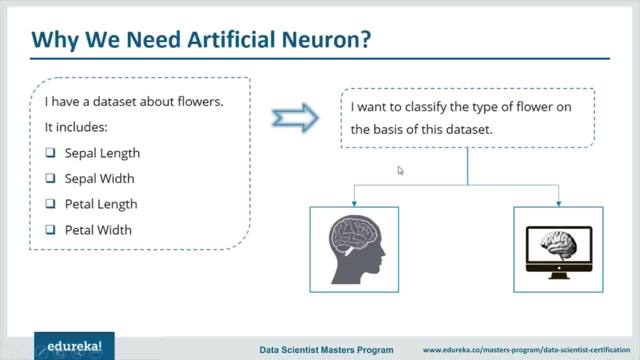 artificial neurons. So let us understand why we need artificial neurons. with an example: So I have a data set of flowers, say, and that data set includes sepal length, sepal width, petal length and petal width. Now what I want to do? I want to classify the type of flower on the basis of this. 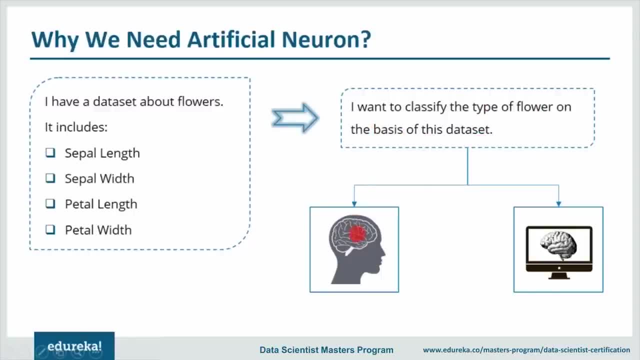 data set. Now there are two options. either I can do it manually- I can look at the flower manually and determine by its color or any means- and I can identify what sort of a flower it is- or I can train a machine to do that. Now let me tell you how to do that. 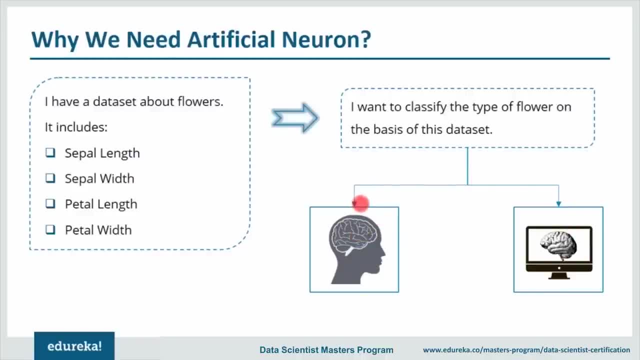 Let me tell you the problem with doing this process manually. First of all, there might be millions of inputs that will be given to you, and for a human brain to perform that particular task is next to impossible. and at the same time, we always get tired at some point of time, right? So we cannot just 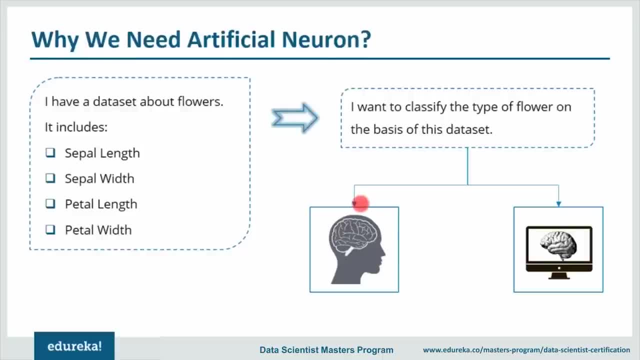 continue working for a long period of time in single stretch. and the third point is human error risk, which is always there. So these are a few limitations with the human brain. So what we can do, we can train a machine to do that task for us, or we can put our brain inside a machine So we 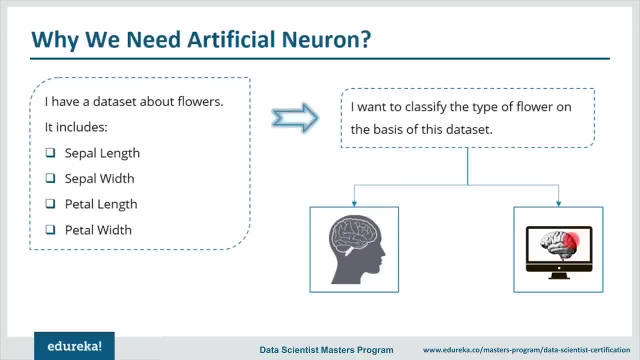 can train a machine to do that task for us, so that it can classify the flowers for us. So, with this, what will happen? the machine will never get tired and it will make better predictions as well. So this is why we create artificial neurons, so that there's a system present that can mimic our brain and this 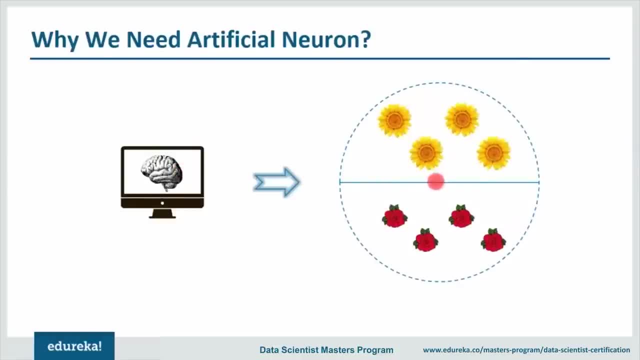 is how this is what exactly happens. So this particular artificial neuron can actually classify the flowers, or you can say, can divide the flowers on the basis of certain features. In our case it is separate length, separate width, better length and better width, So we can classify the two flowers. So what we need here? we need some sort of a system that can actually 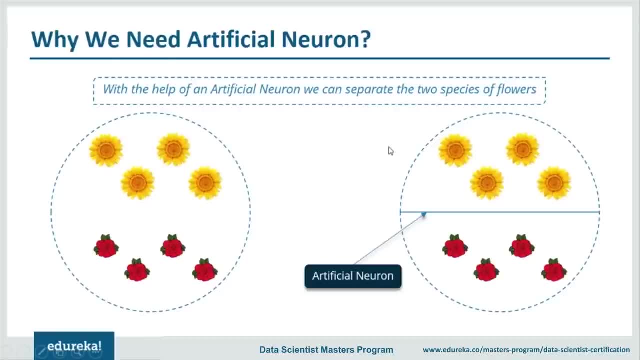 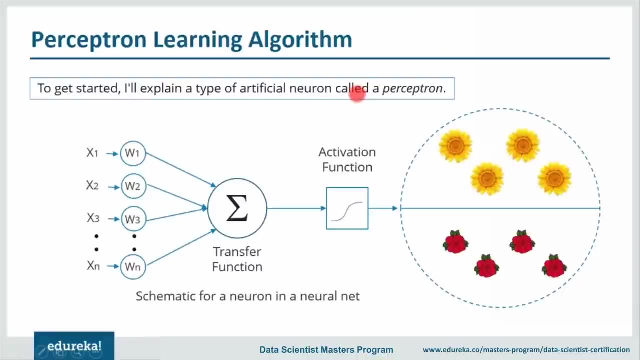 separate the two species. and what is that system is nothing but an artificial neuron. So we need artificial neuron, and one type of artificial neuron is a perception. Now let me explain you perception with the flow diagram that is there in front of your screen. Now, over here, what happens? we have set. 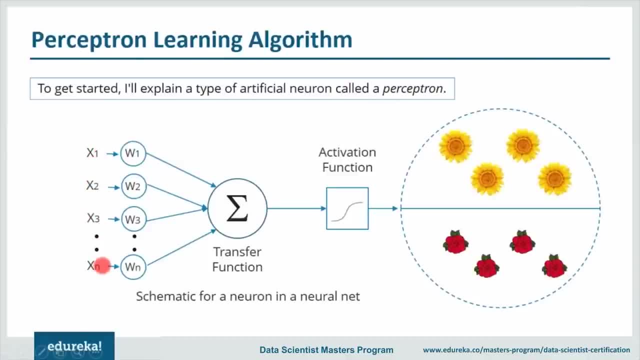 of inputs like X1, X2, dash, dash, dash till XF. Now these inputs will be multiplied with their corresponding weights, which is W1, W2, W3 till XF. So we can see that the inputs are multiplied with their corresponding W1 in our case. Now these weights actually define how important our input is, So the value of weight is: 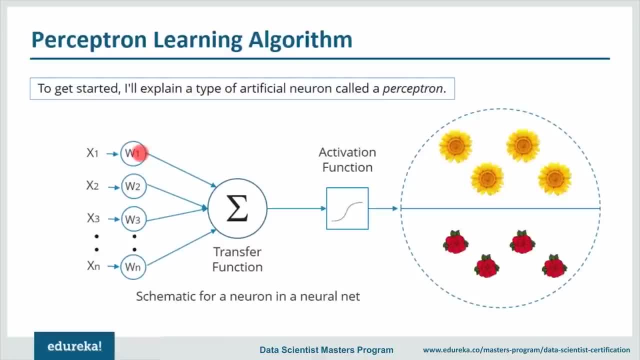 high. We know that this particular input is very, very important for us. After multiplication, all of these are summed together and then it is fed to an activation function. Now, the reason of using activation function is to provide a threshold value. So if our signal is above that threshold value, a neuron or you 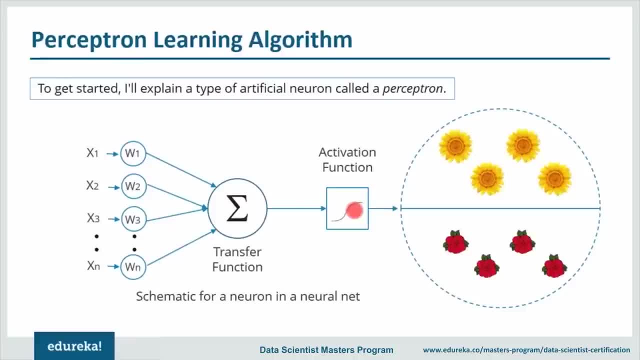 can say our perceptron will fire, else it won't fire. So that is the reason why we use an activation function. There can be different types of activation function. there can be sigmoid, there can be step function, sign function. depending on our use case, we define the activation function. Now, the main idea was to define an. 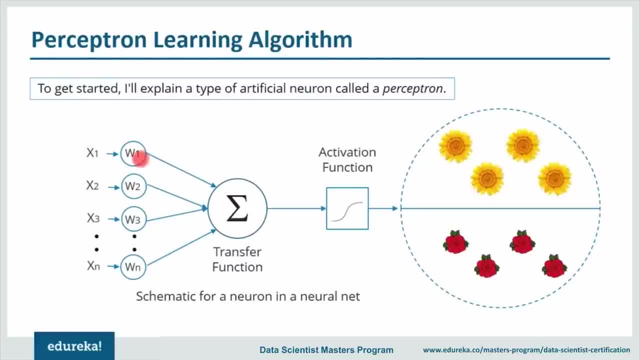 algorithm in order to learn the values of the weights, which are W1, W2, W3 in our case, to learn the values of the weights that are then multiplied with the input features in order to make a decision whether a neuron fires or not, In context of pattern classification, which is, in our case, flowers. So we are trying to 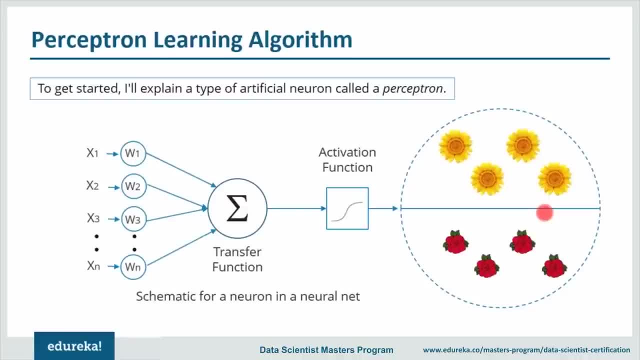 classify the two species of flowers. Such an algorithm could be useful to determine if a sample belongs to one class or one type of a species, or another class or another type of the flower. We can even call perceptron, as a single layer, binary linear classifier, to be more specific, because it is able to classify inputs which are linearly separable, and our 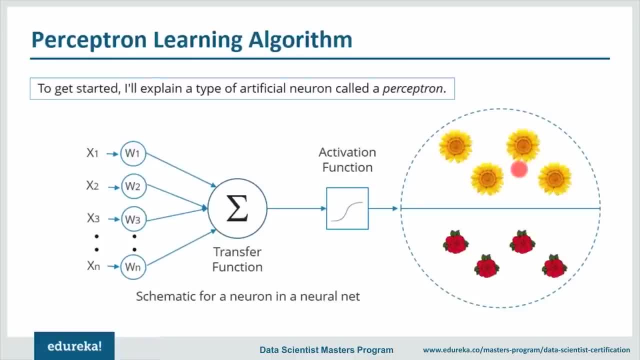 main task here is to predict to which of the two possible categories a certain data point belongs, based on a set of input variables. Now there's an algorithm on which it works, So let me explain you that the first thing we do is we initialize the weights. 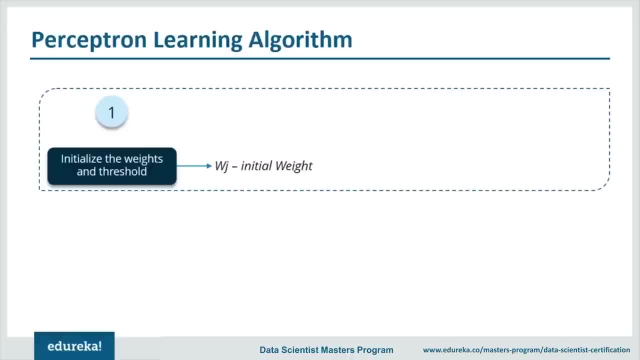 and the threshold. Now, these weights can actually be a small number or a random number, and it can even be zero. So it depends on the use case that we have. Then what we do: we provide the input and then we calculate the output. Now, when we are training our model or we are training our artificial neuron, we have the output values for a. 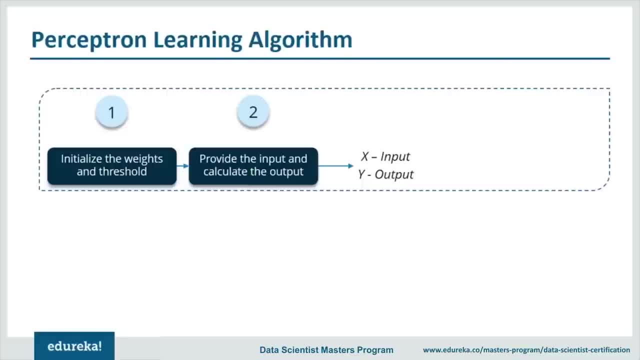 particular set of inputs. So we know the output value. but what we do, we give the input and we see what will be the output of our Particular neuron and accordingly we need to update the weights in order to reduce the loss, or you can say, in order to 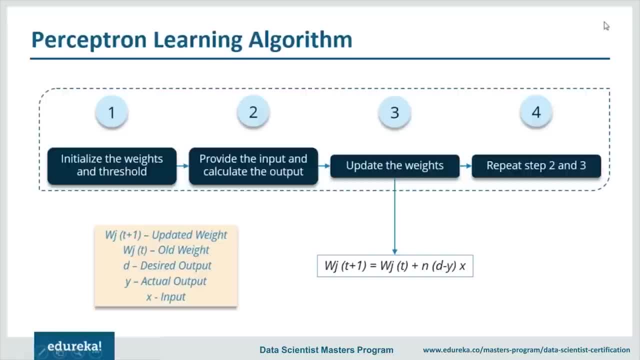 reduce the difference between the actual output and the desired output. So what happens? Let me tell you that. So we need to update the weight. So how we are going to update the weight is we can say the new weight is equal to the old weight plus the learning. 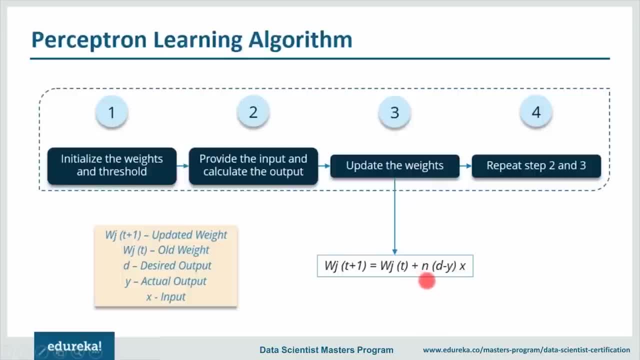 rate. learning rate will discuss about it later in the session, But generally we choose learning rate somewhere between point five to point zero one. After that what happens? we find the difference between the desired output and the actual output, and then we multiply it with the input. 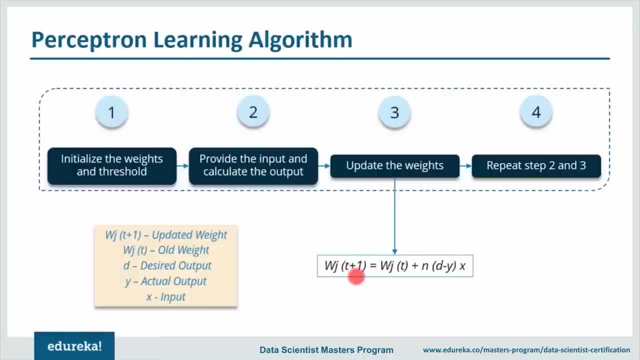 So on that basis, we get a new weight. So this is how we update the weights and then what happens? we repeat the steps two and three. So we are going to repeat the steps two and three, that is, we are going to apply this new weight again. 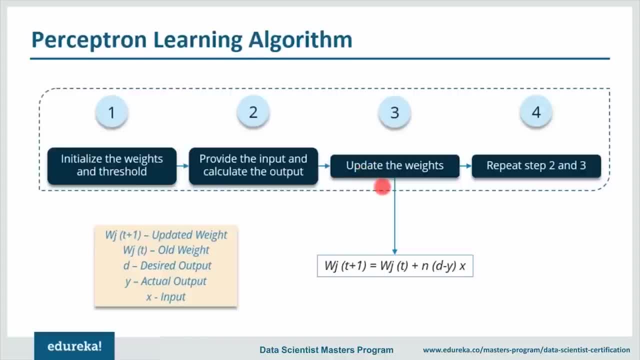 We are going to calculate the output again, We are going to compare it with the desired output and if it matches, then it's fine. Otherwise we are going to update it again. So this is how the whole perceptron learning algorithm works. and don't worry, guys. 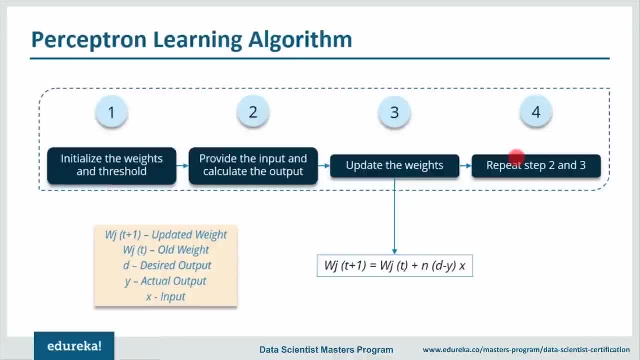 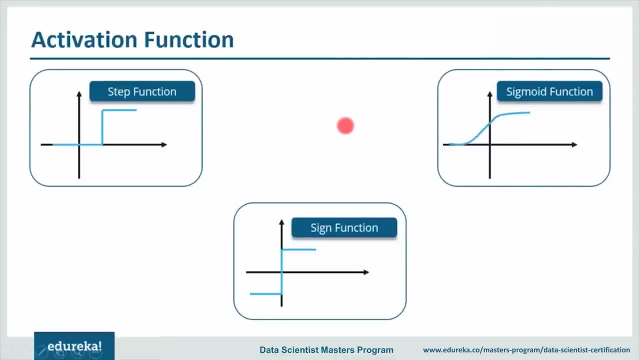 I'm going to show it to you practically how it actually works in my Fine guys. So we'll move forward and we'll see the various types of activation functions. So these are the various types of activation functions that we use, Although there can be many more activation functions again. 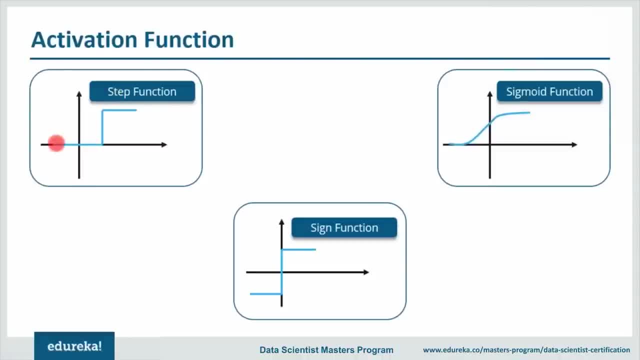 I'm telling it depends on your use case. So we have a step function. So if our output is actually above this particular value, then only a neuron will fire, or you can say the output will be plus one, or if it's less than this particular value, 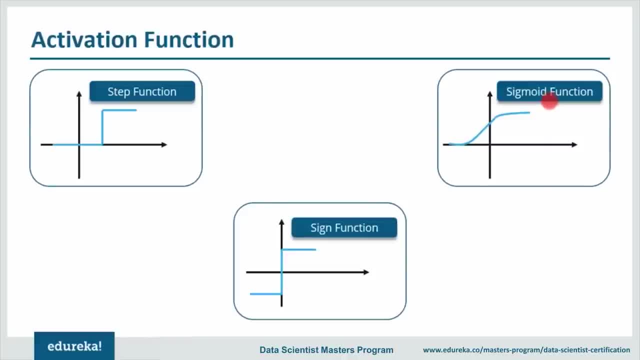 then we'll have no output, or we'll say zero output. similarly for the sigmoid function as well, and same goes for sine function. So let us move forward and we'll focus on various applications of this perceptron Now, as I've told you earlier as well. 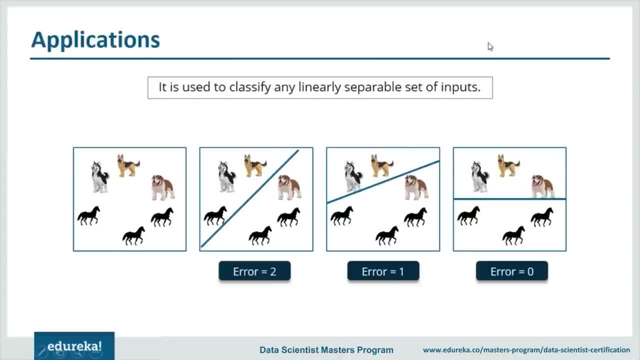 it can be used to classify any linearly separable set of inputs. Now let me explain to you with the diagram that is there in front of your screen. So we have different types of dogs and we have horses and we want a line that can separate these two. 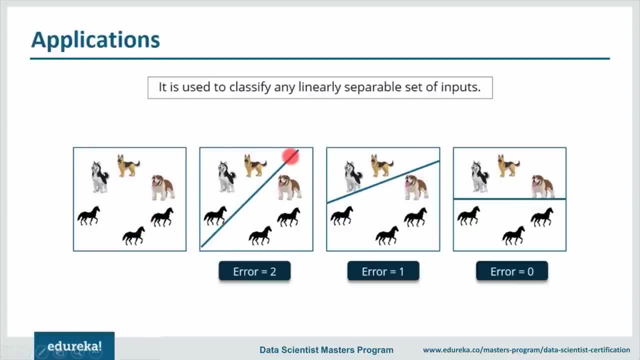 So our first iteration will produce this sort of a line. But here we can notice that we have error here, as we have classified horse one of the horses as a dog and a dog as a horse. So error is two here. Similarly, we now what happens. we have updated the weights now. 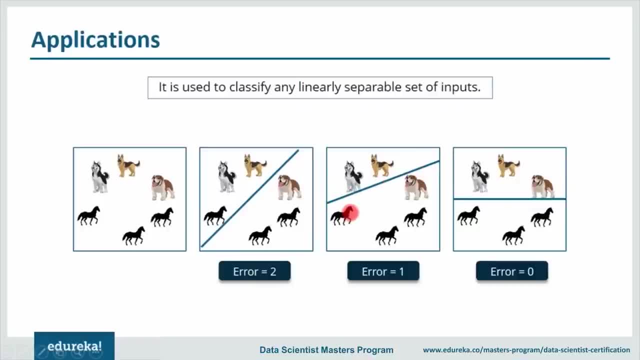 after updating the weight, what happens? our error has reduced. So what happens now? we have actually classified all the horses correctly, but one dog we have classified wrong and we have considered it as a horse, So our error becomes one once again. what will happen? if you can remember the step two? 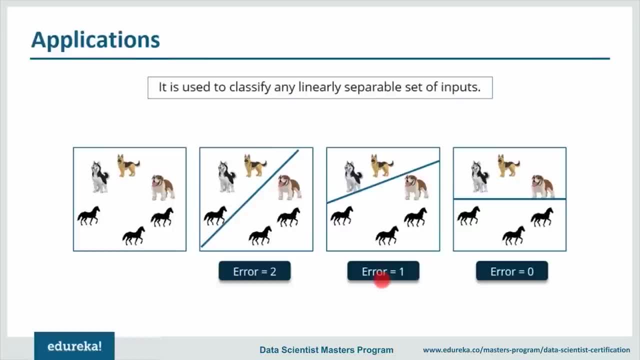 and three of a perceptron learning algorithm will be done, and then, after that, our weights will be updated and our desired output will become equal to our actual output, and we get a line something like this: So what we have now: we have properly classified dogs and horses. 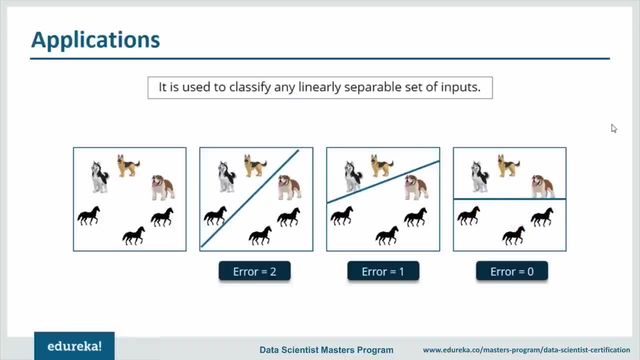 So this line separates both of them. This is how we can actually use a single layer perceptron in order to classify any linearly separable set of inputs. Now we can even use it in order to implement a logic gates that is or and and. now. 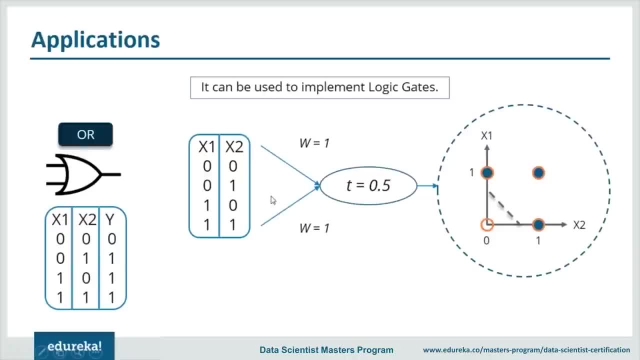 let me tell you how you can do that. first, We'll look at our gate now. in our gate, What happens here is the truth table. truth table: According to that, we have two inputs: x1 and x2.. So if both are zero, we get a zero. 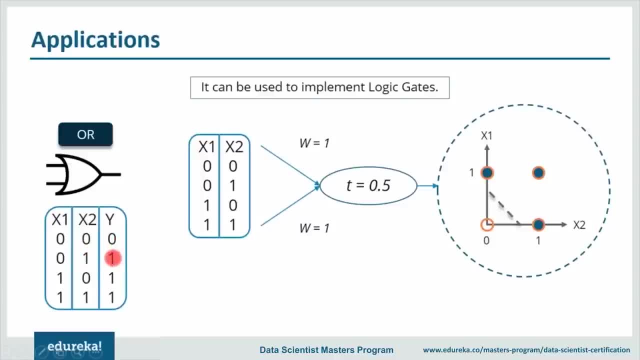 If any one of the input is high, or any one of the input is one, we get the output as one. So what we need to do is we need to make sure that our weights are present in such a way that we get the same output. 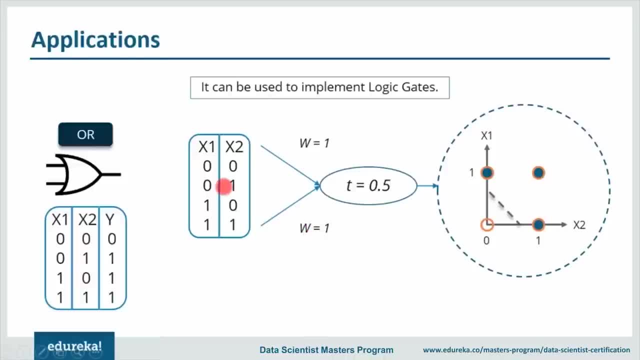 So how we have done that, when the value of weight is equal to one, and then we provide the input x1 and x2, after passing through this activation function, we get this sort of a graph, which is the graph for our order, a gate. Now, if you want, I could use a pen and I can explain it to you. 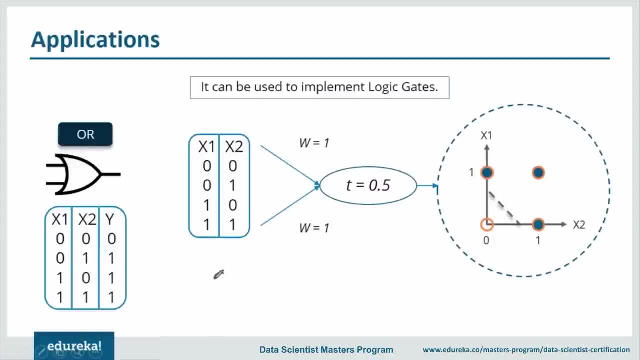 Now we have x1, x2 as inputs, So we provide first input as 0, x1 and this also as 0, so 0 into 0 is again 0, 0 into 0 is 0, and then we passes through this activation function. 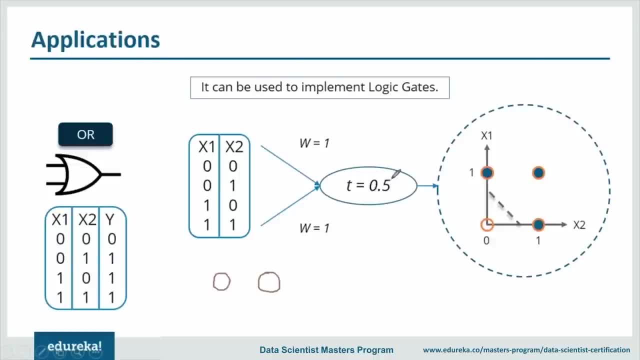 Now we need to make sure that whatever value that comes here should be greater than 0.5. then only our neuron, or the perception, will fire, But since this value is actually less than 0.5. So the neuron won't fire and our output will be 0, as you can see it over here. 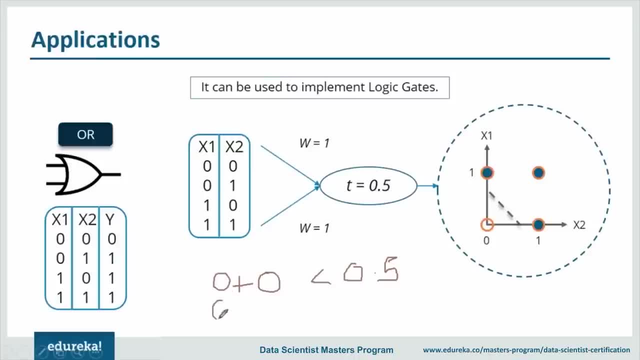 Now let's take the other set of inputs. Now our x1 is 0 and our x2 is 1, so 1 into 1 will what will be obviously 1.. Now, in this case, our output is bigger than 0.5.. 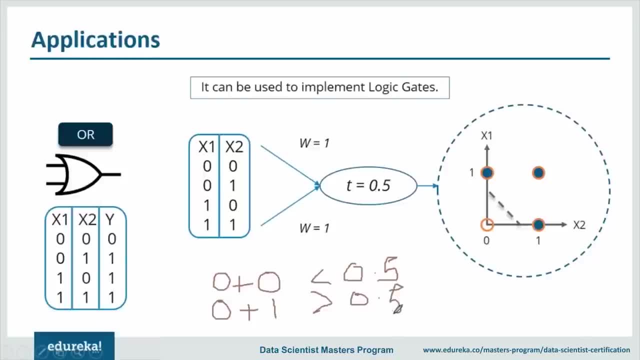 Then what will happen? our neuron will fire and we'll get 1, the output 1 here, as you can see it in the graph. Similarly, when my x1 is 1 and x2 is 0, in that case also, our output is greater than 0.5. 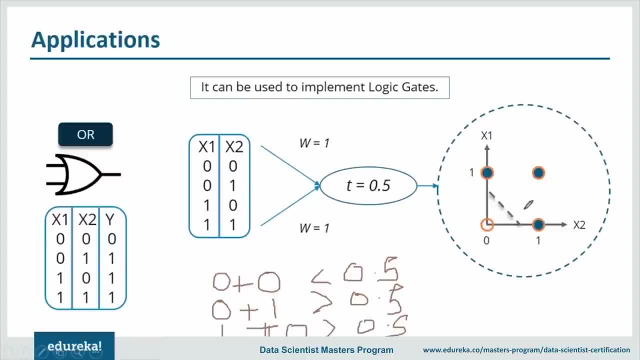 and neuron will fire And we'll get this sort of a graph. when I talk about 1- 1, then our output will be 2, which is greater than 0.5.. So we get an output that is 1, and this is how we get the graph. 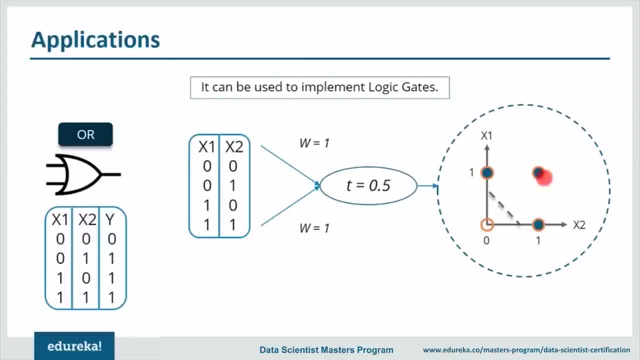 So this is how we get this graph. And now, if you notice, with the help of the single-layer perceptron, we are able to classify the ones and zeros. So this line, anything above this line, is actually 1 and anything below this line. 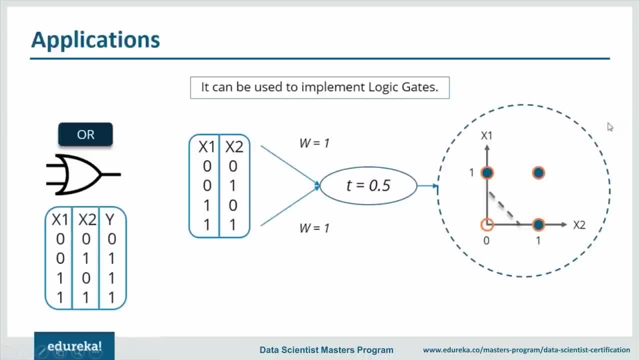 We have zeros. So this is how we are able to classify or able to implement or gate, Similarly when I talk about and gate as well. So there's a difference in the truth table of and gate in and gate What happens. We need to make sure that both of our inputs are high in order to get a high out. 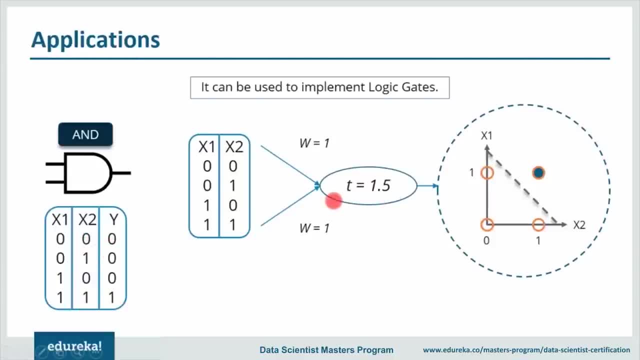 If any of the input is low, we get a low output, And that's the reason we choose an activation function that is 1.5, which means that if our value or the output is about 1.5, then only our neuron will fire and we'll get one here. 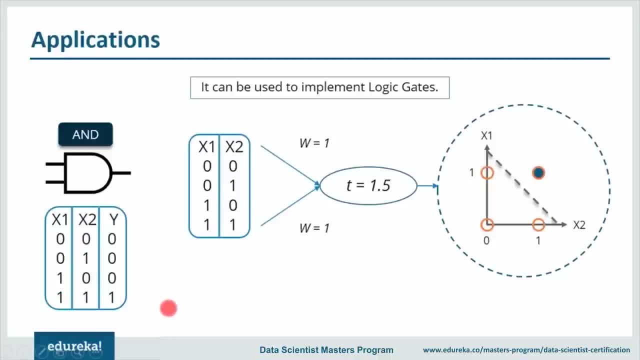 And there's only one case, that is when both the inputs are high. So when both the inputs are, I let me just use my pen again and I'll explain to you. So x1 is 1, x2 is 1, we get something which is 2, which is obviously greater than 0.5. 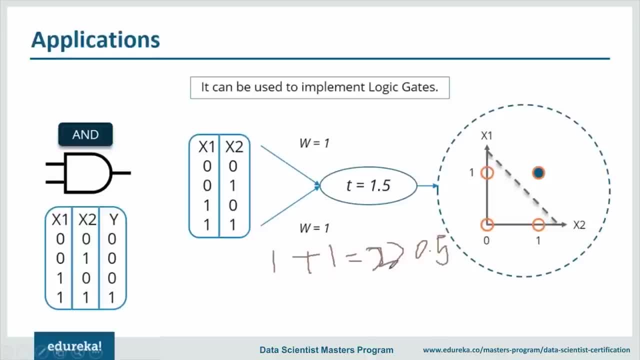 Pardon me for my writing, But yeah, this is how it is. Yeah, so 1 plus 1, 2, which is obviously greater than 0.5.. So what we get, we are neuron fires and we get one here, but for the rest of the inputs, all will be less than 1.5.. 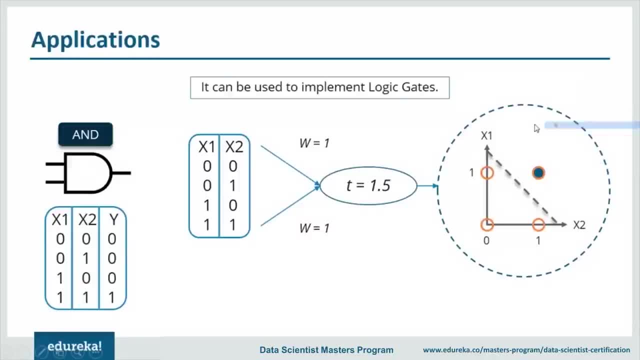 So that is why our neuron doesn't fire and we get a zero output. Don't worry, guys, I'll actually tell you how to implement it. I'll open my pie charm and I'll be showing it to you practically how to implement these. 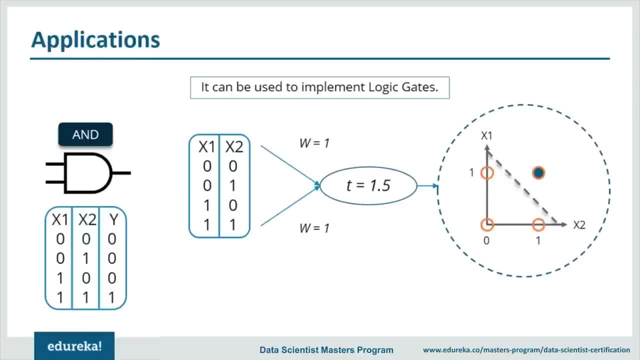 Gates. So for that, what I'm going to do is I'm going to first import a python library called tensorflow. the installation guide of this particular library is present in an LMS for both Windows as well as for Linux, So you can just go through it and it's very easy to install that. 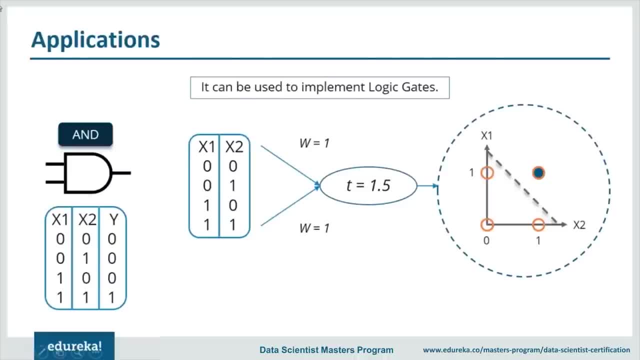 and I'll actually execute this practically later in the session. You don't need to worry about it. This is how we can implement and and or get. so let's move forward, guys, and we'll actually understand a use case, that is, of MNIST data set. 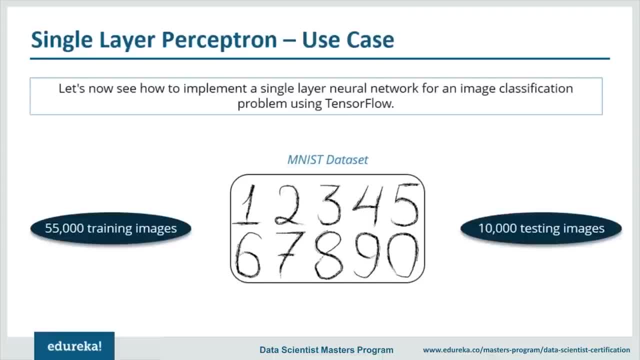 The reason for using MNIST data set is because it is already clean and will be a perfect example for this. now what this MNIST data set contains. It basically contains handwritten digits from 0 to 9, and in that data set We have 50,000 training images, along with 10,000 testing images. 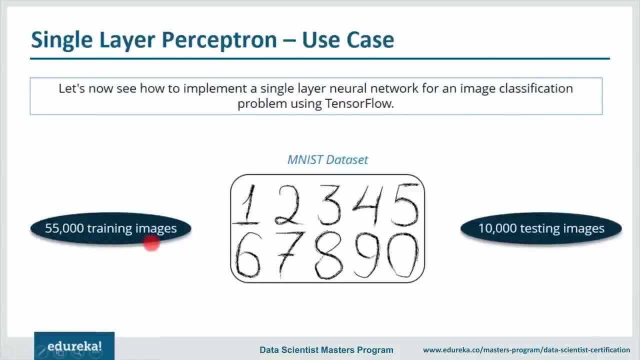 So we will train our model with those 55,000 training images, and then we are going to test the accuracy of a model with the help of those 10,000 testing images. and for all of this we need to understand first What exactly is tensorflow? 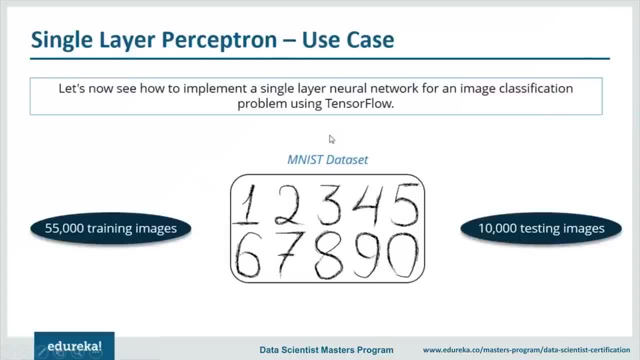 So let us move forward, guys, and will understand tensorflow, and then we are going to implement all these things that we have discussed, that is, and gate or gate and the MNIST data set that I'm talking about. So let's move forward, guys, and understand what exactly is tensorflow. 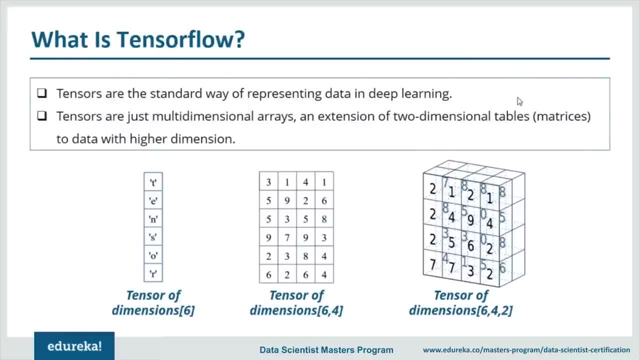 Now, what is tensorflow? as I've told you earlier as well, We use this tensorflow library in order to implement deep learning models, and the way the data is represented in the deep learning model is called tensors. Now, what are tensors? now, tensors are just the multi-dimensional arrays. 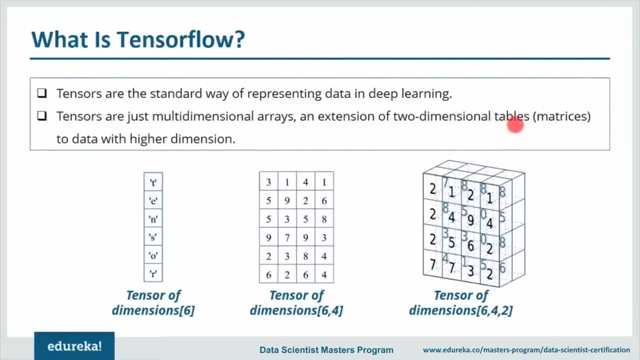 or you can say an extension of two-dimensional tables, matrices, to data with high dimension. Now let me explain you with the examples that are there in front of your screen. So this particular data is nothing but a tensor of dimension 6, because we have six rows. 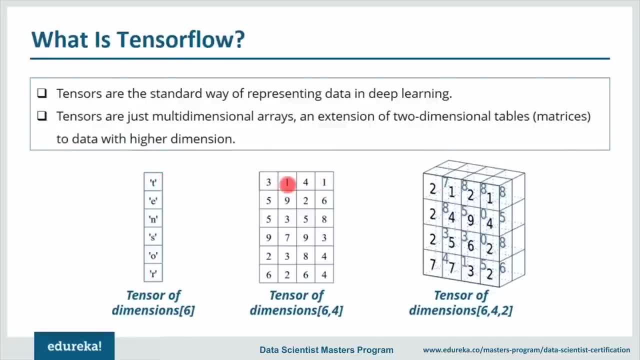 and we have only one single column. now over here We have four columns as well as six rows, So this becomes a tensor. of dimension 6 comma 4, similarly over here as well. So we have another dimension, that is the third dimension, in which we have two values. 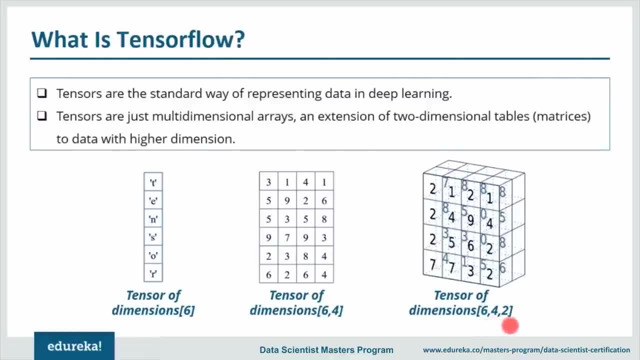 So we consider this as a tensor of dimension 6, 4 and 2, so this is nothing but a way of representing data in tensorflow. Now, if you consider the tensorflow library at its core, it is nothing but a library that performs Matrix manipulation. 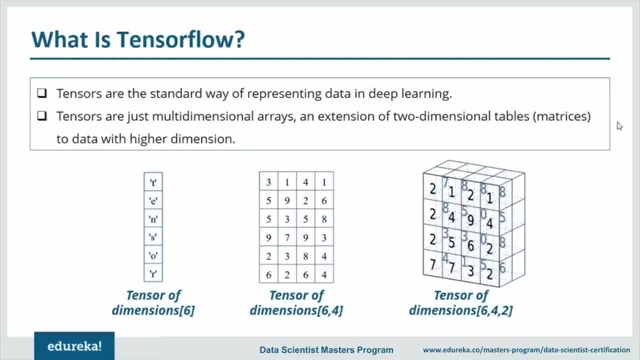 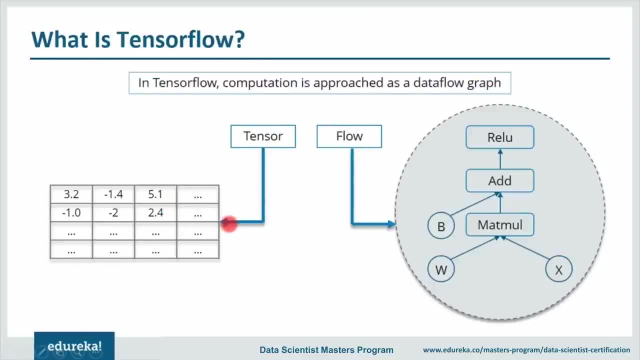 That is what tensorflow is. now Let us move forward and understand tensorflow in a bit detail. So, as the name tells that, it consists of two words: tensor as well as flow, now we understood what exactly tensor is. We saw it in the previous slide as well. 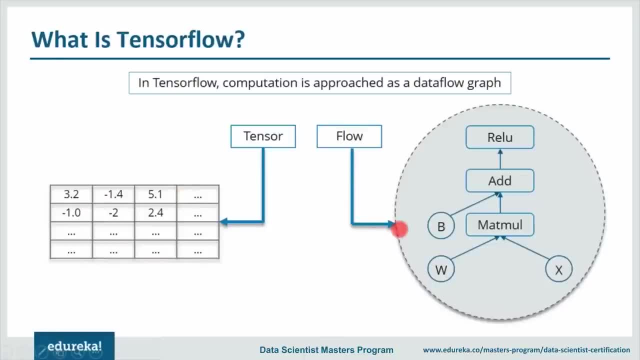 Now, when I talk about flow, it is nothing but a data flow graph. So let me just give you an example that is there in front of your screen. So we talked about weights and inputs. So we provide these weights and inputs and we perform a matrix multiplication. 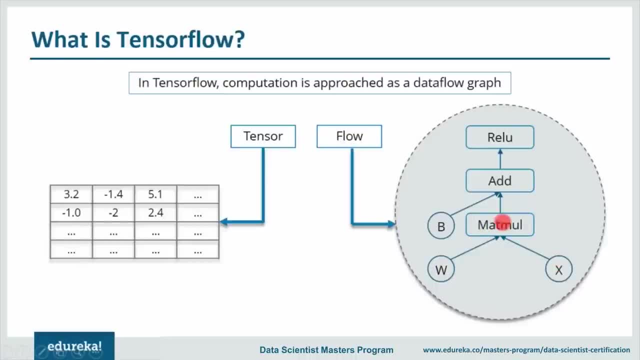 So it's: beta is one tensor, X input is one tensor. Then we perform Matrix multiplication. after that, We add a bias, which will actually see it later in the session. You don't need to worry about this term. Then what we do? we add all of these. 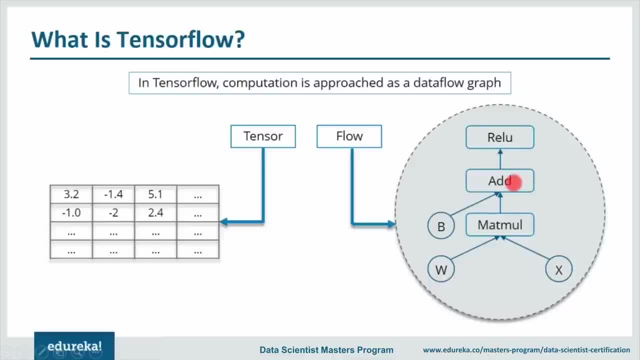 So what is this? This is nothing but the Sigma function in this perceptron that we have seen. Then we pass it through an activation function, and the name of that activation function Is RELU, or ReLU, what you can say it, and then a neuron will fire. 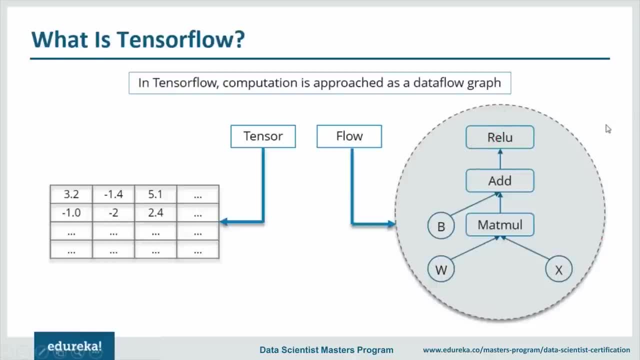 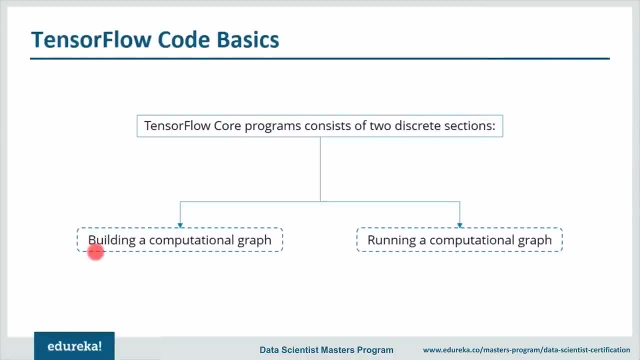 So this is nothing but a flow, or you can say a data flow graph. Now let us understand few code basics of tensorflow. Now the tensorflow programs actually consists of two parts. One is building a computational graph and another is running a computational graph. 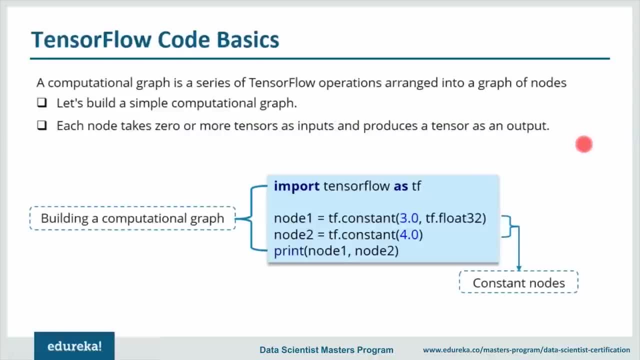 So we'll first understand how to build a computational graph. Now you can think of a computational graph as a network of nodes and with each node known as an operation And running some function. that can be as simple as addition or subtraction, or it can be as complex as, say, some multivariate equation. 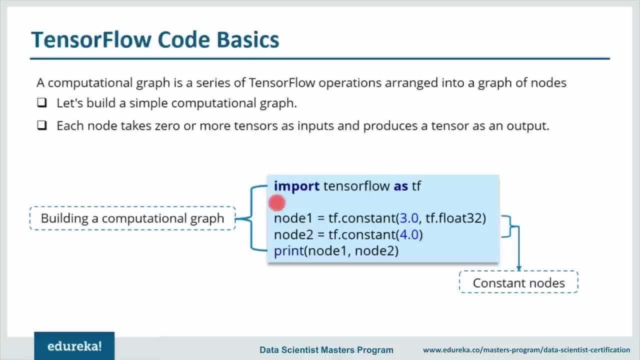 Now let me explain it to you with the code that is there in front of your screen. So the first thing you do, you import the tensorflow library. Then what do you do? you define two nodes and these nodes are constants. So we'll call that function, will call it as TF dot constant. 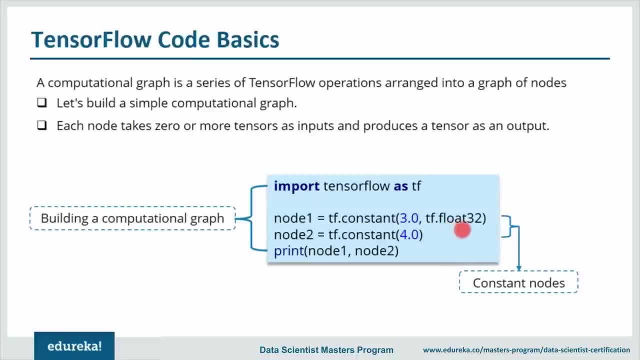 and will provide a value that is 3, and it is nothing but a float number of 32 bits. Similarly, We defined One more node, which is a constant, and it contains value for. so these are nothing but your constant nodes. This is basically what computational graph is. 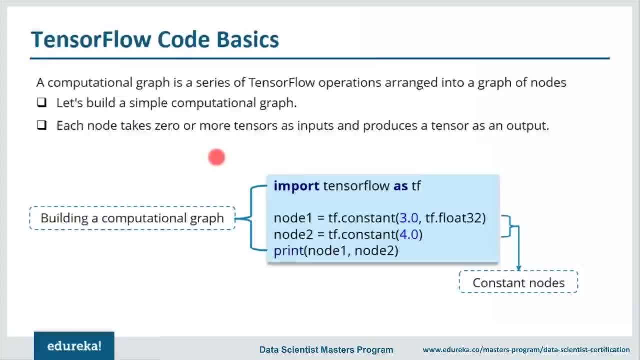 So, basically, we have built a computational graph and in this graph, each node takes 0 or more tensors as inputs and produces a tensor as an output, and one type of node is a constant that I've told you earlier as well, and these tensorflow constants. it takes no inputs. 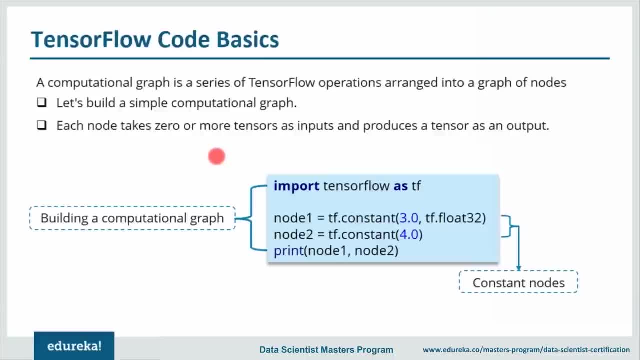 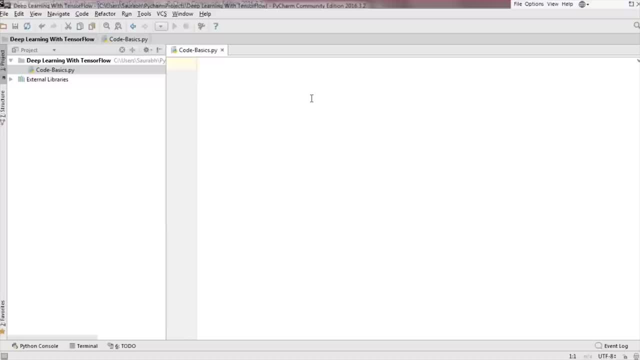 and it outputs of value which is stored internally. Now what I'll do? I'll actually execute this in my pie chart, so for that I'll open it. So this is my pie charm, guys, and I've already installed tensorflow and I'm telling it to you again. 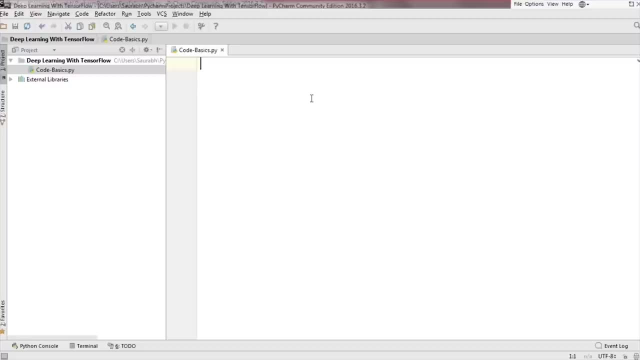 that the installation guide for your tensorflow in Windows as well as Linux is present in your elements to just go through it, and it's pretty easy. So the first thing that I need to do is import the tensorflow library. for that I'm going to type in here: import tensorflow as TF. 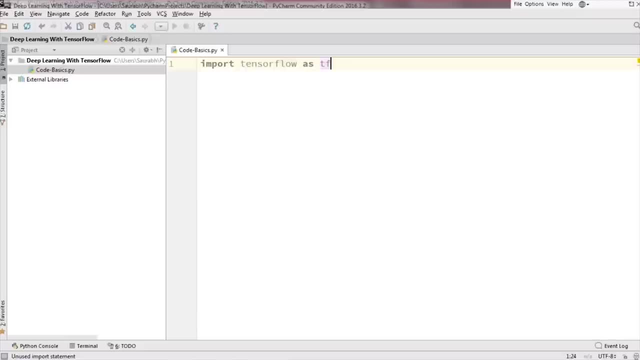 So if you are familiar with the python basics, you know what it means actually. So I am importing tensorflow library And in order to call that, I'm going to use the word TF. So after that, I'm going to define my node 1 and node 2, which are constant nodes. 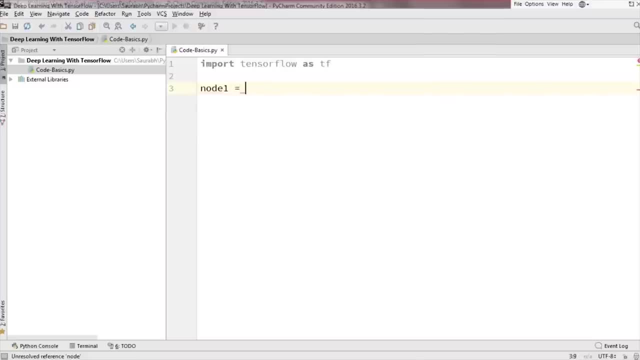 So for that I'm going to type in here node 1, equal to TF dot constant, And then I'm going to define the constant value in this. So it will be 3 and it will be a float value of TF dot. float of 32 bit. 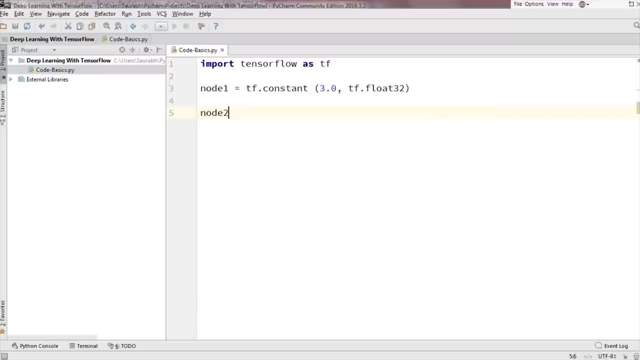 All right, and now I'm going to Find my second constant node, So I'll type in here node 2: TF dot constant. I'll put 4 in here and 4, that's it. And so the TF dot float 32 will be present implicitly. 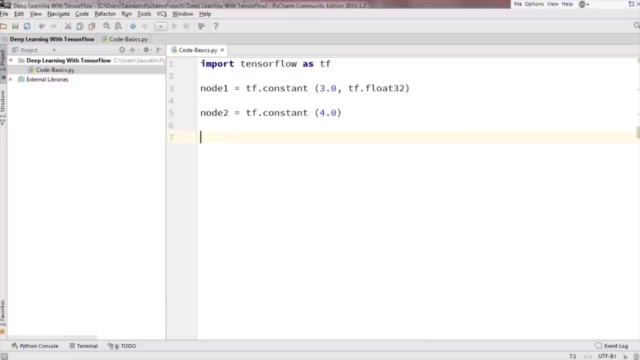 I don't need to do that again and again. So I have created a computational graph here. So what if I print it now? So let us see what will be the output. node 1: comma. node 2.. Let's go ahead and run this and see what happens. 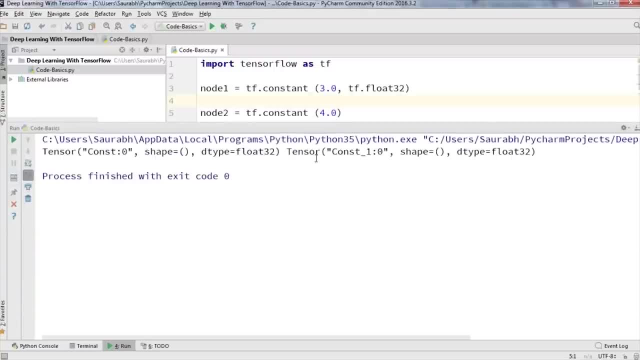 If you notice here that printing the nodes does not output the values 3 and 4, you might be expecting that right, that it should print 3 and 4. but instead they are nodes that, when evaluated, would produce 3 and 4 respectively. So to actually evaluate the nodes, what we need to do is we need to run this computational graph. 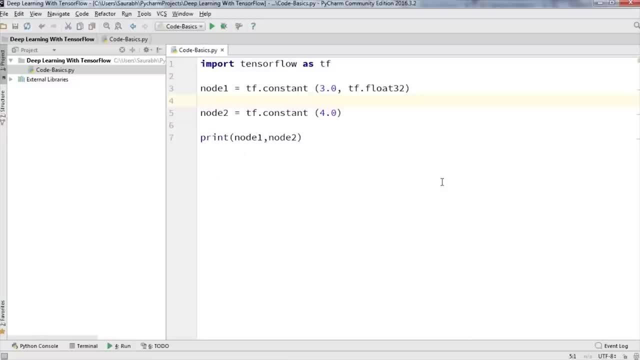 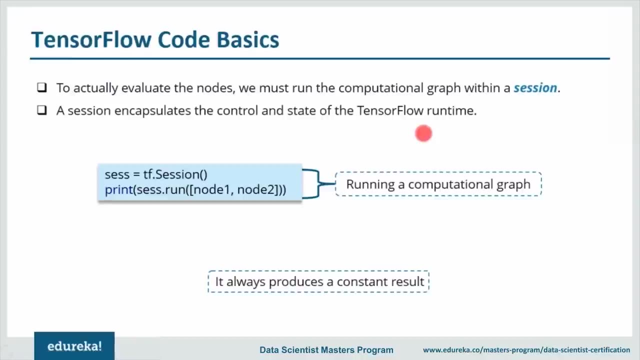 So let me show you that. for that I'm again going to open the slides. So, since I've told you earlier as well, we need to actually run this computational graph within a session. And what is this Session? its session actually encapsulates the control and state of the tensorflow runtime. 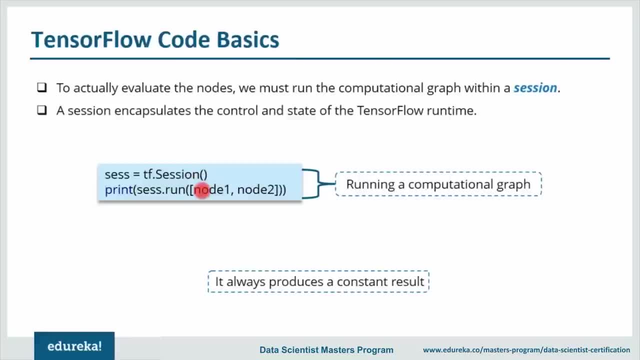 Now the code that is there in front of your screen. what it will do? It will actually create a session object and then it invokes its run method to run enough of the computational graph in order to evaluate node 1 and node 2. and how it does that? by running the computational graph in a session. 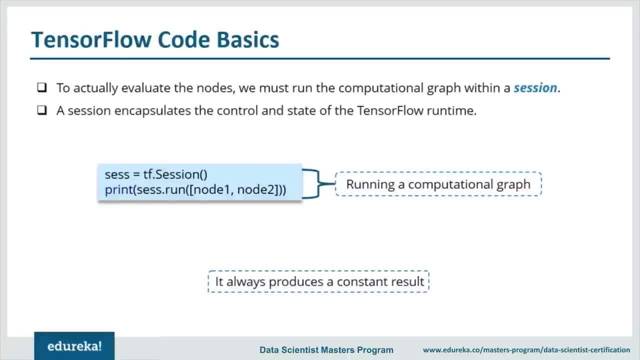 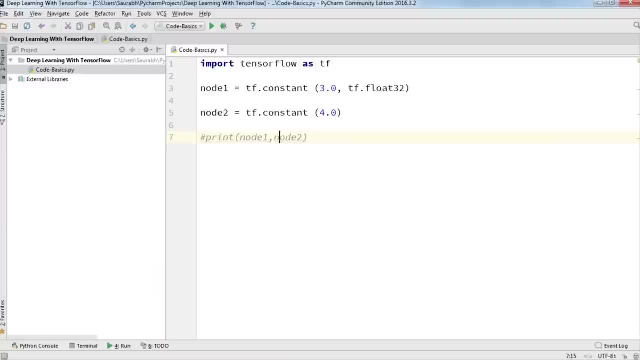 So now let me show it to you practically how it happens. So again, I'm going to open my pie charm. This is my pie charm, guys. So let me first Comment this print statement, and now I'm going to run a session. 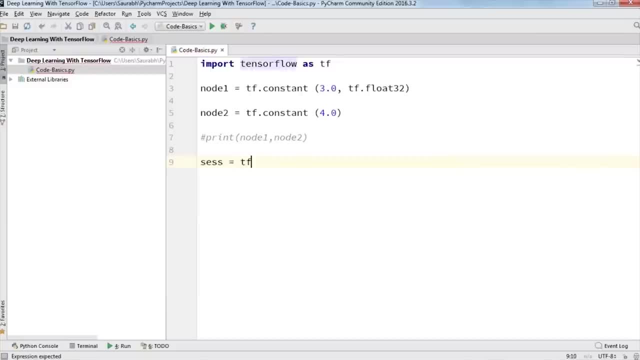 So for that I'm going to type in here: says: equal to TF dot session. and now I'm going to print it. So for that I'm going to type in: print: says dot run and what I want to run. I want to run node 1 and node 2.. 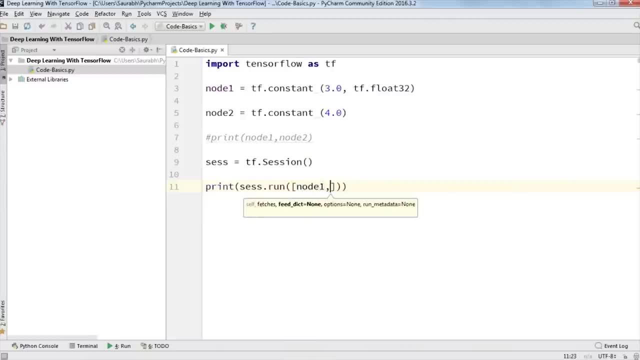 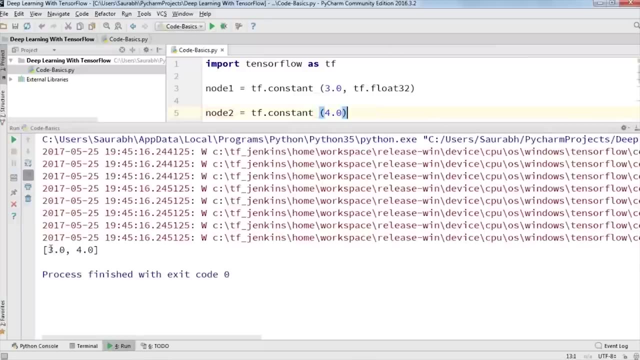 So I'm going to type in here node 1, comma, node 2.. That's all. and now, when I run this, it will actually give me the value 3 and 4.. And yup, it does. it gives me the value 3 and 4.. 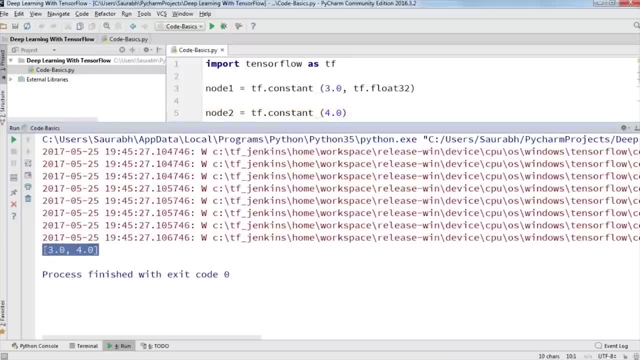 So what we did? we first build a computational graph. We first saw how to build a basically a computational graph, and then we understood that these all are nodes. So in order to get their value, we need to evaluate those nodes. and how we can do that by running the computational graph inside a session. 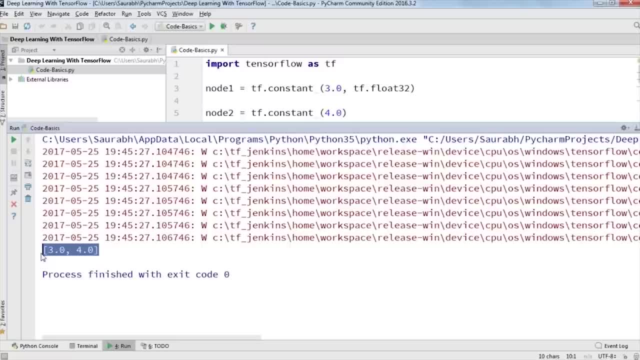 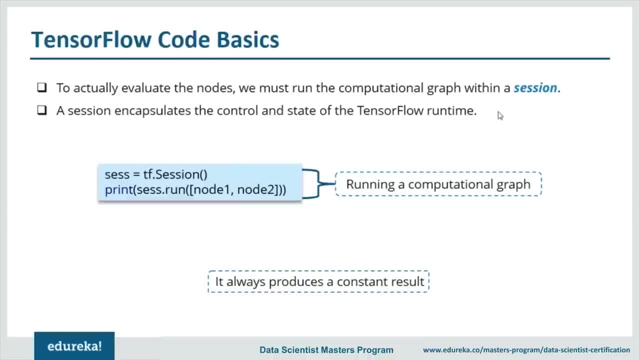 And then, finally, when we run that session, we get the output 3 and 4, which is nothing but the values of those nodes. fine, So I'll again open my slides, and the one thing that you must have noticed Here is that it will always produce a constant result. 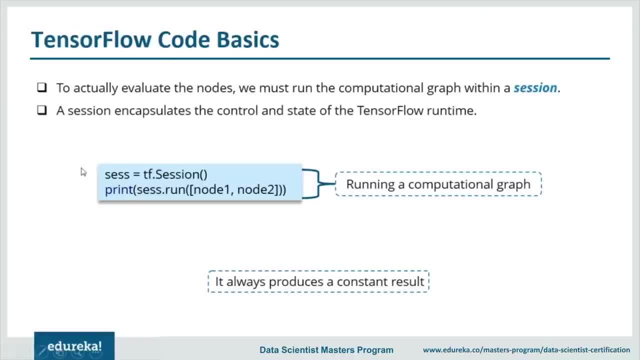 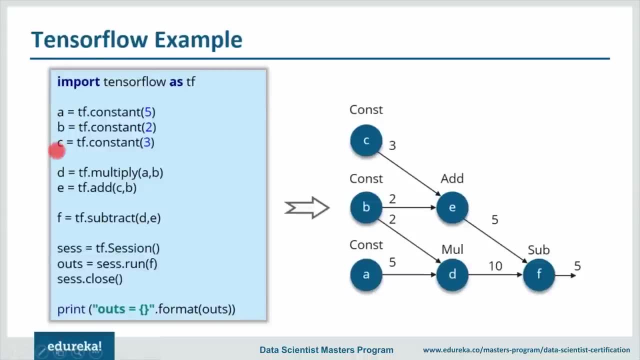 right. So how to actually avoid that? So we saw how to run a computational graph as well. Now let me explain it to you with one more example. So this is one example in which we take three constant nodes- a, B and C- and we perform certain operations like multiplication, addition and subtraction. 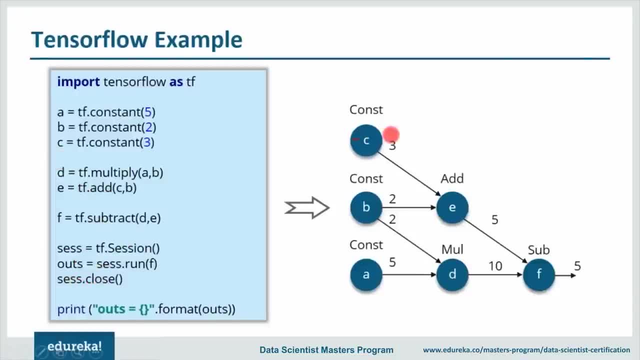 And then we run the session and then we finally close it. and this is the diagram how it looks like. So we have three constant nodes: C, B, a. a contains value 5, B contains two. similarly, C Contains three. first we add C and B, then we add B and A, then we get two other nodes, that is, E and D, and then from that E and D. 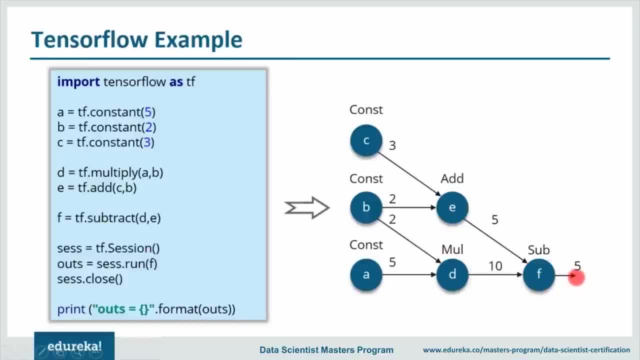 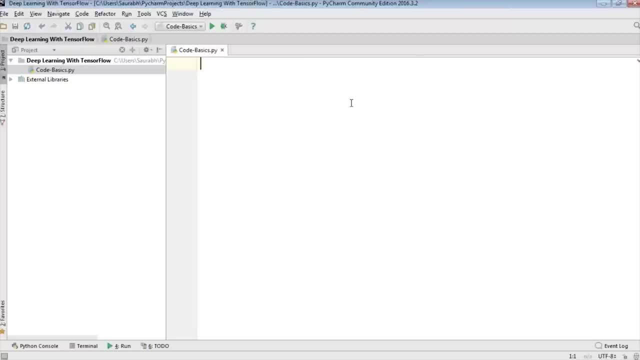 What we are going to do is we are going to subtract both of them and then we get the final output. Now let me go ahead and execute this practically in my pie charm. So this is my pie charm again, guys. First thing I need to do is import tensorflow as TF. 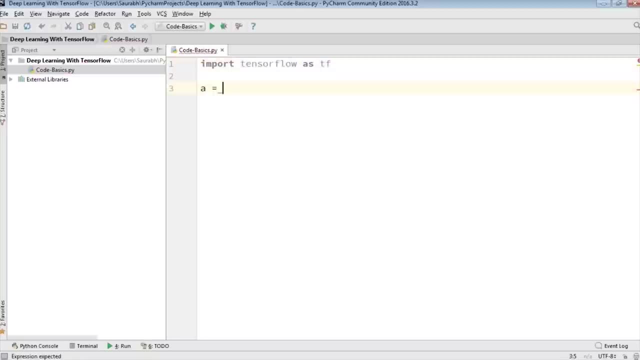 Then we are going to find the three constant nodes. So first is a equals to TF dot constant, and the value that will be there in a will be five. Then I'm going to find one more constant node, that will be B- TF dot constant- and the value that will be there in it will be two. 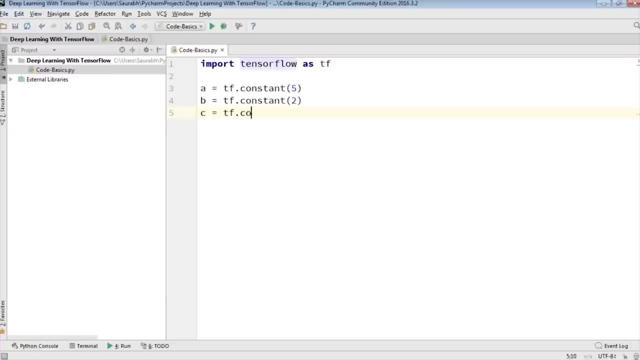 And then I'm going to find the last constant node and TF dot constant, The value that will be. there is three. All right, so we have three constant nodes and now we are going to perform certain operations in them. for that I'm going to find: 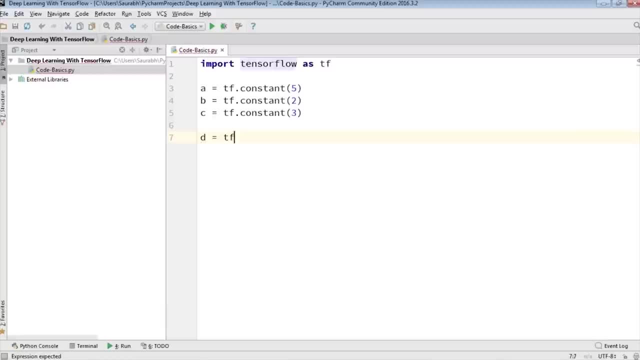 One node, Let it be D, which will be equal to TF dot. multiply, So the two nodes that we want to multiply, so that will be a comma B And then there will be one more node in order to perform some operation. that is addition to TF dot. 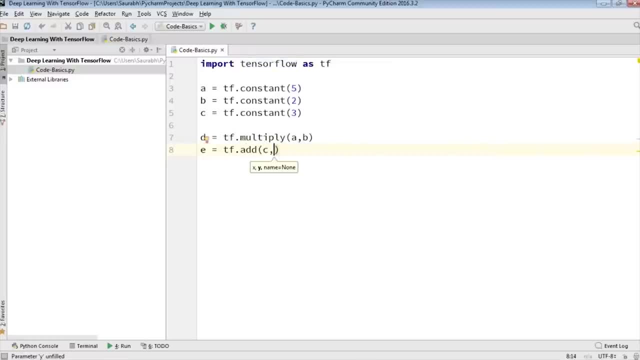 Add, add C and B, And then we're going to find one more node- Let B, F- and inside that node We're going to perform the subtraction operation: TF dot subtract D and E. So we have built a computational graph. Now we need to run it and you know the process of doing. that says is equals to TF dot session. 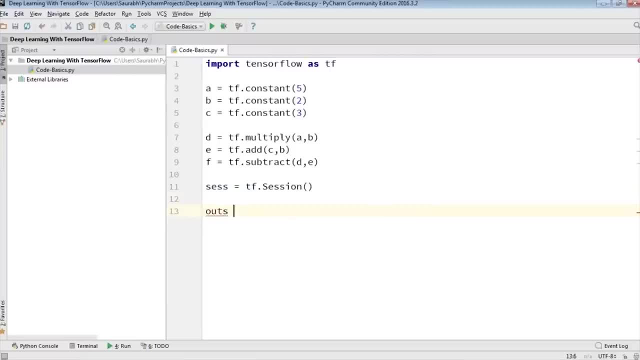 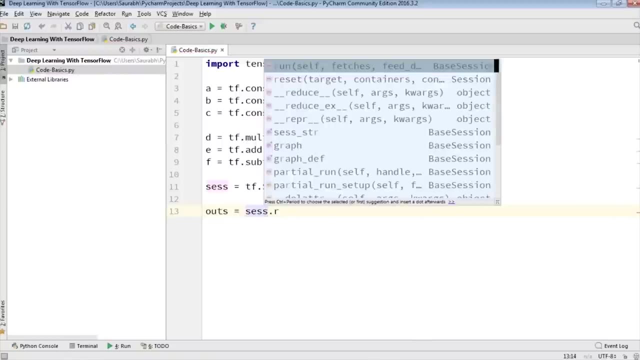 Then we are going to define a variable- Let it be O U T S outs, whatever name that you want to give in- and just type in a says a dot F. let's see if that happens or not, And then we're going to print it for that. 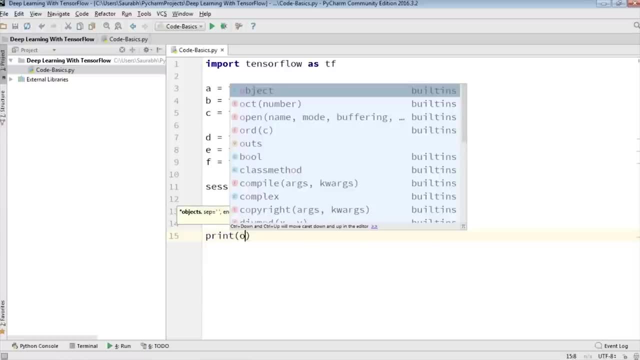 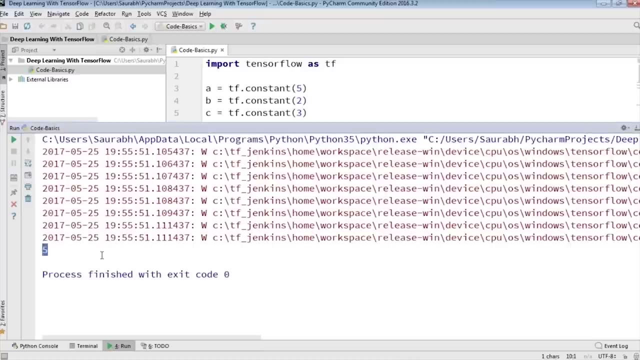 I'm going to type in here, print Out. Let's go ahead and run this and see what happens. So we have got the value five, which is correct, because if you notice our presentation as well, let me open it for you Over here. 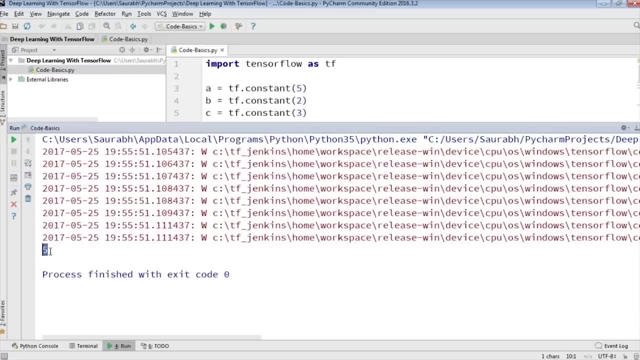 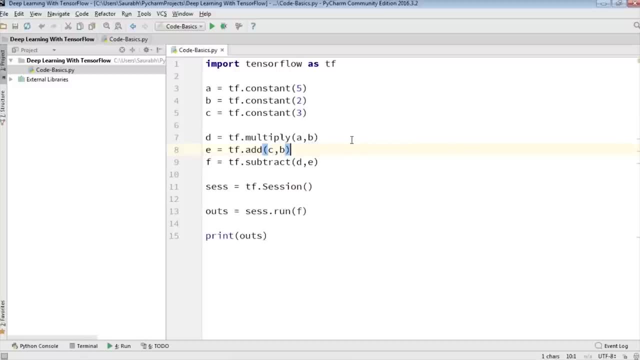 We also. we get the value five, similar to our implementation, and pie charm as well. So this is how you can actually build a computational graph and run a computational graph. I've given you an example. now, guys, let us move forward, because these are all the constant nodes. 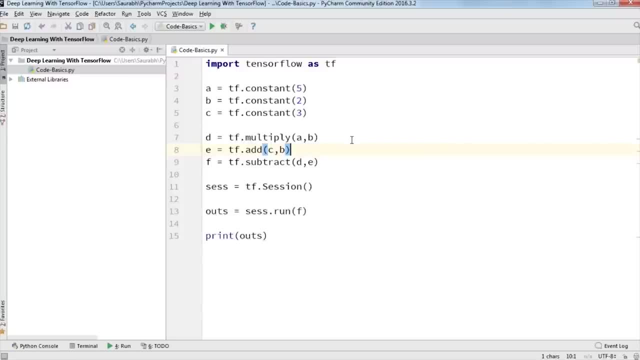 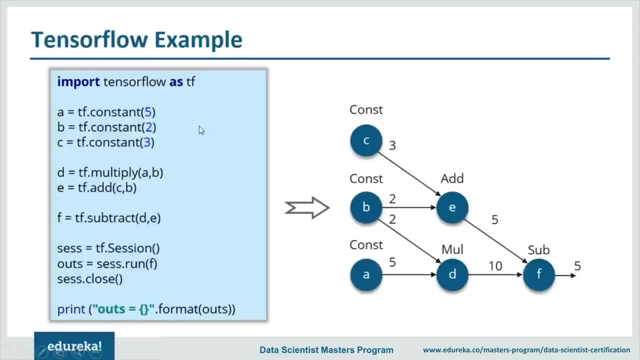 What if I want to change the value that is there in the node? So for that we don't use a constant nodes, for that We use placeholders and variables. Let me explain it to you first. I'll open my slides. So, since these are all constant nodes, 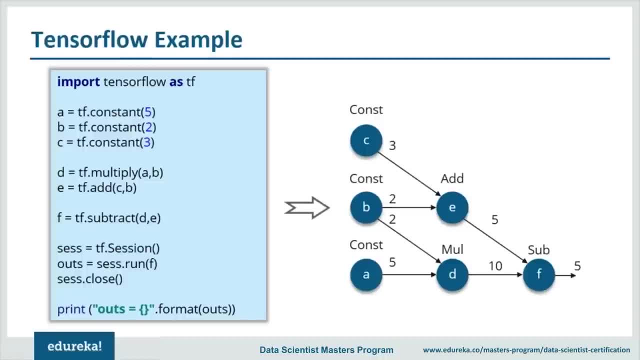 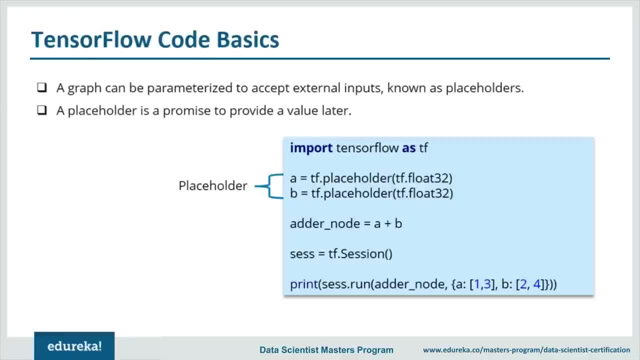 we cannot perform any operation. Once we have provided a value, it will remain constant. So, basically, a graph can be parameterized, except external inputs as well. And what are these? these are nothing but your placeholders, and these placeholders is basically a promise to provide values. 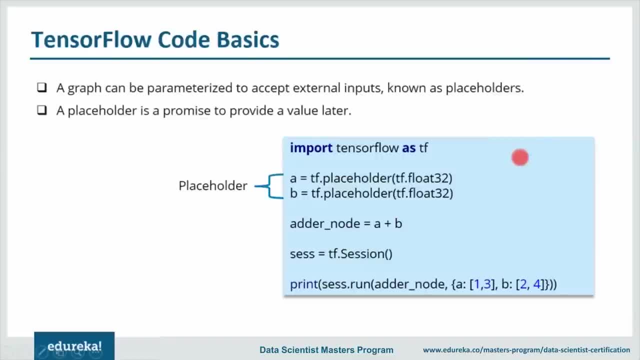 Later. So there's an example that is there in front of your screen over here. These three lines are bit like a function or a lambda, in which we define a two input parameters, a and B, and then an operation possible in them. So we have actually performing addition, so we can evaluate this graph with multiple inputs by using feed underscore dict parameter. as you can see, we are doing it here. 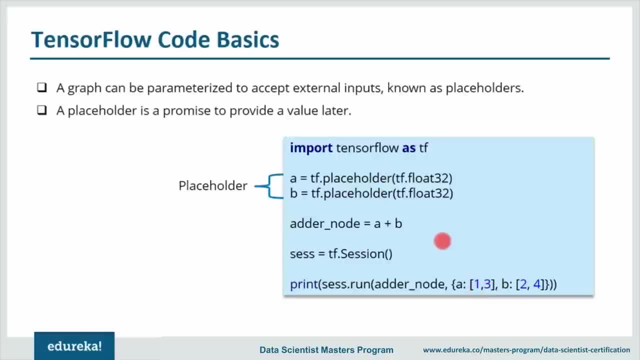 So we are actually passing all these values to our placeholders here. So these all values will be passed and accordingly will get the output. So let me show you practically how it happens. So I'm going to open my pie charm once more. I'll remove all of this. 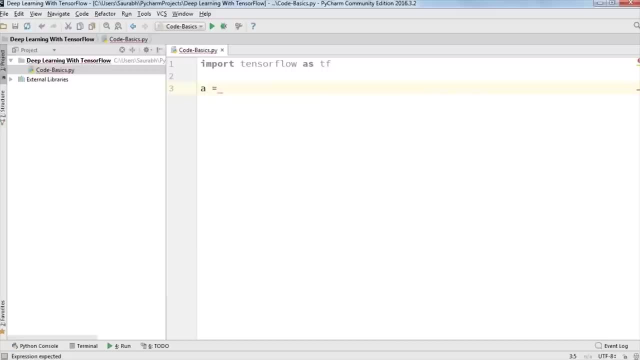 and yeah, so the first placeholder. I'm going to name it as a tf dot placeholder, and what sort of a placeholder it'll be? So I'll consider it as float number of 32 bits. Similarly, I'm going to define one more variable as well. 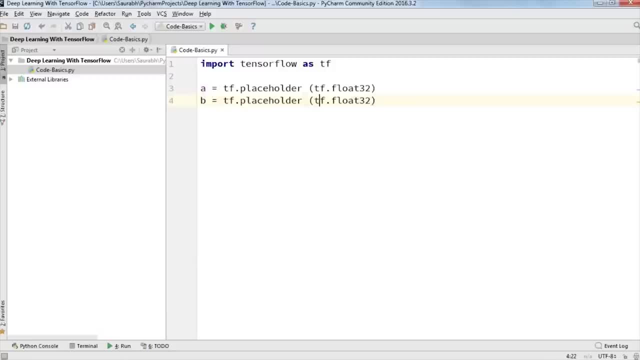 I'm going to name it as B, Then I'm going to define an operation that I'm going to perform them. So I'm just going to type in here: adder, underscore node equals to a plus B. And now our placeholders are currently empty. 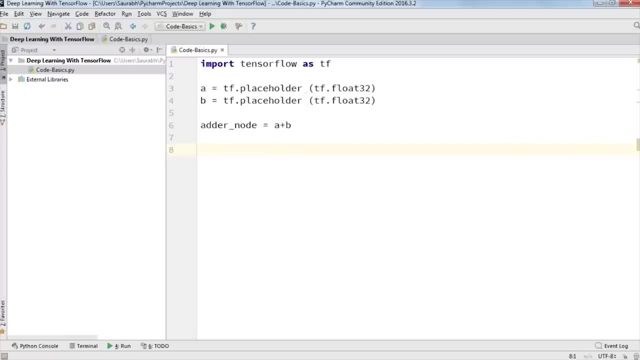 So that, totally earlier as well, placeholders are nothing but a promise in order to feed values later. So this is how we have built a computational graph. Now our next step is to start a session, So for that I'm going to type in a: assess equals to tf, dot. 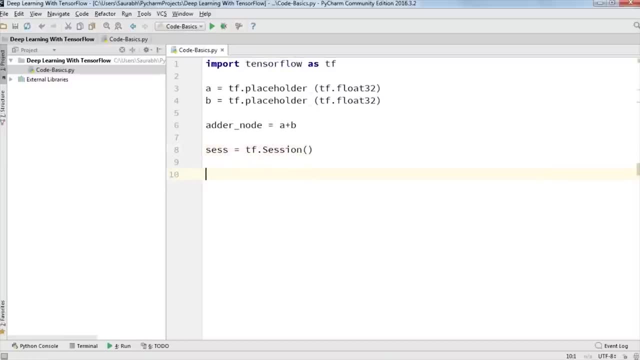 Session right, Since these placeholders are currently empty and we know that these placeholders are nothing but a promise, in order to provide them with certain values later. So let's go ahead and provide the values, or you can say a list of values, So I'm going to type in here. print says: dot run. 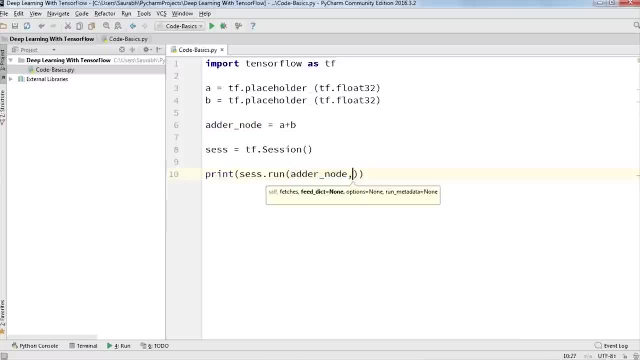 adder underscore node And then the values that I'm going to feed in. So basically, I'm going to feed in a dictionary: A colon, three, A colon- a list of integer values between one to three, and one more will be B colon, a list of integer values between two and four. 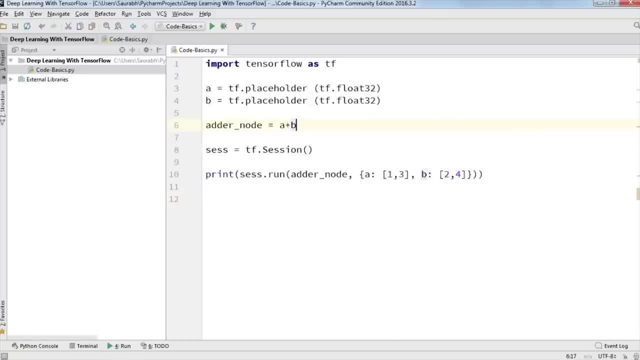 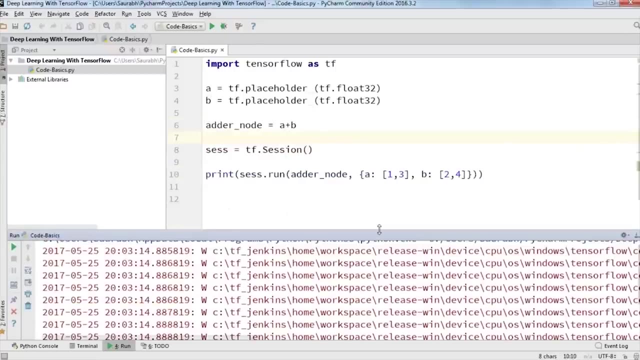 All right, so this is done. Now let us go ahead and execute this and see what happens. So we have got the output of three and seven. So basically, if you add one into, you get three. similarly, you add three and four, you get seven. 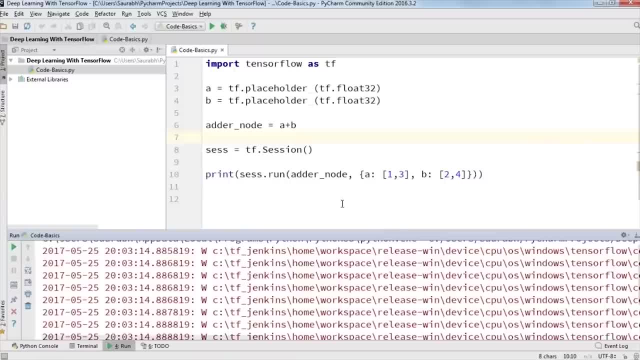 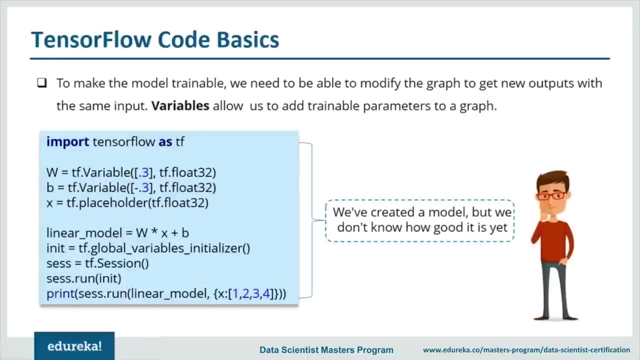 It's pretty easy mathematics, But my main focus was to make sure that you understand what our placeholders. So we understood What exactly our placeholders. now the time to understand what our variables. So basically, in deep learning, We typically want a model that can take arbitrary inputs. now, in order to make the model trainable. 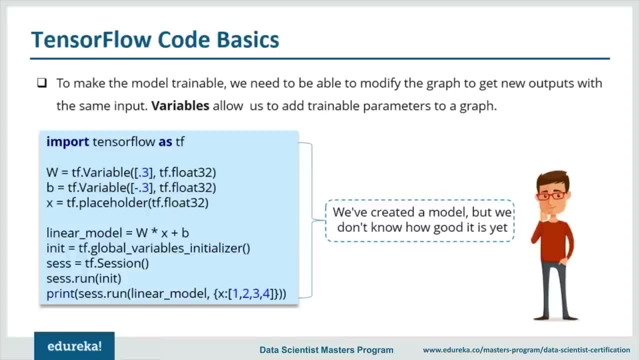 We do able to modify the graph to get new outputs with the same input, and what helps us to do that? variables basically allows us to add a trainable parameters to our graph. So, in order to declare variables, what we do is you can refer the code that is there in front of your screen. 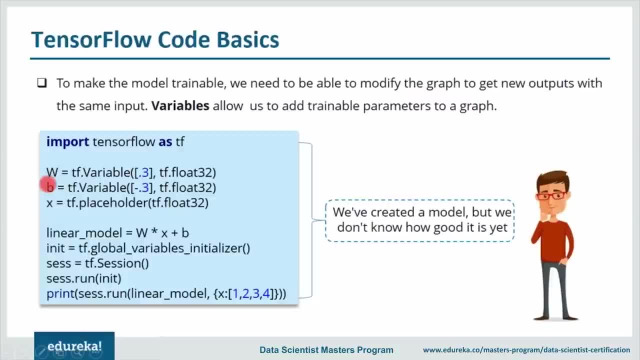 So we have taken two variables in one placeholder and the first variable has a value 0.3.. The other variable has minus 0.3 and the placeholder obviously it will remain empty and then later on we feed in some values to it. Then we create a linear model. 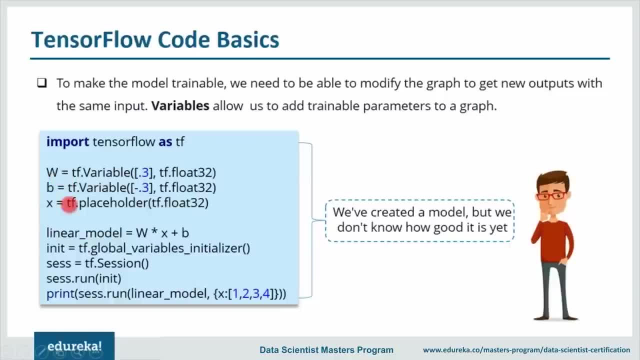 or you can say some operation in which we are going to multiply this W with X and then we are going to add a bias or a B value to it. Then what we need to do is we need to initialize all the variables in the tensorflow program. 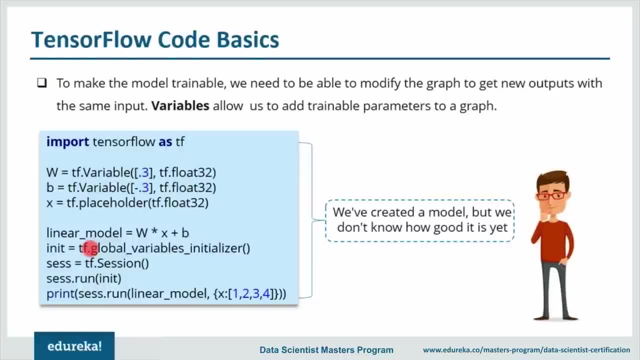 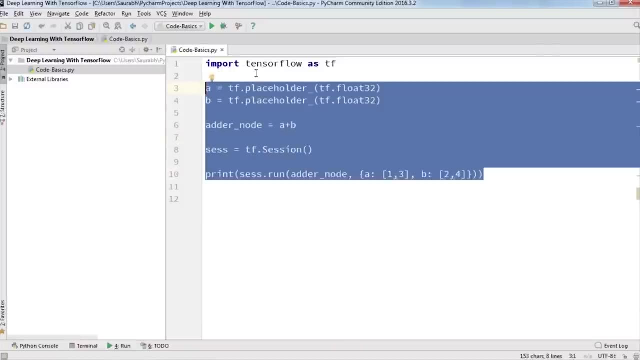 So for that you must explicitly called a special Operation, which is a TF dot global variable initializer, and then just directly run the session. Now let us go ahead and execute this practically, guys. Let me remove all of this. Yeah, so our first variable will be a W and we are going to call in a TF dot variable. 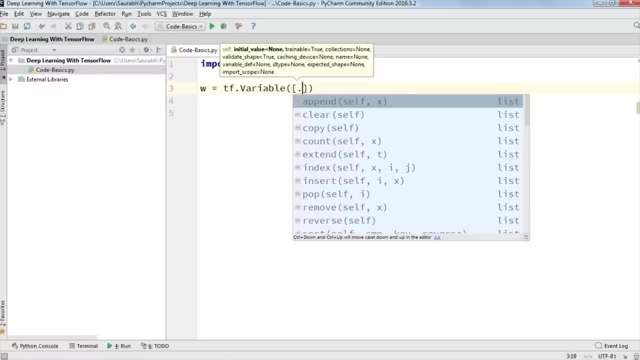 And in that variable we are going to store a value which is 0.3.. And it is of a float type 32 bit. So just type in here: TF dot, float 32.. Yeah, then we are going to define one more variable. 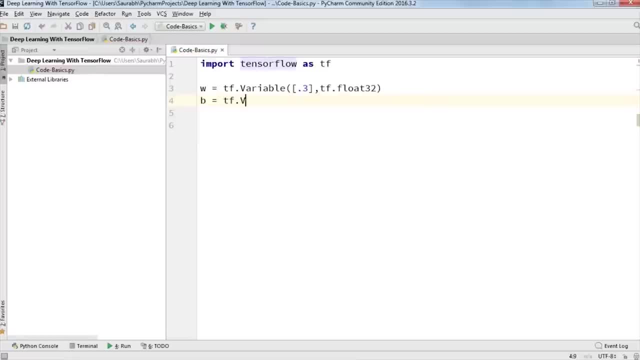 Let it be B. So I'm going to type in here TF dot variable and the value of this variable will be minus of 0.3.. Again, it is float type of 32 bit, So just type in that TF dot, float 32.. 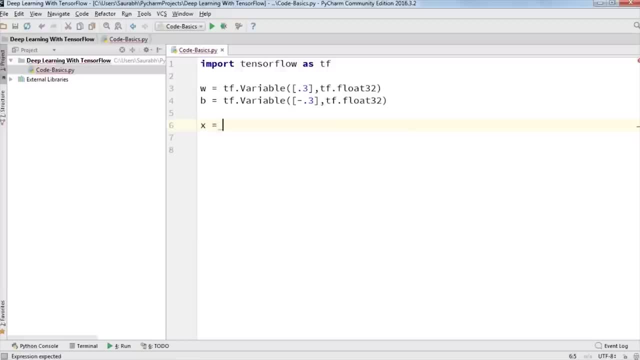 Now I'm going to define a placeholder That is X, X is equals to TF, a dot placeholder and it is again a float type 32 bit And then some operation that we are going to perform. So I'm going to type in here: linear underscore model. 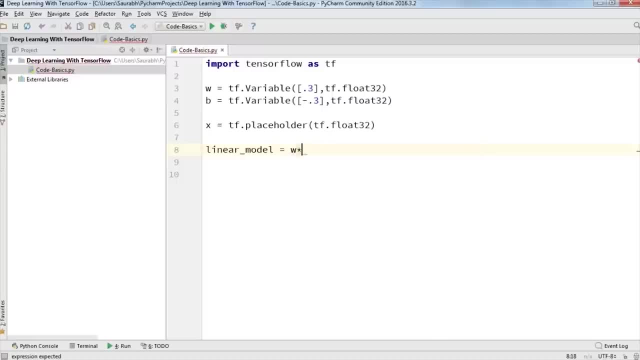 equal to W multiplied by our X value. That is a placeholder, and then we want to add a bias to it or B value to it. All right Now, as we have seen earlier as well, in order to initialize constants, we call TF dot constant, and their value will never change. 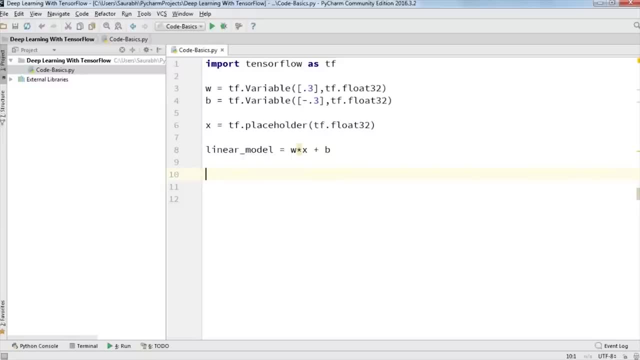 But, by contrast, variables are not initialized when you call TF dot variable. So to initialize all the variables in the tensorflow program, what you need to do is you need to explicitly call a special operation. and how you're going to do it. Just type in here: INET equal to TF dot. global underscore variables- underscore initializer. 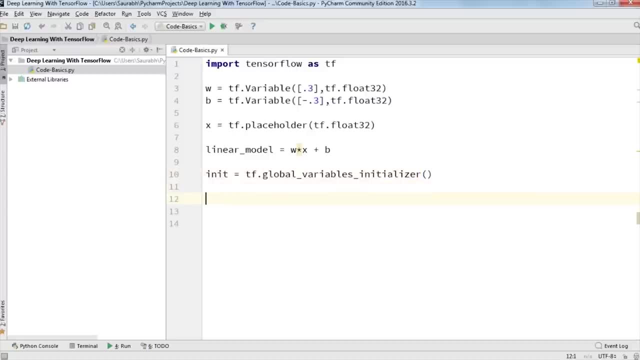 That's all, and then, and then we're going to run a session. So you know, the process says is equals to TF dot session INET. Now let's print it. And before that, what we need to do is need to provide the X placeholder with some values. 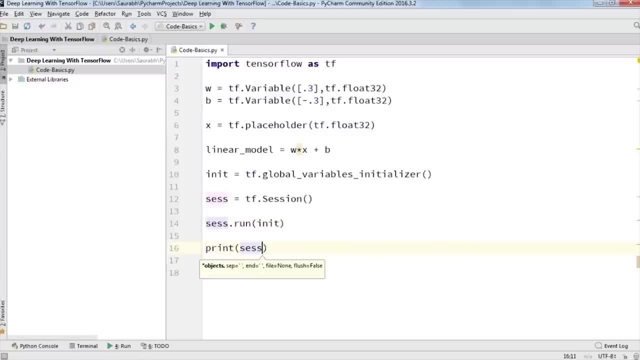 We'll actually going to do that at the print statement itself, So I'm going to type it: says dot run, Run What run? a linear model And the values that we are going to pass in X will be a dictionary again, And let me show you how you can do that. 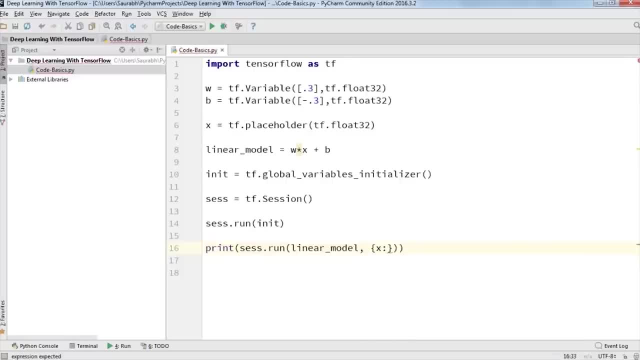 So X colon, and it will be a list of values from 1 comma, 2 comma, 3 comma 4.. Yeah, that's all, and we are going to run it now. So this is how we get the output. It's simple mathematics. 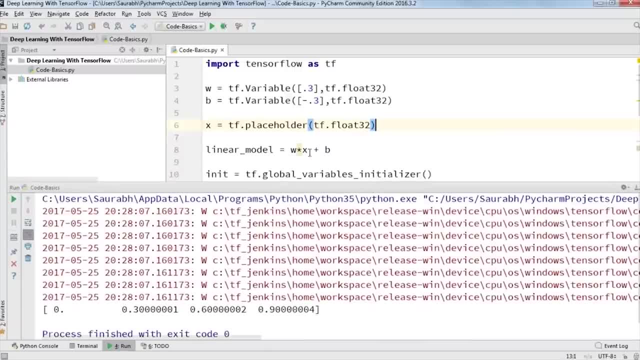 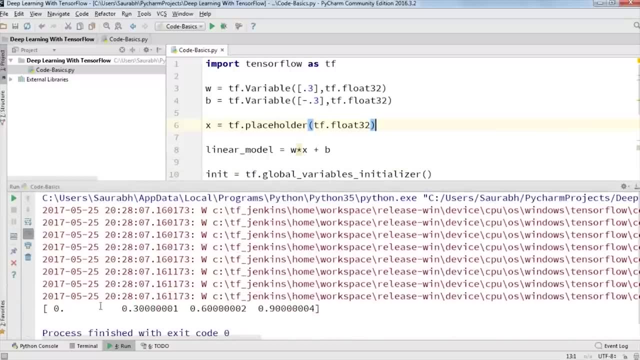 What we have? the first value of W will be 0.3 and the first value of a- B will be A minus 0.3 and the first value of X will be 1.. So it will be 3 minus 3, which is again 0, similarly for other values as well. 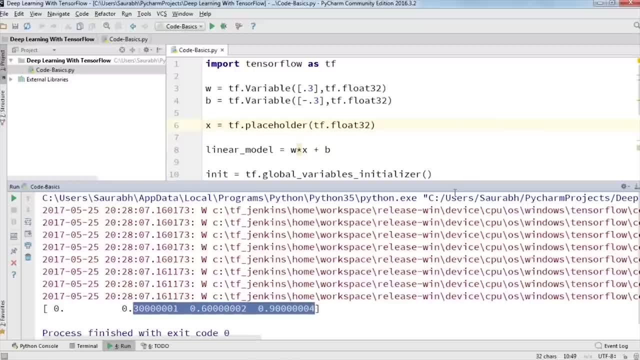 You can calculate it. It's absolutely correct. So what we have done? we have created a model, but we don't know how good it is yet, So let's see how we can actually evaluate that. for that I'm again going to open my slides. 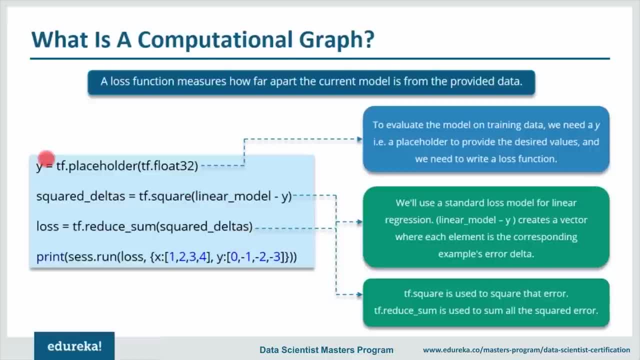 So now, in order to evaluate the model on the training data, we need a placeholder Why, as you can see in front of your screen, to provide the desired values and we need to write a loss function. So this placeholder Y will actually be provided with the desired values for each set of inputs. 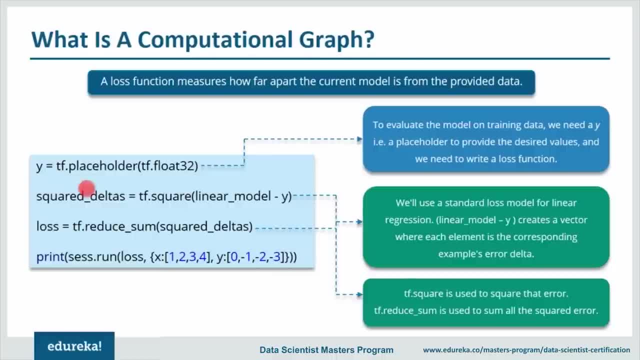 and then we're going to calculate the loss function. And how are we going to do that? We're going to minus the actual output with the desired output and then we are going to do the square of it. After that, we're going to sum all of these square deltas and then we're going to define one single scalar as loss. 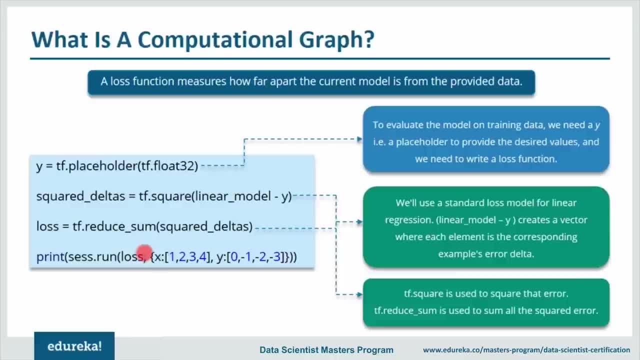 So this is how we are actually going to calculate the loss, and then, after that, we need to provide the values to X and Y placeholders. So what I'm going to do, I'm going to open my pie charm and then I'm going to show you how correct our model is, on the basis of the values that we provide to Y placeholder. 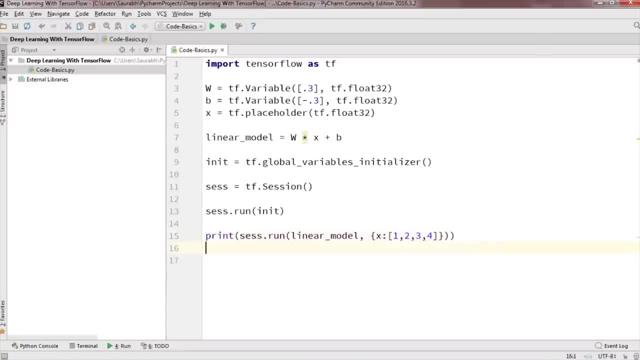 So, guys, this is my pie charm again. And since here, what I'm going to do is I'm going to define a placeholder first. Y is equals to TF dot- placeholder, TF dot- float 32.. So I'm going to type in a TF dot- float 32.. 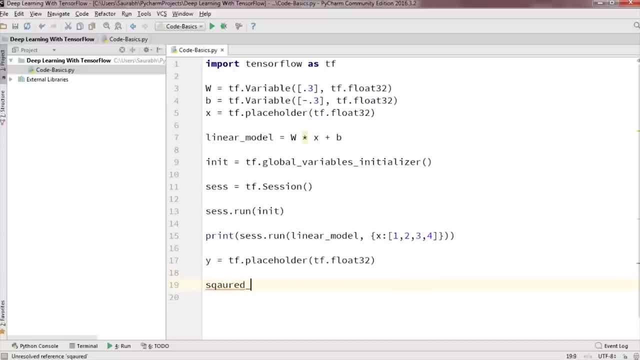 Square Delta. I've explained you all these things, but yeah, I'm going to tell it to you again as well, Don't worry about it. TF, dot, square, The actual output minus the desired output, And then I'm going to sum all those losses, or you can say square deltas. 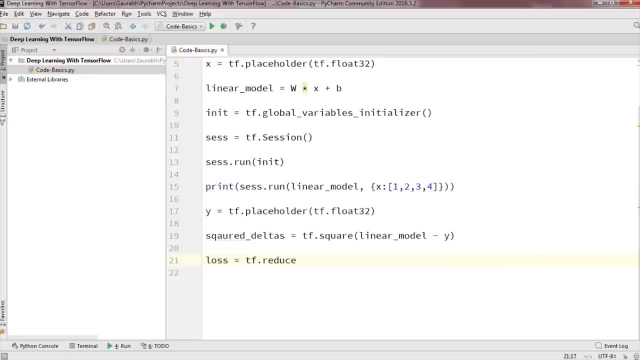 TF: dot reduce Underscore sum. So I'm going to type in here: square deltas. Then finally print it. So I'm going to type in: says: dot run Loss X colon 1 comma, 2 comma, 3 comma 4.. 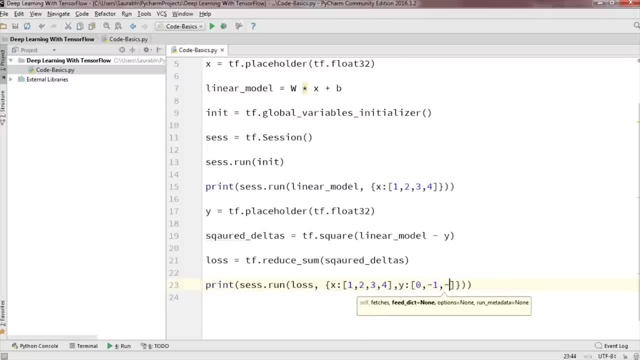 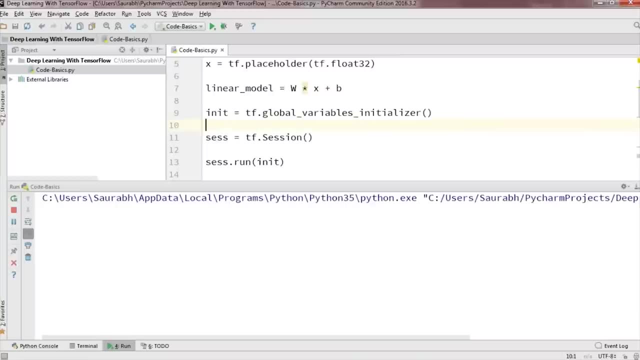 0 comma minus 1 comma, minus 2 comma minus 3, and that's all and we are good to go. Let's run it and see what will be the loss. So the loss is 23.66, which is very, very bad. 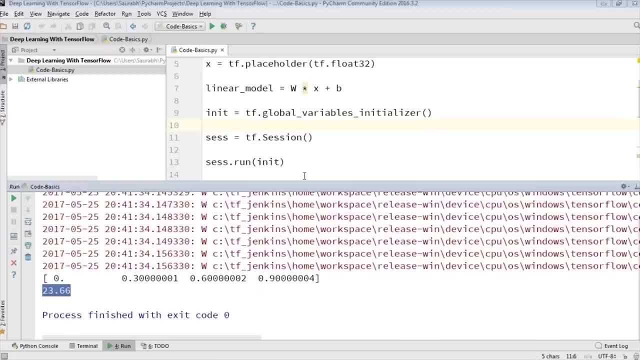 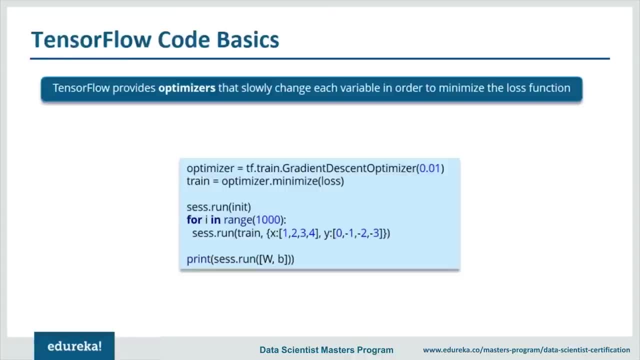 Now our next step is to realize how to actually reduce this loss. So let's go ahead with that. I'm going to open my slides once more. So, in order to minimize the error, Now in order to reduce this loss, TensorFlow provides optimizers that slowly change each variable in order to minimize the loss function. 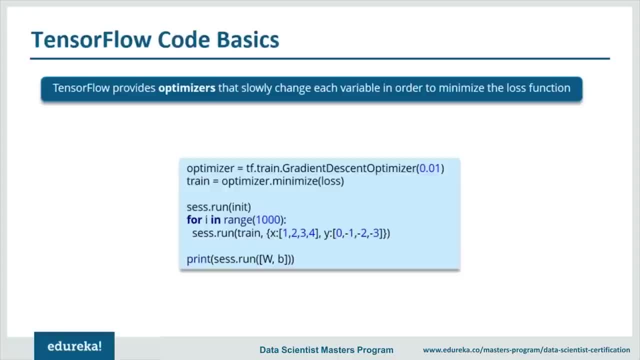 And the simplest optimizer is gradient descent. In order to do that, we have to call the function called TF dot gradients. So, as you can see it in the code itself, so we have a TF dot train dot gradients, Gradient descent optimizer, and this is nothing but the learning rate 0.01.. 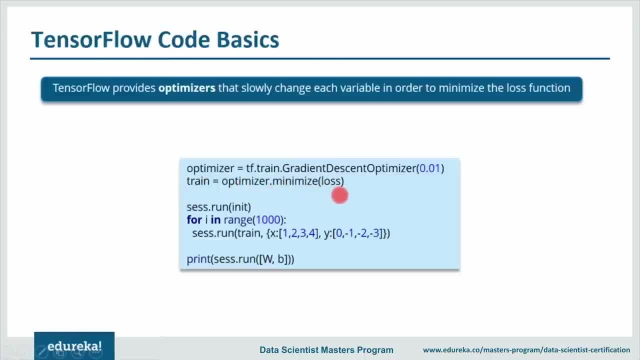 Then train equals to optimizer, dot minimize the loss. So we're going to call this optimizer, which is nothing but the gradient descent optimizer, in order to minimize the loss, and then we are going to run it. So let's see if that happens or not. 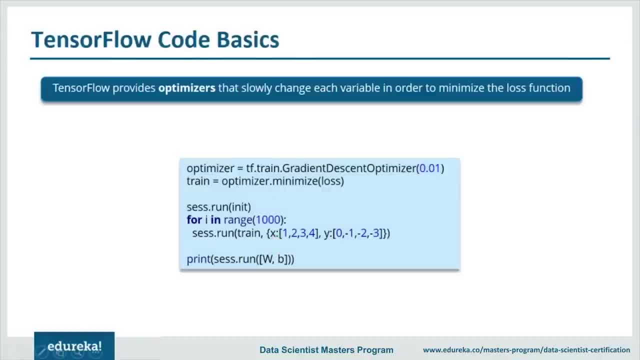 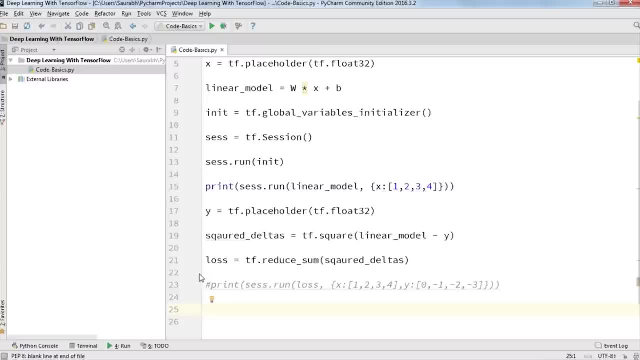 So for that again I'm going to open my pie charm, And over here let me first comment this print statement And now I'm going to type in here: Tim miser equals to TF, dot train Gradient descent optimizer, And the learning rate will be 0.01.. 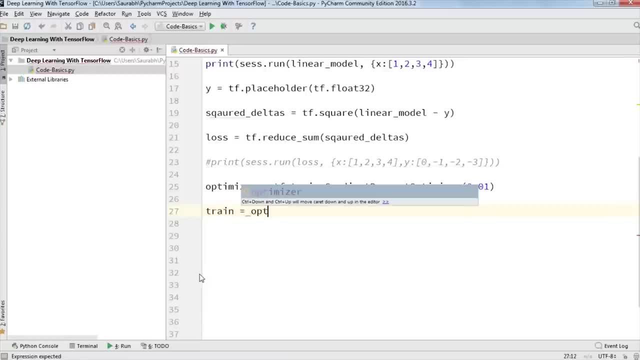 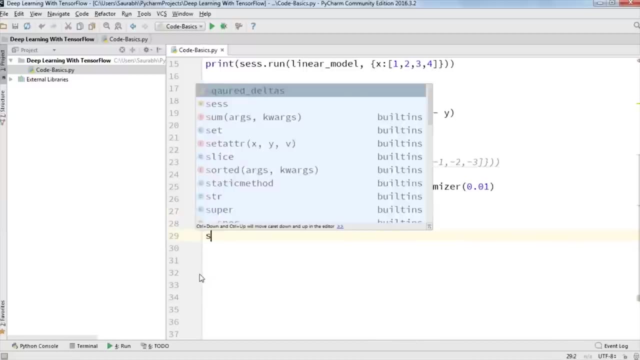 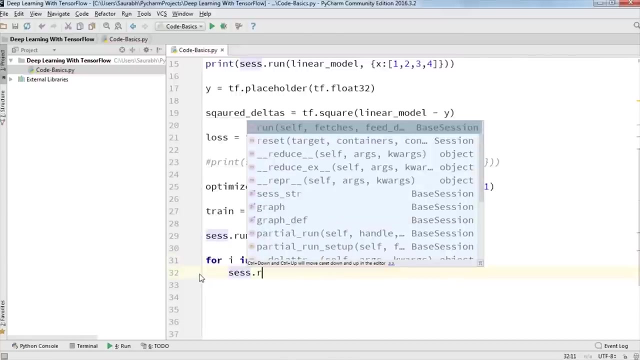 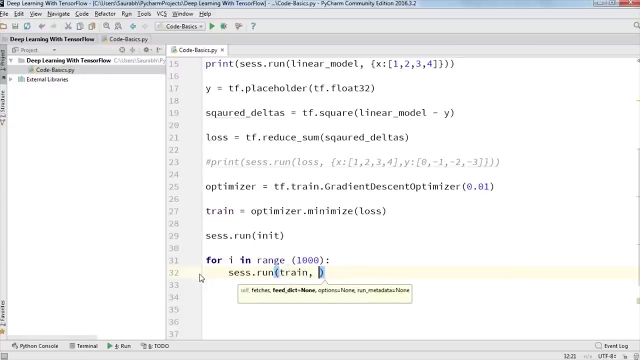 Now I'm going to type in here: train equal to optimizer, dot minimize loss. And then now let's go ahead and run. this says dot run, And we're going to fill in values to our X and Y placeholders. train comma X will have values 1,. 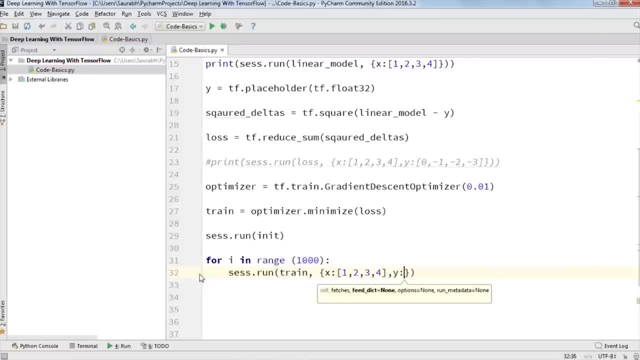 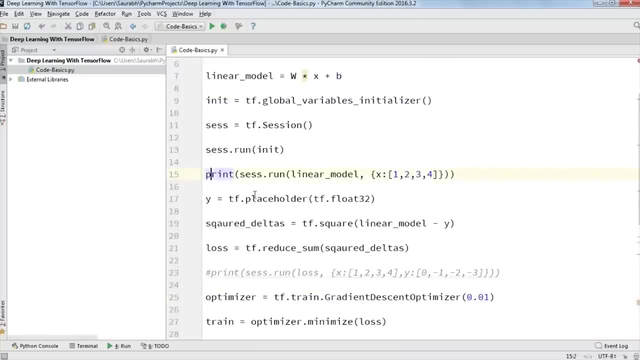 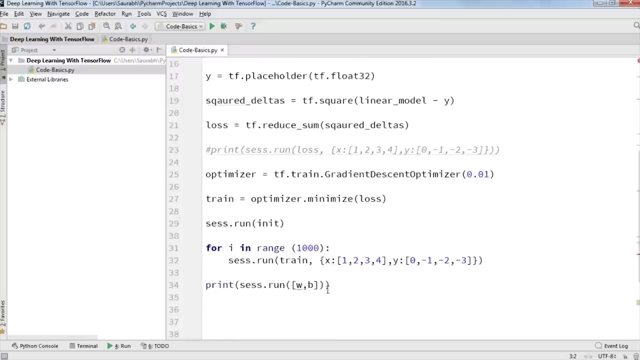 2,, 3,, 4.. And Y will have values 0 comma minus 1 comma minus 2 comma minus 3.. Print says: dot run W comma P. Now let me first go ahead and comment these lines. All right, 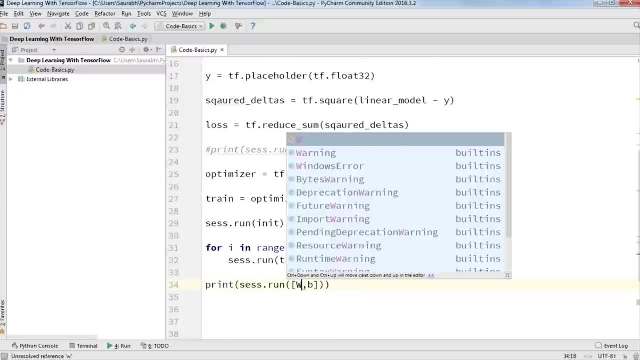 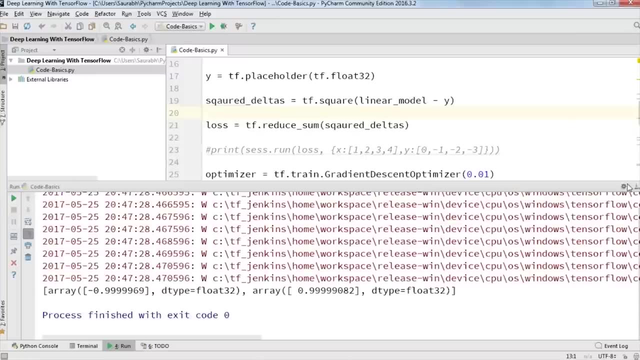 so I've just made a mistake here. This is in uppercase W, and yeah. so now we are good to go and let's run this and see what happens. So these are our final model parameters. So the value of a W will be around the point nine, nine, nine, nine, six, nine. 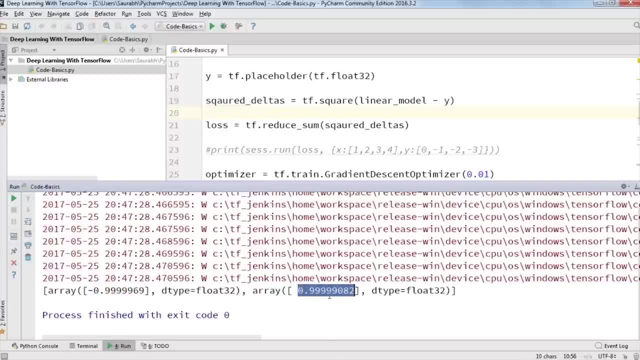 and the value of our B will be around a point nine, nine, nine, nine zero eight two. So this is how we actually build a model, and then we evaluate how good it is And then we try to optimize it in the best way possible. So I've just given you a general overview of how things works in TensorFlow. 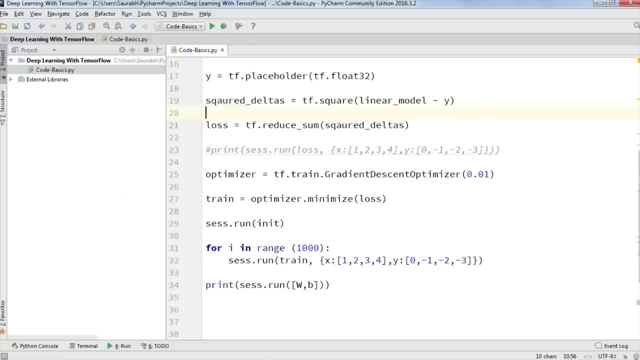 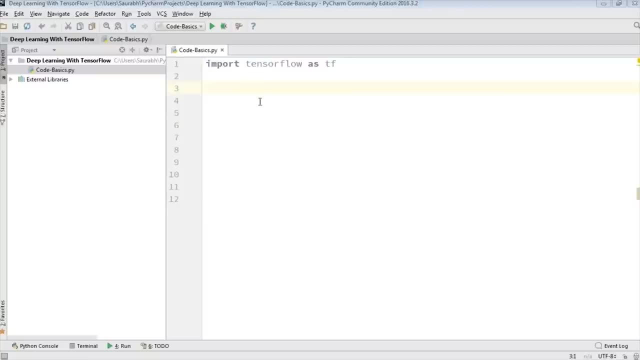 So now is the time to actually implement the and and or gate that I was talking about at the beginning of the session. So for that, let me first remove all of this. Yeah, Now, in order to implement and gate, our training data should consist of the truth table for and gate. 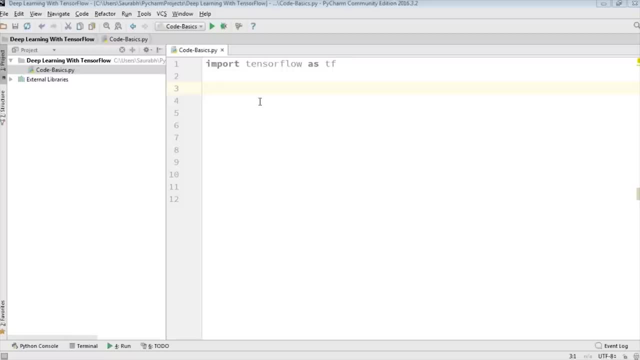 and we know that truth table and we know that if any of the input is low, then the output will be low, and and if both the inputs are high, then output will be high. One thing to note here, guys, is that the bias is implemented by adding an extra value of one to all the training examples. 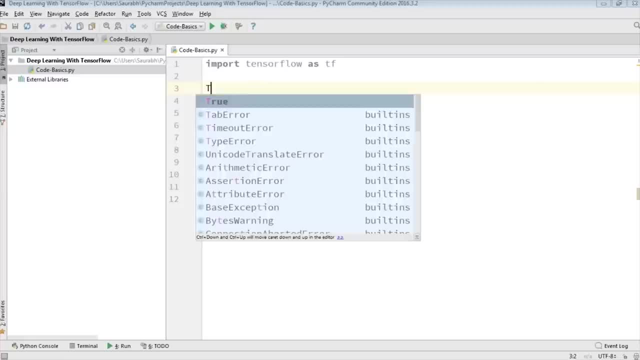 So yeah, enough of the explanation, Let's go ahead and code it. So I'm going to type in here: T comma, F, F equal to one point, comma minus one point, and bias will always be one. So I'm going to type in here: bias is equals to one point zero. and now I'm going to provide the training data. 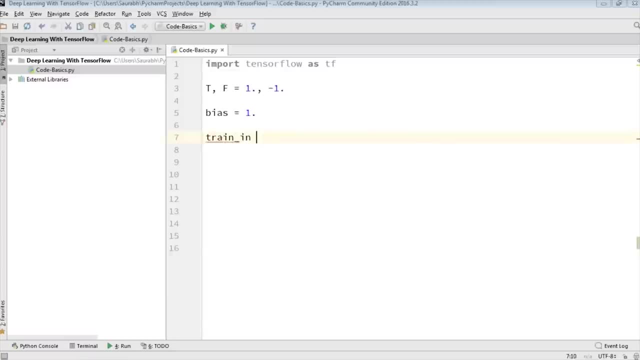 So for that I'm going to type in train underscore in equal to: If one input is true and the another input is also true, Then we have bias. Then again, if one input is true, The other input is false, Then also we have bias. 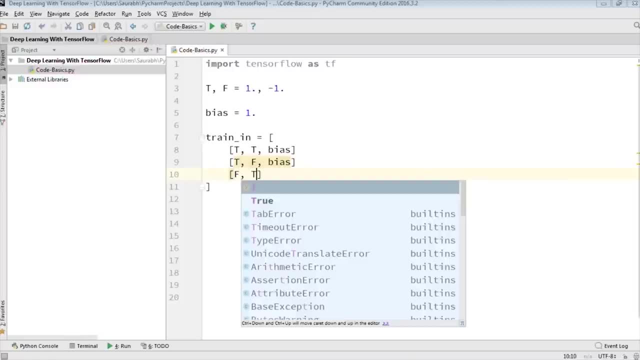 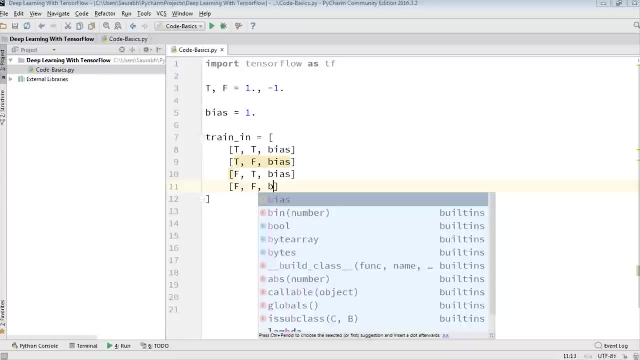 Similarly, one input is false, Another input is true, Then we have bias, And then finally, when both the inputs are false or zero, Then we have bias. right, This is our training data and the train out will type in here as the output. basically, train underscore out will be equal to: 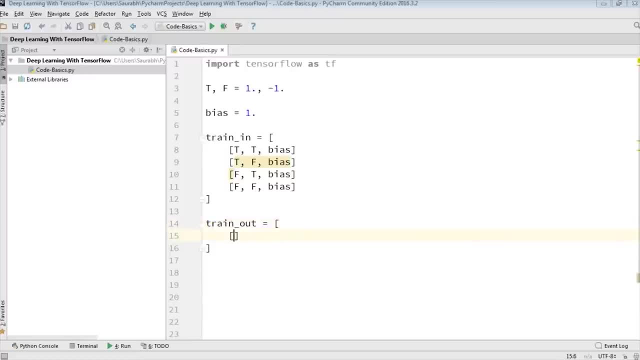 So, yeah, if both the inputs are true, or both the inputs are one, then output is true. Oops, I forgot a comma everywhere. Let me just go ahead and do that. Yeah, so if both the inputs are true, the output will be true. 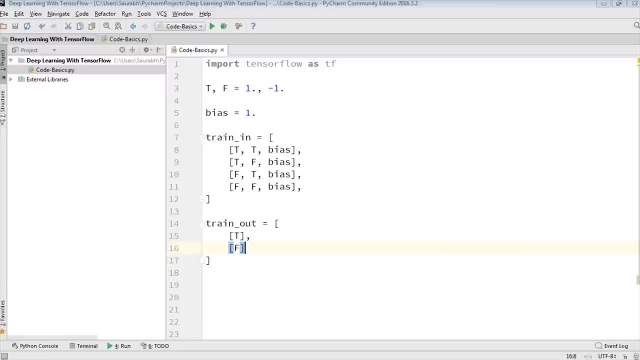 If any of the input is false, the output will be false. So I'm just going to type in here: falls everywhere, because there's only one condition in which we have the true output. All right, so this is done now. Now, as we know that tensorflow works by building a model out of MQT. 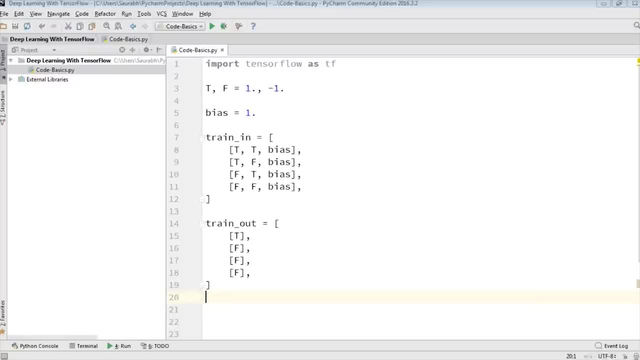 Tensors, then plugging in known values and evaluating the model, like we have done in the previous example, Since the training data that we have provided will remain constant. The only special tensorflow object we have to worry about in this case is our three cross one tensors of vectors. 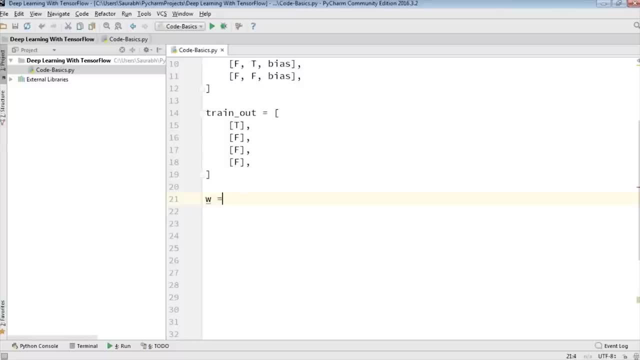 And now what are we going to do? We're going to define a variable and we are going to put in some random values in it. So I'm just going to type in TF a dot variable and generate the random function: TF Dot, random underscore normal. 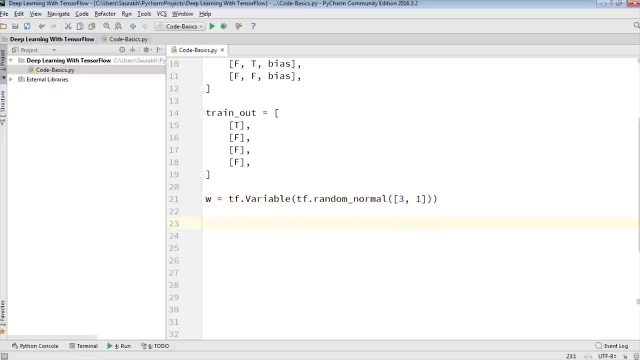 Three comma one. Now what it is? it is basically a variable, So its value may be changed on each evaluation of the model as we train, with all values initialized to normally distributed random numbers. Now that we have our training data and weight tensor, 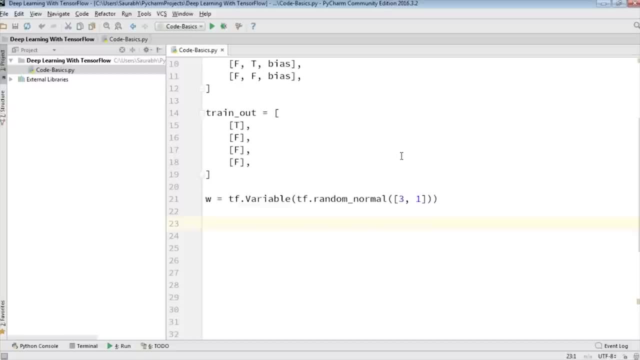 we have everything needed to build a model using tensorflow. So what we need to do, we need to define an activation function and we're going to define a step activation Function or step function. So for that, what I'm going to write here is a function: step. 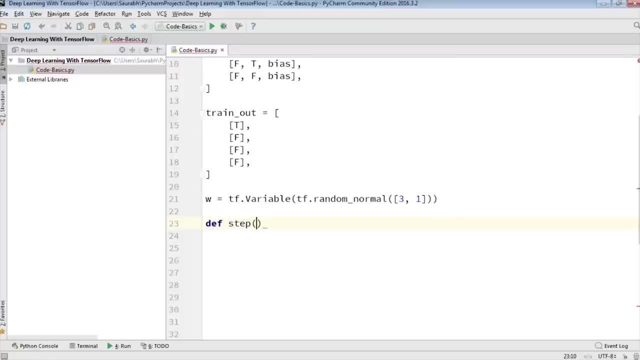 We're going to define our own step function, although you can use the predefined function as well. That totally depends on you. I'm going to type in here: is greater equal to TF, dot greater X, comma zero. Then we're going to define one more variable as float. 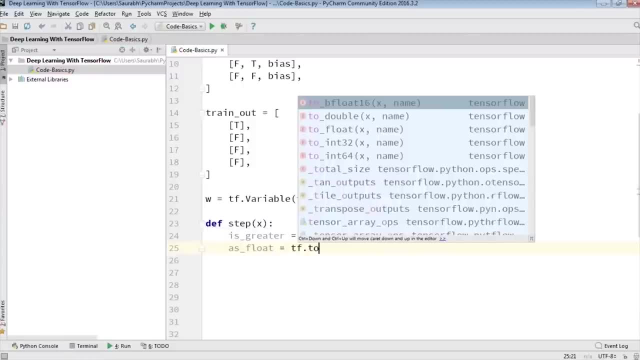 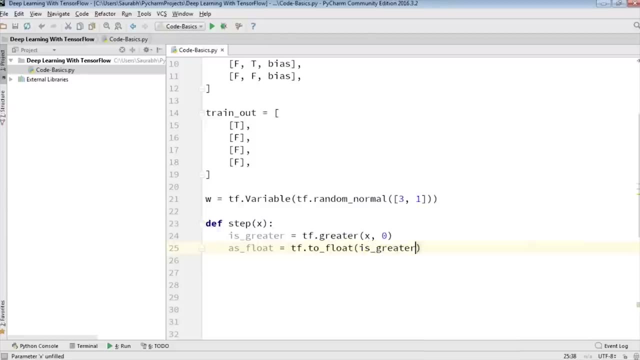 TF dot to underscore float. Is underscore greater, Then we're going to define one more variable, doubled equal to TF dot. multiply As underscore float comma two, Then return TF dot subtract doubled comma one. So now this is how we have defined our step function. 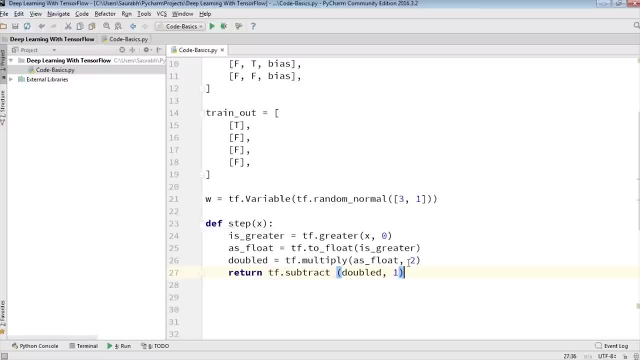 So with the step function defined, the output error and the mean squared error of our model can be calculated in one short line each. Let me show you how you can do that. So just type in here output equal to call that function. that is step. 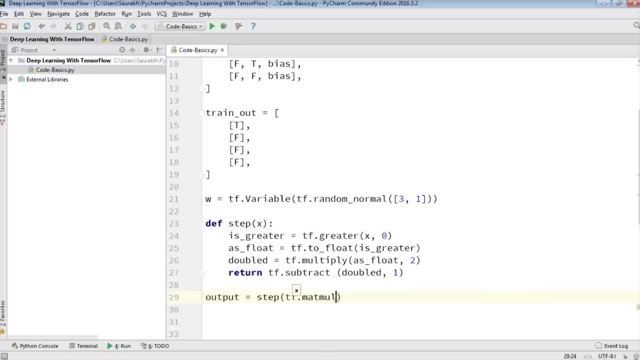 TF dot matrix Multiplication matmal Train underscore in comma W. Now for error. we're going to type in here: error equals to TF dot subtract Train underscore out Comma output. And for mean squared error I'm going to type in here: MSC. 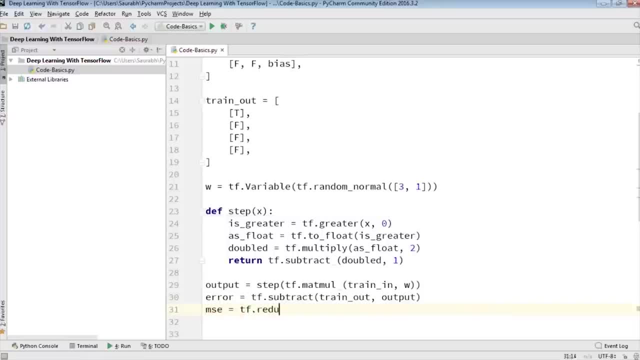 Equals to TF dot reduce, underscore, mean, TF dot square, And then error. Now the evaluation of certain tensor functions can also update the values of variables, like our tensor of weights W. So in our case, basically we're going to update the weights W. 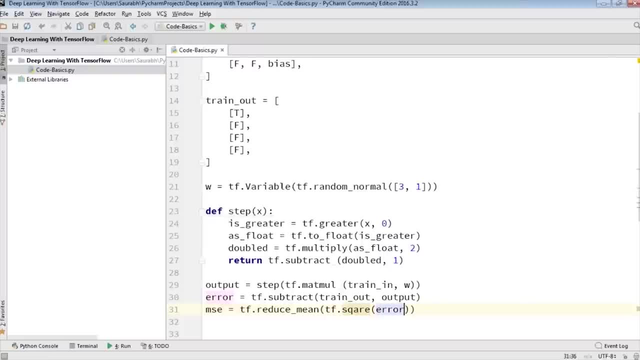 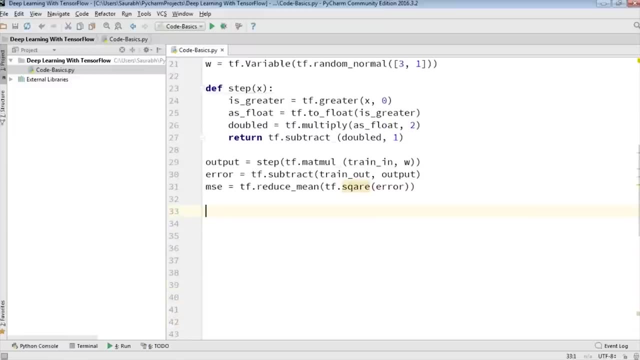 So first we calculate the desired adjustment based on error, Then we add it to W. Now let me show you how we'll do that. So, if you can recall, we have done that in the previous example as well, where we were updating the weights and bias. 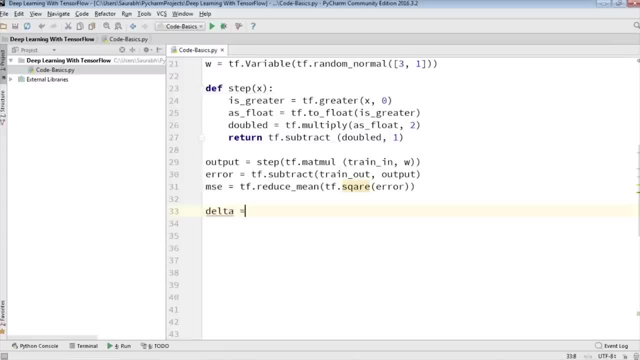 So now I'm going to type in here: Delta is equals to TF dot matmal. or you can say: matrix multiplication Train underscore in comma error comma transpose underscore a Equals to true. Then we're going to type in here: train Equal to. 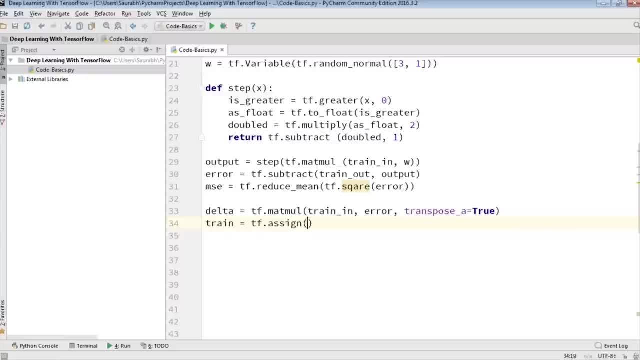 TF dot. assign W comma TF dot. add W comma Delta: The first matrix multiplication and then we're going to add it all. The model has to be evaluated by tensorflow session, which we have seen earlier as well, But before that we also need to initialize all the variables. 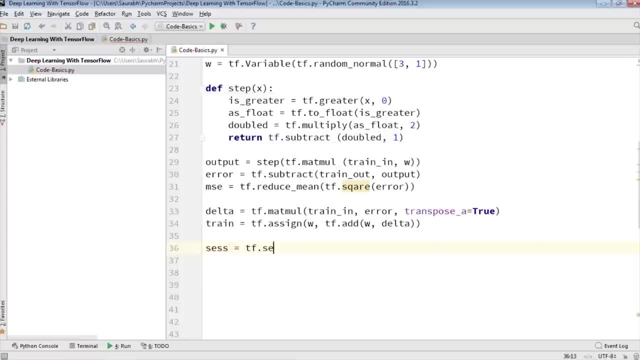 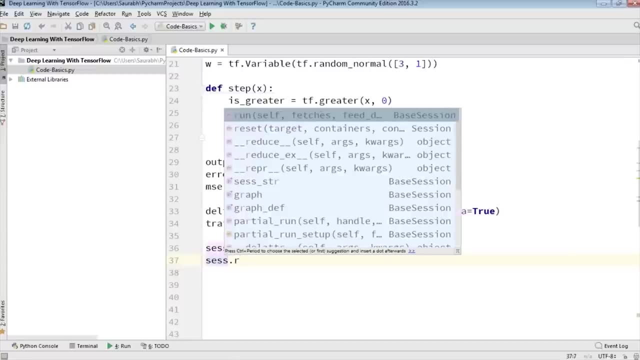 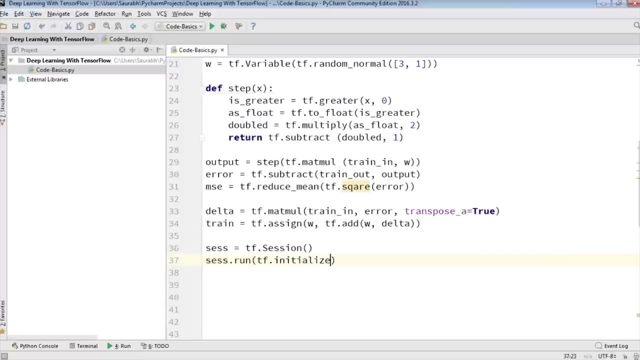 So first let me just type in here: says equals to TF, dot session. And then I'm going to type in here: says dot run, TF, dot initialize, Underscore, all variables. So now what our next task is in order to perform various iterations so that we get zero error. 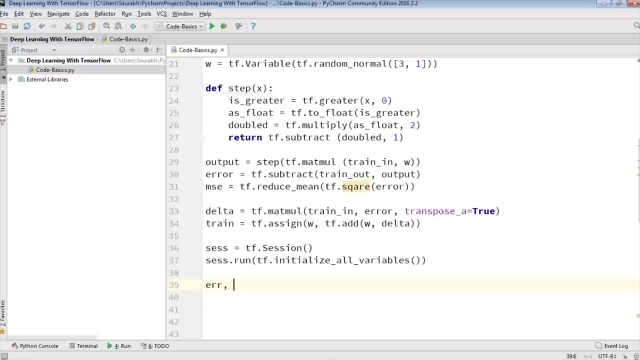 So what we're going to do, we're going to define a variable, ERR, and our target. So, basically, our ERR is nothing but error, which can be equal to 1 or 0, because we are using binary output. So our error can be 1 and our target is to make it as 0. right now. 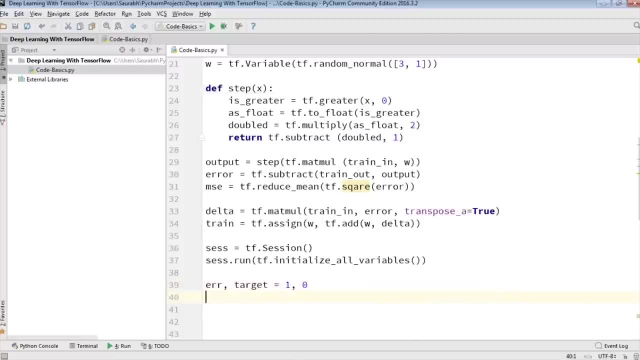 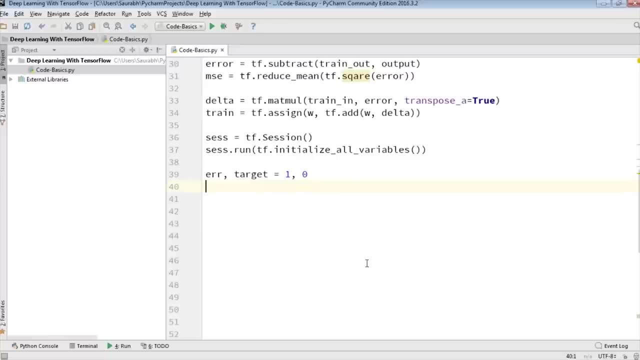 Next, what we're going to do. We're going to define a park. Now. you can consider right now a park as nothing but the number of cycles, or you can say number of iterations that will be required in order to reach the desired output. or you can say, in order to reduce the error to 0.. 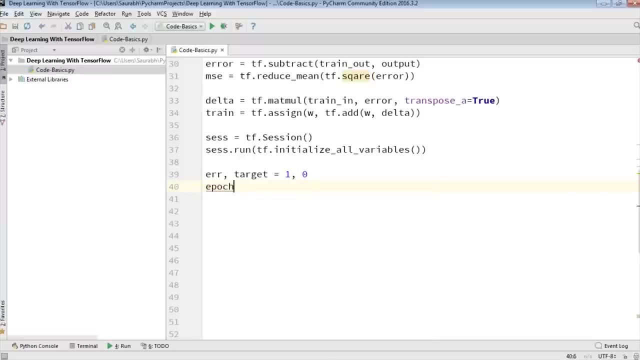 So I'm just going to define that. so I'm going to type in here a park, or you can give whatever variable name you want, And I'm going to type in here, Max underscore, a park Equal to 0 comma 10, which means that our it will start from the 0th Epoch and our maximum value of Epoch will be 10.. 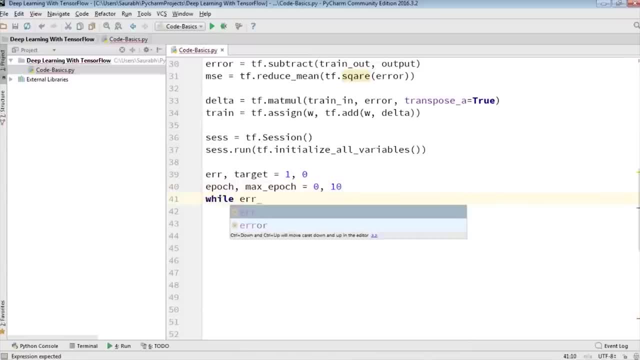 Now I'm going to define: while ERR should be is greater than Target And Epoch is less than maximum, Epoch Increase the value of Epoch y1.. Then I'm going to type in: ERR says dot run Mean squared error, comma train. And let's just finally print it and see what happens. print a park. 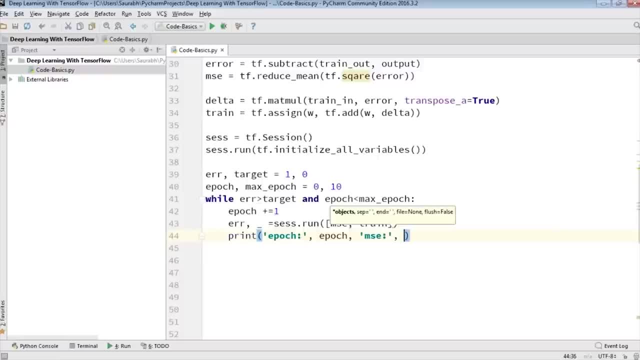 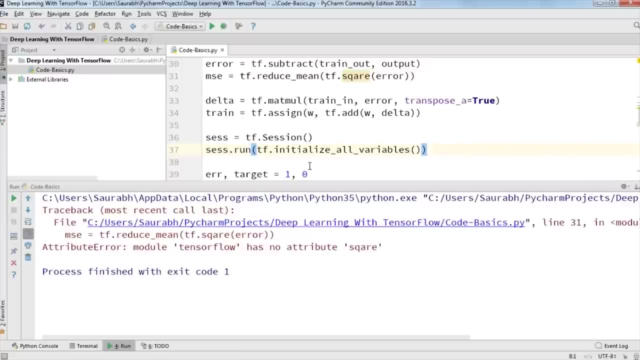 Mean squared error, colon ERR. So, basically, what it will print? it will print the cycles, or Epoch, and the error with respect to that particular cycle. So let us go ahead and execute this and see what happens. Oops, I've typed the spelling of square wrong. 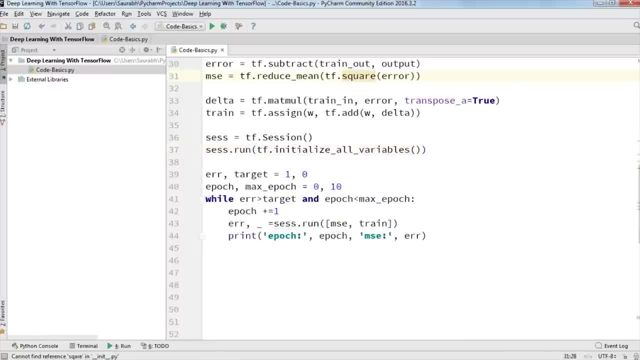 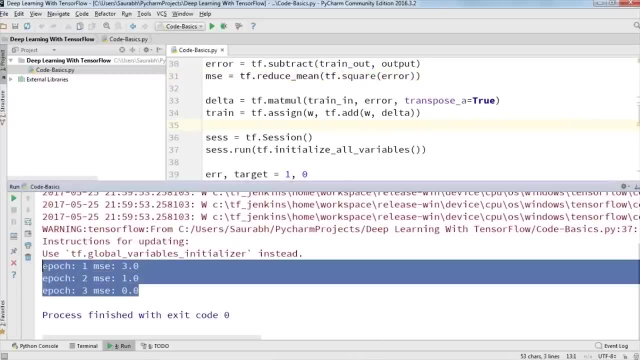 Pardon me for that, So I'm just going to make it right now. SQ, you are e? All right, let's go ahead and execute it once more. So yeah, in three Epochs we got the value of mean squared error as 0.. 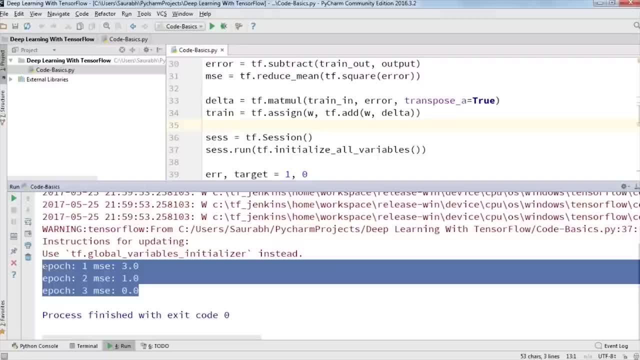 That means it took us three iterations in order to reduce The output to 0.. So this is how you can actually implement a logic gate. or you can say: this is how you can actually classify the high and low outputs of a particular logic gate using single-layer perceptron. 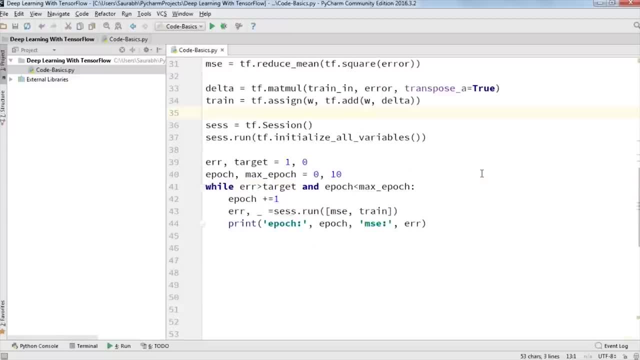 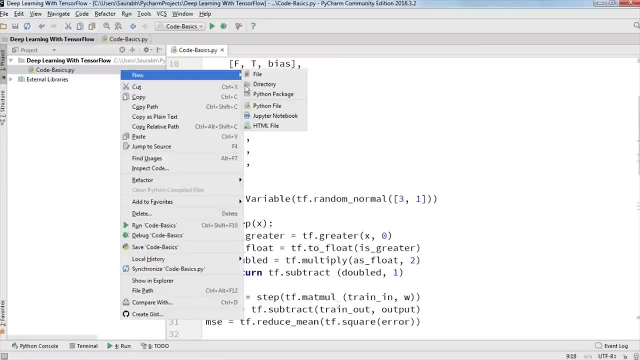 Similarly, you can do that for our gate as well. Consider this as an assignment. come up with a code that can actually classify the high and low outputs of an or gate. So what I'm going to do? I'm going to create a new python file. 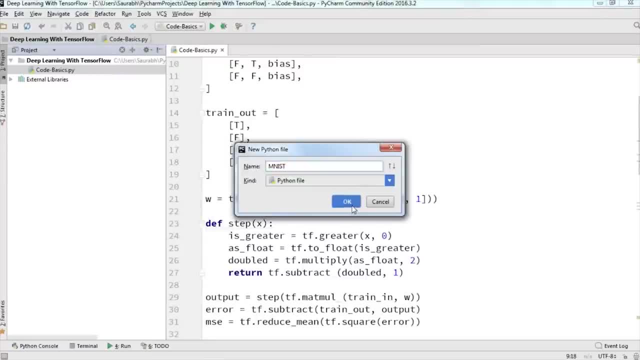 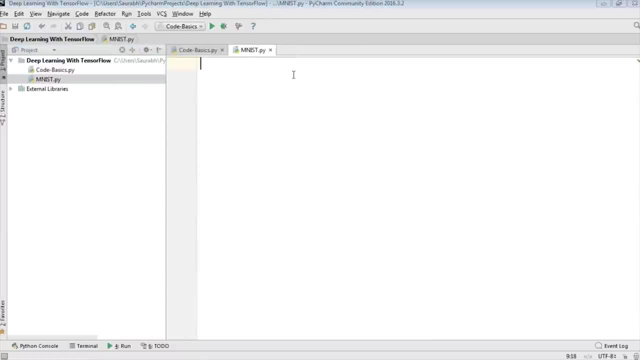 and I'm going to name it as M NIST, which is nothing but the data set on which we are going to perform the classification of handwritten digits. So we're going to execute a use case- and we have told you earlier as well- in this MNIST data set. 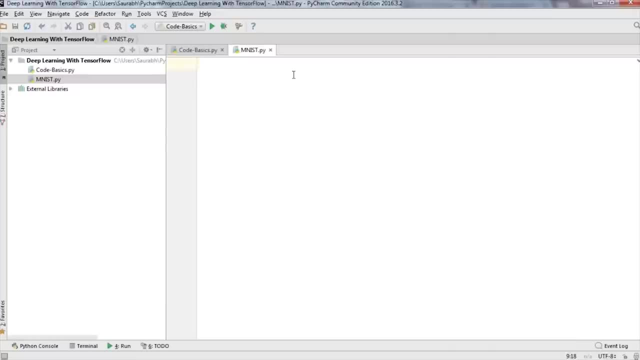 We have handwritten digits between from 0 to 9, and it has 55,000 training sets as well as 10,000 test sets, So let's go ahead with that. The first thing I'm going to do is download the data set. 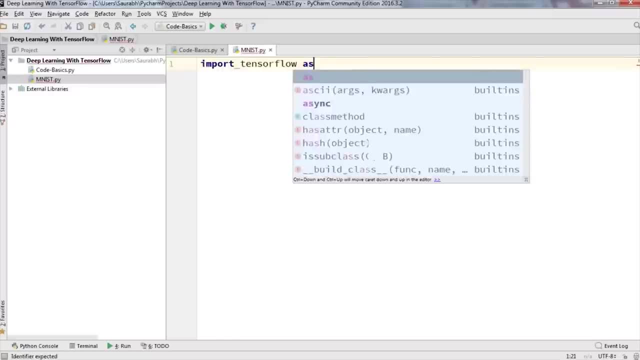 But before that let me just import tensorflow library as TF. and yeah, now let us download the data set. So for that I'm going to type in from tensorflowexamplestutorialmnist: import input underscore data. And now I'm going to type in here: 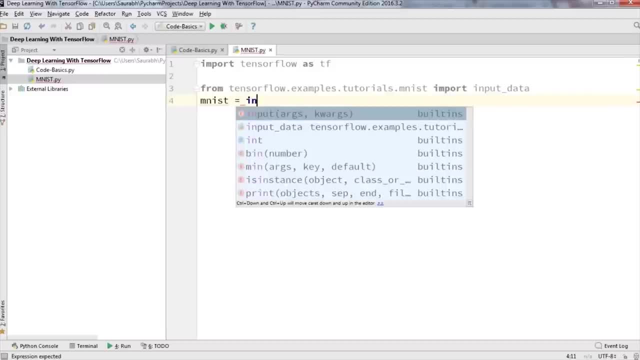 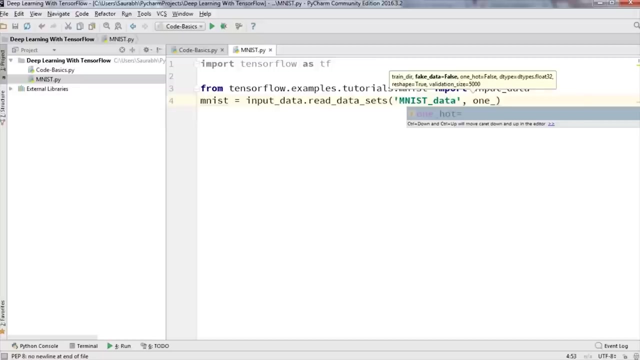 MNIST is equals to input underscore data and this underscore data dot read data sets. Type in here: MNIST underscore data. Comma 1 underscore hot equals to true. Now here, MNIST is nothing but a lightweight class which stores the training validation. 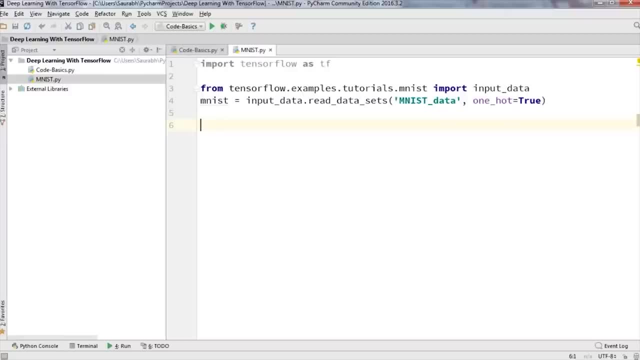 and testing sets as a numpy y arrays. And when I talk about this, one hot equals to true, is nothing but one hot encoding. Now let me tell you what one hot encoding is. So for that, let me just comment. I'll give you a few lines. 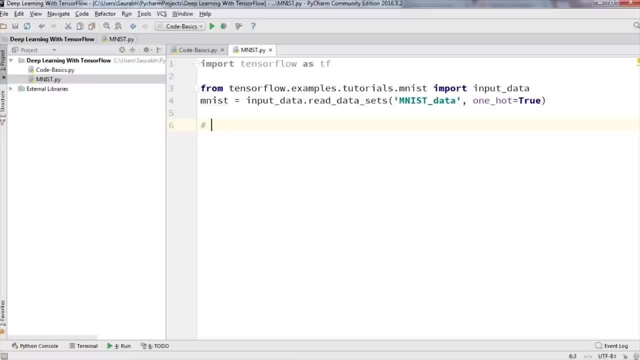 So one hot encoding means that if I'm classifying something as a seven, so if I classify that my digit is seven. so how am I going to represent that? So I'm going to type in here: 0, 1, 2, 3, 4, 5, 6, 7th. a bit will be active. 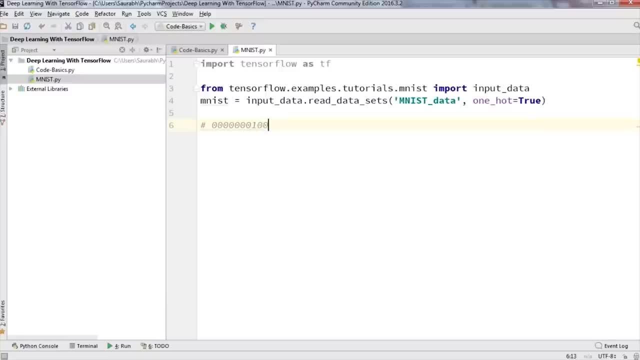 So I'm going to type in there one, then eight and then nine. Similarly, if I want to represent, say, that my digit is two, So I'm going to type in zero, one. on the second digit, I'm going to type in here as one and the rest all zeros. 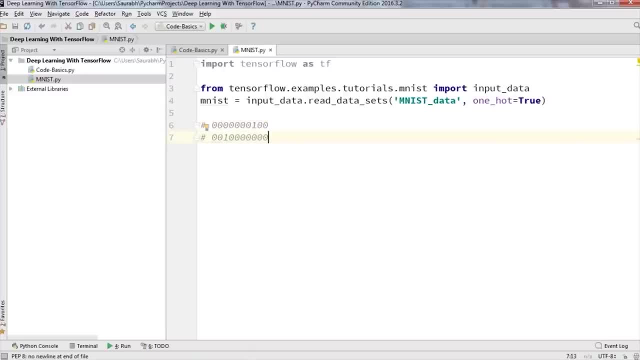 So I hope you got the concept of what exactly one hot encoding is. So it's like only one output is active at a time. That's all, and I'm telling it to you again and again. We are going to discuss everything in detail in the upcoming sessions. 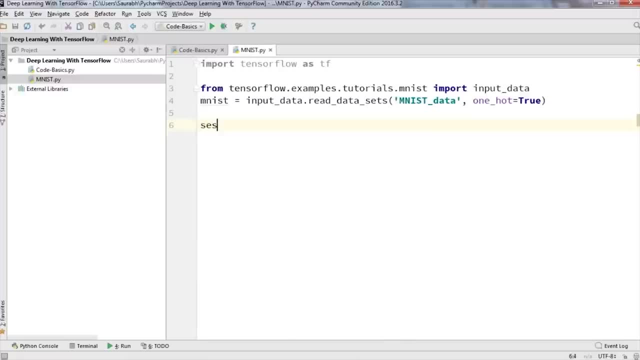 So our next step is to start the session, like we do every time. So I'm going to type in here: sets equals to TF dot interactive session. So I'm just going to type in here: interactive session. Yeah. And now we are going to do: we're going to build the computation graph by creating. 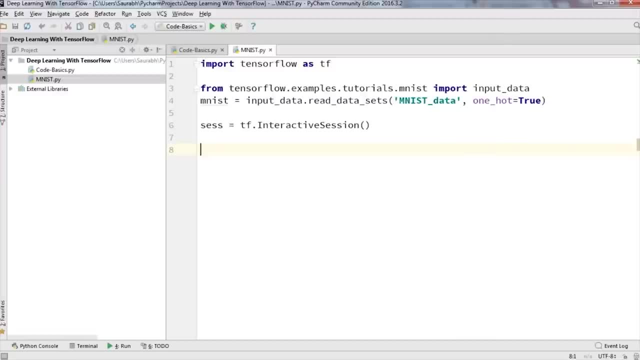 nodes for the input images and target output classes. So for that I'm going to define some placeholders, for that I'm going to type in: X is equals to TF dot placeholder, TF dot. floor 32, 32, and the shape will be none comma 784.. 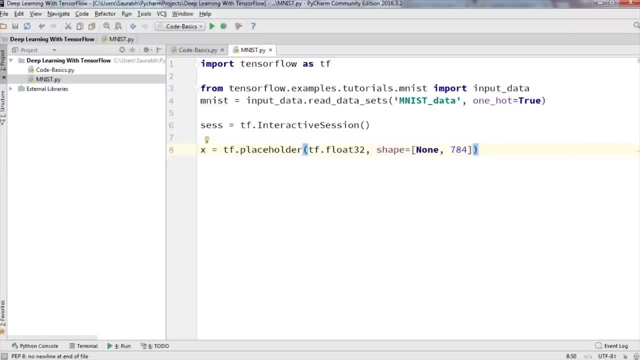 Now the input images X will consist of 2D tensors of floating point numbers. Here we assign it a shape of say none comma 784, as you can see. So where 784 is the dimensionality of single flattened 28 by 28 pixel MNIST image of handwritten digits. 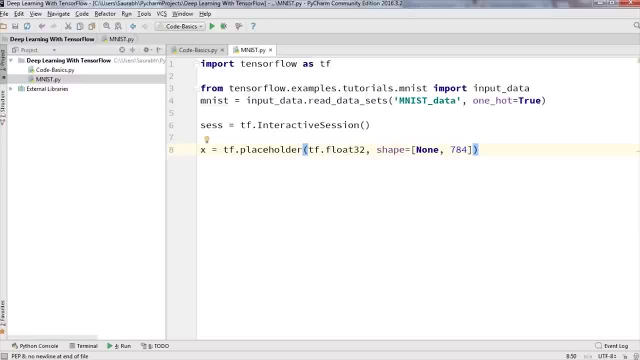 and what none indicates. it indicates that the first dimension corresponding to the batch size can be of any size, means The first dimension can be of any size. We are not putting any restrictions on that. Now I'm going to define the variable Y, which will nothing, which will be nothing but our real labels or, you can say, the desired output. 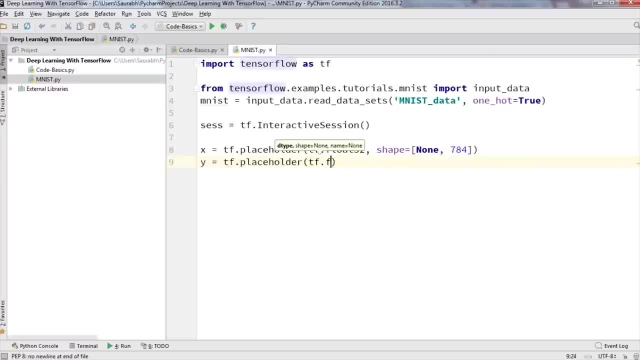 placeholder and I'm going to type in here TF, dot, float 32, and I'm going to define the shape, which will be none comma 10, because we have 10 classes. and similarly, Y is also a 2D area where each row is One hot 10 dimensional vector indicating which digit class the corresponding MNIST image belongs to. 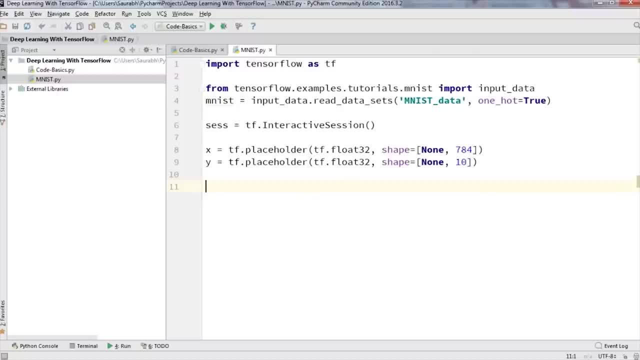 and now next step is to define weight and biases for our model, like we have done in the previous example. So we could imagine treating these like additional inputs, but tensorflow has even a better way to handle them, and what it is? it is nothing but variables. 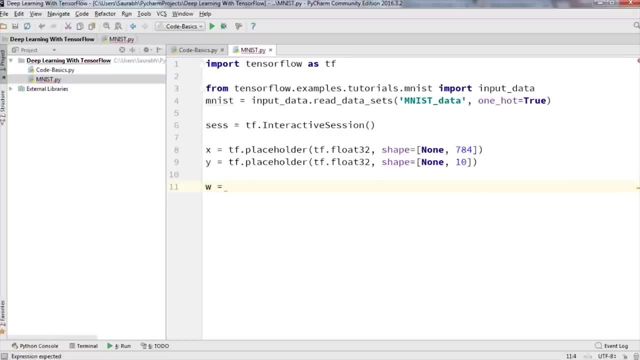 So let us go ahead and do that. I'm going to type in here W TF dot, variable, TF dot zeros. I'm going to initialize it to zeros and the shape will be a 784 comma 10.. So it's like 28 cross, 28 pixels and a 10 classes. 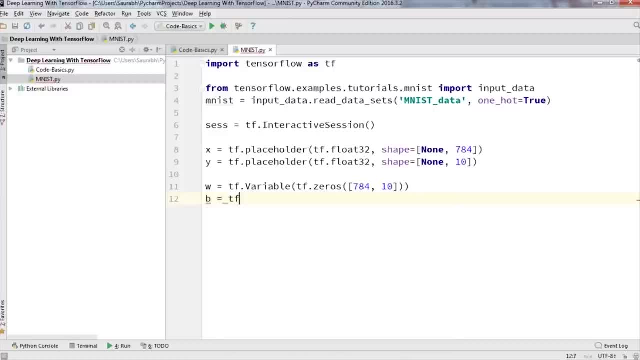 Similarly when I talk about bias. so it will be TF dot variable. TF dot zeros. initialize it to zeros and the shape will be 10.. We pass the initial value for each parameter In the call to TF dot variable. Now over here, as we can see that we initialize both W and B as tensors full of zeros. 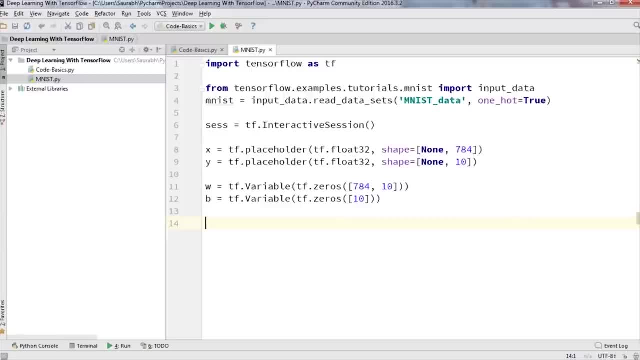 and W is a 784 cross 10 matrix because we have 784 input features and 10 outputs. and when I talk about bias B, it is a 10 dimensional vector because we have 10 classes And we have learned that before we can use variables in a session. 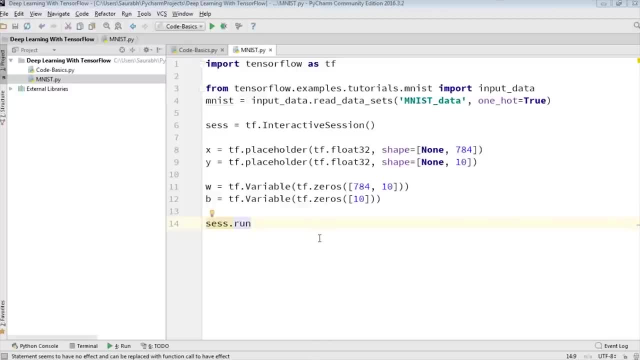 We need to first initialize it. So we're going to type it here: says a dot run, and after that I'm going to type in F, dot, global underscore variables- Underscore initializer. All right, so we have initialized all the variables. 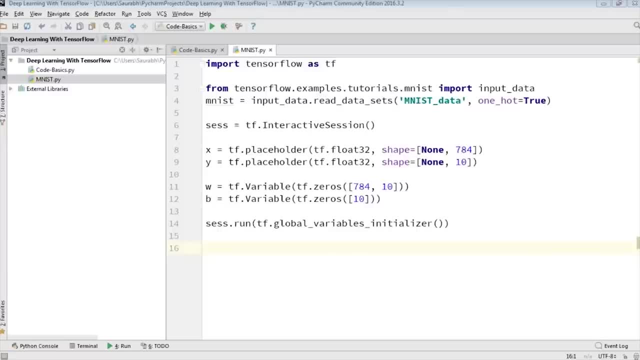 So our next task is to predict the class and the loss function. So we can now implement a regression model. It takes only one line: We multiply the vectorized input image X by the weight matrix W and add the bias. So for that. 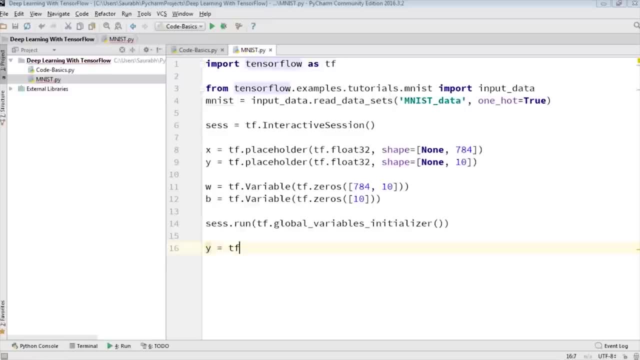 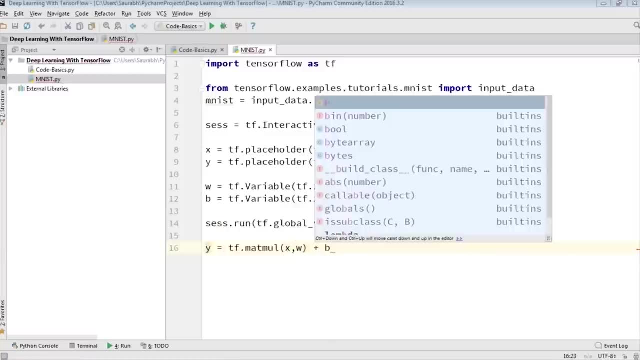 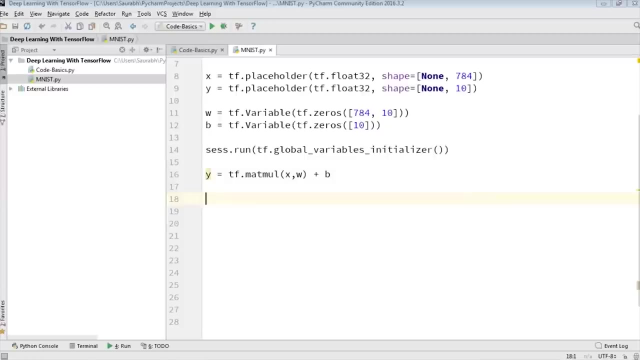 I'm just going to type in here: Y equal to TF, dot matma. That is nothing but matrix multiplication, X, comma, W plus B. All right, So now we can specify a loss function very easily. So the loss indicates how bad the model's prediction was on single example. 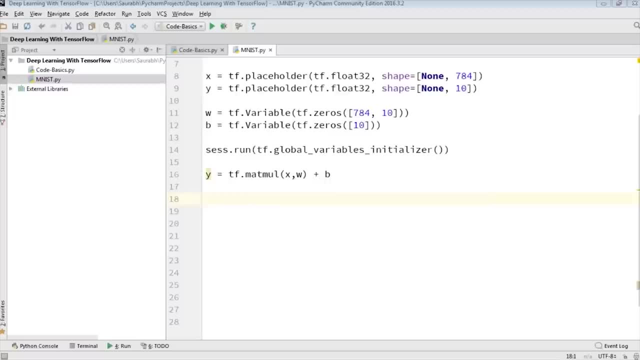 We try to minimize that while training across all the examples. So now we can specify a loss function. Now, loss indicates how bad the model's prediction was on a single example and we try to minimize that while training across all the examples. Now, here our loss function will be cross entropy. 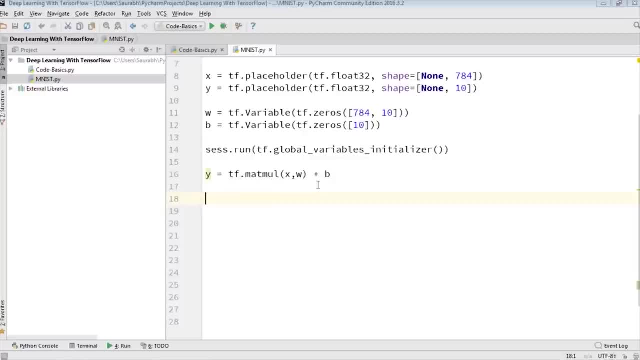 or you can say the difference between the actual output and the predicted output. So for that, what I'm going to do, I'm going to you make use of softmax cross entropy function. So here the loss will be the difference between the target output and the actual output. 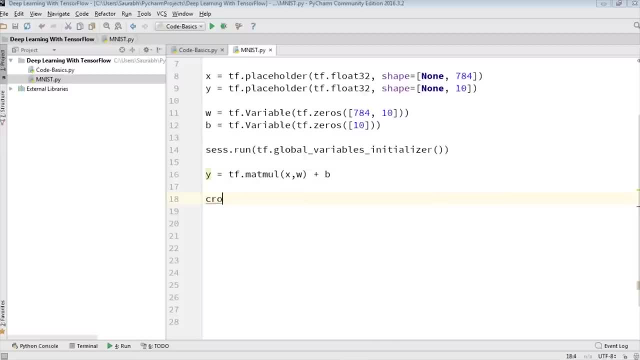 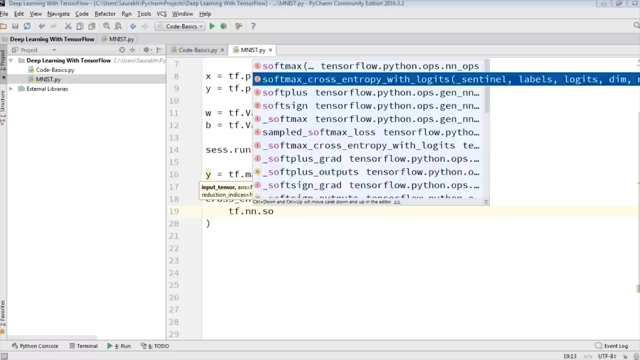 So for that, what I'm going to do is I'm just going to type in here a variable name. I'm going to name it as cross entropy, And yeah, entropy equals to TF, dot, reduce, underscore mean- And then just type in here: Let me just enter the next line: TF, dot, NN, dot, softmax, underscore cross entropy, with logits. 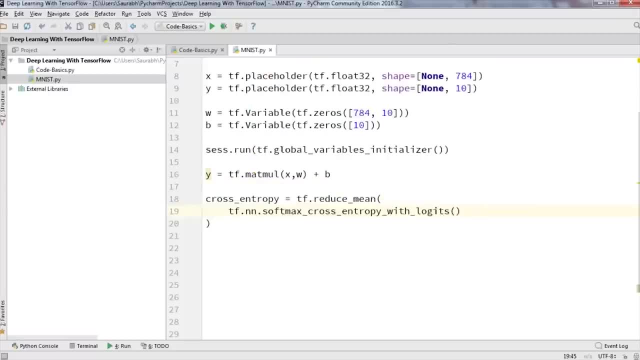 And now over here, I'm going to type in first our target output, which will be labels, equals to Y comma. our actual output, So it'll be logits, is equals to Y. That's all So over here. let me just give you a brief idea of what is happening. 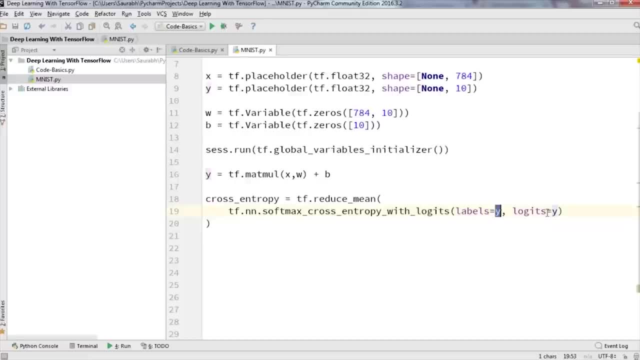 So labels is equals to Y Means that this is our target output and this is the actual output. So it will be, will name it as Y underscore, And so what exactly is happening? It will calculate the difference between the target output and for the actual output. for all the examples: 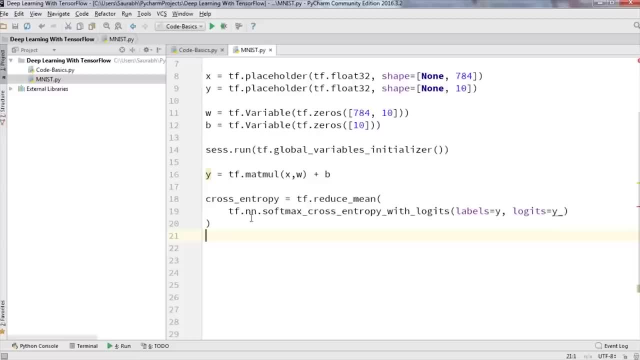 Then it is going to sum all of them and then find out the mean. So this is what, basically, this cross entropy variable will do, Now that we have defined our model and training loss function. It is straightforward to train using TensorFlow. Now we need to train our model. 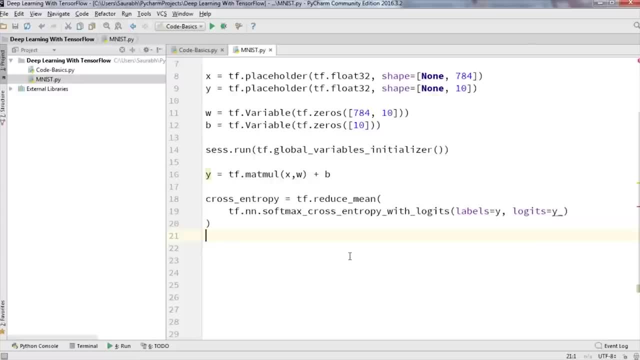 So TensorFlow has a wide variety of built-in optimization algorithms, as I've told you Earlier as well, And for this example we'll use steepest gradient descent with a length of about 0.5 to descend the cross entropy. So basically, we're going to use a 0.5 learning rate or you can say the step length. 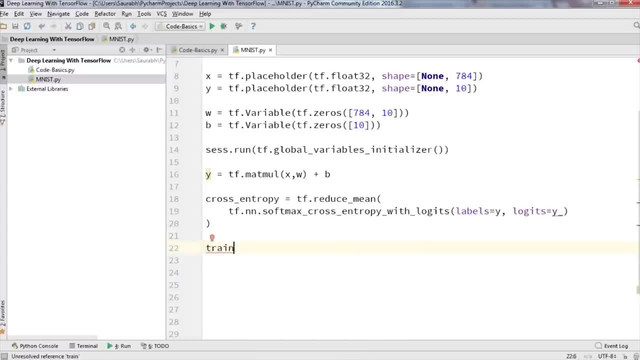 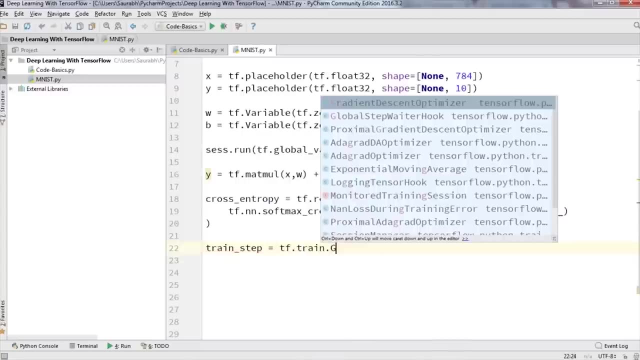 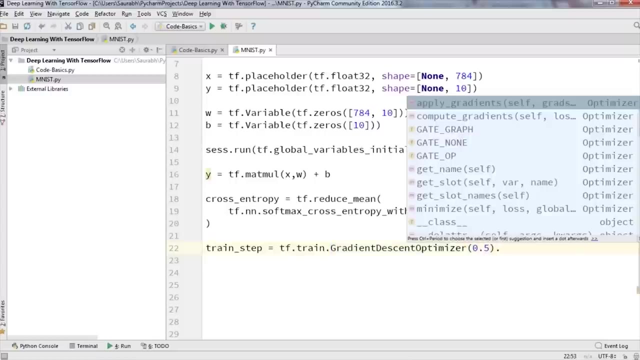 So for that I'm going to type in here: train underscore step Equal to TF dot, train Dot gradient descent optimizer and the step will be 0.5 and minimize The loss, minimize cross entropy, That's it. So what this one line basically will do, it will minimize the cross entropy. 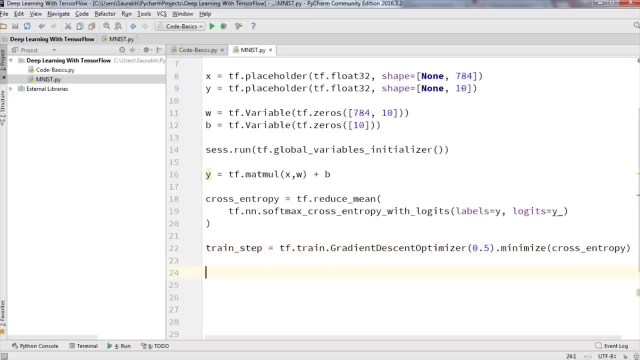 which is nothing but the loss function that we have defined. Now, in the next step, what we are going to do: we are going to load hundred training examples in each training iteration. So each time the training iteration happens, it will take hundred examples. We then run the train underscore- step operation. 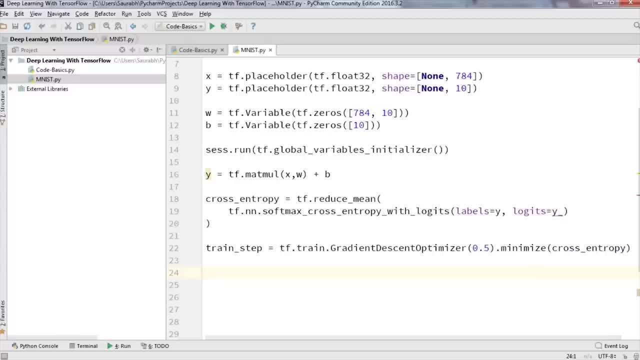 which is nothing, but to reduce the error using feed, underscore, dict, or which is nothing but we are going to feed the real values to our placeholder Y now. next, what we are going to do: We're going to load a hundred training examples in each training iterations. 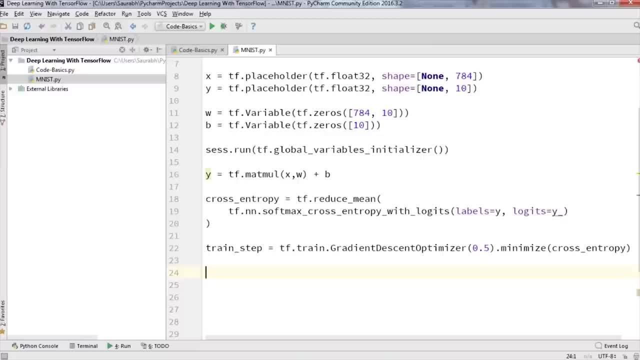 which means that for each iteration will take hundred training examples and will run the train underscore step operation, which is nothing but the optimizer. here and after that we're going to use a feed underscore dict to replace the placeholder tensors X and Y with the training examples. 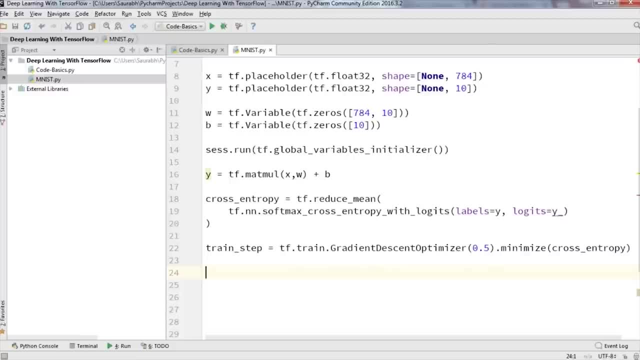 So basically X will contain the input images and Y will contain the actual outputs, or you can see the desired outputs for that. I'm going to type in here for underscore in range: thousand Batch equals to mnist dot, train dot. next underscore batch: hundred train underscore step dot run. 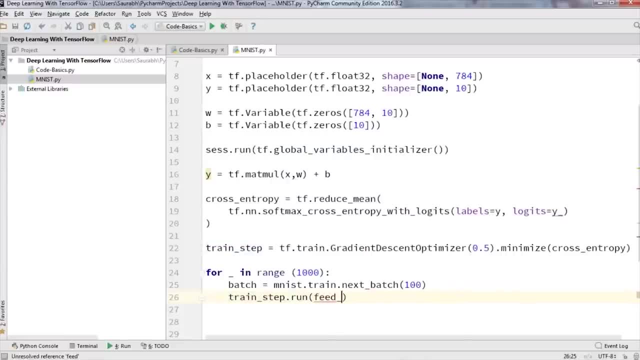 and I'm going to feed in the values to X and Y variable feed underscore: dict: equal to X colon Batch zero comma Y colon, batch one. That's it. Now we need to evaluate our model, We need to figure out how well our model is doing, and for that, 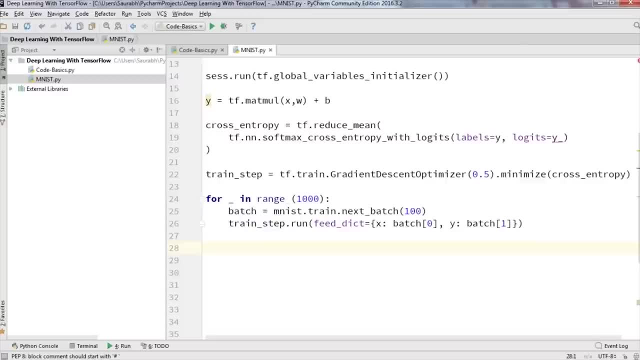 I'm going to make use of TF dot- argmax function. Now, this TF dot- argmax function. Let me tell you how it works. first I'm going to type in here correct underscore: prediction: Equals to TF dot. equals TF dot- argmax. 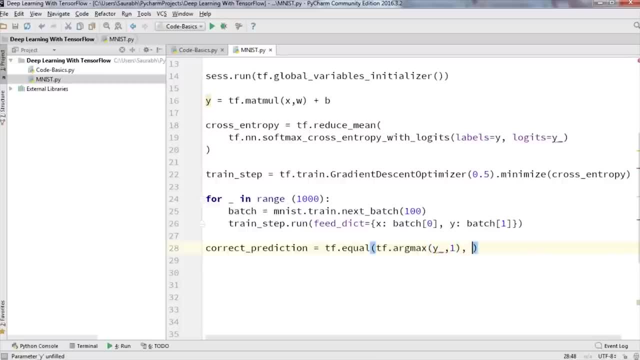 Y underscore comma one. Comma TF dot argmax Y comma one. So basically, this TF dot argmax of Y underscore comma one is a label. Our model things is most likely for each input That means it is a predicted value, While TF dot argmax of Y comma one is a true label. 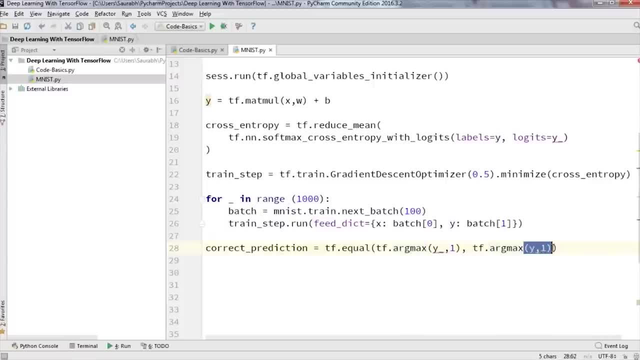 It is there in our data set present already, and we know that it is true. So what we are doing? we are using TF dot equal function to check if our actual prediction matches the desired prediction. This is how it is working. So now what we're going to do. 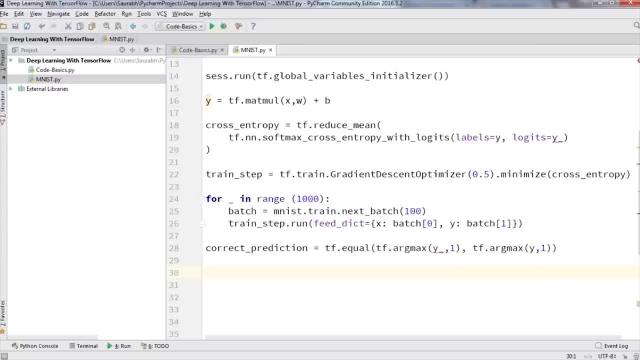 we're going to calculate the accuracy to determine what fraction are correct. We cast a floating point numbers and then take the mean, repeat. So now I'm going to define a variable for accuracy, So just going to type in: accuracy equals to TF, dot, reduce, underscore mean. 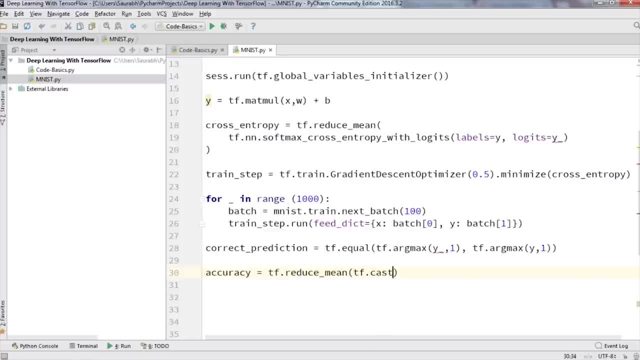 TF dot cast correct underscore prediction Comma: TF dot float 32.. And what we can do? finally, we can evaluate our accuracy on the test data, and this should give us accuracy of about 90%. So let us see if that happens. I'm going to type in here: print: accuracy dot- evaluate eval feed underscore dict. 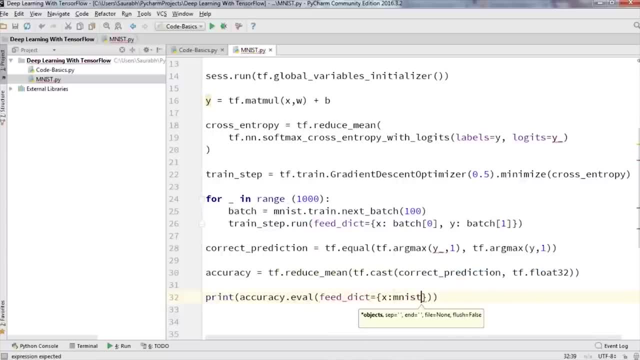 Equal to X Colon: MNIST dot test dot. images. Comma Y colon: MNIST dot test dot labels. That's it, guys, and I've done a mistake here. Instead of Y, it will be Y underscore, because this is our predicted value, not the actual value. 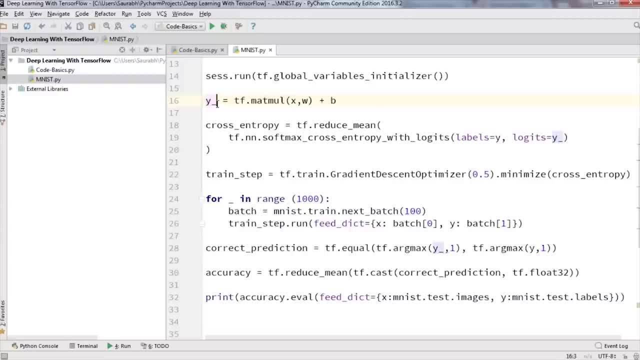 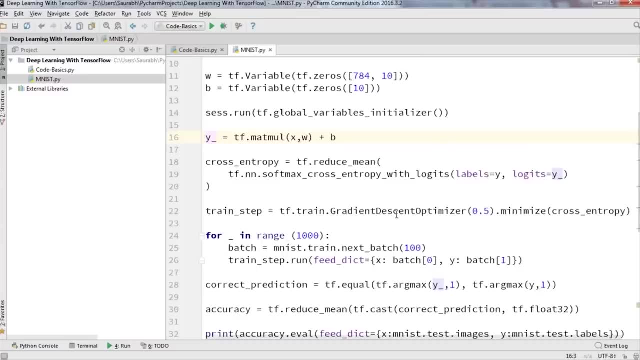 and why we have considered as actual value and this Y underscore will be our predicted values. This is the mistake that I made. So, yeah, now I think the code looks pretty fine to me and we can go ahead and run this. Let us see what happens when we run this. 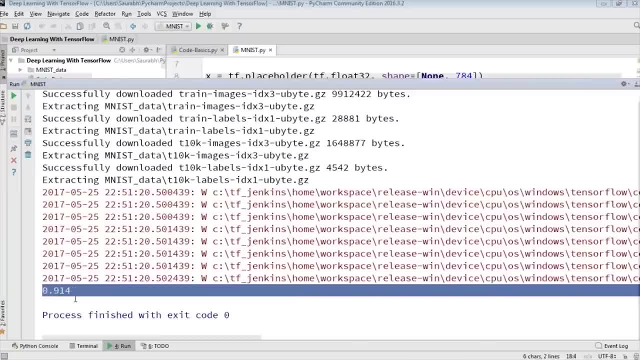 So, guys, it is complete now, and this is the accuracy of a model, which is 91.4%, and which is pretty bad, though, when you talk about a data set like MNIST, but yeah, with a single layer which is very, very good. 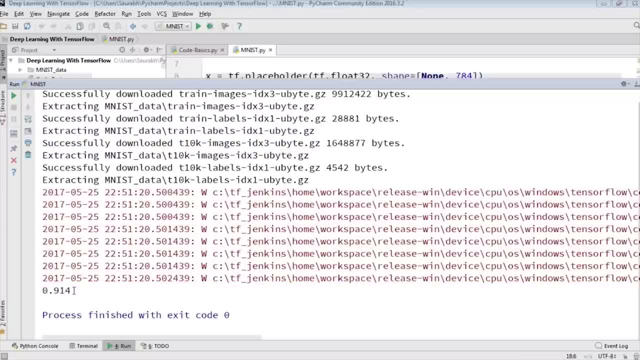 So we have got an accuracy of around 92% on the MNIST Dataset, which means that whatever the test data sets were there, that is like 10,000 test images. So on those test images, whatever the prediction our model has made, are 91.4% correct. 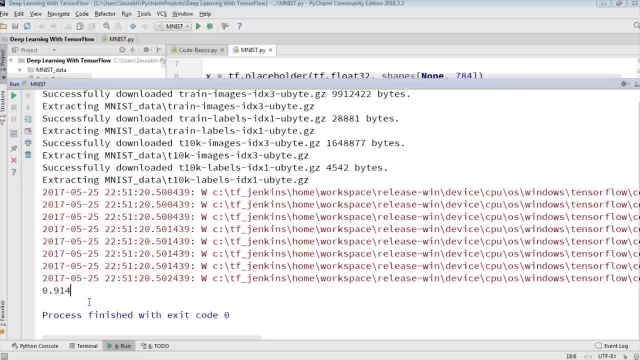 So, guys, let me just give you a quick recap of all things we have discussed. So first we saw what exactly is deep learning and how it is different from the traditional machine learning. Then we understood the motivation behind deep learning, which is nothing but your brain cells, which are called neuron. 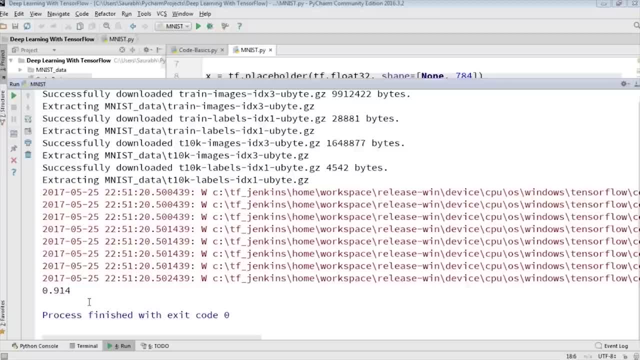 Then we understood the importance of why we need artificial neurons. And then we took the example of artificial neuron, which is called a perception, and we are looking at a couple of examples in which we implemented the AND gate, We performed image classification on the MNIST data sets. 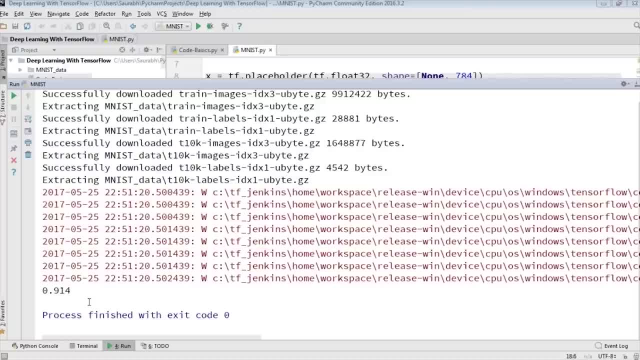 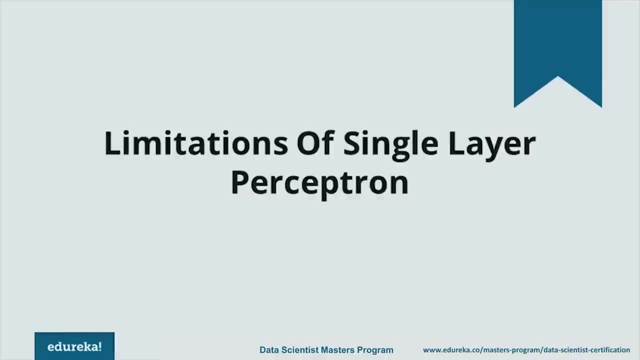 which is nothing but handwritten images between 0 to 9.. And we also implemented a couple of examples in order to understand what our placeholders, variables and constants. So now there are certain limitations of single layer perception. Let us understand that. So, in order to understand that, we'll take an example. 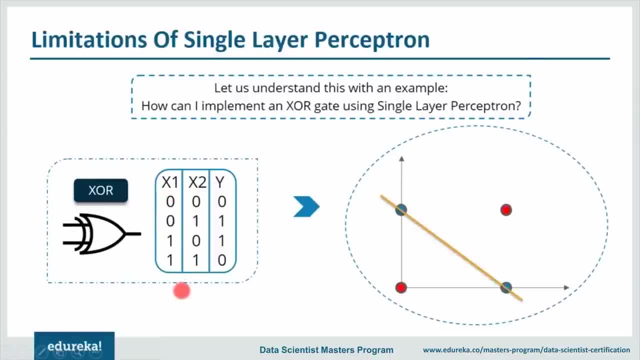 So we have an XOR gate here And this is a truth table. So, according to this truth table, if any one of the input is high, then the output is high, And if both the inputs are low, output is low, And if both the inputs are high, output is low. 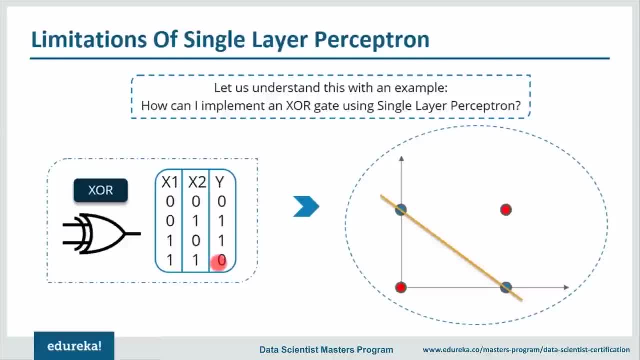 So how can you classify the high and the low outputs with a single line? Definitely you can't, if you see the points. So one point is here, one is here, here and here, and which? these two points are high outputs and these two are low. 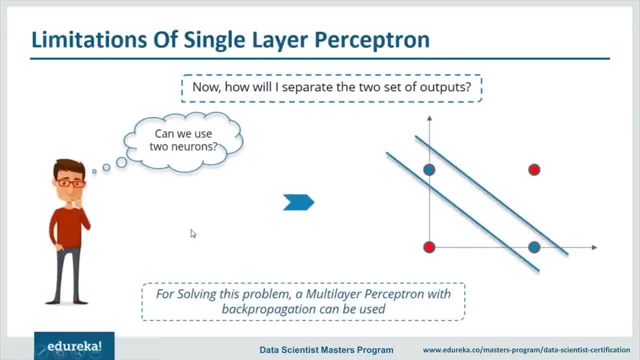 So how can you classify with a single line? Definitely you can't. So now, what's the answer to this? What if we use multiple neurons? using multiple neurons, We can have two lines that can separate it. Now we can solve this problem if we have multiple neurons. 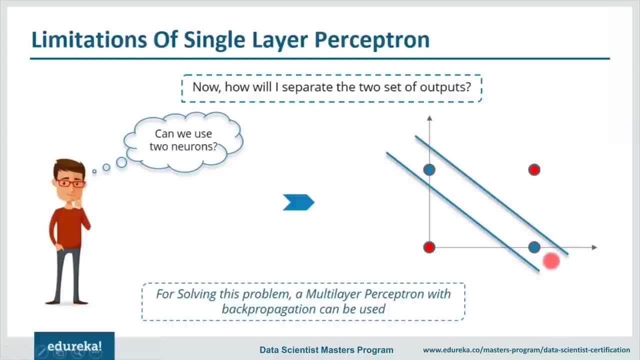 So if we use two neurons, we can have two lines and that can actually separate the high outputs as well as the low outputs. So this is where we use multi-layer perception with back propagation. So what are multi-layer perception, multi-layer perceptions? They have the same structure like the single layer perception. 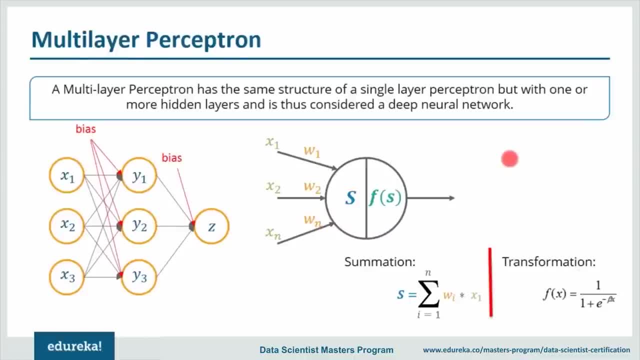 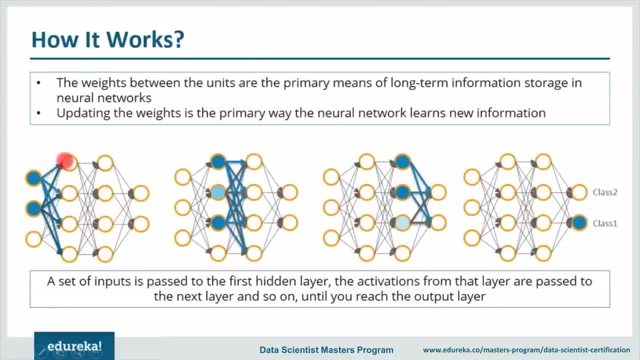 The only difference is they have more than one hidden layer. So let me Explain it to you with an example. So this is how a typical multi-layer perception looks like. So we have input layer, We have two hidden layers and we have one output layer as well. 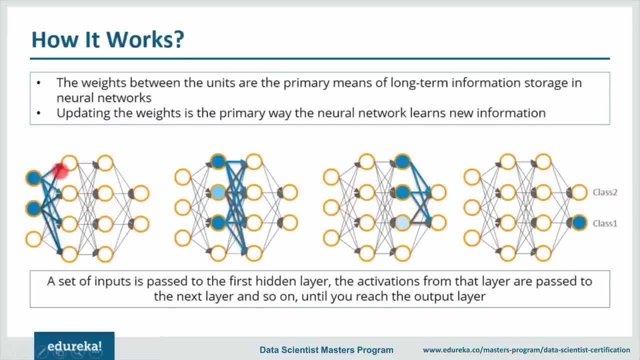 Now, typically, each of these input layers are connected to the next hidden layer. Each neuron is connected to the next neuron present at the adjacent layer, but the neurons of the same layer are not connected to each other. Now what happens? a set of inputs are passed to these input layers and the output of this input layer will be passed to the first hidden layer. 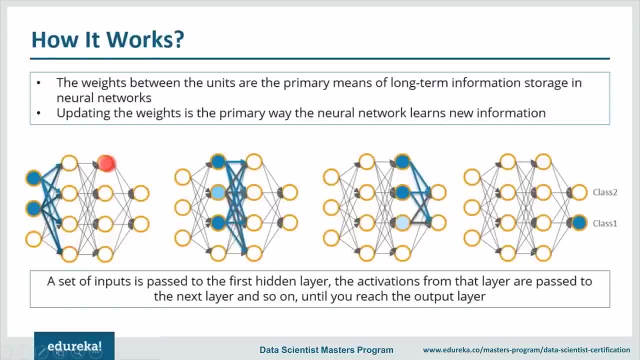 Then, after activation function Of the first hidden layer, the output will be passed to the next hidden layer as the input and similarly, finally, we get the output. Now you must be thinking how the model learns from here. So the basically, the model learns by updating the weights, and the algorithm that it uses is called back propagation. 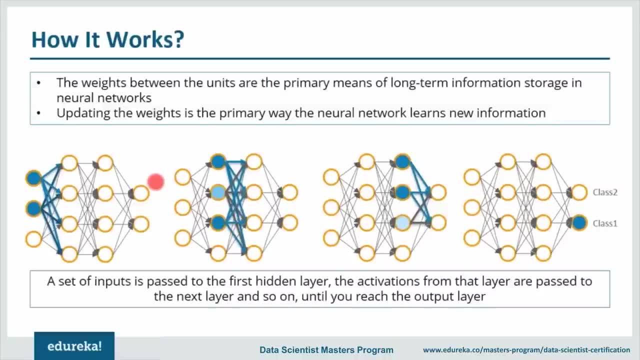 So the back propagation algorithm helps the model to learn and update the weights in order to increase the efficiency. So basically, at this process of from input layer to the output layer is called a feed forward process And then, when we back, propagate it in order to increase the efficiency or accuracy. 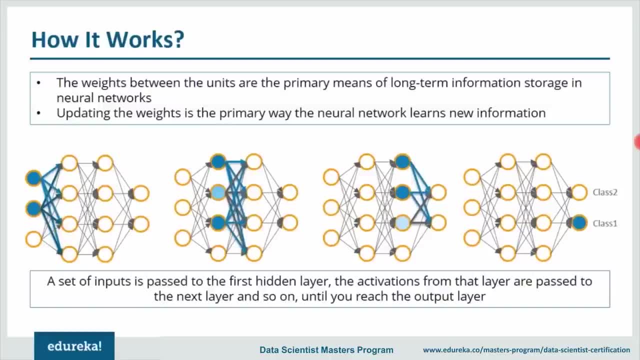 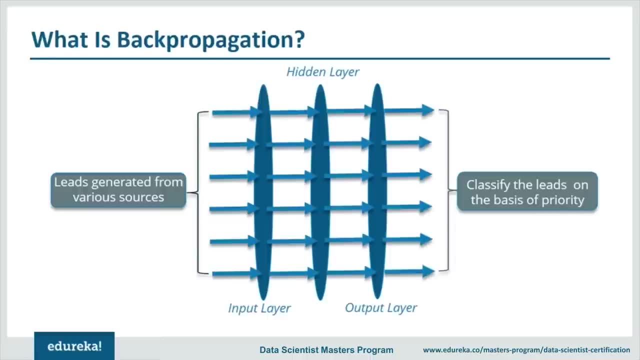 so that we can update the weights. that is called as a back propagation. We'll understand back propagation in more detail. So let us move forward and understand what exactly is back propagation. So what is back propagation? Now let us understand this with an example. 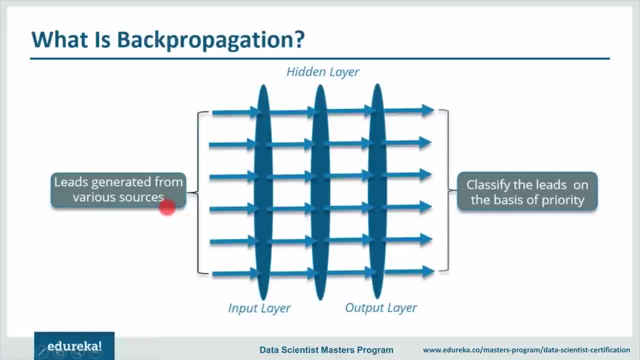 So we'll take the inputs as the leads generated from various sources, and my aim is to classify the leads on the basis of the priority, So there might be certain leads which won't make it that much difference to me, whereas compared to the other leads. 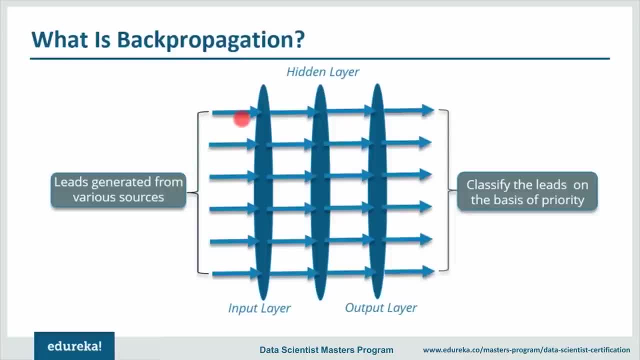 So in that case, I need to make sure the leads, Which are important, gets the highest amount of weight. How am I going to do that? first We'll see the output, then, accordingly, will calculate the error and, based on that error, We are going to update the way. and this process is nothing but your back propagation. in a nutshell, 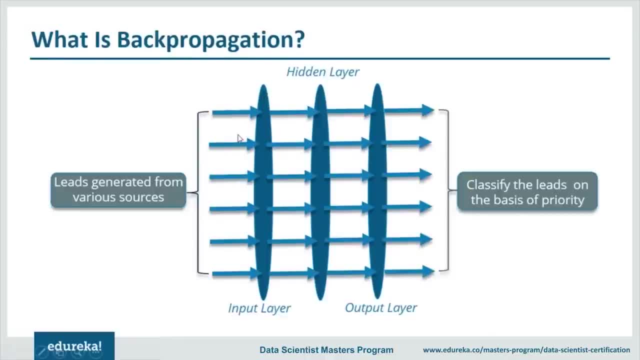 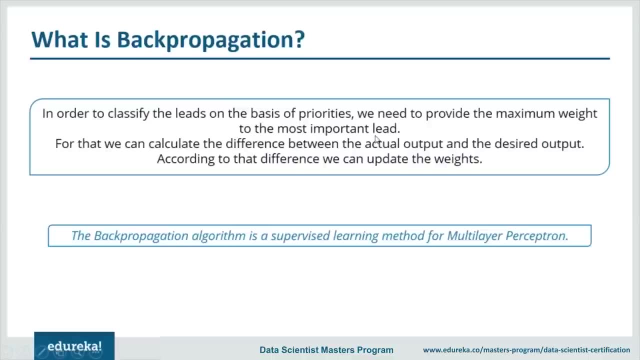 I can say right, although the algorithm is pretty complex. But yeah, this is basically what happens. So, in order to classify the leads in the basis of priorities, we need to provide the maximum weight to the most importantly. and how are we going to do that? 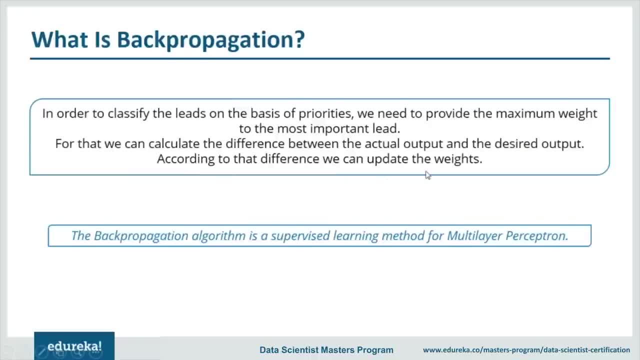 We're going to compare the actual output and the desired output And according to the difference, we can update the weights. So what is back propagation? So back propagation is nothing but a supervised learning algorithm for multi-layer perceptron. Now let us understand. what exactly is this algorithm? 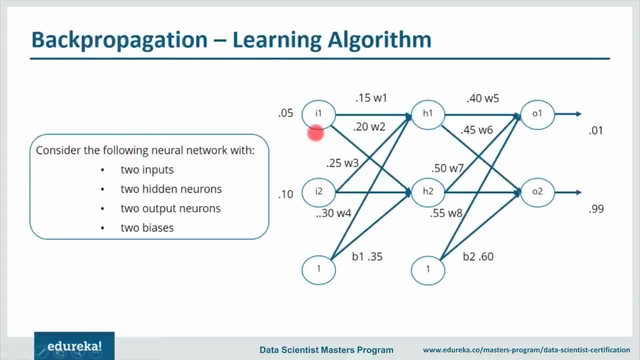 Let us understand this with an example that is there in front of your screen. So these two are our input neurons, These two are our hidden neurons and these two are our output neurons. Now our aim is to get point zero one and point nine nine as our output and at the same time, we have inputs as point zero five and point one zero. 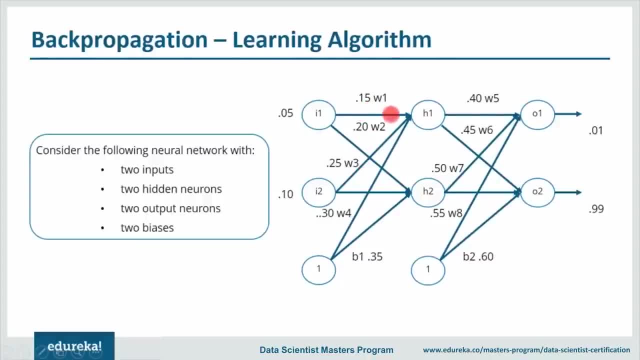 Initially, we take the weights as we can see it here. So point one: five W one. point two: zero W two. So these are the weights. plus we have two biases as well. Now what we need to do is we need to make sure that we have weights in such a way that we get output as point zero one and point nine nine. 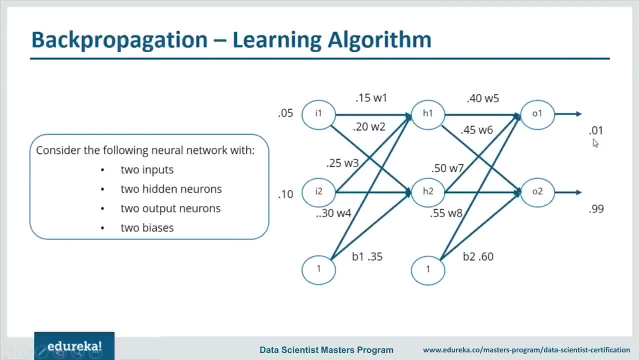 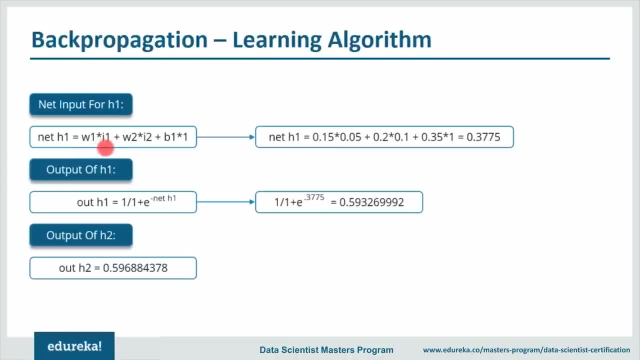 But let us see if we get that same output when we provide these kind of weights. The net input for this particular H one will be what it will be: W one into I one- That is the first input- plus W two into I two, plus B one into one. 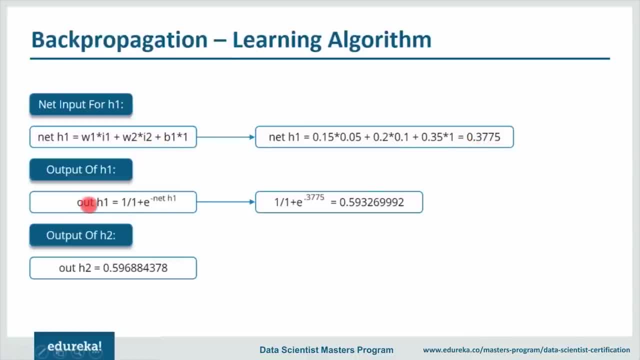 which gives us the answer as point three, double seven, five. Similarly, the output for H one will be nothing but the activation function, the output and after the activation function. and we are using her sigmoid function because our brain also uses a sigmoid functions. That's what we believe in and at the same time it is easily differentiable, and if you differentiate it twice you get the same number. 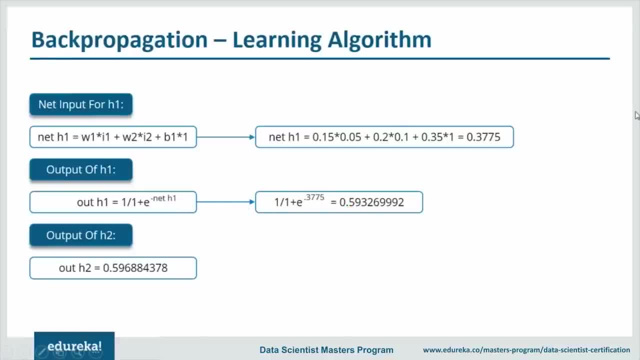 So the output of H one will be point five nine something. So let me go back. So the output of this particular H one will be point five nine something. Then we're going to calculate the output of H two as well, Similarly, and we get the output as point five, nine, six, double, eight, four, three, seven, eight. next up: 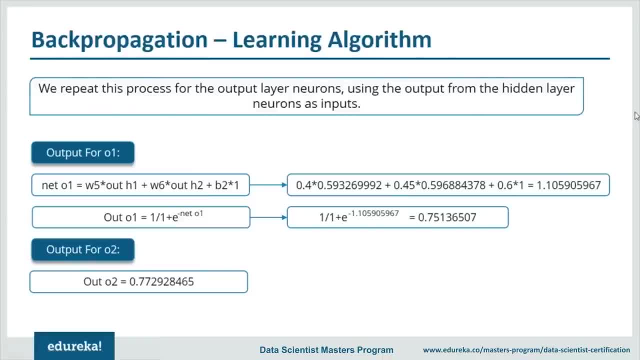 We are going to repeat the process for the output layer neurons as well. So for the output layer the net input will be W five into out of H one, W six into out of H two plus B two. That is the bias. So we get the output somewhere like this and then the net output for out O one will be after the activation function. 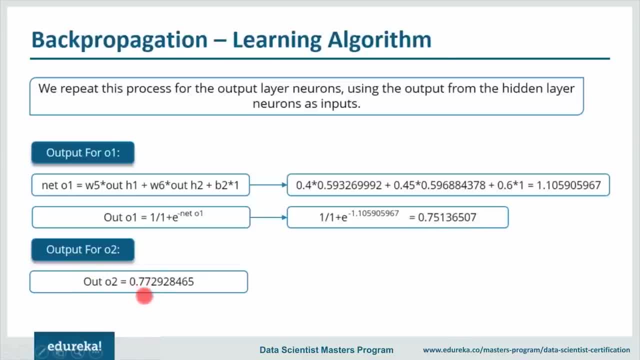 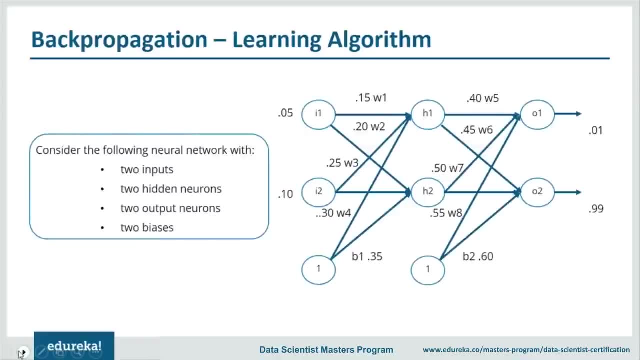 which will be point seven five one. Similarly, the output function for O two will be point seven seven. Now, if you notice that this is not the desired output, our desired output was point zero one and point nine nine. What we got instead, 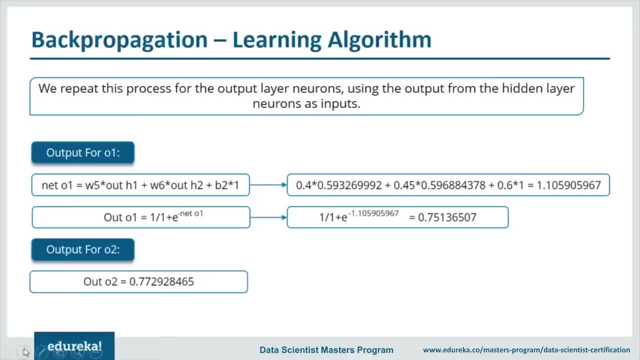 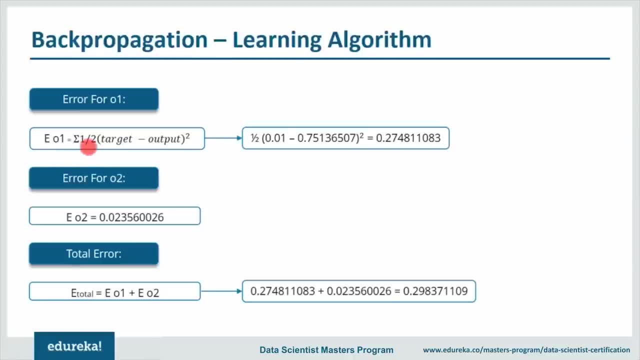 we got point seven five and point seven seven. So what we need to do, we need to update the weight. So for that we're going to calculate the error now. error for output: O one is nothing but the Sigma of one by two. target minus output. whole square target is nothing but your desired output and output is your actual output. 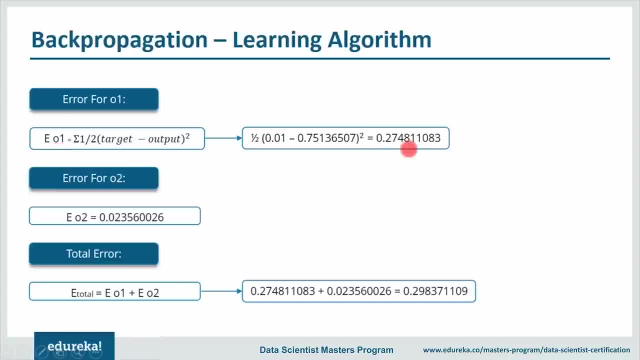 So your error of output of O one neuron will be point two, seven, eight. Similarly, for O two will be point zero, two, three. So the total error comes down to point two, nine, something Next up. we need to update the weight so as to decrease this error. 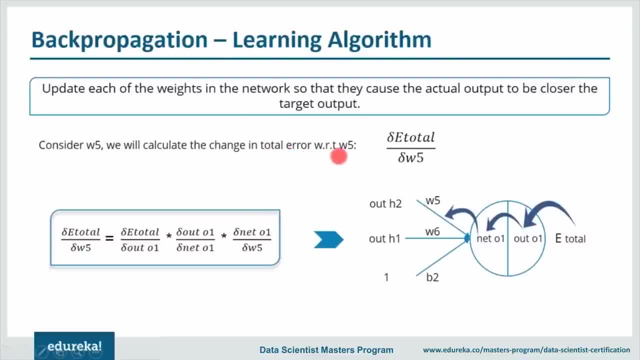 Now what we're going to do. we're going to first calculate the change in total error with respect to any of the random weight. will take W five, for example, just to show you. So we're going to calculate the change in the total error when we change with respect to the weight: W five. 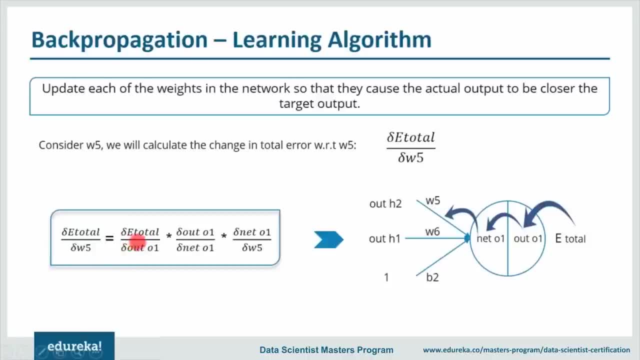 So we're going to apply a chain rule here. So using partial derivative, we're going to calculate a total by Delta of auto one into Delta of auto one by Delta of NATO one, and then Delta of NATO one by Delta of W five. 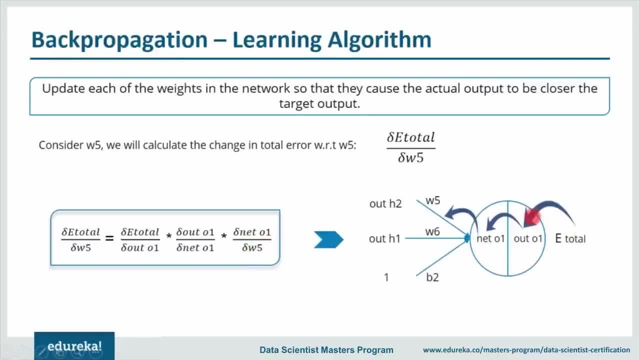 As you can see it from this particular example as well, He total, change in e total with respect to auto one, change in auto one with respect to NATO one and change in NATO one with respect to W five. We're going to multiply that and we're going to get this particular term. and let us see how we do that. 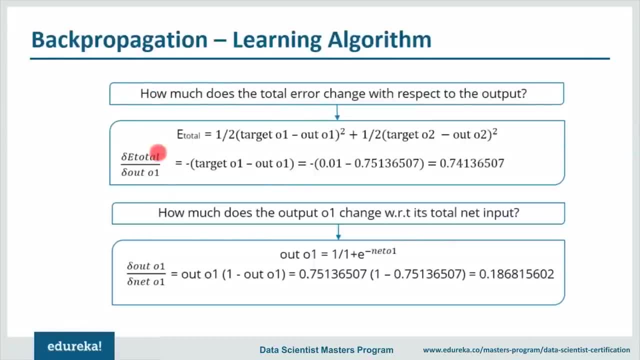 So how much the total error change with respect to the output, e total by e out one. We're going to calculate it. It came around point seven four one. Similarly, we're going to calculate how much this output or one, change with respect to the net output and we get this after that. 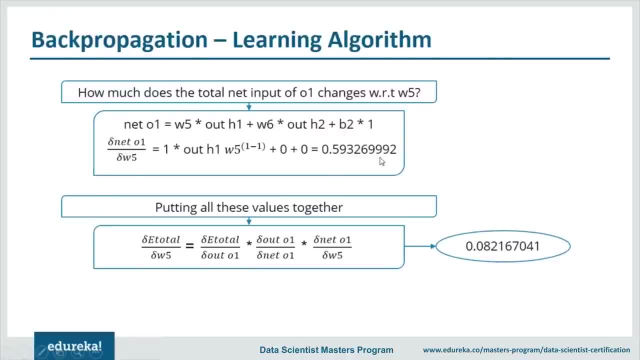 We're going to calculate it for net output change with respect to W five Also, we got this. and then, finally, what we did: we put all these values together and we found out to change in the error with respect to the change in weight, W five. 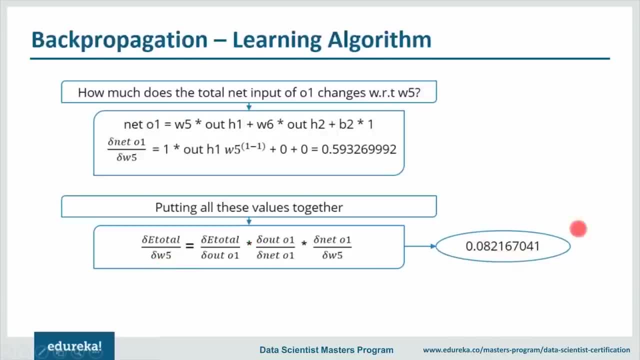 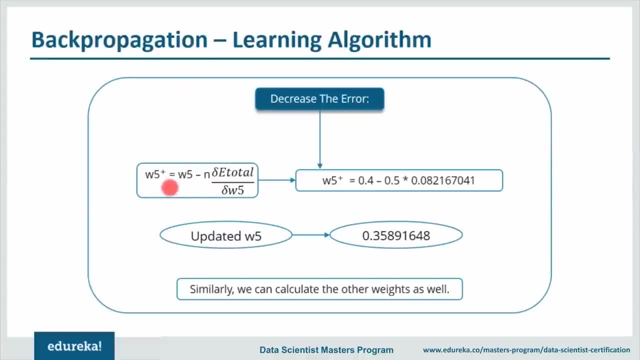 which came to up around point zero eight two one. six seven zero four one. Now is the time to update the weight. So how are we going to update the weight? First thing we need to do is we need to follow this formula: So W five plus 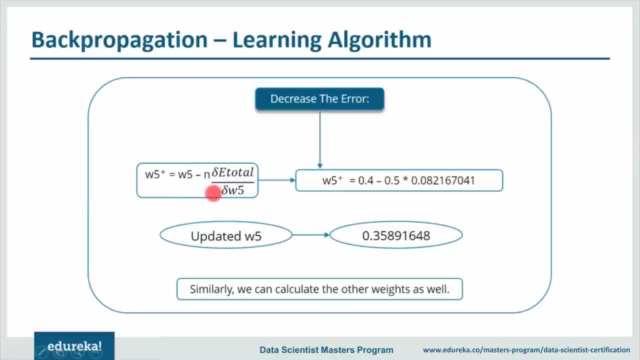 is nothing but the updated weight, which is equal to W five minus the learning rate into Delta of e, total by Delta of W five, So which came to around a point three, five, eight, nine, one, six, four, eight. Similarly we can calculate the other weights as well. 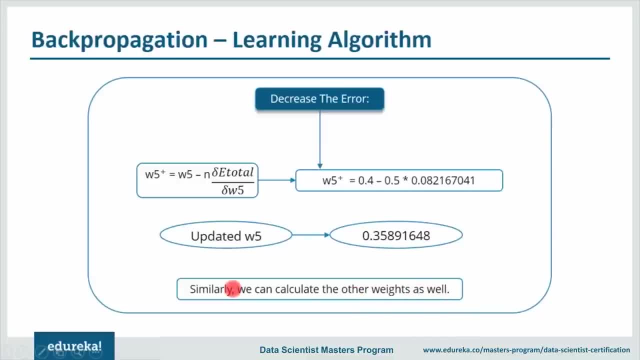 So we're going to repeat the same process and we're going to calculate the other weights as well. Then again we're going to see how much is the loss. if still the loss prevails, then we're going to repeat the same back propagation learning algorithm again, for all the ways. 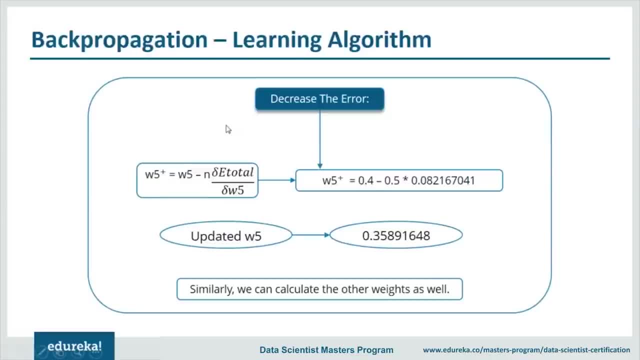 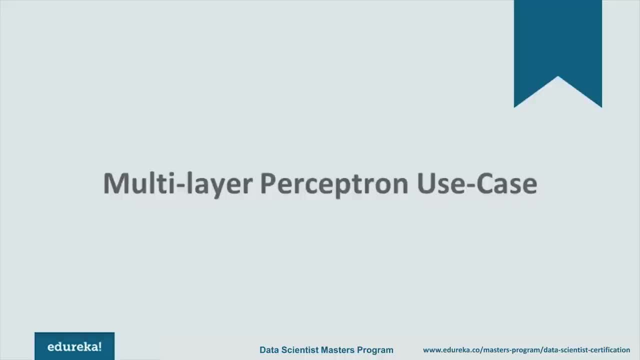 So this process will keep on repeating. So this is how back propagation actually works. So now what I'm going to do? I'm going to make use of the same MNIST data set and I'm going to increase the efficiency of that data set by 97 to 99% with the help of multi-layer perceptron. 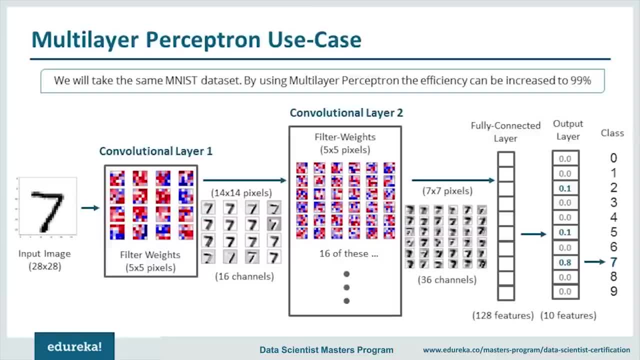 So, guys, let us go ahead with that. So, guys, as I've told you earlier, is where we are going to use the same MNIST data set which we have used in the single layer perceptron. So I'm going to perform a classification using multi-layer convolutional networks. 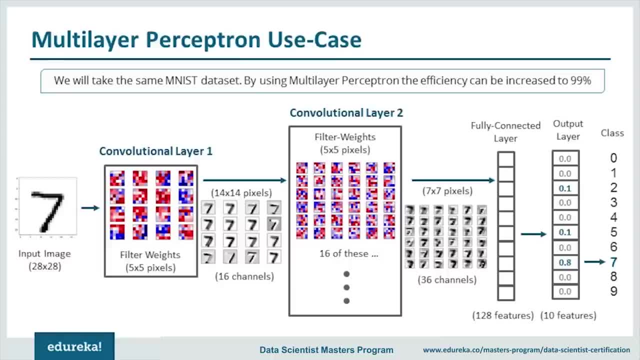 Now, what are convolutional networks? Basically, these networks are used In order to classify images. We have a separate module on convolutional networks, So you don't need to worry about it right now. So, basically, what I'm doing is I'm just trying to show you that how we can increase the efficiency using the convolutional neural networks. 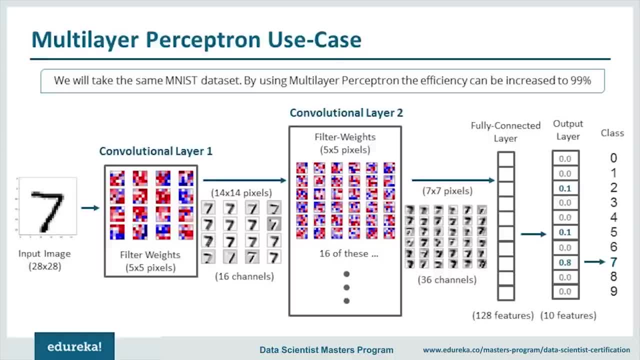 You don't have to go in much detail about it, because we'll be learning about it in the upcoming modules. I'm just giving you a general overview, or you can say a taste of how things work in convolutional neural networks. So we give an input image to this convolutional network. 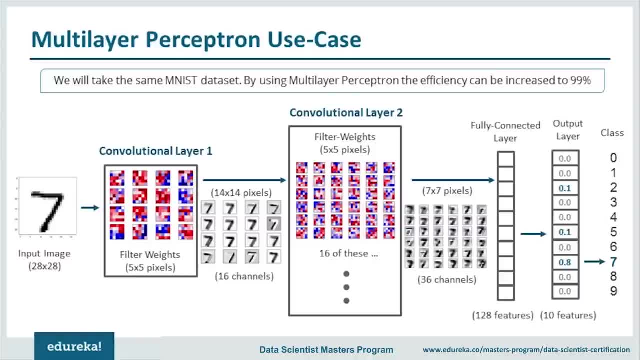 Then this input image is processed in the first convolutional layer using the filter. Wait now. this result in 16 new images, one for each filter in the convolutional layer. The images are also down sampled, So the image resolution is decreased from 28 cross 28 to 14 cross 14.. 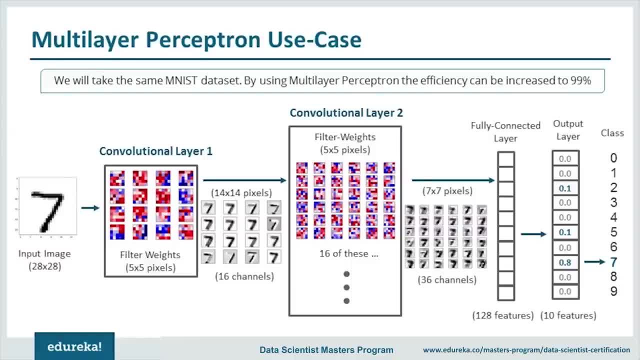 Now these 16 smaller images and from the first convolutional layer are then processed in the second convolutional layer. We need filter weights for each of these 16 channels and we need filter weights for each output channel of this layer. Now there are total 36 output channels. 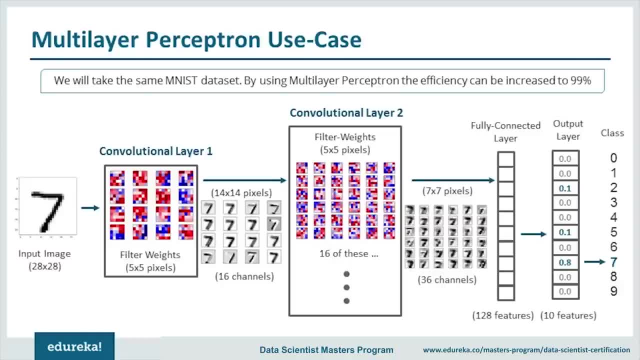 So there are total of 16 cross 36, equal to around 576 filters in the second convolutional layer. Now the resulting images are down sampled again to 7 cross 7 pixels. The output of the second convolutional layer is 36 images of 7 cross 7 pixels each. 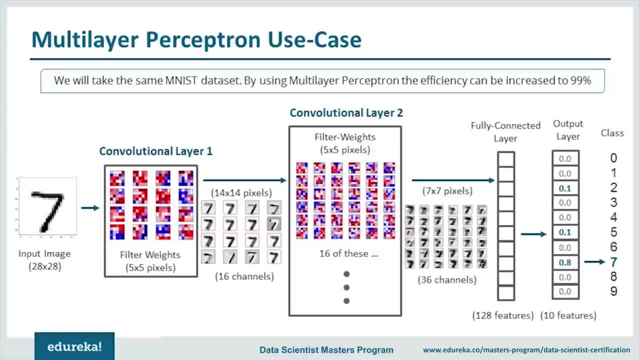 Now these are then flattened to a single vector of length 7 cross 7 cross 36, which is a 1764, which is used as the input to a fully connected layer with 128 neurons And this feeds into another fully connected layer With 10 neurons, one for each of the classes which is used to determine the class of the image, that is, which number is depicted in the image. 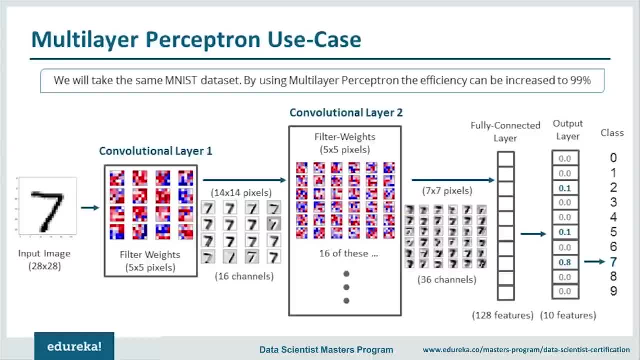 So whatever number that we provide in. so basically the output layer, or you can say the last layer or the fully connected layer with 10 neurons, is used to determine the class or which digit is the input image of. now, the input image depicts the number 7, and the 4 copies of the images are shown here. 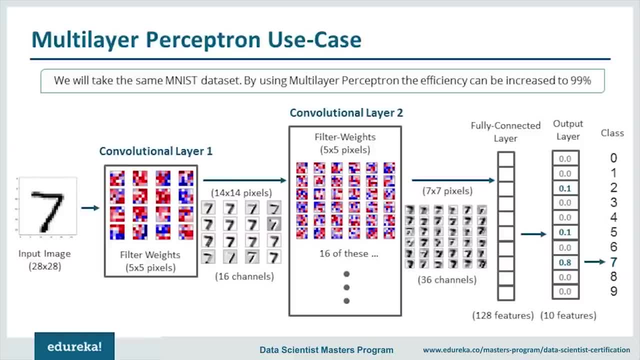 So basically what happens, whatever filter we have in each layer, it will be present on the image pixels. So there'll be a dot product of the filter And the image pixel behind that. So we'll get a dot product there. We are going to repeat that same process in each of these layers and for each of these layers and for each of these images, and we are calculating the dot product. 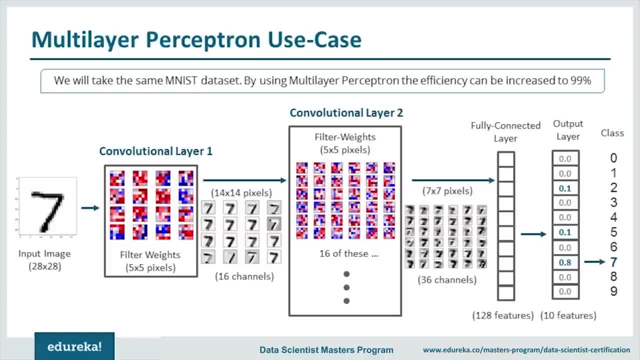 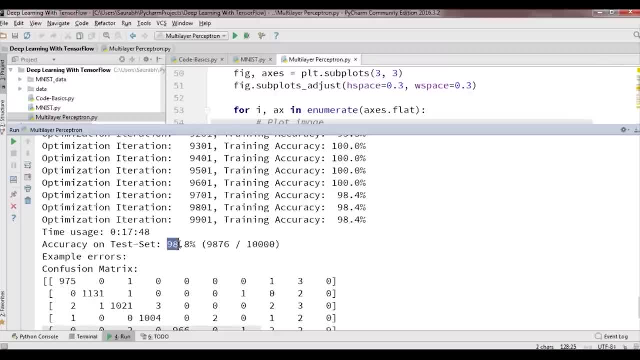 So I hope you get the point. So let me just show you that we can increase the efficiencies. So I have already done the code and it will take time if I do it right now. So this is what the efficiency we ended up with. 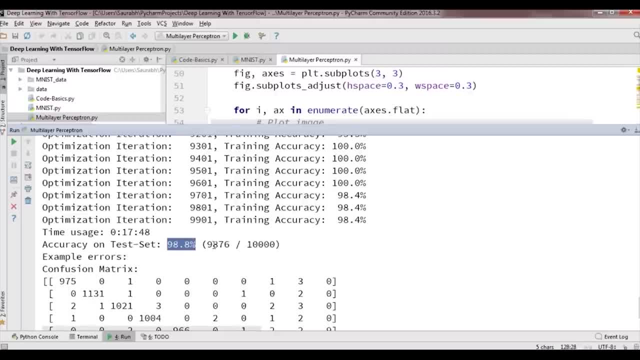 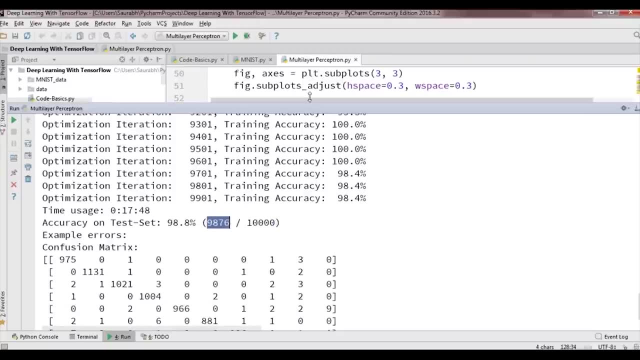 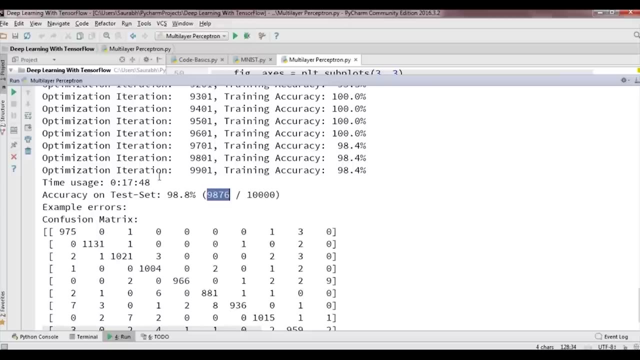 So it is 98.8 percent. So, on the test sets, we had around 10,000 test samples, Out of which we predicted 9876 correctly, So which is pretty good actually, if you see so it because in the single layer perceptron example that we took, we were getting accuracy of around 92%, but here we are getting around 99%, which is actually very good. 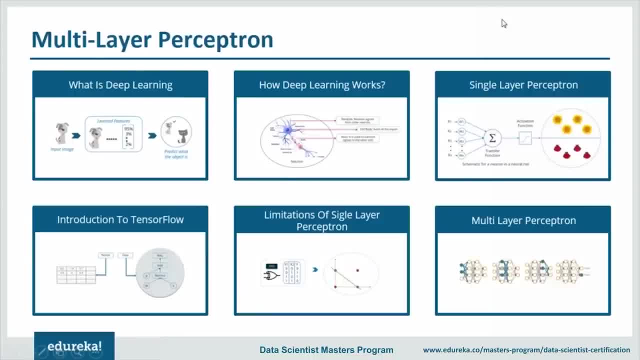 All right, So these are the topics that we have covered in today's session. We started with what exactly is deep learning? We took an analogy of classification of cats and dogs. We understood how humans identify the difference between a cat and a dog and, similarly, how we can train a machine to do that. 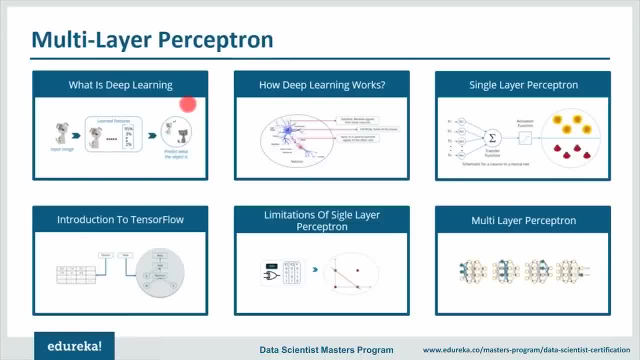 So we first looked at a machine learning model and then we focused on certain limitations of that machine learning model and then we understood that what exactly is deep learning? Then we saw how deep learning works with the motivation behind deep learning is your brain cells. So we understood how our brain cells, or neurons, work. 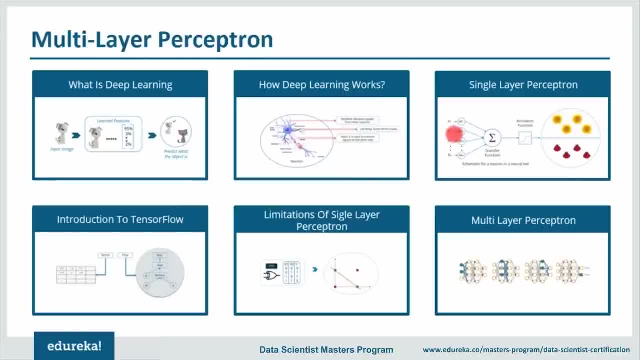 Then we focused on single layer perceptron, which are nothing but the early deep learning models, or you can say an artificial neuron, a single artificial neuron. We saw various examples of single layer perceptron as well as, for example, how to implement and gate and how to perform classification on the MNIST data set. 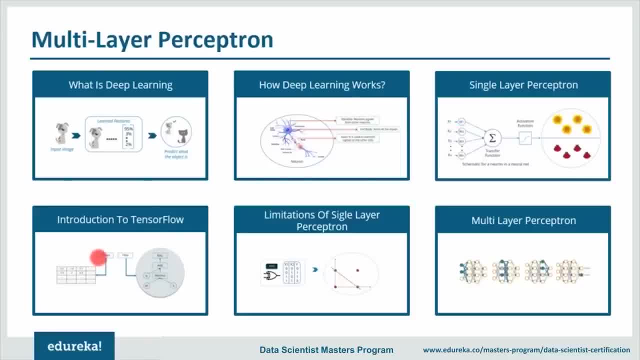 Then I introduce you to tensorflow. We understood various code basics of tensorflow. We understood what exactly are tensors as well. Then we focus on various limitations of single layer perceptron, and we took an example of exorgate in which I told you that if the data points are not linearly separable, then we cannot apply single layer perceptron. 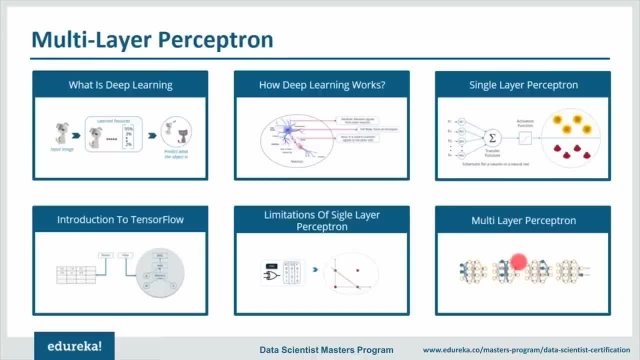 Then I introduce you to multi-layer perceptron that overcame the limitations of single layer perceptron. We understood the learning algorithm of multi-layer perceptron, that is, the back propagation algorithm. Finally, we saw a use case of the same MNIST data set, in which we increase the efficiency from 92% to 95%. 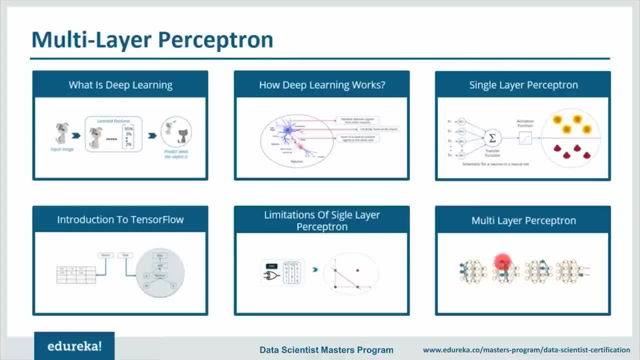 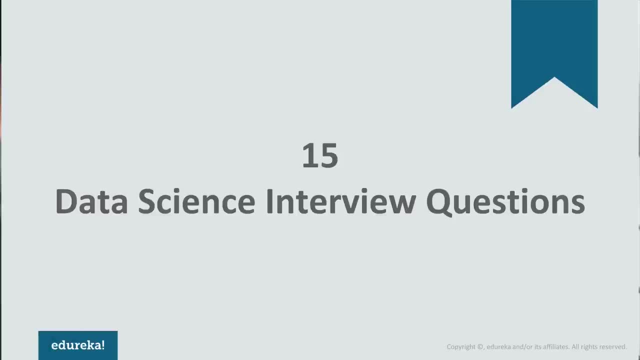 So the 92% was there in the single layer perceptron. but the same thing when we did with multi-layer convolutional networks, we got the efficiency which was around at 99%. So these are the things that we have discussed today. In this session we are going to focus on certain fundamental questions and the thought processes you need to sit for, and data science interview. 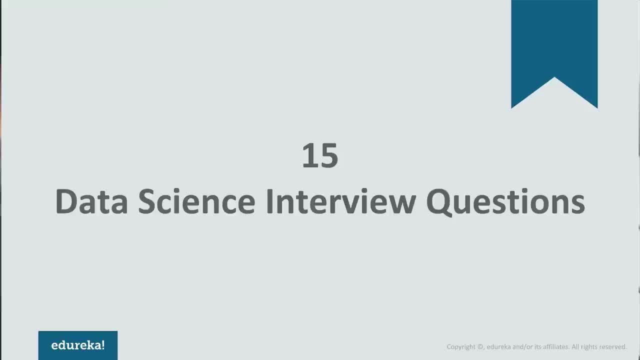 And then from there on we'll make the questions a bit More complex as we move on and we will try to answer which kind of skill sets people normally look at when you appear for a data science interview in any company. So there are like various roles. depending on that, the complexity and the variety in the questions might change. 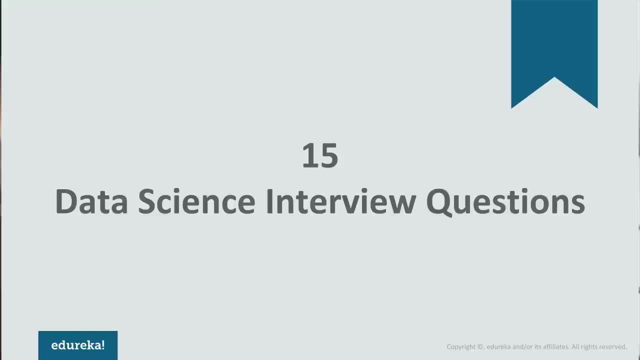 But this session will try to cover things in a fundamental level so that it prepares in a very common ground, irrespective of which role you are applying for, you might be able to at least get a perspective of what data science requires as such right? So with that note, let's see how we going to structure the various questions that's going to come up in this session today, majorly focusing on statistics, data analytics, machine learning and probability. 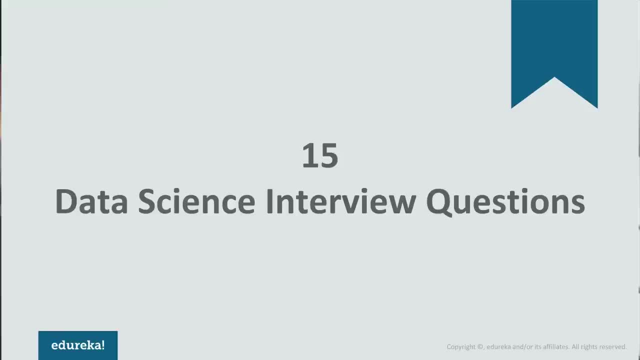 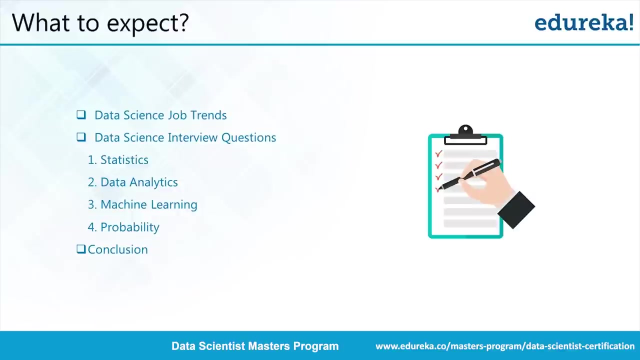 So these are the four headers under which the questions will come and I'll discuss the question and how to approach a particular question and the structured approach right in a structured manner, and once we understand the problem Well, we will see. How does that thought process of coming out with the solution really works. 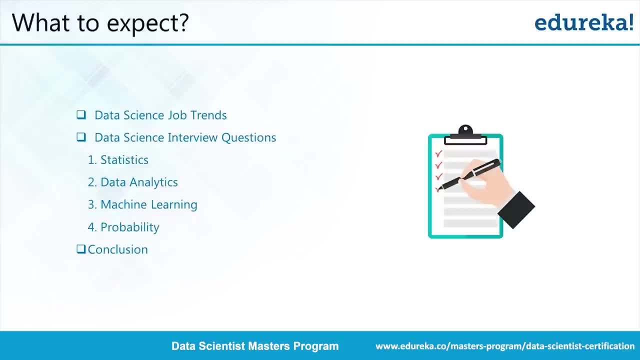 So all of you you know that data science is in booming state. many openings are coming up in across the globe in various companies, irrespective of which company it is, which particular business It deals with. there is a potential of some applications from data science. right, they have a lot of data, different systems of their business as generating the data. 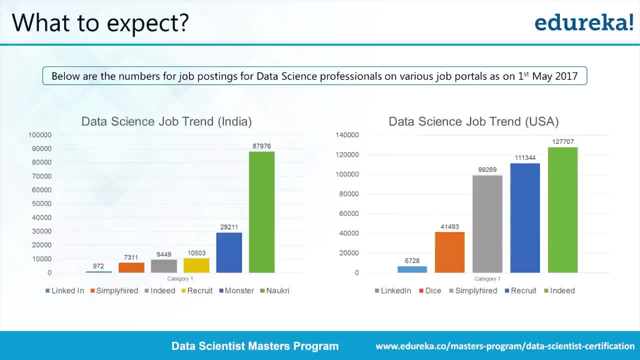 With an enormous amount of volume, velocity and variety. So with that sort of data asset that every company has now got, they want to now leverage it towards growing the business to the next level. so you have some of these stats here like this is more than sufficient motivation that getting into data science would definitely land you in some really good professional career. 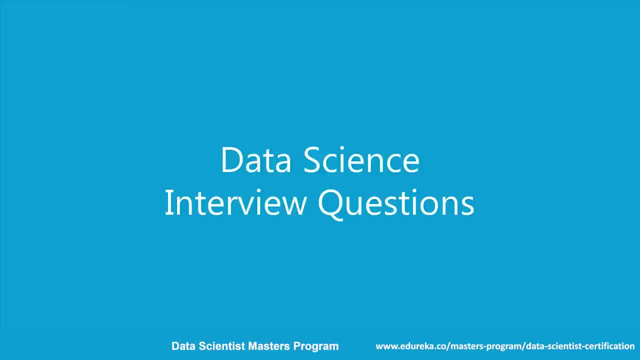 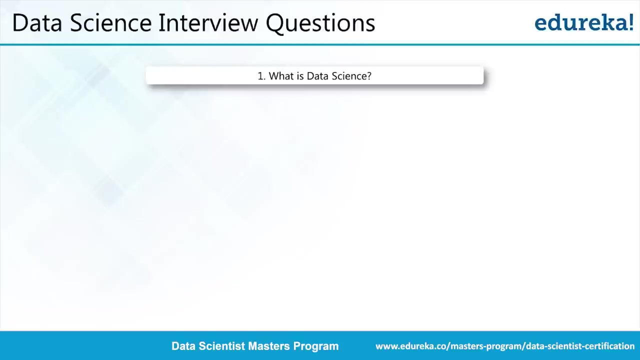 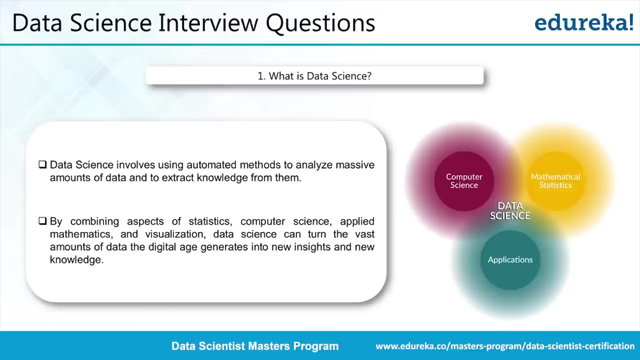 Okay, so let's start with the questions here directly. Well, in the beginning, start to focus on some of the fundamental questions, which is more for you to understand. what is data science then? like a particular interviewer asking you that question, for instance, many people wonder what data science is all about. right, though, there are many online sources and blocks. which describes data science in a very nutshell? this is what it boils down to, right? a person who is very good in understanding the computer algorithms, A person who understands the statistics and mathematical ideas and applying these two knowledges from the computer science and mathematics into a particular application, right, a business application where somebody sees a value coming out from the data. so how do you apply that? so that's how kind of data science approaches. so when you combine these two powerful concepts coming in from computer science and mathematics on a real world application, the sort of outcome that comes from particular applications, 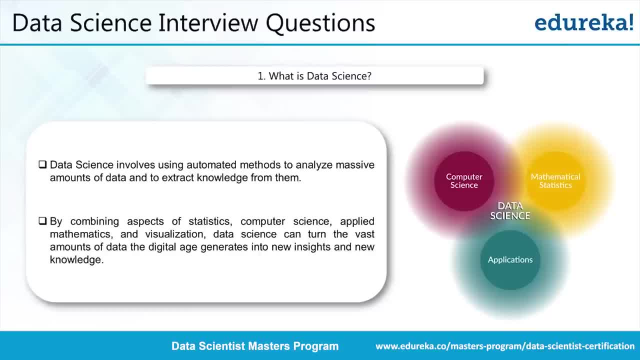 Data science project goes in a direction where people see our return on investment right. so the people you bring in, the technology, you bring in the ideas you are working on all of it should kind of give you some return on the investment you have put in. so that's where industries are started to looking at data science. so various subjects which are very important for you to know: statistics, computer science, applied mathematics, and then subjects like linear algebra, calculus and few more. 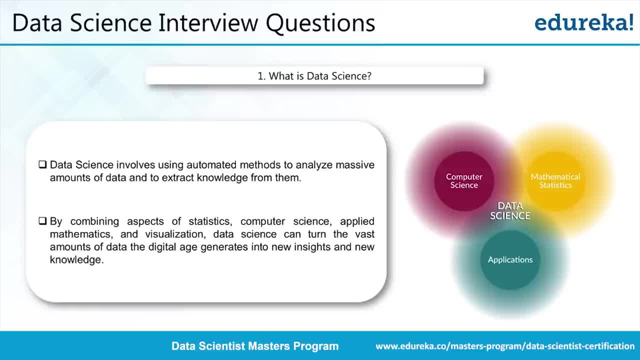 Right. so fundamentally from computer science, algorithms and data structures- why might be very useful- from the mathematics or statistics and things like calculus, linear algebra, matrix, factorization and concepts like that. and from the application. it is more from your experiences from the industry. if you have worked for retail you know how the business process in retail works right. so people often also ask: from the technology. and do we need any sort of experiences in python? 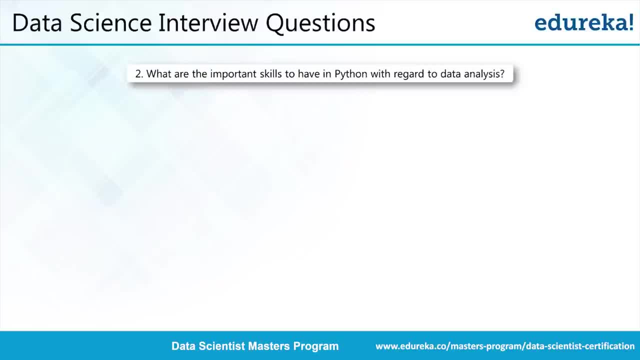 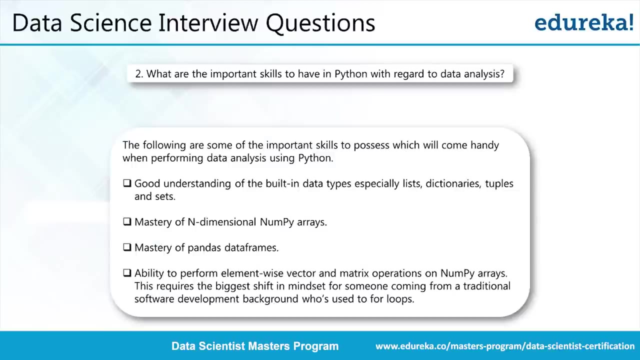 Language, right, python or like, for example, our programming as well. so python is one of the most looked out for kind of programming skills, particularly when you want to build solutions in data science domain and with availability of libraries like numpy pandas. python has now established its ground very strongly in giving a very robust framework for designing data science solutions right and, in particular, things which 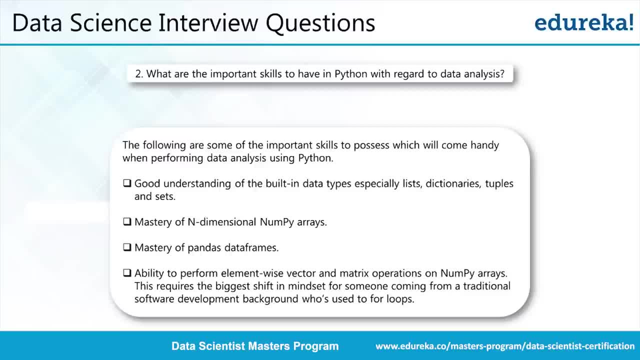 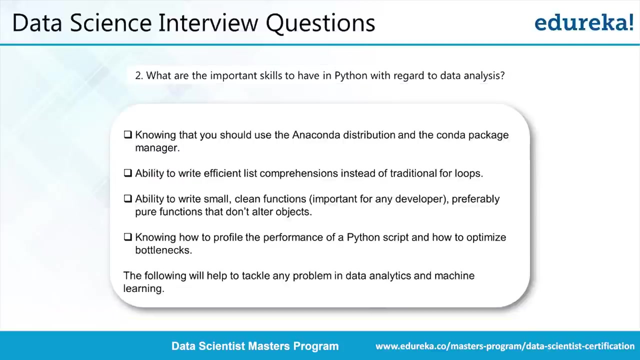 It has, like lixed dictionaries, tuples and stats are one of its own sort of one of its capabilities, which sets python in its own league of programming languages suitable for upcoming out with data science solutions. so there are many more other libraries as well, apart from this for building machine learning algorithms, but these are some common libraries that you would not really find people using it, and also with distributions like anaconda, python has shown its capabilities. 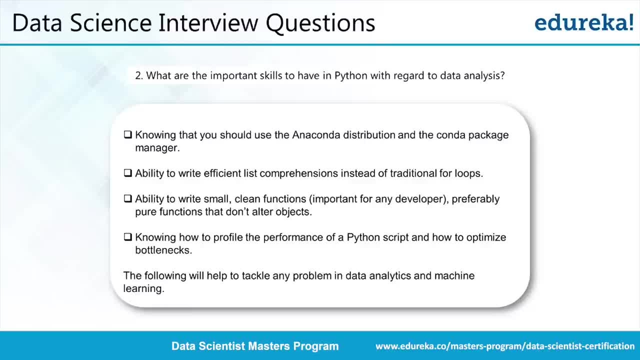 Even for a production grade solutioning right there, and you make sure that all the dependencies that one particular library has for building a data science solution is all in one place. so quite a popular programming language. in the recent kind of happenings, though, our programming is also equally good in terms of producing a quick prototype for most of your modeling tasks, but python is moving itself into a production grade where things can be deployed after the sort of prototype in terms of 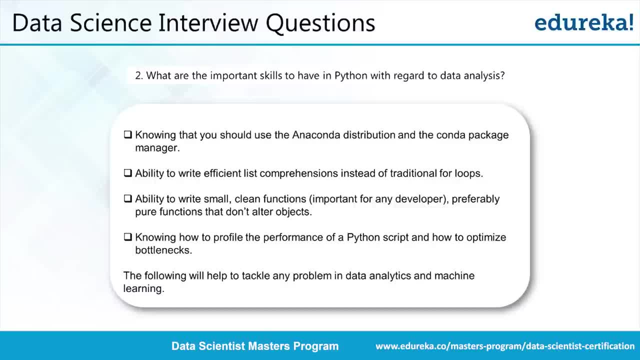 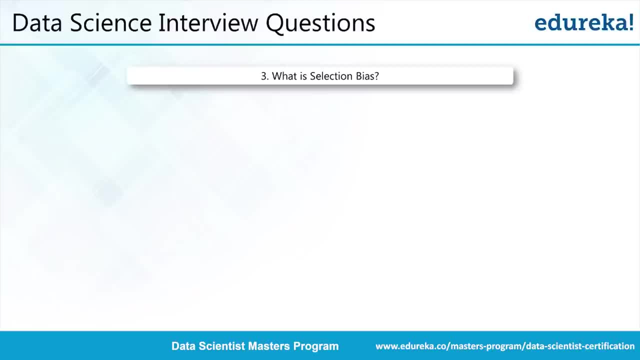 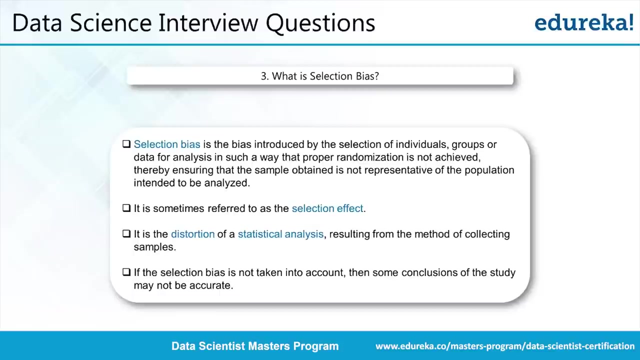 Into a production environment and it can face the customers from day one. so that sort of capabilities are coming up with python, right? so let's talk something a bit more specific with the data, right? so when people are doing any sort of data analysis, they normally face something that we know by the name selection bias, right? so what is actually a selection bias? the fundamental place where you start doing a data analysis is by selecting a representative sample. 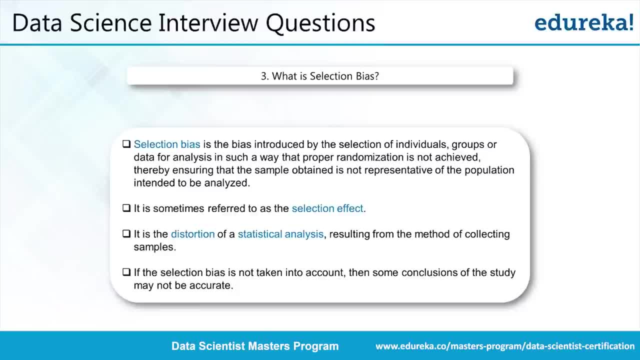 Right. so that's where we like normally start doing any analysis. so when you like, working for a company which has, let's say, 1 billion records in their databases, like 1 billion is like very, very large number which represents various customer customers data, or it might also be, depending on which feature you are working on, and so on. so if you collect all of those, it might very easily come to 1 billion records, which is nothing but in a structured form, number of rows. so with that, an enormous amount of volume in the data. any analysis. 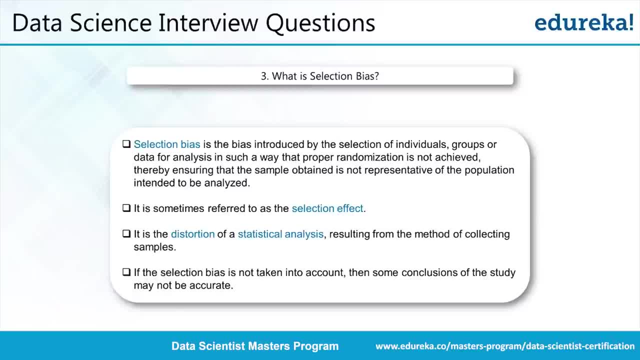 This is that you take up, might have to have a lot of filters, like saying I only want to analyze a particular feature in my products, let's say right, and I won't only want my customers from XYZ region, which is, let's say, top 4 region or top 5 regions. so you might like put many features or filters like this, but later on, if you would like to do a kind of an analysis which covers most of your customer base, right there comes the tricky situation of not being able to use the entire volume of the data. 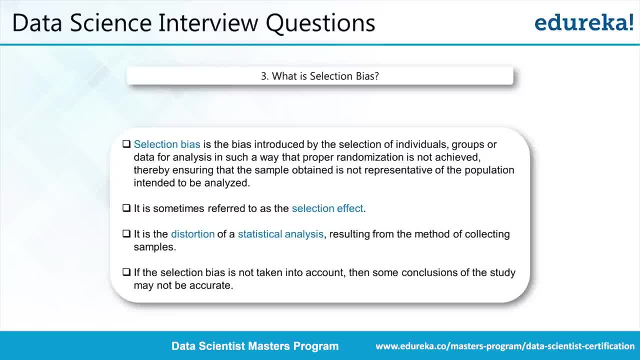 Of 1 billion records. at the same time, you want to do a really good study or analysis based on what data you have. so in statistics we normally use this idea of doing a kind of a randomized selection, right? so with this randomized selection, we make sure that out of these 1 billion records, we are choosing a small subset, let's say of 1 million, which is a true representation of the entire population, right? but what happens with this is, while we do this 1 million record selection in a randomized way, 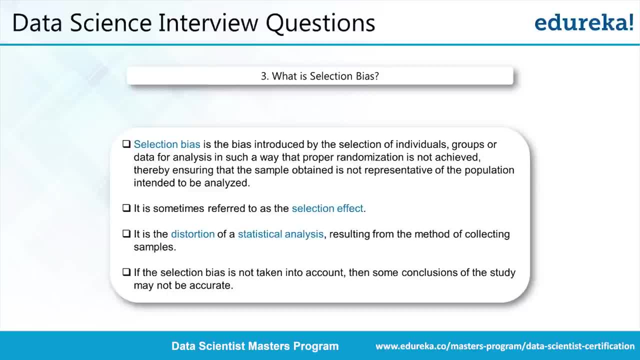 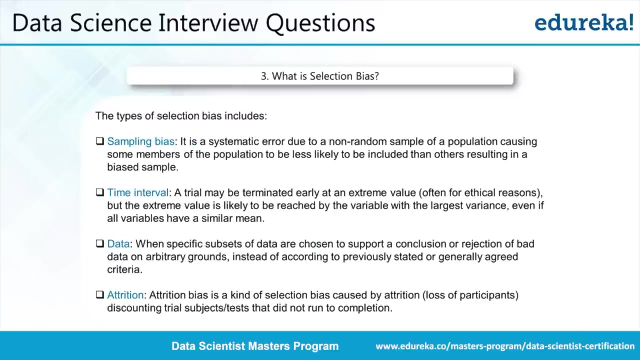 There are chances that you might have certain bias in the analysis, obviously because you are not using the entire population. so selection bias is this particular sort of a characteristics while you are doing a sampling on a large population of data. very common example for this is if you want to do a exit poll analysis of particular election, even before the election results are coming up, and you have not chosen a representative sample for doing that exit poll analysis. right by that you- I mean you- only have 1 billion records. 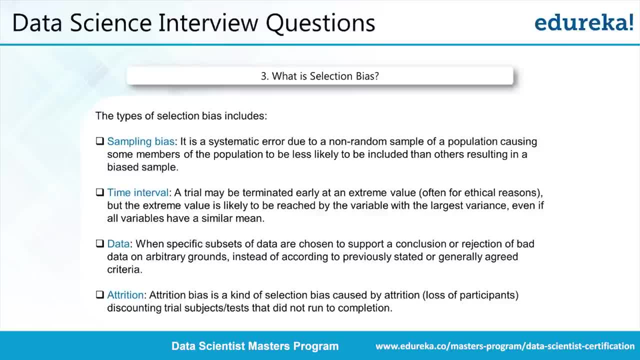 Of 1 billion records. I mean you only have 1 billion records. Asked some questions for a selective view from the particular constituency and they have an opinion towards 1 candidate, but that doesn't represent the entire opinion of the population in that constituency. so selection bias is, like very important to handle and most of the time people employ things like randomized selection or selection sampling techniques like stratified sampling and so on. so by that you can minimize this selection bias. so these are some very general questions, so let's start with some. 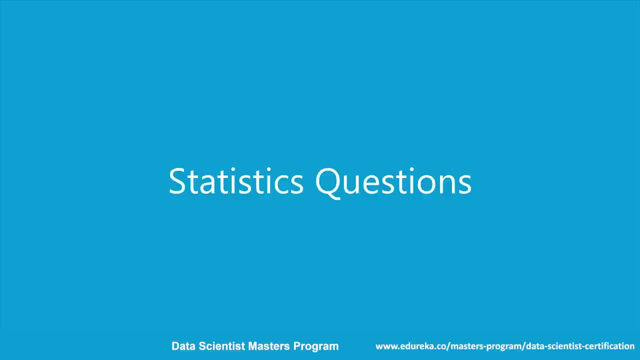 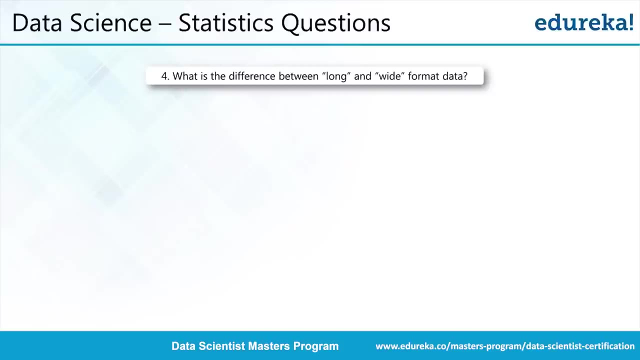 sort of statistical questions and also how to deal with different types of data. okay, so doing any sort of data with a structured information. so structured information I mean there are many rows and like many columns and it looks more like a tabular data, right? so with such a data in in place, there are like these: 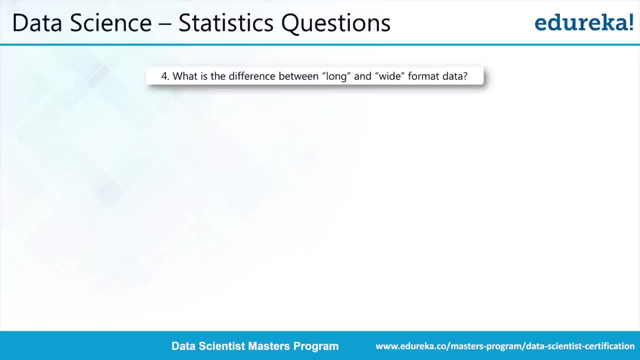 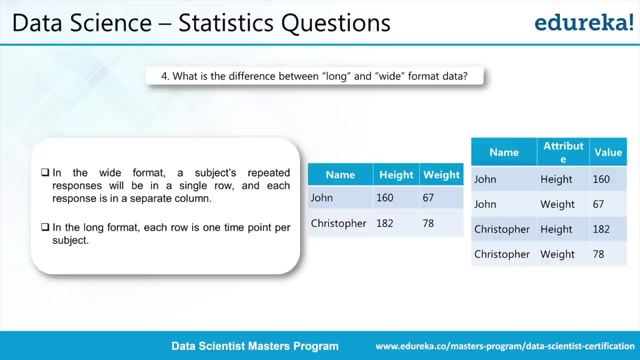 two different formats, one saying the long and the wide. so let me like show you an example here. you have a record of two customers, right, and you store just two values, which is the height and the weight. so these are like in columns. so with the these two customers, these height and weight being a separate. 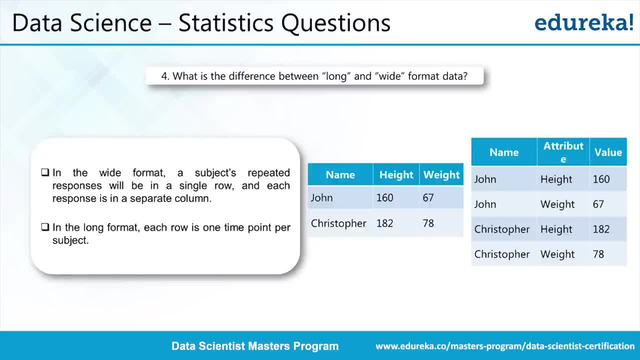 column is one format like a long format. let's say, transform this by having only one particular column which will say attribute, right by that I will bring in these two columns as one column by calling that as an attribute, and put the values in one column. so this sort of format is called the long one. so what really happens is: 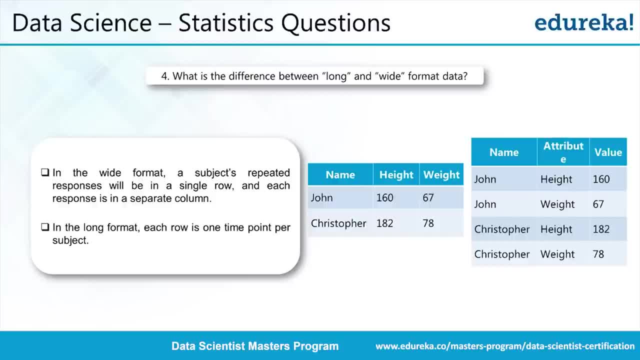 instead of having two separate columns for two of your attributes, you put, or both of those into one column, and by doing that there are a lot of benefits with respect to the task you have in your hand, particularly in data visualization. certain data visualizations would need you to not put. 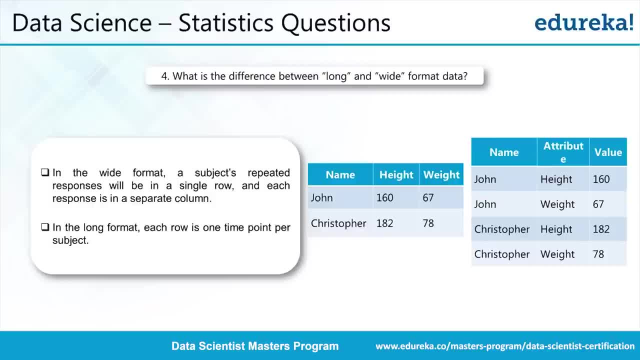 your attributes as a separate column but rather as the one column which can have the attribute names, so which might then go into building your legends right. so these kind of techniques are kind of very common formats between like the long and divide, and very frequently will people like deal with both these data formats, depending on what tasks they are doing. 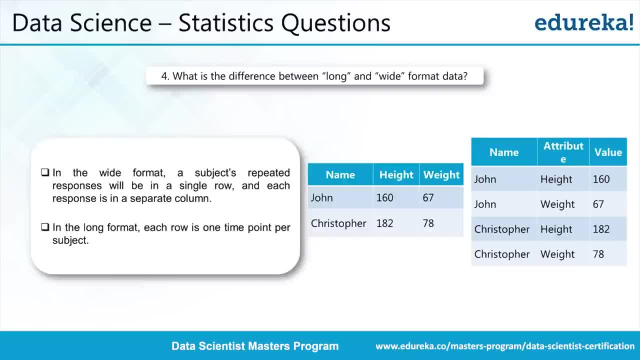 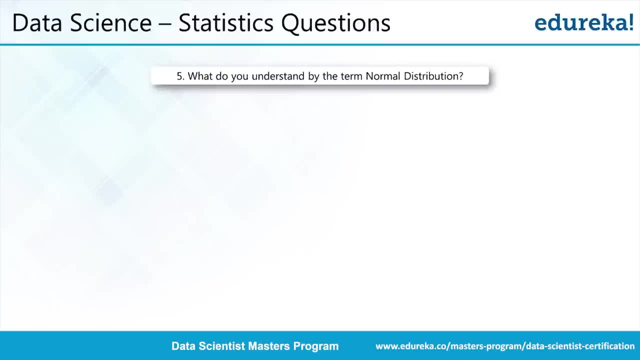 particularly when we are building the visualization dashboards. okay, talking a bit more on the data analysis perspective, people like know that in stats normal distribution kind of is that one like the data is a lot farther of the distributions. you have many distributions which normally people try to see if is present in my data or not. but the moment people 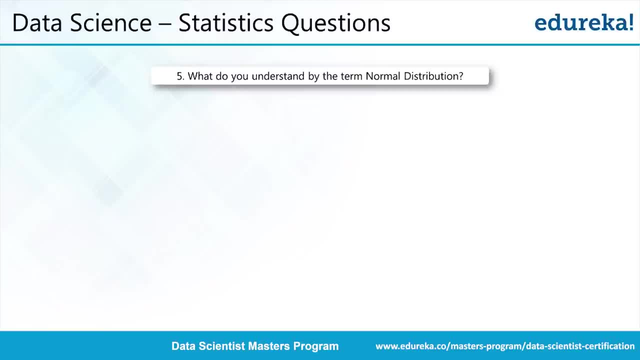 kind of see normal distribution coming up in any data. things are kind of bit easy to understand and, in typical case, any distribution, any data distribution that you would like to find out, given data for analysis, it gives us a lot of characteristics around what the data is about, if I'm, let's say, analyzing. 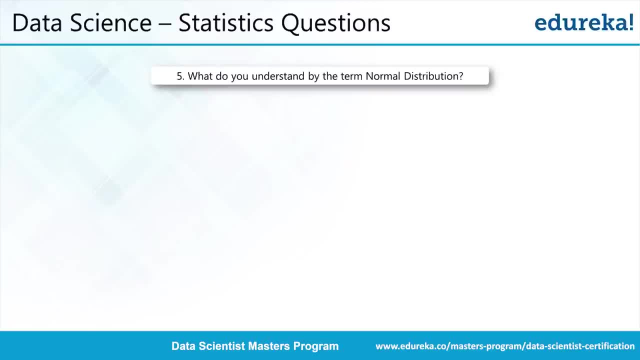 data and I'm not just having a good idea like this particular one, if I've got, like, the data in the database, like I've got the data in the table, which is a lot of information, and I'm going to have to look at all of the data in this document. 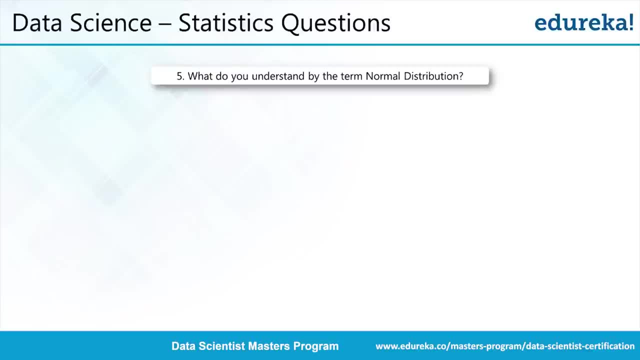 which is being used, but at the same time, I was looking at the data of my organization, which is being used by my organization, right? so it's very common for people to view data in a certain manner, right, and so data can be becoming more and more common. looking at that data, the data can start to appear. 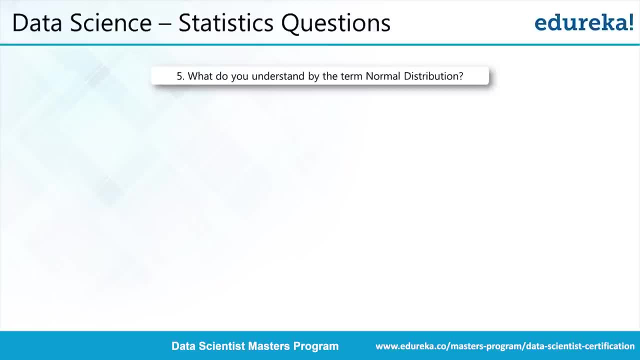 and the middle one, which you like, are sort of the normal performance. so this sort of bell curve distribution is very commonly understood and as well as used in doing many data analysis. so is the other distributions as well. but normal distribution has its own significance. so when somebody asks you around anything, 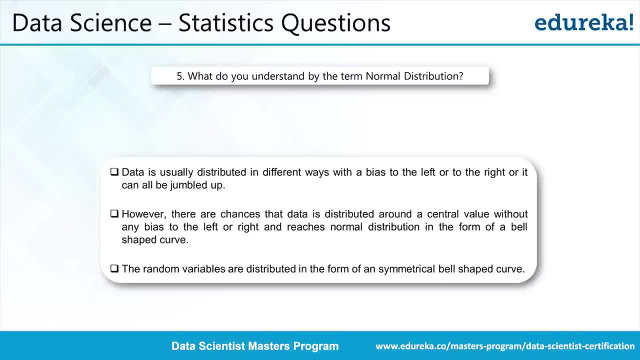 around, not normal distribution. the first thing you should visualize is the symmetrical bell-shaped curve right, and the moment you get that bell-shaped curve in your imagination, start thinking of certain properties like: what is the mean of a normal distribution? what is the standard deviation of a normal? 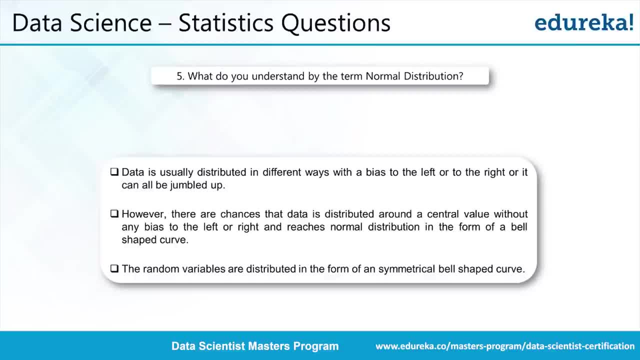 distribution and in particular a special case of normal distribution which we call the standard normal distribution. so in that standard normal distribution we know the mean is exactly zero all the time and the standard deviation is exactly one right. so there are different places where normal distributions are kind of used and if you are comfortable with ideas like central, 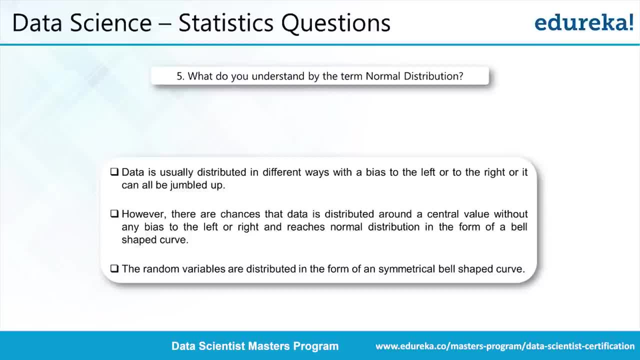 limits theorem or the law of large numbers. you might want to relate that as well to normal distribution, particularly the central limit theorem. right, but the idea is a distribution which is symmetrical around the mean. so that's what a normal distribution is. so, depending on which variable you are trying to analyze, even 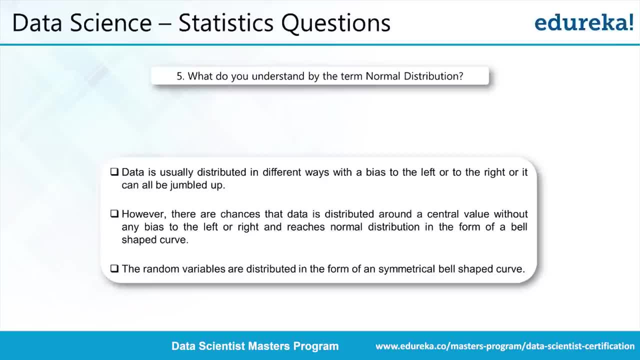 a given data set, whether it could be like an employee's salary or your sales in a for a business of yours right, or your number of, let's say, interactions of the customers on your product. so any variable that you define can have a symmetrical bell-shaped distribution, which we normally refer by normal. 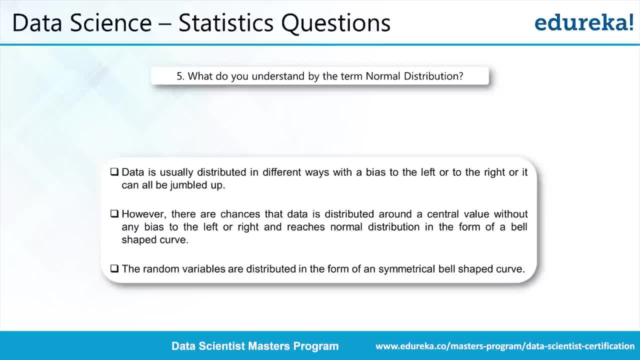 distribution and the moment we understand that something follows a normal distribution, all these properties of that distribution is like revealed. so that's sort of the importance of doing any analysis around the distribution of data and normal distribution like very common one and in many statistical techniques, in even model-building exercises, if you. 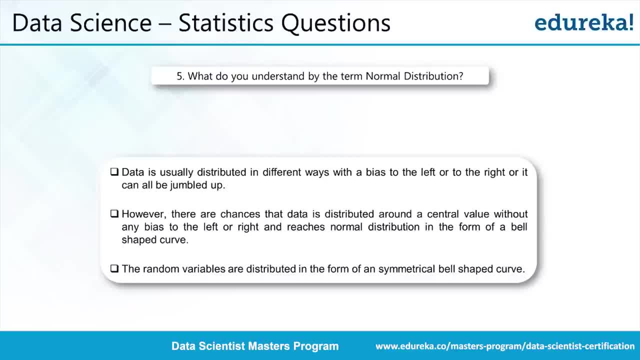 have anything in a normal distribution. many other possibilities of applying certain modeling techniques comes out evidently there, and also there are many other modeling techniques in stats and machine learning where there is an fundamental assumption that things should follow a normal distribution. if it is not following, then the model is wrong. there are many use cases of for 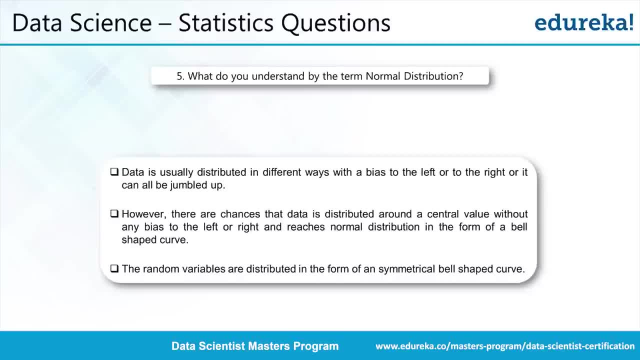 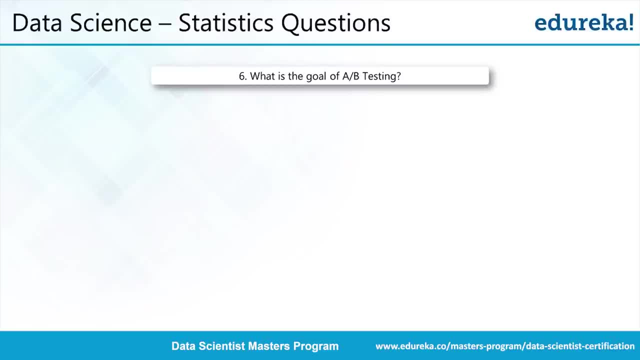 knowing what normal distribution is. but in simple terms, it's a symmetrical bell-shaped curve right A-B test testing. so quite a popular approach- people particularly who are working with product right- and what happens is when you are, as a company, having lot many features inside a product. for instance, if LinkedIn is a company which has a 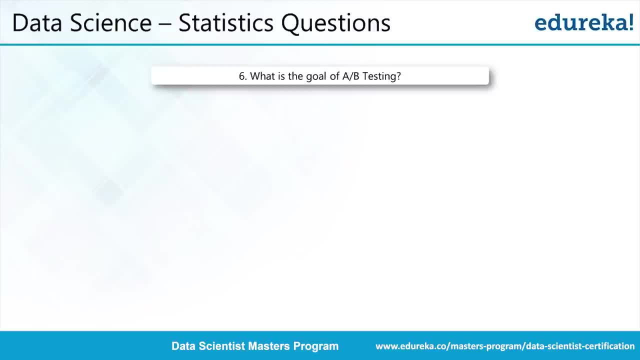 web page right. it has a lot of features inside that. you have some jobs portal. in LinkedIn you have places where you can connect to your professionals in the similar industry. you can also read about the post people are doing. you can also read about the post people are doing. 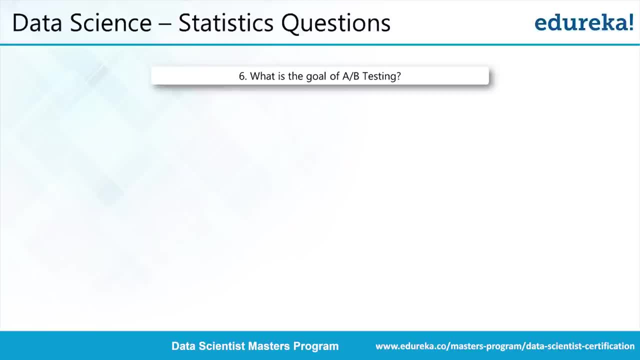 in the portal and so on. so there are different places in the website with many features. so what happens is if LinkedIn as a company is looking for some changes, for instance, changing the entire websites, design in aesthetics, design and aesthetics, or changing one particular feature inside their website, right so? 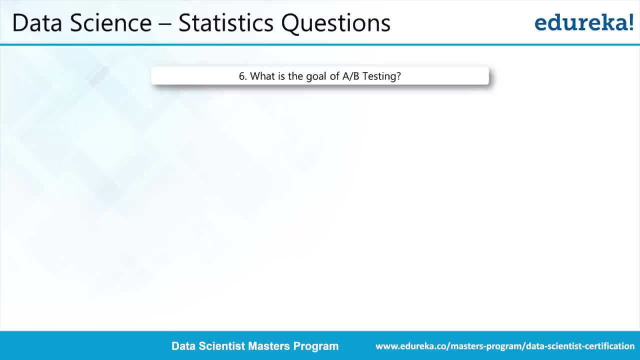 these changes are normally accompanied by sort of a process called A-B testing. so what happens? as an analyst, you might be working with LinkedIn and say, on a fine day, they might come out with a new feature, new design or new sort of changes in their website. so you as a person would tell: okay, this is my. 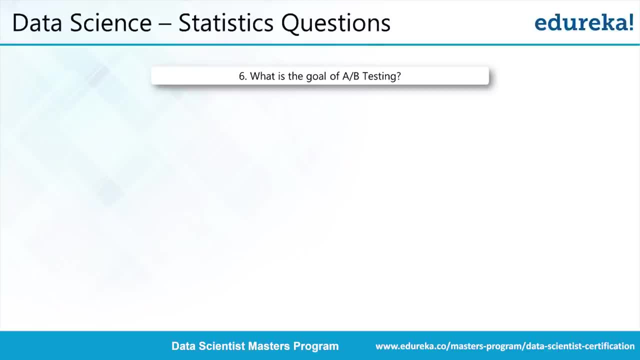 framework for testing this new change by defining a metric. so my metric would be, in simple terms, saying: if I change this website from A to B, is my number of footprints on the website going to go down or not? so this is my metric and if I successfully established the fact that, after rolling out this new website, my 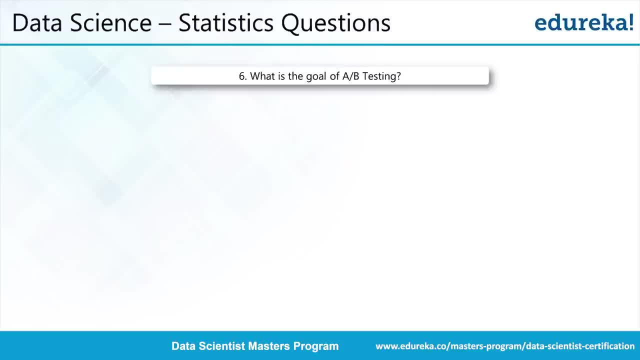 number of customers who are going to visit my website is not going to go down. I can be confident that. okay, find this works. now roll out this new feature. so in this framework, we normally have two set of users to identify the particular risk associated with getting this new feature into the platform and in which we, in a randomized way, put one. 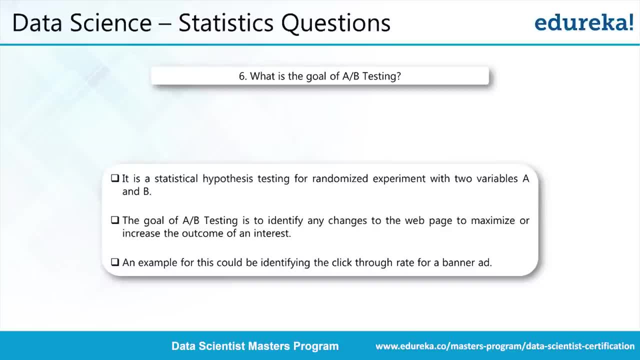 user group and expose them to an older website, and another user group and expose them to the newer new features, right or the new website. and when we compare the results of a particular metric, like the number of clicks or the number of purchases and so on, we should be able to see that these two groups are. 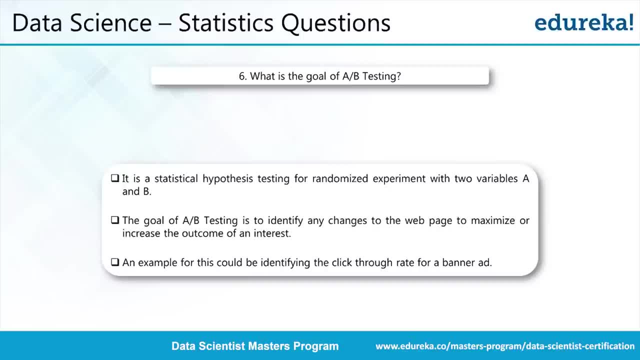 either exactly the same or quite different. and if it is on the negative side of the difference, we say the feature is not good. and even if, when the difference is not at all there, we say: even if we bring this new feature, nothing is going to happen. so this AB testing framework is quite robust in its 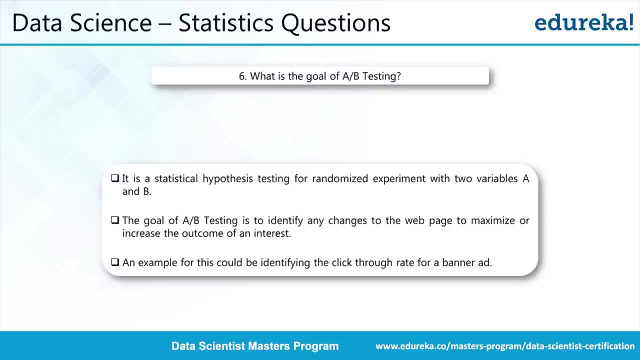 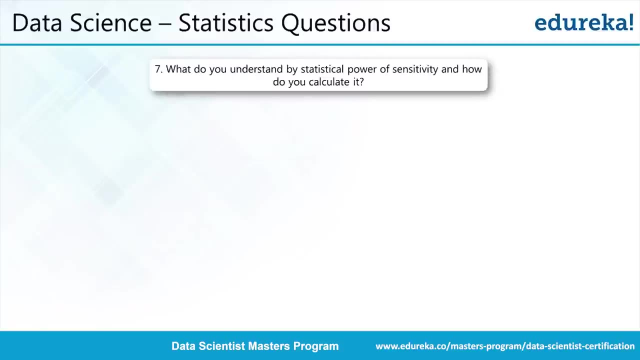 own way right? and a very common question now: if you have like a worked as data analyst or if you are expecting to be like sitting for this data analyst kind of a role, knowing AB testing framework is very important, okay. so sometimes also when you do these kind of AB testing sort of analysis, people normally come 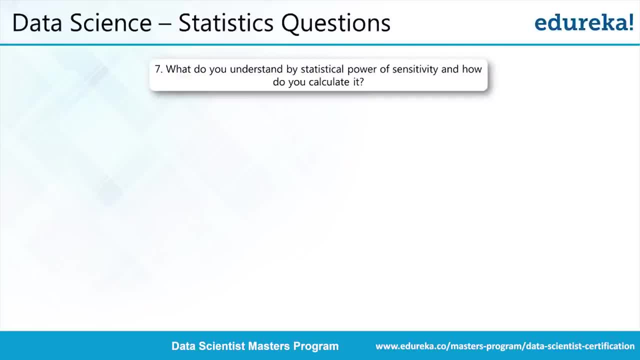 out with sort of saying what should be the sample size of my users whom I should be getting to participate in my AB testing framework? or also, when you are building some models, you might see that there are certain statistical measures which has to be evaluated by the end of model building. 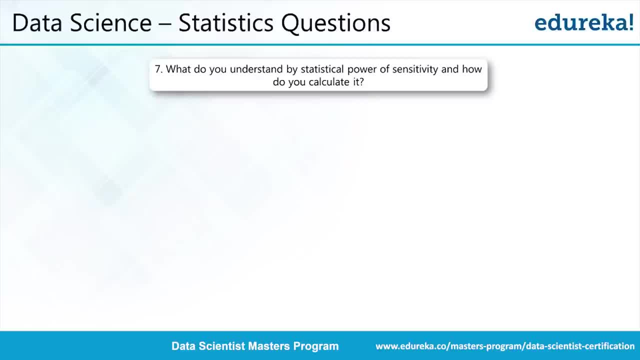 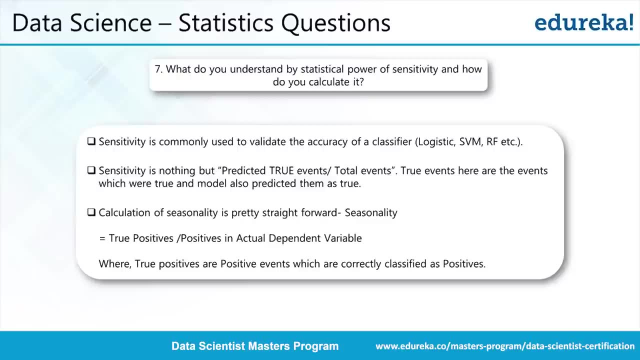 exercise, like if you are building a machine learning model, let's say, and you want to see if the those metrics on which I am evaluating are really good or not right. so in that sensitivity is one of those methods, or like metrics, which we normally evaluate, and I am going to show you some, something that we normally refer by the name of an example where you have a few models that I am evaluating, a number of models, and then you will hear the name of the model that I am evaluating and then you will hear the name of an example on, and then you will hear the name of the. 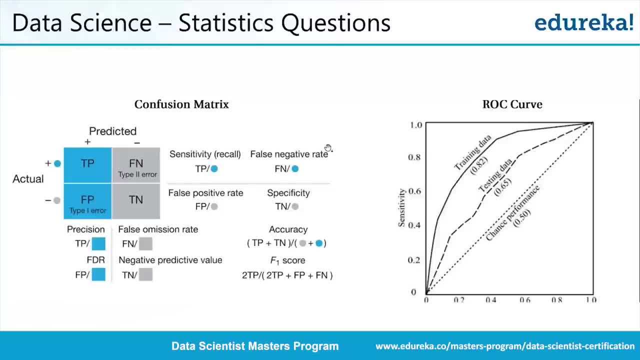 confusion matrix. so I will spend some time explaining this and then come to what we mean by, like, sensitivity. so let's say you are building a model, right? a model for predicting whether a particular customer is going to purchase from my platform within one month or not. right, so very. 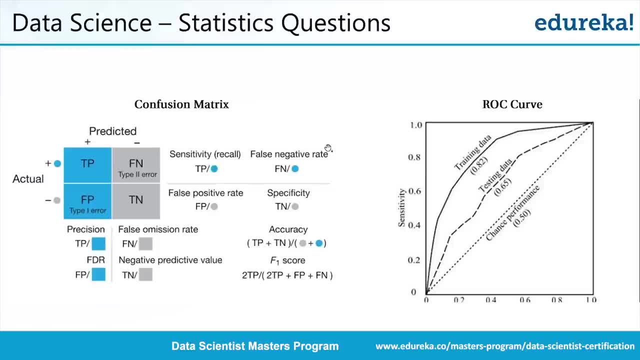 simple problem statement, which might include many variables that we would bring in, and then finally build this model saying: okay, this is my final model which says with 90 accuracy whether my customer is going to buy from my platform- let's say, an online e-commerce platform- within next. 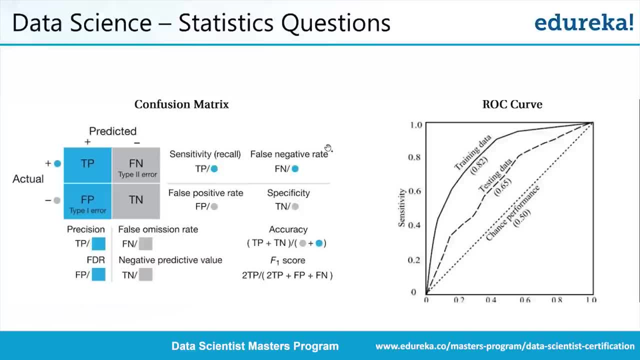 month or not. so this is my model. so now, as you, without going into the details of the model, let's assume that after you build the model, you have got the results. so while we analyze and evaluate what the result is all about, we might come out with a confusion matrix. so what it says. so obviously, when 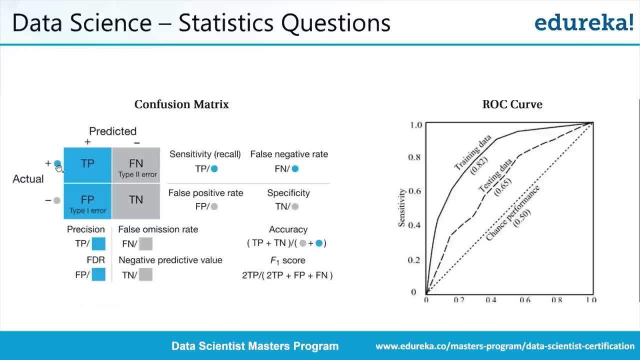 you are building a model which follows a supervised way of learning. you will see from the historical data after people have purchased in the platform within next one month, whether they are buying or not. so I can obviously create a really good training data set right which will contain the information after. 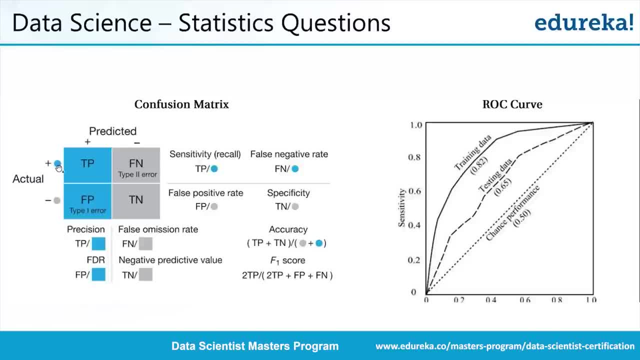 people, let's do the first transaction with me in next one month, whether they are buying the next product or not. so with that data set, I train my model and the way of confusion matrix puts that is by saying: my actual data says something and you have predicted something right. so let's kind of 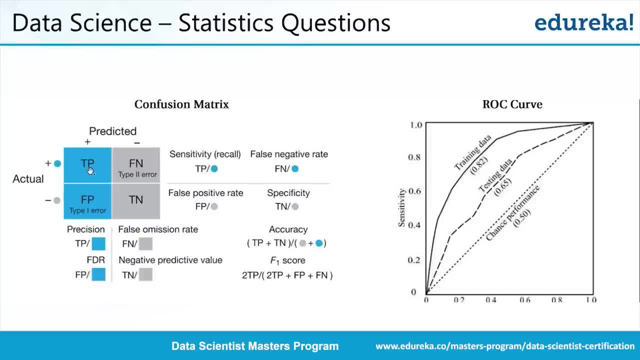 get into the details of that. so this particular box which says my actual data, says the customer will buy and you are also predicting the same. so this we call the true positive. the prediction is actually true right in a positive direction, saying the purchase happened now, like move there or diagonally opposite to this TP, which is this: 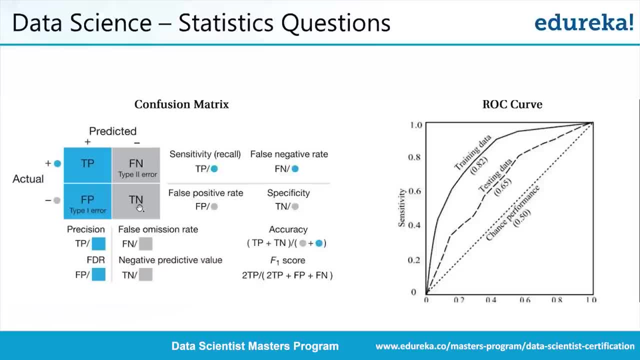 TN, which is true, negative, which means the prediction of your model saying the customer will not buy, is actually matching with the actual data as well. well, right. so both of these values, the true positive and the true negatives for the two cases, is the right predictions from your model. but consider the off. 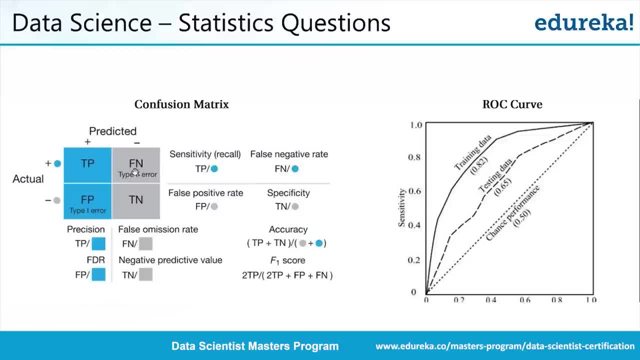 diagonal elements, the false negative and the false positive, and these two cases. this is sort of an error, why? because your actual data says the customer is not going to buy. in this case, let's say, but your prediction says he is going to buy, so the prediction is actually positive, whereas the actual data is on. 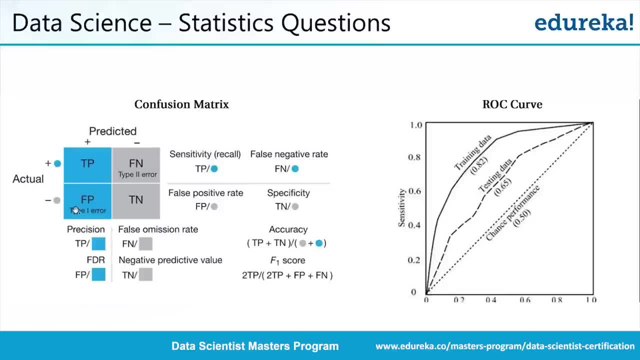 the negative side. so this is a false prediction, right? so you have your, in this case, your FP, which is the false positive cases, and on the off diagonal element, if you look at this one, which is FN, which is your false negative, for the cases where you are predicting the customer is not going to buy, but in the 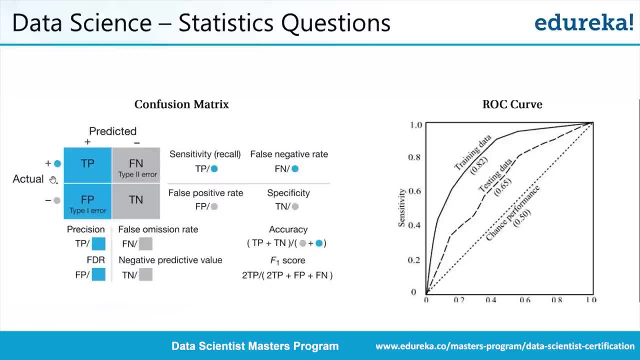 actual data. it says that customer actually has brought the product. so in this case the model is wrong. so the type 1 and type 2 errors needs to be taken care of when you are building any machine learning model. if these errors are low then your model is going to move towards that hundred percent accuracy. 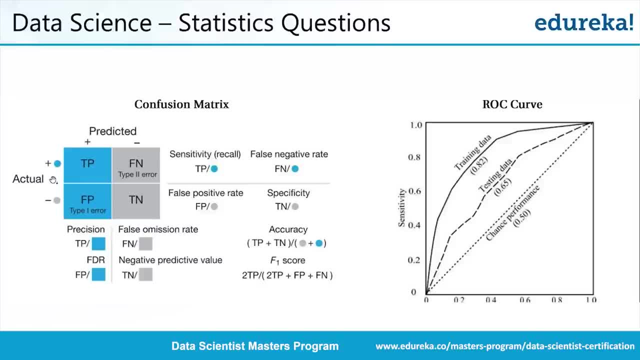 mark. but normally any machine learning model has its own limitations. so particularly there is one metric which we refer by calling sensitivity. so what happens is these true positives and true negatives needs to be controlled, right, if my model is very good in true positive ones, like the positive cases of 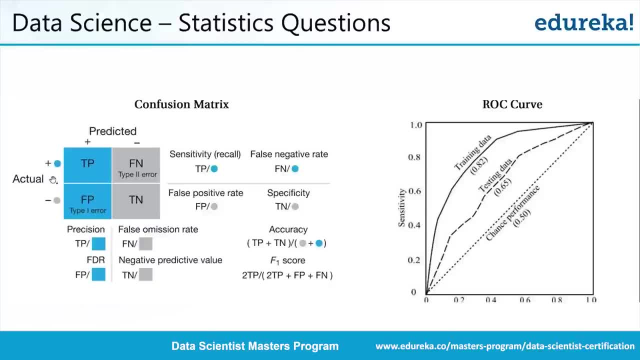 when the customer is buying, but it is doing very bad job when the customer is not buying. so cases in which the customer is not buying, then the model has some sort of issues. right, it is doing only good in one place but doing very bad on the other case. so I need to find out that by some metric. so sensitivity help us to. 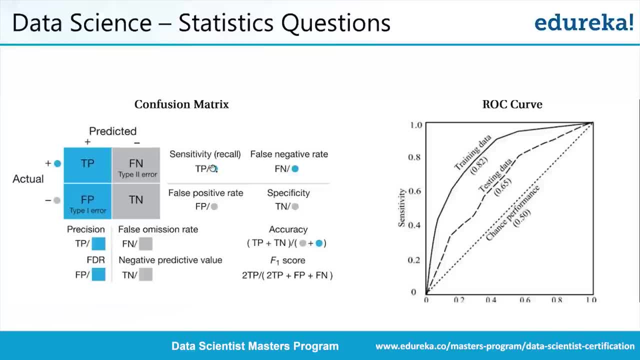 find that out, which is in simple terms, is a ratio between the true positive in the denominator. we have all the cases of positive predictions. so imagine now if the type 1 error is going to grow, my sensitivity is going to come down. so if my true positives are like very high, the 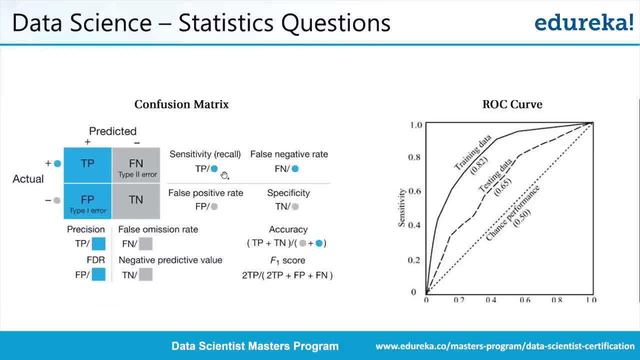 sensitivity will also be high. so this is sort of what we call the statistical power. if this sensitivity is really good, I would say that my positive cases are predicted well, and the exact opposite of this sensitivity is what we know by specificity. so we need to make sure that in a very good machine modeling model. 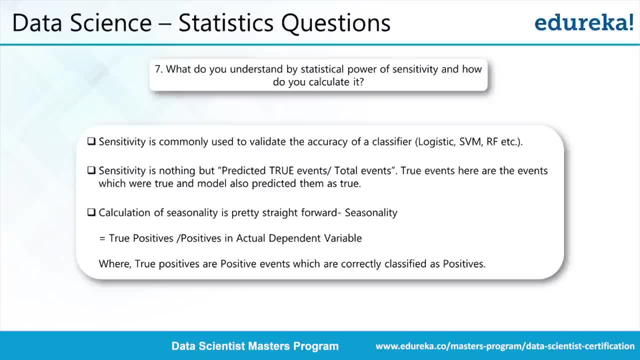 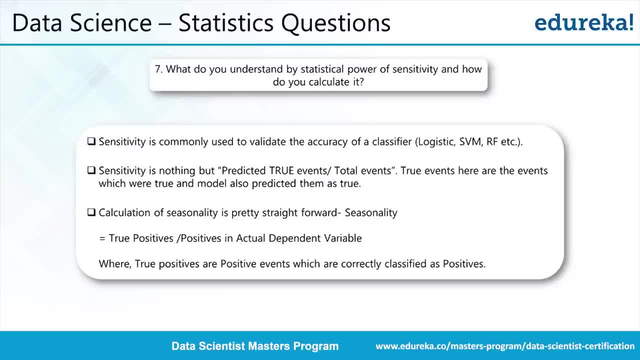 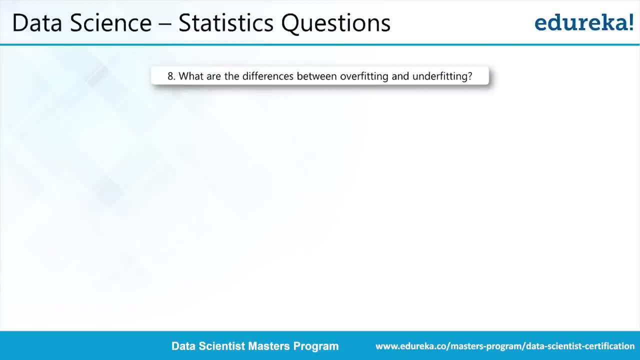 total positive events there and, as I mentioned, both of these- sensitivity and specificity- play in good role when you want to evaluate a model's output. right and one more common problem. so these questions might be immediately following one another when people ask you about sensitivity and specificity, as you know, 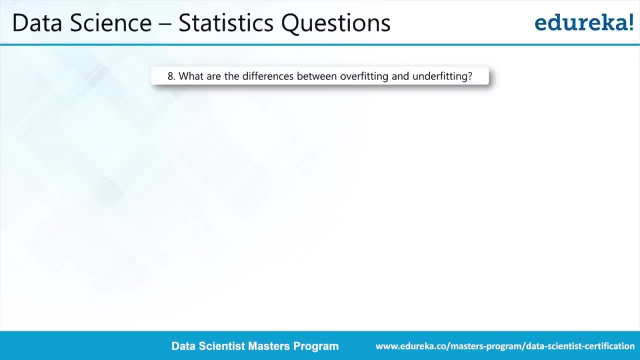 it's about the machine learning models output right. when the model is done, you understand whether the model is good or not. so in those cases we also come across some kind of issues like overfitting and underfitting, given machine learning model right. so these words are very common and the idea is depending on the complexity of 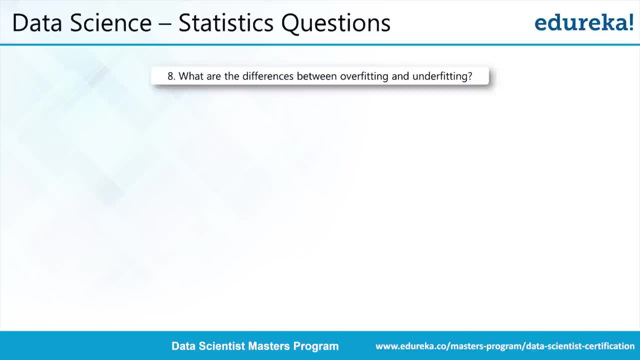 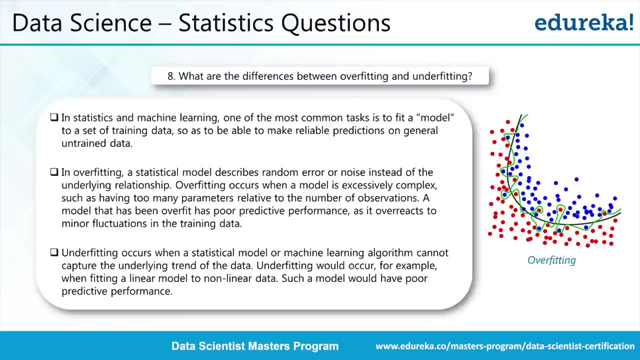 your model, you might see that you want to adapt very sort of exactly to your data points, or you might want to do a generalization. so for instance here, if I have these red and blue dots here, right, and if I draw a curve like this which separates the red from the blue, and when this separation 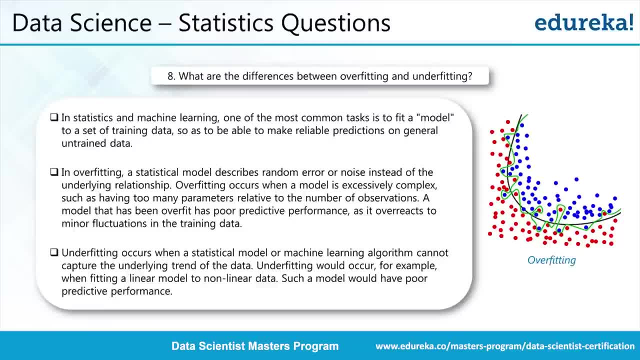 happens. I am building, actually, a classifier using some sort of modeling technique. but now imagine, by drawing a smooth curve like the one which is given in black, you might be over generalizing it right, by which I mean there might be some red dots on the other side of this boundary. you can obviously see that. 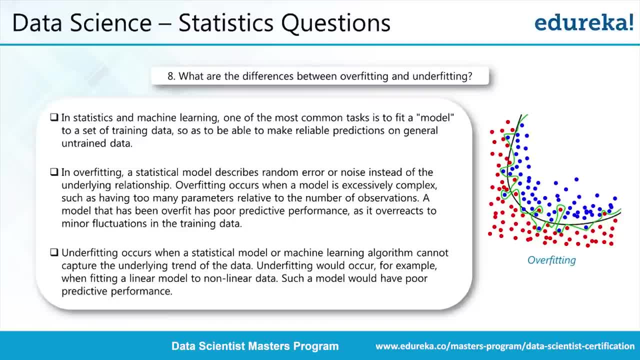 but the moment I am kind of a bit more flexible by drawing this green boundary which actually covers all that issue, To see if I can leave that as a problem, like by going from one side to the other issues which is coming out with these red dots on the other side of the boundary. so this green 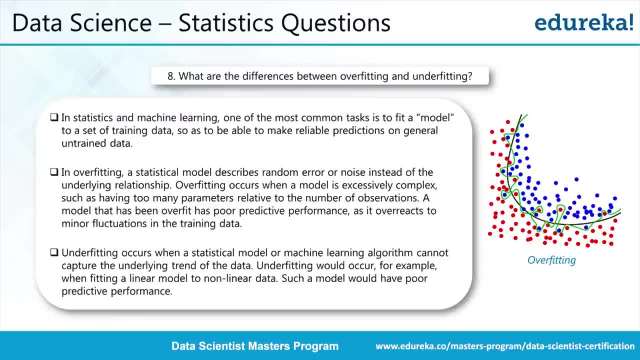 boundary has like taken care of that. but the problem, when we are building any model right, the idea is you need to generalize to the pattern found in the data. so if you don't do that generalization, well, you are underfitting. but if you do that generalization like too specific. 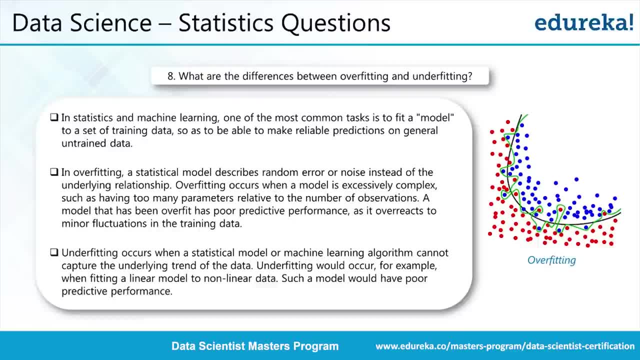 you are overfitting. so this curve might be represented by some polynomial right. but that zigzag kind of a polynomial might be bit more complex than a smooth curve like the one which is shown in the black. so you need to be very careful when you are building a model, particularly 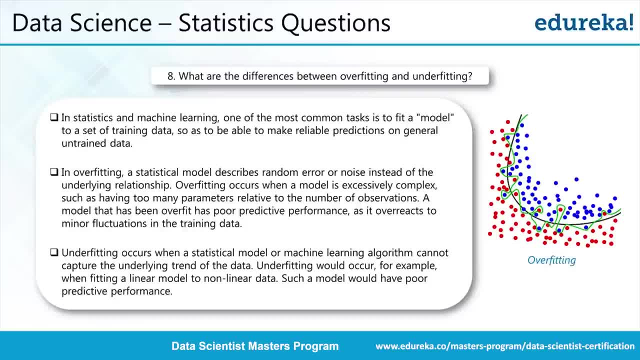 in the cases of regression models, where it is represented by a line and a polynomial, you need to make sure that the polynomial is not so complex, at the same time not so simple. then you will either end up in an overfitting situation versus an underfitting situation. so 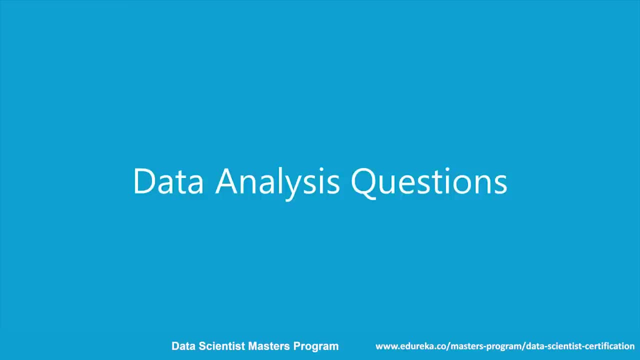 we need to have a good balance between these two, right? so, in summary, when kind of statistical questions comes in, it would mostly covering things like some basic statistical properties as you would be like, very aware of, like things like standard deviation averages, how to interpret median, how to interpret quartiles, right, the 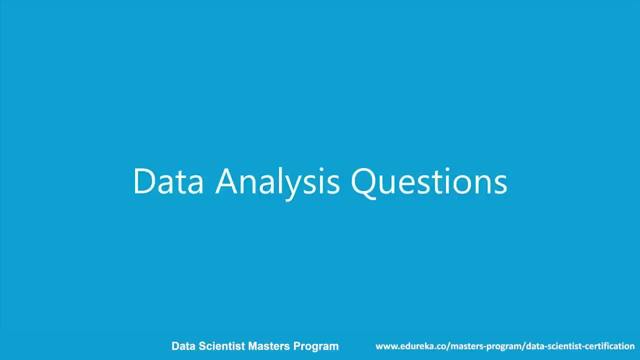 first quartile, second quartile and so on. and what do you mean by percentiles? right, these are some basic questions. a bit more complex in nature might be discussions around sense, sensitivity, overfitting, underfitting. these are like statistical ideas. so you want to prepare, maybe from a basics level, using the properties like standard deviation, mean and 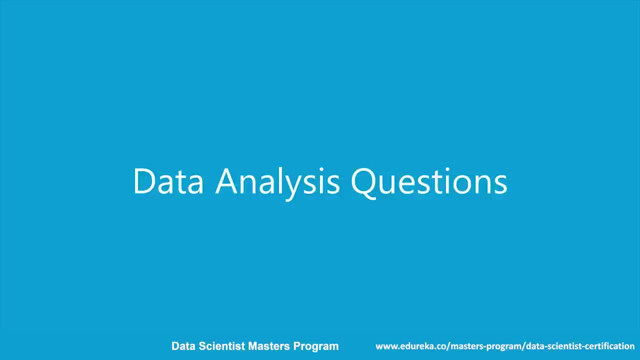 so on till things like overfitting, underfitting, statistical desensitivity and specificity kind of ideas. so that will like make your ground a bit more stronger when you are going for the interviews. and these are at least the bare minimum for you to understand in the statistical concepts, right, even anything you want to understand about the interview. 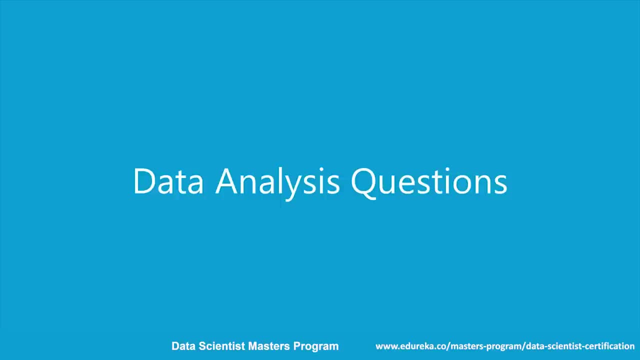 anything less than that, you might like face some difficulties in the interview. ok, but let's also talk about now questions which are related a bit more on data analysis. so let's see how, what kind of data analysis questions which might pop up in the interview, ok, so 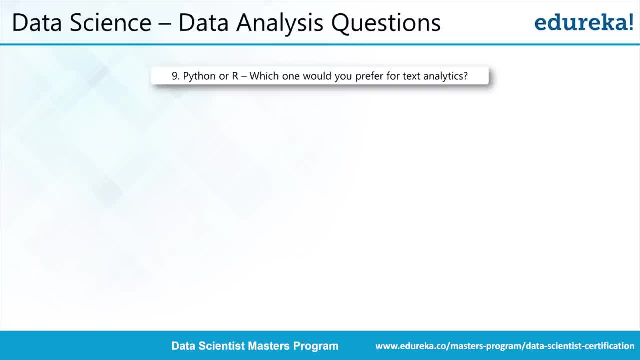 some generic questions like this. people normally do analysis on structured data, which is in rows and columns, but there might be cases when the data is not so well structured and those places the data might be textual, For instance, in twitter. right, if you are doing any sort of algorithms like sentiment analysis? 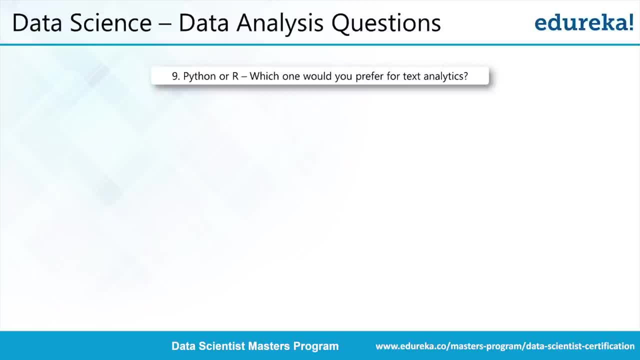 quite commonly known algorithms. so in that case the sentiment analysis could be for a brand, for a election campaign or maybe something else around your product features and so on. so text analytics in its own are really large domain, and in python as well as R there are number of libraries, so in particular R has libraries like tm right, the text mining package. 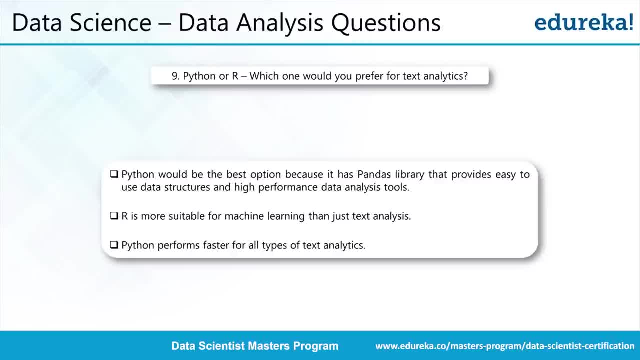 python as well. we have packages like pandas, packages like the numpy ones right, and also packages like nltk, which is built only for a natural language processing so it can deal with many different sort of text mining approaches or text analytics approaches. so in comparison, if you talk about, as I said, the robustness in python is much more than in R, but in terms, 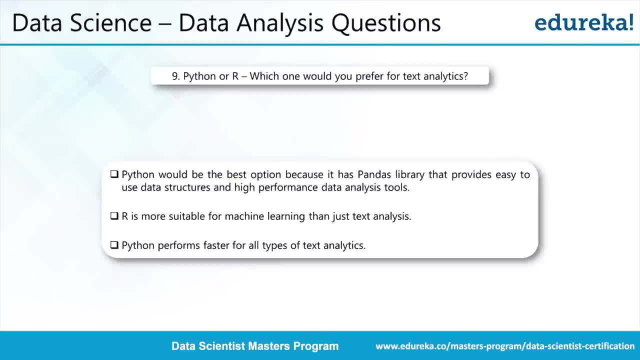 of features. both are powerful enough with the libraries and packages that it offers, right? So this is a fundamental sort of starting place when you do any analysis. so when you are given a data set and you are asked to do some sort of basic analysis of what that 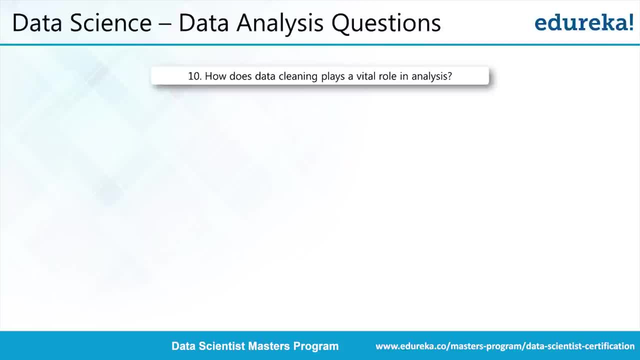 data tells you, maybe typically of questions like: I am in a retail business and my sales in a particular region is going down. so this is an analysis that is expected out of you and you need to dig through in understanding what really is the problem in the sales going. 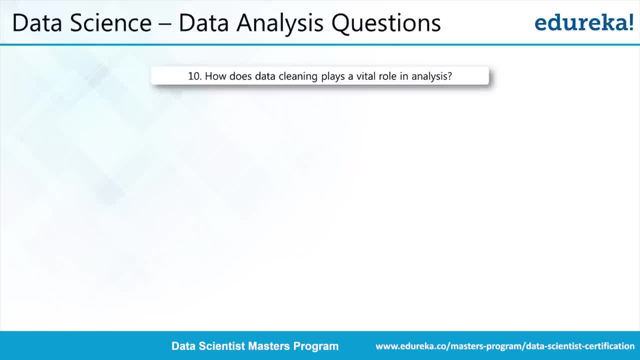 down. so if this is sort of the data, this which is given to you, you might want to first look at the transactional data, What is present in the system. then you might also want to go to outside of your network. maybe you might get the sentiments of your customers from social media platforms and 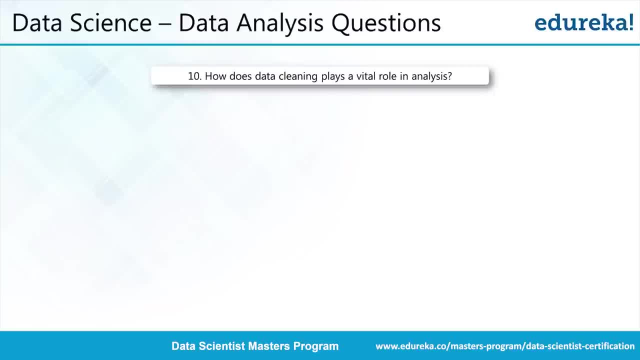 so on. so there will be different sources of data that you will collect, but often times collecting the data is not only the task right and not like only building a model or doing statistical analysis might like come very later in the stage, but what comes before that, after you have collected the data, is to make sure that the integrity of the data is maintained. 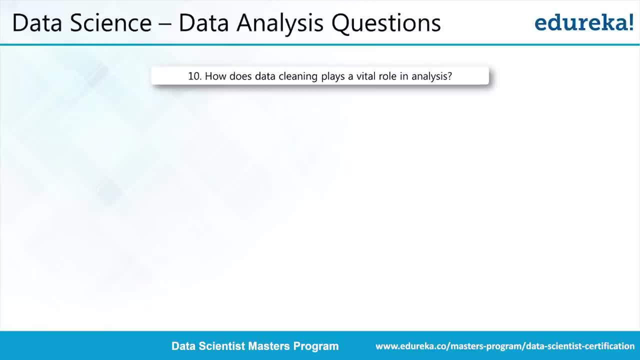 You will get rid of all the unwanted noise from the data and then finally prepare the data for doing the sort of modeling exercise or doing descriptive analytics on top of it. So this cleaning and understanding the data, doing lot of explorations with plot, in essence takes close to 70 to 80% of your time in any data analysis task. so if your company maintains 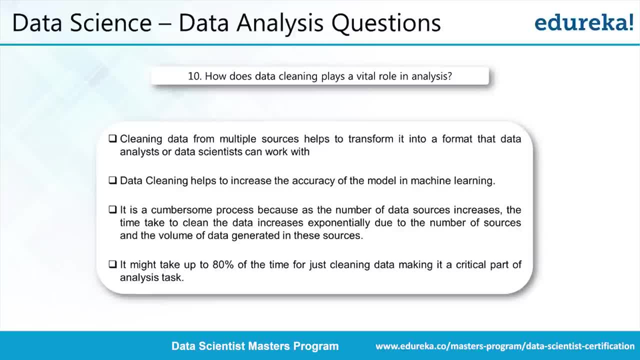 the data in a very well structured way. this kind of heavy time which we spend on data analysis might be reduced. The data cleaning might be reduced. otherwise, you need to like take this up for any new project that you take. take up which for which data is not available in prior or you don't. 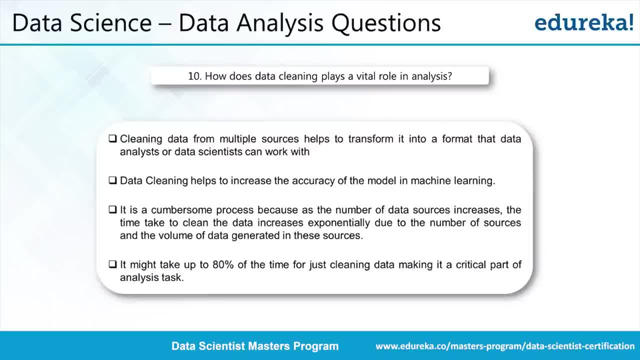 have, like any pipeline, which do this cleaning. you have to write it down of your own. So very, very important. if you don't do the cleaning part and understanding the data well, the analysis or the models that you build might end up giving you a very, very bad performance. 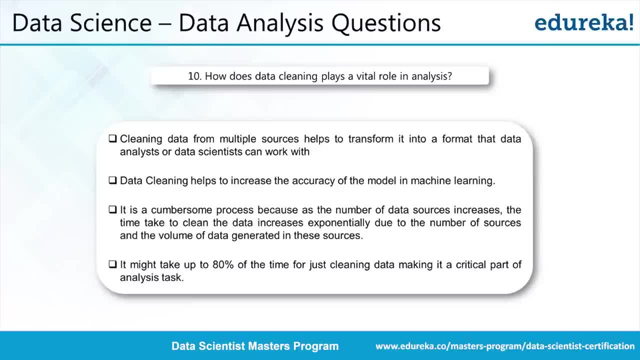 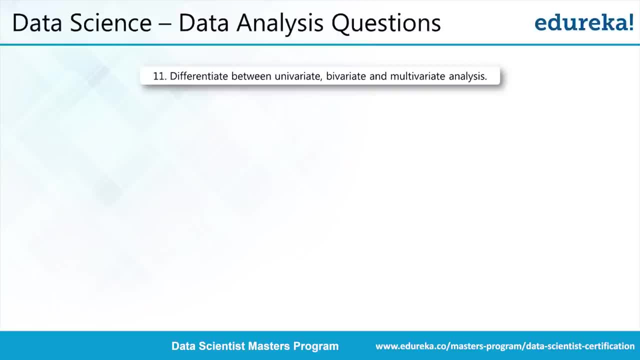 right, So very important. as I said, 80% of the time people normally spend on This task right, and often times when you are analyzing things like the example I told my sales are going down. what do I do? it is not possible to come out with such answers to. 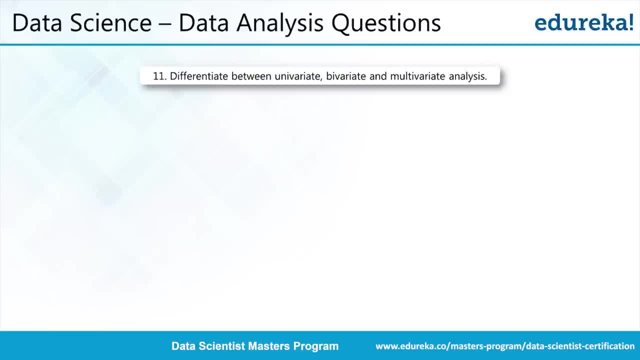 complex problems like this with just one variable right. so you might also want sometimes to move beyond one variable and talk about, let's say, how to do multivariate or bivariate kind of analysis. So often times this question comes up When, Where you like, ask to distinguish between this univariate, bivariate and multivariate. 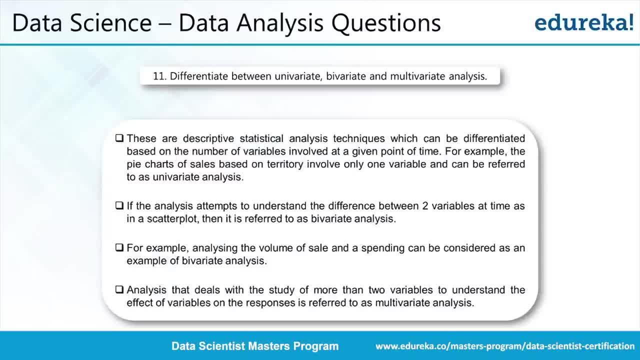 analysis, and the idea is very simple: in any sort of analysis it is not only one variable which kind of decides the end output of your analysis, but there are multiple factors involved. So when there are multiple factors involved, you might also want to look at things like 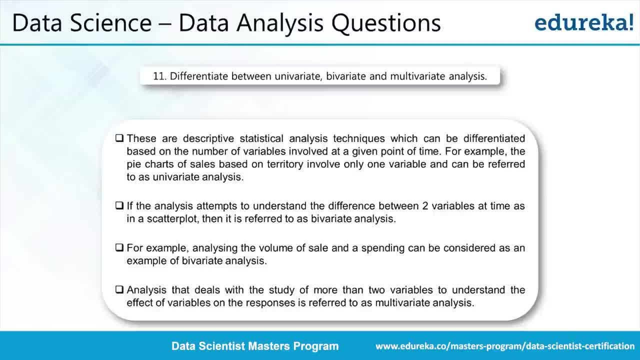 correlation. there are multiple variables. you want to see if there is any correlation between these things. sales are going down, but because of what? is it because my sales representatives are not going to the market? or is it my products are bad? or is there some other reasons? 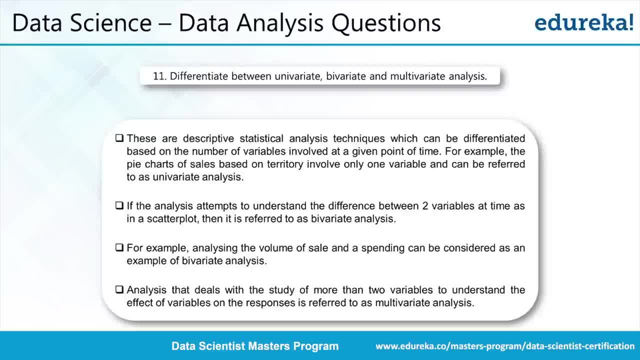 So with all the variables in one place, you might want to go and dig deeper to see if there is any relationships coming in the variables or not. and when we collectively get all these variables together and do some sort of coherent analysis around the problem you come out with. 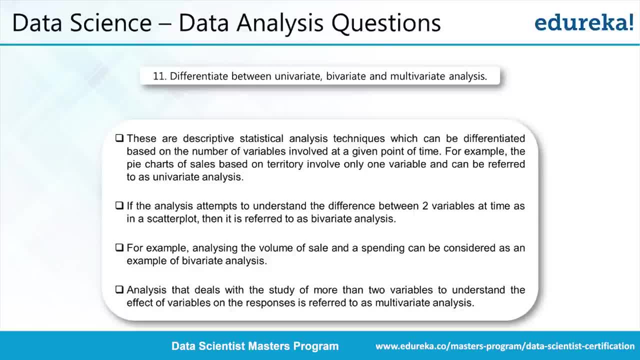 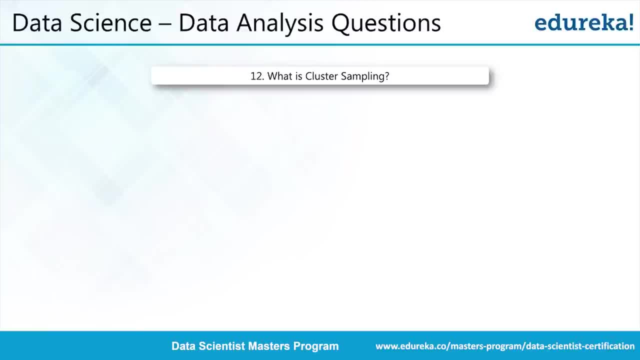 a really crisp answers to what you are trying to analyze right and moving on. there is also times when people Do some sort of grouping right with the data. you do a sampling right, you get a data set in your system or in whichever servers you are doing the analysis. but in that there might 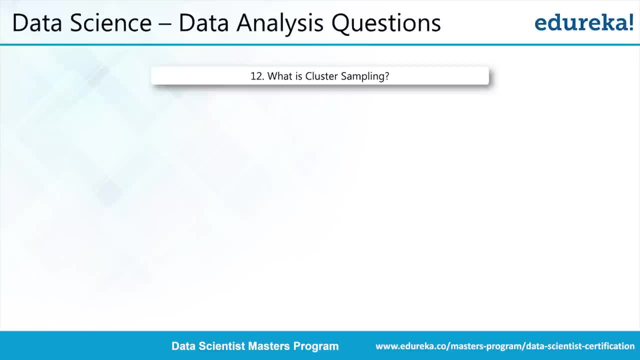 be lot, many number of times when even the randomized sampling of getting the true representative from the population, like that, might not work well right. so in those cases you might want to do some sort of systematic sampling, or maybe a cluster based sampling as well, wherein you might 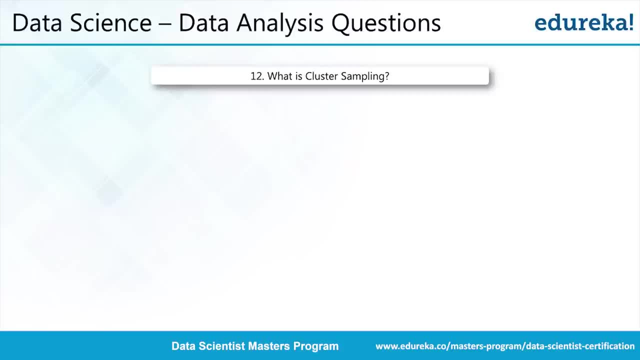 Decide to say I want to analyze the issue with only five regions in my mind and with the five regions I am going to form different clusters or in the systematic sampling. you might also want to say that with the five regions that I have got, I might want to analyze. 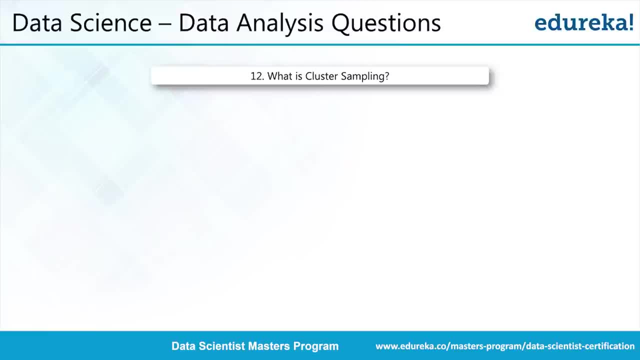 only for one product right which is not doing that good in the sales. so these kind of sampling techniques, like the cluster based one or the systematic sampling techniques- and there are different names for this- People might be able to Give a very good interpretation of what really went wrong. in whichever sort of analysis you 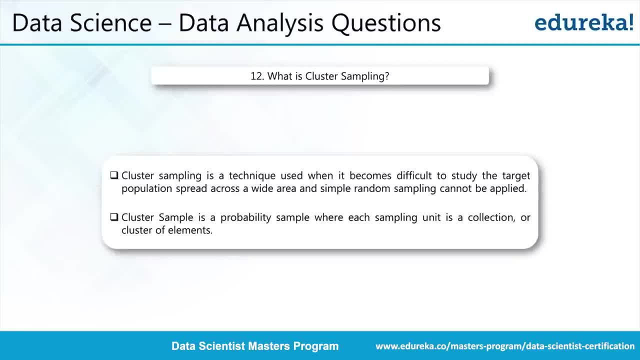 are doing so. one example is like sales going down, but you can adapt this to other analysis as well. but the idea is, instead of doing a randomized sampling by which we are not very sure which kind of data is coming in the data set which we want to use for analysis. but 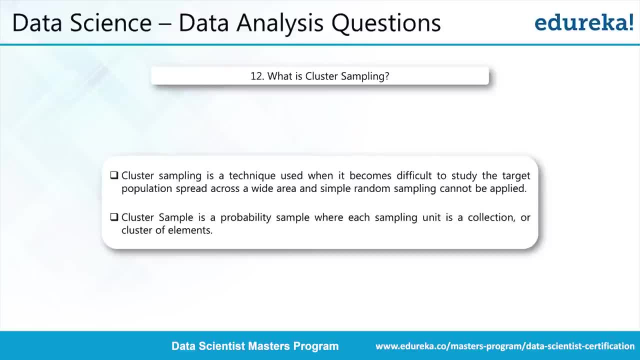 if you do it in a cluster basis, a cluster or a systematic sampling, you know exactly which clusters or which sort of regions in in this Example. you are like analyzing and in your end of the analysis you will be very able to say: this is not like a randomized sample that I have taken, but from these five regions. 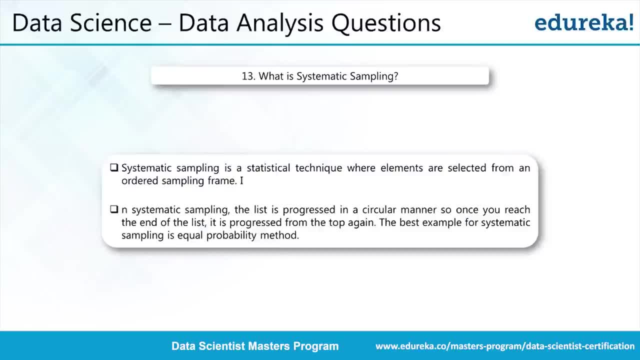 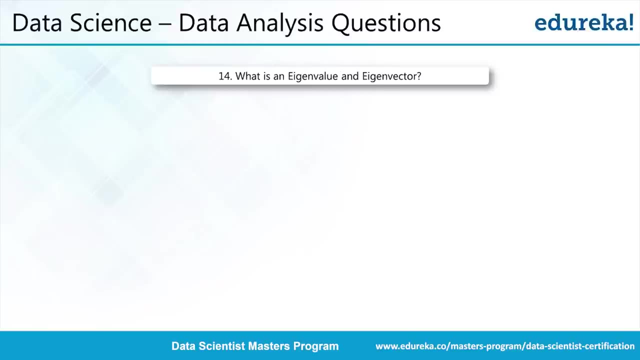 so there are many different ways of doing clustering, cluster or sort of the systematic sampling which kind of helps in this particular final end results of your, to put your end results in the right perspectives, right, instead of doing a randomized sampling. okay, one more, quite a useful 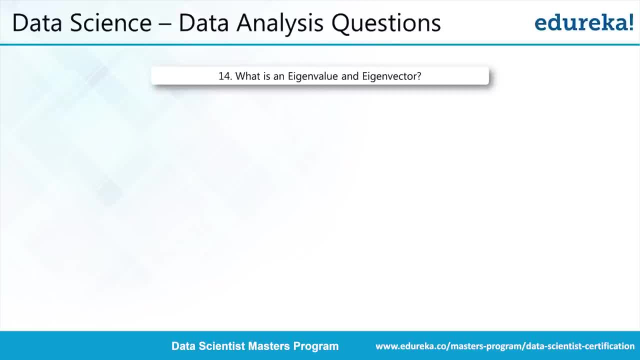 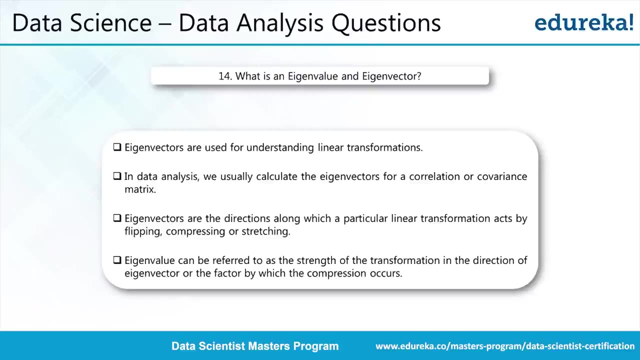 Sort of an idea kind of widely borrowed from the field of linear algebra- and this is a bit related to what we earlier saw- between moving from one variable to multiple variables, right and Egan value and Egan vectors, kind of a concept borrowed from linear algebra- helps us to bring in some in some way a linear combination of different variables together. 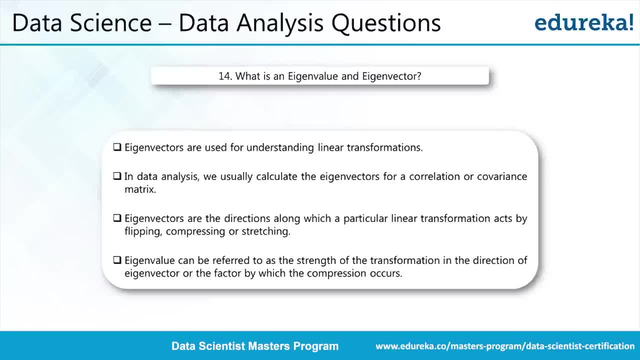 for instance, in some complex analysis, it might happen so That, given a data set, it might have many columns, right? let's assume you have a data set with 1 million rows and let's assume 10,000 columns. so, and these 10,000 columns are some features. 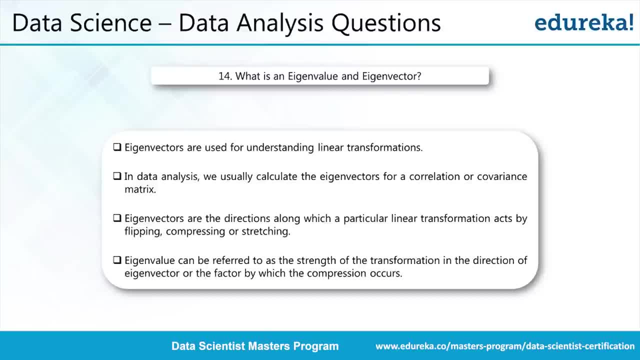 there are complex problems like that, but in most often, like most of the time, not all the 10,000 variables are useful, right, the input variables. so what we can do is we might want to transform this data set in a lower dimensional space, By which we mean this: 10,000 columns can be reduced to, let's say, only 100 columns. right? 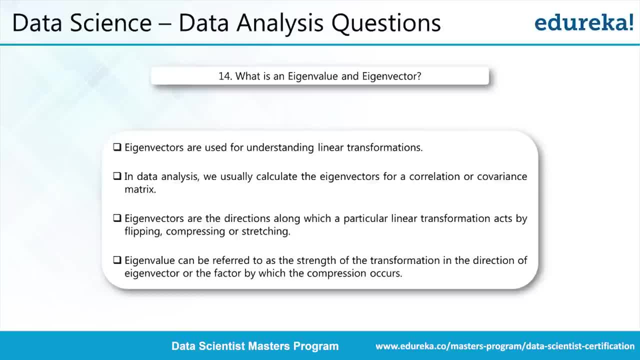 so Egan value and Egan vectors, are these ideas which helps us in this transformation? and the idea is: can this 100 variables be represented as some sort of linear combinations of the 10,000 variables? and if I am able to do that, my dimensionality is reduced the time I take. 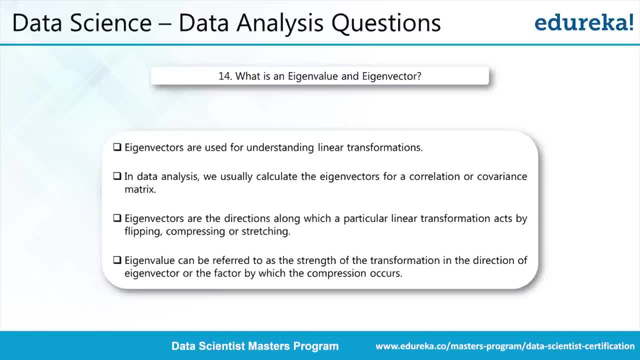 to do the analysis is kind of also reduced and the representability, which will come with only 100 variables, Will go up right. so quite a powerful idea. Egan values and the Egan vectors- and as I said, the Egan vectors is kind of that linear combinations of many kind of variables there. 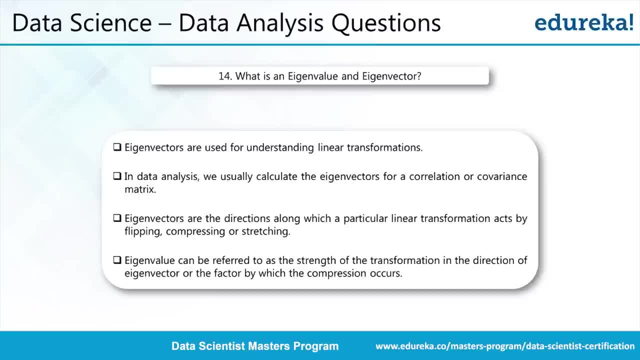 and this calculations around Egan vectors- normally happens for a correlation or a covariance, kind of a matrix which, as you know, the measure. correlation is also about how two variables are related, How strongly two variables are correlated, right? so that's why we are also saying this. 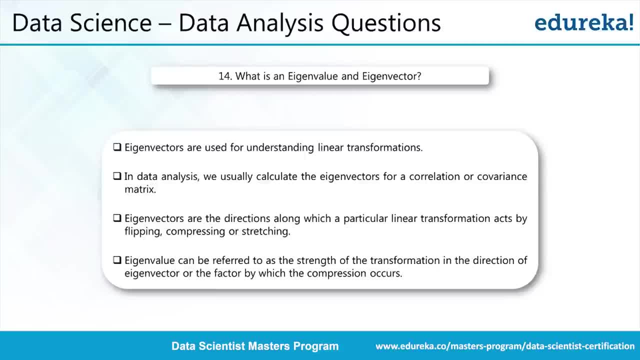 Egan vectors can help us to compress the sort of data that we have, right, and that's because of one Egan vector can be representing a 100 column, 100 variables together, right? so that's sort of how it works. so quite a powerful idea and commonly used methods for reducing the 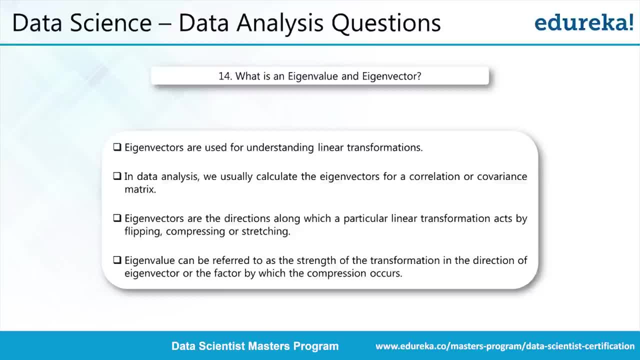 dimensions of an enlarged data set like the PCA, A principal component analysis is actually based on Egan value and Egan vectors. so if somebody asks you about Egan value and Egan vectors in an interview, also talk about the PCA principal component analysis, which is actually based on these two concepts, so that 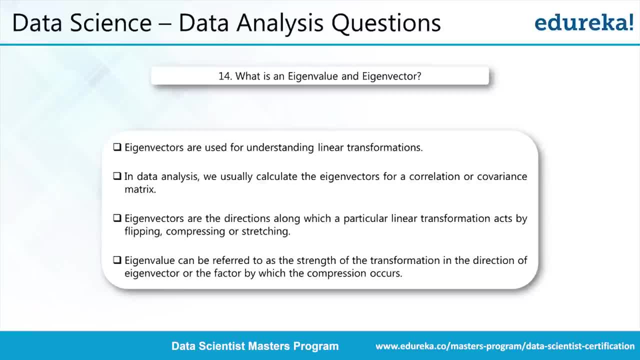 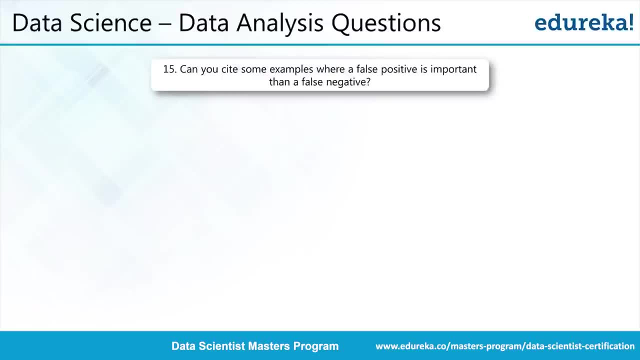 gives them a good idea to the interview view. you let you know about Egan values and Egan vectors and you are also able to think of its application, like in PCA right. so we talked about this false positive and the false negative cases in our confusion matrix example. 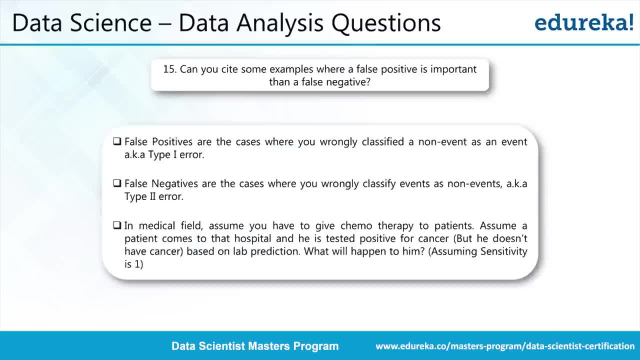 So this is exactly the same. you also talked about the type 1 and type 2 error. okay so, but let's now also drill further and say examples or kind of scenarios when the false positives are important, in scenarios where the false negatives are sort of important and the by 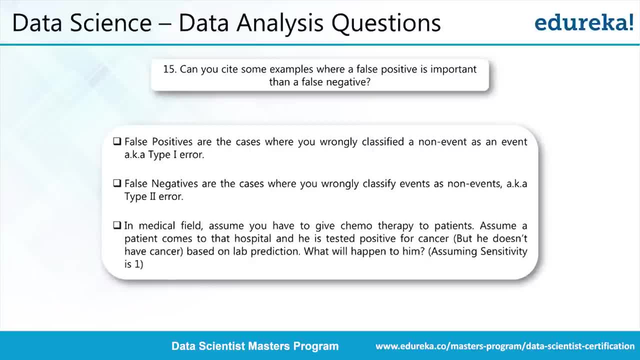 the term importance we mean: are we like allowed to do this mistake? if you are building a machine learning model, are we even allowed to do a mistake on either of the cases, The positive or the negatives? so for instance here, if I take an example in a medical domain, 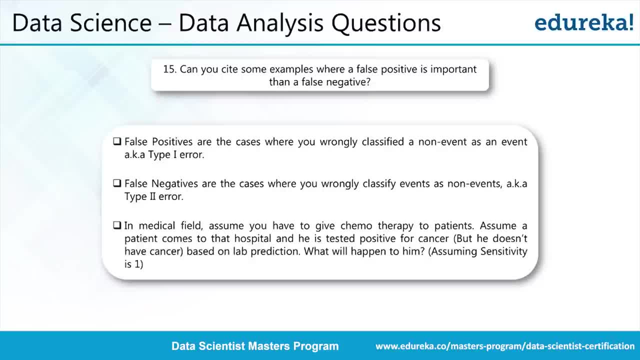 where we have, let's say, a process called chemotherapy, which is normally given to cancer patients, which is a radioactive kind of a therapy which kills the cancerous cells, right. so it is very focused sort of a therapy on the cancerous cells. so what will happen, if you like, predict? 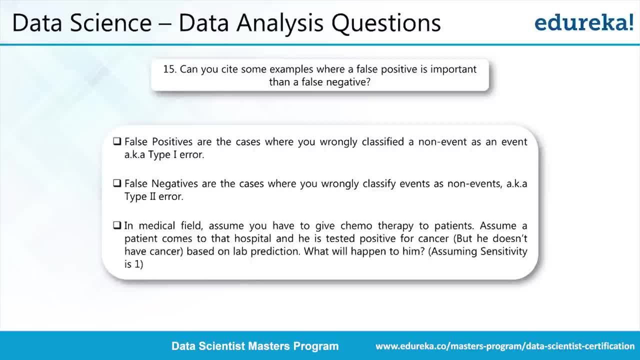 let's say you are building a model For Detecting cancers, right given a CT image, and this model would obviously not be 100% correct. all machine learning model has its limitations, but you are here required to predict this- whether a patient has cancer or not- and based on that, radiologist might decide that. 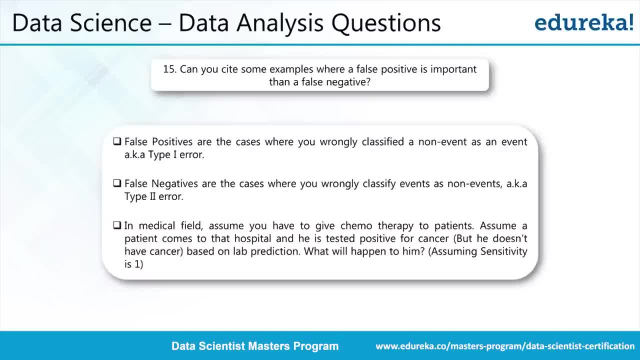 whether the chemotherapy is right for this patient or not. but imagine now if you have predicted somebody to be positive for cancer but the patient is actually not having the cancer cells there, right? so in those cases you might end up saying let's go ahead with the chemotherapy. but the side effects of chemotherapy are like very, very adverse right because you 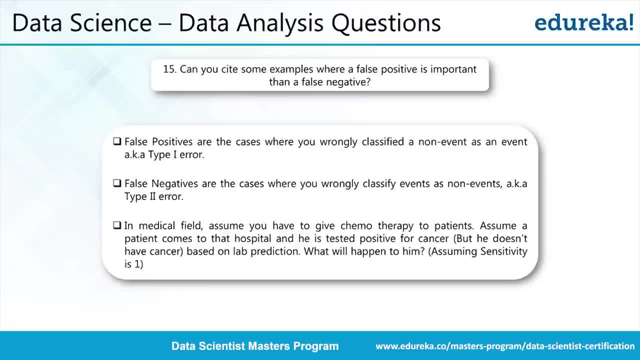 are giving these therapies on the healthy cells if the patient is not having the cancers. so in these cases sort of the false positives becomes a bit more important. so it will be absolutely fine if your model says the patient doesn't have cancer. if, even if there is like 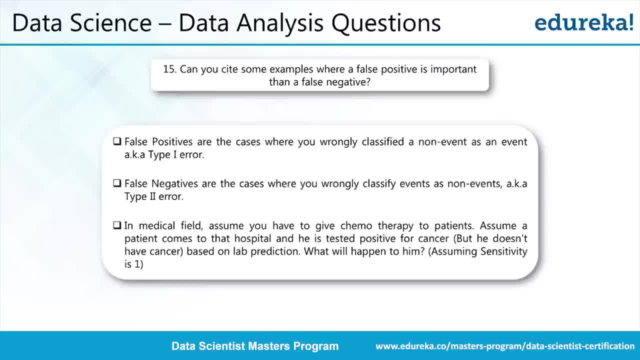 this slight possibility of cancer present In the cells of the patients, but in that case you are not like exposing the patient with a chemotherapy there, right, which is like more harmful than saying that the patient doesn't have the cancer, right? so in these cases, the false negative, though the false negative itself, 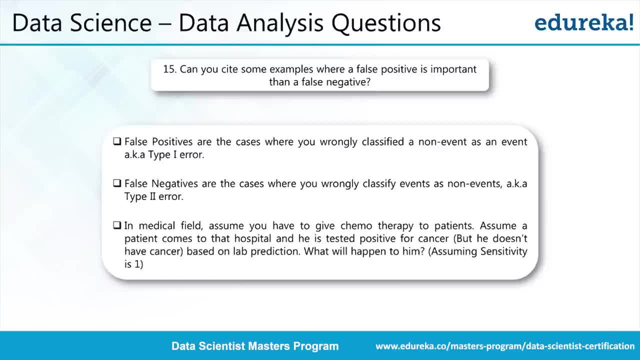 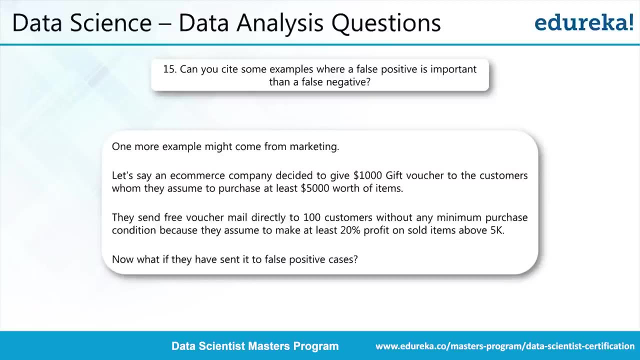 is not so good in this case, but at least with this particular example, the false positive gets the importance than the false negative, but both are bad, as you know right from the confusion matrix discussions. so, in simple terms, it is better to not expose the patient with a false positive, with a treatment like this, chemotherapy, like treatment, then it 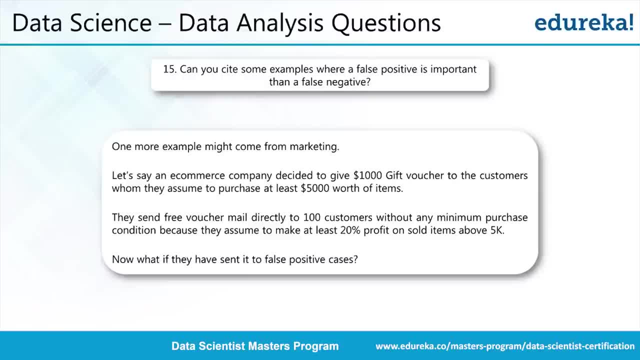 is like much better than saying you don't have cancer, okay. and a very similar example in some other context might also come up, so if you would like to think of some other examples in the same context, okay. so where is the other case now, which is the false, negative right? 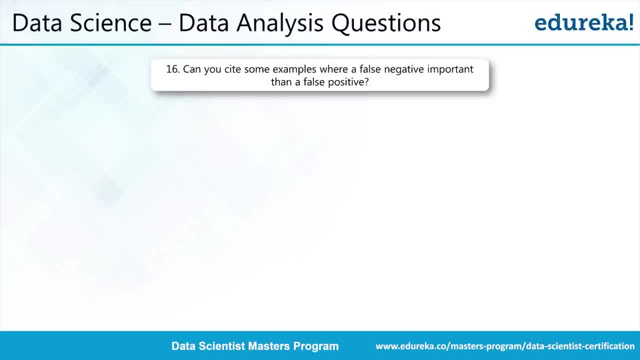 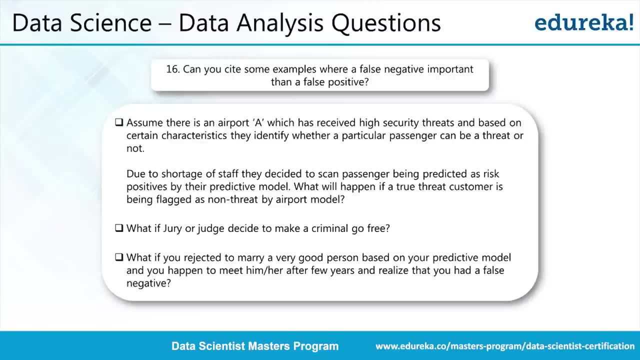 so we talked about the false positives importance, but there might be also cases where false negative might become a bit more important there, And for examples Like this: if you are, let's say, building a model where you want to convict a particular criminal basis, all the records and the arguments which has happened in the court right and 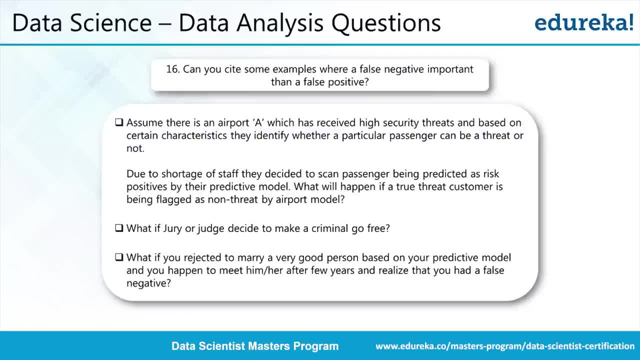 let's see what would happen if you make a criminal go free. right, because your model says it's false, negative, the, though the person is actually a criminal. but because your model predicted, based on all the evidences you had, the person is not a criminal. so you are letting. a criminal like walk free in society. So that kind of is More harmful than convicting that person, and maybe for a prolonged period you might also want to get more evidences and build a stronger case. So it is fine to keep a suspect in behind the bars for a longer period then letting 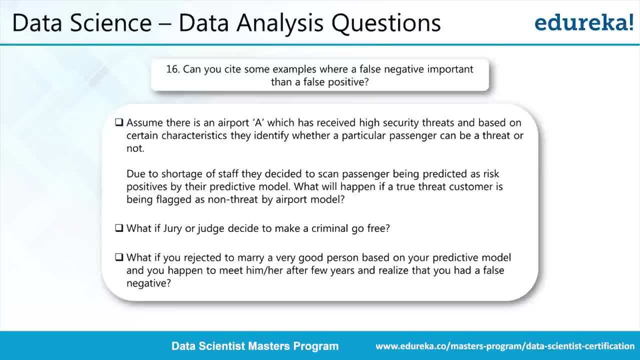 the suspect go free there when we like, know that that it might be a case of a criminal going free from the judicial systems there, right? so in these cases the other case becomes more important. so keep in mind it is very easy to get yourself confused between this. 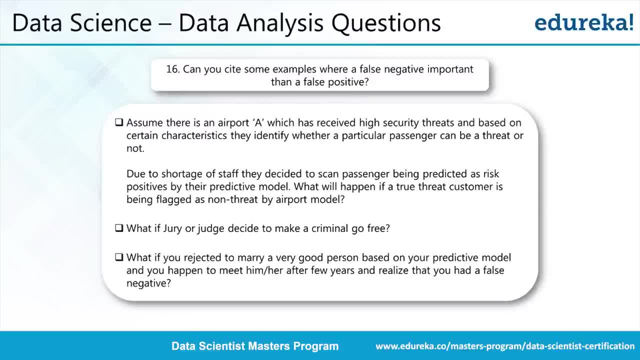 false negative and false positive, But if you keep an example in mind always and like, don't give any room for confusion there, though it is a confusion matrix based on which these two ideas comes in, you will be able, at every time, put these examples in front and talk from that. so if you start to 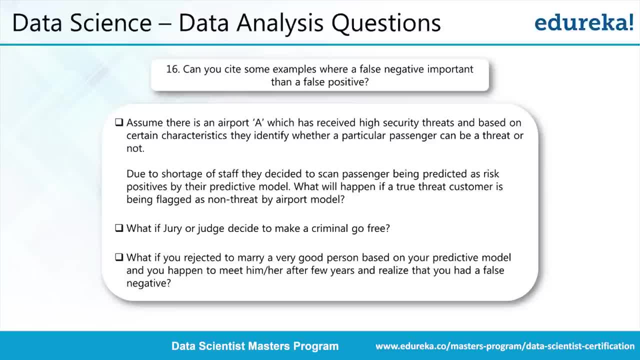 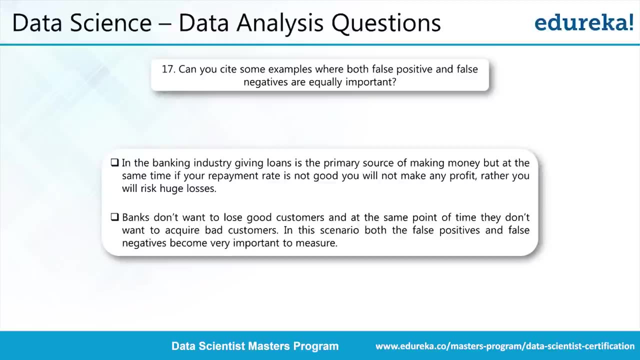 explain what false negative is in terms of the formula, you might get confused, but if you take an example and then explain, things are much more clear for you as well as the person who is hearing that in the interview. right, and in cases when both are important, typically the one which relates to banking industry- you are building a model which will 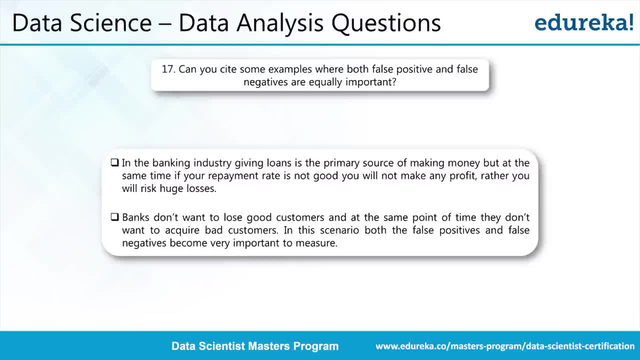 decide whether to give a loan to a person or not, bases many of the input attributes that around which you have like collected the application from the customer. but here you say, if the customer is really good and you are missing the opportunity there of not giving the loan versus the customer is really bad in terms of its, his or her credit history. 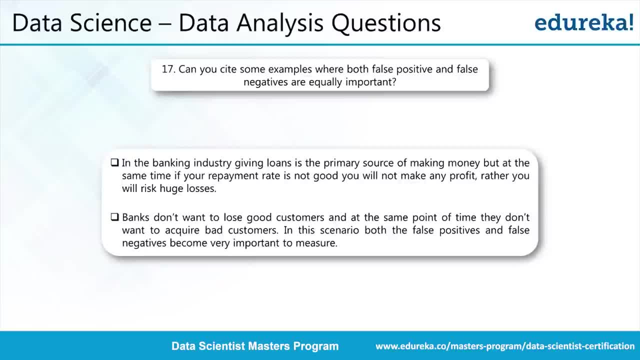 and you are giving the loan In both the cases. in one case you are losing the business, in the other cases you are taking a risk in which you will lose your money right. so in this case and in this example, both kind of has an equal role. so if you are positive or false, negatives are in either of this is 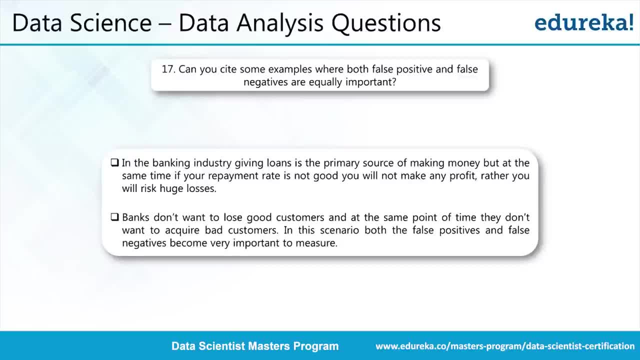 high, you will end up losing some chunk of your money there. keep these three examples in mind and every time you get to like here false positive, false negatives- things should not be like confusing at all. okay, So now let's also talk about building a machine learning system. 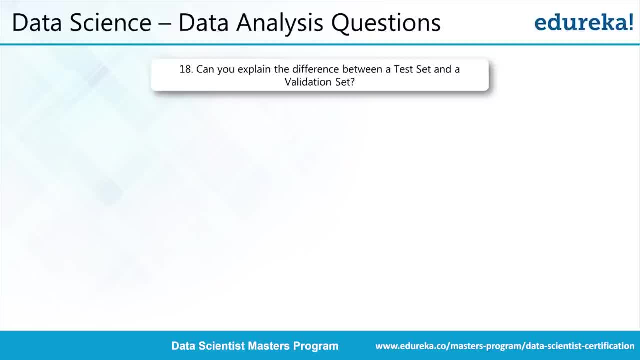 Okay, So let's talk about building a machine learning model. so so far we have discussed about what happens after building the model, right, but let's step one, like get one step back and see how do we normally build a machine learning model and what kind of processes we normally. 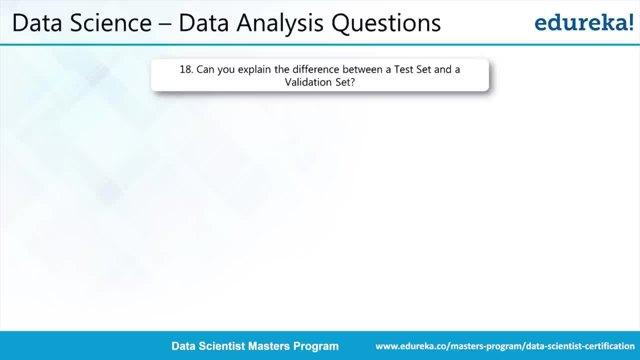 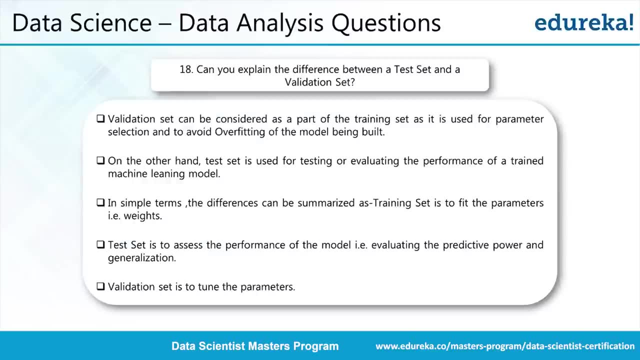 follow. so when we are like building a machine learning model, we know that we need to. given a data set, we need to divide it into different buckets or different parts. so the commonly known divisions that we like have is your training data. right then we also divide the. 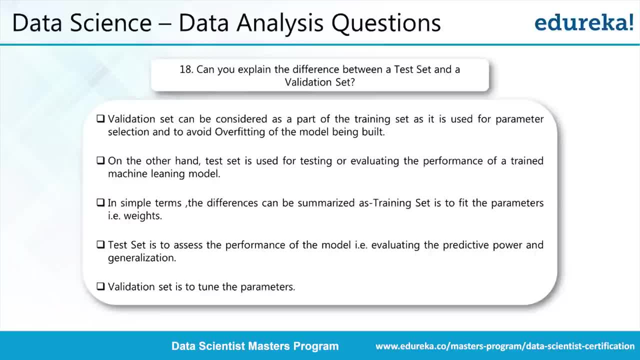 data into something called test data, and sometimes we will also divide or keep one portion of your large data set, which is called the validation data. so often times people confuse between the test data and the validation data. right, so what happens is in the training process. there are certain models wherein, while you are training, you will use the training data. 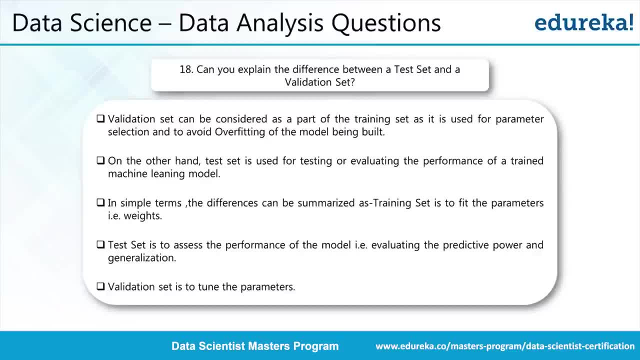 obviously, but in the process of training you can also involve something like a validation step right which will make sure that during the process- Okay, During the process- there is one part dedicatedly given for the validation of the model, and when the model is done, you might see that the final model is well trained on the data. 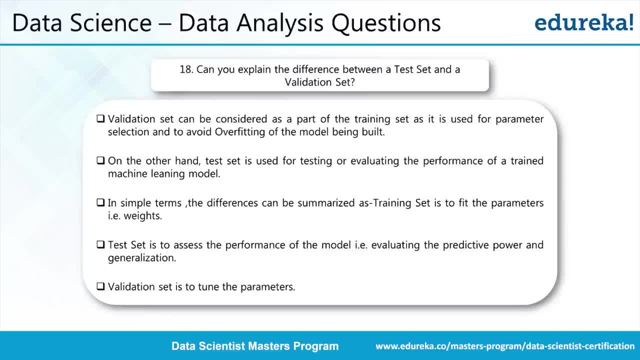 at the same time validated. but when the model is completely done, then only you get into a process that we call testing, right? so you can imagine like this: you have a data of thousand records. you keep some seven hundred records for training, hundred record for validation and the remaining two hundred records for testing. so there are three splits, right? if 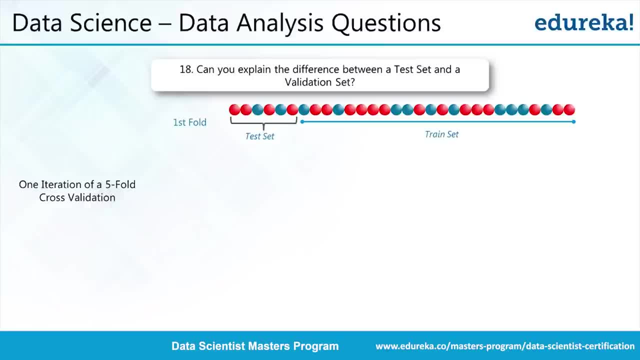 I would like to explain this with an example. this is how it will happen. so there is a process called k fold cross validation in which k can be any number like between five and ten. mostly there are like standards saying five fold cross validation or ten fold cross validation. 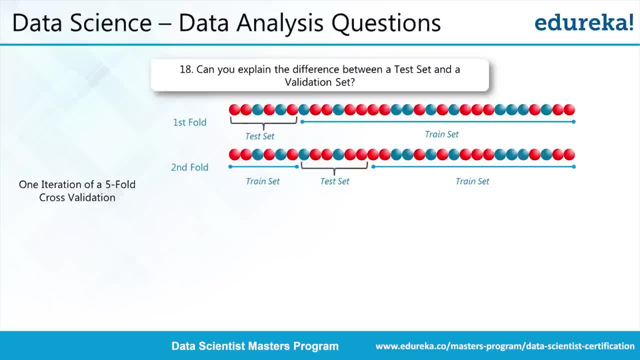 and idea is, when you are building your model, you will work with a training set right and a validation set In which a small portion of the data you keep for validation and the rest you use for training. so what you see here- test set- can be like replaced with a validation set right, and you 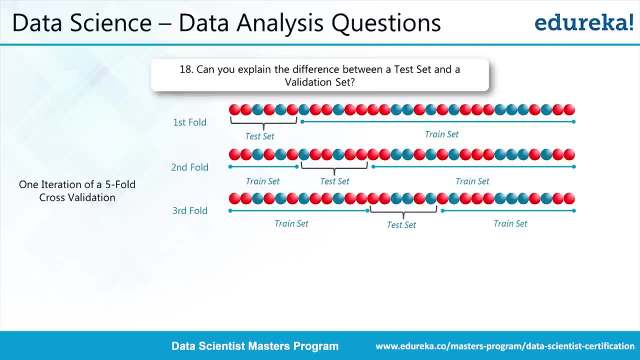 can see that this is a rolling sort of subset and you keep changing it in each fold. so you go for the first fold of the iteration. you keep one validation set and the rest of it is the training set and the next fold. you move this window to another subset and the 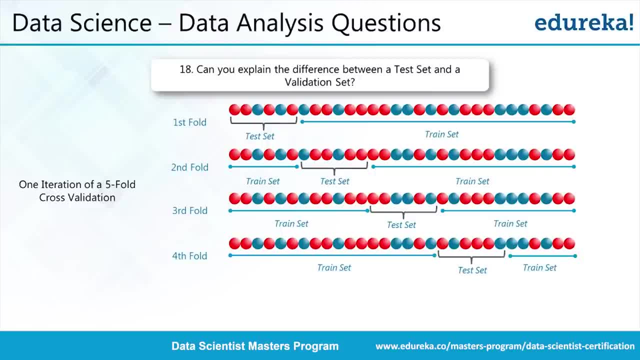 rest is training data and so on, And when this model is done, Using this k fold cross validation approach, in the end you will get a model which you can then use on the testing data to see if the accuracies are good or not. so this kind. 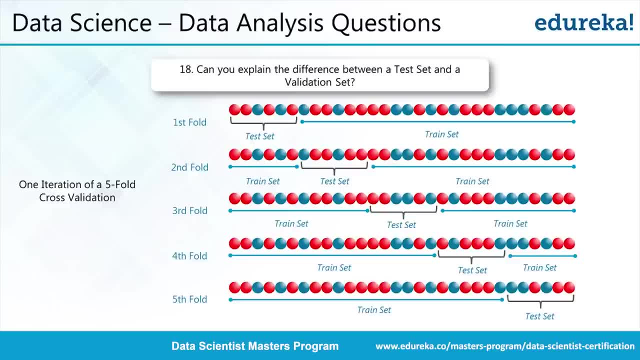 of brings in a lot of performance improvements. people have also found validation set to be an really good way of tuning the parameters in many machine learning models. as you might know, there are something called parameters, typically in the neural network models, and these parameters need to be tuned as the model is kind of proceeding. 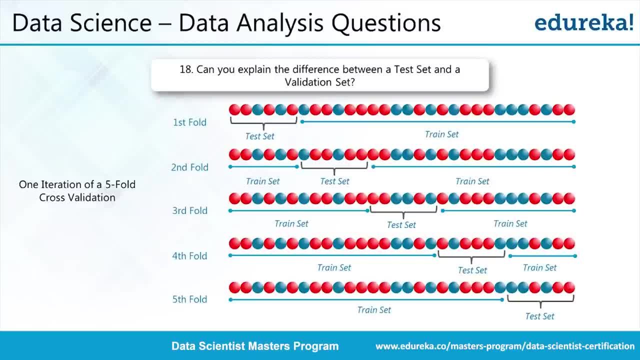 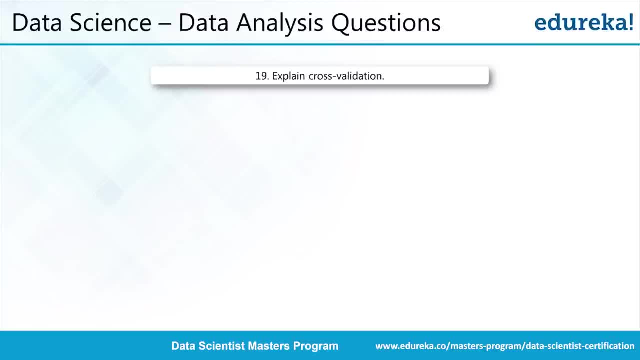 So we cannot use the testing data set for tuning this parameter. so validation set kind of comes very handy in those cases. So we just talked about the cross validation. so when you keep moving this validation set in each of the fold- first fold, second fold, third fold- and the validation set is keep. 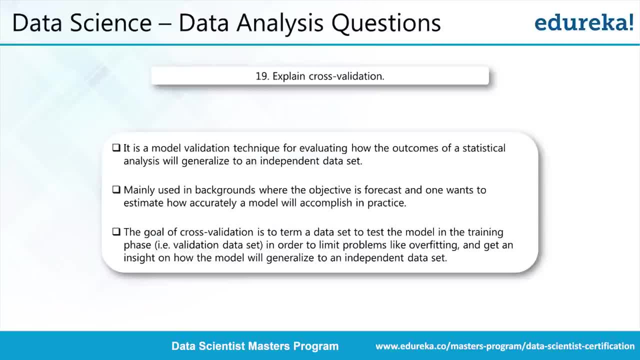 changing. you kind of do this process of cross validation And the idea behind doing cross validation is to see how well is your final model generalizes to the data That you have. so, independent of which data you use for training, your model should generalize because oftentimes it happens when you train your machine learning model it works very. 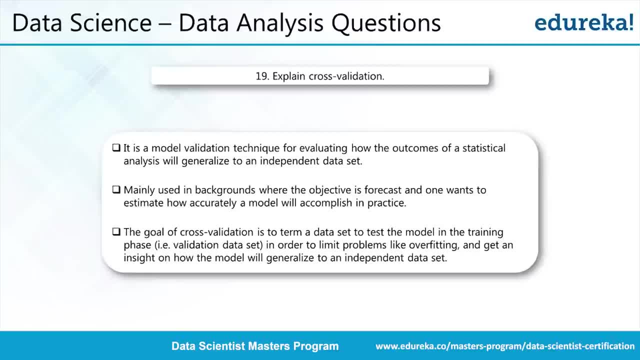 good in the training part, but when it comes to the testing the model does very bad. the same problem with the overfitting and the under fitting cases. So in this approach of cross validation, you have made sure that your model has trained on various subsets of the data right and in the process we also have this small validation. 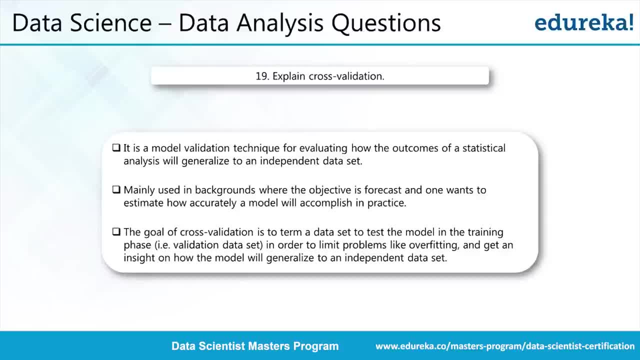 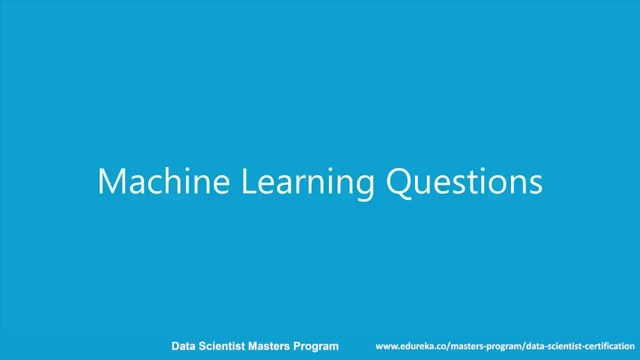 set. So in this stage of the cross validation process you are able to use a different subset. so that means you have trained your model very well. So irrespective of which data you use, your model is going to do well in the testing cases. So that's how cross validation brings in the capabilities. 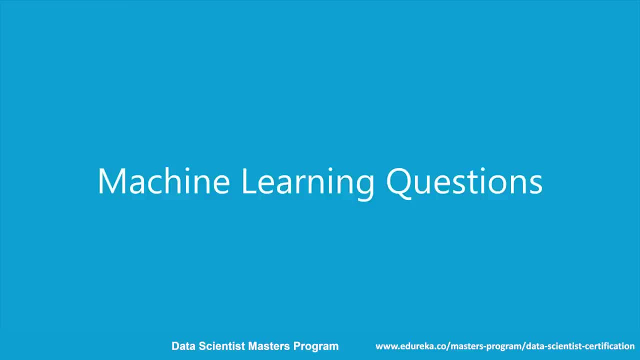 So with the two pillars, like the statistical analysis and the basic data analysis, I hope you are getting some sense of how people ask a particular question, coming from either the model building perspective or from normal data analysis perspective. right, So we're going to know. now go a bit more deeper into questions which might relate directly. 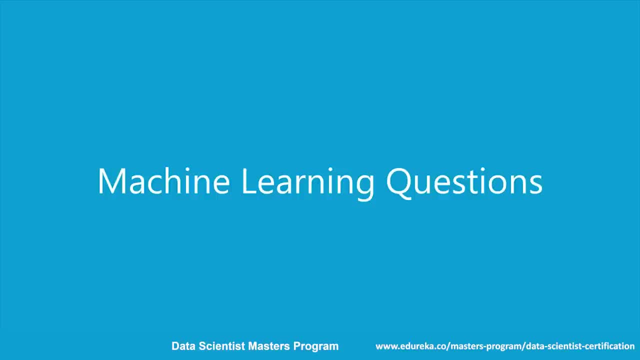 to machine learning. So these are all the most questions that you have seen so far are either saying: how do we do analysis after the model is built, or how do we normally perform simple data analysis, like AB testing frameworks and so on? But what if you are asked something very particularly from a machine learning domain? right? 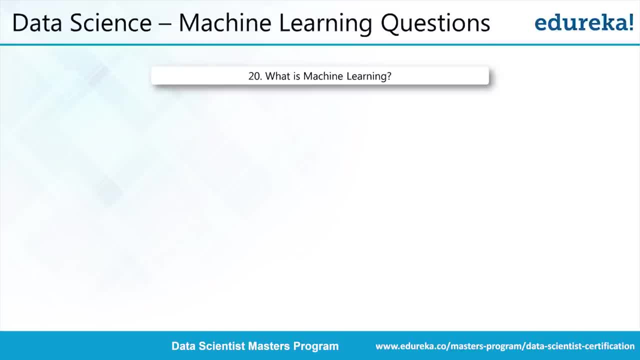 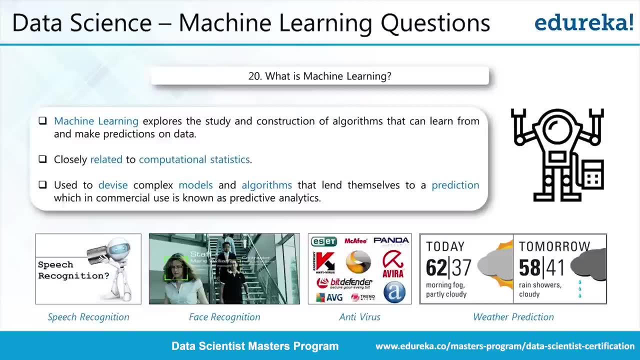 So the next set of questions- We'll cover those part. like people might also start with the basics, like: what do you mean by machine learning? So the idea, I think, must be very clear. you are given a set of data points particular to a given domain, right, and you would like to build a learning algorithm which will take 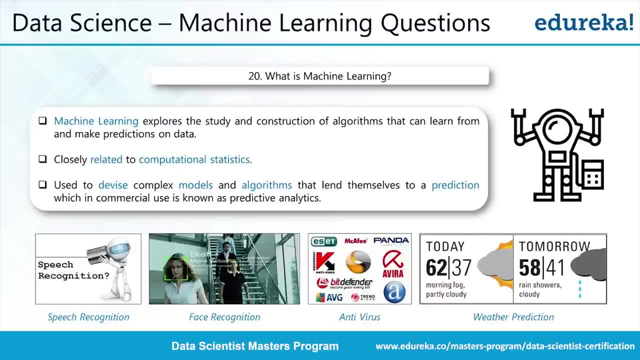 the historical data and predict something for the future. So, as we talked about many examples, finding whether a convict is actually convict or not, like predicting if, given the evidence is, a person is is a convict Convict there or not, or predicting whether we should be giving a loan to a customer, or 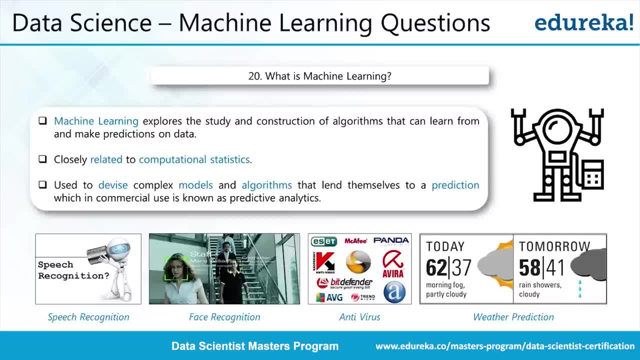 not right? predicting the onset of cancer in a given patients by using the given patients historical records and so on. And now this algorithms are now even becoming more complex, like it is starting to work on speech data, face data, which are mostly used for biometric authentication systems, right? 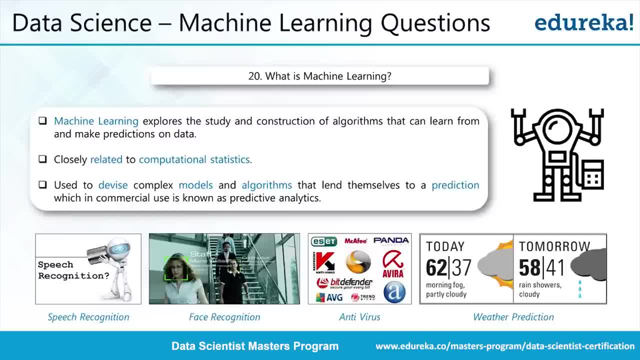 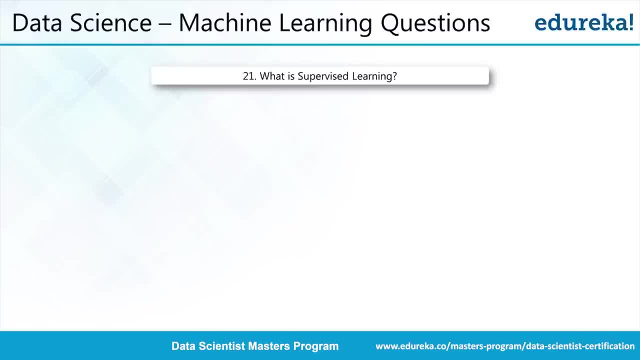 So many use cases coming up from various industries, right? So in machine learning, the most commonly used two types of learning, the supervised and the unsupervised learning. there are, like two other types as well- the semi supervised and the reinforcement learning- and the idea is around if you are given a set of input attributes. 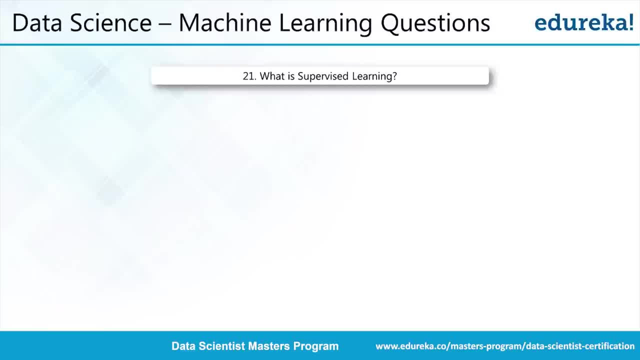 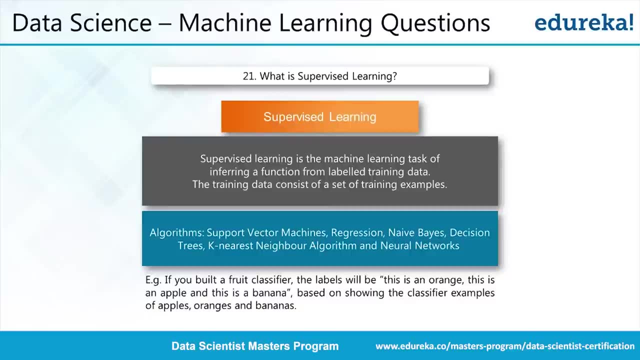 do you have a label which can help to learn the input attributes around any data points that you have or you don't have, right? So if you have, then the approach could be a supervised learning approach, versus if you don't have, then the approach is more. 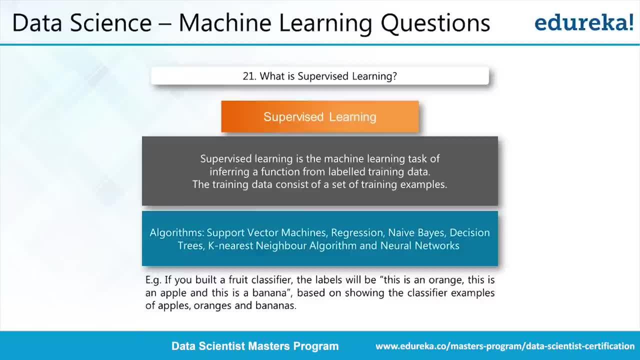 An unsupervised. so some examples of the algorithms are like support vector, machine regression, a base decision trees- all of these are the supervised learning algorithms. So now, very simple terms. if I say you are given an input, attributes for identifying, let's assume a sort of given an image of different fruits based on the characteristics of the 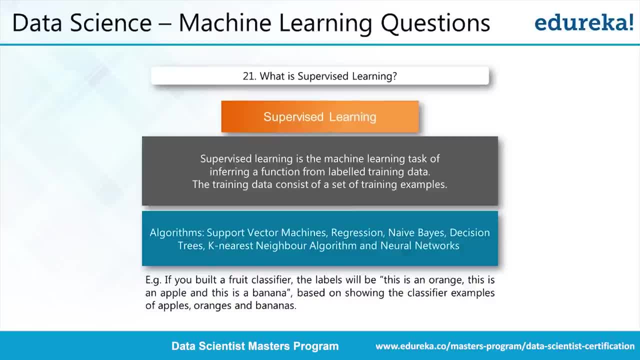 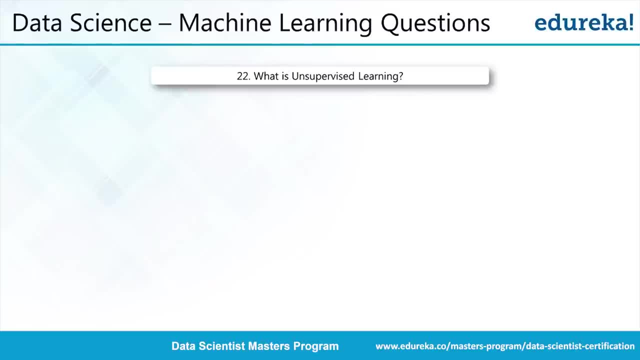 fruit. Can you like identify whether it is apples, bananas or the oranges? So if I'm given that label with me, the model will Run keeping in mind that, given these characteristics, this is an apple, this is an orange and this is a banana. But in the other case, if you go for a clustering approach, where such a label of saying that 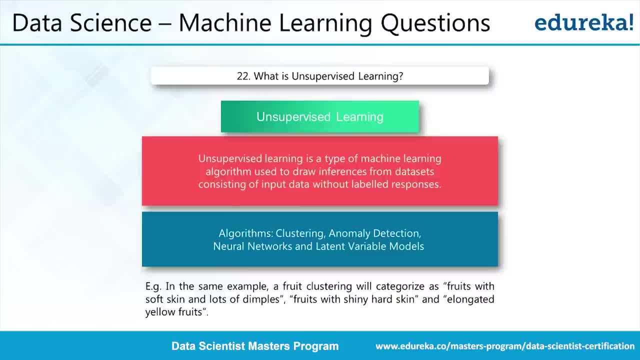 it is an apple, banana and orange is not available, then we might just simply segregate the data points with the input features, maybe with color, with texture or with the shape. right with that we can maybe say that particular fruit with this shape is, like you know, into. 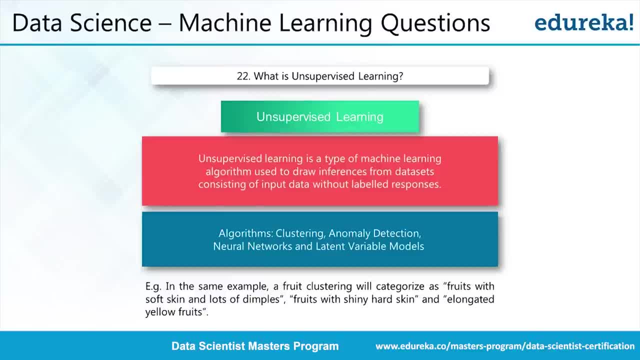 a bucket And, like all banana or another kind of a spherical shape, it might be apple or an orange. So, depending on the presence of a label, we can say either to use supervised or an unsupervised learning, and both of these approaches are quite common and sometimes there are certain. 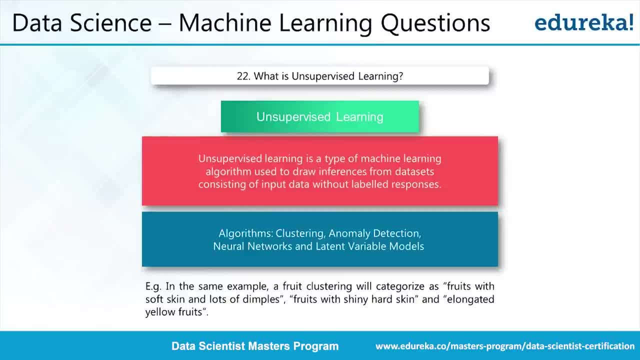 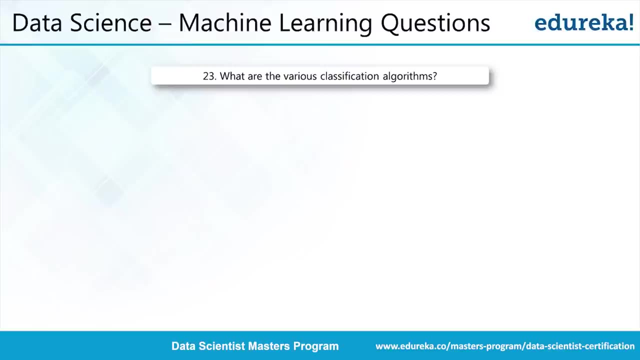 algorithms which can have the both ways. It can also learn an unsupervised manner and the supervised manner. So, depending on how you model the problem, the fundamental difference comes from the fact on whether we have the label or not. Ok, so when we talk about the supervised learning algorithms- other name for supervised kind- 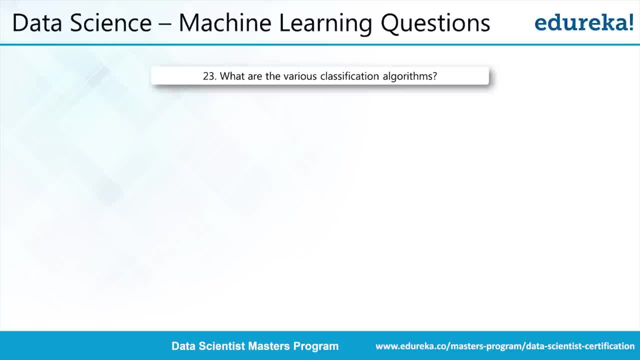 of one of the types in the supervised learning algorithms is classification right and the classification is around, given a set of input attributes, and the label is like categories right, for instance, if it is fruit, bananas, apple and oranges, like if it is a customer whom we want to predict into either kind of a defaulter type or a good customer. so the 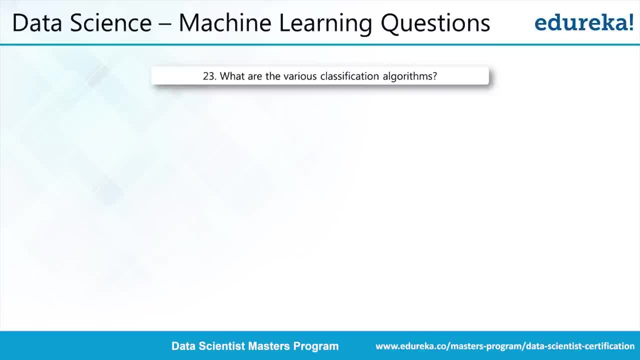 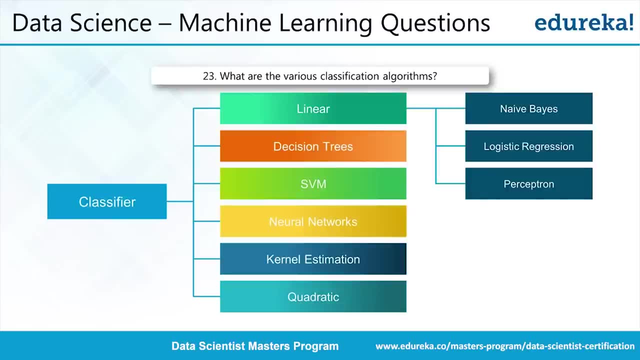 classes are two like: one, which is saying the customer is going to be a defaulter. the other says the customer is going to be a good customer. same is true for when you want to build a classification algorithm for detecting cancer, whether the patient has a cancer or 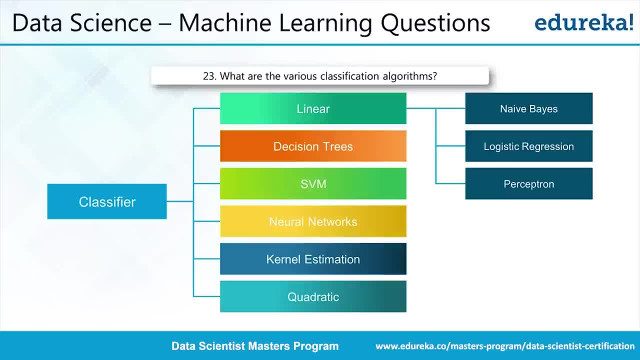 not has a cancer, right. or if you want to detect, let's say, a malicious content or a malicious file which might be a virus, trojan or worm or something else, right. so in that case the classes are now many, so more than one class can also be there. but the fundamental idea- 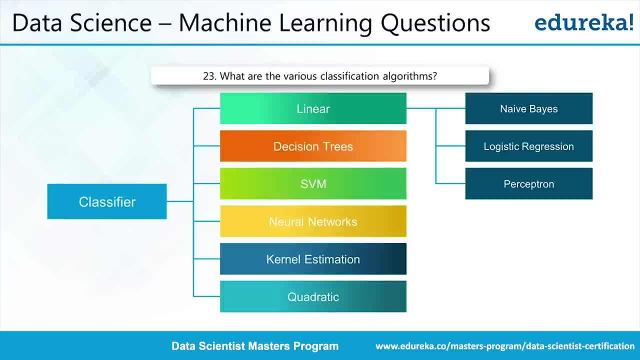 is, We are following a supervised learning algorithm, but the type of problem we are solving is a classification problem. so instead of saying classification algorithm, we can also say it's a classification problem using a supervised learning algorithm. so these are the various types of classification algorithms, like the linear regression decision tree. then you have 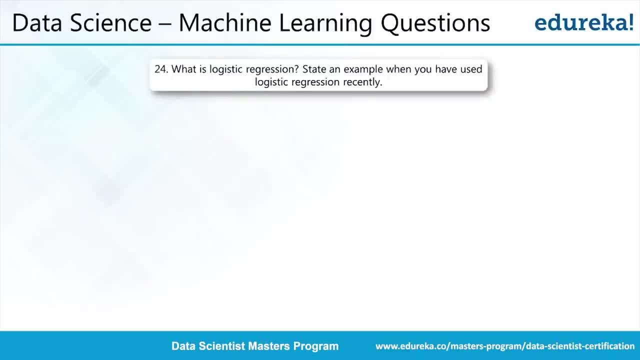 the support vector machines and so on, right. So now let's talk about one of the types of classification algorithm called the logistic regression Right, so very commonly used algorithms, and banks or companies as big as like American Express, so sort of, have leveraged the logistic regression algorithms to quite a extent, and 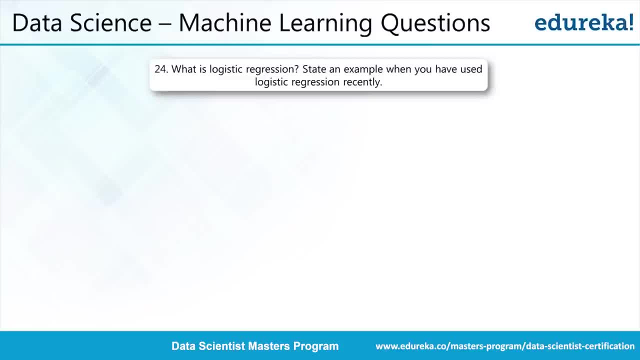 they have like built a really, really robust implementations of these algorithms, particularly in banking sector cases like predicting whether a customer is going to be a defaulter or not, given if I issue the customer a credit card or give a loan right, these kind of decisions can very robustly be taken from. 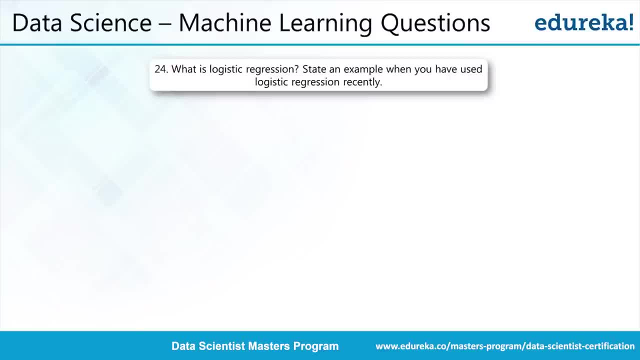 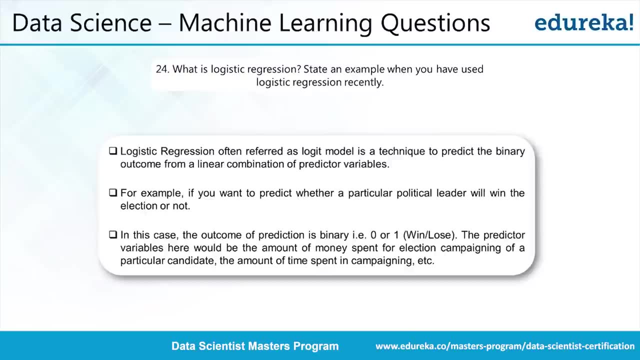 A logistic regression algorithm, and these algorithms are best suited for two class problems or a binary problem, right where you have either- why yes or no? quite a common technique, as I mentioned, and in all the possible cases, wherever you have these binary classes of problems, you might use a logistic regression, a political leader winning a collection, or 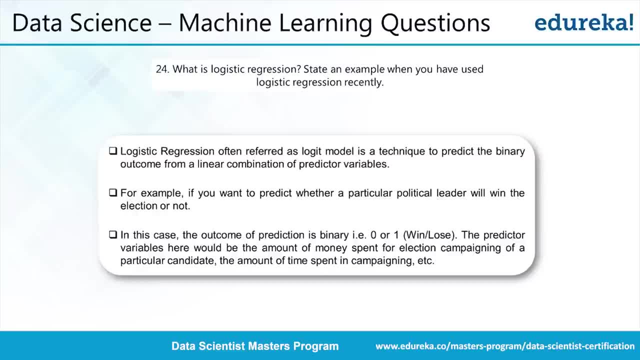 not somebody getting a success in an examination or not, and, as I mentioned, whether to give a loan to a customer basis, whether he or she or is going to become a defaulter Or not, and many of these like binary types. so keep in mind: logistic regression works. 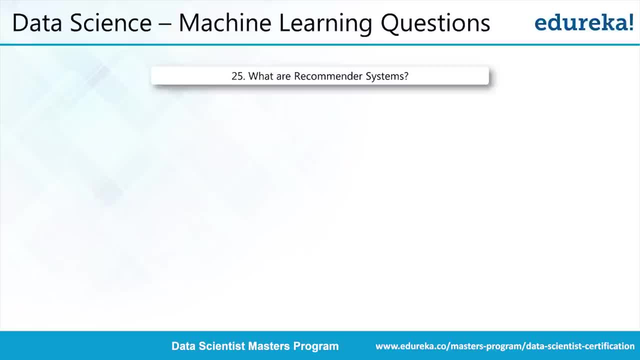 best for classification problems with two class, so one of another, widely used algorithms like the recommender systems and like. I think this particular algorithm doesn't need introduction. so this is that common nowadays. take an example: in Amazon you have a product which you are browsing, the products which comes in bottom of the widget which says you may also like. 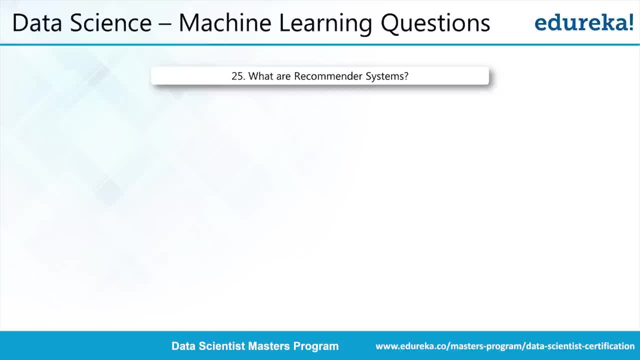 or customers Brought. this also brought this right. so these sort of recommendations is actually from recommender system which is running in the back end, if you like. take YouTube example: if you watch one video, the next video is like starts to come, one after the other. right that again. 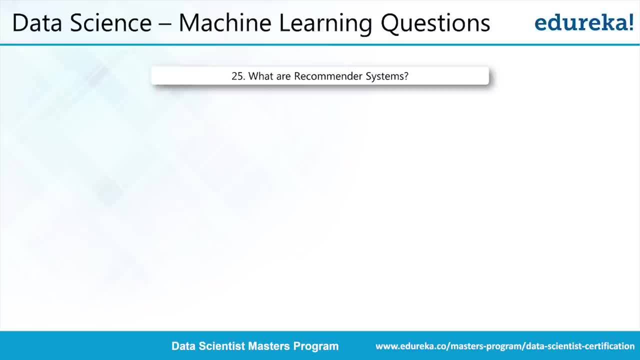 is a recommender system working in behind the scene. or if you take Netflix, if you watch a particular movie, it starts to adapt right to a movie which you might like. Netflix also uses recommender systems. The applications are like coming More and more as sophisticated systems are building in right. Facebook uses it for recommending. 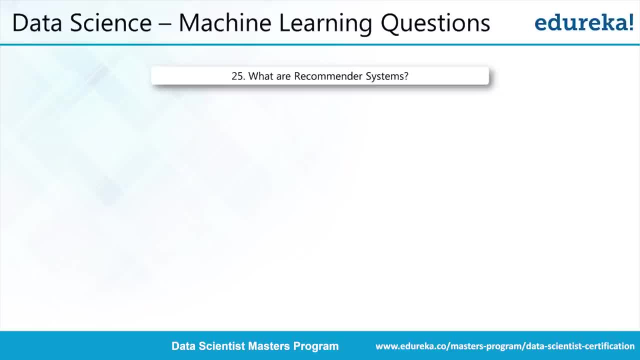 friends. right, you have a set of friends and, based on your data coming from the contact mail list, Facebook starts to curate friend suggestions. and all of these are algorithms which might benefit the business in some way or the other. for Amazon it is: if you give a recommendation below a page, people might buy one more than one product in a transaction. 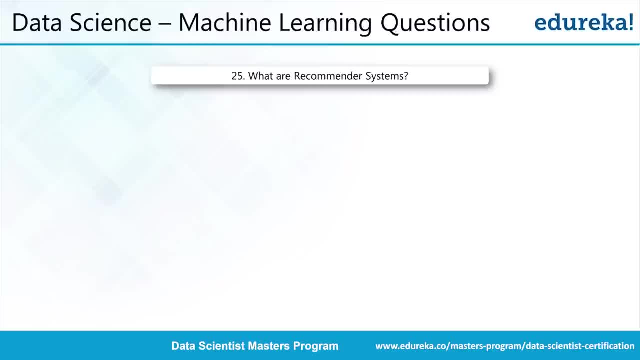 for Facebook. They will grow their network of people right. their connection between the users are going to go stronger and hence, obviously, the kind of ads that Kufa is Facebook wants to sell will also starts to grow right and more the users, more the connections, more is the sort. 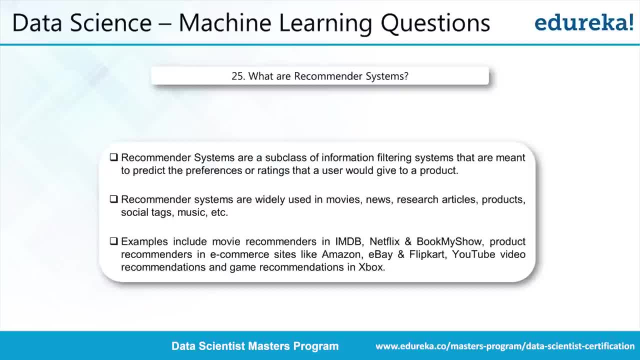 of interactions. you know about the connections as well as the behaviors that people show in a social network. So the fundamental idea behind all these recommender systems is to get a meaningful comparison between two users or between two items right for Amazon, between any two products. 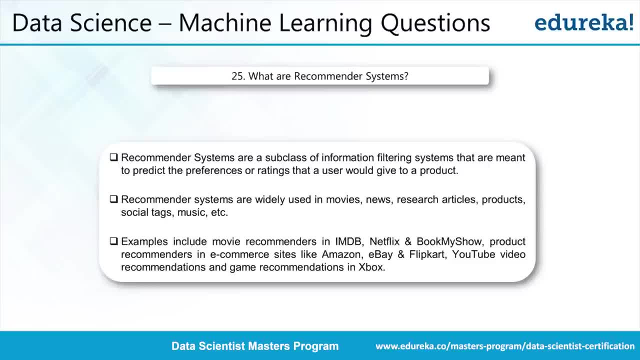 What's the similarity? if the similarity is really high, recommend that product to the for a given product in consideration. or if you find that two users are very similar in, let's say, Facebook, you might want to show to each other that you have another friend whom you might want to connect right. 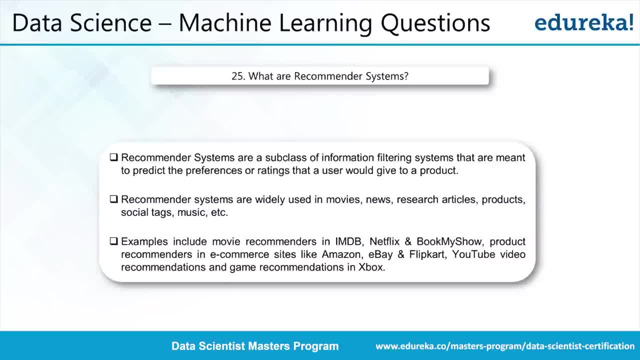 So there are, like many such use cases which comes out the moment you get into the deeper understanding of recommender systems. But the fundamental idea is: how do I compare two items- the items might be product, people, movies and so on- and how do we compare two users in simple terms? 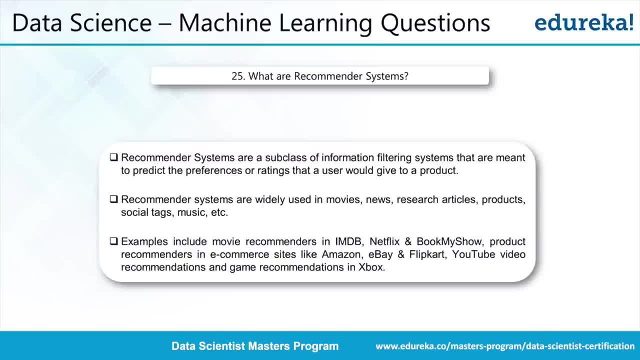 So this is what a recommendation system works on. So there are quite famous examples like the collaborative filtering approaches- user based collaborative filtering algorithms or the item based collaborative filtering algorithms. both of the algorithms are quite commonly used in recommender systems and nowadays people have also moved on to Latin factor based models. 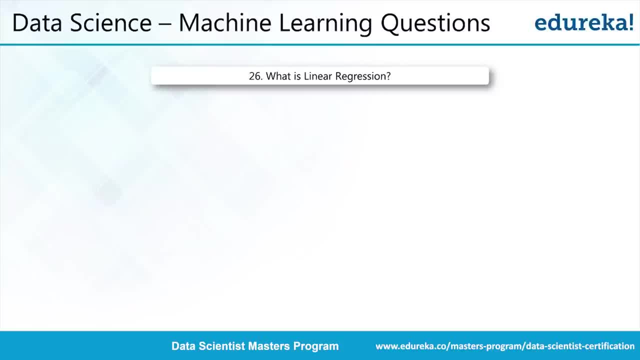 Like the SVD, single value decompositions and many others. So we talked about classification problem and then we said logistic regression is a binary class problem, right? So you might also be asked something around linear regressions: So what if I don't want to have a class of a particular user or a patient or something? 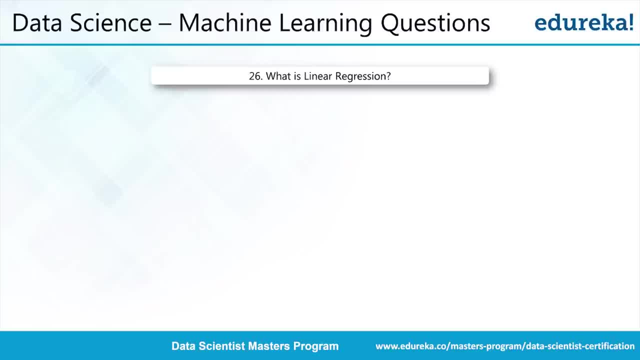 like that right, But instead, if I would ask you, can you give me a crisp value instead of a class right? So when I'm like classifying a given file into good, bad, Right, Which bad can be, virus, worms, frozen, These are the classes. 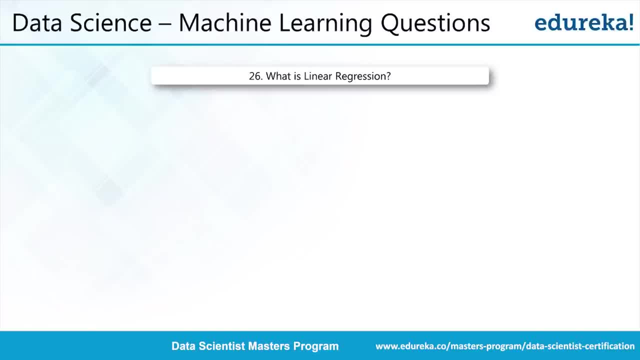 But if I don't want class but rather, for example, if I want to know the exact value of a house in a particular locality in my city, How do I calculate that right? So linear regression models and machine learning is one such technique which can regress over. 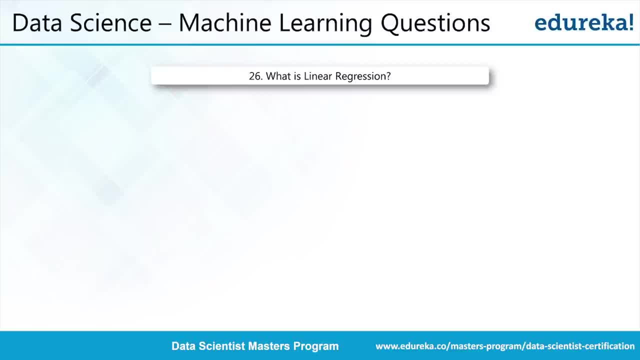 a given input data, which might include the properties of the houses, like number of bedrooms, the area in square feet and so on, and finally predict a value, a crisp value, Which will be exactly in terms of, let's say, dollar or in any other currency, the value. 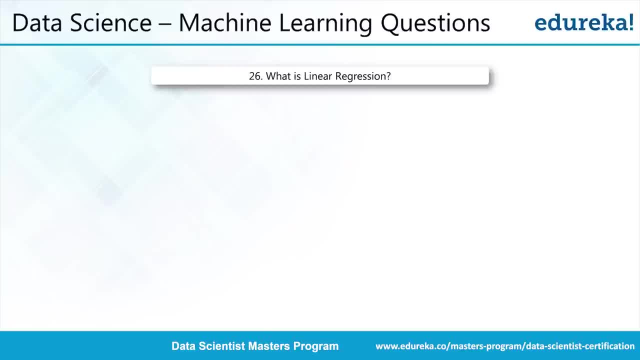 of the price, and the idea is, once again, that you have a training data with you which has labels. so from the past data, I know that, given these attributes of the house, what should be the ideal price of a house? I'll use that as my training data and then build my model for future. 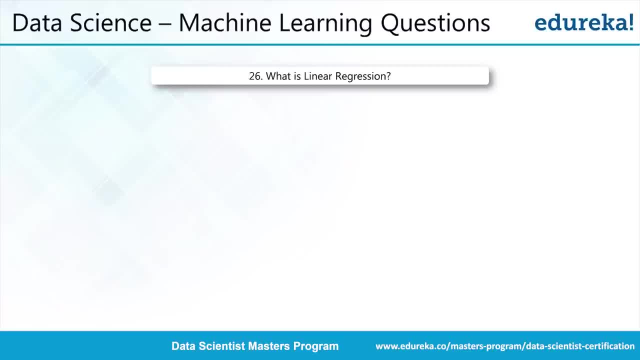 So now, with any such similar pattern in any data which is going to be coming in future for maybe our new property which is built in some XYZ location, I can use the model and predict exactly because these features are somewhere similar in that locality, the prices might be in a particular range. 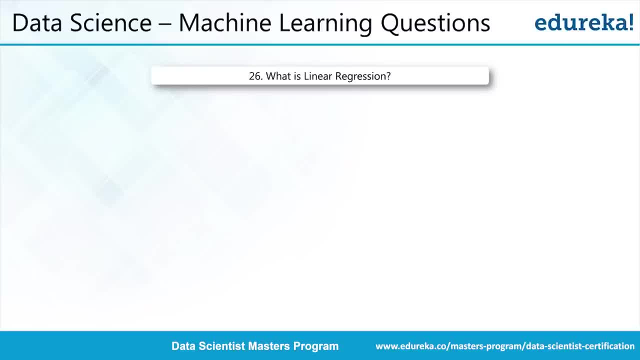 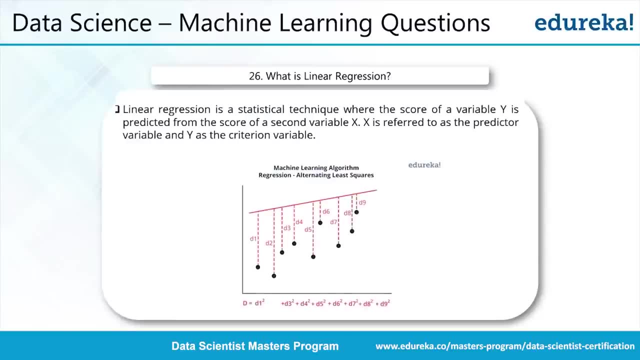 So a model like linear regression will learn those patterns in the given input attributes and try to predict the price of the house. right, and the idea is, if I have a set of data points, I want to build a very generic model, like drawing this line, which is as close as 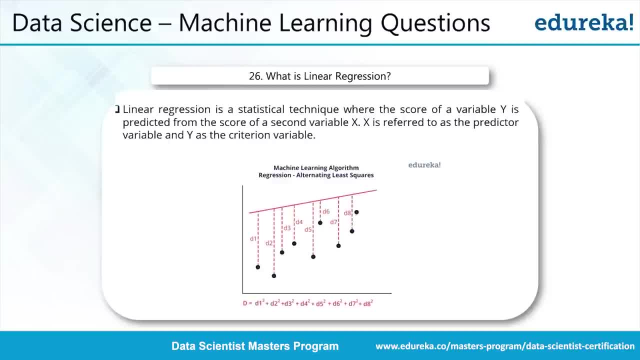 to all the points, right. So you can like draw infinitely many number of points if you are given a set of data points like this. So you can see here that I have a set of data points which is as close as to all the points, right. 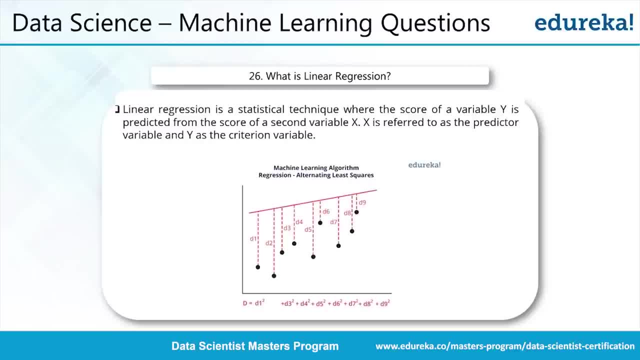 So the idea here is to fit a line passing through as closely as possible to all the data points that I have and minimize these so-called the error, which is nothing but the sum of all the distances. So there are simple linear regression ideas and the fundamental idea that we are following. 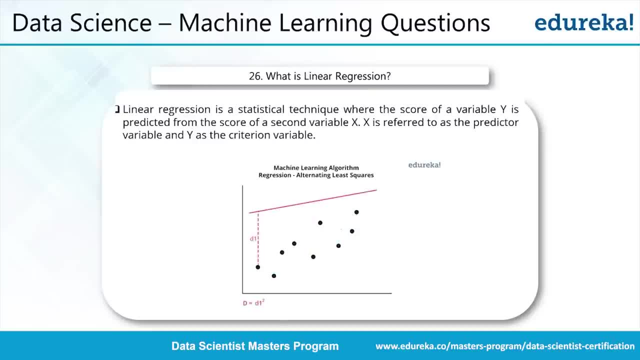 here is your variables are having a linear relationship, which means with the increase of one variable, the other also increases. but if you have a pattern which is not so linear in shape- like if you are like not able to draw a generic line, but the representation or the sort of points are aligned in a way that you can only create a model which is 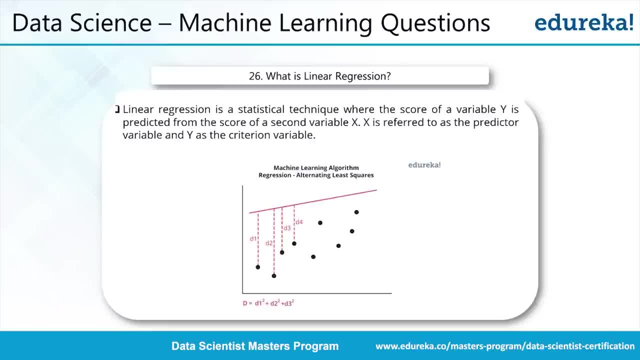 polynomial. So in that case, So the regression will not be so useful because the relationship is not linear anymore, right? So in that case you might want to go for some other regression approach, maybe like a polynomial regression, which has a non-linear relationship between the independent attributes. 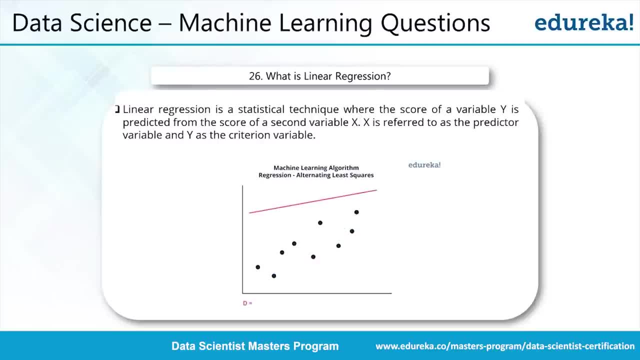 So quite a common approach and it has like a really large chunk of its explanation coming from the statistical ideas. Statistical ideas like hypothesis testing, p-values, confidence intervals and so on. So So what somebody is asking you around linear regression would be to start with saying how. 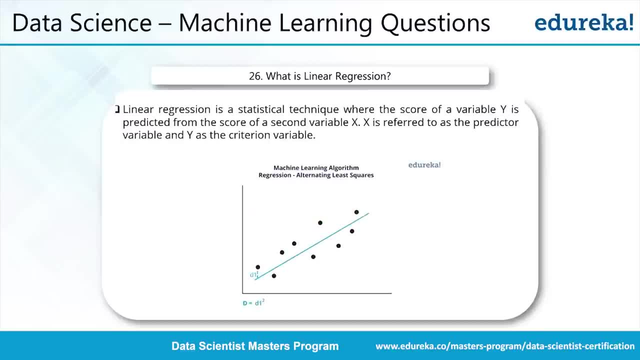 you build a linear regression model right, and then you might give some examples of it. So at best, if you're not comfortable with these ideas like p-value or hypothesis testings, you might want to refresh that before you like go for any interview because of linear. 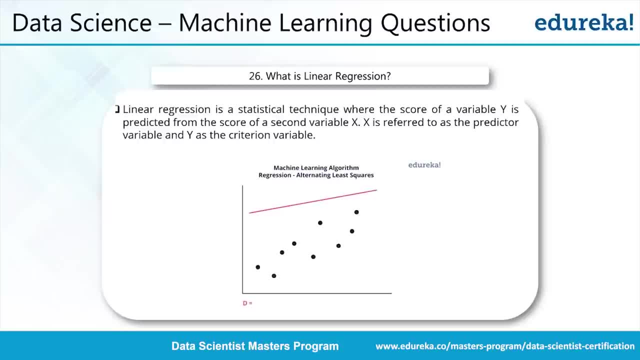 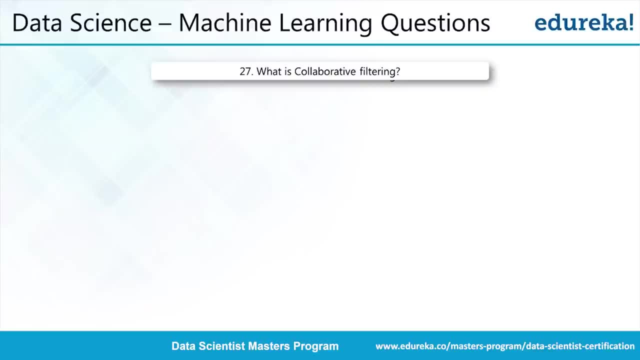 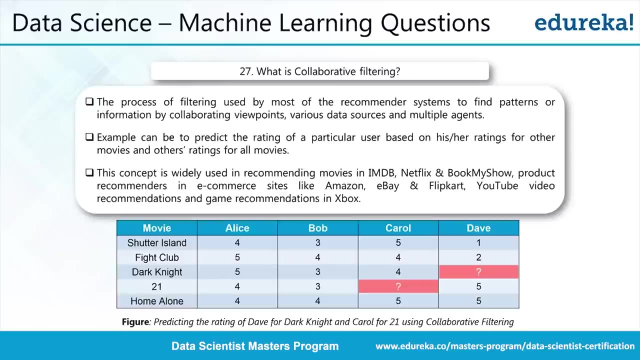 regression comes up. these concepts needs to be a bit more explained, right? So when I talked about the recommendation algorithm, I mentioned something about collaborative filters, right? The user-based collaborative filtering or the item filter? Right? So these are the two commonly used sort of recommendation algorithms, right? normally referred. 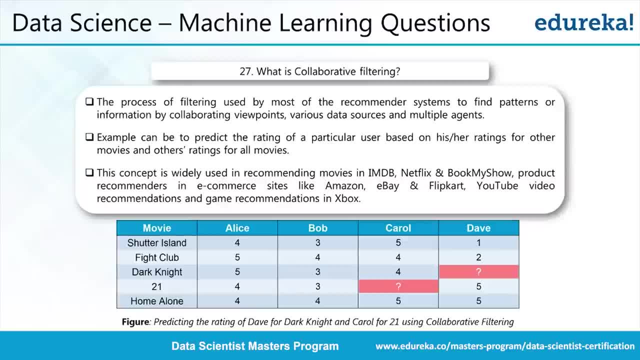 to as item based, so IBCF and the UBCF, and the idea, as I mentioned, is to compare to users or to compare to movies or, let's say, items in particular. so the item can be anything- a product, a movie or a person- and the sort of way it builds the model is given lot of. 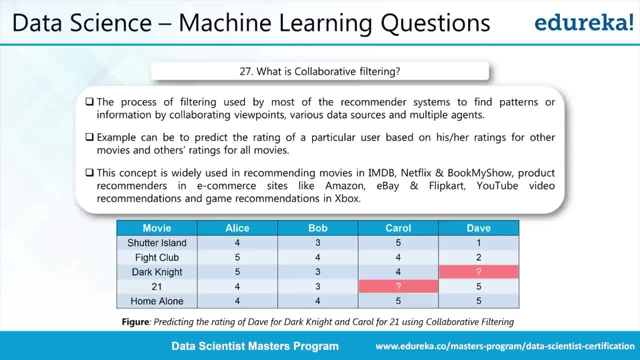 users. So let's say a particular, let's say in this example the rating to a movie. we now need to find out. can we recommend for some users, based on the behaviors of other users or their ratings to the movie, some suitable movies or not. So for example, here for Carol: Carol has not seen the movie 21 right. 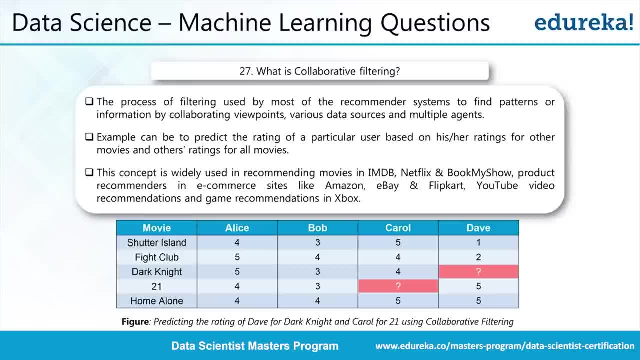 So there is a question mark there. So can I predict this value? if it comes to be, let's say, like close to two, I don't recommend the movie. but if it comes to, let's say, somewhere three, four or five, Yup Carol says yes, recommend this movie to Carol. 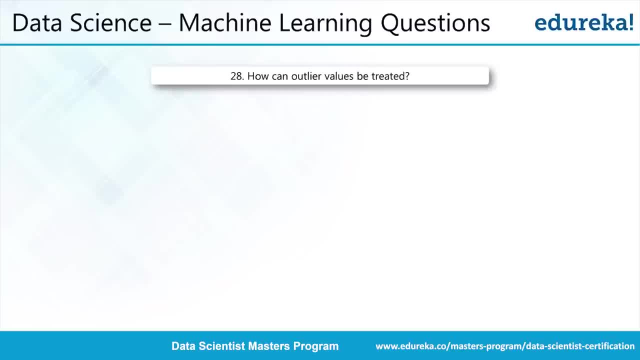 Okay, So one more fundamental problems on when you build the models. So, as I mentioned in the earlier discussions, that when we are doing some analysis with the data after you collect the data there requires a lot of cleaning right and exploration as well. So in that process of cleaning and exploring the data sets, you might often find there are 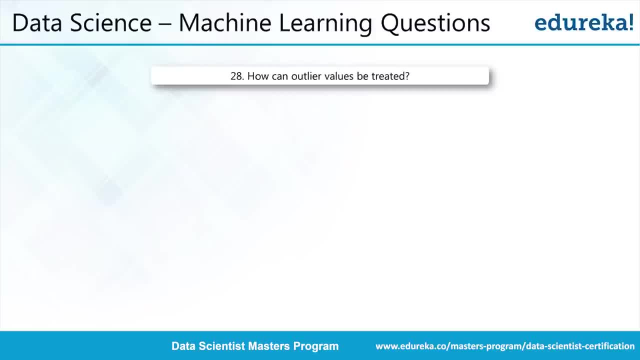 some extreme points. So, for instance, if I'm building a regression model for predicting the house prices and there is this one house Which somebody has sort of able to sell for a very high price by means of maybe some auction or some other sort of marketing gimmick, there the point might mislead the model to predict. 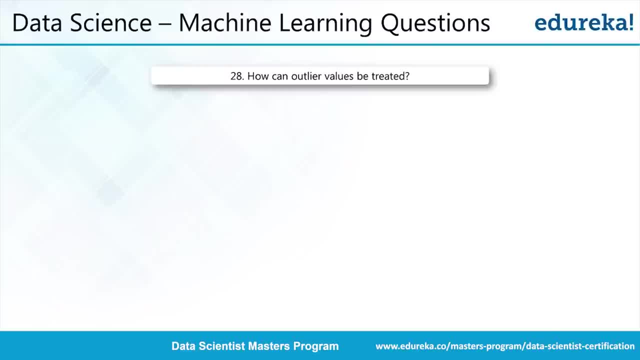 or get itself towards that outlier point, right. So we don't want to like move towards an outlier point, but we need to deal it separately. So if you don't have a better explanation for why that outlier is in terms of an input attribute, better is to remove it. 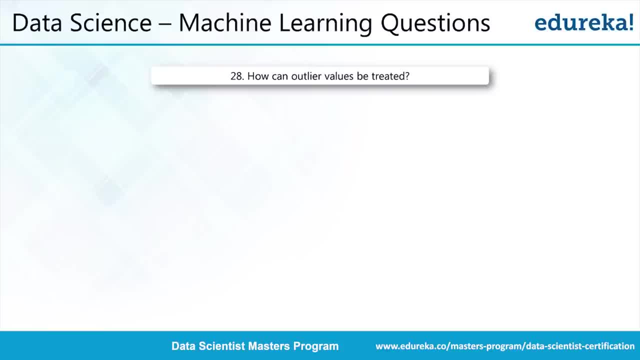 So, for instance, Like analyzing any data in an e-commerce world where I am going through all the products and the sales that the product has seen in last one week and on the last one week there was a particular day when a kind of a sales day was there, like nowadays e-commerce companies. 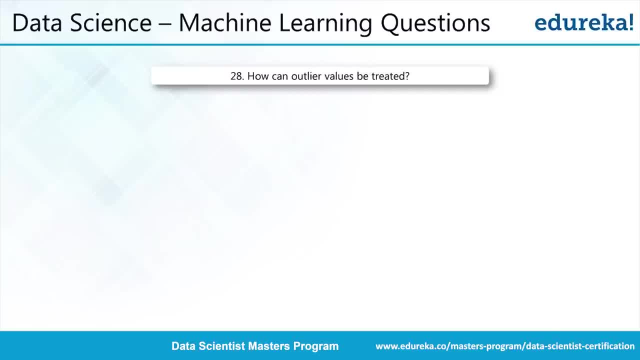 do this a lot, but in those sales days you would obviously expect that the products purchase is going to go very high, right, but does that mean that it's an outlier to me? not, because if I am able to explain an outlier by saying that this was a discount day, I might be able. 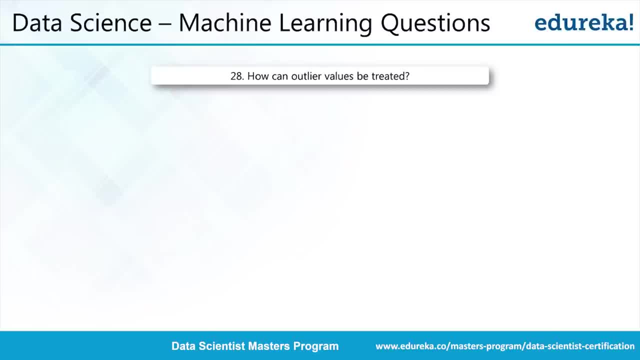 to handle it separately. either I can like simply take all those points which are for the discounts day or sales day and keep it separately, or if I would like to have the variable, like saying whether the given day is a sales day, and keep the outlier as well. 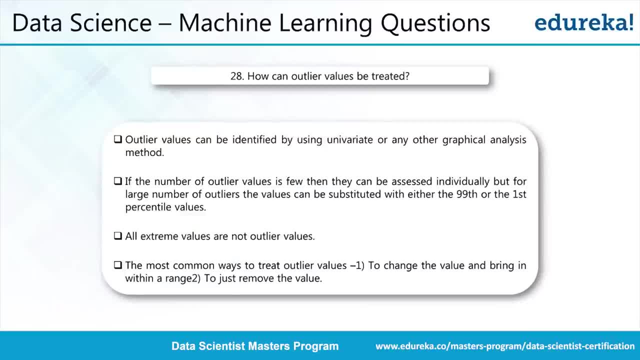 then the analysis goes in a different direction. So it's important you handle the outlier before you start to build your model or do any analysis, otherwise your insights or your models output might totally give you a different direction And there are very different. Okay, 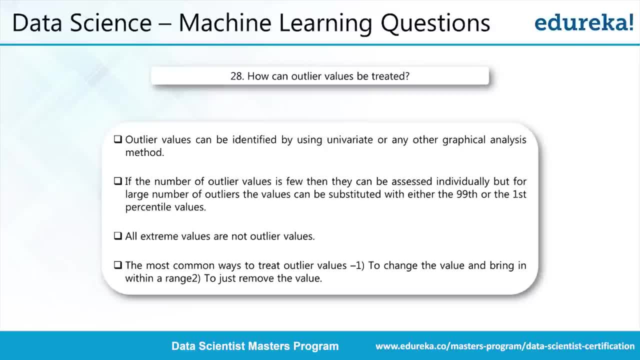 There are different ways to handle the outliers. So some people use approaches like removing any data points which is like outside of the range of mean plus three standard deviation right. or sometimes people also use the percentile way of doing it: any point which is greater than the 99th percentile can be, like removed. 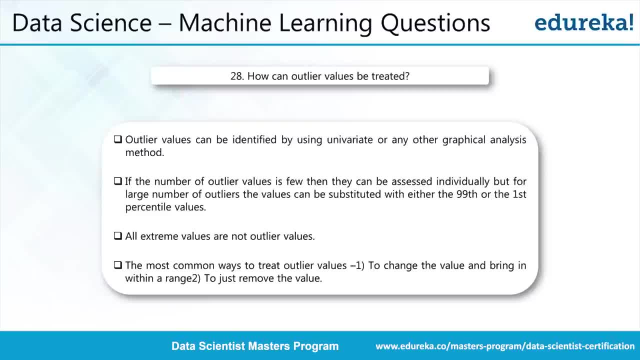 So these are like you are removing the toppers from the data points of yours of, let's say, a SAT examination or a CAT examination. So the outliers Sometimes can cause certain issues in explaining the model. so you can obviously imagine this in very intuitive terms. also, if you have a set of scores for candidates who appeared, 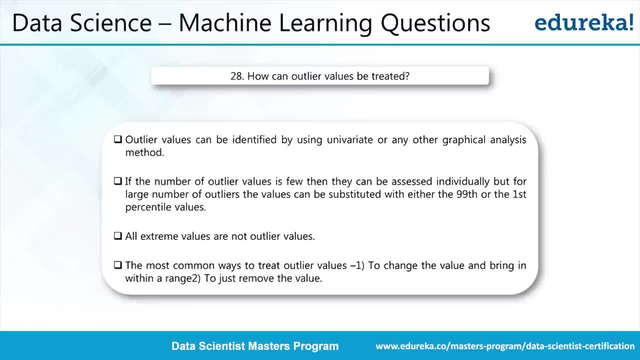 for an examination and there was one outlier candidate who scored really, really high. So do you have a way of explaining that outlier? you might be simply calling that person a talented person, but does that like explain the model may be difficult, right? So better is to keep those exceptional cases separate and do the analysis with the rest. 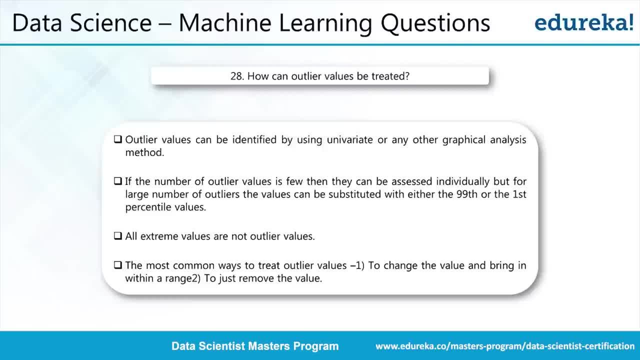 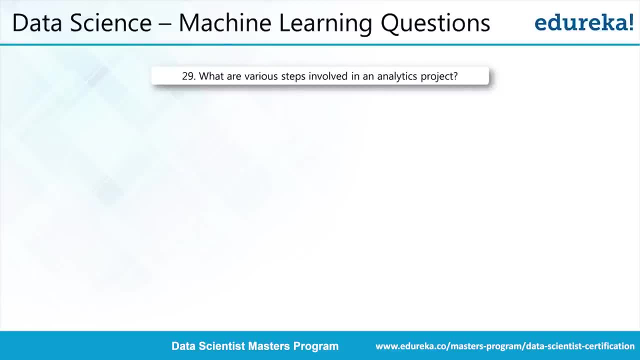 of it. So which gives you the good pattern, The good insight from a data. So that's how you like normally handle an outlier right- and this quite often is an important question- to answer that, if you are given an analytics project with lot of data, how do? 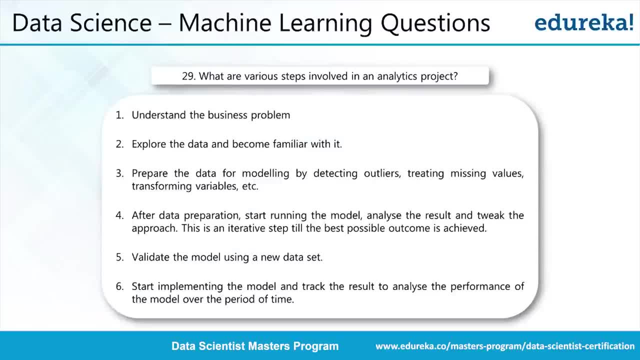 you normally approach it right. In typical cases, the first step is to really go deep, dive into the problem in hand, and the problem needs to be defined very crisply. So no, never define a problem which is broad in sense. So, for example, I'm building a model for customer segmentation using a clustering approach. 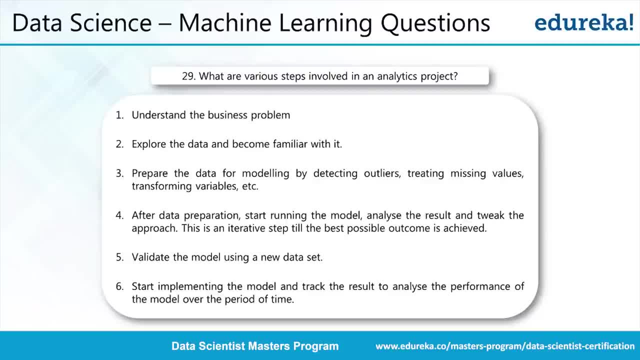 So instead of saying: build a customer segmentation model for all the categories of products, that can be like a broad problem. But if I say build a customer segmentation model only for fashion category of products, right, then the problem becomes crisp. So defining a problem statement and its understanding is the foremost task. and then comes the kind. 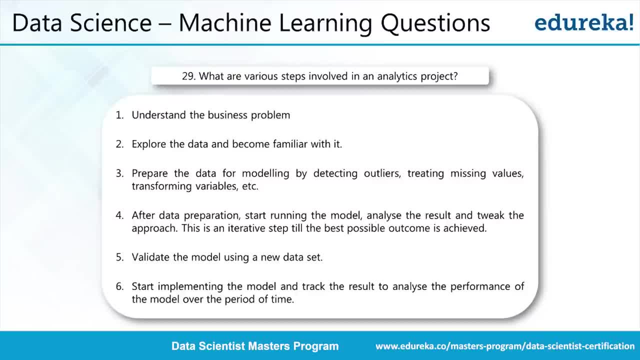 of exercise, of exploring the data, in which you will identify outliers, missing values and if you need any transformations, Like converting from a log format to a wide format or the vice versa. you do all that steps in the second and the third step and once we have found out that the data is very good, 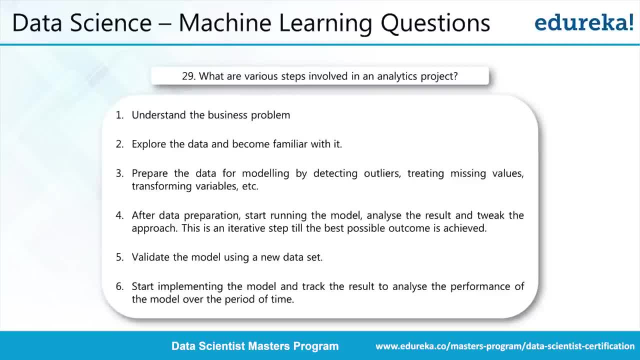 now, after we have removed all the outliers and the missing values and so on, you then start to understand certain relationship like given in input. attributes relate in some way or the other right. So this is a stage where you start to prepare for any further inside building exercise or 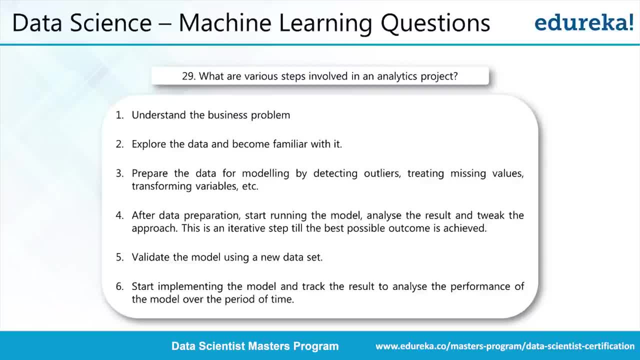 like model building exercise And let's say, if you build the model in this step, the immediate step is to validate it right, whether the model is really good or not, by using a testing data right. and once let's say all of these is done and you are either coming out with a insight or a model. 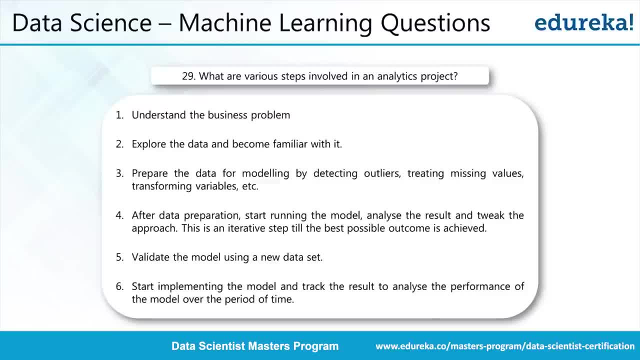 you would like to see in long term how this model is going to perform. So it might happen. so, because every model is not static, your data is growing on daily basis, so if you want to build a really robust model on a growing times, It should append. the model should update based on the new data which is available. right, 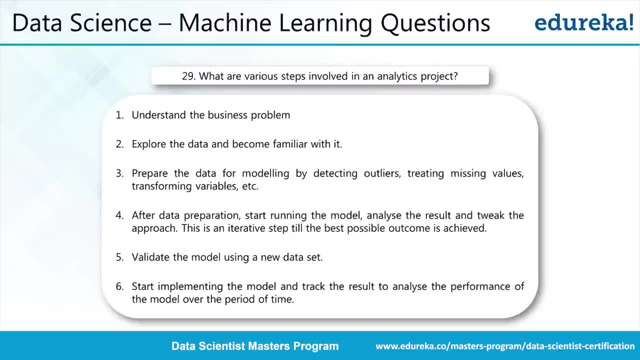 so over a period of time. you should track and analyze how good the model is performing on a real world data, and if the performance is going down, then it's time to retrain the model and maybe come out with an updated model on the data that you are already given right. 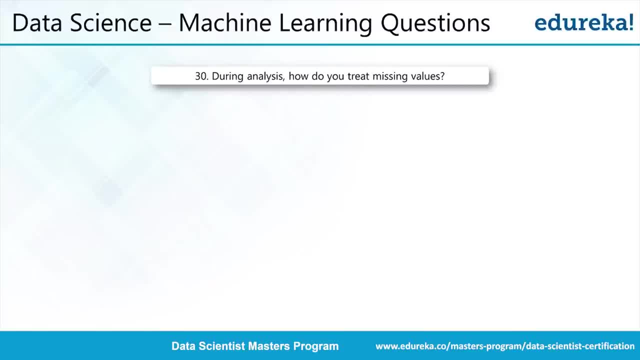 okay, so one more task. as I was explaining in the cleaning process, how do we treat the missing values? so there are quite a number of techniques to do that. So, for instance, if you have an attribute, let's say age right, and you are analyzing this age in various segment of people: a people who are teenagers, people who are professionals, 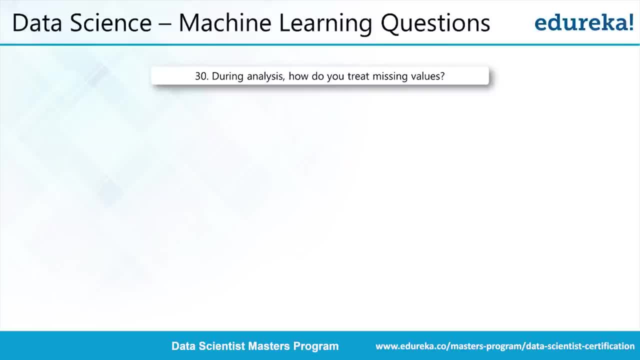 people who are still in their college and so on. right, and there is one value missing in one of these categories of people, let's say teenagers. So if the age is missing, because I know I am analyzing a group of people who are teenagers by looking at the average age in the teenage group, right, 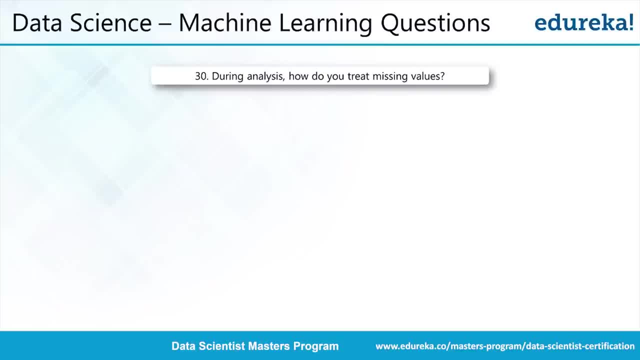 I can maybe impute a value. So instead of discarding the entire row because I don't have the value of age, I might be able to impute it by some simple measures like this: calculating the average in that group and putting the value there, which will not be completely wrong, because I know there is. 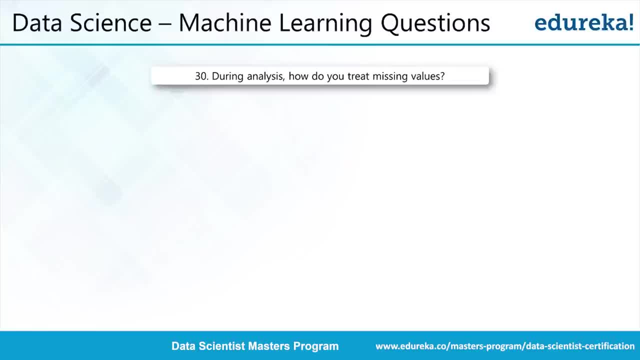 a very strong evidence. teenagers would be more or less in the range of, let's say, 16 to 20, right? even if I am wrong in my average calculation, it might not be so high. it might be like just plus or minus 1 or 2 years. 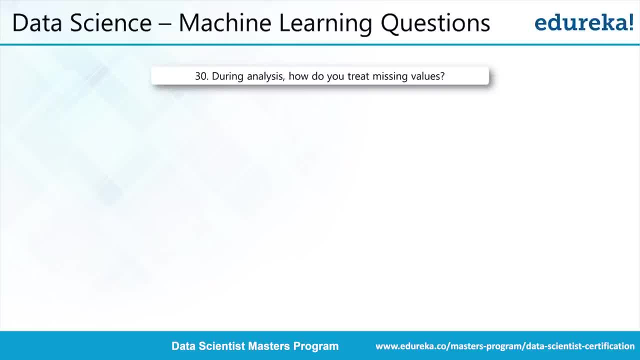 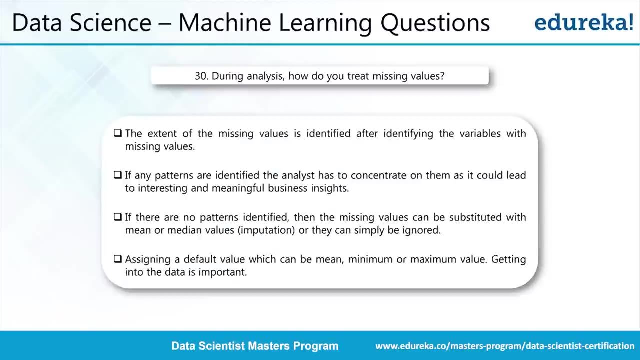 So, which I am like, fine with if I want to keep my data retained. and you might see that in your many applications sometimes having a kind of discarding a particular row because of missing values might be very costly, because the data is limited in number. So that's why people normally do this out of sort of mean minimum or maximum kind of. 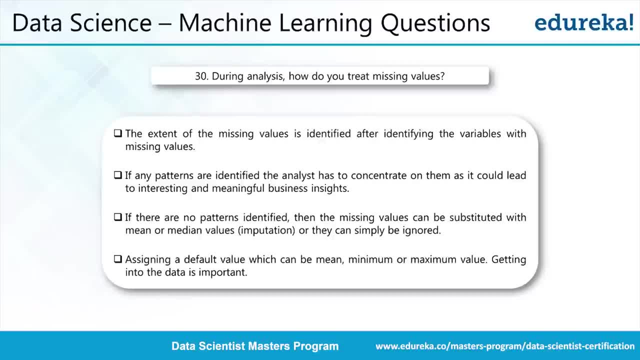 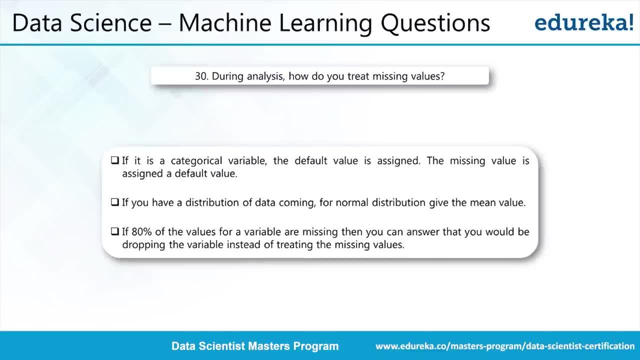 a value, or they also calculate the average and impute the value there. So there can be some other pattern based imputation also possible. but I'll just give you an example. And in other cases, if nothing is possible by putting a value, if everything is going, 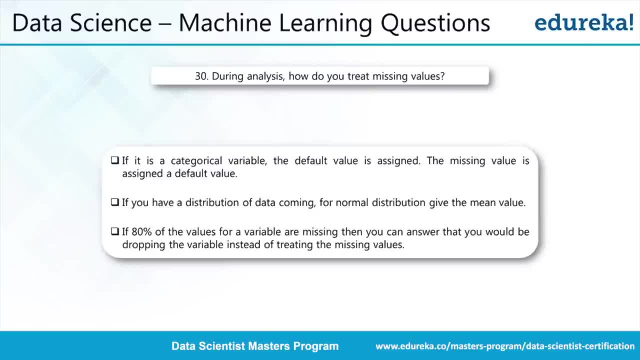 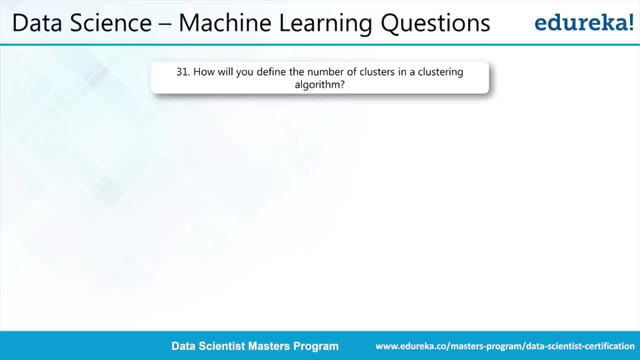 to be misleading, then better is to like remove that, but that can only be done if you have a surplus of data with you. If not, then be cautious of removing any values, particularly the missing ones. ok, So this question particularly pertains to a machine learning algorithm called k-means. 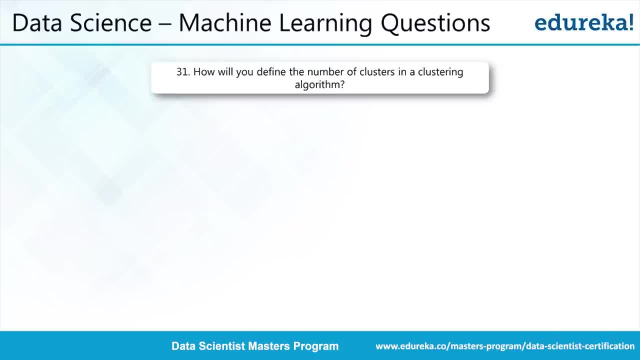 right. every time you run the algorithm you have to define what should be the value of k, right? So there are approaches like elbow curve, Which plots the kind of a plot, scatter plot- between the x-axis, which is the number of clusters, versus y-axis, which is the WSS, or within sum of square, which is also known by. 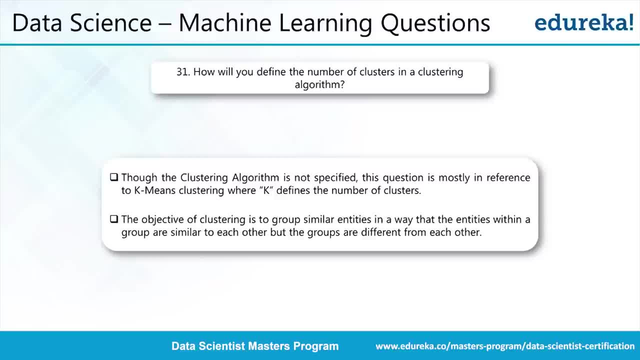 the name distortion. The idea is, when we are building the k-means clustering algorithm, if we find at one point- if you like, keep increasing the value of k, then one point, we find that the distortion is low, which means the distance between the data points within a cluster is as close as 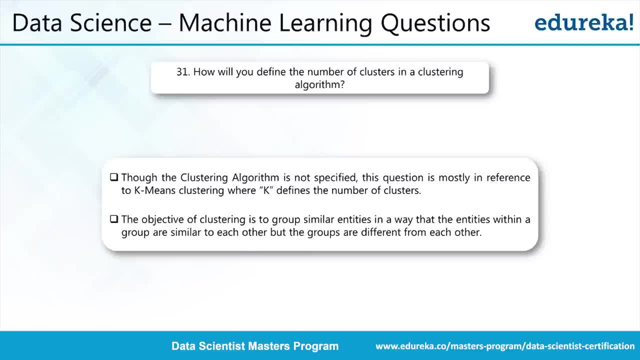 possible and the distances between two cluster points, like a point in cluster one and a point in cluster two, is as far as possible. So if that's the case, then the distortion will be like very low. but if your points inside a cluster itself is very spread out and your clusters are very close to each other, then 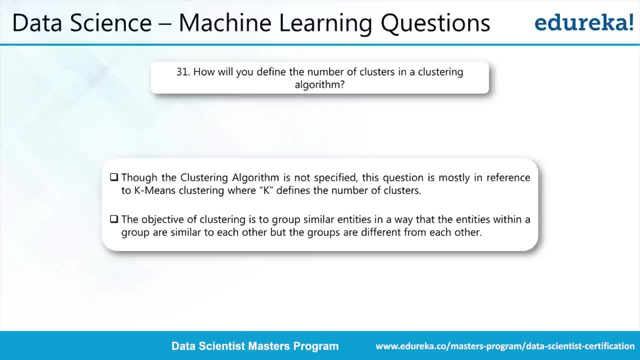 the distortion is going to be very high. So in those cases the value of k needs to be maybe further increased and at one point, using an idea called an elbow curve, which will show you a small kink from where there is a A sharp dip in the distortion values and that is an appropriate value for k. while we are, 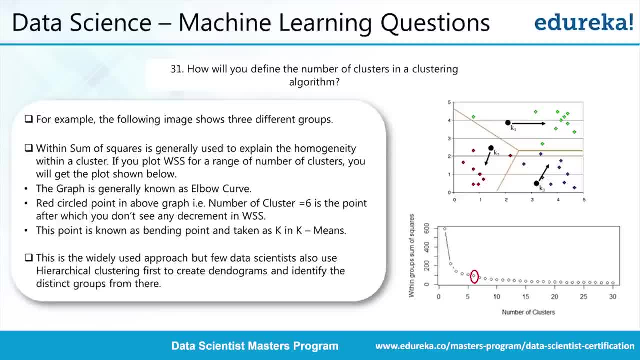 building a k-means algorithm. So this is how it looks like. So you can see here the x-axis is the number of clusters and your y-axis is your within group of sums of square. and at one point you can see there is a sharp dip here. here and 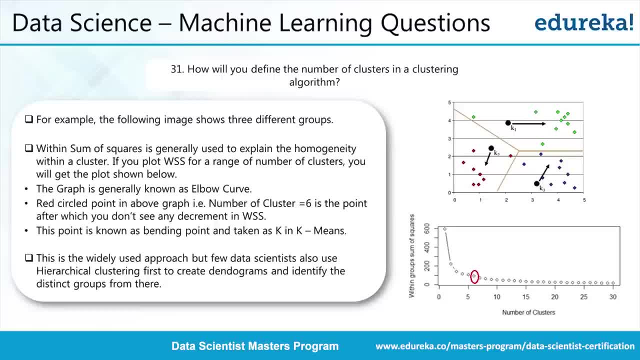 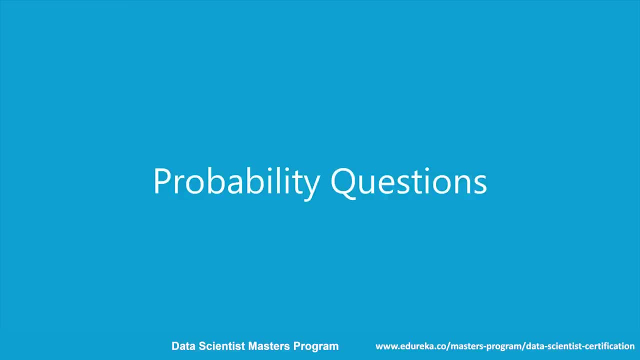 after this point, which is like circled in red, the values sort of almost saturates. So this maybe I can use as the appropriate value of k. so value of k can be like 6 in this case. So I hope you are now getting comfortable with questions around data analysis statistics. 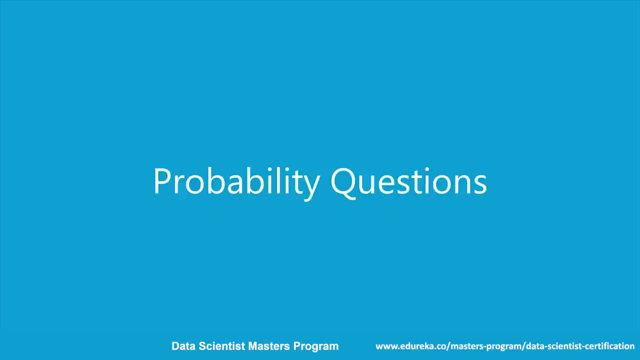 and even the machine learning part. So the next pillar, which might very closely be associated with statistics as well, is around probability right. So it is like in sometimes in most of the standard literature, probability and statistics comes together. that is now inseparable anytime. So in the name base algorithm like this is one of the machine learning algorithm which 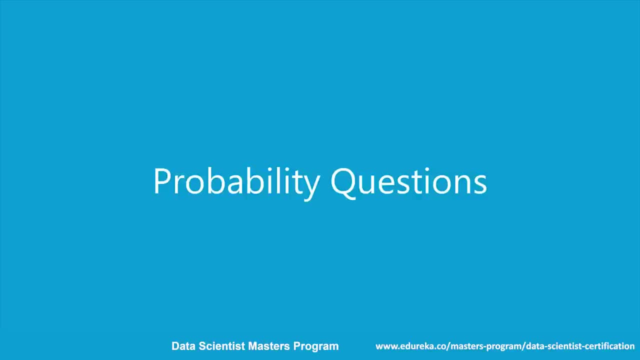 is based on the Bayes theorem. Probability ideas are quite a lot used and there are some really niche probability concepts like the probability graph models, which is actually based on the basics coming from Bayes theorem and the fundamental properties around probability. I will not go to that detail of probability in interview questions. if you have an expertise. 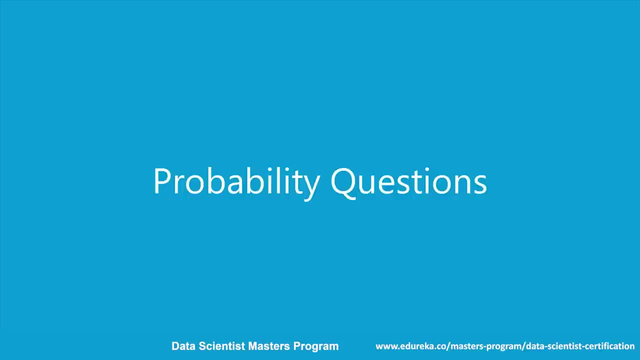 around probability and probability graph models or name base kind of algorithms. I feel like confident to speak about it, But most of the time Probability questions are quite basics and fundamentals, like the one which is asked in interviews, depending on, obviously, in which place you are giving the interview at. 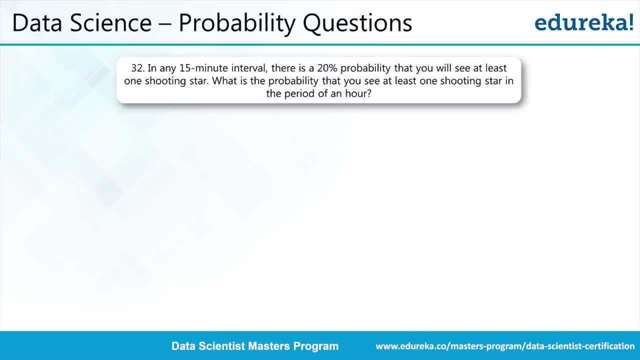 So let us also like see some sort of approach in attacking a probability problems. ok, So I will like read it out for you what the problem is here. So it says: in any 15 minute interval there is a 20% probability that you will see a shooting. 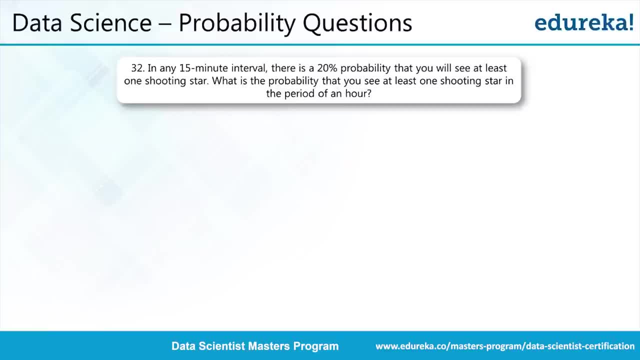 star, like a good example rather. So what is the probability? Probability that you you see at least one shooting star in a period of an hour. so there is unknown information given to us that every 15 minute interval there is this 20% probability, you will see at least one star. 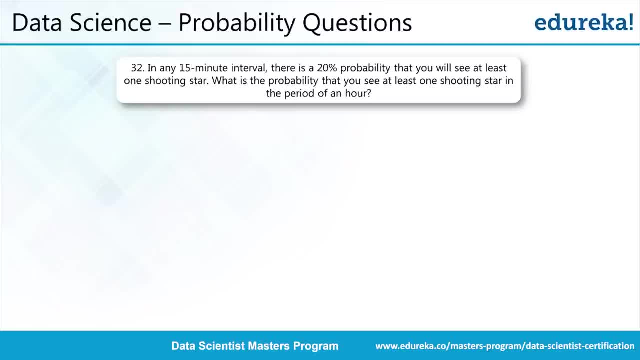 So we now want to calculate this probability in a period of one hour, right? So what is the sort of approach we would take here? So let's build this systematically. so we know one fact: that probability of not seeing the shooting star In every 15 minute interval is 20%, which like comes down to 0.2 in probability terms- 20%. 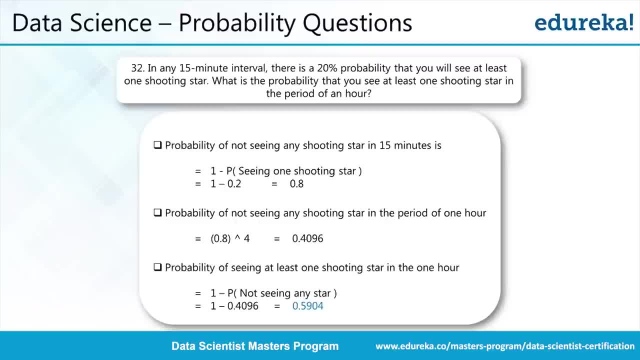 chances, or 0.2 probability, and, as you know, probability is always between 0 and 1.. So if I would like to calculate what is the probability of not seeing the shooting star in 15 minutes, which is like the opposite of this right, 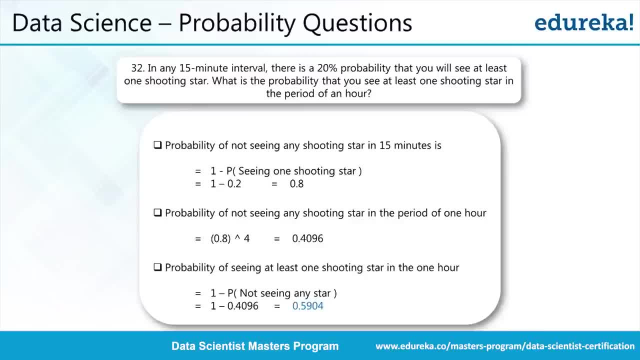 If I take from. so these are like independent events, right? so if I take 1 minus of the probability of seeing one shooting star, 0.8 will then become the probability of not seeing the shooting star in 15 minutes interval. ok, what I need to do is then probability of not seeing this shooting star in another one. 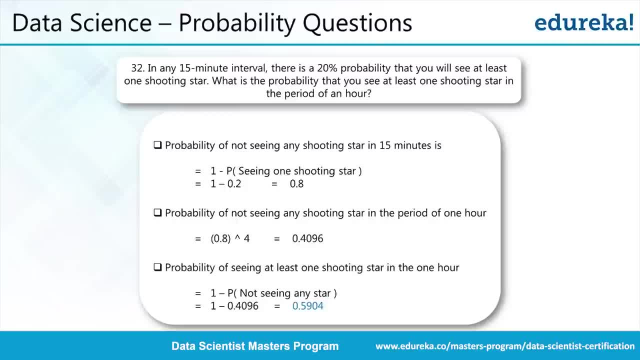 hour, because these are now independent events, like seeing a shooting star in first 15 minute interval, the second and third and the fourth in an hour's period is independent of each other. we can multiply this probability like this: so 0.8 into 0.8, into 0.8, into 0.8, which. 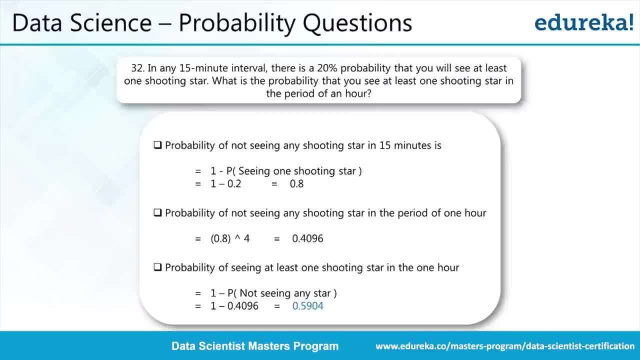 comes down to A value of 0.4. so the probability of not seeing the shooting star in an period of one hour is 0.4. right, and if we know the value of this probability here, all we like have to do to get the value which we are interested in is, which is the probability of seeing the shooting. 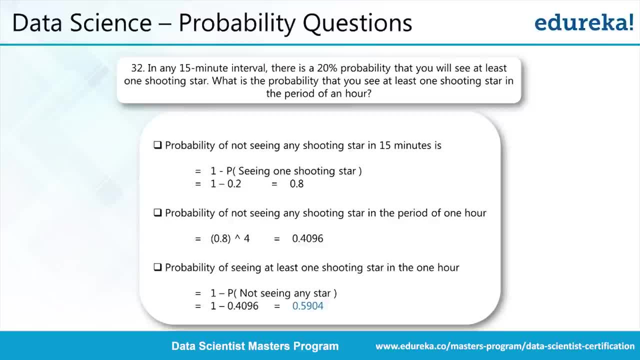 star is 1 minus the probability of not seeing it right. So the probability here comes down to 0.5. quite a simple approach in terms of how it works right. So there might be like similar tricky ways to calculate the probability of not seeing. 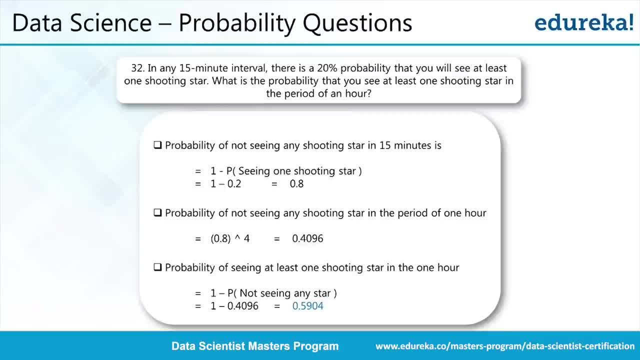 the shooting star in another one hour. But if you know one approach and having the idea of independent event is right, you may be able to get the understanding or like formulation in this way and also keep in mind, given a sort of a sample space and many events from the sample space, the sum of the probabilities. 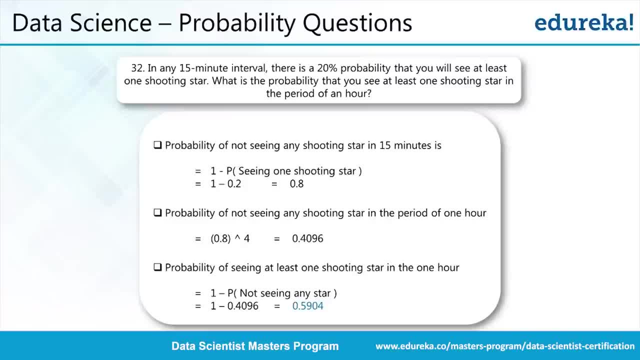 cannot exceed one right, so that's why we are able to do this. if I am saying tossing a coin, the probability of tail is going to be 0.5.. Ok, And the probability of head is going to be the other event which is going to be 1 minus. 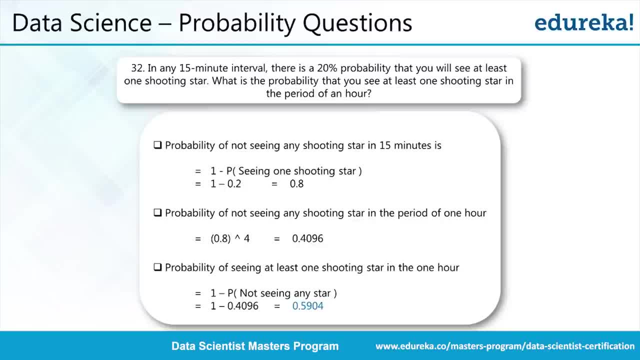 the probability of tail right. So similar is the case with here as well. we are like treating this as a binary problem. So depending on which problem you are going to tackle, the approaches are going to be the same, but the language and sort of the trickiness in the question might increase, right. 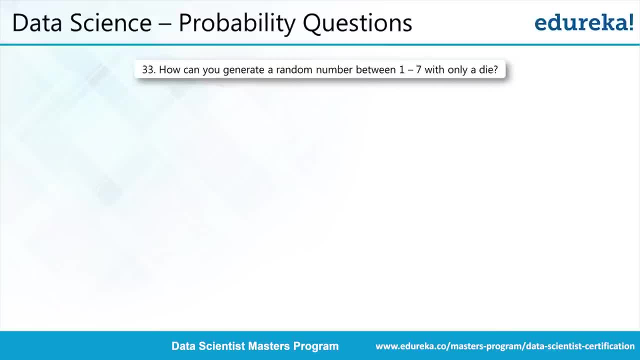 So this is how you can attack that. Ok, so there is this one more question, which is around generating a random number between 1 to 7.. Ok, so let's also think about this, how we can like approach this problem. So we have like seen how we generate random numbers from a given set of points, but this: 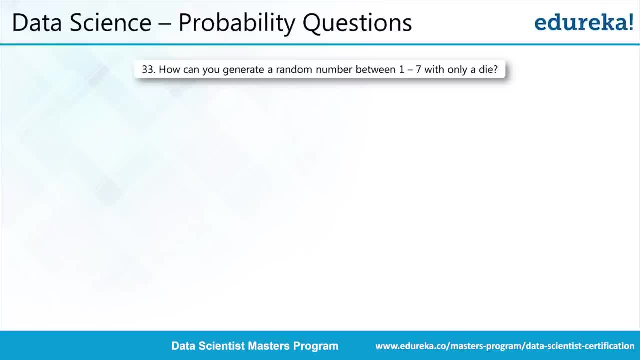 kind of says that we want to do this with a die right by rolling a die we want to find out a random number between 1 to 7.. So obviously we know that the die has numbers between 1 to 6.. So the probability of getting any one digit in the die is 1 by 6.. 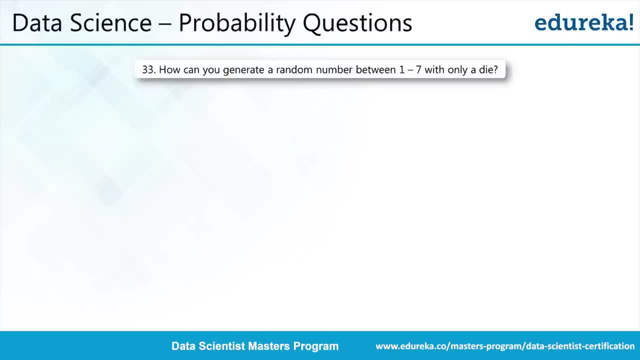 So like if I do 1, 2, 3, 1 divided by the total number of possibilities, that is, 1 by 6.. So that will be my probability of choosing any one of the digits there. but it is saying it is we want to generate this random number between 1 to 7.. 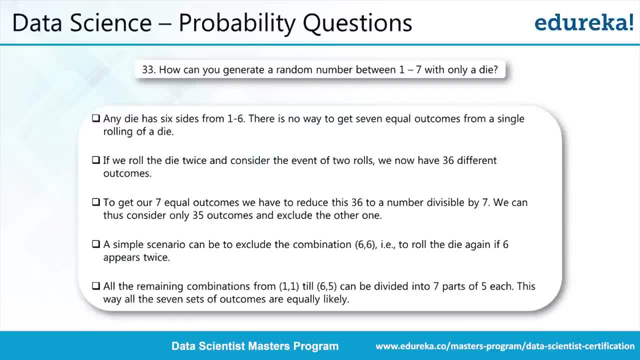 So where do we get the 7.? So obviously the requirement is that we can like roll the dies twice, right, then the number of possibilities increases. So, as I said, there is no way we can get the seventh one right, because we have only six digits. 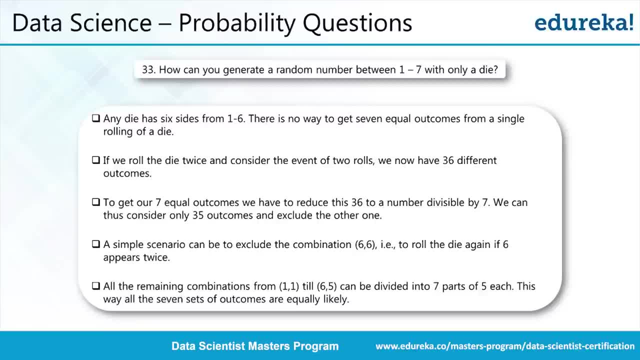 So if we die twice, the number of possibilities of generating this seven random numbers increases. So in this case we have now 36 different outcomes possible. You can like do the match there, which is nothing but 6 cross 6. so 1, 2, 1, 3, 1, 4, 1, 5, 1, 6 and for: 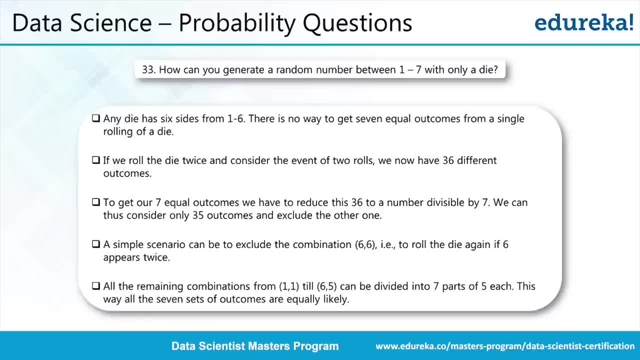 the rest of the digits the same way. right, 6 cross 6.. So that's the different number of outcomes we can get. So now for us to get this 7 sort of random numbers, and imagine that this idea actually relates to Sampling technique as well, when we say we want to get the numbers between 1 to 7 all. 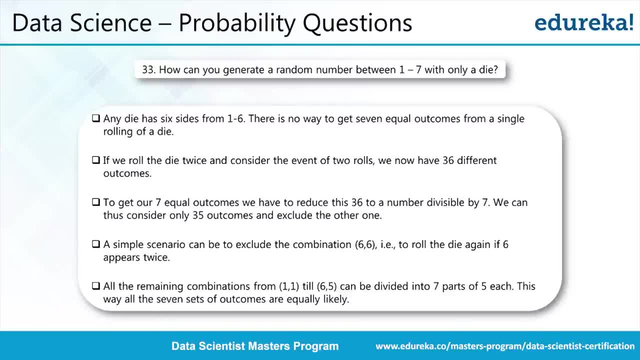 of those numbers should be equally likely, right. otherwise it will happen that I might get one and maybe quite a number of times, versus one particular digit. like to only once or so on. but if I want to do a very good randomized selection I need to be making sure the probability 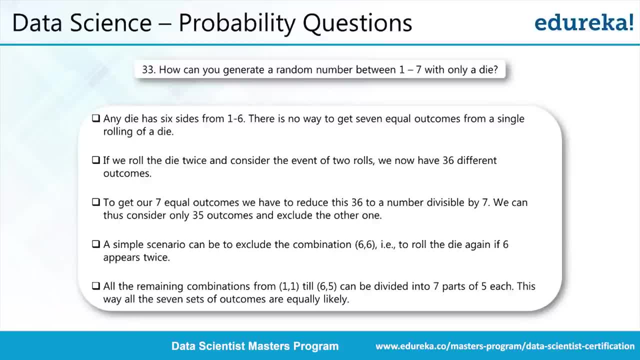 of picking any one digit between 1 to 7 is equally likely. if I am not doing that, I might have a bias Right. so we have this: 36 different outcomes. so how do we now make sure that this is like kind of equally likely? 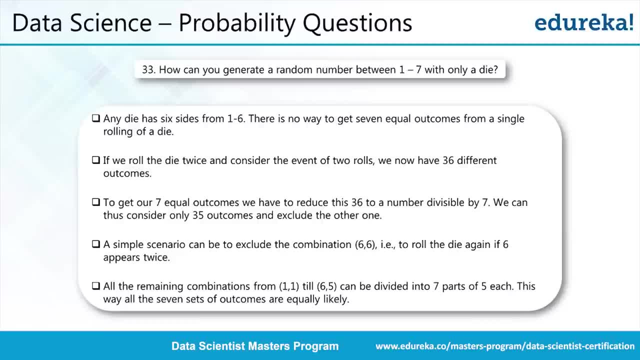 So first we have to like find out a number which is divisible by 7, which is close to 36, so maybe we can exclude one of the possibilities from the 36 combinations we have and keep only these 35 possible outcomes, So like excluding maybe 6 comma 6, this possibility. if we remove we are left with the remaining. 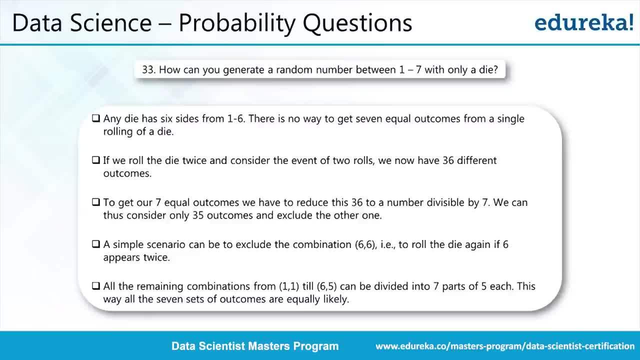 35 possible outcomes. So, with this one reduction in the possible outcome, all we are left out with is all the possible combinations, starting from 1. 1 till 6, 5. right now, if you divide this into 7 parts, where each like contains 5 possible outcomes, so what will happen is with the 7 parts each. 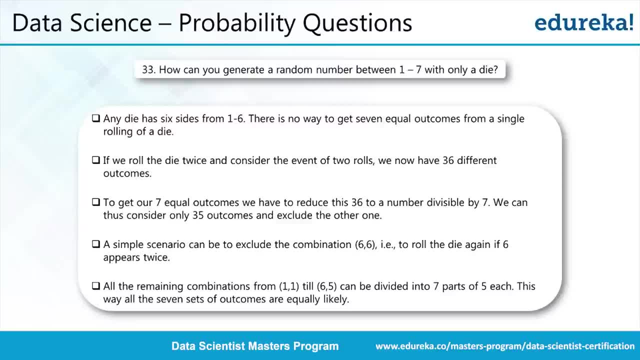 having 5 outcomes. whenever any one outcome comes in these 7 parts, I am going to assign a value to it. So, for instance, if I assign The first 5, because we are going to divide it into 7 parts, where each part will contain: 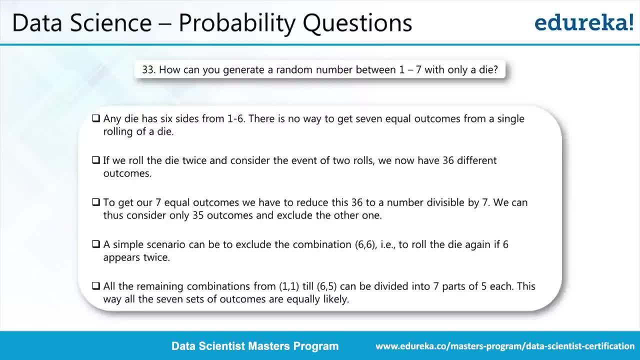 5 possible outcomes. so maybe the first 5 outcomes I will assign to the part 1, so whenever that 5 of that 5 outcomes comes up, I will say the random number which I have generated is 1.. In the second part I will keep the next 5 outcomes and whenever that 5 outcomes comes, 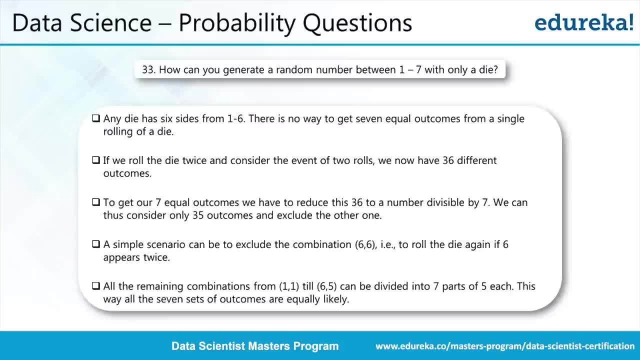 in rolling these 2 dice, I will assign that a value to, and so on. So this way, what we have done is we have made sure that the random number That we are picking between 1 and 7 are equally likely. if you don't do that, then there will. 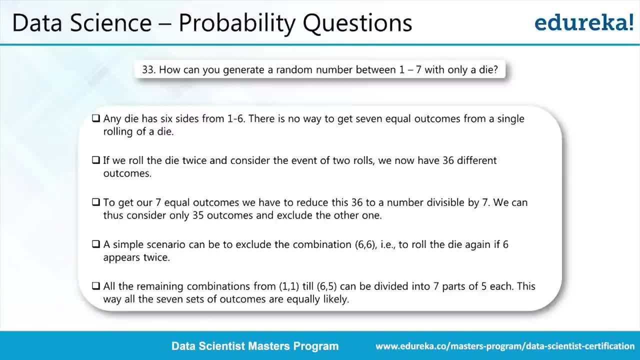 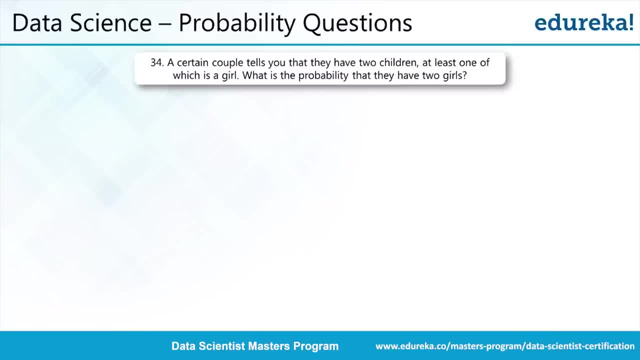 be a bias. so you see here how sort of a statistics is like, merged with the probability that this is how the 2 ideas and subjects travel together. ok, so one more question on the same line. so for instance here, if you have a couple and let's say they have 2 children's, so at least, 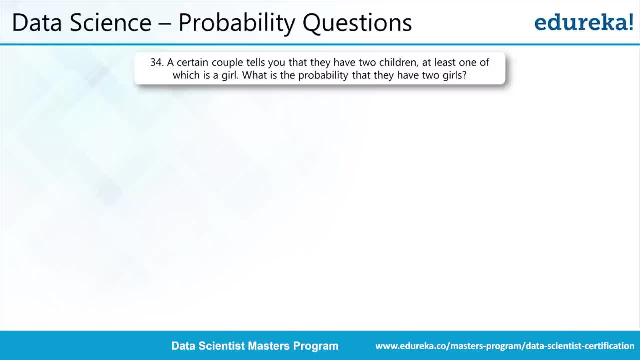 one of which is a girl, so this is a given scenario. so the question asks you: what is the probability that they have 2 girls? Right? it becomes a bit more like tossing 2 coins problem, right, where there are different combinations. so what you can see here is a couple has 2 children, so at least one of which. 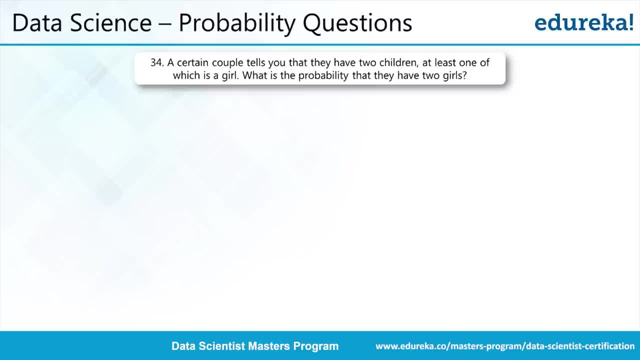 is a girl, so we have a known fact with us. so now all we need to do to kind of calculate this probability is to generate all the possible combinations: the first child being boy, the second child being girl, the first being girl, the second being boy, and so on. right, if you? 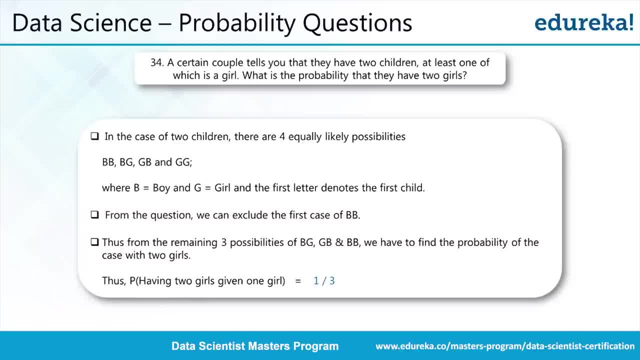 write that down. this is what the possible combinations are, and both- all these 4 are equally likely, as you could see. so with this case we have, like in the question, at least one of the children is a girl. so that means only 3 combinations are left out. 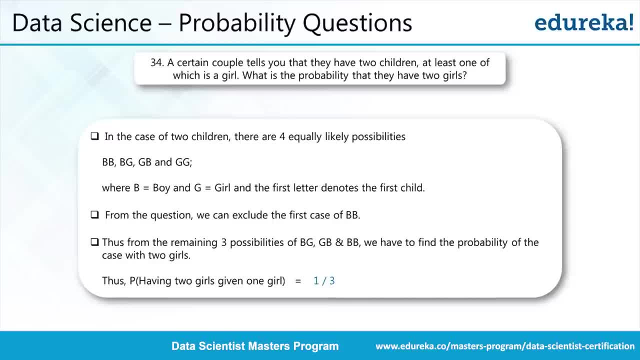 with us. the combination where both the children were boys is excluded. so in a very simple manner, you can like just go ahead and calculate: the probability of having 2 girl childs will be 1 by 3, so there are total 3 possibilities, which comes in the denominator and you have 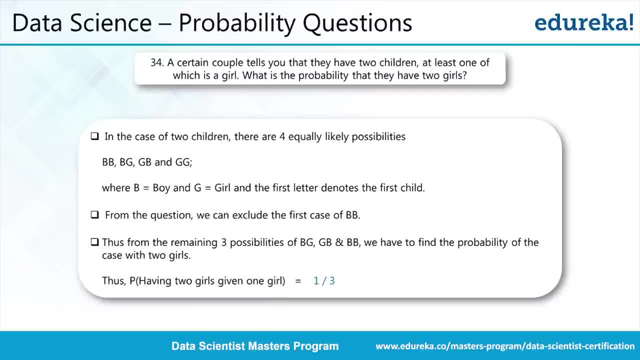 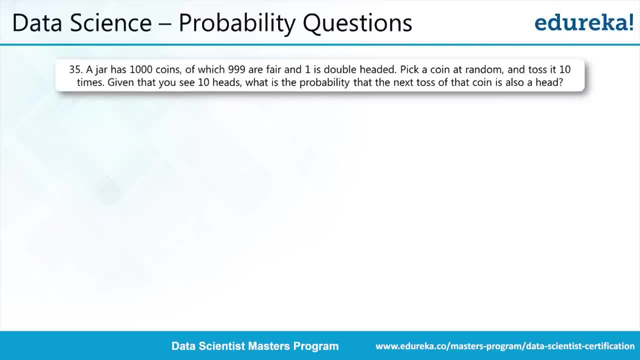 like the probability to choose. So there is only one event which favors this probability, like saying 2 girls out of the 3 that we have, so 1 by 3. so let's take up this question here which says the jar has 1000 coins, of which there are like 999 coins which are fair right, which means the head. 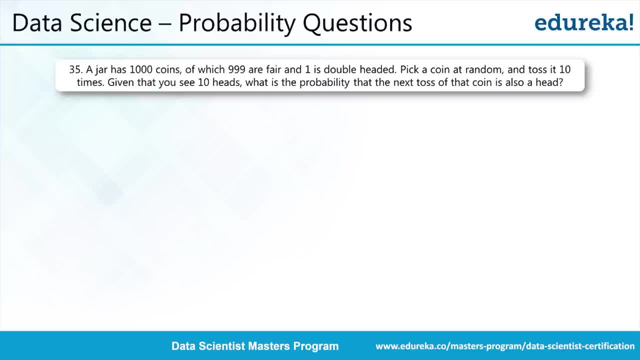 and there is one head and one tail and there is one coin which is like tampered with, and both the sides of that coin is head. We need to now pick a A coin at random from this jar and toss it 10 times right? so, given that we have seen, 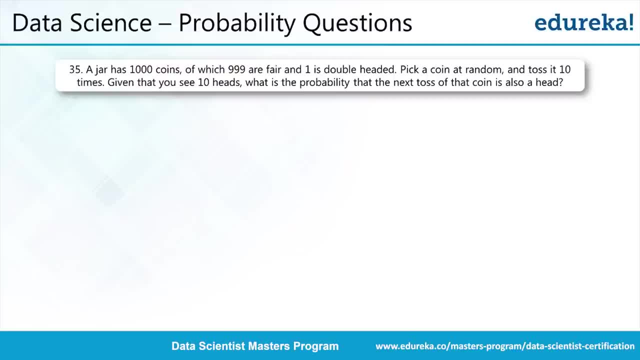 then 10 heads already of in that 10 times of tossing the coin. what is the probability that the next toss of the coin is also going to be head, and we are given a statement here that 10 heads are already seen. what is the probability that the 11th toss would be a head? 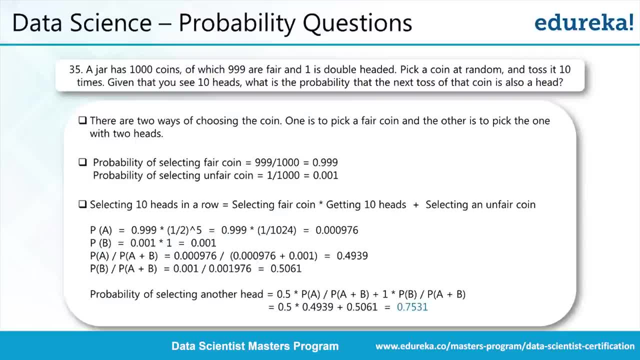 ok, so let's see how we approach this. so let's first put these 2 possibilities in place. there is this 999.. One fair coin and one doubly headed coin- right, double headed coin. so we need to see the probability of how many times we can get that double headed coin. so if I look at from the jars perspective, 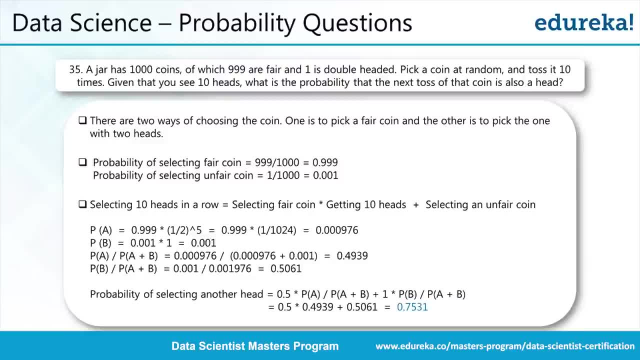 choosing a fair coin from this jar is 999 times out of all the 1000 possible coins, so which comes to be 0.9, so high probability. but for the unfair one, there, though, there is a small probability, but it might also appear some point right. so the probability of selecting 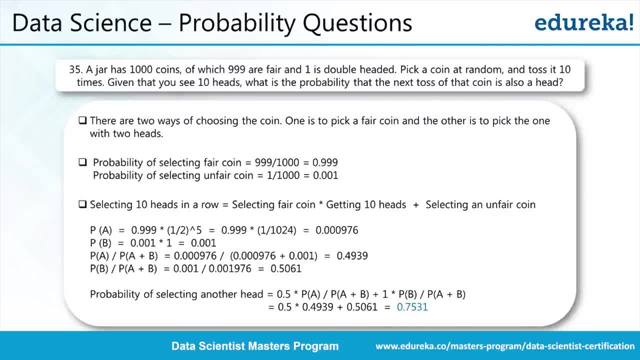 10 heads in a row Would then be: either you would get a fair coin and toss 10 head continuously. so this is one possibility. the second possibility is to select an unfair coin where the possibility of head is like 100%, because there are both the sides of the coin is head, so the probability 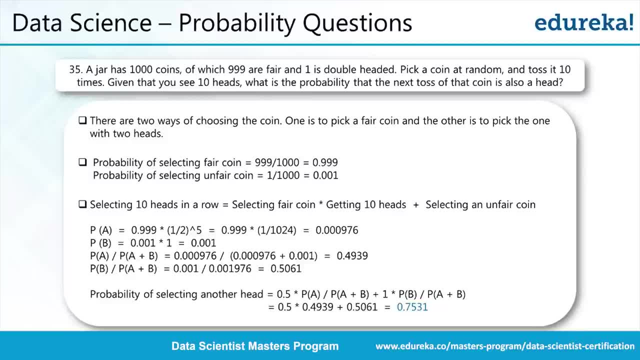 of selecting 10 heads in a row would be the selecting fair coin multiplied by probability of selecting 10 heads, which is nothing. but each coin which you are picking up is independent of each other. getting a head there is also independent there, So 0.5. that's why we are able to multiply it, so you have here the probability of picking a fair coin. 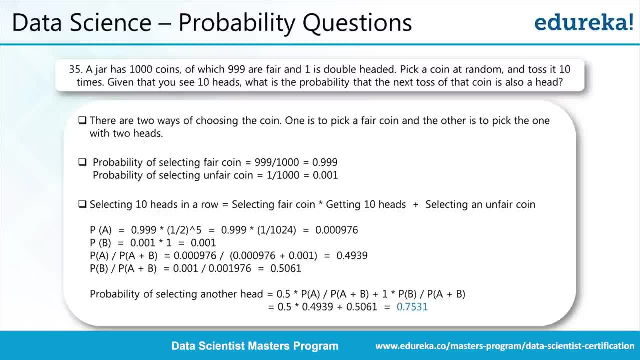 to be 0.9 and multiply that with 0.5 10 times and that's your like probability which you get after that. so this probability of a is selecting a fair coin and getting 10 heads, and the probability of b is selecting an unfair coin, and we know whenever we select that, the surety is we always get a head. 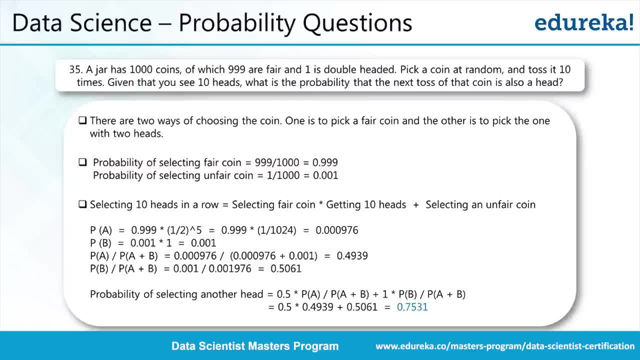 so then that probability of b becomes 0.001. so now what we need to find out is this probability where we can sort of say, given we have these two cases, what is the probability that we are able to come out with the 11th head right? so how we going to do that is by selecting this kind of combining. 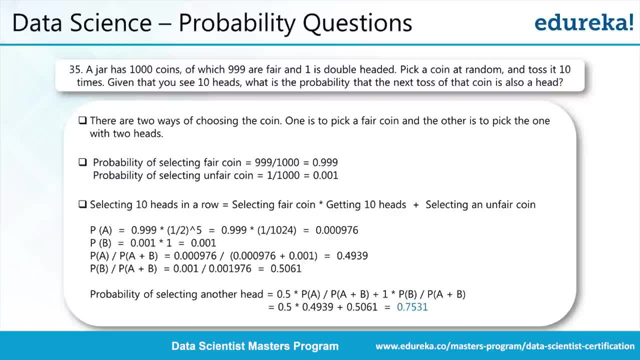 this probabilities into a sort of form like this where we are calculating, given these two possible cases, what is the sort of likelihood of with a fair coin getting 10 heads and with an unfair coin getting that one head right. so those two are the probabilities written here: 0.49 and 0.50. 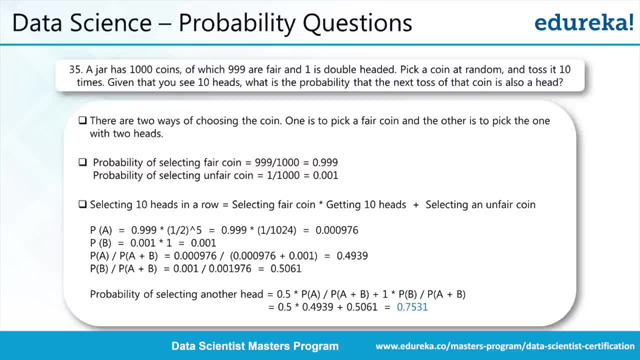 so, finally, with these two probabilities known to us, the probability of selecting one more head would mean that in the fair coin, the probability is 0.5, right so, which you already know, and in the unfair coin, the probability is always going to be one because we have both the sides, as 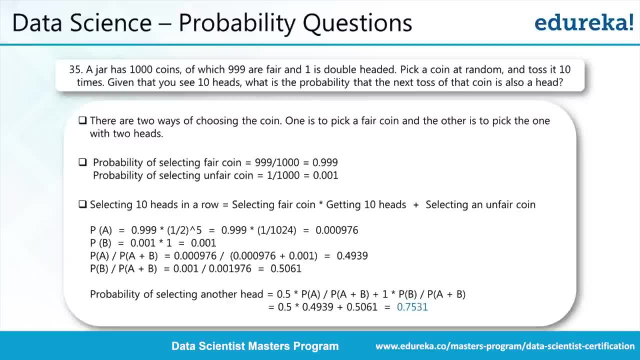 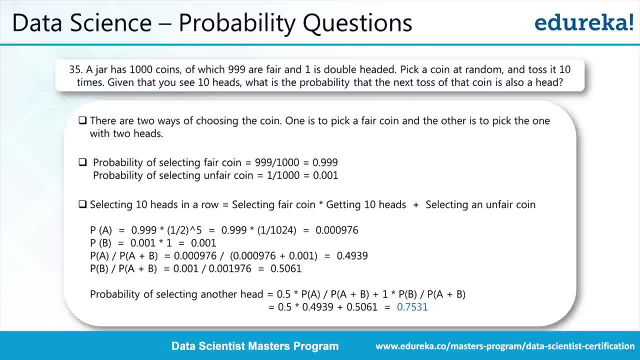 front of it. so if you put this into one formulation, you will finally get. the probability of selecting another head is 0.75, so which is like slightly more if you didn't had this sort of one double headed coin. if that coin would not have been present, the probability would be a bit more. 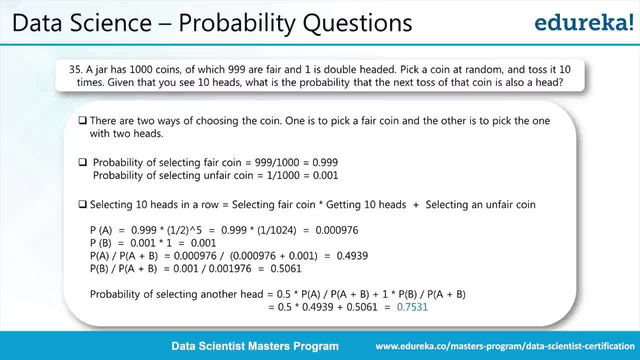 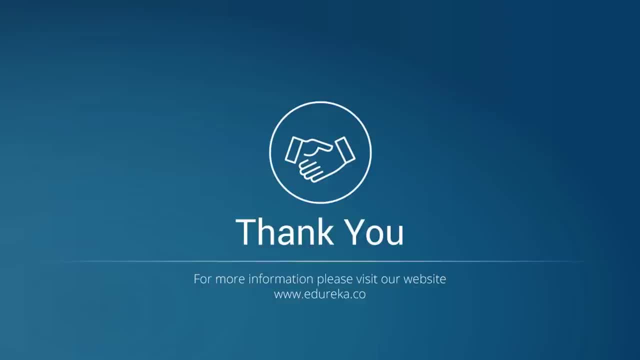 less here, because all the coins are then fair, okay. so thanks a lot for listening to this session. hope this helps for you to prepare for your interviews. so, reiterating the fact, give a very good emphasis on basic ideas from stats and probability. also spend some amount of time understanding machine.